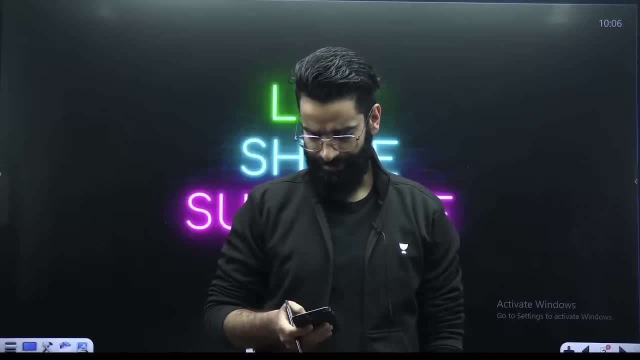 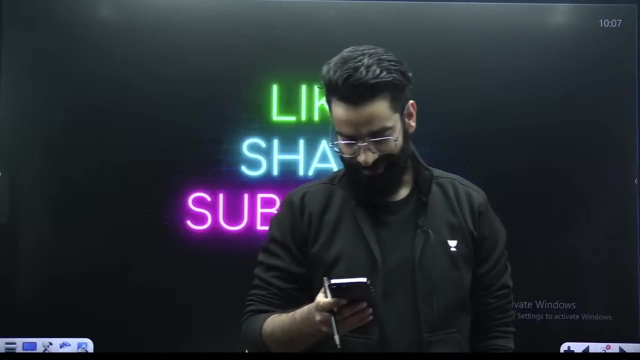 perfectly audible, visible to every one of you. Let me know in the chats quickly with some fire emojis. Good morning people, good morning, good morning and welcome back. So quickly, give me some fire emojis in the chats so that I'll get to know I'm perfectly. 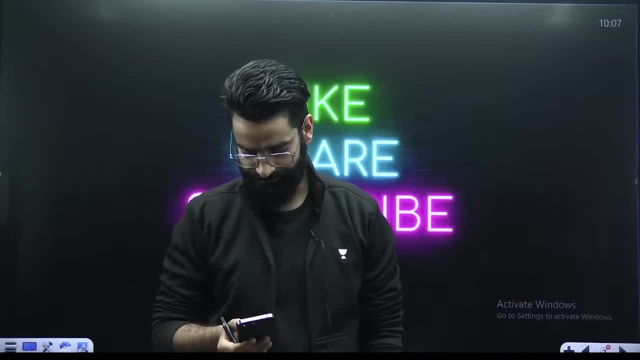 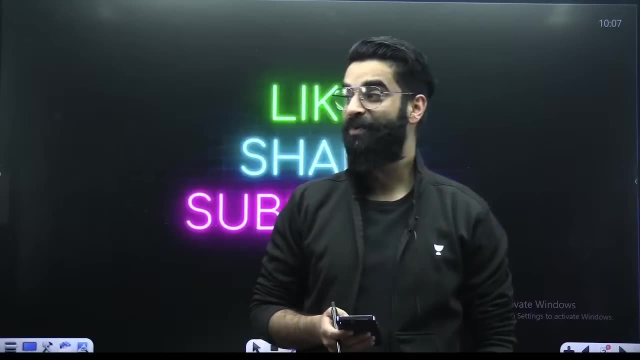 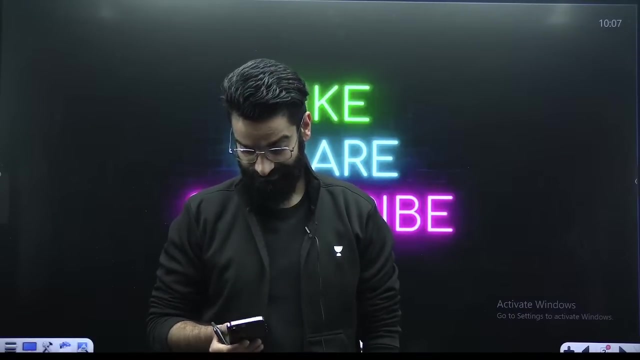 audible. I believe that I'm perfectly audible and visible to every one of you. Quickly people: Yes, I'm not well, I have got cold cough fever etc, etc. Yeah, But still it's okay Perfect. 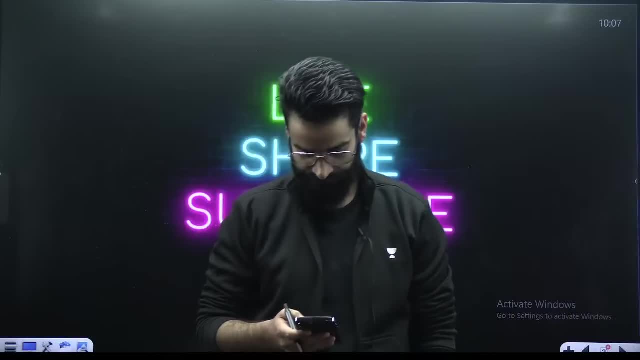 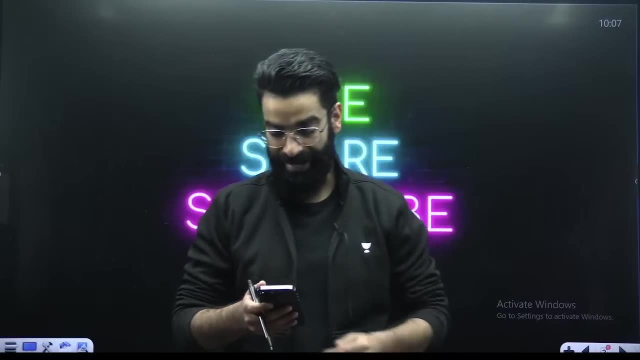 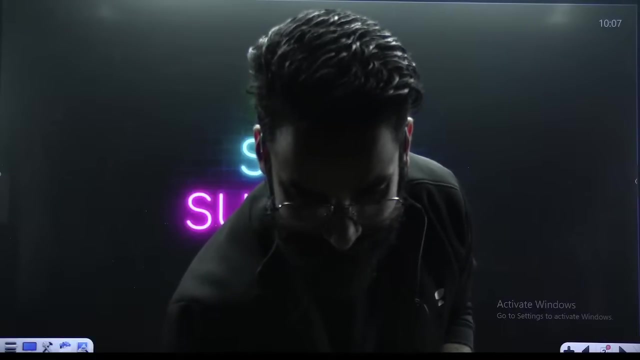 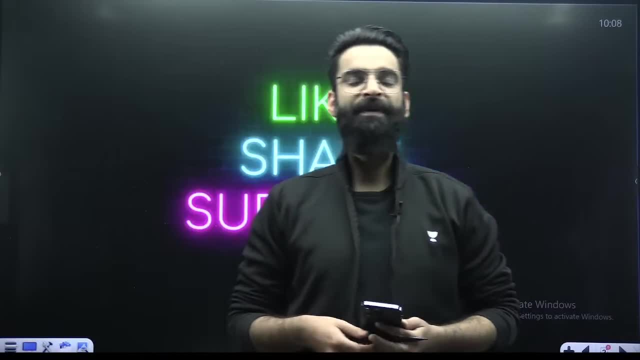 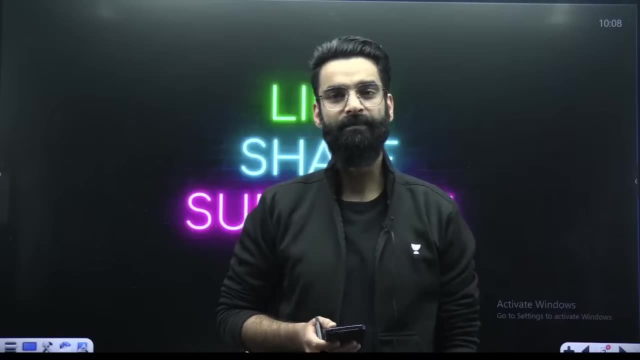 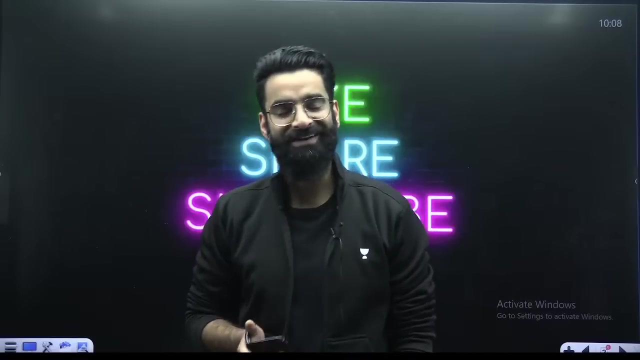 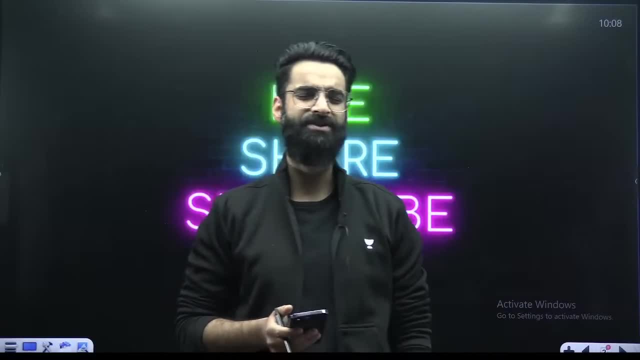 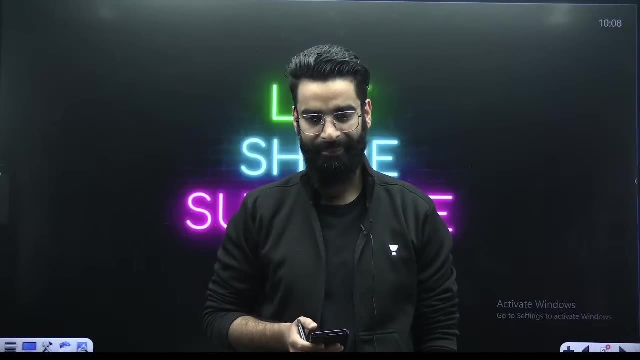 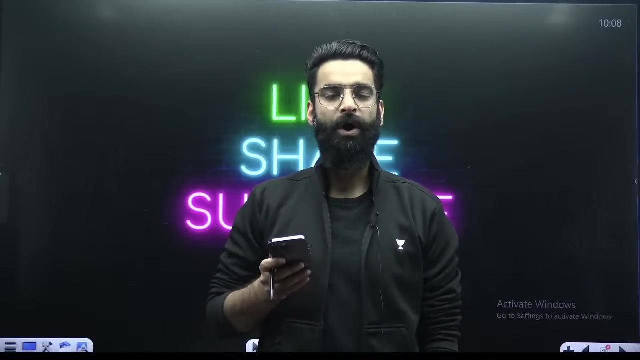 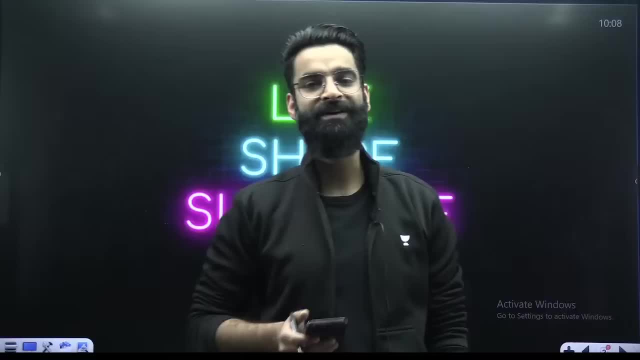 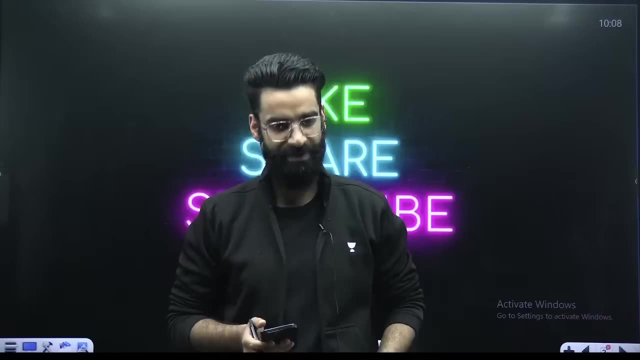 guys to be with me till the end? so first of all, let me know in the chats: are you guys ready to be with me till the end? because whatever I'll be teaching you, you know I'll be starting everything from the basics itself, from the scratch itself. so no worries if you have not studied these chapters before you need. 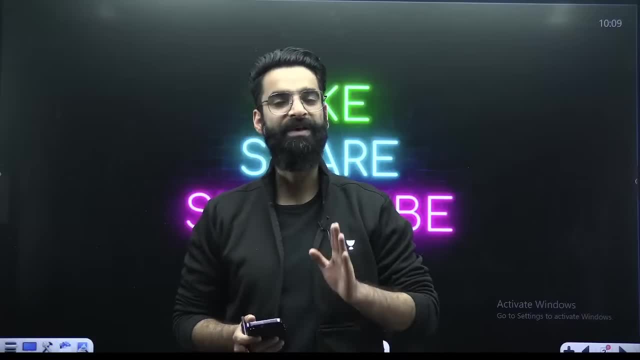 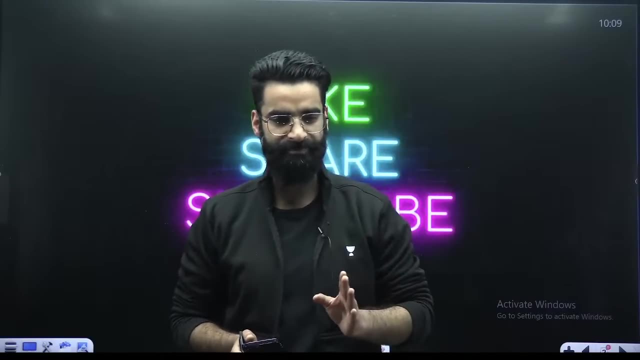 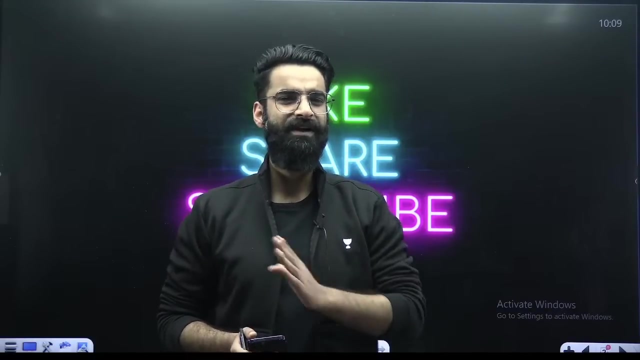 not to worry about them at all. right, everything will be discussed in detail. I'll be touching every single concept which will be asked in your NEET examination. okay, and people at the same time. whatever I'm going to teach you today, that's going to be complete relevant stuff. no irrelevant stuff. I'll 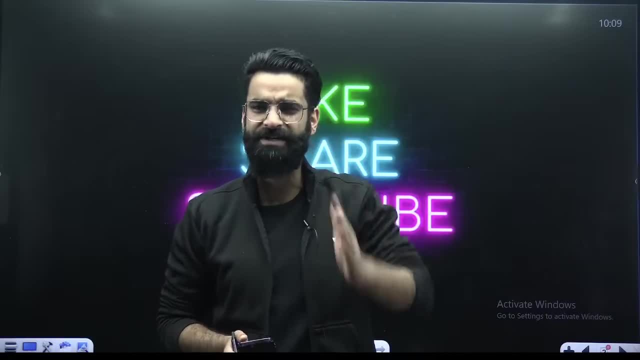 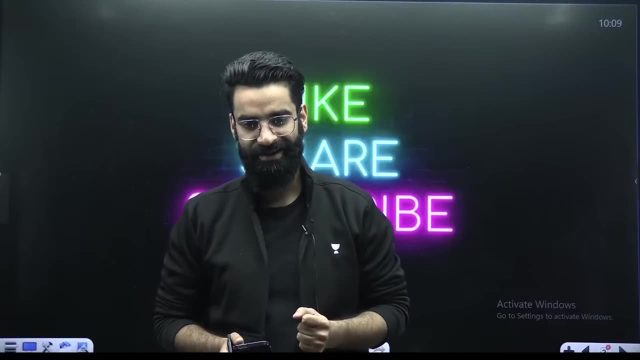 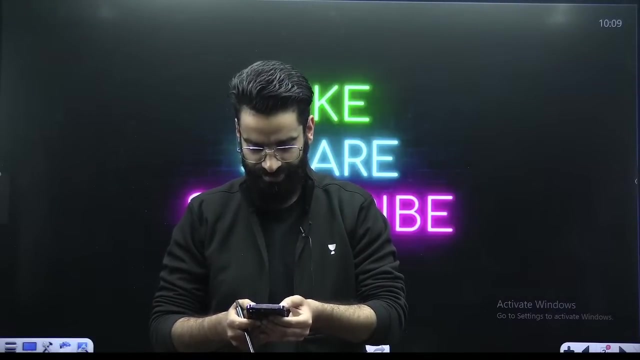 be teaching you. I'll be teaching you straight away those concepts. I'll be teaching you straight away those questions which will be asked in your NEET examination. okay, perfect, so should we start then? should we start, sir? where are you from? I'm from Srinagar, J&K. 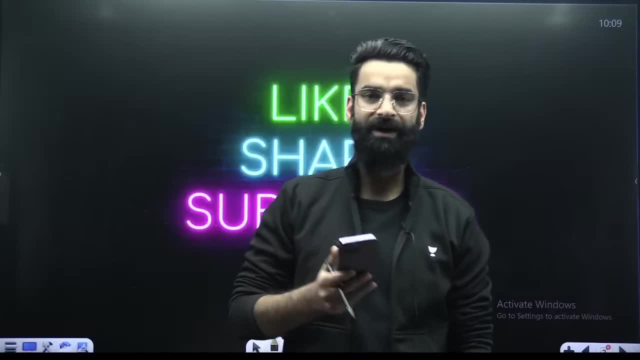 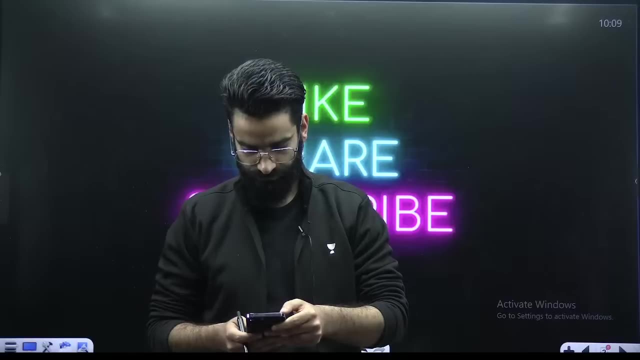 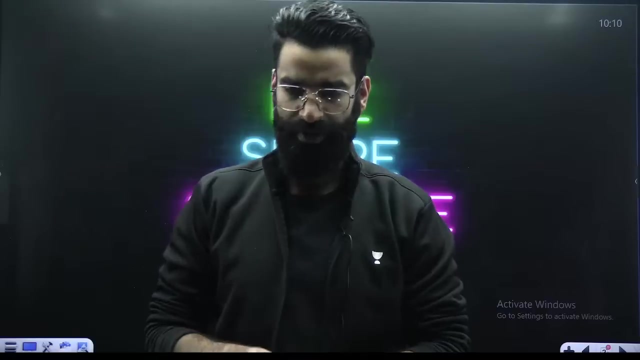 and the session PDF. you know I'll be sharing it with you on the telegram group. I hope you are already enrolled. you're already there in the telegram. perfect guys, perfect. so without wasting a lot of a time, let's get going. then let's get started with the first chapter. 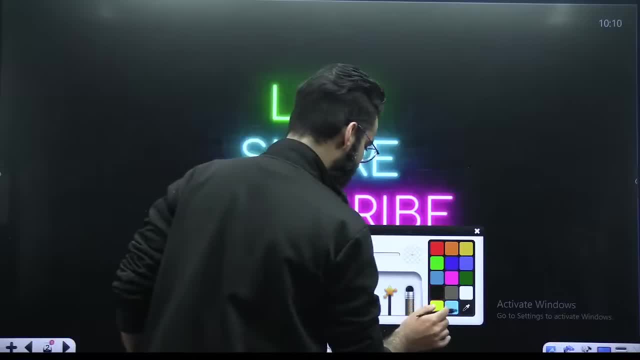 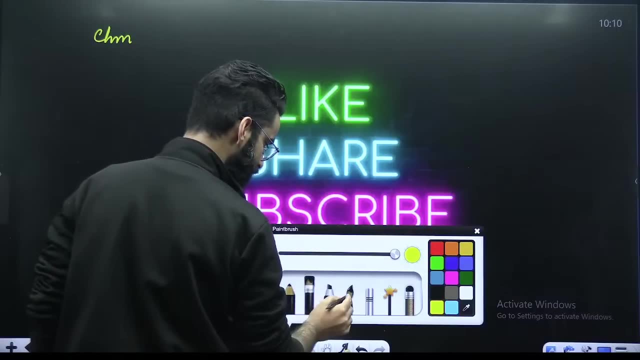 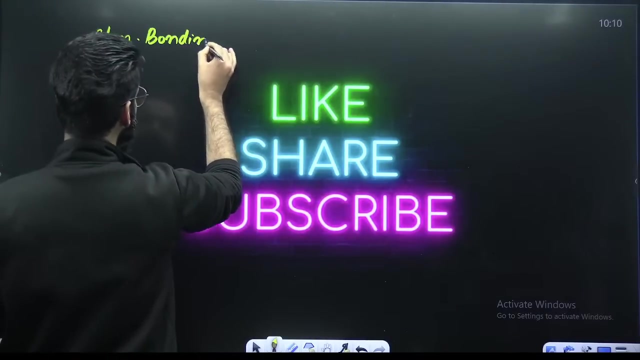 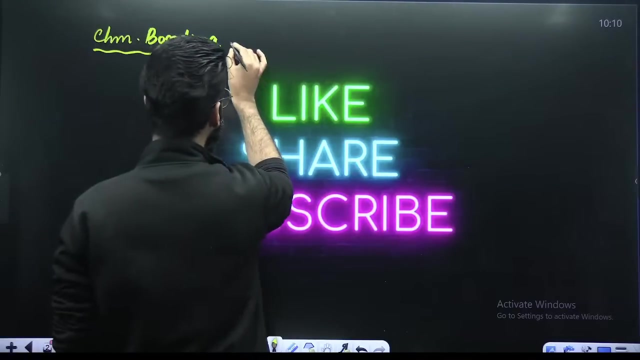 of your class 11th in organic chemistry and that first chapter is your. that first chapter is your chemical bonding. that first chapter is your chemical bonding. why do is students? first of all? first of all, from this particular chapter alone, from chemical bonding chapter alone, let me tell you you are going to get four to 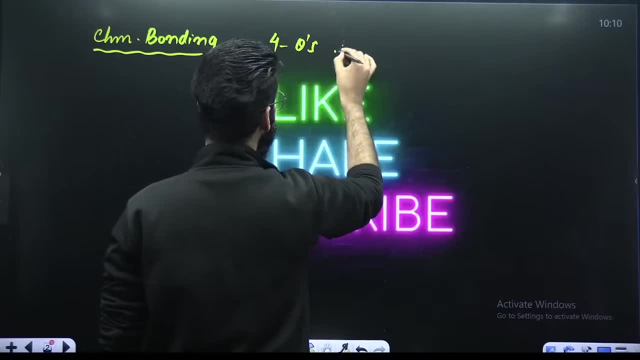 five questions. you are going to get four to five questions in your Culinary Reersonic Chemistryести. ребята from parle hoy policy: first ate paul from this particular chapter alone, from the chemical bonding chapter alone. let me tell yu: yeah, in here we are going do mission there. Random Collective. Thank you for an opening here, everybody. 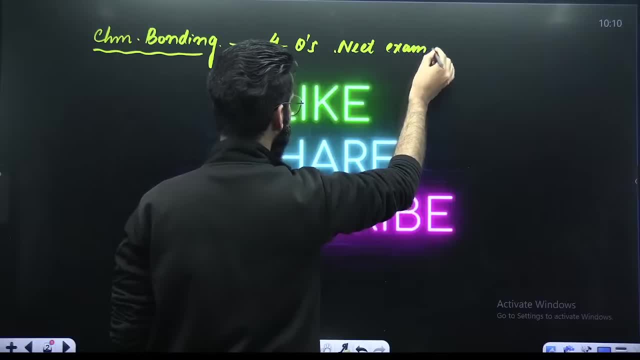 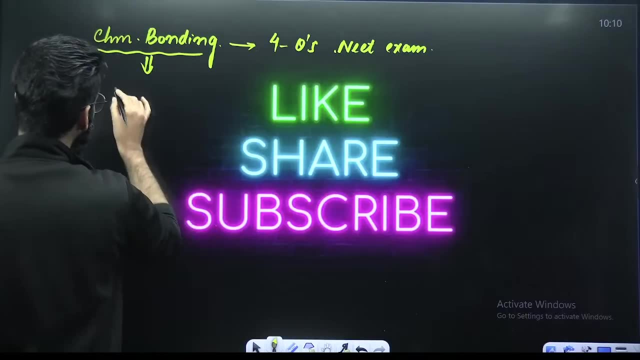 your upcoming NEET examination. number one, number one, number two: if your chemical bonding chapter is strong, then only your organic chemistry can become strong. so basically, in the organic chemistry you need some fundamentals of chemical bonding. so let's make sure those fundamentals of chemical bonding get stronger in this particular session so that your organic chemistry will get automatically. 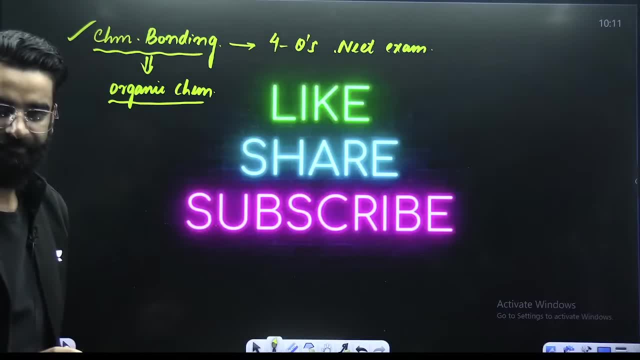 stronger, right, right, people? and after chemical bonding, once we are done with chemical bonding, then there is going to be periodic classification of elements as well. right, which is one very small chapter. perfect from this particular chapter itself. also, you'll get some two questions in your upcoming NEET examination. okay, 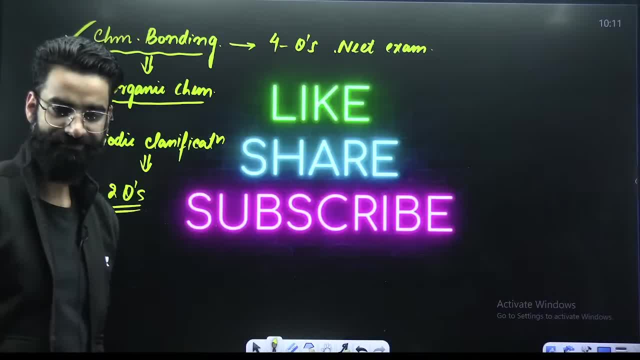 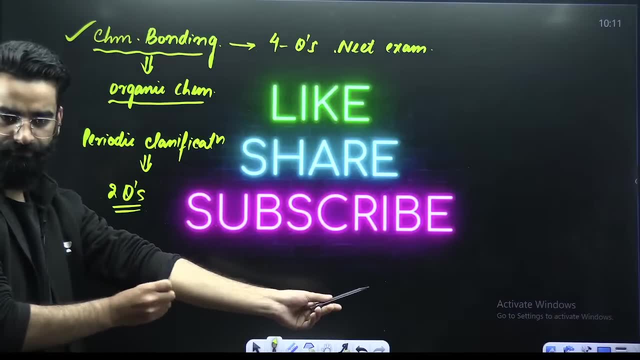 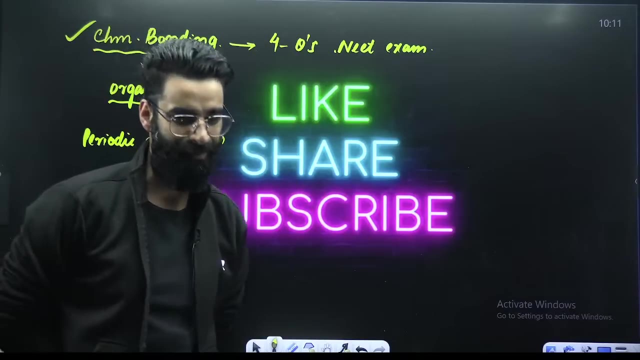 perfect. so are you all ready? should we start? should we start people? should we start? are you all ready? yeah, exactly, this particular bounce back series will be getting over by 20th of April. right, we'll make sure it gets over by 20th of April. so let me know in the chats quickly. 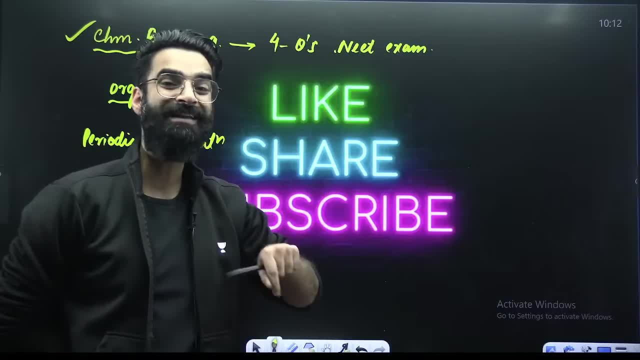 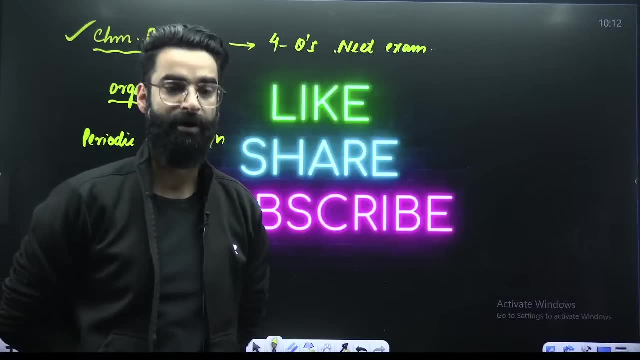 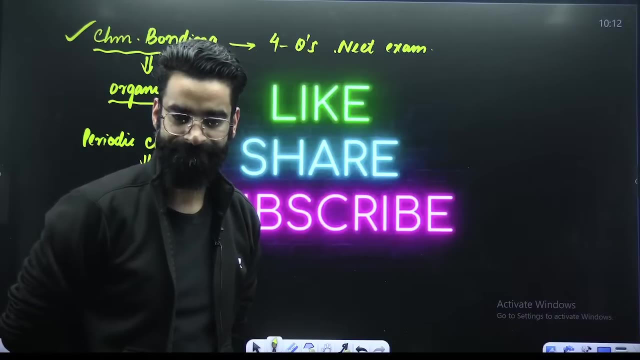 okay, a lot of people are asking about p-block. p-block won't be done in this session. this session includes class 11th inorganic and your p-block will be done in your class 12th inorganic marathon. okay, perfect, p-block will be done in class 12th inorganic chemistry marathon. 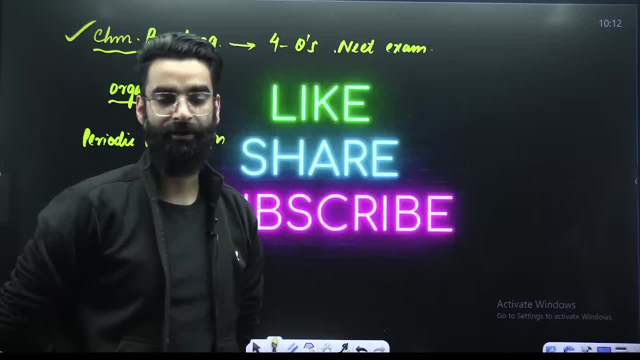 today it's going to be class 11th, inorganic. so quickly, people, are you all ready? i want to start this session, so i'm going to start. i want you guys to let me know in the chat. so are you all super excited about the session? are you all ready? 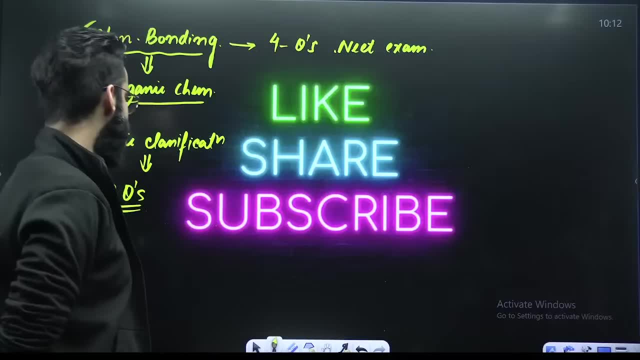 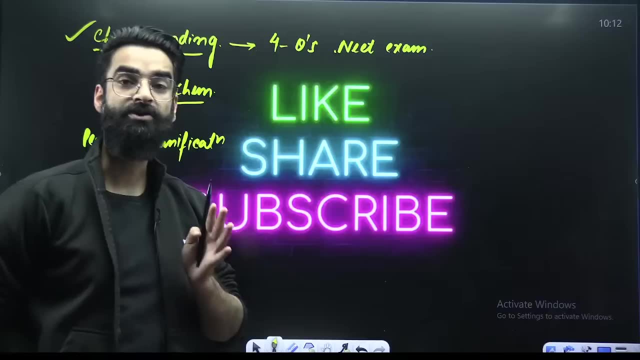 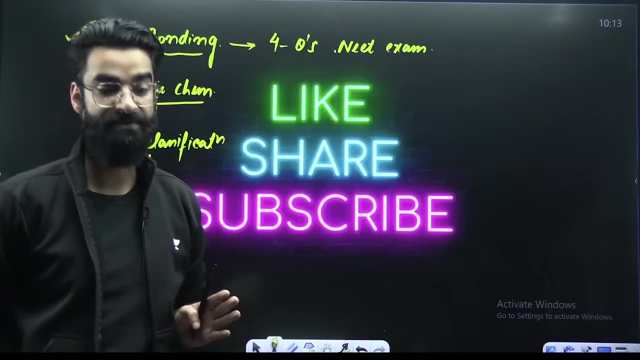 okay. so let's get going. then let's get started. so, my dear students, again i'm repeating in the today's session, almost eight questions you'll get from the today's session: number one, number two: if this session gets clear, then only you're chemistry can become stronger. otherwise, not, otherwise, not okay. and tomorrow, tomorrow i'll. 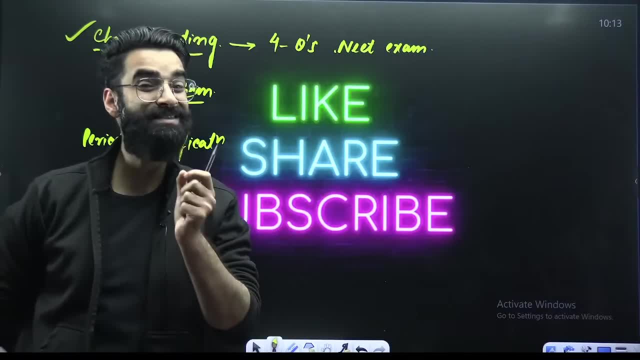 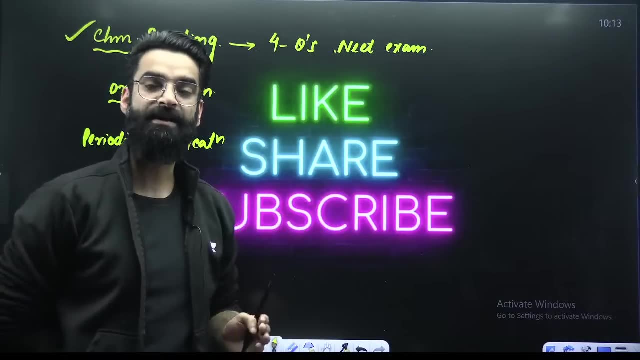 be doing some 500 questions of your class 11th in organic chemistry, which will be extra 500 questions. you know that right after every marathon on the next day we take extra question practice session right in which we solve a lot of questions which can be asked from the marathon which can be asked. 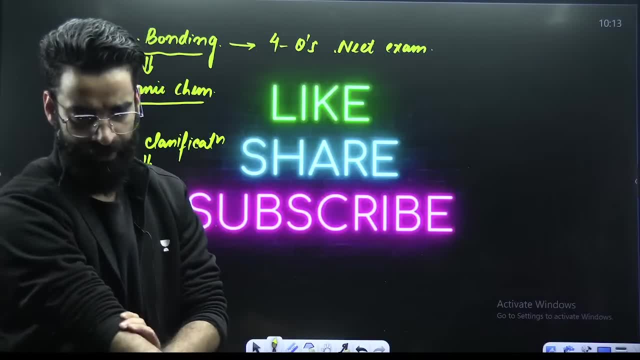 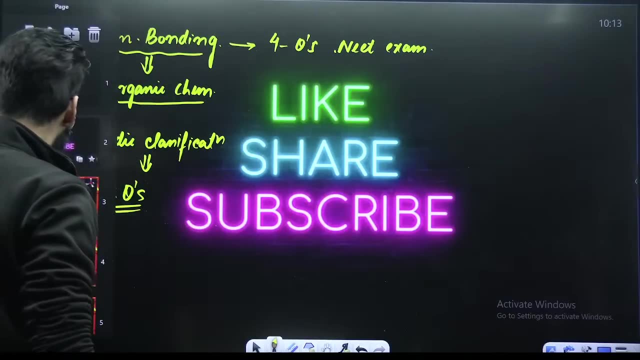 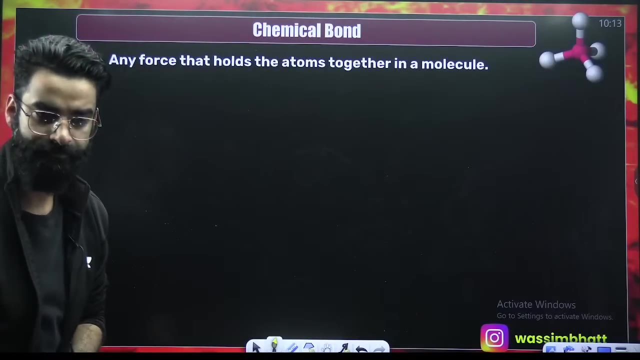 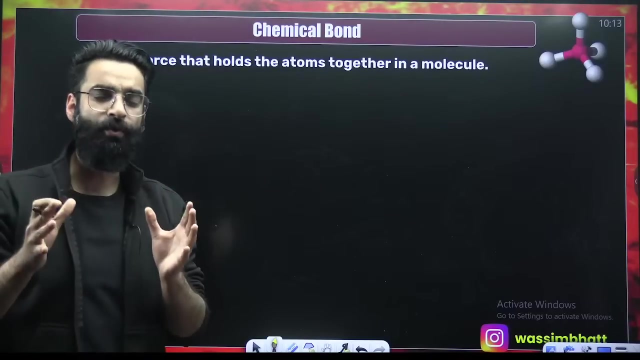 from the chapters which we do in the marathon, exactly okay, so let's get going. then let's get going. no spamming, nothing, let's have a look. my dear students, if i ask you, how do you define the term chemical bond? what is a chemical bond? basically, all of you must be knowing any force. 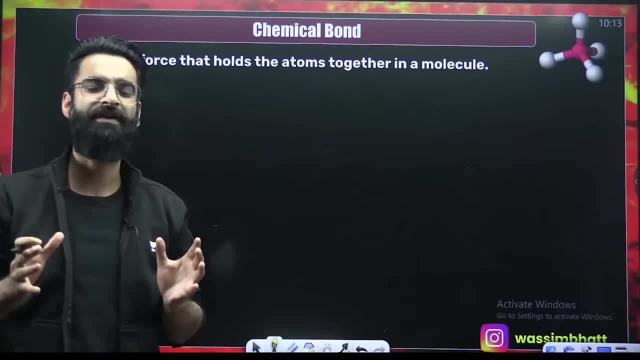 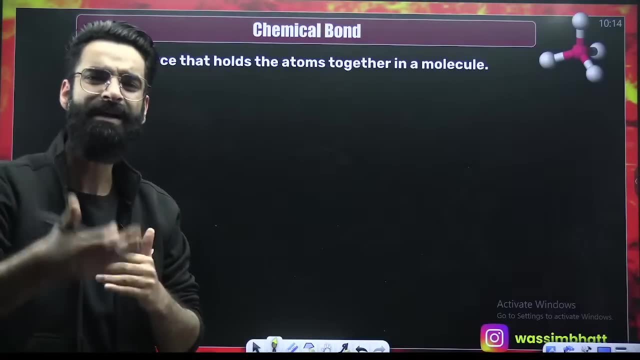 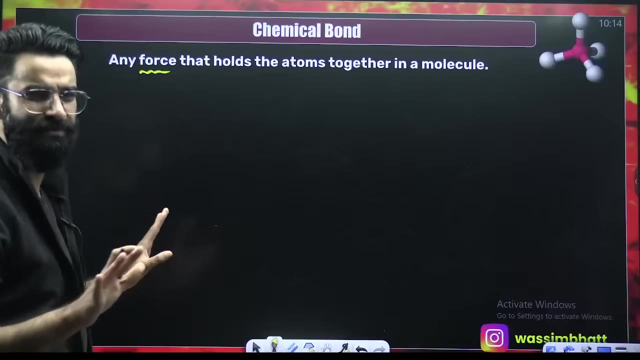 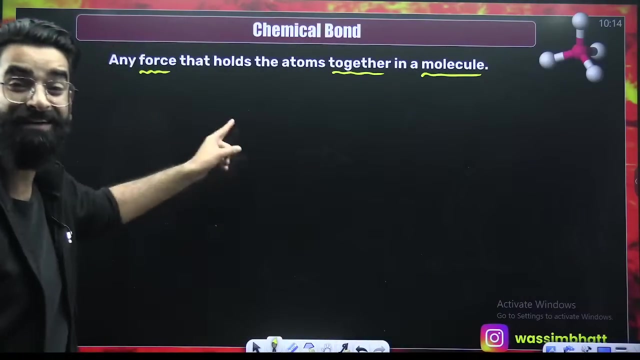 any force of attraction, any force of attraction which holds the atoms or ions together. that is something which you'll be calling as the chemical bond. in short, any force, any force, whatever is the nature of the force, any force which holds the atoms together in a molecule, any force that holds the atoms together in a molecule, that force of. 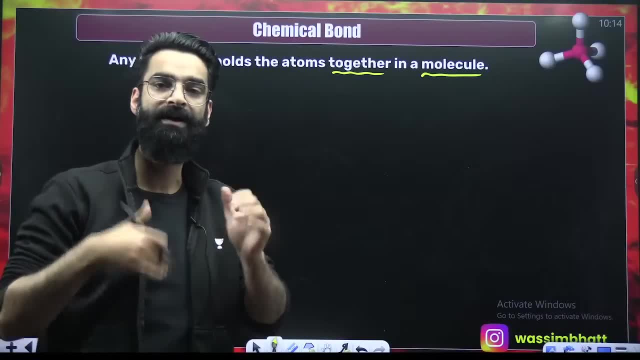 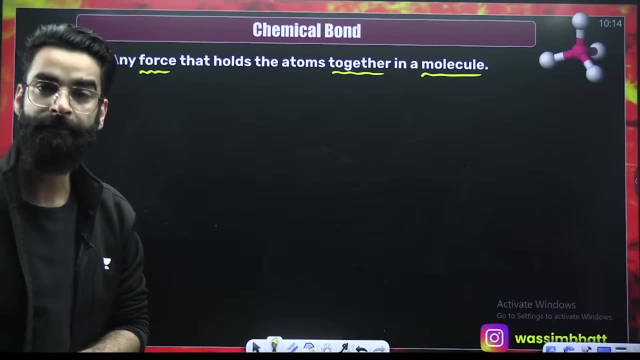 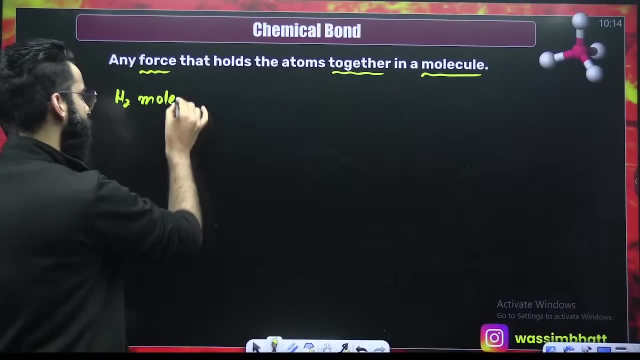 attraction, which holds the atoms together in a molecule. that force of attraction is something which you call as chemical bond, which you call as chemical bond right. for example, you have got h2 molecule right, one simple molecule, h2 molecule. in your h2 molecule there are two hydrogen atoms. you know it right, there are two hydrogen atoms. 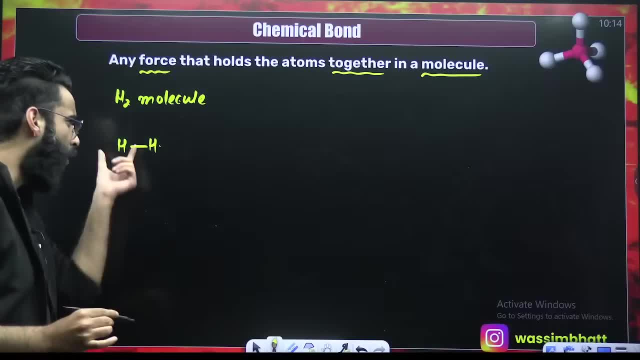 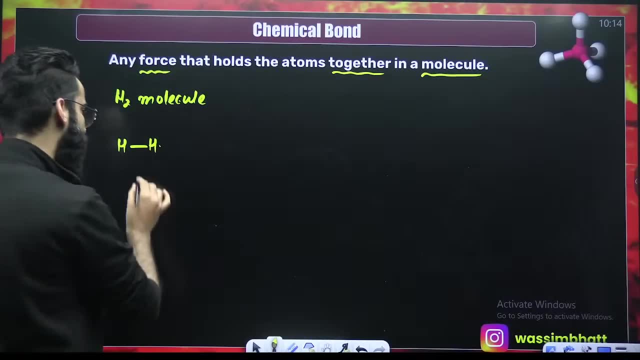 so there is some force of attraction which is holding these hydrogen atoms together and any force of attraction which holds the atoms together in a molecule. that force of attraction is something that you'll be telling this session, something which you call as chemical bond. which you call as chemical bond right, for example, if 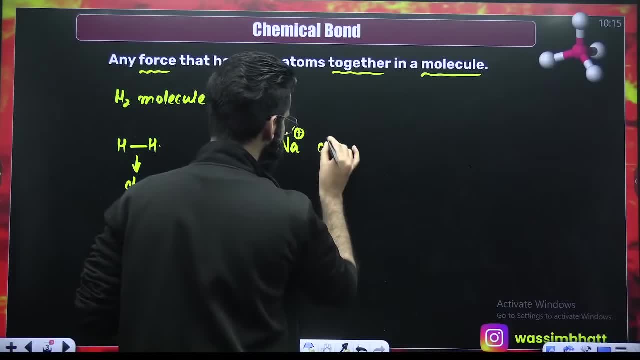 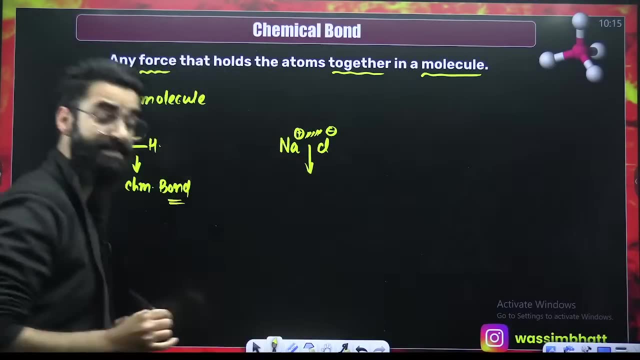 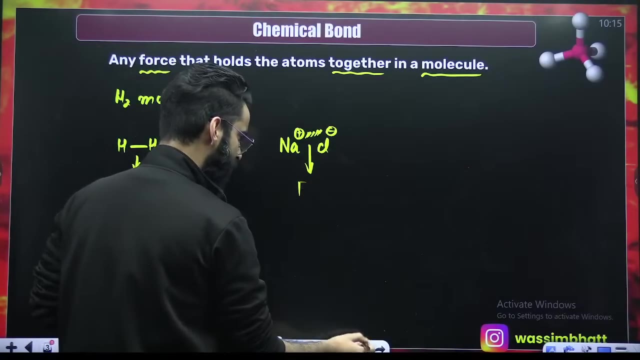 you talk about any seal. this is any positive. this is CL, negative, any positive, CL negative. there is some force of attraction which is holding these ions together. there is some force of attraction which is holding these ions together and any force of attraction. right, that is something which you'll. 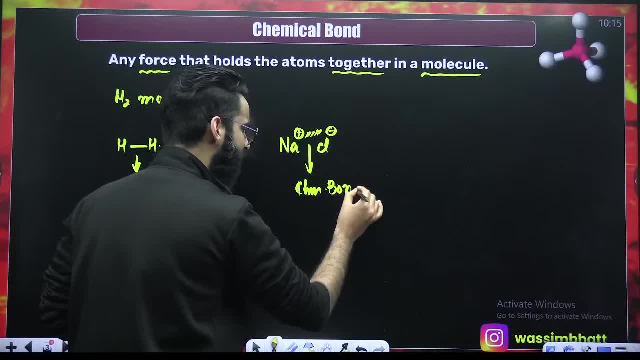 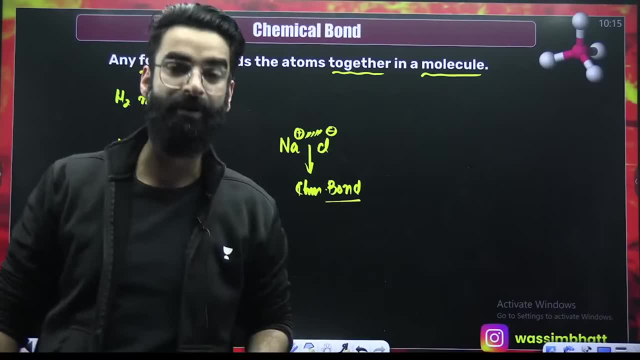 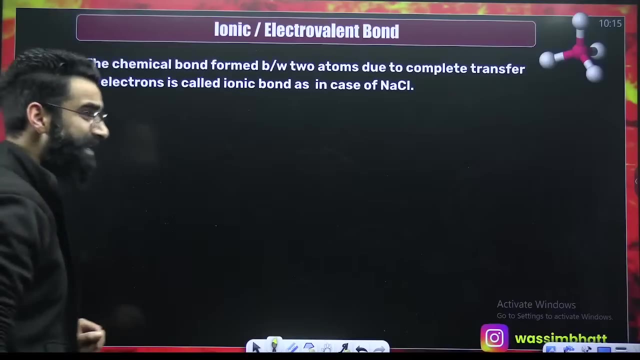 be calling us your chemical bond. so, in short, what a chemical bond is all about? chemical bond is nothing. it is just the force of attraction which holds the atoms together in a molecule, right in short, my dear students, the first type of the chemical bond, the first type of the chemical 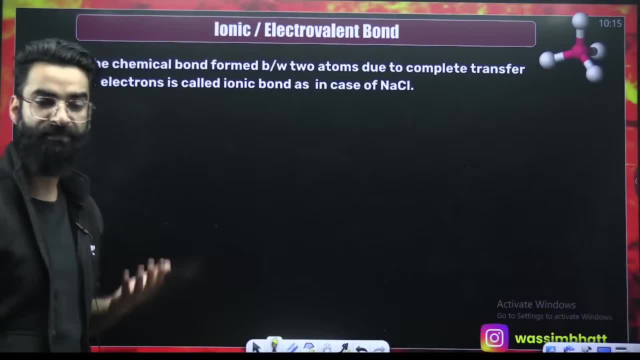 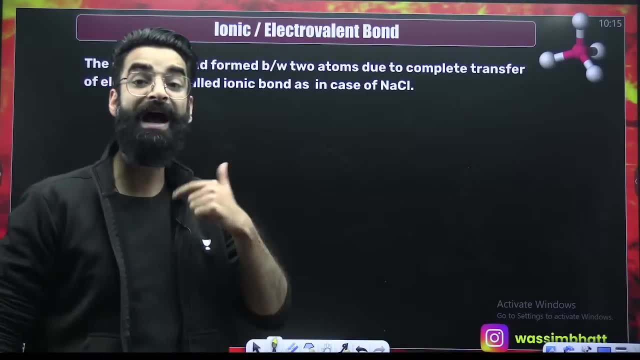 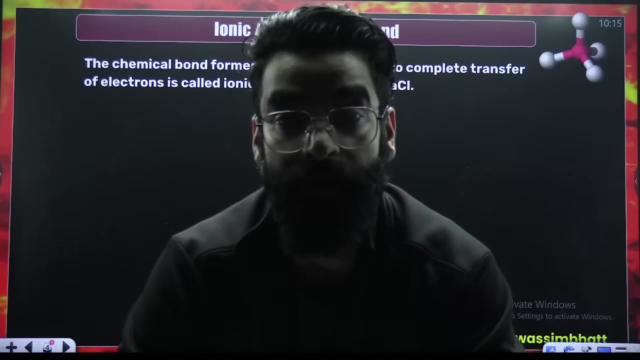 bond which you need to know which one? is that the first type of the chemical bond which we are going to do, right, which we are going to talk about? what is that way to be? that is going to be ionic bond. someone is spamming Barney. let me tell you this is class 11th in organic chemistry: marathon, right. 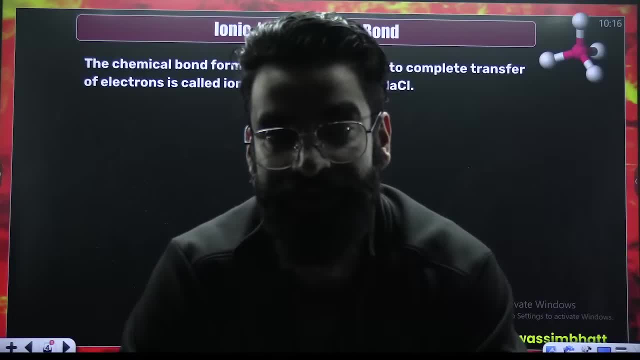 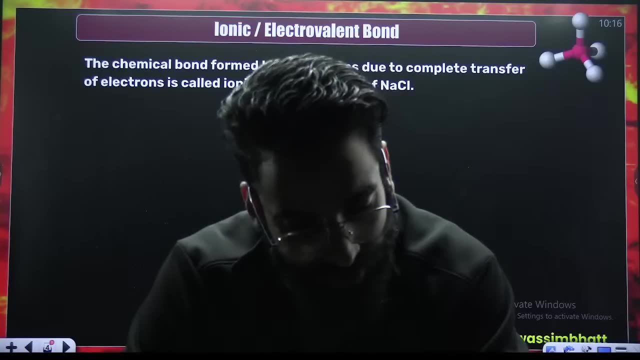 okay, so don't spam. whatever chapters are there in class 11th in organic chemistry, I'll be doing them. okay, please don't spam. okay, cool, cool. just see the title of the video. it's class complete in organic chemistry, class 11th. there is one more marathon. 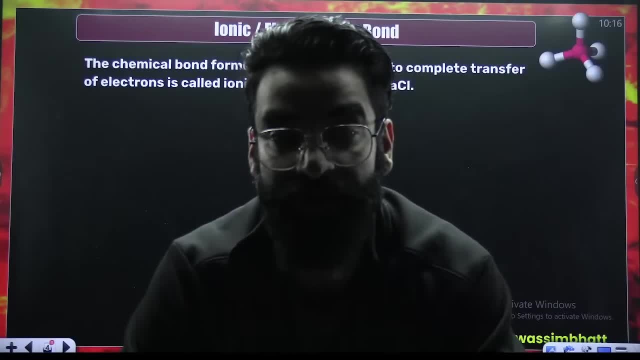 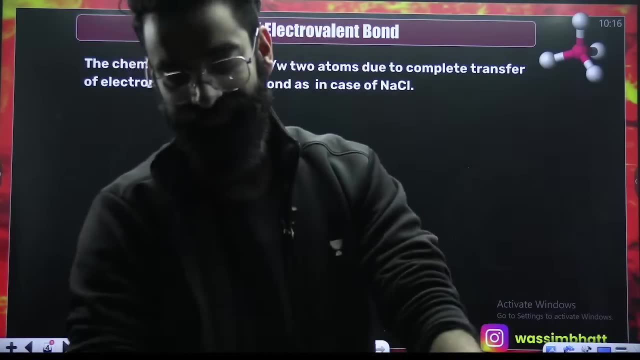 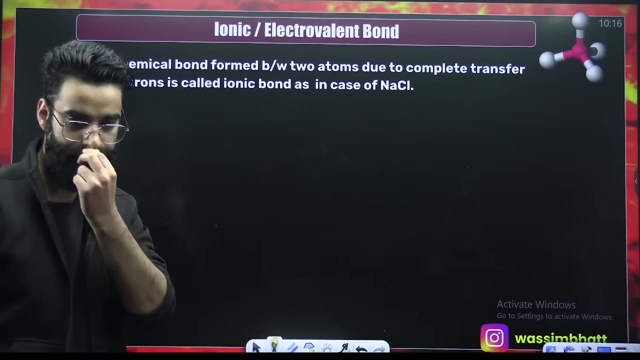 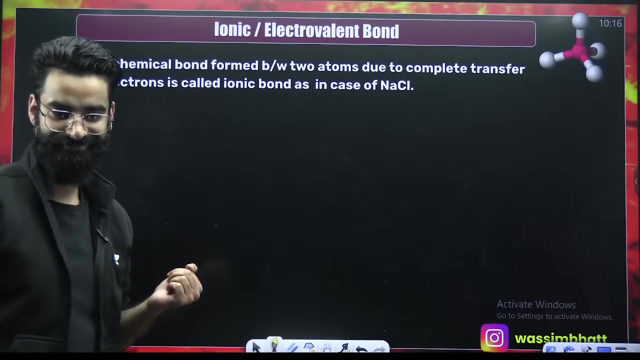 which is scheduled in this week itself. that is going to be complete in organic chemistry, class 12th. now I hope I'm clear. okay, someone is asking me why you went to unacademy. I think you are new to the channel, right? it's been more than one year I'm here, okay, so the first step of the chemical bond which we are 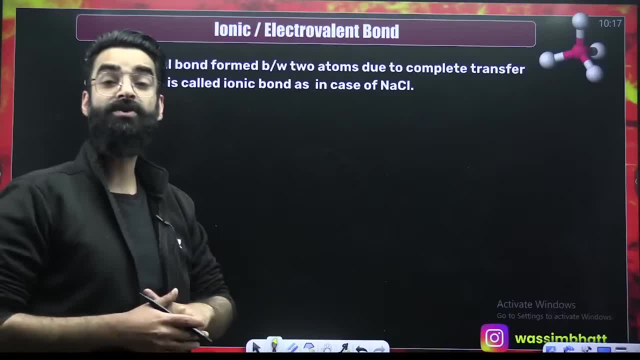 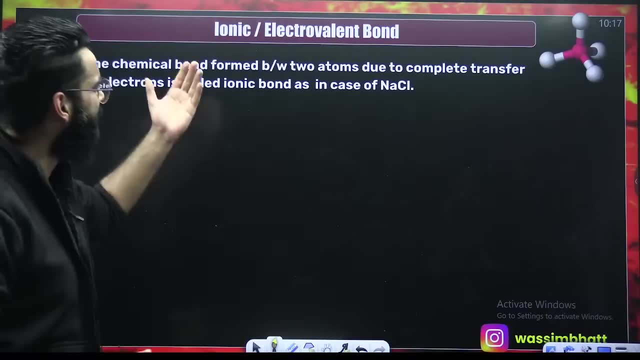 talking about right now. that is, your ionic bond, or you call it as the electrovalent bond. this is the first type of your chemical bond. now, what an ionic bond is all about? what an electrovalent bond is all about? try to understand. try to understand. 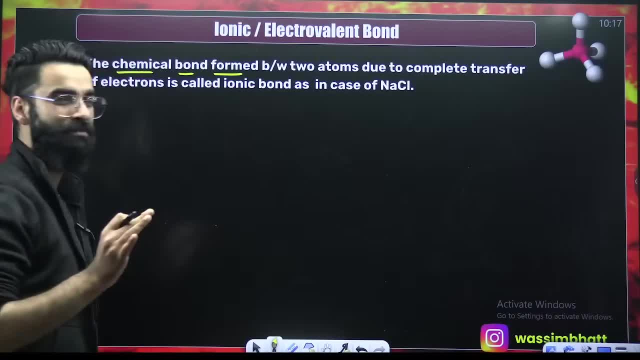 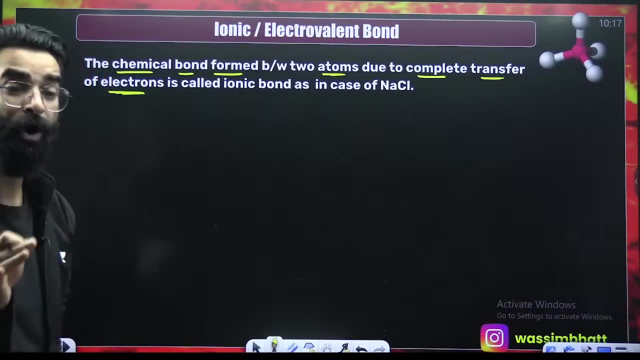 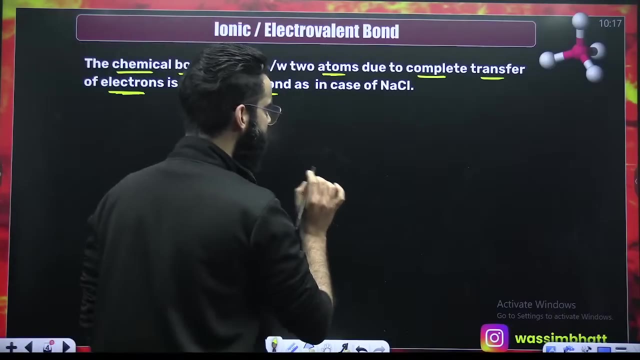 let me tell you the chemical bond. the chemical bond formed between the two atoms due to complete transfer of electrons. the chemical bond formed between the two atoms due to the complete transfer of electrons is something which you call as ionic bond. what does it mean exactly? let's try to. 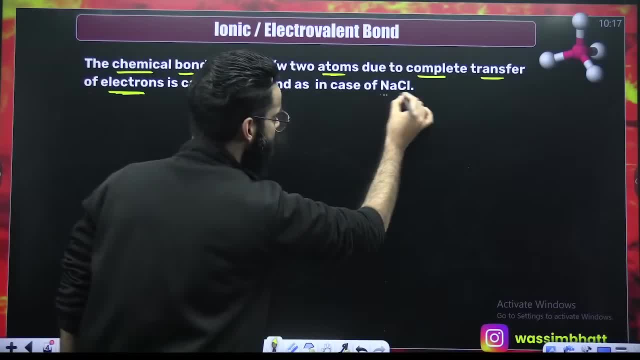 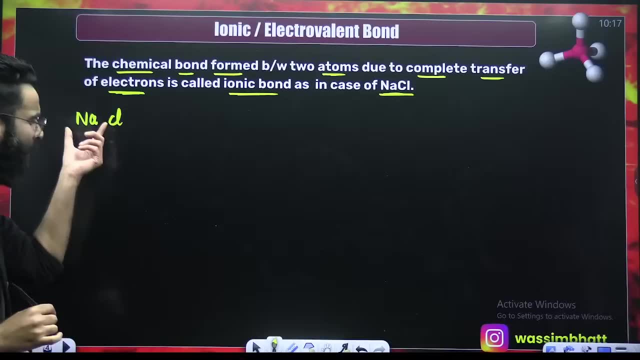 understand, but your students, for example. for example, I'm taking NaCl. for example, I'm taking NaCl right in your NaCl. as you can see, you have got two elements. one is sodium and one is chlorine. sodium, it belongs to group one, you know it, and chlorine, it belongs to what it belongs to, group 17.. 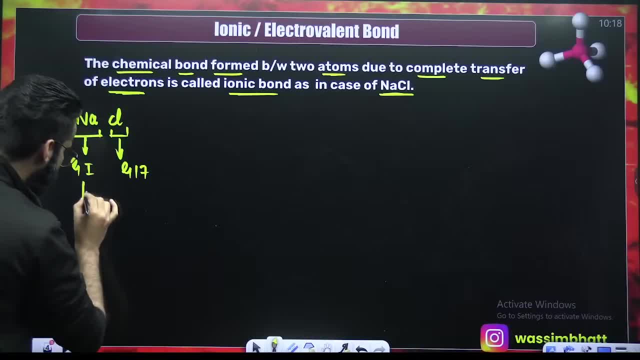 chlorine belongs to group 17.. I'll say sodium, as you all must be knowing, it is metallic in nature. it is metallic in nature and your chlorine, it is non-metallic in nature. right, if sodium is metallic in nature, it has got tendency to lose electrons. it has got tendency to. 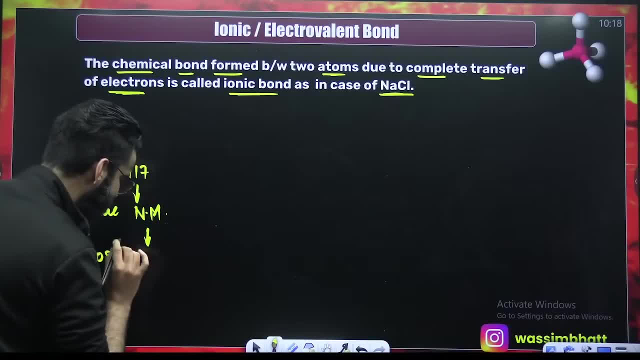 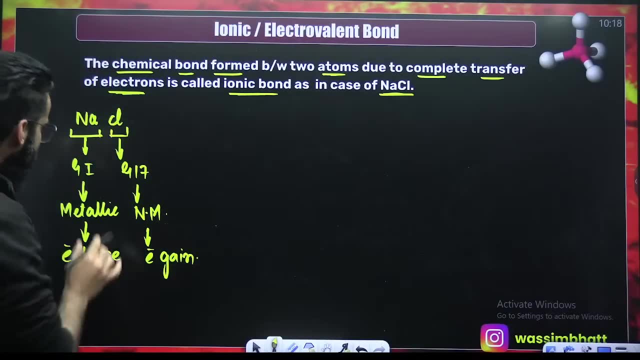 gain electrons, chlorine being your non-metal right, it has got tendency to gain electrons. it has got tendency to gain electron right now. if I talk about this particular Sodium, since sodium belongs to group first- that means it has got one electron in the outermost shell. that means it has got one electron in the outermost shell. so what this Sodium is going. 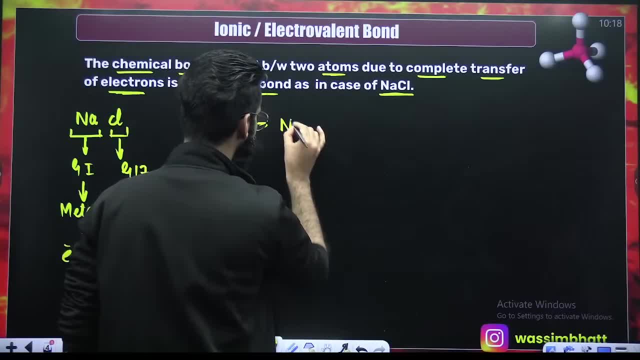 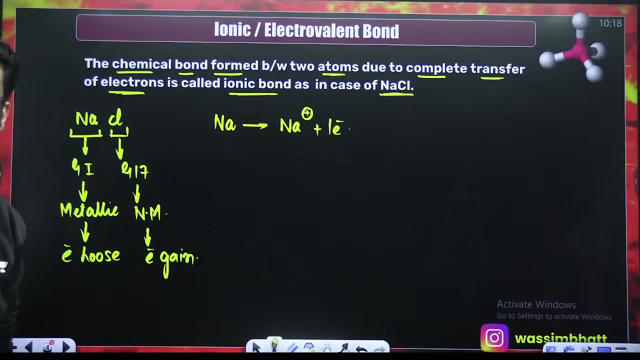 to do? Sodium is going to lose that outermost electron and when loses an electron, it gets converted into Na positive. It gets converted into Na positive, right? Similarly, this particular chlorine which I am talking about, this chlorine, it is non-metallic in nature, right, It has got high tendency to gain electrons. 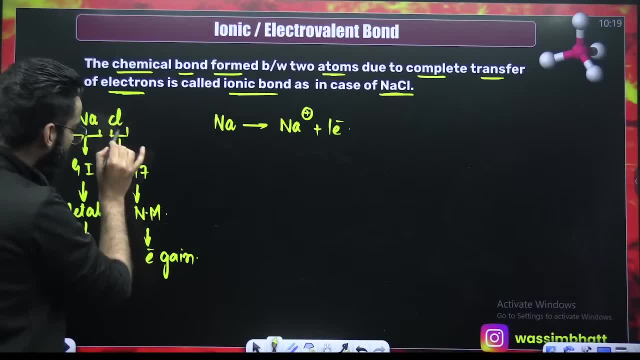 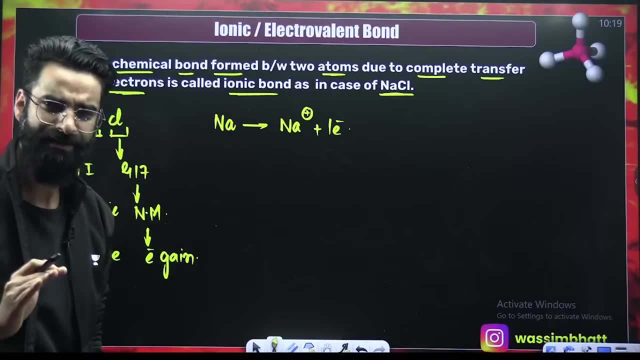 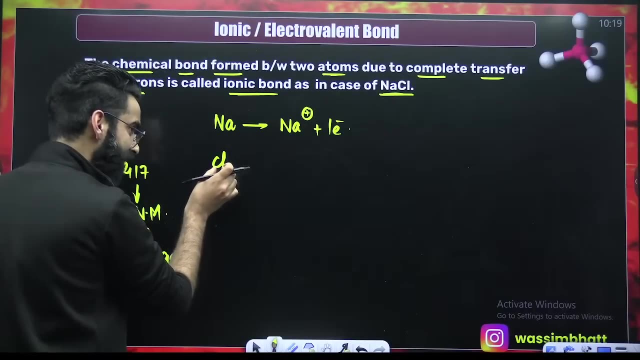 So what happens? Since sodium- sorry, since chlorine- it is a group 17 element. If it is a group 17 element, it has got 7 electrons in its outer motion, right? So what this chlorine is going to do? since this chlorine, it has got 7 electrons in its outermost shell, So it just 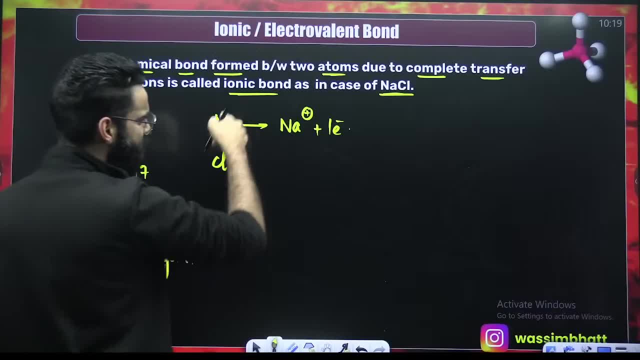 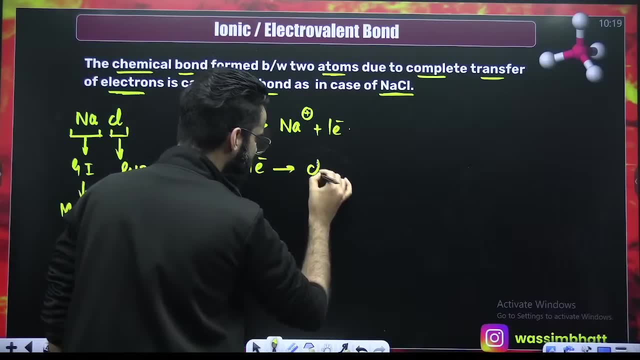 needs 1 electron to complete its octet. Now, since the sodium has lost 1 electron completely, this 1 electron will be gained by chlorine completely and will get converted into what? And it will get converted into Cl negative. So what happened? first of all, Sodium lost its 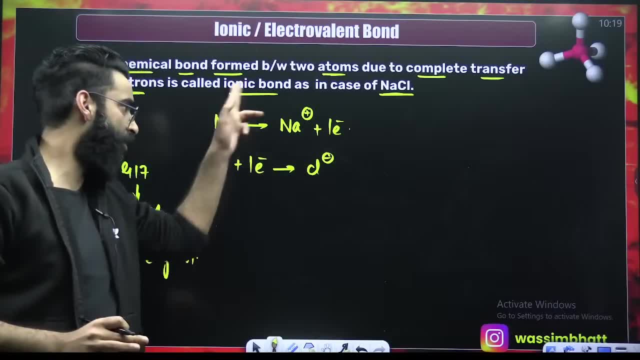 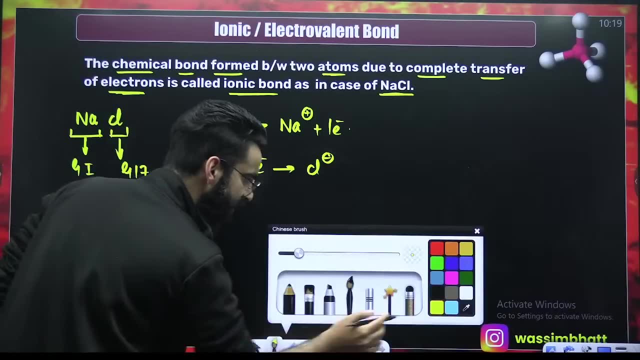 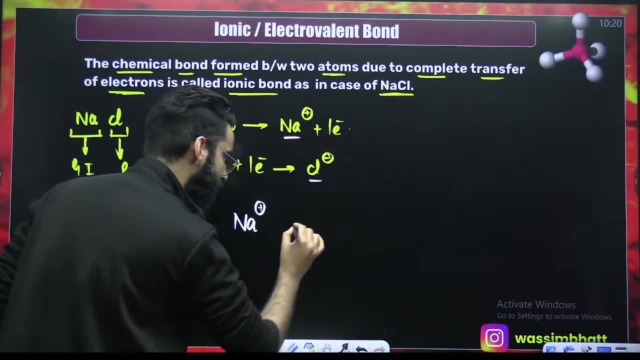 electron Chlorine gained the same electron Sodium got converted into Na positive Chlorine got converted into Cl negative. Right. So, my dear students, I got, if you look carefully, I got the cation and anion formed over here. The cation is your Na positive, The anion is your Cl negative. Since this is cation, this is. 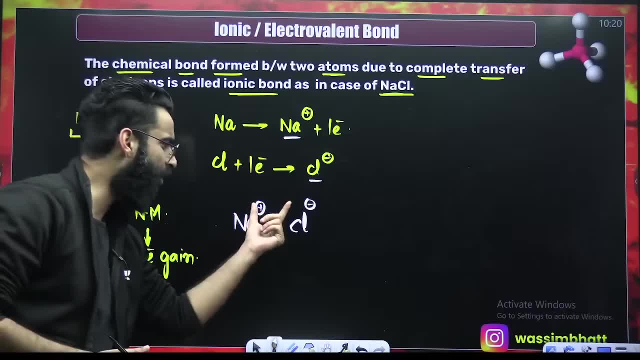 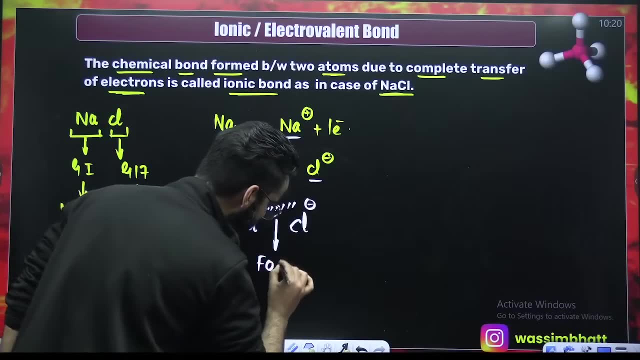 anion. They have got opposite charges. If they have got opposite charges, don't you think there will be electrostatic force of attraction between them? Absolutely, there will be electrostatic force of attraction between these oppositely charged electrons. So if you look carefully, I got the. 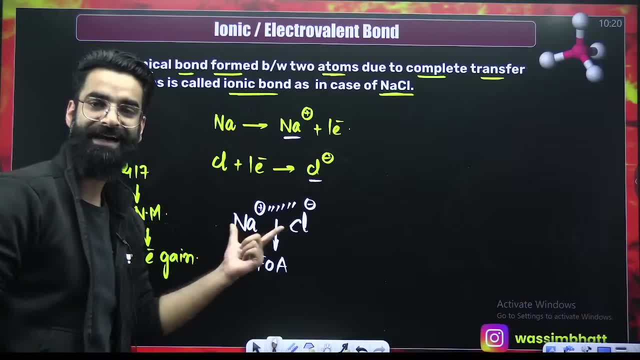 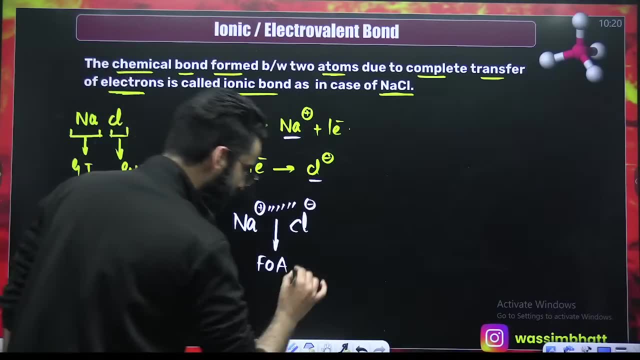 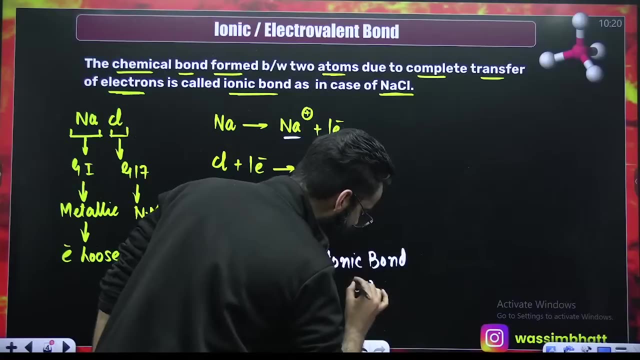 charged ions and that electrostatic force of attraction, that electrostatic force of attraction which arises between these two oppositely charged ions, that electrostatic force of attraction you will be calling as ionic bond. So either you will be calling it as ionic bond or let me tell you. 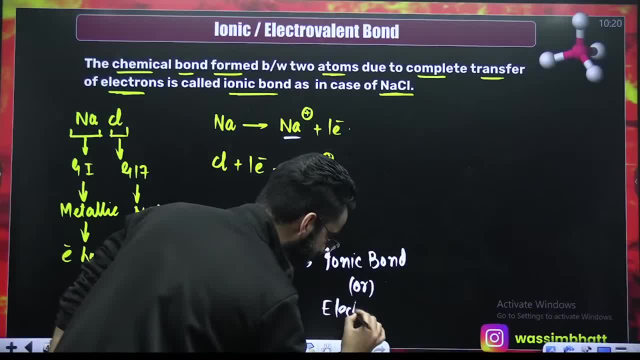 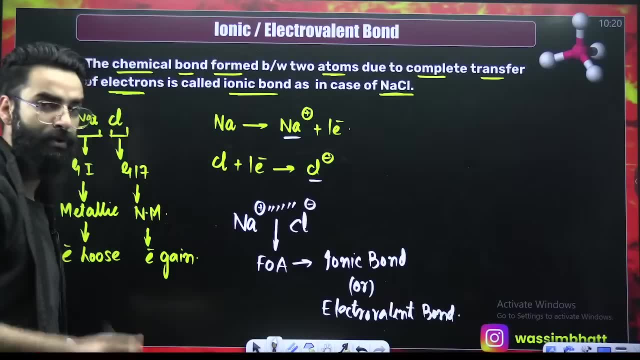 you will be calling this as the electrovalent bond. You will be calling it as the electrovalent bond. Can you let me know in the chats if you got the idea of what this ionic bond, what this electrovalent bond is all about? right? 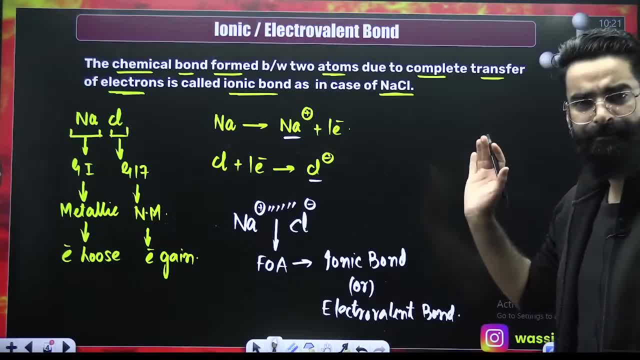 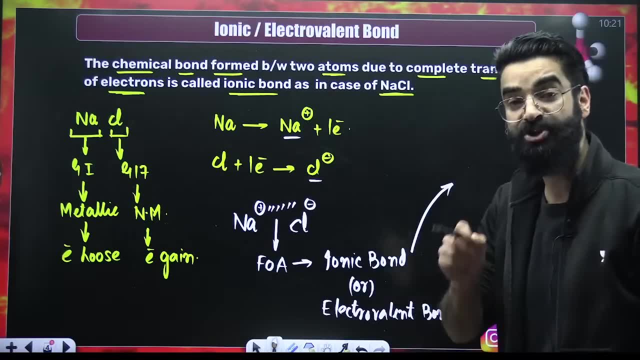 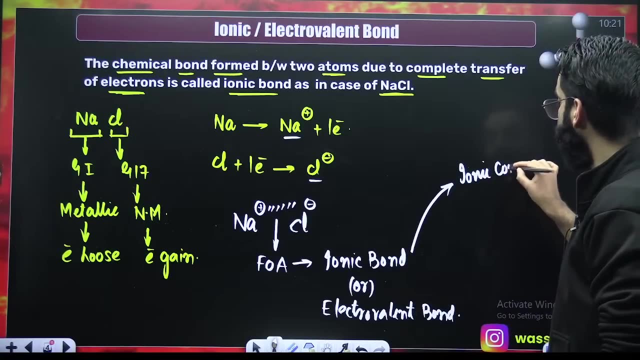 I hope I'm perfectly clear and let me tell you. let me tell you that particular compound, that particular compound in which ionic bond or electrovalent bond exists- that is something which you will be calling as ionic compound- That particular compound in which ionic bond or your 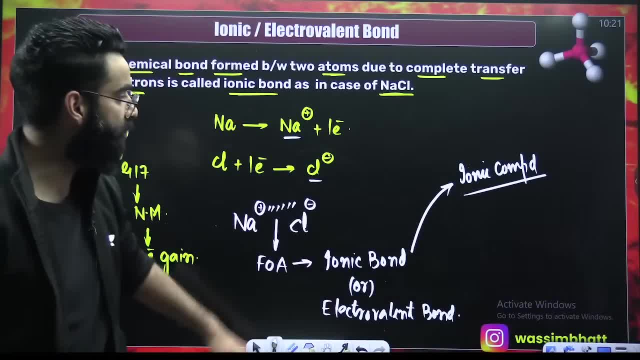 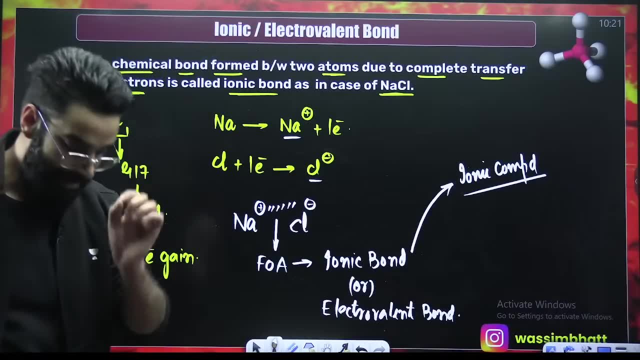 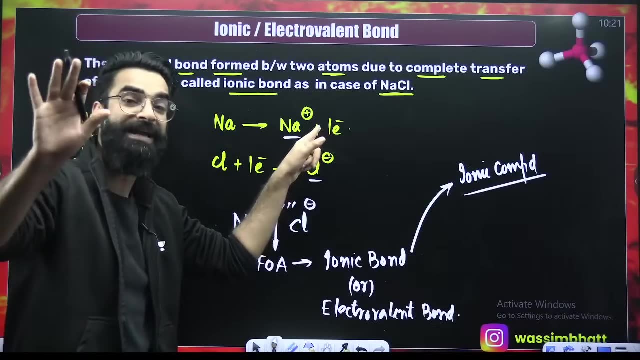 electrovalent bond exists. that particular compound is what you will be calling as ionic compound. Perfect, I hope I'm perfectly clear to everyone. My dear students, one more thing, one more thing. Remember: sodium lost its electron completely. Chlorine gained that electron. 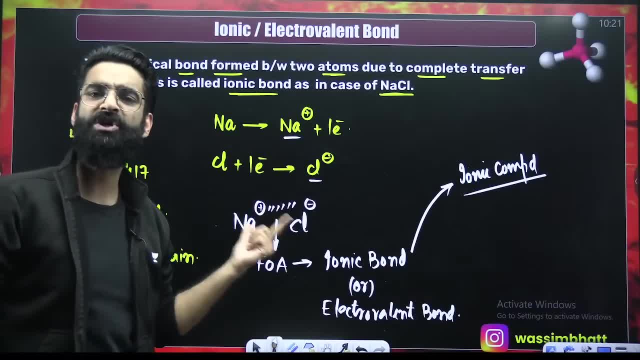 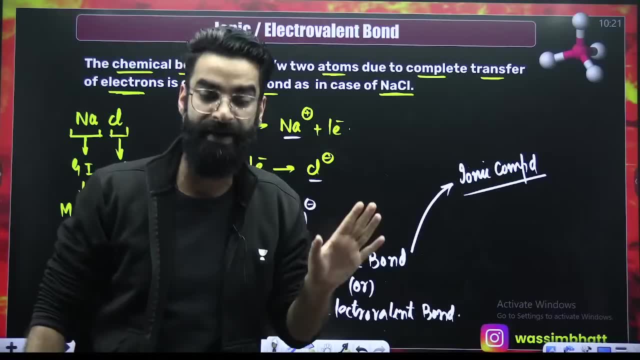 completely. So, can I say, during the formation of ionic bond. during the formation of ionic bond, can I say, complete loss and gain of electron is taking place Absolutely. So do remember, in your ionic bond, in your ionic bond, 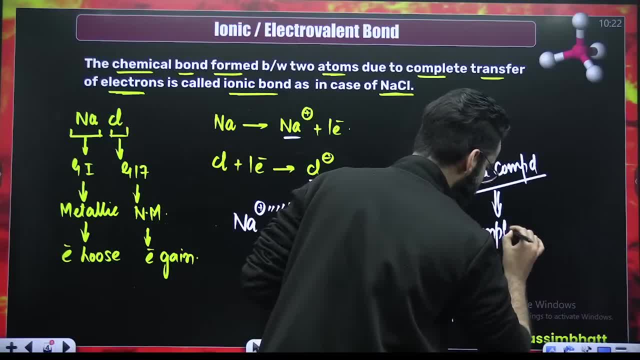 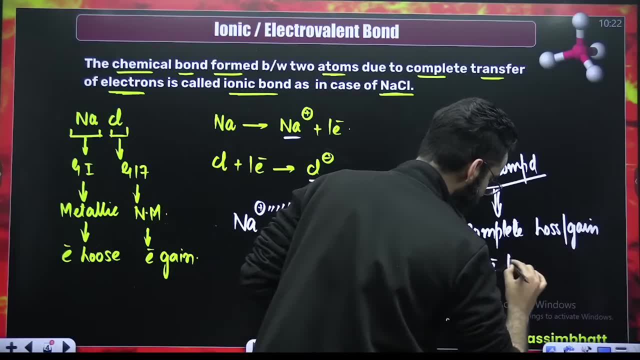 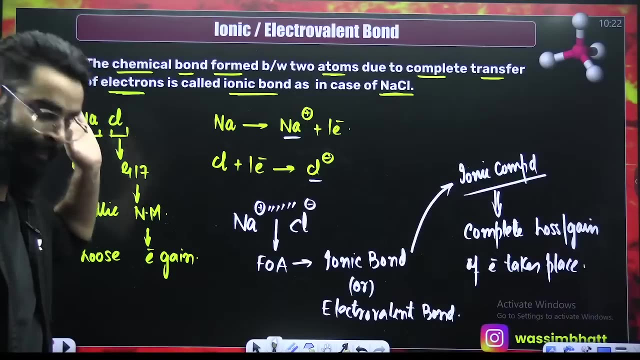 what happens? Complete loss and gain of electron takes place. Complete loss and gain of electrons takes place, Perfect. This is one more important point. I hope this is clear to everyone. Now, my dear students, the point is: what are the favorable conditions? 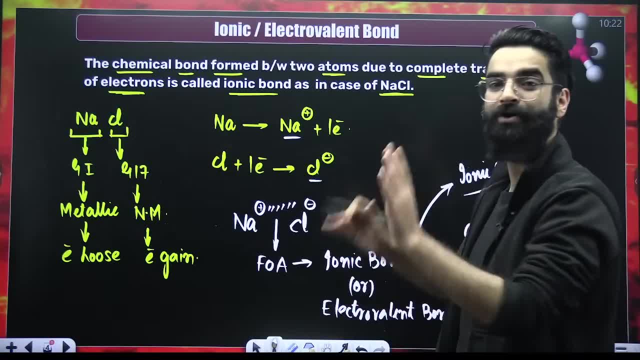 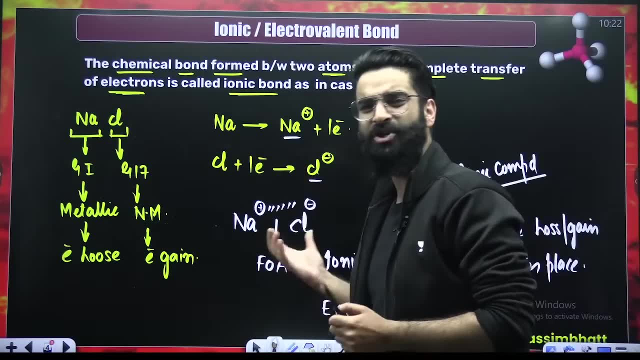 What are the favorable conditions for the ionic bond to get formed? What are the favorable conditions for the ionic bond to get formed? See, guys, it's evident For the formation of ionic bond what has to happen. Ketane has to get formed easily, Right, Ketane has to get formed. 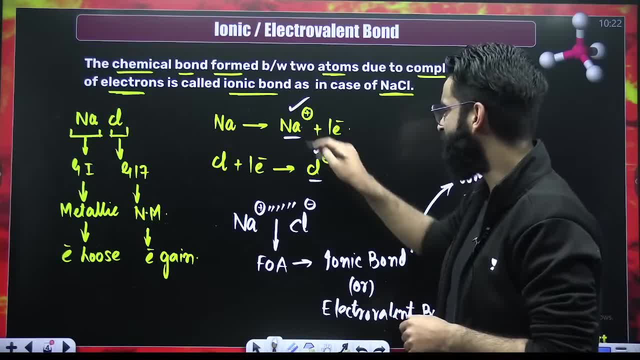 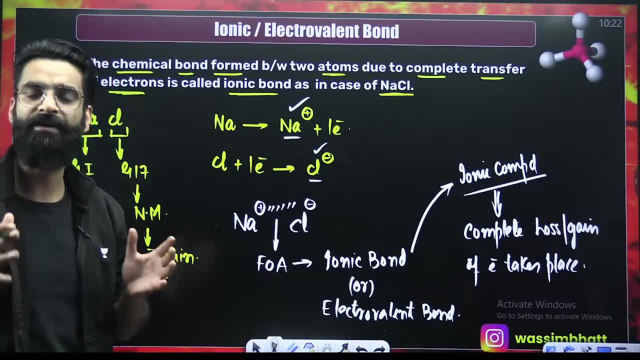 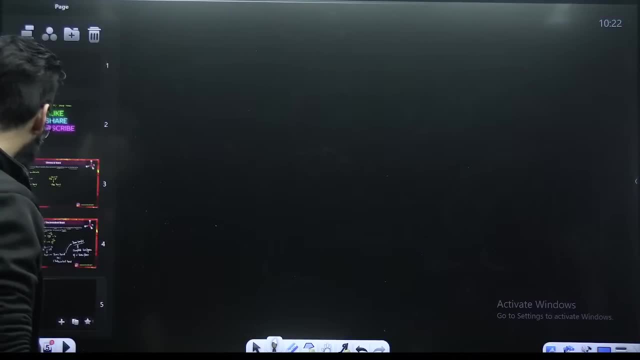 Anion has to get formed. Once ketane anion is formed. once ketane anion is formed, then there will be attraction between them. Then there will be attraction between them Right. Then there will be attraction between them- Perfect. Now try to understand what exactly I'm going to talk about. 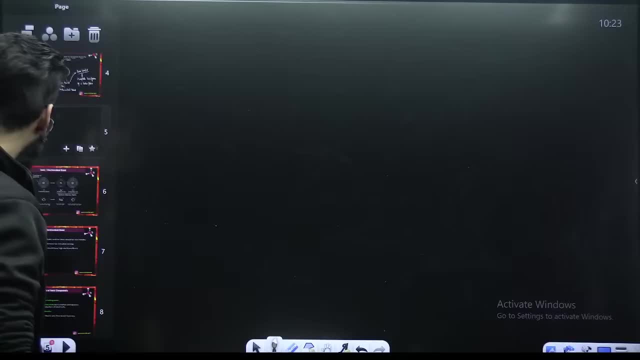 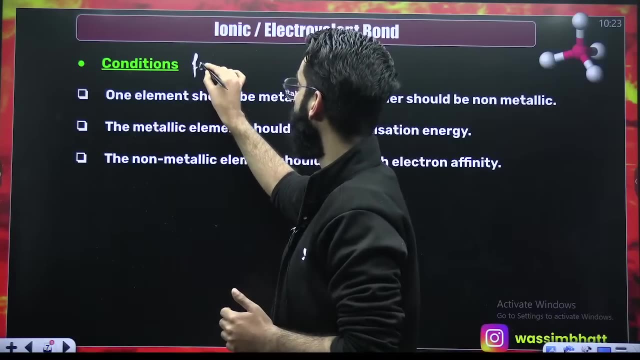 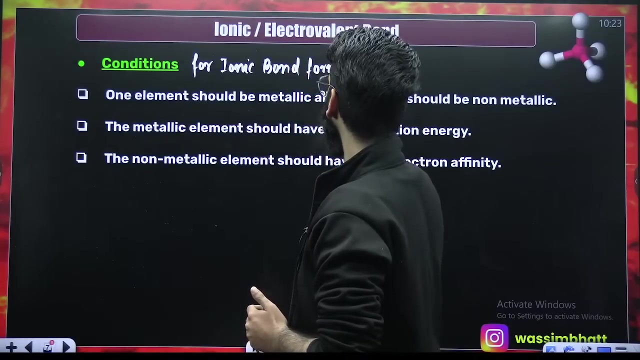 Try to understand what exactly I'm going to talk about, My dear students. what are the conditions? Conditions for the ionic bond formation, Conditions for the ionic bond formation, Or I'll say, conditions for favorable conditions for the ionic bond formation. Try to understand what. 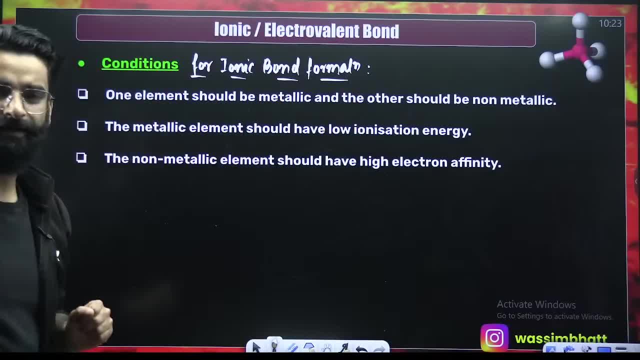 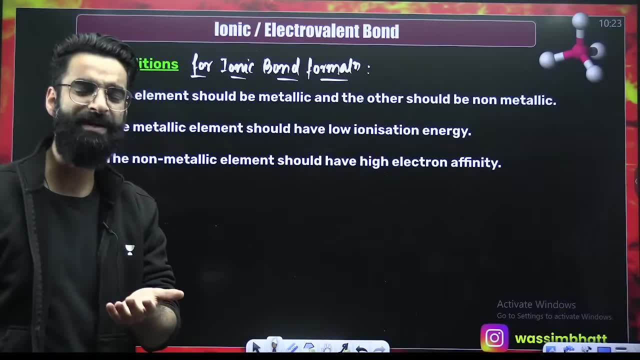 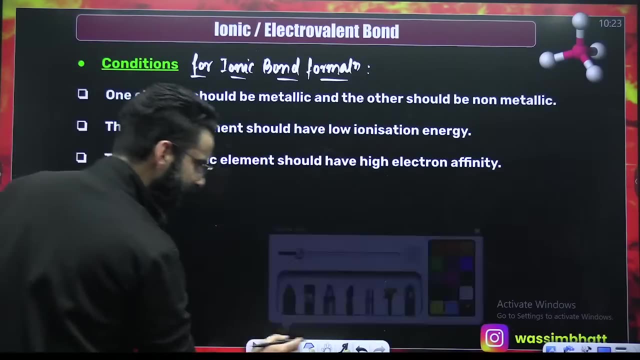 exactly. I'm going to say The first thing. the first thing, it's evident. it's evident, my dear students, for the formation of ionic bond, keta, n formation has to take place, nn formation has to take place right. So I'll say one simple thing. I'll say one simple. 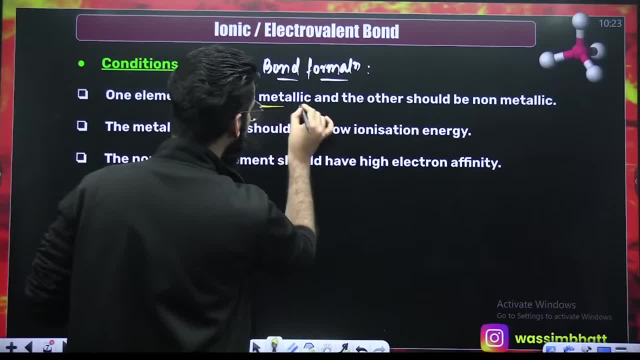 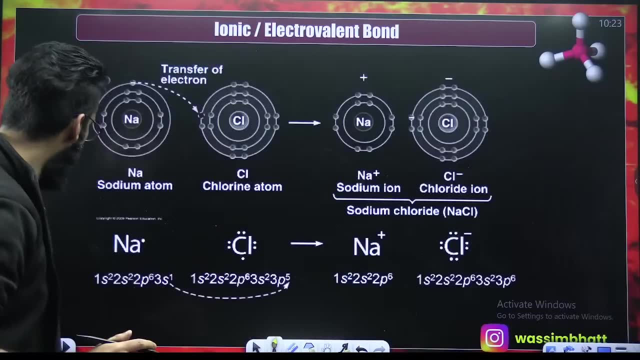 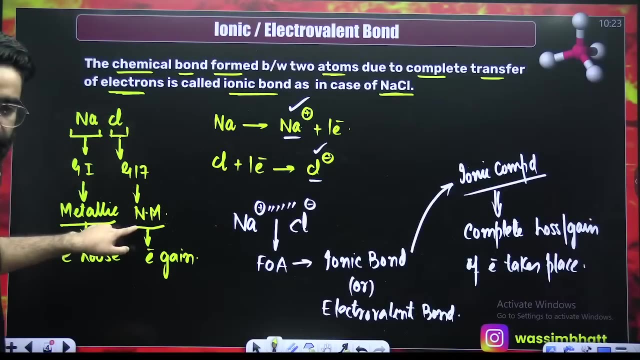 thing, The first condition: one element should be metallic and another should be non-metallic. right, As you have seen over here, your sodium, your sodium, it was metallic in nature. Your chlorine, it was non-metallic in nature. Metallic one, it has got tendency to lose electrons. 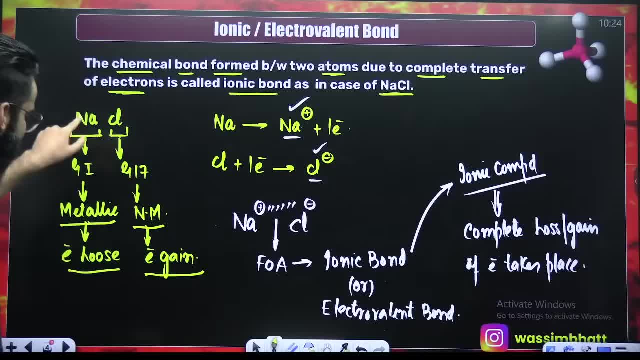 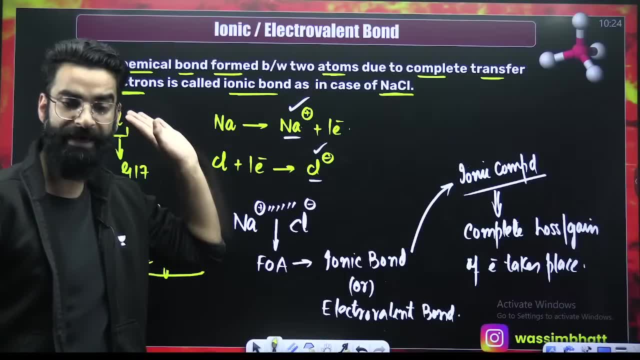 non-metallic one. it has got tendency to gain electrons, right. If one has got tendency to lose electrons, then only it can form keta n. If one has got tendency to gain electrons, then only it can form anion right. Then only it can form anion perfect, And once keta n. 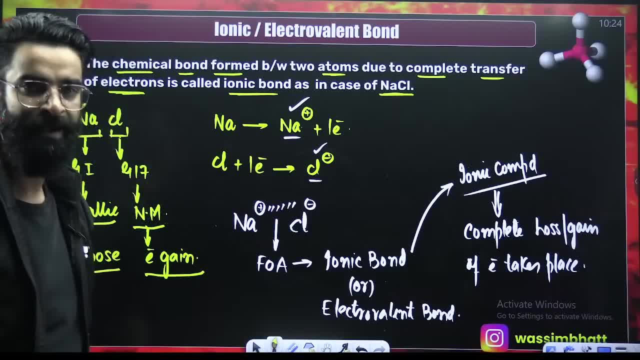 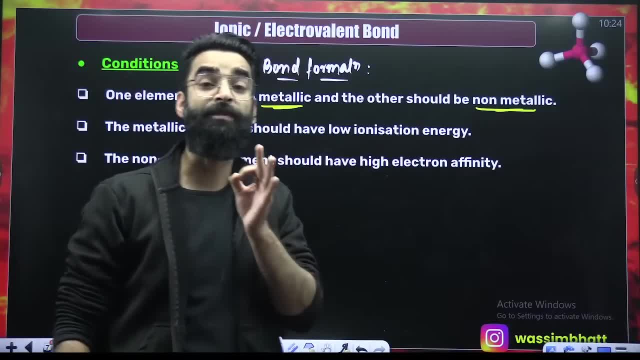 gets formed, then automatically, Automatically, there will be force of attraction between them, and that force of attraction is your ionic bond. So remember the first thing, the first condition: One element definitely should be metallic, another one should be non-metallic. 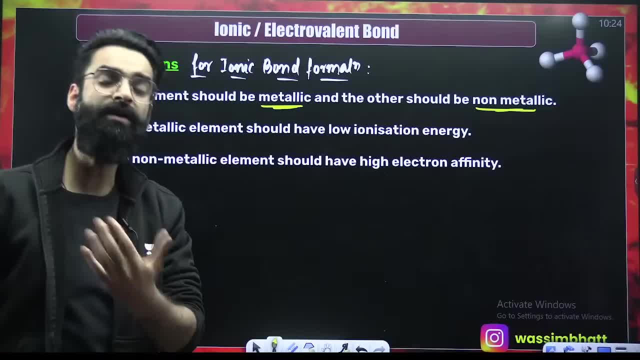 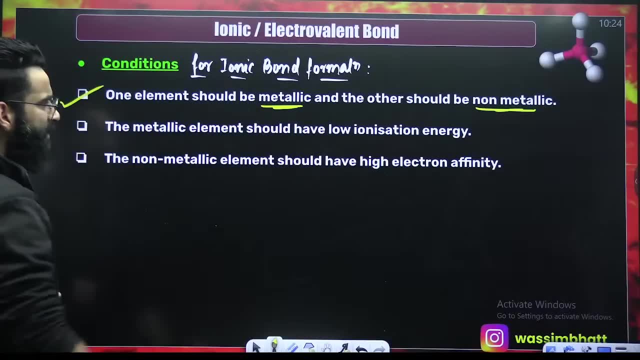 Metallic one loses electron forms cation. Non-metallic one gains electron, forms the anion. right Now, my dear students, try to understand very carefully. One element should be metallic in nature and another one should be non-metallic in nature. 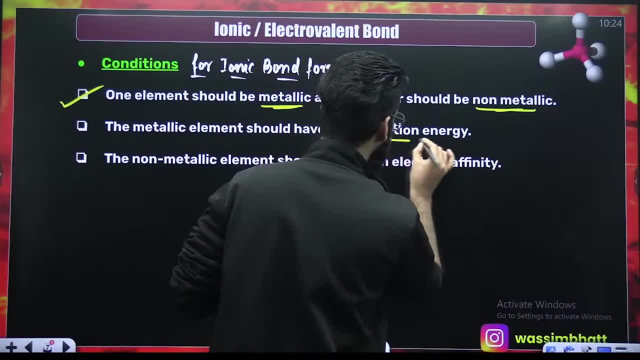 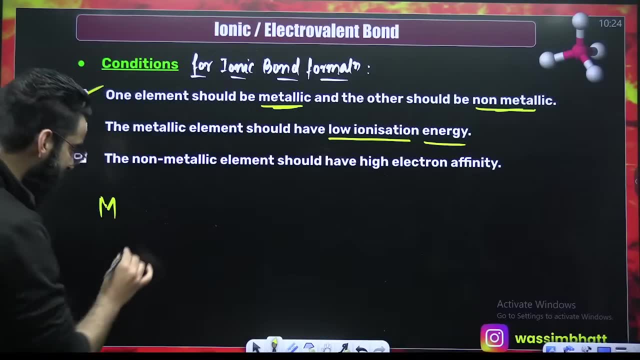 The one which is metallic in nature, it should have low ionisation energy, right? So the one which is metallic in nature, which loses electrons and forms cation, Now the one which is metallic, it should have low ionisation energy. If it has got low ionisation energy, 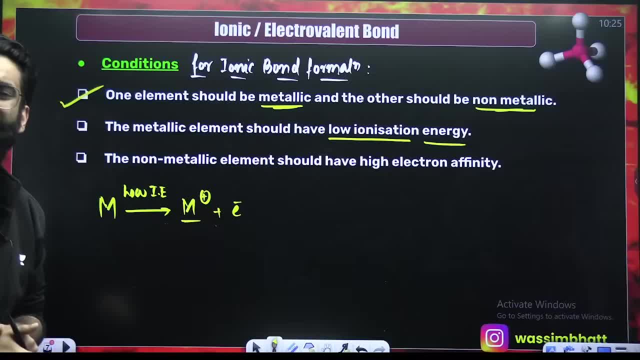 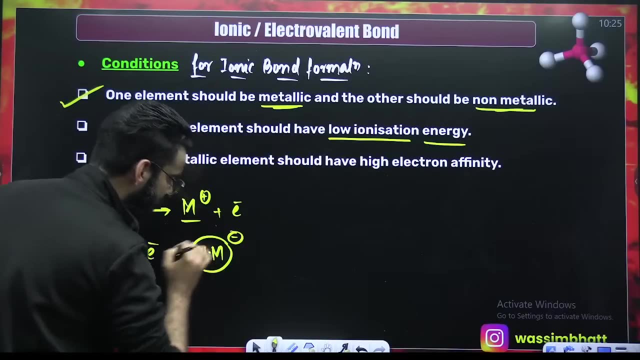 can form the cation easily, then it can form the cation easily. right, then it can form the cation easily. similarly, that element which is non-metallic in nature, that element which is non-metallic in nature it gains electron, gets converted into what gets converted into the anion gets converted in. 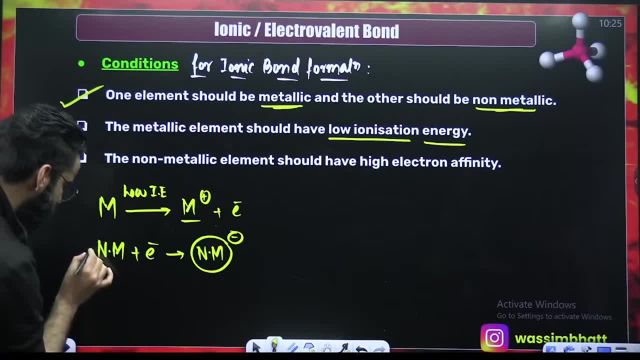 the anion perfect, since it's gaining electron. can i say this: non-metal should have high electron affinity. it should have high electron affinity. this should have low ionization energy, because if the metal has got low ionic energy then it can form cation easily. if it has got more high, 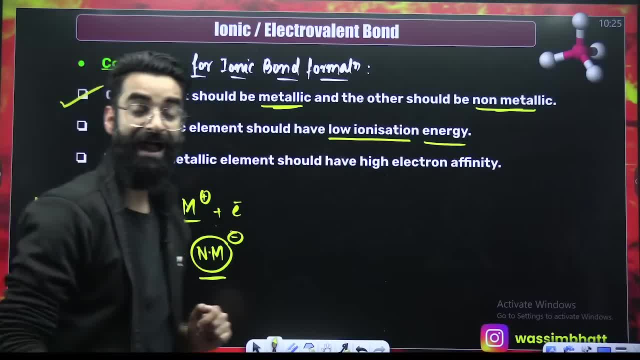 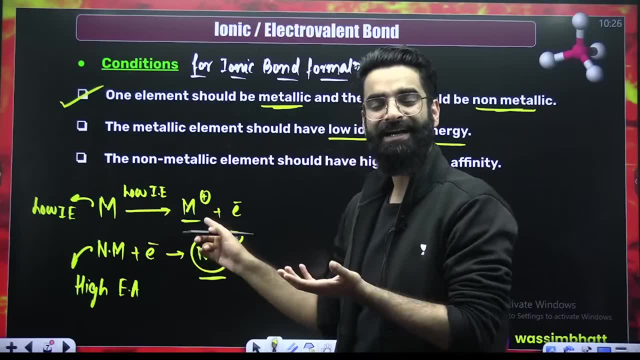 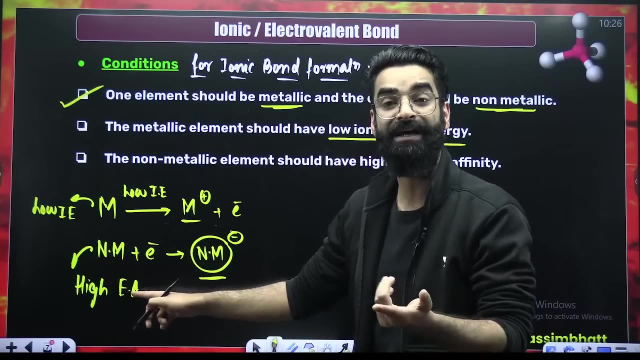 electron infinitely, then it can form anion easily. right, and as as that particular metal which has got low ionish energy, that forms the cation easily. so that is the best candidate for the formation of cation. similarly, that non-metal which has got high electron affinity, that is the best candidate for. 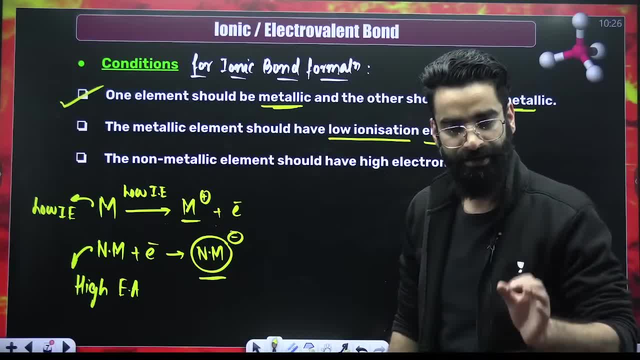 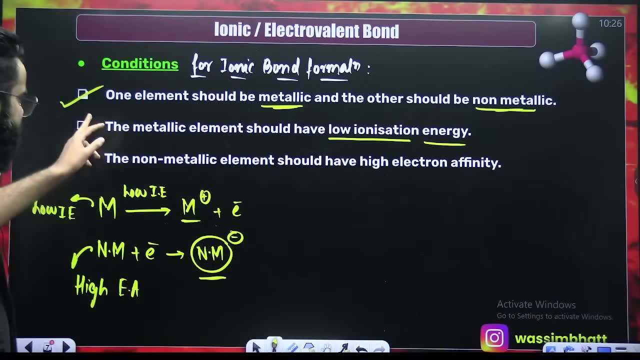 the formation of what? for the formation of anion, perfect. so, my dear students, remember, remember from now onwards, remember from now onwards. this is very important. one element has to be metallic, another has to be non-metallic. number one, number two: the one which is metallic that should have low ionization energy. 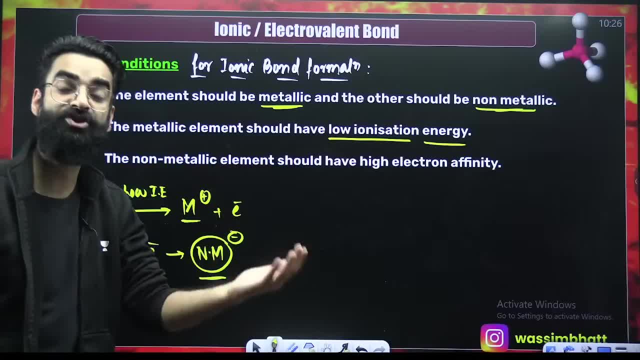 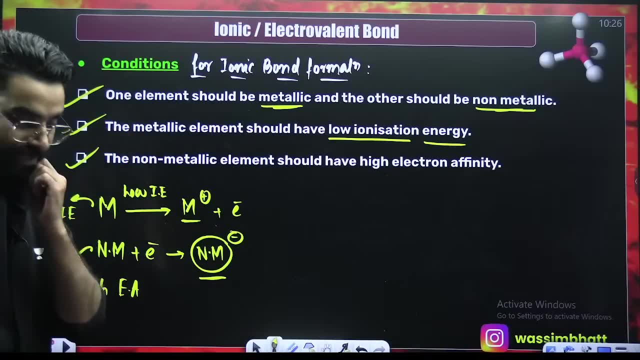 then only it can form the cation easily, the one which is non-metallic, that should have high electron affinity. then it can form anion easily. right, then it can form anion easily. I believe these conditions are absolutely clear to everyone of you. okay, now people. 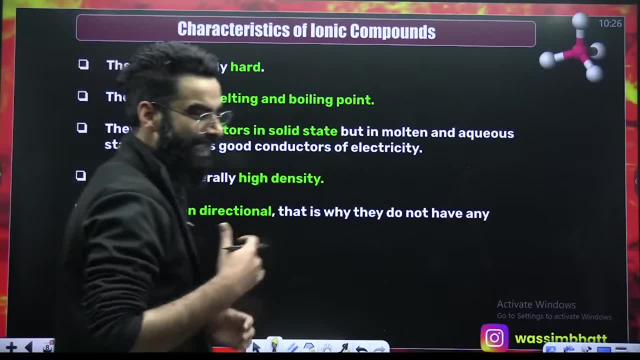 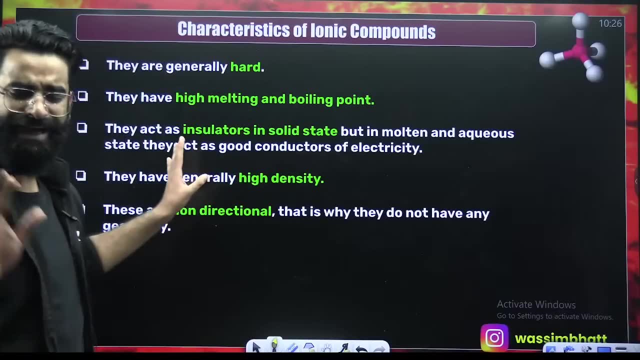 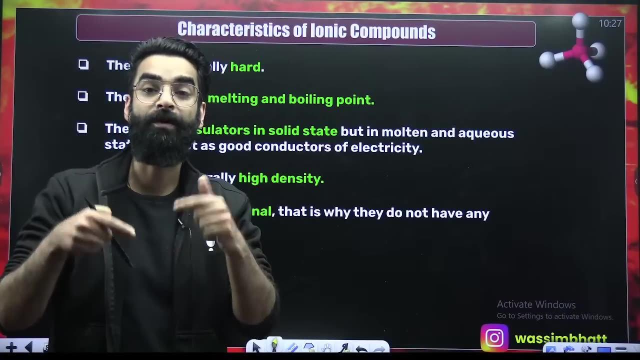 now, people, there are some important characteristics of these ionic compounds which you need to know, some important characteristics. try to understand. notes at the end I will give you okay in the telegram. my dear students, since we saw, in ionic compounds there is ionic bond. what is ionic bond? 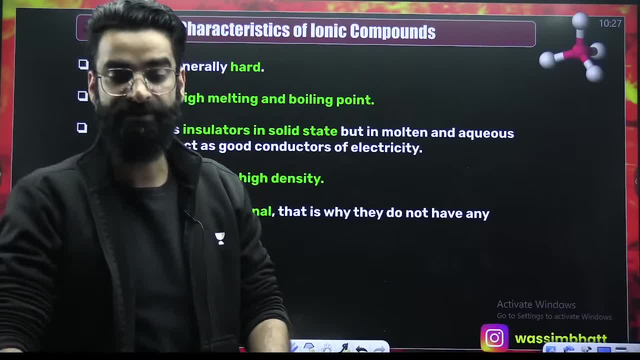 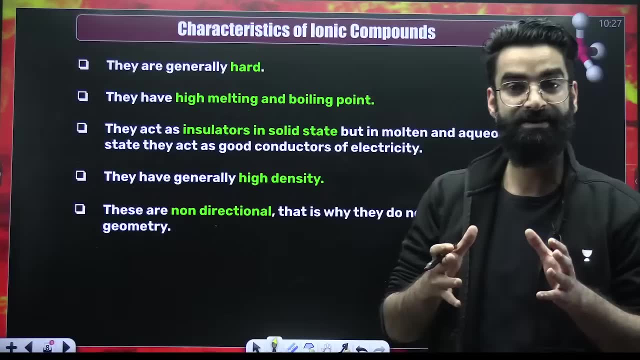 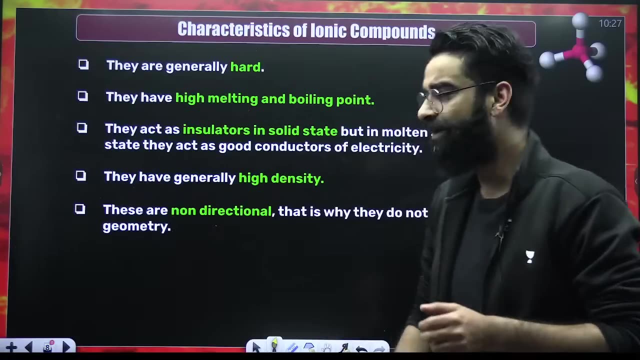 electrostatic force of attraction and you know, electrostatic force of attraction, that is very strong, that is very strong, right, electrostatic force of attraction is one of the strongest forces, perfect right, due to which, if electrostatic force of attraction is the strong, stronger force, right. can I say? 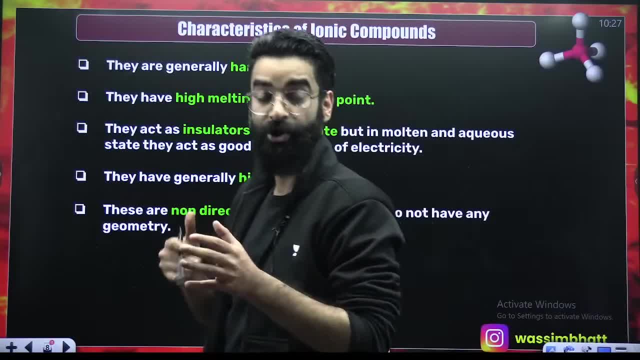 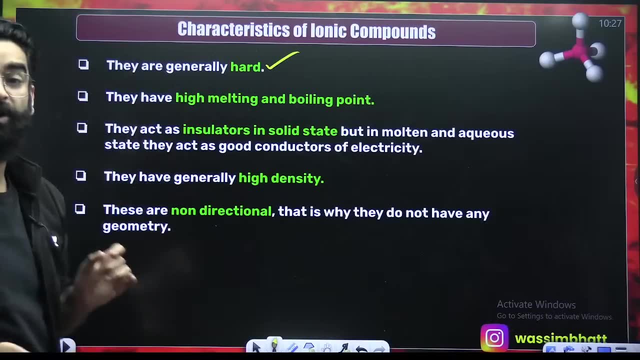 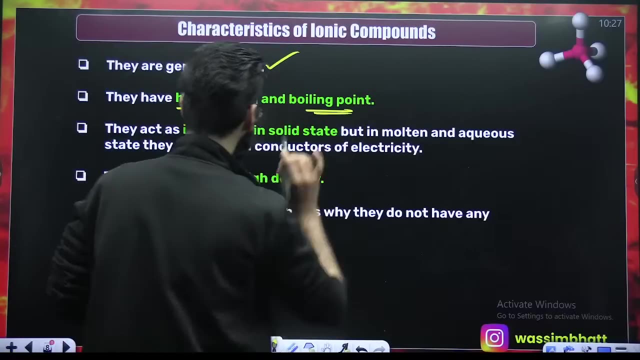 your ionic compounds. they will be generally hard due to the strong electrostatic force of attraction which exists between the ions right, your ionic compounds. they are going to be generally hard. number one, due to the strong electrostatic force of attraction, they will have high melting and boiling points. 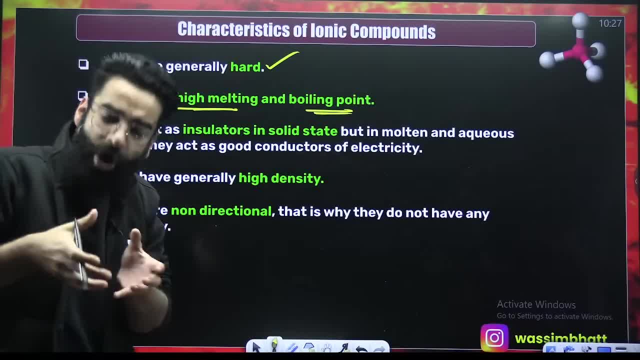 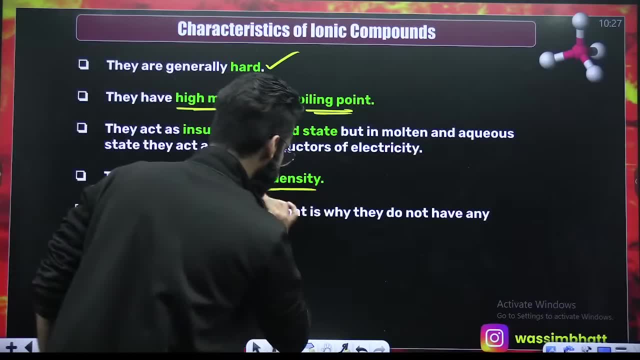 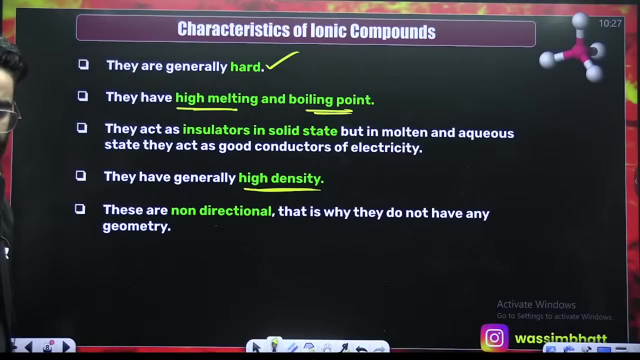 they will have high melting and boiling points due to the strong force of attraction. these ions will be very close. if the ions are very close, my dear students, these ionic compounds, they will have high density, they will have high density, they will have high density, right, they will have high density. 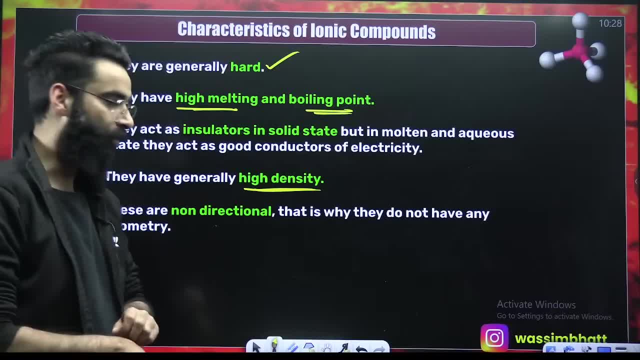 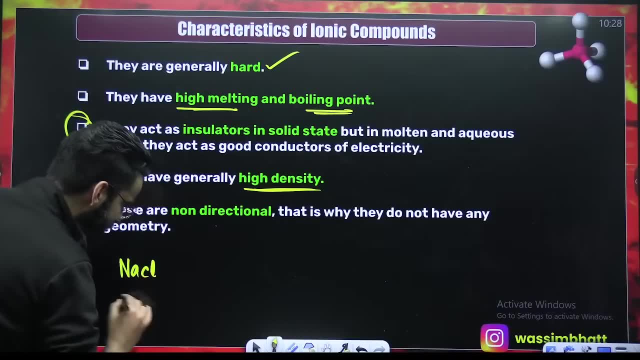 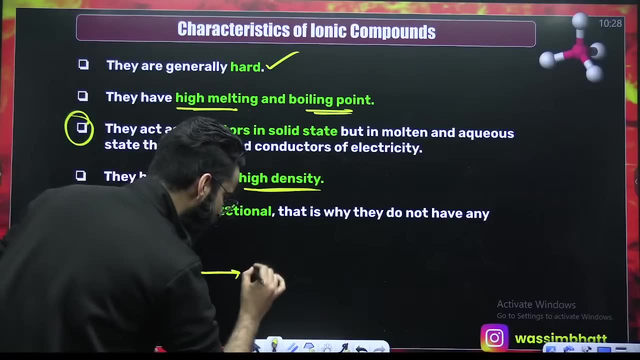 perfect. one more thing, one more thing. do remember this particular point, my dear students. for example, you have taken the ionic compound as NaCl. let's say it's in solid state here. NaCl solid- perfect. now, for example, I am converting this into NaCl liquid. 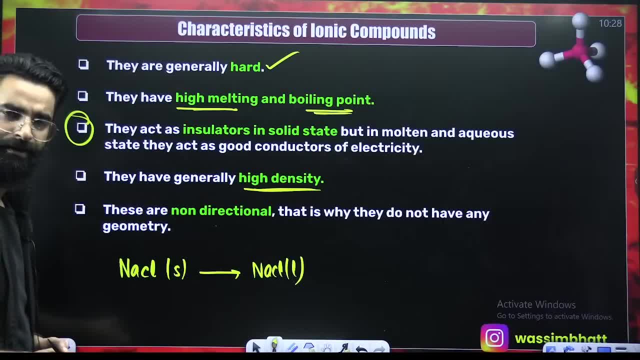 perfect, I am converting this into NaCl liquid. I had NaCl solid. now I am, for example, heating it up, continuously heating it up. I am heating it up till it gets converted into a liquid. perfect, my dear students, when your ionic compound is in solid form, 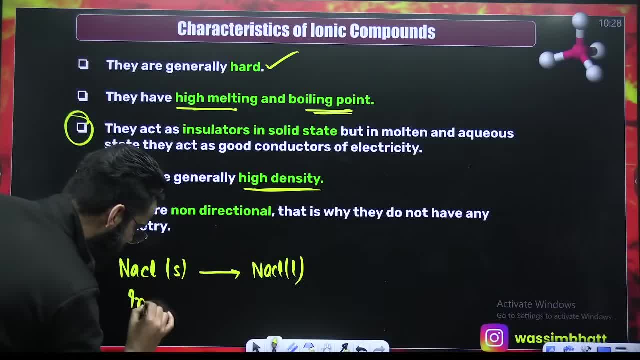 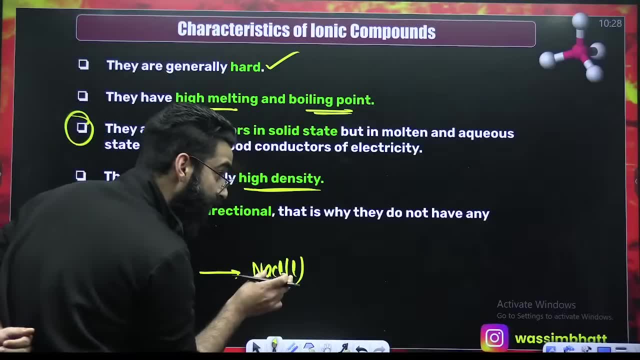 when your ionic compound is in your solid form, it behaves like your insulator. it behaves like your insulator when the same ionic compound is in molten form, is in molten form, you call this state as molten state. you call this state as the molten state. 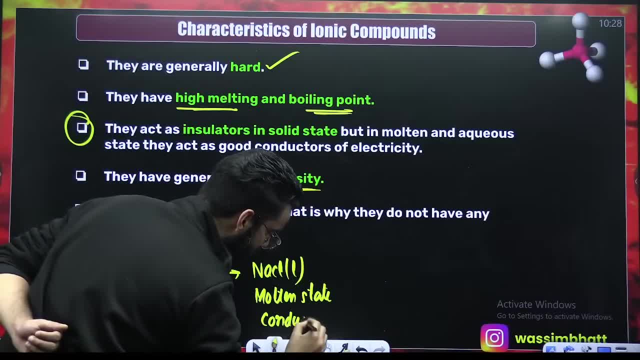 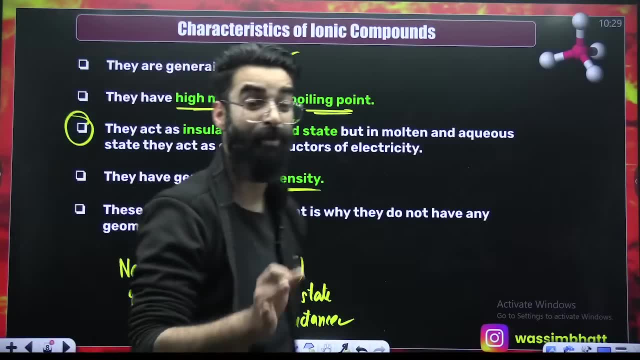 remember it behaves like your. it shows the conductance. it shows the conductance when it is in solid form. it does not show conductance when it is in liquid form. it shows the. when it is in molten form, it shows the conductance. or when the same ionic compound. 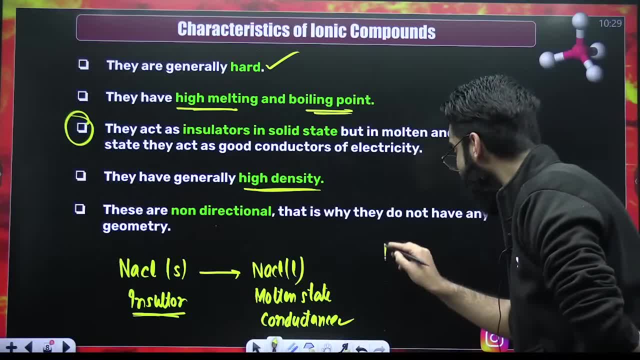 is in aqueous form is in aqueous form, it also shows the conductance. when the same ionic compound is in aqueous form, it also shows the conductance. when the same ionic compound is in aqueous form, it also shows the conductance. it also shows the conductance. 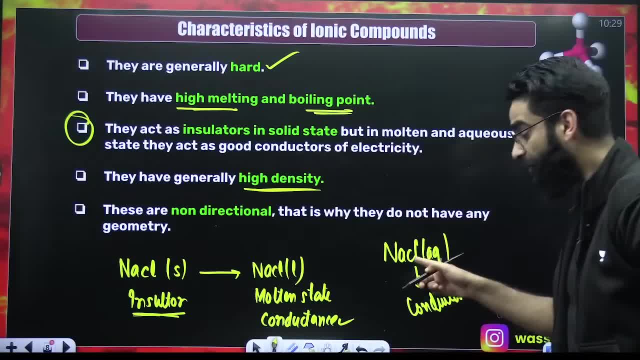 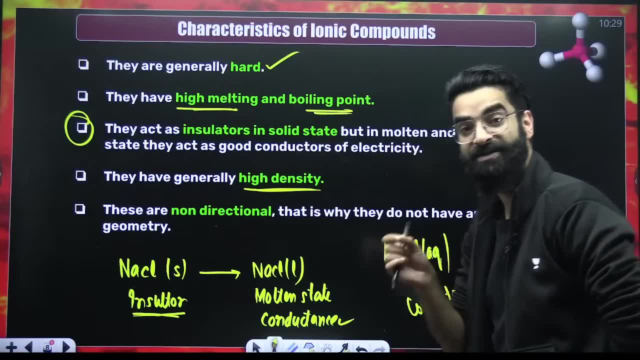 when the same ionic compound is in aqueous form, it also shows the conductance right. i hope you know what is meant by NaCl aqueous. that means with NaCl there is water associated as well. with NaCl there is water associated as well. perfect. 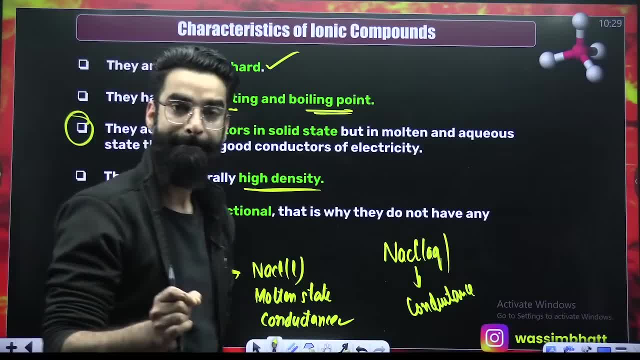 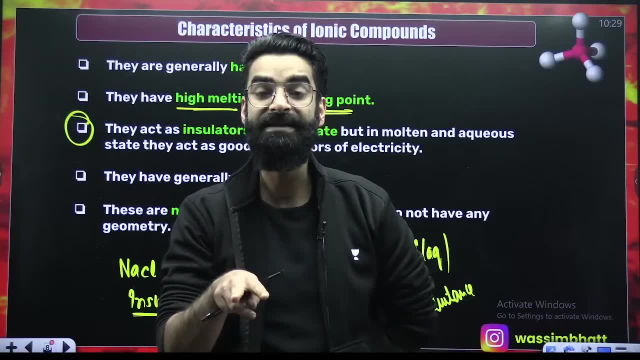 right. so do remember this particular point from now onwards, my dear students. when ionic compound is in solid state, it behaves like the insulator. it behaves like the insulator. when it is in molten or aqueous state- molten or aqueous state- it is going to behave. 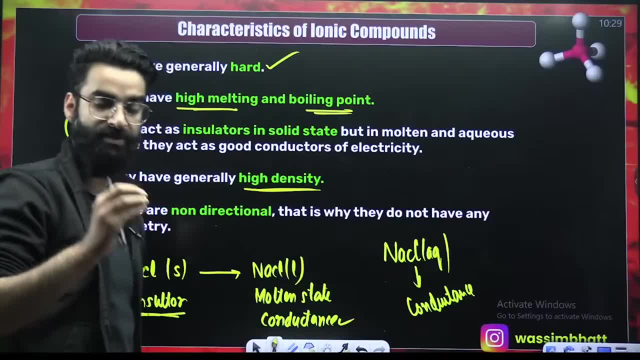 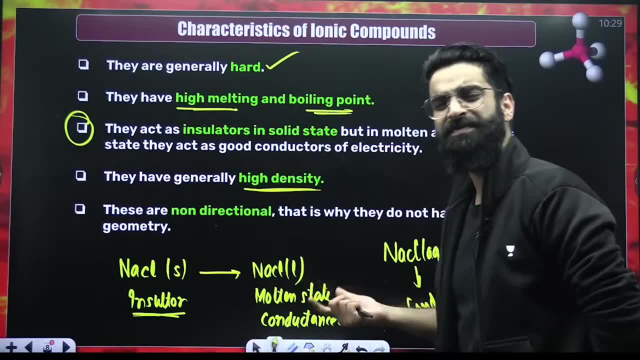 it is going to show conductance right, it is going to behave like your conductor, perfect. one more thing, dear students. one more thing, dear students. these ionic compounds which we are talking about right now, they do not show any regular geometry. they do not show any regular geometry. 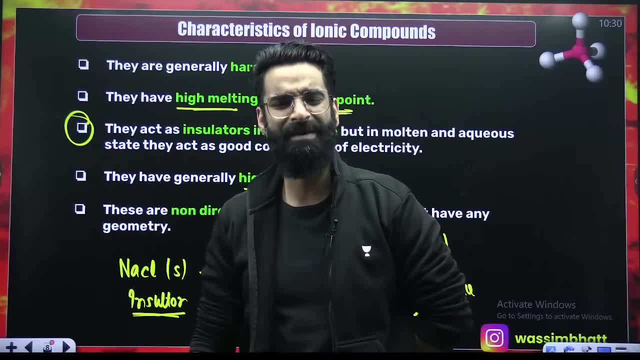 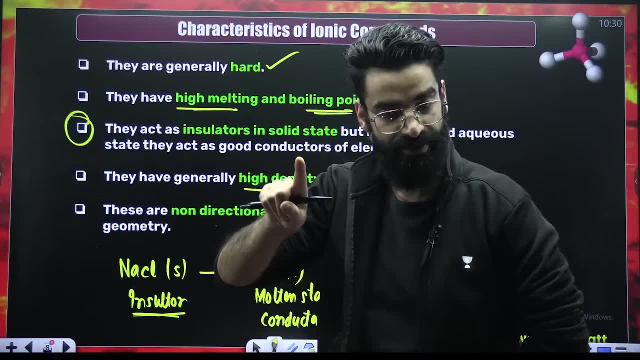 have you heard ever that this ionic compound is trigonal, bipyramidal, that this ionic compound is linear? this ionic compound is bent? no, that we see in covalent species, that we see in covalent compounds. right, that we see in covalent compounds. 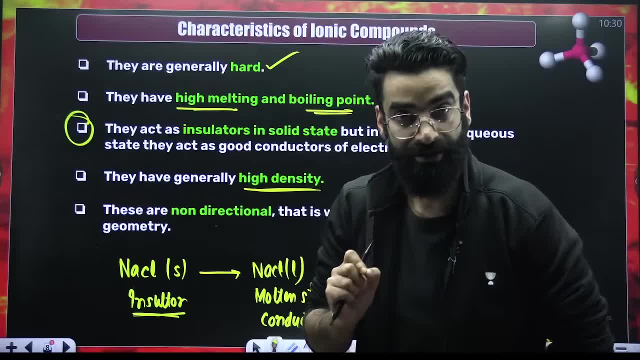 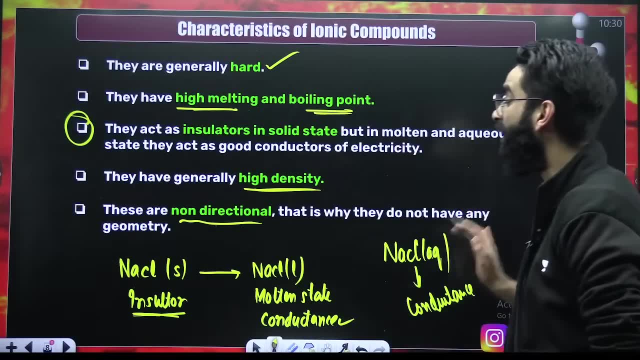 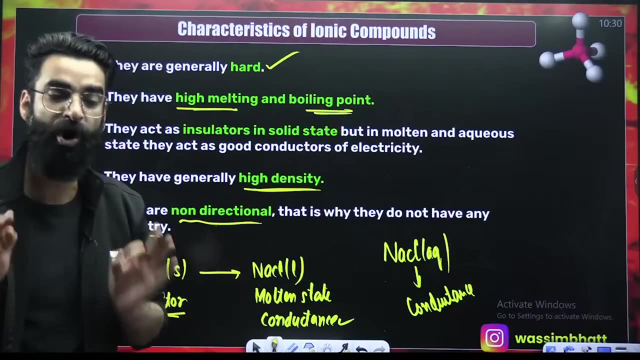 in ionic compounds, the bonds are non-directional. the bonds are non-directional, right. the bonds are non-directional, perfect right. there is no regular geometry. we do not say: ionic compound has got this shape, has got that shape, no right. geometry is not defined. 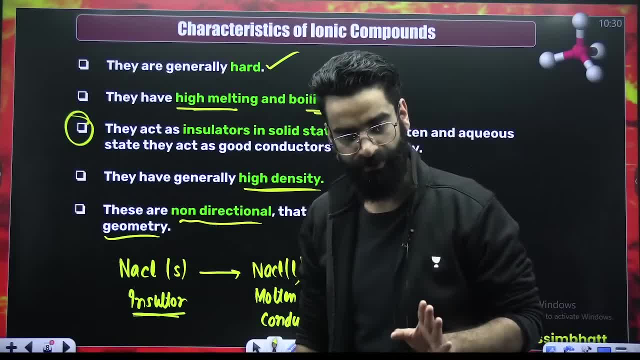 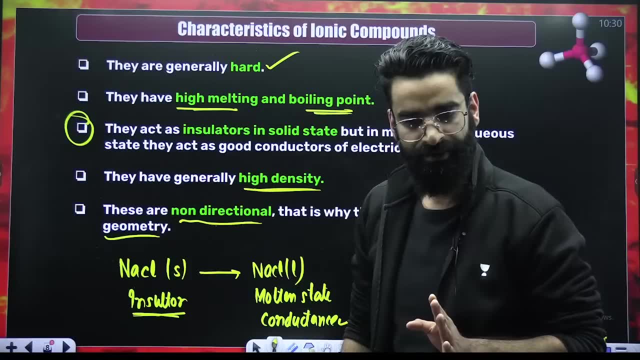 geometry is not defined for what geometry is not defined for the ionic compounds? this one more thing which you are going to remember from now onwards: what is the difference between ionic compound and non-directional in ionic compound? guys, its simple. over here you have taken. 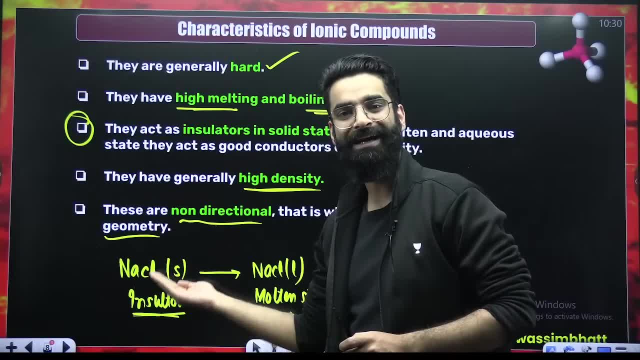 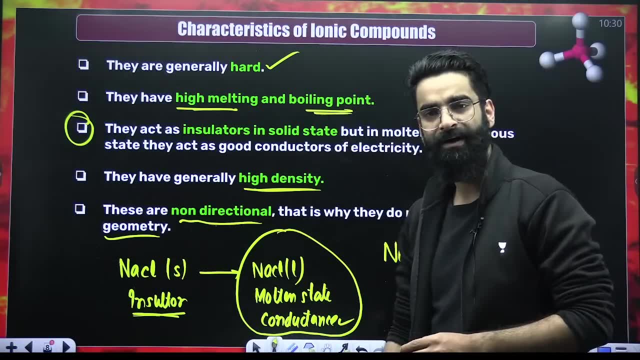 NaCl solid. right, you are heating it up. you are heating it up. you are heating it up till it gets converted into liquid. right till it gets converted into liquid, perfect. what is meant by this? this is NaCl in liquid form, for example. this is the marker. 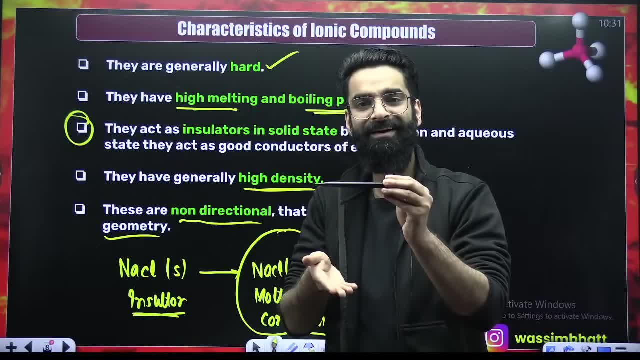 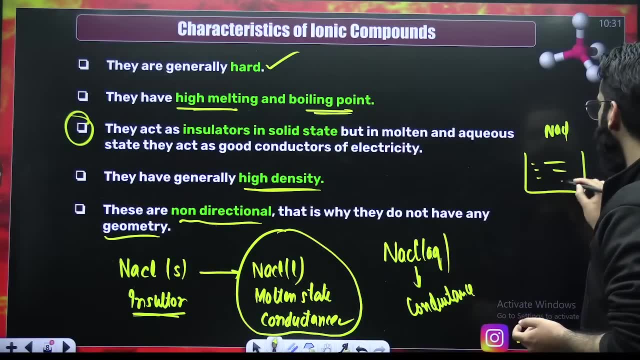 right. it is in solid form. i am heating it up. it will get converted into liquid, right, perfect, same NaCl. If I take same NaCl and I'm introducing it into water, I'm introducing it into water, Perfect Right. Then NaCl- over here I'll be writing as NaCl aqueous. There is water associated with. 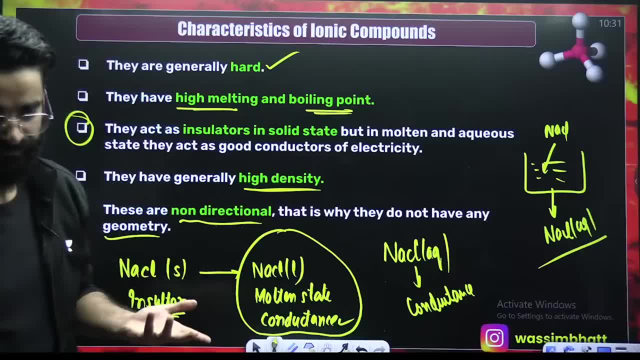 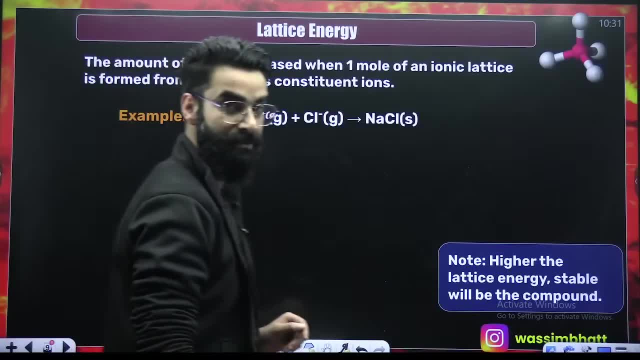 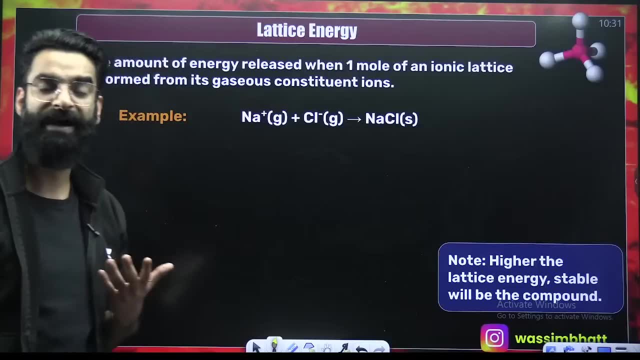 this NaCl as well. So remove these points. It's simple. Perfect, Now people, Now people. There are few things which you need to know about their ionic compounds. Few things which you need to know about these ionic compounds. Number one: Lattice energy. Lattice energy- How do we define the term? 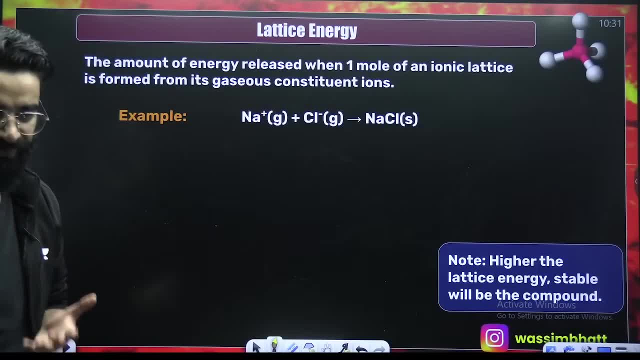 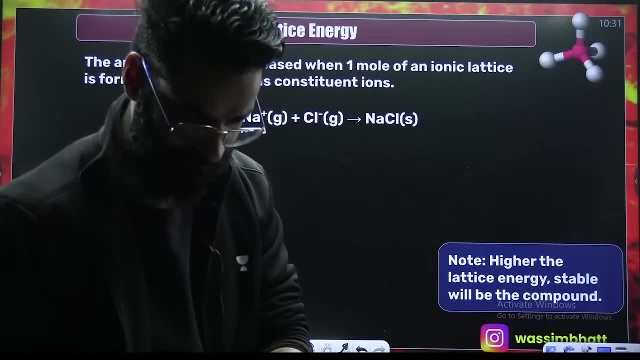 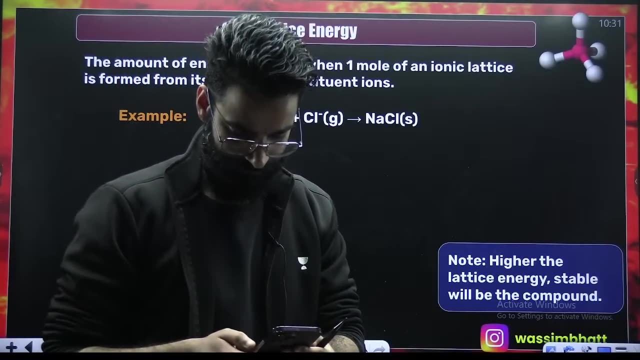 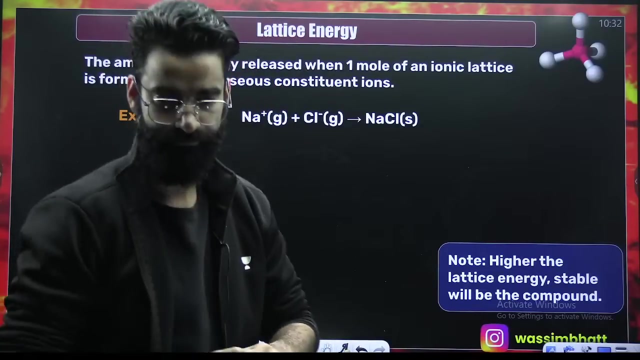 lattice energy. Okay, How do we define the term lattice energy? Try to understand. This is important. Okay, Just a second. Just a second: people. Okay, Lattice energy. If you look at its definition, The first definition about lattice: 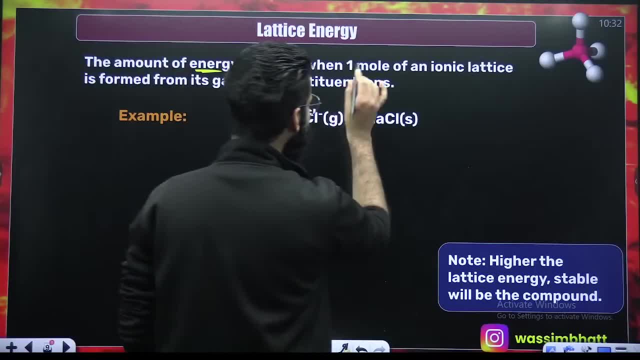 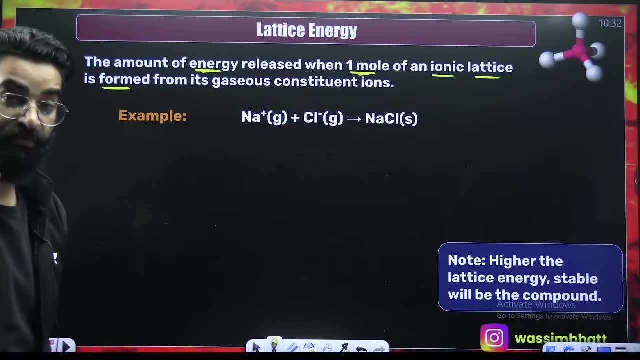 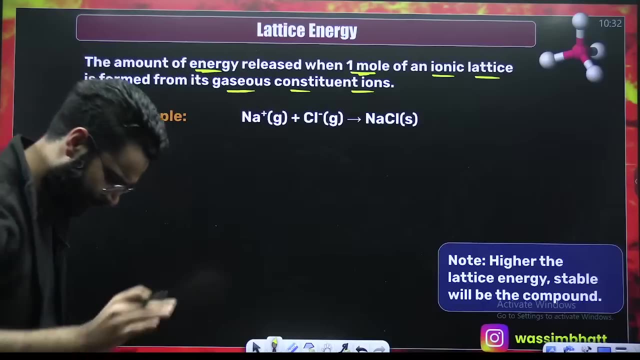 energy. The amount of energy which is released when one mole of an ionic lattice is formed. The amount of energy which is released when one mole of an ionic lattice is formed from its constituent gaseous ions. What it means, First thing: do remember, Do remember. 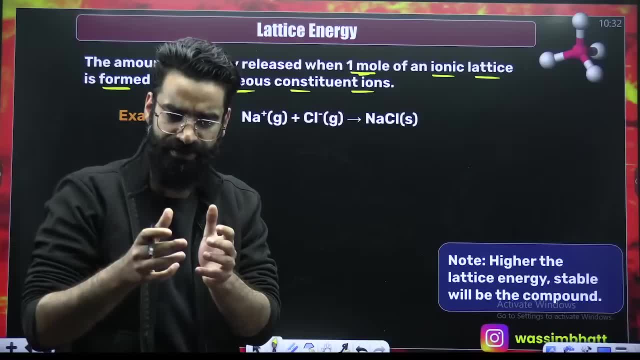 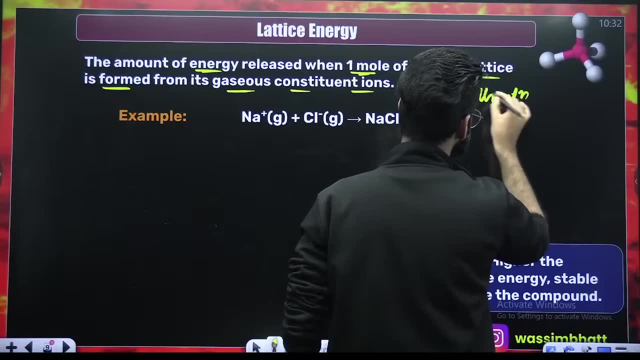 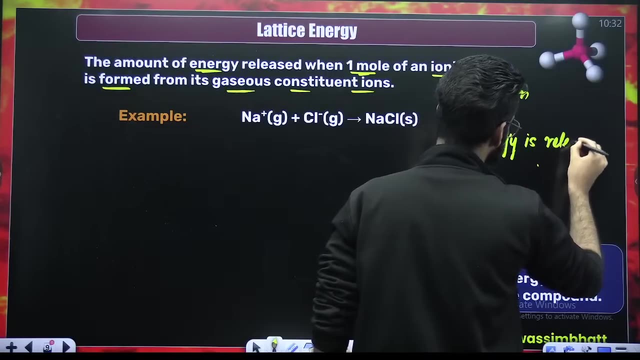 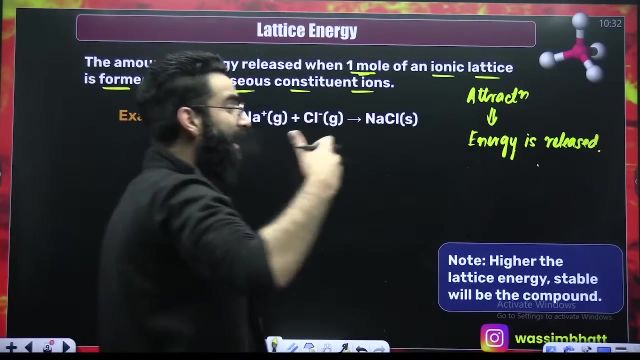 Whenever you see attraction Between the species, Whenever you see attraction between the species, Whenever you see attraction between the species, Do remember Energy is released at that point of time. Do remember Energy is released at that point of time And, due to the release of energy, Do remember. 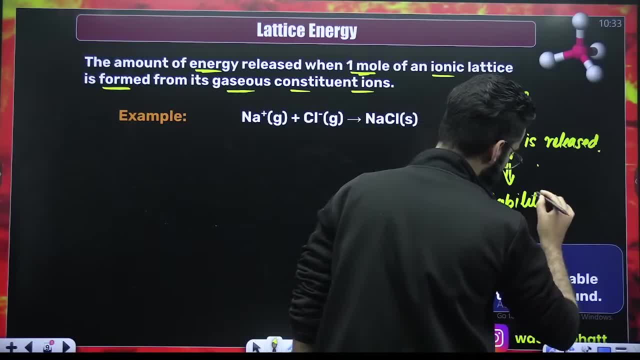 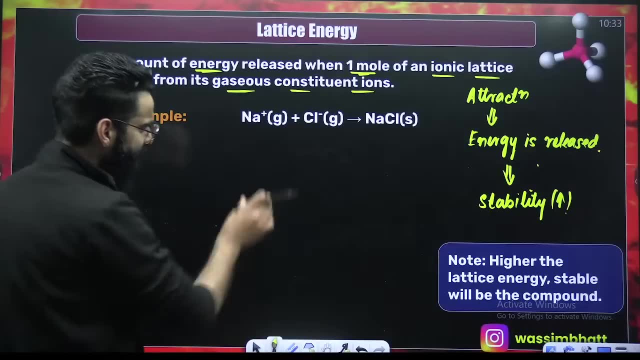 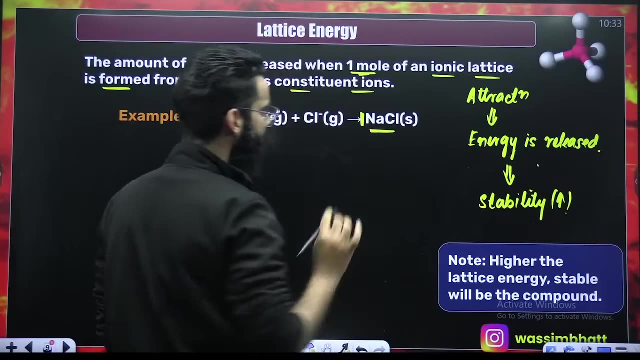 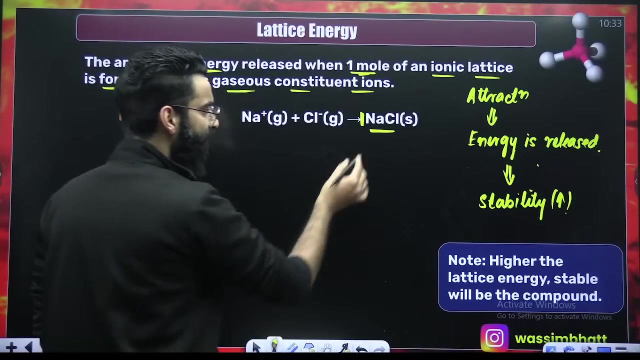 Stability increases. Do remember Stability increases, Do remember Stability increases. Now, If you look carefully, Look carefully, Can I say, in this particular reaction, One mole of ionic compound is getting formed. Absolutely One mole of ionic compound is getting formed From what? From what? From what? From its constituent gaseous ions. 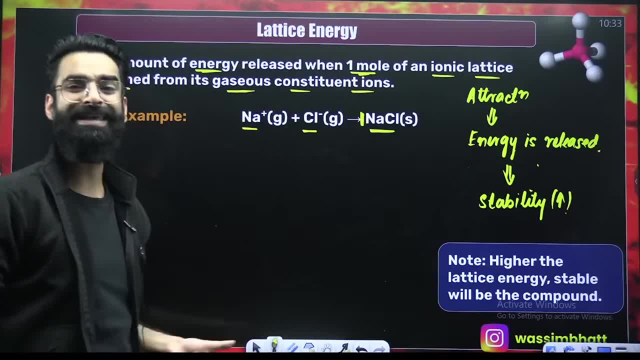 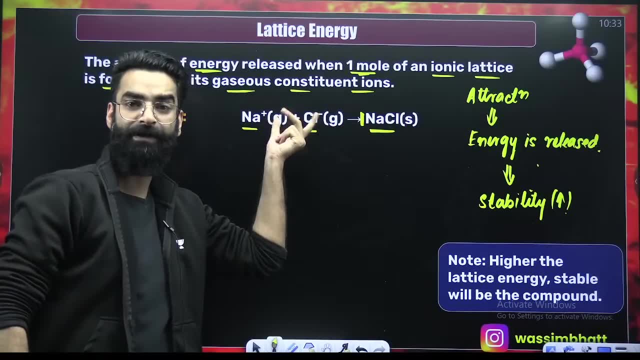 One mole of ionic compound is getting formed From its constituent gaseous ions. This is positive, This is negative And it's forming NaCl. So there will be attractions. There will be attractions. This Na positive would have attracted Cl negative. 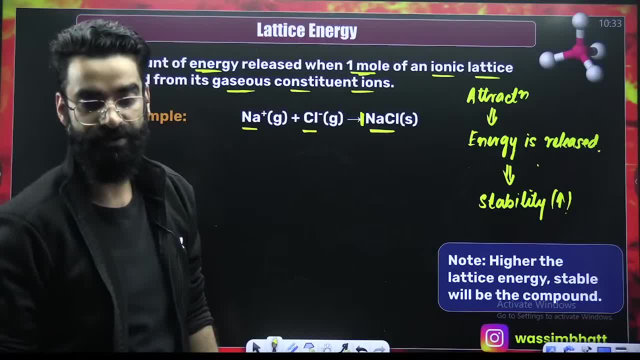 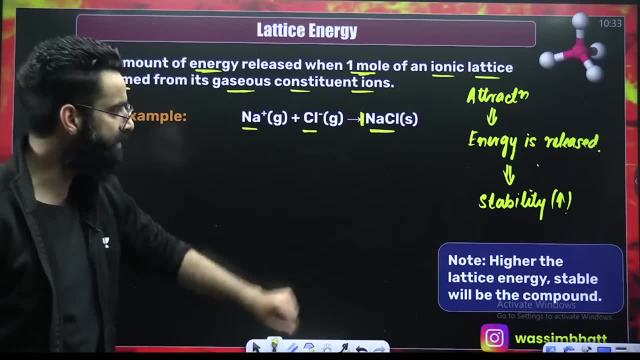 Formed NaCl, There will be attractions. And due to attractions, What happens? Due to attractions, What happens? Energy is released. Stability is increased. Right, My dear students, Look carefully. One mole of ionic compound is getting formed from its constituent gaseous ions. 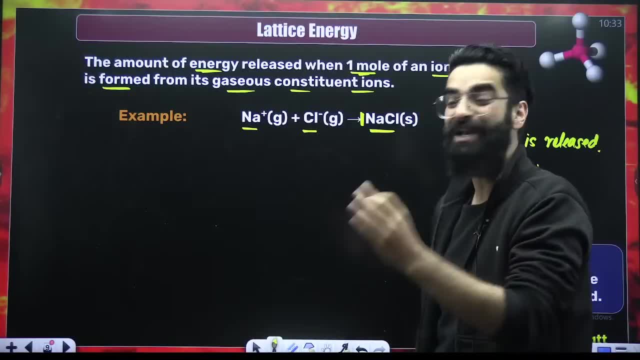 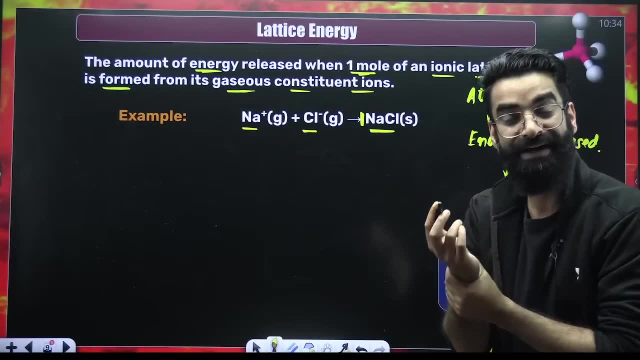 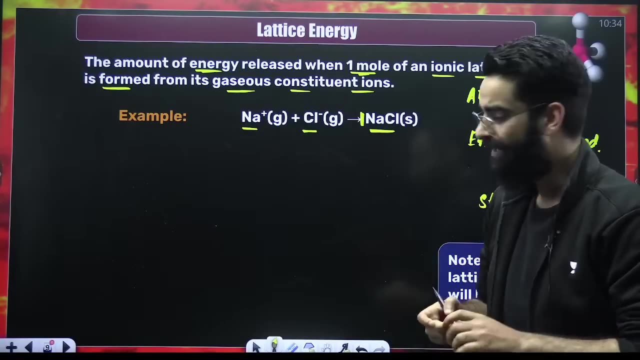 At that point of time, Whatever energy will be released during this particular process, Whatever energy will be released during this particular process, That amount of energy released is something which you will be calling as lattice energy, Number one, Number one. So what is lattice energy? It is the amount of energy which is released. 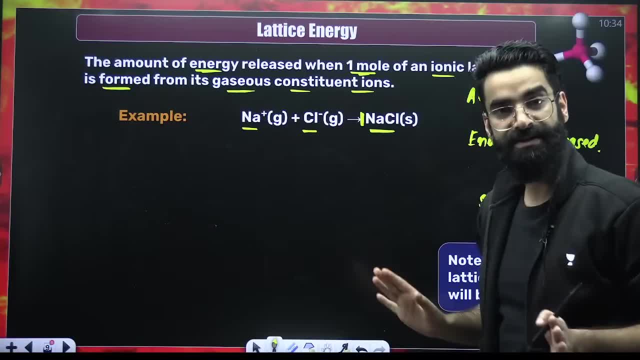 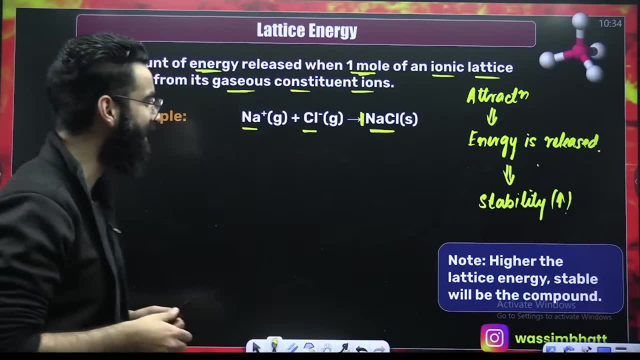 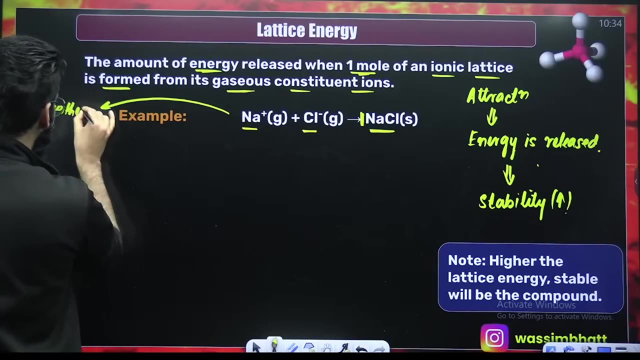 when one mole of ionic compound gets formed from its constituent gaseous ions. Okay, Since energy is being released in this process And that particular process in which energy is being released, That's something which you call as exothermic one. So over here I can say: your process, over here It is exothermic. And if the 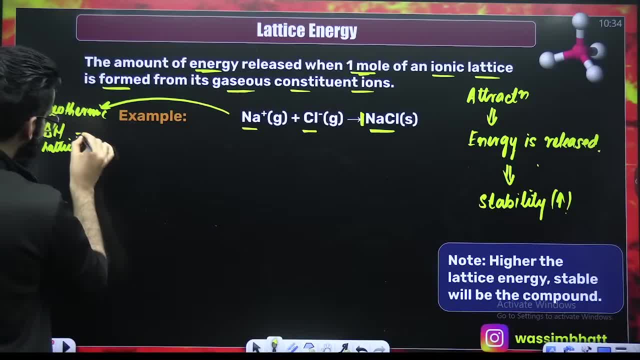 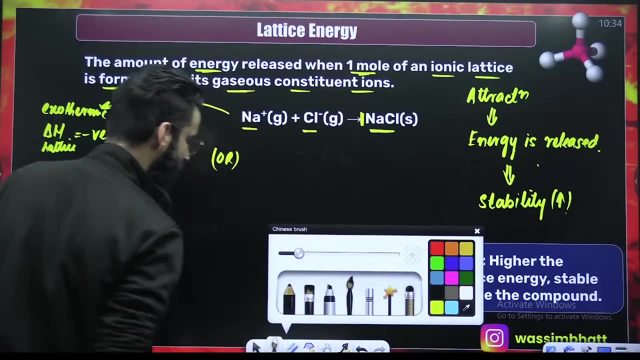 exothermic. I will say delta H lattice here. Delta H lattice here will be negative. This is one way of defining the lattice energy. This is one way of defining the lattice energy. Second way, Second way, Second way of defining the lattice energy, Which I believe is more important: 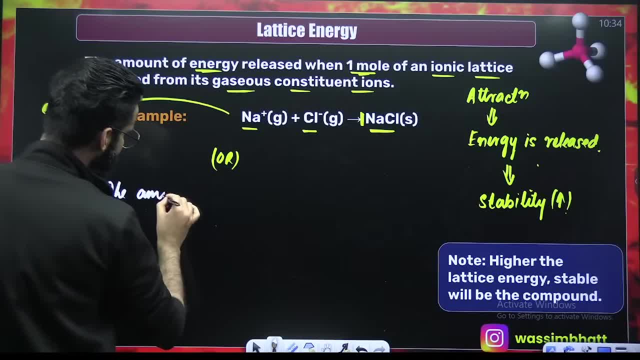 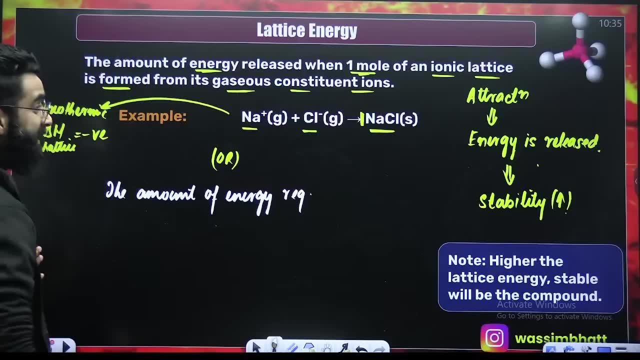 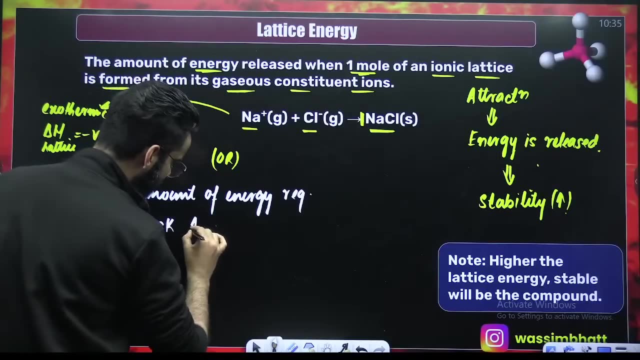 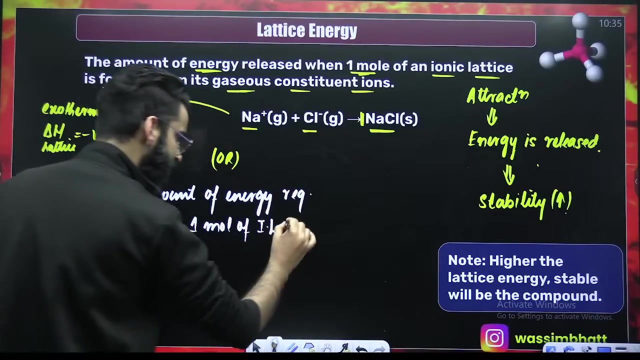 What is that? I will say the amount of energy, The amount of energy which is required, The amount of energy which is required To break, The amount of energy which is required to break one mole of ionic lattice, One mole of ionic lattice, Into, Into its constituent gaseous ions. 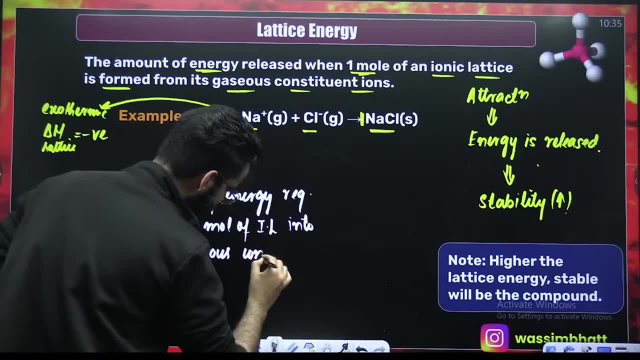 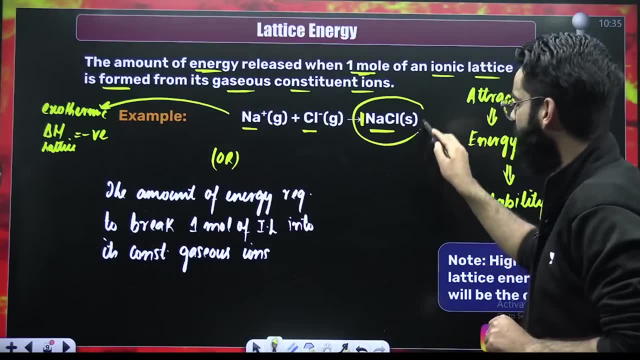 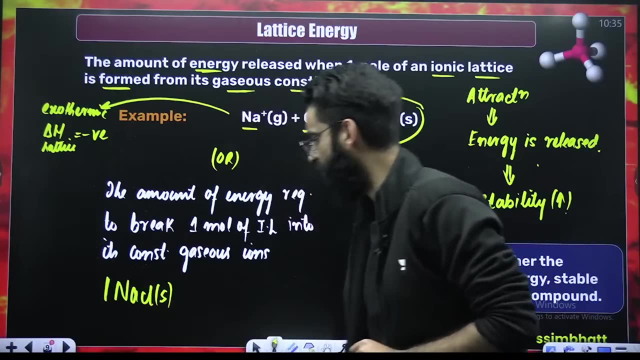 Into its constituent gaseous ions, Into its constituent gaseous ions. What it means. Try to understand. Why do you students? for example, you are taking an acl solid. You are taking an acl solid. In your an acl solid You are taking one mole of an acl solid. 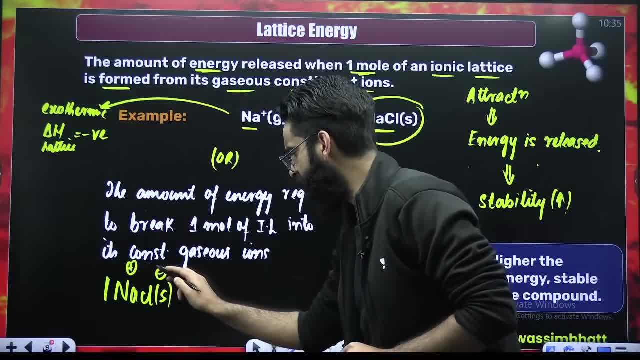 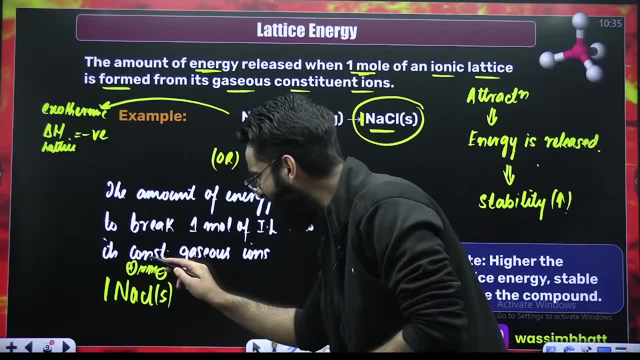 In your an acl solid, You have got Na positives, Cl negatives, And there are attractions, Electrostatic force of attraction. Now, if I ask you, If I ask you In order to break this attraction, In order to break this attraction, In order to break this attraction in such a way, 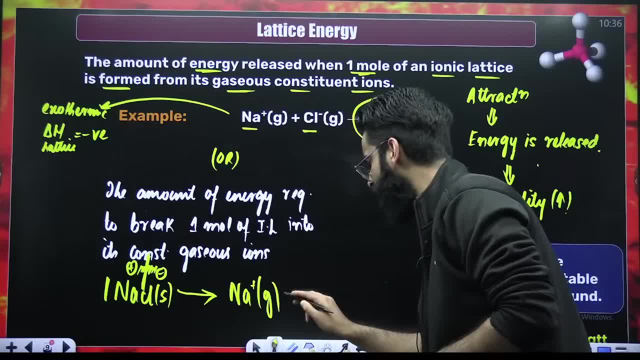 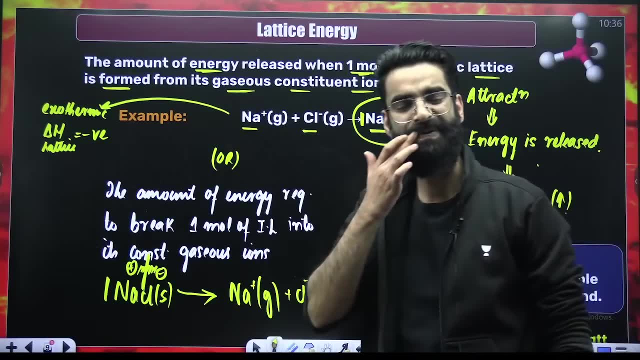 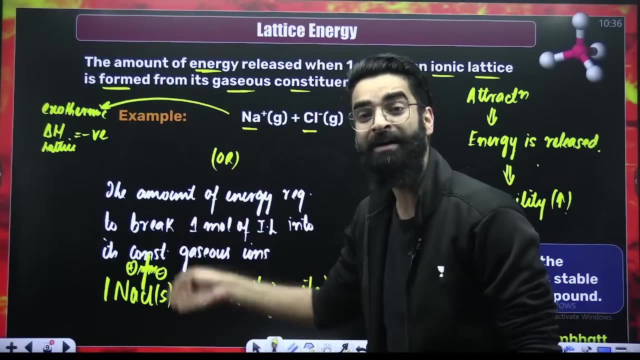 This NaCl gets converted into Na positive gas Plus Cl negative gas. In order to break this attraction, Energy is required. Energy is required And, my dear students, Let me tell you The amount of energy which is required. The amount of energy which is required to break One mole of ionic lattice into its constituent. 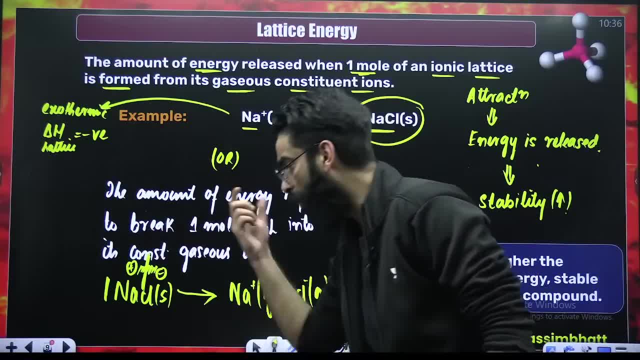 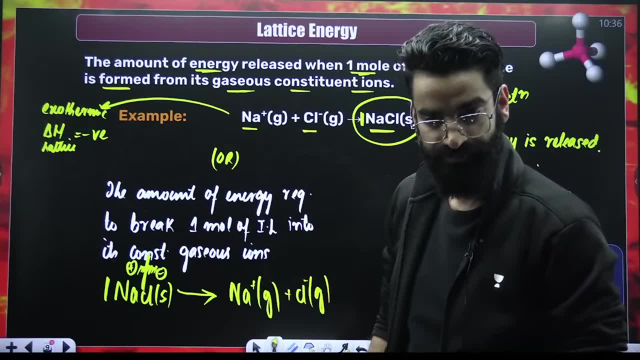 gaseous ions. The amount of energy which is required to break One mole of ionic lattice Into its constituent gaseous ions. That's also what you call as lattice energy. That's also what you call as lattice energy. In this particular case over here Is energy released. 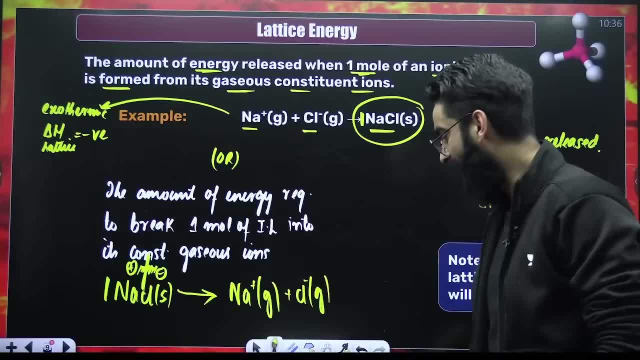 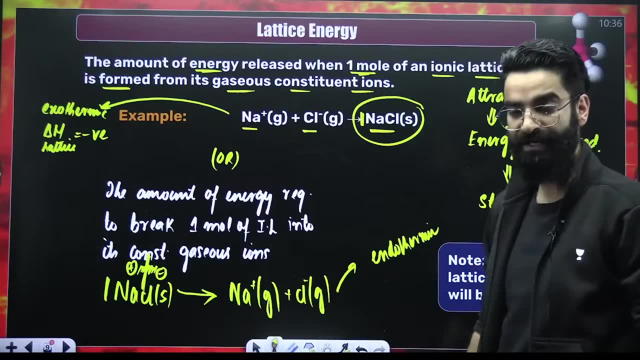 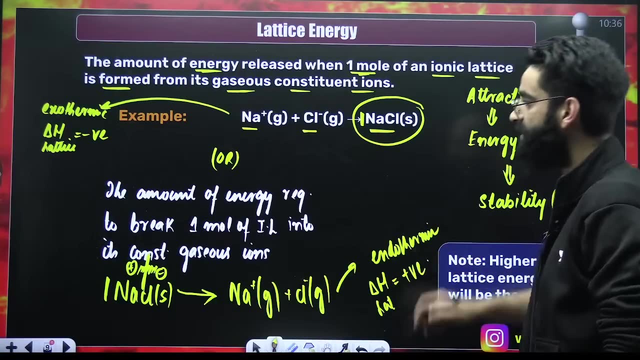 Or energy is absorbed. It said: energy is required, Energy is absorbed, And over here I will be calling this process Endothermic. This will be endothermic here, This will be endothermic in nature, Right, If it is endothermic. So for this process I will say: delta H lattice will show positive sign. 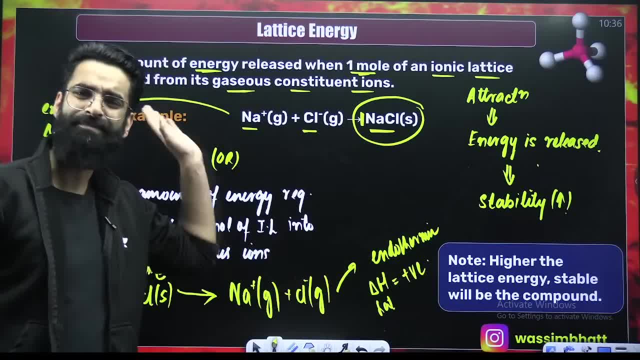 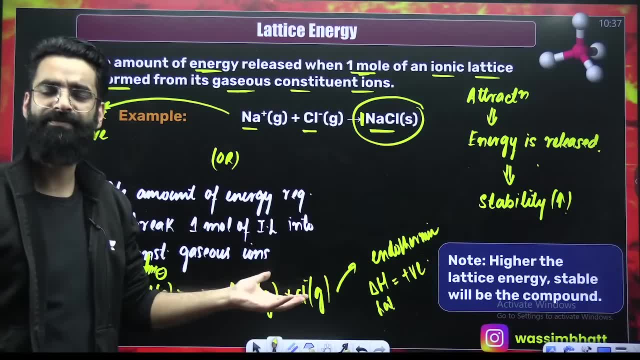 Over here, delta H lattice is negative. Over here, delta H is positive. See, magnitude wise, both will be same. Magnitude wise, both will be same, Perfect. But signs will be different. Signs will be different if you are defining lattice energy in this way. right, the amount of energy released when one 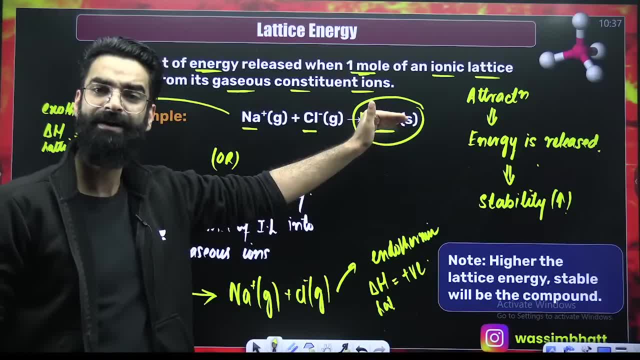 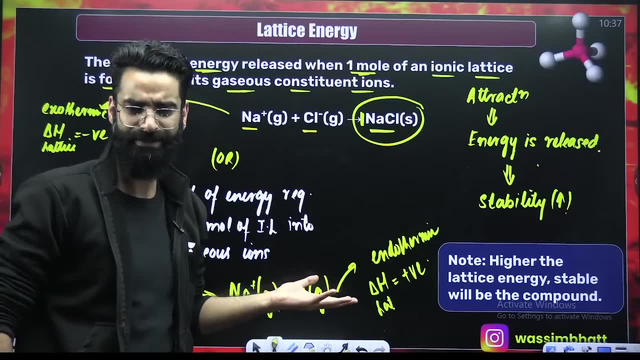 mole of ionic lattice is formed. at that point of time delta is lattice is exosomic, right. delta is negative, right? if you are defining it in this way, then delta should be positive magnitude wise. both are going to be same, perfect. let me know once in the charts. if it is clear, let me know. 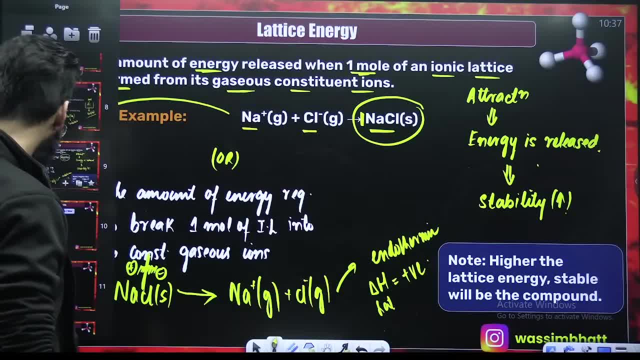 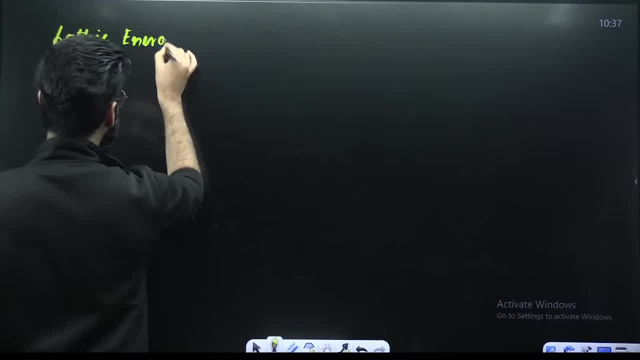 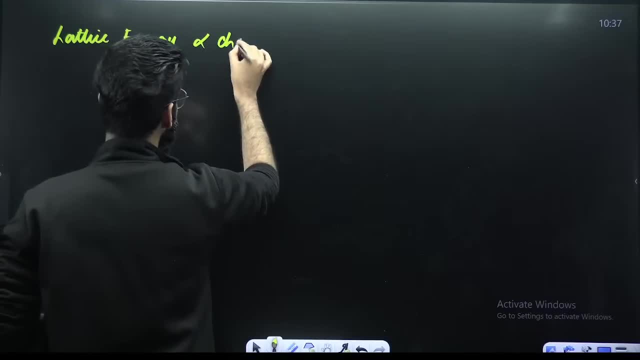 once in the charts if it is clear. let me know once in the charts if it is clear. my dear students, lattice energy, it depends on two factors. lattice energy, it depends on two factors. it is directly proportional to the charge on ions, inversely proportional to the size of ions. 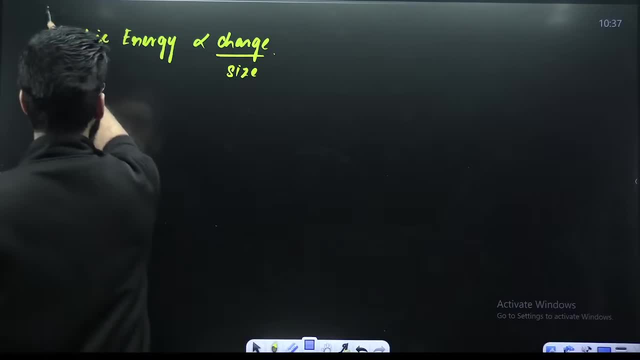 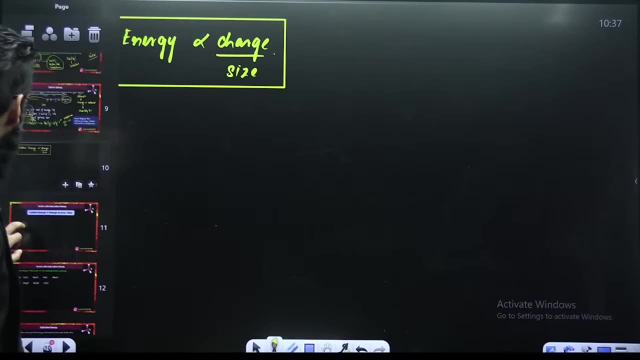 directly proportional to charge inversely proportional to size. directly proportional to charge inversely proportional to size. directly proportional to charge inversely proportional to size. right. directly proportional to charge inversely proportional to size. tell me the answer of this particular question quickly. arrange in the order of increasing lattice energy: 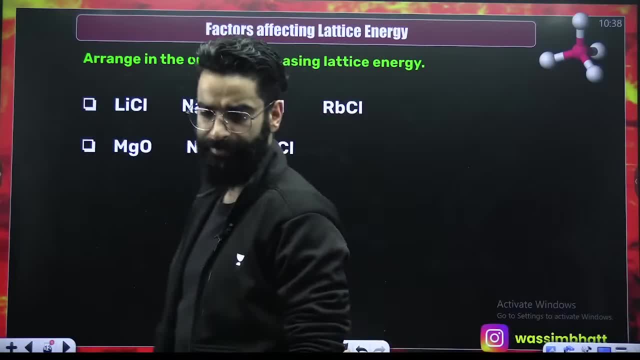 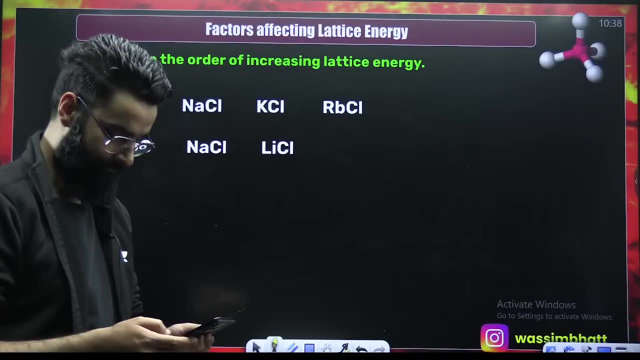 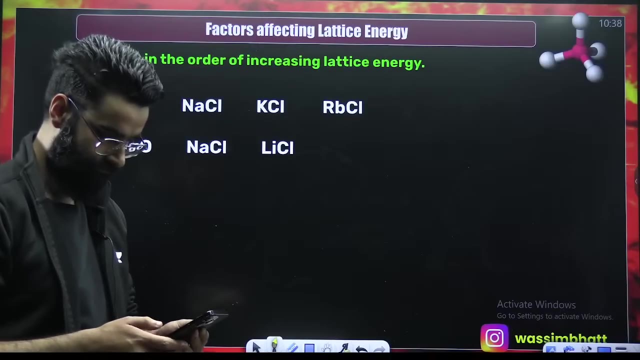 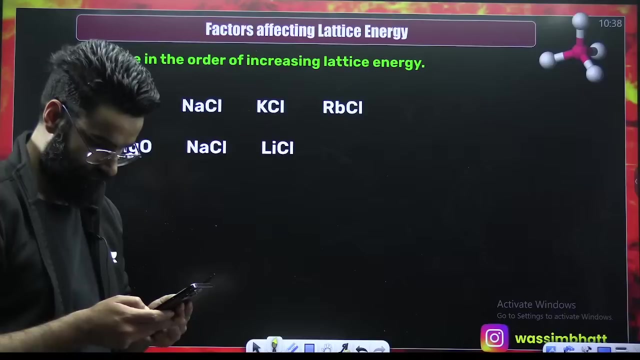 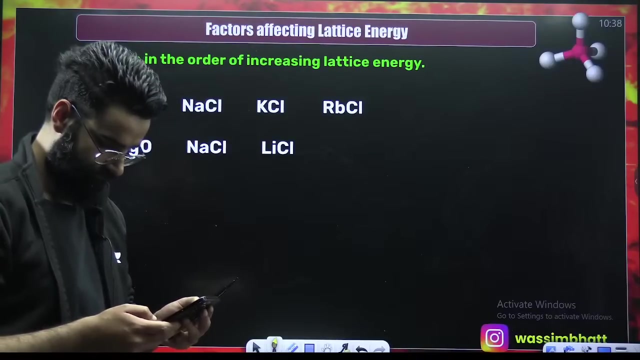 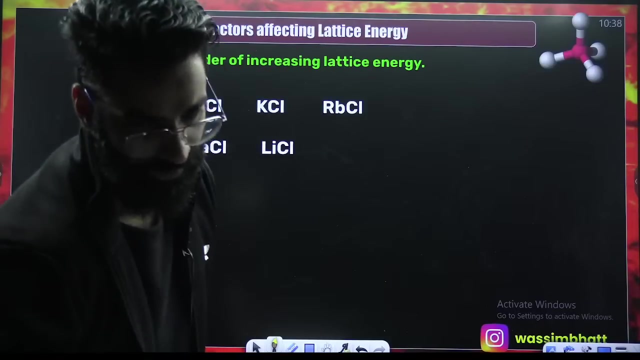 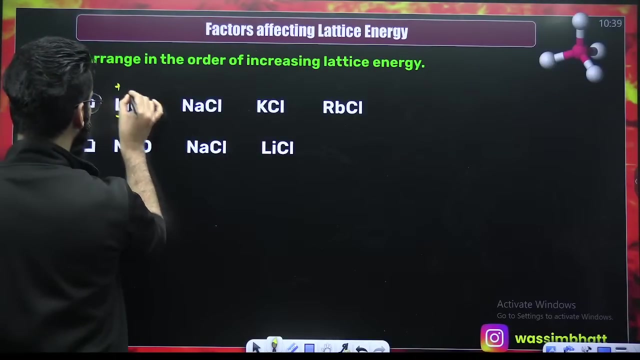 quickly, people, quickly, quickly. i don't want you guys to waste the time. quickly, quickly, quickly, quickly. that see you guys. what's the one la. see you guys, what's the one la. see you guys: NaCl, KCl, RbCl. This is basically La positive Cl negative, Na. positive Cl negative, K positive. 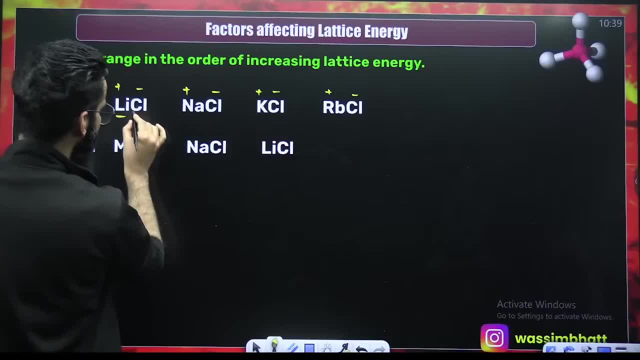 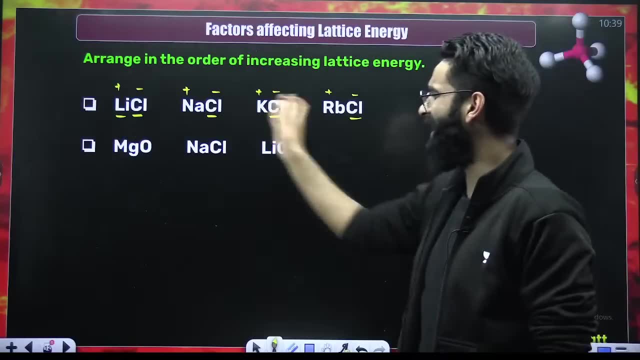 Cl negative, Rb positive, Cl negative. What is same here? Your anion is same everywhere. Your anion is same everywhere. So you are not going to decide on the base of anion, Because anion is same everywhere. Now decide on the base of cation. 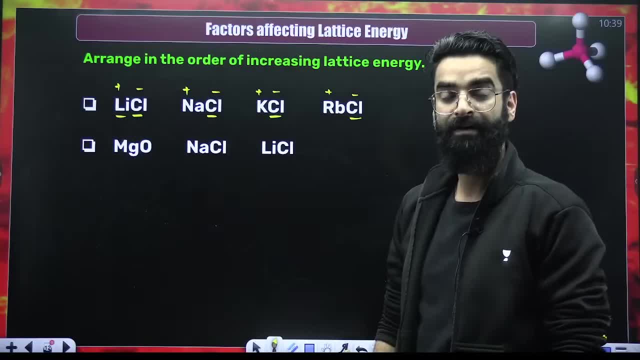 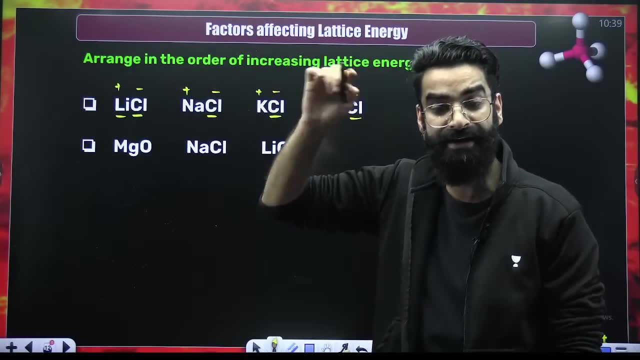 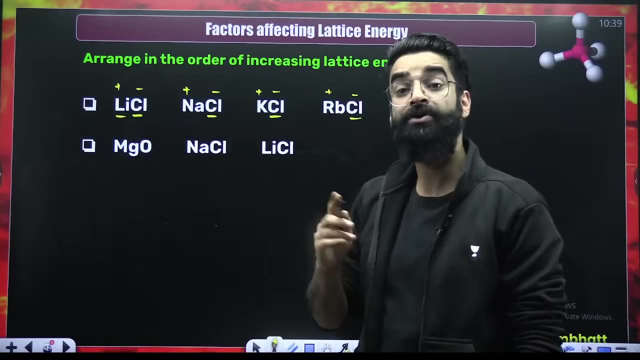 Cation is different here, Cation is different here, But charge on every cation is same. Charge on every cation is same. The magnitude of charge on every cation is same. Are you students? If the magnitude of charge on every cation is same, you are not going to decide. 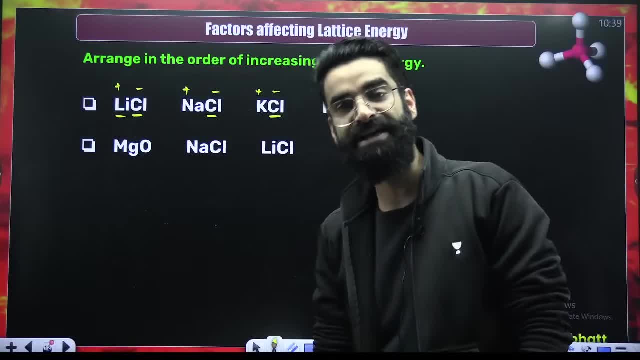 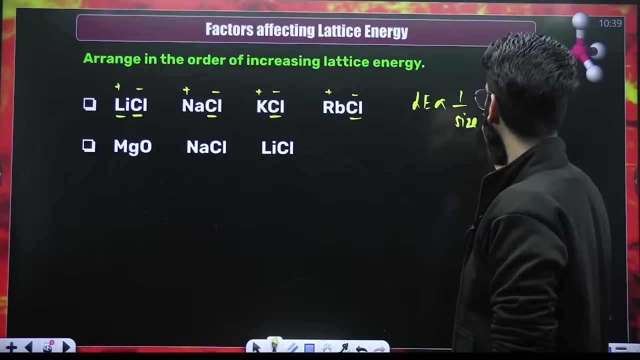 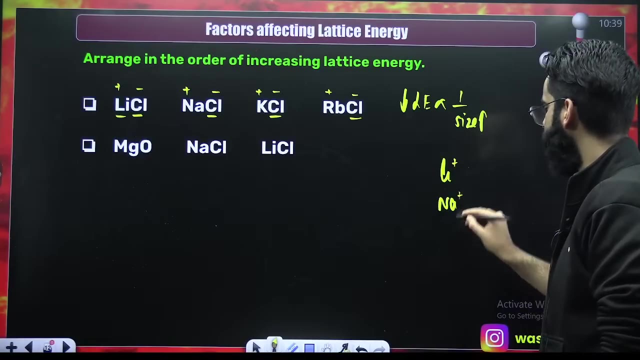 on the base of charge of cation. You will be deciding on the base of size of cation And you know, lattice energy is inversely proportional to the size of ions: More the size, lesser the lattice energy. Now, La positive Na positive, K positive. La positive, Na positive. 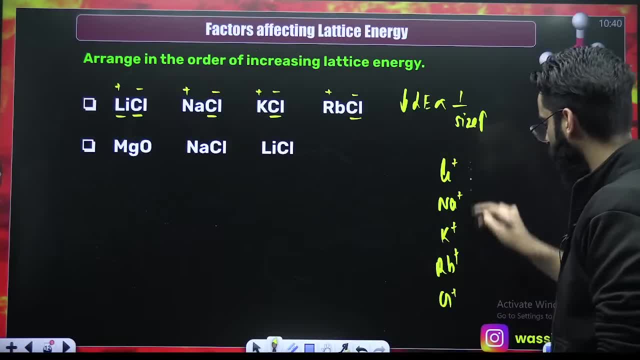 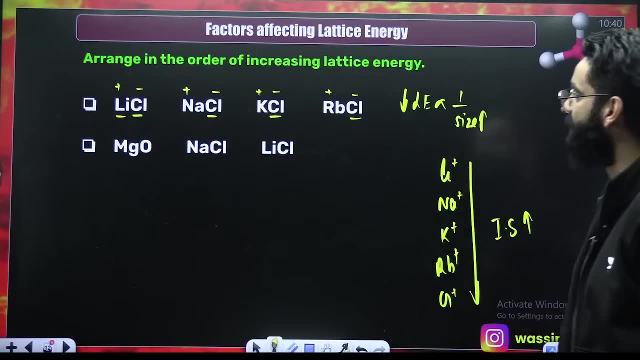 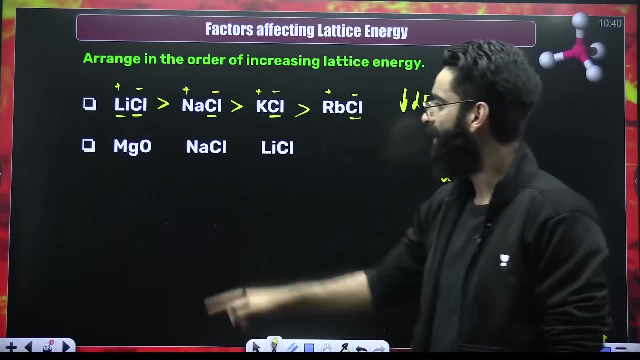 K positive, Rb positive, Cs positive, And, moving from top to the bottom, the ionic size. the ionic size increases. If ionic size increases, size increases, lattice energy decreases. So this is going to be the order of lattice. As simple as that: 1,, 2,, 3, 4.. Correct. 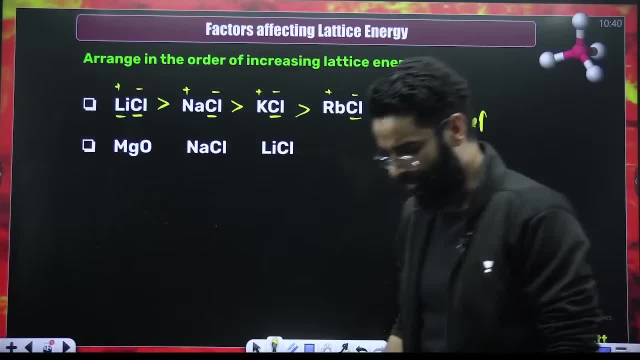 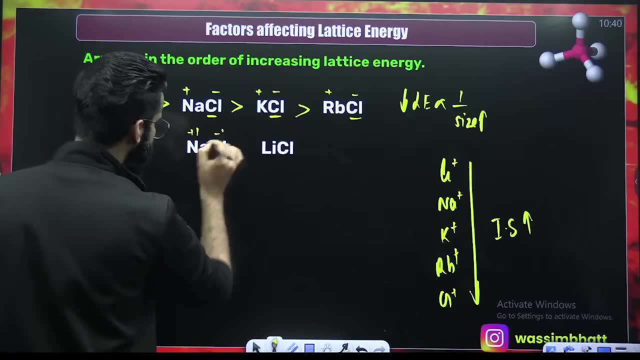 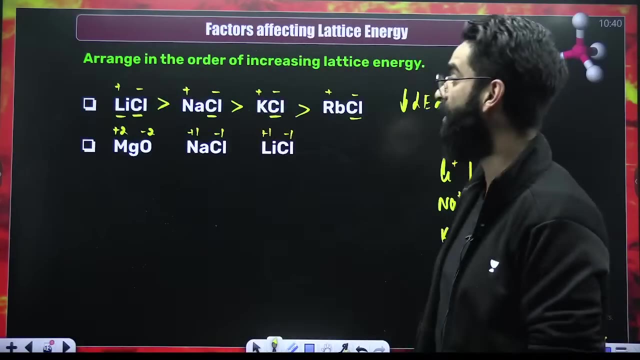 Now people MgO, NaCl, LiCl Over here. if you look carefully, if you look carefully, this is MgDi positive, this is ODi negative, Na positive, Cl negative, Li positive, Cl negative. First of all, first of all, first of all, try to understand, Do remember, Do remember. 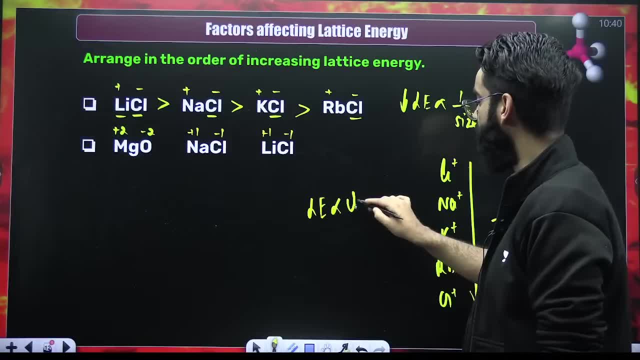 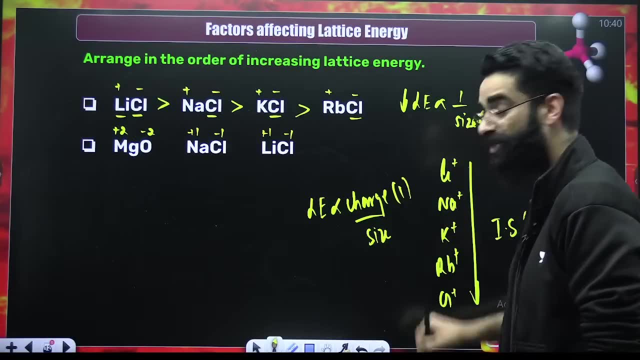 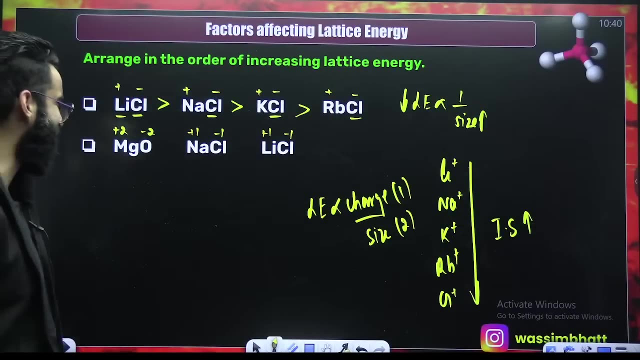 I told you lattice energy. I told you lattice energy, It's strictly proportional to charge, Inversely proportional to size. Remember, always prioritize charge first, then prioritize your size. Always prioritize your charge first, then you'll be prioritizing your size Right. So, people, if you look carefully, where is the charge on the atoms? more Charge is maxed out. 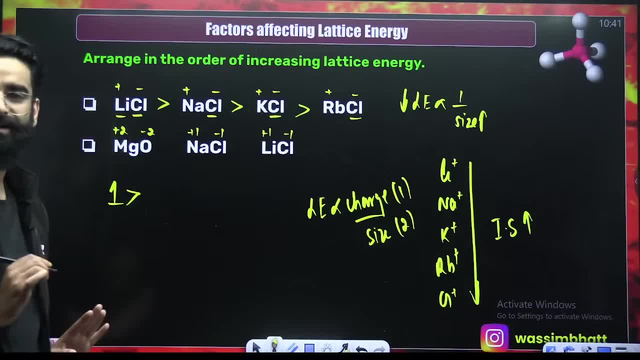 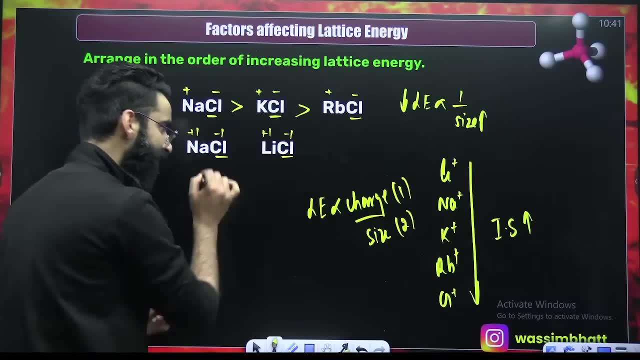 It's maximum here. So first we'll have maximum lattice energy Right Plus 2, minus 2.. Plus 1, minus 1.. Plus 1, minus 1.. So charge over here is more. Now among these two Na is same Cation is. 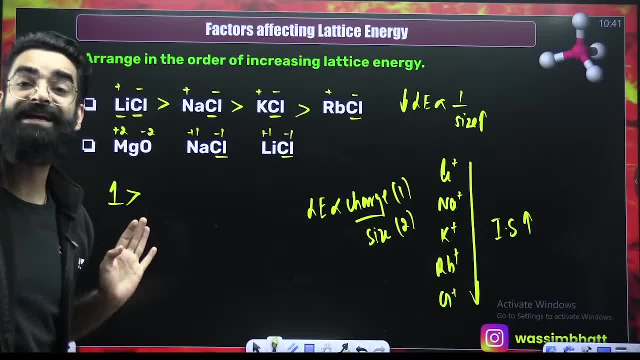 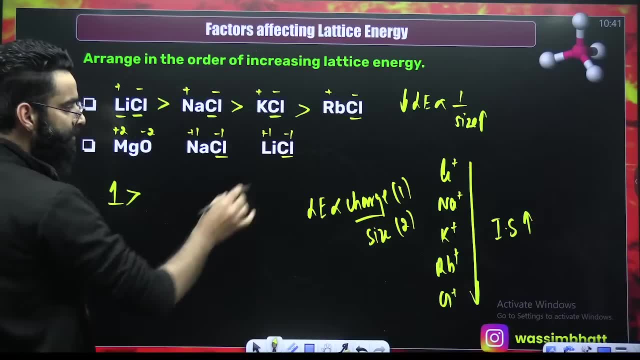 different. Charge on cation is same, But size of cation is different. Right, Lesser the size of lesser the size. lesser the size, more the lattice energy, Right. So Li positive has got lesser size then Na positive. So 3 will have more then 2.. I believe it's clear. If it is clear, say yes in the. 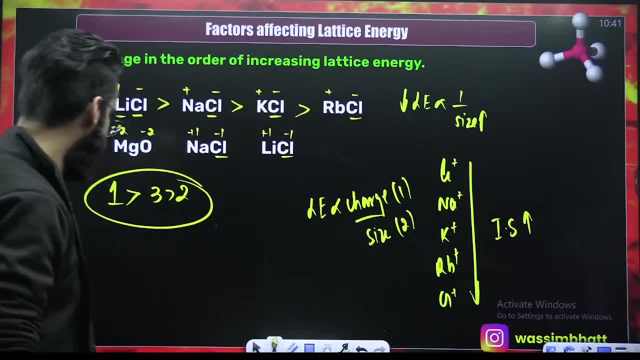 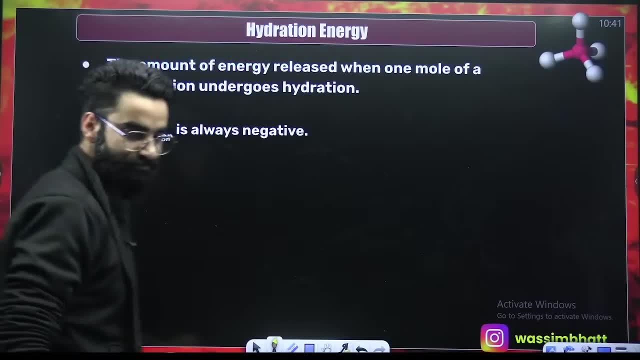 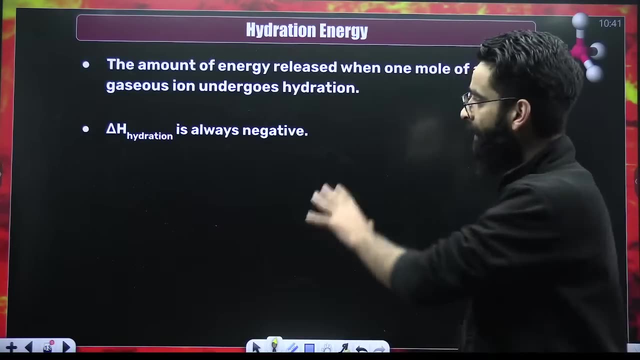 charts quickly. If it is clear, say yes in the charts quickly. So 1,, 3, 2 is going to be the order. Absolutely right, Perfect, Perfect guys. Now what is hydration energy? You would have discussed, you would have studied. 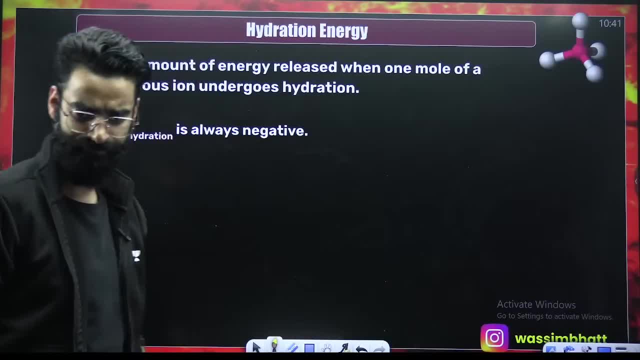 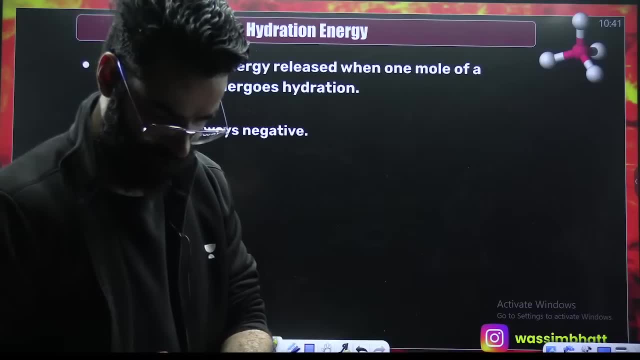 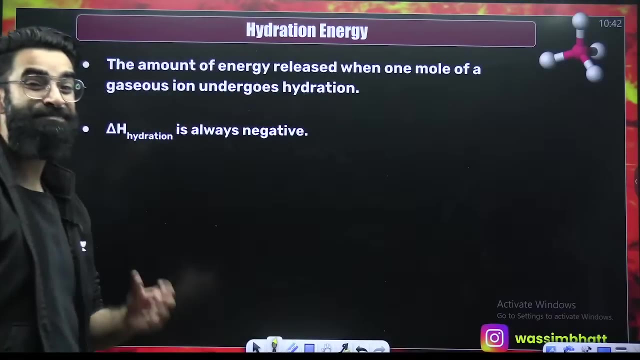 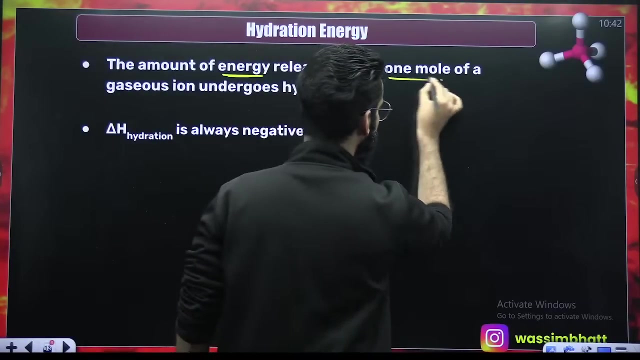 hydration energy as well. Okay, What is hydration energy? What is hydration energy? What is hydration energy? See, guys, as per as per the definition, hydration energy: the amount of energy, the amount of energy which is released, the amount of energy which is released when one 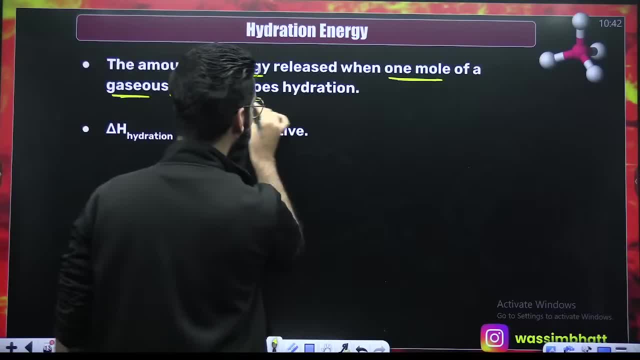 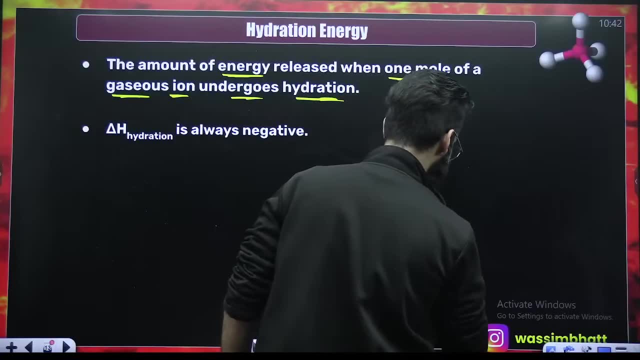 mole of a gaseous ion. when one mole of a gaseous ion undergoes hydration, What is meant by that? What is meant by that? Try to understand, My dear students. this is the container. This is the container. Imagine, in this particular container, I have kept 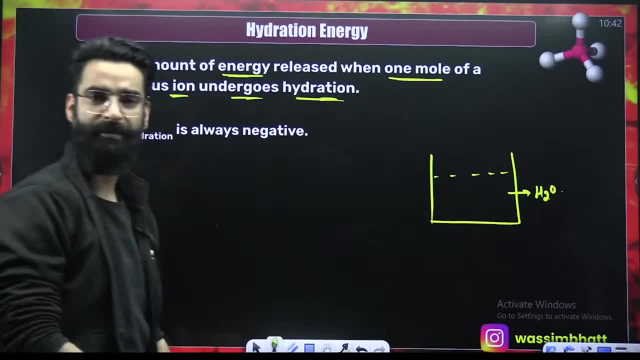 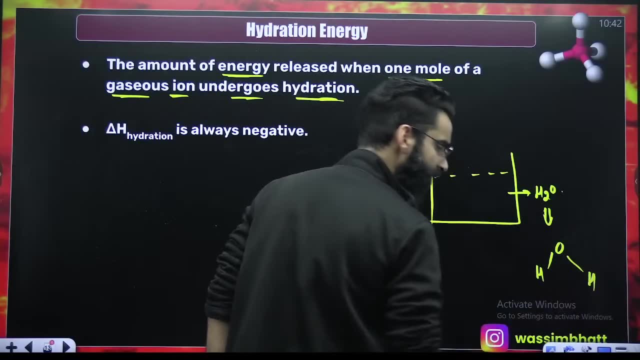 water. Imagine, in this particular container I have kept water, If I have kept water since I believe all of you know about the structure of water. this is the structure of water Among oxygen and hydrogen, which one is more electronegative- Oxygen, So it will carry delta negative. This will 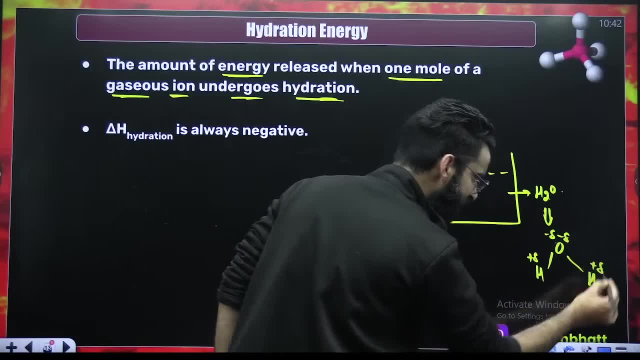 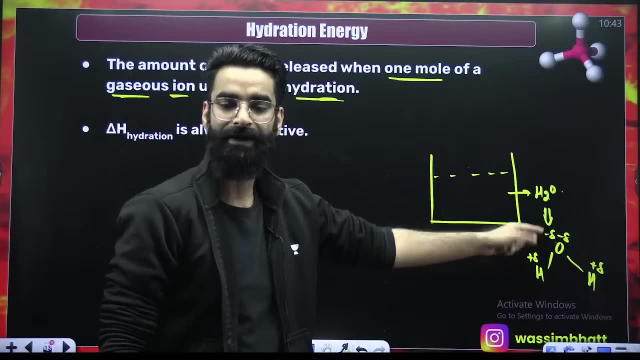 carry delta positive. Similarly, this carries delta negative, This carries delta positive. So can I say: In water, oxygen is your negative end, It is your negative end, Hydrogen is your positive end. In your water molecule there are two ends. 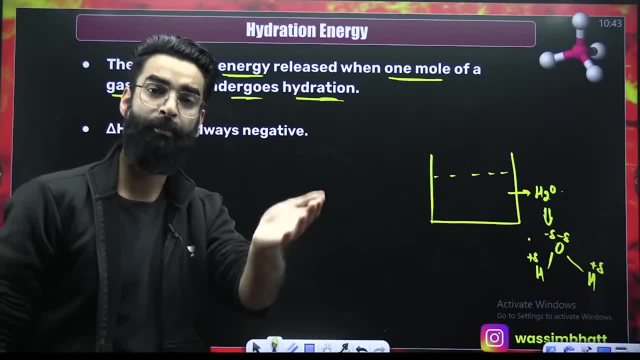 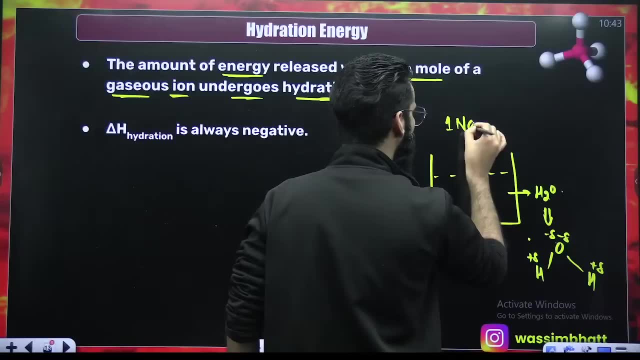 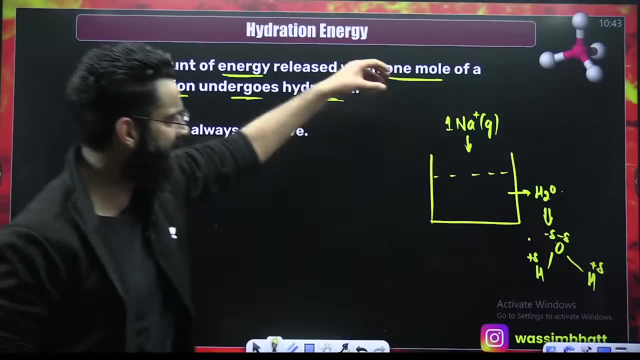 Negative end, positive end. Negative end means oxygen, Positive end means hydrogen. Simple. Now imagine that I am introducing 1 mole of Na positive gas. Imagine that I am introducing 1 mole of Na positive gas here. Imagine I am introducing 1 mole of Na positive gas here. 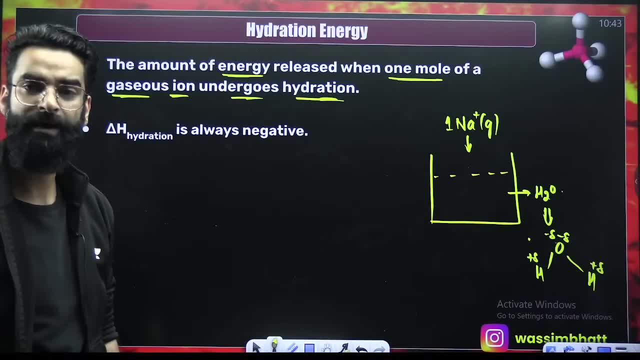 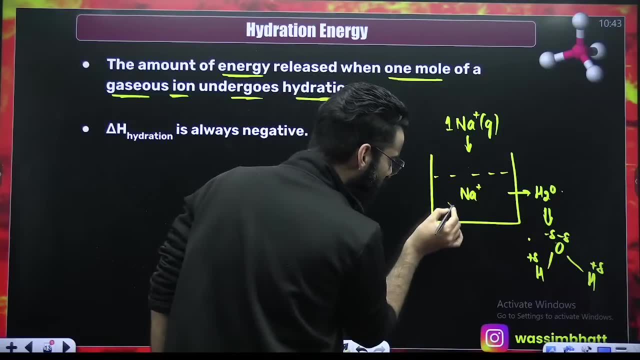 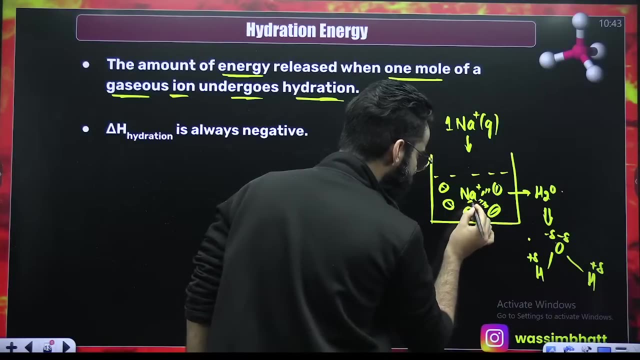 1 mole of Na positive gas here. Imagine that. Okay, What will happen When this 1 mole of Na positive will enter into this water? can we say the negative end of water will show interaction with this positive ion. The negative end of water will show interaction with this positive ion. 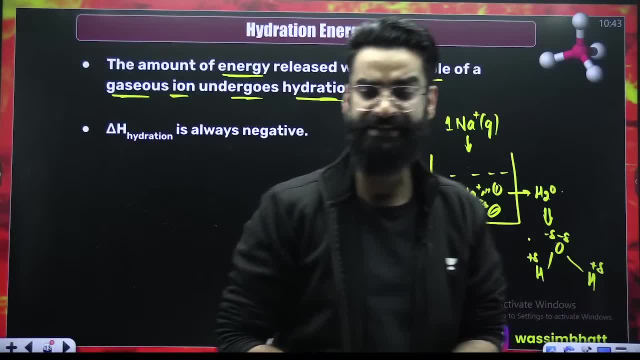 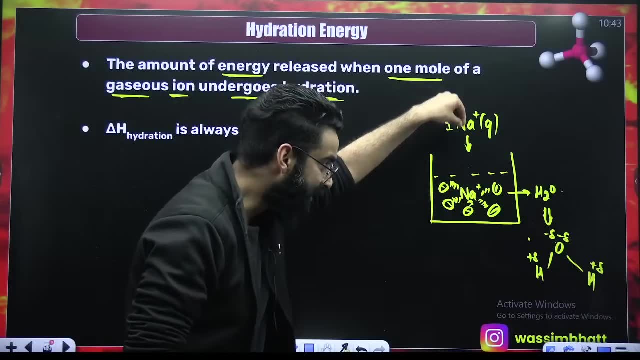 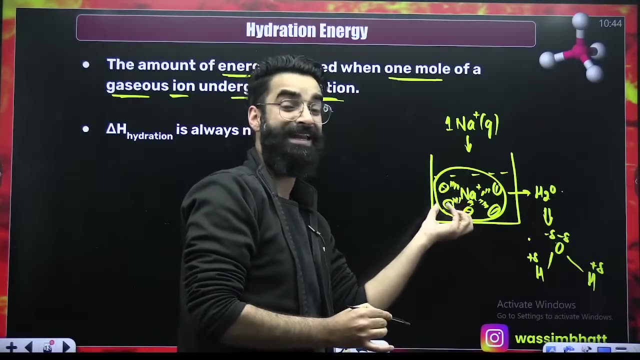 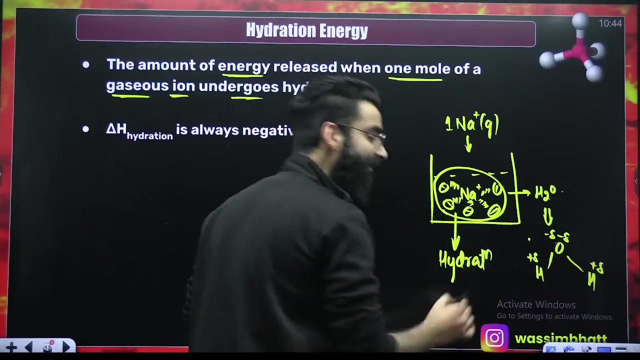 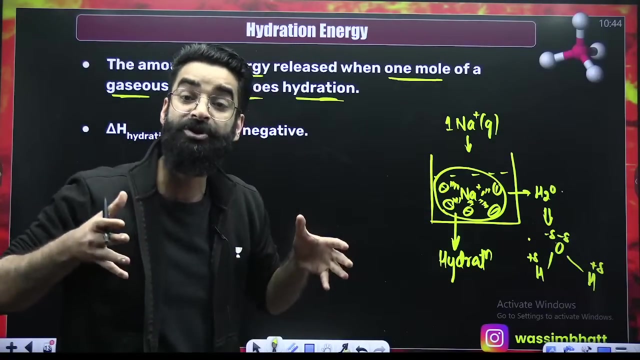 And whenever there are attractions, energy is released. Whenever there are attractions, energy is released, Right, So can I say, during this particular process, first of all, when you're putting a gaseous ion here in water, in water, water molecules are getting associated with this gaseous ion. Water molecules are getting associated with this gaseous ion And this process overall is what you call as hydration. This is what you call as hydration, Right, Your water molecules, they're getting associated with this Na positive, Right, The process is called as hydration. During hydration, during hydration, what happens? Attractions are there, Energy will be released. 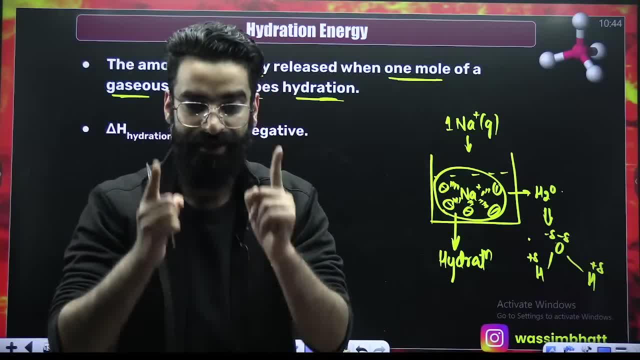 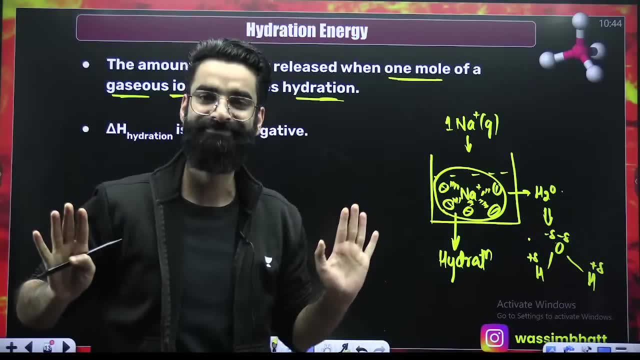 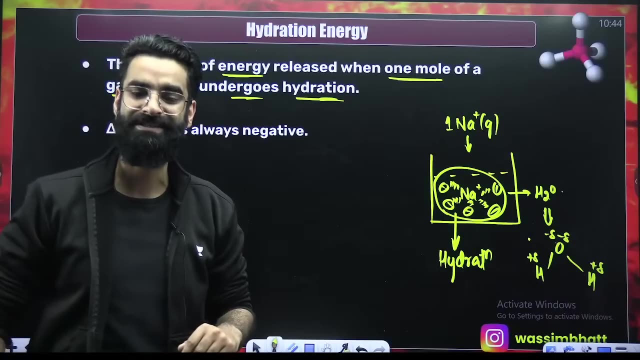 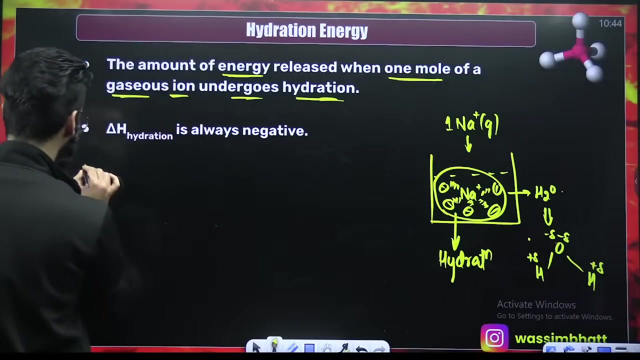 And that amount of energy which is released, that amount of energy which is released when one mole of a gaseous ion undergoes hydration. Okay, Clear, Clear people. Now, since energy is released during this process, since energy is released during this process, that particular process in which energy is released, you call that particular process exothermic. 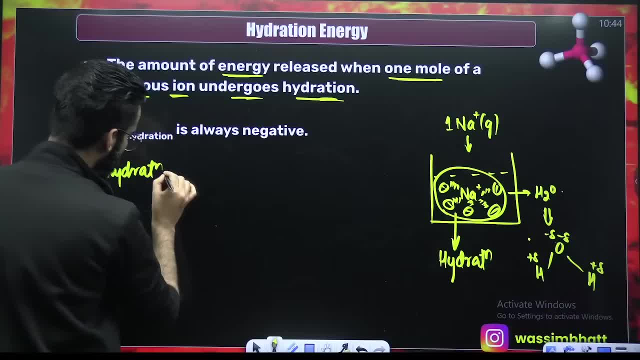 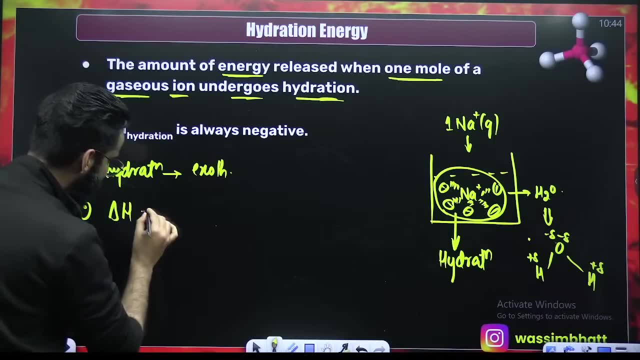 So hydration is exothermic in nature, Hydration process is exothermic, Hydration process is exothermic And if it is exothermic, so delta H value will be negative. Delta H hydration will be negative, As Prasannakar mentioned. you know it. 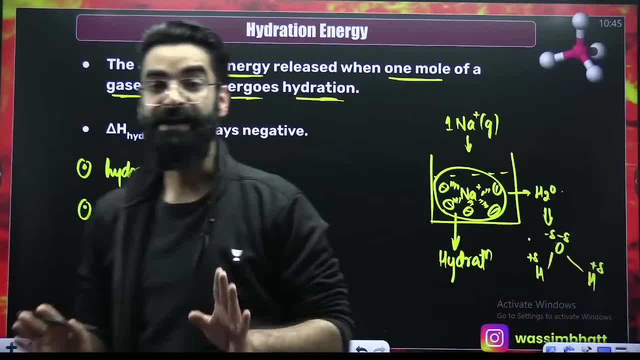 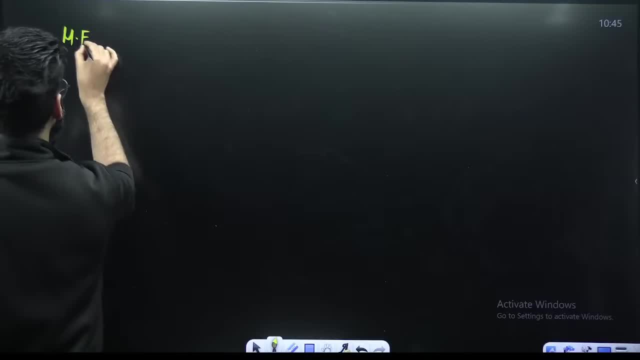 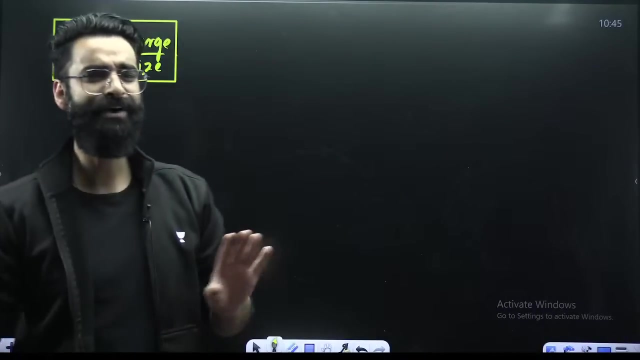 Perfect, Perfect people. I believe it's clear. I believe it's clear Right Now. hydration energy: it is also directly proportional to charge And it is also inversely proportional to size of the ions. Right? Just two things you have to remember. Don't go into details why, etc. etc. Right, We don't have time for that. Remember: hydration energy: that's directly proportional to charge, Inversely proportional to size. 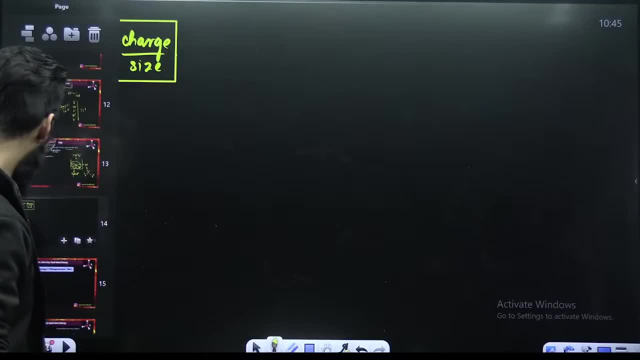 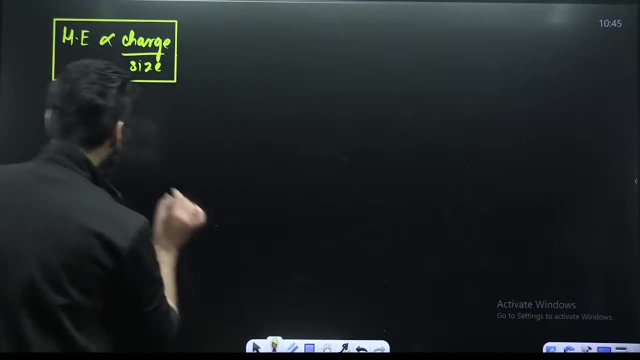 As simple as that. As simple as that. Try to understand what exactly I'm going to say. Try to understand what exactly I'm going to say, My dear students, try to understand. Okay, Let's say I'm writing Li positive, Na positive. 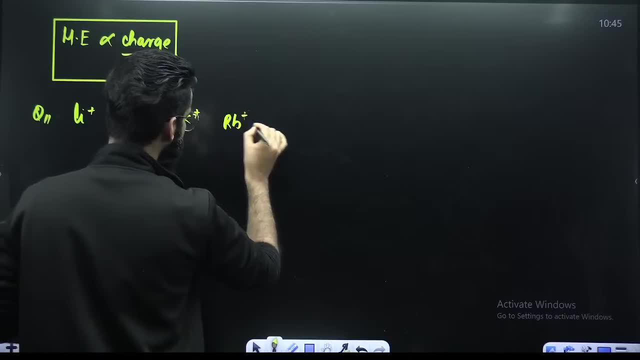 My dear students, try to understand what exactly I'm going to say. Try to understand what exactly I'm going to say. Try to understand what exactly I'm going to say. My dear students, try to understand what exactly I'm going to say. Try to understand what exactly I'm going to say. 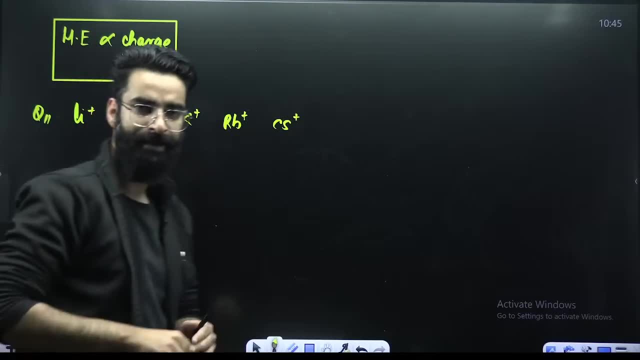 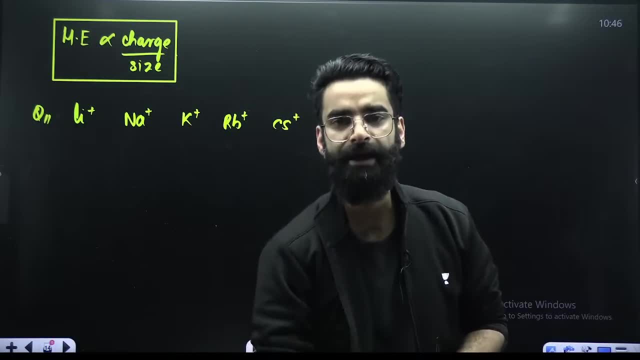 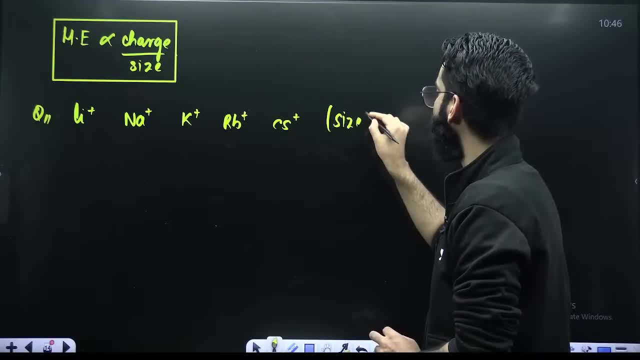 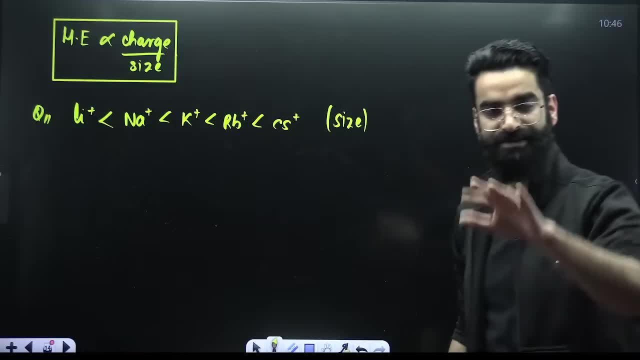 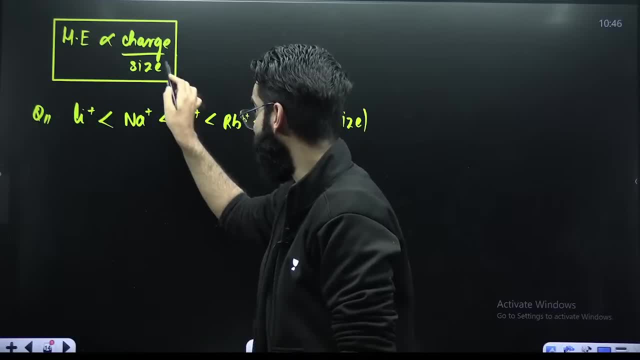 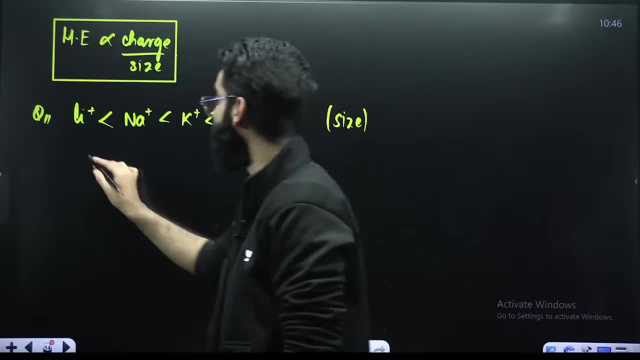 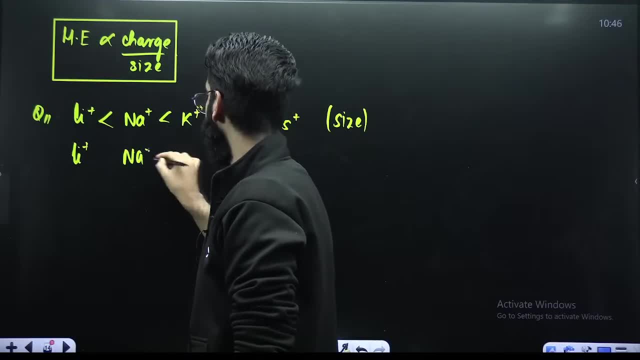 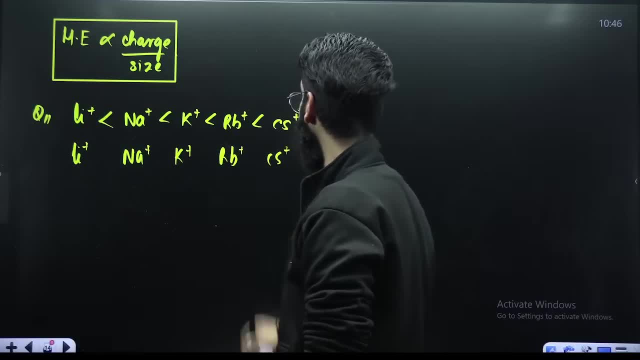 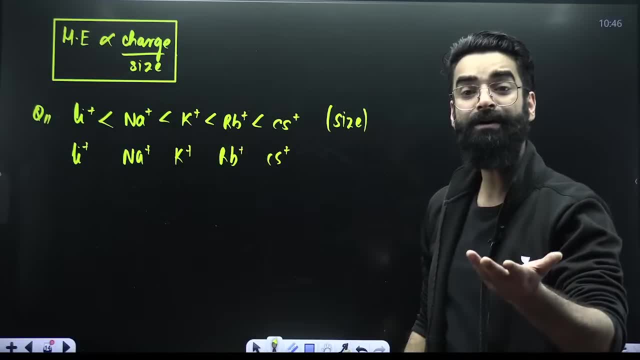 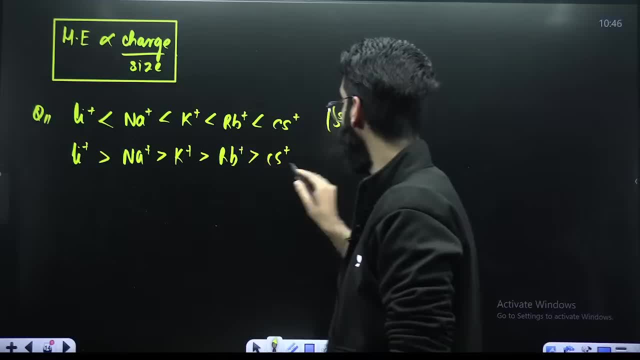 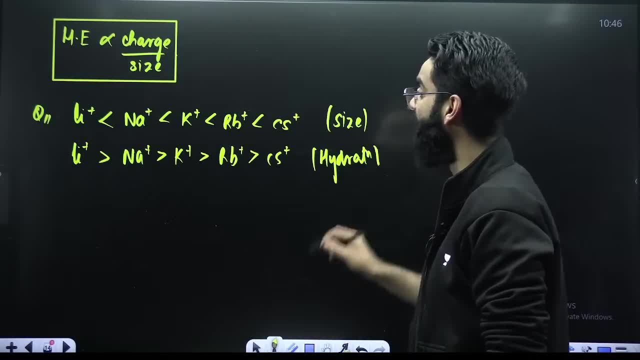 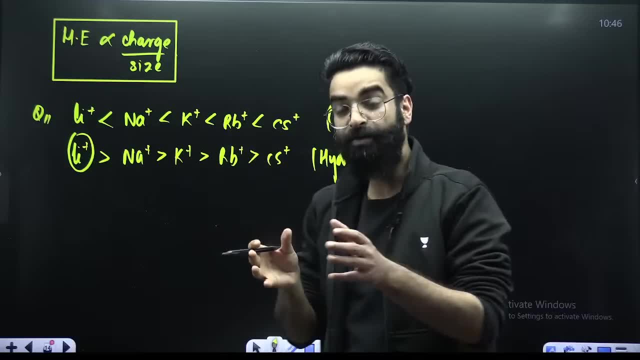 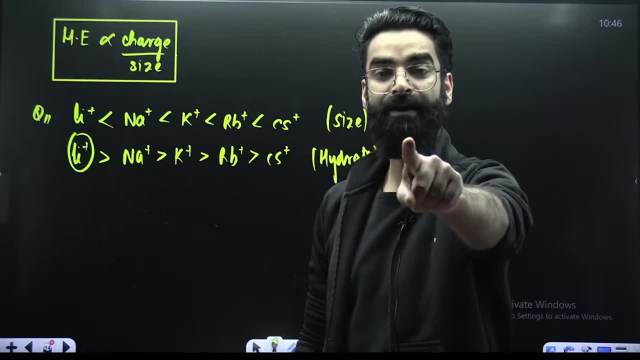 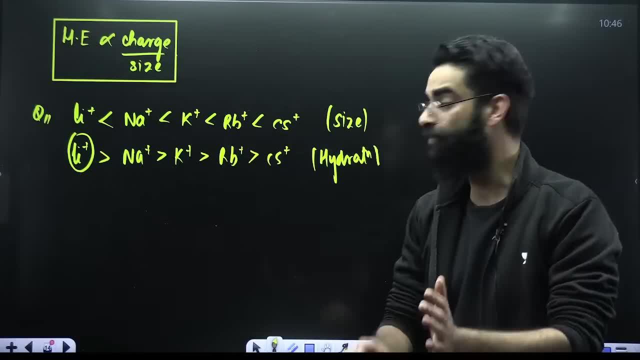 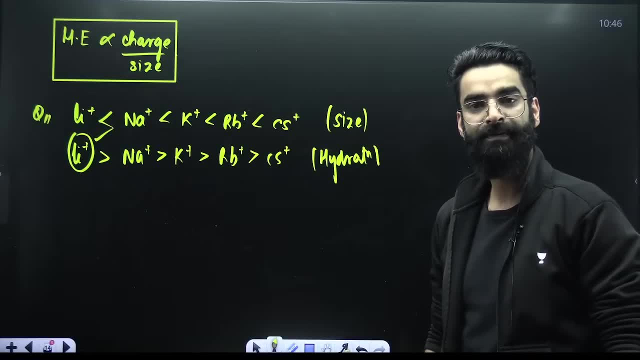 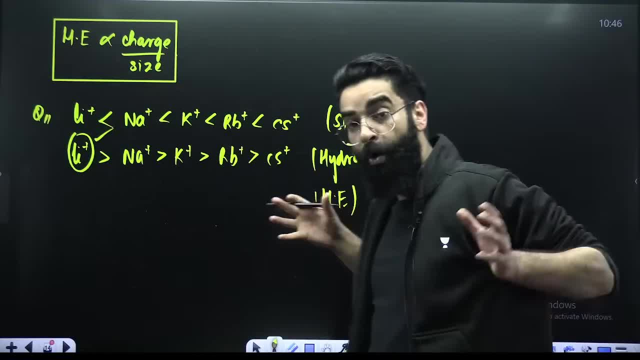 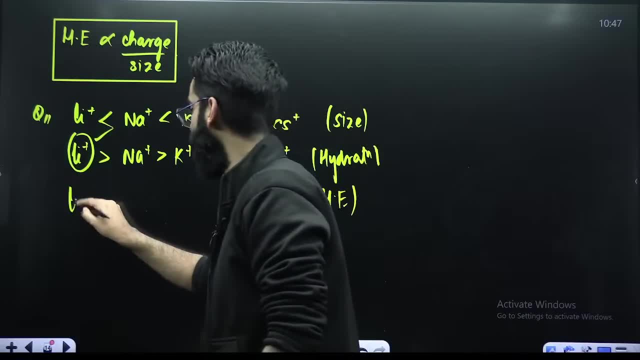 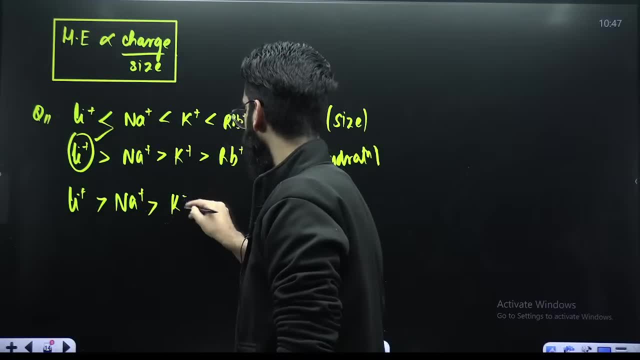 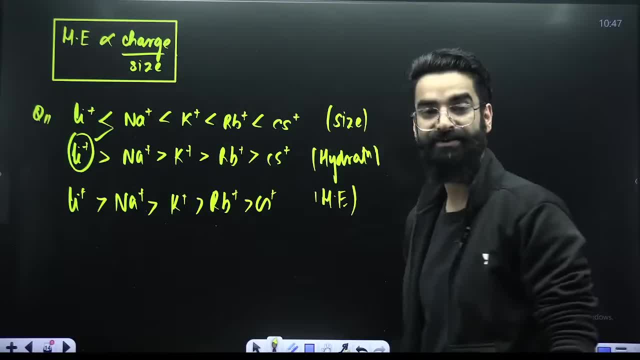 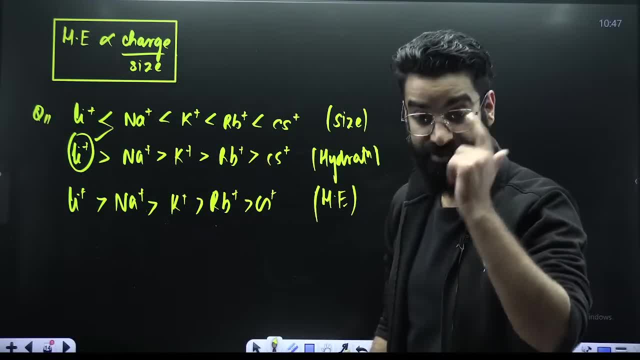 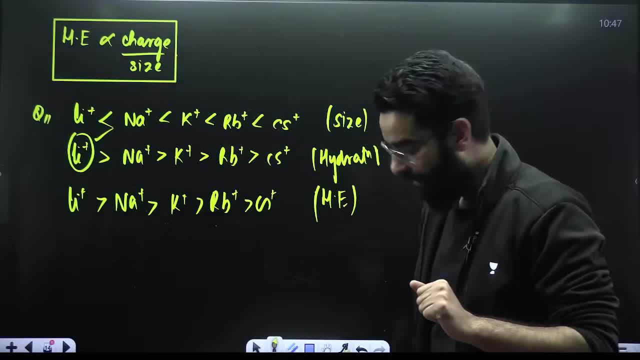 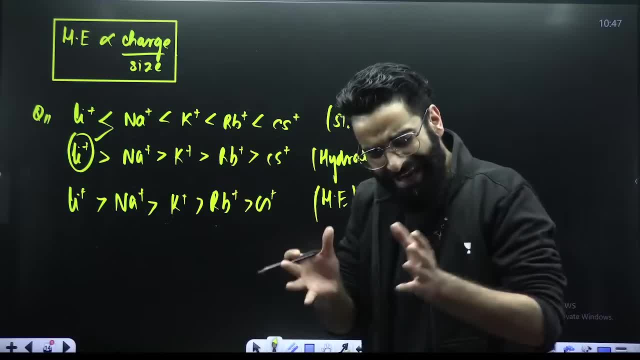 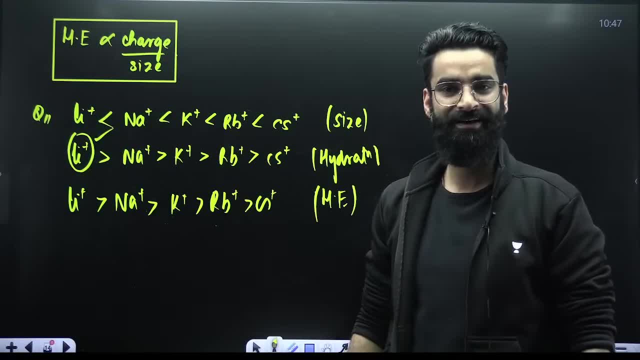 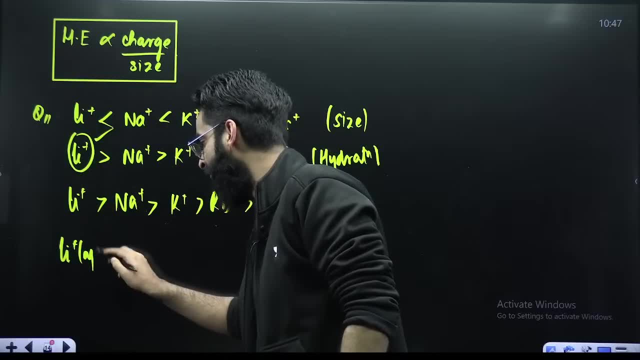 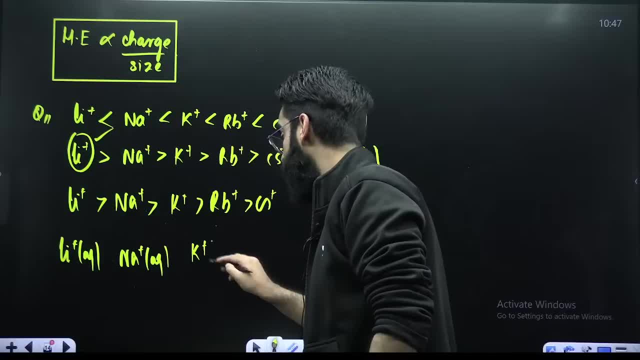 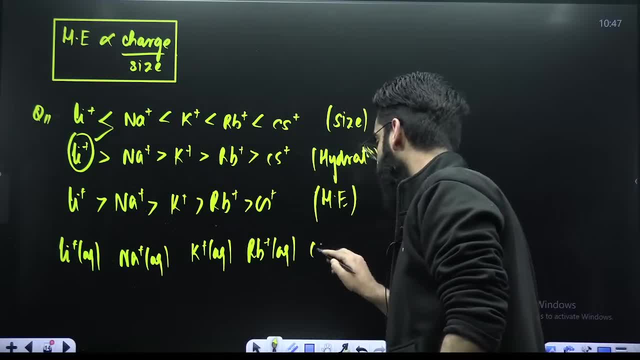 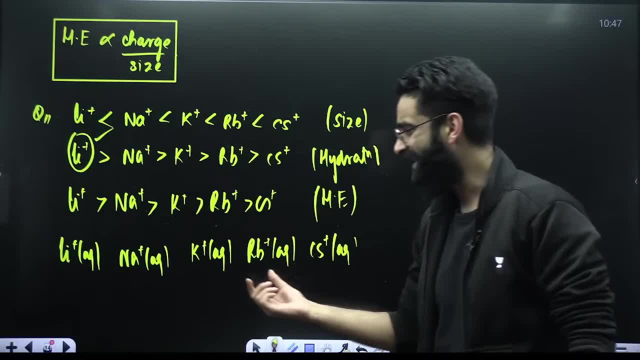 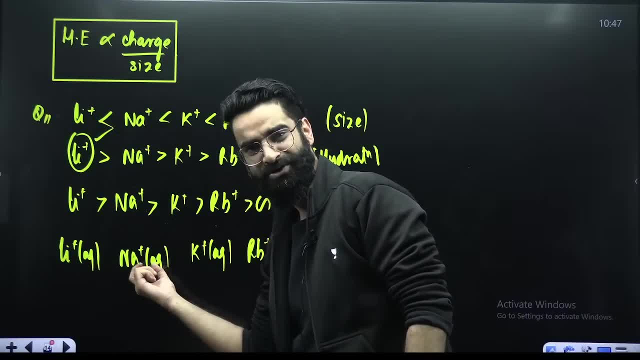 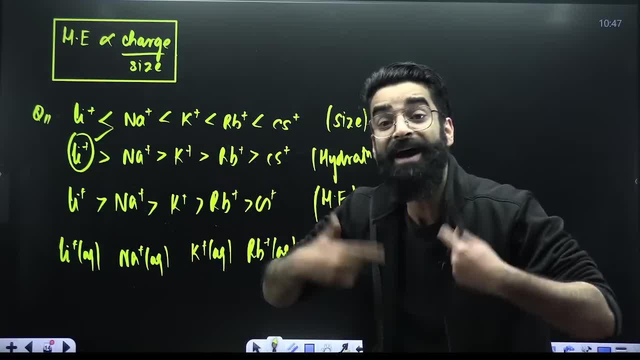 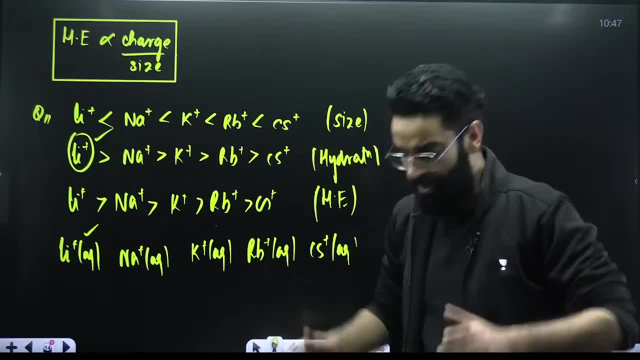 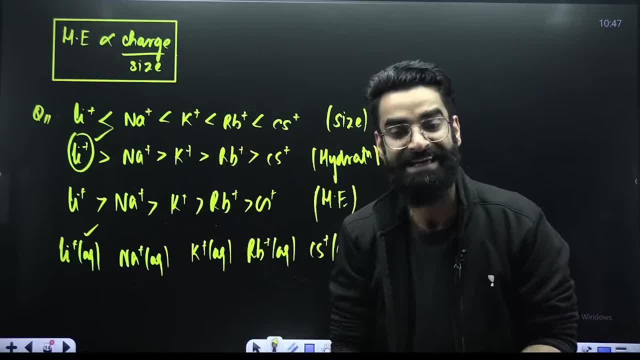 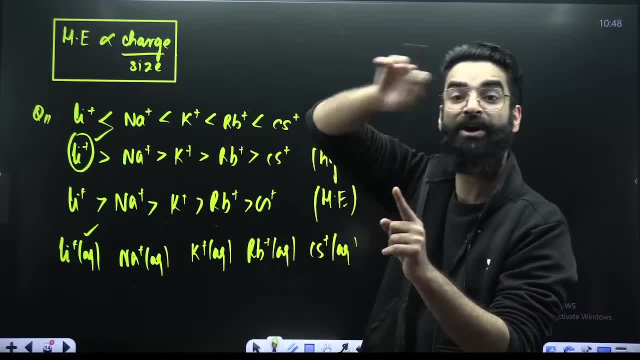 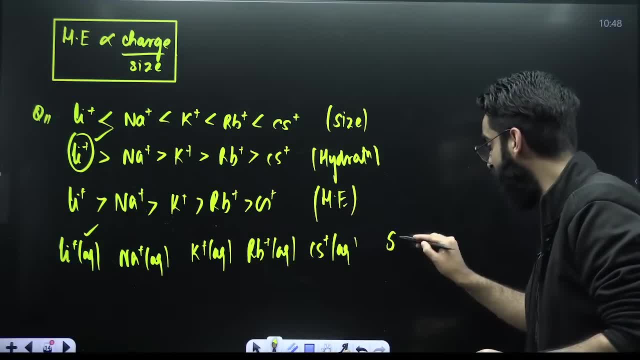 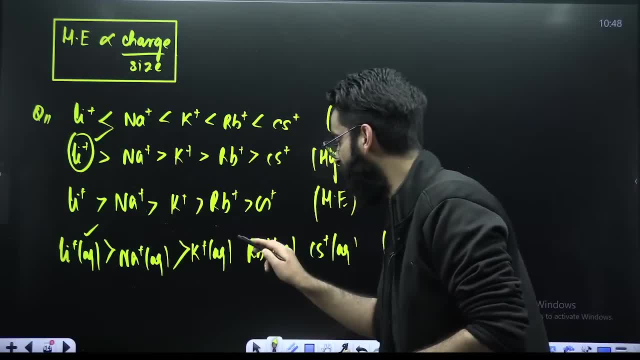 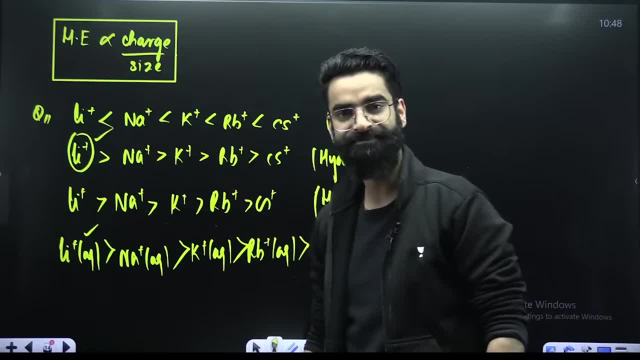 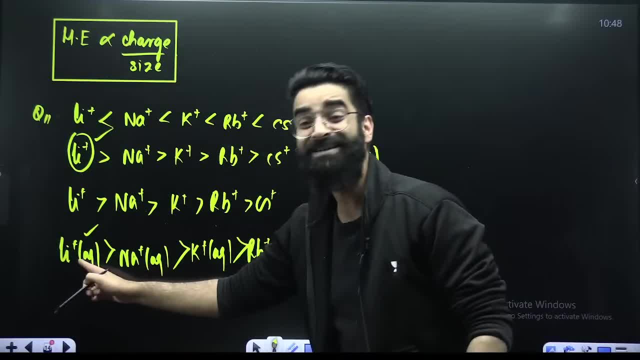 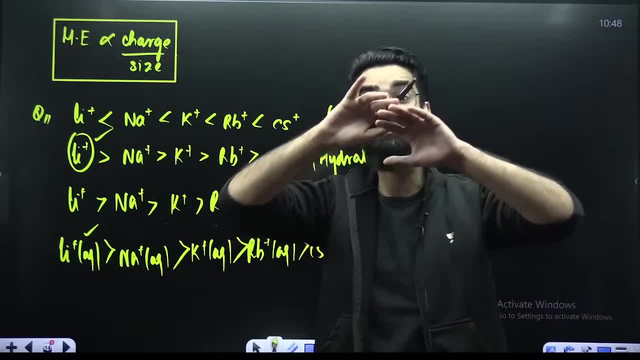 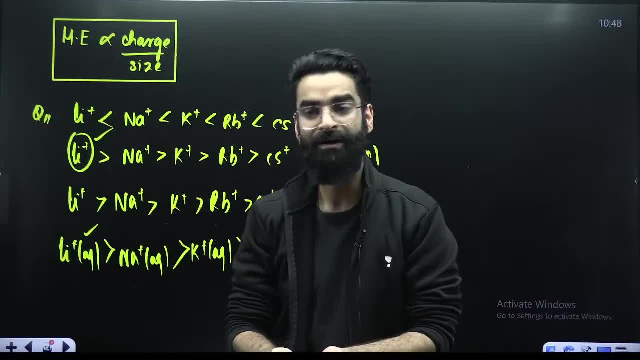 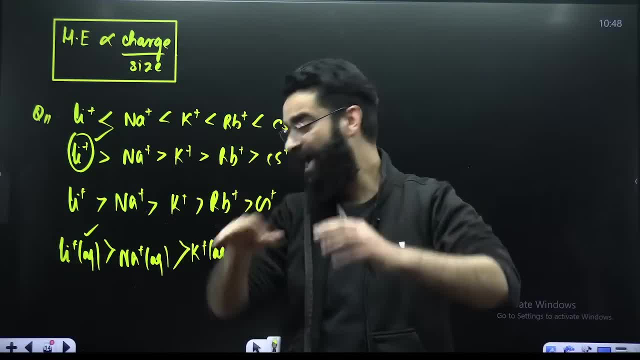 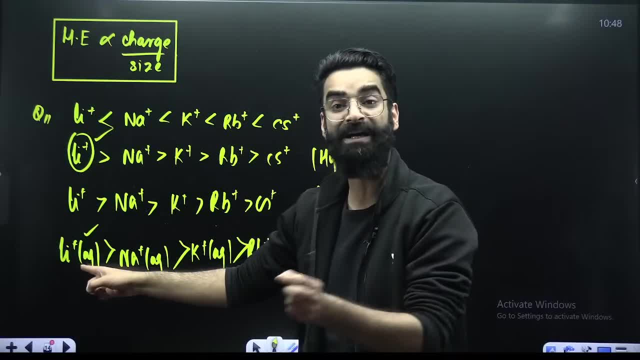 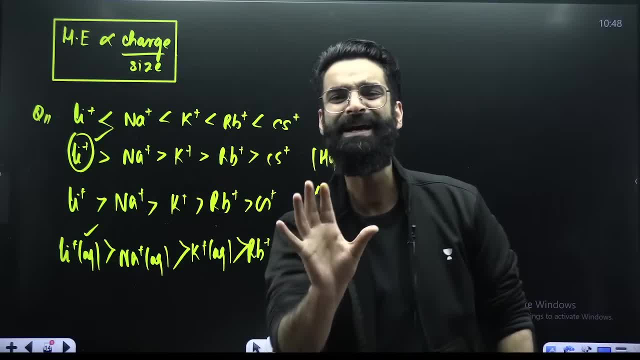 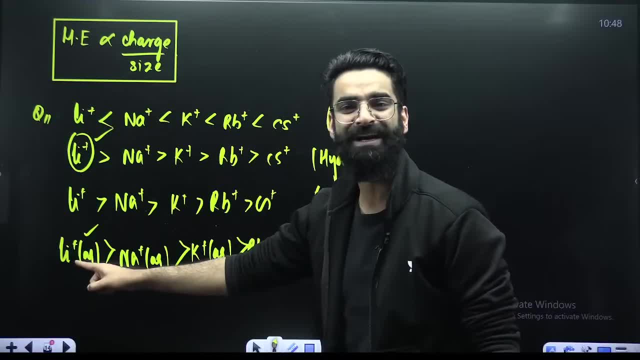 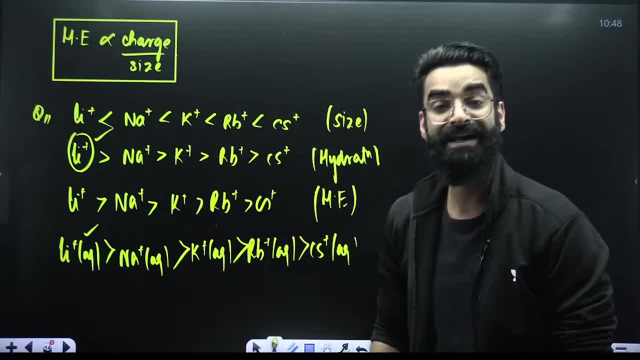 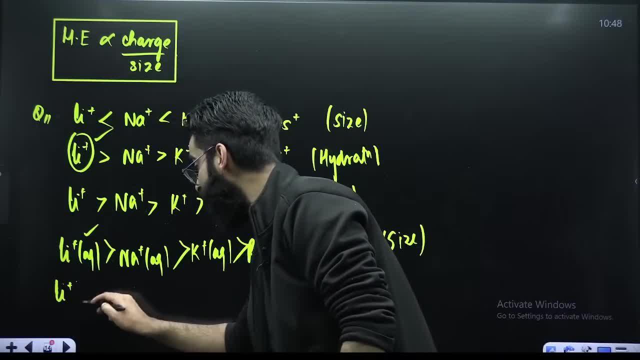 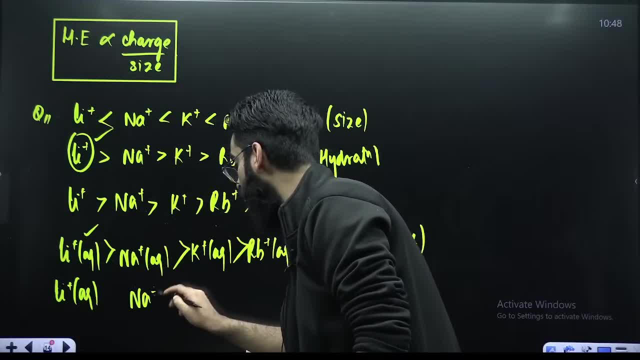 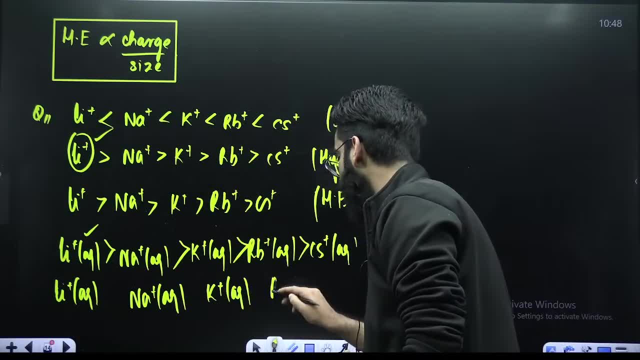 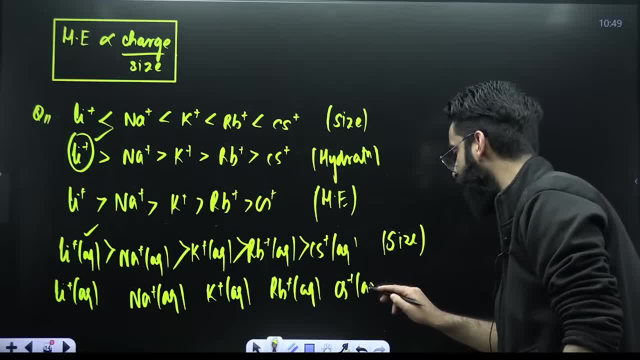 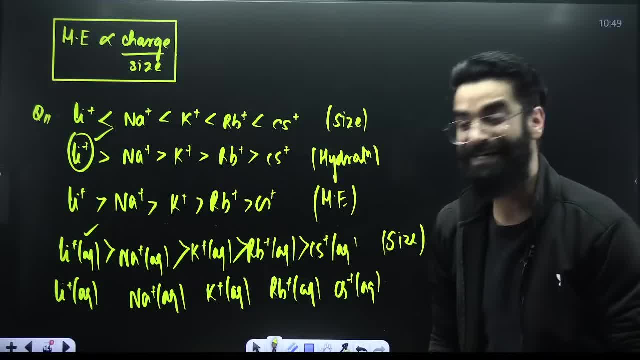 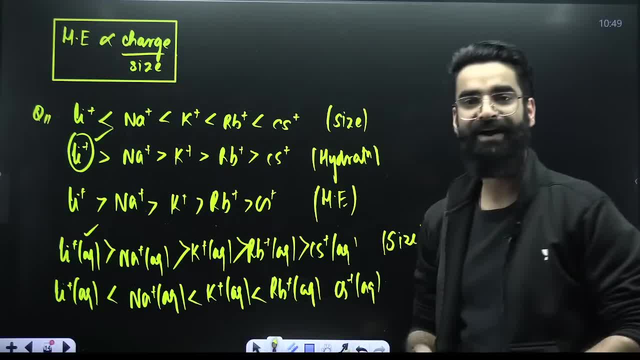 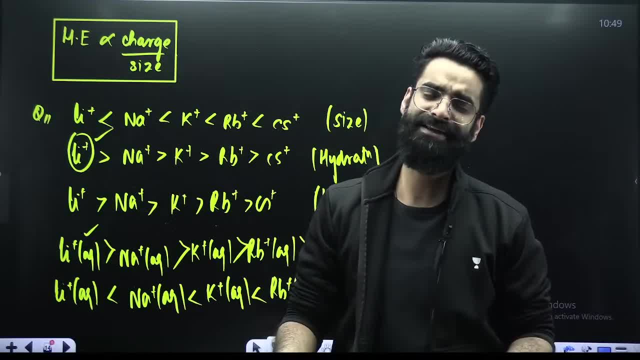 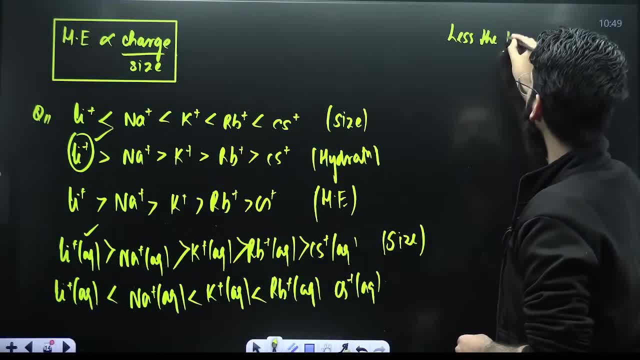 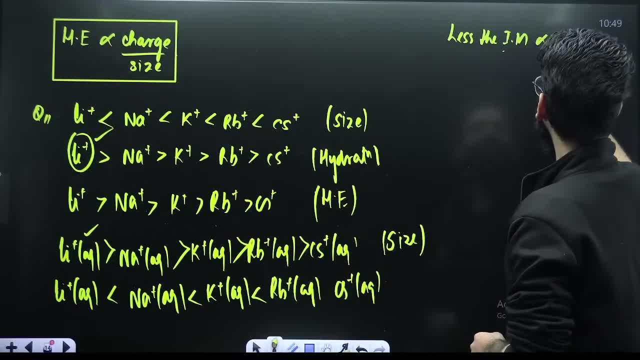 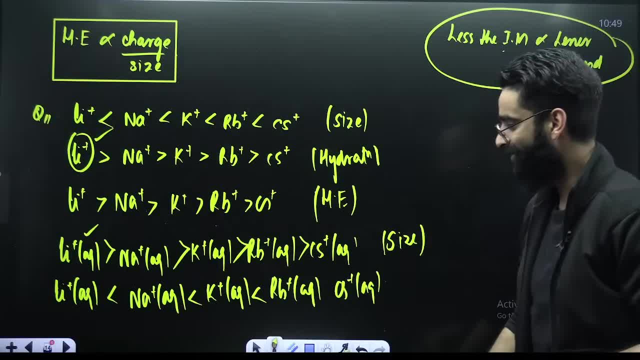 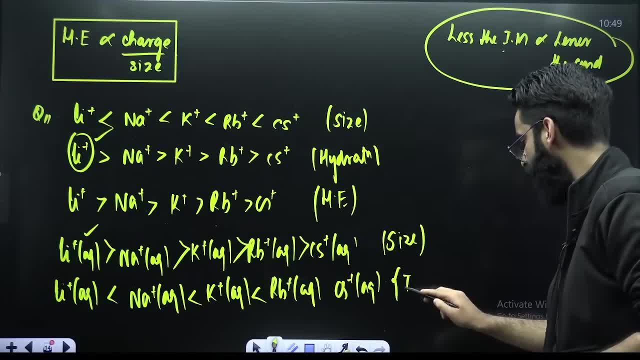 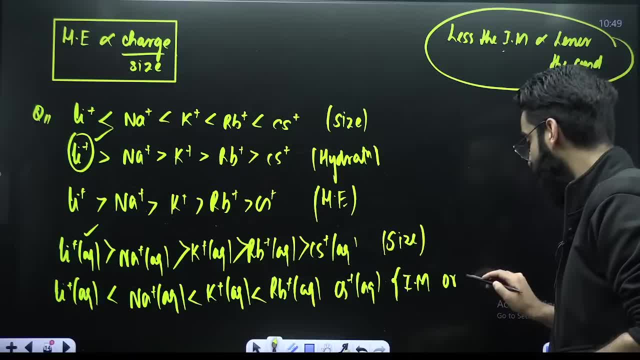 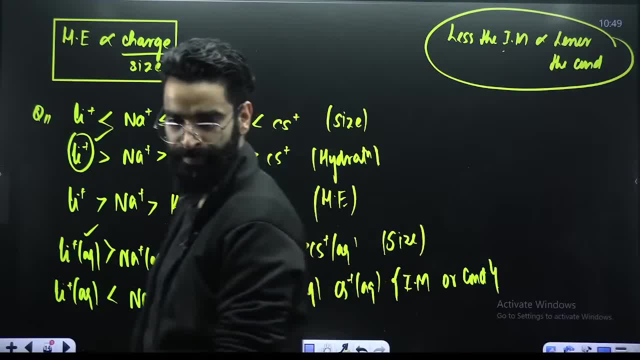 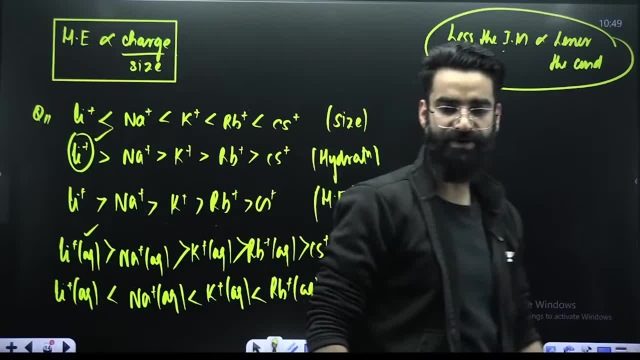 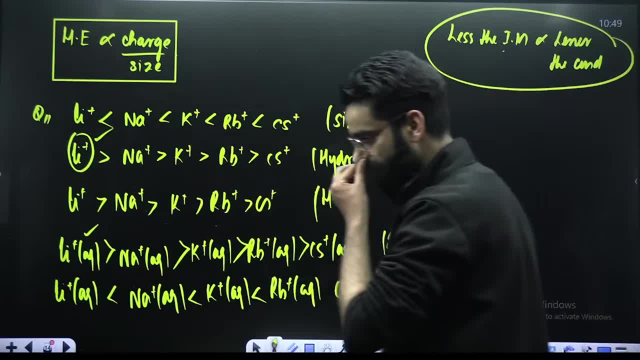 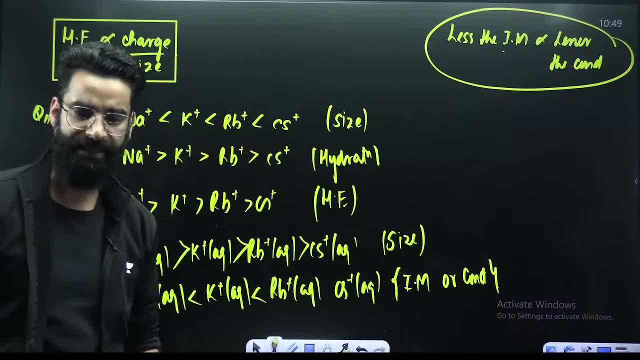 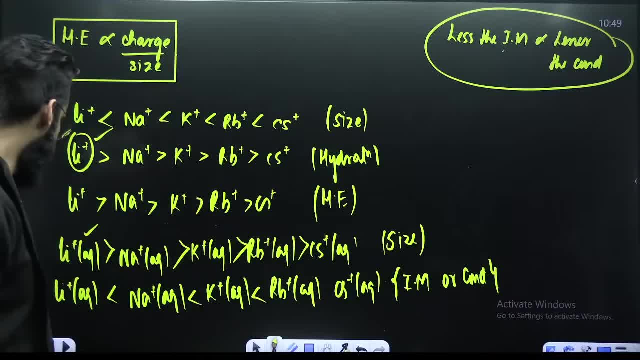 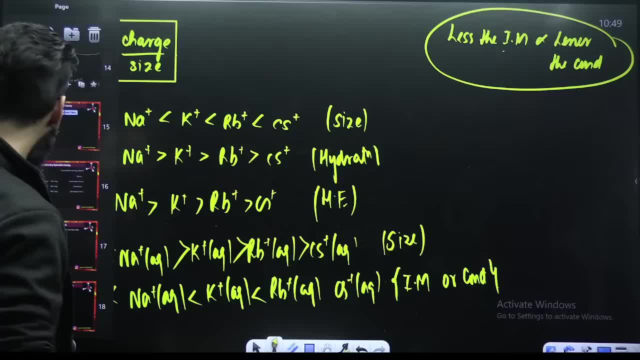 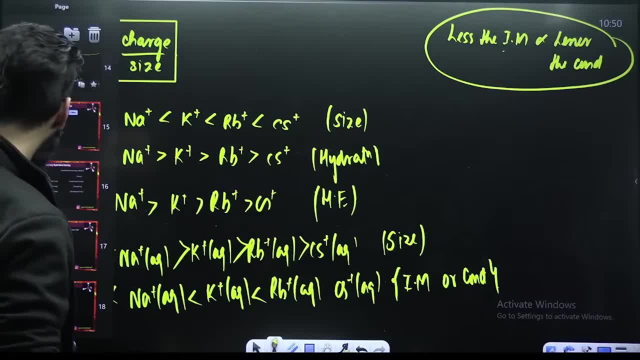 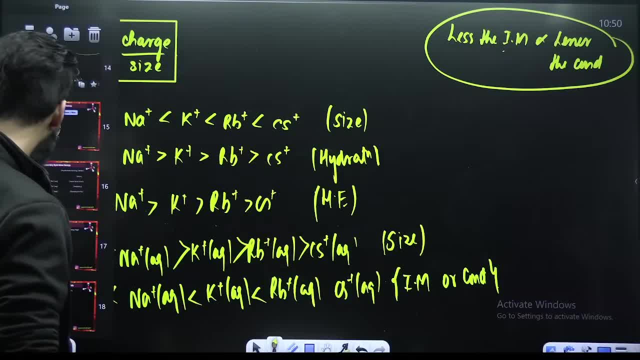 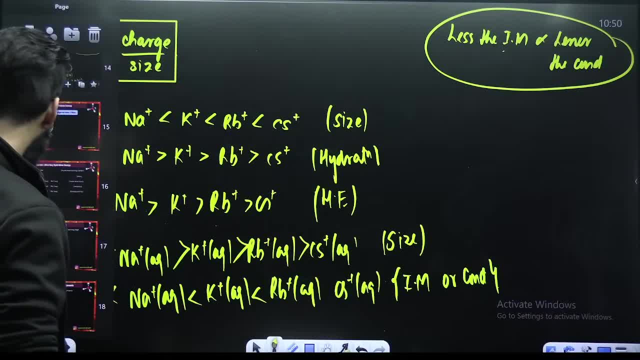 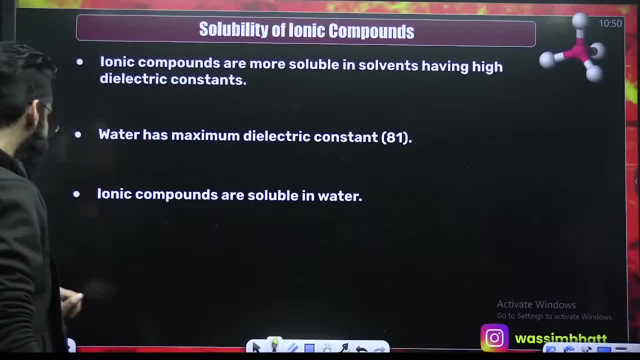 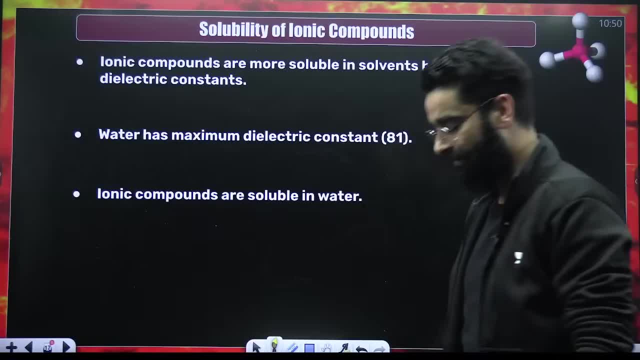 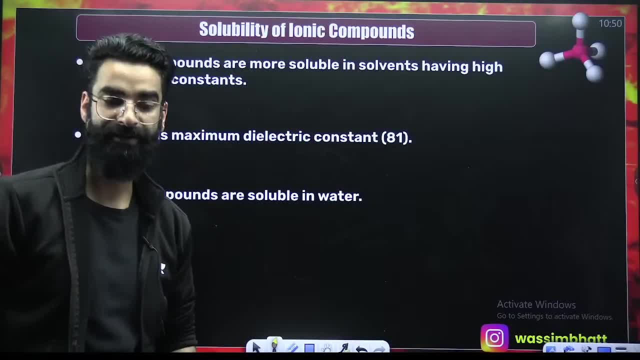 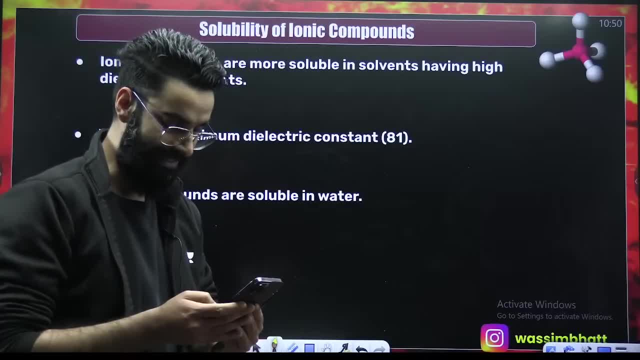 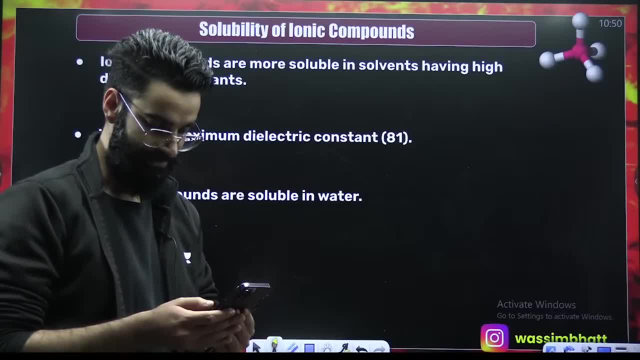 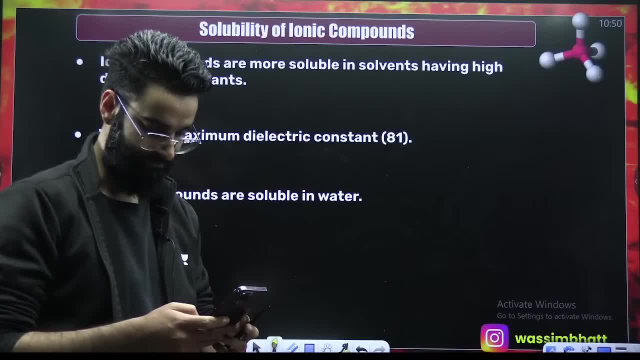 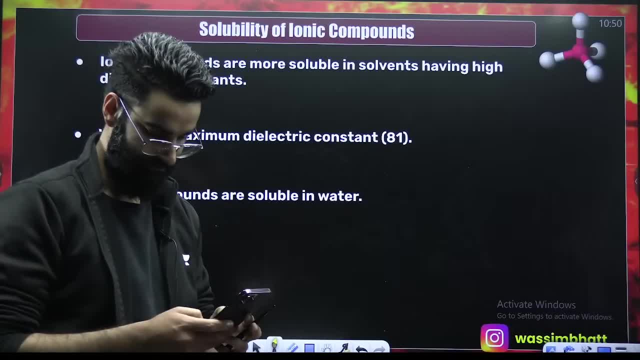 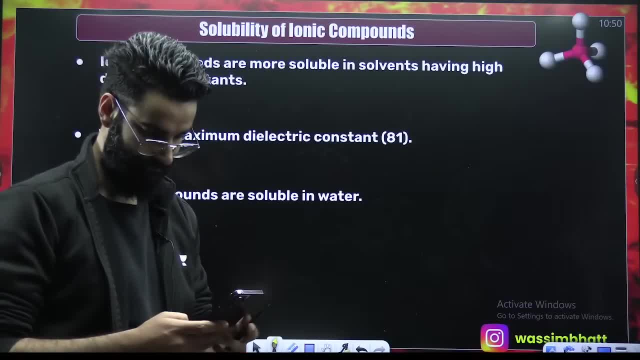 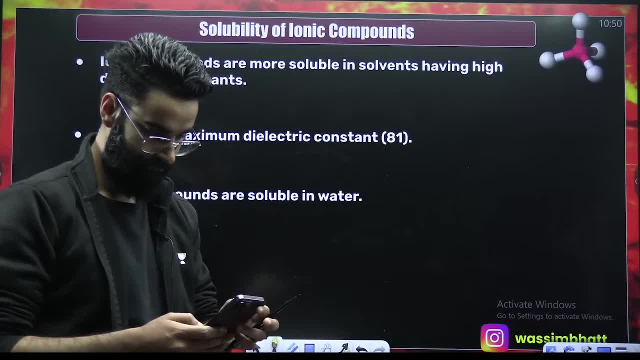 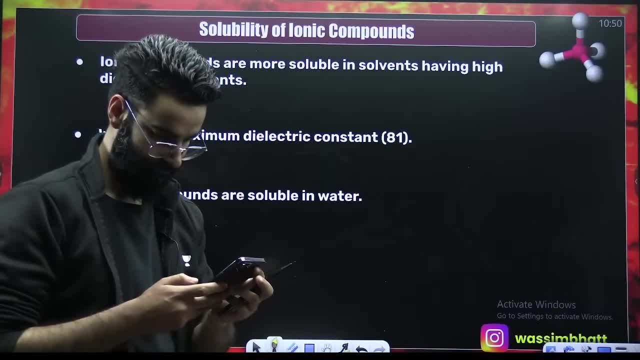 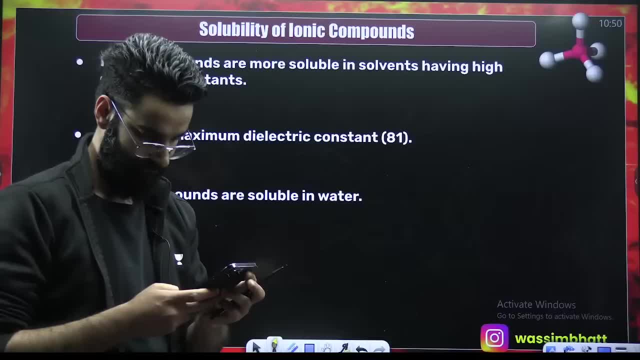 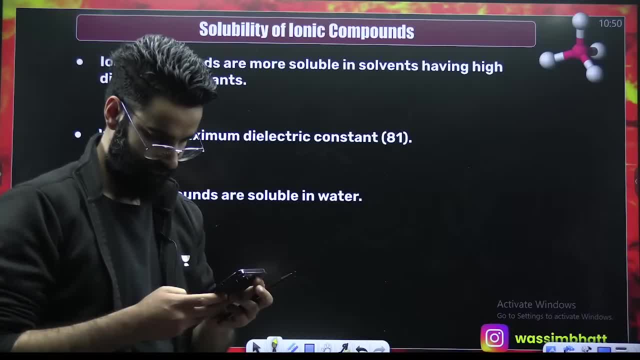 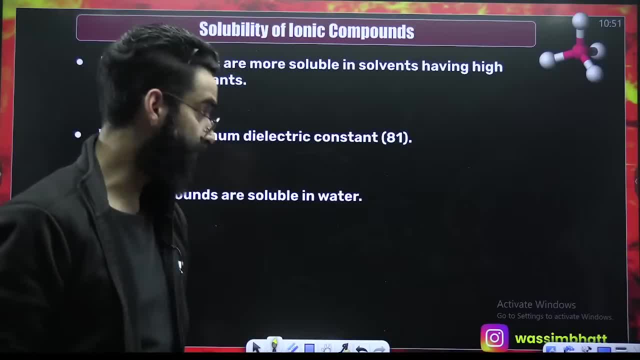 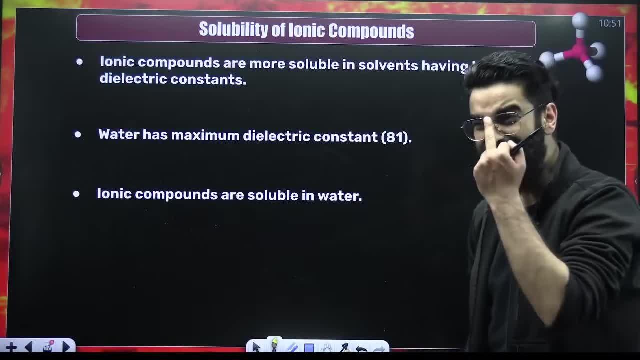 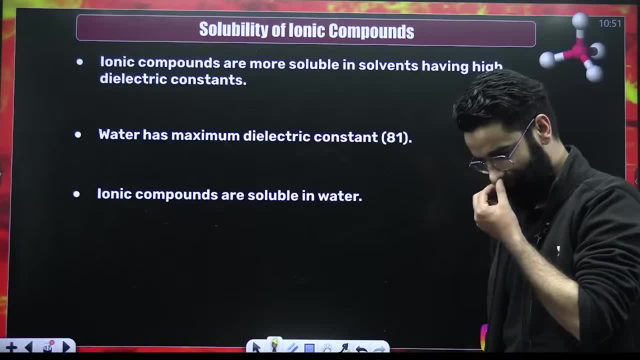 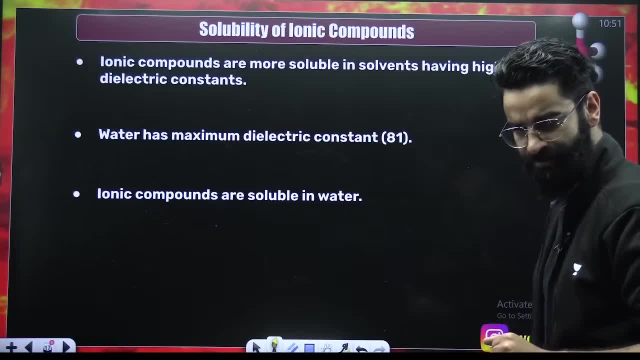 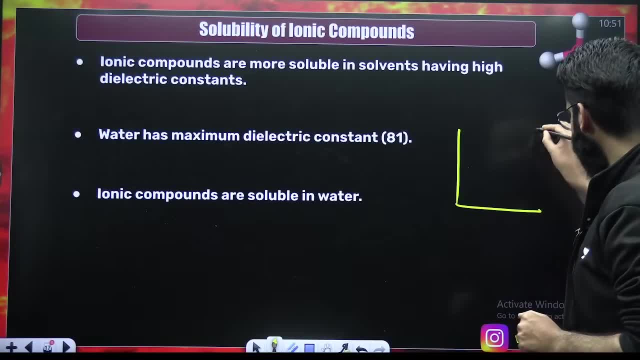 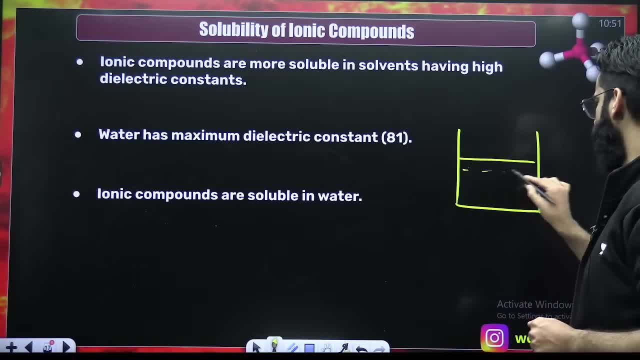 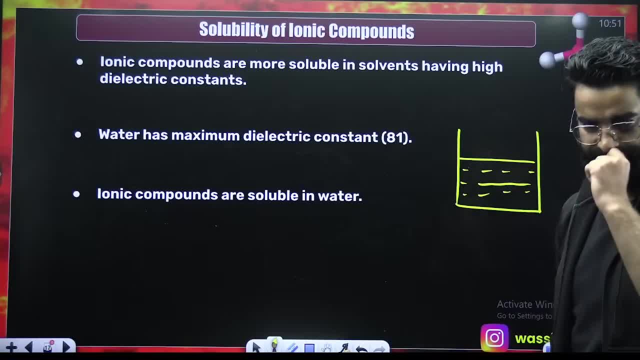 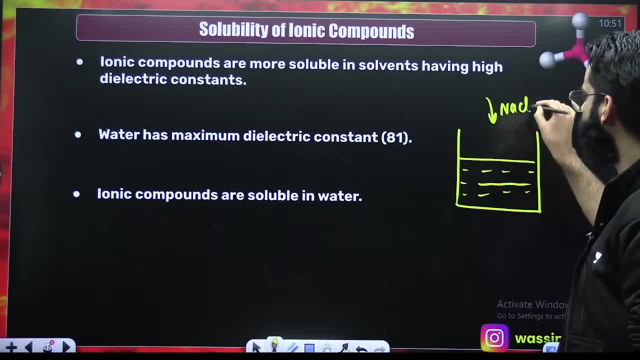 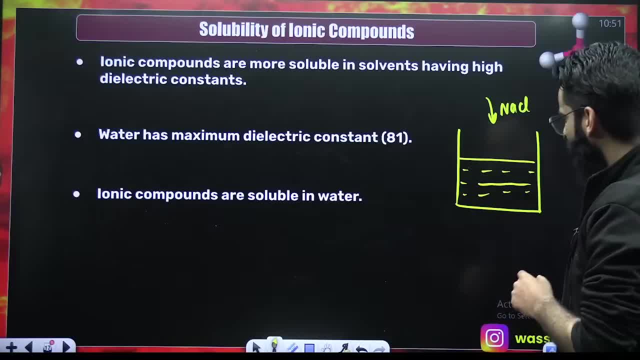 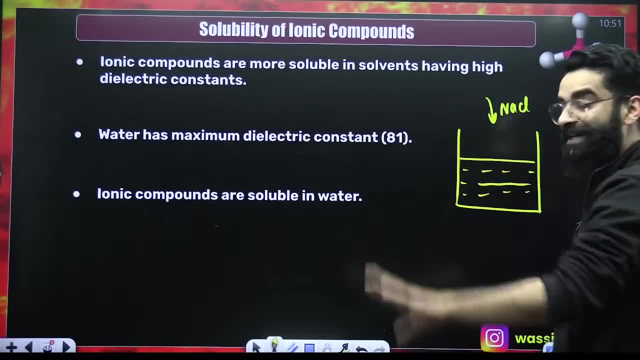 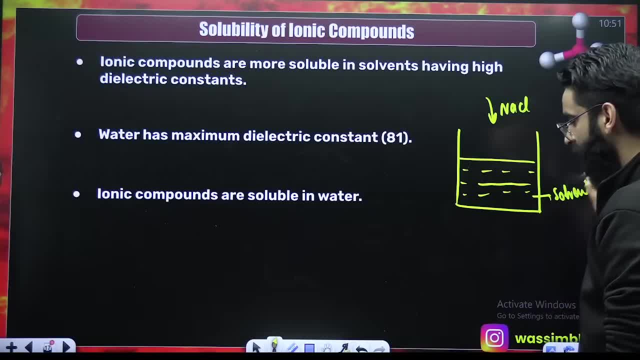 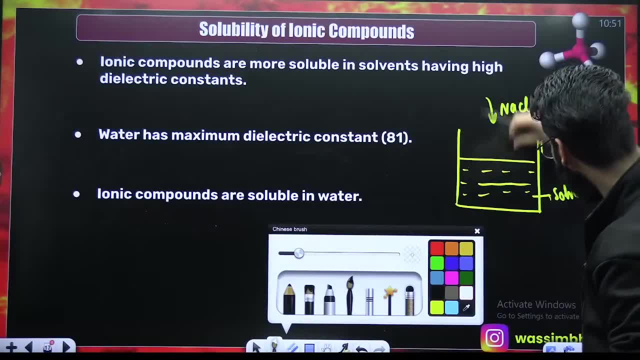 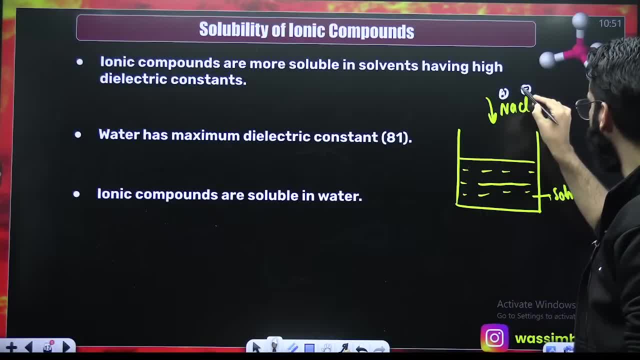 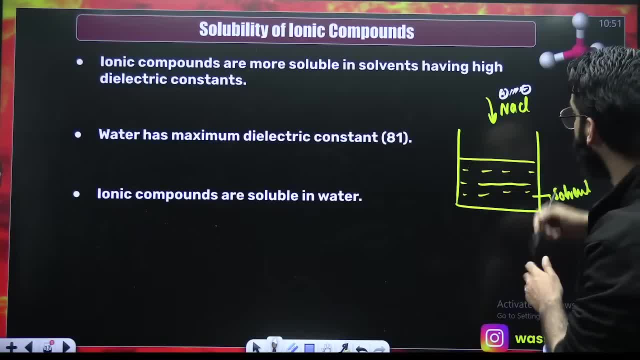 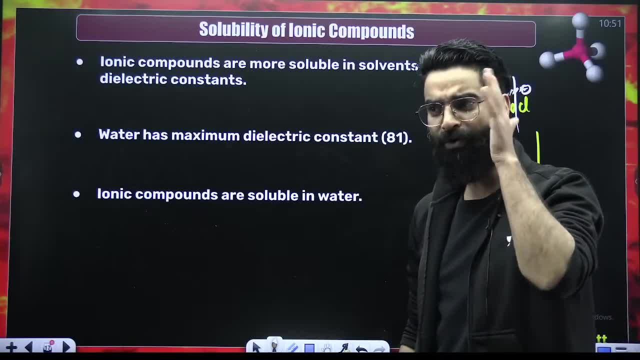 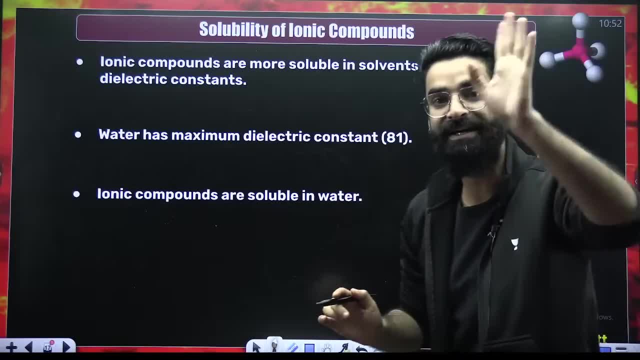 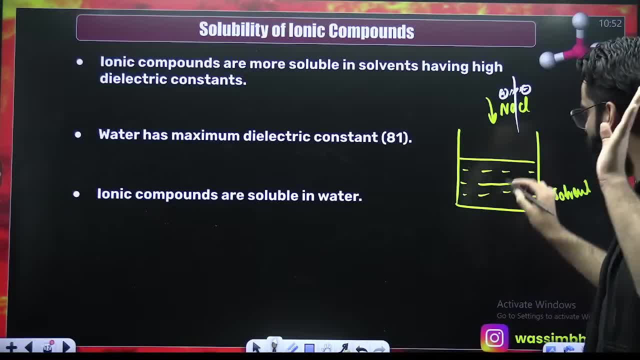 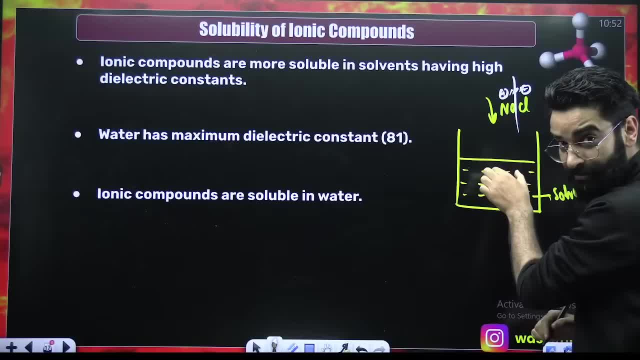 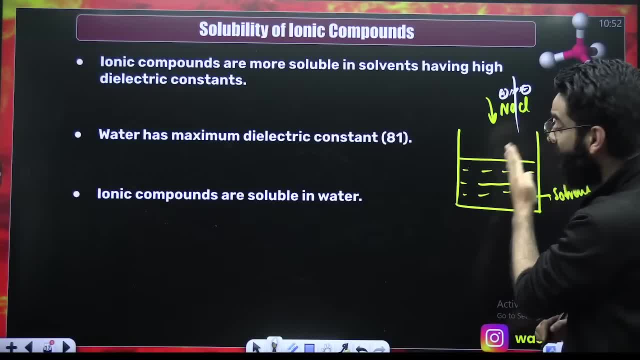 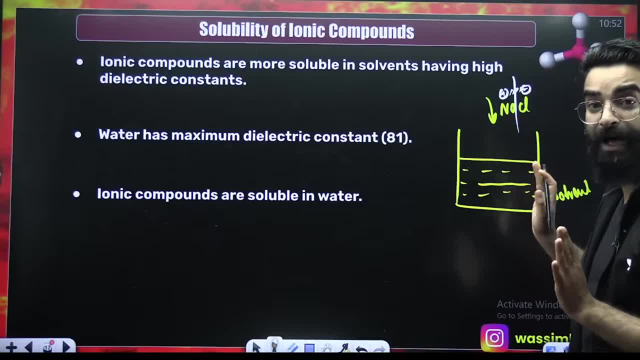 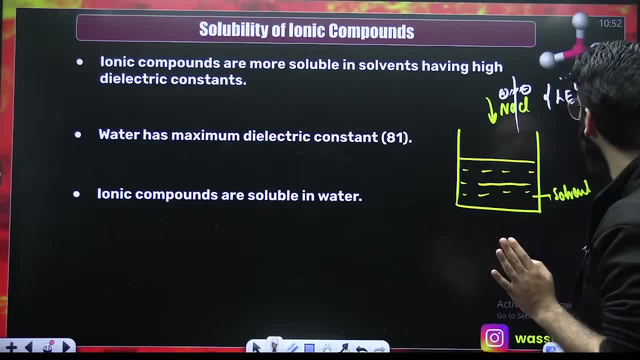 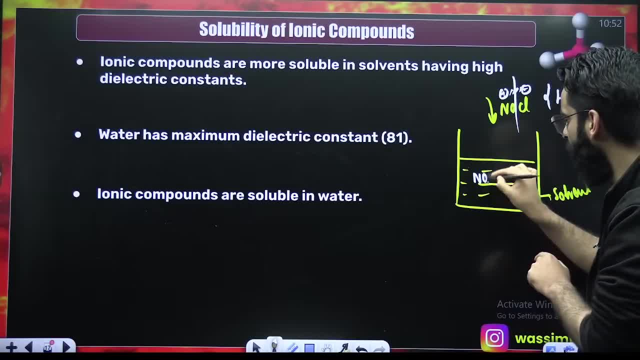 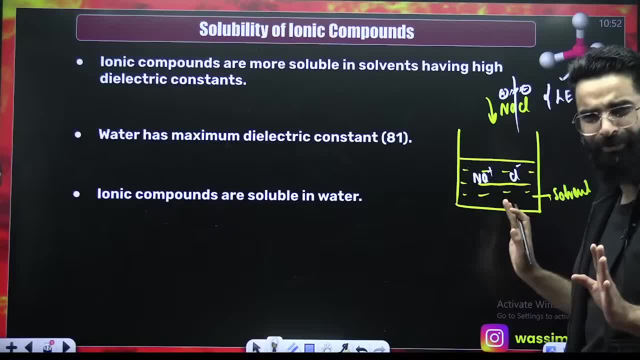 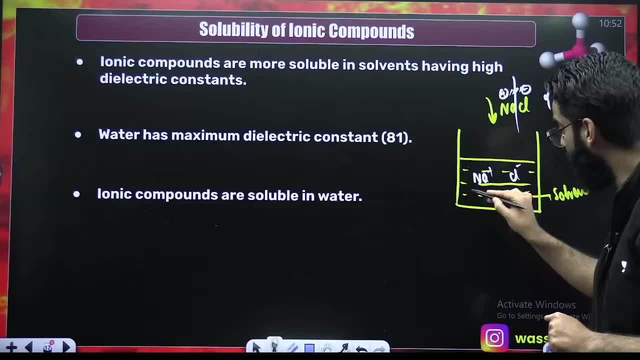 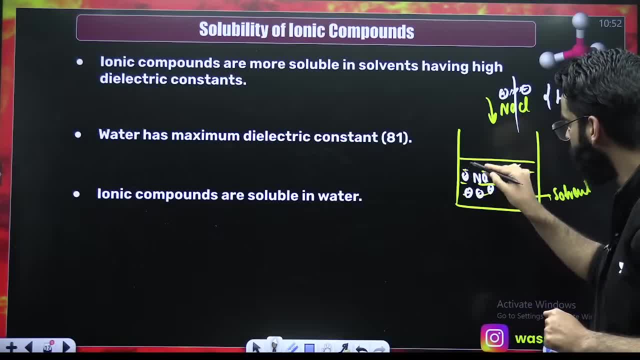 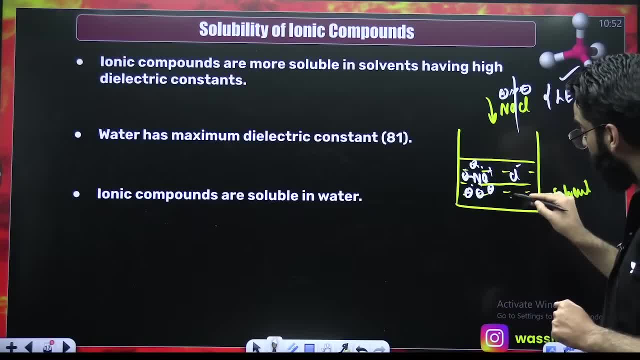 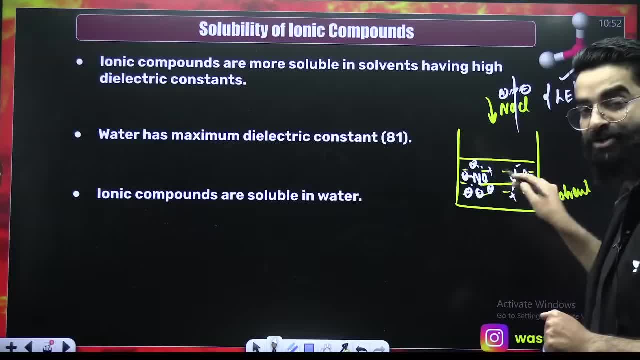 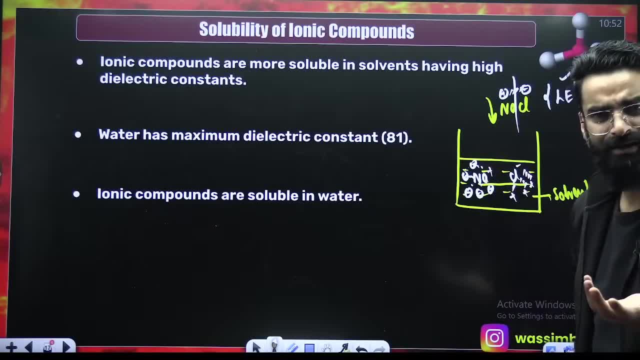 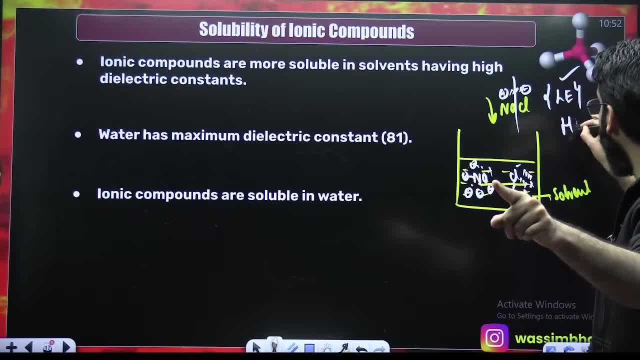 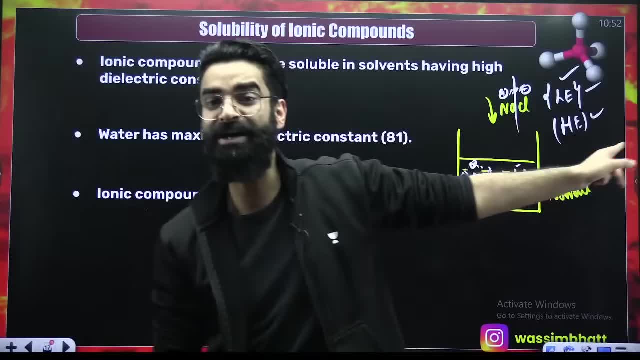 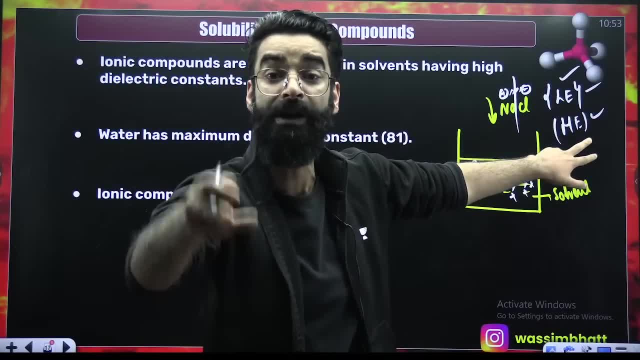 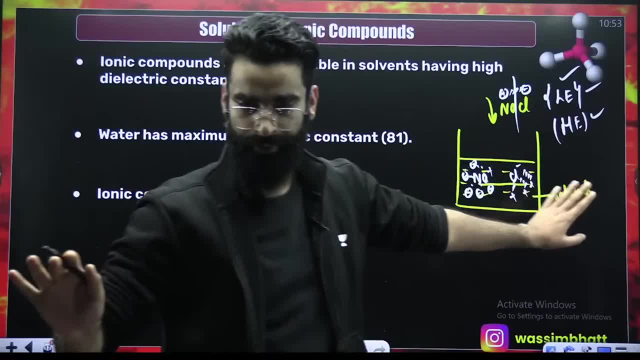 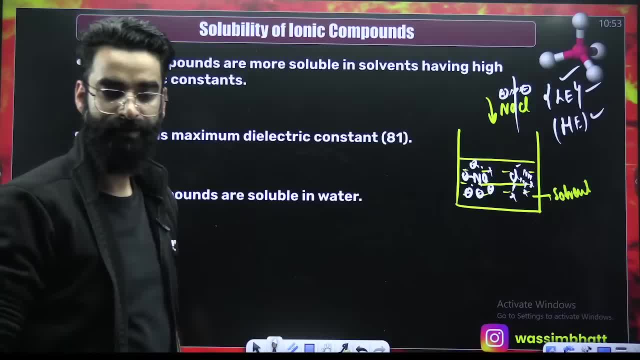 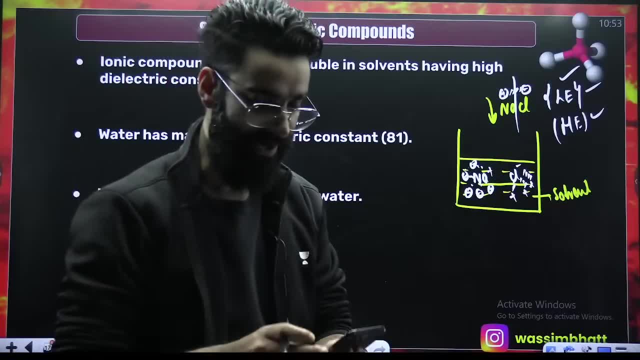 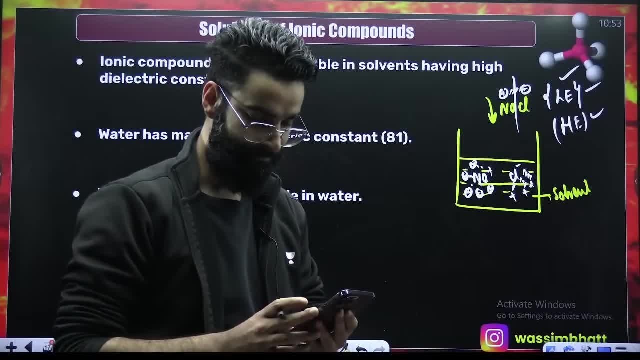 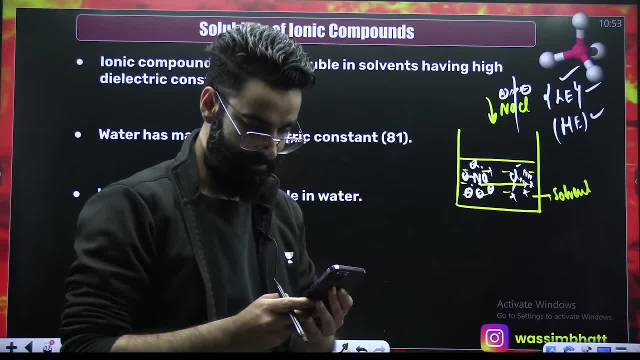 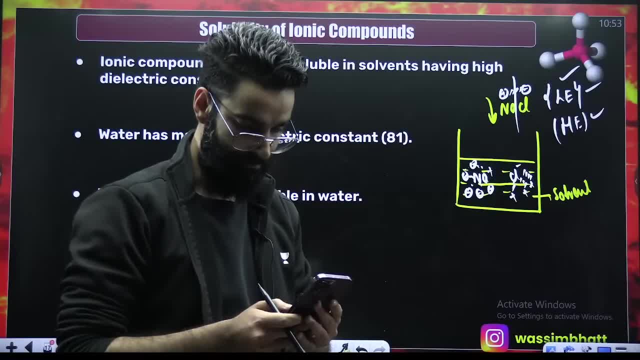 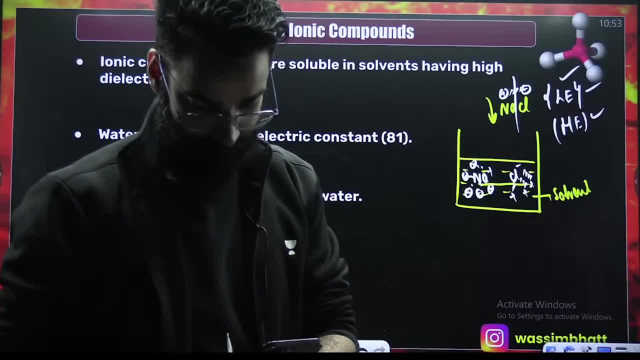 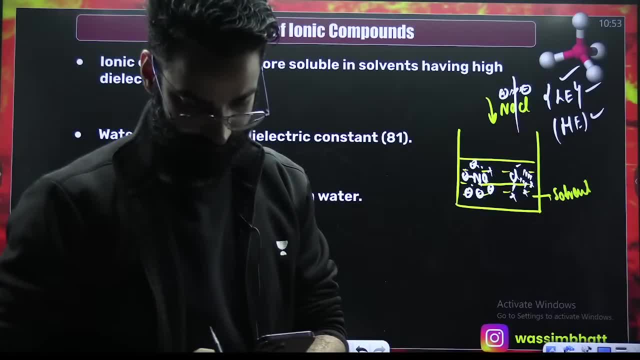 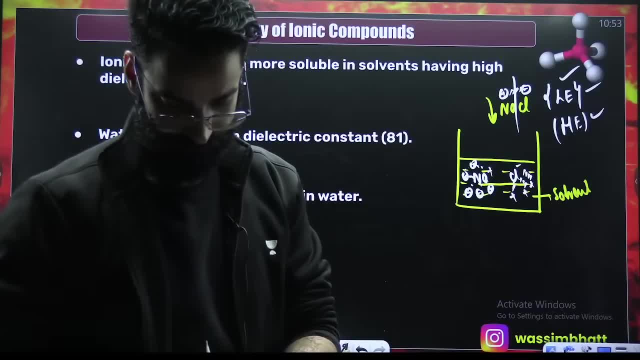 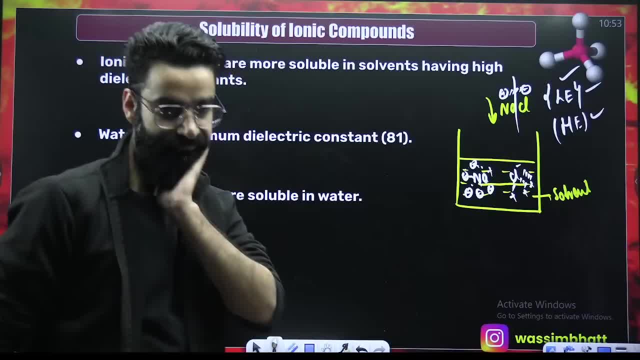 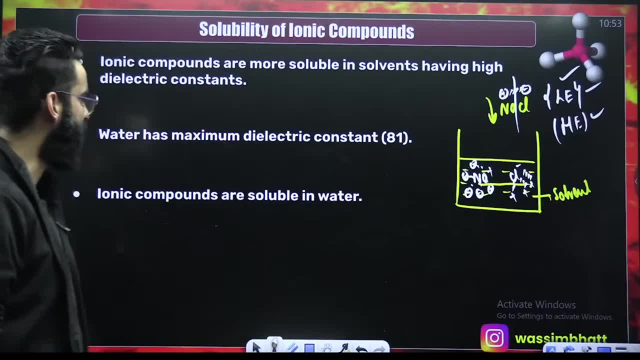 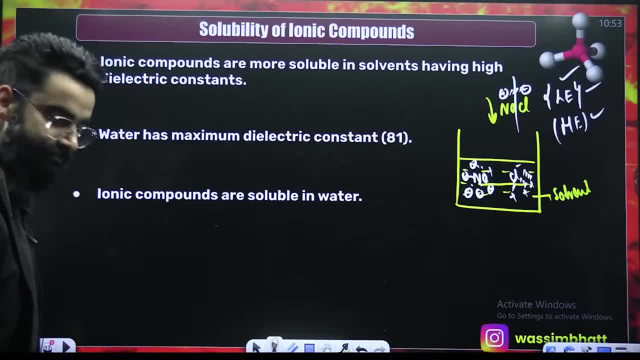 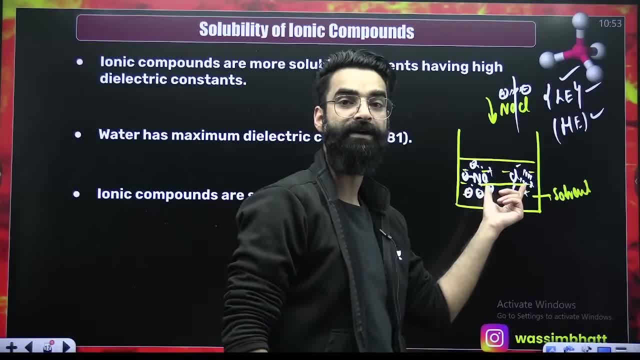 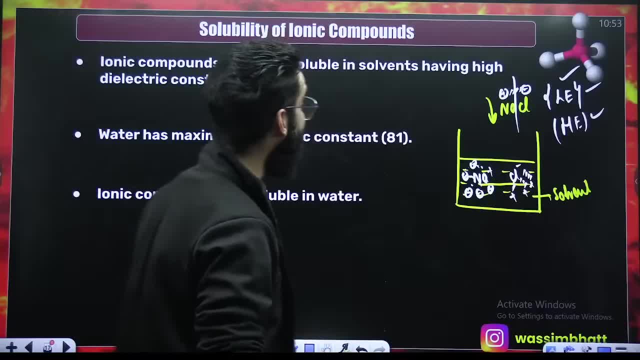 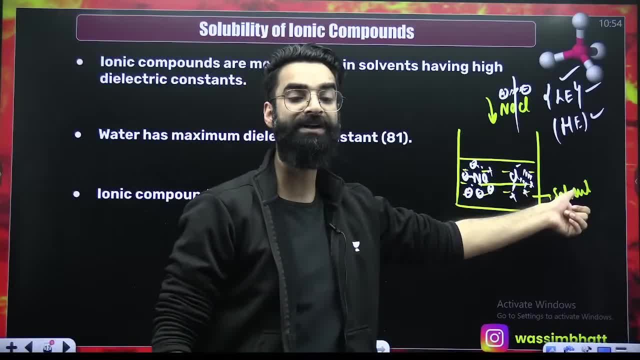 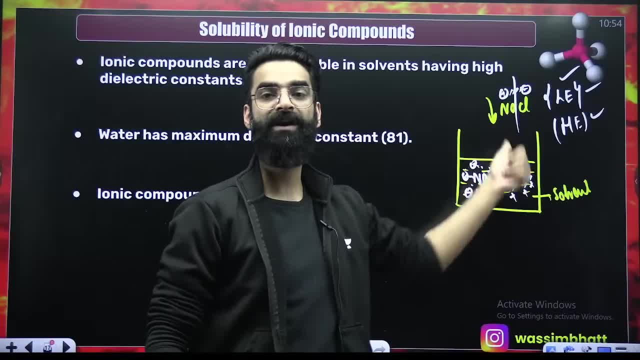 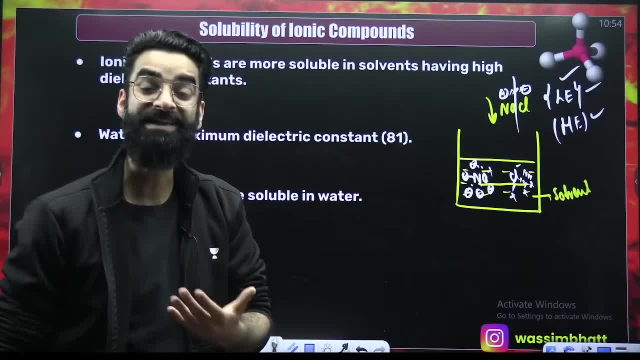 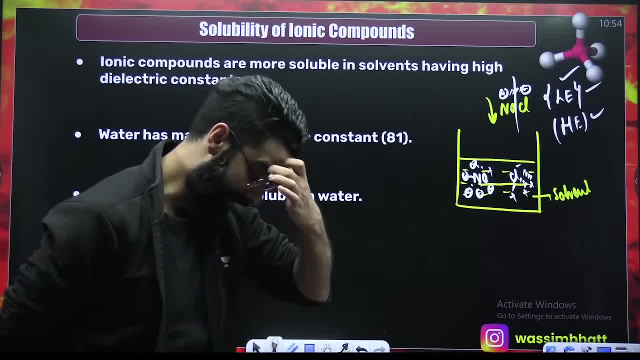 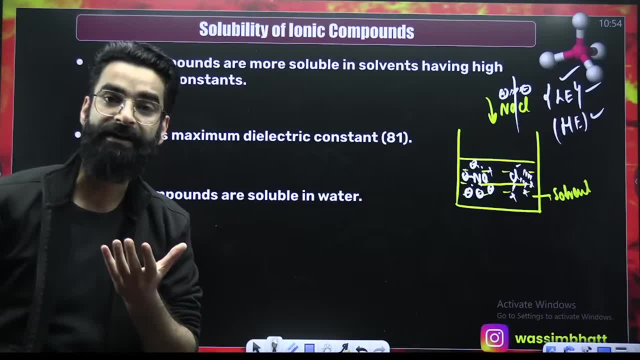 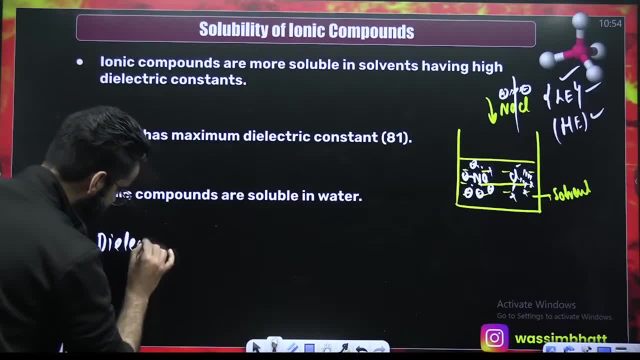 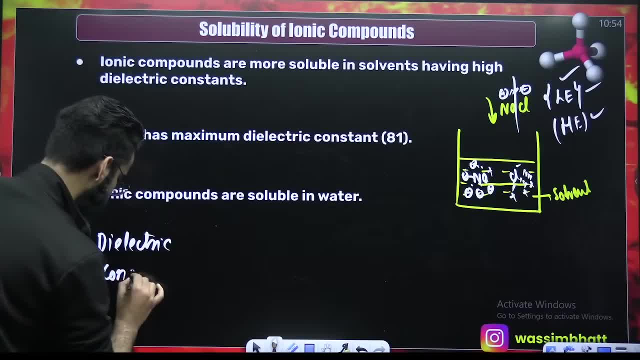 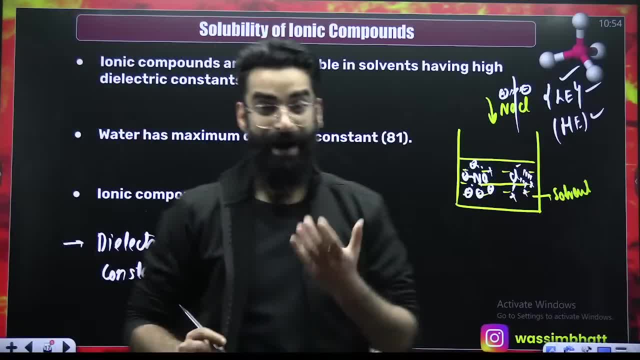 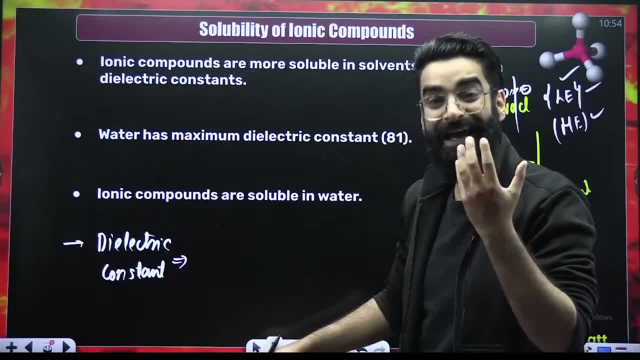 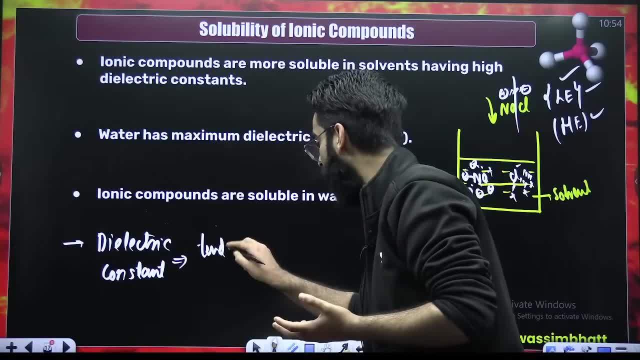 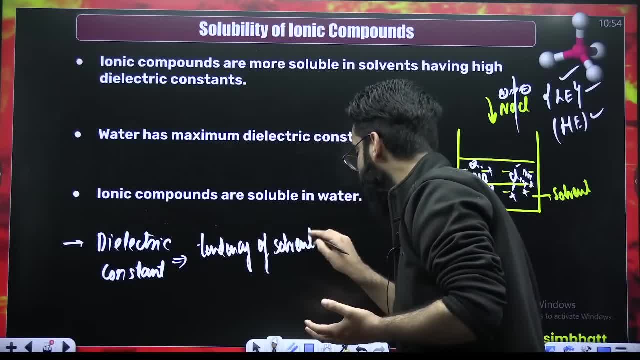 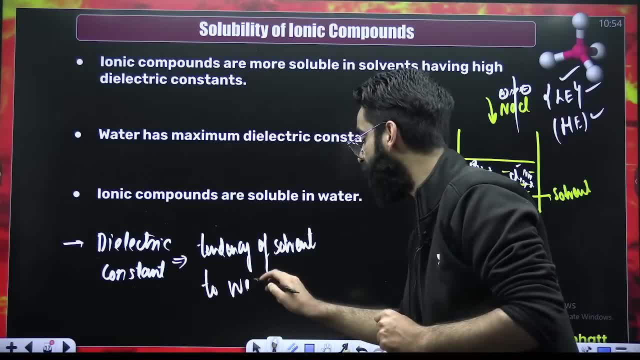 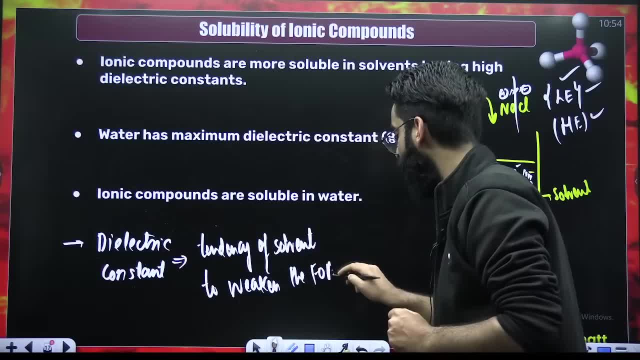 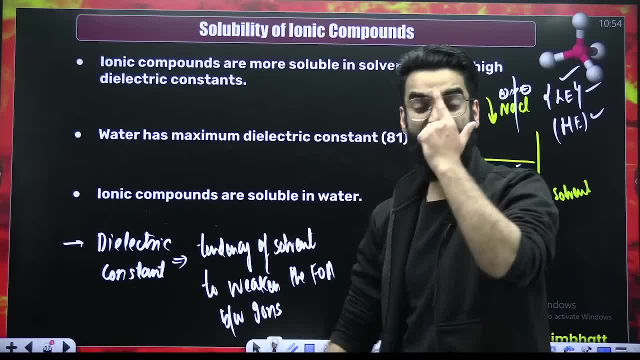 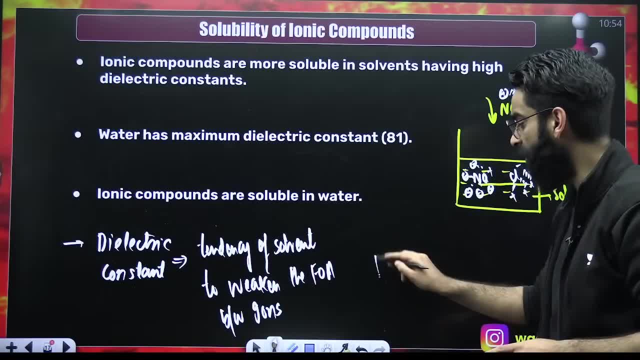 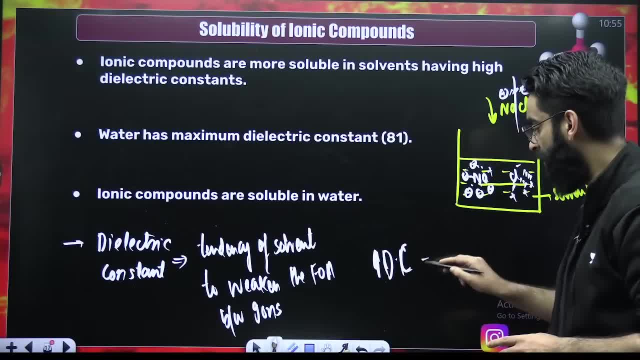 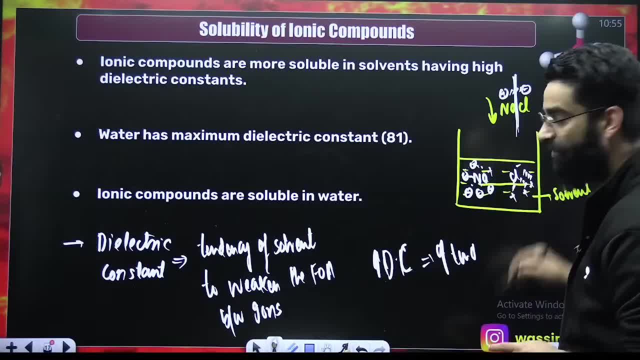 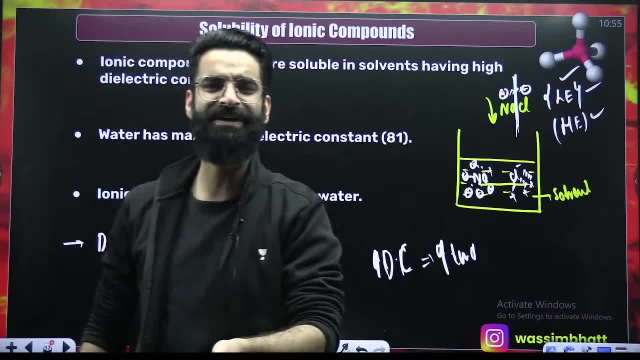 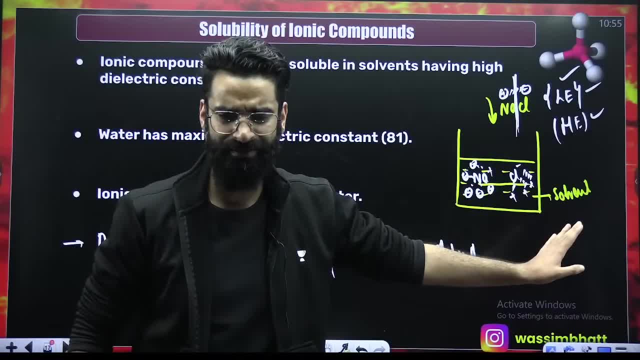 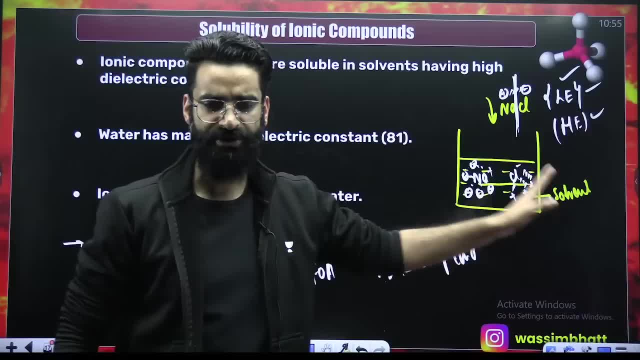 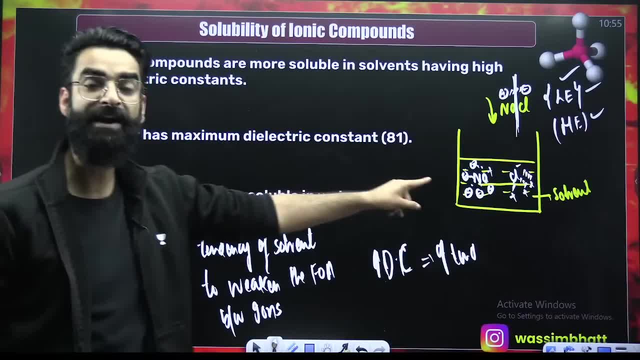 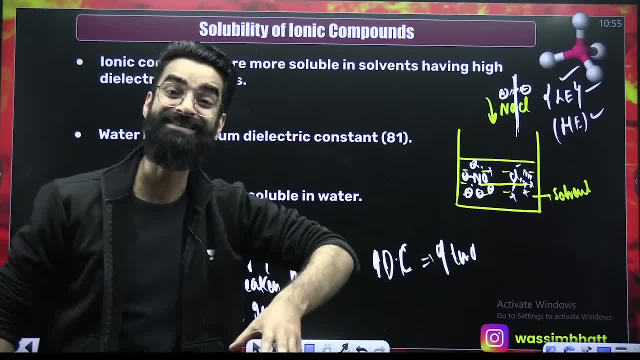 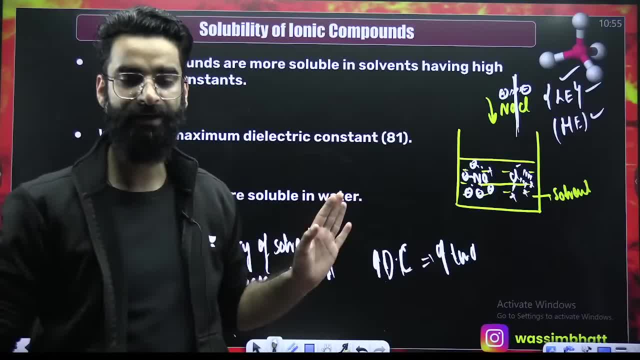 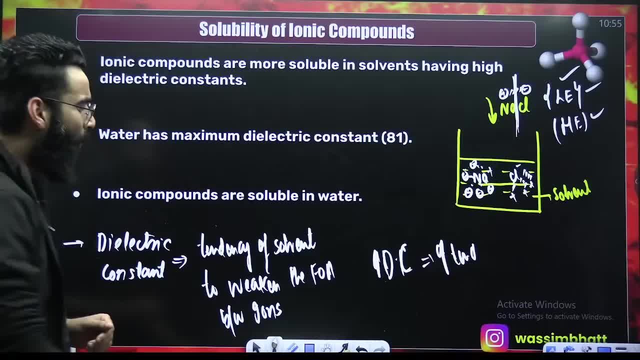 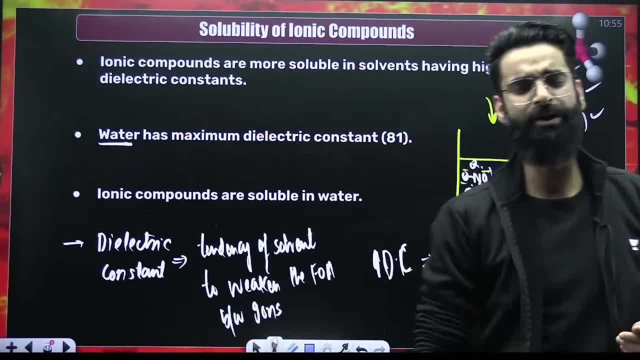 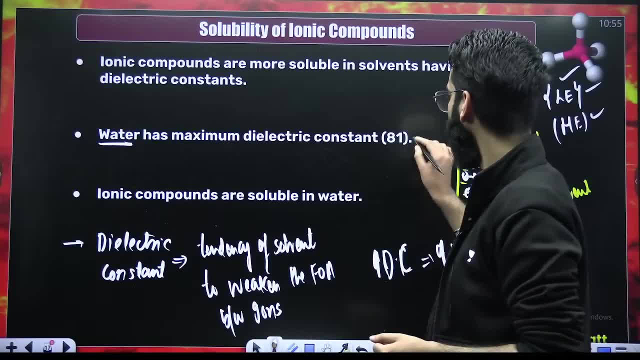 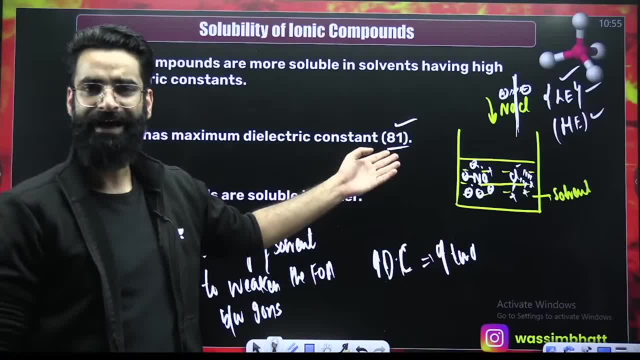 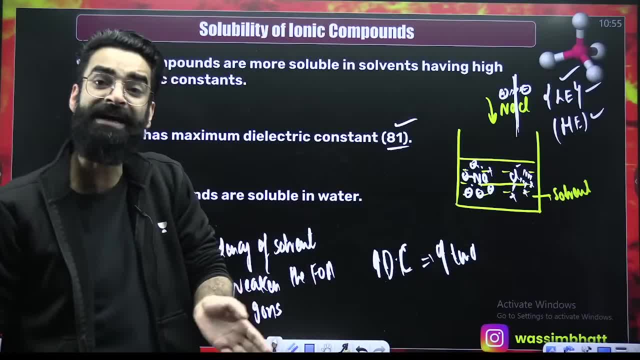 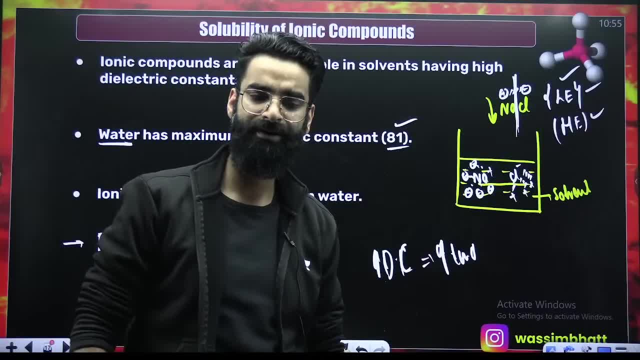 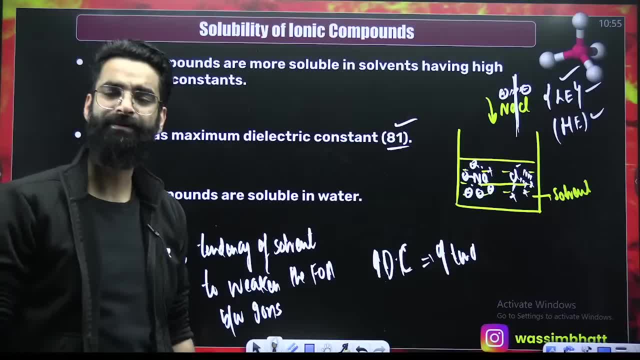 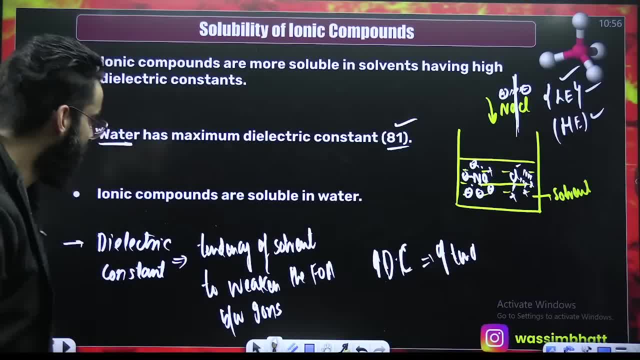 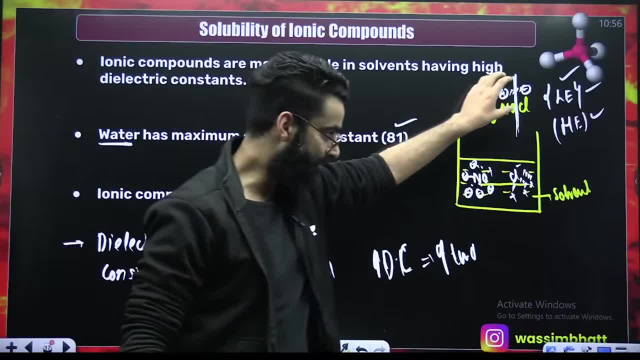 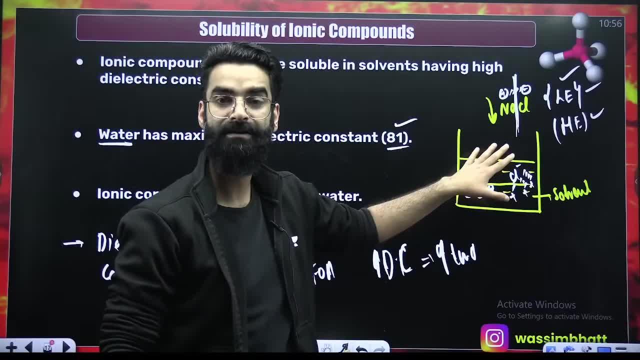 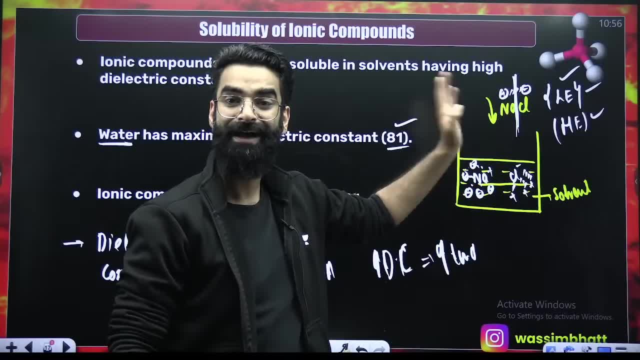 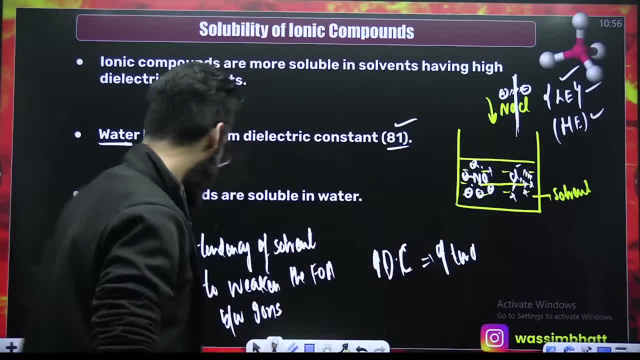 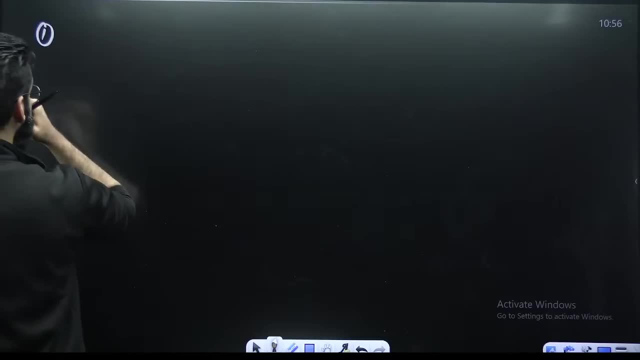 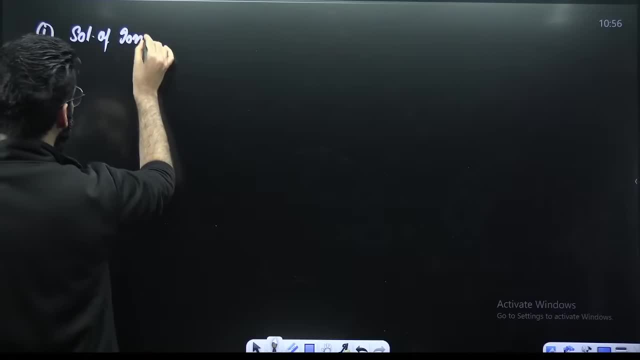 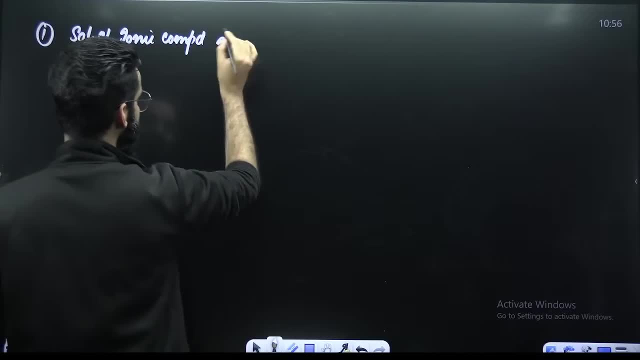 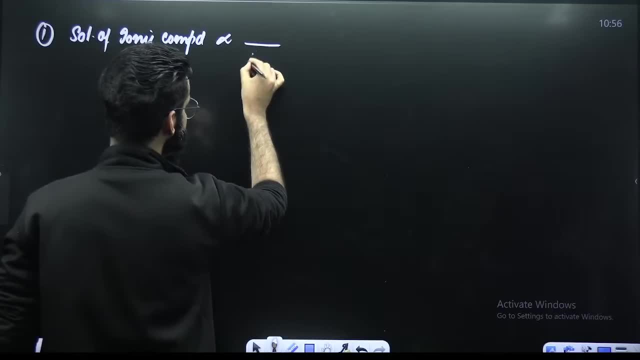 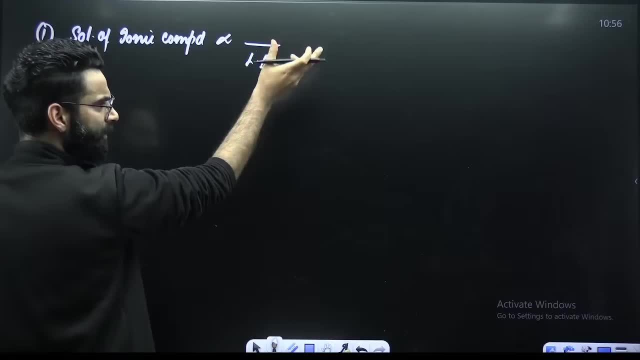 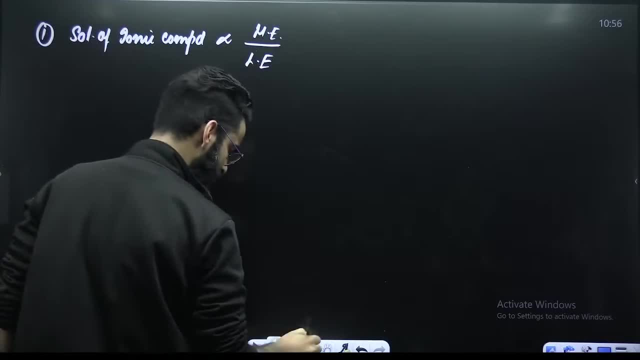 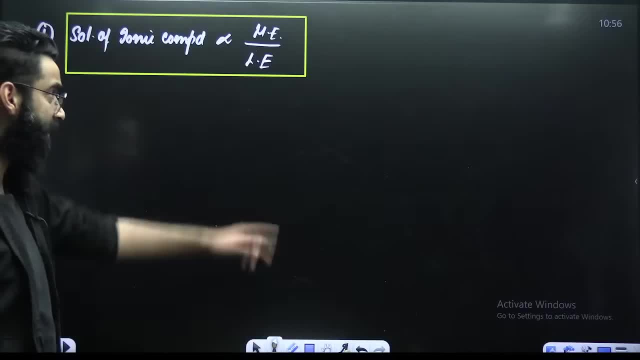 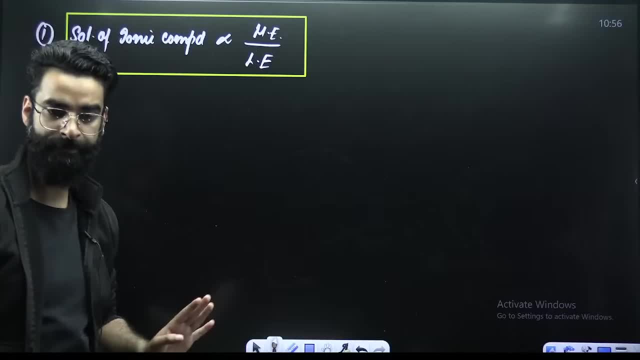 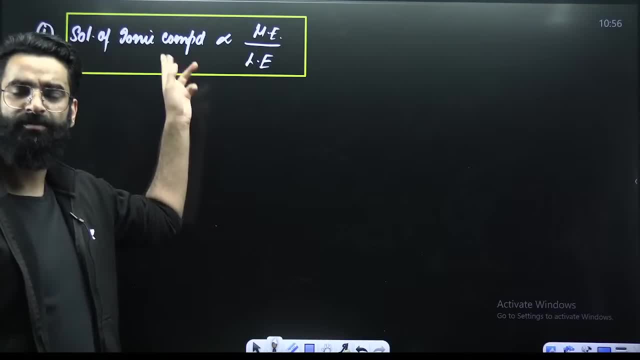 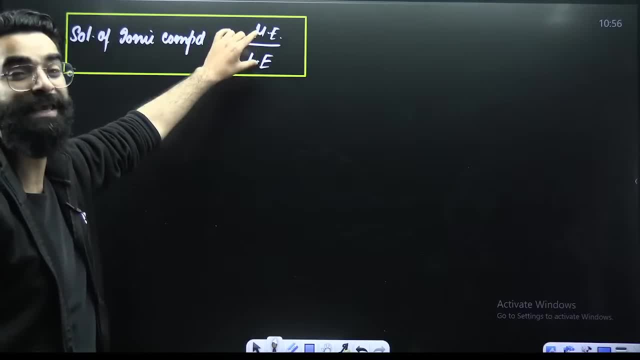 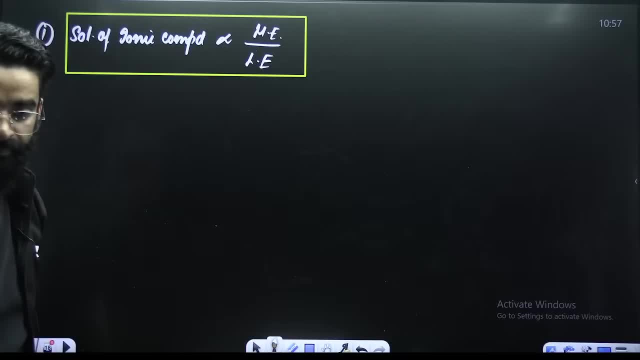 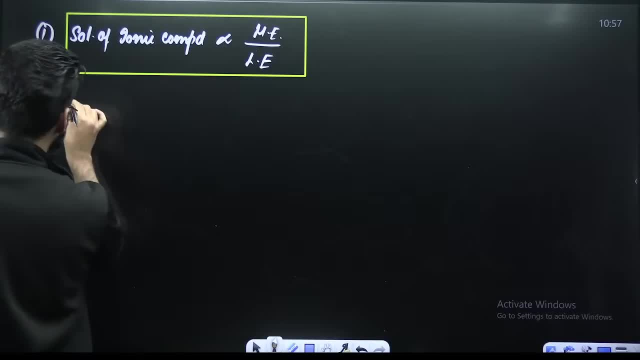 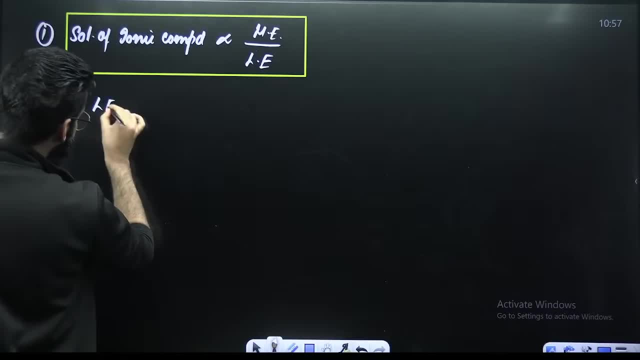 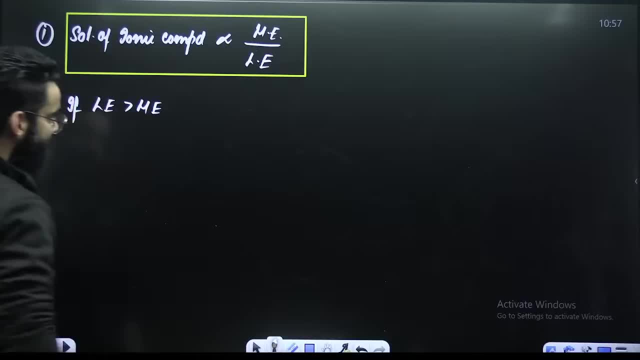 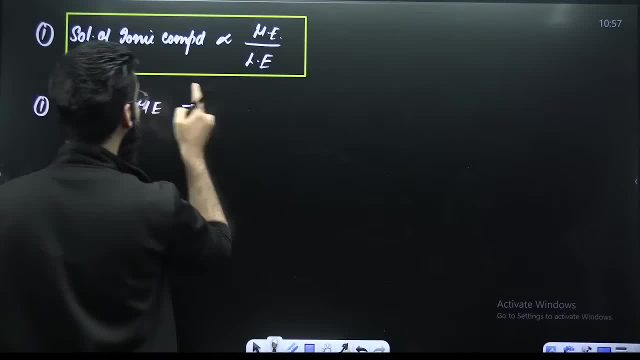 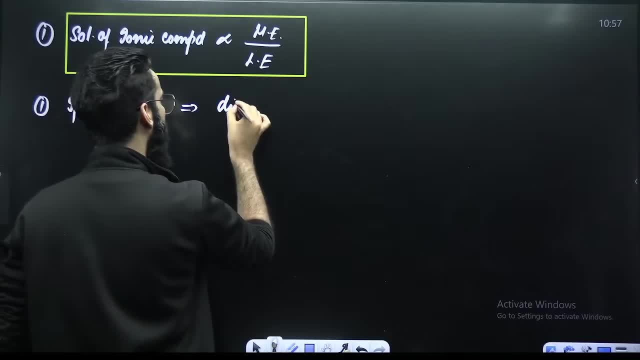 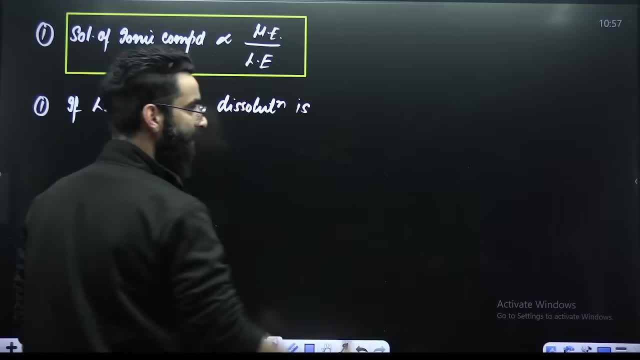 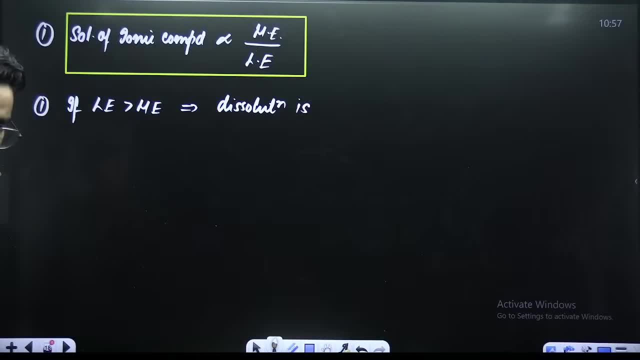 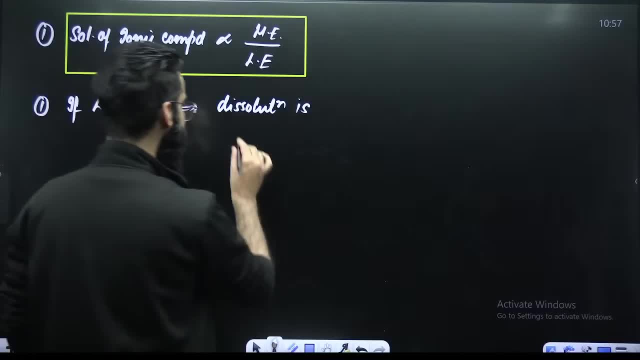 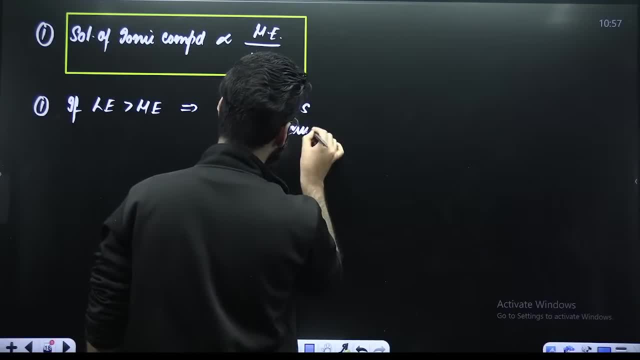 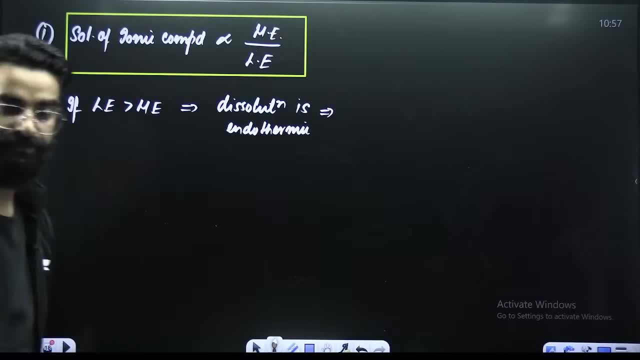 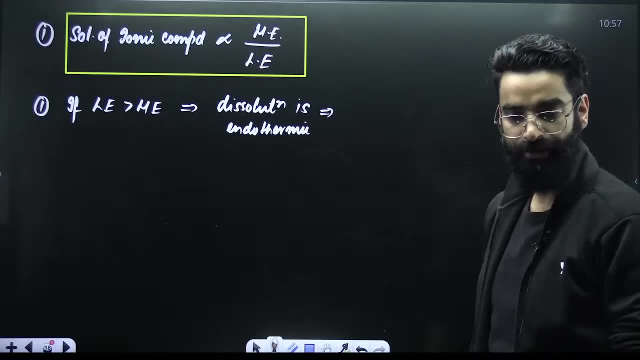 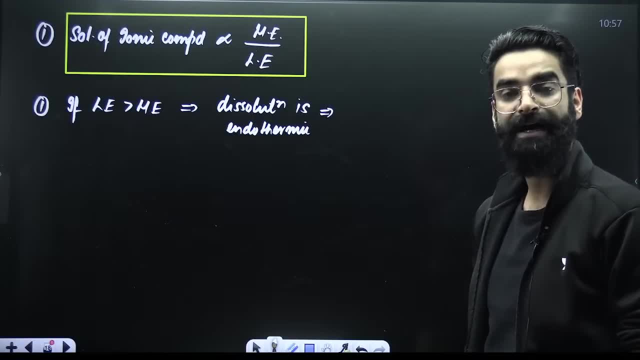 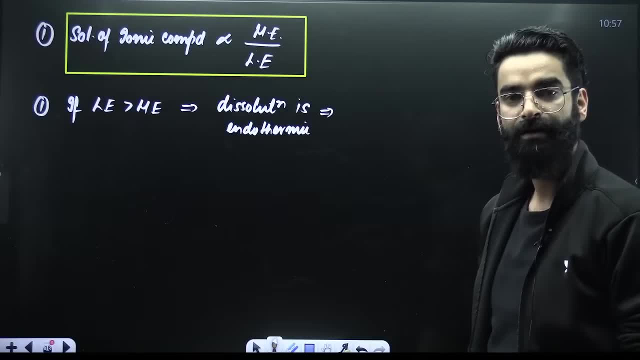 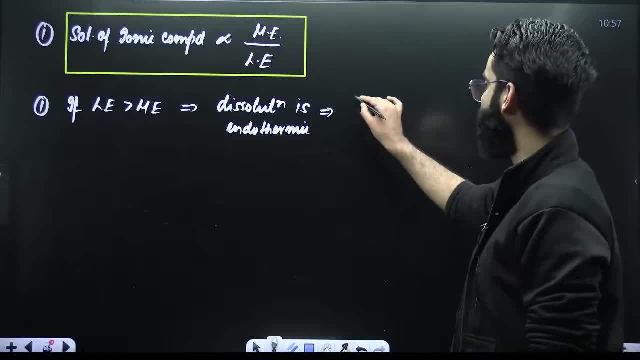 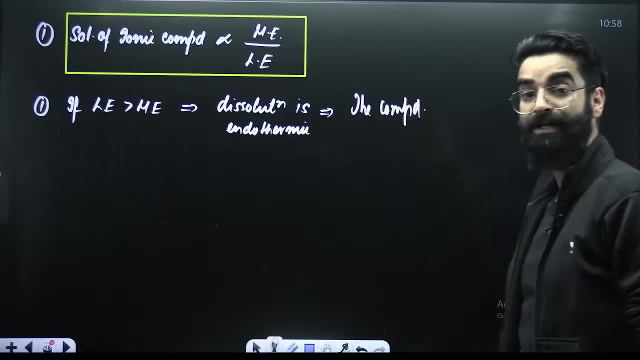 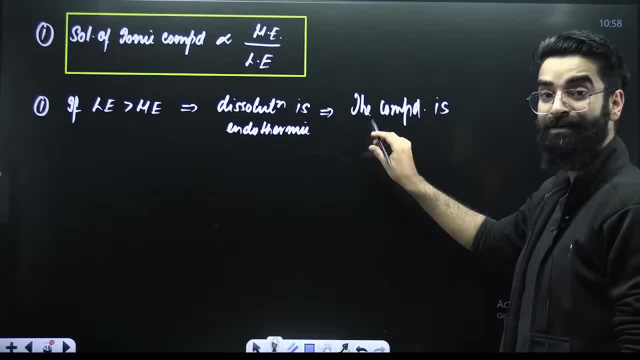 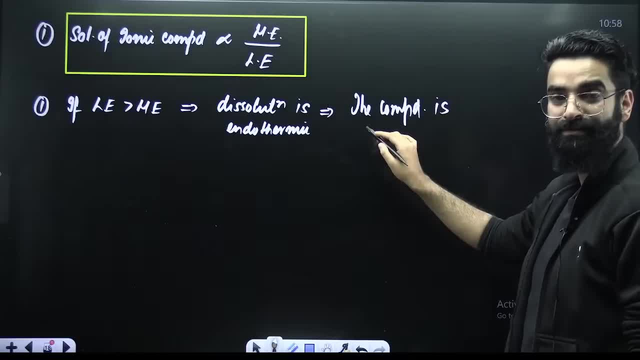 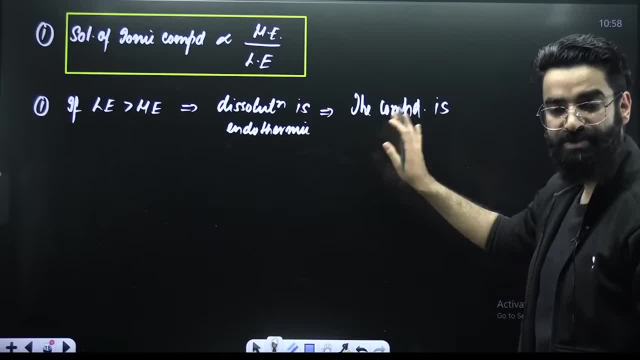 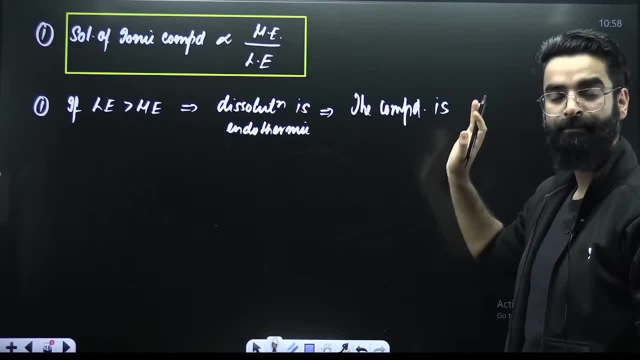 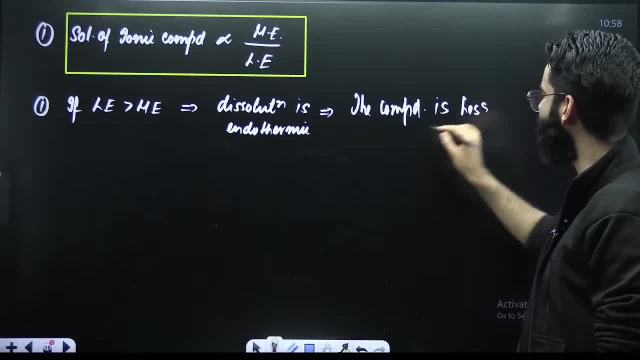 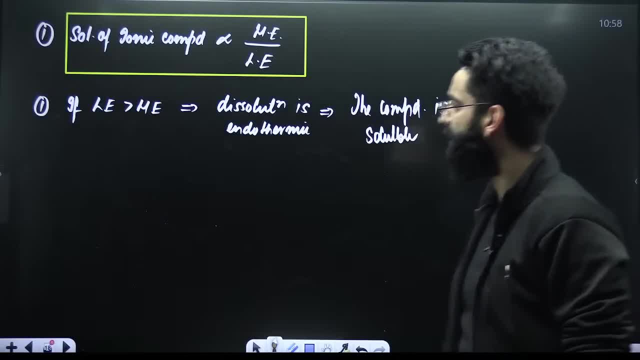 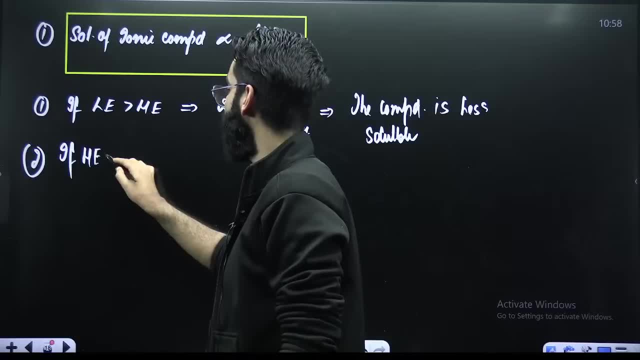 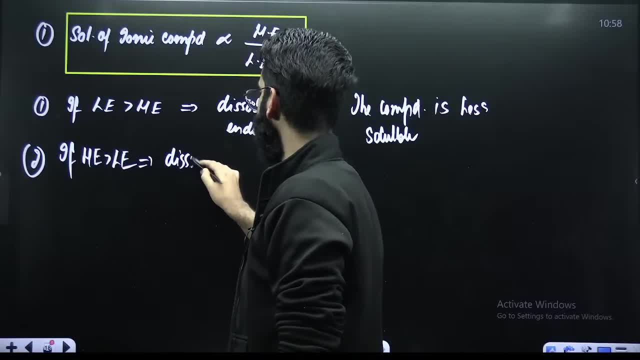 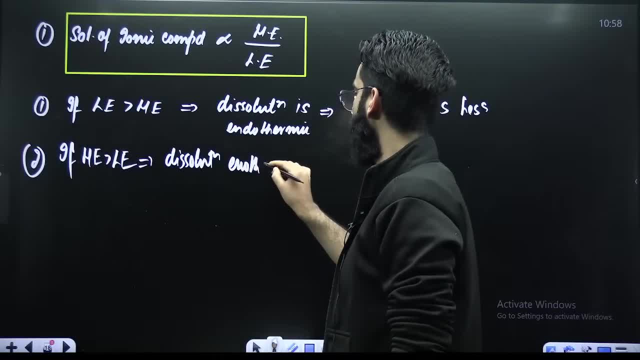 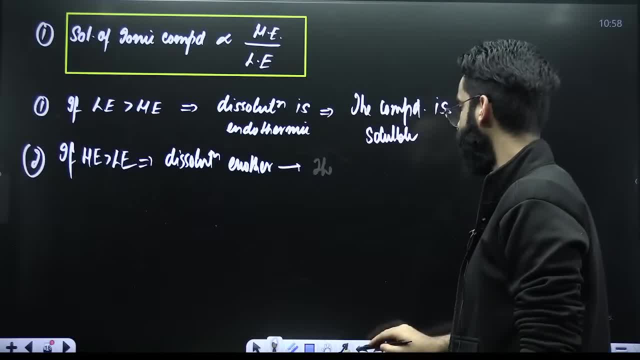 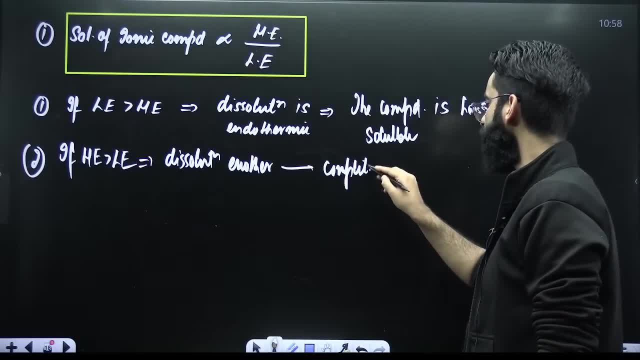 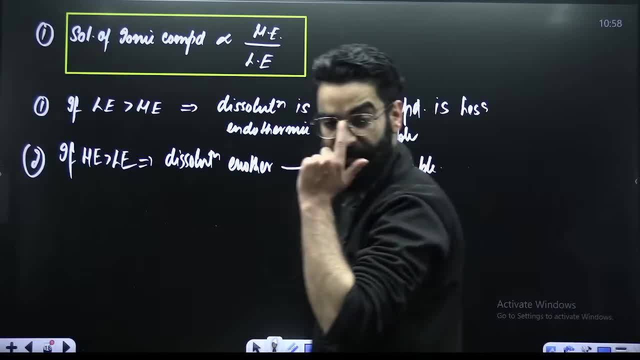 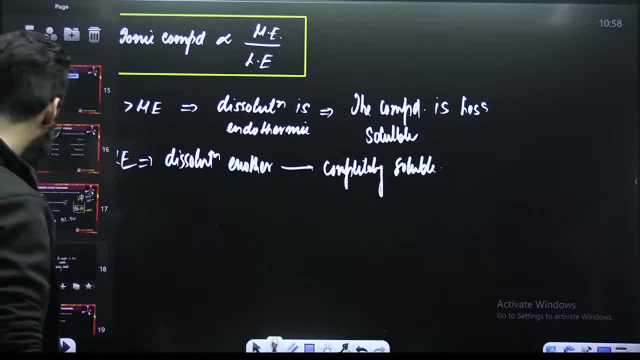 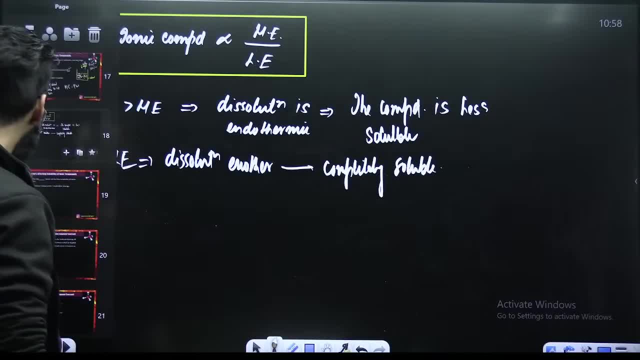 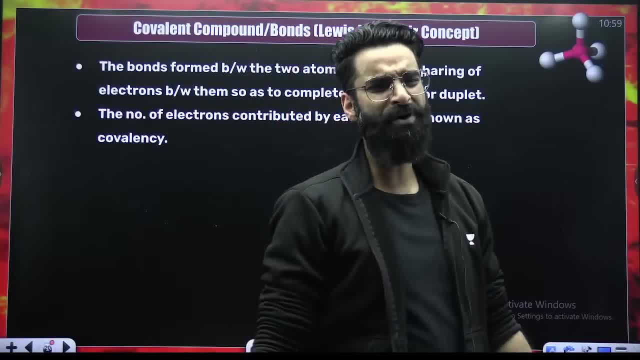 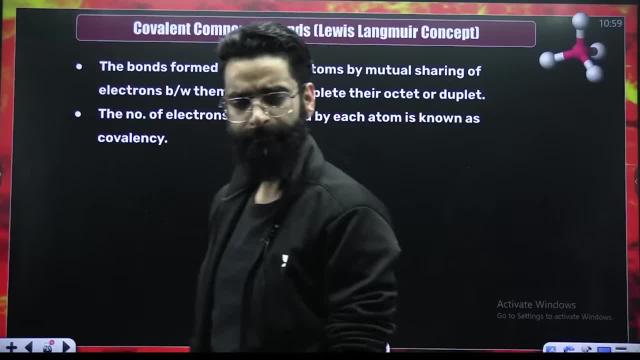 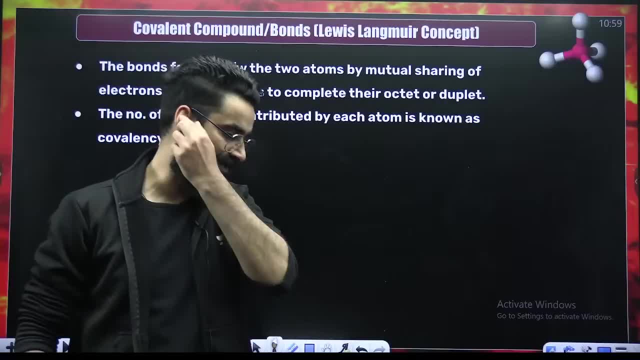 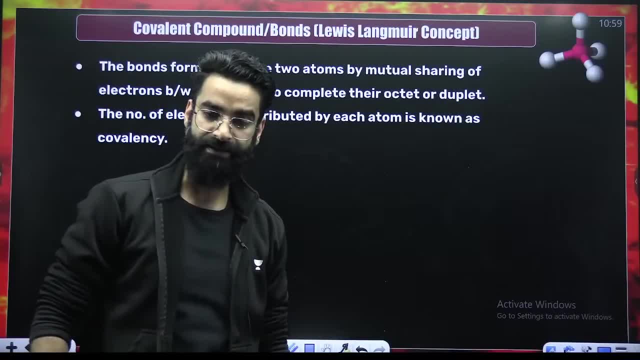 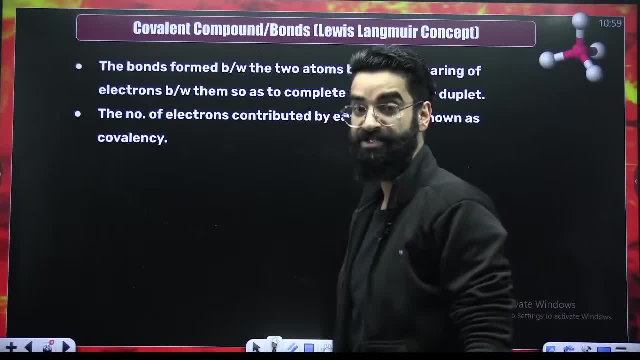 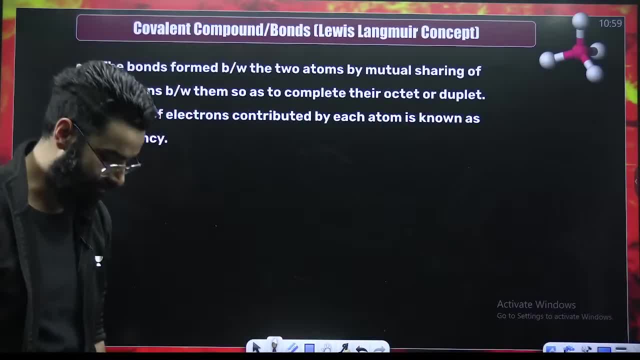 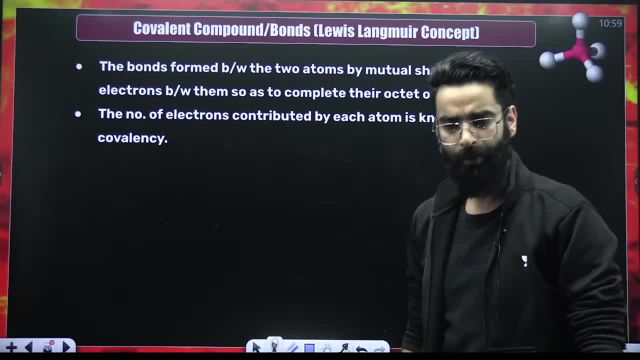 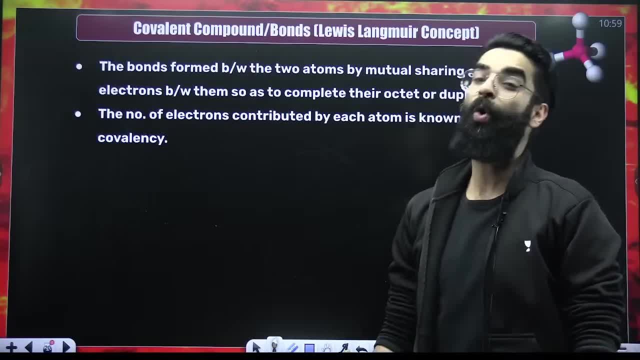 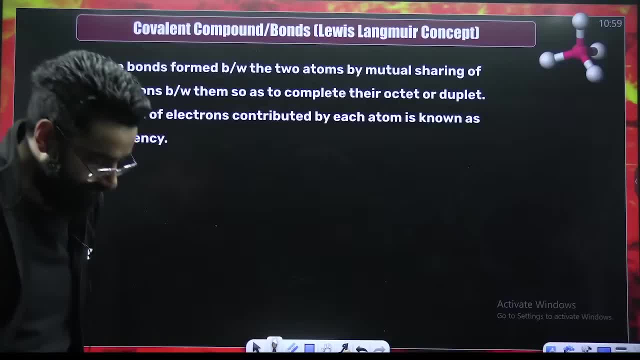 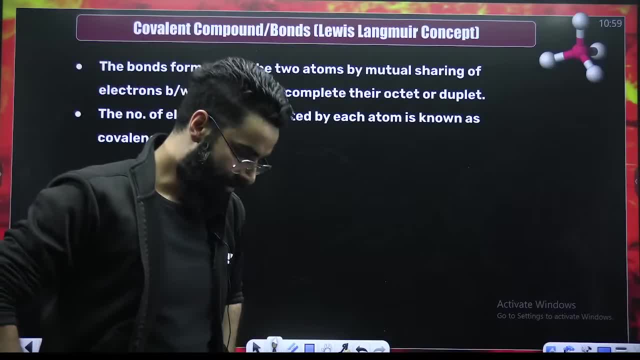 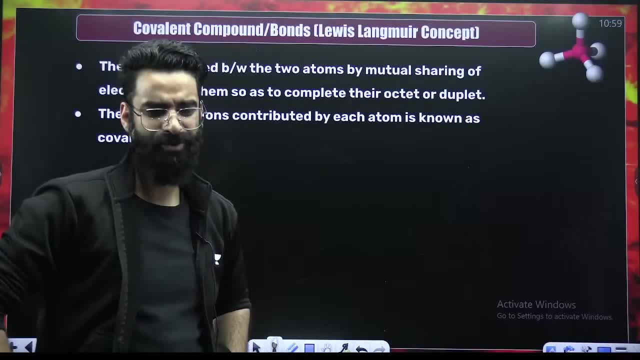 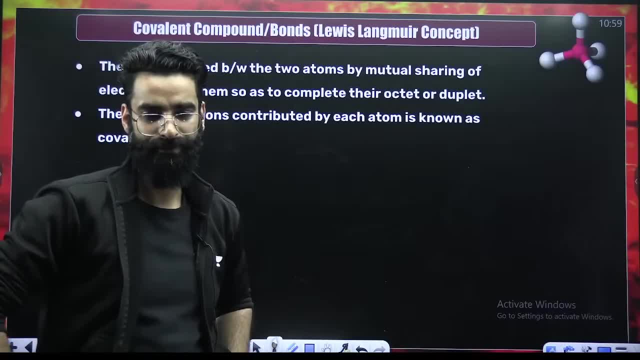 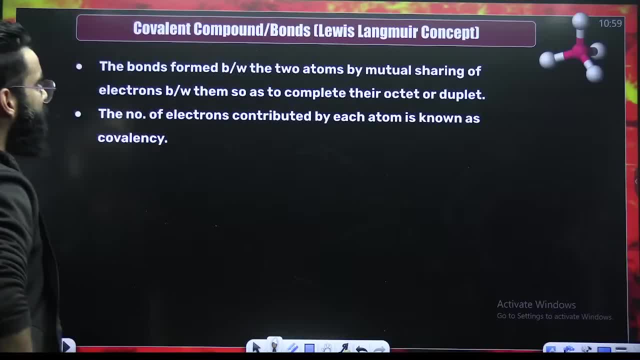 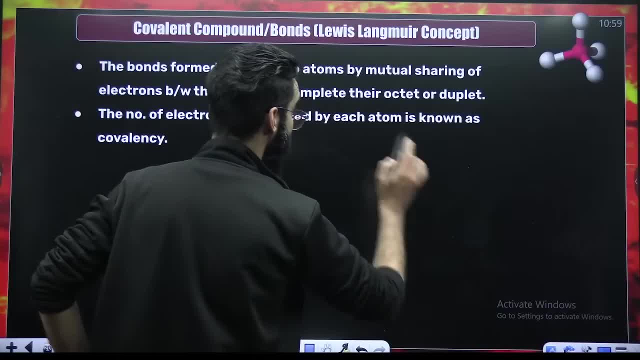 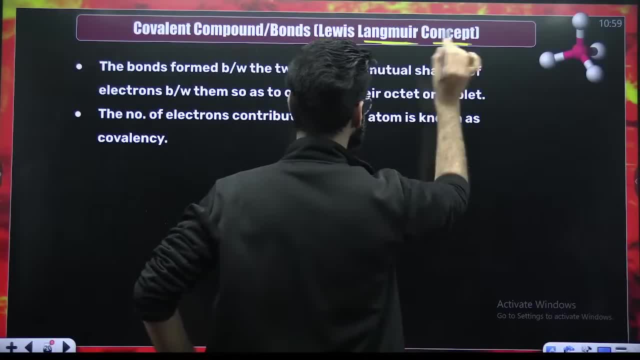 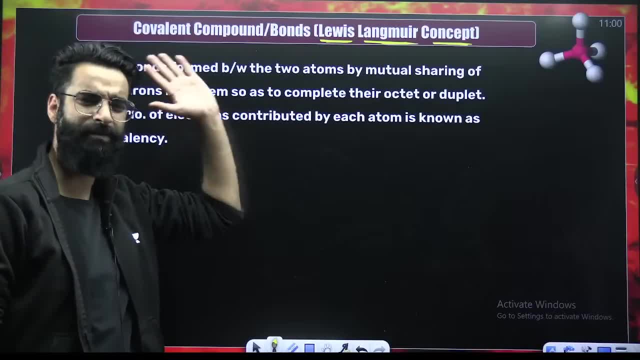 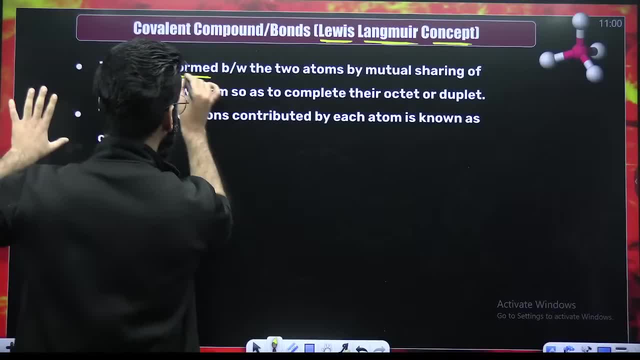 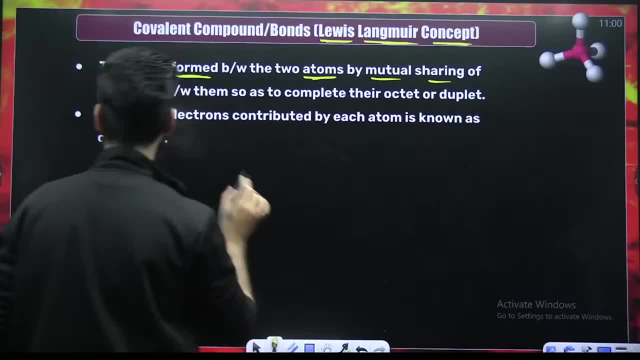 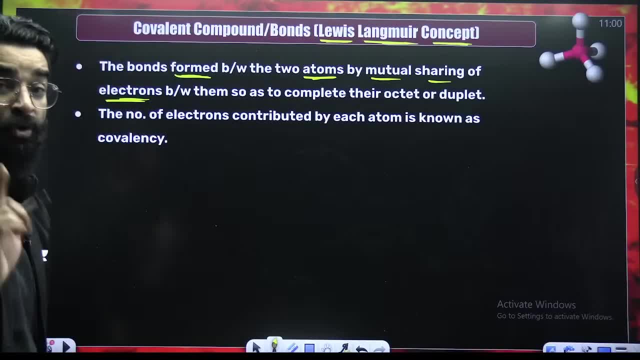 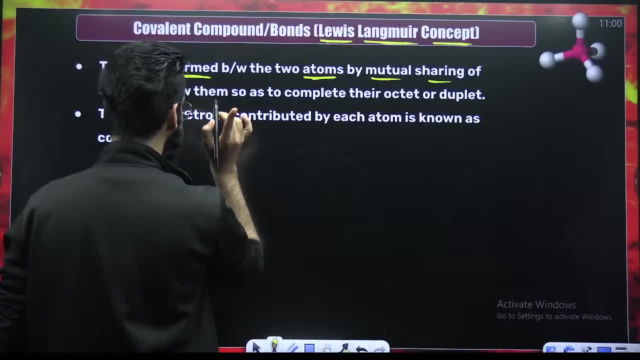 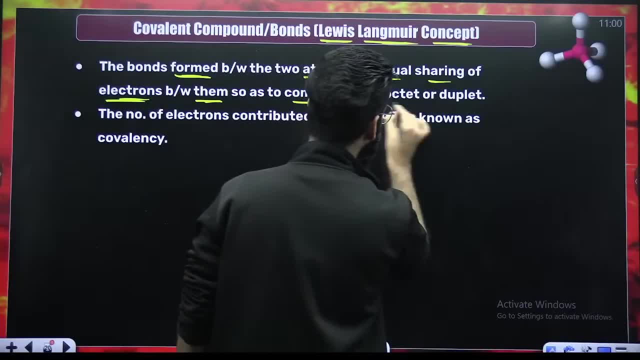 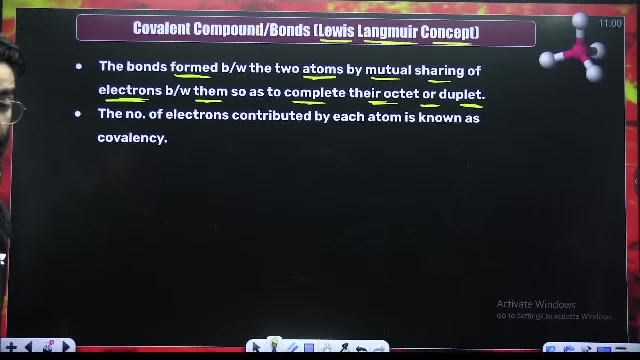 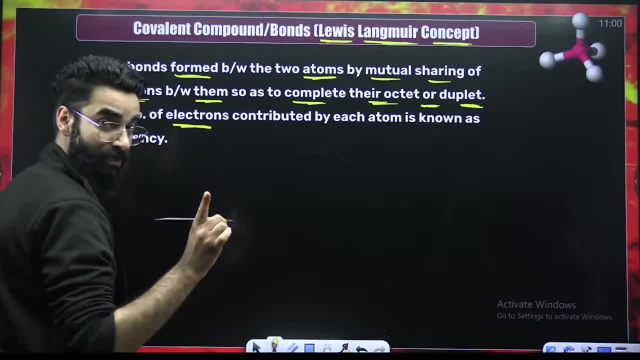 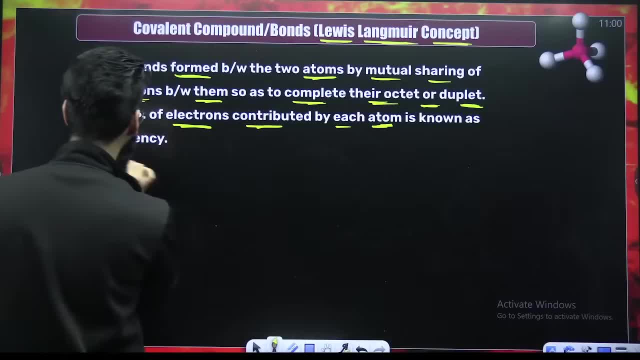 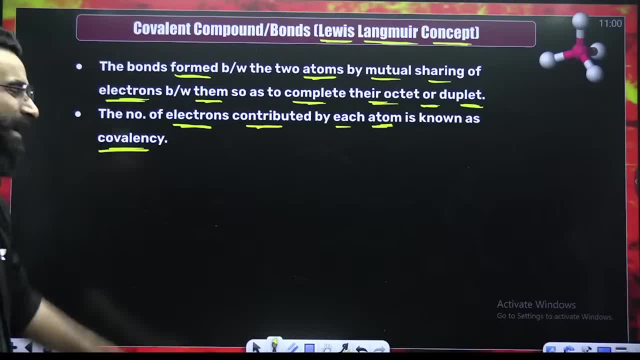 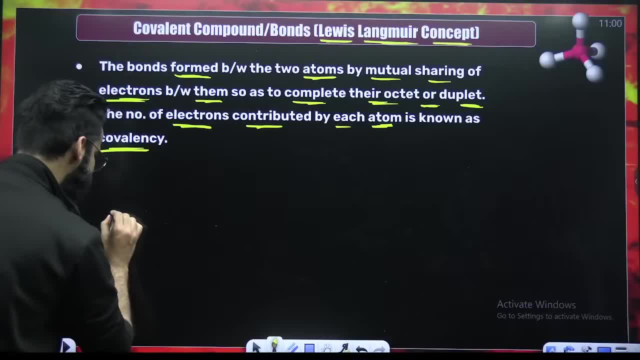 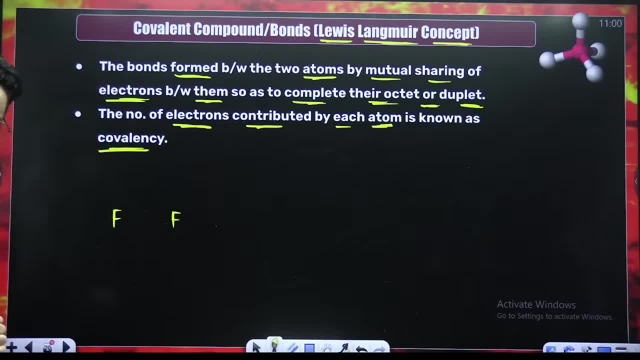 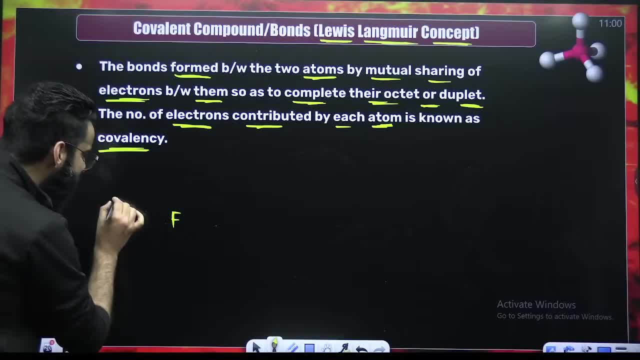 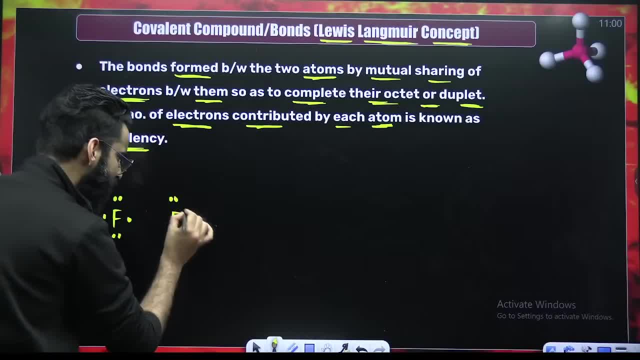 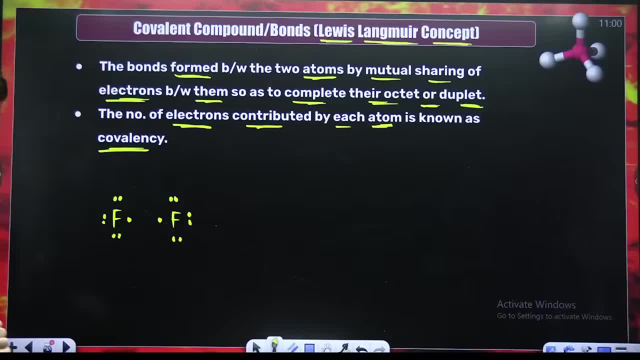 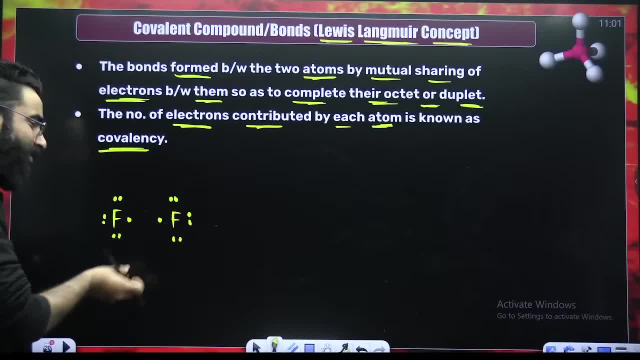 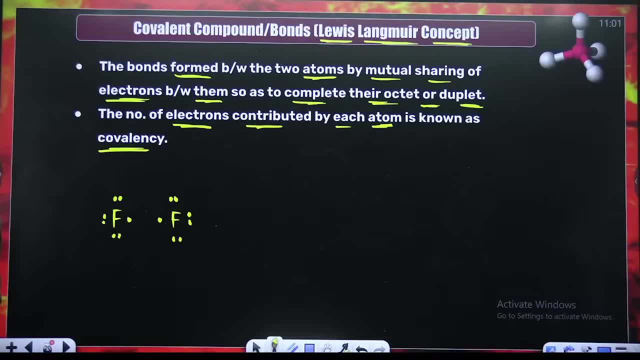 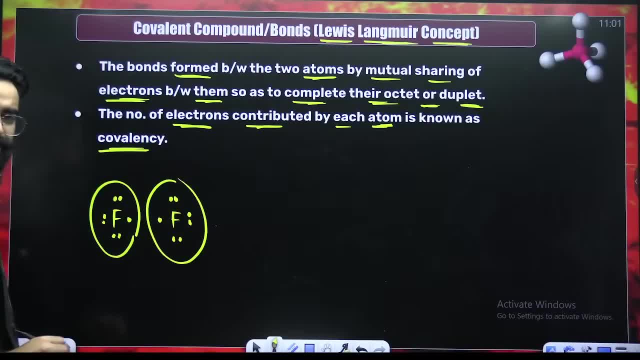 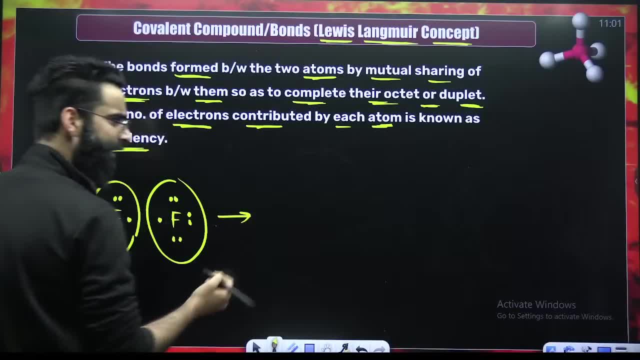 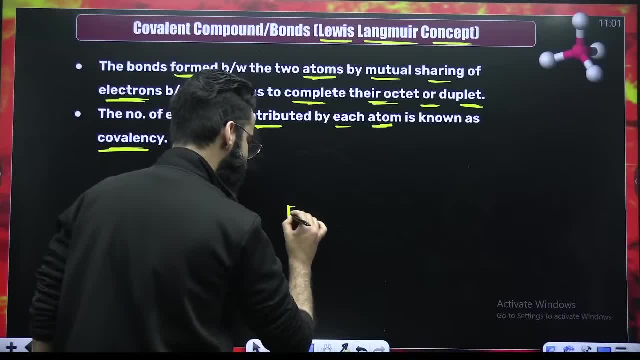 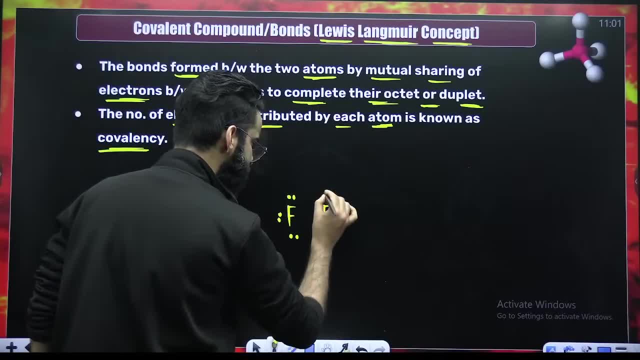 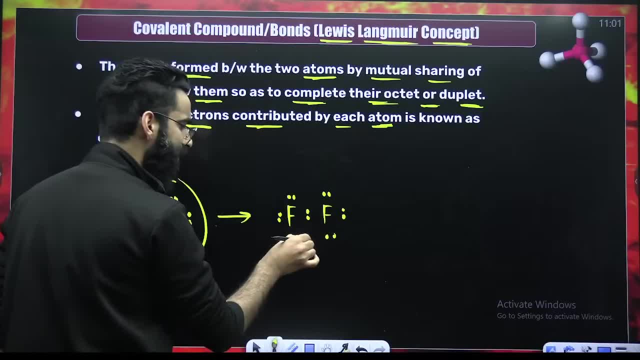 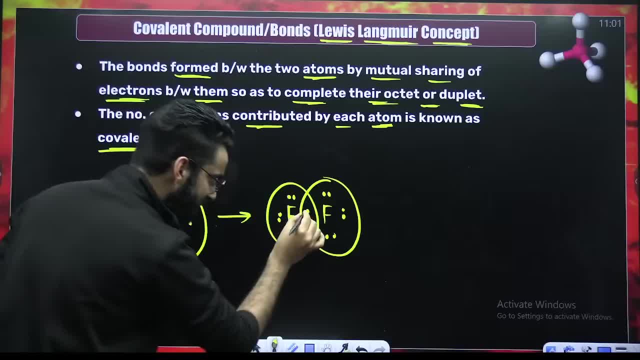 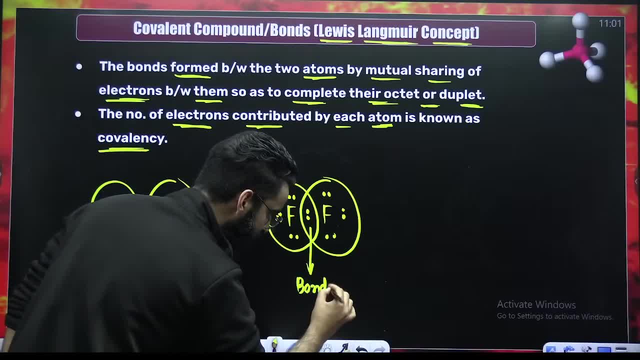 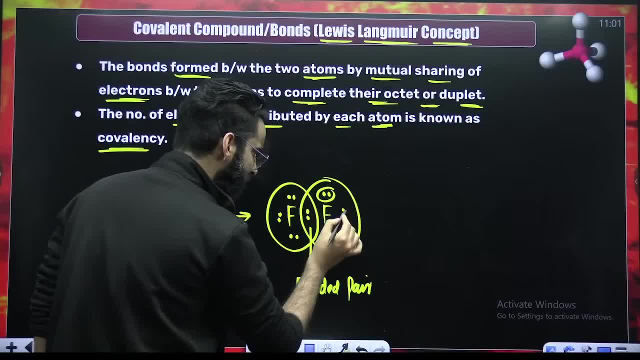 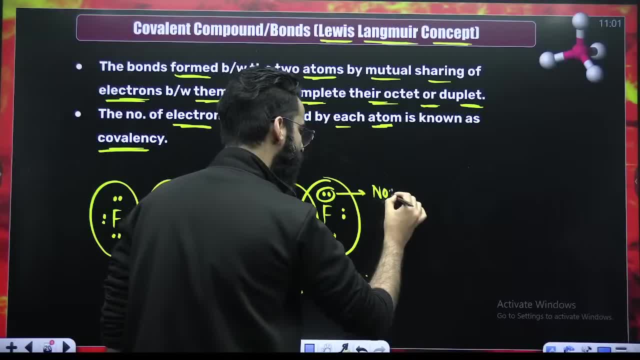 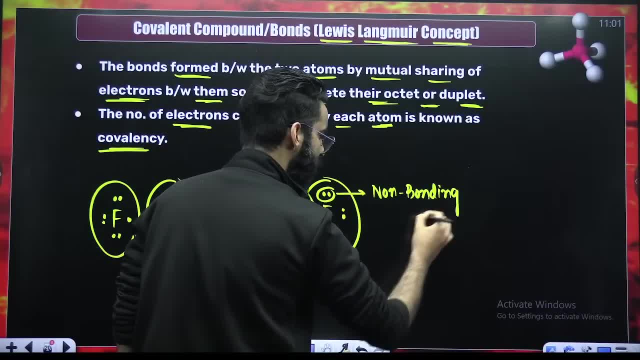 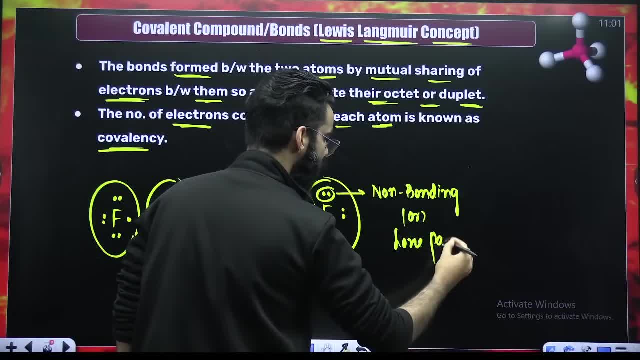 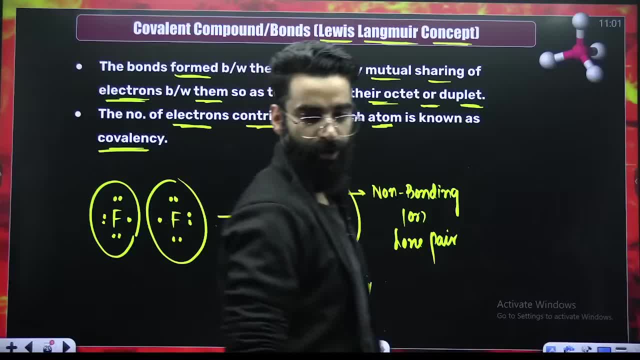 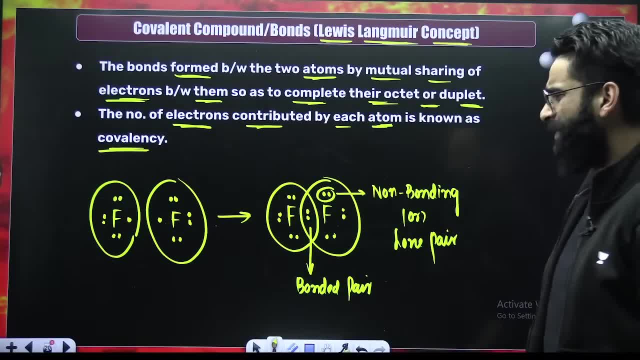 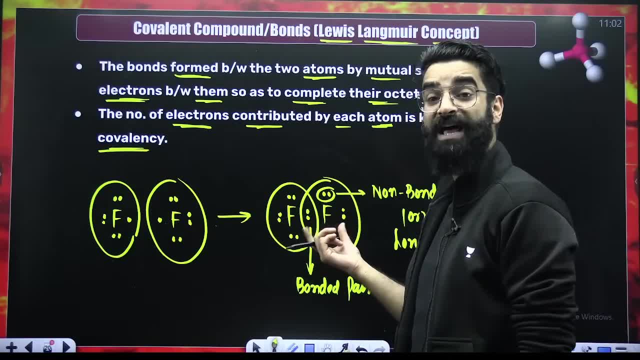 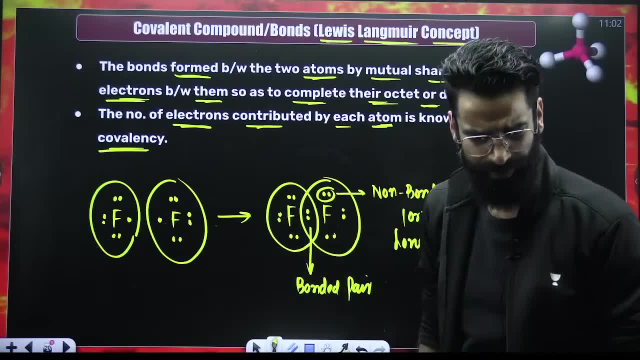 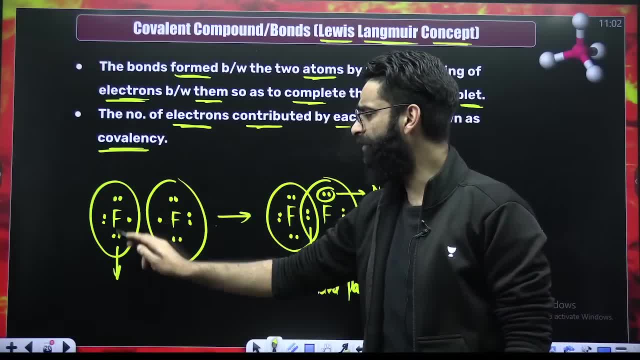 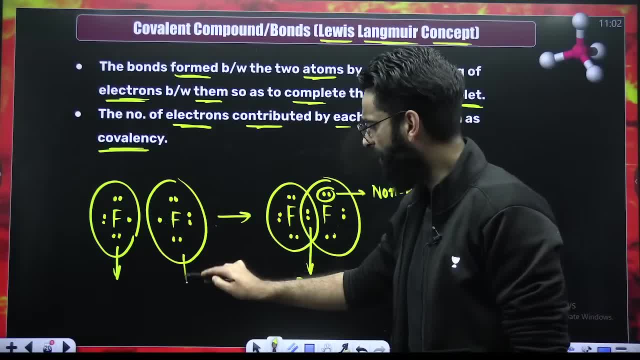 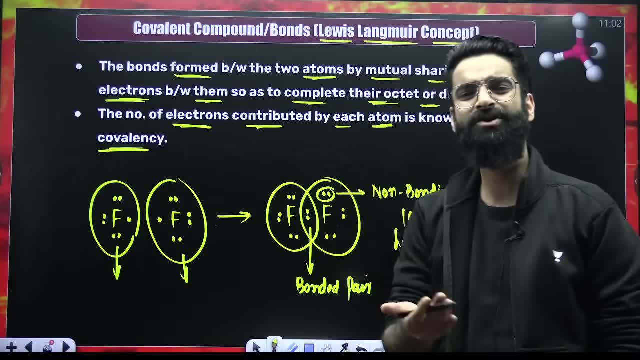 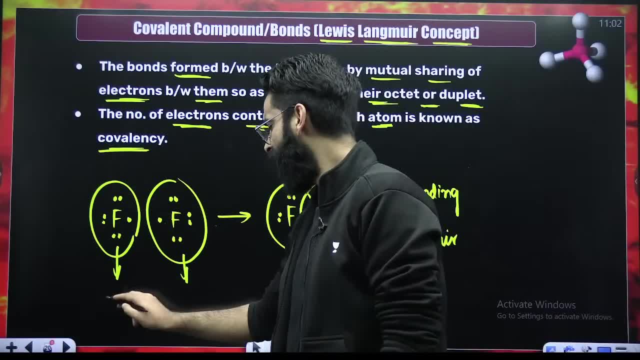 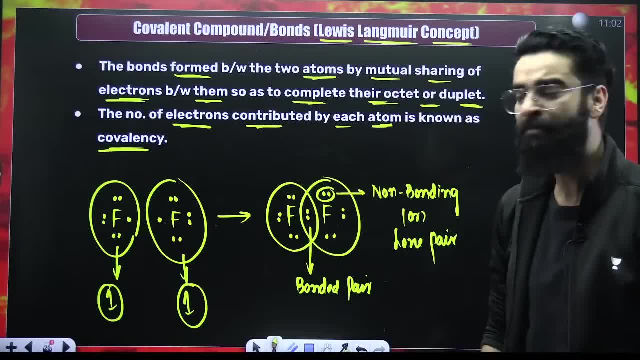 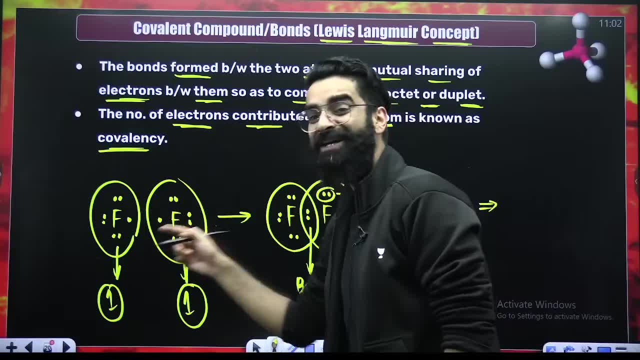 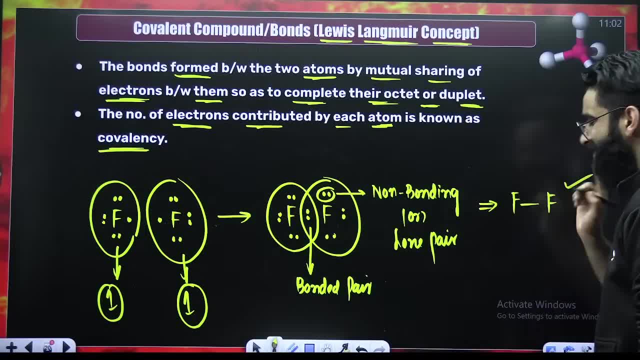 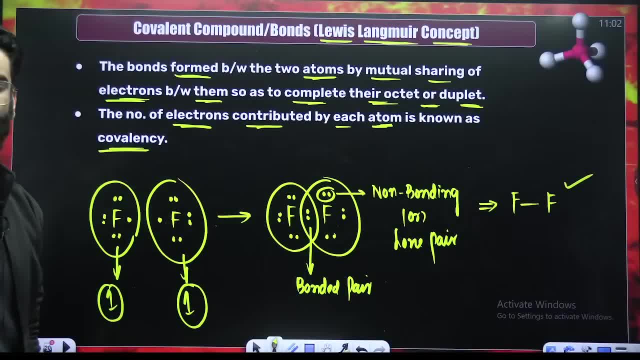 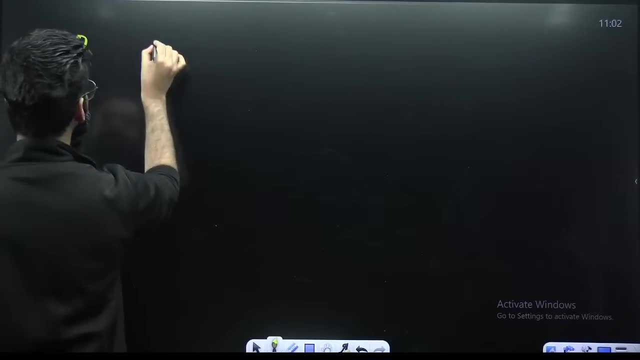 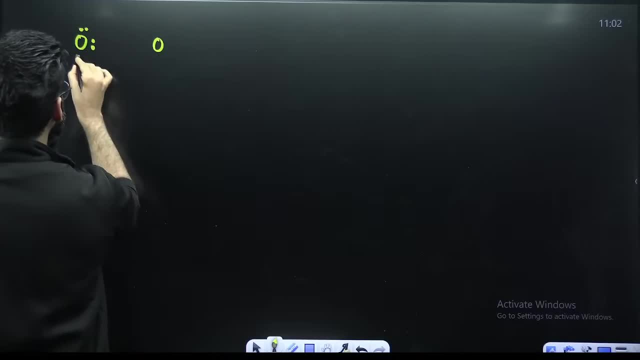 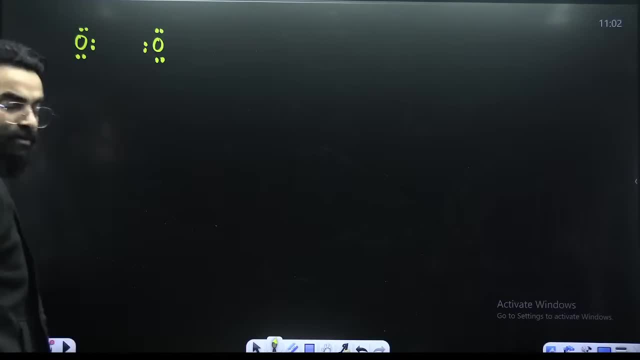 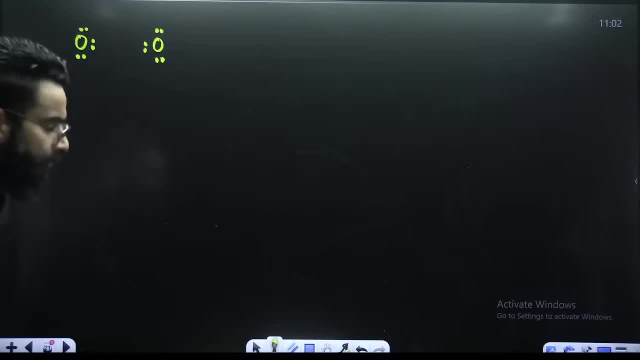 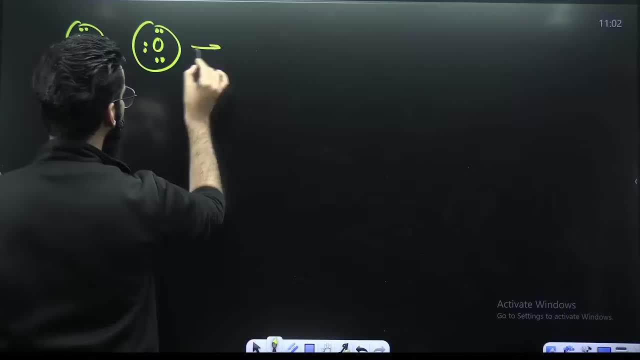 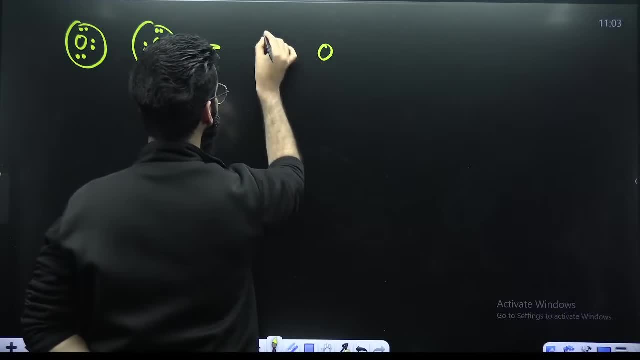 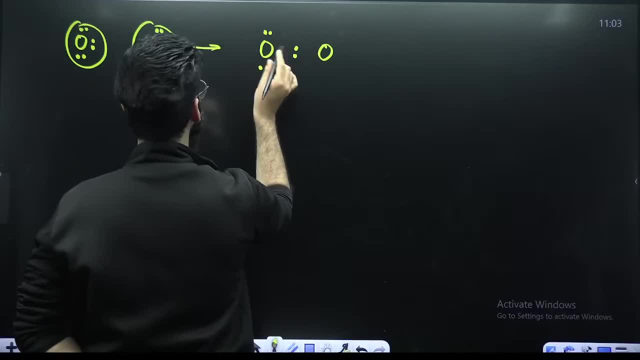 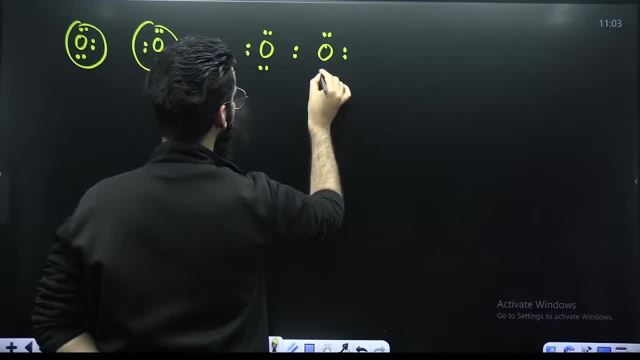 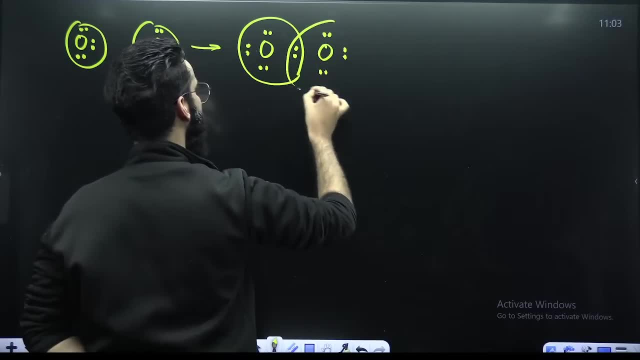 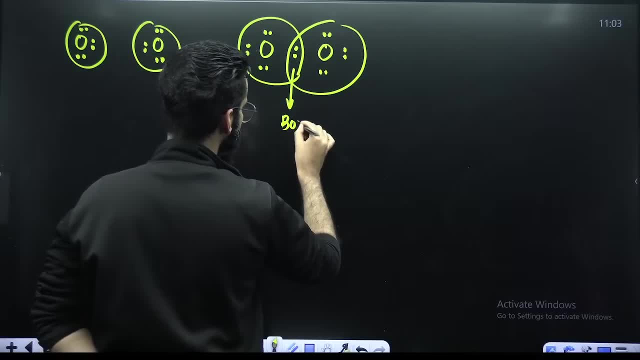 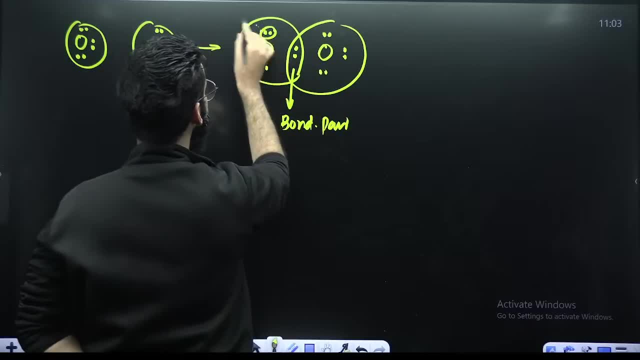 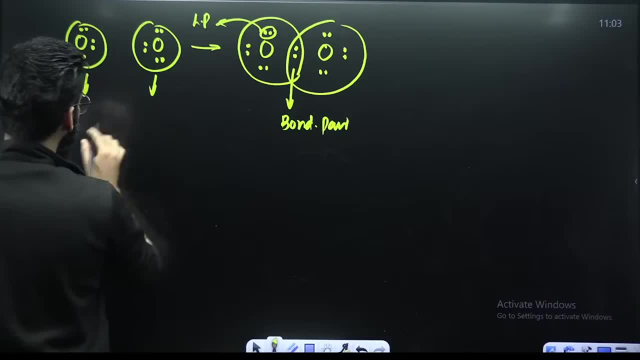 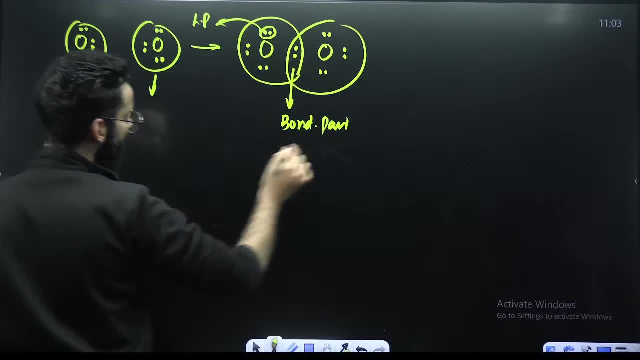 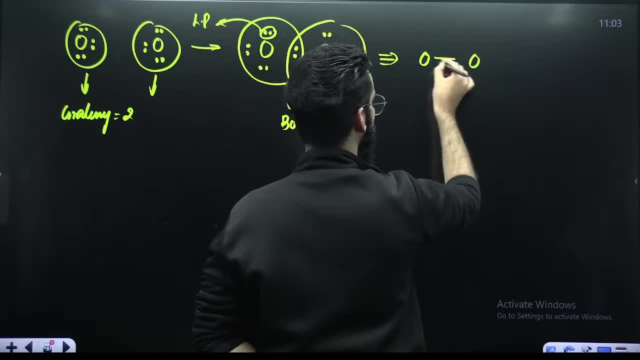 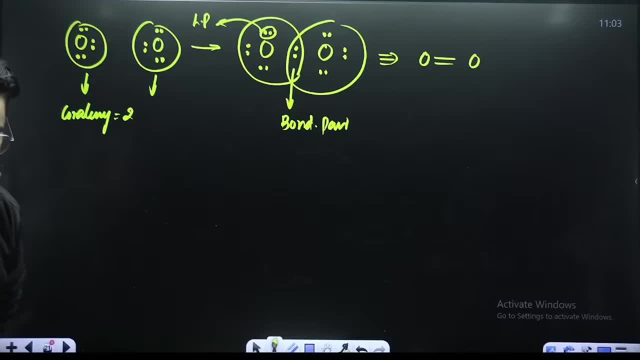 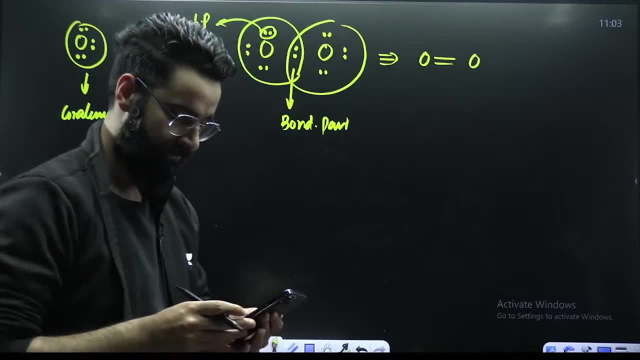 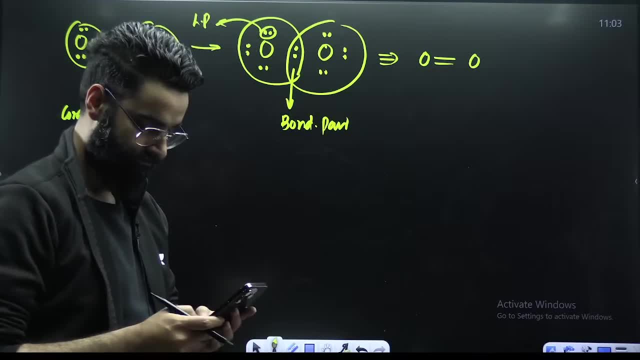 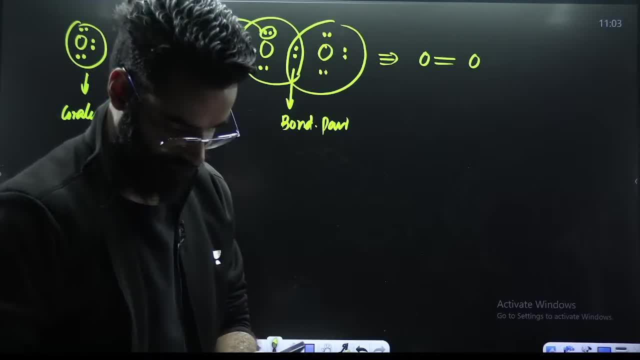 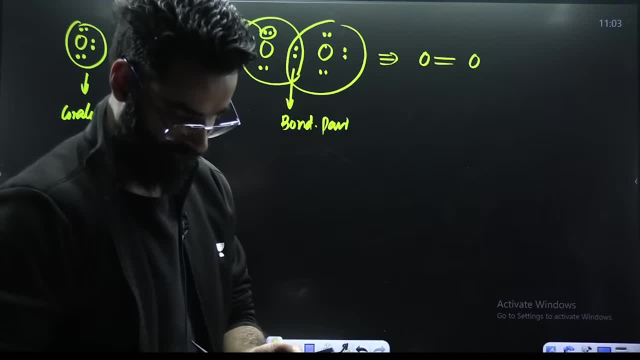 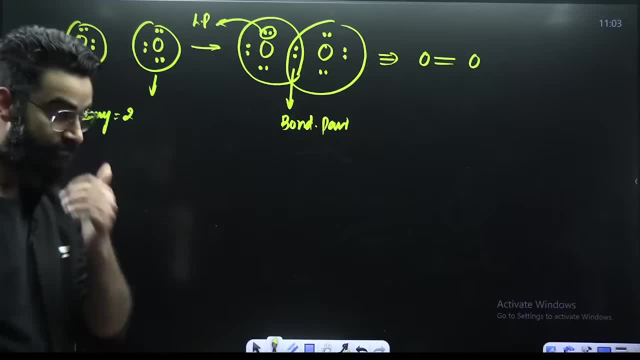 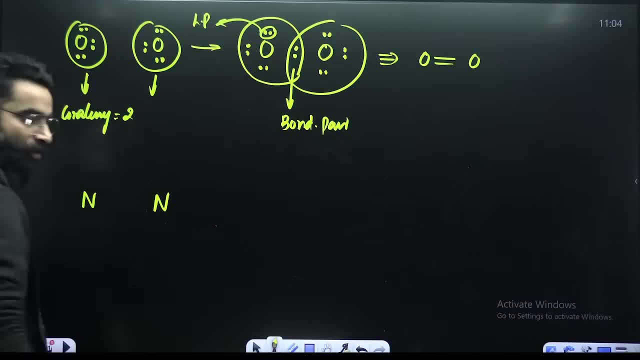 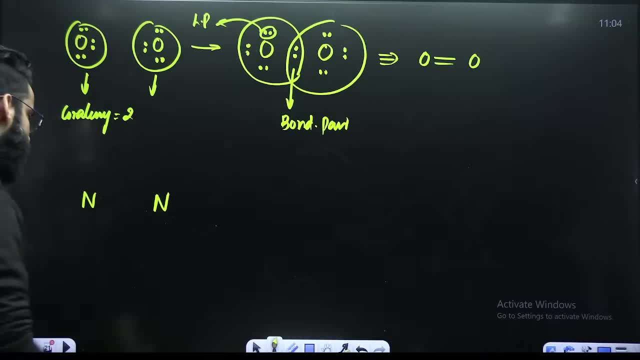 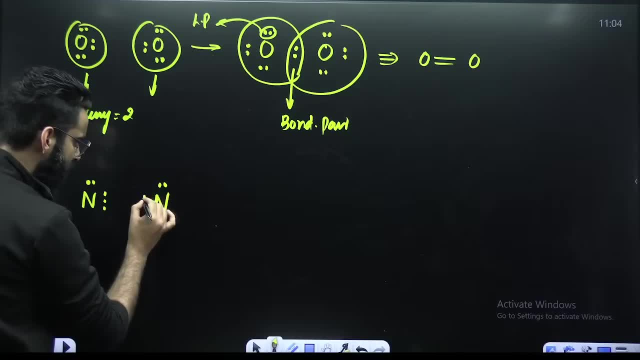 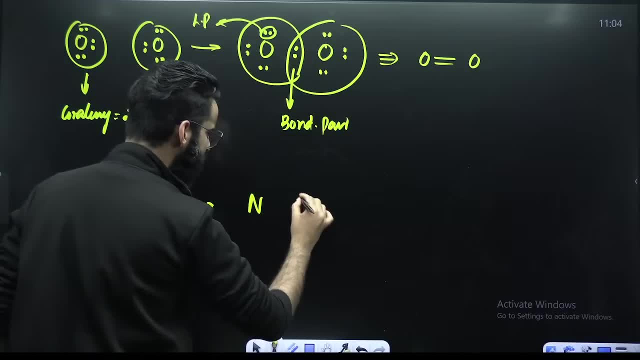 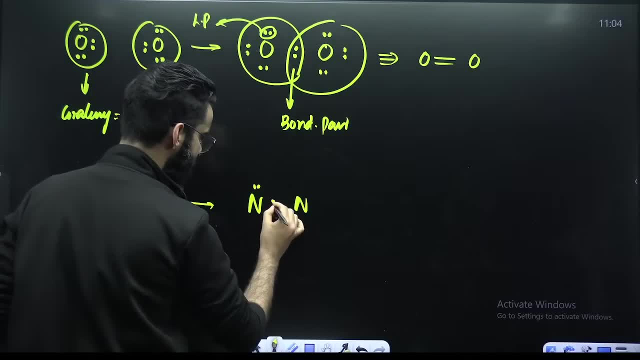 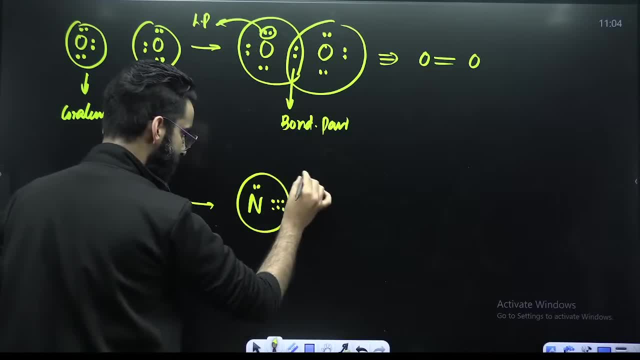 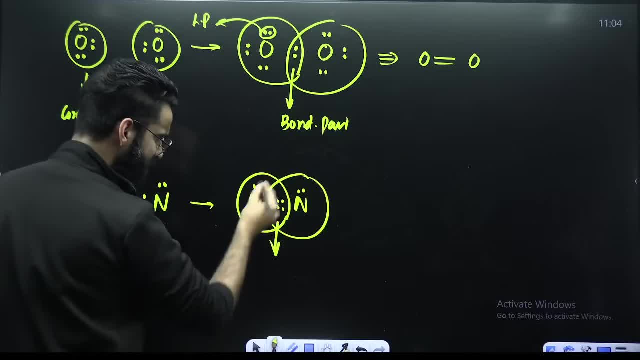 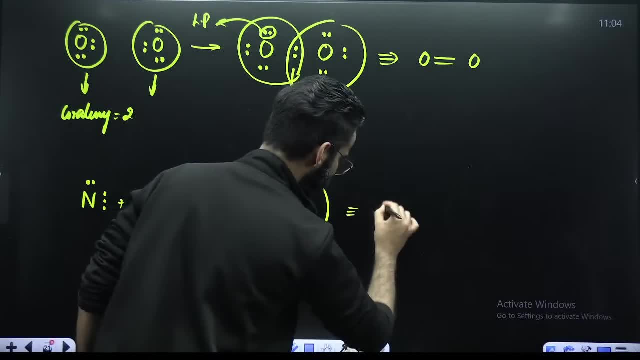 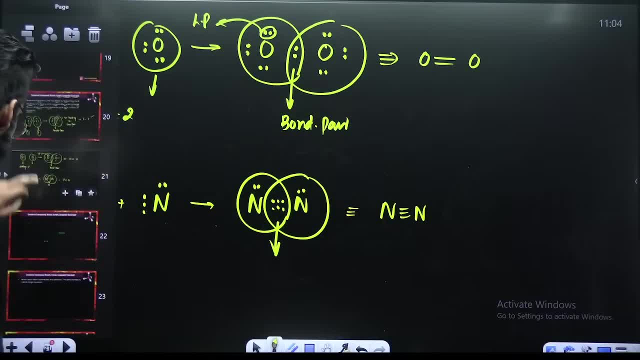 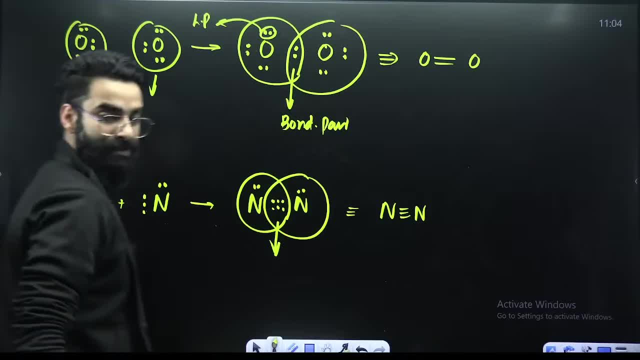 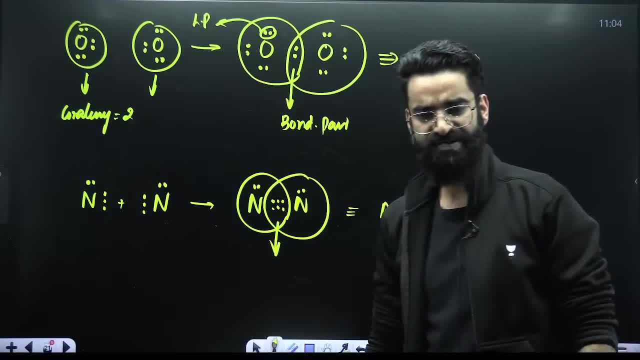 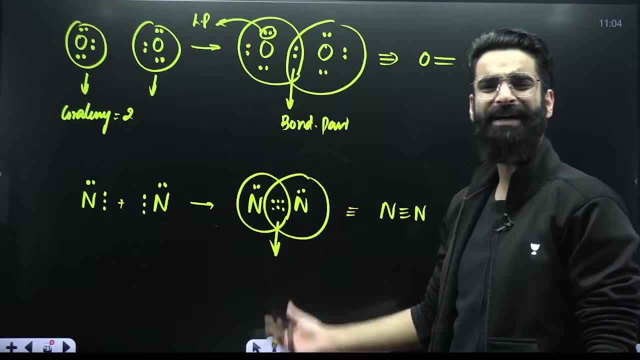 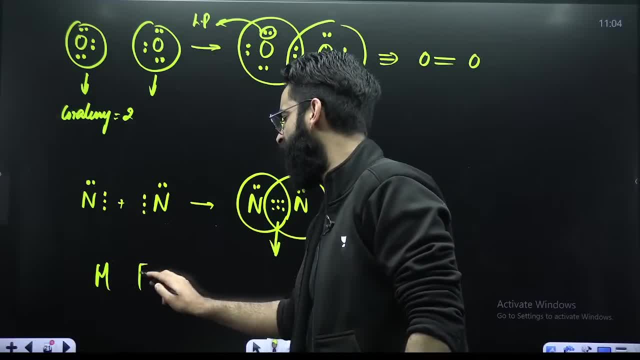 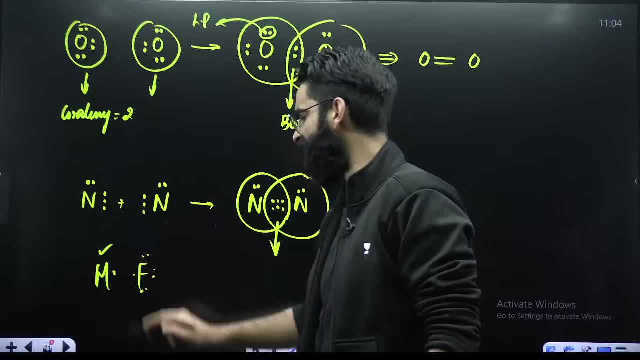 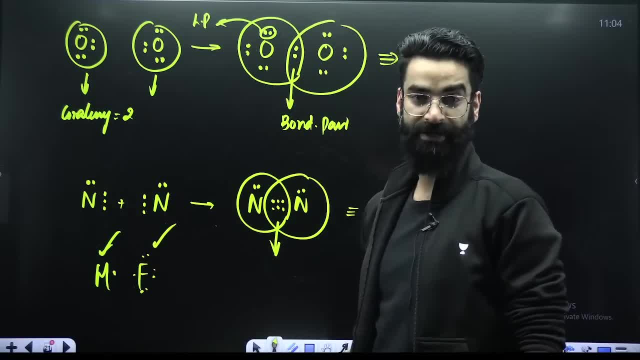 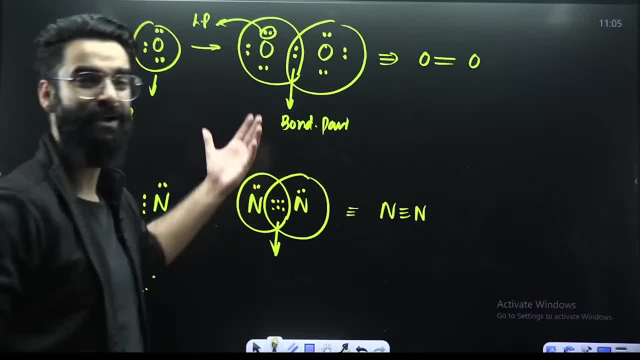 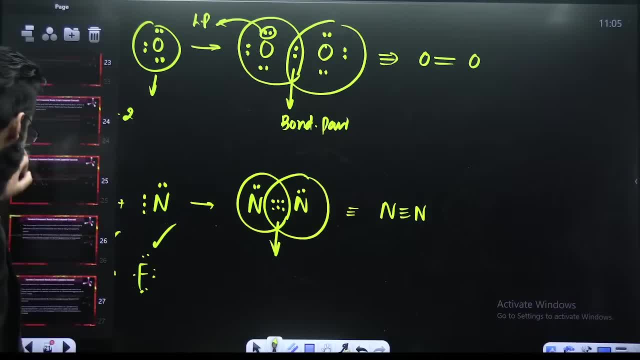 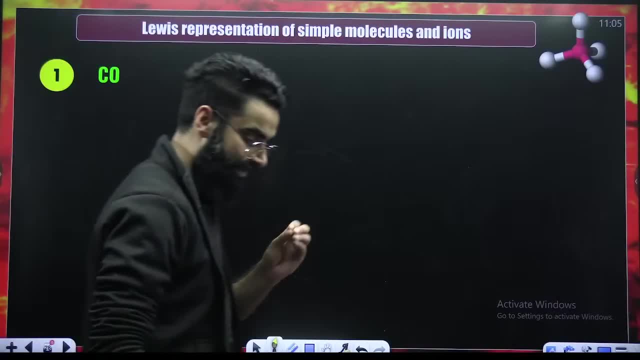 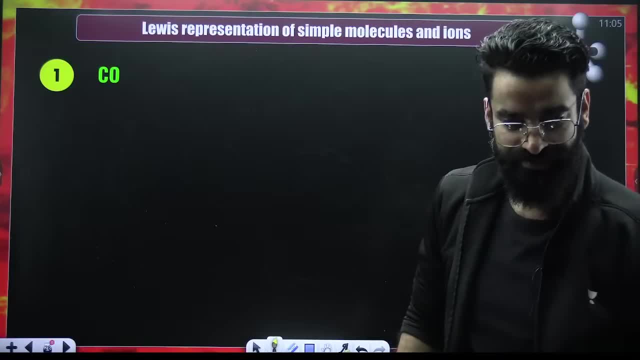 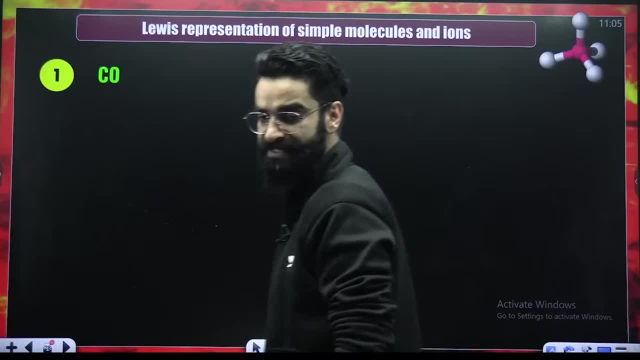 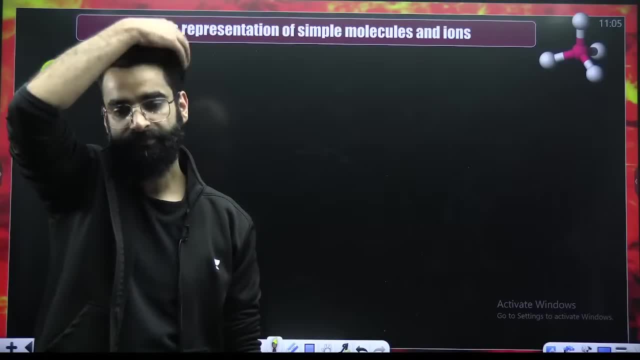 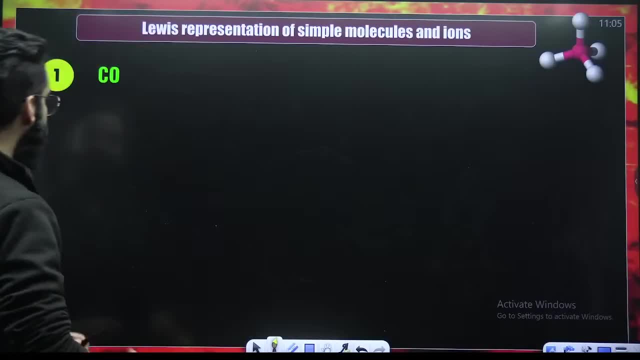 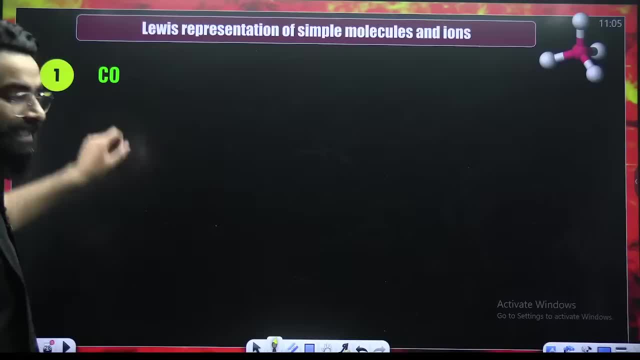 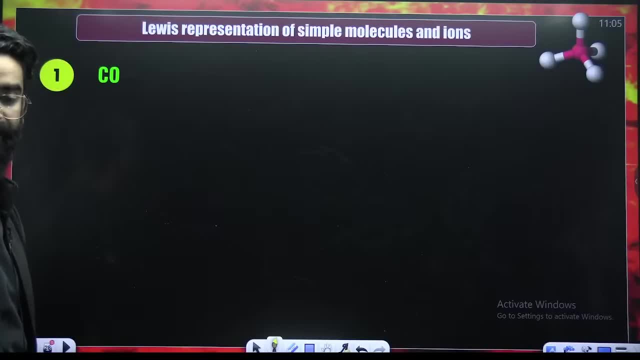 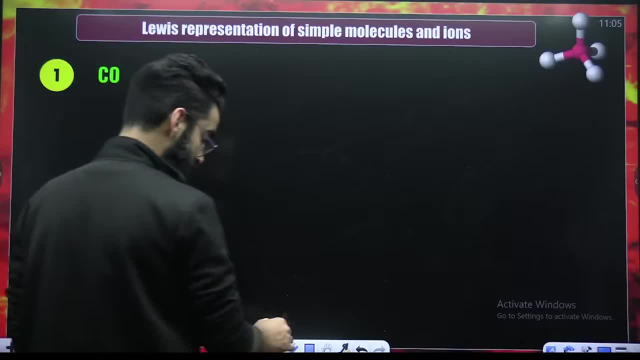 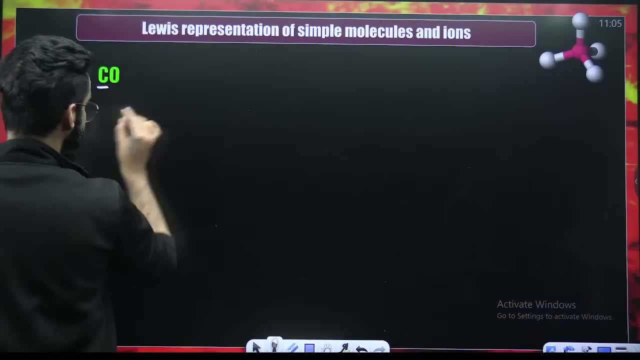 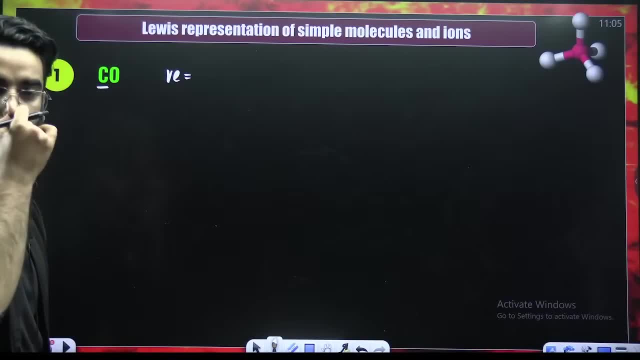 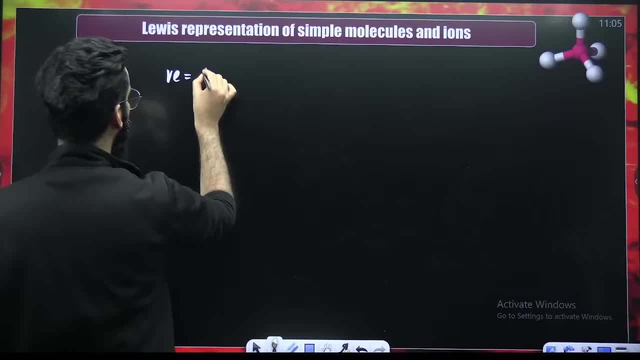 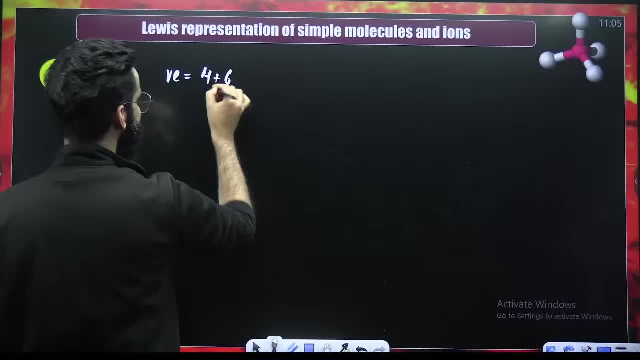 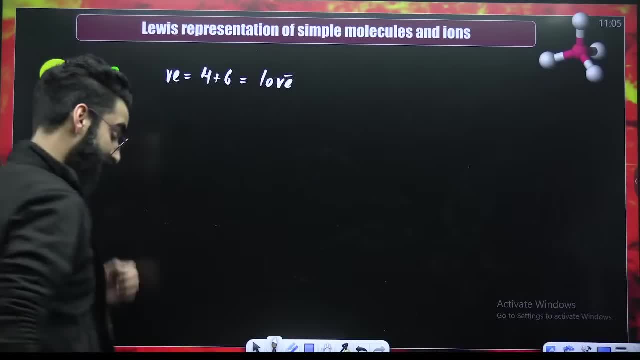 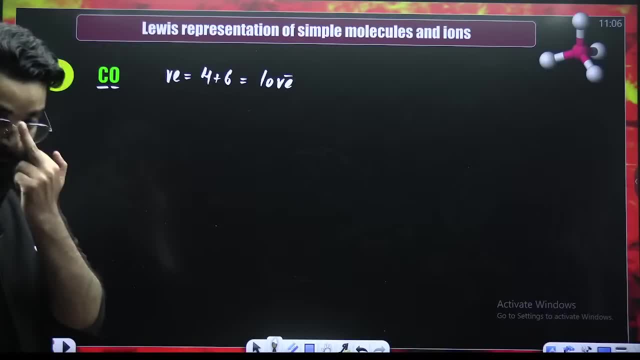 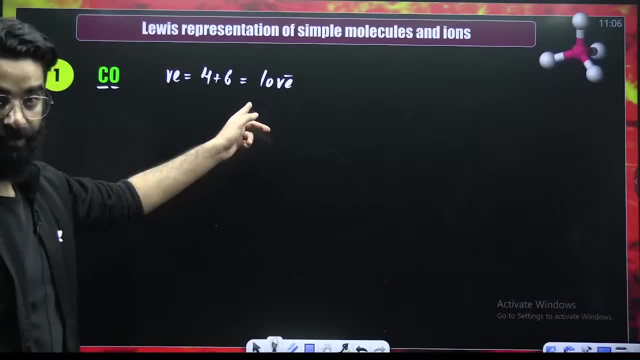 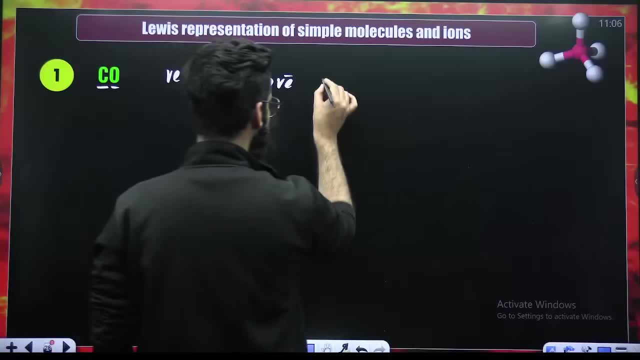 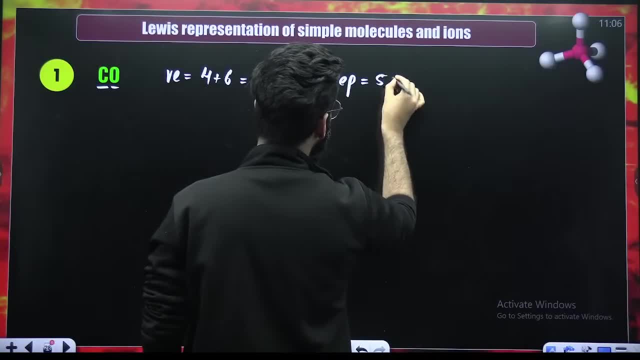 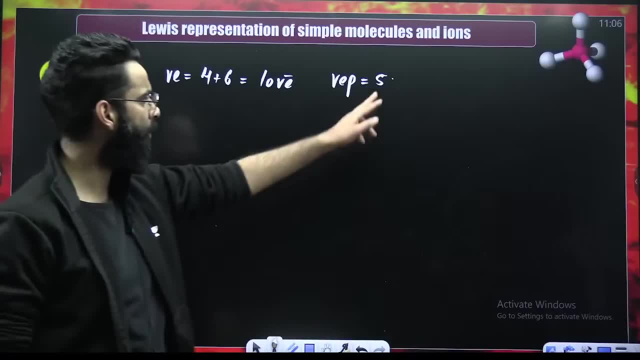 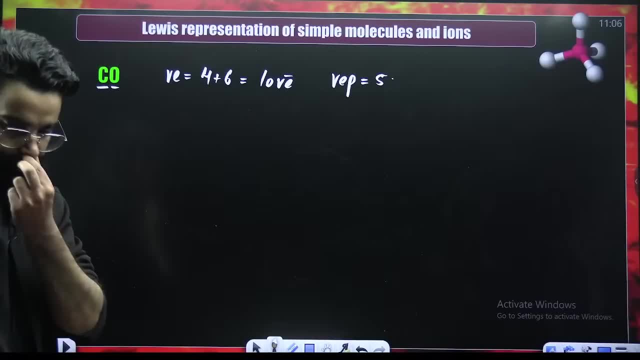 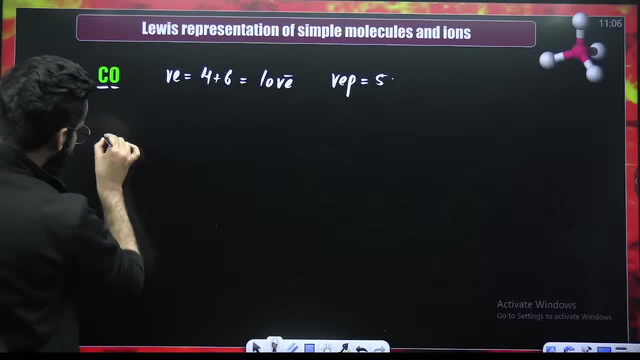 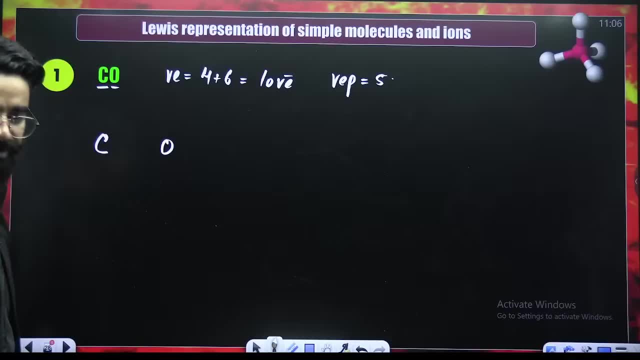 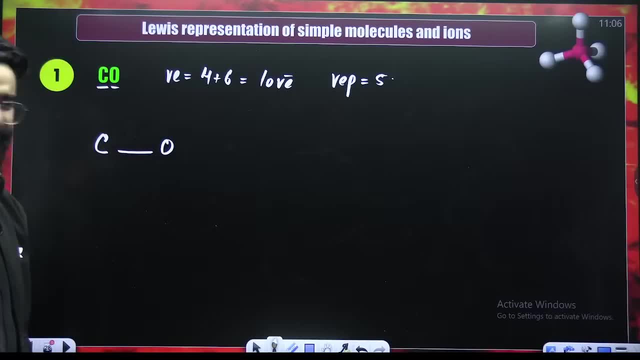 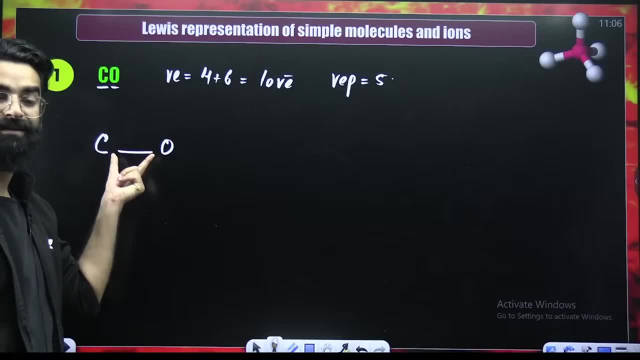 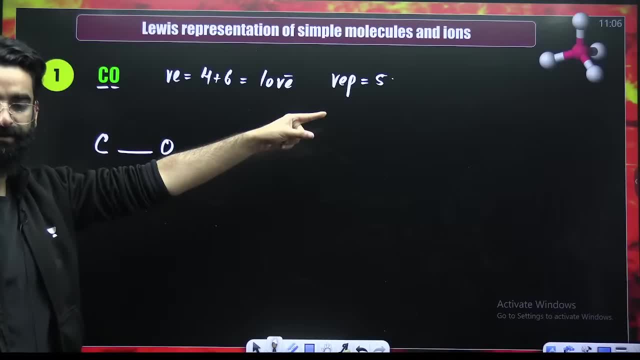 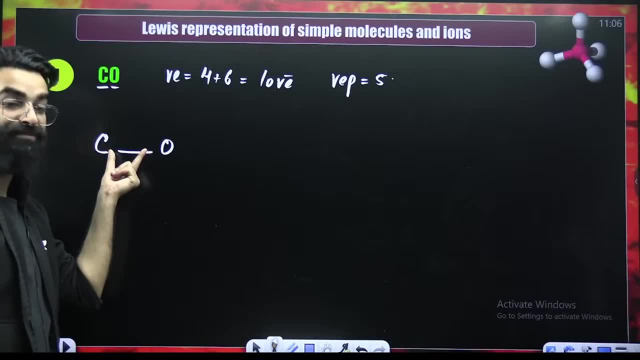 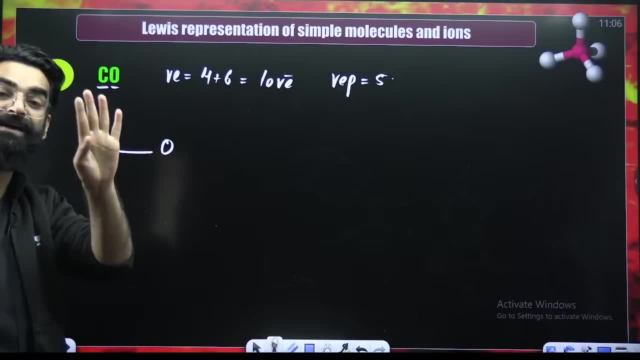 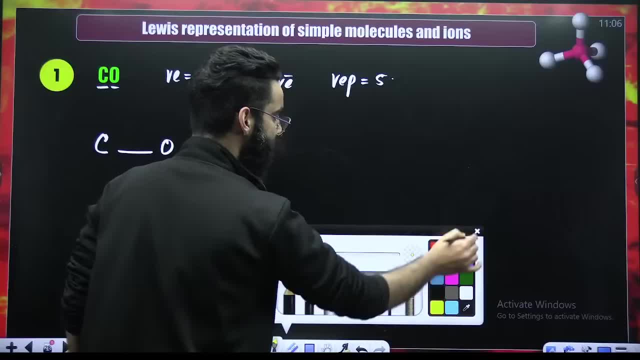 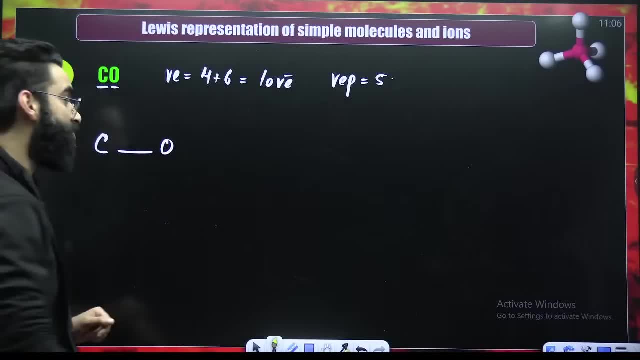 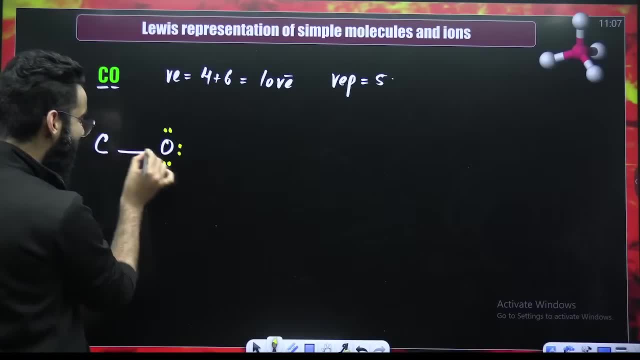 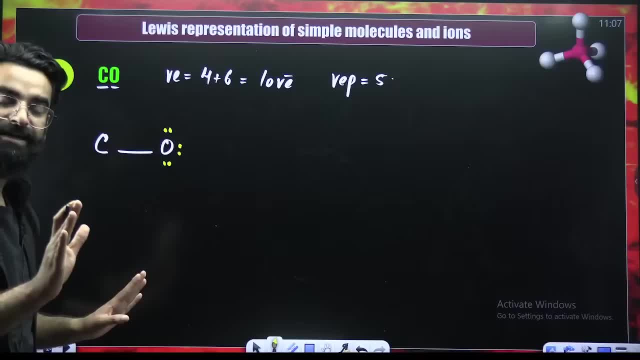 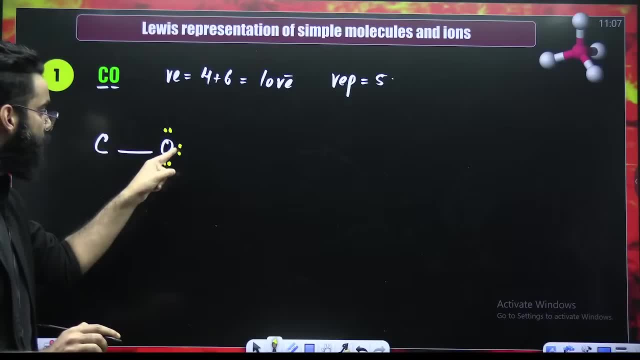 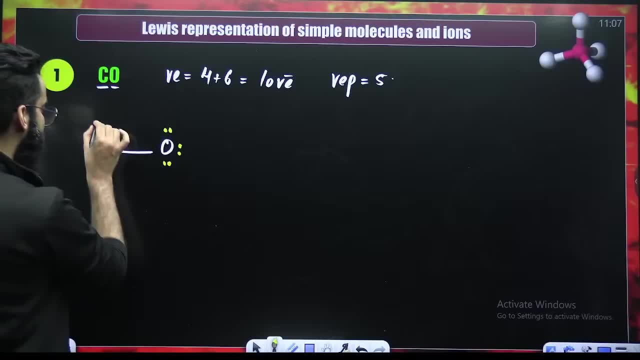 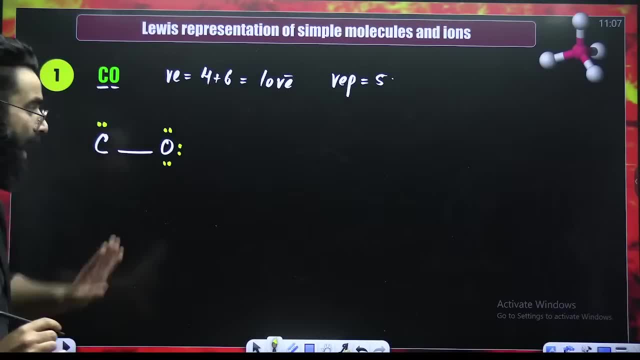 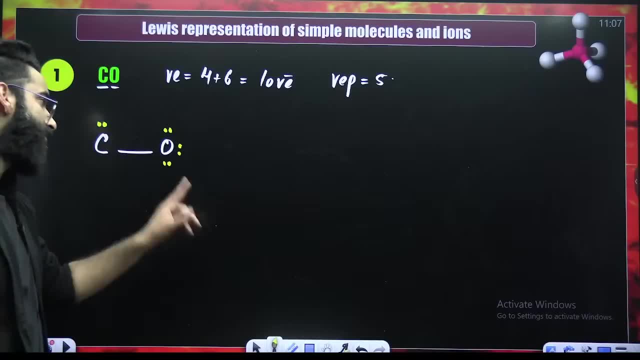 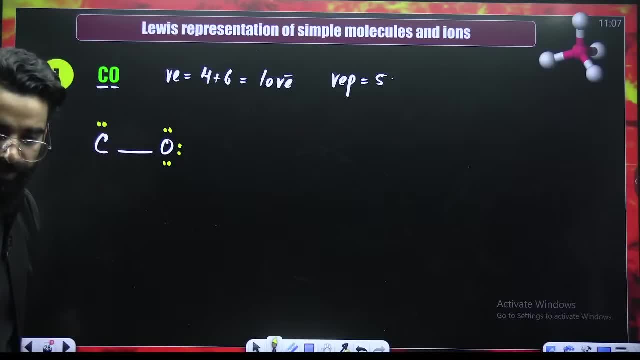 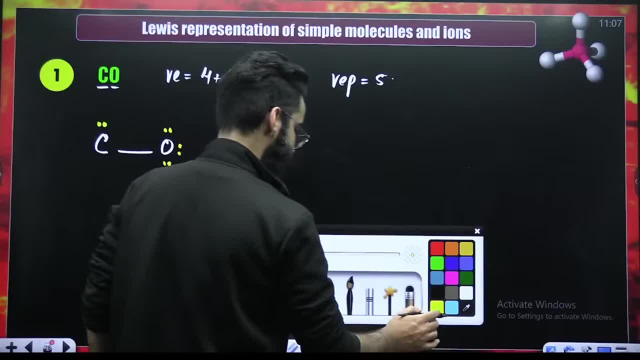 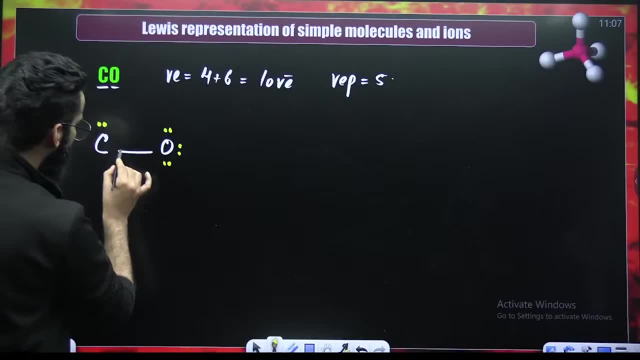 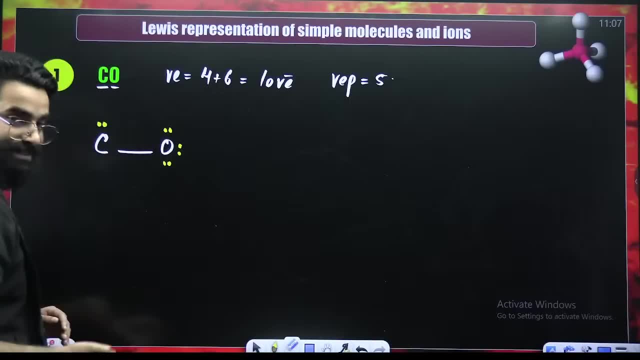 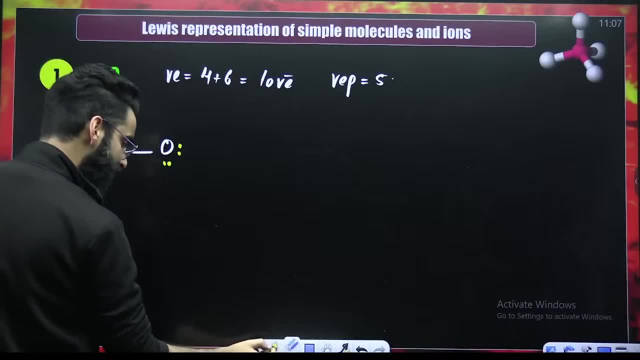 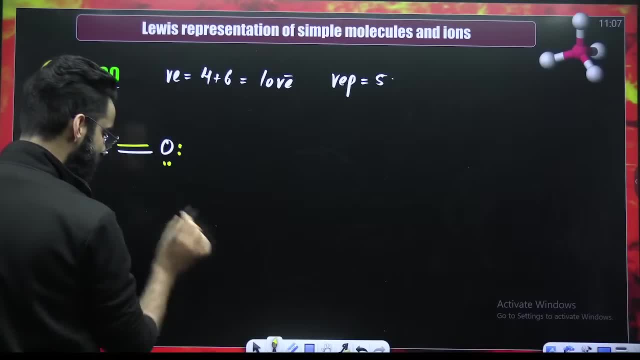 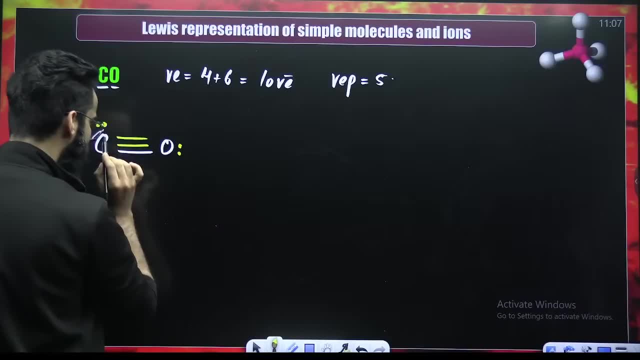 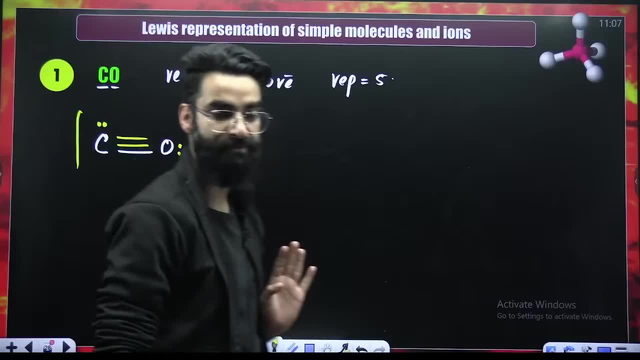 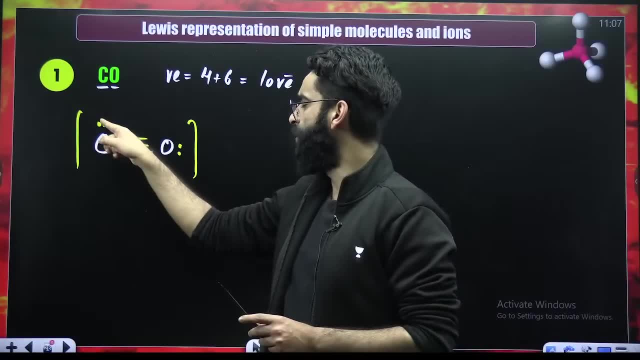 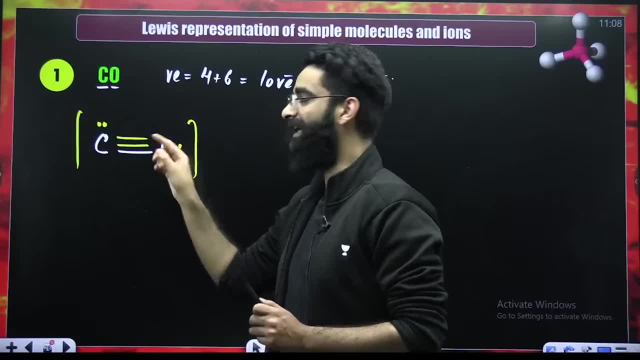 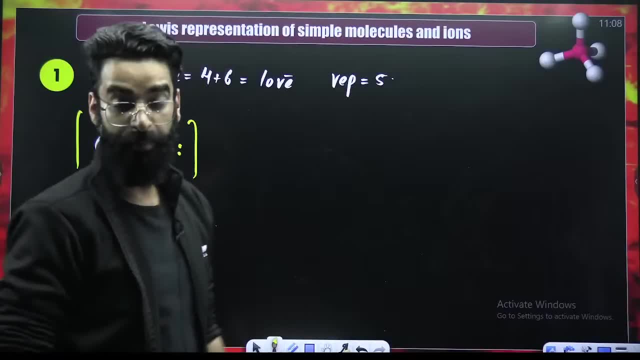 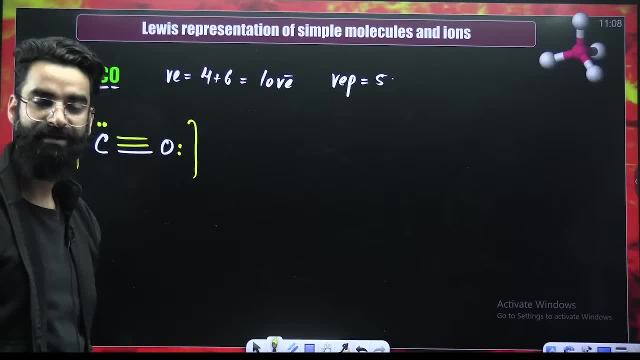 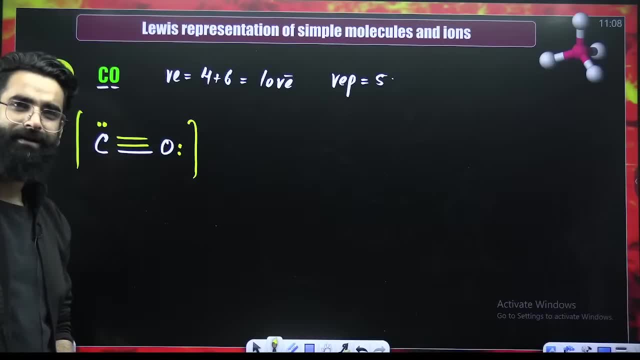 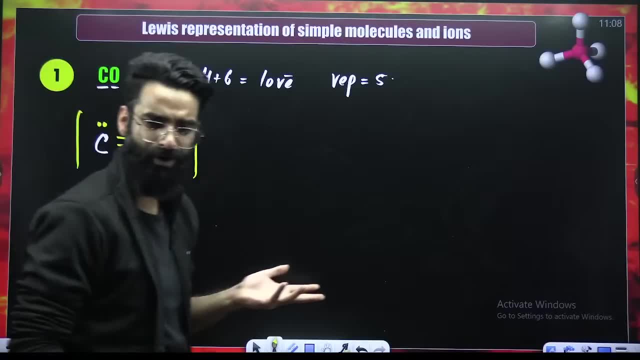 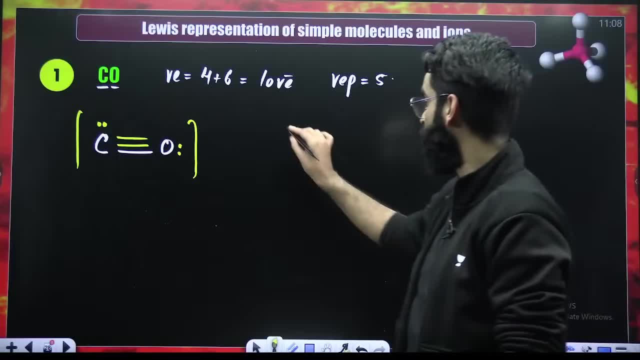 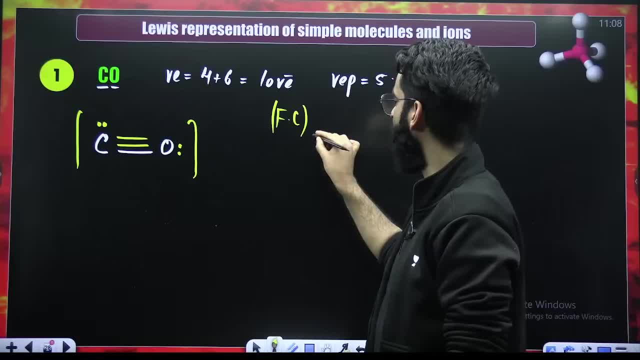 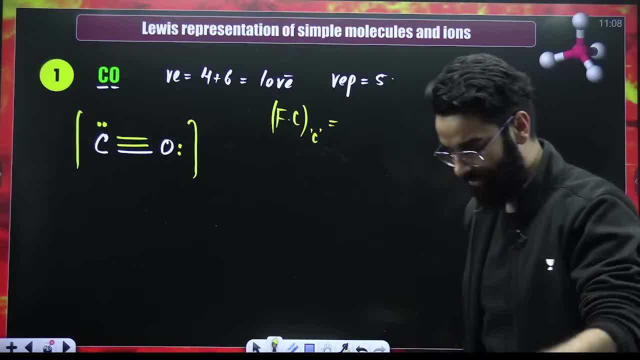 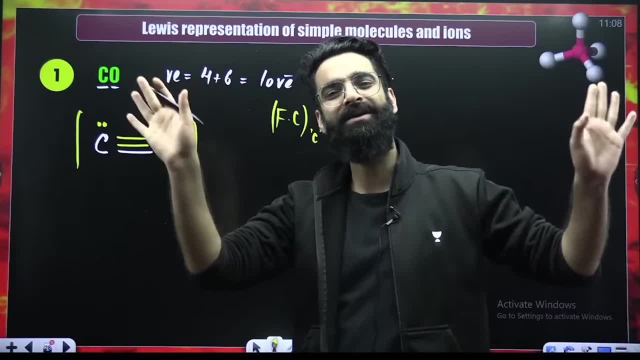 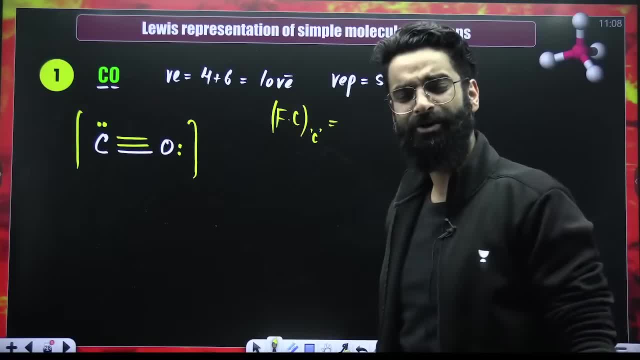 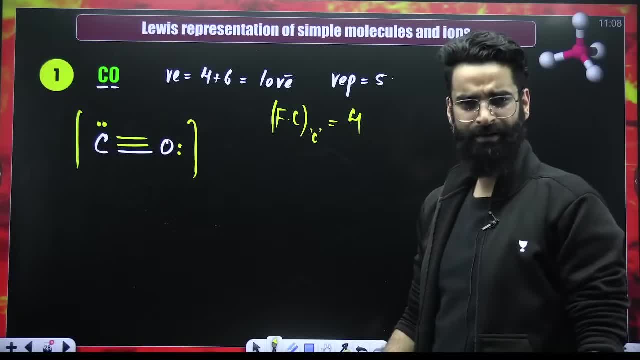 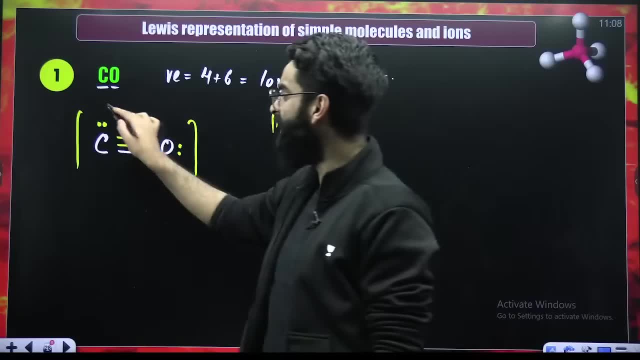 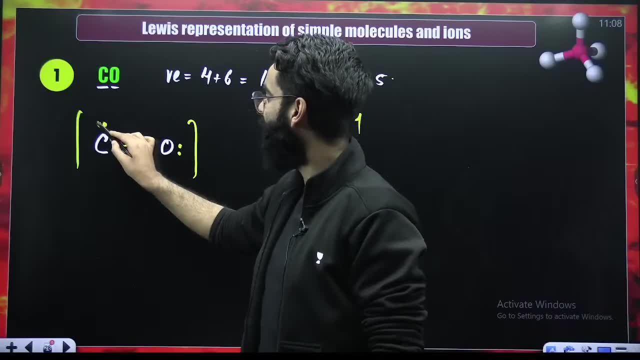 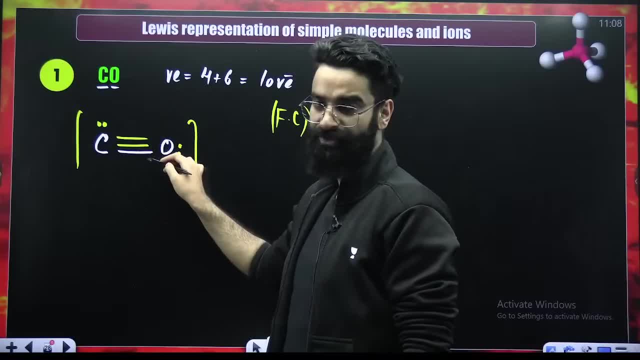 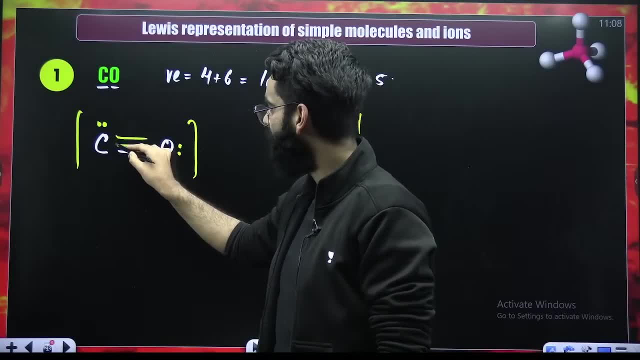 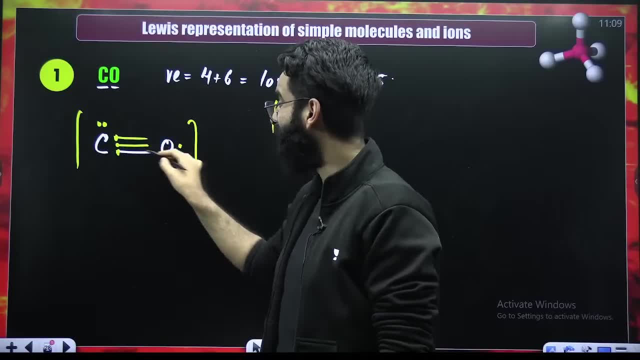 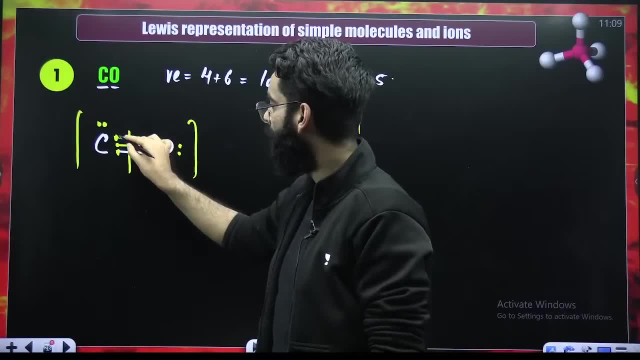 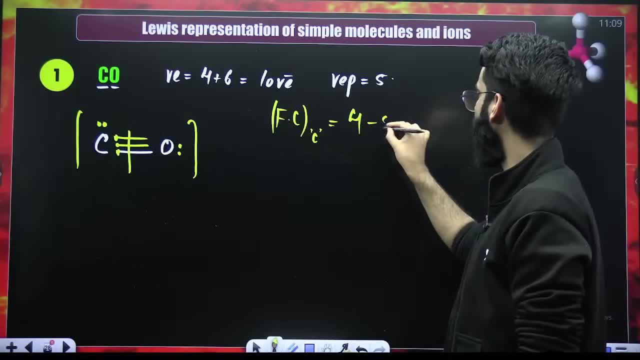 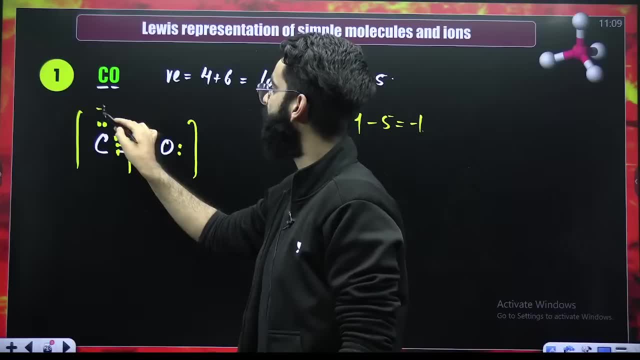 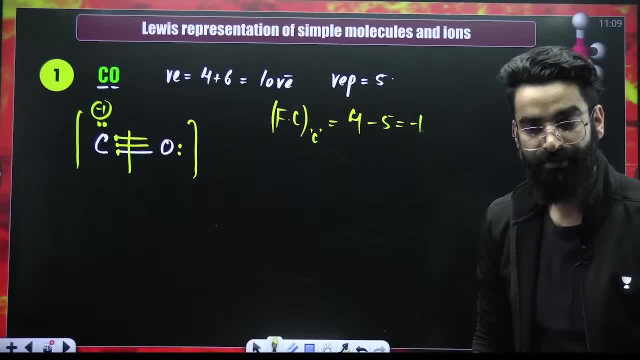 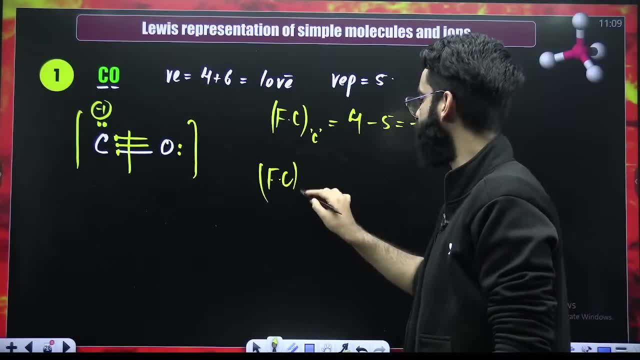 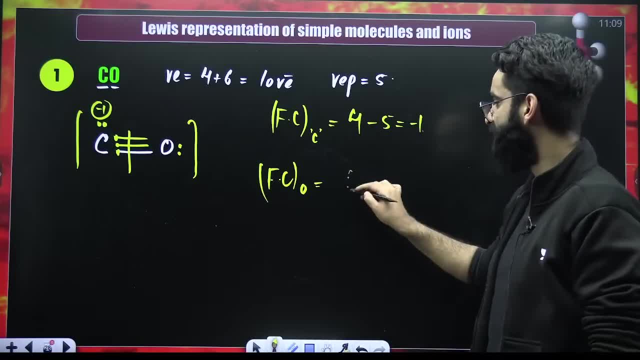 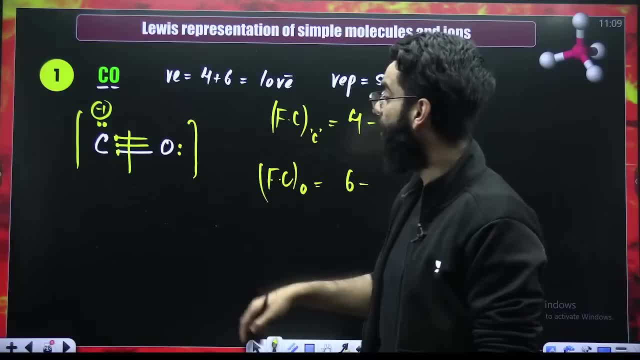 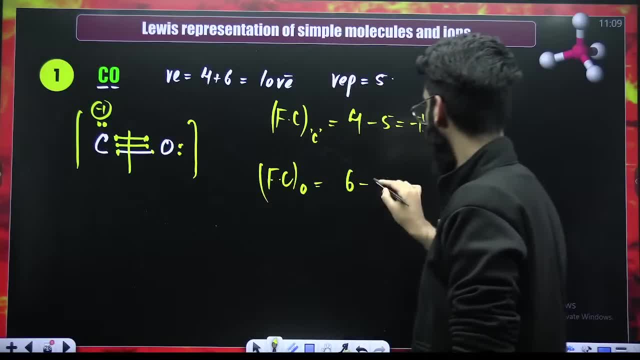 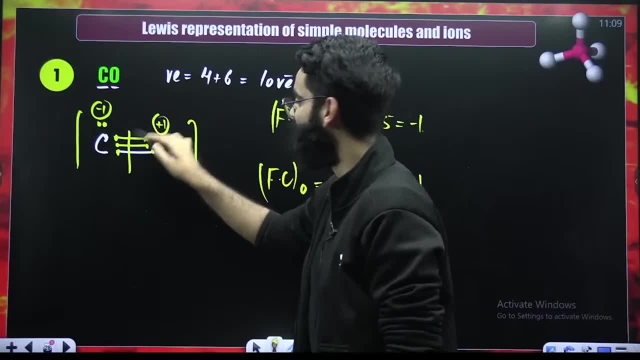 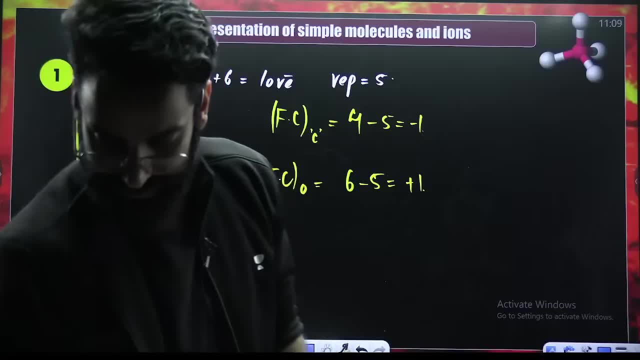 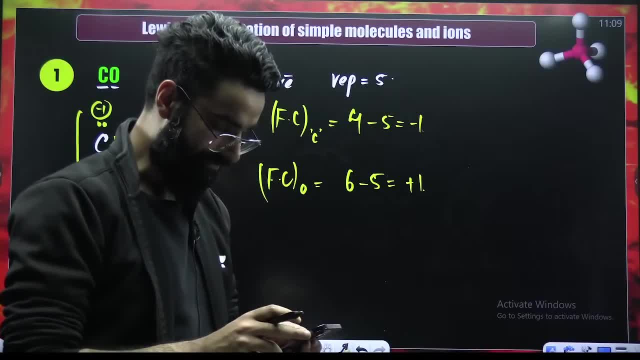 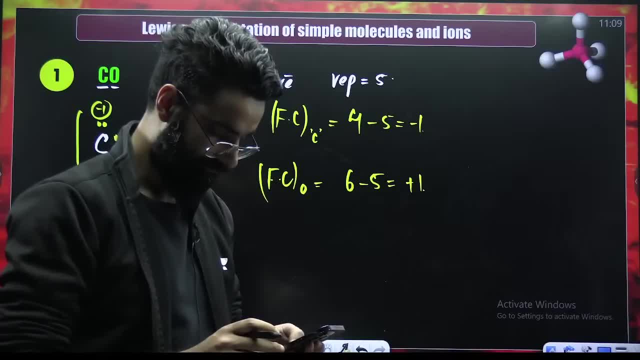 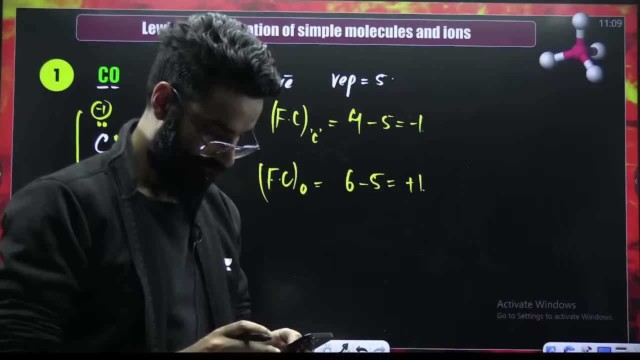 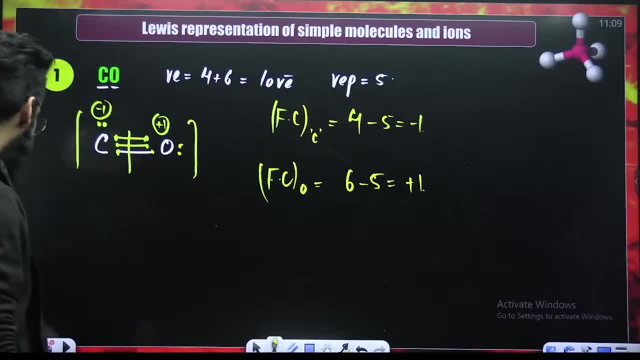 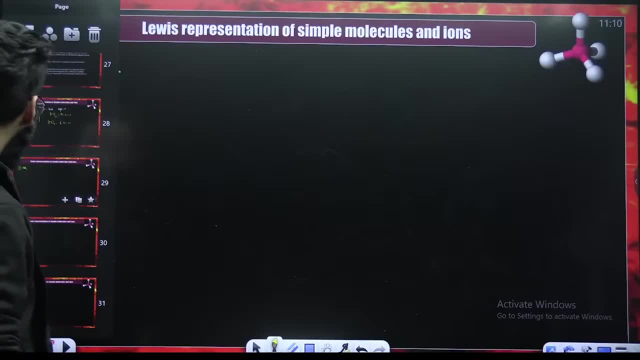 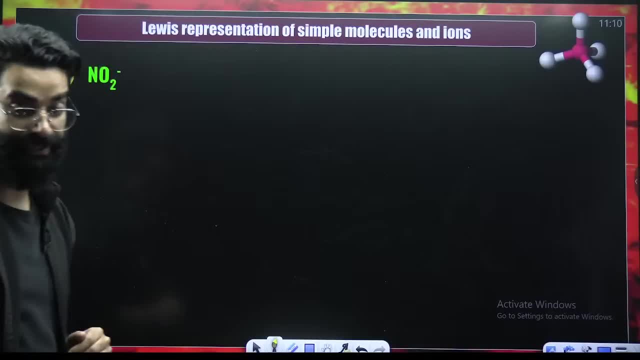 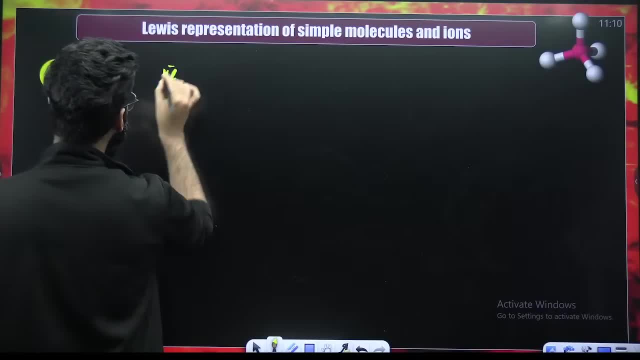 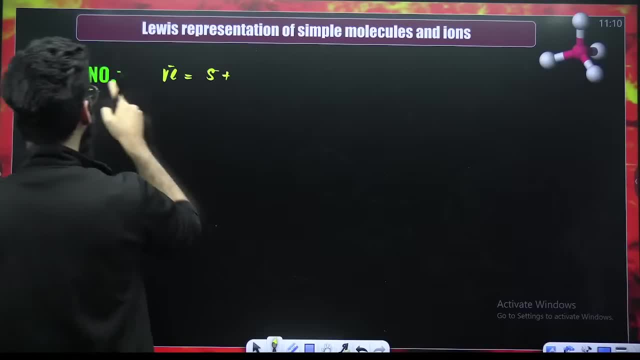 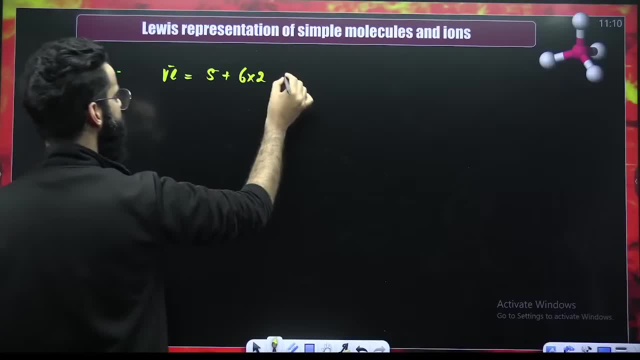 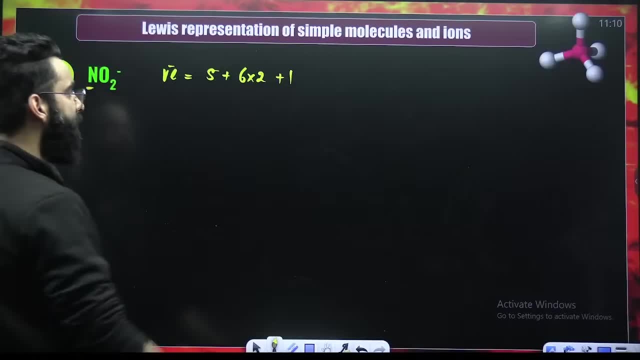 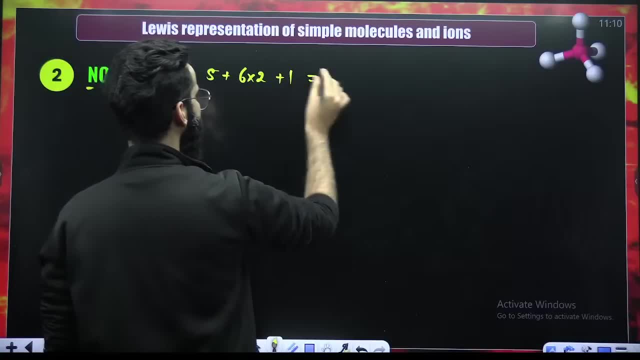 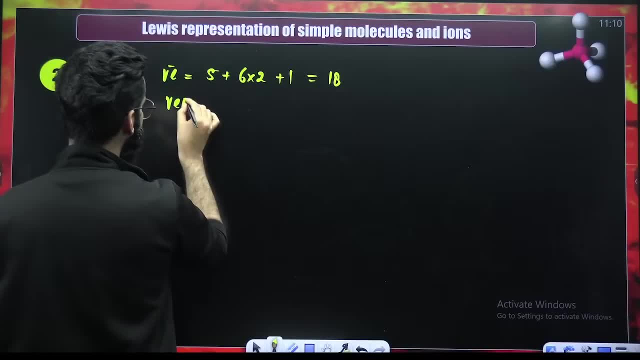 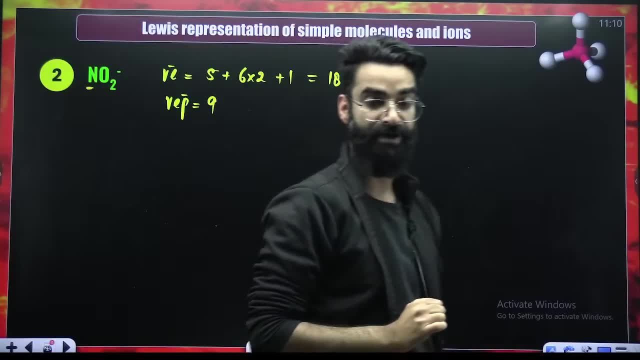 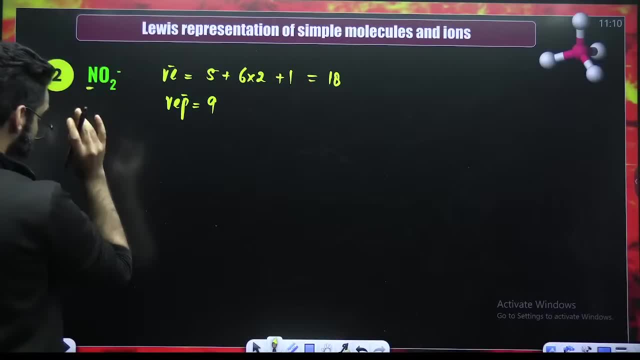 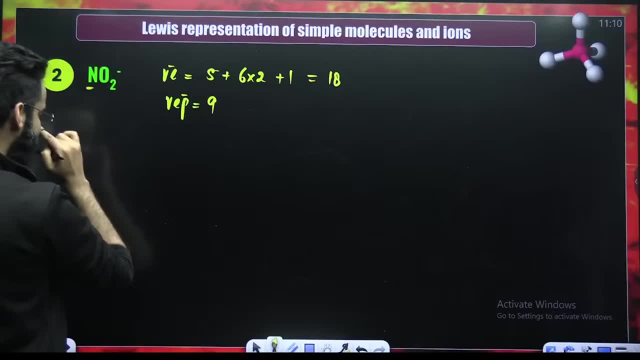 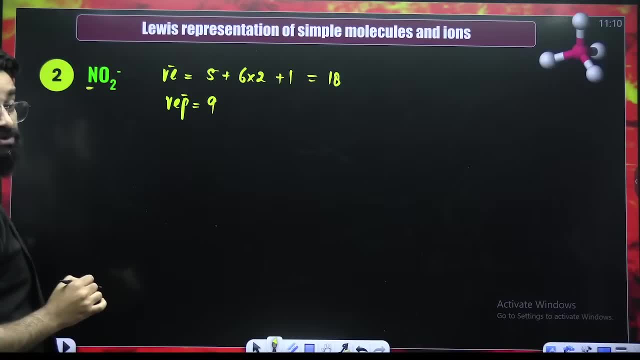 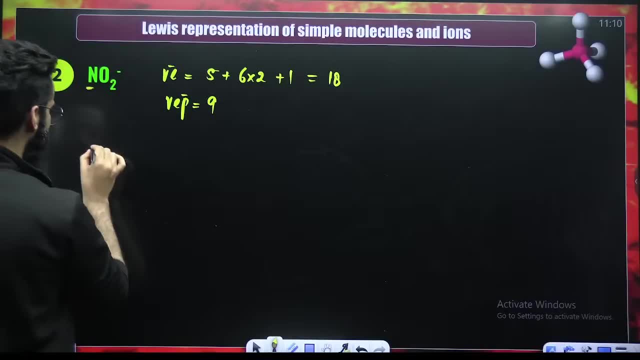 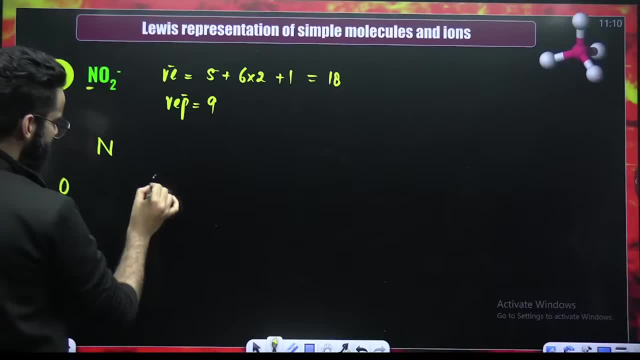 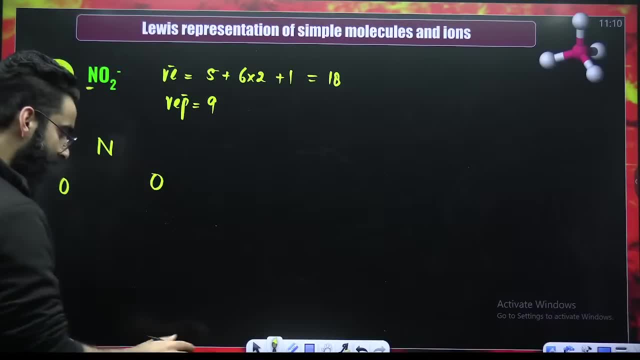 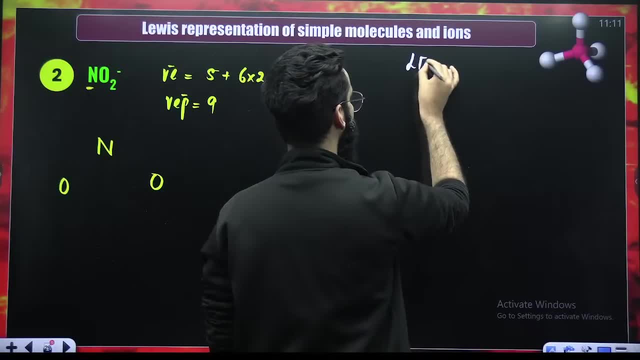 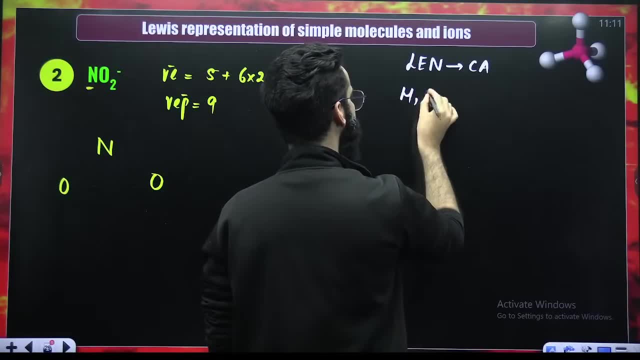 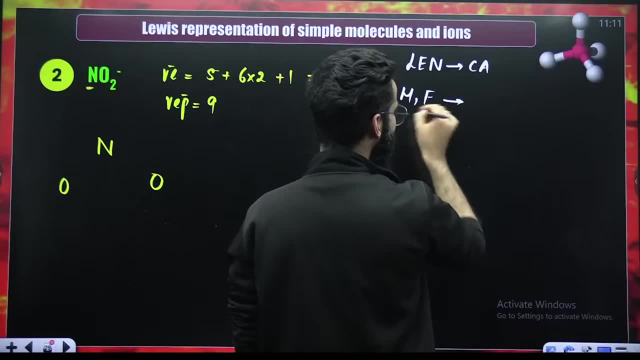 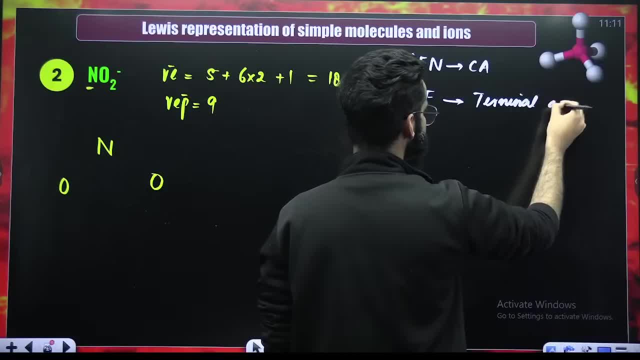 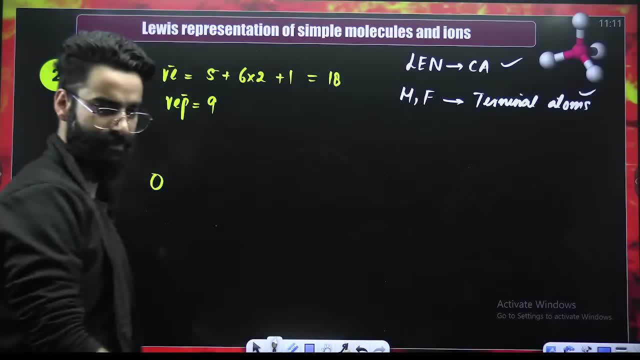 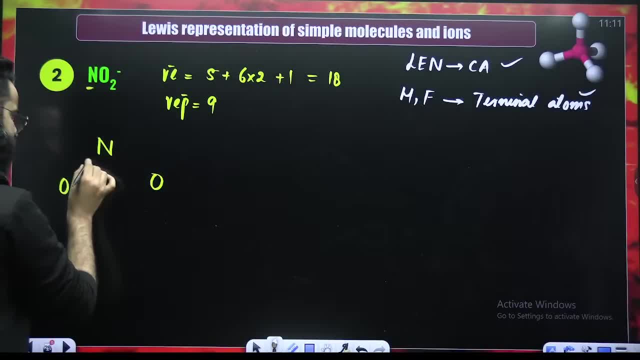 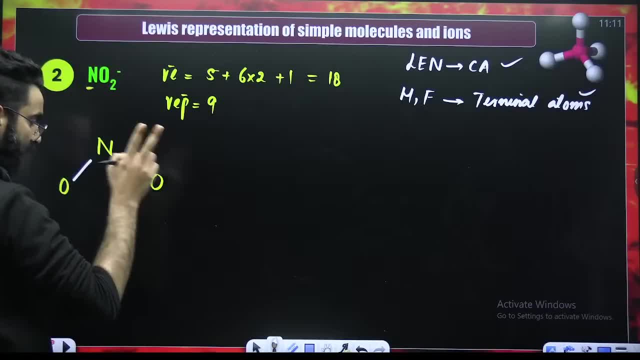 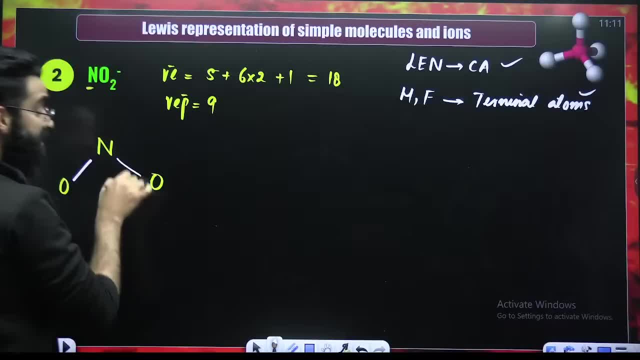 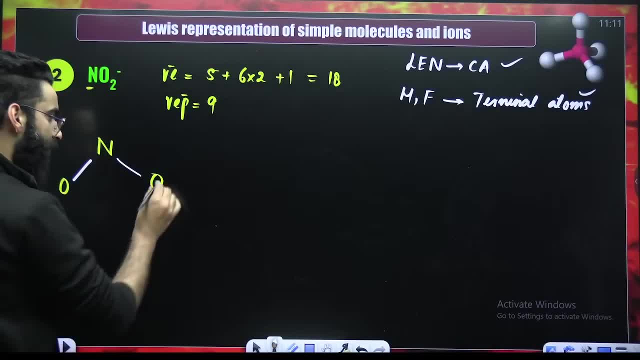 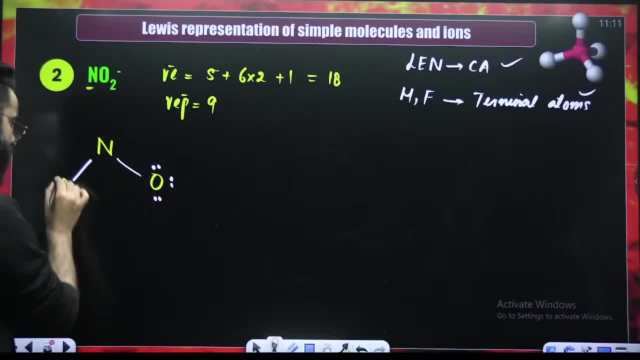 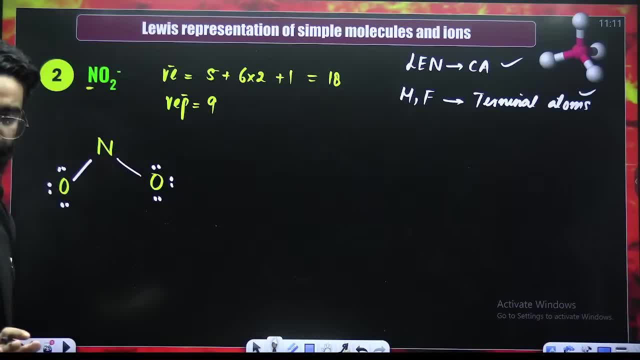 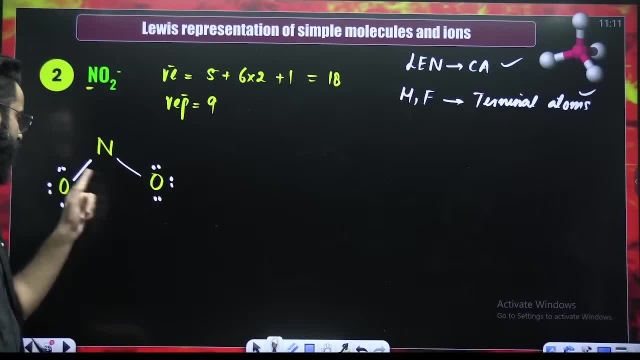 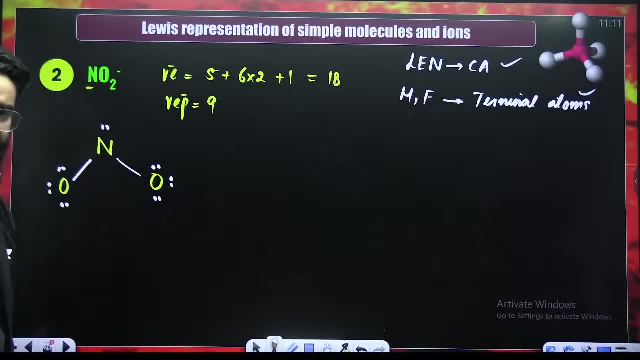 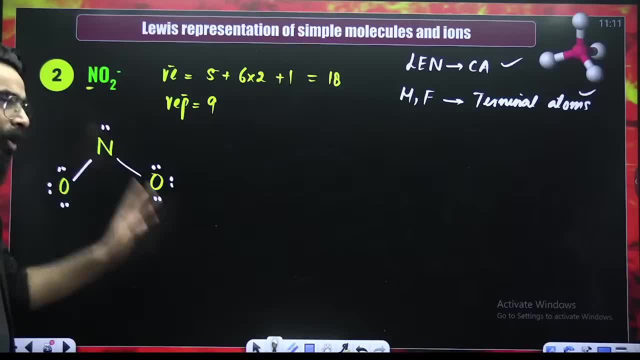 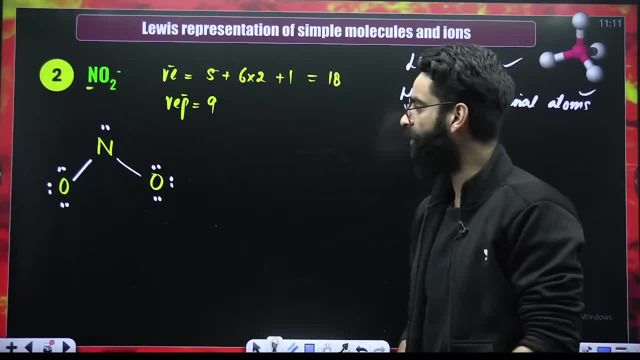 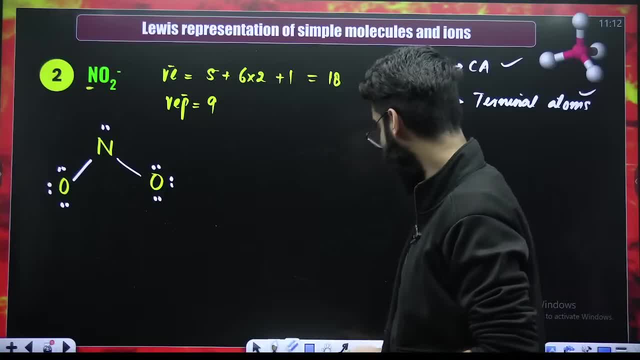 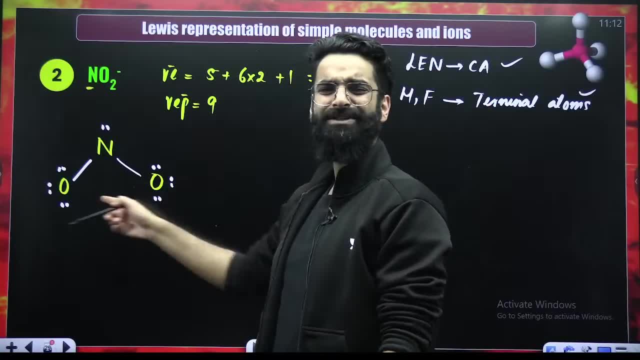 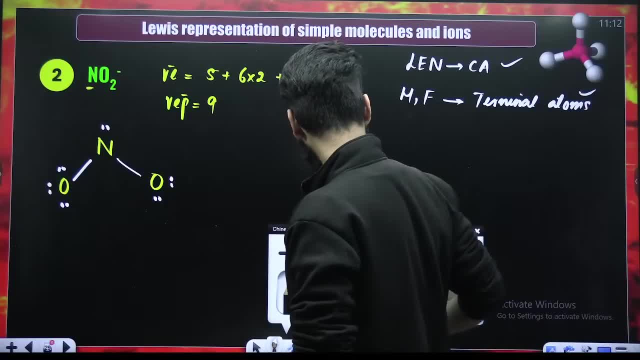 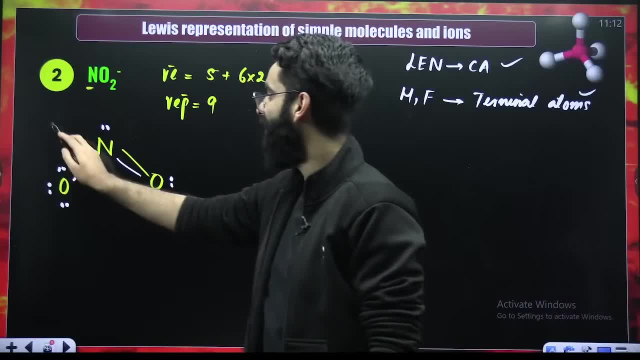 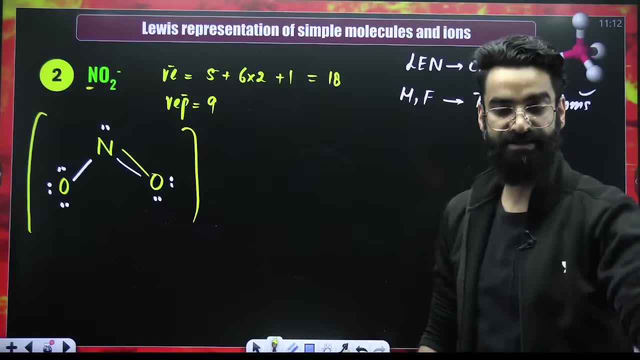 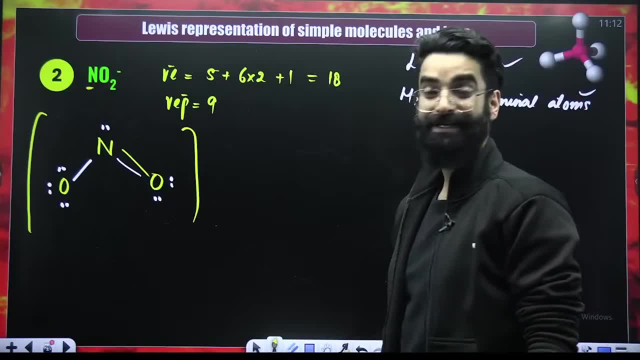 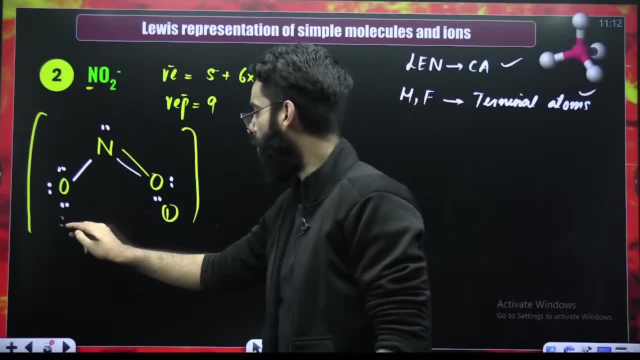 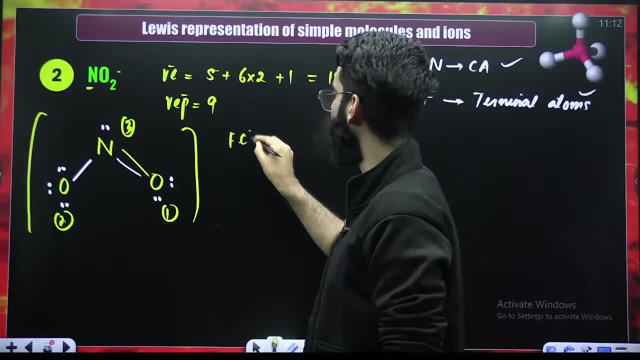 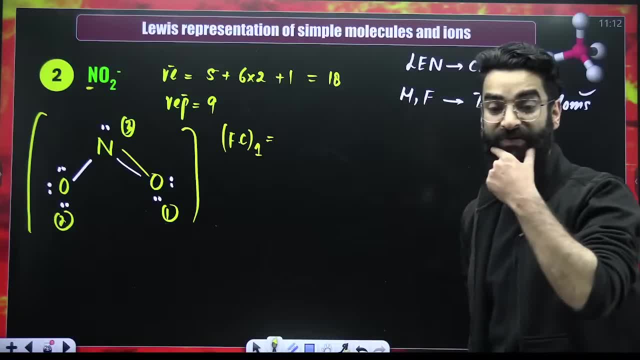 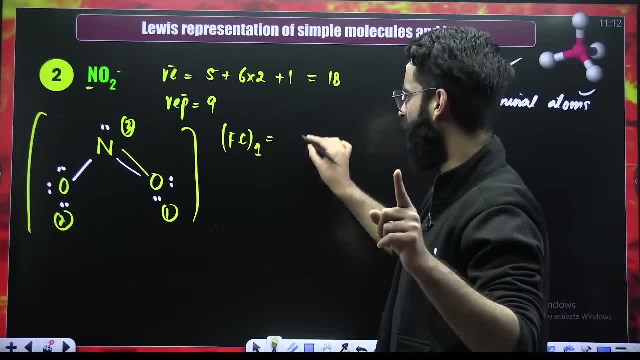 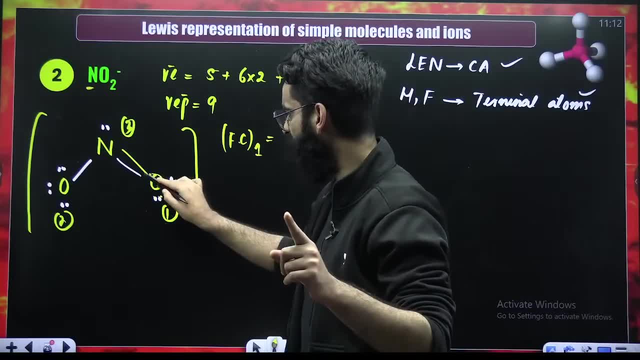 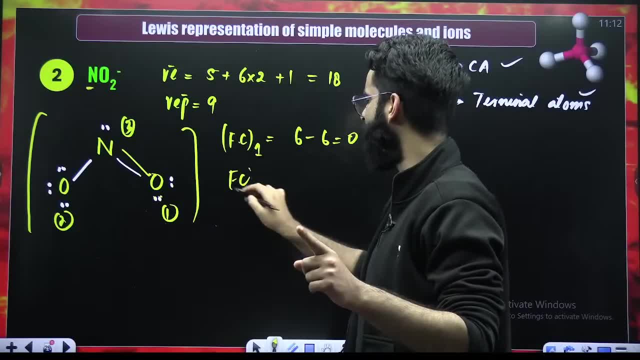 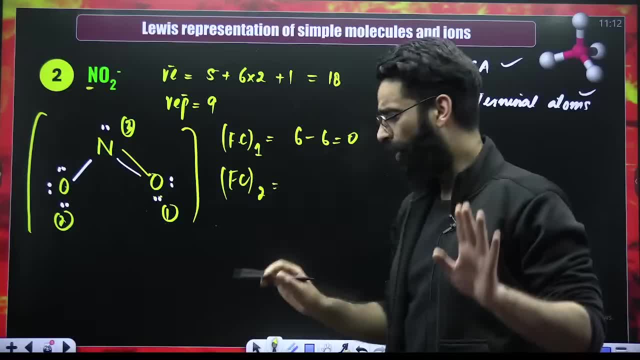 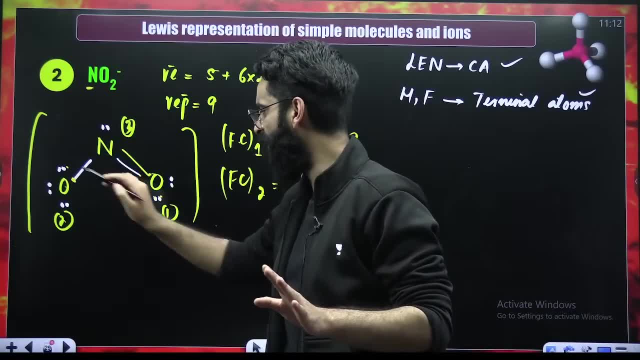 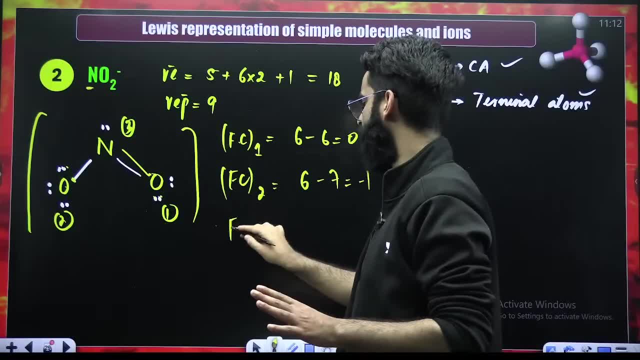 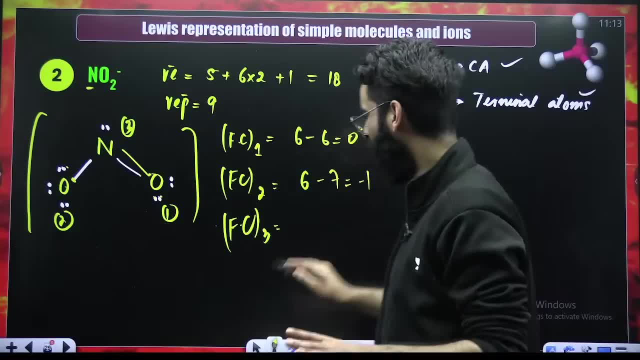 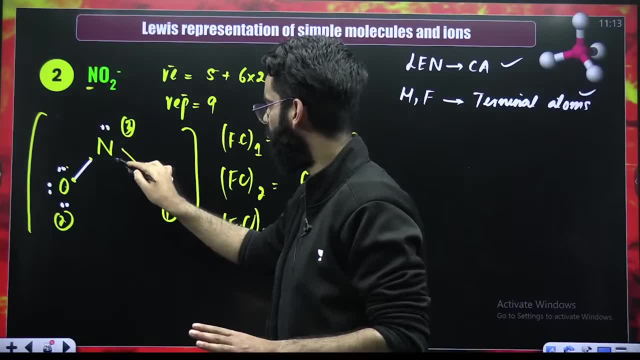 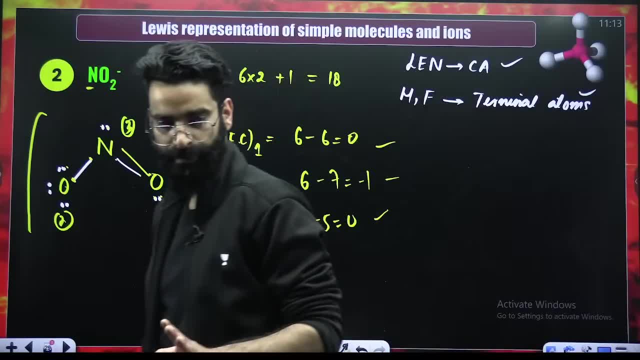 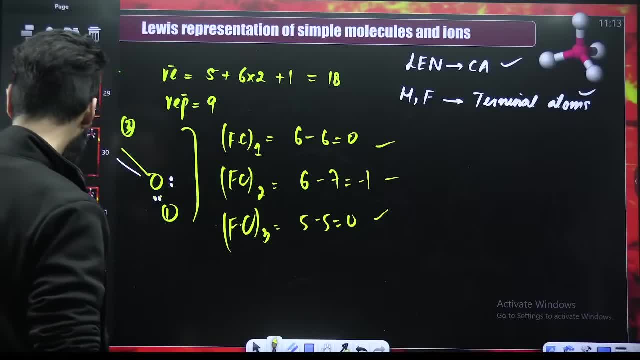 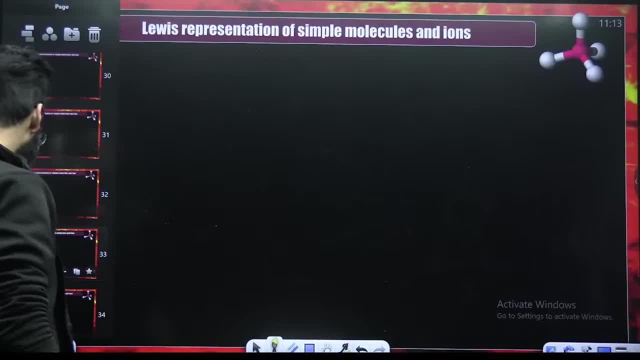 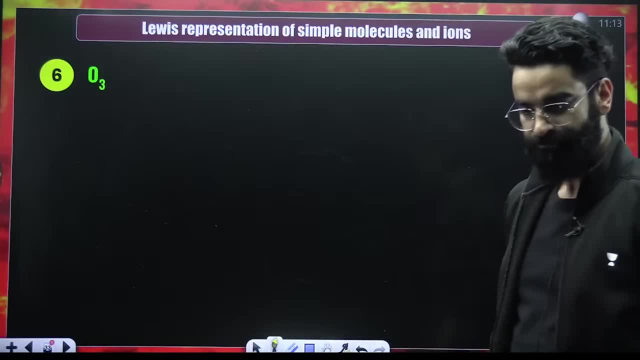 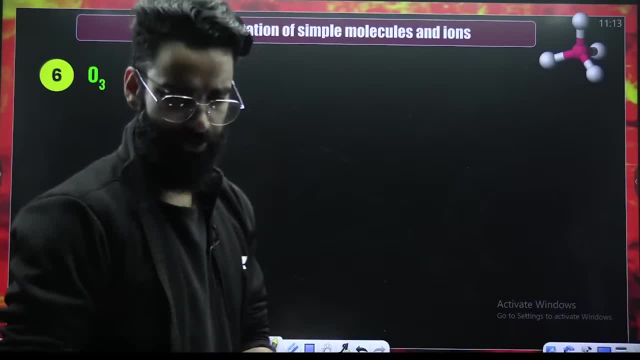 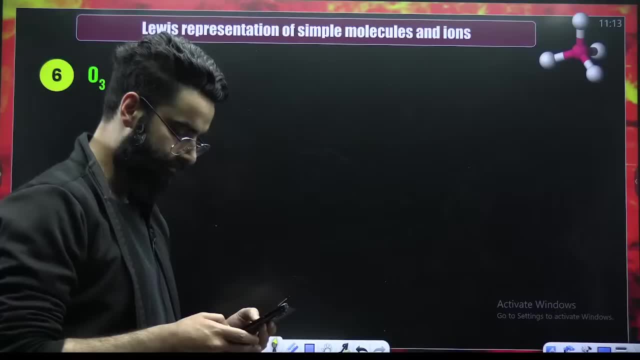 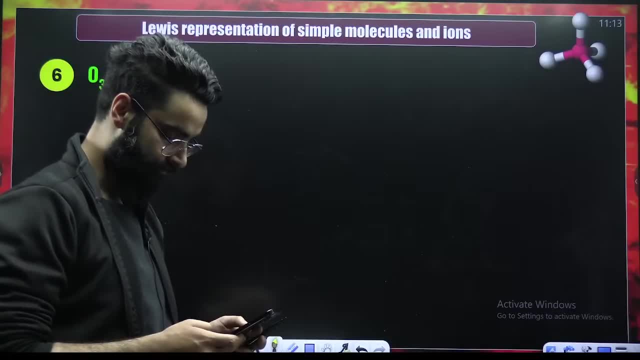 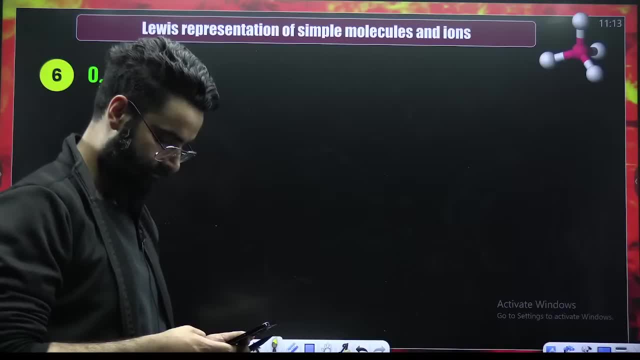 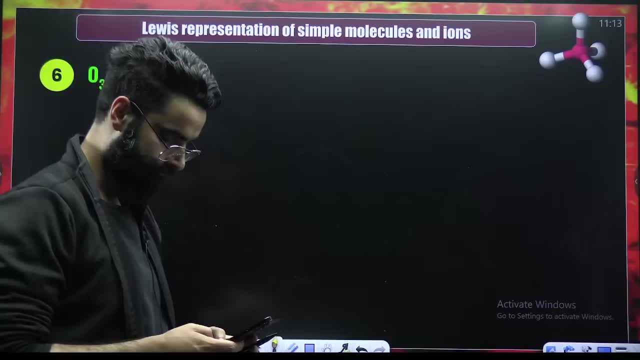 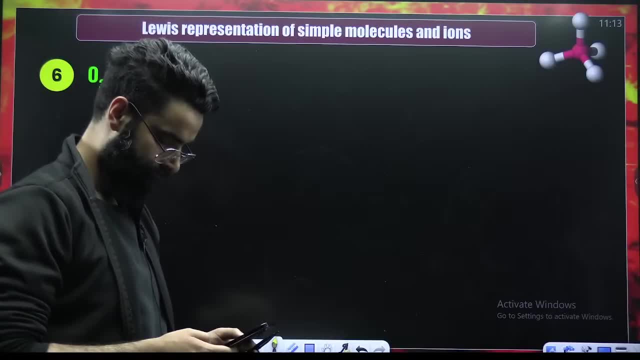 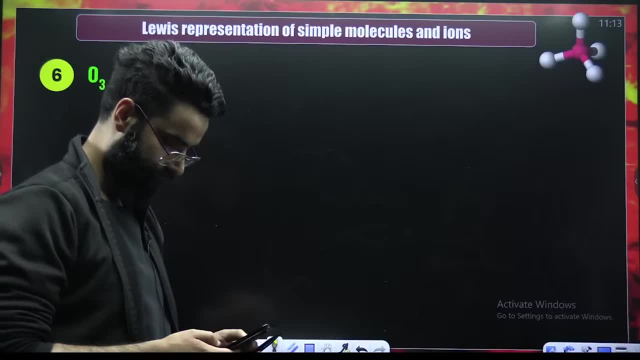 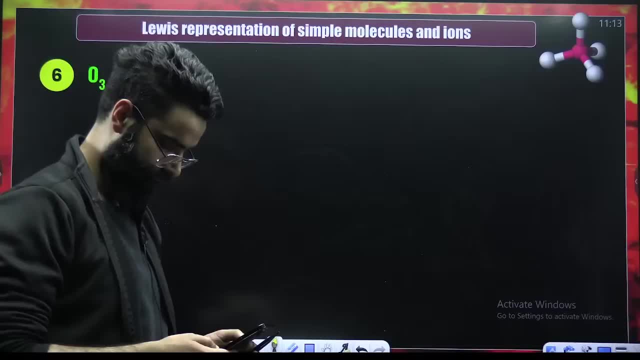 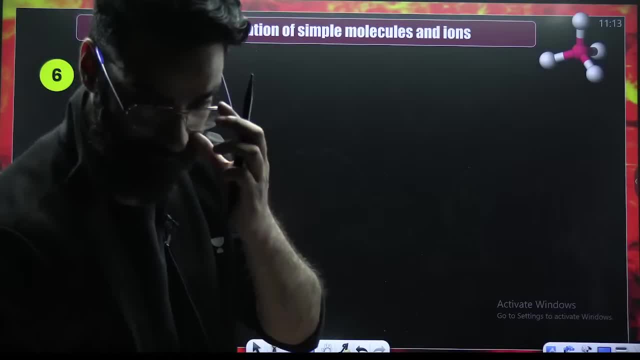 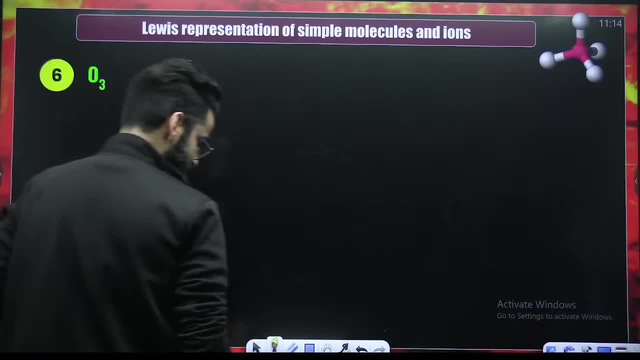 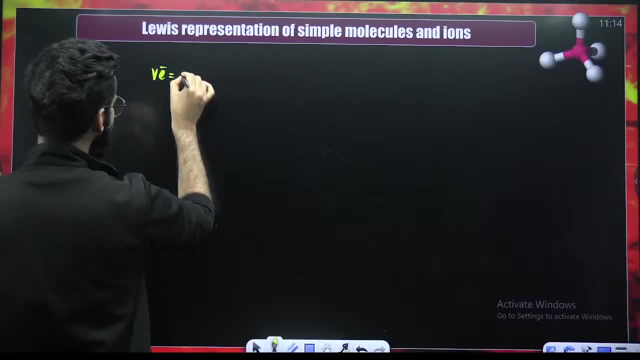 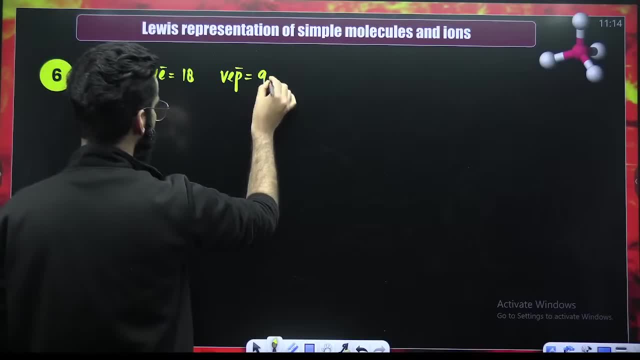 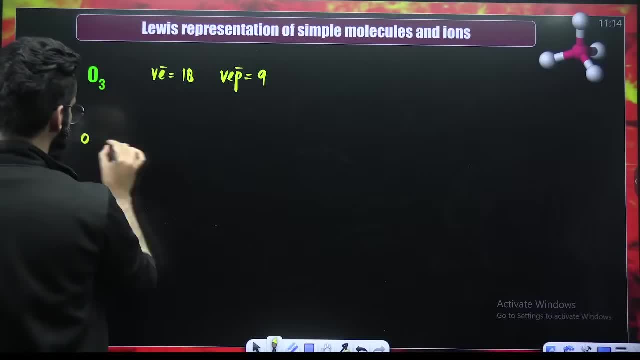 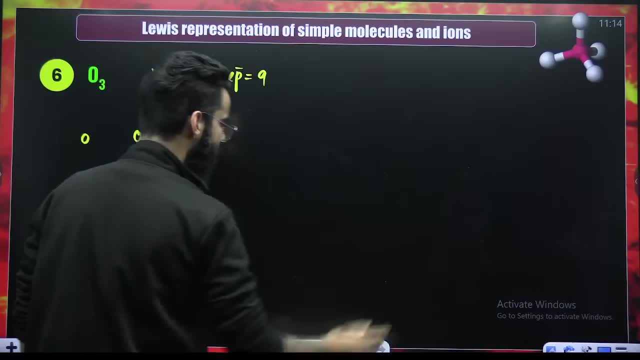 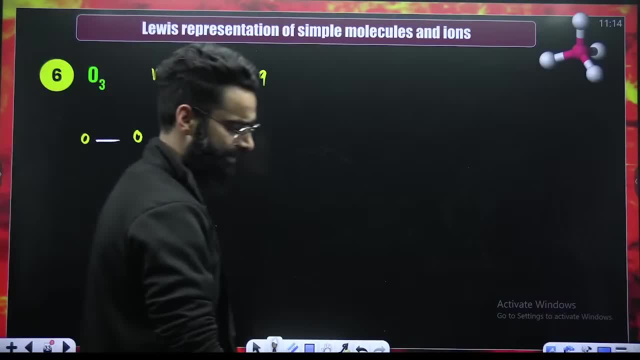 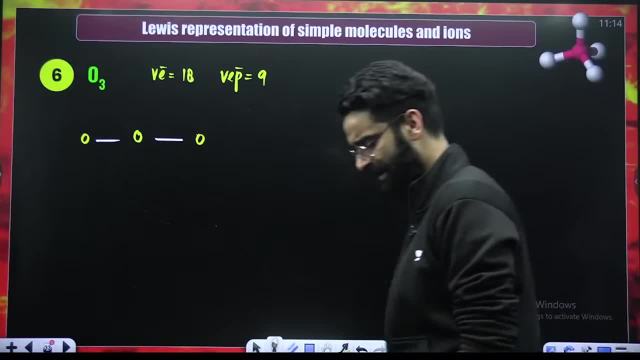 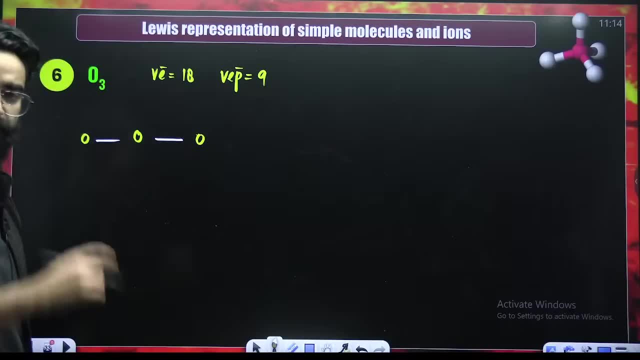 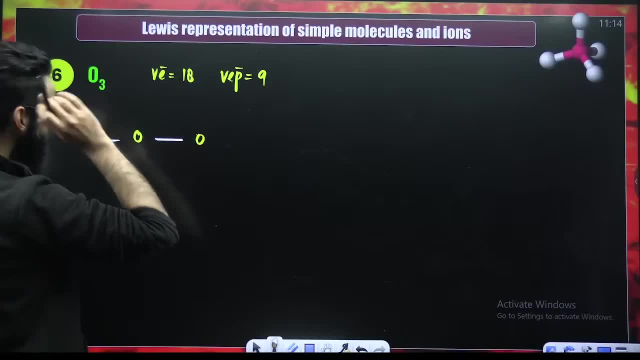 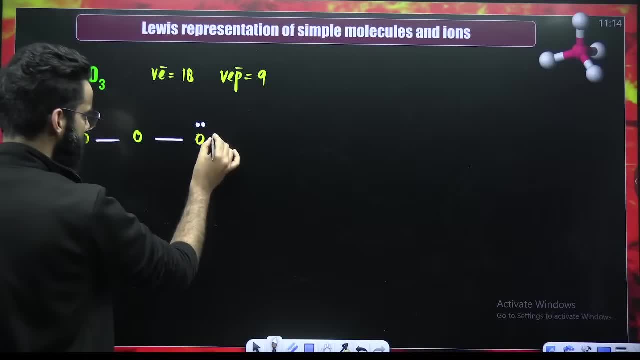 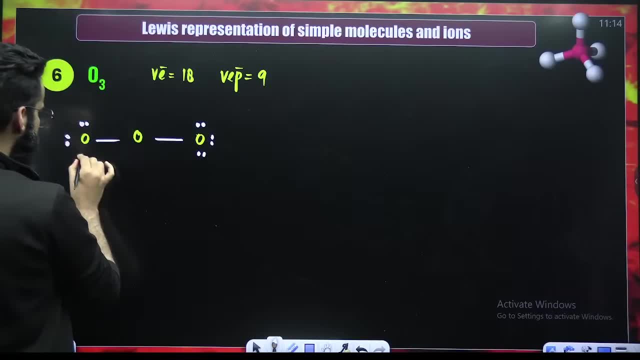 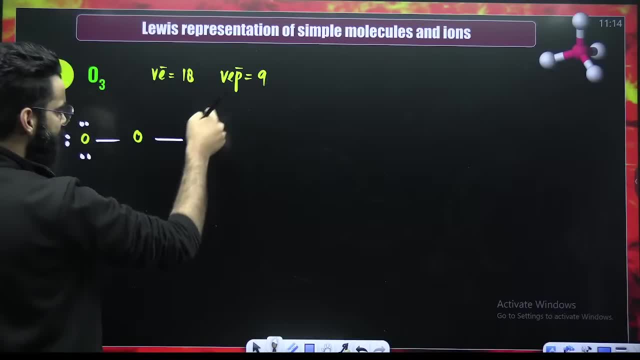 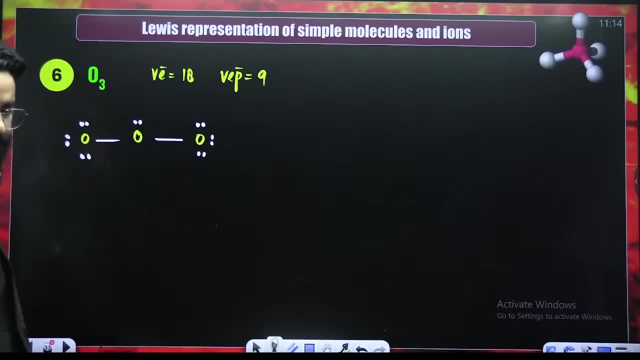 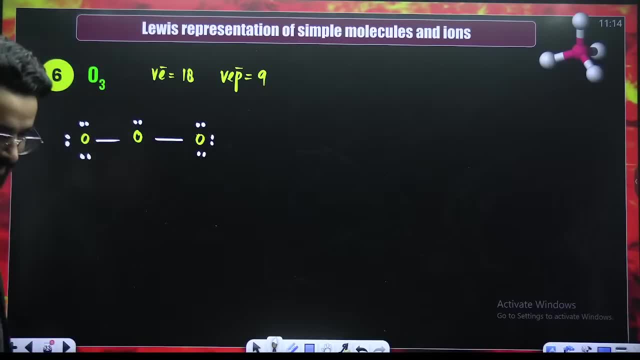 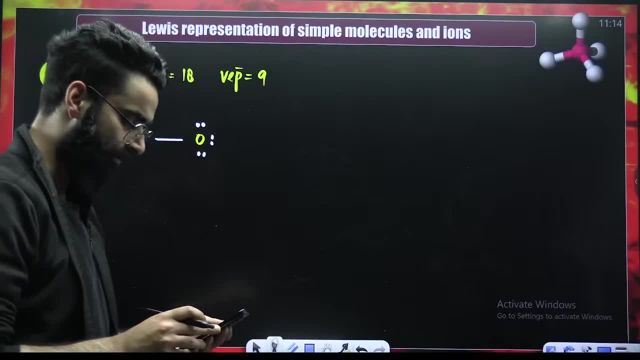 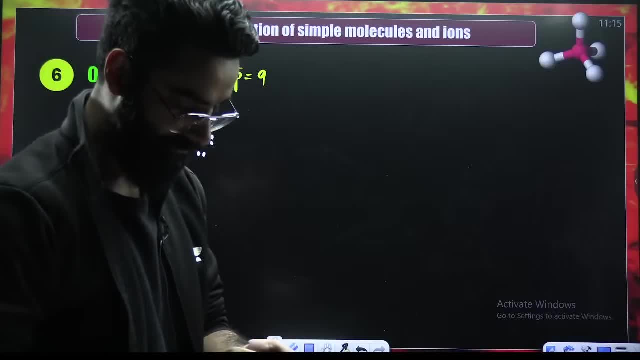 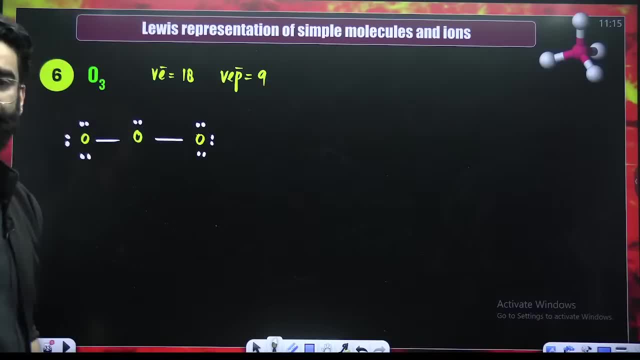 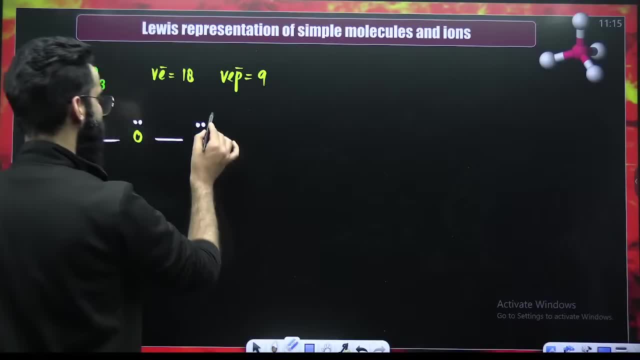 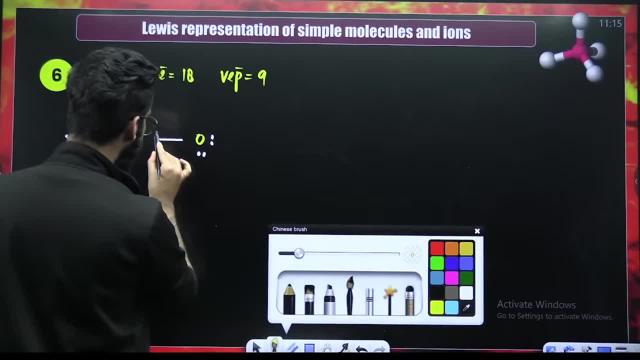 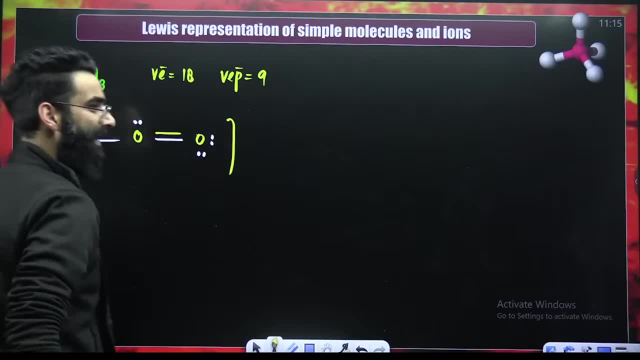 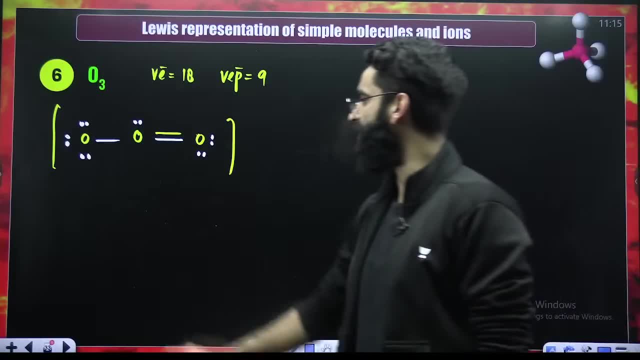 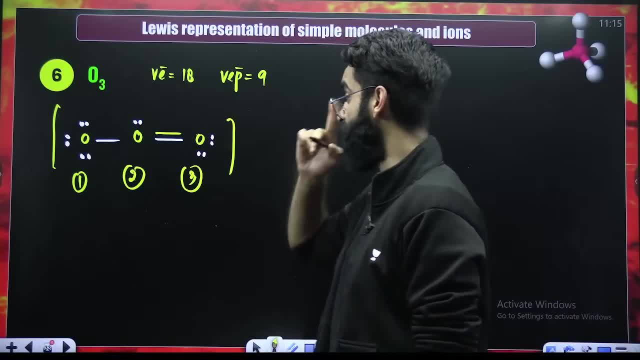 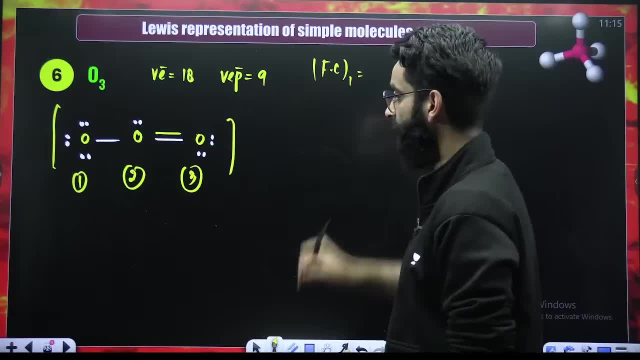 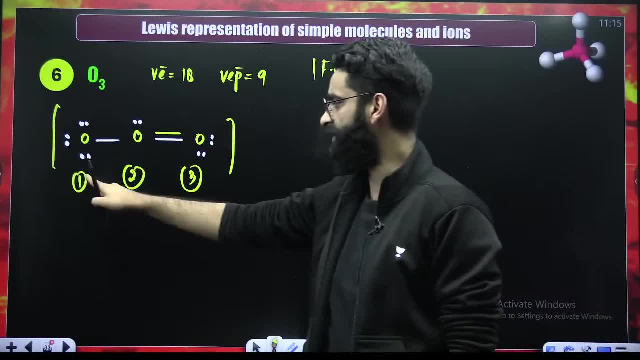 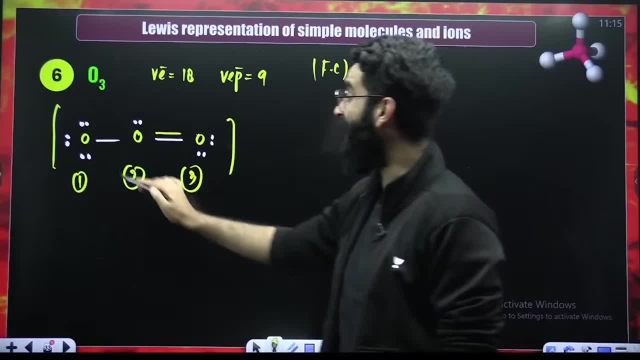 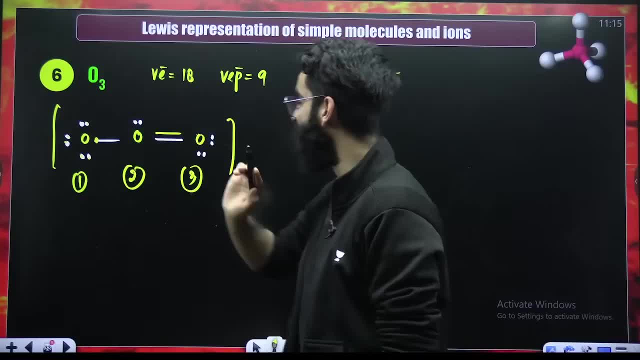 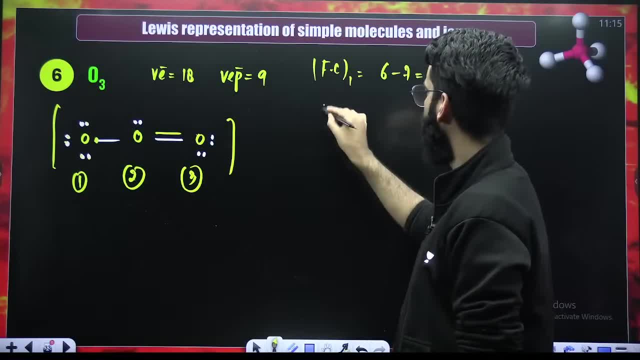 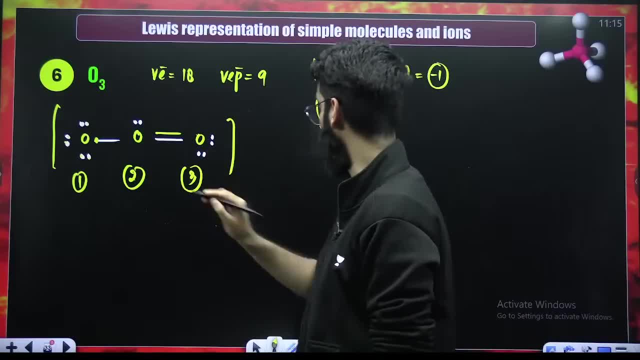 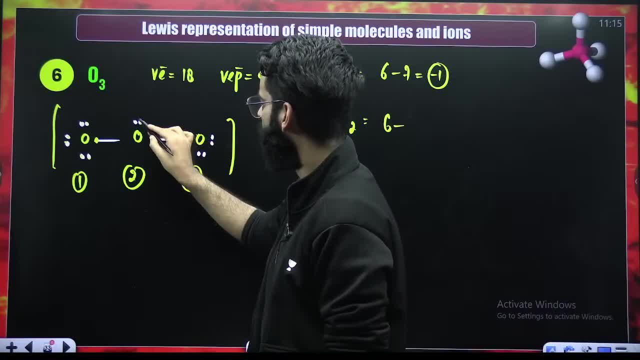 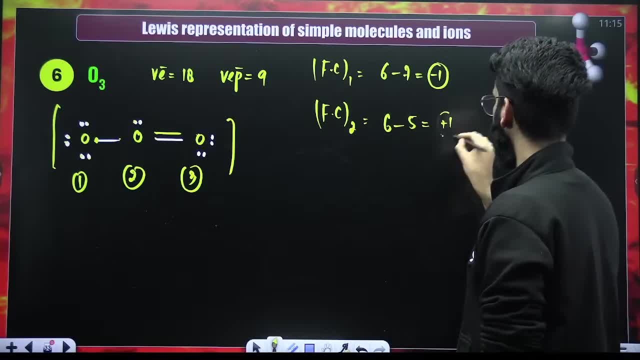 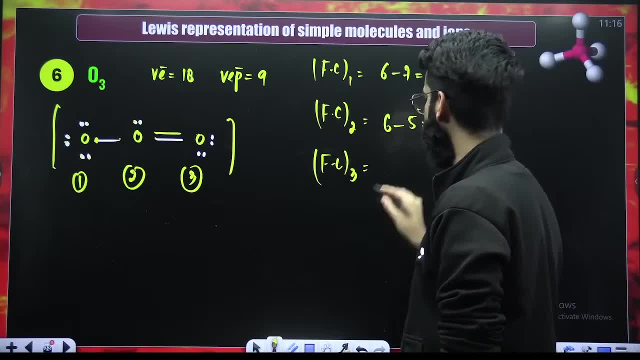 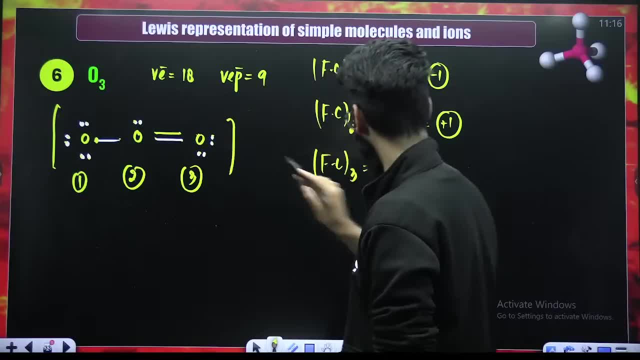 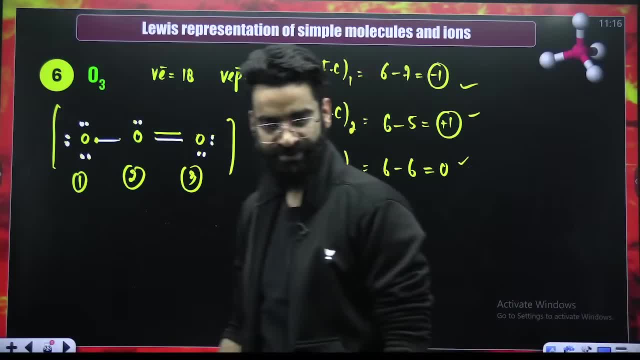 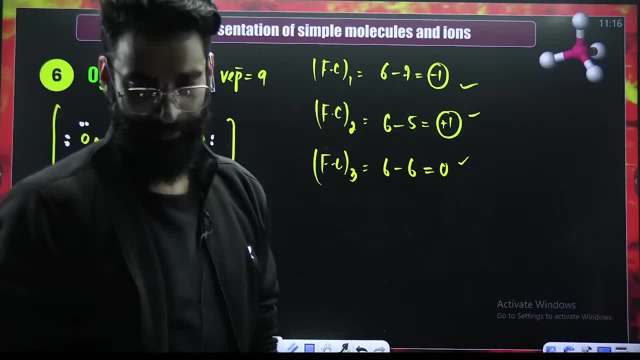 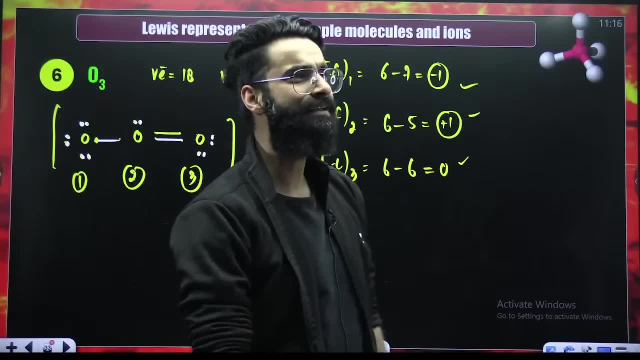 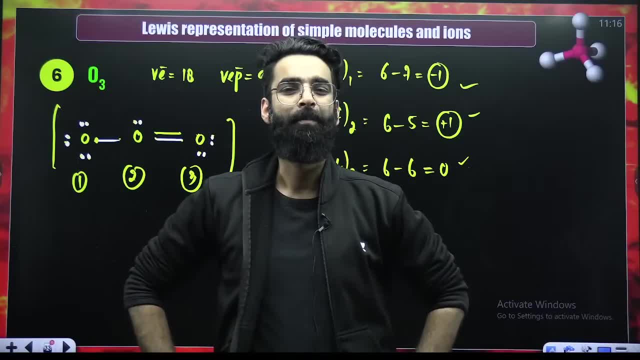 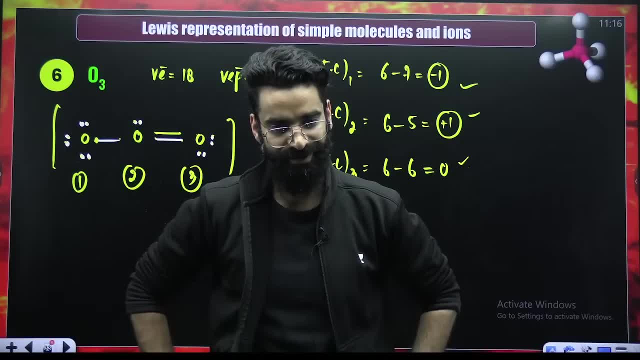 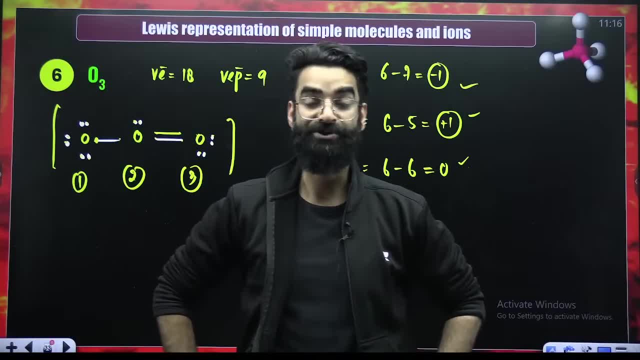 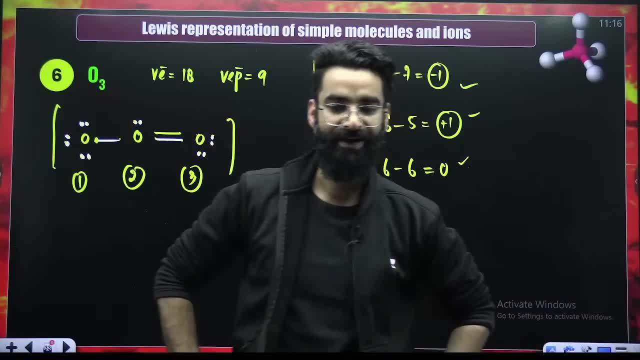 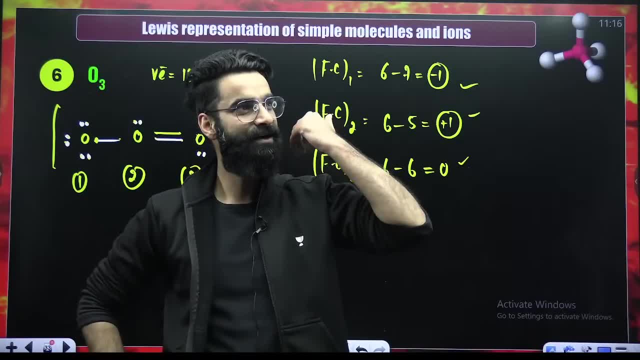 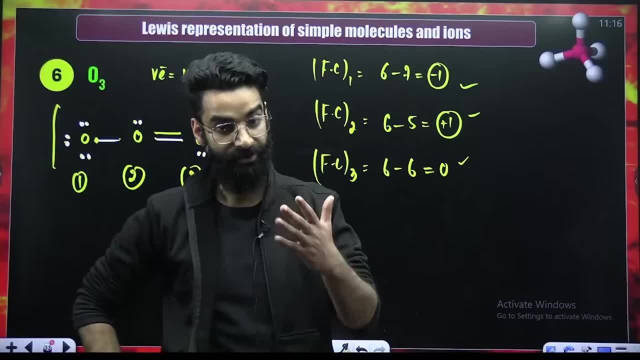 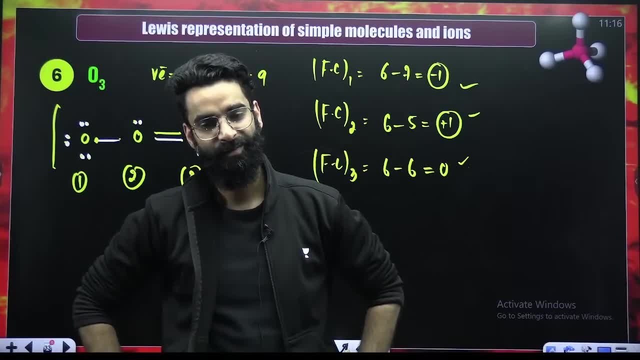 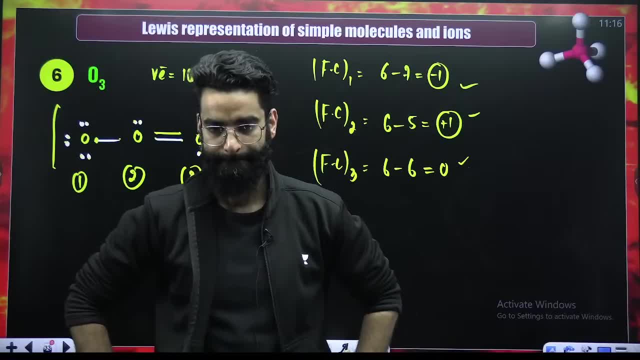 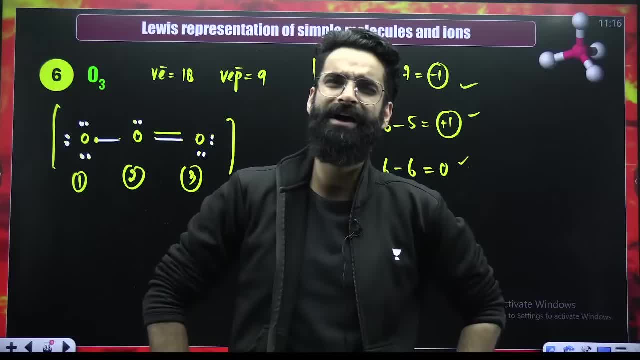 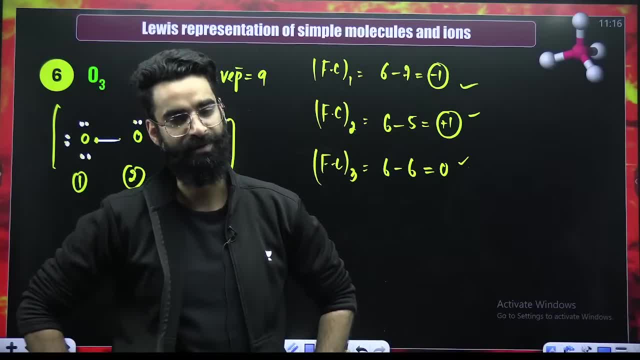 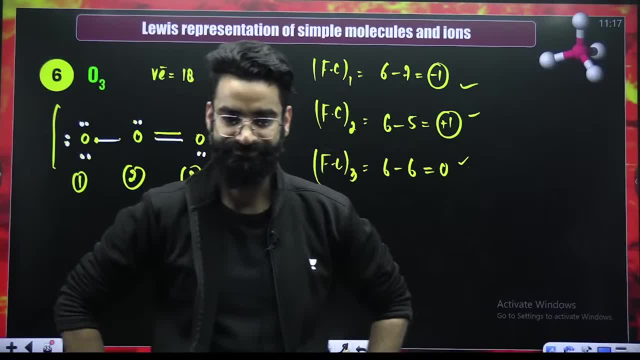 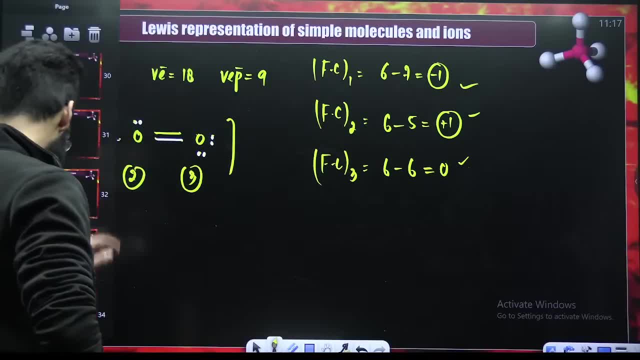 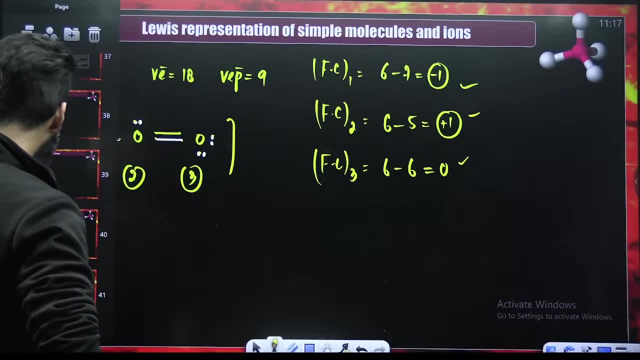 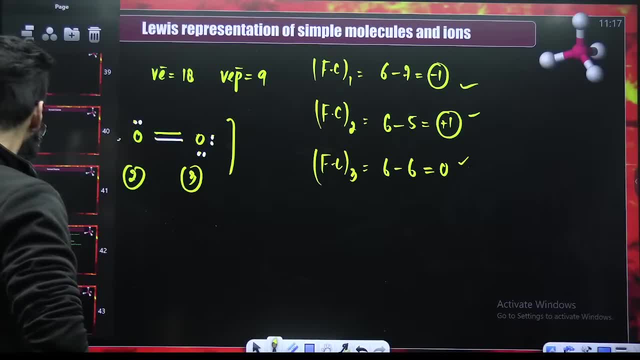 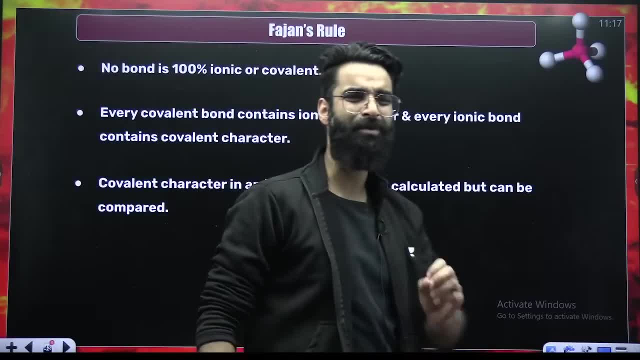 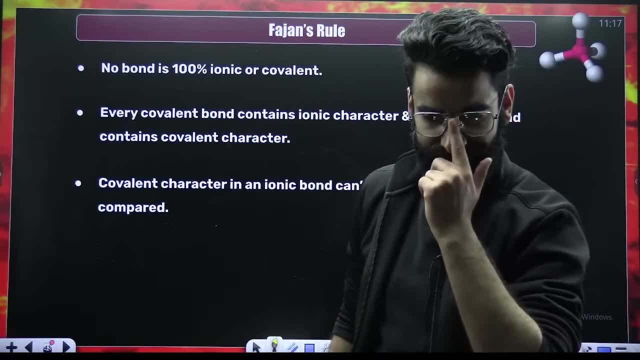 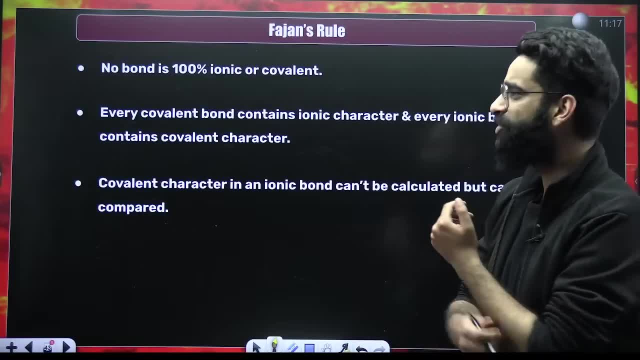 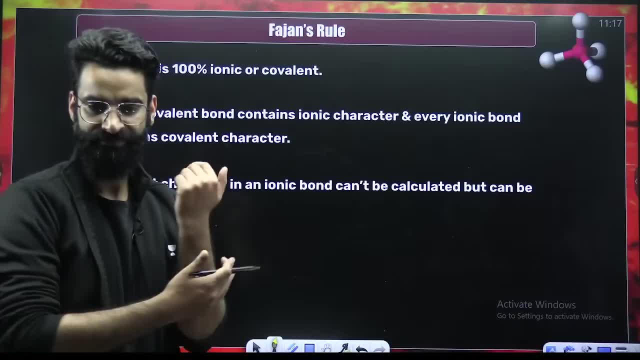 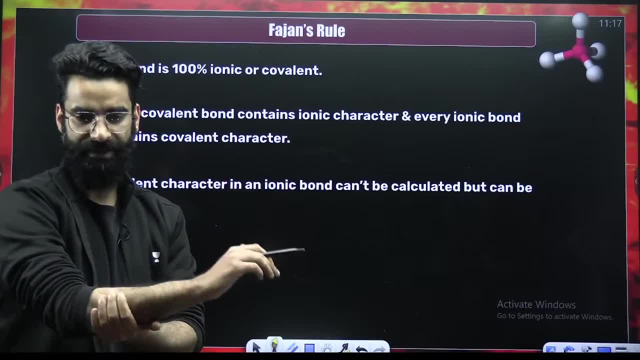 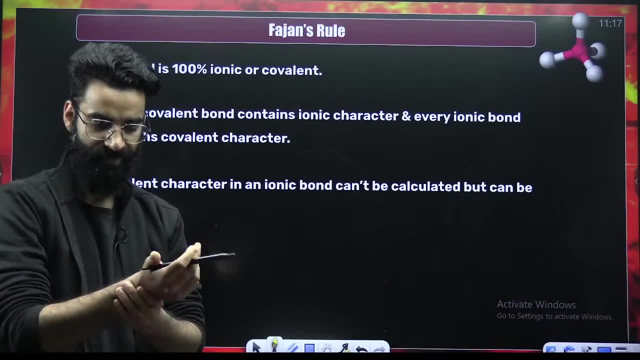 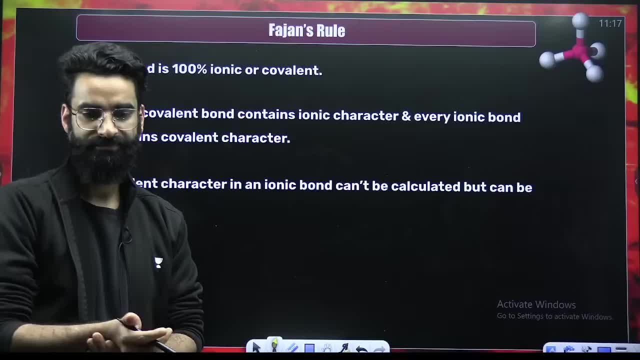 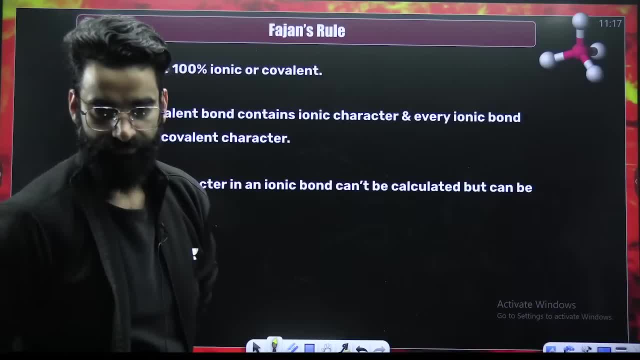 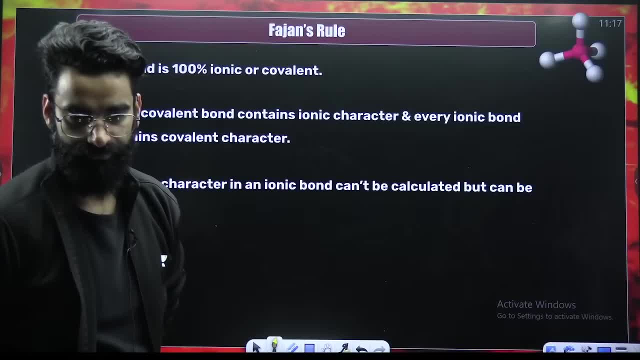 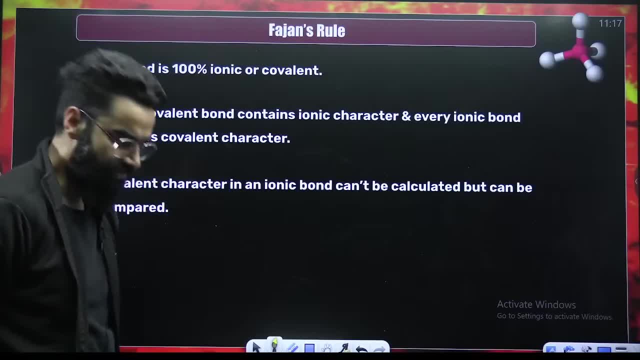 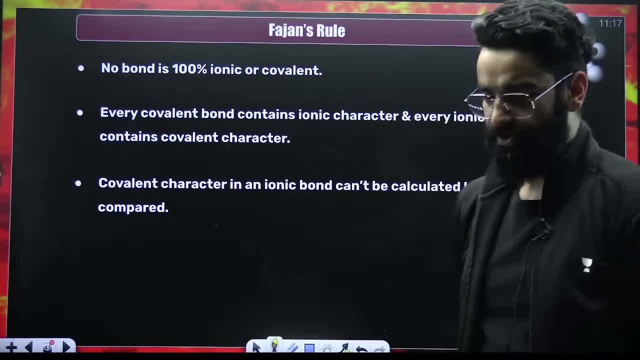 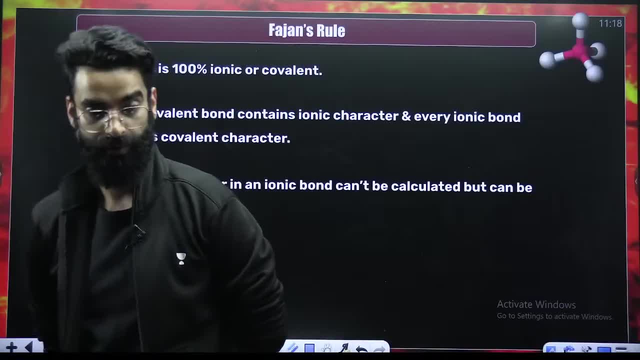 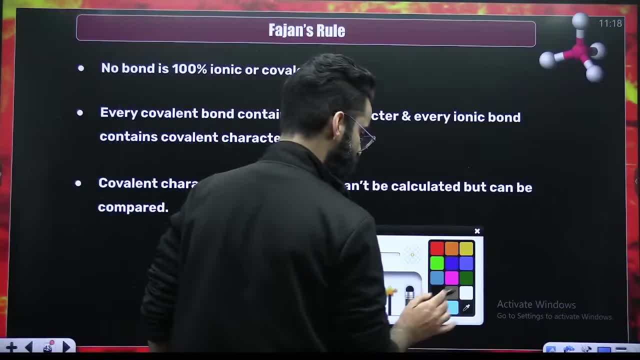 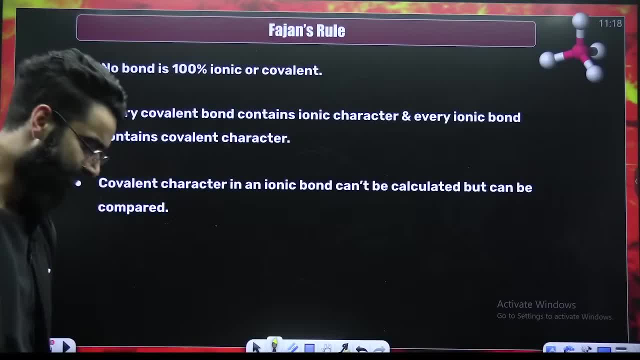 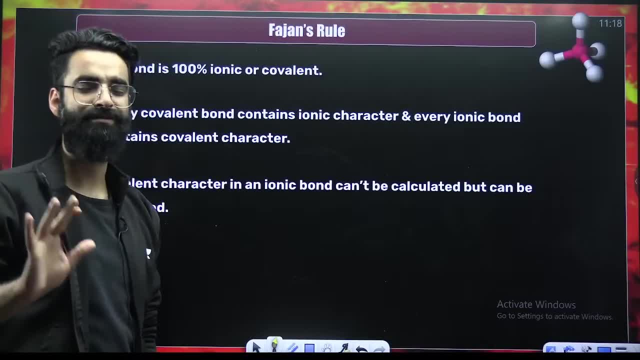 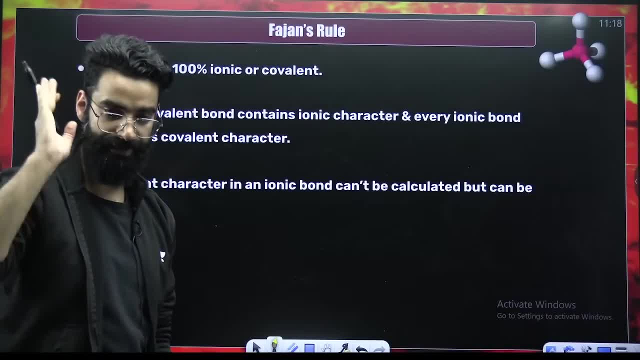 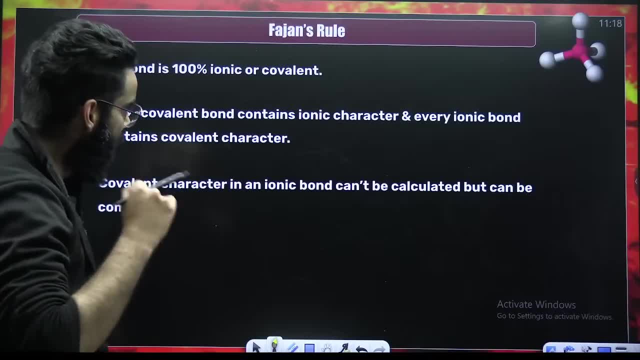 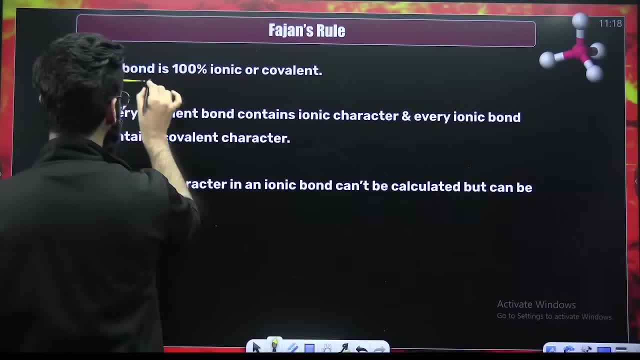 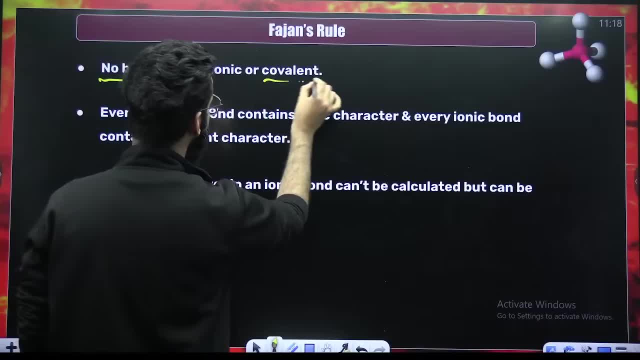 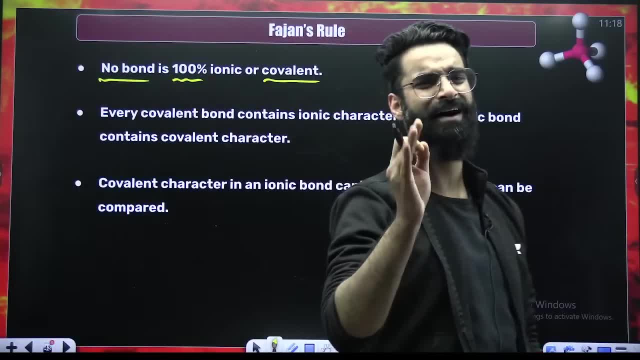 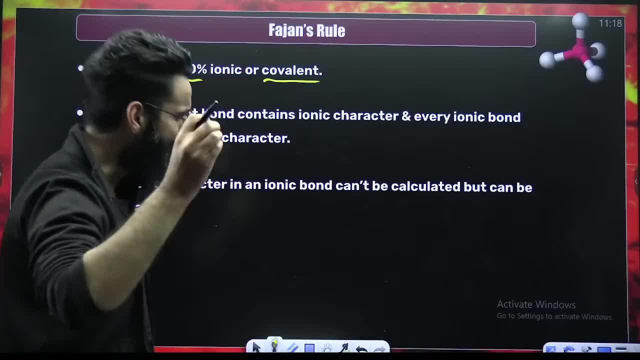 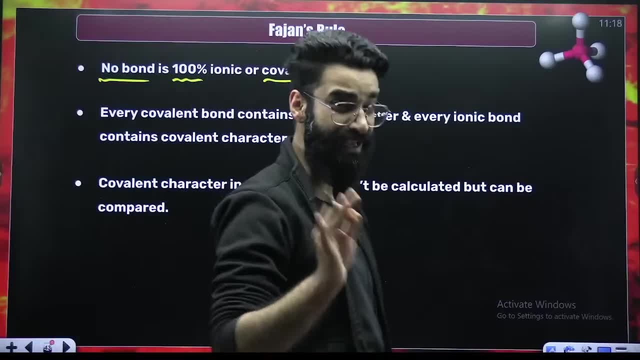 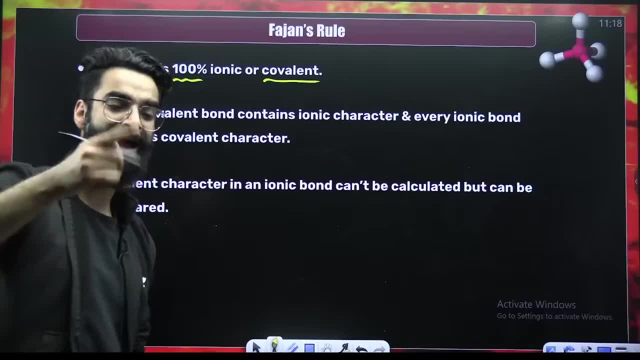 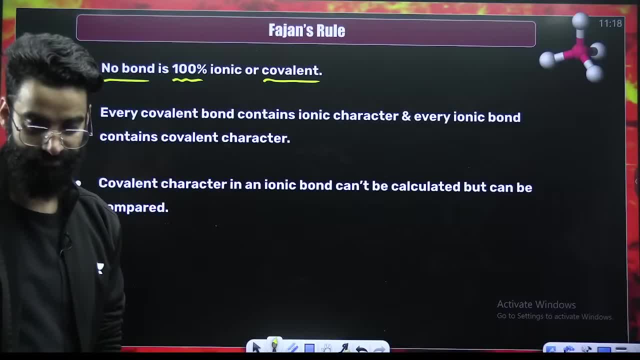 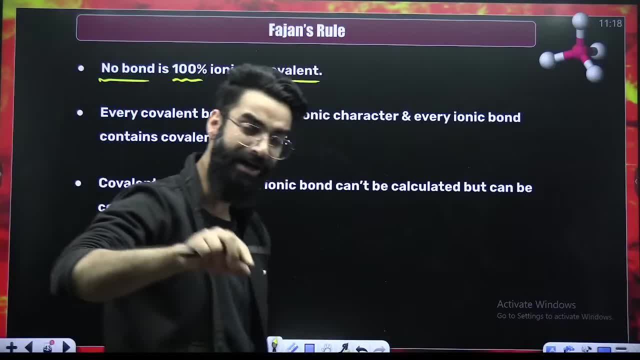 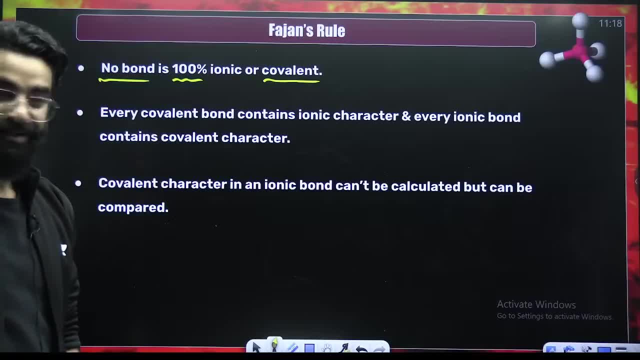 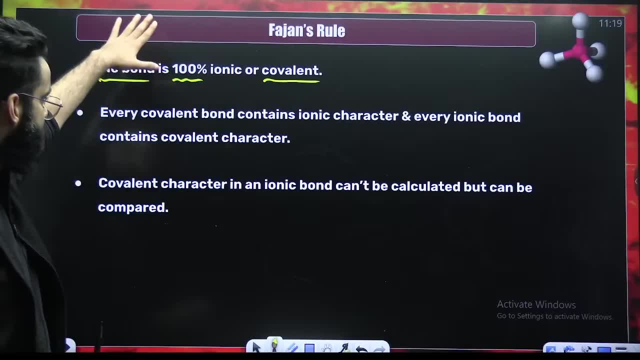 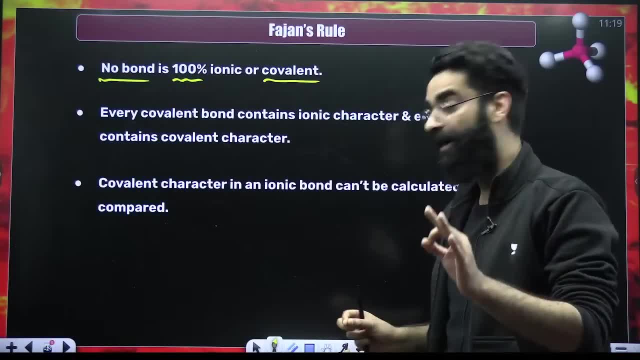 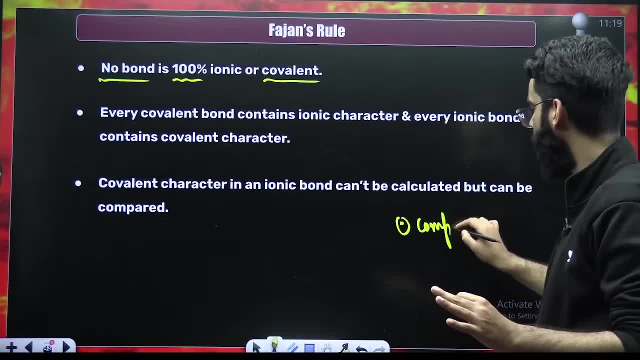 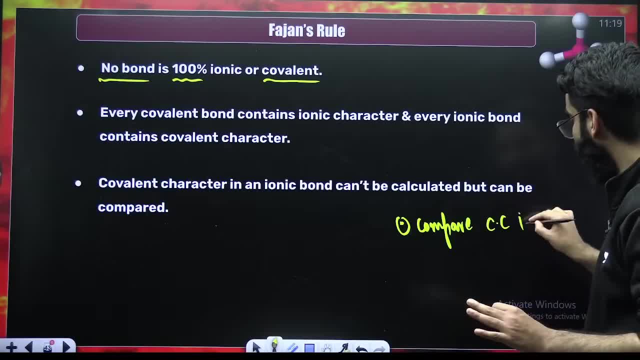 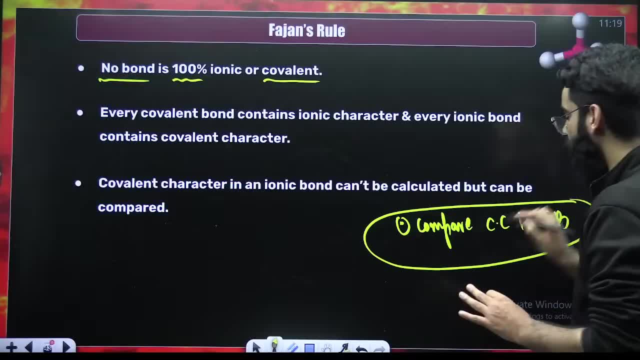 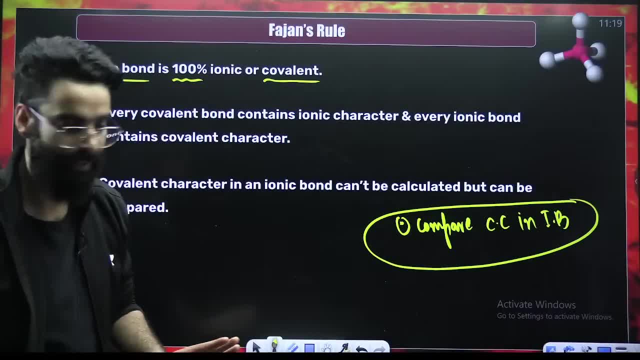 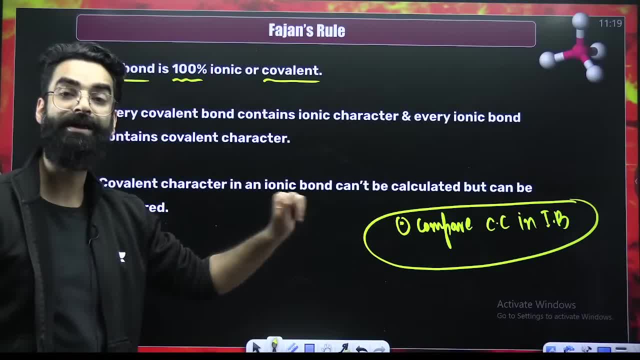 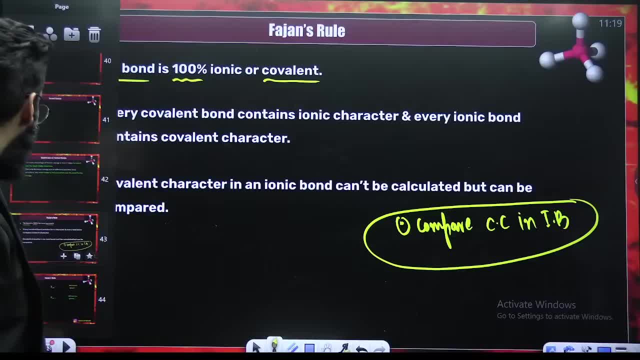 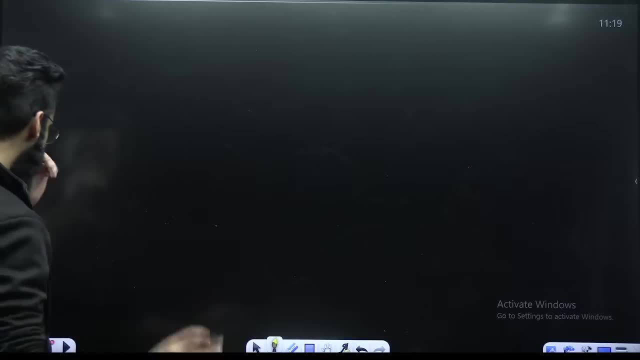 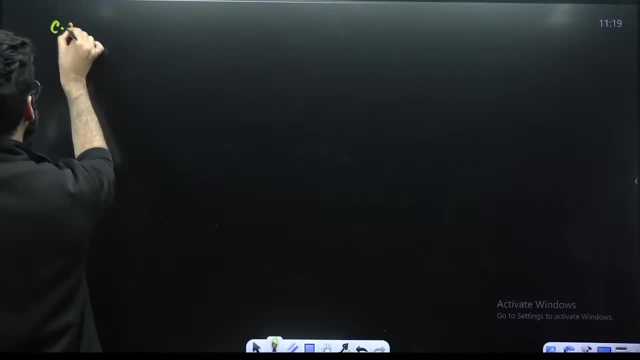 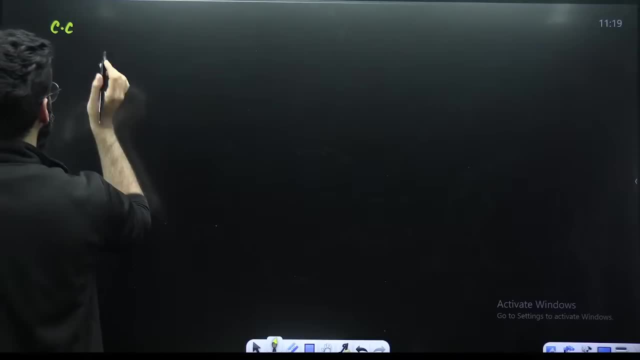 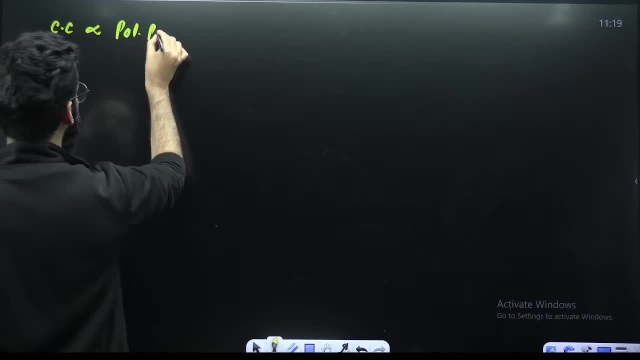 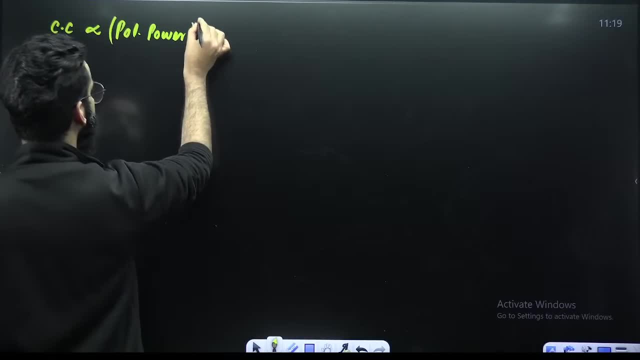 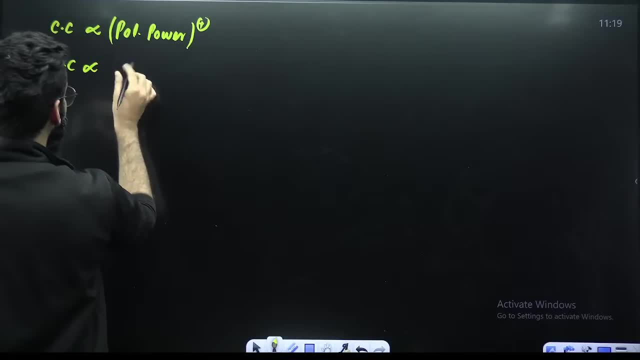 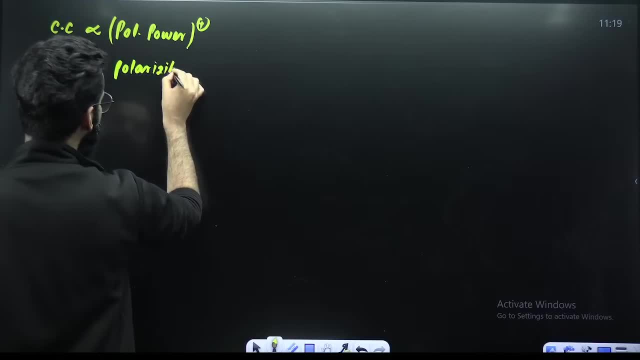 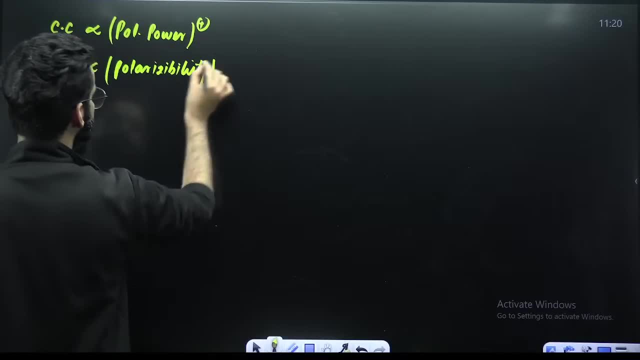 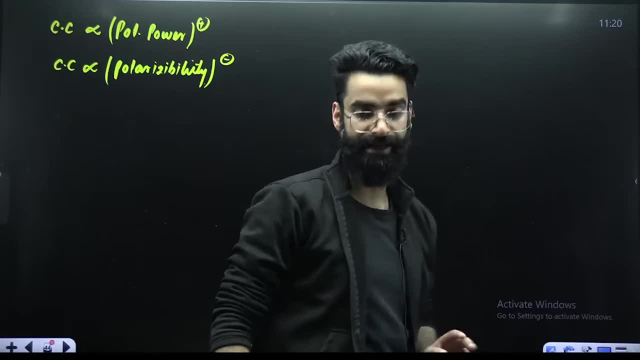 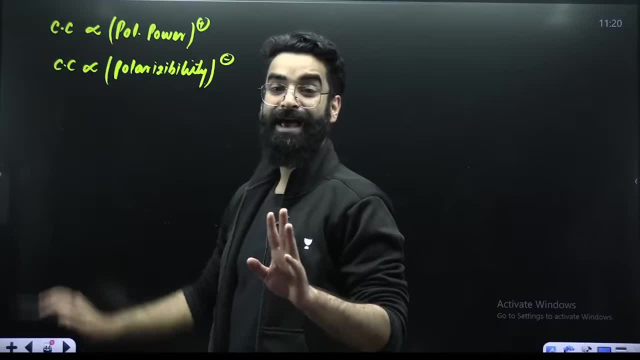 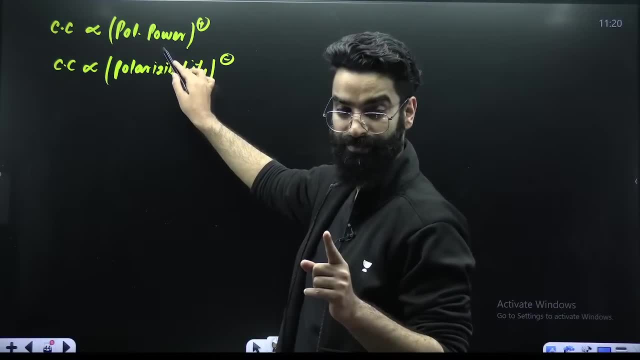 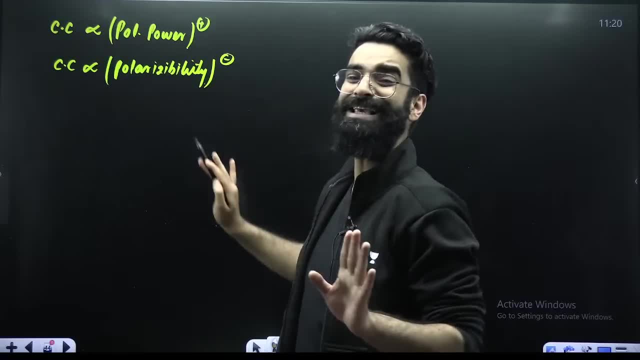 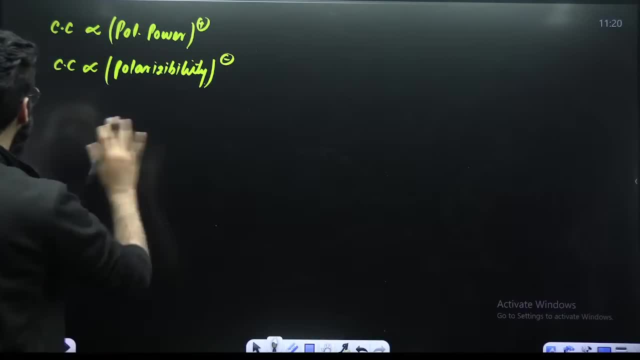 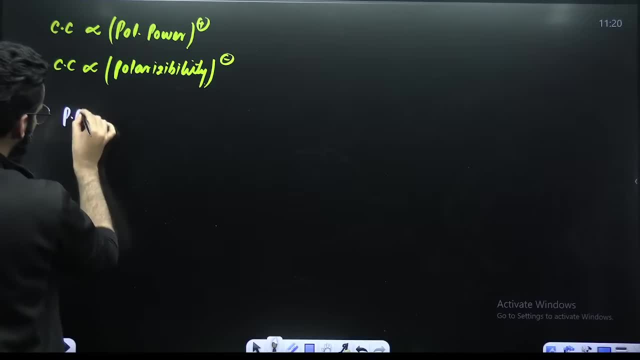 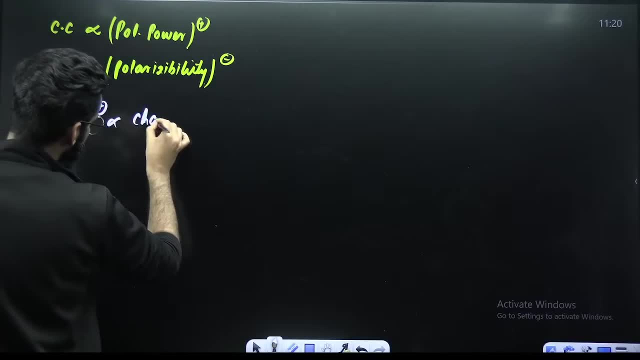 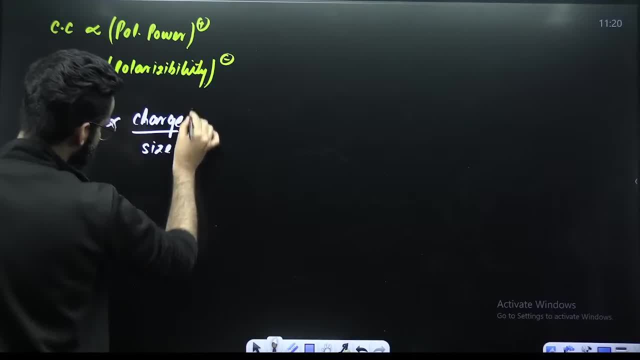 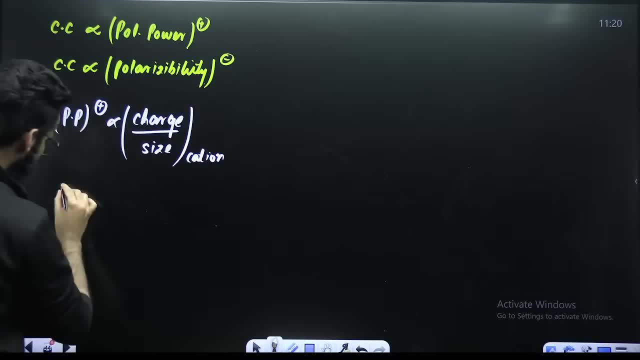 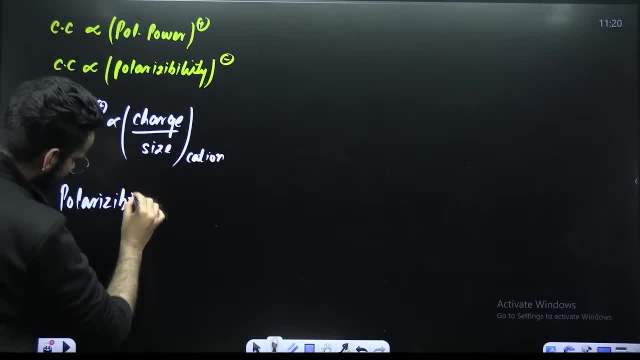 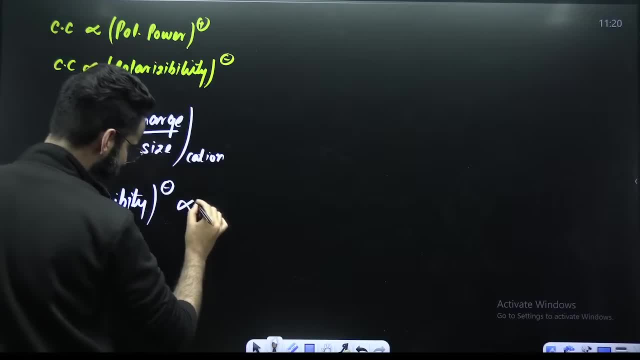 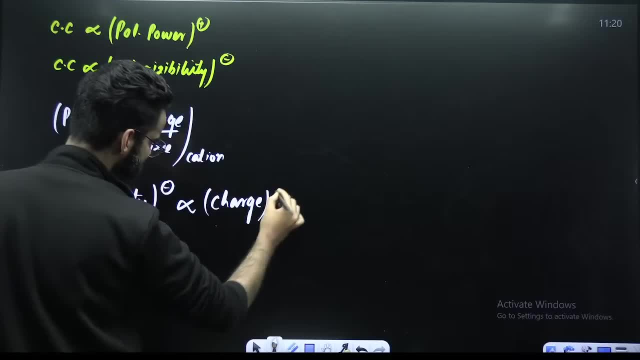 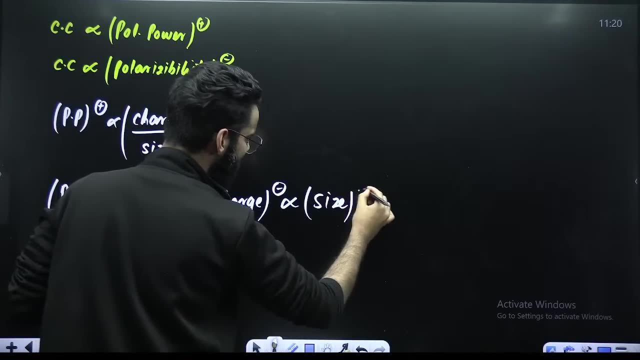 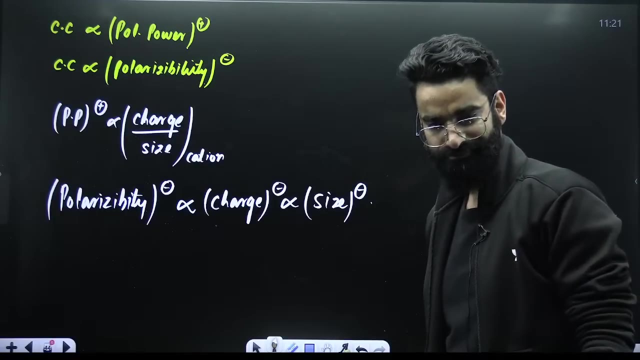 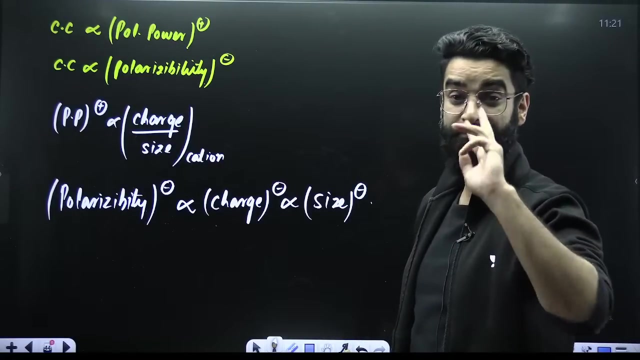 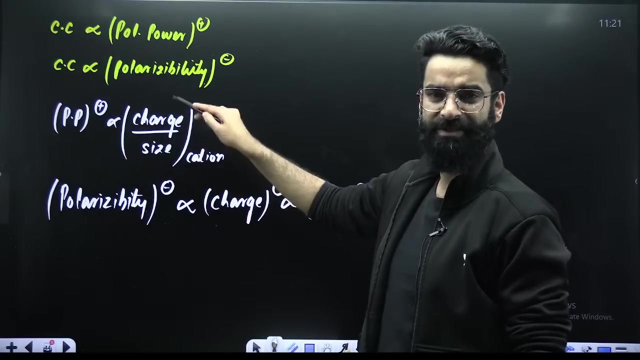 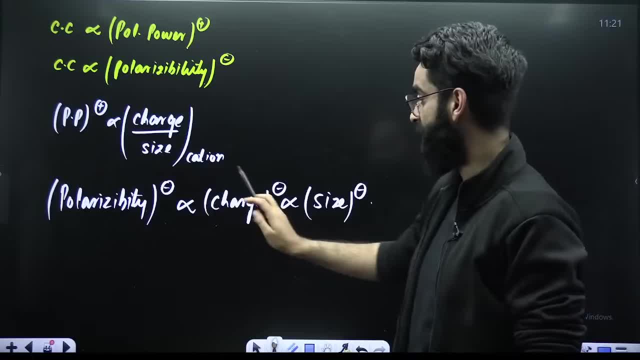 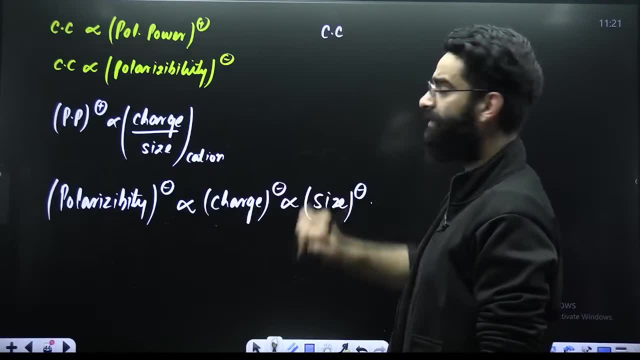 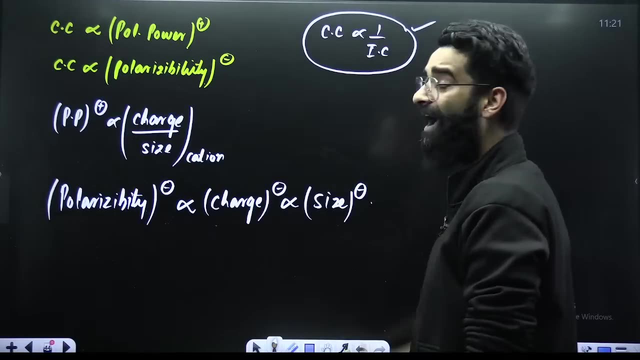 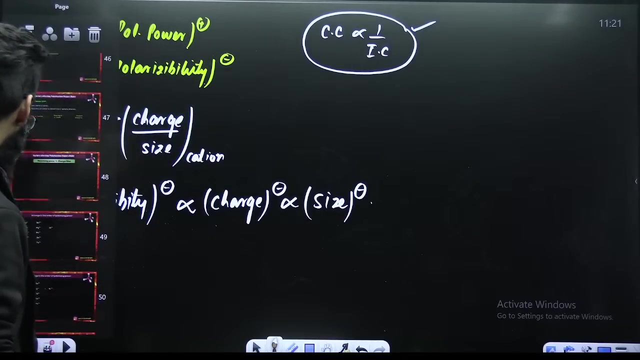 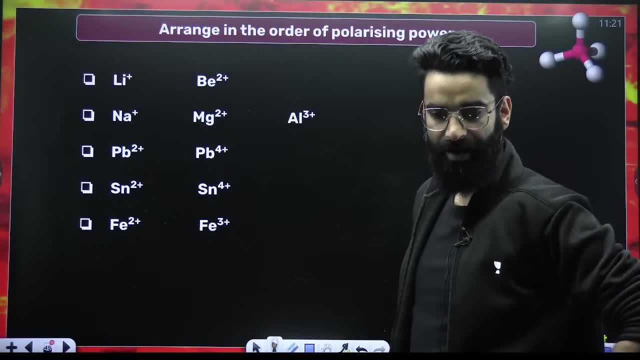 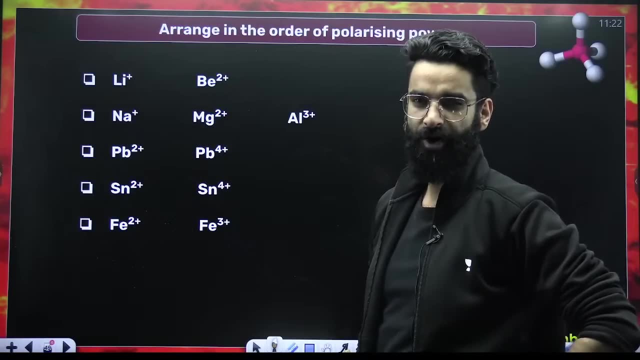 Polarizing power: Quickly, Quickly, Quickly. Arrange the following on the basis of polarizing power. Quickly, Li positive, Be positive. Polarizing power of ketone Depends on two factors: Charge and size. Prioritize size, Charge first, Right. 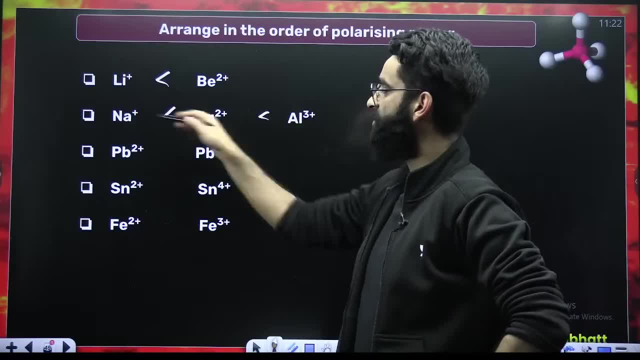 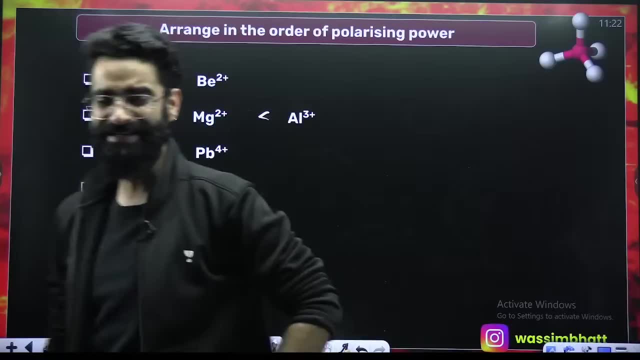 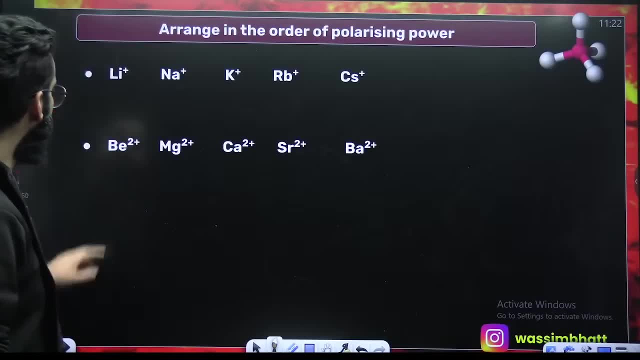 And more the polarizing power of ketone. Okay, Li, positive Na, positive K, positive Rb, positive Cs, positive Charge. everywhere is same, But size of these ketones is different. Lesser the size, more the polarizing power. 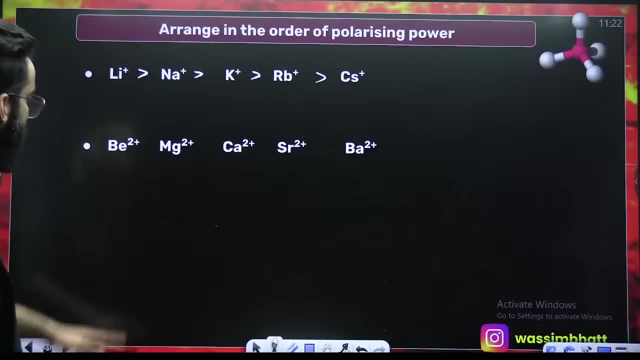 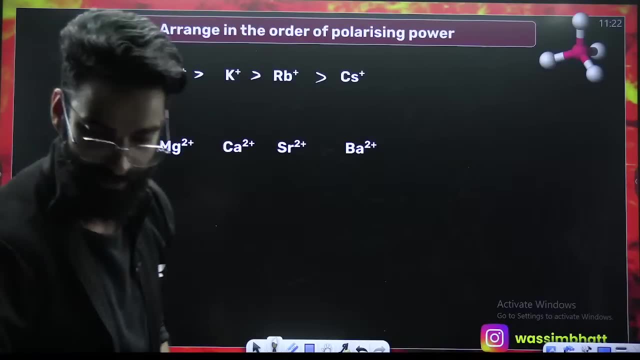 Lesser the size, more the polarizing power. of the ketone: Right Be positive, Mg positive, calcium positive, strontium positive, barium positive. Down the group ionic size increases: Right: Lesser the size, more the polarizing power. 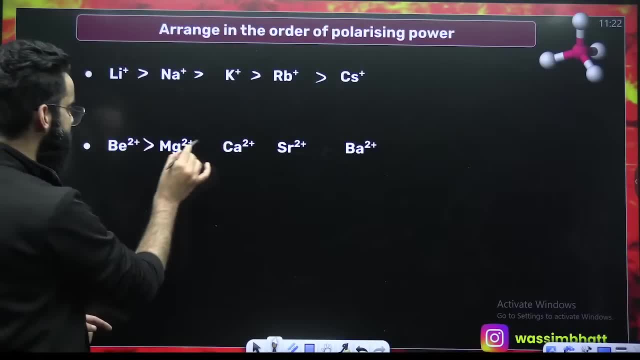 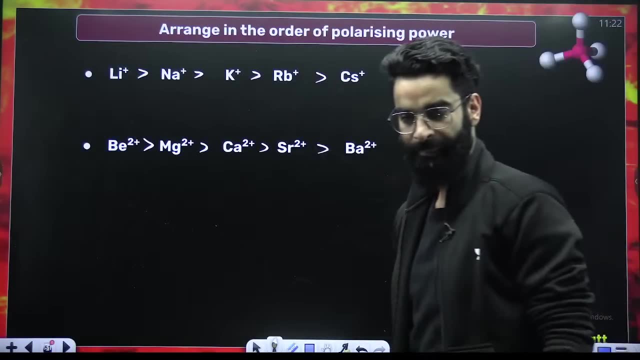 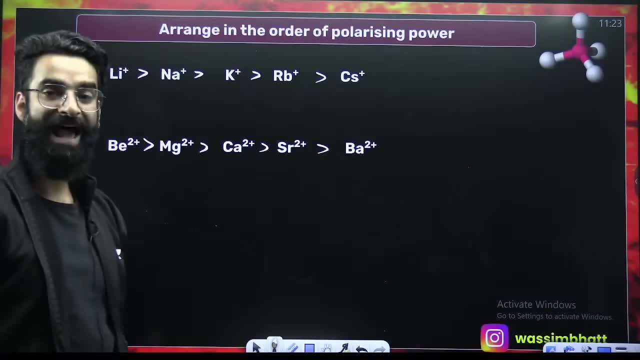 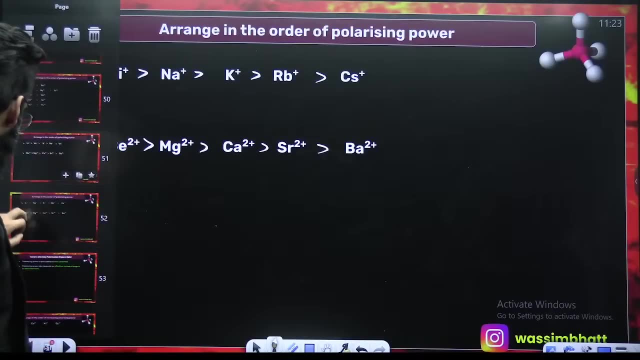 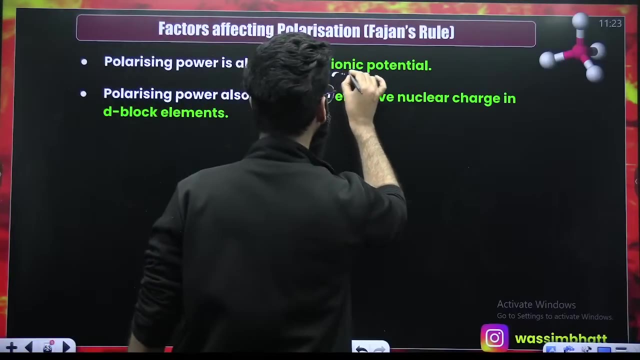 Are these two questions done and dusted? So, people, as you know, your polarizing power, directly proportional to charge, inversely proportional to size, Right, And we are done. We are done. Okay, Remember the polarizing power of the ketone. 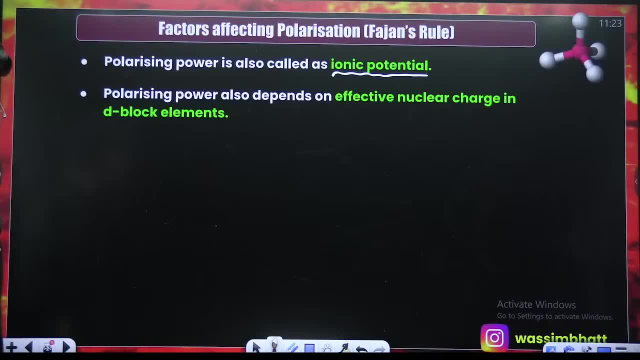 It is also called as ionic potential. It is also called as ionic potential. Sometimes they might ask you a question, not in terms of polarizing power, directly in terms of ionic potential. In terms of ionic potential Right. 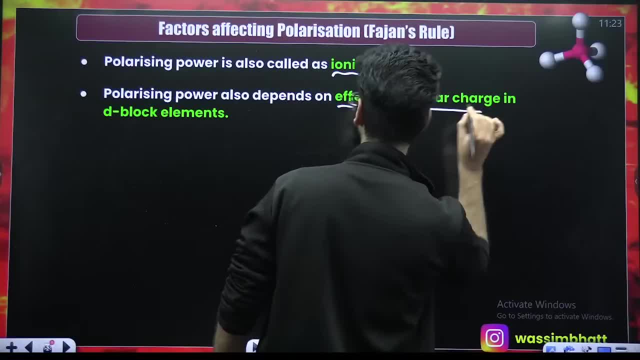 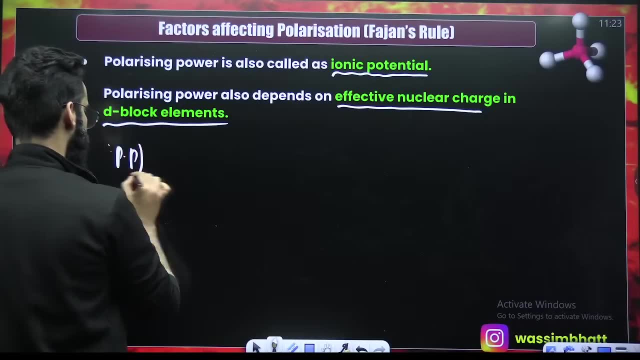 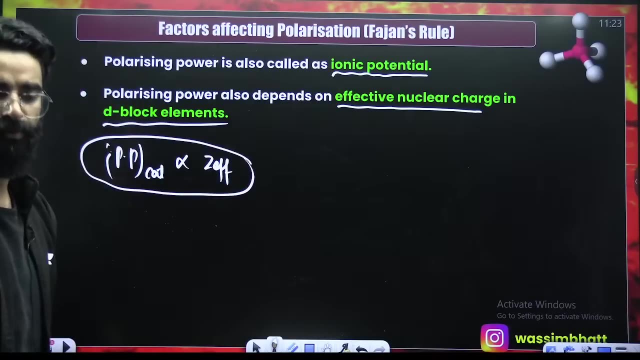 And your polarizing power. it also depends on the effective nuclear charge. in case of the d-block elements, More the effective nuclear charge, more the polarizing power. More the effective nuclear charge, more the polarizing power. In case of what? In case of d-block. 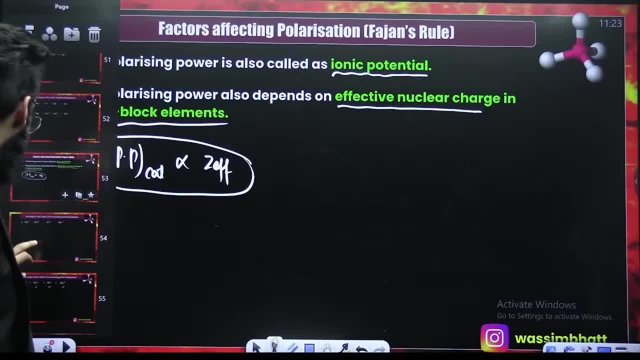 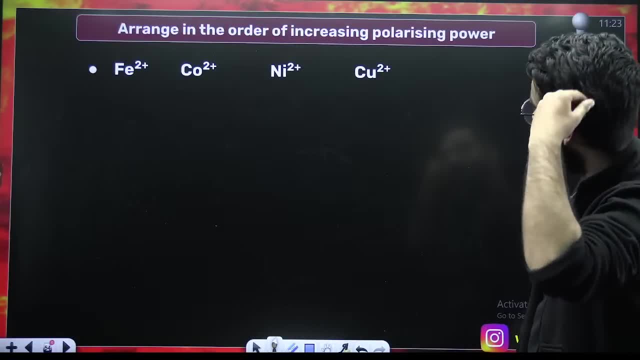 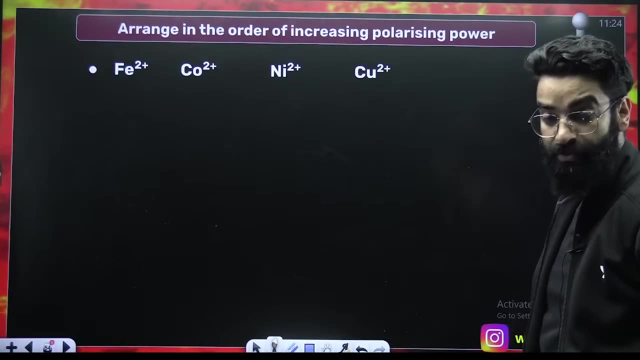 elements. In case of d-block elements. In case of d-block elements, Now, Fe di-positive- these are all d-block, Fe di-positive, Cu di-positive, Na di-positive, Cu di-positive, Quickly Polarizing power. it depends, also depends on effective. 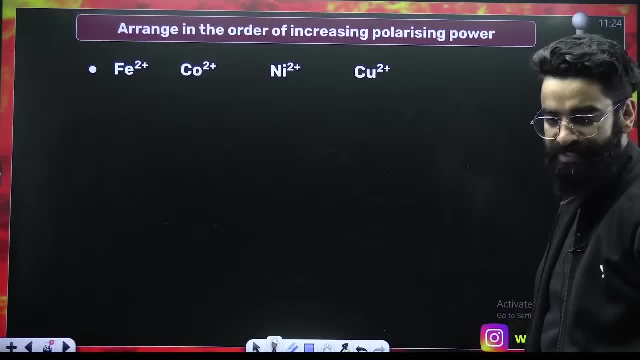 nuclear charge. in case of d-block elements, Tell me which one has got more polarizing power, Where the effective nuclear charge is more Right, Effective nuclear charge is more. Which one has got more effective nuclear charge? It's copper di-positive. 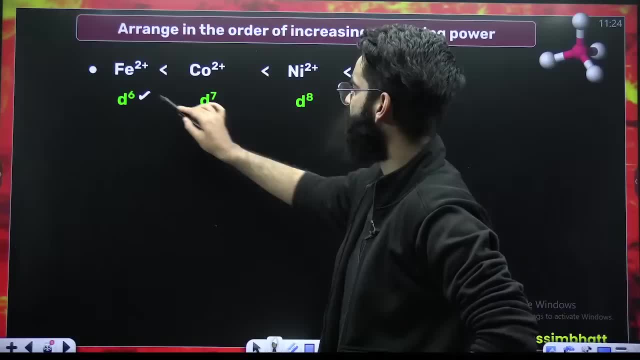 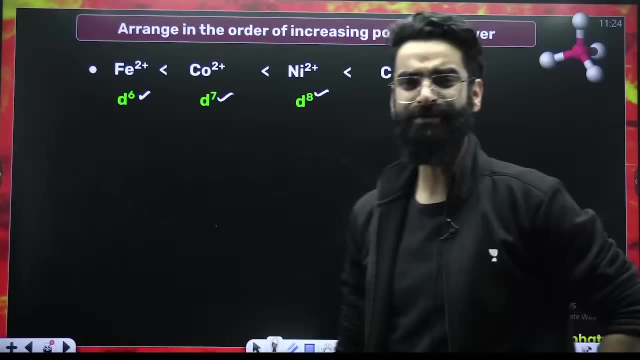 Copper di-positive will have maximum polarizing power Since it has d-6 configuration, d-7,, d-8, d-9.. Perfect. And in case of d-block elements generally, on moving from left to right, what happens to the effective nuclear charge? 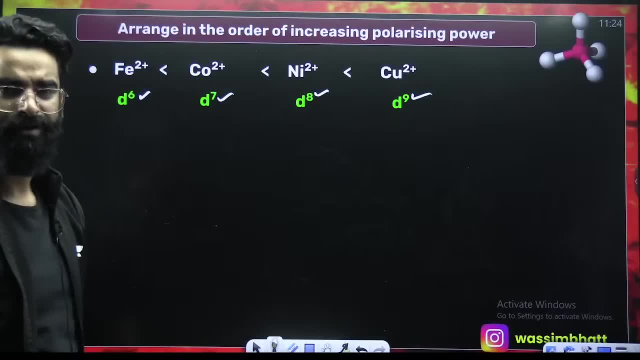 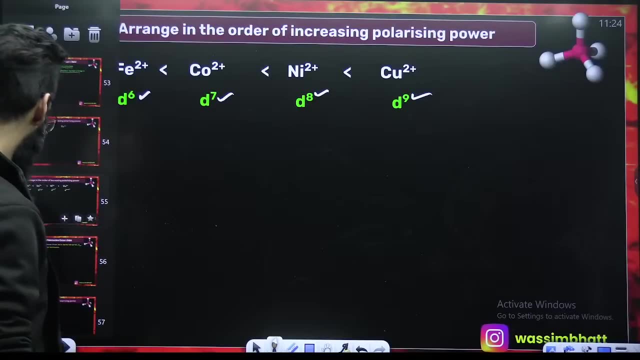 Effective nuclear charge increases. therefore, polarizing power is going to be maximum for Fe, di-positive Right, Particularly. in case of what? In case of d-block, In case of d-block elements. Do remember one more thing On moving from 3D. 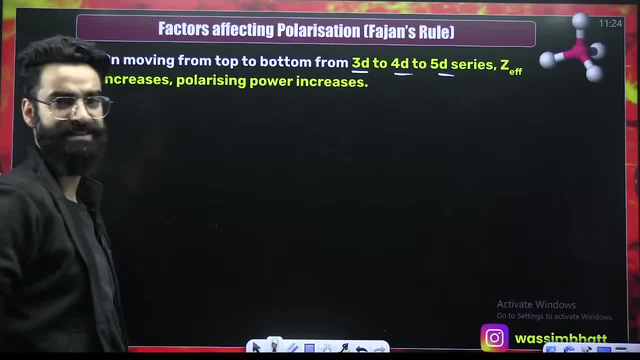 to 4D to 5D, 3D series to 4D, 5D series to 5D series. Right Effective nuclear charge increases, hence polarizing power also increases. 3D, 4D, 5D. 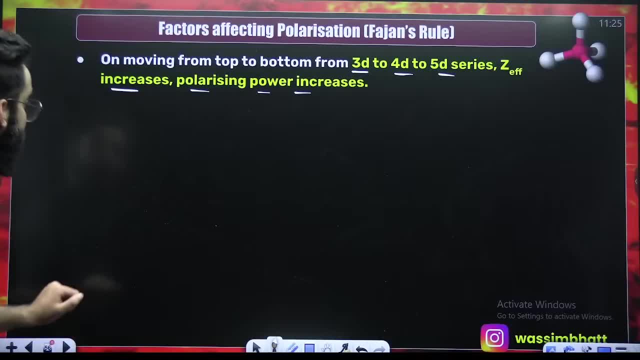 Effective nuclear charge down. the group increases Right. So polarizing power of ketines increases. Now if I ask you which one has got more polarizing power? This is the 3D element. This is the 4D element. 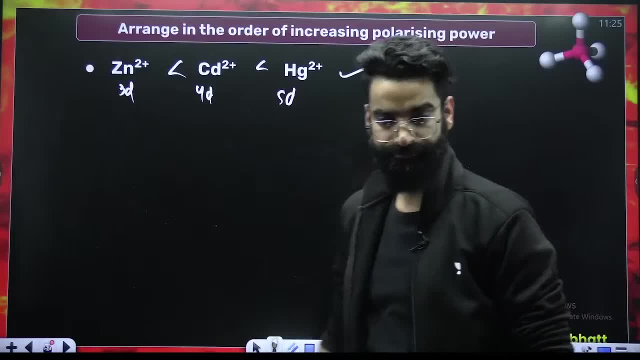 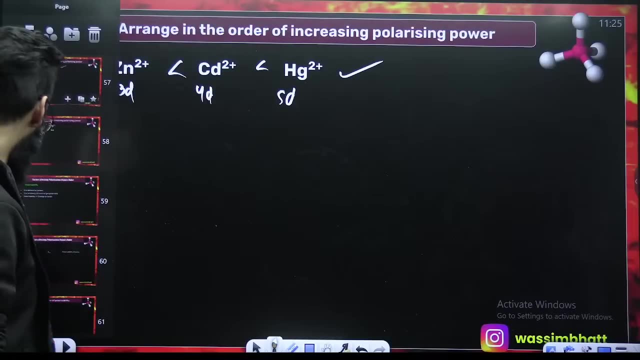 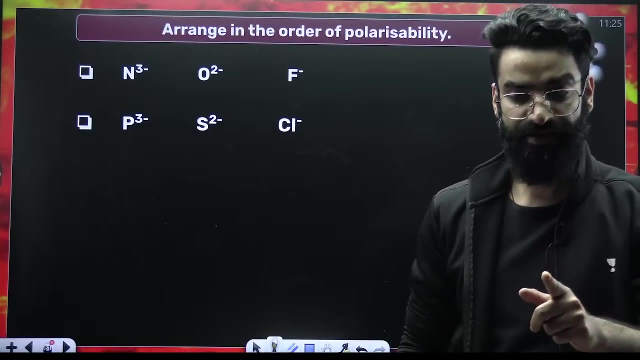 This is the 5D element. 5D will have more polarizing power Done and understood. It has got more polarizing power done and dusted- right. it has got more polarizing power done and dusted. now, if you talk about the polarizability which is defined for anion, which is defined for anion, 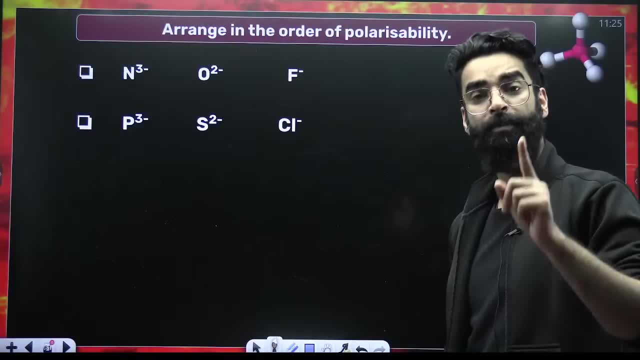 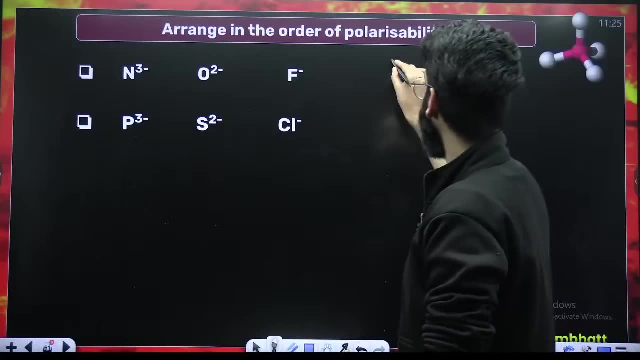 which is defined for anion. you know, as i told you, polarizability: it is directly proportional charge, it is directly proportional to size of anion as well. okay, polarizability: polarizability of anion is directly proportional to charge on anion and, at the same time, it is 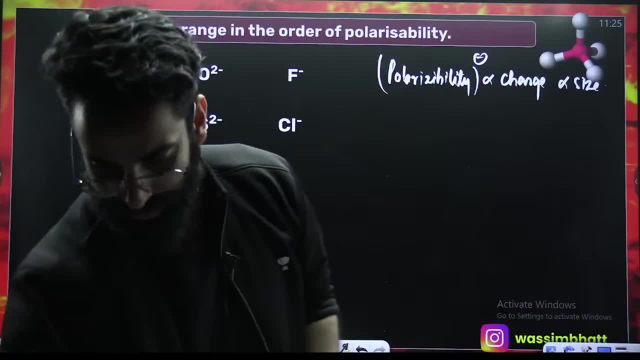 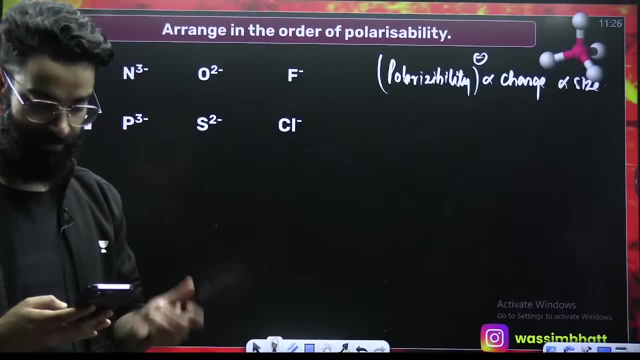 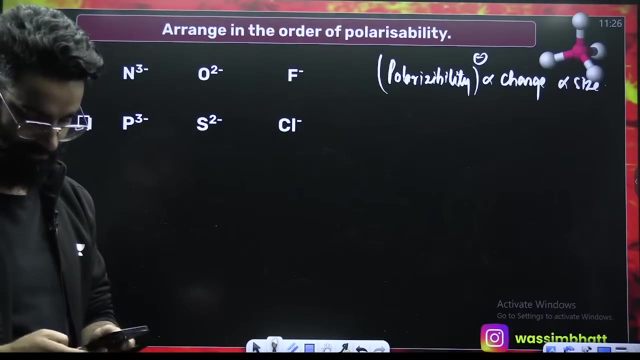 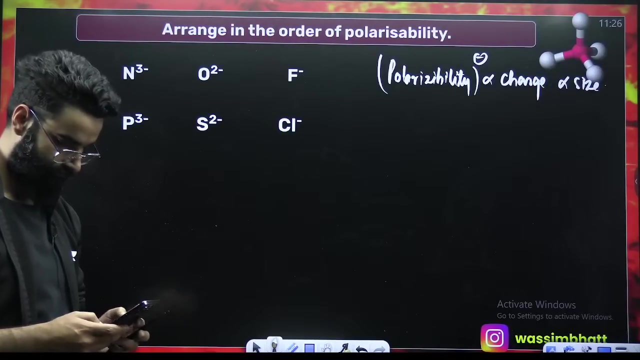 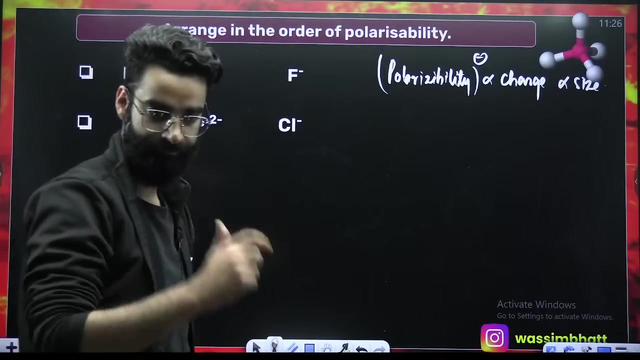 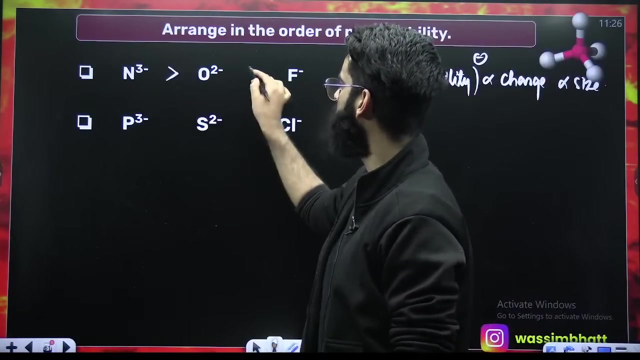 directly proportional to size of anion. it is directly proportional to size of anion. right, it is directly proportional to size of anion. yeah, it is directly proportional to size of anion. tell me the order quickly, quickly, guys: n tri negative o di negative, f negative, more the charge, more the polarizability. 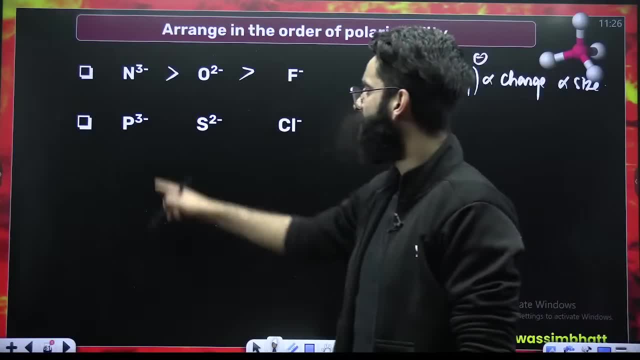 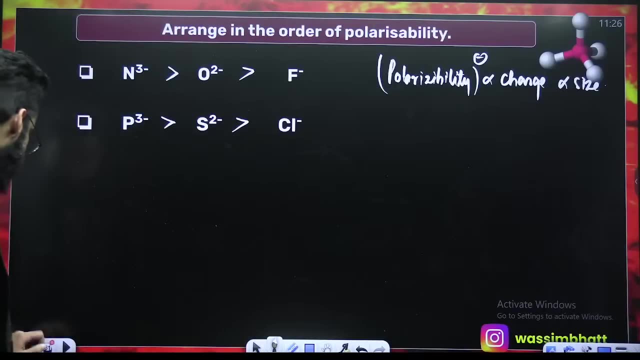 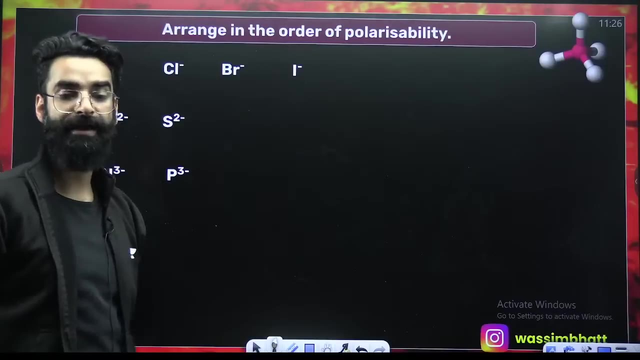 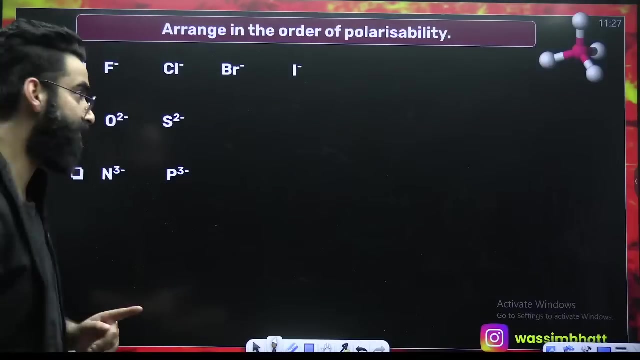 of anion. okay, p tri negative, s, di, negative, cl, negative. more the charge, more the polarizability right, more the polarizability done, more the polarizability f, negative, cl, negative, br, negative, i, negative charge on every anion is same. talk about size. polarizability is directly proportional to size as well. more the size of anion, more the 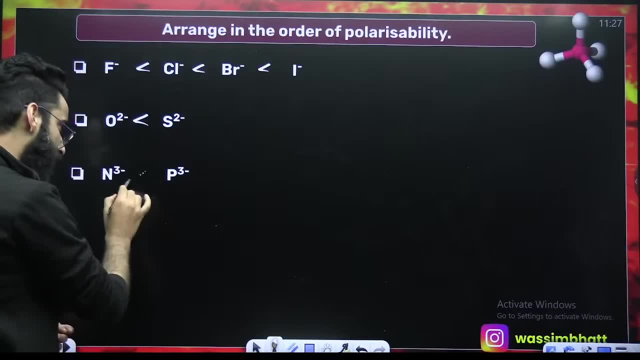 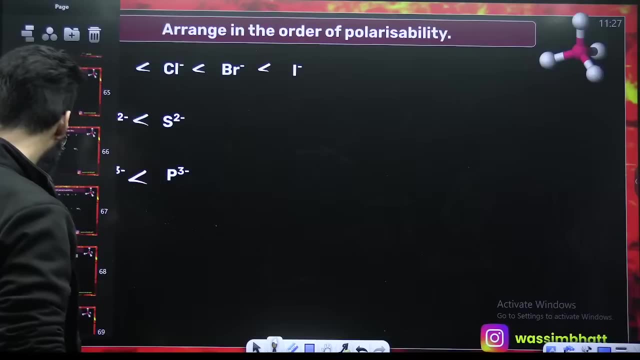 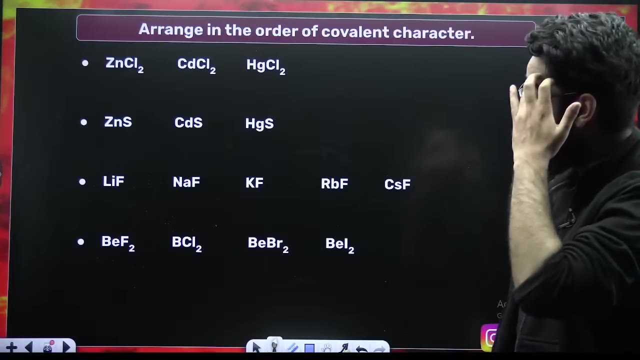 polarizability: more the size of anion, more the polarizability. more the size of anion, more the polarizability. done, done, people. okay, now here are the equations. here are the equations. here are the equations which are asked. here are the equations: zm, cl two, cdcl, gcl two. arrange them on the basis of covalent. 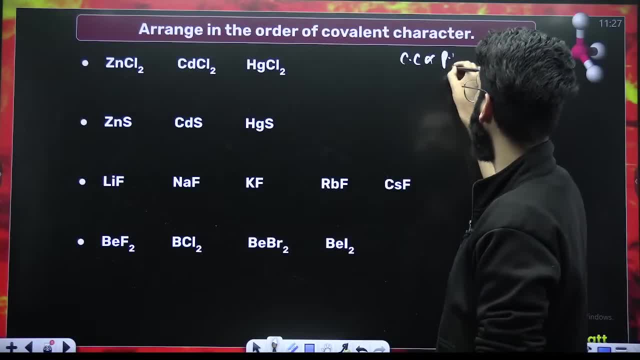 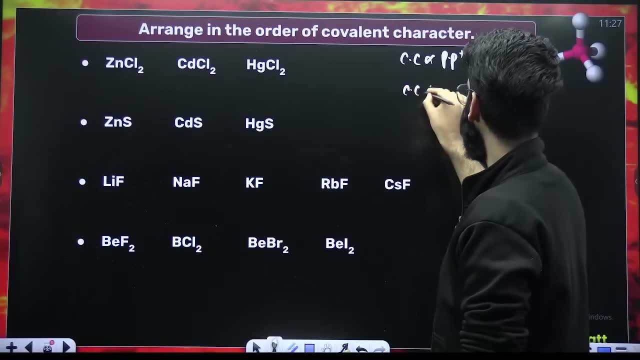 character, you know, covalent character. it is directly proportional to polarizing power of cation and it's inversely proportional to sorry it is. it is directly proportional to scales, breakdown, imaginary dimensional, the kennel parameters of all negatives. we will gone to this, to polarizability of. 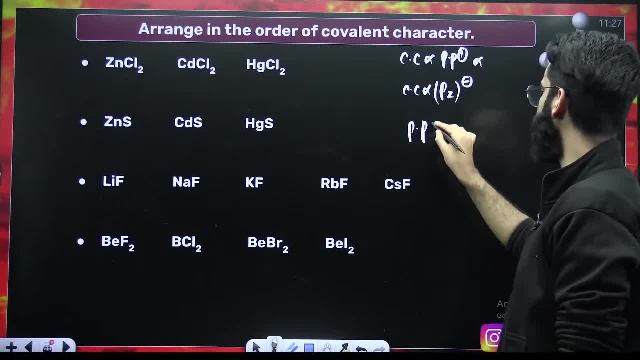 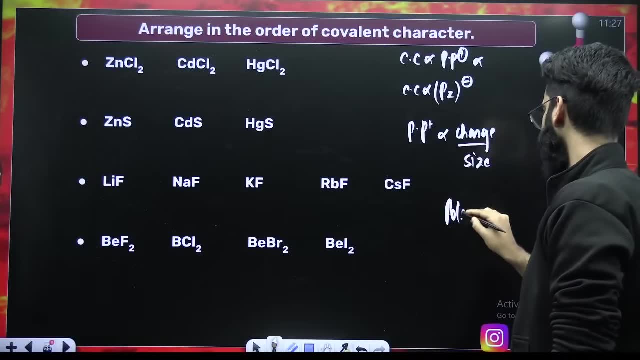 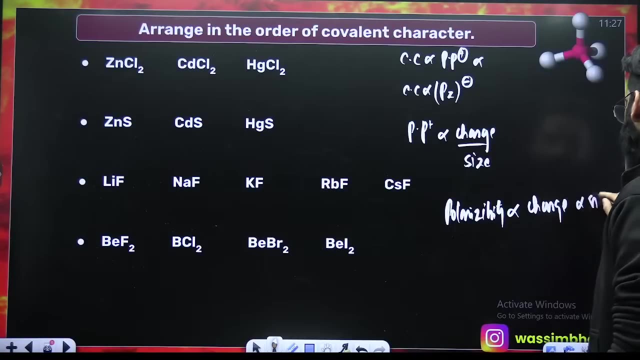 anion as well. Right, And you know your polarizing power of cation, directly proportional to charge of cation, inversely proportional to size of cation. polarizability is directly proportional to charge on anion, directly proportional to size of anion as well. Think carefully. 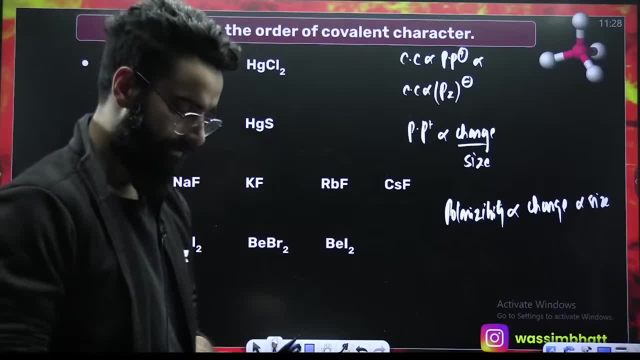 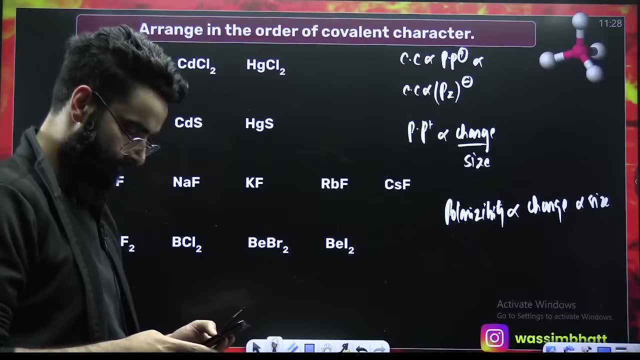 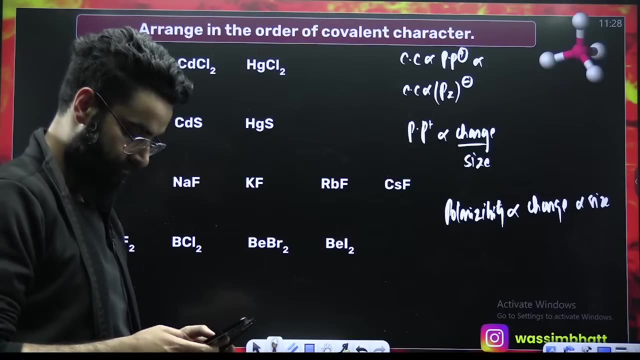 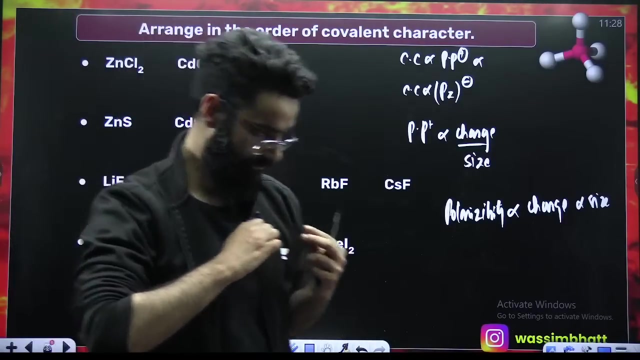 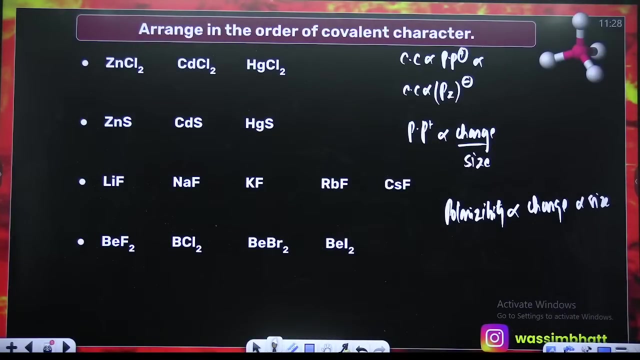 now, Think carefully, Think carefully, people. Guys, just give me a second, I'll be back. Just give me a second, Okay, Are you done with this? Are you done with this? My dear students, if you look carefully, this is Zn di positive. this is. 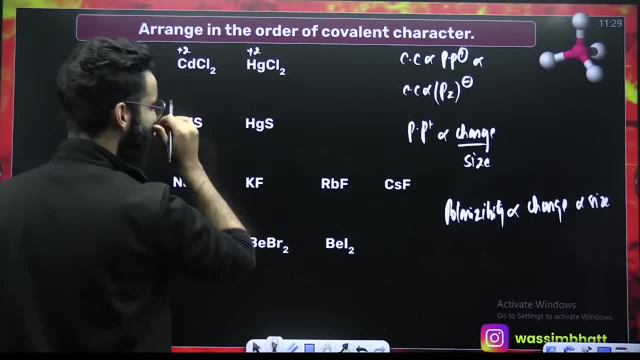 Kp. This is Zn di positive, Cadmium di positive. This is Hg di positive Right Cl negative. Anion everywhere is same, So leave the anion aside. Look at the cation. Look at the cation. 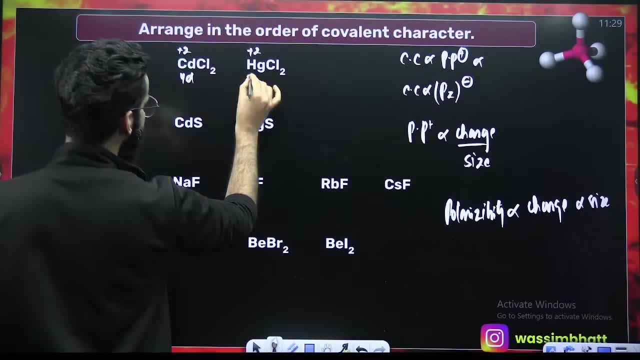 people. This is your 3D, This is 4D element, This is 5D: 3D to 4D, 4D to 5D. What happens? Effective nuclear charge increases. Effective nuclear charge increases Polarizing power. 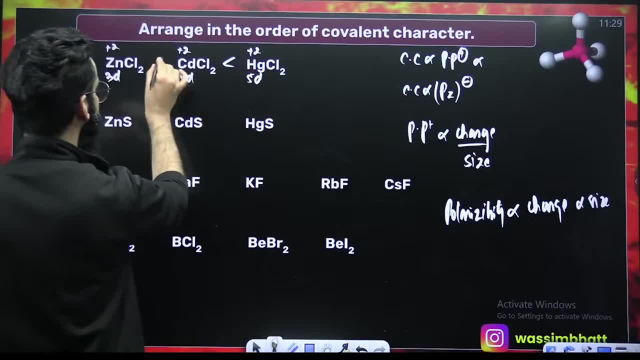 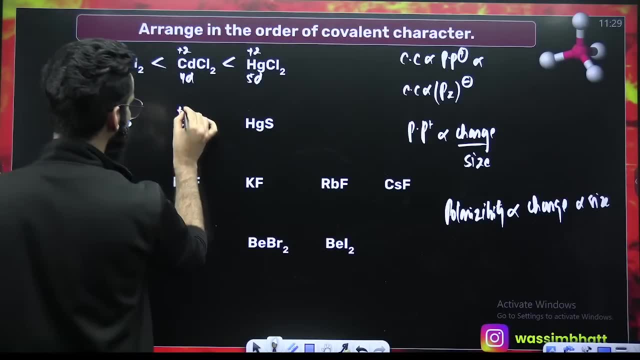 increases Polarizing power increases Covalent character increases. So this is the order of covalent Right. Look at the next one: Zn di positive Cadmium, di positive Hg, di positive N-ion- everywhere is same. N-ion, everywhere is same. 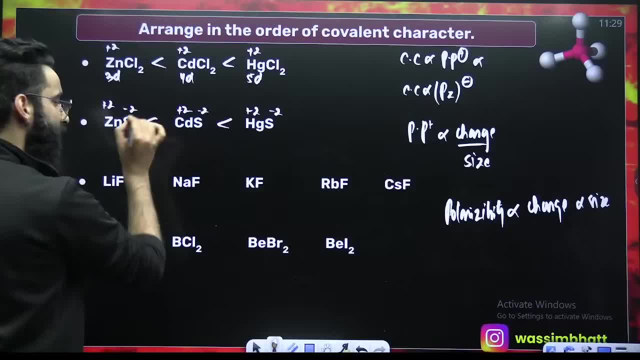 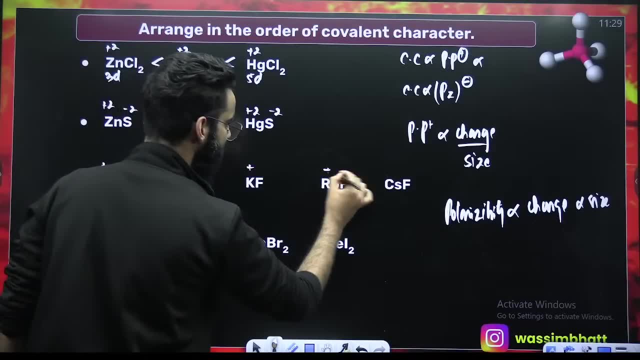 Right, This is 3D. This is 4D. This is 5D. Right, Perfect. This is the order Done. Look at the next one: Li positive Na positive K positive Rb, positive Cs positive. 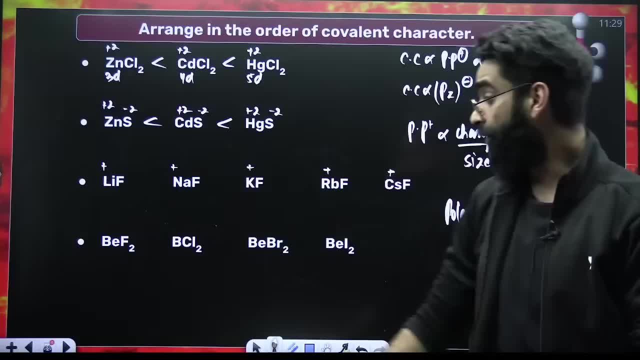 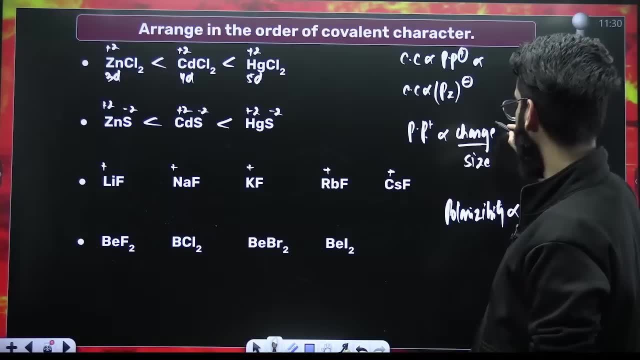 N-ion. Leave the N-ion aside. N-ion is everywhere, same Right. Look at the cations. now For cations, what do we define? Polarizing power And polarizing power of cation Breakly proportional charge. Inversely, 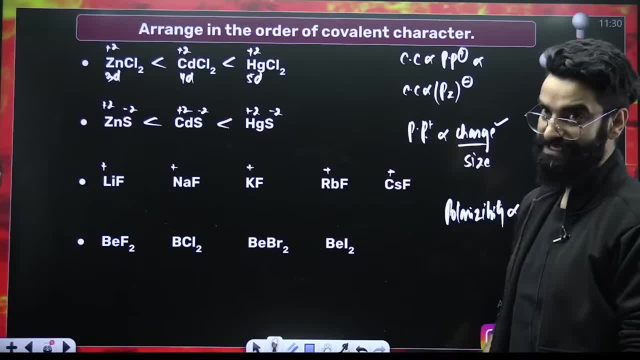 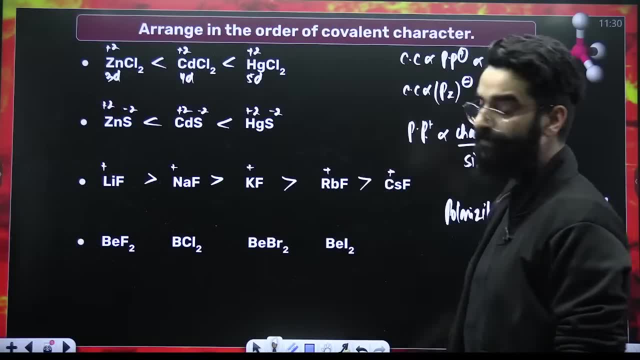 proportional size. Charge on every cation is same Now size: Lesser the size, more the polarizing power. Lesser the size, more the polarizing power, More the polarizing power of the cation, more is the covalent character. 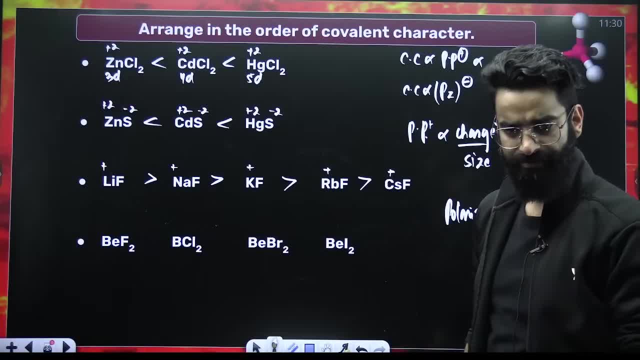 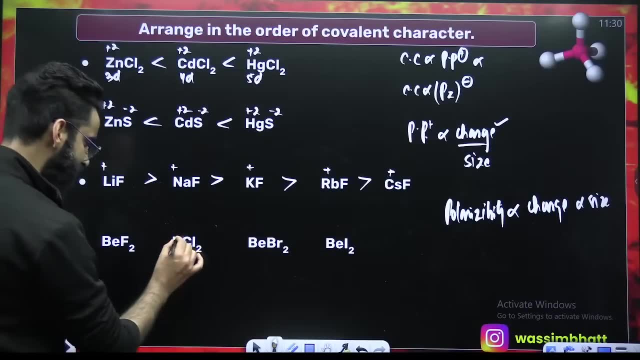 Done. Okay, Look at the next one. Look at the next one, guys, Look at the next one. This is Be here, Okay, This is Be Perfect. So Be di positive F negative. Be di positive Cl negative. 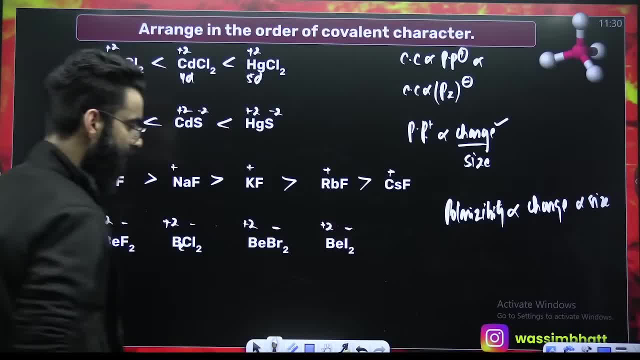 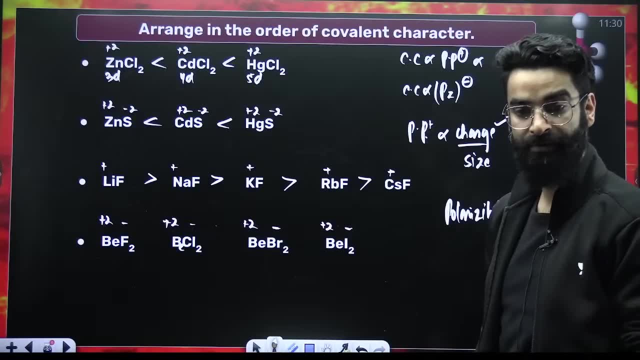 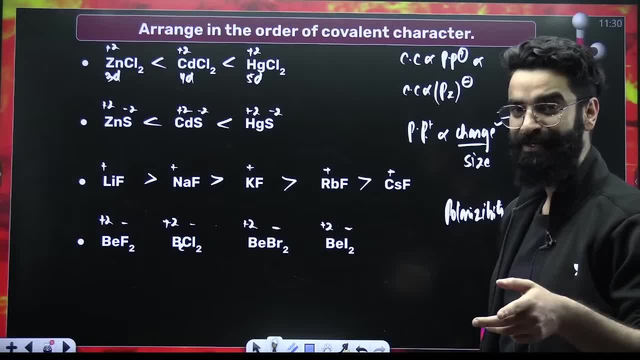 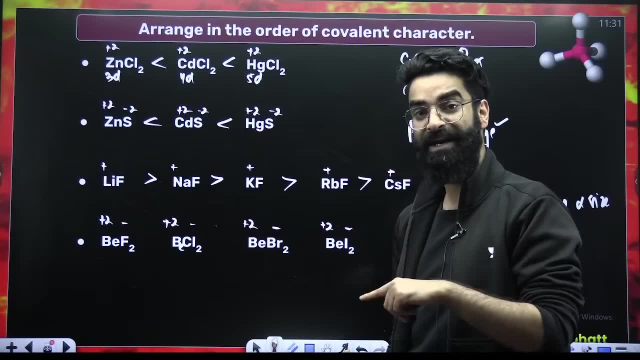 is different For N-ions. what do we define Polarizability? Polarizability Charge on every N-ion is same. Talk about size. More the size of N-ion, More the size of N-ion, More the polarizability. 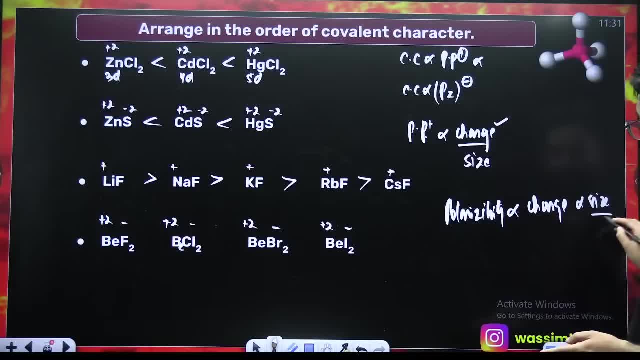 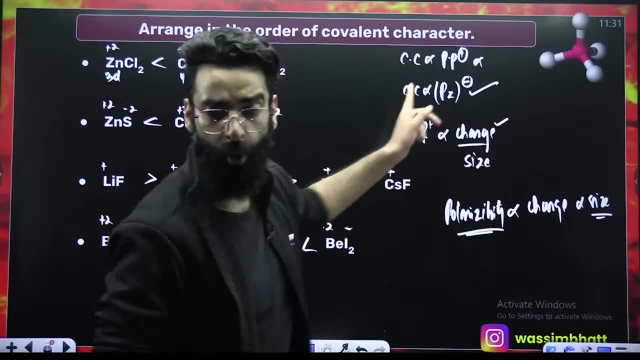 of N-ion, More the size of N-ion, More the size of N-ion, More the polarizability of N-ion And more the polarizability of N-ion, More is going to be the covalent character. These are the covalent character order. 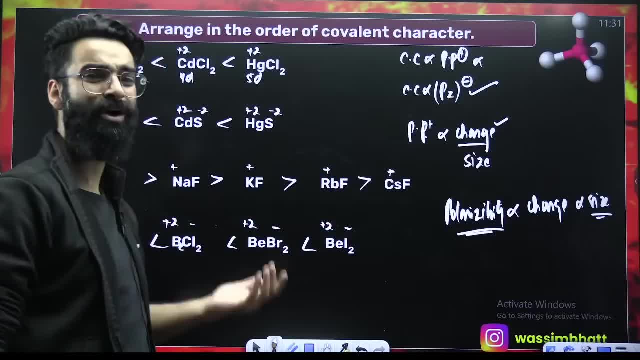 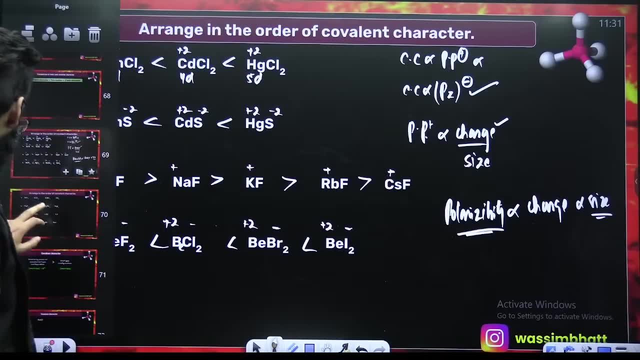 This is the covalent character order. If you reverse these orders, you get the ionic character order, Right? If you reverse all these orders, you get the ionic character order. Okay? Few more questions. Tell me the answer here. 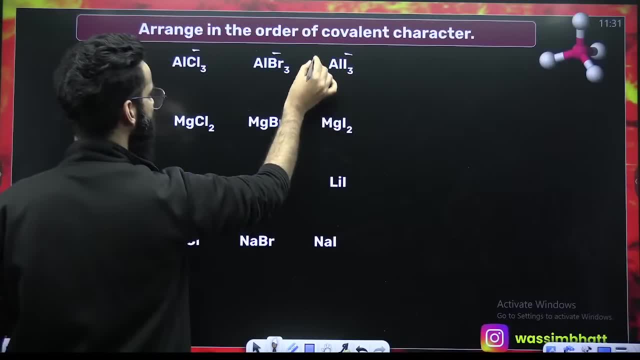 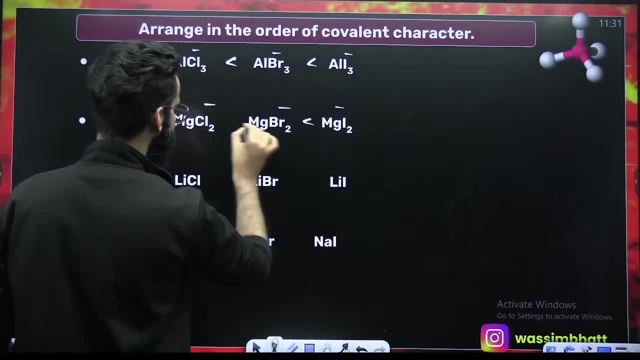 F negative, Cl negative, Br negative, I negative. More the size of N-ion, More the polarizability And more the covalent character. This is F negative, Cl negative. Again the same Right: F negative, Cl negative, Br negative, I negative. 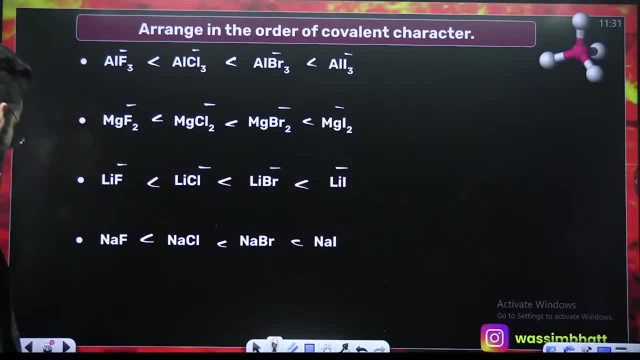 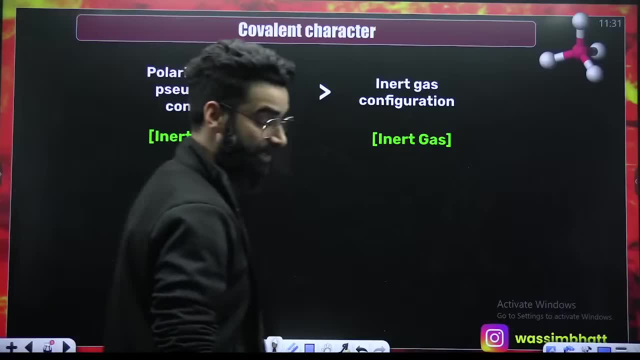 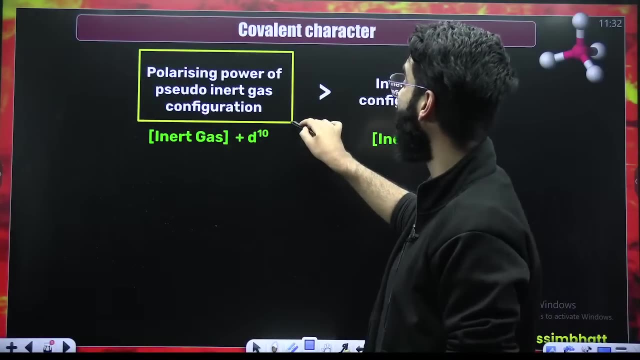 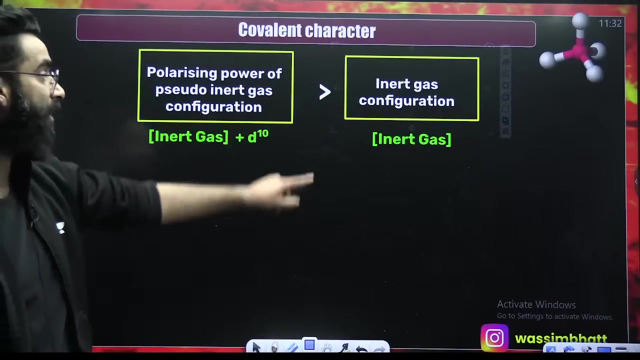 Again, the same, Again, here the same, Perfect, Perfect guys Remember this particular point as well. This is important: Polarizing power. Polarizing power of the pseudo inert gas configuration is greater than that of Polarizing power of the inert gas configuration. 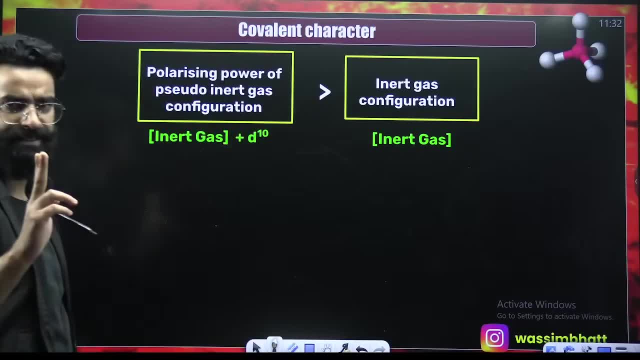 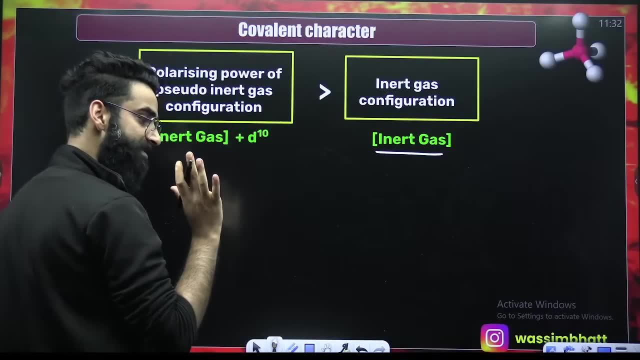 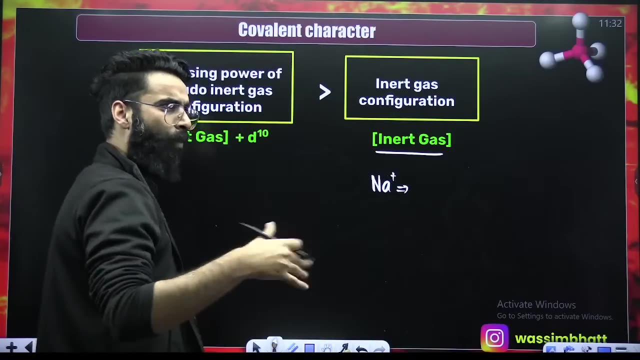 That means if you will be having two cations, If you will be having two cations, One having inert gas configuration, One having inert gas configuration, Like Na positive. Talk about Na positive. Talk about Na positive Right, What is the? 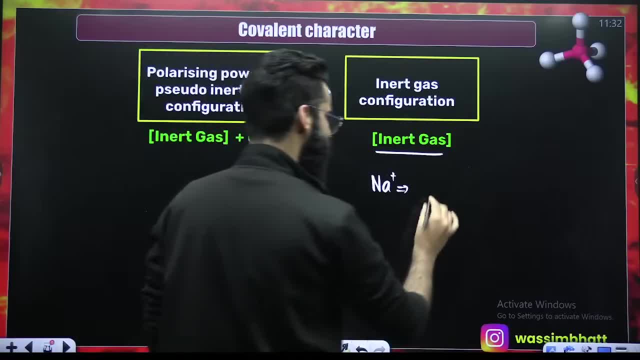 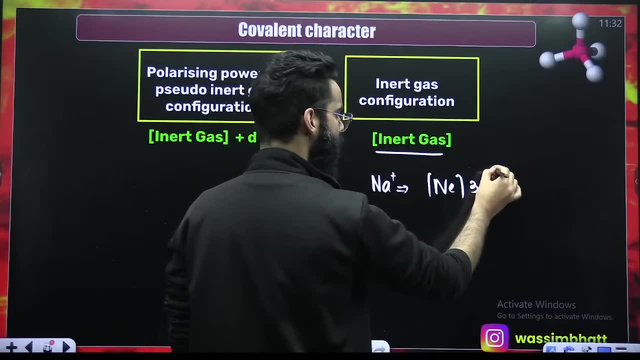 configuration of sodium. basically, What is the configuration of sodium? I will write N-ion, Then 3s1.. But this is Na positive. So take one electron out. If you take one electron out, This is 3s0.. Perfect. 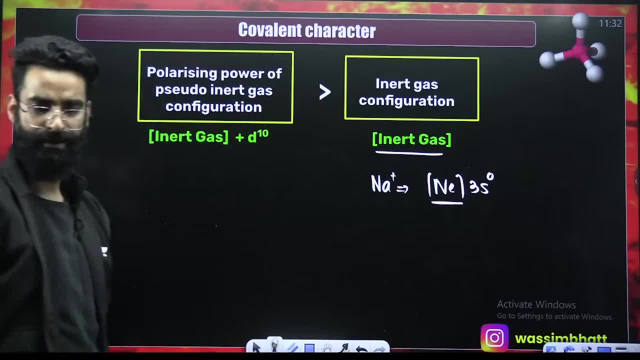 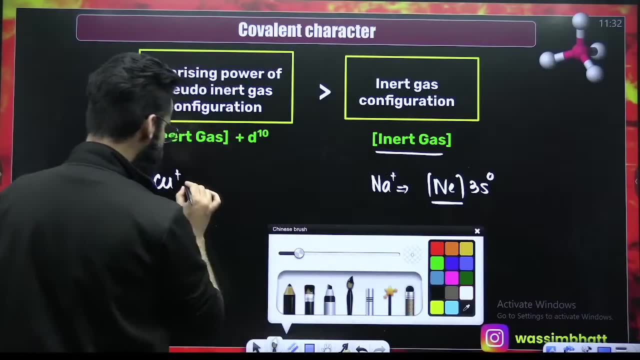 So Na positive has got noble gas configuration, Na positive has got noble gas configuration. But if I talk about Cu positive, Cu positive, What is the configuration of Cu? I will write argon 3d10.. 4s1.. 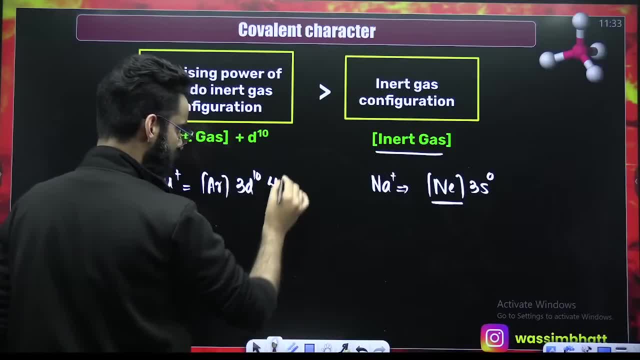 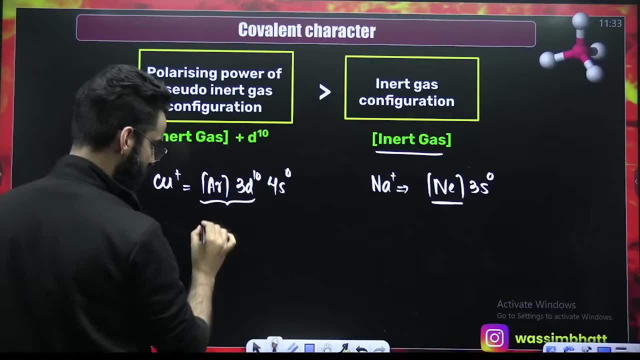 But this is Cu positive. Take one electron out. If I take this electron out, If I take this electron out, This particular configuration, Noble gas With d10 configuration. Noble gas with d10 configuration. This is called as pseudo noble gas configuration. 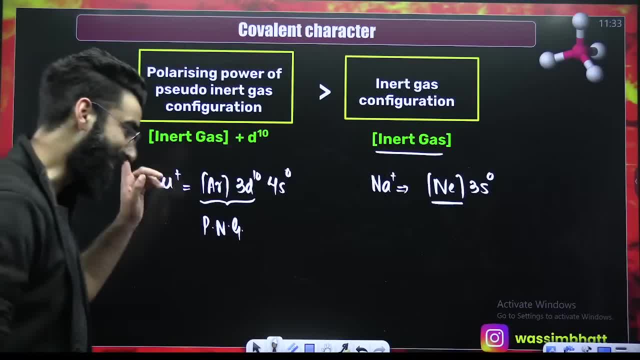 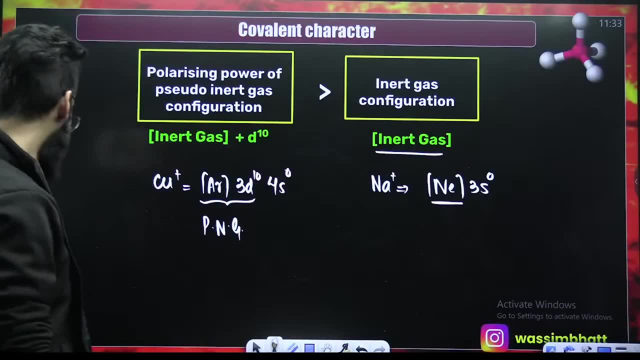 This is called as pseudo noble gas configuration. This is called as pseudo noble gas configuration. That cation which has got pseudo noble gas configuration will have more polarizing power. More polarizing power means more covalent character. Why I told you this one. 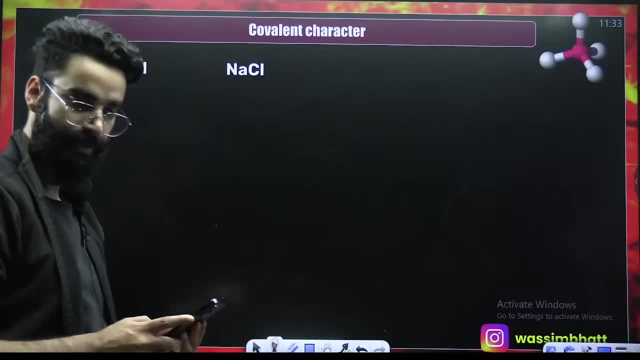 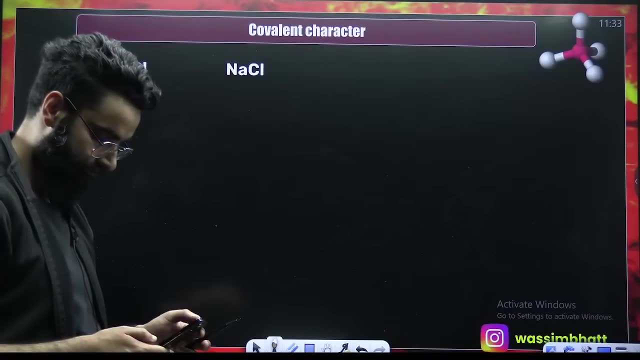 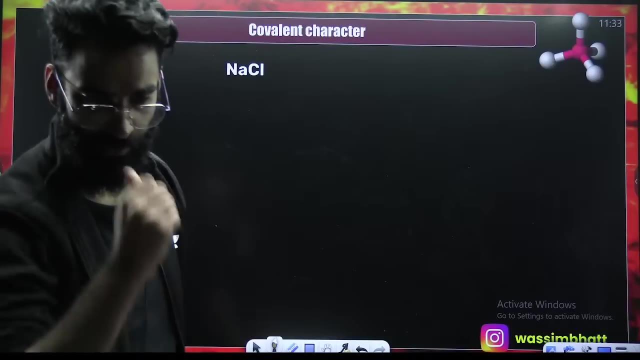 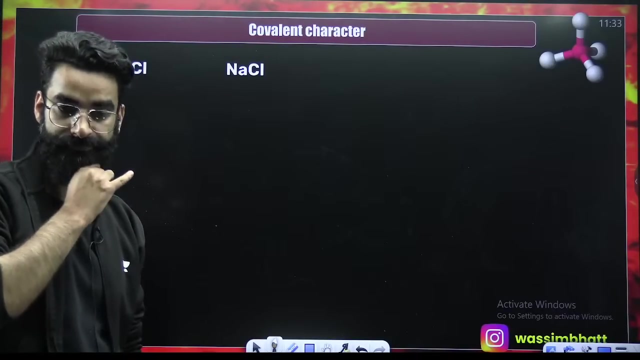 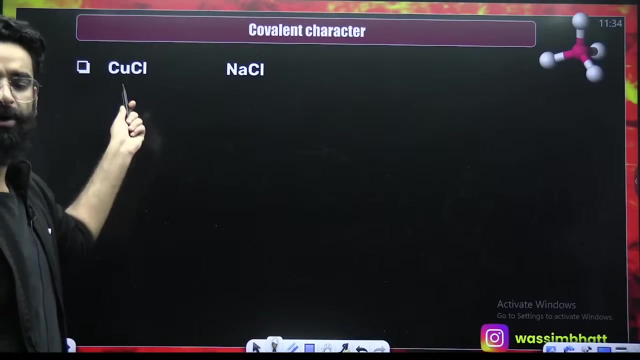 Because you have to solve this question. Tell me the answer of this one now. Quick, Quick people. Quick people, Quickly guys, Quickly, Quickly. Everyone Cu positive. Na positive. Cu positive has got pseudo noble gas configuration. Na positive has got noble gas configuration. 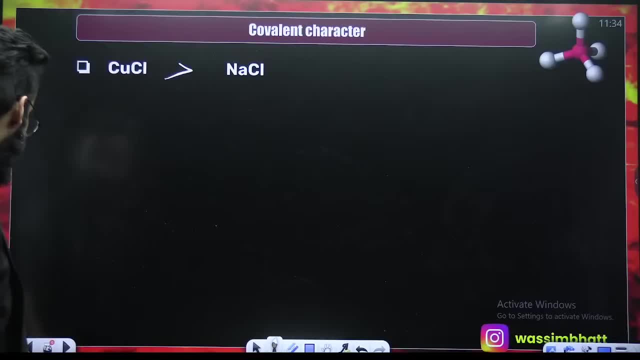 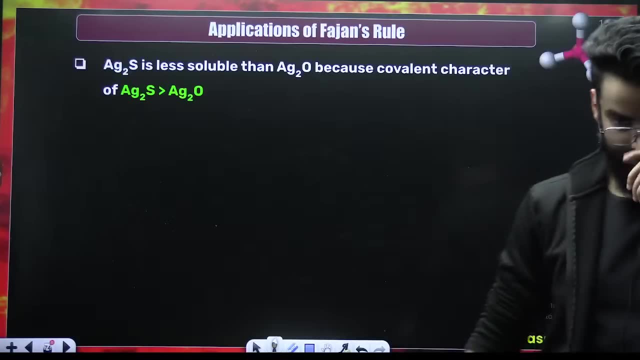 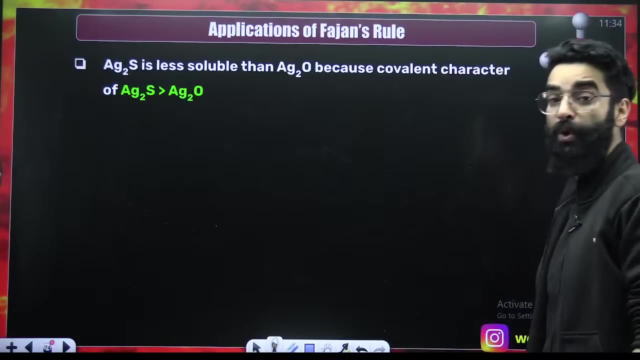 Polarizing power here is more, Covalent character is more Done. There are some applications of this Fajan's rule as well. Some application of Fajan's rules as well. Ideas students: Ag2s is less soluble than Ag2o. 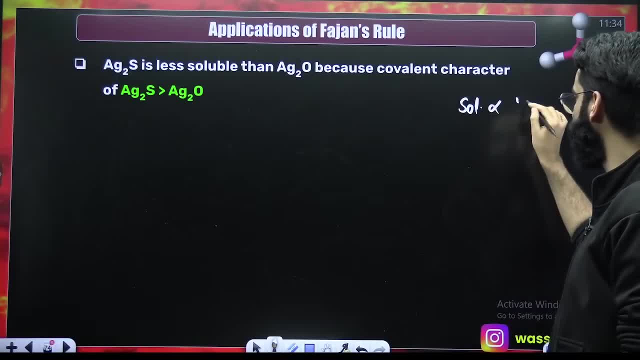 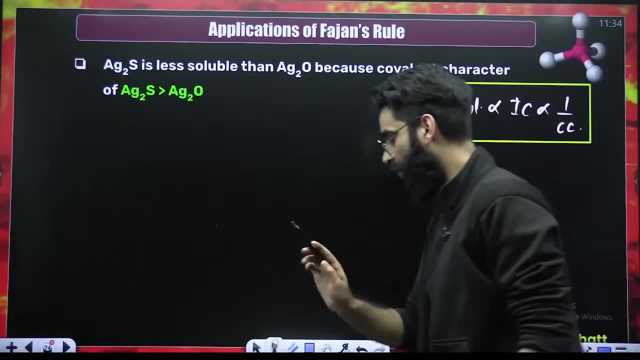 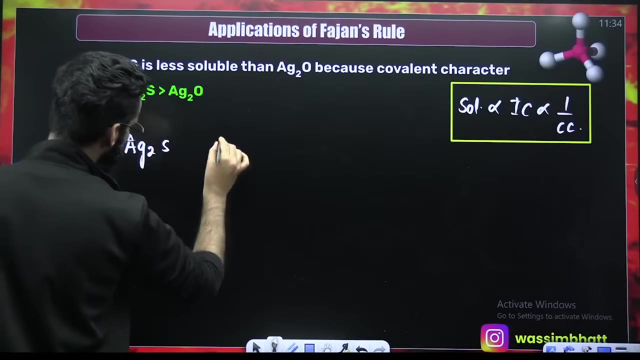 Remember: the solubility is directly proportional to ionic character. It is inversely proportional to covalent character. Remember this particular statement directly over here, Now, Now, Now, Talk about your Ag2s, Talk about their Ag2s. 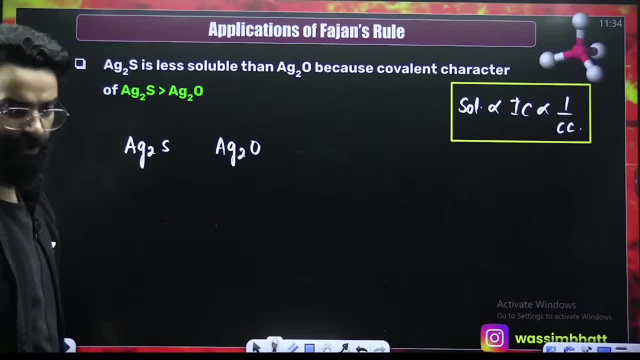 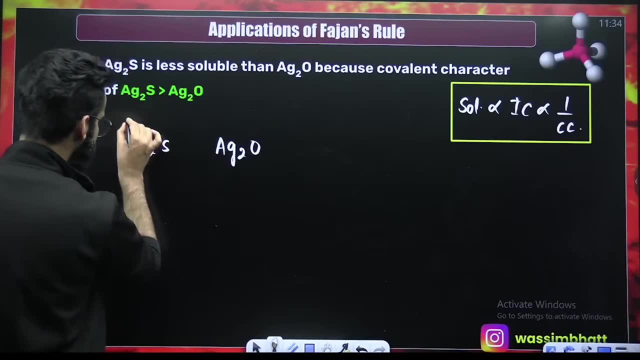 and Ag2o. Give their solubility order. Give their solubility order Right. Solubility order will be decided by the ionic character or covalent character. Understand one thing: This is Ag positive. This is S di negative. Ag positive O di negative. 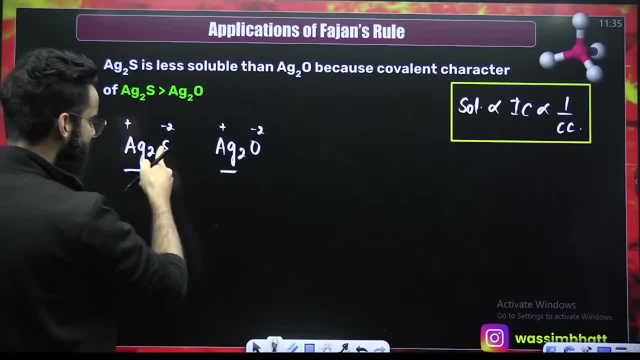 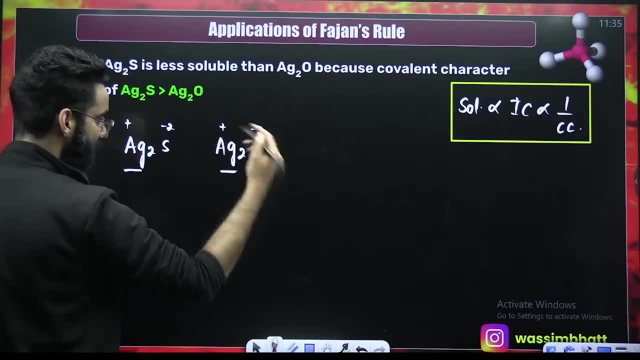 Ag positive here is same, So leave that aside. S di negative, O di negative Charge is same. But look at the size Size of S di negative is more Right. This oxygen, This sulfur, Perfect Down the group size increases. 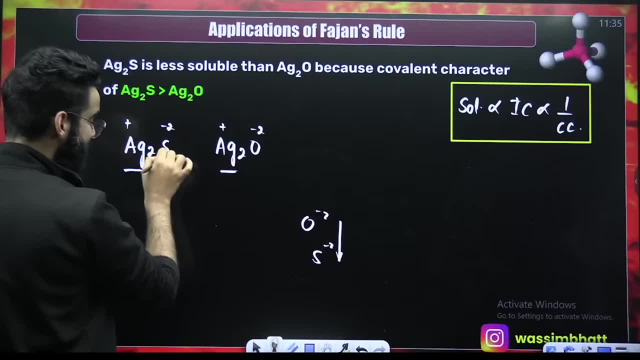 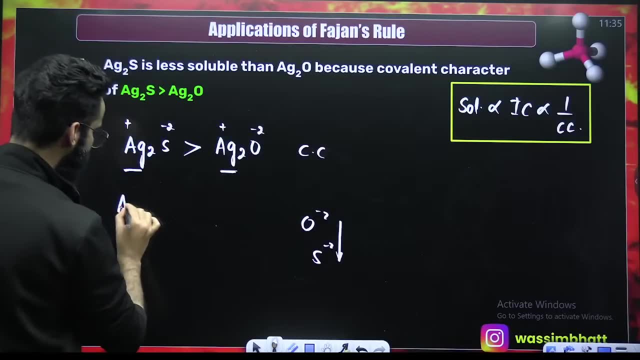 Oxygen of- I mean size of S di negative is more Right, More the size, More polarizability Right, More covalent character: This is the covalent character order. If this is the covalent character order, 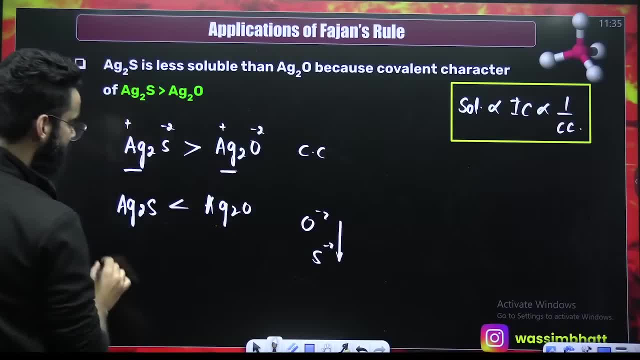 If this is the covalent character order, Give me the order of ionic character. This is the order of ionic character. Whatever is going to be the ionic character order, Same is going to be solubility, So same is the order of solubility. 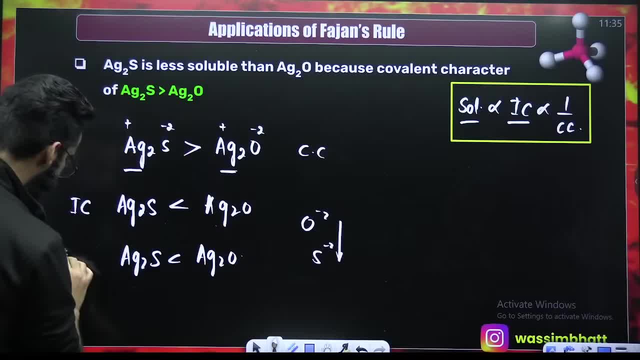 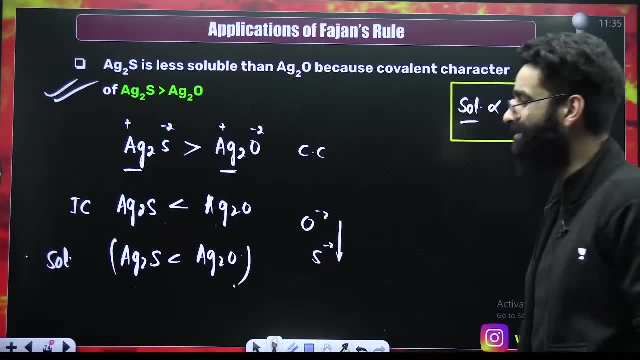 So Ag 2 S: it is less solubile than Ag 2 O. Correct, That is what I had written over here. That is what I had written over here: Simple, simple, simple stuff. Right Number one, Number two: 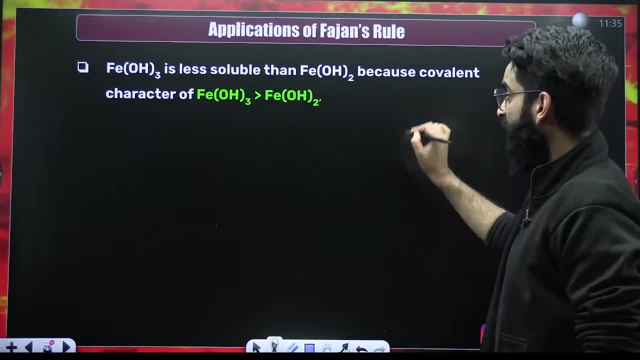 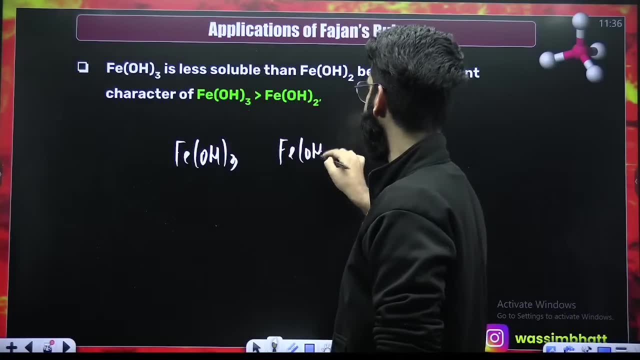 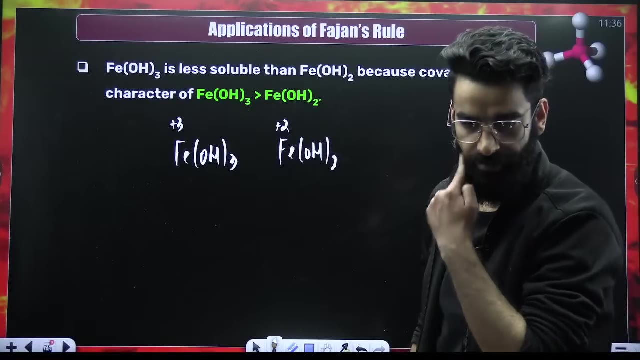 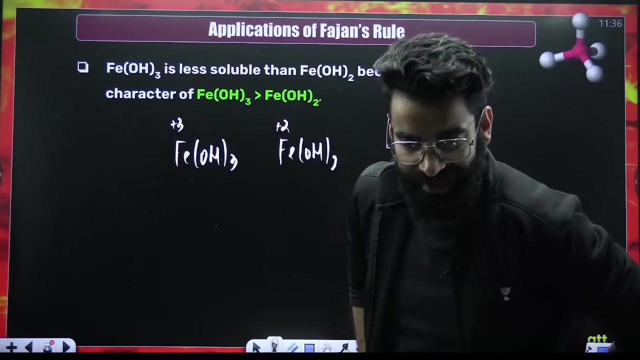 Number two. Number two: If you compare the solubility of FeOH whole trace, hold twice with FeOH. hold twice right. this is Fe tri positive. this is Fe di positive. where is the polarizing power? more polarizing power is more here. this session is for NEET 2024. yes, okay, so polarizing power is more covalent character. 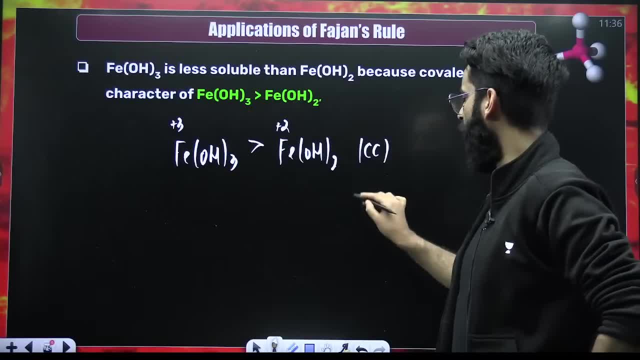 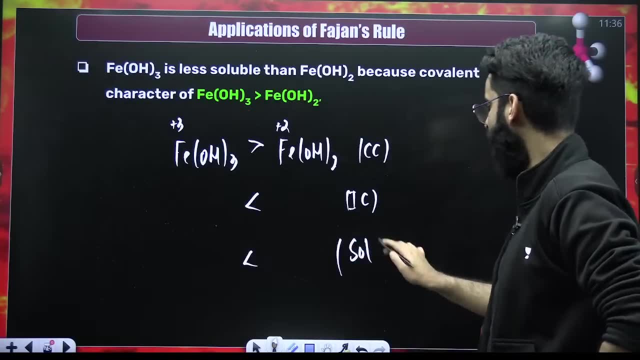 has more. if this is the order of covalent character, what will be the order of ionic character? ionic character order will be this right. what will be the order of solubility? same ionic character order done. I hope I'm clear. number one: melting point order. 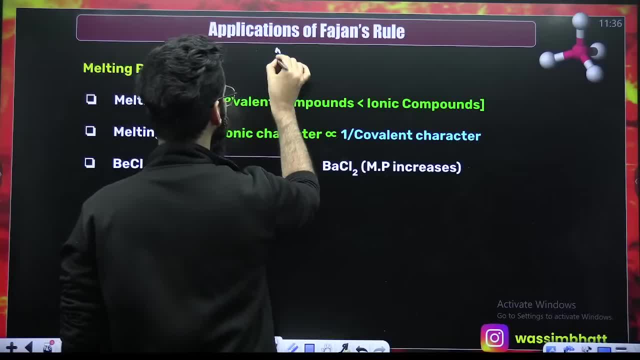 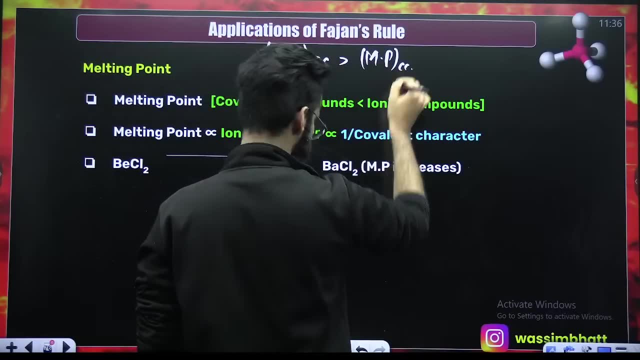 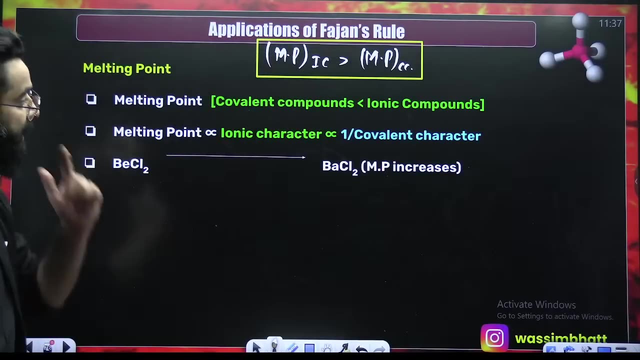 melting point order. do remember melting point of. melting point of ionic compounds is generally more than that of melting point of covalent compounds. melting point of ionic compounds is direct, is greater than that of, is generally greater than that of melting point of covalent compounds. and remember one thing. remember one thing. 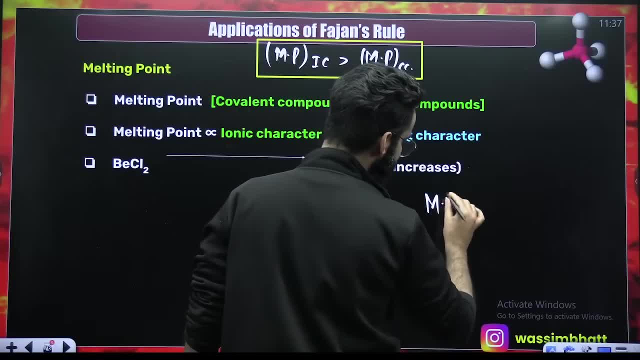 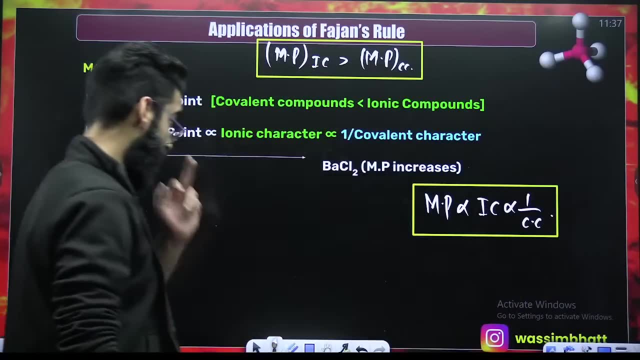 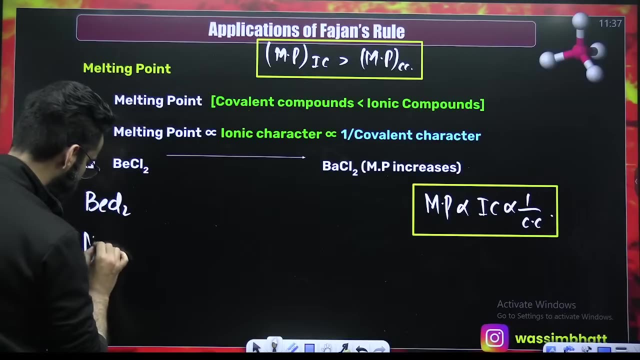 which you already do. now melting point, I can see, is directly proportional to ionic character, or I can say it's inversely proportional to covalent. correct, is inversely proportional to covalent character. now you have got, for example, BeCl2, right, MgCl2, CaCl2, magnesium calcium, strong magnesium calcium, sorry, barely magnesium calcium, strontium. 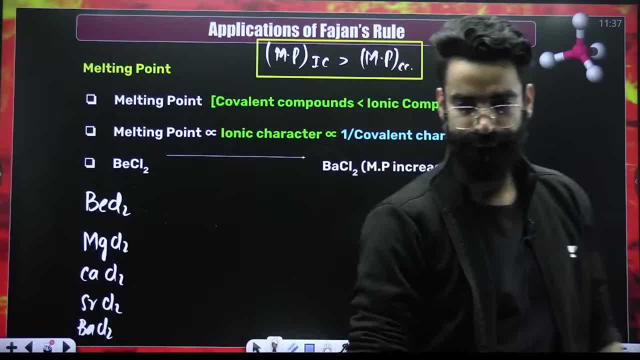 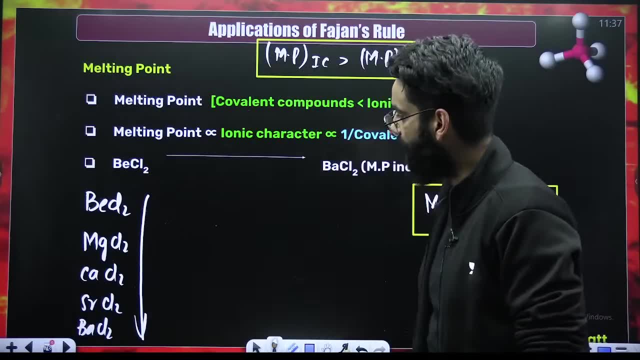 BaCl2. right, if I ask you, if I ask you, what is the order of melting point, what is the order of melting point down the group tell me the order of covalent character. size of cation is increasing. size of cation is increasing covalent. 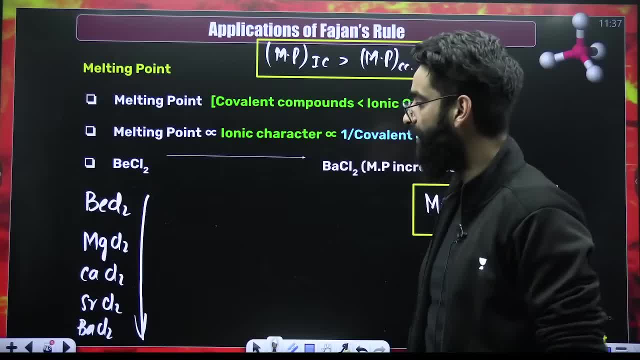 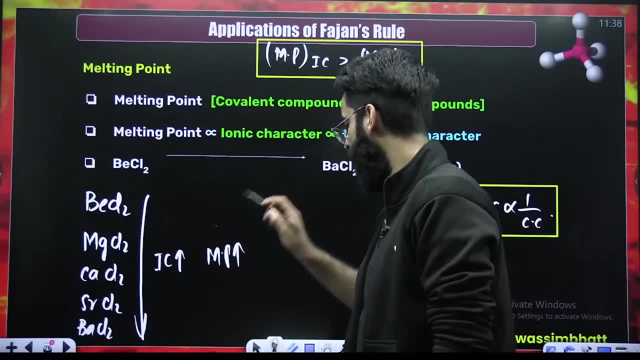 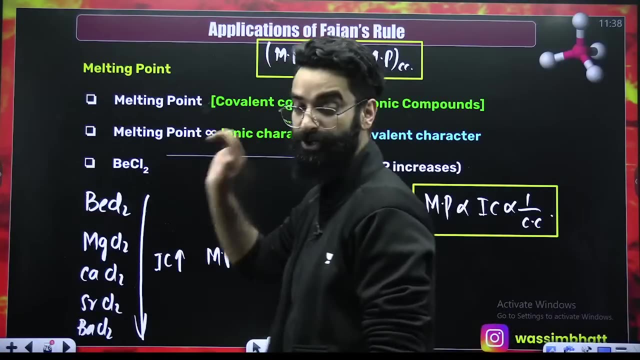 character is decreasing. if covalent character decreases, that means ionic character increases. if ionic character increases down the group, that means their melting points will increase down the group. so BaCl2 will have maximum boiling point. BaCl2 will have maximum boiling point right BeCl2. 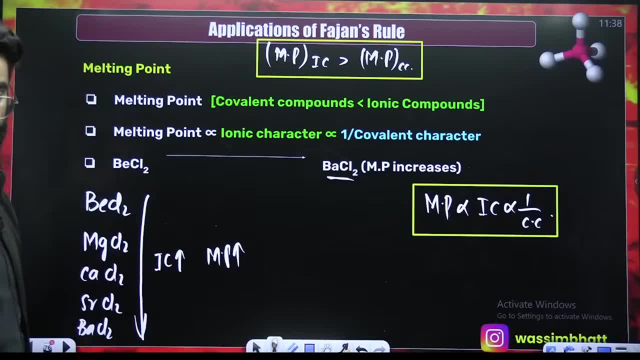 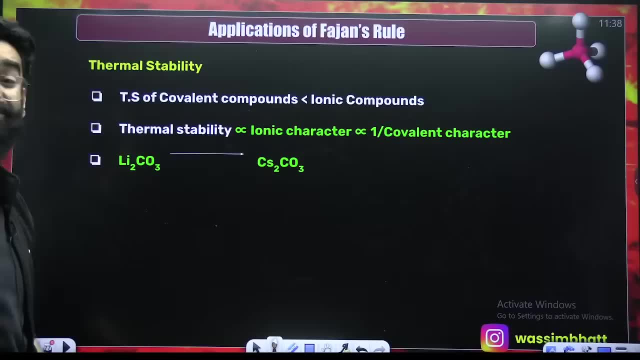 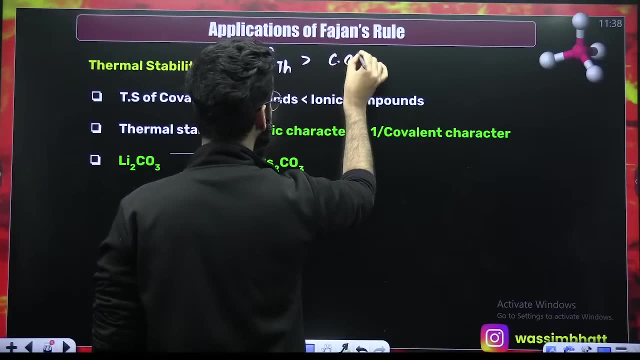 will have least boiling point. am I clear? I mean, if you talk about the melting point, I'm giving the melting point order. similarly. similarly, you can talk in terms of thermal stability as well. remember, ionic compounds have got more thermal stability than covalent compounds. then covalent compounds. ionic compounds have got more thermal stability than covalent compounds, then covalent compounds, ionic compounds have got more thermal stability than what? then covalent compounds, right? or in short, you can say: thermal stability is directly proportional to ionic character, inversely proportional to covalent character, inversely. 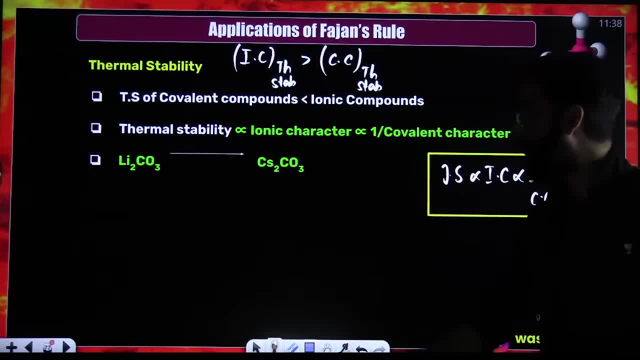 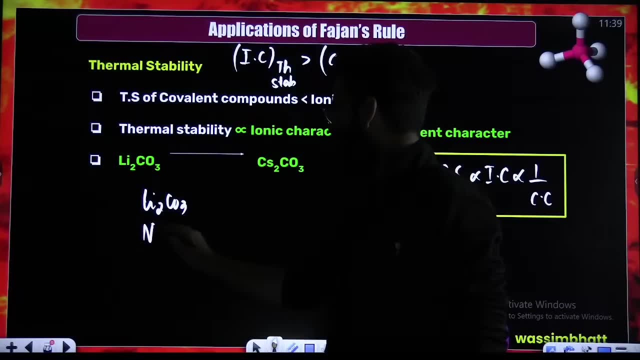 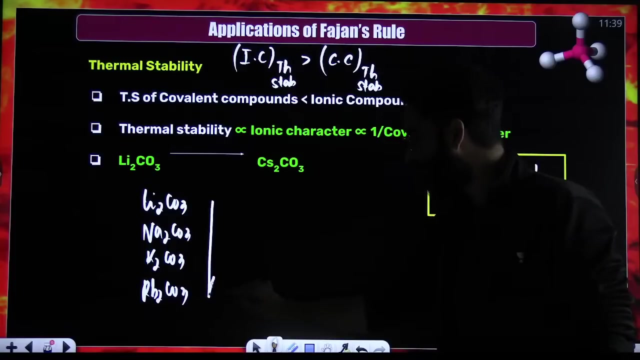 proportional to covalent character. inversely proportional to covalent character. now, for example, you have got Li2CO3- right, perfect, you have got Na2CO3. you have got K2CO3. you have got Rb2CO3- perfect, you have got Rb2CO3. if you look at them carefully down the group anion is same. look at the. 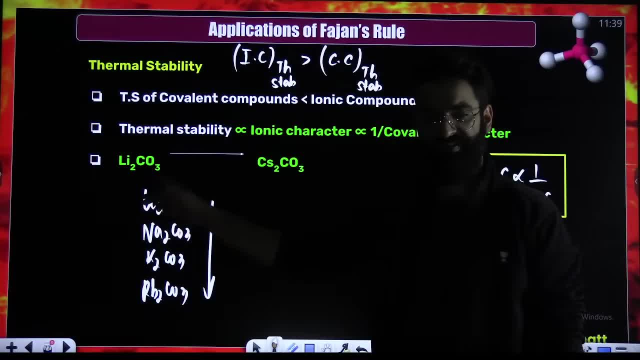 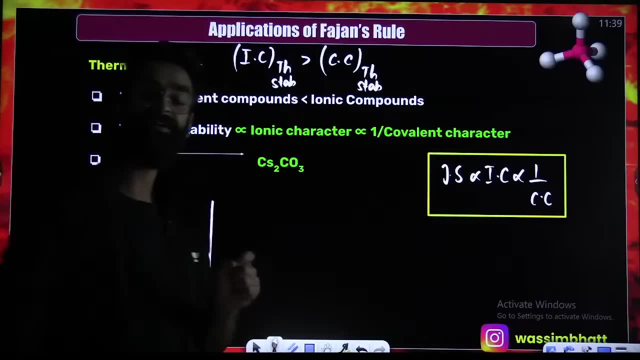 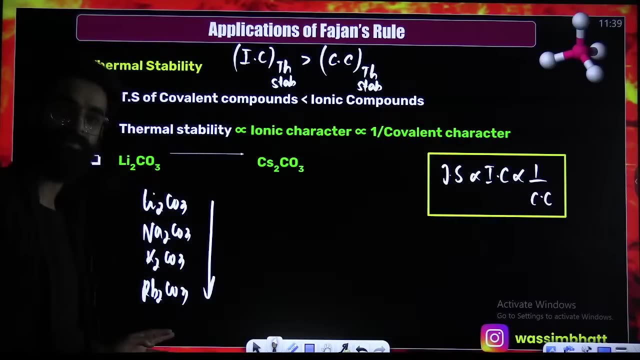 cation. size of cation is increasing. if size of cation is increasing, if size of cation is increasing, then what's happening? basically, if size of cation is increasing, polarizing power of cation is decreasing. polarizing power is decreasing down the group, polarizing power decreasing. 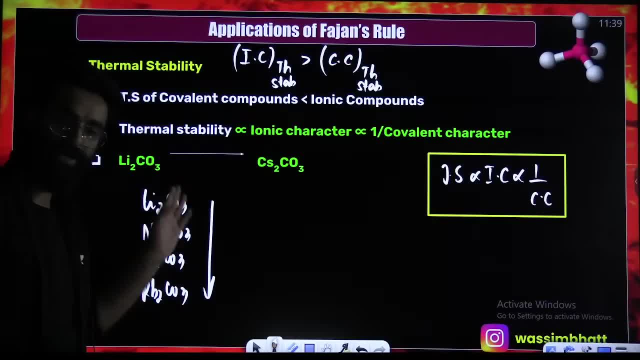 covalent character decreasing. right covalent character decreasing, that means ionic character increasing. so down the group ionic character increases. and if ionic character increases, the character increases, that means your thermals thermal stability will increase. your thermal stability will increase right, so down the group thermal stability. 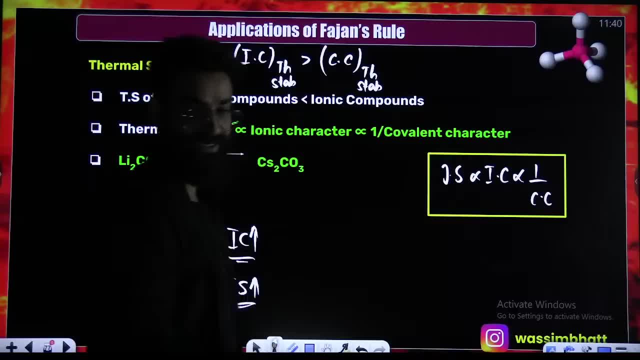 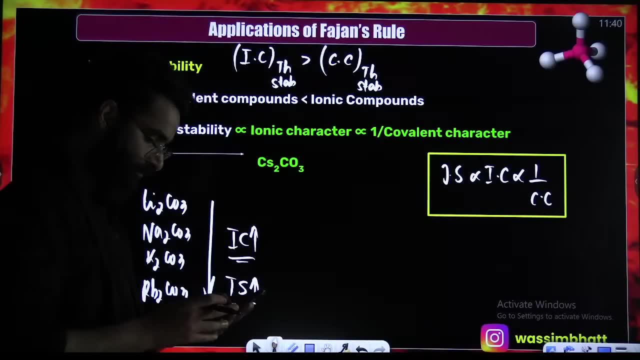 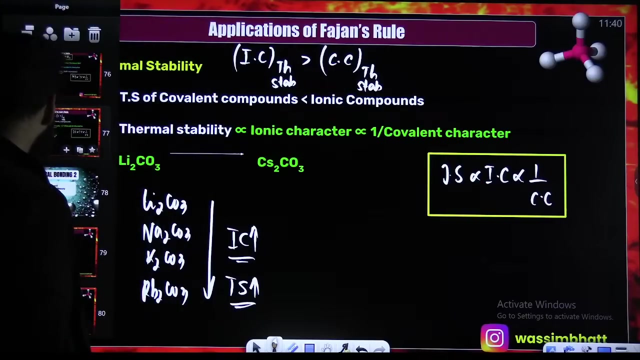 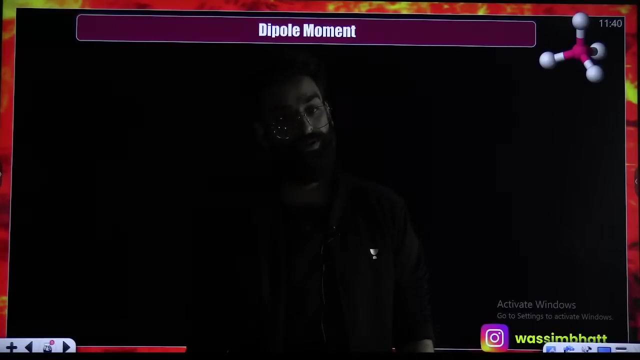 of these one. they increase, it increases. I hope I am clear to everyone. yeah, I hope I am clear to everyone. perfect guys. now one more short short question. one more short short question from one more topic, that is dipole moment. but but before discussing dipole moment with you, 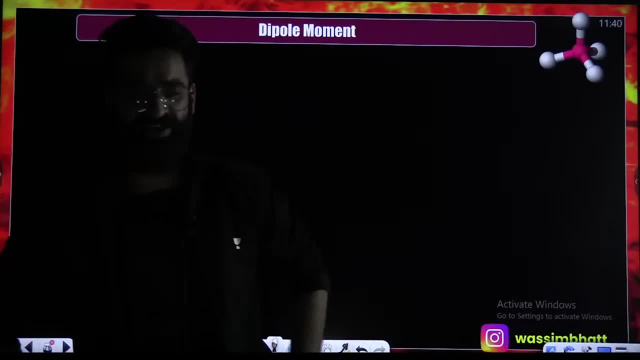 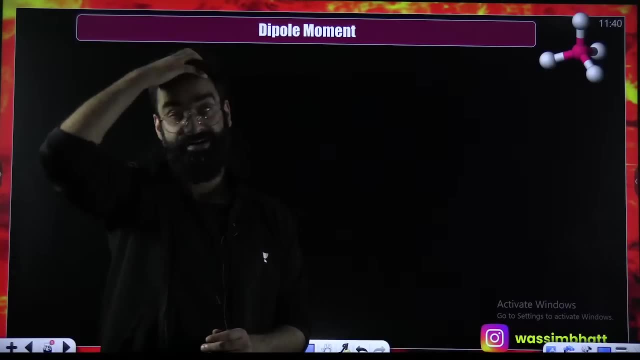 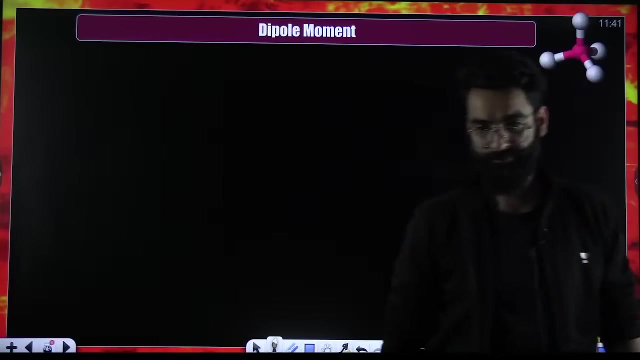 can you quickly let me know whatever things I discussed with you till now. all the things are clear. are all the things clear? there are some electricity issues. I hope this is fine. yeah, I hope it's fine. now, quickly, people in the charts, quickly in the charts. are all the things clear? 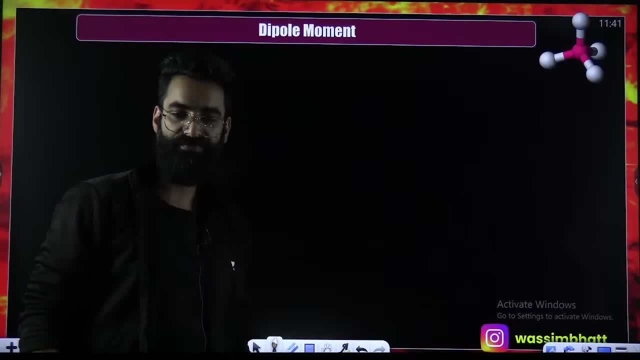 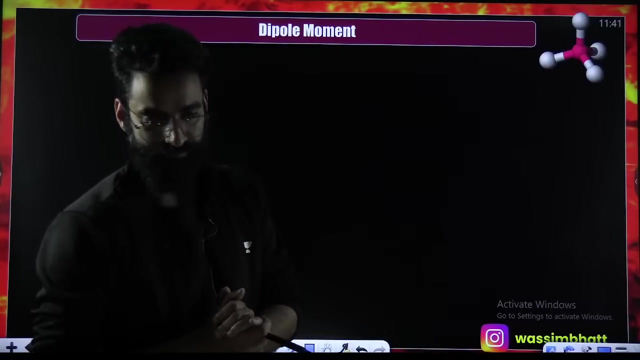 I want every one of you to say: I want every one of you to say: I want every one of you to say it, I want every one of you to say it quickly: perfect, talking about the dipole moment. now from this again, I'm saying a short- 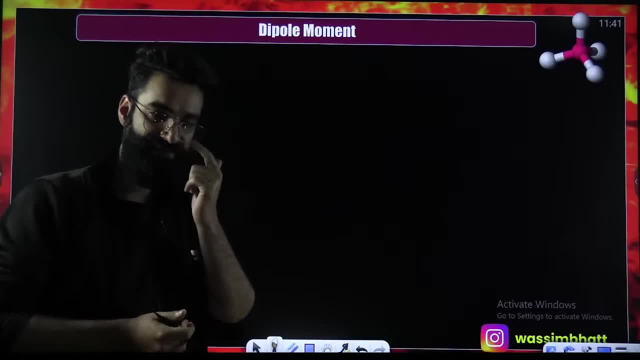 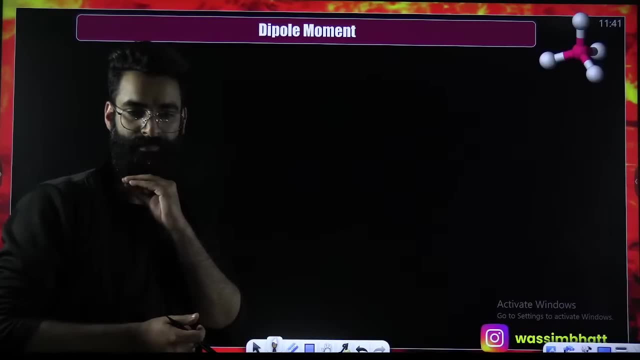 short question is asked: bond parameters. everything will be done, relax everything. everything will be discussing related tonight. so this one is drove by you, okay? so let's Okay, perfect, so let's talk about dipole moment. So, first of all, what does dipole? 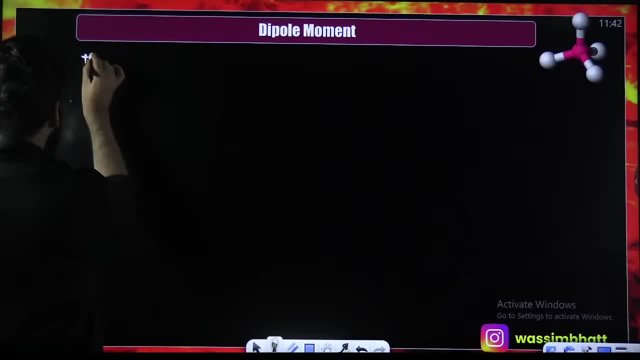 What is a dipole? whenever you have got two equal and oppositely charged species, who equal and oppositely charged species separated by certain distance? where is equal? Where did we get it? Where did we get it? Whenever you have two equal and oppositely charged species separated by certain distance? 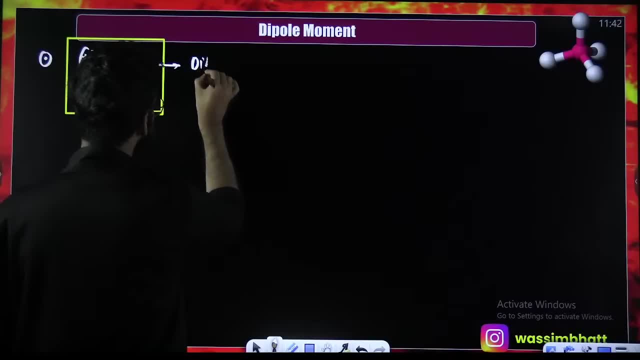 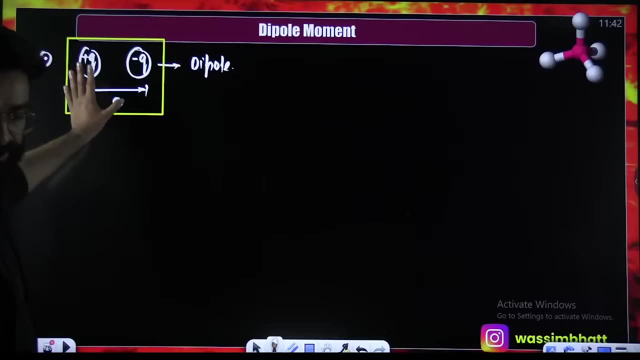 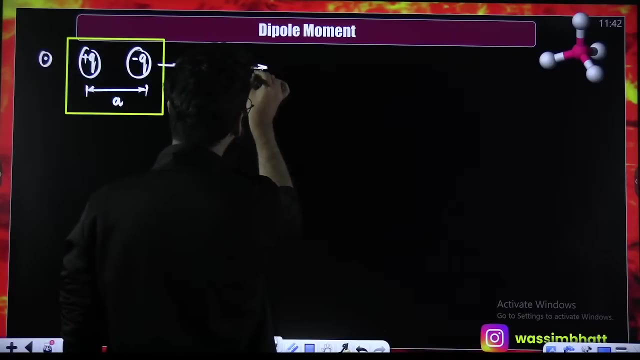 the system of charges over here is what you call as dipole, The system of charges over here. you will be calling as dipole Two equal and oppositely charged species separated by certain distance. you call the system of charges as dipole. And for the dipole, what do we calculate? 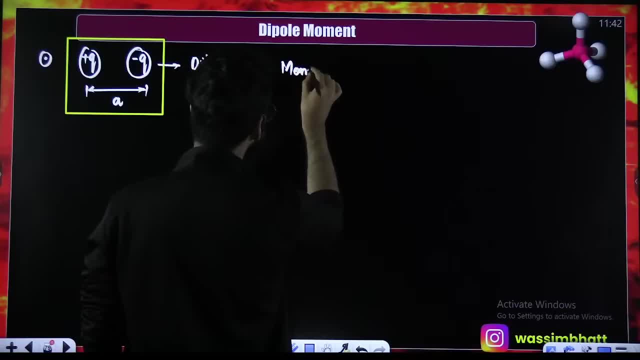 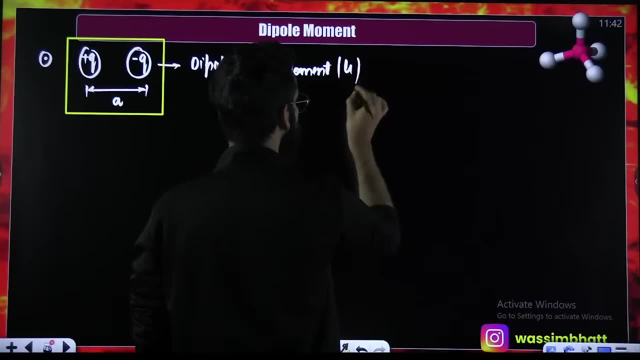 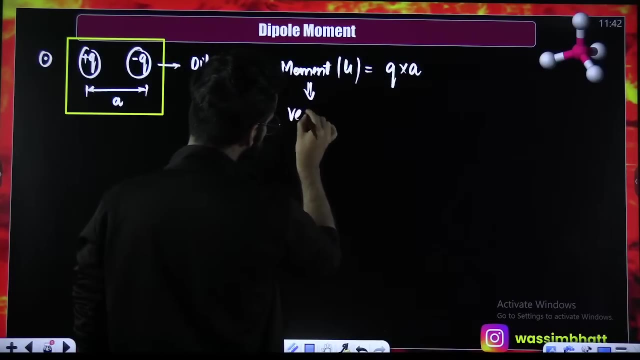 For the dipole, we calculate its moment, We calculate the dipole moment, Dipole moment which is represented by mu, which is defined as charge multiplied by distance. And this dipole moment, let me tell you, it is a vector quantity. 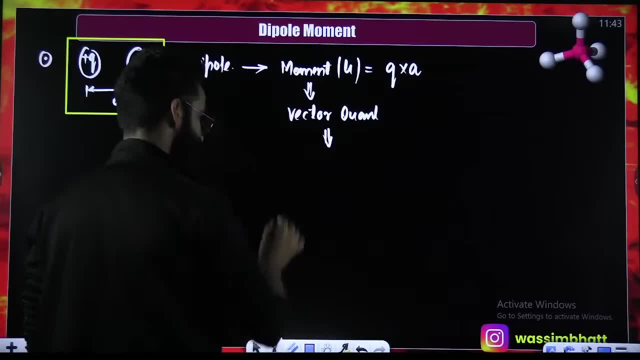 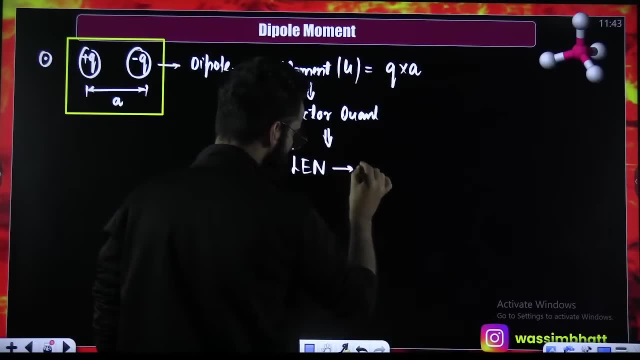 And if it is a vector quantity it will be having the direction as well. And the direction of the dipole moment is taken from less electronegative element to more electronegative element, More electronegative element, Or in general you can say it is taken from positive to negative in chemistry. 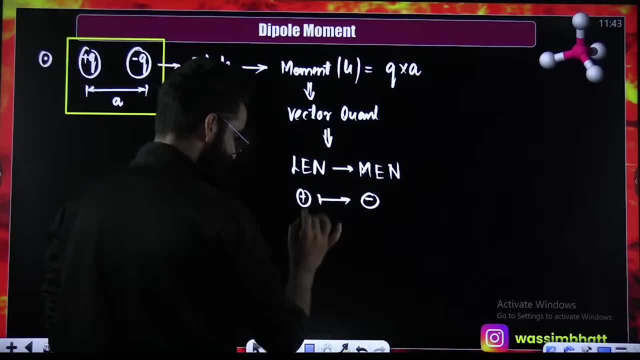 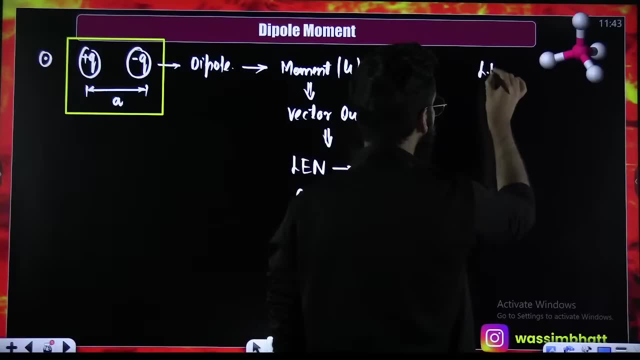 Positive to negative in chemistry, Or I can say one more thing. I can say one more thing. I can say one more thing. Lone pair also contributes. Lone pair also contributes to the dipole moment And the direction of dipole moment. 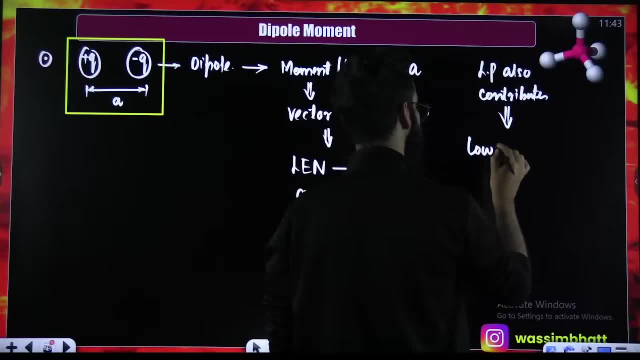 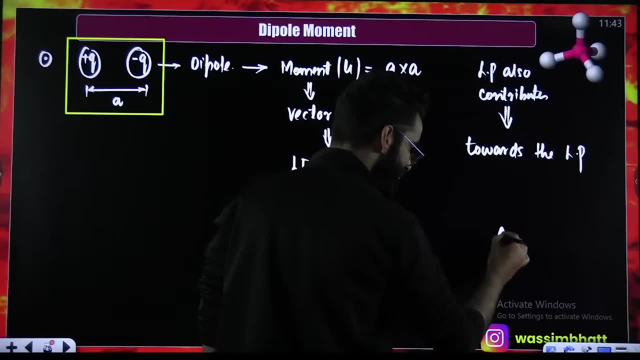 Direction of dipole moment due to lone pair Is towards alone Is towards the lone pair. What is meant by that? For example, this is atom A. It has got the lone pair like this, Perfect. So lone pair also contributes to dipole moment. 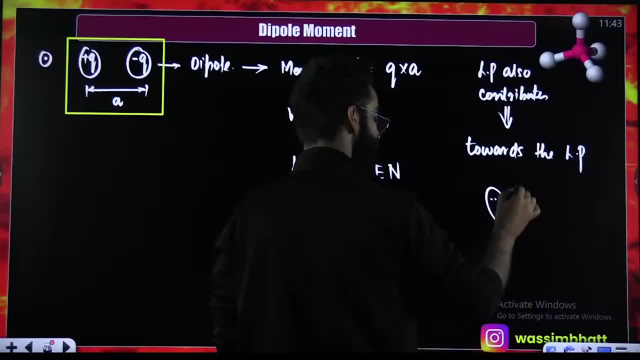 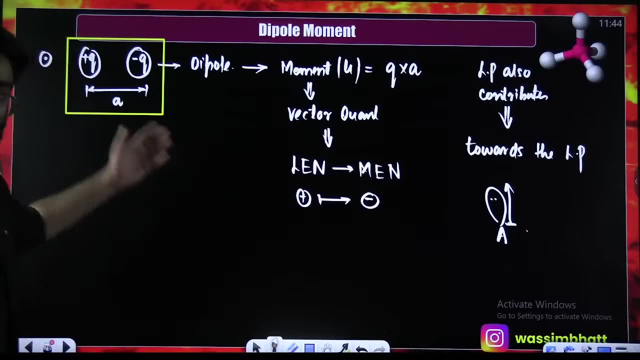 Right, It is the moment. due to this lone pair, Its direction is towards the lone pair. Remember this particular point as well. Remember this particular point as well Again, whenever you have got a system of equal and opposite charges Separated by certain distance. 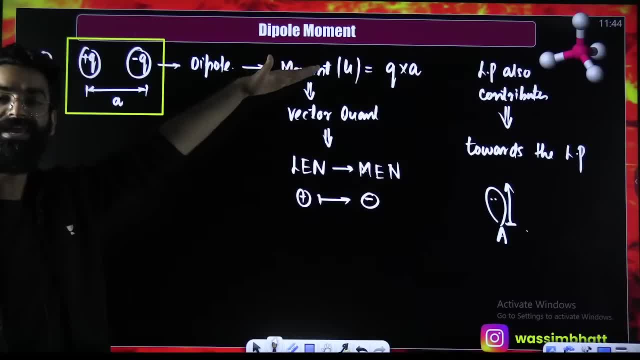 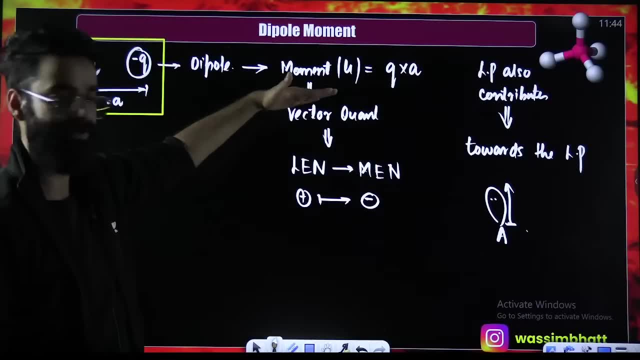 You call the system of charges dipole. For the dipole, We define its moment, Dipole moment, Which is the product of charge multiplied by distance. This dipole moment is a vector quantity. Its direction is from less electronegative to more electronegative element. 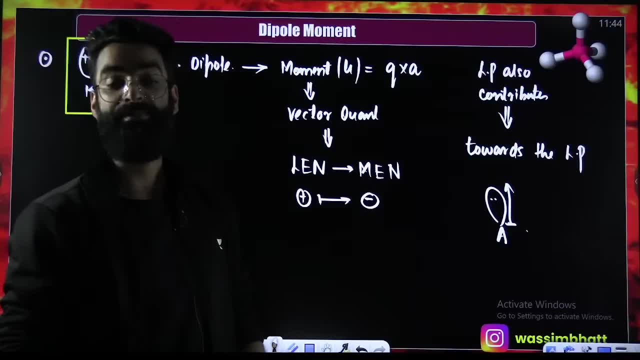 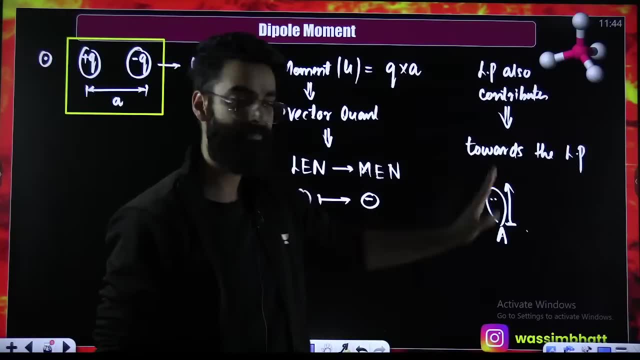 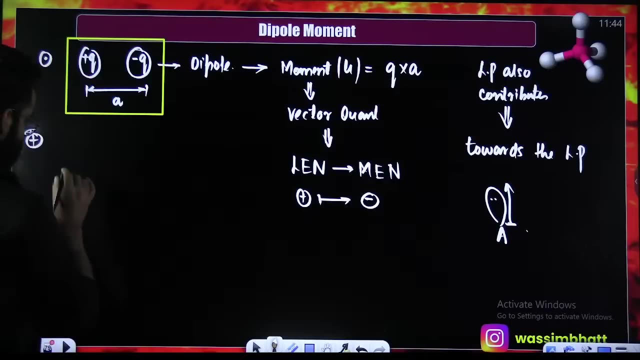 Positive to negative Lone pair also contributes towards the dipole moment And its direction is from positive to. I mean its direction is always towards the lone pair. Simple, Simple, Okay. One more point. One more point, people You see, 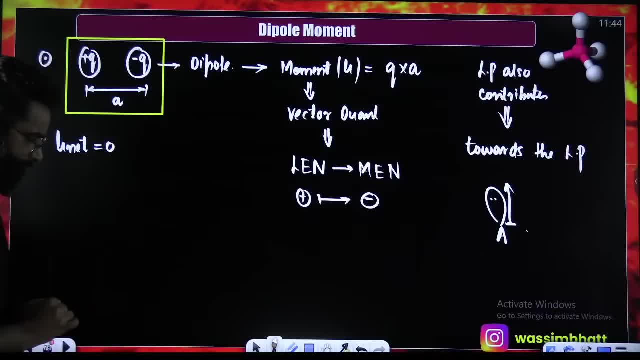 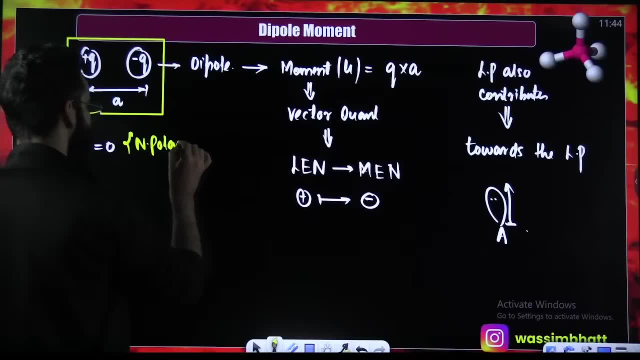 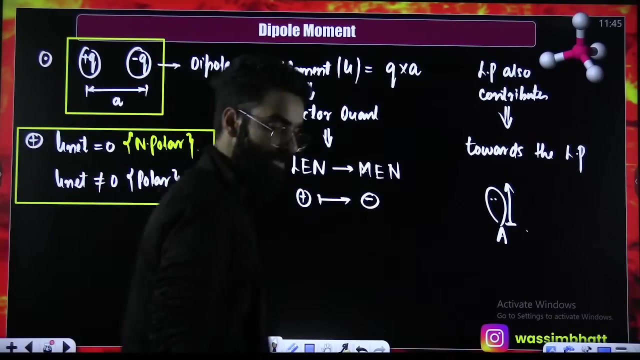 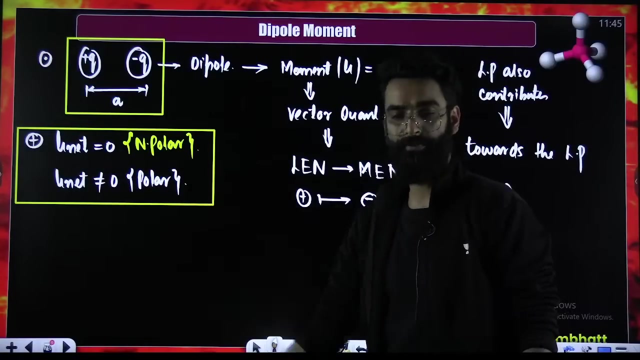 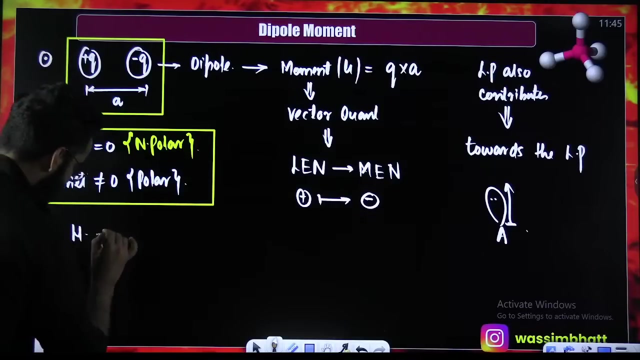 Let us break the Microness. If the net dipole is zero in a molecule, non-polar Net dipole is non-zero. polar molecule, Okay. Polar molecule, For example, you have got HF, HF, HF, Okay. 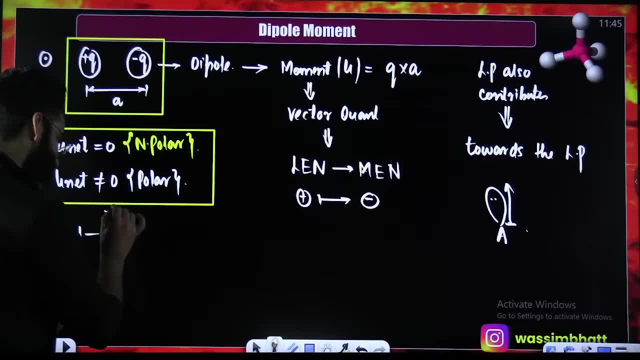 Fluorine is more electronegative, So it will attract the bonded pair towards itself. So, delta negative, Delta positive, Delta, negative, delta positive, Right. So if this is positive, this is negative. Can I say? this molecule is behaving like a dipole. 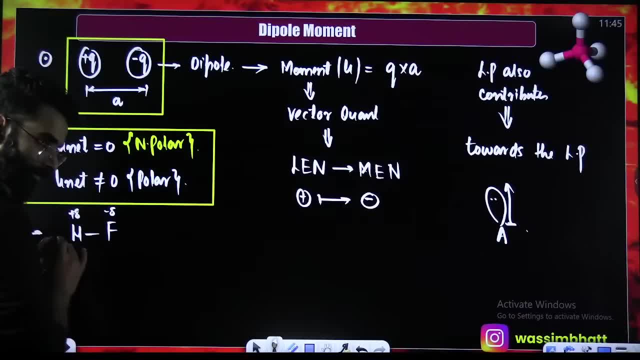 Positive and negative charge, separated by certain distance. It is a dipole. now, Right For the dipole, we define a moment, And dipole moment is from positive to negative. Dipole moment is from positive to negative. Dipole moment is from positive to negative. 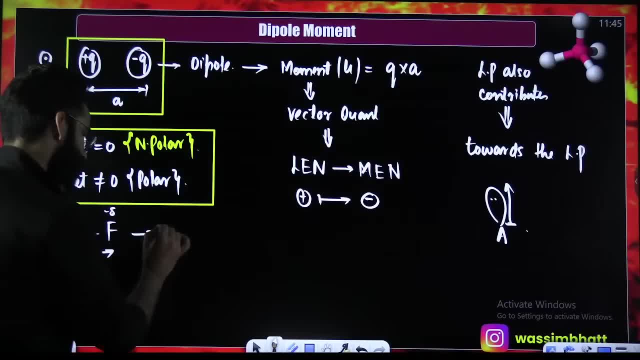 Right. So this molecule has got some dipole moment. If it has got some dipole moment, it is definitely a polar molecule. It is definitely a polar molecule. Let's say: you have got carbon dioxide, You have got carbon dioxide. 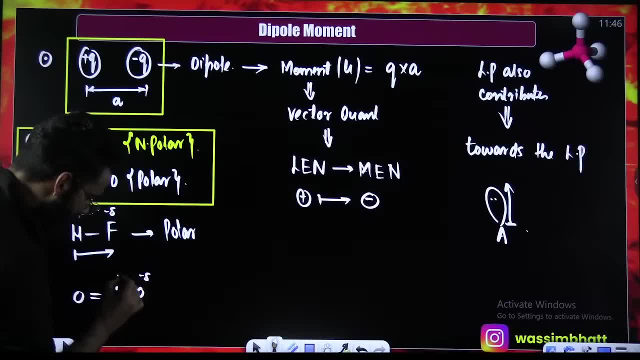 Due to this particular bond, This is negative, This is positive. Right Negative, Positive. Similarly, this will be negative, This will be positive. So, moment in this direction, Moment in this direction: Positive negative. Positive negative. 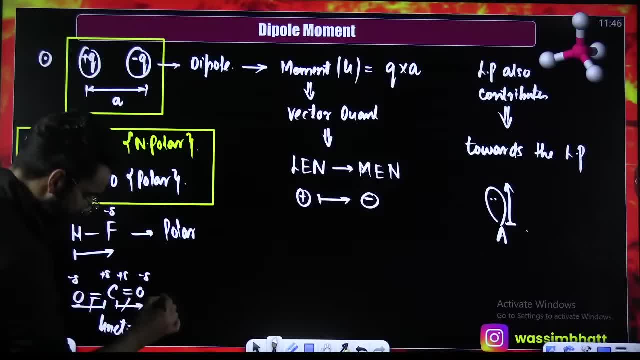 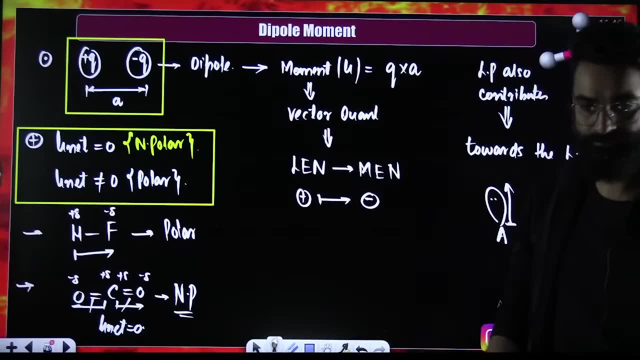 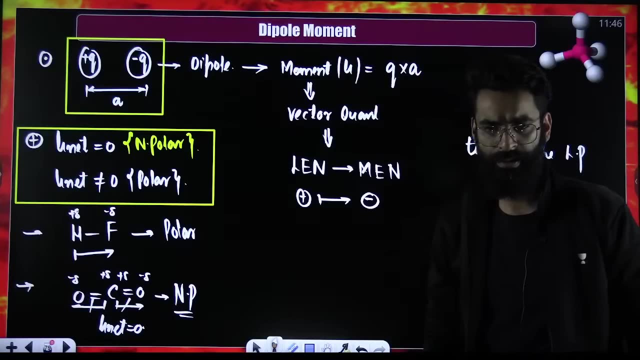 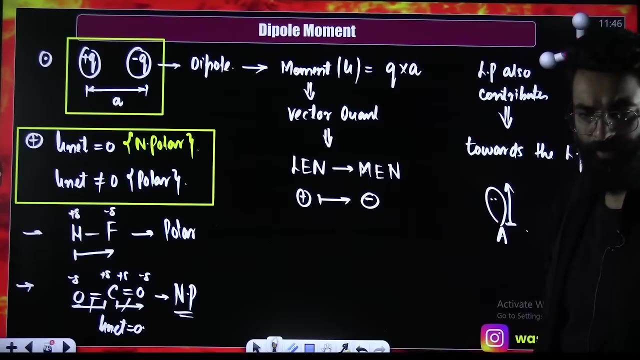 They will cancel out. If they cancel out, net dipole moment is zero. So carbon dioxide, It is a non-polar molecule Because its net dipole moment is zero. Because its net dipole moment is zero. Okay, I will read it this way: 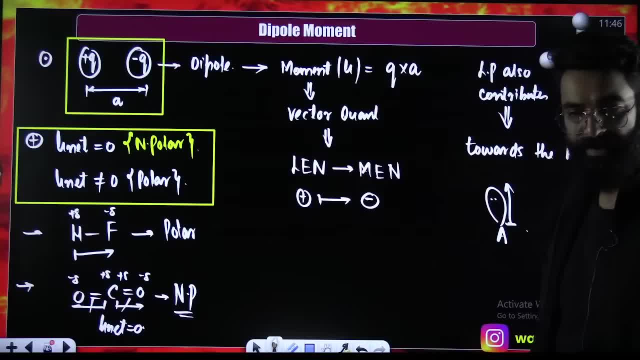 Because after now, after I've done all of theaker competitions good, you are still trying to guess into myяниí thought that this is from positive or negative time. This is not positive. Okay, I am expecting the same thing. But people surprising me at whatever you want, Because all I said was I am the ever grandeur of everybody too. Time is giving me an baton line now That I am like the pontoon, for какой point? to the catching a bird. Watch this. Come on, Try continue with yourten minute. Haha, Know the difference between electricity compared to such a coupled piston? I know this number is up, so tell, But you can't get it out of your head and drive on as such. 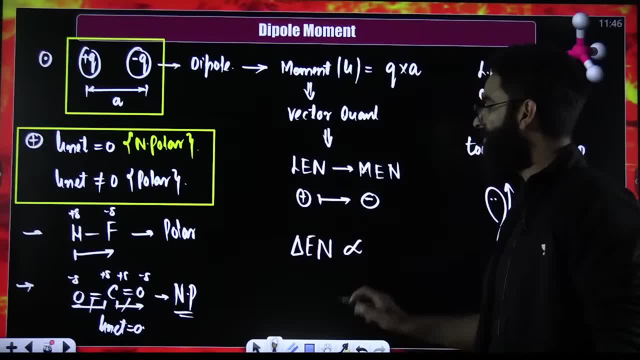 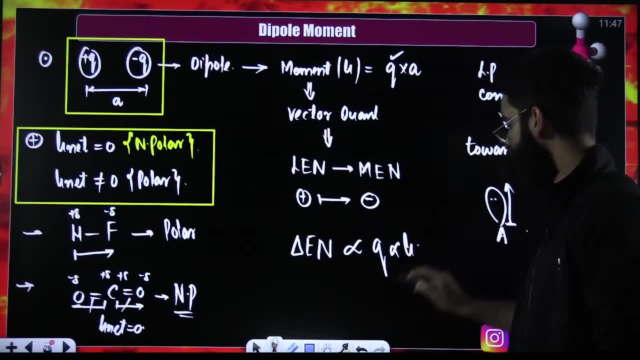 It is as well'cause this will get to you quickly. So in the Ley crossing of 1 minute, Electronegativity difference: more the electronegativity difference between the atoms, more the charge on the atoms, and more the charge means more the dipole moment. 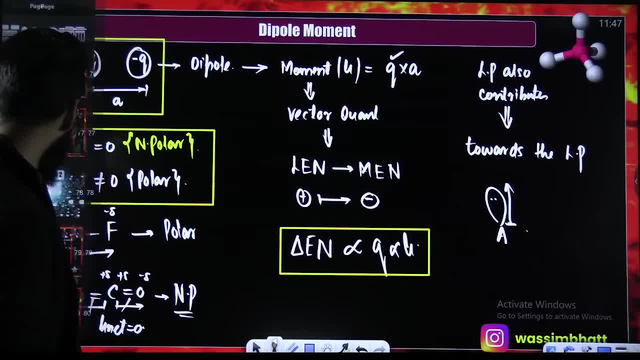 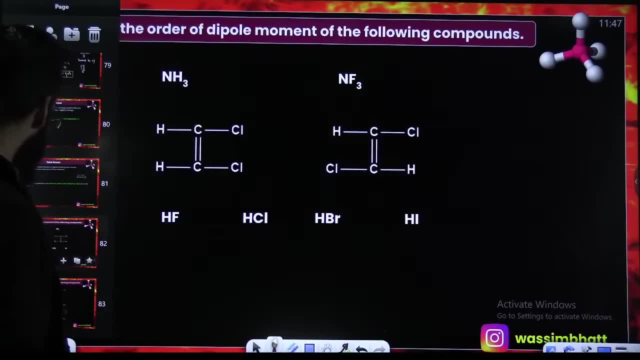 More the charge means more the dipole moment. Let's try to solve the question so that it becomes clear. Let's solve the question so that it becomes clear. Let's solve this question first. HF, HCl, HBr, Hi. 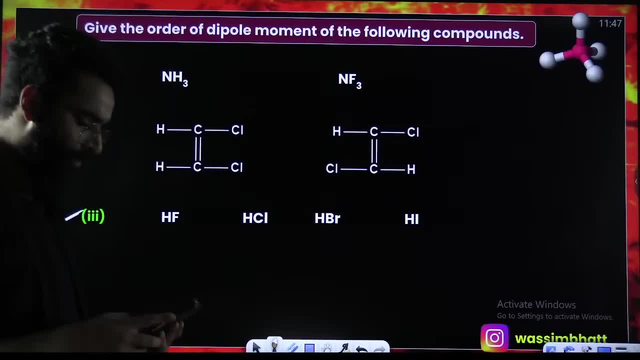 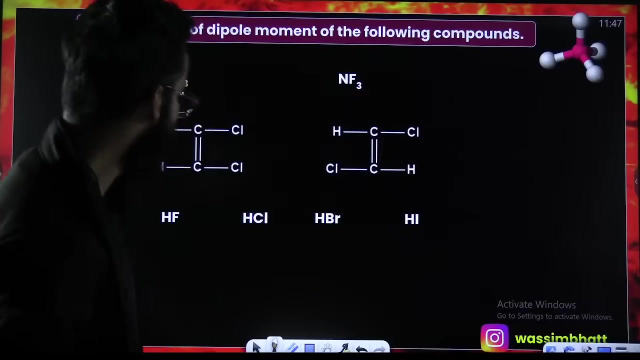 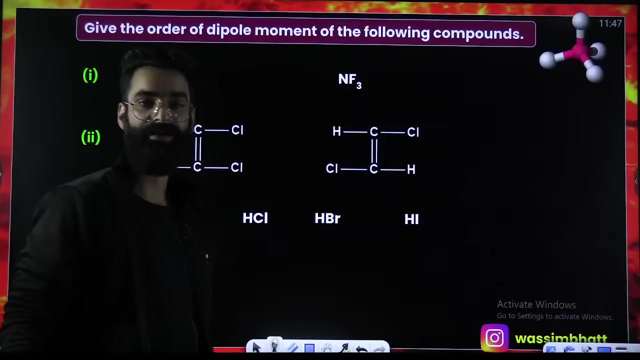 Give me the order of the dipole moment quickly. Give me the order of dipole moment quickly. Give me the order of dipole moment quickly in this question. See, guys, This is HF, This is HCl, This is HBr, Hi. 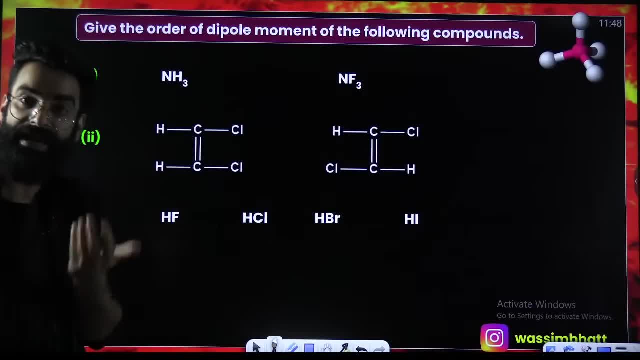 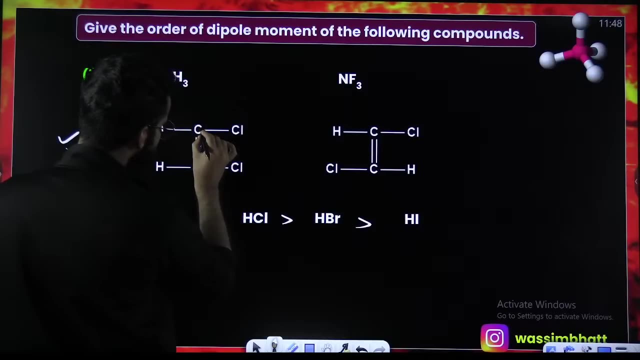 More the electronegativity difference, more the electronegativity difference, more the dipole moment. In short, clear. Look at this particular question. This is CCl. This is CCl. Chlorine is more electronegative than carbon. 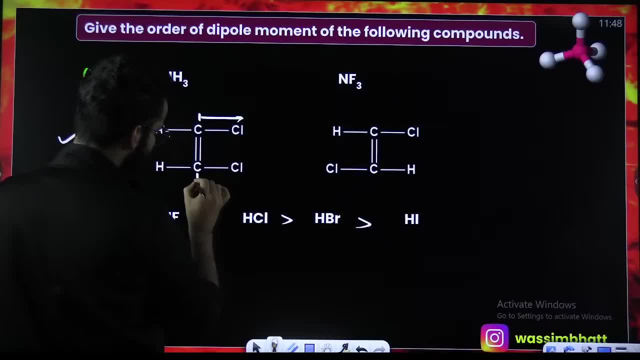 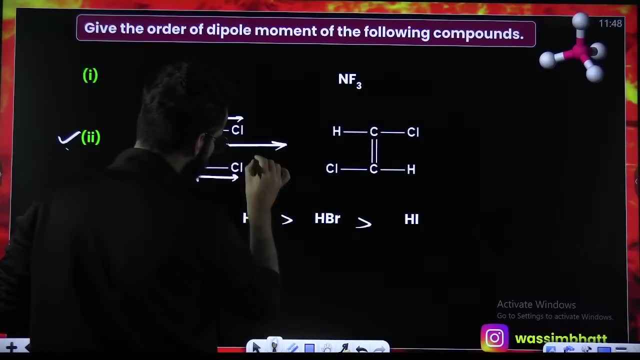 So lesser to more, less electronegative to more electronegative, Less electronegative to more electronegative. So both these vectors are in the same direction. So this is your net dipole moment. direction Right. 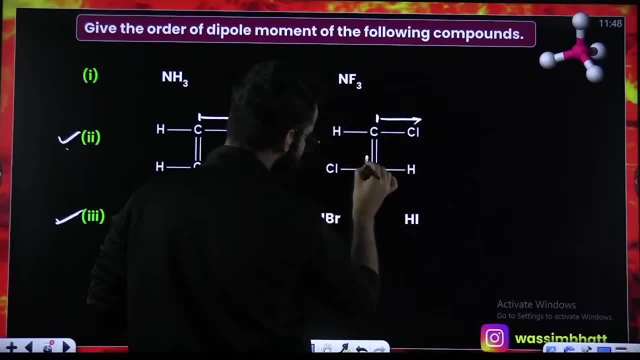 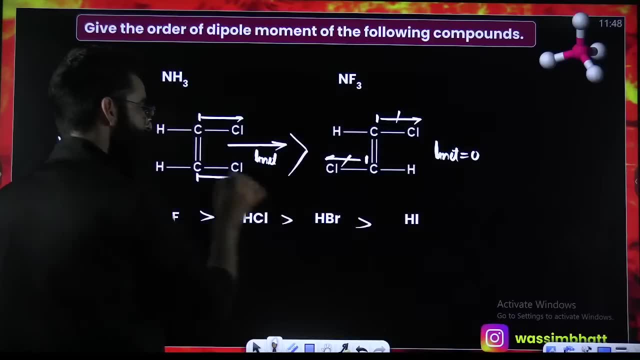 Less electronegative to more electronegative, Less electronegative to more electronegative. It cancels out. So net dipole moment here is zero. Net dipole moment is zero, Right. So where is the dipole moment more? 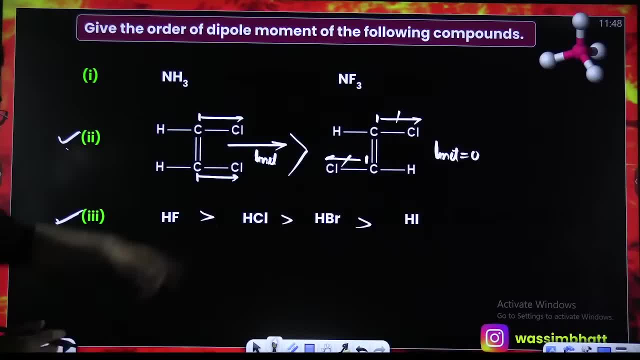 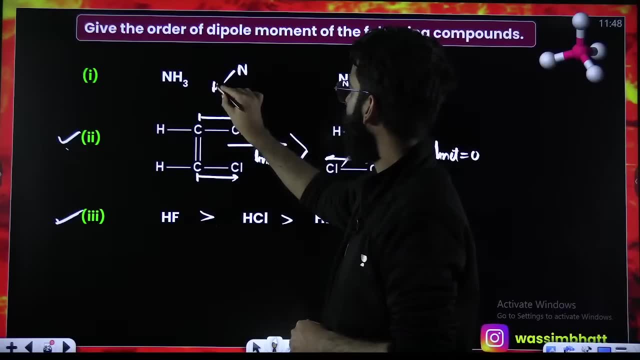 In the first case. In the first case, NH3, NF3.. NH3, NF3.. It is a special case. Have a look. NH3.. This is nitrogen, This is hydrogen, Hydrogen Hydrogen And. 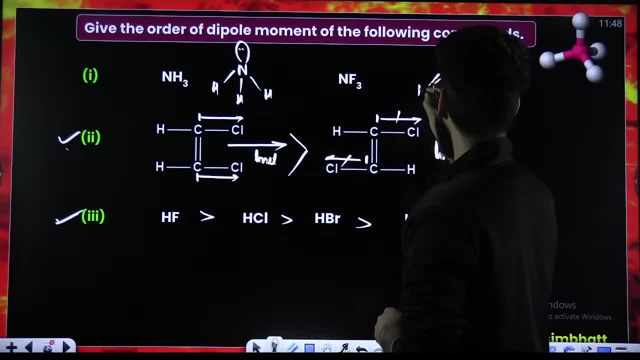 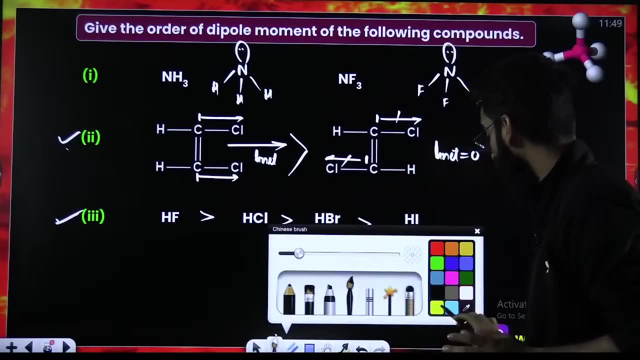 It is a lone pair: NF3.. This is nitrogen, This is fluorine, Fluorine, Fluorine And a lone pair. Perfect And a lone pair. First of all, lone pair also contributes towards dipole moment. 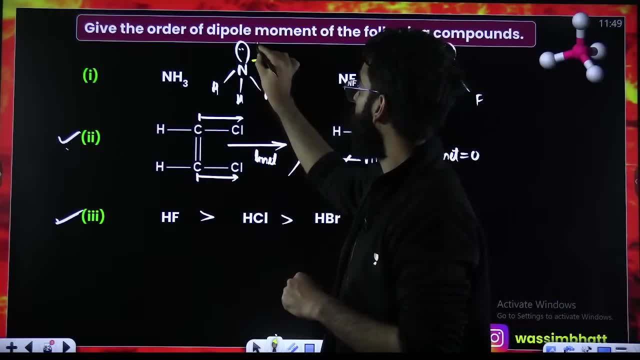 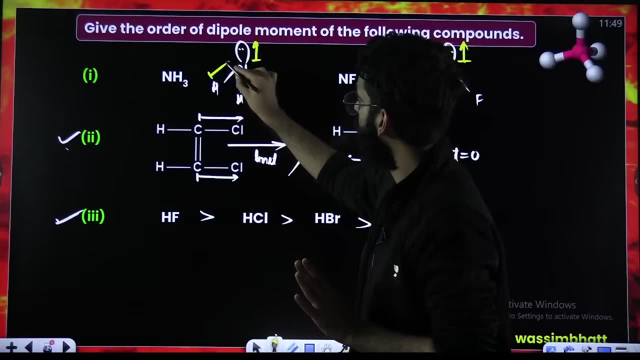 Right. So the moment due to lone pair is towards the lone pair. The moment due to lone pair is towards the lone pair. Okay, Leaving aside NH. Less, electronegative to more electronegative, Less to more, Less to more. 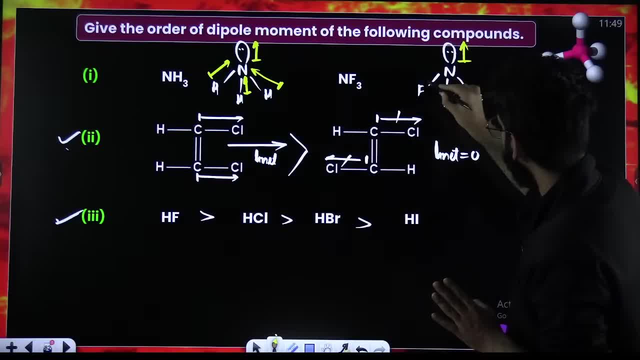 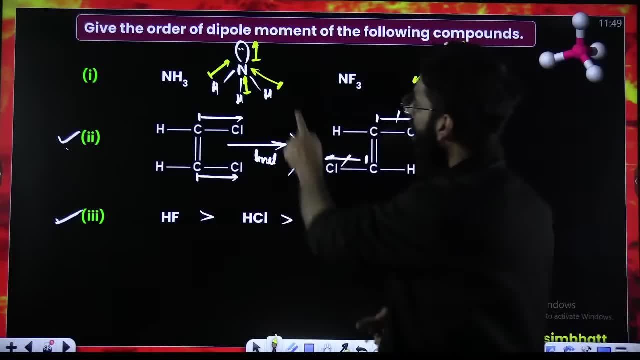 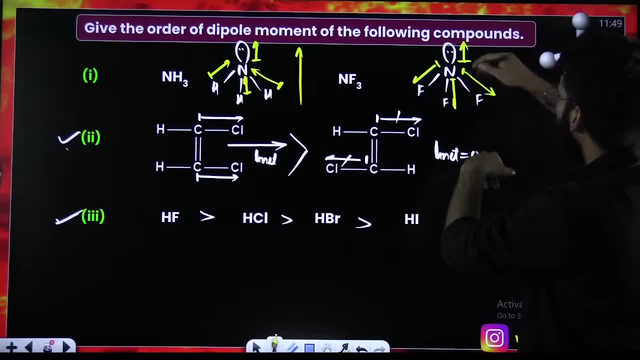 They are converging in the same direction Over here. one is going up, One is going down. There will be some cancellations. There will be some cancellations Here. you don't have any cancellations Here. cancellations are there. 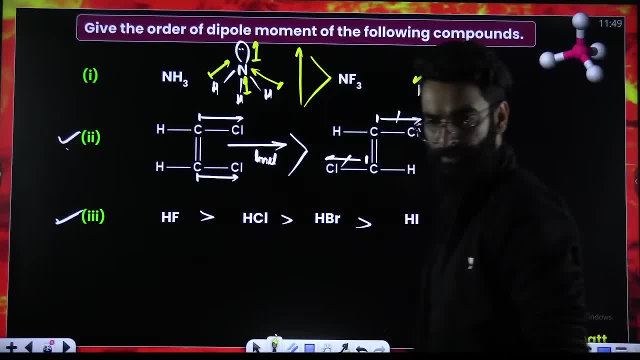 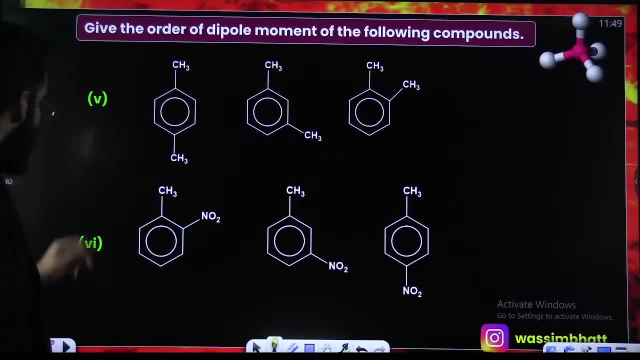 Right, No, cancellation means more dipole moment. Done, Yes, Done. Is it done and dusted? Recently you have studied your CH3.. Is CH3 donating or withdrawing? Is CH3 group donating group or withdrawing group? Tell me that. 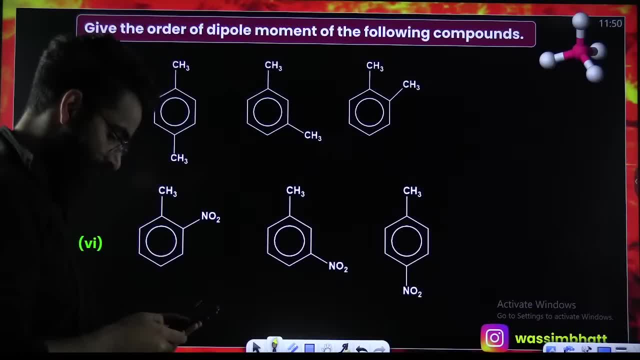 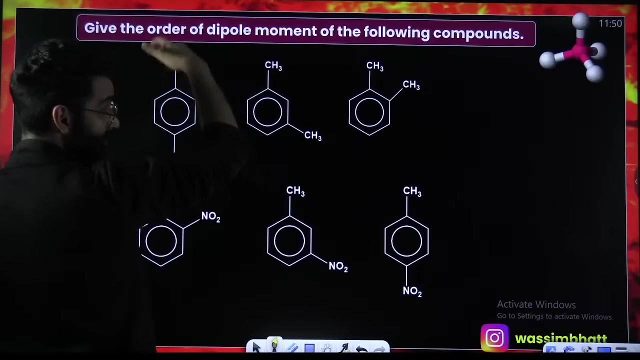 Just that: Quick people, quickly, quickly, quickly, everyone, quickly, everyone in the chats. absolutely, you know it. CH3 is donating if it donates, if it donates delta positive, delta negative. this one will be donating delta positive, delta negative, positive to negative, positive to negative. 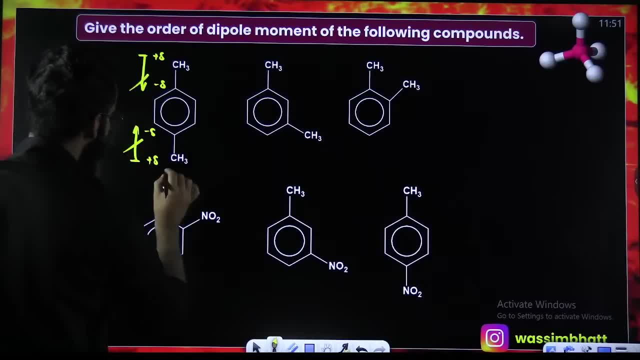 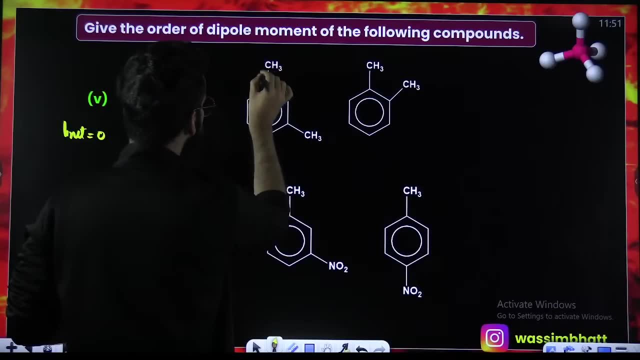 both the vectors are in the opposite direction. right: net deployment here is zero. net is zero. right see: positive to negative, positive to negative, positive to negative. one vector is pointing downwards, one vector is pointing in this direction. both the vectors are at: 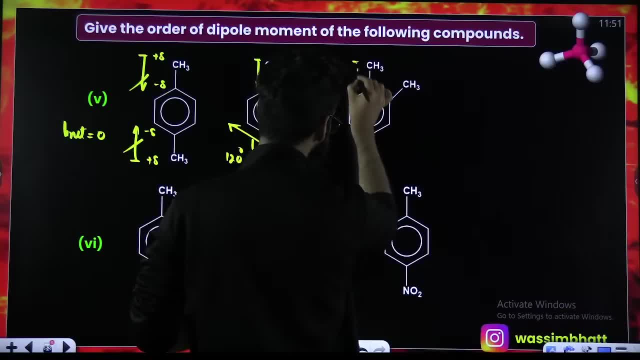 an angle of what? 120 degree Right. positive to negative, positive to negative. one vector is pointing downwards, one vector is pointing in this direction. angle is 60,. angle is 60,. perfect, here the angle was 180,. 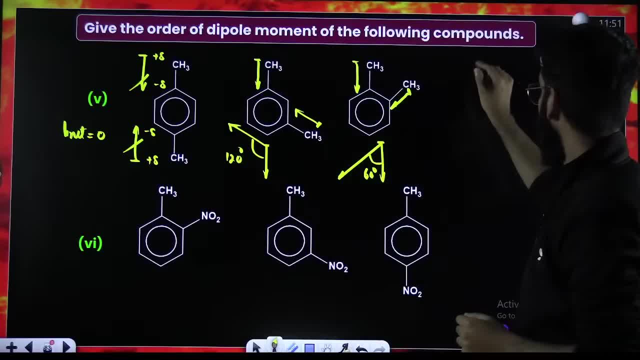 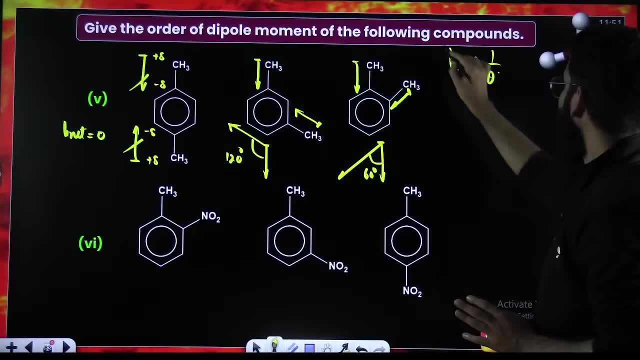 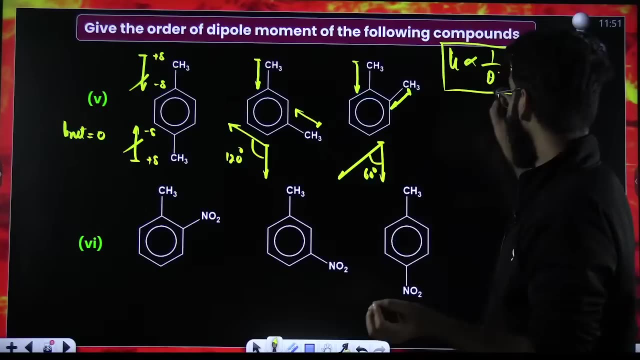 120, angle is 60, dipole moment. dipole moment is inversely proportional to the angle between the vectors. Lesser the angle, more the dipole moment Right, Lesser the angle more the net dipole moment. Lesser the angle more the net dipole moment. so 3, greater than 2, greater than 1, okay. 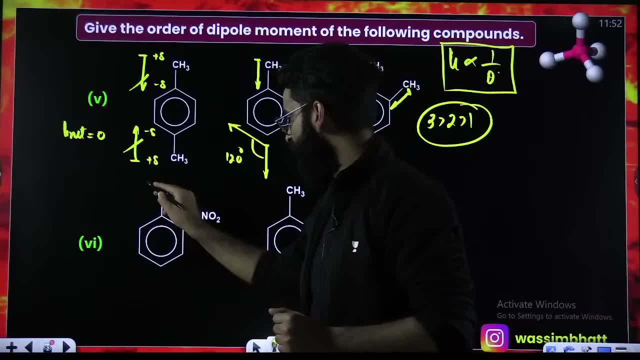 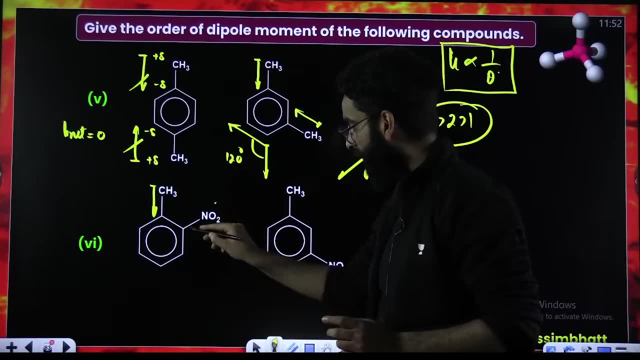 perfect. look at this particular equation. This will have positive and negative, so positive to negative downwards. NO2 is withdrawing, it will withdraw. it will get delta negative. This will get delta positive. positive to negative in this direction. so one vector. 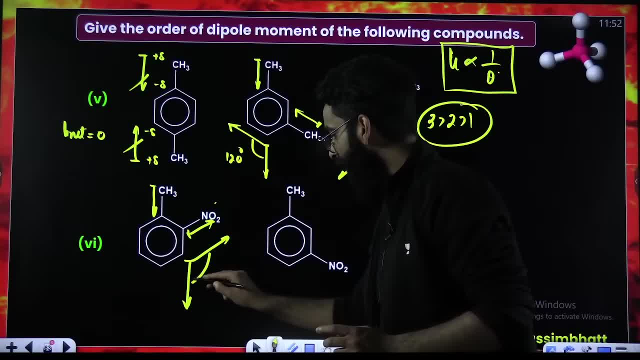 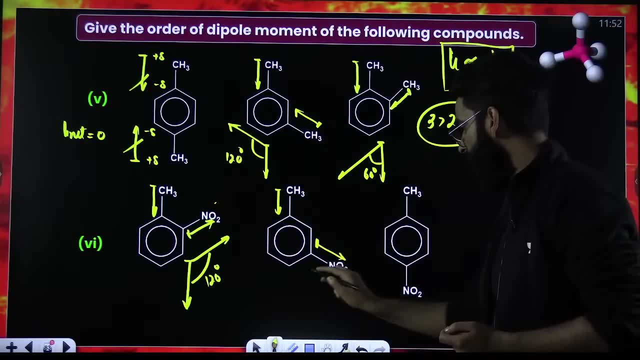 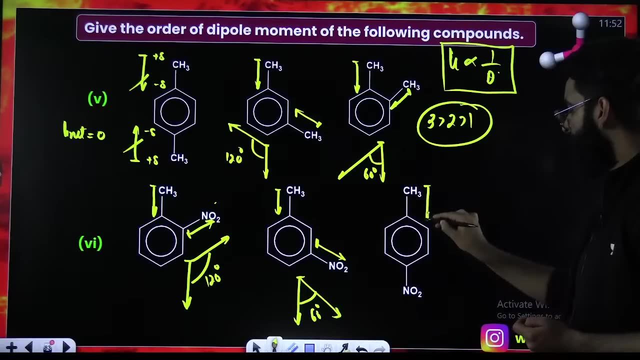 is pointing downwards, one in this particular direction. the angle over here is 120,. perfect, positive to negative, positive to negative, one vector pointing downwards, one in this particular direction. the angle here is 60, right. positive to negative, positive to negative, both vectors downwards, so angle here is zero, lesser the angle, so we will have more dipolement followed by two. 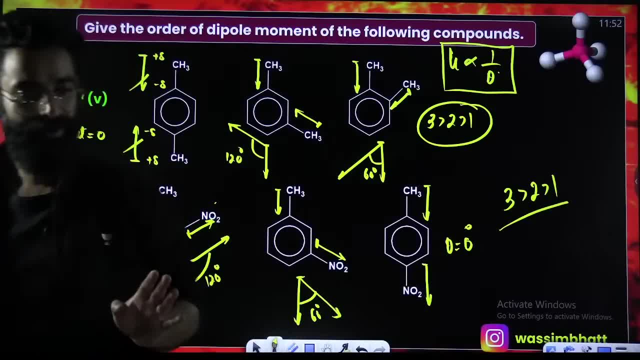 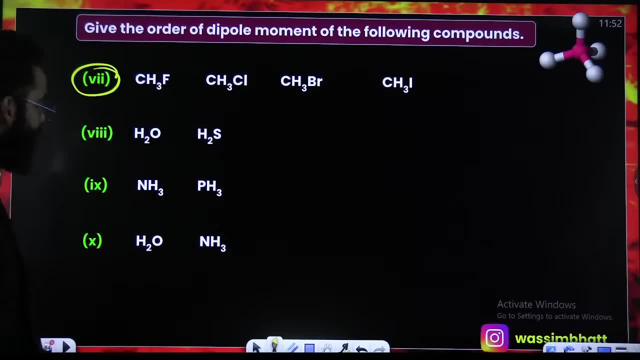 followed by one. yes, am i clear people? am i clear to everyone? leave this particular case aside, talk about the other ones. h2o, h2s, more electronegative difference, more dipolement- here it is oxygen hydrogen, here it's sulfur hydrogen. where is the electronegative? 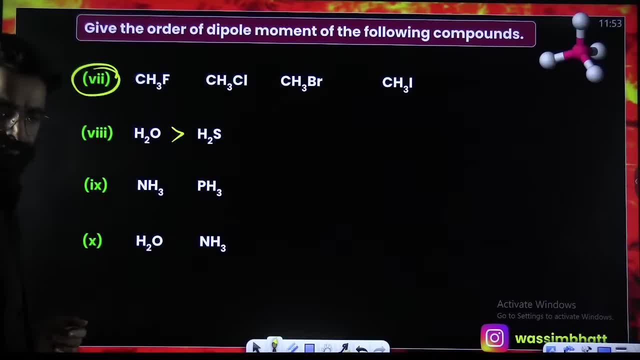 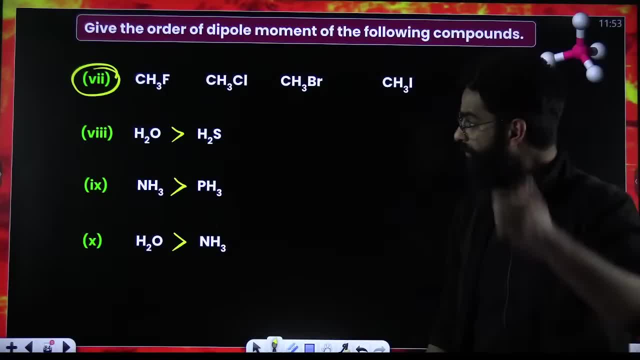 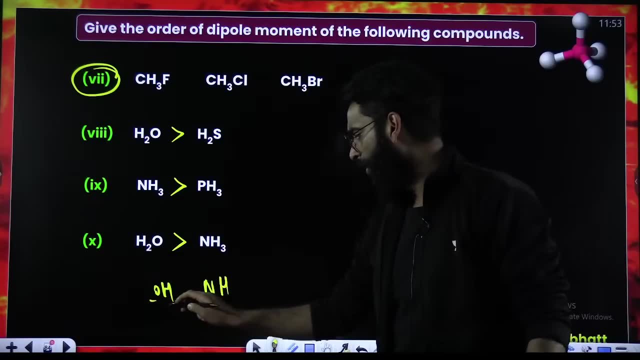 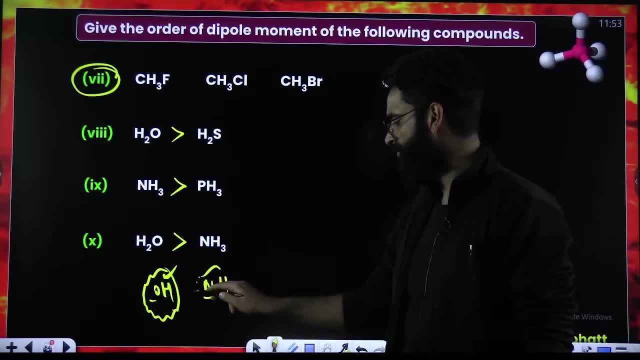 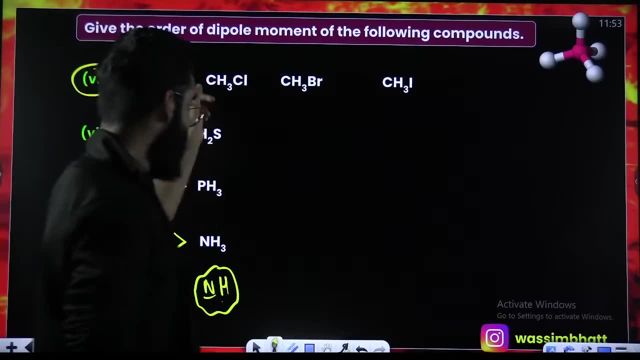 difference here is more. if difference there is more, Dipolement is more. difference here is less, Dipolement is less. i believe i'm clear. i believe i'm clear. look at the first case. i mean, look at the first case. right, this is something which will remember. this is something which you will remember. 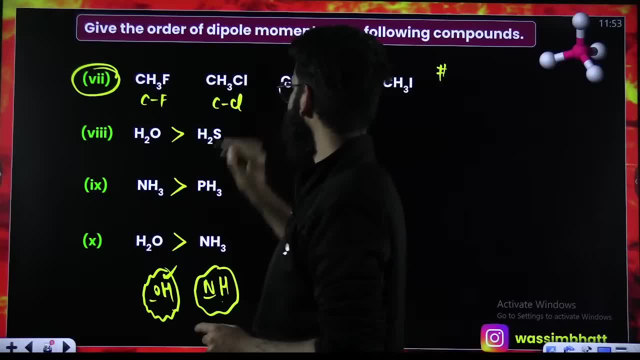 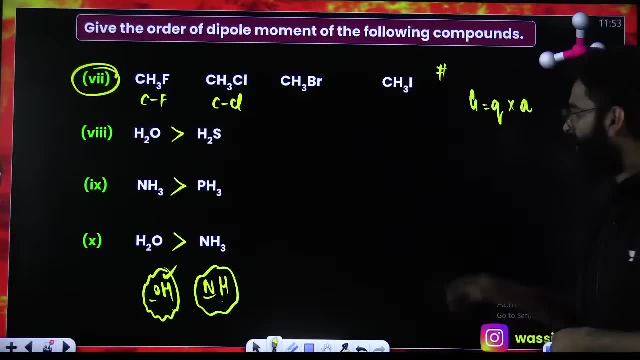 is students, here you have gone with bond between c and f area, bond between c and l, c and l, correct dipole moment. it depends on two factors, basically: charge and distance. right. so more the charge, more the charge, more the charge means more the electron negative difference. more the charge, more the. 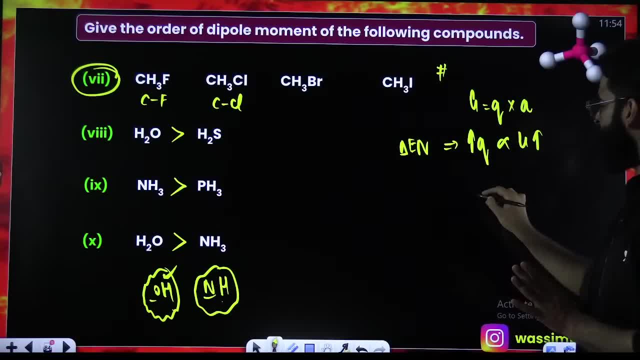 dipole moment, you know it. at the same time, it is directly proportional, distance as well. distance, more the distance, more the dipole moment. perfect, these are the two factors, basically charge and distance, which which actually decide the overall dipole moment right, charge as well as distance. 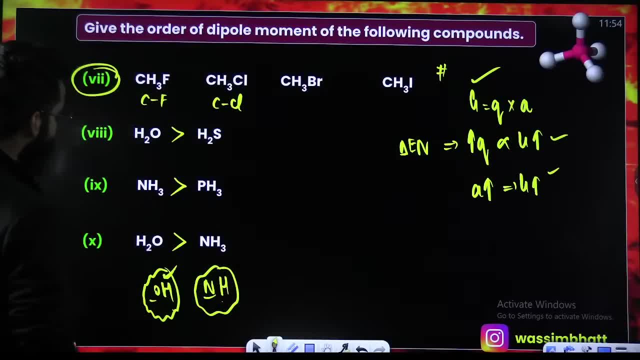 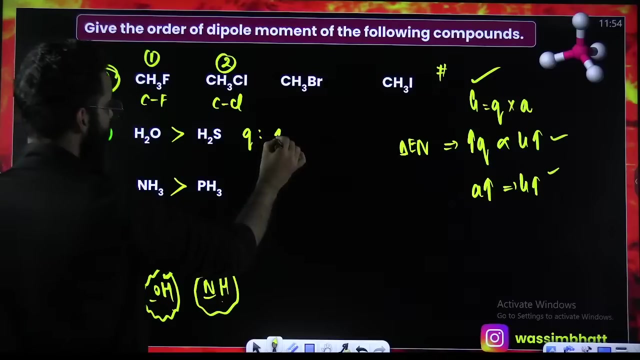 charge as well as distance, perfect. now, as for electro negative difference, as per electro negative difference. as per electro negative difference as per electro negative difference. if this is one, if this is one, this is two. as per charge factor. as per charge factor, which one should have more dipole moment. 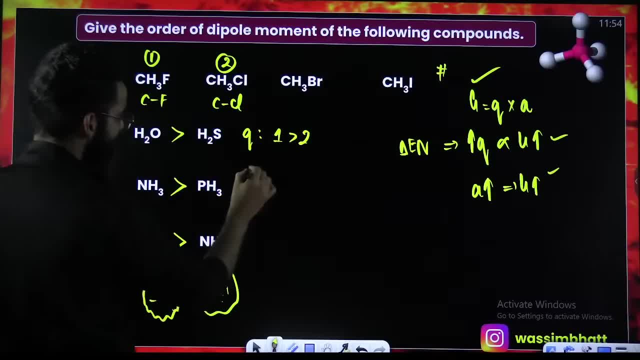 which one should have more dipole moment one will be greater than two. because more one will be greater than two. because more one will be greater than two, because more electron negative difference here, electron negative difference here, electron negative difference here. as per distance factor, ccl bond length is. 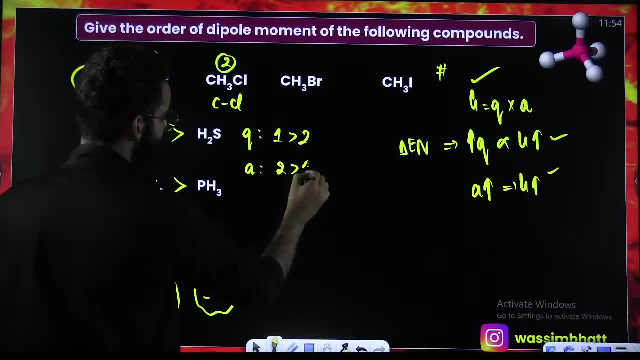 as per distance factor, ccl bond length is. as per distance factor, ccl bond length is more, more, more than cf. as per distance factor two is than cf. as per distance factor two is than cf. as per distance factor two is greater than one, greater than one. 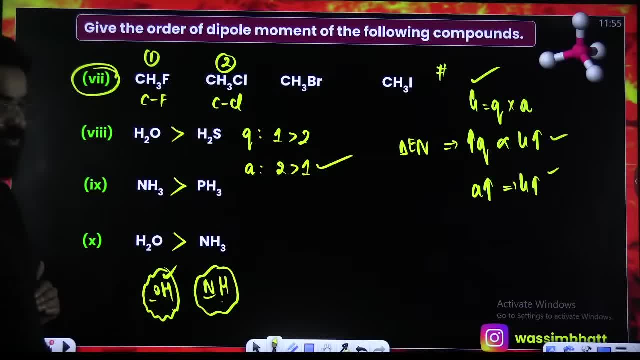 greater than one right. this is the special case. where is right? this is the special case. where is right? this is the special case. where is distance factor dominates? distance factor dominates? distance factor dominates. where is distance factor dominates, so in where is distance factor dominates so in where is distance factor dominates? so in this particular case, in this particular? 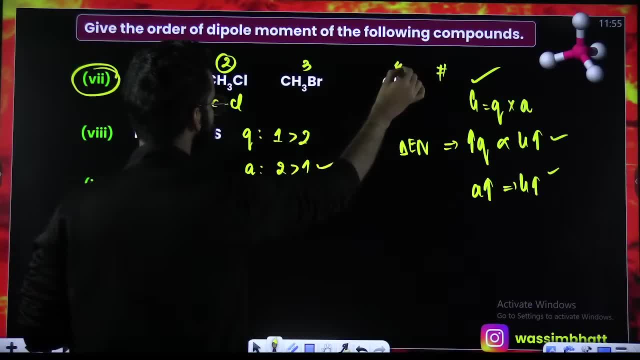 this particular case, in this particular, this particular case, in this particular case, let me tell you this is three, this case, in this particular case, let me tell you this is three, this case, in this particular case, let me tell you this is three, this is four. right, the order will be two. 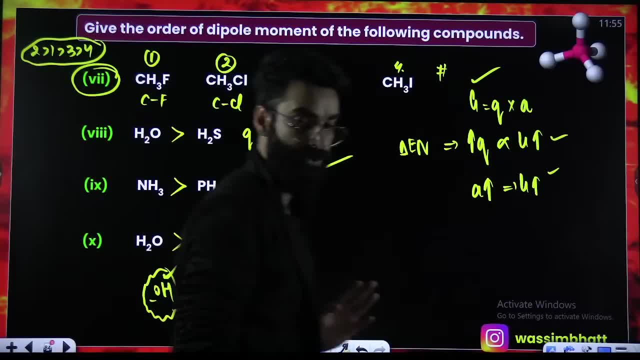 is four right, the order will be two. is four right, the order will be: two, one, three, four. two, one, three, four. do one, three, four. two, one, three, four. do one, three, four, two, one, three, four. do remember it directly, remember it directly, remember it directly. distance part dominates over here in this. 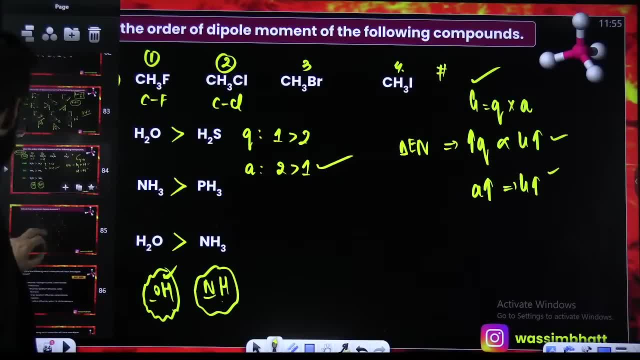 distance part dominates over here, in this distance part dominates over here in this particular case, particular case, particular case, in this particular case, in this particular case, in this particular case. look at this nice question among these, look at this nice question among these. look at this nice question among these four. among these four give the order of. 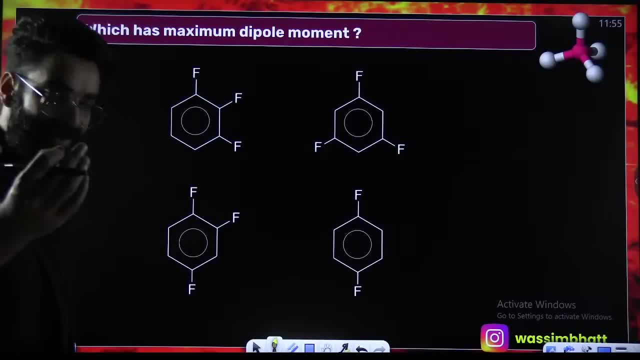 four among these four, give the order of four among these four. give the order of dipole, give the order of net dipole, give the order of net dipole, give the order of net dipolement, dipolement, dipolement. understand one thing, guys, just one thing. 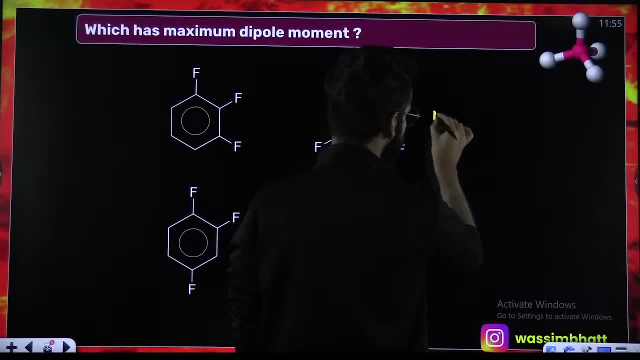 understand one thing, guys, just one thing. understand one thing, guys, just one thing, just one thing. this i believe you would just one thing. this, i believe you would just one thing. this i believe you would have studied in your vectors, have studied in your vectors, have studied in your vectors, if this is one vector pointing in this. 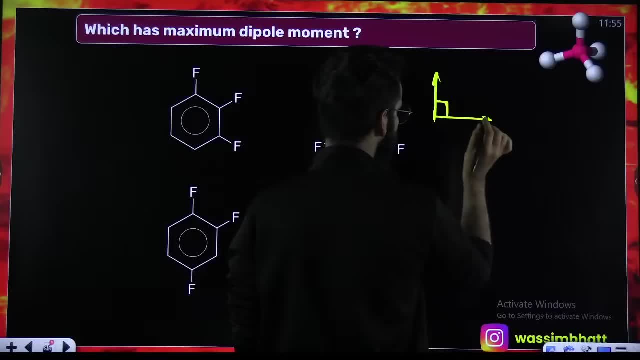 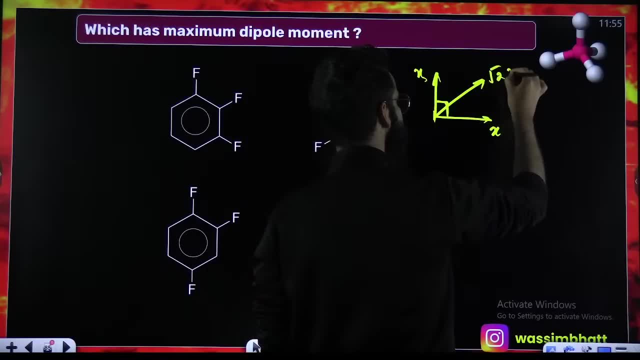 at an angle of 90.. its magnitude is x at an angle of 90.. its magnitude is x. this is x. your resultant will be in: this is x. your resultant will be in. this is x. your resultant will be in this direction. it will be root to x. 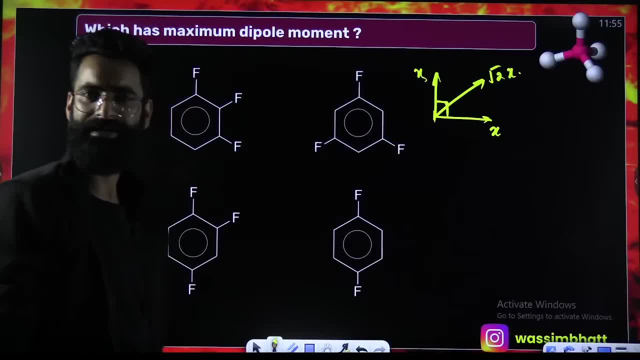 this direction, it will be root to x. this direction, it will be root to x. which would have studied right, i believe, which would have studied right, i believe, which would have studied right, i believe. i believe you have studied that. i believe you have studied that. i believe you have studied that. okay, perfect, let's say this one vector: 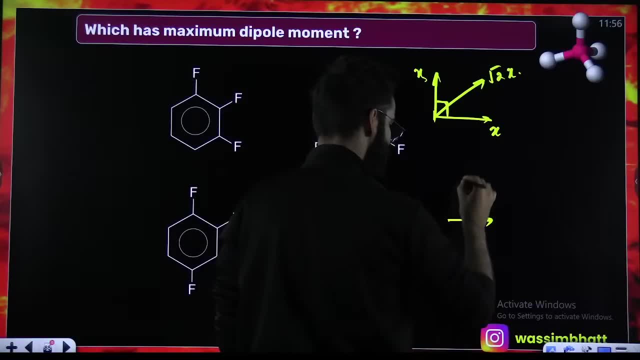 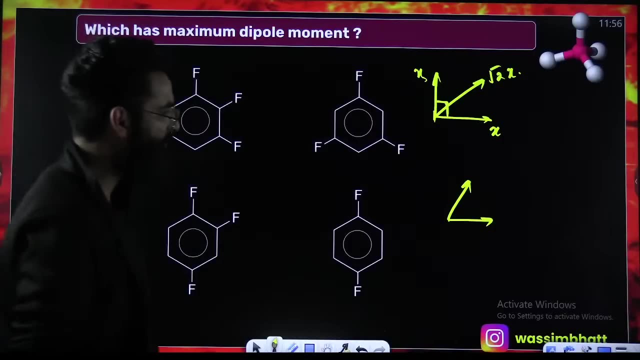 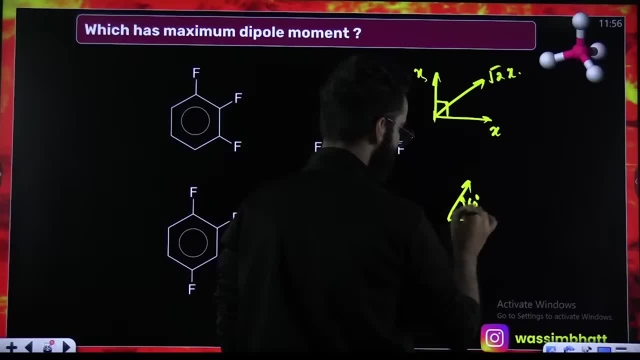 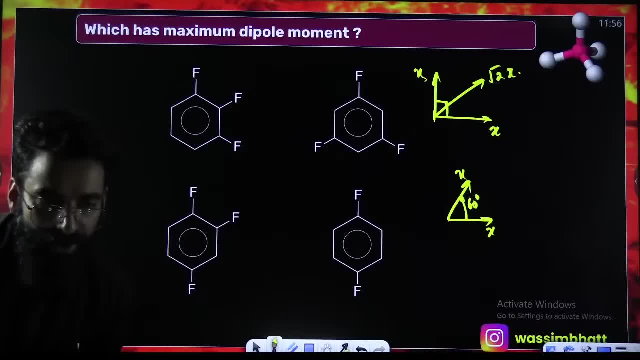 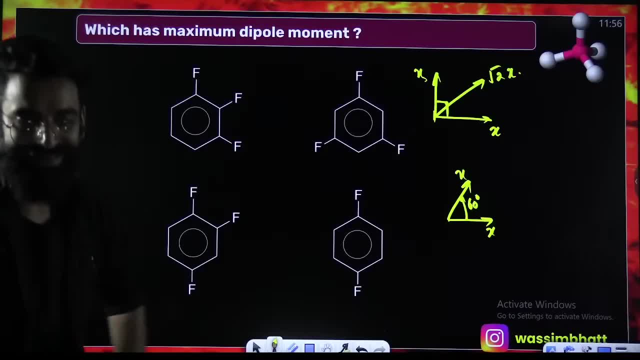 quickly, quickly, resultant masking at 60. what is the resultant? guys, recently yavarsan was teaching you guys. recently yavarsan was teaching you guys. recently yavarsan was teaching you all this in electrostatics right two: all this in electrostatics right two. 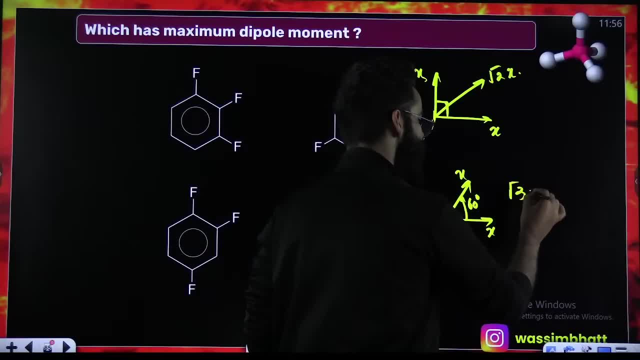 all this in electrostatics, right two days back, only days back, only days back. only right resultant is going to be root of right resultant is going to be root of right resultant is going to be root of 3x correct, 3x correct, 3x correct. if this is one vector, this is one more. 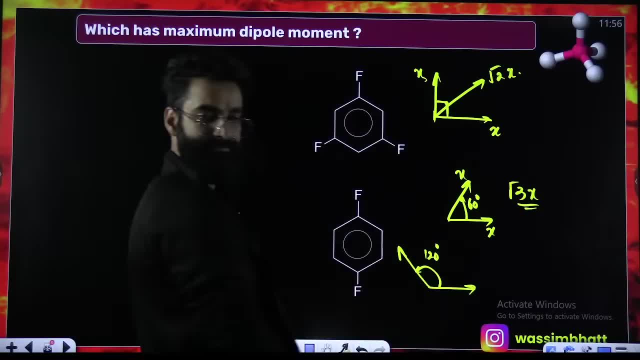 if this is one vector, this is one more. if this is one vector, this is one more. vector at an angle of 120. vector at an angle of 120. vector at an angle of 120 resultant at an angle of 120 resultant resultant at an angle of 120 resultant. 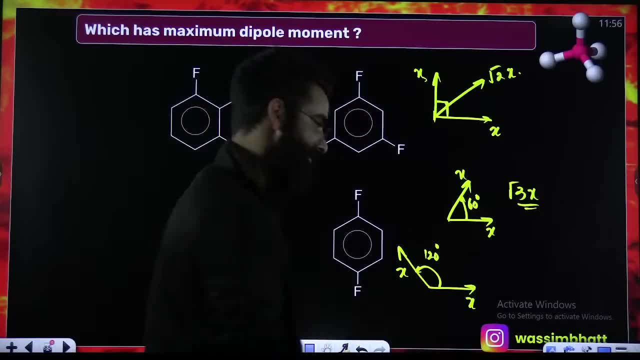 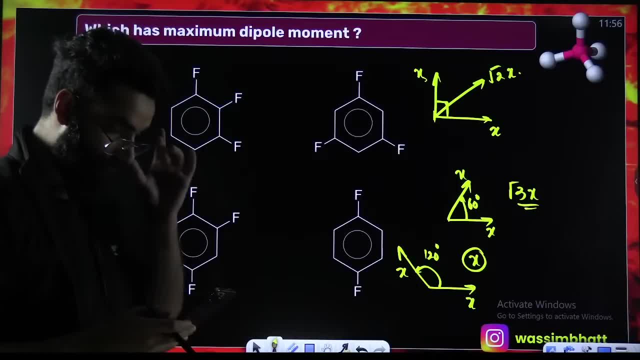 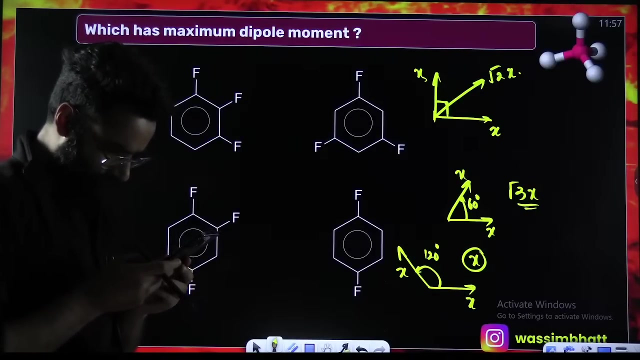 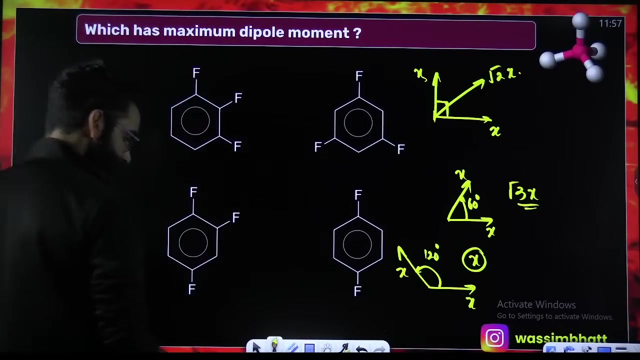 resultant here is going to be x only. resultant here is going to be x only. yeah, the resultant here is going to be x only. resultant here is going to be x only. the resultant here is going to be x only. okay, moving ahead, see guys. okay, moving ahead, see guys. 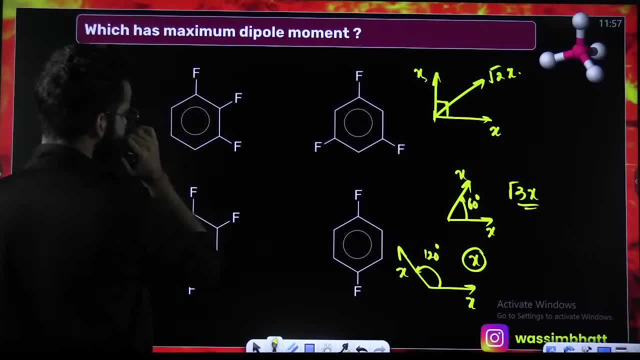 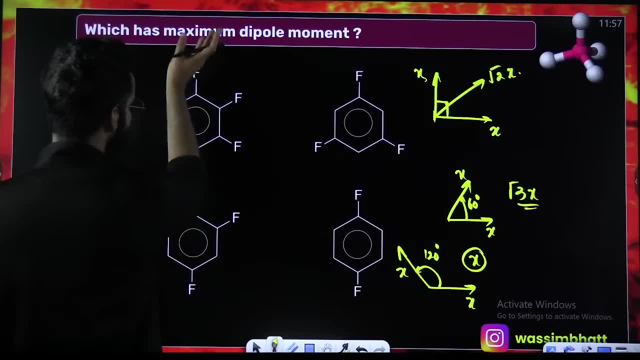 don't again withdrawing donating or don't again withdrawing. donating or withdrawing quickly withdrawing quickly, withdrawing quickly. chlorine donating or withdrawing. it's chlorine donating or withdrawing. it's chlorine donating or withdrawing. it's withdrawing, withdrawing. withdrawing it's withdrawing. it's withdrawing right so delta negative. withdrawing right so delta negative. 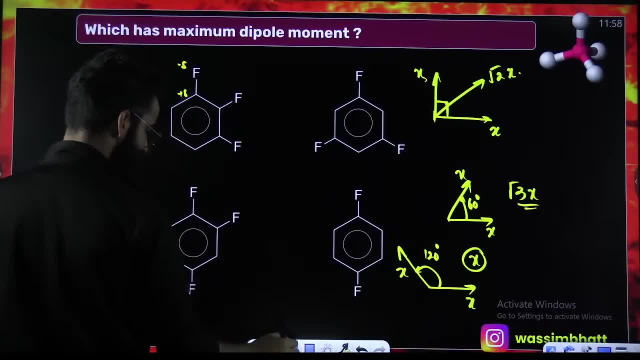 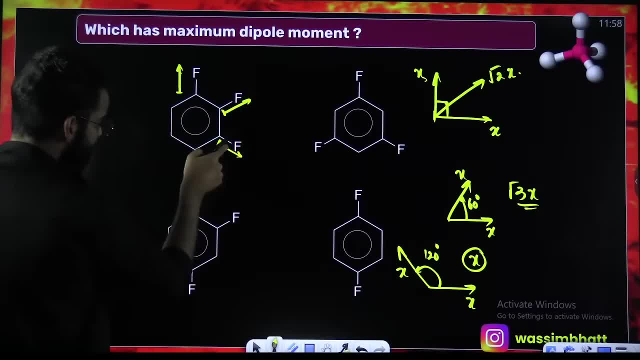 this is going to be positive, negative. this is going to be positive, negative. similarly, this is going to be positive. similarly, this is going to be positive. similarly, this is going to be positive, negative. perfect if you look at this negative. perfect if you look at this negative. perfect if you look at this vector and this vector: they are at an 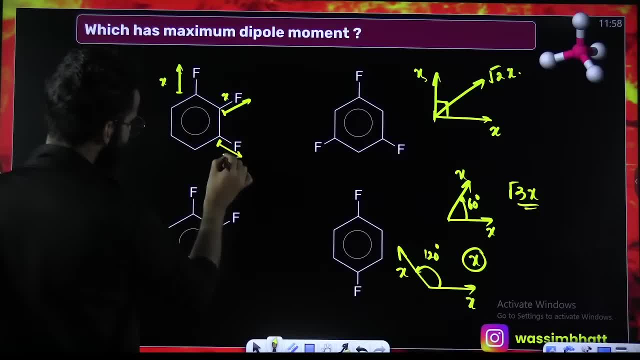 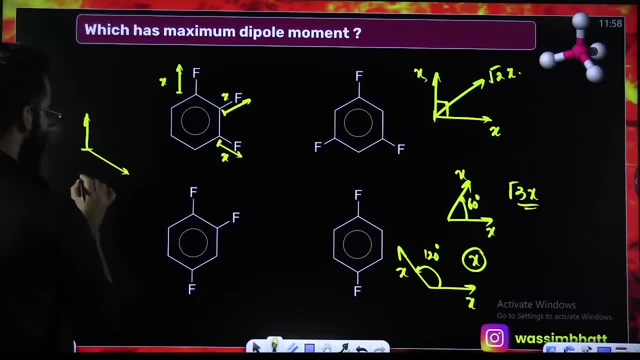 let's call this as x this and this. they let's call this as x this and this. they are an angle of one is going upwards. are an angle of one is going upwards. are an angle of one is going upwards. one is going in this direction, right. 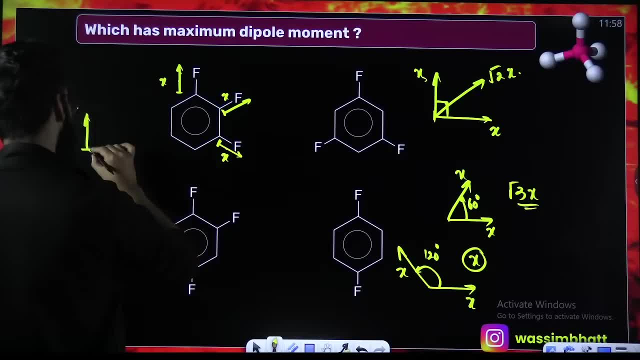 one is going in this direction, right. one is going in this direction, right. they are an angle of 120, so resultant of. they are an angle of 120, so resultant of. they are an angle of 120, so resultant of this and this, this and this, this and this, at an angle of 120, is going to be x only. 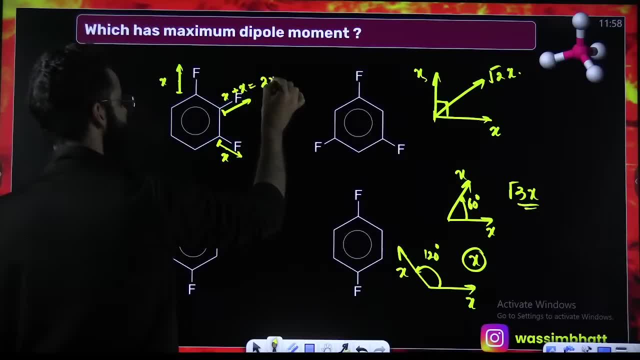 at an angle of 120 is going to be x. only at an angle of 120 is going to be x. only already in this direction there was x. already in this direction, there was x. already in this direction, there was x. so x plus x makes it to x. 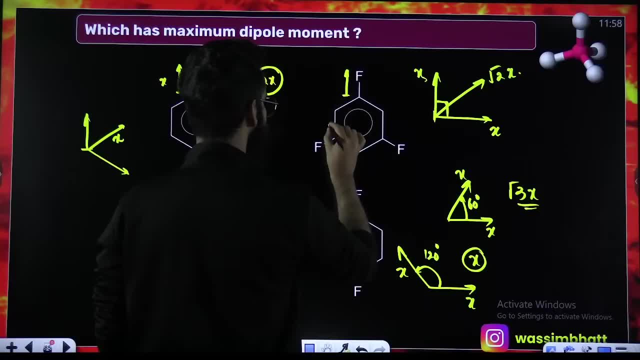 so x plus x makes it to x, so x plus x makes it to x. right, right, right. similarly positive to negative, positive. similarly positive to negative, positive, similarly positive to negative, positive to negative, positive to negative, correct to negative, positive to negative, correct to negative, positive to negative, correct these two. they are at angle of 120, so 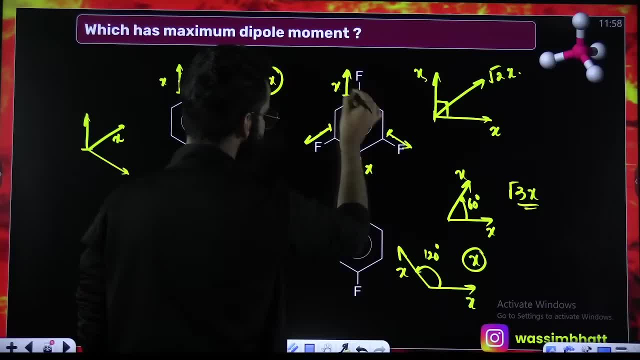 these two, they are at angle of 120. so these two, they are at angle of 120. so resultant is x, so this is x. resultant is x, so this is x. resultant is x, so this is x. and this is x. right? they'll cancel out. and this is x, right? they'll cancel out. 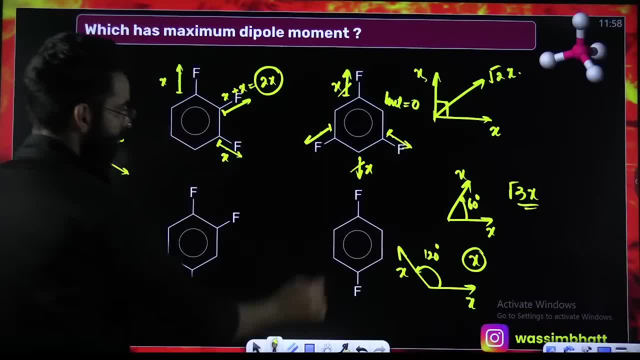 and this is x right. they'll cancel out. so net is zero. so net is zero. so net is zero. this is the resultant of these two. this is the resultant of these two. this is the resultant of these two. resultant of these two, and this one: resultant of these two and this one. 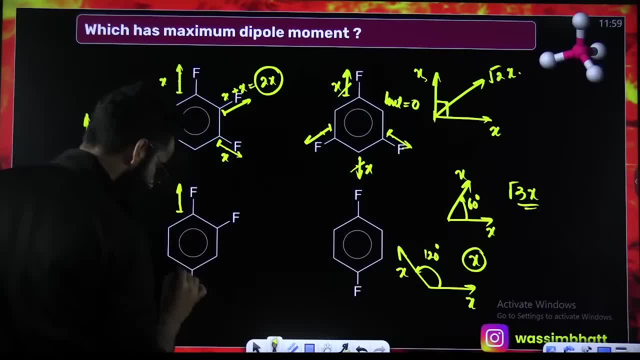 resultant of these two and this one: they'll cancel out. net is zero. similarly, they'll cancel out. net is zero. similarly, they'll cancel out. net is zero. similarly, positive to negative. two positive, positive to negative, two. positive, positive to negative, two positive, negative, two. positive to negative, two. 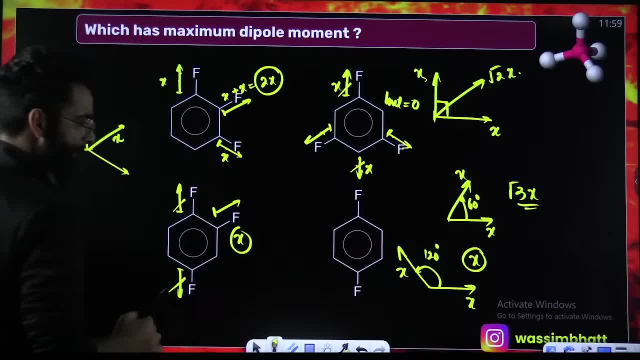 negative two. positive to negative two negative two positive to negative two perfect, so this. and this cancels the perfect, so this and this cancels the perfect, so this and this cancels the resultant. here is x resultant. here is x resultant. here is x. right, okay, positive, negative two. 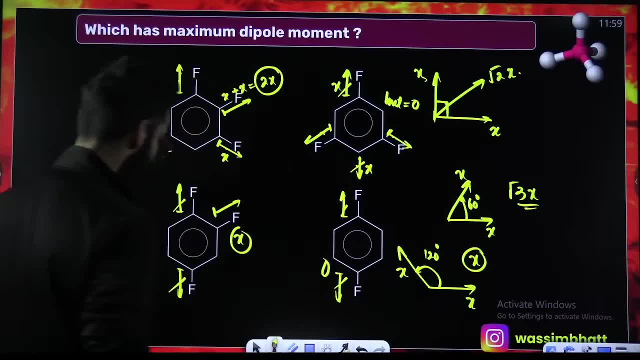 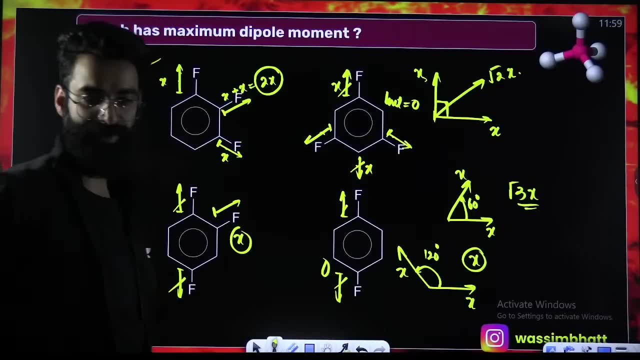 right, okay, positive negative. two right. okay. positive negative. two positive negative. two right- cancel out. positive negative two: right, cancel out. this is zero, perfect. now which one has got a maximum dipole moment here? this is 2x 0, 0 X, so first one has got a maximum dipole moment. I hope you can solve these. 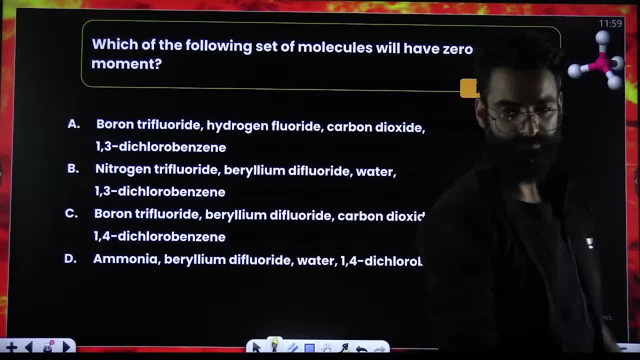 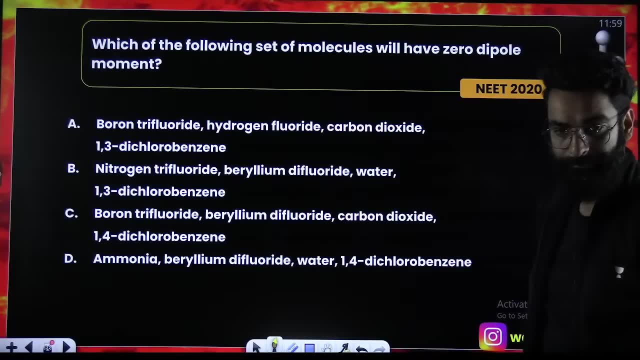 sort of questions. NEET 2020: one question was asked from the same. NEET 2020: one question was asked: can you give it a try? which of the following set of molecules will have zero dipole moment? zero dipole moment quickly. is this something which you should answer now? 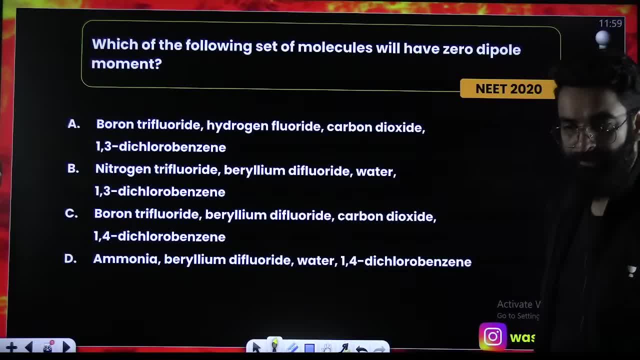 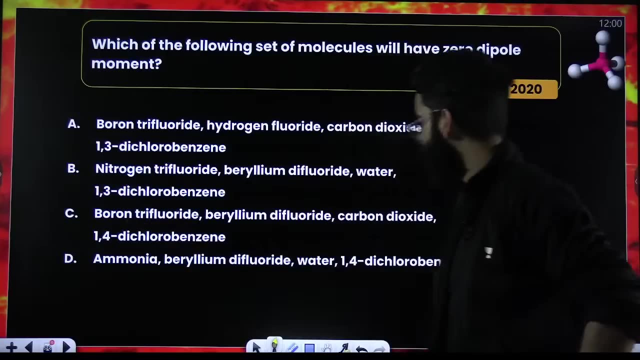 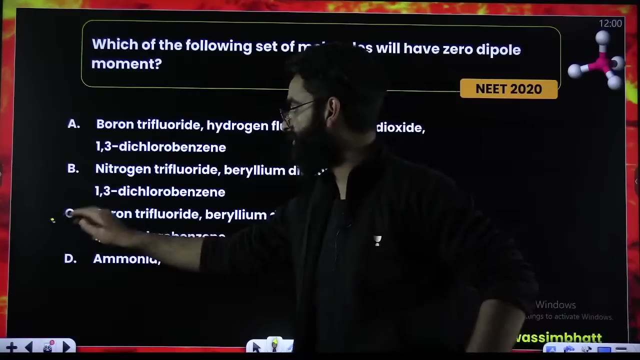 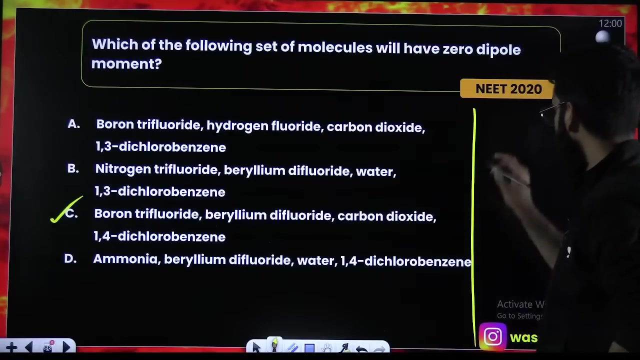 you quickly in the charts, quickly in the charts. everyone you which of the following will have zero dipole moment? we BF3, BF2 for dichlorobenzene. This is going to be the answer. One more thing which I want you guys to remember for now. You will get the actual idea in some time. Remember whenever you see. 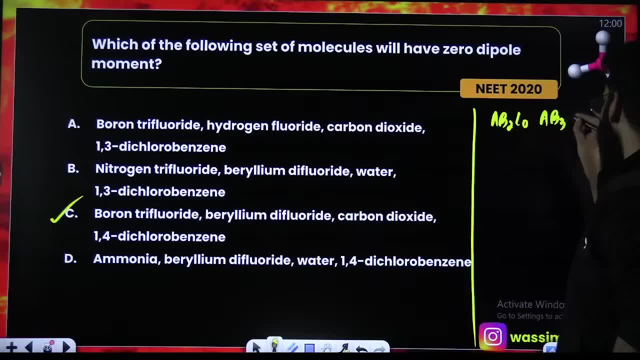 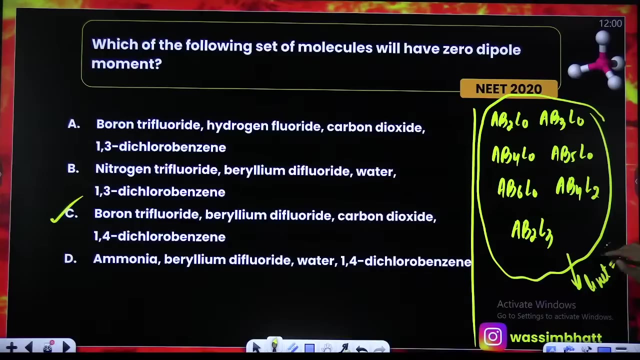 a molecule of the type AB2L0, AB3L0, AB4L0, AB5L0, AB6L0, AB4L2, AB2L3, AB2L3,. all these molecules have got their net dipole. moments will be zero. 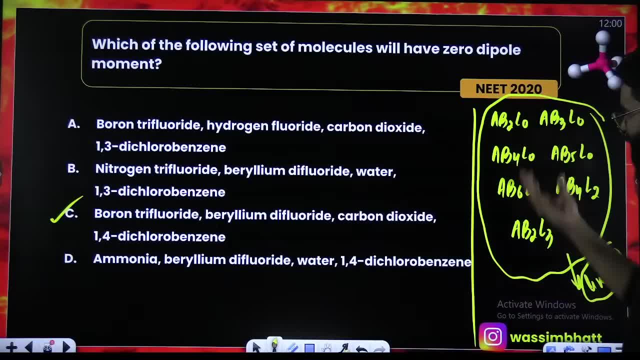 Now, how do we check this? How do we check what is the type of the molecule, whether it is roadsorban, whether it is waving? where does it come from? what is the curve? AB2L0,, AB3L0, etc. 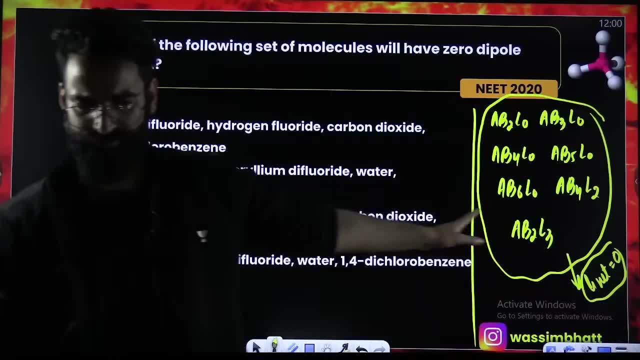 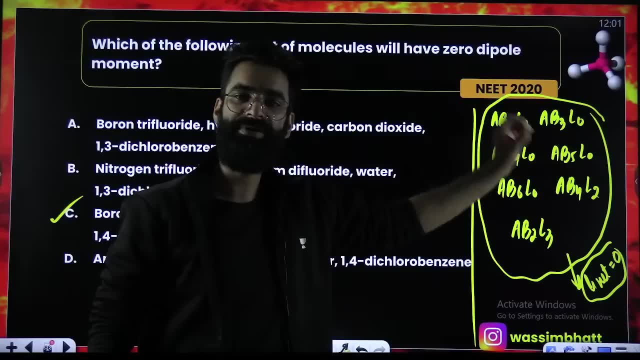 That is something which you will understand in some time. Just remember it for now. Just remember it for now. Okay, All these molecules, all these types of molecules, will be having net deployment always 0.. Right, How do we check? How do we check it? What is the type of? 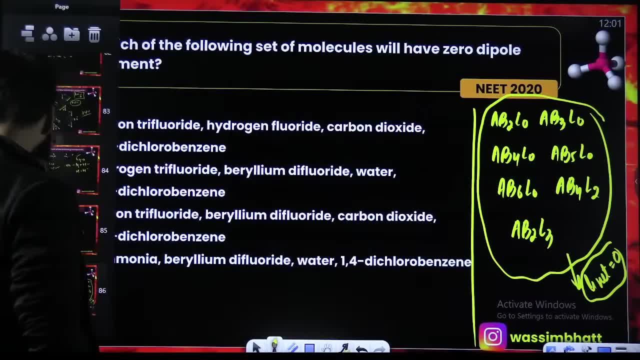 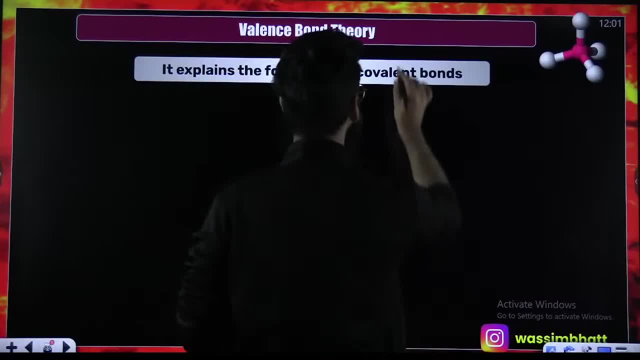 the molecule that you will understand in some time. Perfect, I hope. all the things are absolutely clear till here, Now, now let's talk about one of the most important theories of this chapter. That is, valence bond theory. my dear students, Valence bond. 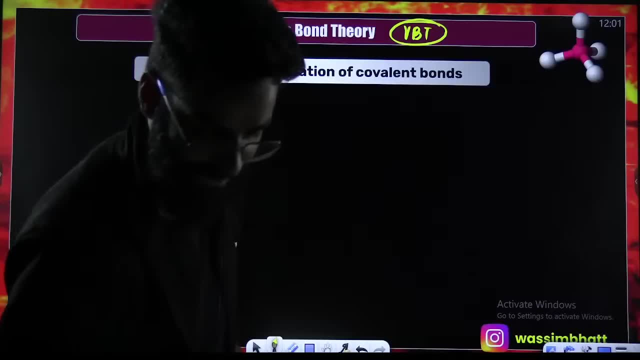 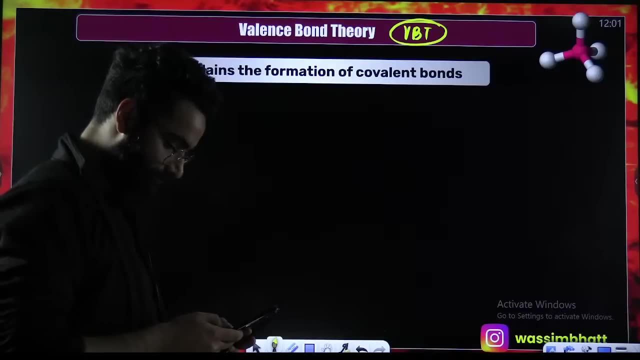 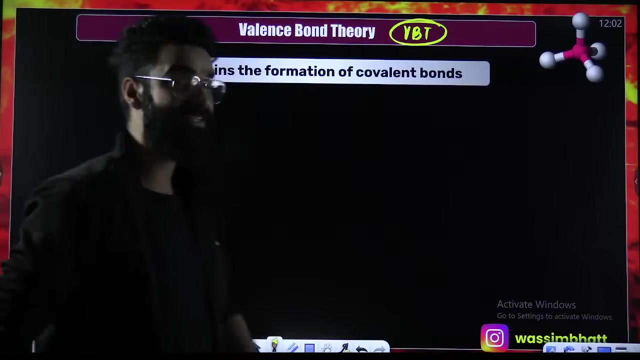 theory. But before starting the valence bond theory, let me know in the chats if every single thing is clear. Quickly people, Quickly people. Okay, guys, Let's talk about, let's start, this amazing theory which is the valence bond theory. 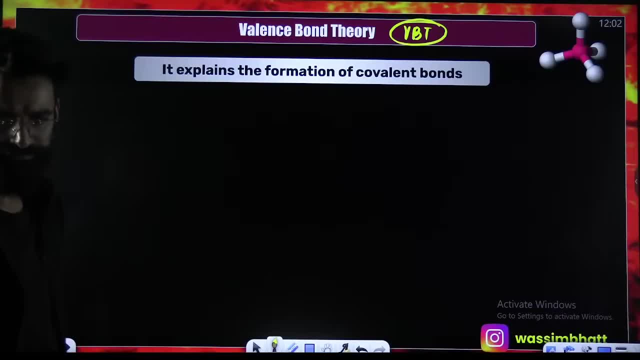 Right From this theory, a short, short question will be asked again. Okay, Short, short question From this particular theory, And it's simple, It's very simple What this VBT is all about, My dear students: this valence bond theory, it. 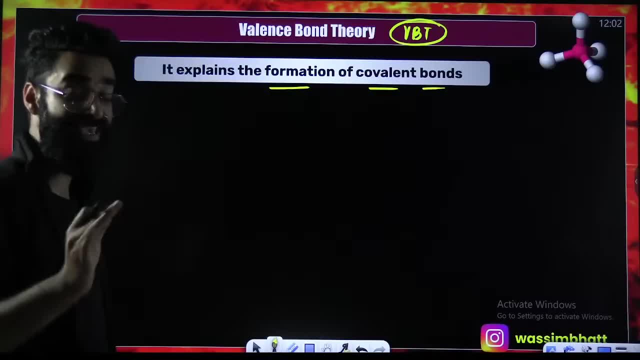 explains the formation of covalent bonds. First thing, it explains the formation of covalent bonds. This theory is going to let you know how a covalent bond actually gets formed. How a covalent bond actually gets formed- Right, How a covalent? 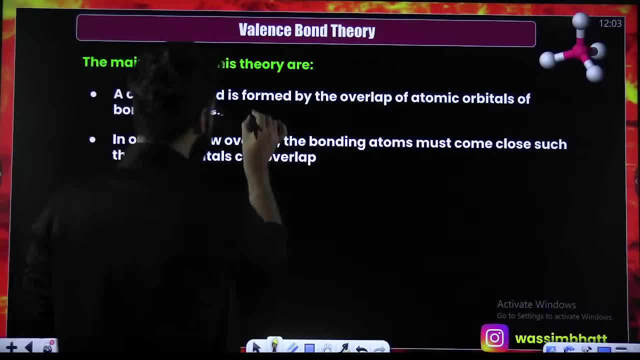 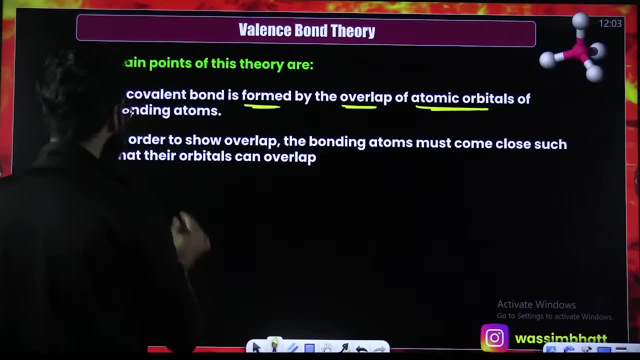 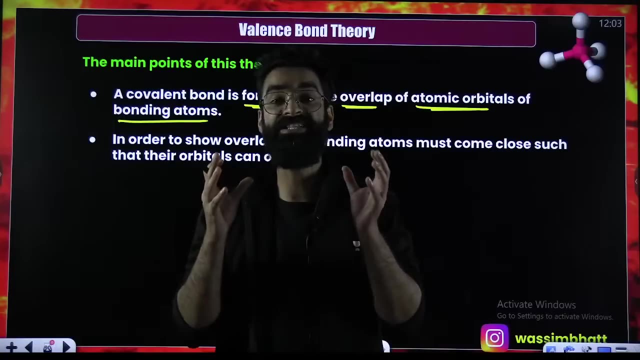 bond actually gets formed. As per this theory is concerned, a covalent bond is formed by the overlap, by the overlap of atomic orbitals, of the bonding atoms. As per this particular theory is concerned, a covalent bond gets formed when the 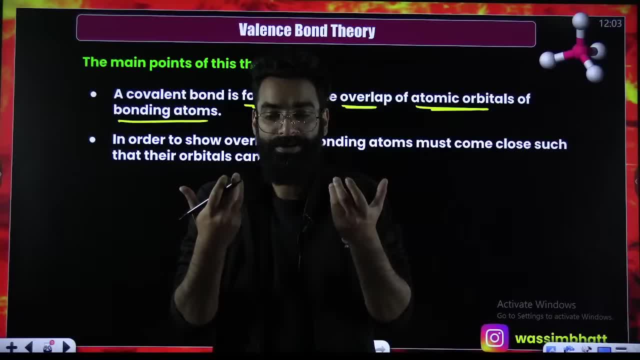 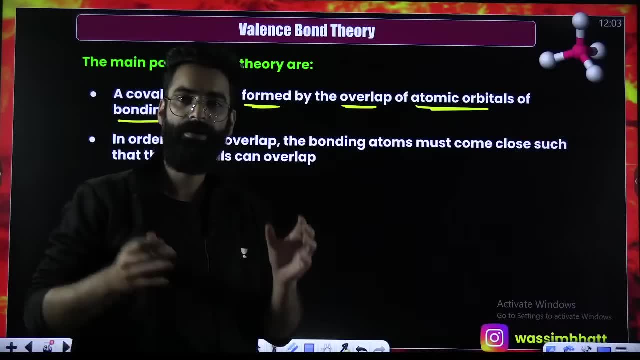 when the orbitals, when the orbitals of the bonding atoms, when they overlap, when they penetrate into each other. First of all, you must be thinking: what is overlapping? Overlapping of atomic orbitals means penetration of atomic orbitals into each other. Penetration of 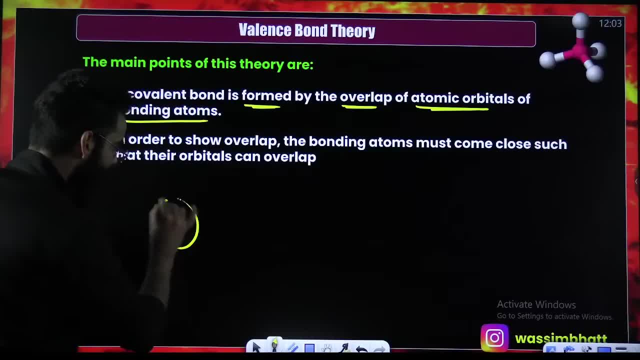 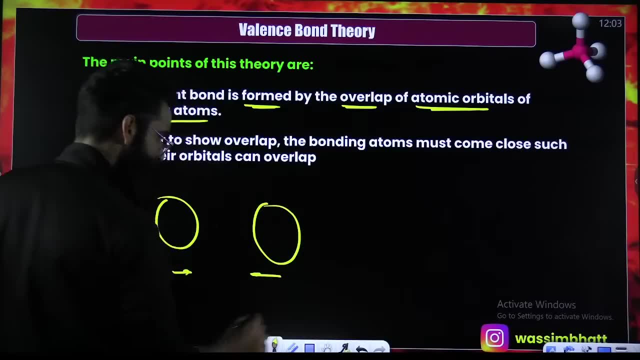 atomic orbitals into each other. For example, this is one of the orbital of one of the atom. This is one more orbital of one more atom. Now let's say they are coming closer. If they are coming closer, what is going to happen? 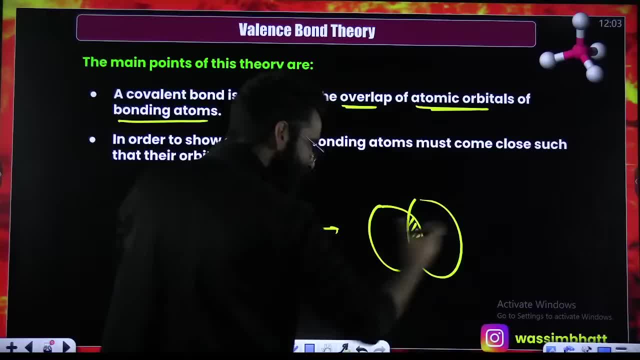 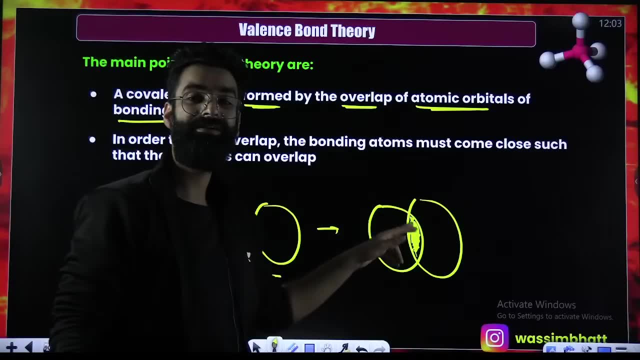 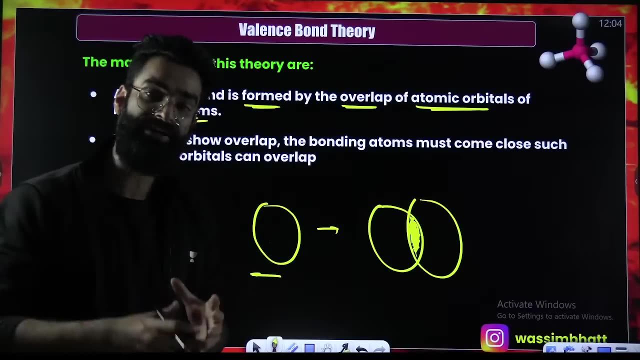 Their atomic orbitals. they will overlap Right, They will merge into each other. This merging of electron cloud, this merging of electron cloud into each other, is something which you call as overlapping Right, And do remember whenever you see overlapping of atomic. 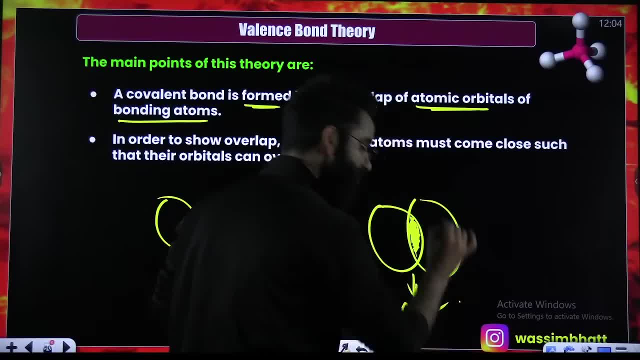 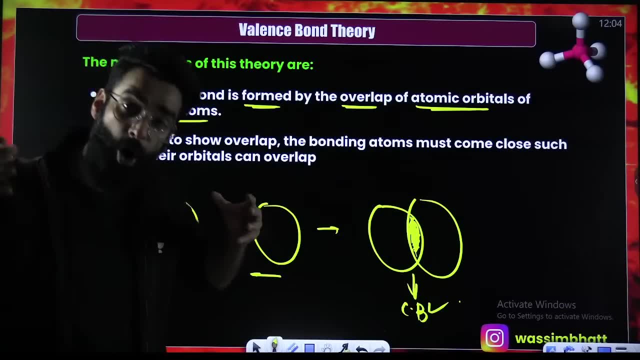 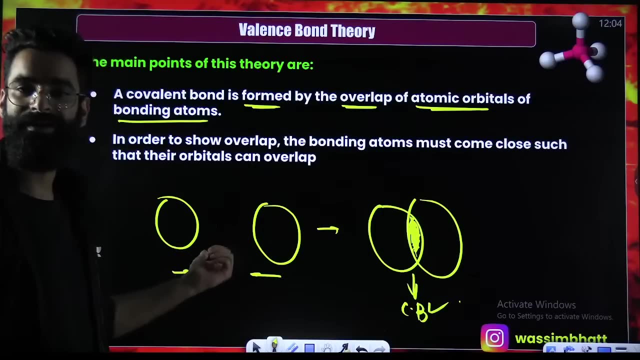 orbitals taking place, it always leads to the formation of which bond? It always leads to the formation of covalent bond. So, as per VBT is concerned, a covalent bond is formed by the overlapping of atomic orbitals into each other. okay, and people you know, in order to show the overlapping in, in order to show the 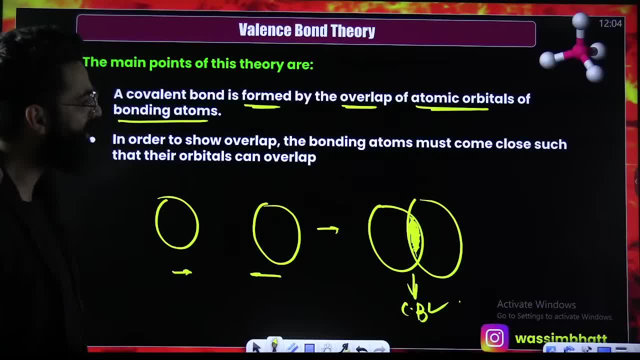 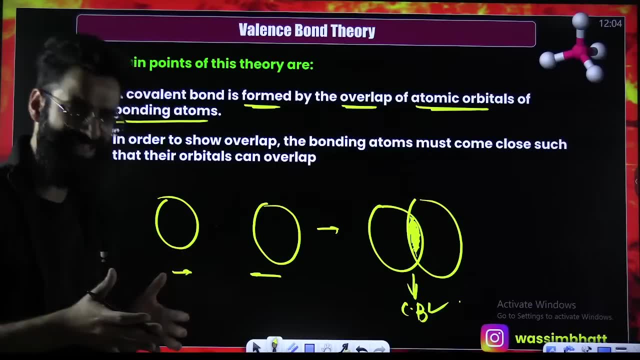 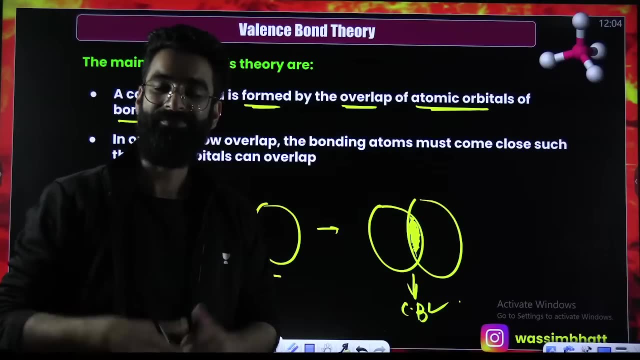 overlapping the bonding atoms. the bonding atoms, they must come close, they must come close, they must come close right in order to show overlapping the bonding atoms, they have to come close. then only this overlapping, then only this merging of electron cloud into each other will happen right. and whenever electron clouds merge into each other, remember overlapping has happened. 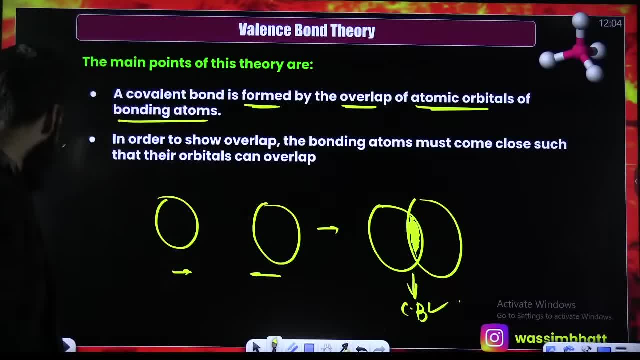 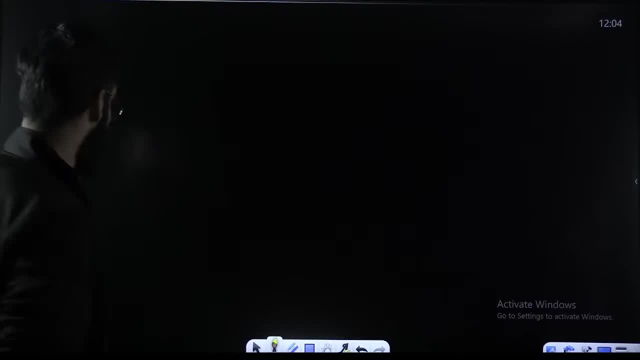 and, due to overlapping, covalent bond gets formed. as simple as that. as simple as that. as simple as that. now, here are a few things which i would want to discuss with you, idea students, before understanding this vbt in detail. there are few things, there are some. 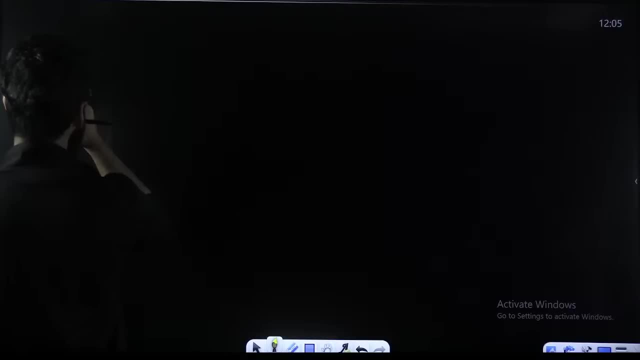 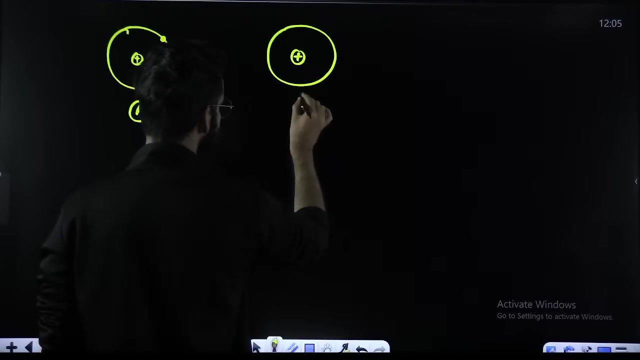 there are some basic things which you need to know. what are the? what are those? let's say this is one atom. okay, this is one atom a. let's see, this is the electron of this atom. let's say: this is the atom b and this is the electron of b. i'm calling this as nucleus of a. 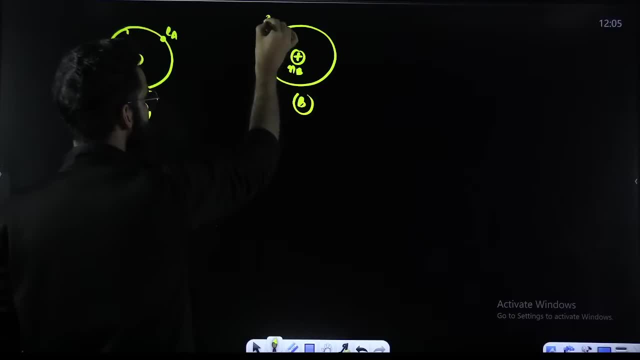 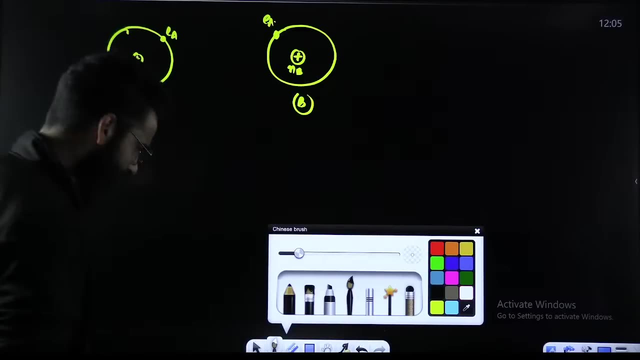 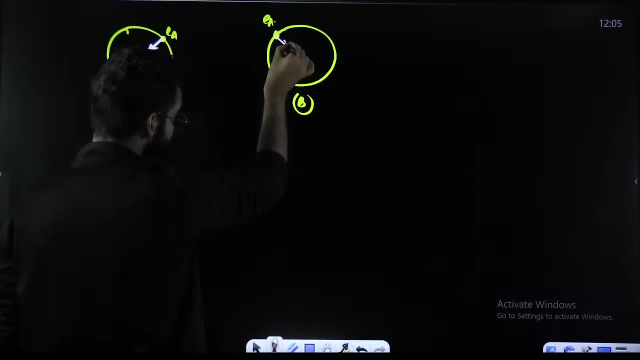 electron of a. i'm calling this as nucleus of b, electron of b. can you let me know how many forces exist, how many forces will arise between these two atoms? first thing, this nucleus will be attracting its own electron towards itself. yes, this nucleus will be attracting its own electron towards itself. 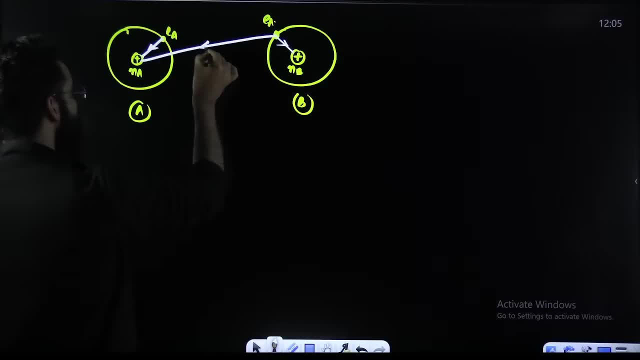 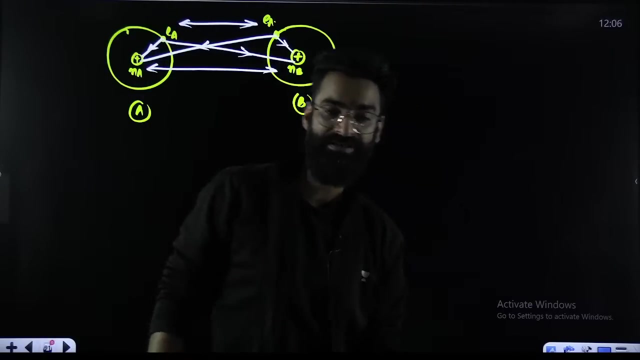 yes, this nucleus will be attracting this particular electron towards itself. yes, this nucleus will be attracting this particular electron towards itself. right, perfect. between these two electrons, there will be repulsions. between these two nucleus, there will be repulsions. so, between these two atoms, how many forces are arising? how many forces do we have? we have got two types of forces. 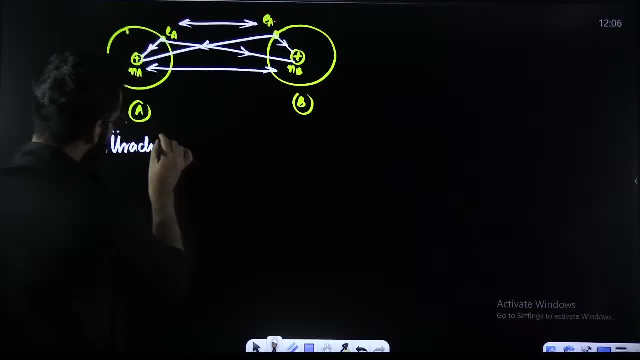 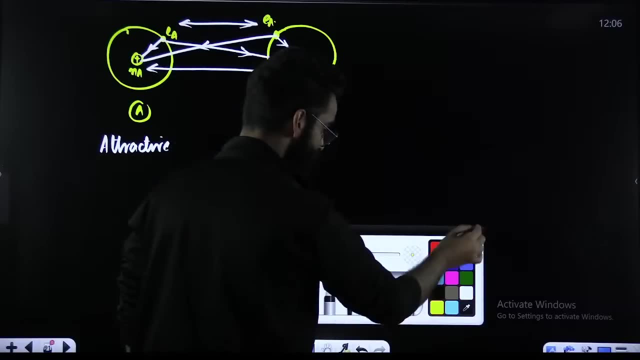 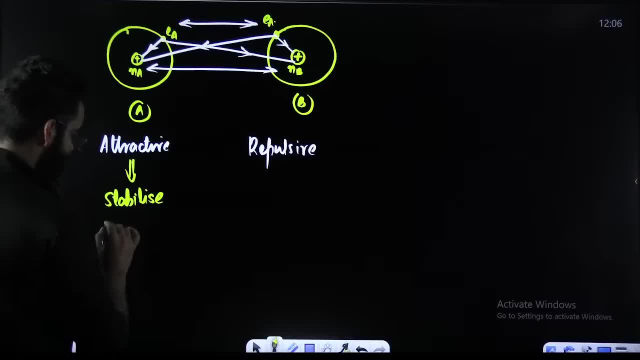 so we have got repulsive forces between the atoms to the atom. so we have got repulsive forces between the atoms to the atom, attractive forces as well as repulsive, attractive forces as well as repulsive, attractive forces as well as repulsive forces. they try to increase the stability of the system. 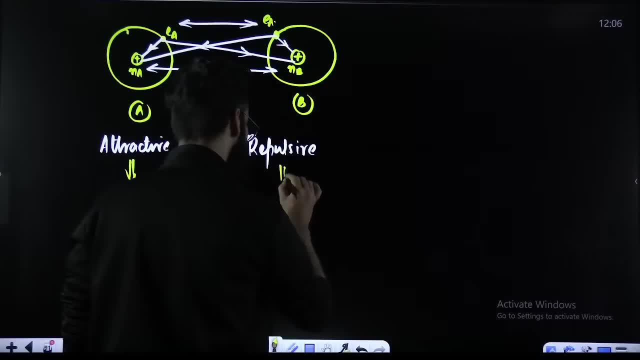 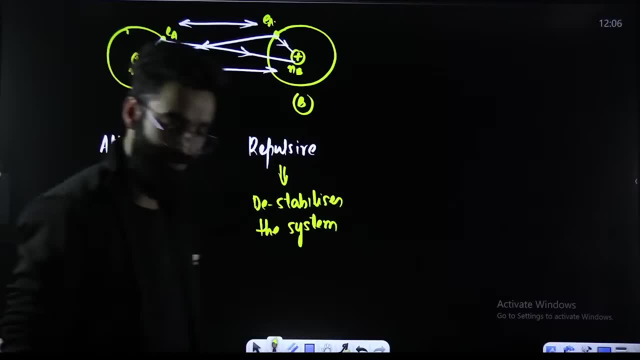 it destabilizes the system. remember these two points. it destabilizes the system. remember these two points. it destabilizes the system. remember these two points. attractive forces: they try to increase the attractive forces. they try to increase the attractive forces. they try to increase the stability of the system. 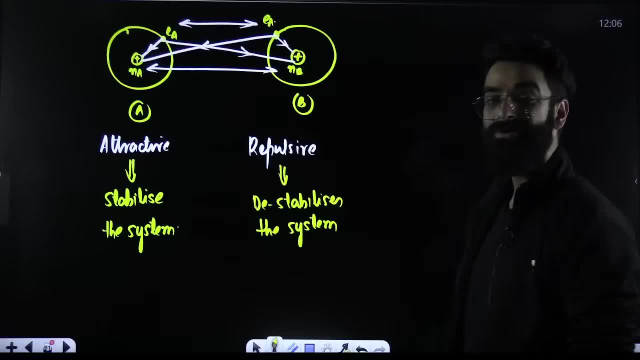 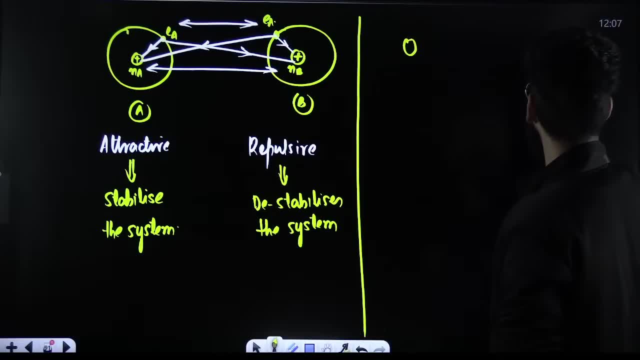 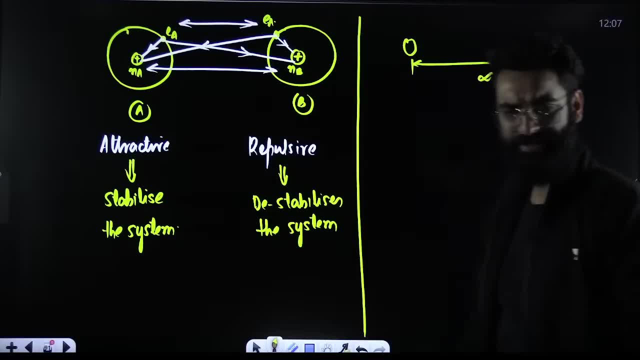 are at maximum. i mean these two are at maximum. i mean these two atoms are at infinite distance apart. atoms are at infinite distance apart. atoms are at infinite distance apart. imagine that these two atoms are at. imagine that these two atoms are at. imagine that these two atoms are at infinite distance apart. 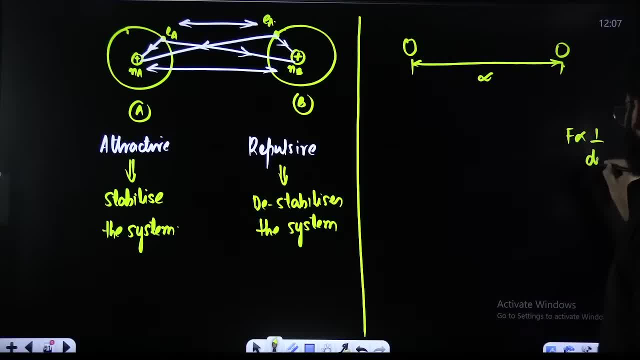 infinite distance apart. infinite distance apart. you know force of attraction is inversely. you know force of attraction is inversely. you know force of attraction is inversely proportional distance. proportional distance. proportional distance is inversely proportional distance if these is inversely proportional distance. if these is inversely proportional distance. if these atoms are at infinite distance apart. 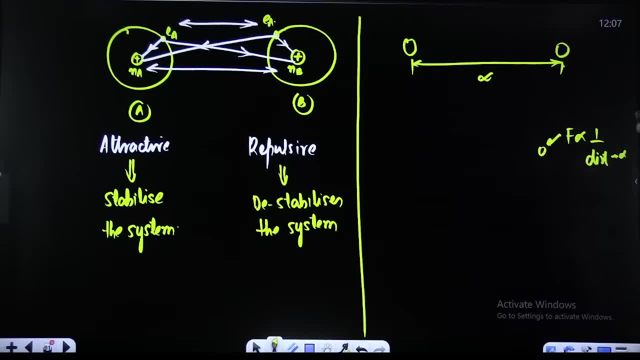 atoms are at infinite distance apart. atoms are at infinite distance apart. can i say force of attraction between? can i say force of attraction between? can i say force of attraction between them will be zero. so right now, between them will be zero. so right now between them will be zero. so right now, between these two atoms, force of attraction will. 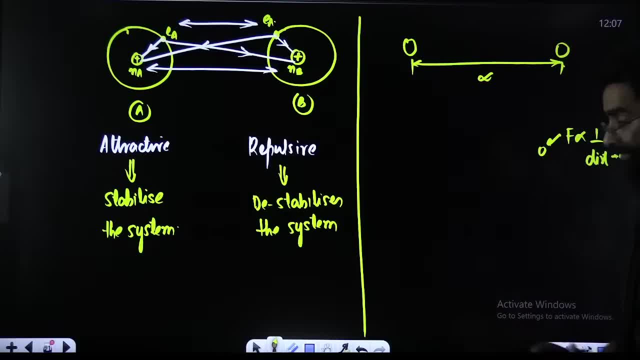 these two atoms force of attraction? will these two atoms force of attraction will be absolutely zero. force of attraction be absolutely zero. force of attraction be absolutely zero. force of attraction will be zero because these atoms are at will be zero, because these atoms are at will be zero, because these atoms are at infinite distance apart. now, 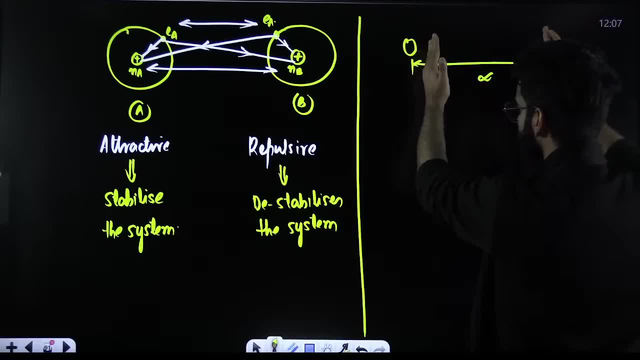 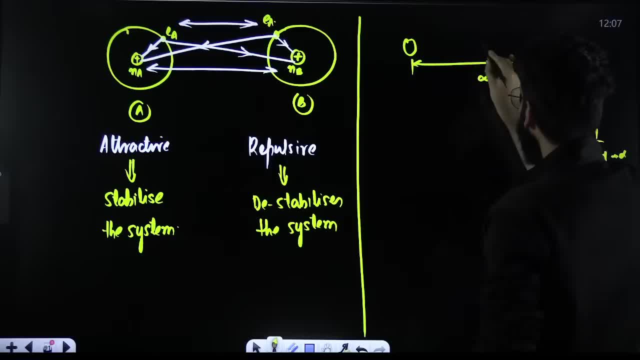 distance between them will decrease. force of attraction will increase. force of of attraction will increase. force of of attraction will increase. force of attraction will increase. attraction will increase. attraction will increase. can i say there will be a scenario when? can i say there will be a scenario when? 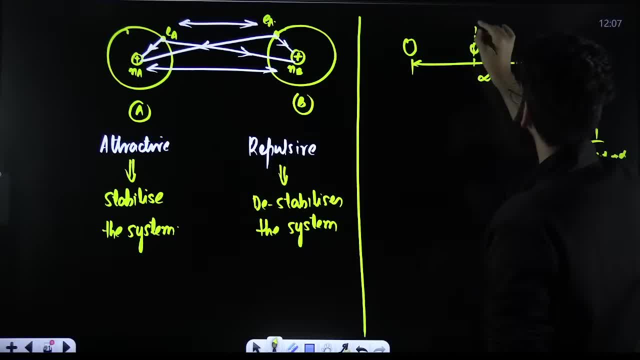 can i say there will be a scenario when these atoms will be at maximum closest. these atoms will be at maximum closest. these atoms will be at maximum closest distance. there will be a scenario when these atoms. there will be a scenario when these atoms. there will be a scenario when these atoms will be at maximum closest distance and 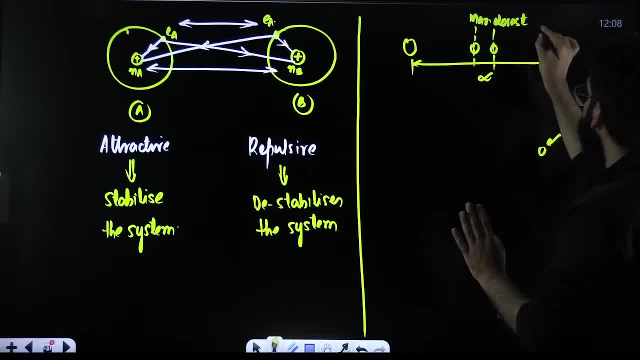 will be at maximum closest distance and will be at maximum closest distance. and let me tell you when the atoms are at. let me tell you when the atoms are at maximum closest distance. force of maximum closest distance. force of maximum closest distance. force of attraction between the atoms is maximum. 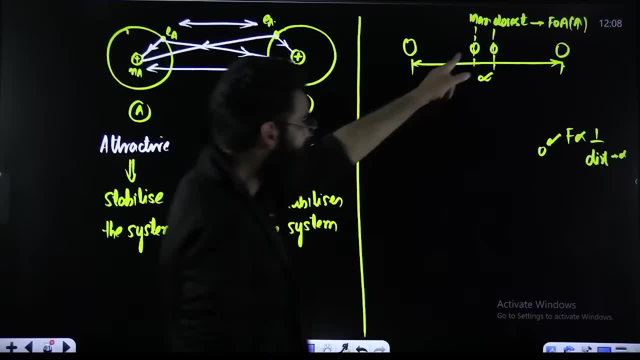 attraction between the atoms is maximum. attraction between the atoms is maximum. force of attraction between the atoms is force of attraction between the atoms is force of attraction between the atoms is maximum, maximum, maximum. at this point when the atoms are at. at this point, when the atoms are at 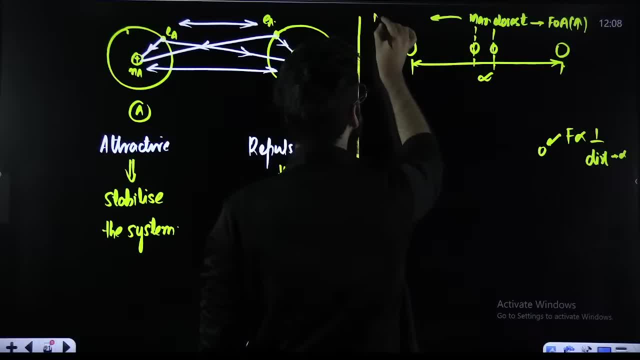 at this point, when the atoms are at maximum closest distance, at this point, we maximum closest distance, at this point, we maximum closest distance. at this point, we say: say: say, molecule has got formed, molecule has got formed, molecule has got formed, molecule formation has taken place, molecule formation has taken place. 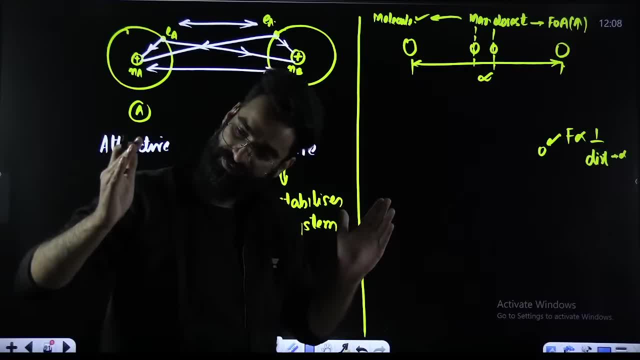 molecule formation has taken place, first atoms will be at infinite distance. first atoms will be at infinite distance. first atoms will be at infinite distance. but force of attraction: zero now atoms. but force of attraction zero now atoms. but force of attraction zero now atoms are coming closer, distance is decreasing. 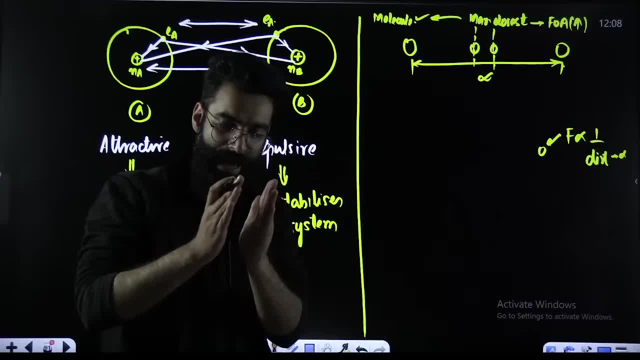 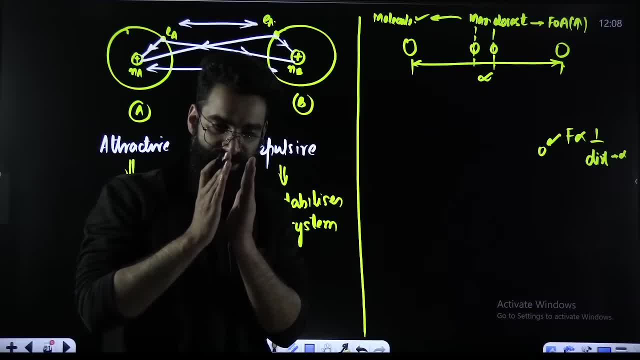 attraction increasing. now the atoms are at maximum closest distance. at maximum closest distance. at maximum closest distance. right force of attraction is maximum. right force of attraction is maximum. right force of attraction is maximum. right right force of attraction is maximum. right force of attraction is maximum. force of attraction is maximum. 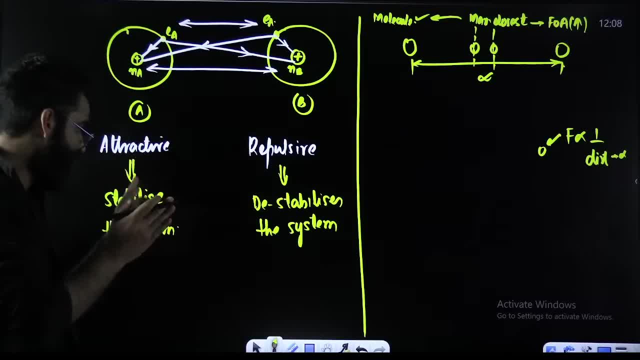 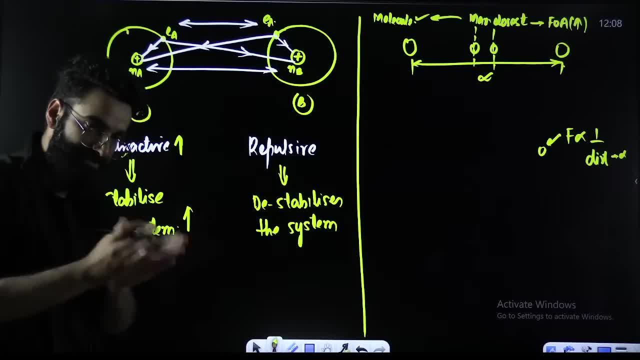 in the stability of the system, if force in the stability of the system, if force of attraction is maximum, stability is of. attraction is maximum, stability is of attraction is maximum. stability is maximum, stability is maximum. that means we maximum stability is maximum. that means we maximum stability is maximum. that means we say molecule has got formed. 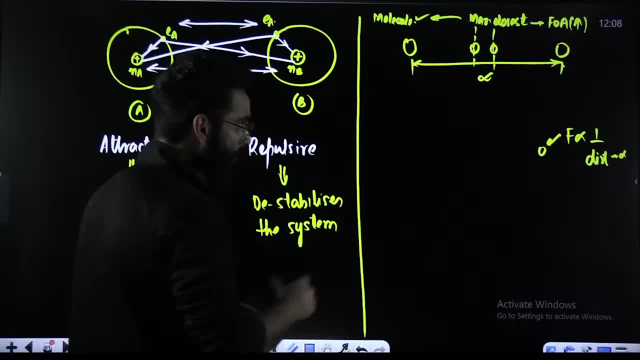 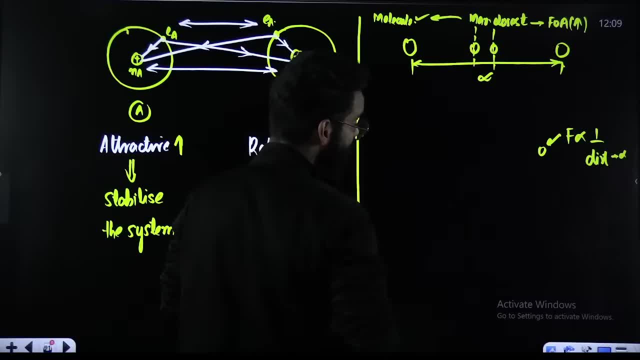 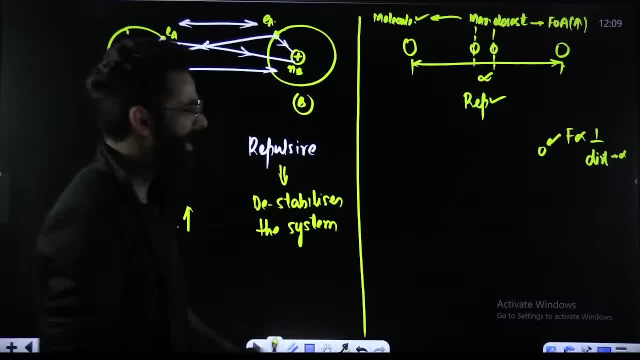 repulsive forces will start after this. repulsive forces will start after this point, point, point. repulsive forces will start after this. repulsive forces will start after this. repulsive forces will start after this point. can i say when atoms were far, point. can i say when atoms were far? 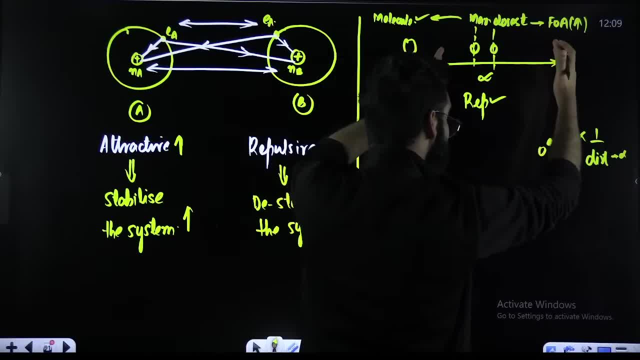 point, can i say, when atoms were far attractive, forces were existing in the attractive forces were existing in. the attractive forces were existing in the between the atoms, between the atoms, between the atoms. when the atoms are so close, repulsive. when the atoms are so close, repulsive. 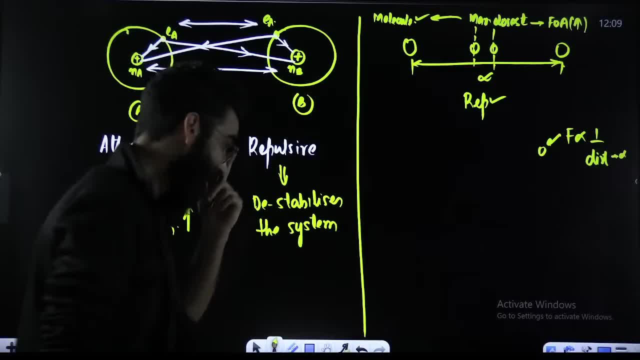 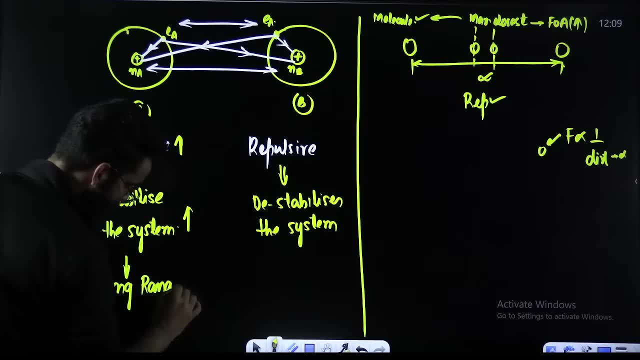 when the atoms are so close, repulsive forces arise between them. forces arise between them, forces arise between them. okay, so can i say your attractive forces. okay, so can i say your attractive forces. okay, so can i say your attractive forces. they are, they are, they are long range forces. 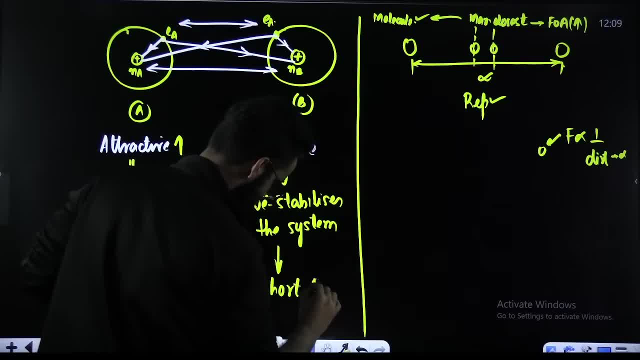 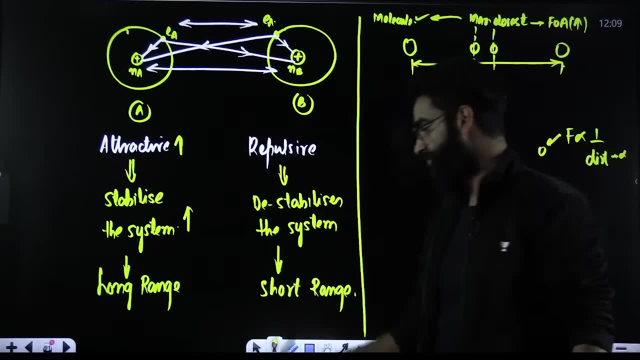 your repulsive forces they are. they are short range forces. can i say short range forces? can i say something like this? something like this, something like this: attractive forces are long range force, attractive forces are long range force. attractive forces are long range force, whereas repulsive forces they are. 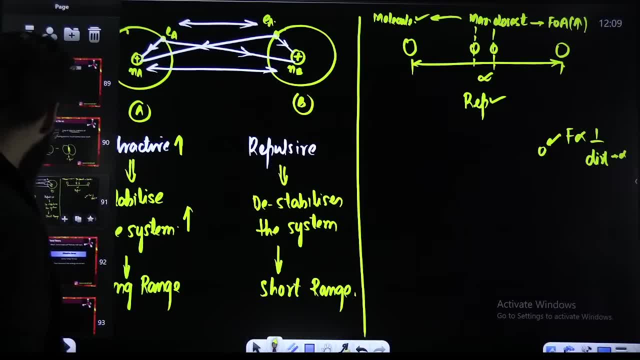 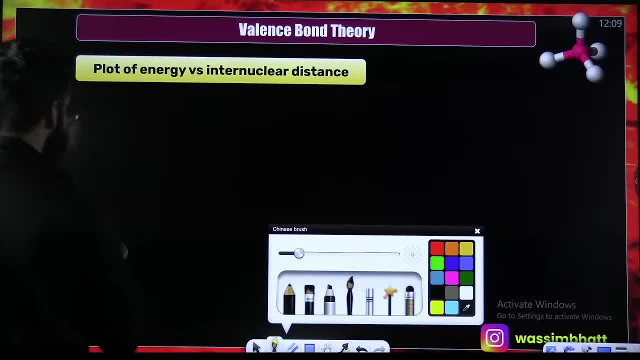 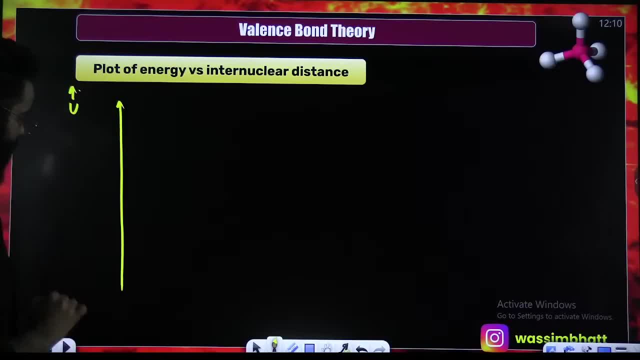 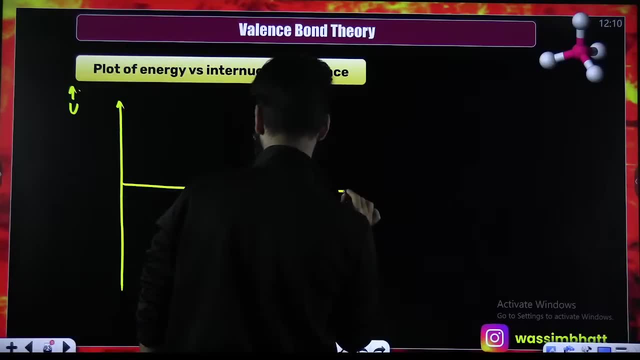 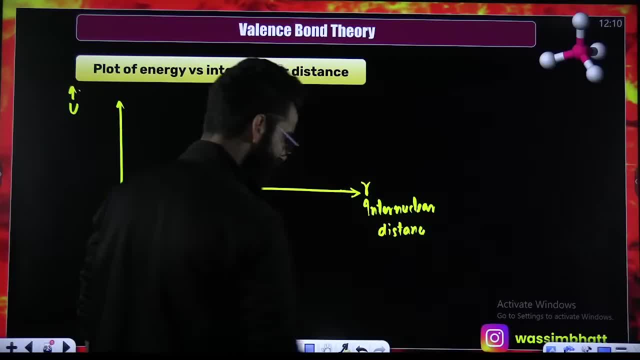 potential energy versus inter nuclear potential energy versus inter nuclear distance distance, distance. please tell me one thing. please tell me one thing. please tell me one thing. tell me one thing at this point. tell me one thing at this point. tell me one thing at this point: what are the coordinates of this point? 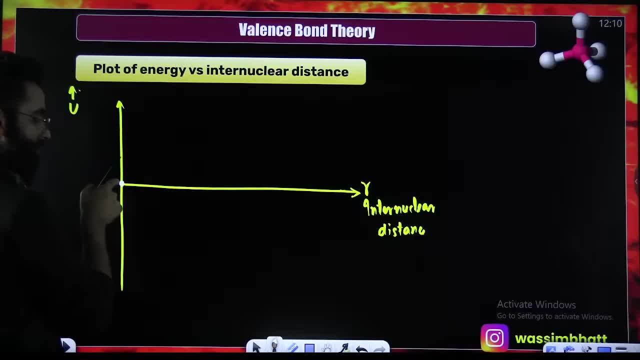 what are the coordinates of this point? what are the coordinates of this point? its origin: its coordinates are 0, 0. its origin: its coordinates are 0, 0. its origin: its coordinates are 0, 0, 0. its coordinates, its coordinates, its coordinates. so, at this point, r is zero, r is zero. 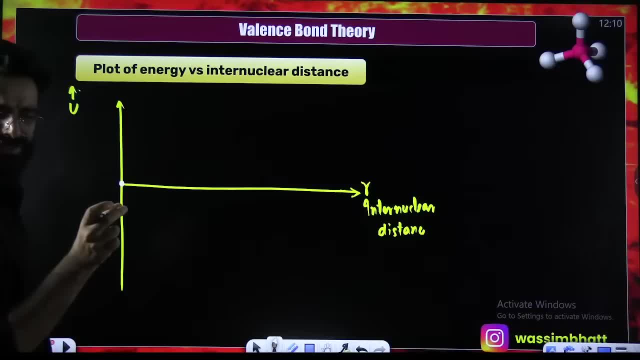 so at this point, r is zero, r is zero. so at this point r is zero, r is zero. means, means, means, means. distance between the atoms is zero. distance between the atoms is zero. distance between the atoms is zero. basically is approaching towards zero. basically is approaching towards zero. 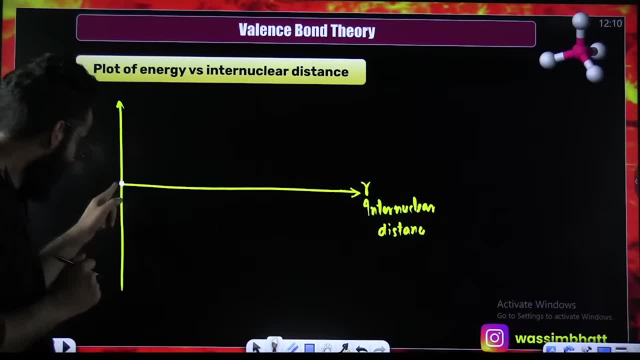 basically, is approaching towards zero. distance between the atoms is distance between the atoms is distance between the atoms is approaching towards zero right now. approaching towards zero right now. approaching towards zero right now. if you go in this direction, r is: if you go in this direction, r is: 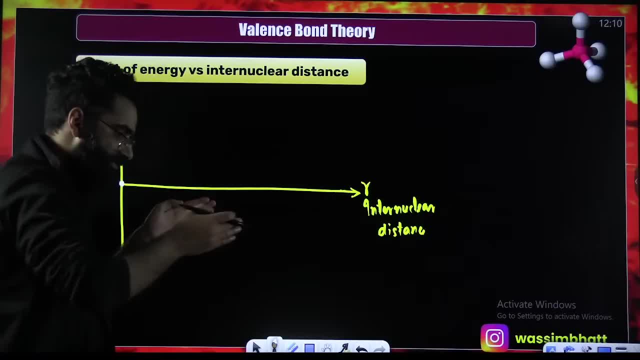 if you go in this direction, r is increasing. r is increasing. that means increasing. r is increasing. that means increasing. r is increasing. that means distance between the atoms is increasing. distance between the atoms is increasing. distance between the atoms is increasing. distance between the atom is increasing. distance between the atom is increasing. 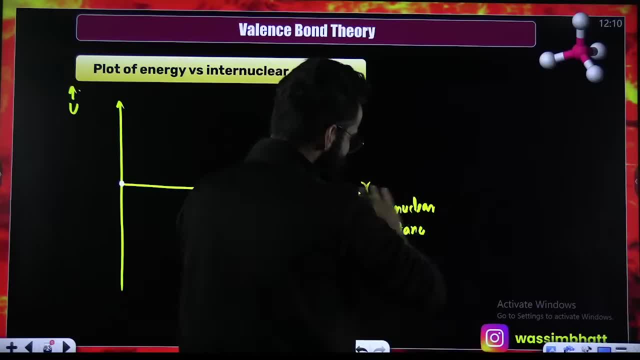 distance between the atom is increasing if you go in this direction. distance, if you go in this direction, distance, if you go in this direction, distance between the atoms is increasing. let me say between the atoms is increasing. let me say between the atoms is increasing. let me say somewhere, somewhere, when r tends to: 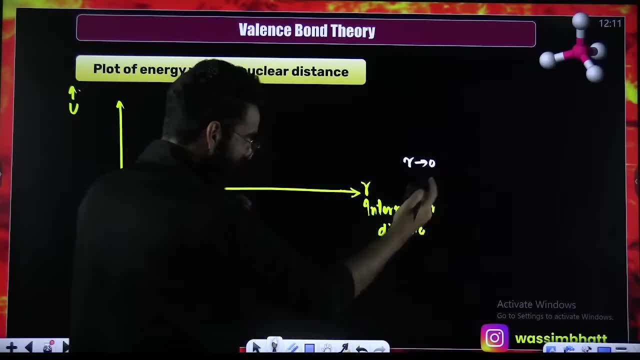 somewhere, somewhere, when r tends to somewhere, somewhere, somewhere, when r tends to infinity, when the distance between infinity, when the distance between infinity, when the distance between the atoms will be infinity, at that point the atoms will be infinity. at that point the atoms will be infinity. at that point of time, force of attraction between the. 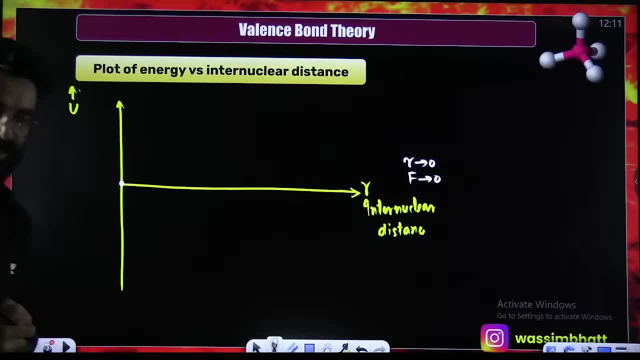 of time, force of attraction between the of time, force of attraction between the atoms will be zero. atoms will be zero. atoms will be zero. right at that time, force of attraction, right at that time, force of attraction, right at that time, force of attraction between the atoms will be zero. you know. 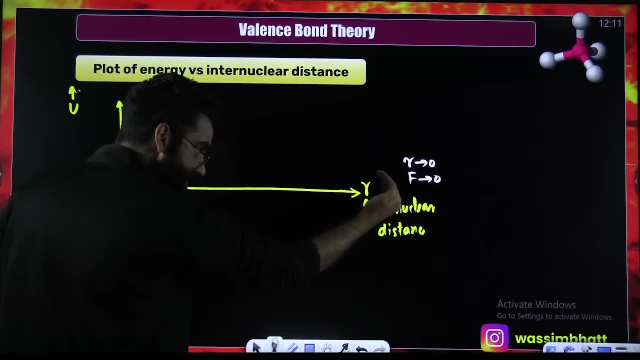 between the atoms will be zero. you know between the atoms will be zero. you know it perfect somewhere here now. if you go it perfect somewhere here now, if you go it perfect somewhere here now, if you go opposite, if you go in this direction, r opposite. if you go in this direction, r. 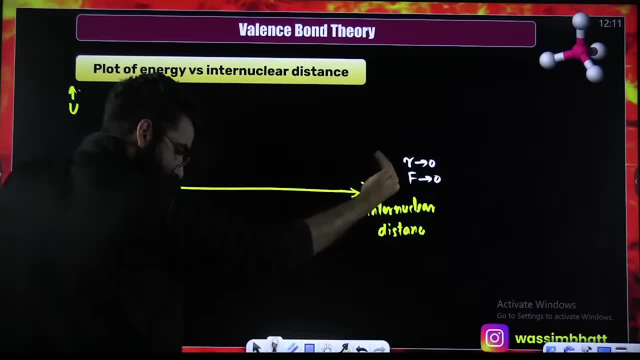 opposite. if you go in this direction: r is decreasing. r is decreasing. atoms are is decreasing. r is decreasing. r is decreasing. atoms are is decreasing. r is decreasing. r is decreasing. atoms are coming closer. r is decreasing- coming closer. r is decreasing. atoms are coming closer. r is decreasing. 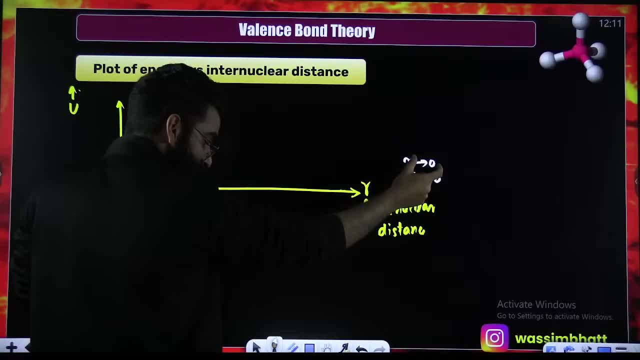 coming closer. r is decreasing. atoms are. was i mean initially, the atoms were at. was i mean initially the atoms were at. was i mean initially the atoms were at infinite distance apart. now you are infinite distance apart now you are infinite distance apart. now you are moving in this direction. r is decreasing. 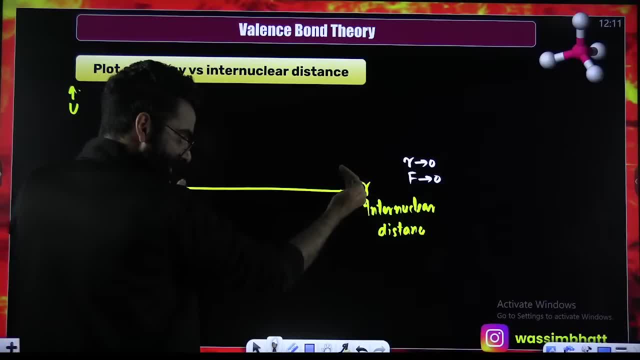 moving in this direction: r is decreasing. moving in this direction: r is decreasing. r is decreasing. atoms are coming closer. r is decreasing. atoms are coming closer. r is decreasing. atoms are coming closer. if the atoms are coming closer. force of: if the atoms are coming closer. force of. 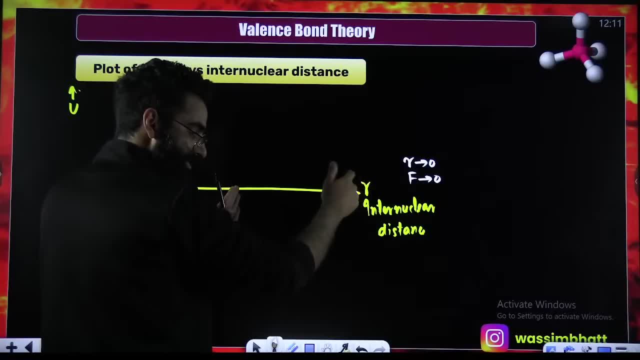 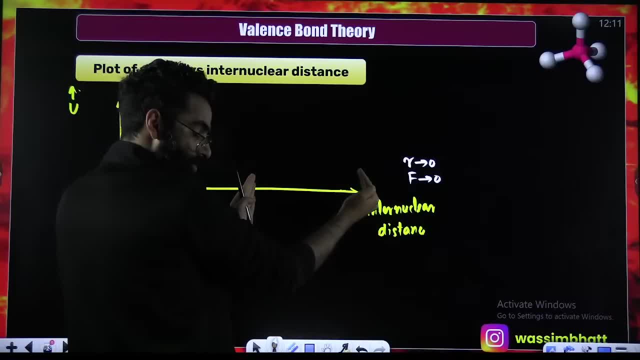 attraction is increasing. due to attractions, energy is released. energy is released due to attractions energy: attractions: energy is released. energy is released due to attractions energy. attractions: energy is released. energy is released due to attractions: energy is released, so is released, so is released, so so continuously energy is being released. 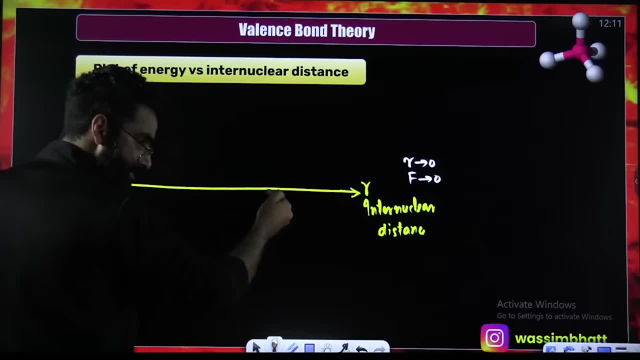 so continuously energy is being released, so continuously energy is being released, continuously energy is being released. if continuously energy is being released, if continuously energy is being released, if, when atoms are coming closer continuously, when atoms are coming closer continuously, when atoms are coming closer continuously, energy is being released, so energy 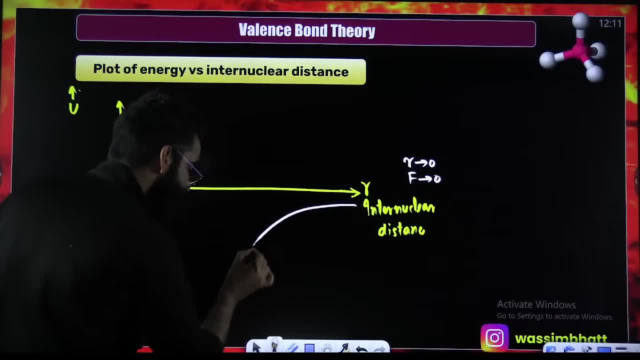 energy is being released, so energy. energy is being released, so energy within the system that is decreasing with within the system that is decreasing with within the system that is decreasing with time, time, time. energy within the system. that is energy within the system. that is energy within the system that is decreasing with time. 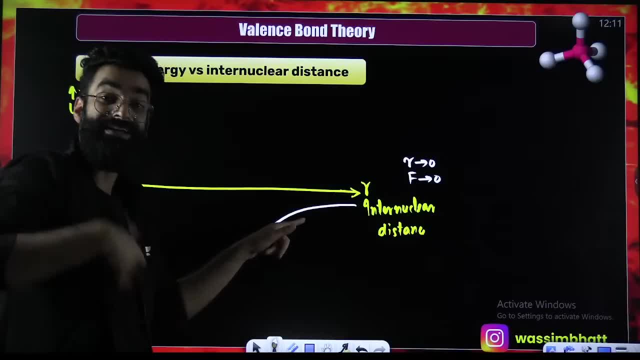 decreasing with time. decreasing with time. right energy within the system that is right. energy within the system that is right. energy within the system that is decreasing with time and stability is decreasing with time and stability is decreasing with time and stability is increasing with time. energy within the. 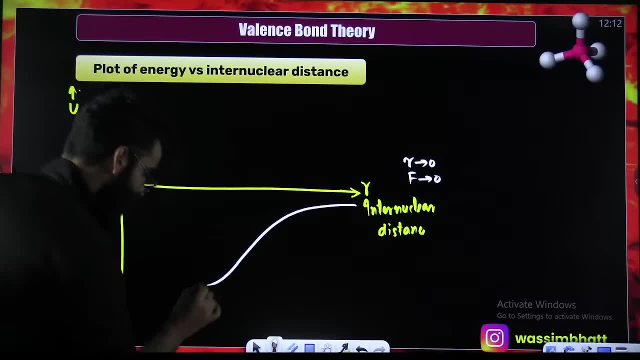 increasing with time energy within the increasing with time energy within the system that is decreasing with time system that is decreasing with time system that is decreasing with time. stability is increasing. this is the point. stability is increasing. this is the point. stability is increasing. this is the point. this is the point. this is the point, this. 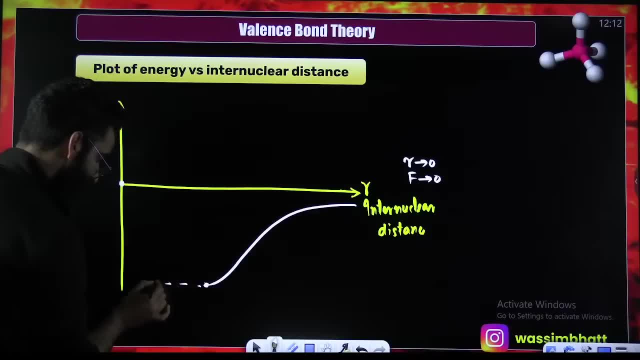 this is the point, this is the point. this, this is the point. this is the point. this is the point at which is the point at which is the point at which energy of the system is minimum. this is energy of the system is minimum. this is energy of the system is minimum. this is the point at which energy of the system 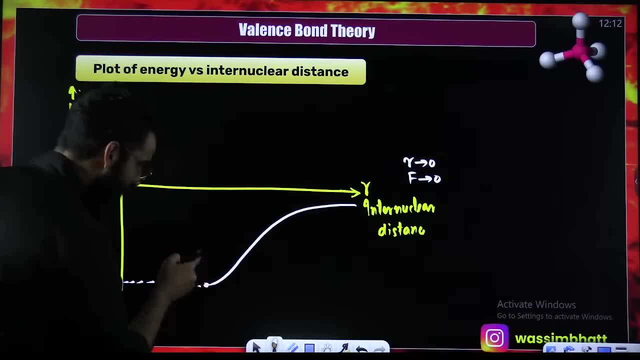 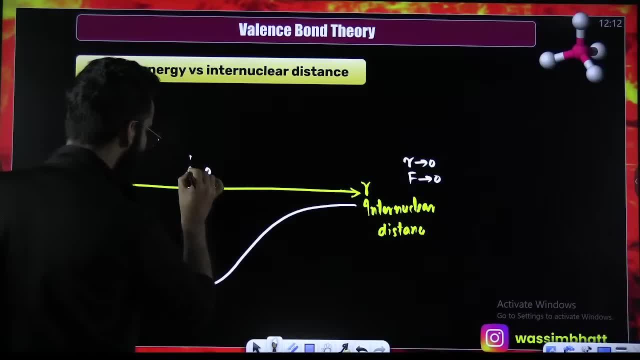 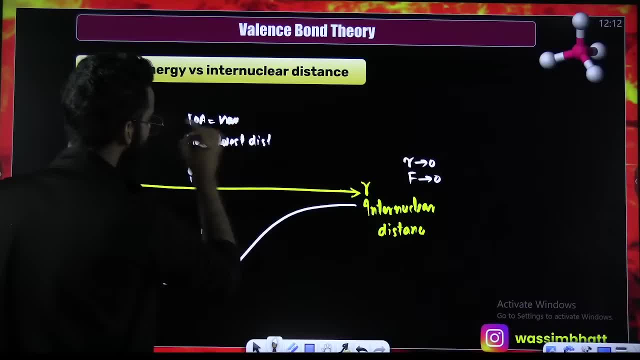 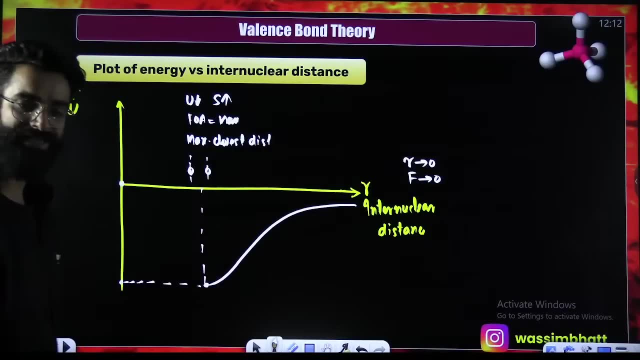 atoms are at maximum closest distance. so i would say force of attraction between the force of attraction between the force of attraction between the atoms is maximum. atoms is maximum. atoms is maximum right. potential energy of the system is right. potential energy of the system is minimum. stability is maximum, perfect. now guys understand, understand. 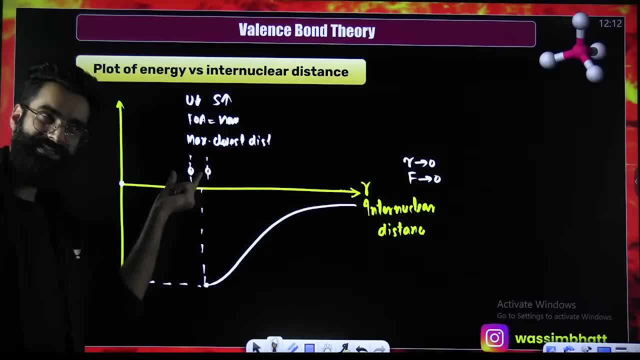 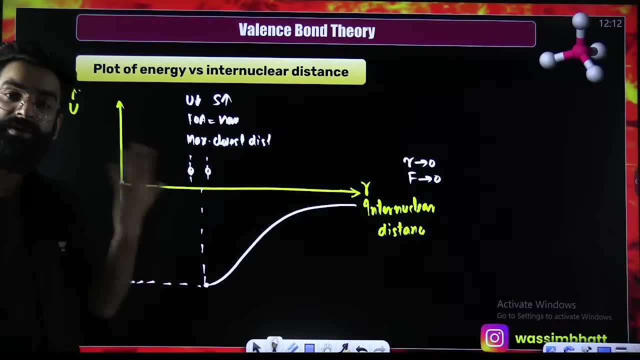 atoms are right now at maximum closest distance. if you want these atoms to come little more closer, what will happen? repulsions arise, repulsion will start and repulsions they will try to do the repulsions. energy of the system will increase, stability will decrease, energy of the system now will increase and 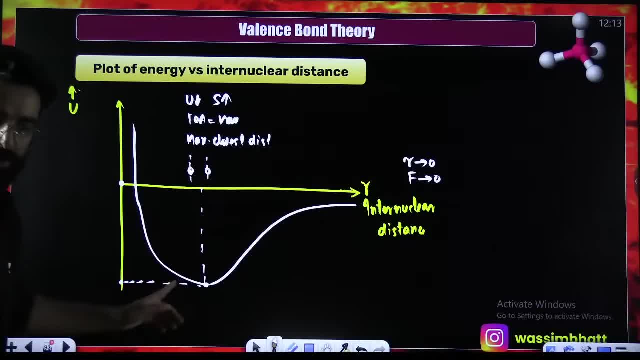 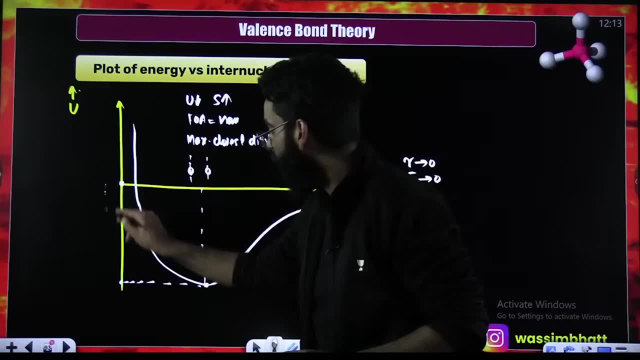 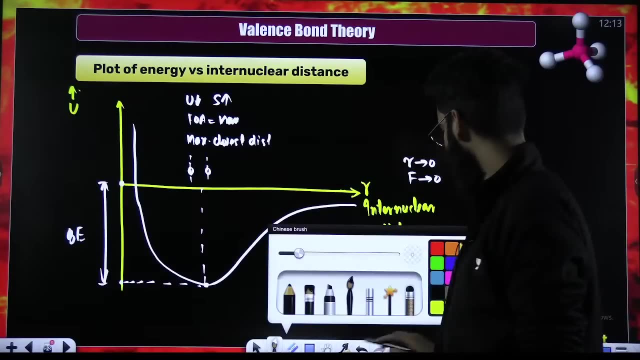 stability will decrease. perfect. so this is the graph. I hope you got to know how this graph is made. I hope you got to know how this graph is made. perfect, right from here to here. you'll be calling this as bond energy of the molecule. right, you will be calling this as bond energy of the molecule and this. 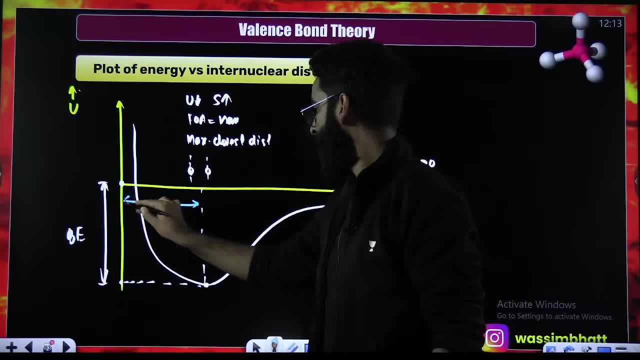 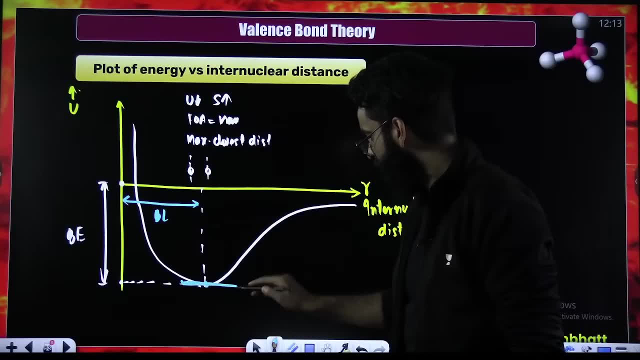 particular distance over here. you'll be calling as bond length. you'll be calling: this is bond length and at this particular point. one more thing: if you draw the tangent at this particular point, slope of that tangent will be 0. so that means EU upon dr at this particular point is equal to 0, is. 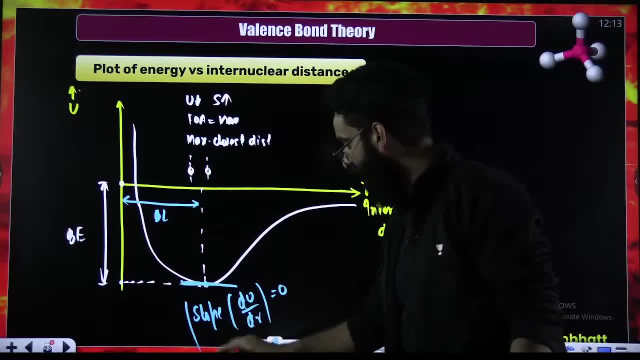 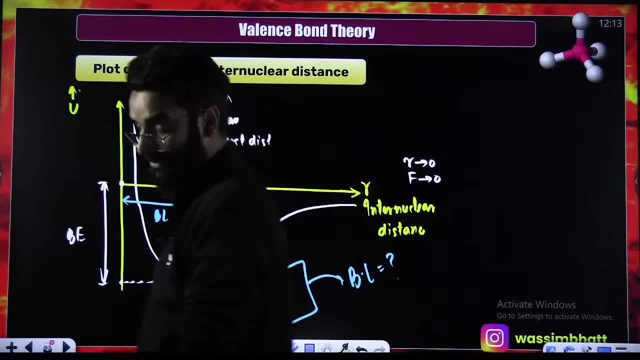 equal to 0, 0. right, so, pop, this is the criteria which I use in order to calculate the bond length. how exactly? this is the criteria which I use in order to calculate the bond length. how exactly? for that, I've got equation for you. let's. 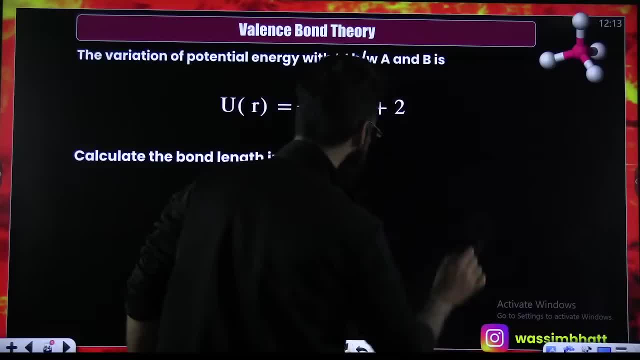 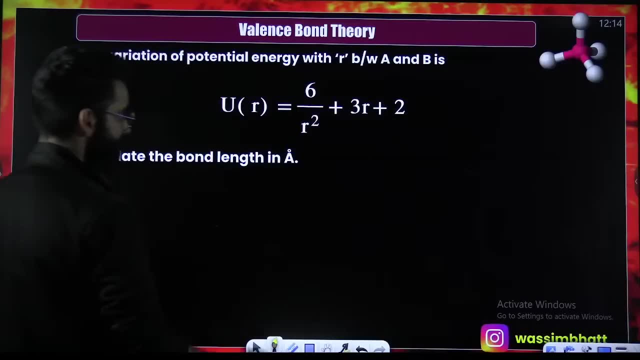 try to solve. see, guys, as per the question is concerned, you are given with the with, with some variation of potential energy. with R between two atoms, U is equal to 6 by R means 6 R raised power minus 2 plus 3, R plus 2. 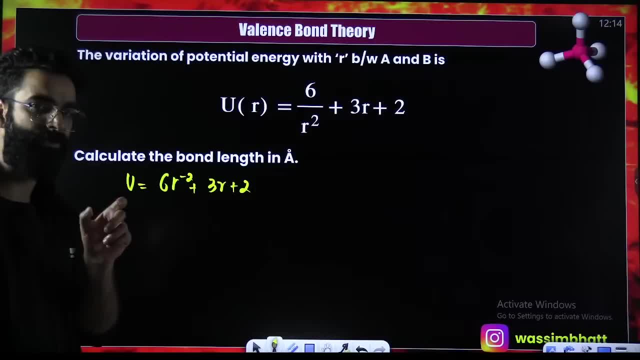 right: variation of potential energy with inter nuclear distance. calculate the bond length. in order to calculate the bond length, what is the criteria we use? du by dr has to be 0. du by dr has to be 0. right du by dr has to be 0. so differentiate, differentiate this U with. 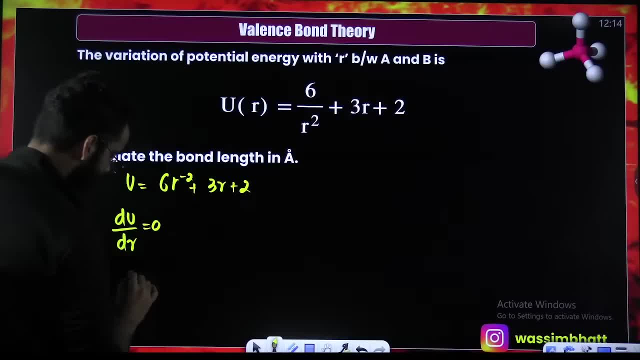 respect to R. differentiate with you. differentiate this U. you differentiate this U with respect to R. differentiate this U with respect to R. with respect to R. so du by dr will be equal. this is 6. I'm writing as such. with respect to R. so du by dr will be equal. this is 6. I'm writing as such. 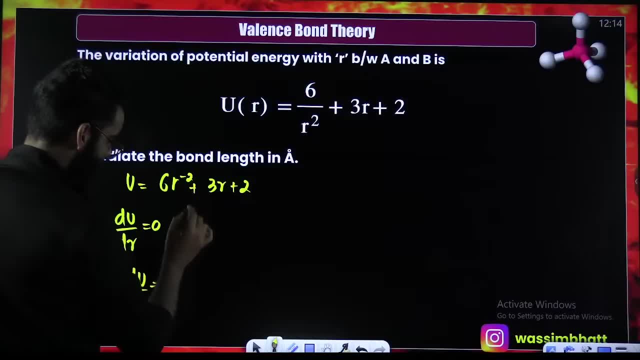 right X. raise power, n, which means N, X and minus 1, so 6, twos are 12, it's gonna be 12 R raised power minus 3. perfect difference, you know. 3 R is nothing but R. perfect, this constant is 0 and this term has to be 0, right? so I'll. 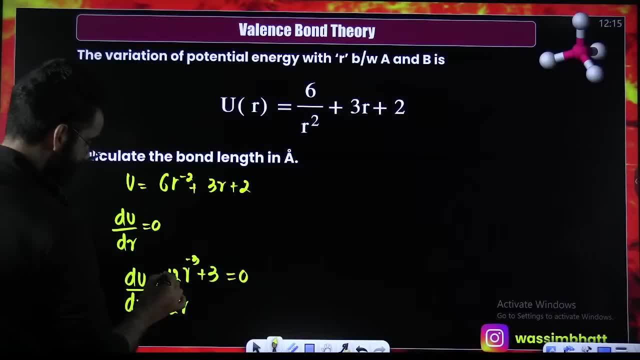 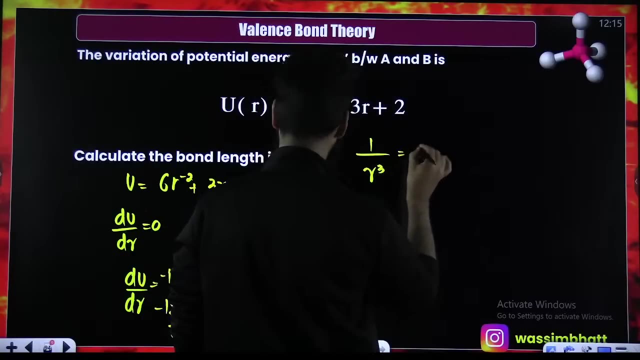 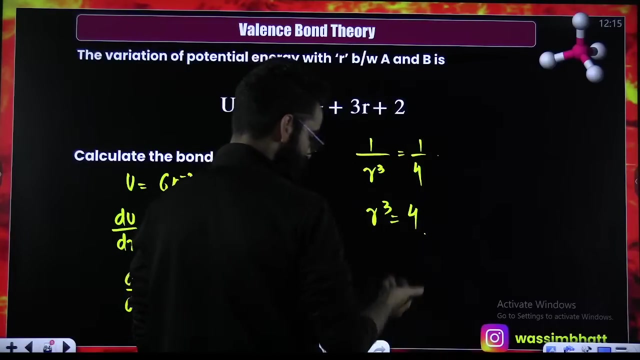 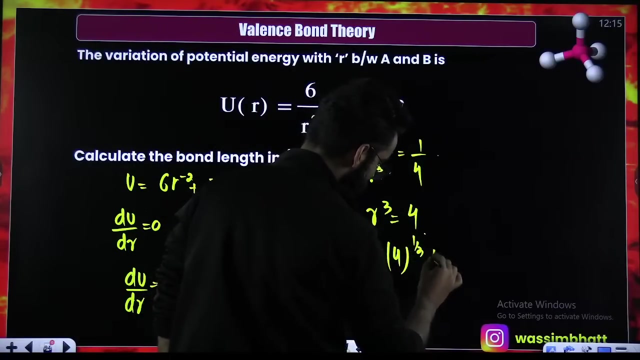 say 12, this minus 12, sorry, so minus 12. R raised power minus 3 is equal to minus 3, right? so R raised power minus 3 is equal to 1 by 4. R raised power minus 3 is equal to 1 by 4. what does that mean? that means 1 divided by R raised power 3 is equal to 1 by 4. so R raised power 3 is equal to 4, if I, if I, if I right, if I take cube root on both the sides, this is going to be: R is equal to 4 raised power 1 by 3, and the answer is going to be in Engstrom's. am I clear? so one criteria I used is that if I take cube root on both the sides, this is going to be: R is equal to 4 raised power 1 by 3, and the answer is going to be in Engstrom's. am I clear? so one criteria I used is that if I take cube root on both the sides, this is going to be: R is equal to 4 raised power 1 by 3, and the answer is going to be in Engstrom's. am I clear? so one criteria I used is that if I take cube root on both the sides, this is going to be: R is equal to 4 raised power 1 by 3 and the answer. 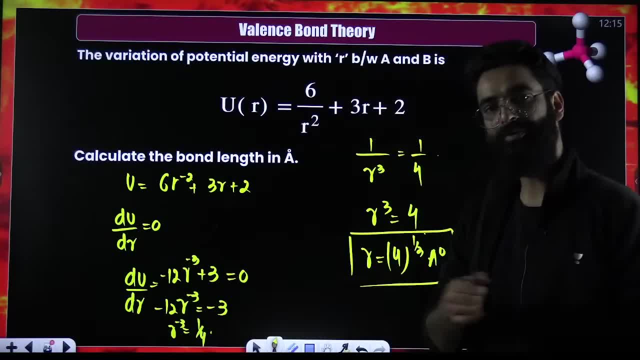 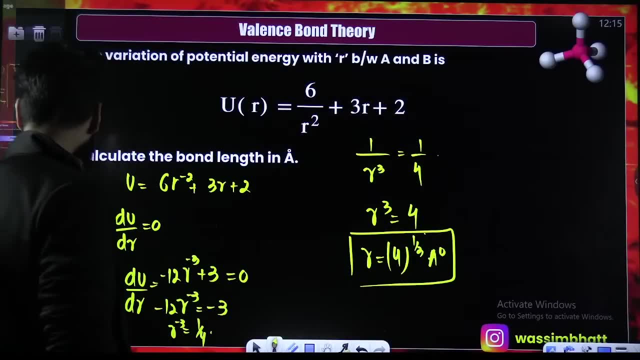 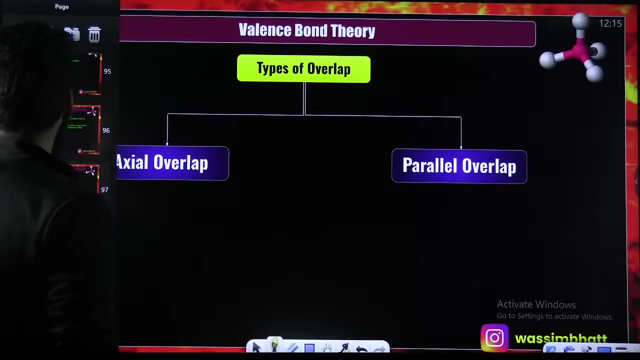 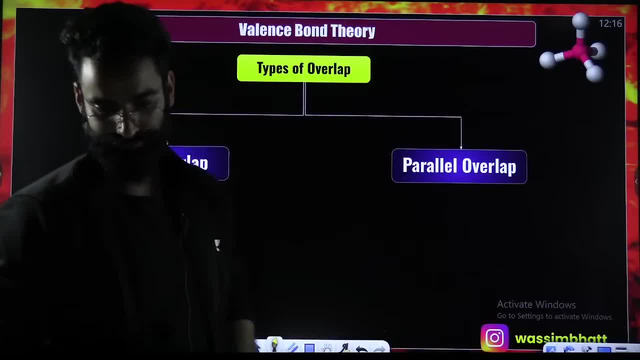 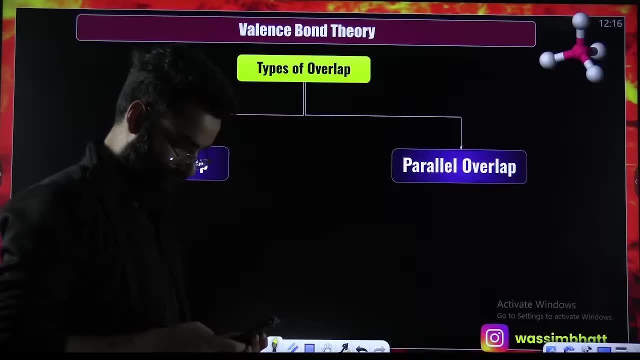 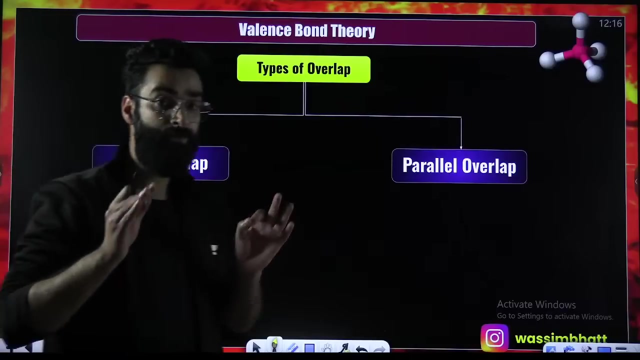 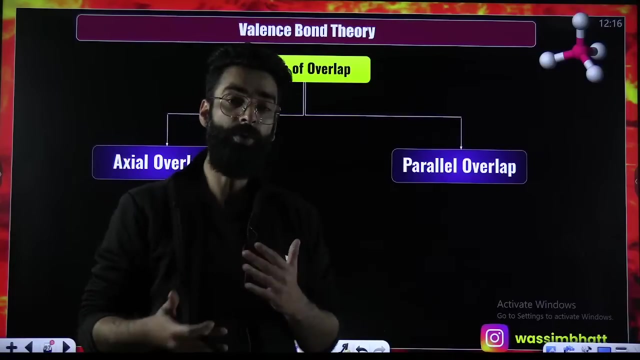 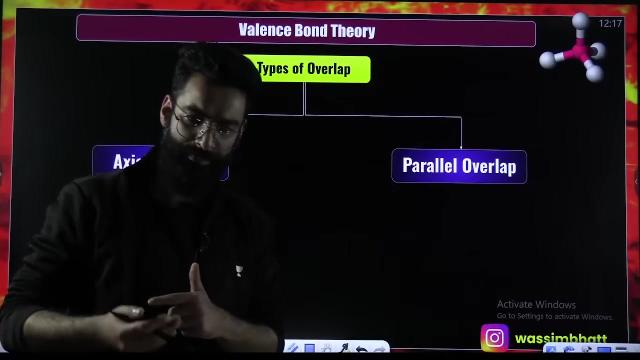 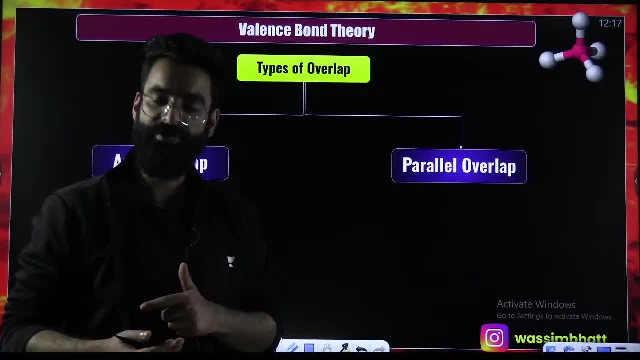 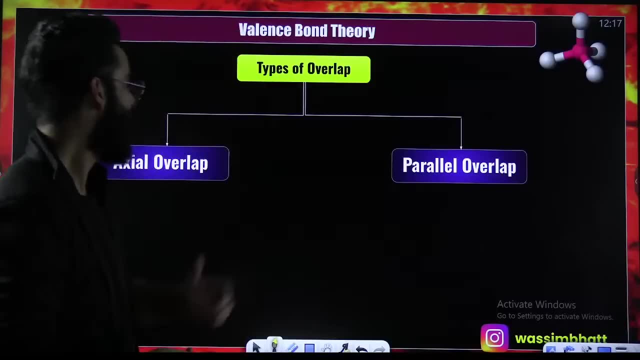 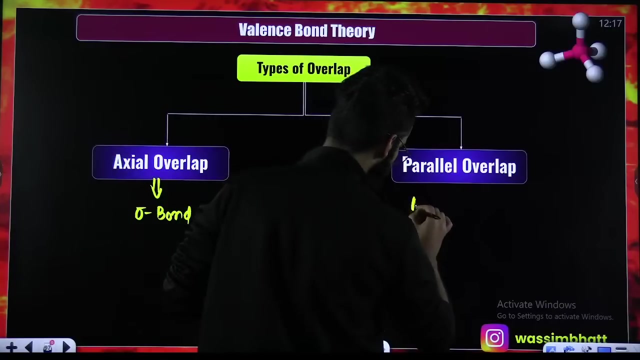 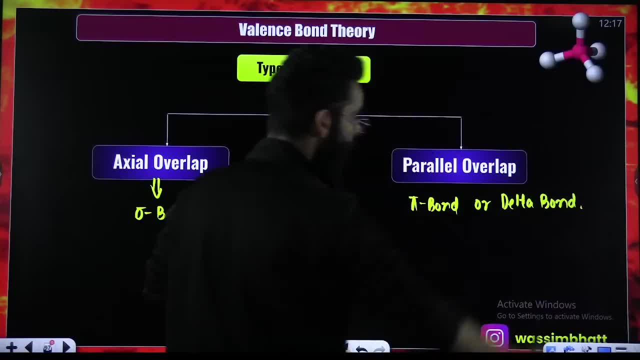 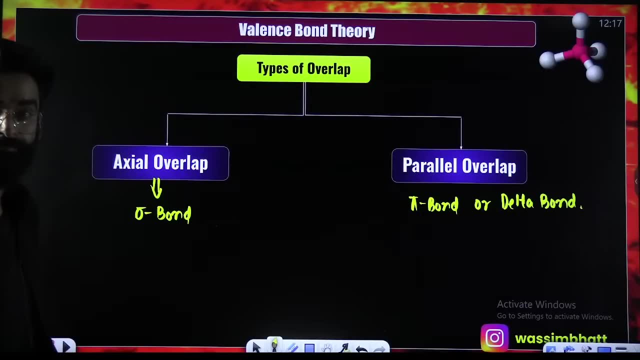 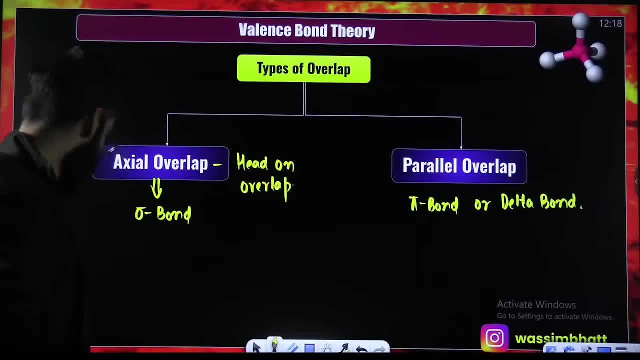 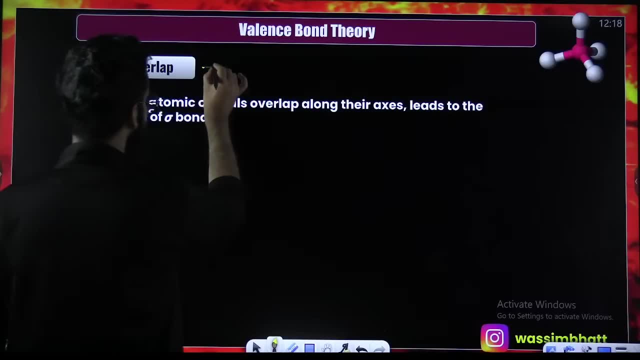 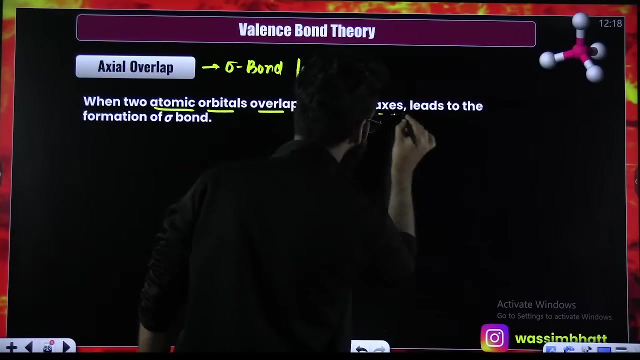 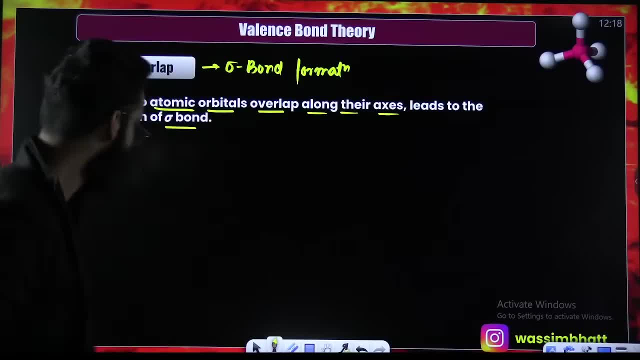 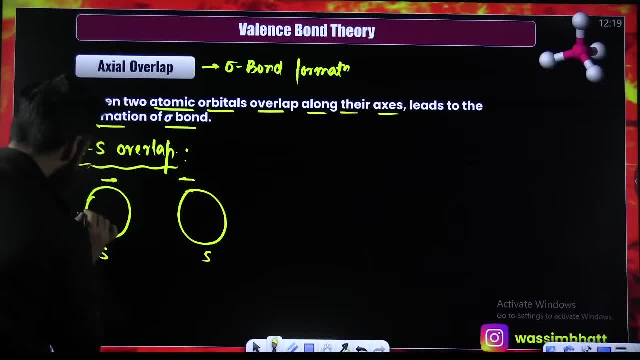 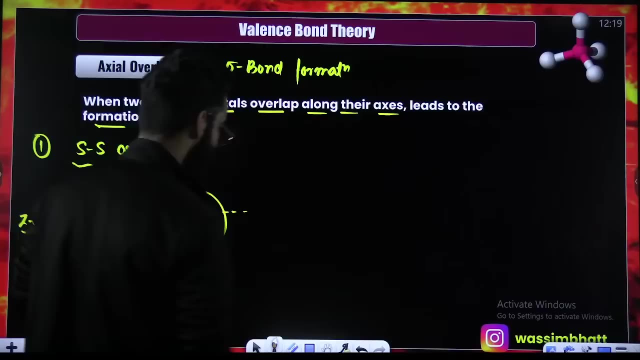 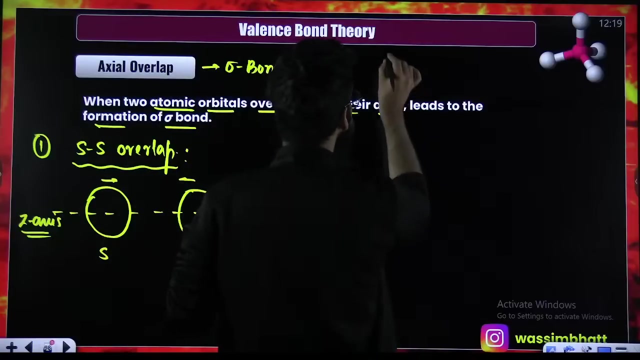 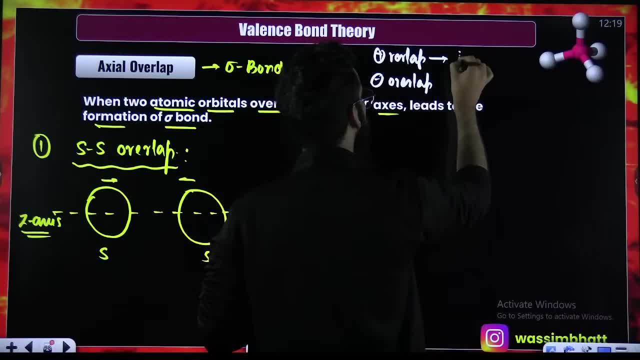 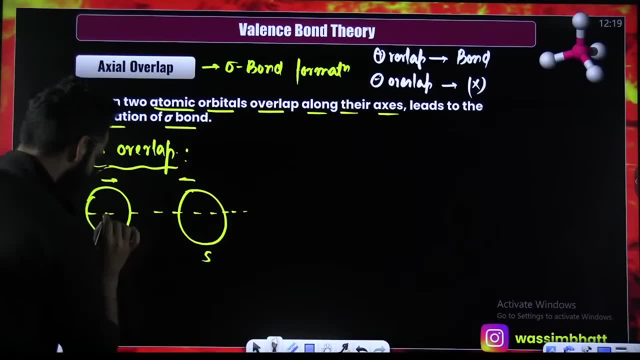 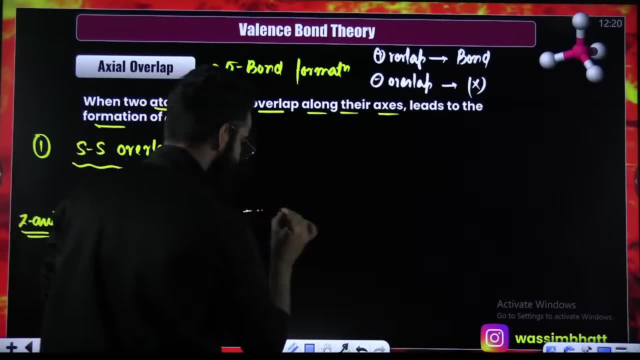 side right. Same sign, same side. So this is the example of what It is going to be, the example of positive overlap, or you call this as in-phase overlap. You call this as in-phase overlap, You call this as in-phase overlap. Now, what's going to happen? They? 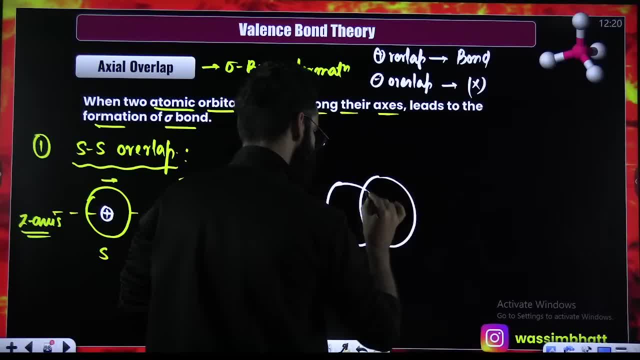 are going to merge into each other. They are going to merge into each other. They are going to merge into each other. right, They are going to merge into each other. What is this called Overlapping? Due to overlapping what happened? Due to overlapping due to. 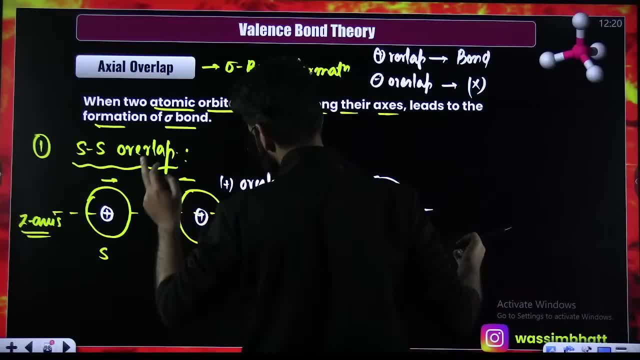 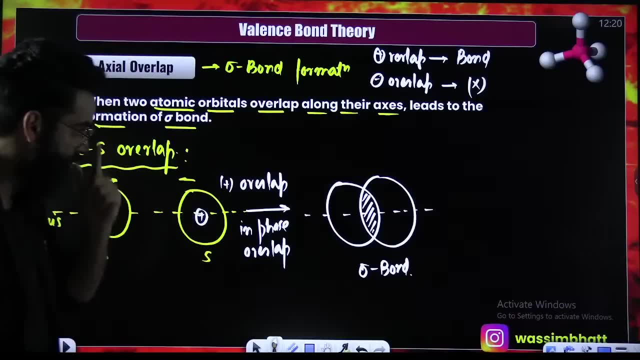 overlapping, covalent bond gets formed. Now, which overlapping this is. This is your actual overlapping. So which bond got formed? It is the sigma bond which got formed. It is the sigma bond which got formed. Okay, It is the sigma bond which got formed here, Perfect. 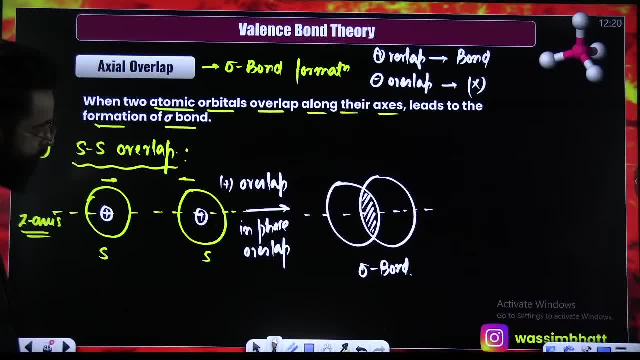 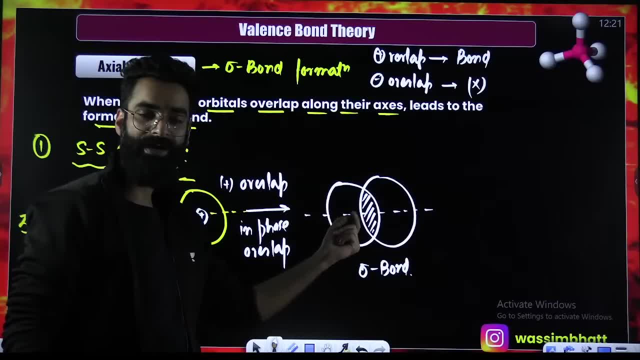 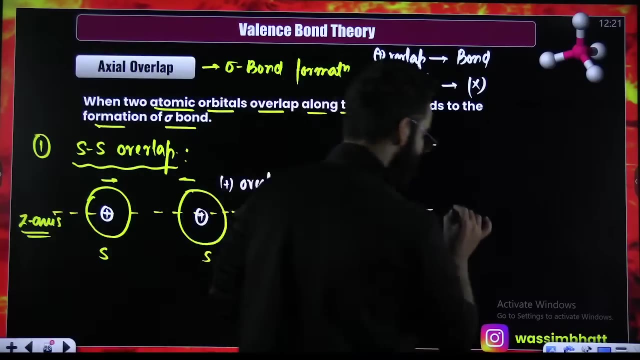 It is the sigma bond which got formed over here, Right people. Now, once this overlapping is done, once this overlapping is done, this electron cloud, it will arrange itself in such a way that it comes under the influence of both these, both the nuclei. 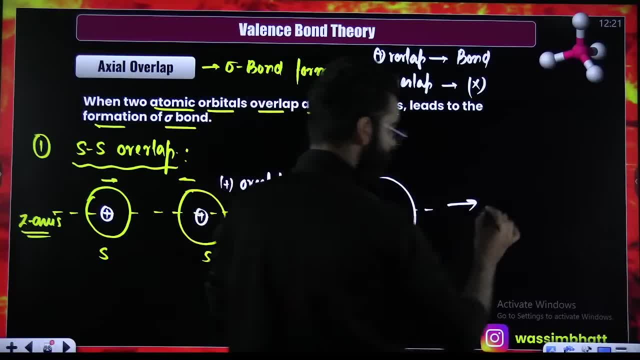 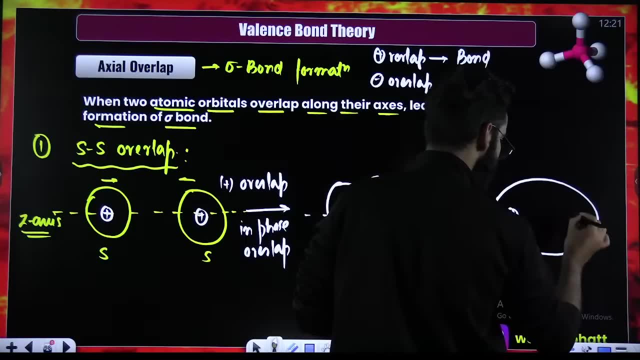 At the end what happens? The electron cloud, it arranges itself in such a way that it comes under the influence of both the nuclei. Let's say this is nucleus of one atom. Let's say this was nucleus of one atom and this is the electron density which has come and gone. 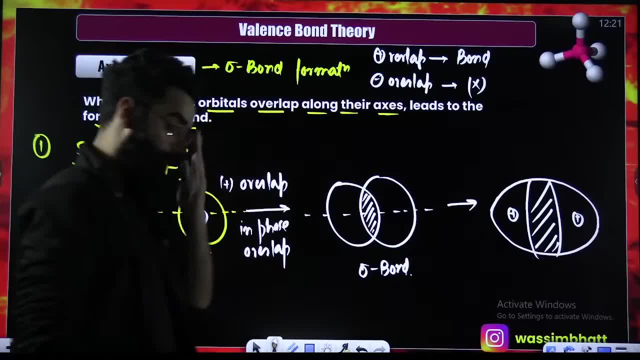 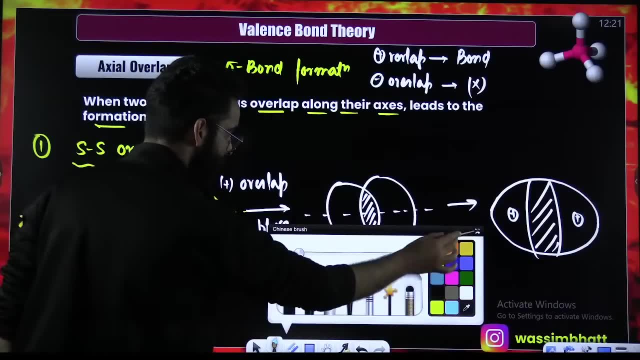 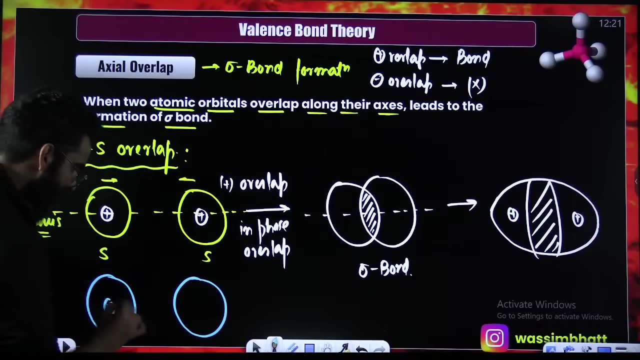 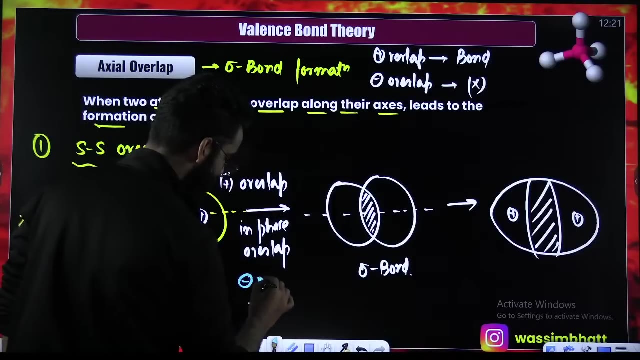 And this is nucleus of one atom. and this is nucleus of one atom. You do not choose a nucleus, so you choose a specjal gradient which will match the zero truth value of zero as the sı over Mic hotter wavelength. Okay, you will see the. 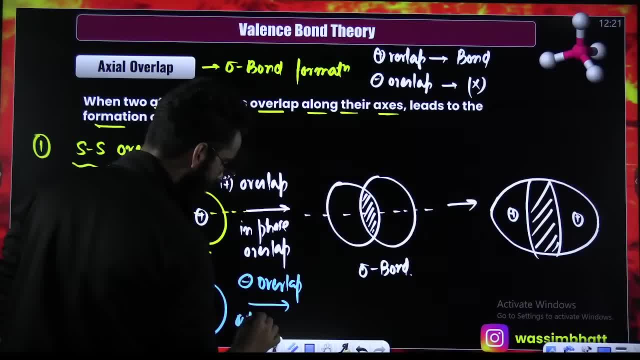 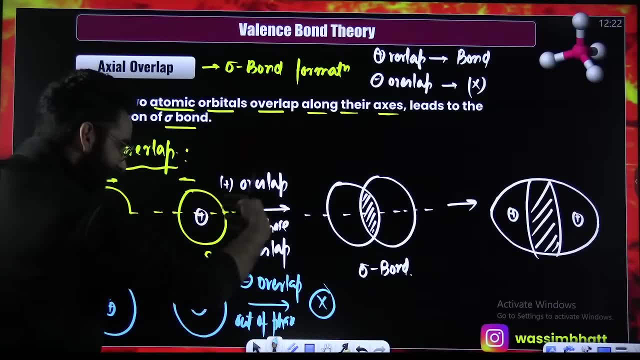 е units are butterflies. The nucleus of one atom is called node-1.. That's theẫn loved one. We'll be calling this as out-of-phase overlap, which does not lead to the formation of any bond. Okay, was this overlap? head-on overlap. 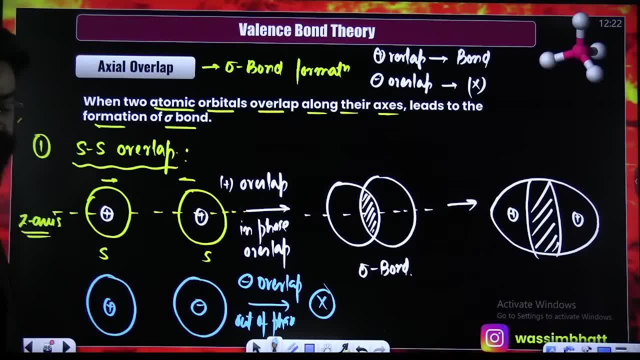 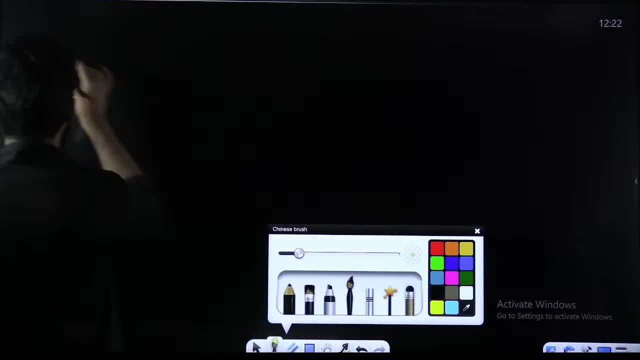 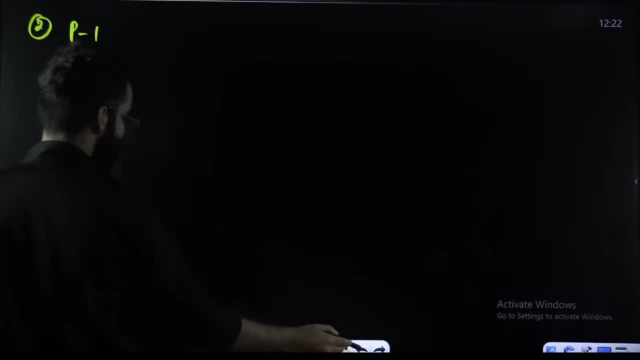 Yes, this was head-on overlap. So this was the first example of here. This was the first example of here. Axial overlapping right. First example. Second example of the axial overlapping. Second example of the axial overlapping: SP overlap. 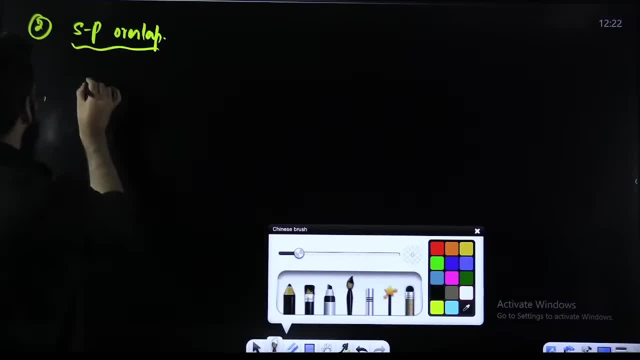 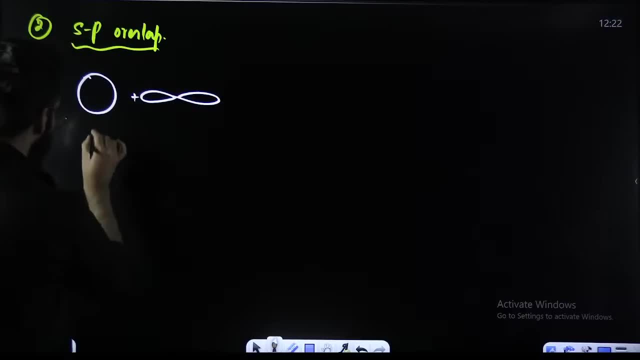 SP overlap- SP overlap. This is the S orbital, for example, And this is the P orbital: S orbital, P orbital. S orbital, P orbital. Okay, S orbital, P orbital. Is this again going to be head-on overlap? 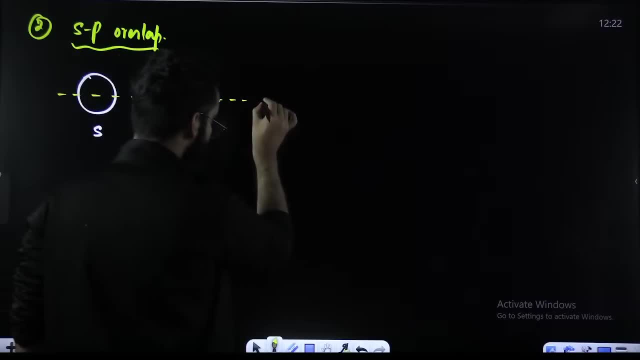 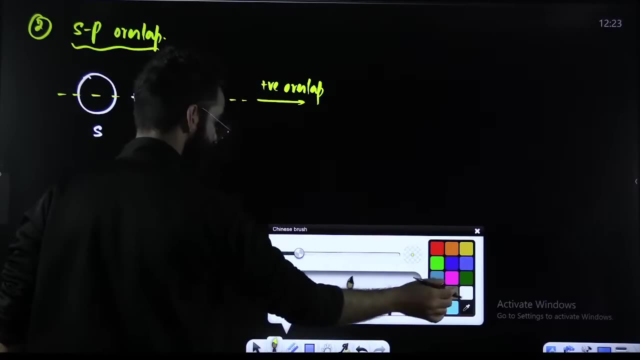 Yes, this is going to be the head-on overlap, Right. Let's say: I'm showing now the positive overlap here, I'm showing the in-phase overlap here. How do I show it? How do I show it Understand If let's say this is positive? 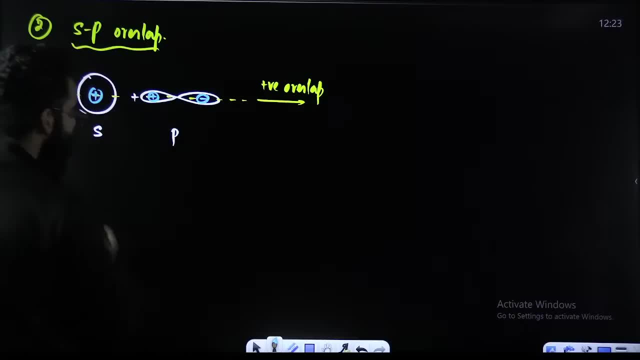 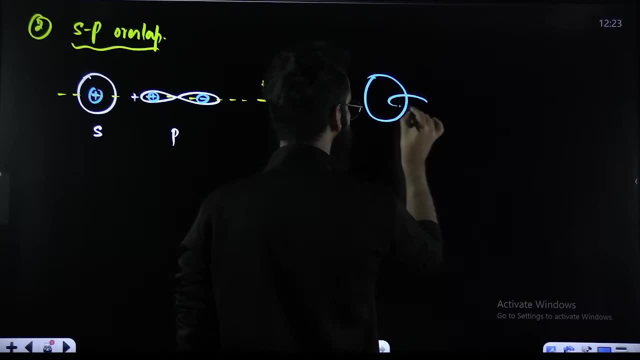 then this has to be positive, This has to be negative. Same sign on same side. It's going to be positive overlap, It's going to be positive overlap, Right? So this one of the atom, and this is one more. 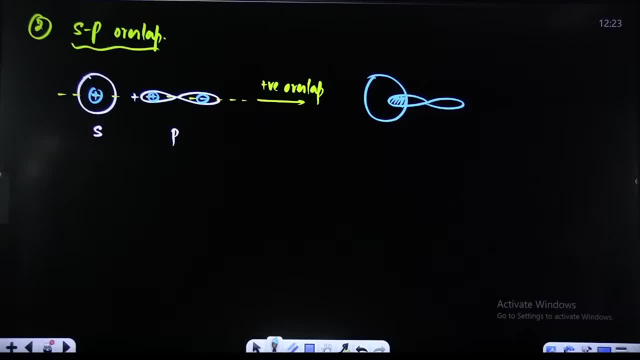 And this is the common electron cloud over here: Perfect. I believe I'm clear till here. I believe I'm clear till here. So this was your SP overlap: positive- Perfect. If you want to have a look on the negative overlap as well. 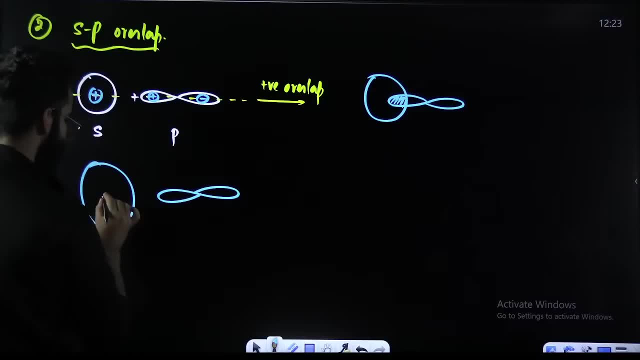 so this is: let's make this S, let's make this as P. If this is positive, call this as negative. This positive Right Opposite sign on same side. Opposite sign on same side. Opposite sign, same side means negative overlap. 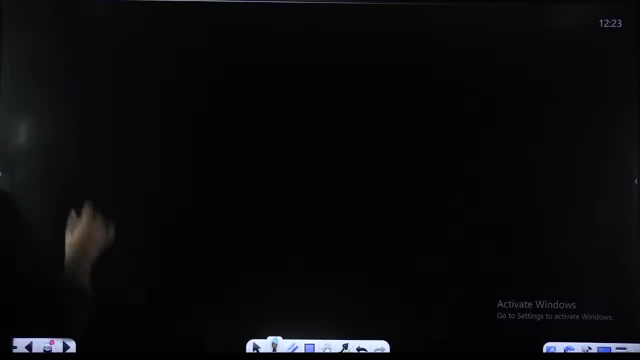 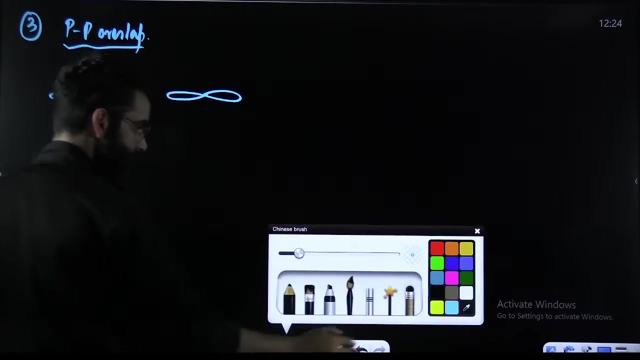 Perfect. So this was your SP overlap. Now, the third in actual overlapping is your PP overlap. It is your PP overlapping, Right. So this is one of the P orbital. This is one more P orbital, Right, Perfect. 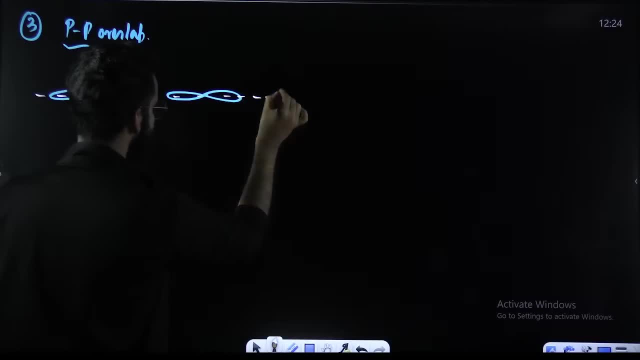 And this is your inter-nuclear axes. This is your inter-nuclear axes, Right? Let's call this positive. Let's call this negative. Let's call this positive, Let's call this negative. Same sign, same side. Same sign, same side. 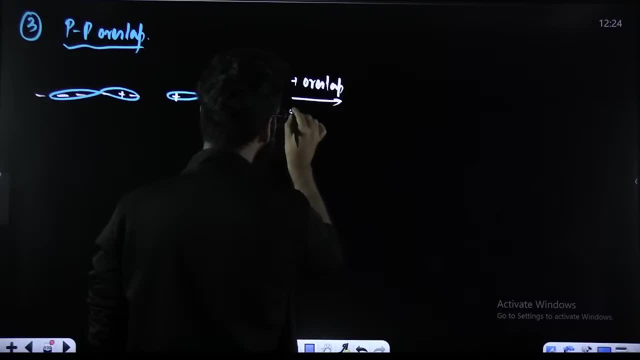 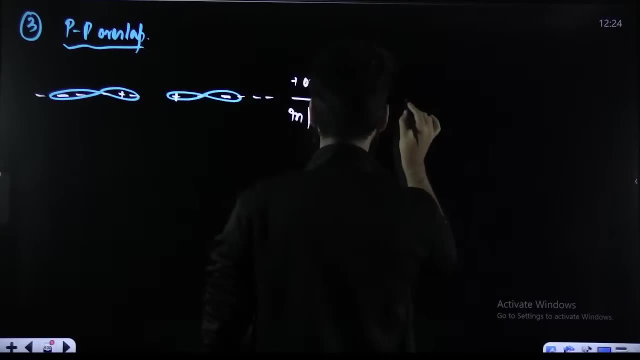 Positive overlap, Positive overlap, In-phase overlap- Positive overlap, In-phase overlap. Right, So it is again the head-on overlap. It will lead to the formation of a sigma bond. Finally, you are going to represent it like this: 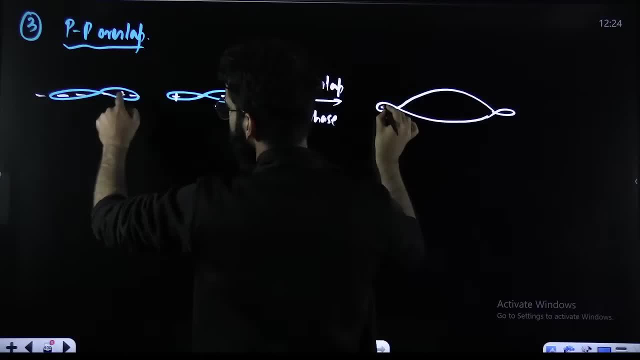 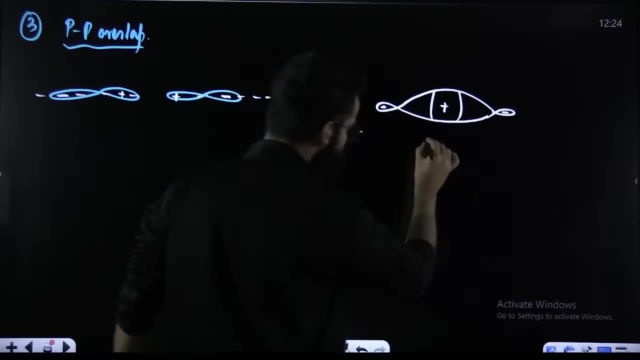 Right, If this is negative, this part is negative. Right, This is positive, positive. So here you will write positive And here you will write negative Again, head-on overlap. So which bond has formed over here? 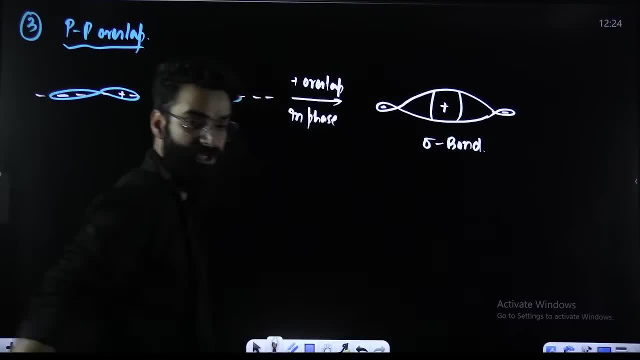 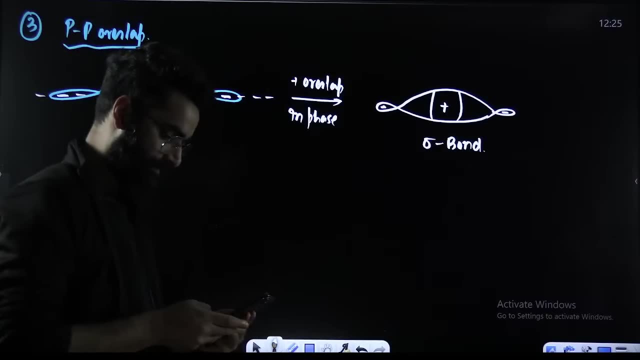 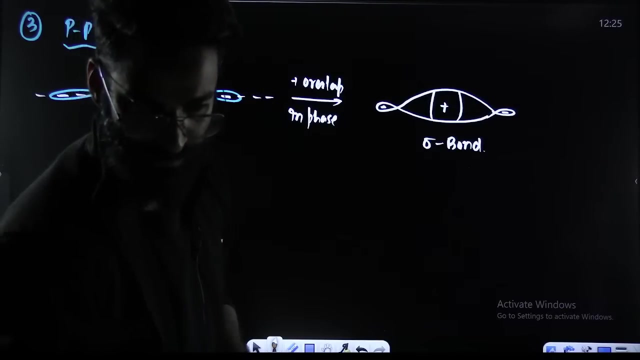 It is a sigma bond which has got formed over here. So in case of actual overlapping, what happens? Overlapping happens head-on. There is head-on overlapping basis, Okay, There is head-on overlapping. basically, Just a second, guys, Just give me a second. 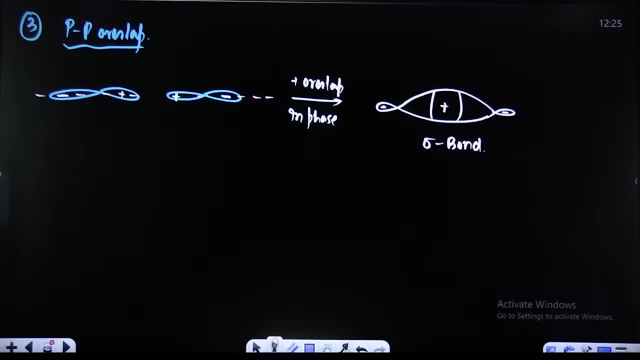 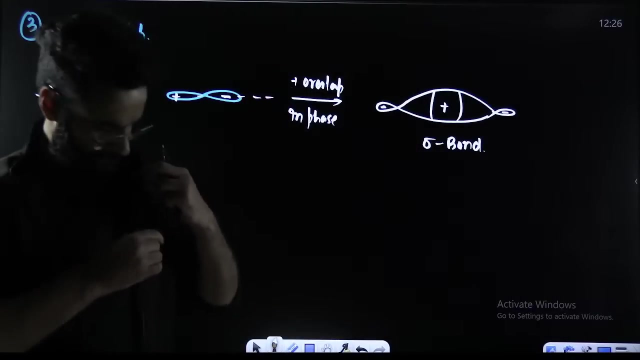 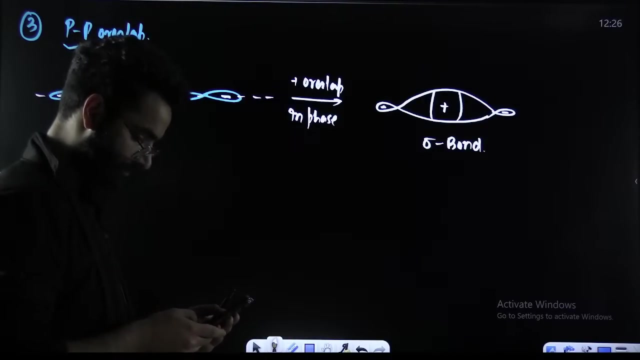 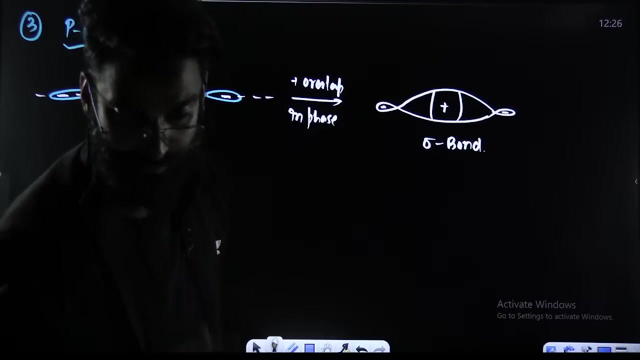 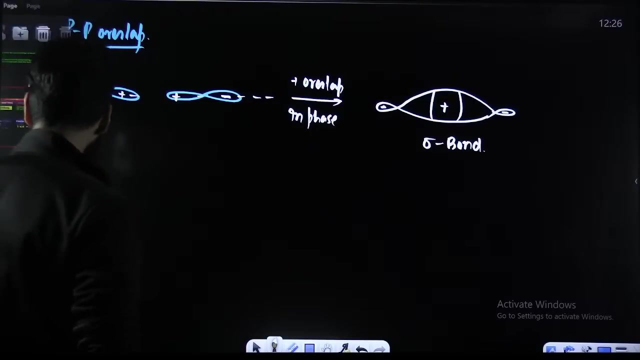 Thank you. Okay, so, guys, is the actual overlapping clear to everyone? is the actual overlapping clear? actual overlapping leads to the formation of what it leads, the formation of your Sigma bond. right Now, I'm going to move on to the parallelism, Parallel overlapping. I am going to move on to the parallel overlapping. 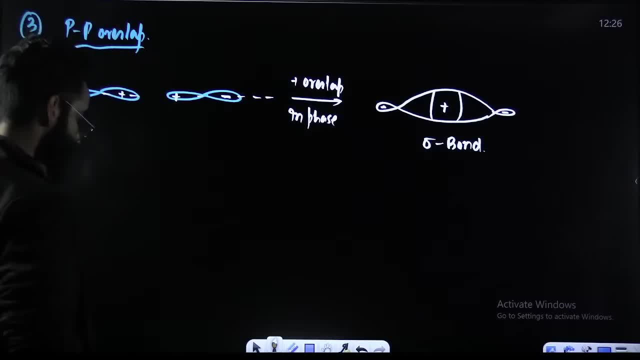 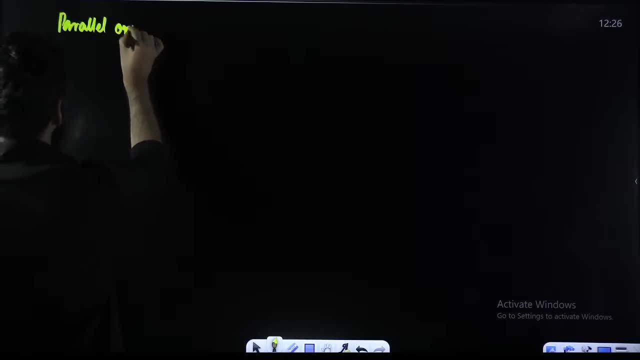 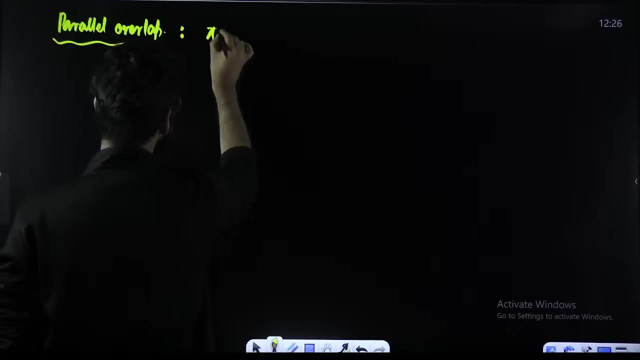 I'm going to move on to the parallel overlap. Parallel overlap, Parallel overlap. What happens in parallel overlap? which bond gets formed? it is the pi bond which gets formed or delta bond. leave delta bond aside. that's not in your syllabus, right? 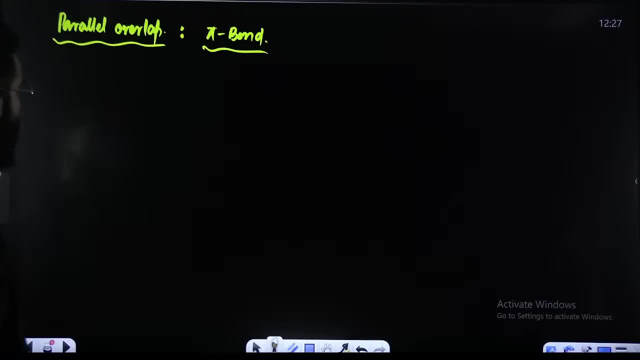 I'm just talking about the pi bond form. I'm just talking about the pi bond formation to parallel overlap, and I'll just show the positive overlap. now, right, It is just, I wanted to show you how to identify whether the overlap is positive or negative. 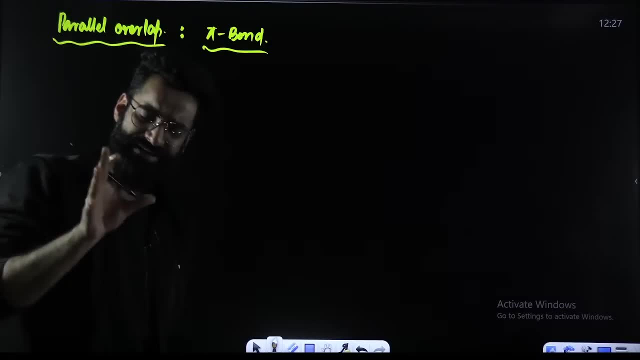 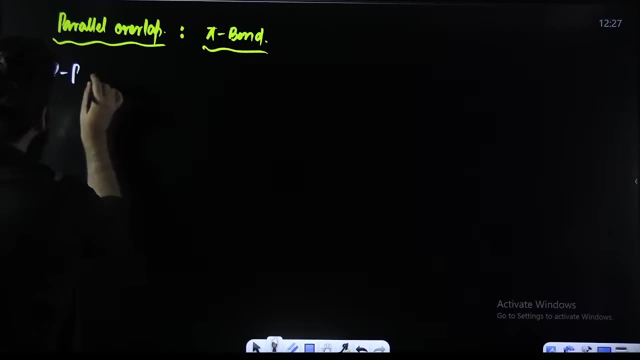 Same sign: same side means positive overlap. Opposite sign: same side means negative overlap. That's all right. Okay, let's say I'm first of all showing you the PP parallel overlap. PP parallel overlap, Let's say this is one of your P orbital. 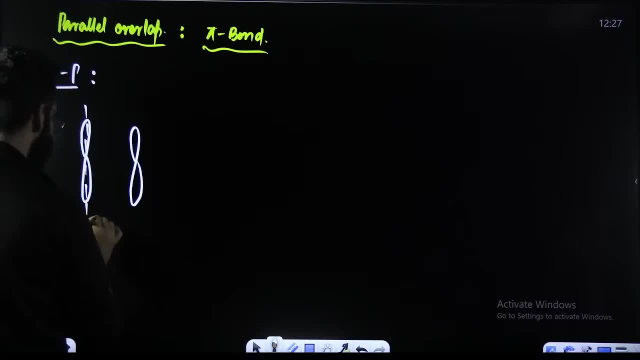 This is one of your P orbital, And they are going to have their x-axis. They are going to have their x-axis parallel. They are going to have their x-axis parallel. Okay, They are going to have their x-axis parallel. Now they are going to overlap in this way, keeping their x-axis parallel. 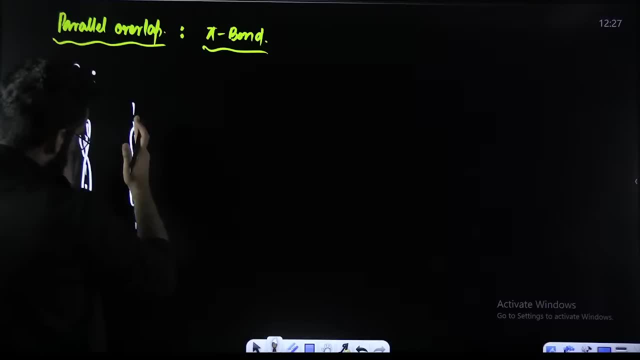 What is going to happen? What is going to happen? What's going to happen. Let me give the signs as well. Let's say this is positive. Okay. let's say this is negative. Let's say this is positive, This is negative. 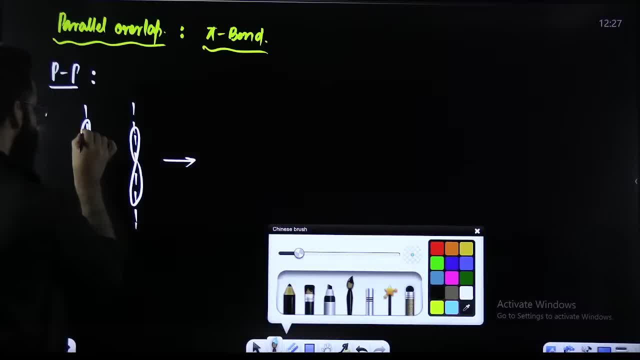 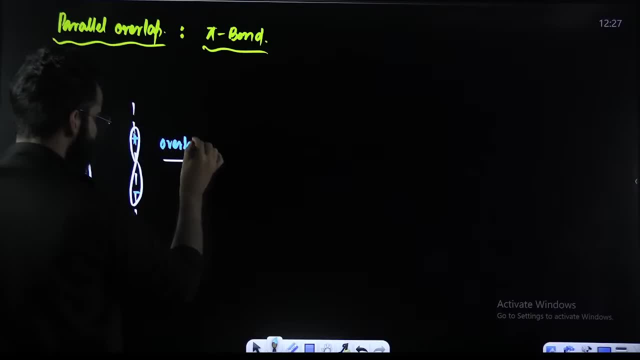 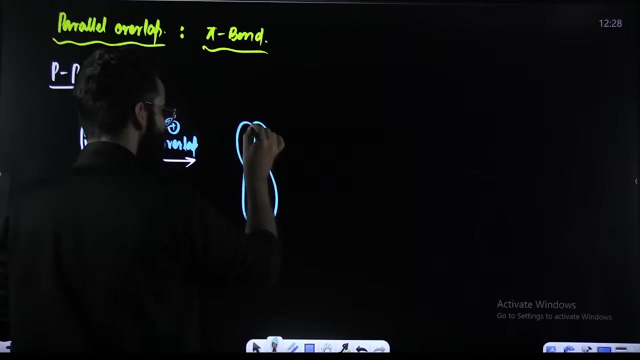 What is going to happen? What is going to happen, My dear students? overlapping will happen over here, Right, Overlapping will happen over here. How do I represent it at the end? How do I represent it at the end? How do I represent it at the end? 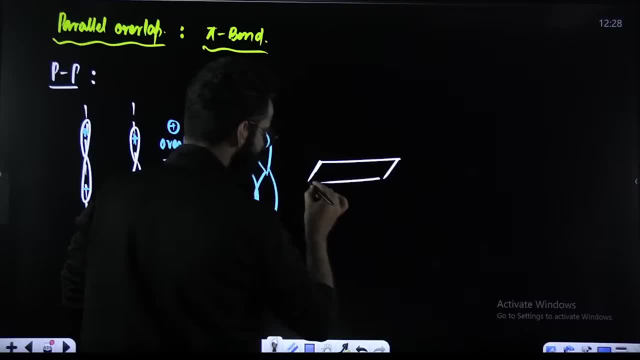 My dear students, first of all I am going to make a plane over here. This is one plane. Above this plane, there is a plane, There is another plane- electron density. and below this plane, again there is electron density. below this plane, again there is electron density. right, this is the nucleus of one. 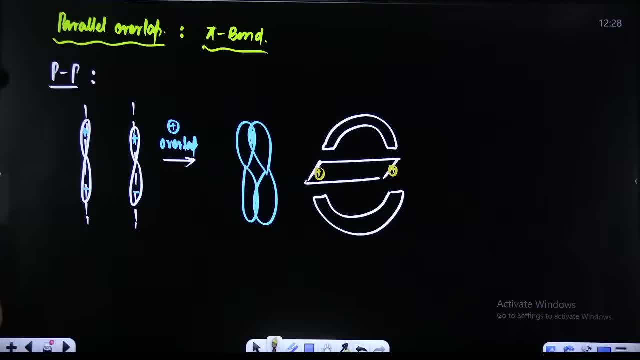 atom and this is the nucleus of one atom. perfect. so through parallel overlapping what happens? a pi bond got formed. pi bond got formed on this particular plane. is there any electron density? no, there is no electron density here. so this plane I'm calling as a nodal plane. this is what I'll be calling as a nodal plane. 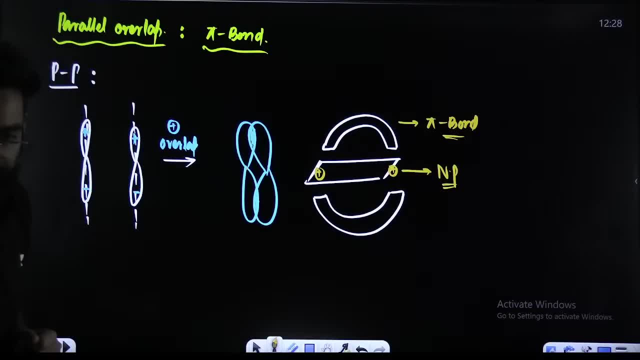 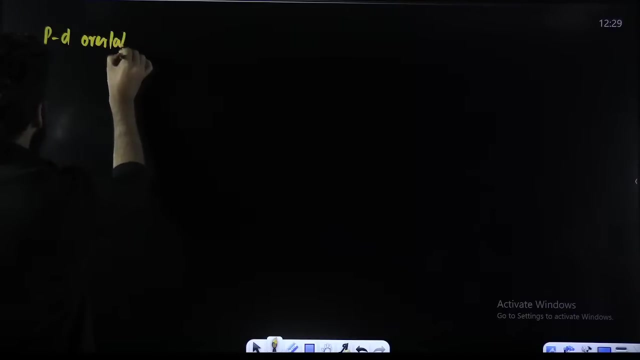 right, this is what I'll be calling as a nodal plane. perfect, am i clear? am i clear? am i clear? people, am i clear? this is one of the example of the parallel overlapping with the help of which pi bond gets formed. take an example, if I talk about PD overlap, PD, parallel overlap. 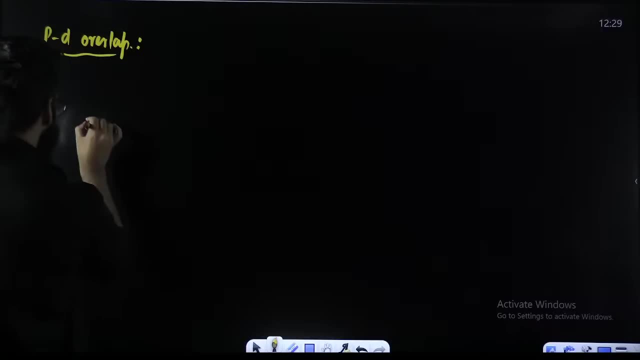 if I talk about PD, parallel overlap, right. let's say: this is your P orbital here, perfect, and this is your D orbital here. this is P and this is D. okay, let's call this positive. let's call this is negative. let's say this positive: this is negative, this is. 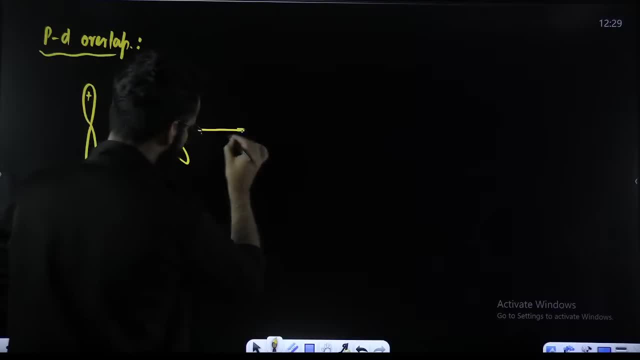 negative. this is positive. same sign, same sign, positive overlap. but right now this is going to be the parallel overlap. how exactly? this was your P orbital? perfect. and this is your D orbital. this is the common electron cloud part, merging of electron cloud into each other- perfect. so what do you get over here? you got a pi. 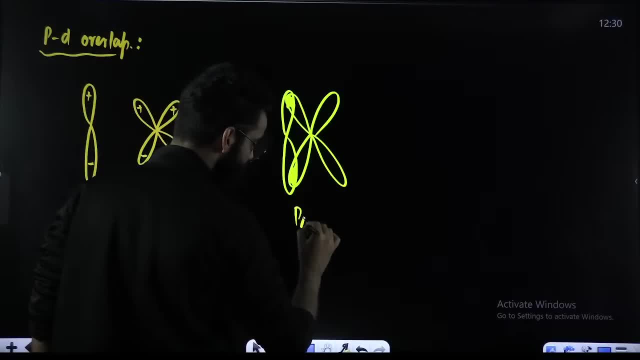 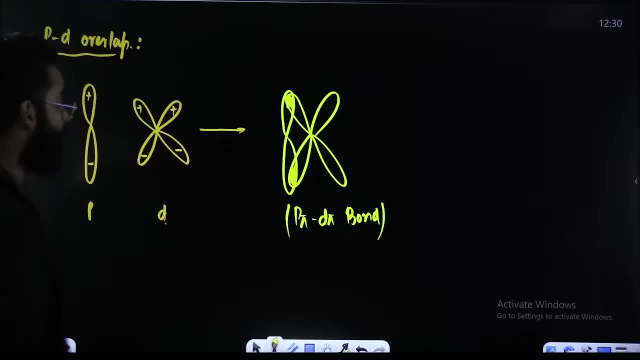 bond. you want a pi bond over here. what do we call this pi bond? as you call this as P pi D pi bond, you call this as P pi D pi bond, and I'm right now showing which overlap- positive overlap, if you want to show the negative. 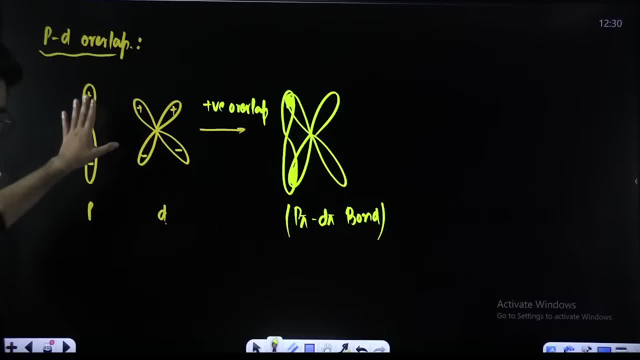 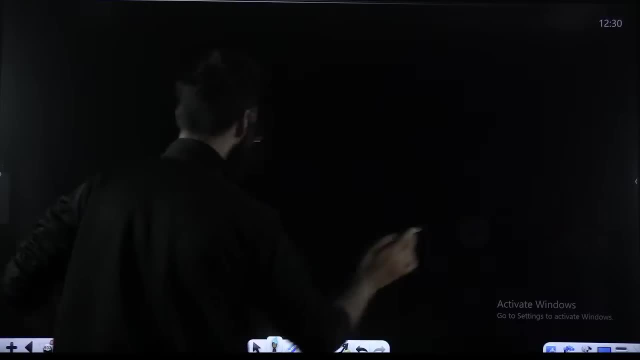 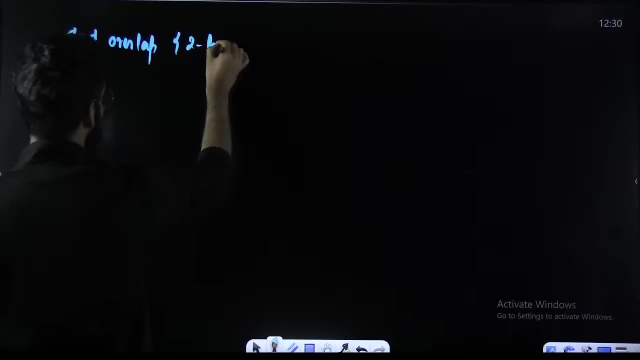 overlap. then keep the signs opposite. opposite signs on the same side. that's all. opposite signs on the same side. that's all right, this was your PD overlap, then all right, this was your PD overlap. then you have got. then you have got DD overlap, then you have got DD overlap. 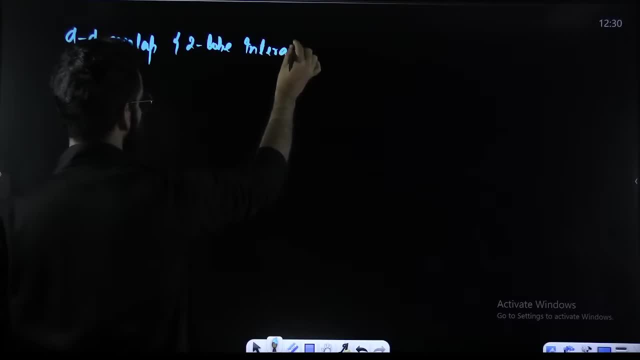 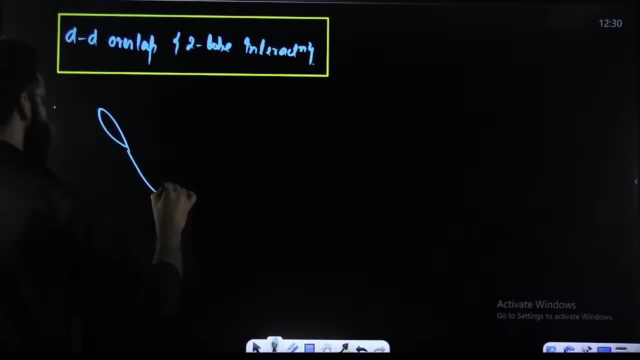 two lobe interaction. two lobe interaction, TD overlap. two lobe interaction. how exactly? let's say: this is your one of the D orbitals. one more time, one more D orbital, right now, how they are going to overlap exactly. first of all, let me give the signs. let's say this positive, this negative, right, perfect. 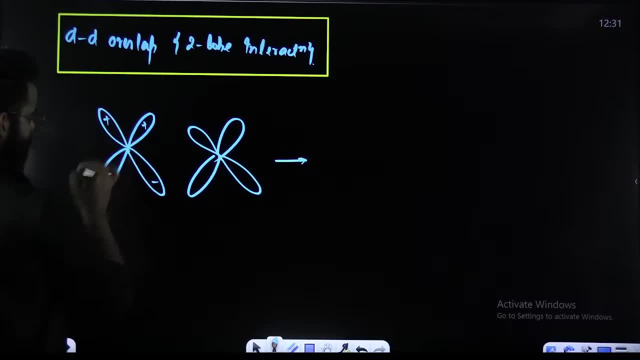 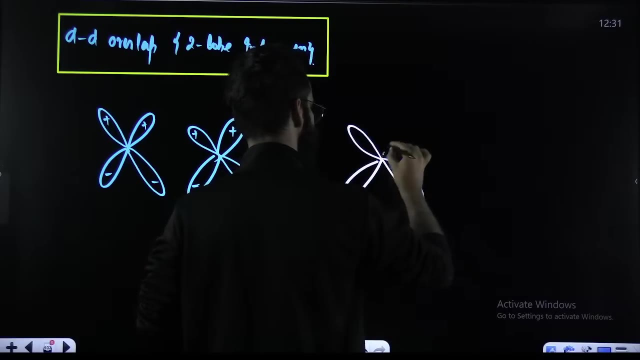 positive, negative, negative, positive, perfect positive, negative, negative, positive. do you see same sign on same side? so it is positive in phase overlap. it is positive in phase overlap. so this is what is going to happen. this is what is going to happen: perfect merging of electron clouds into each other. 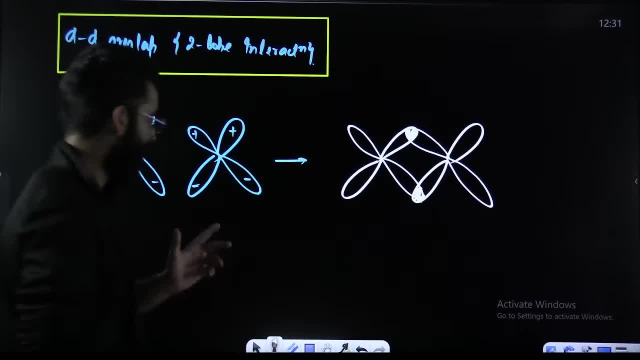 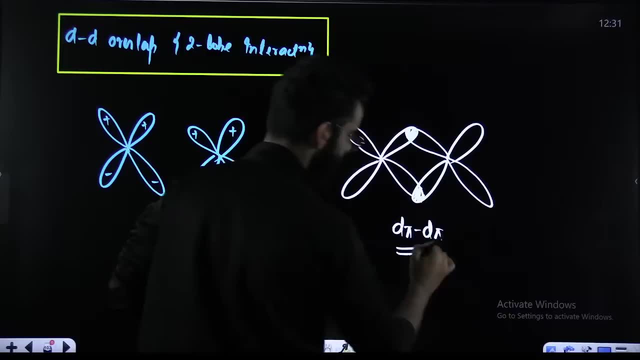 merging of electron clouds into each other, perfect. this is called as two lobe two lobe interaction and it leads to the formation of your pi bond. this is D, this is D. you call this particular pi bond as D pi D pi bond. you call this particular pi bond as D pi D pi bond. I hope I am. 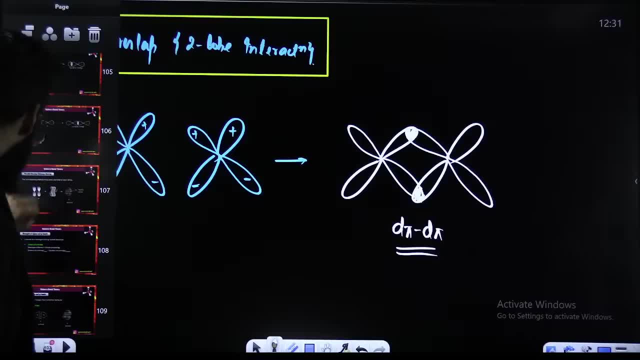 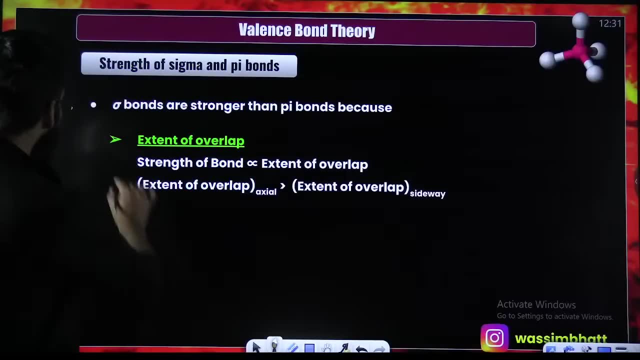 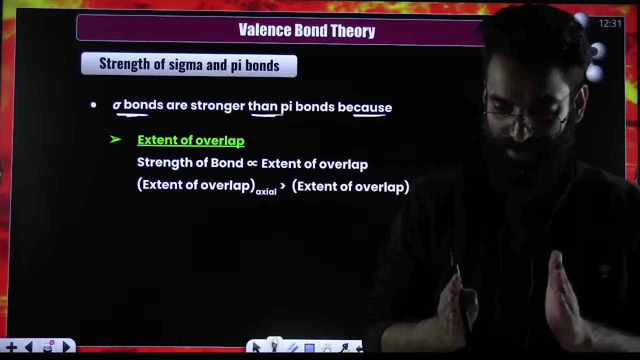 clear with every single thing. okay, and my dear students, so one thing which I would want to, which I would want you guys to remember: You know your sigma bonds. they are stronger than your pi bonds. Sigma bonds gets formed by the axial overlapping. Pi bond gets formed by the parallel overlapping. 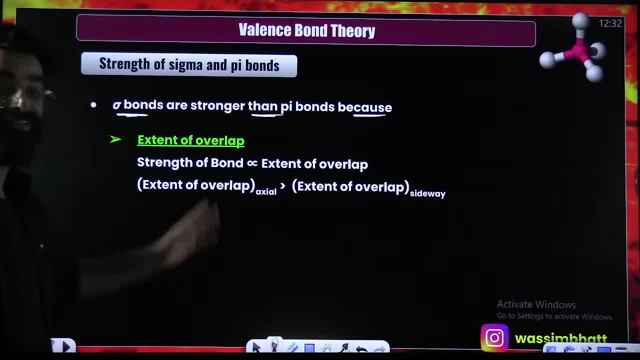 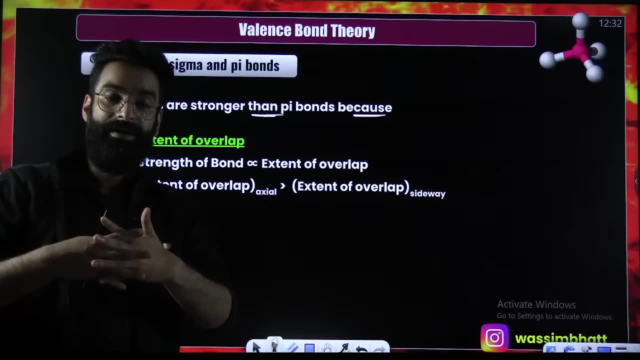 Pi bond gets formed by the parallel overlapping. Do remember, do remember sigma bonds. they are stronger than pi bonds. What is the reason? What is the reason? Because in axial overlapping extent of overlap is more Extent of overlap, Extent of overlap in axial. 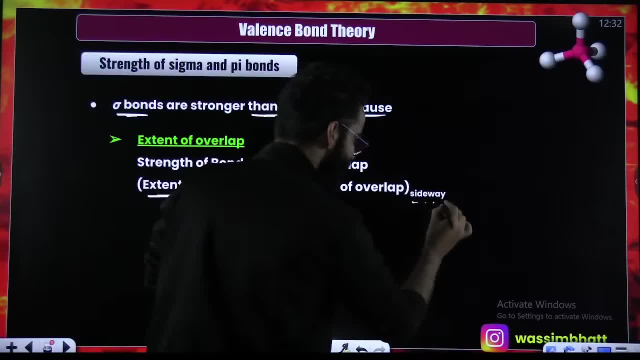 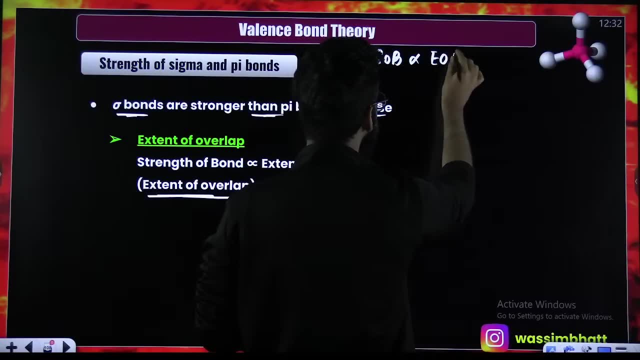 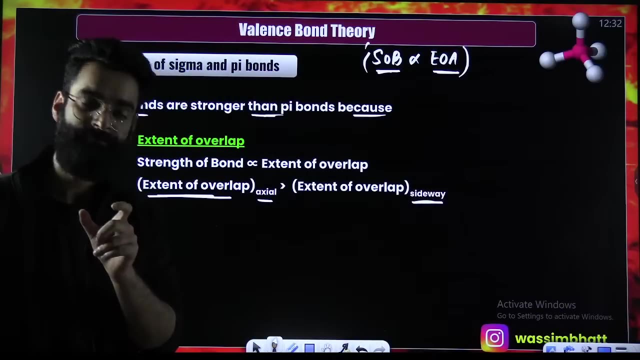 In axial is always more than that of Extent of overlap. in parallel, And do remember, Strength of the bond Is directly proportional to extent of overlap. More the overlap, Stronger the bond In case of axial overlap. What happens In case of axial overlap? What happens? 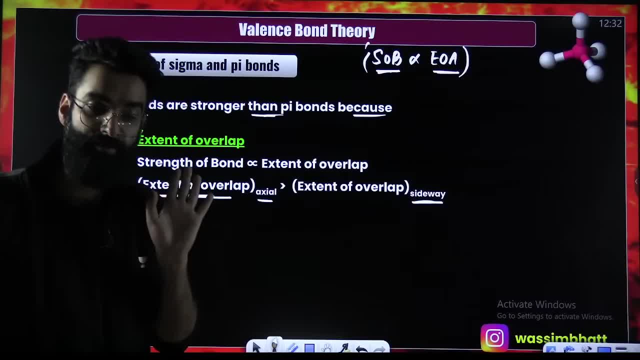 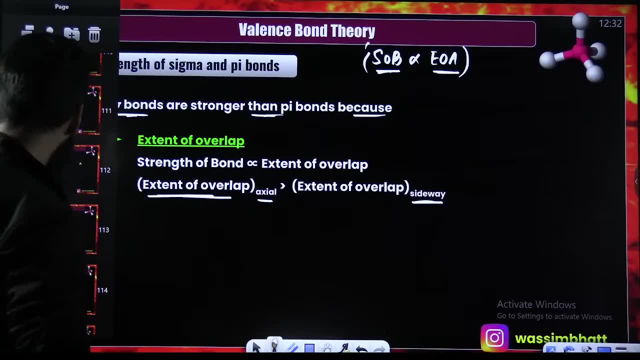 Extent of overlap is more. More the extent of overlap, More the strength of the bond. That's all. That's all people. Now I am going to take few examples So that you can understand all this in detail. All this in detail. Few examples, With the help of few examples. 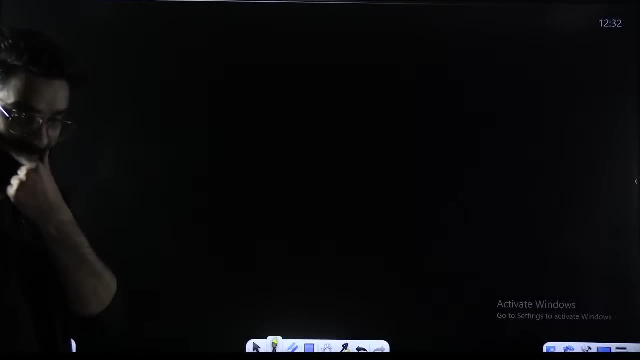 Try to understand what exactly I am going to do Now. I am going to apply the valence bond theory. For example, I have to show the F2 molecule formation. Let's say, I have to show the F2 molecule formation With the help of what? With the help of VBT. 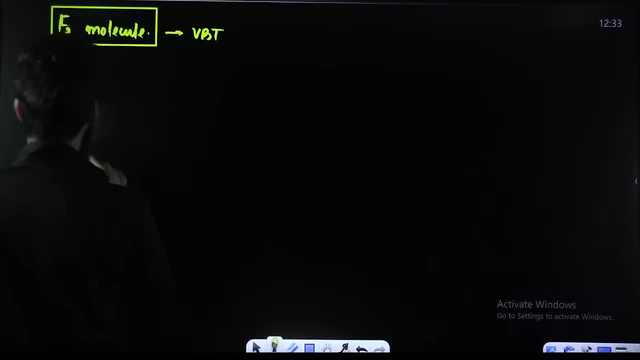 With the help of VBT: Correct. So this is your one fluorine atom. This is one more fluorine atom. Can you let me know the outermost configuration of fluorine? It is 2P5. This one is also what. This is, 2P5 configuration. 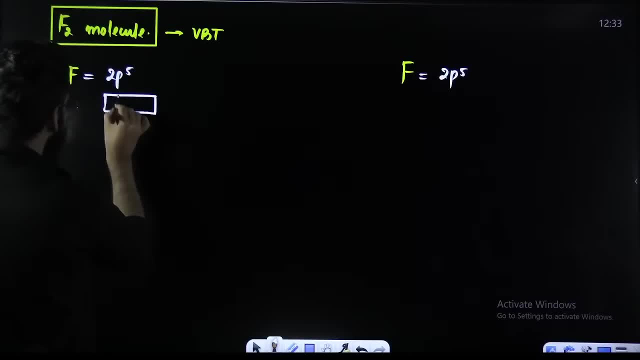 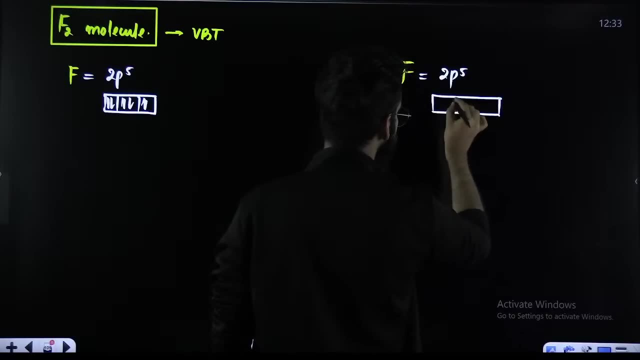 How do I show this 2P5 configuration: 1, 2, 3, 4, 5. Similarly over here: 1, 2, 3, 4, 5. Let's say I have to show the 2P5 configuration. This is your one fluorine atom. 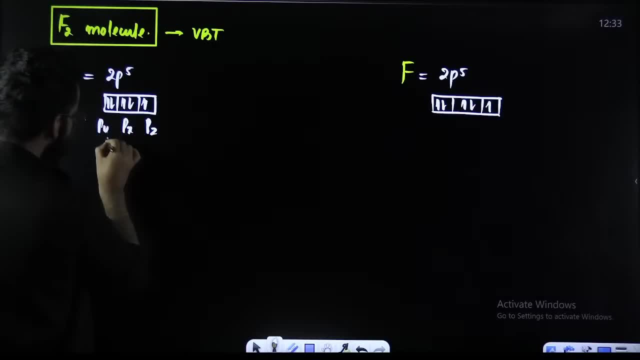 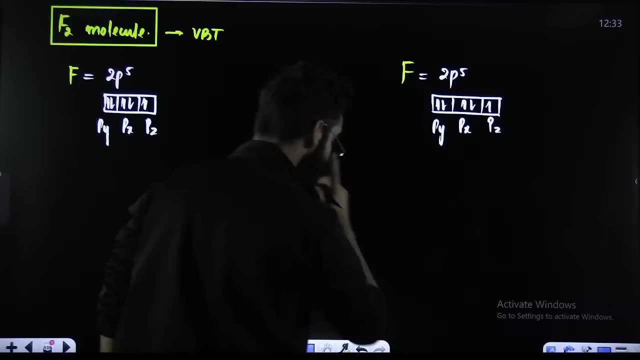 Let me call this as PZ. Let me call this as PX. Let me call this as PY. Let me call this as PZ. This is PX, This is PY. Now, what is going to happen If I talk about this fluorine atom? How many orbitals do we see here? 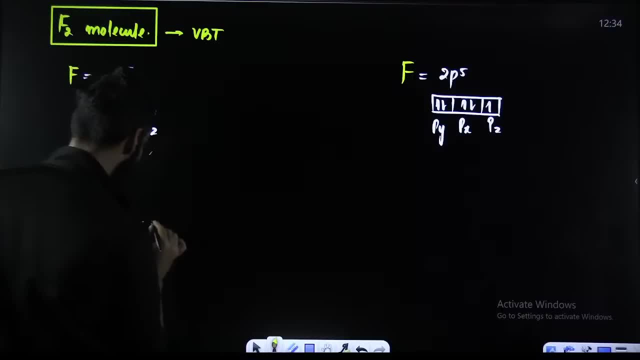 3 orbitals Right. This axis I am calling as Z axis Inter nuclear axis. This is your Z axis Inter nuclear axis. Right, If I look at this: fluorine, This is PZ. This is PZ Containing 1 electron Containing 1 electron. 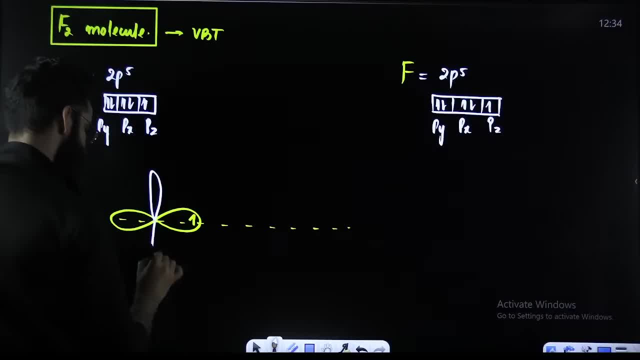 Now, PX is containing 2 electrons. Let's say: this is PX. This PX is containing 2 electrons. Now, this is PY. PY is also containing 2 electrons. Let's say: this is your PY containing 2 electrons. Right Now, if I look at this particular fluorine, 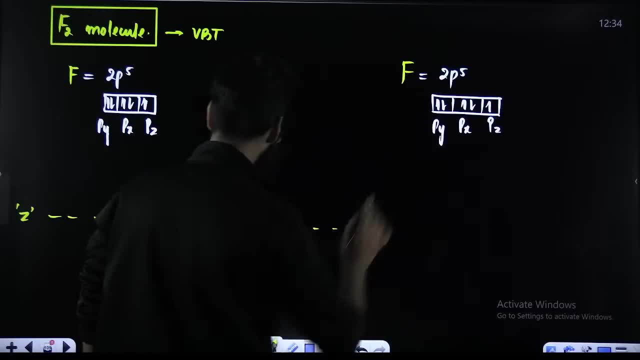 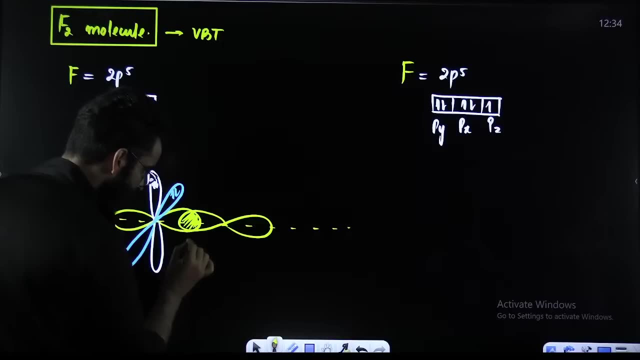 What is going to happen here? What is going to happen here? This is PZ containing 1 electron. That PZ will come from here and will do the head-on overlap. This is the head-on overlap. So which bond got formed here? Sigma bond got formed. 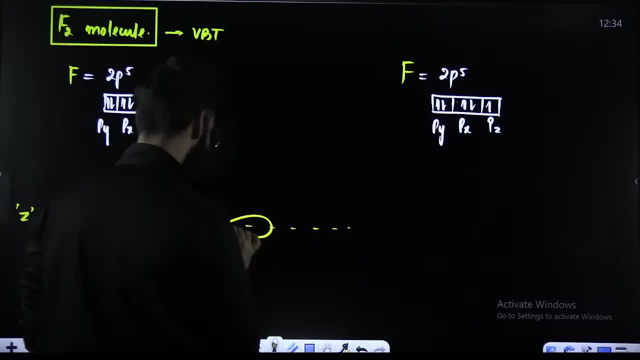 Now, what about the rest? What about the rest? This is your PX. So PX containing 2 electrons, PX containing 2 electrons And at the same time, And at the same time, Your PY is also containing 2 electrons. So this is PY containing 2 electrons. 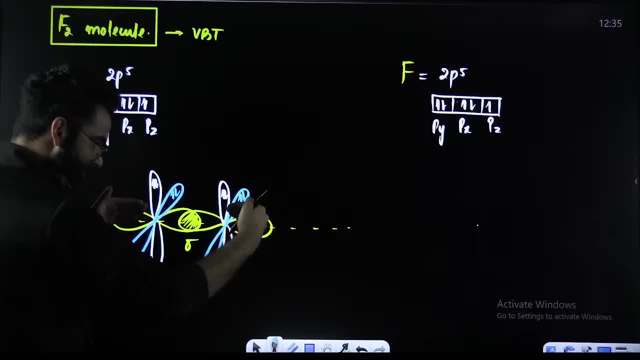 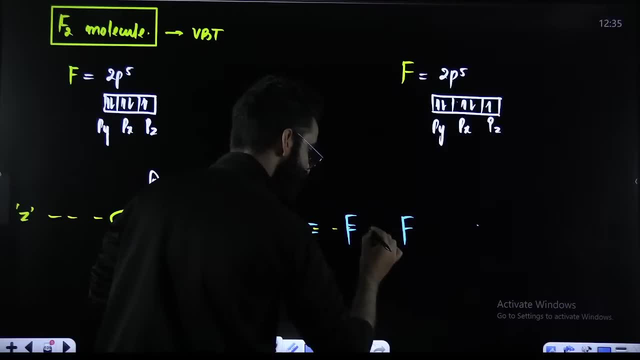 Do you see? an overlap happened. Right, It was the head-on overlap Which leads to the formation of sigma bond. How do I show it at the end? One fluorine, One fluorine, Fluorine and fluorine. Between them there is a single bond. 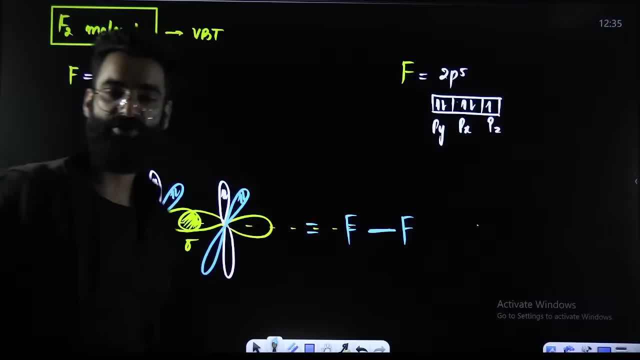 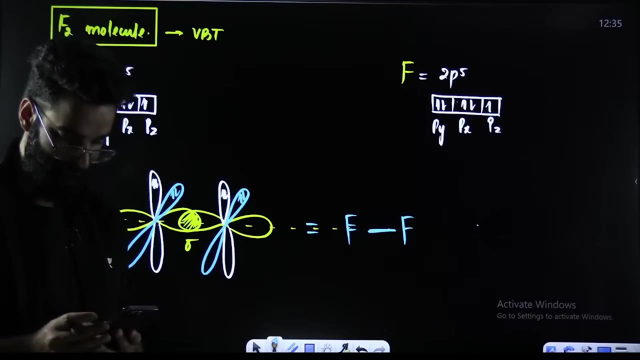 Right. Between them there is a single bond. I hope you got to know about the formation of F2 through VBT. This is the formation. This is the formation of F2 through VBT, If I am clear, Let me know once in the chats If I am clear, people. 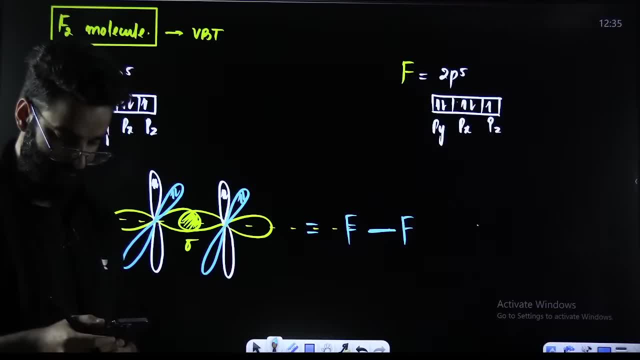 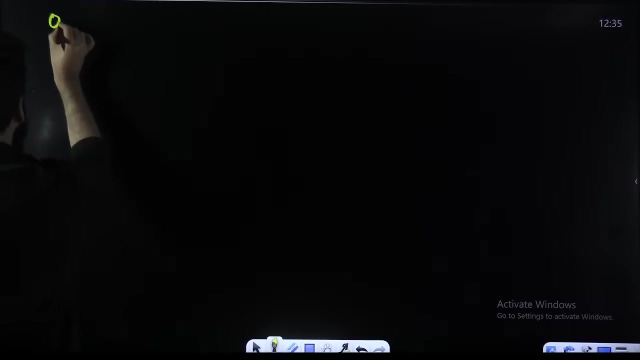 Let me know quickly in the chats, All of you, For example, Yeah, All clear. One more example which will make it more interesting. One more example which will make it more interesting. Let me show you the formation of O2 molecule. O2 molecule formation through VBT. O2 molecule formation through VBT. 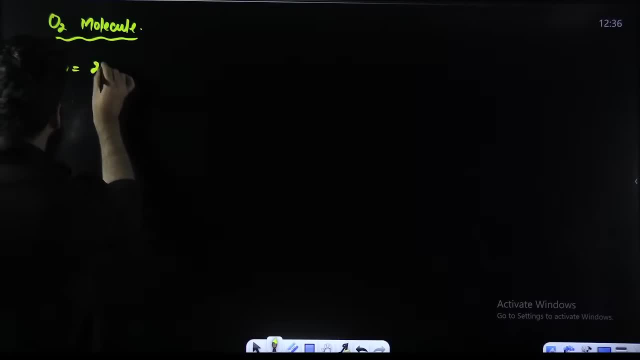 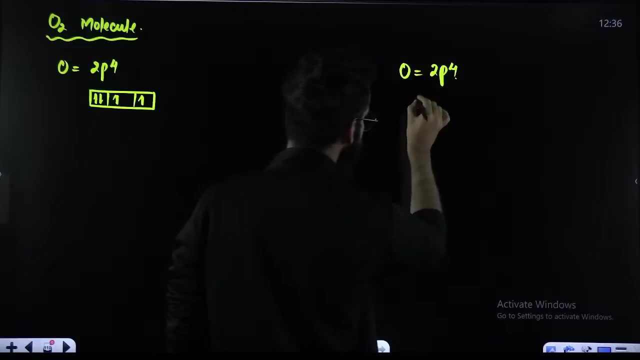 My dear students, If I talk about oxygen, Its outermost configuration is 2P4?. If I talk about one more oxygen, Its outermost configuration is 2P4?. Right Now, This is 1, 2, 3 and 4: 1. 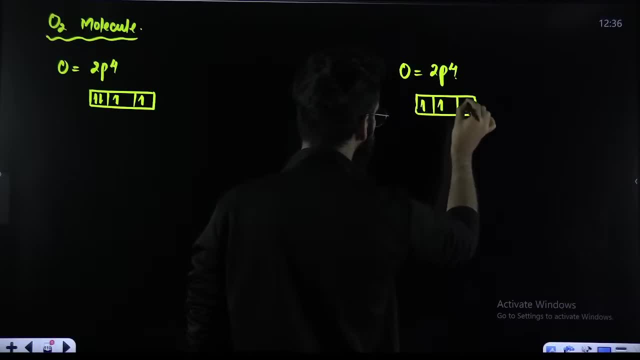 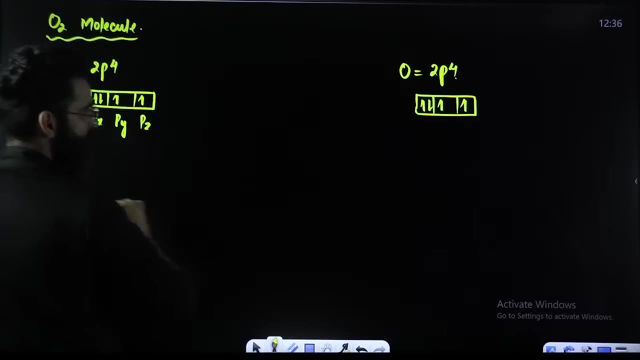 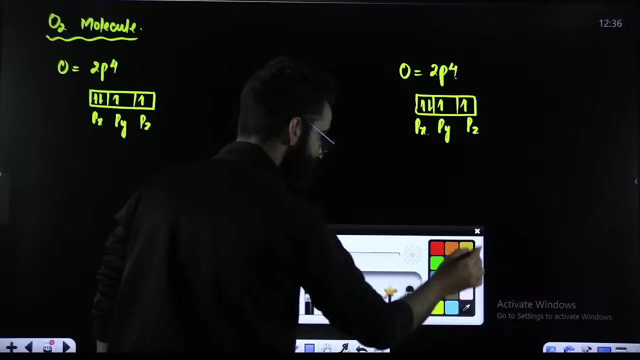 2, 3 and 4. If I call this as Px, This is your Py, for example, This is your Pz, for example: Pz, Py, Px. This is your Py, for example. This is your Pz, for example: Pz, Py, Px, Px. First of all, I am going to draw the internuclear axes. 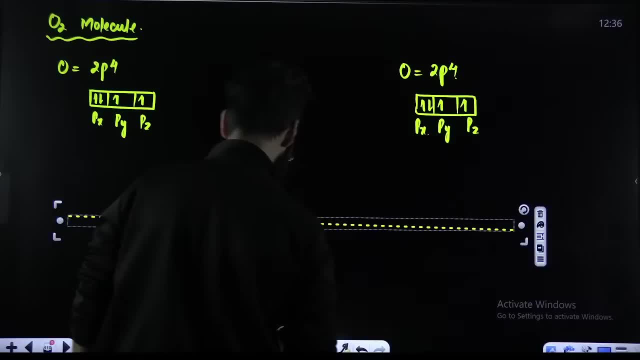 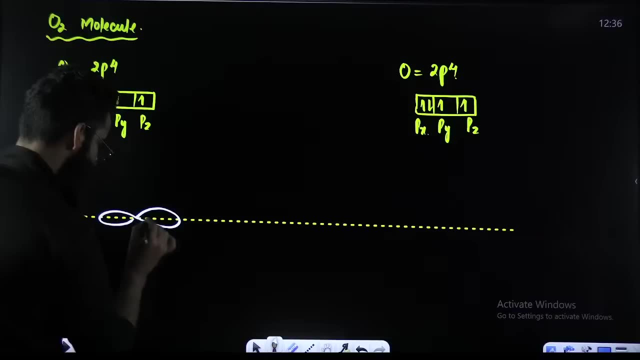 This is your internuclear axes, which you call as Z-axis, Z-axis Right. This is your Pz here containing one electron. Then you have got Py containing one electron. This is Py containing one electron. Then you have got Px containing two electrons. Let's say this is Px containing two electrons. 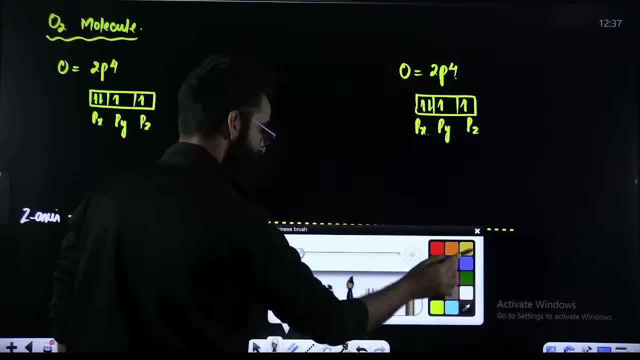 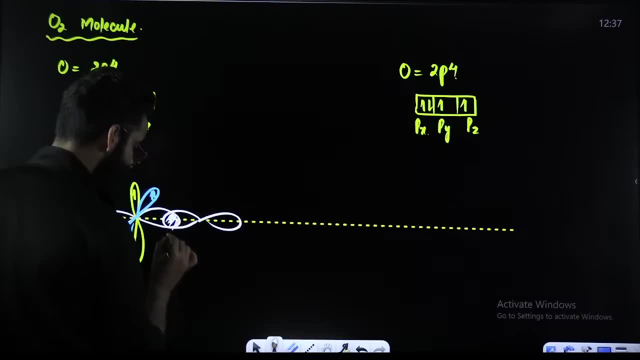 Correct. Now what's going to happen? What's going to happen? This is PZ. PZ of one more fluorine will come from this side. We'll do the head-on overlap. So which bond got formed? It's the Sigma here. It is the Sigma here. 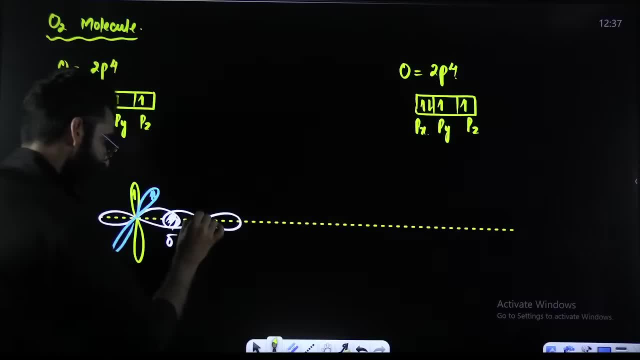 It is a Sigma here now. now, P Y is also containing one electron, So this is P Y containing one electron. perfect, So this P Y and this P Y. they are going to show the sideways overlapping, So they'll show the sideways overlapping, parallel overlapping. So this is a pi bond here. right then, you have got. 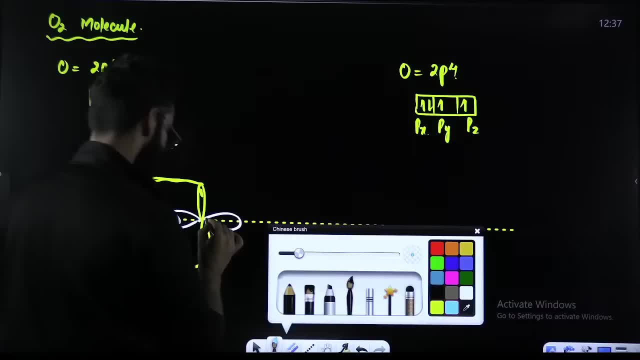 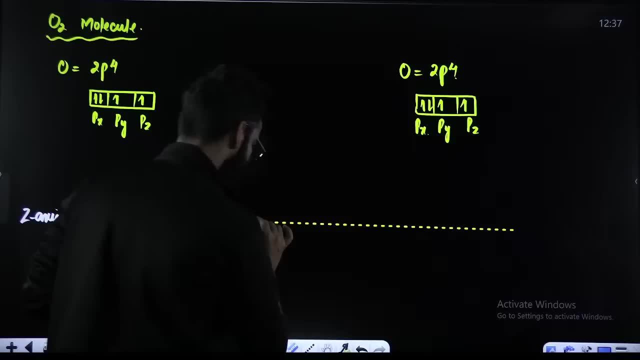 You have got P X as well, So P X is already full fulfilled two electrons there. So this is P X, Correct? So one Sigma and one pi got formed. one Sigma and one pi got formed. which bond got formed first? a Sigma bond got formed first a. 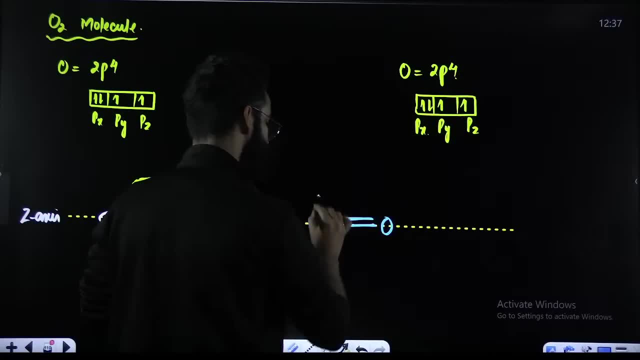 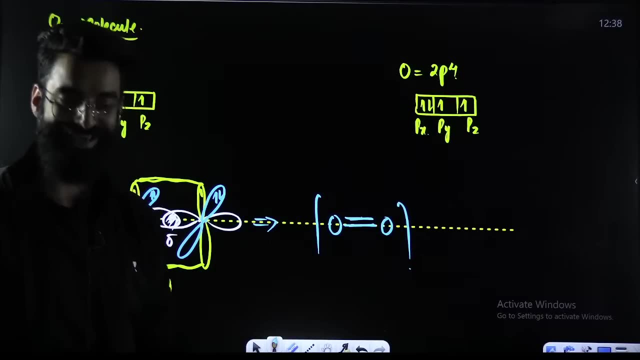 Sigma bond got formed first. after that a pi bond got formed. So do remember Sigma is formed first, followed by pi. Do remember Sigma is formed first, followed by pi. Am I clear till here? Am I clear till here, people? Okay, Do you want to see more about it? 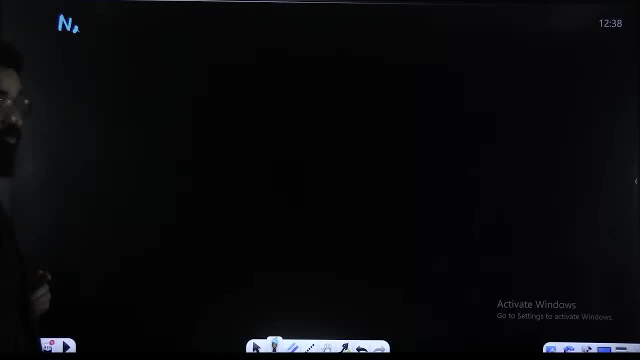 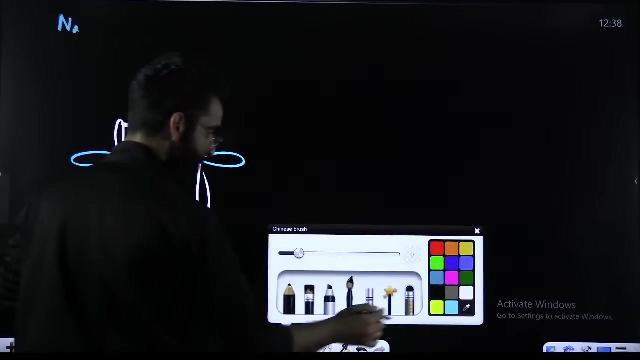 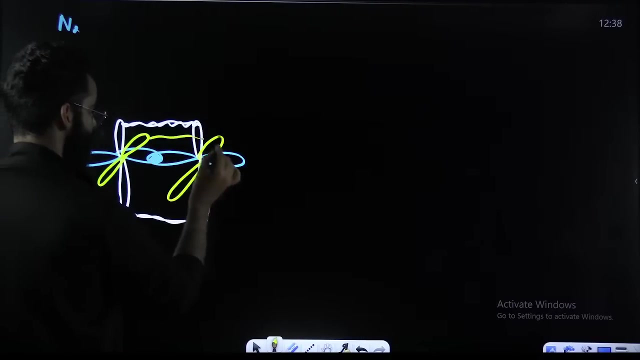 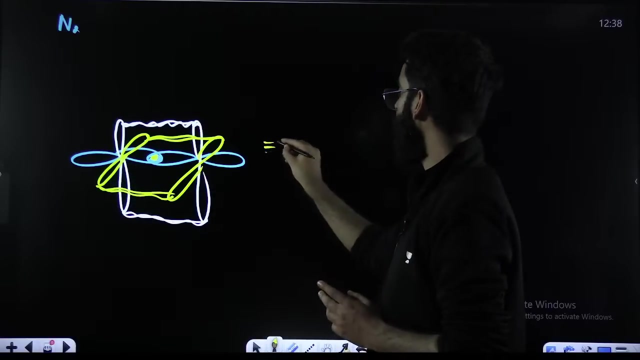 I believe n to molecule formation. you can easily do n to molecule formation. I Believe n to molecule formation. you can easily do right the final structure. I'm making Sigma, Pi, Pi, One more pi, So one Sigma, one Sigma and two pi bonds here in case of n to. and finally, how do you represent it? 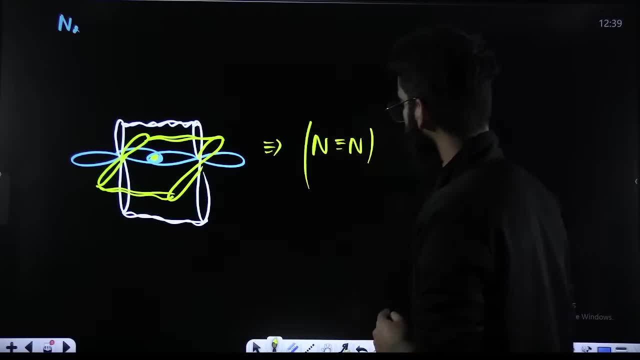 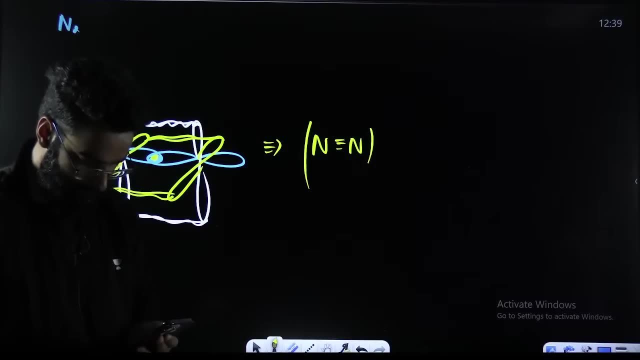 This is n triple bonded. out of this triple bond, one is Sigma and one is pi. right, I think let's take a break for 20 minutes and be back up and We'll be right back. Okay, What time you guys are going to be back? 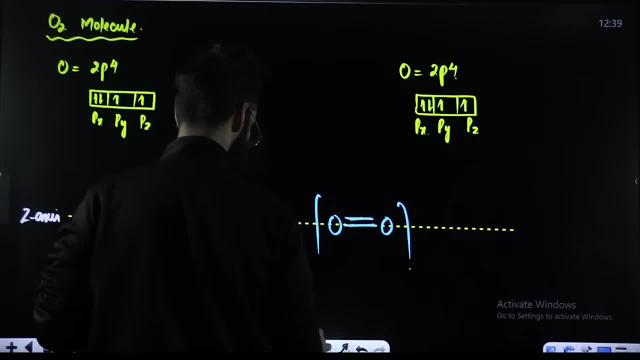 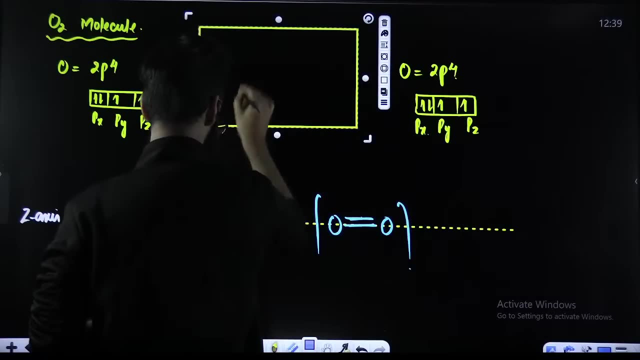 Hmm, I will just be seeing this for like 20 seconds and we will see what time is it. So, no, I mean 2021 should be like the same time, like I said, but its like you're not even that old. It is usually like훗. 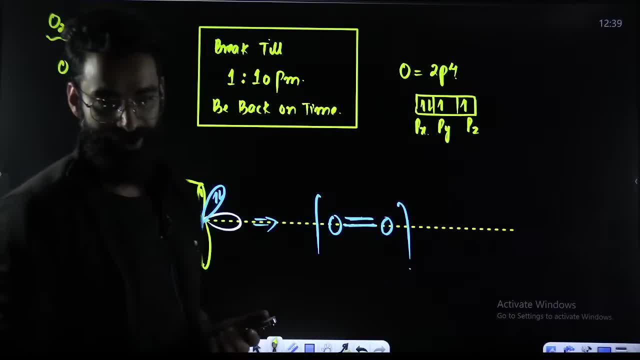 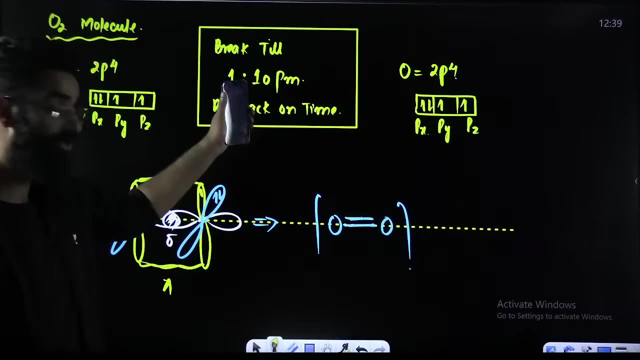 Or if you are not born yet. I'm so excited. So are you guys going to be back or not? Honestly, I would want every one of you to be back on time. Okay, I'll see you all at 1: 10 PM sharp. 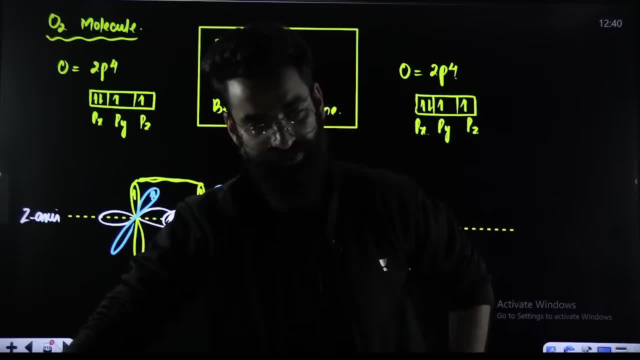 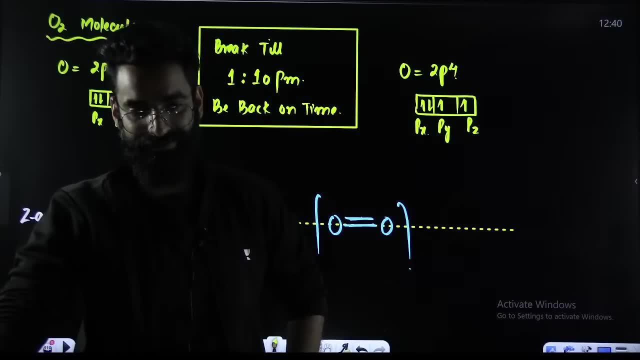 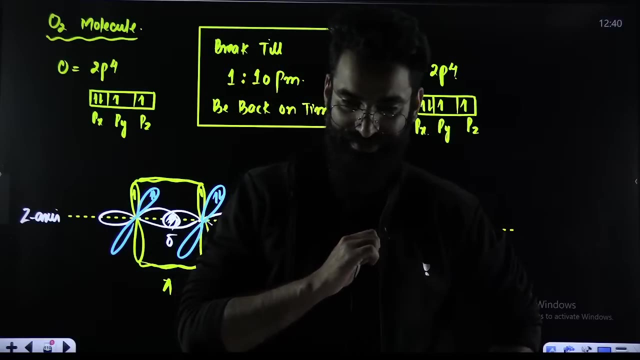 Perfect. till then you can have. yes, Yes, I'll cover all the topics. I'll cover all the topics. you need not to worry, but be back on the time, otherwise there is no fun in teaching. yes, it is your lunch break. go and come back. 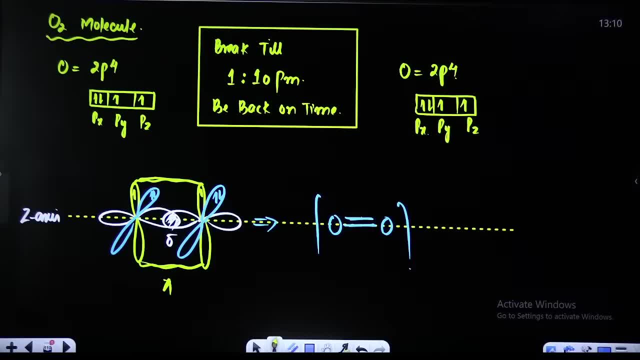 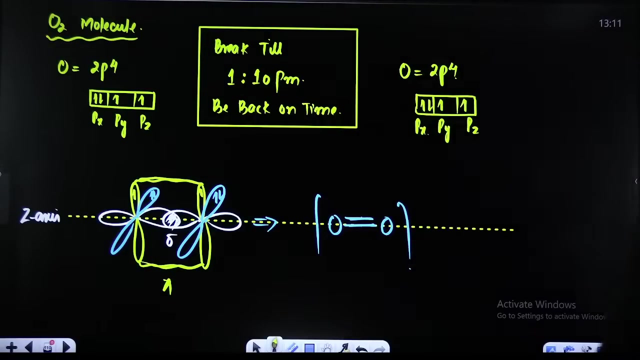 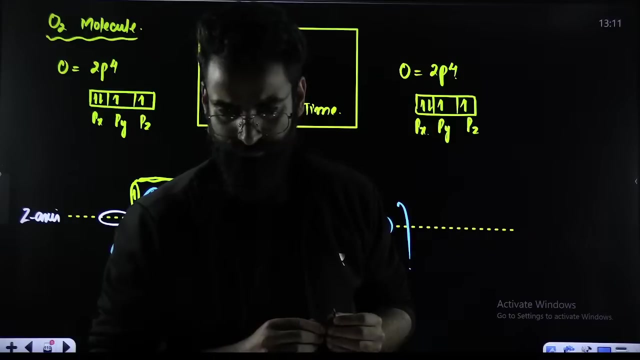 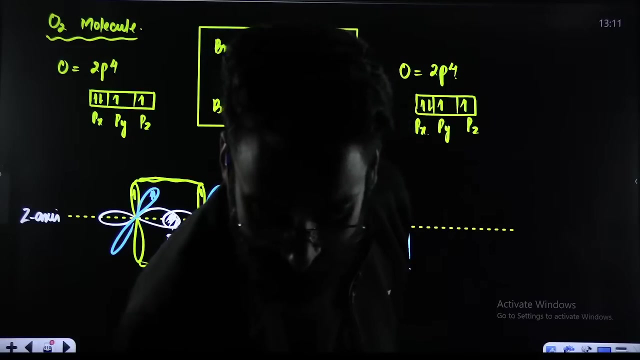 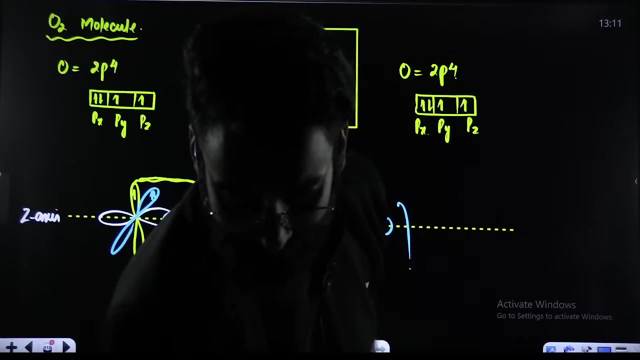 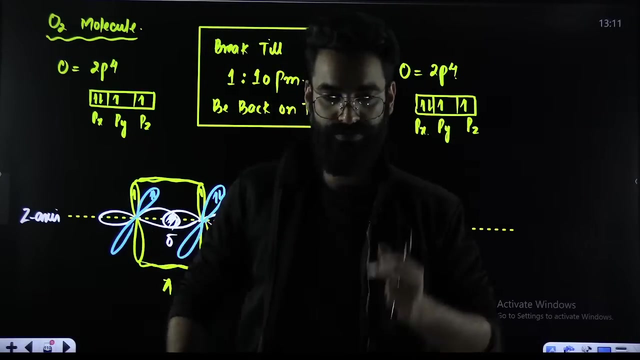 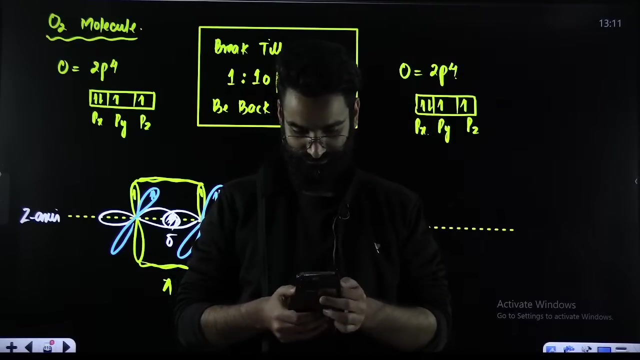 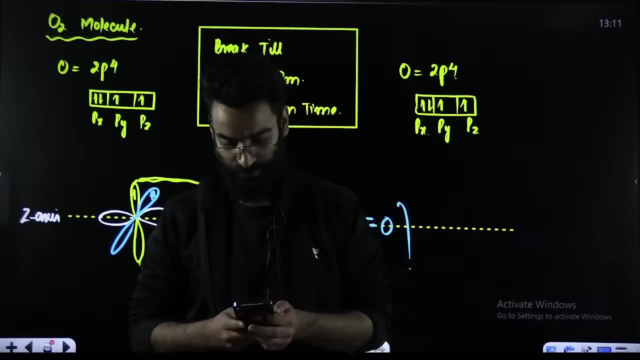 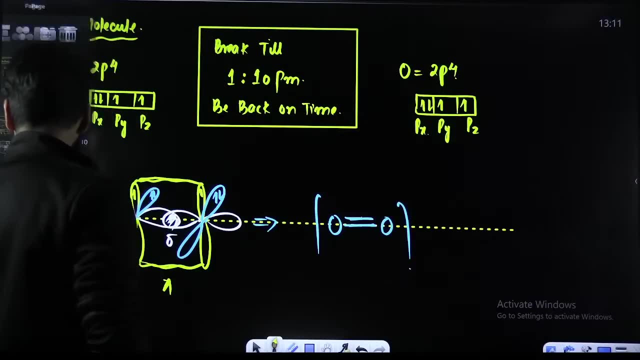 So once let me know in the chats Whatever I discussed till now, are all the topics absolutely clear. Let me know in the chats quickly: people, Let me know in the chats quickly Whatever I discussed till now. are all the things clear? 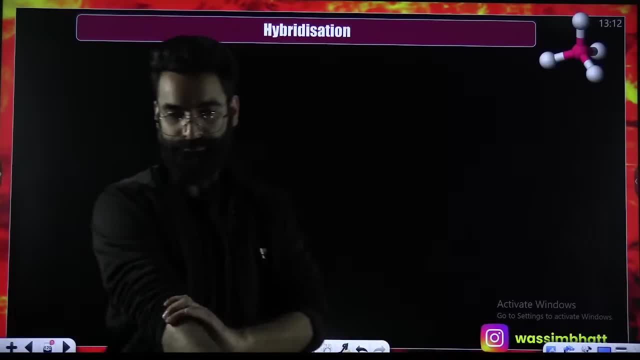 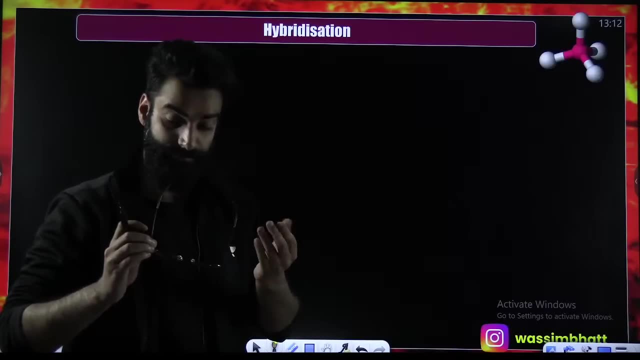 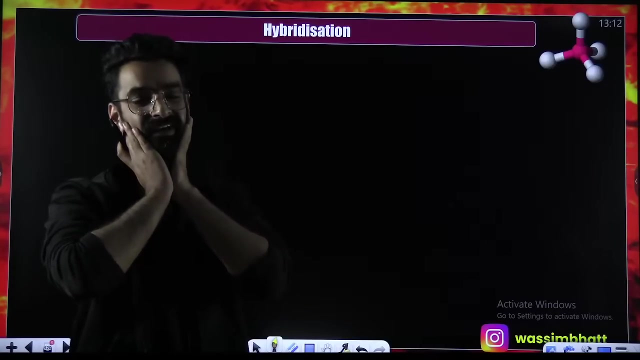 Are all the things absolutely clear? Yes, And guys, one thing I'm telling you: Whatever I'm going to discuss in the today's session, you're not going to get anything apart from these things in your actual examination. Okay, Okay. 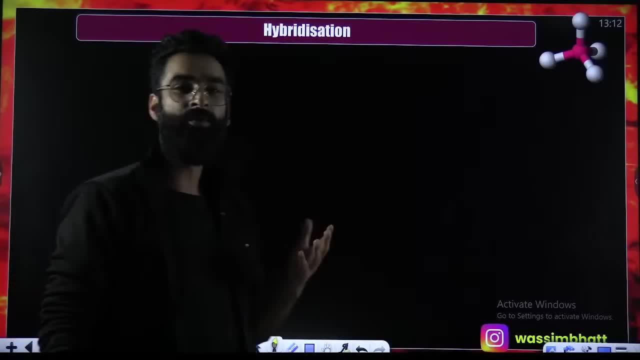 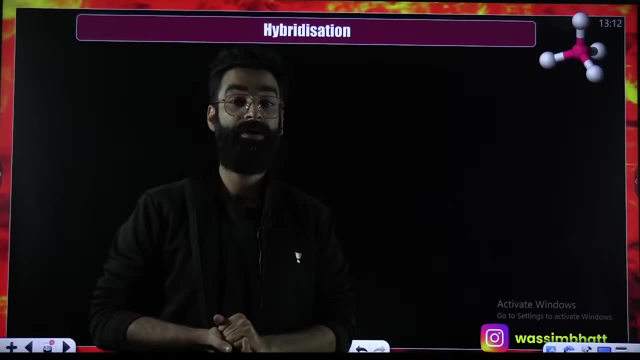 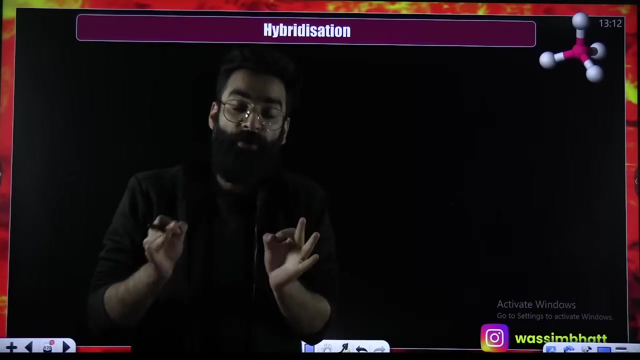 Perfect. Now comes one more important- I would say the most important- topic of the chapter, The most important topic of your inorganic chemistry, That is hybridization. Okay, That is hybridization. Before knowing the meaning of hybridization, you should know exactly why do we need this concept? 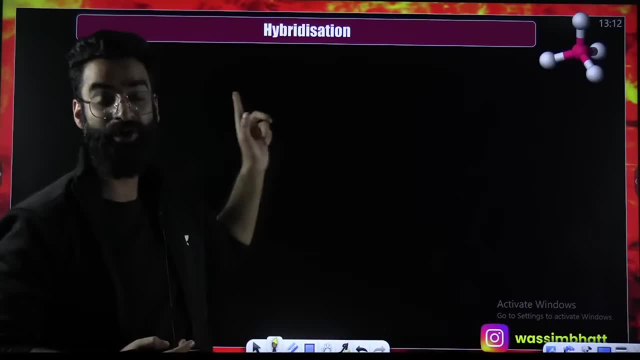 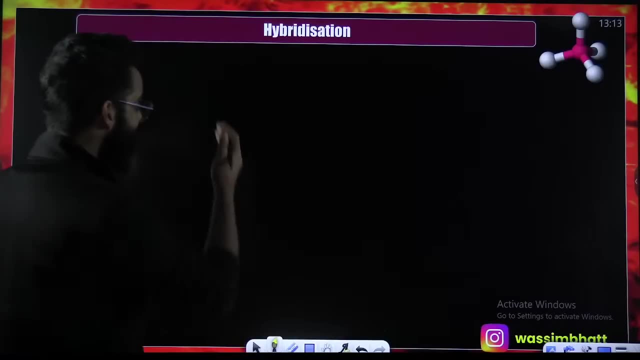 That is more important. Why do we need this concept of hybridization? That is more important, Guys. Okay, So let's have a look why the concept of hybridization was introduced. Right, Let's get to know about that. For example, 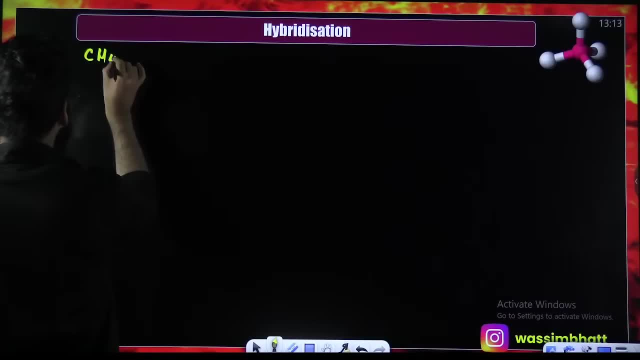 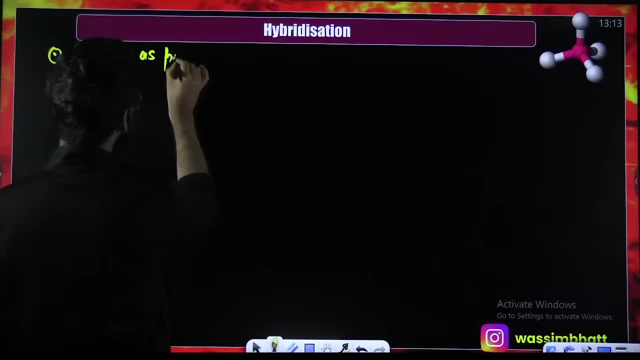 For example, I'll show you the formation of CH4 molecule. I'm going to show you the formation of CH4 molecule as per VBT. Formation of CH4 molecule. Formation of CH4 molecule as per VBT. As per VBT. 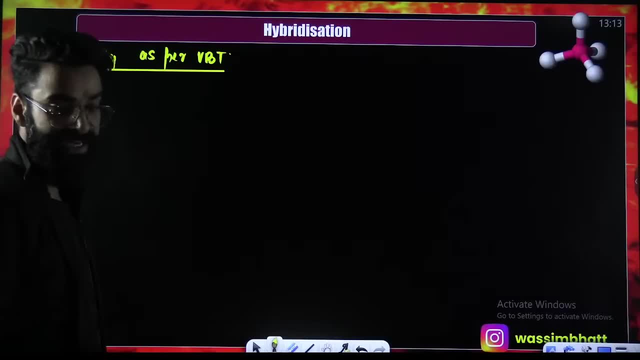 My dear students Try to understand very carefully. In case of CH4, The central atom is your carbon. The central atom is your carbon. If I ask you What is the outermost configuration of carbon, You will say 2s2, 2p2. This is the outermost configuration of carbon. 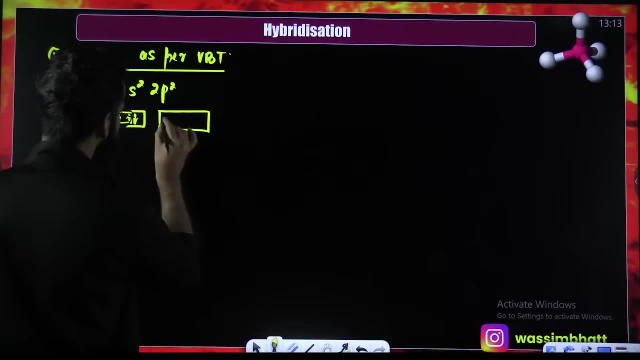 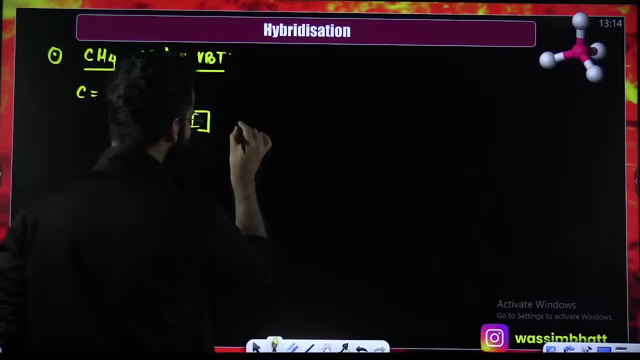 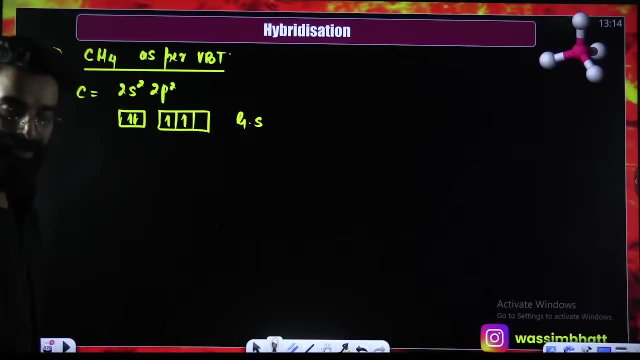 This is 2s2 And this is 2p2. This is the outermost configuration of carbon. Right now I can say Carbon is present In its ground state. Right now the carbon is present in its ground state. If I ask you, How many unpaired electrons? 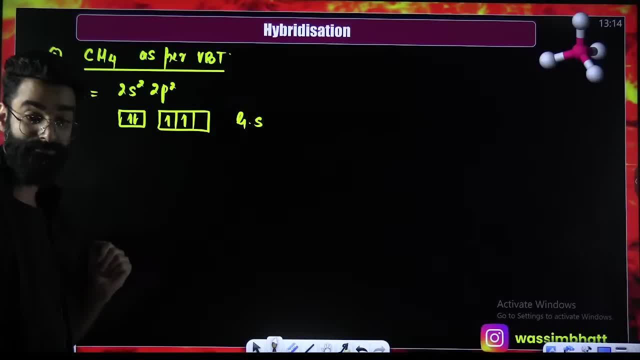 Carbon has in ground state? It has got 2 unpaired electrons. It has got 2 unpaired electrons, But how many bonds Carbon is forming? Carbon is making 4 bonds. In order to make 4 bonds, As per VBT, There should be 4 Unpaired electrons. 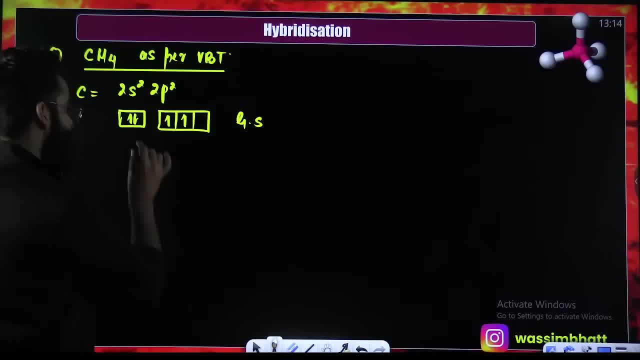 Now, how do you get the 4 unpaired electrons here If one of the electron from here Shifts? here, When one electron shifts, I am getting the excited state of carbon like this. This is the excited state of carbon. This is the excited state of carbon, Right. 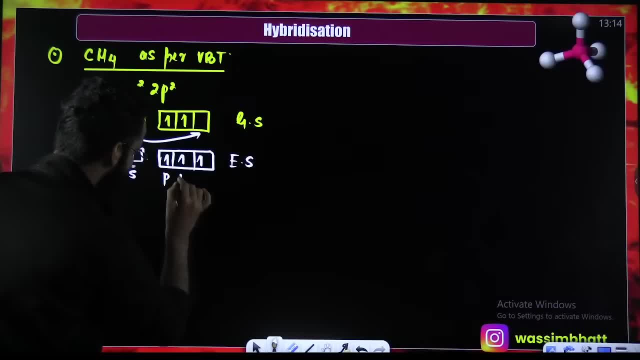 This is your s electron, This is p orbital containing one electron, One more p, One more p. Right Now, my dear students, This is s, This is p, This is p, This is p. Now, carbon has to form bonds with hydrogen. If I ask you, What is the configuration of hydrogen? 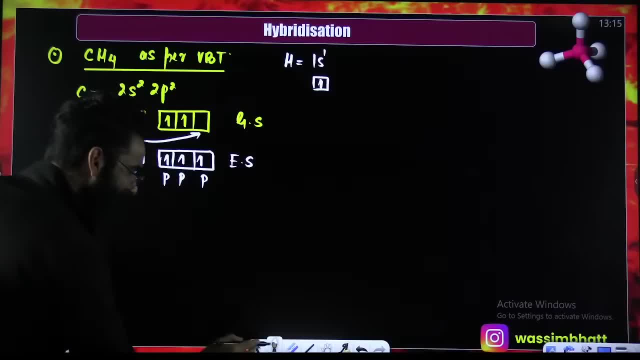 You will say 1s1. Perfect. So what I will say? I will say: One of the s orbitals of hydrogen will come from this side, Right, One of the s orbitals of hydrogen Will come from this side And will do the overlapping. Similarly, One more s orbital of one more hydrogen. 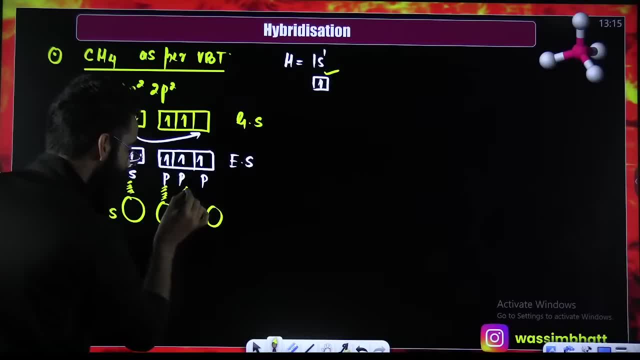 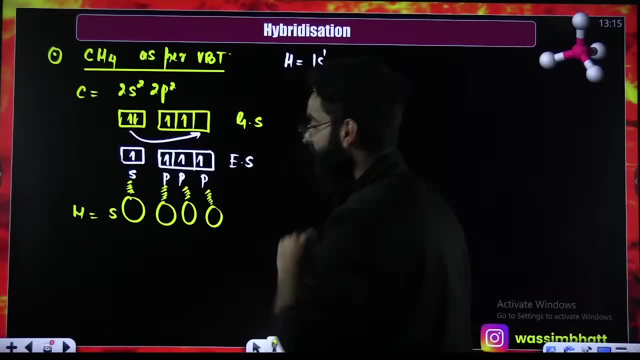 Will come from this side And will do the overlapping. One more, one more Perfect. And due to overlapping, what happens? Covalent bond formation takes place. So how many bonds are taking place? Four, So see this, for example: H, This is H, This is H And this is H. 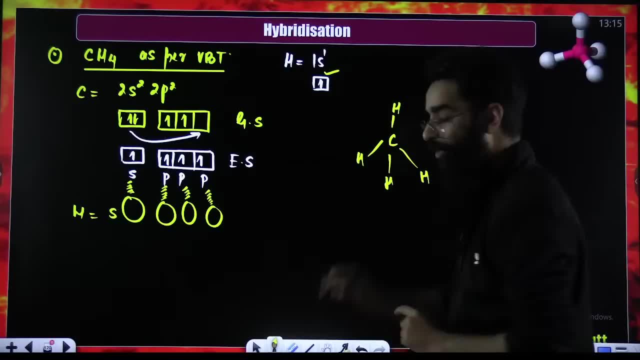 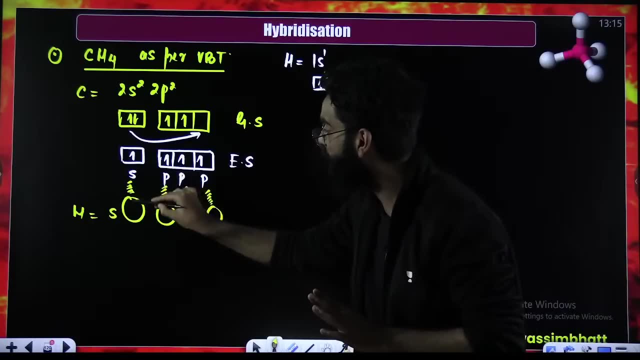 So, how many bonds? Four Now, if I ask you, Out of this, these four bonds. Out of these four bonds, One bond is forming These. One bond is formed Due to s s overlapping. One bond is formed Due to s p overlapping. One more s p, One more s p. 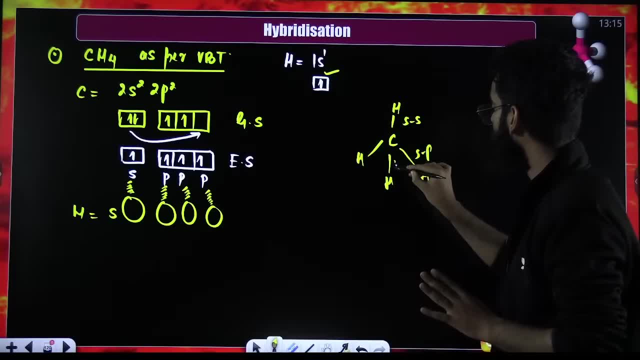 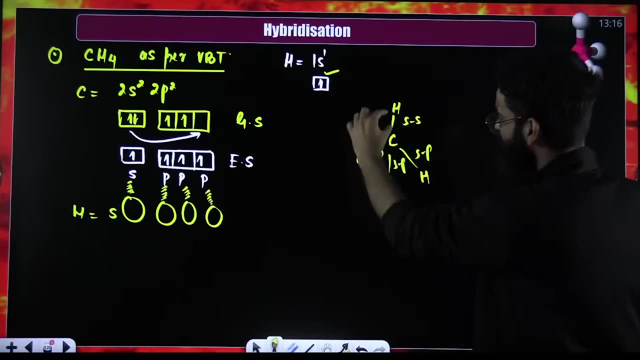 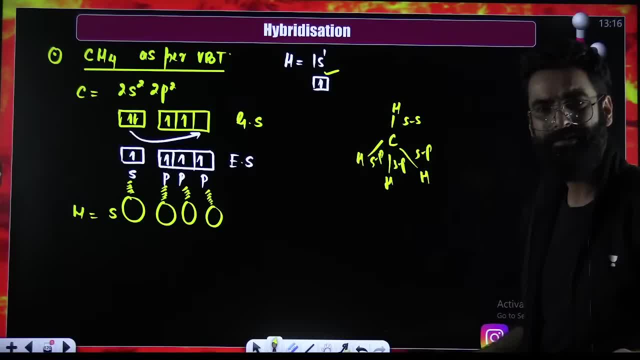 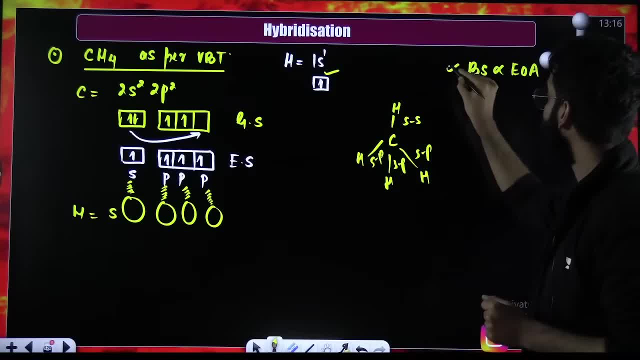 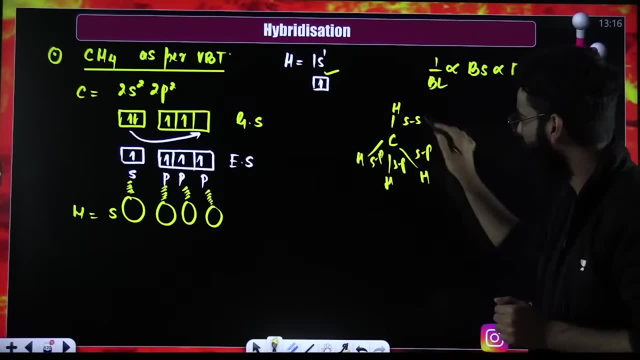 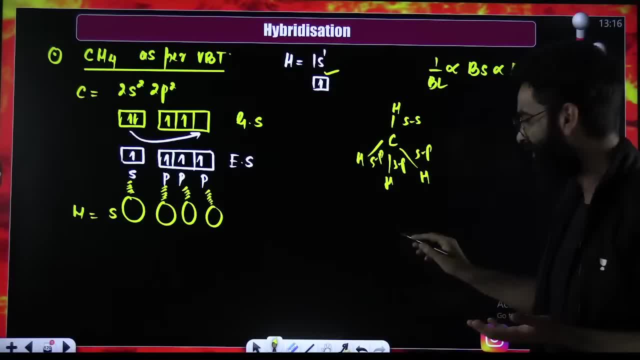 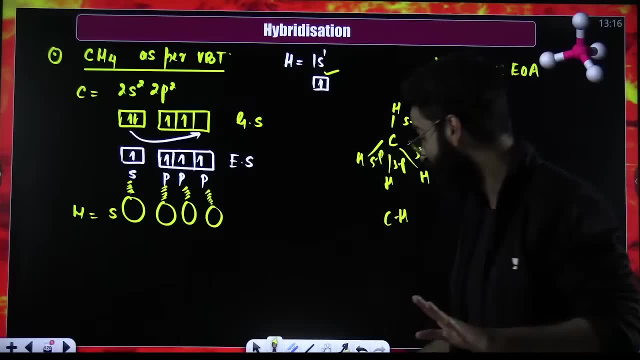 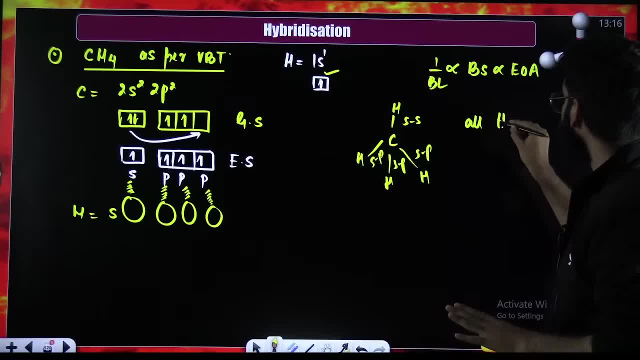 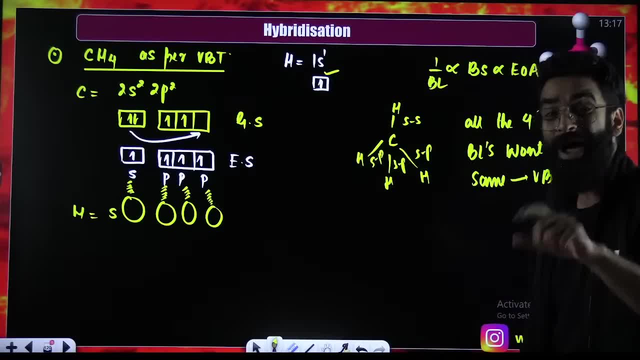 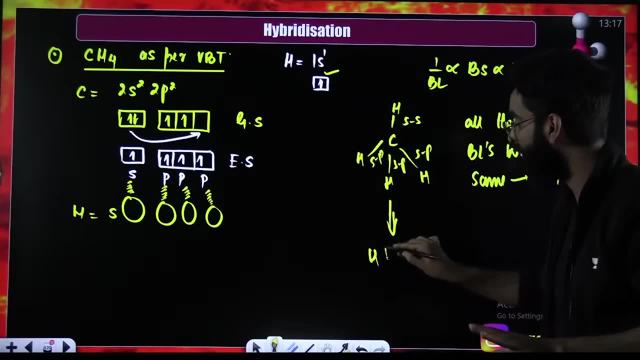 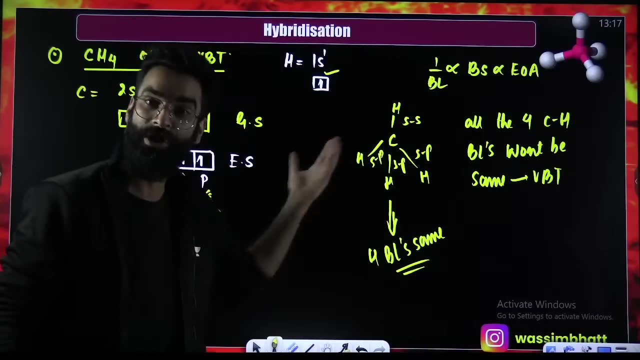 But, but, but. but. when you analyze the CH4 molecule, actually you will find all the four bond lengths are same. When you analyze, it is observed, it has been seen that in CH4, all the bond lengths are same. 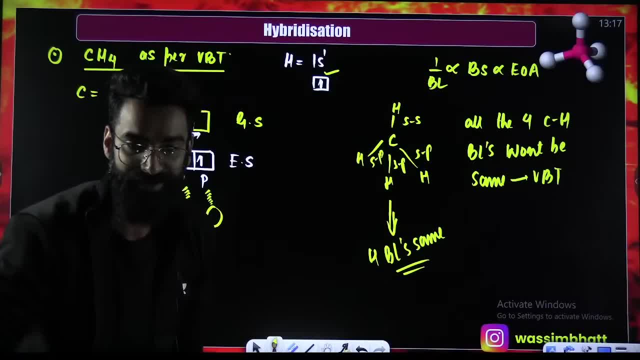 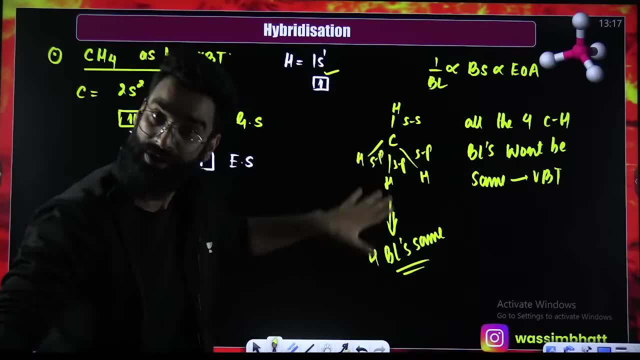 But, as per VBT, all the four bond lengths won't be same. Now, how do you explain it? How do you explain it? As per VBT, all the bond lengths should not be same, But in reality, all the bond lengths are same in CH4.. 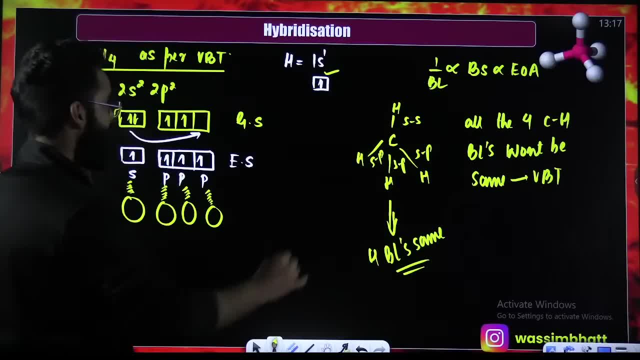 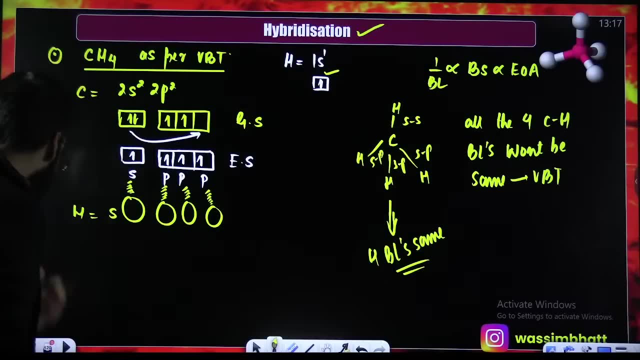 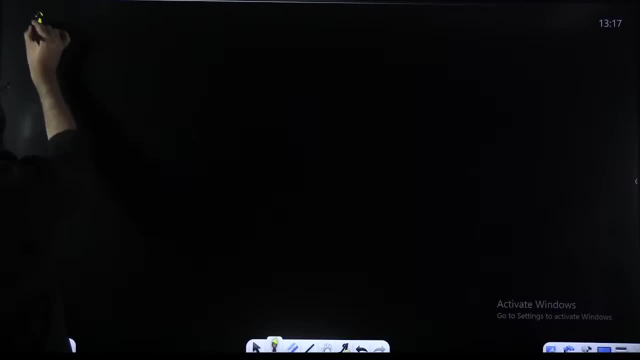 Now, how do you explain it? Explain it: we introduce a concept of hybridization. To explain it, we introduce the concept of hybridization. Now, what happens in this hybridization concept? What happens in this hybridization concept, My dear students? first point you have to remember: hybridization is a complete theoretical concept. 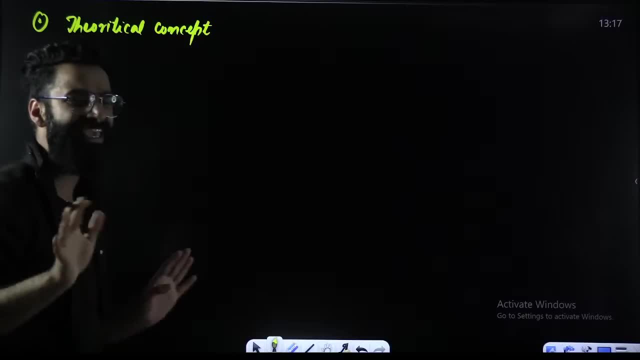 It is a complete theoretical. It does not have any experimental background. It is a complete theoretical concept, No experimental background. Number one, Number two, Number two, Number two: How do you define the hybridization? What happens in hybridization? 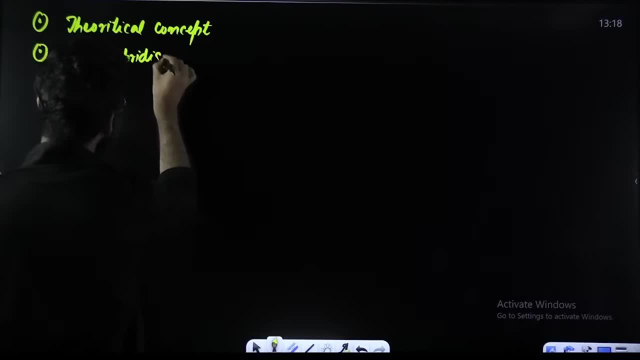 My dear students, in hybridization, in hybridization, what happens? Atomic orbitals. atomic orbitals which have got nearly same energy. Atomic orbitals which have got nearly same energy, belonging to the same atom. Belonging to the same atom. 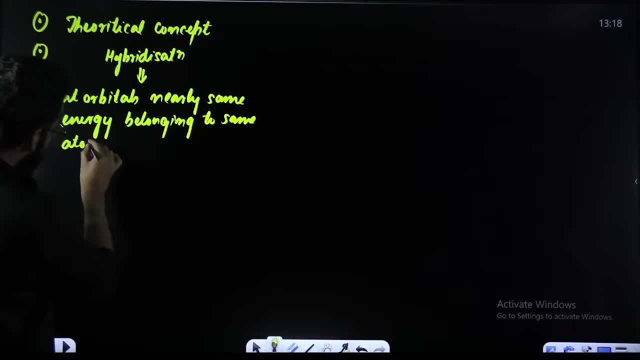 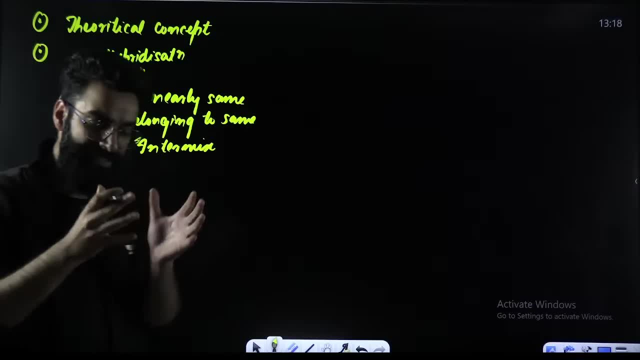 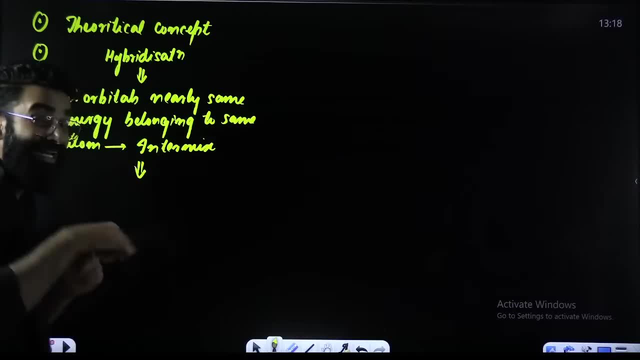 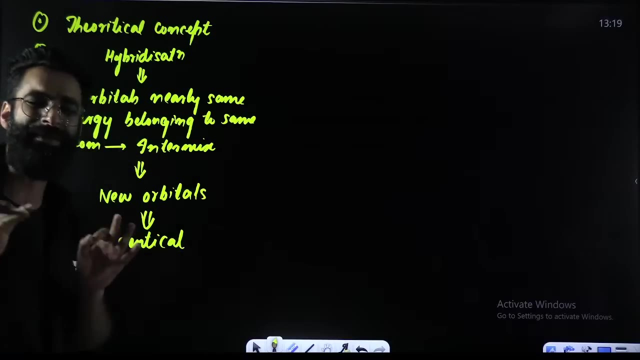 They are going to intermix And they are going to lead to the formation of new orbitals. They are going to lead to the formation of new orbitals Which have got which are identical in all the respects, Which are identical in all the respects, be it shape, be it size, be it energy. 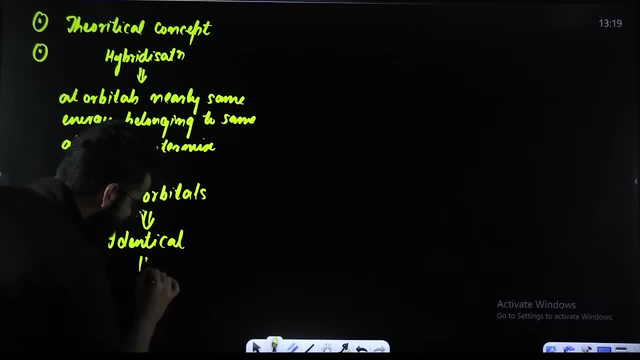 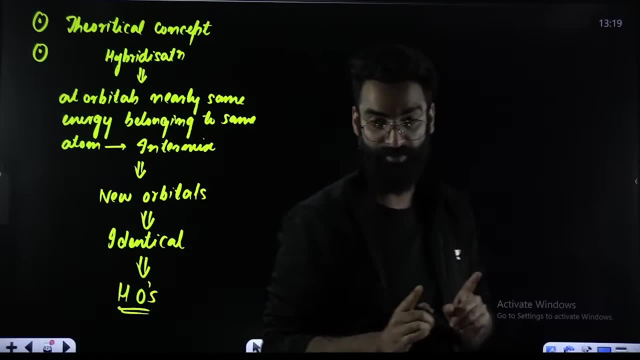 They are identical in all the respects, And those new orbitals which are identical in all the respects, those are what you call as hybrid orbitals. Those are what you call as hybrid orbitals As per hybridization atomic orbitals of the bonding atoms, which have got nearly same. 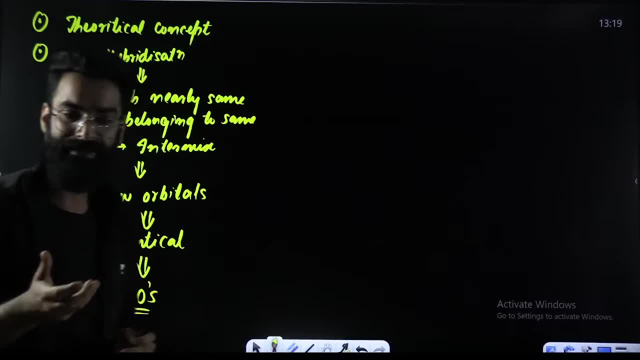 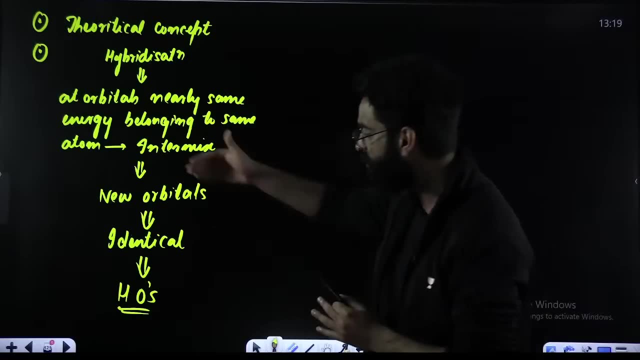 energy. They are going to intermix. They are going to intermix. They are going to lead to the formation of new orbitals which are identical in all the respects, Be it shape, be it size, be it energy. And those new orbitals which we get, those are called as hybrid orbitals. 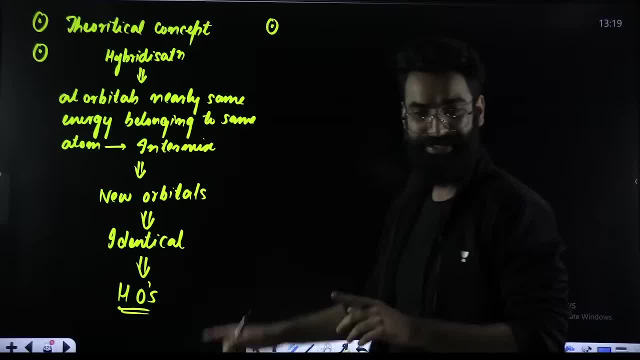 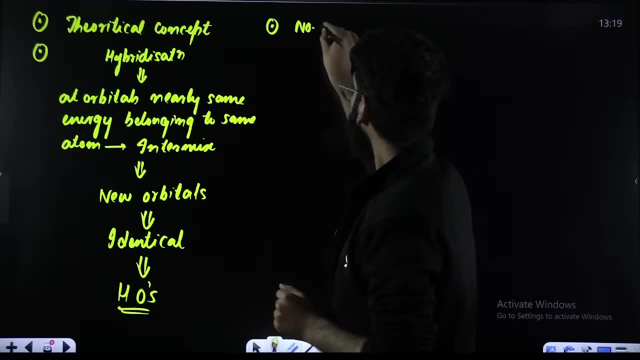 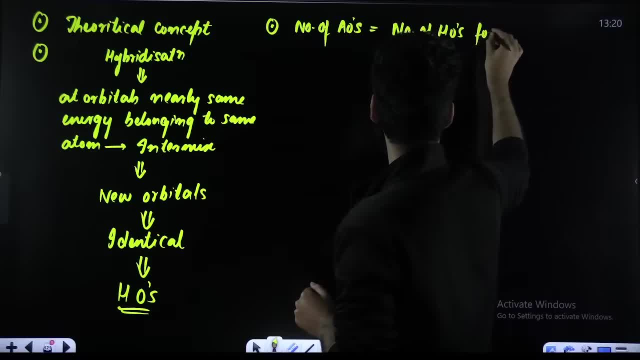 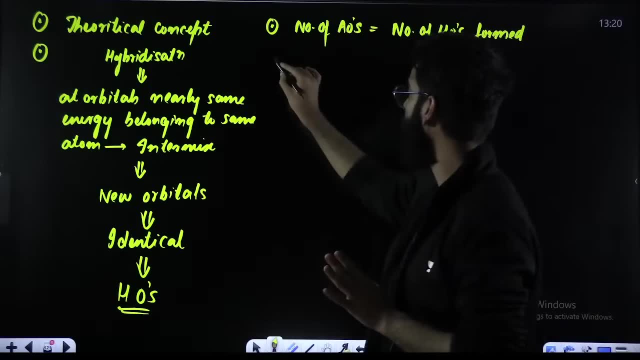 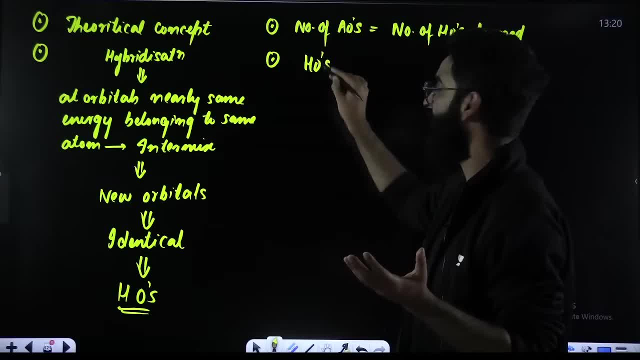 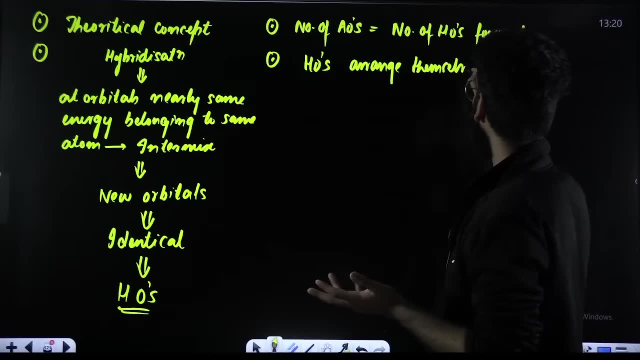 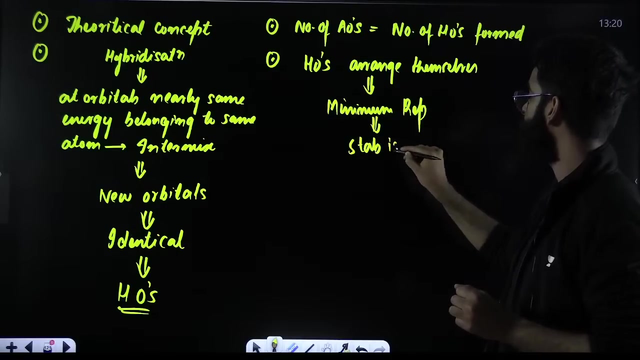 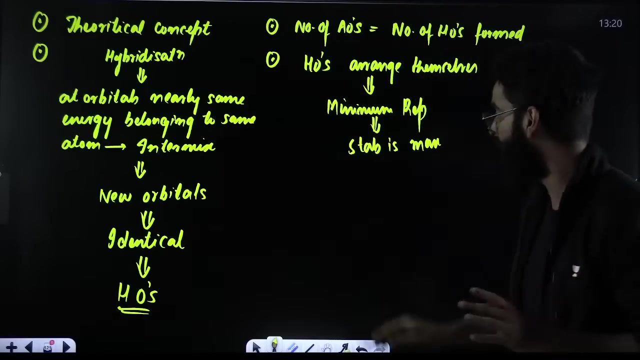 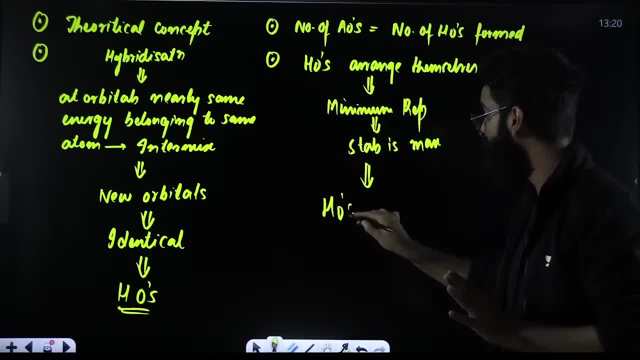 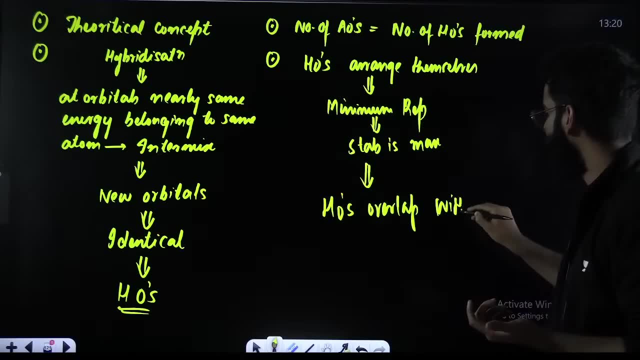 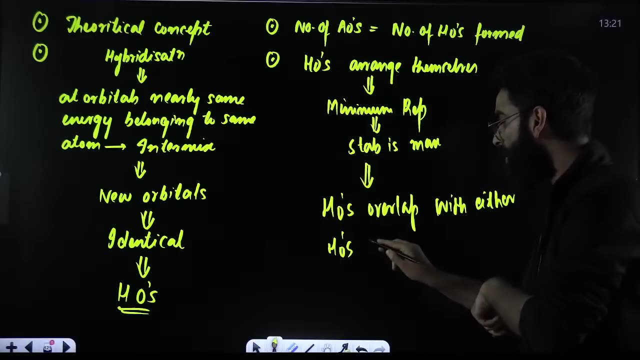 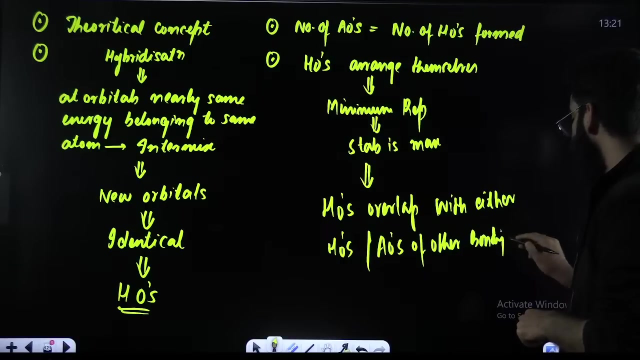 Then what happens? Then what happens? Then these hybrid orbitals overlap. Then these hybrid orbitals overlap with either the hybrid orbitals of other atoms or atomic orbitals of other atoms, of other bonding atoms. And remember, when hybrid orbitals overlap, they 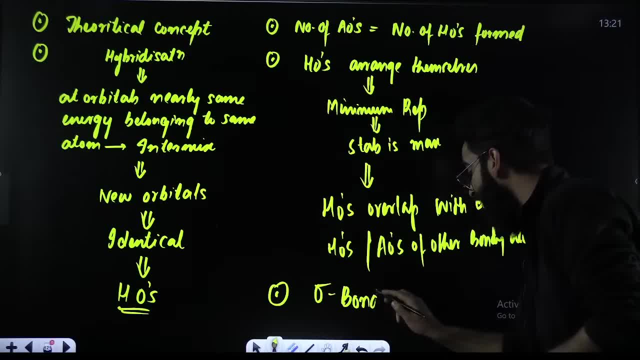 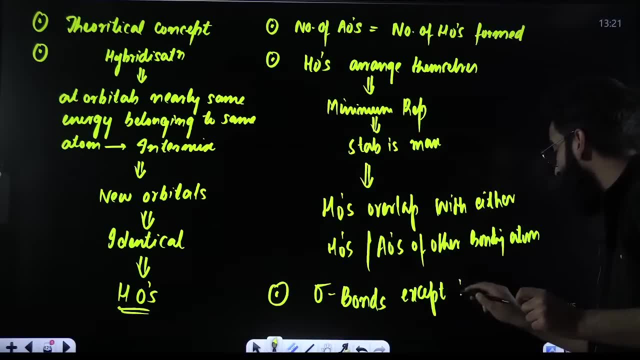 lead to the formation of sigma bonds. When hybrid orbitals overlap, they lead to the formation of sigma bonds. One exception, Except benzyne. In case of benzyne, hybrid orbitals overlap and lead to the formation of pi bonds. lead to the formation of pi bond. 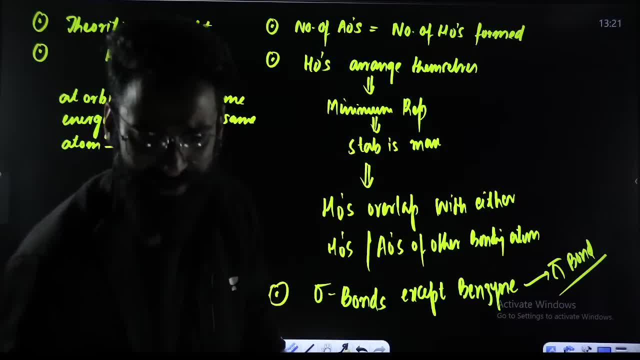 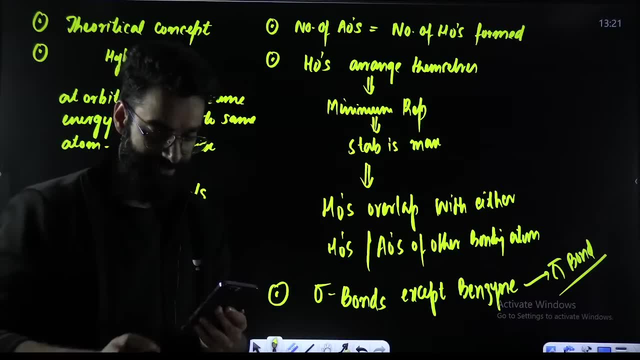 Is all this theory clear? This is the only theory which is required here. Now we are going to apply this theory. Now we are going to apply this theory. Now we are going to apply this theory. Yes, I believe this theory is clear till here. 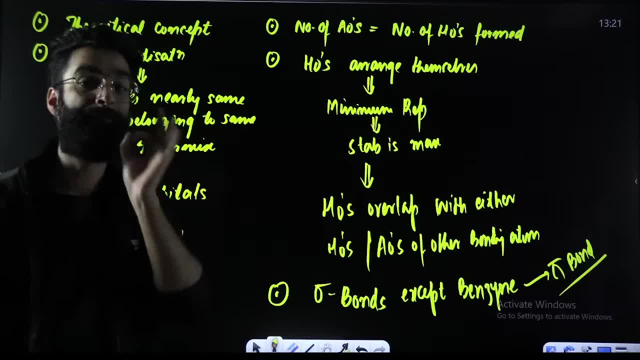 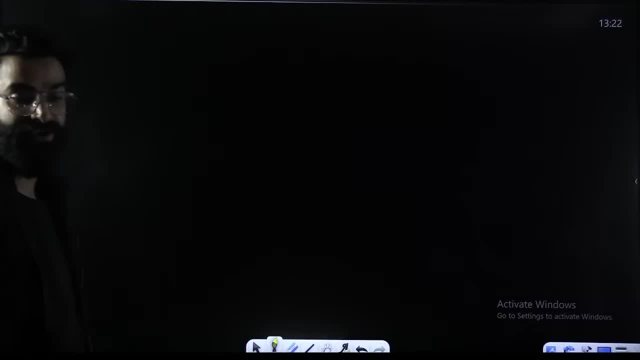 Okay, Now it is the time to apply the theory, But. but. but before applying the theory, you should know few things more. Then I will apply the concept. You will get to know how this hybridization is beneficial. 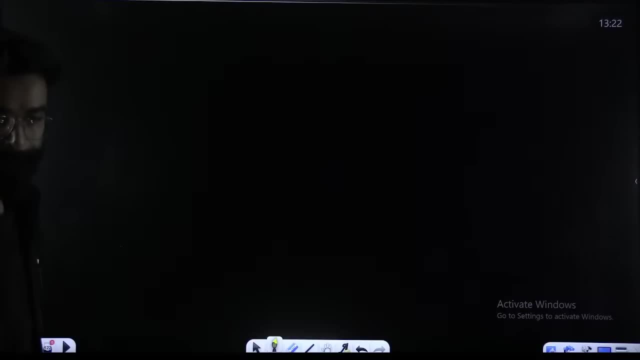 Right And what kind of things we get from it. Try to understand people. Hybridization: there is a method which I am going to define over here. That is steric number method. Steric number method is used to check the hybridization. Steric number method is used to check the hybridization. What is the steric number? Steric number is the number of sigma bonds plus the number of lone pairs. Steric number is basically the number of sigma bonds plus the number of lone pairs. 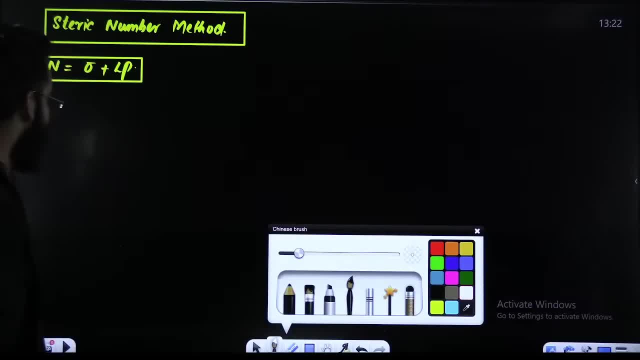 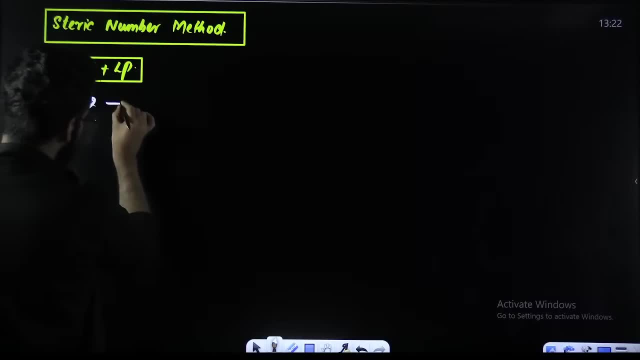 Plus the number of lone pairs. Right Now people try to understand. Try to understand If steric number comes out to be 2.. If steric number comes out to be 2. Hybridization involved is going to be sp. 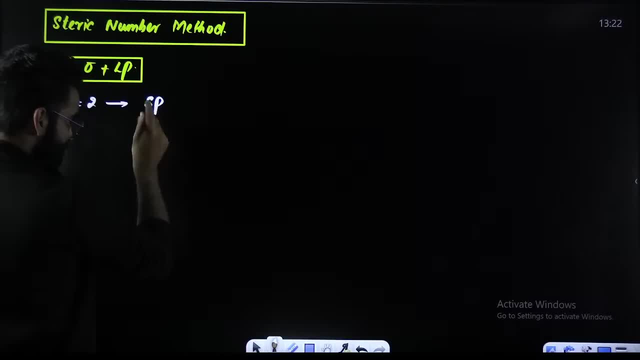 That means one of the s orbital and one of the p orbital have intermixed And they have led to the formation of two hybrid orbitals, Because two are intermixing, so two hybrid orbitals will get formed. Okay, And in case of sp hybridization, the geometry which is predicted through hybridization 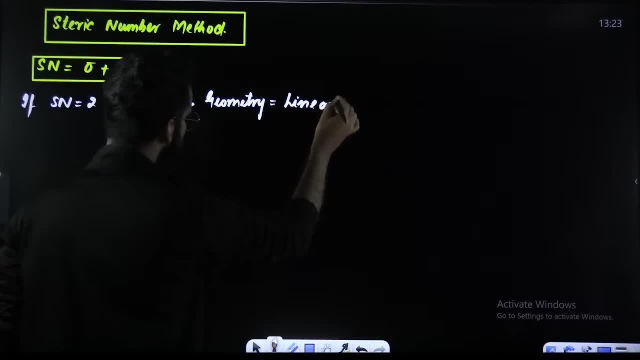 Linear, Linear. Linear Linear If steric number is 3.. Hybridization involved is sp2.. sp2. Right And the geometry involved, The geometry which is predicted through hybridization, That is planar, Triagonal planar. 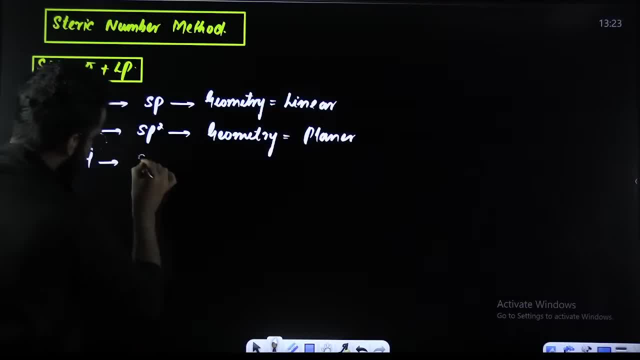 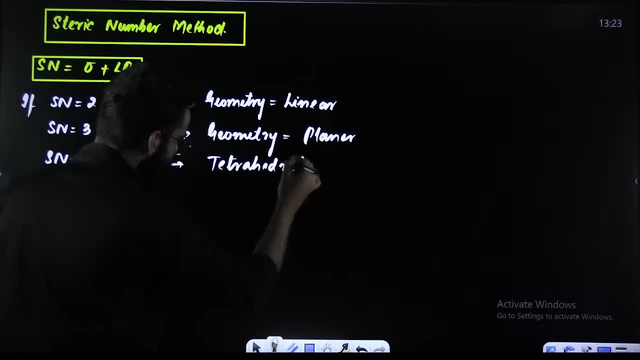 Triagonal planar. If steric number comes out to be 4.. Hybridization involved is sp3.. The geometry involved is tetrahedral. The geometry which is predicted through hybridization That is tetrahedral. Similarly, if the steric number is 5.. 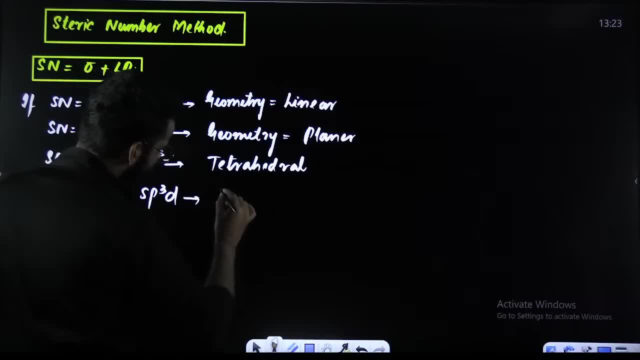 Hybridization is sp3d, The geometry involved, The geometry which is predicted through hybridization. That is what you call as trigonal bipyramidal geometry: Trigonal bipyramidal. Trigonal bipyramidal If steric number is 6.. 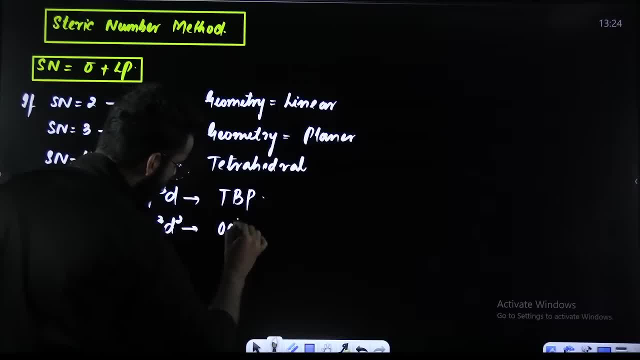 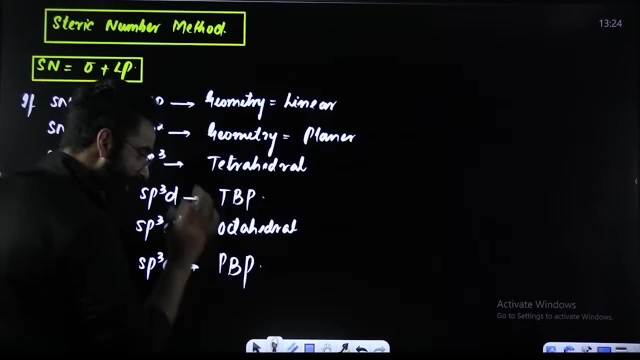 Hybridization involved is sp3d2.. Geometry involved is octahedral. Geometry involved is octahedral And if the steric number is 7.. The hybridization involved is sp3d3. And geometry predicted through hybridization is going to be pentagonal bipyramidal. 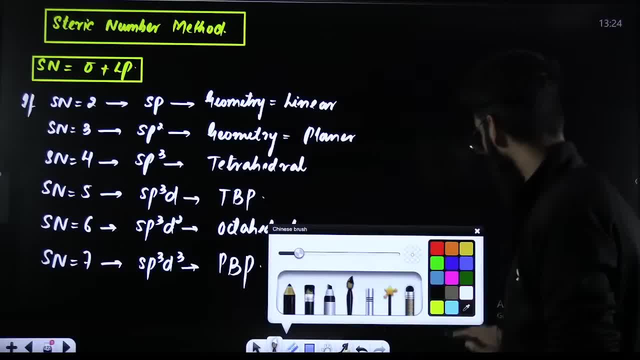 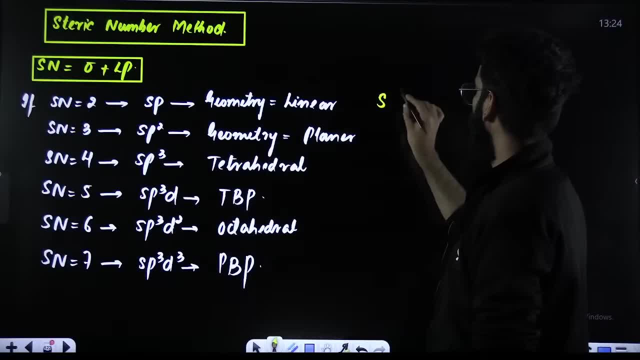 It is going to be pentagonal bipyramidal. It is going to be pentagonal bipyramidal. Now remember one more thing. Now remember one more thing. In case of sp hybridization, One of the s orbital and one of the p orbital. 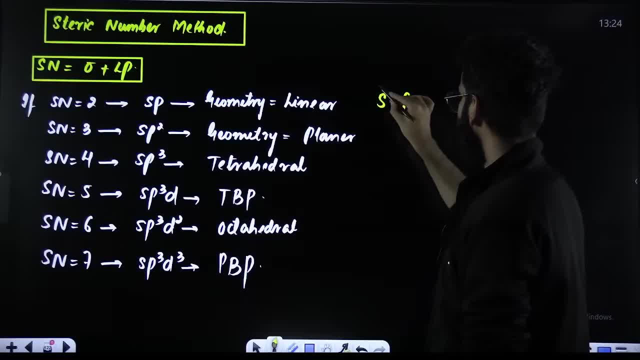 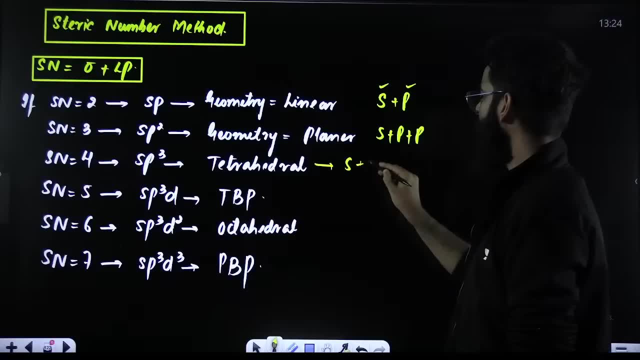 It can be either x or y or z, whatever Right, They have intermixed One of the s orbital, One of the p and one more p, Right sp2.. Over here s orbital, Your px, py and pz. 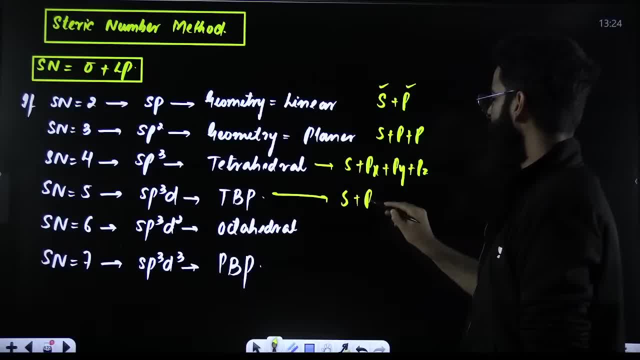 They have participated in the intermixing sp3d, One of the s orbital px py, pz and dz2.. They have participated in the intermixing s? px py, pz, px2-y2.. 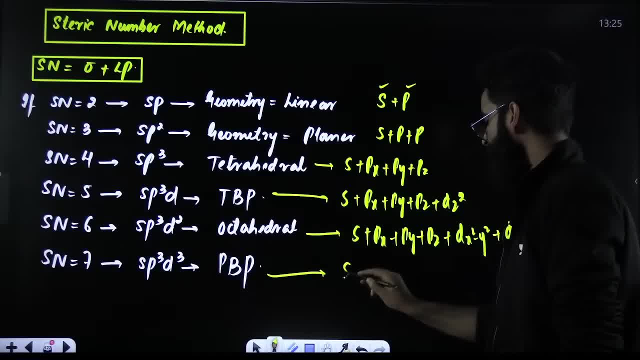 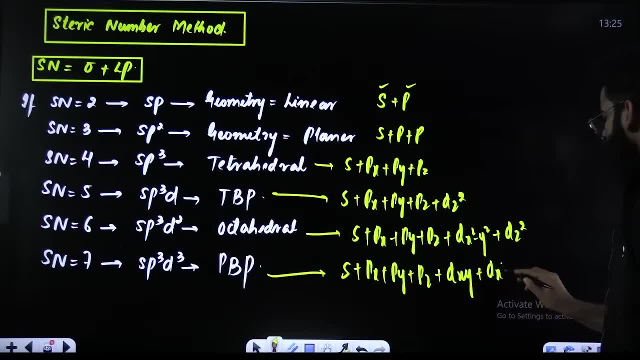 dz2.. Participate in the intermixing s: px, px, py, pz, pxy. dx2-y2. dz2.. They have participated in the intermixing: px, px, py, pz, pxy. 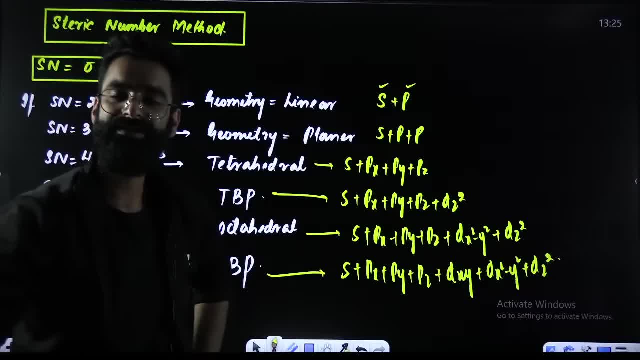 dx2-y2.. dz2. participated in the inter mixing. They have participated in the intermixing. These are the questions many times asks Which d orbital is? Which d orbital participates in sp3d? It is dz2.. Which d orbital participate in sp3d3. 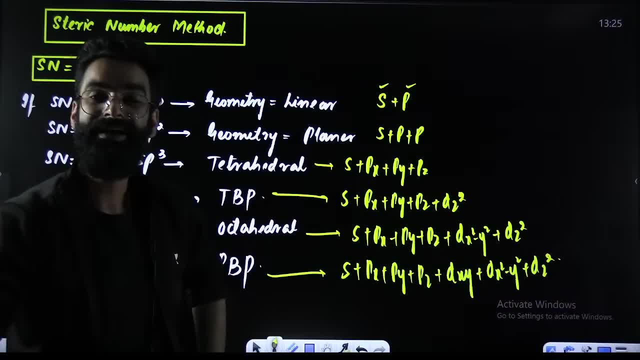 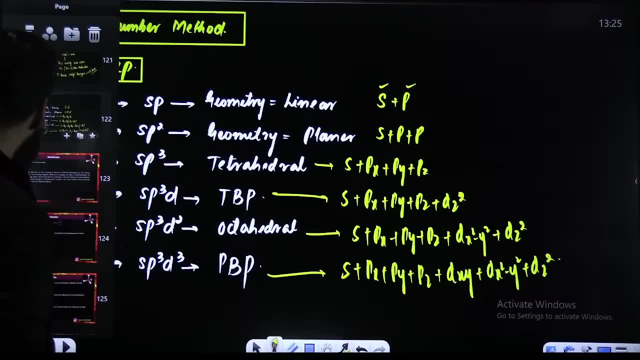 Right. Look at the d orbital. Which d orbital participate in sp3d2? 3D2.. You should know that. Okay, Now guys understand where and how we are going to introduce this concept of hybridization. Understand carefully what exactly I am going to talk. 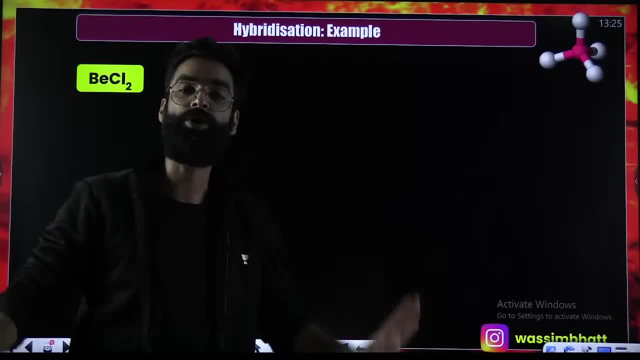 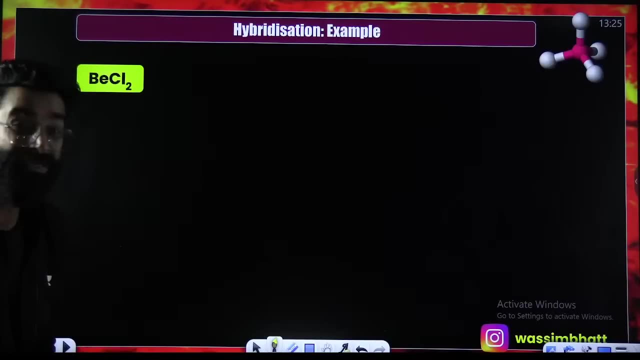 about. This is something super important, on which entire bonding is based, on Entire bonding. Try to understand The first molecule which I have taken over here. that is BECL2.. BECL2.. Try to understand BECL2.. The central atom is beryllium. over here, The central atom is: 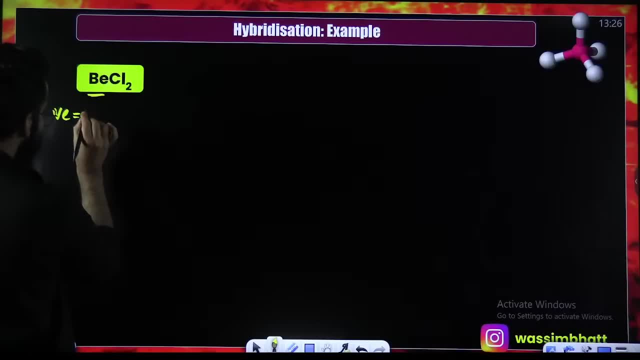 beryllium over here. If I ask you how many valence electrons beryllium has, Beryllium atomic number: 4. 2, 2. How many valence electrons it has? 2. Right, How many surrounding atoms are. 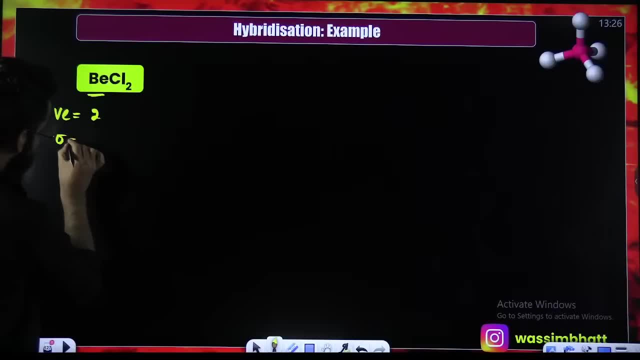 here There are two surrounding atoms. Do remember: the number of surrounding atoms is equal to number of sigma bonds. The number of surrounding atoms is equal to number of sigma bonds. Now, beryllium had two valence electrons. Beryllium had two valence electrons And both these valence. 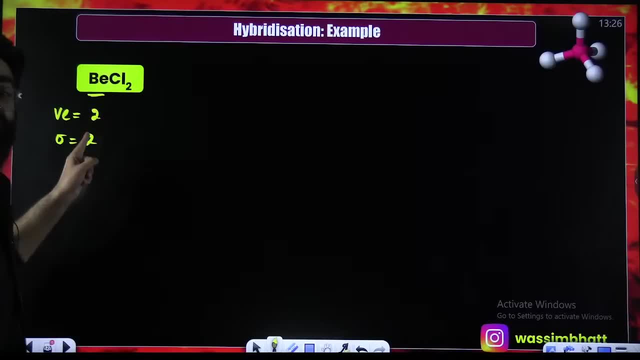 electrons of beryllium have been used to form two sigma bonds. Both these valence electrons of beryllium have been used to form two sigma bonds. That means: will there be any lone pair on beryllium? There will be no lone pair. Right Beryllium had two valence electrons. 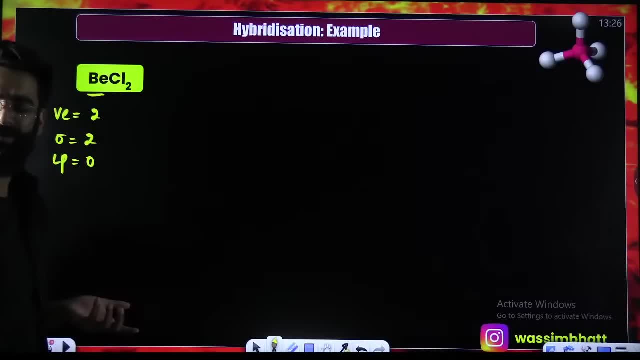 and all these valence electrons have participated to form two sigma bonds. So there will be no lone pair on beryllium If there is no lone pair. if I ask you, what is the steric number? Steric number is sigma plus lone pair. So 2 plus 0 is 2.. 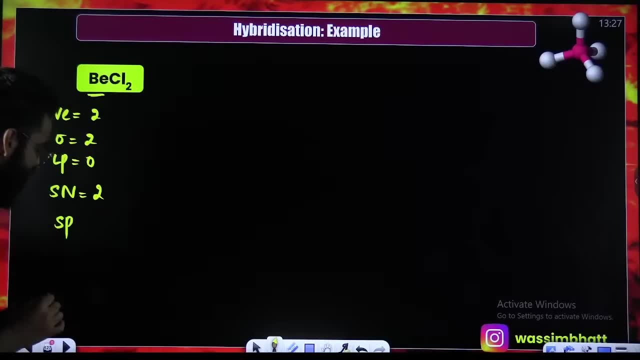 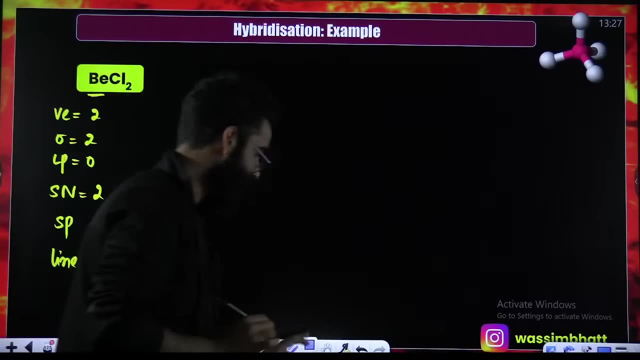 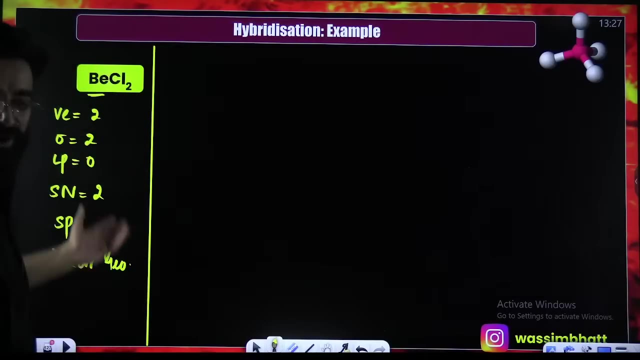 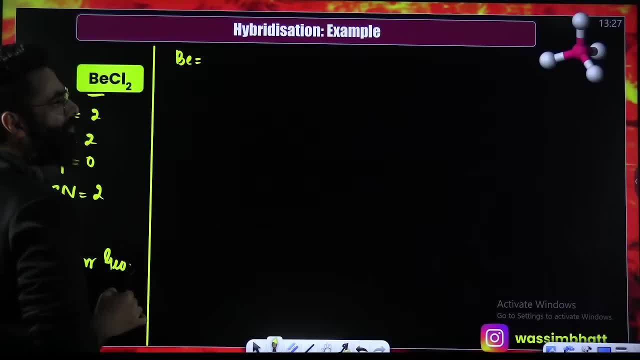 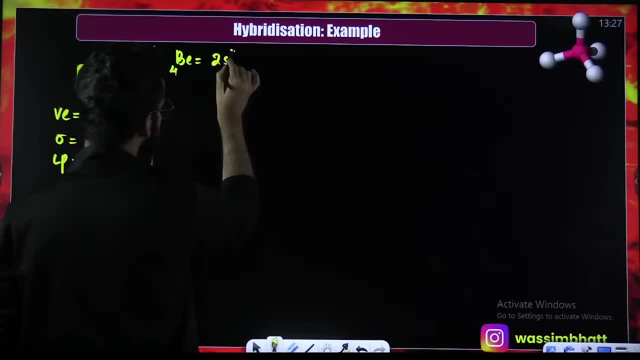 If I talk about beryllium, what about the outermost configuration of beryllium? Beryllium has got atomic number 4, hydrogen lithium lithium, It has got atomic number 3, hydrogen term number 4.. So outermost configuration is 2s2- 2p0.. This is the outermost configuration. 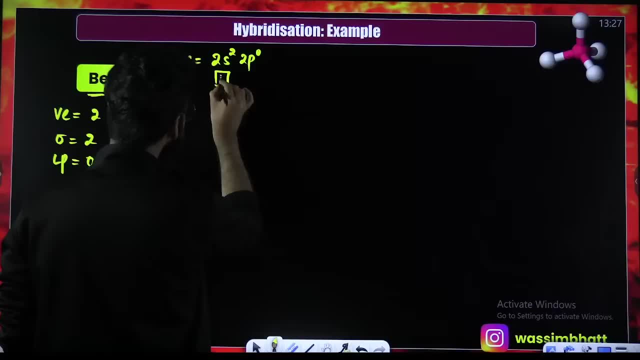 But people, if I ask you, is this the ground state configuration? Yes, this is the ground state configuration of beryllium. This is the ground state configuration of beryllium. If I make the excited state of beryllium, what is going to happen? This electron, one of the electron, will shift here. 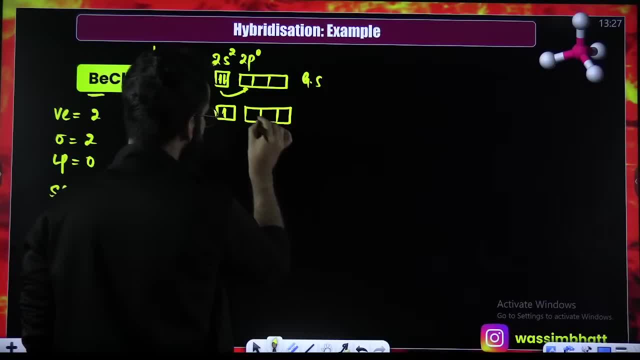 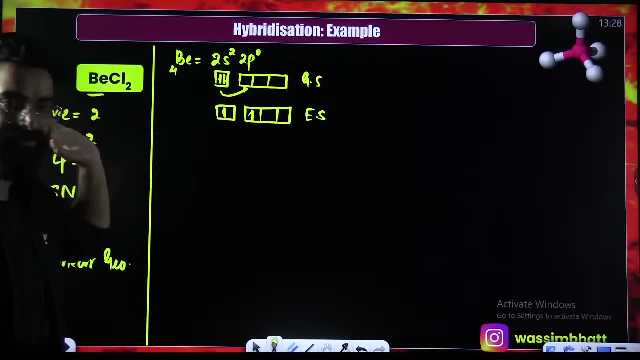 and it's going to be one here, Right? This is the excited state of beryllium. This is the excited state of beryllium. This is s, this is p, containing one electron. Now which which hybrid addition is involved, sp. So, this s and this p, they are going to involve in the 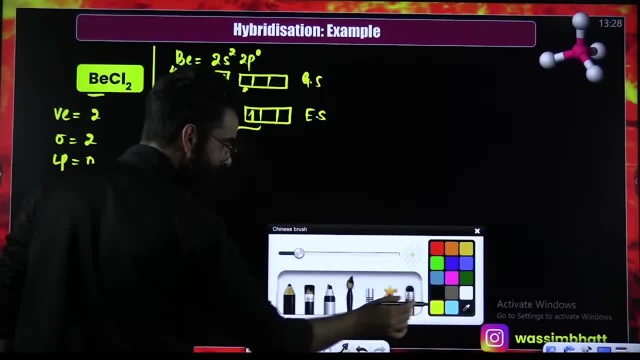 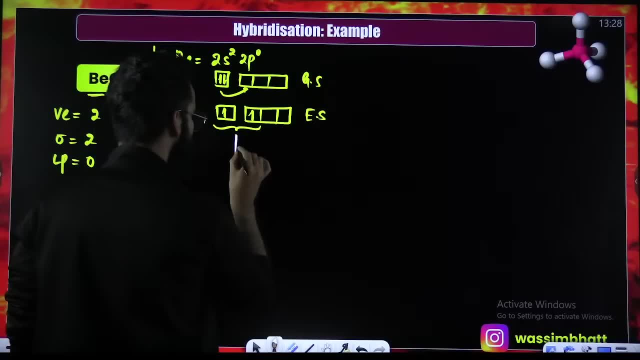 intermixing And when they get involved in the intermixing. since two atomic orbitals are participating in intermixing, so two hybrid orbitals will get formed, Two hybrid orbitals. So there has been sp intermixing and two hybrid orbitals will get formed over here. 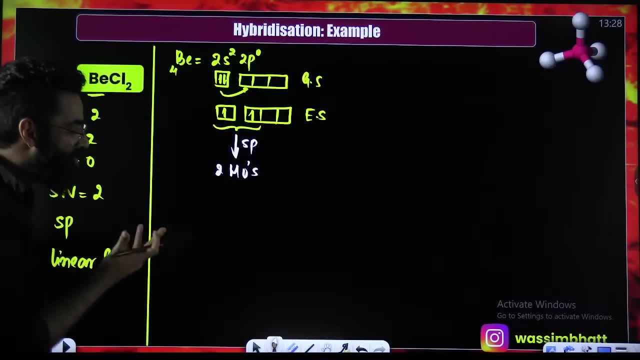 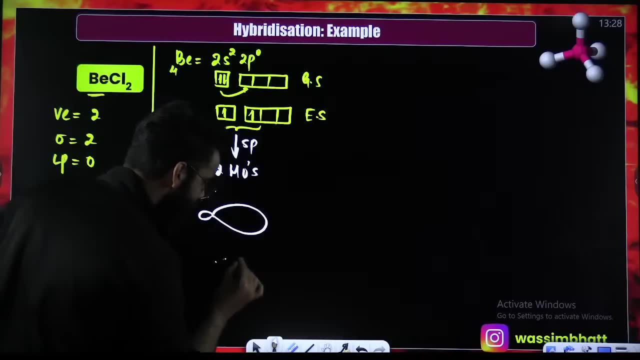 Two hybrid orbitals will get formed over here. How, What is the shape of these hybrid orbitals? One lobe is made bigger in size and the lobe is made smaller in size. So these are the two hybrid orbitals which got generated over here, And 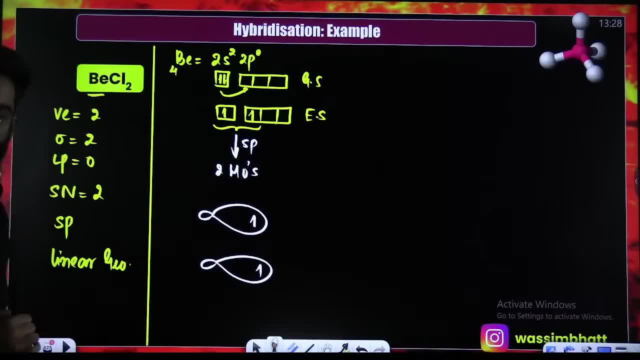 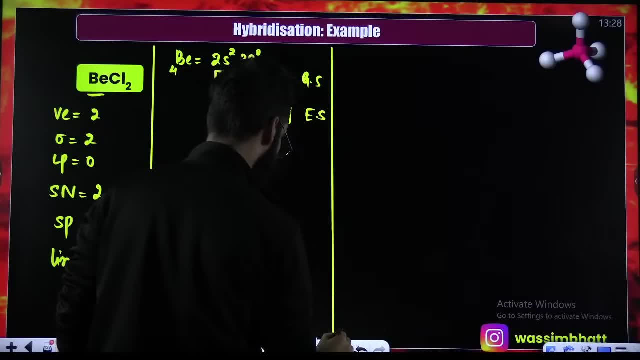 these hybrid orbitals, they'll be containing one electron each. Okay, Now, once these hybrid orbitals are made, once these hybrid orbitals are formed, once these hybrid orbitals are formed, now, these hybrid orbitals, they are going to arrange themselves in such a way that there are 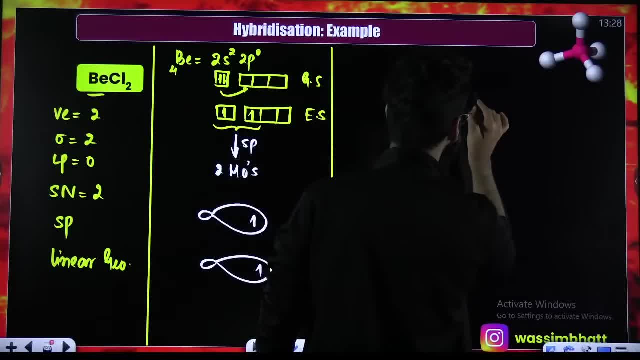 minimum repulsions between them. Now you think How they are going to arrange themselves. If this is one hybrid orbital containing one electron, right, This is going to be one more hybrid orbital containing one more electron. Perfect Hybrid orbitals. they have arranged themselves in such a way that there are minimum repulsions. 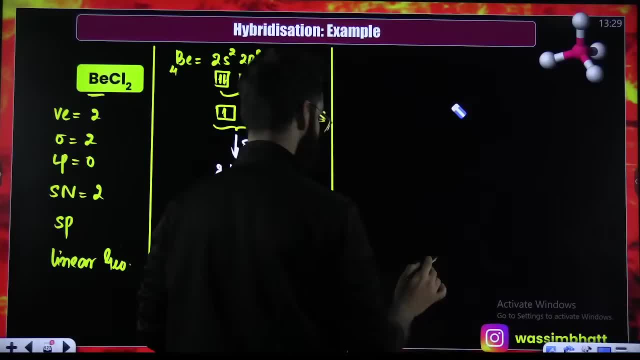 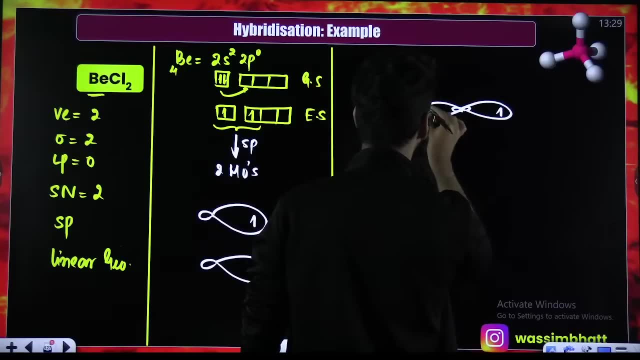 between them. Let me make them properly. Just a second, Let me make them properly. This is one of the hybrid orbital containing one electron and one more hybrid orbital containing one more electron. Okay, Perfect, Now people understand. Beryllium has to form bonds with chlorine. 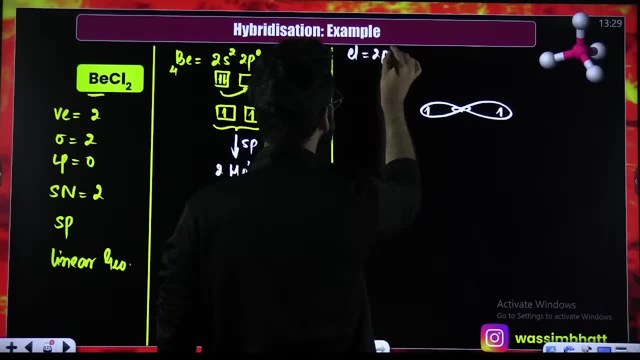 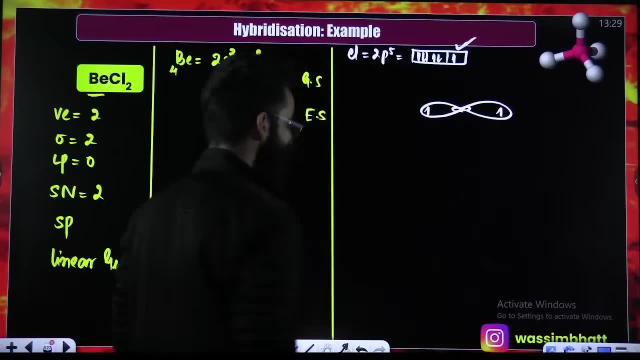 Right, If I ask you about the outermost configuration of chlorine, it is 2p5.. It is 2p5.. Right, It is one, two, three, four and 5.. This is the unpaired orbital, The unpaired orbital of chlorine. 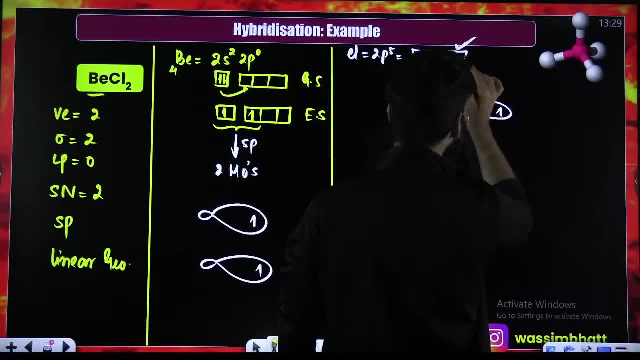 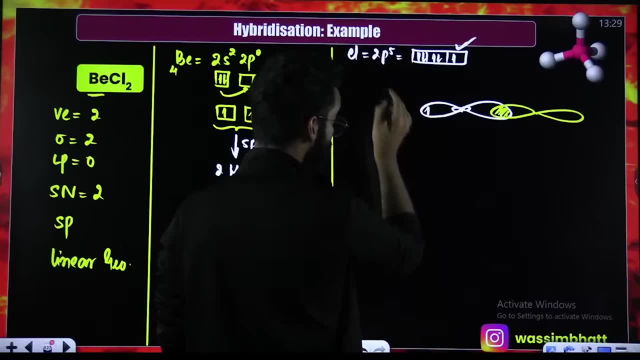 the unpaired orbital of chlorine, which is the p orbital. it will come from this side, Will show the overlap. One more, chlorine, will come from this side. Its p orbital and it will show the overlap. If I ask you which overlap is the p orbital? 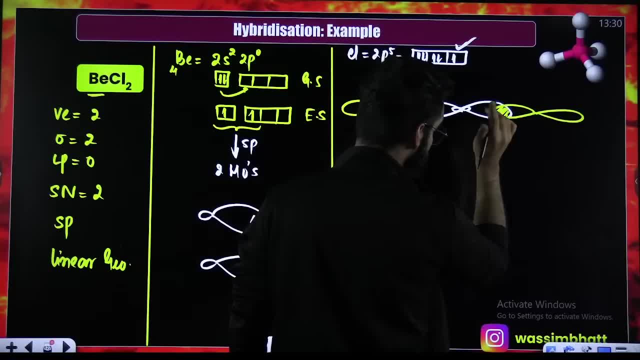 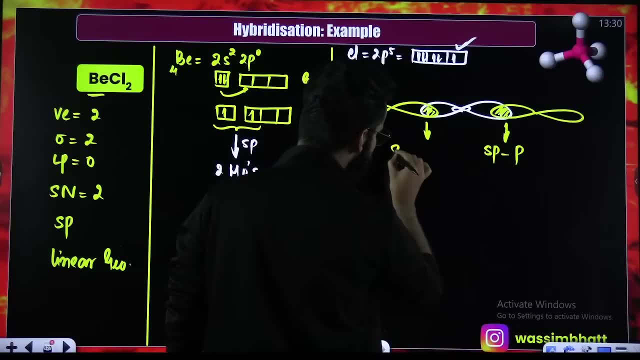 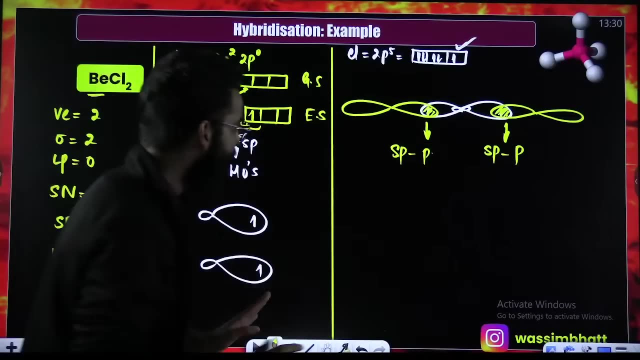 this is Which overlap this is. First of all, it's a head-on overlap between sp hybrid orbital of beryllium and pure p orbital of chlorine. Similarly, sp hybrid orbital of beryllium and pure p orbital of chlorine. Was the overlap head-on? Yes, the overlap is head-on And due. 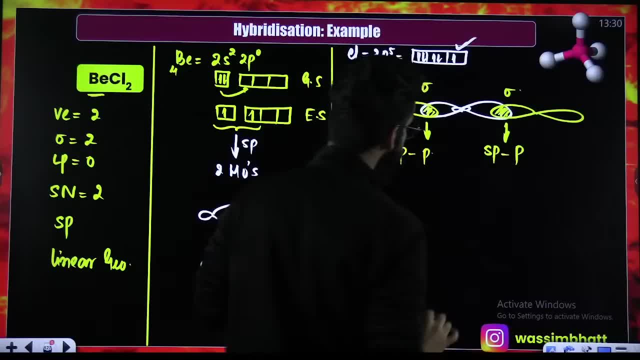 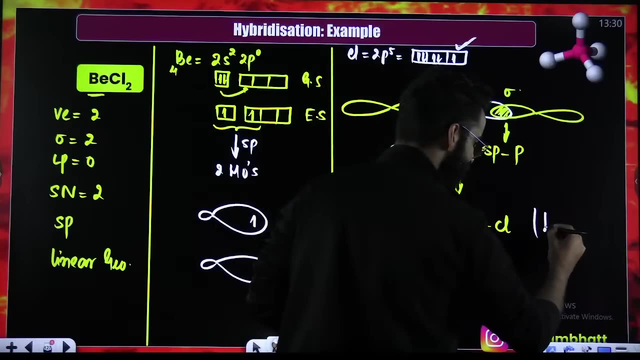 to head-on overlap. I would say: sigma bond got formed, Sigma bond got formed. So if I show it at the end, this is beryllium. There is one chlorine from this side, one chlorine from this side right. This geometry is something which you call as linear geometry, Linear geometry, right. 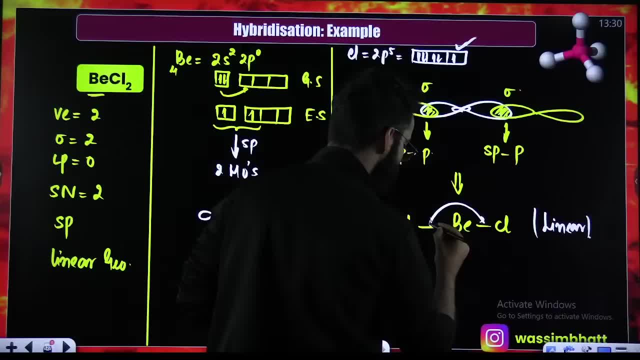 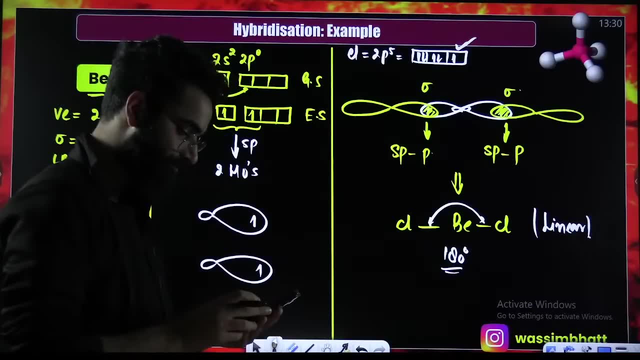 Linear geometry. If I ask you what is the bond angle here? Absolutely, you should say it. It's 180 degree, Perfect. Am I clear to everyone, Quickly, people. Am I clear to everyone? Quickly, people, Quickly people. 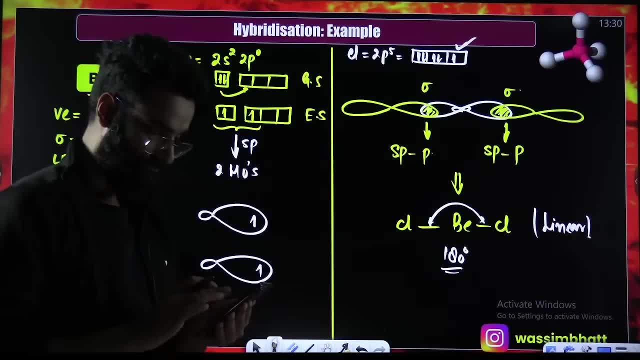 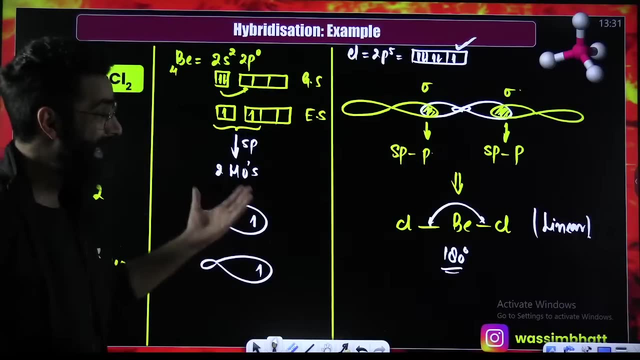 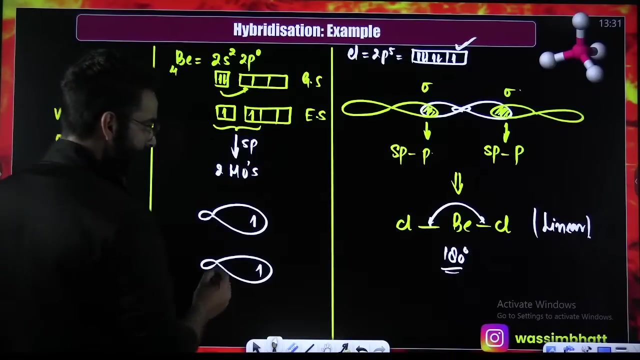 Quickly people, Quickly quickly. Everyone in the chats. Everyone in the chats. Yes, So this was your sp hybridization. This was your sp hybridization. Now, guys, there is one more question which is asked, If they ask you, in these sp hybrid orbitals, since this sp hybrid orbital, 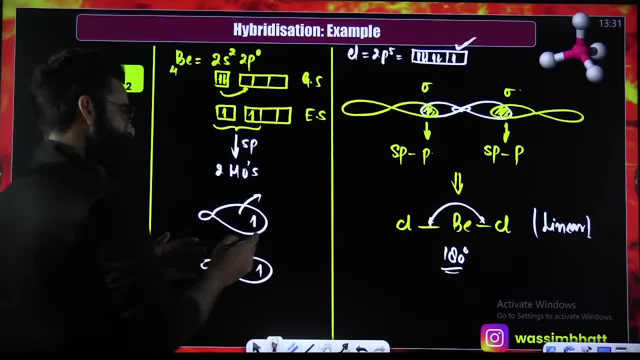 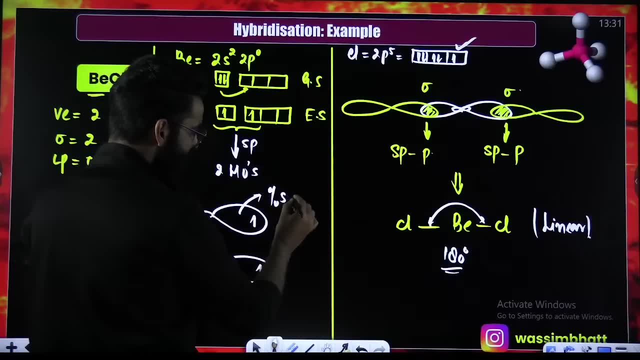 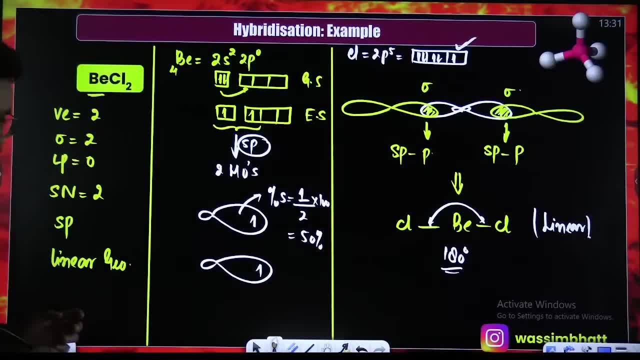 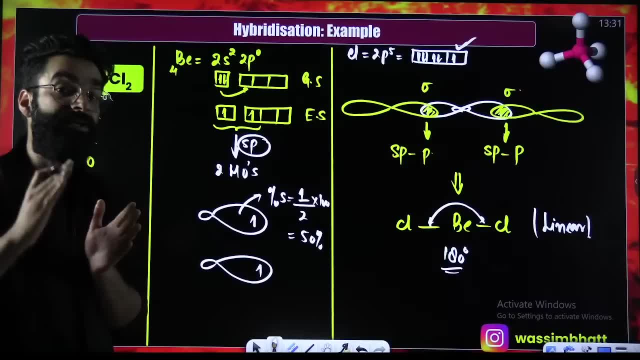 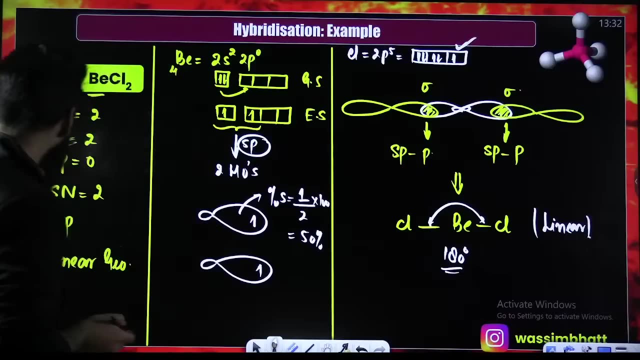 right here. So what are these? first number of these poles, The sp-ps moc. Okay, So if So, sp hybrid orbital will have equal characters of s orbital and p orbital. Am I clear? Am I clear, people? Let me take one more example. 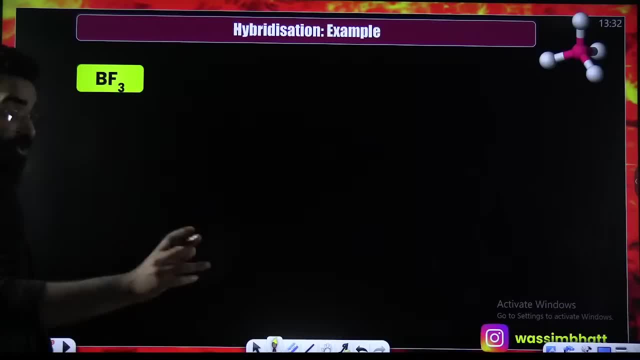 Let me take one more example. Look at this particular example Now. you are going to write everything in the charts. You are going to write everything in the charts Over here. the central atom is boron. How many valence electrons boron has? 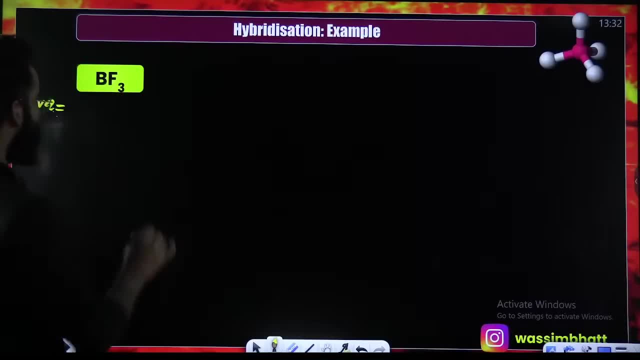 How many valence electrons? boron has Quickly Atomic number: 5. 2,3.. 3 valence electrons. How many surrounding atoms? 3 surrounding atoms. Number of surrounding atoms is equal to number of sigma bonds. How many lone pairs? 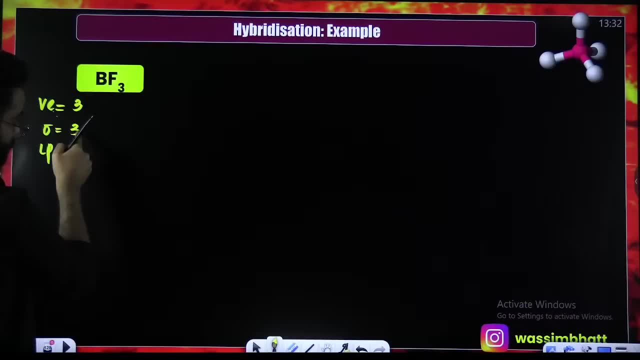 There were 3 valence electrons and all the 3 have been used for 3 sigma bonds. So no lone pair Stereic number: Sigma plus lone pair 3 plus 0 is 3.. Right Hybridization involved. 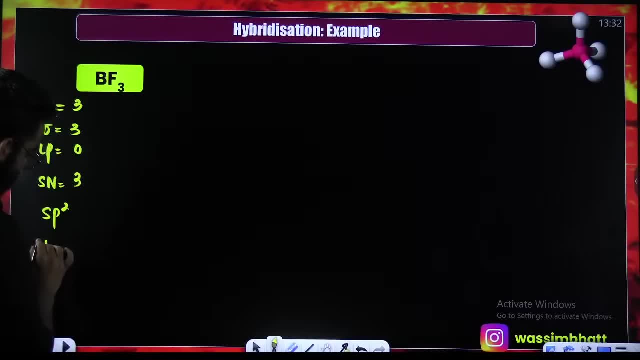 sp2.. Right Geometry, predicted through hybridization, That is, Triagonal planar. This is something which I concluded till now. This is something which I concluded till now. Now comes a point: How the formation has taken place, How the molecule will look like exactly. 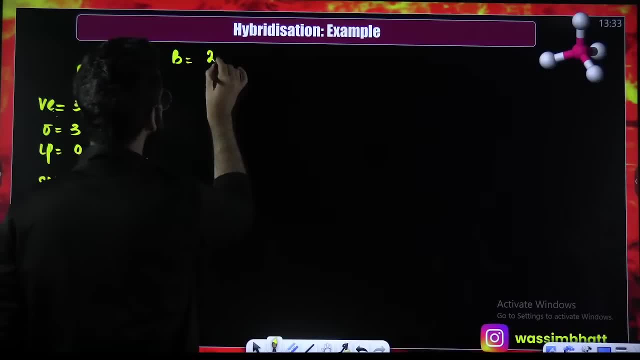 If I talk about boron, its outermost configuration is 2s2- 2p1.. 2s2- 2p1.. So 2 electrons here, and in case of p there is 1 electron. This is the ground state. 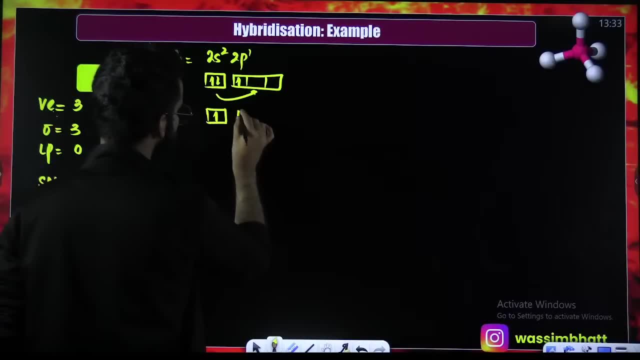 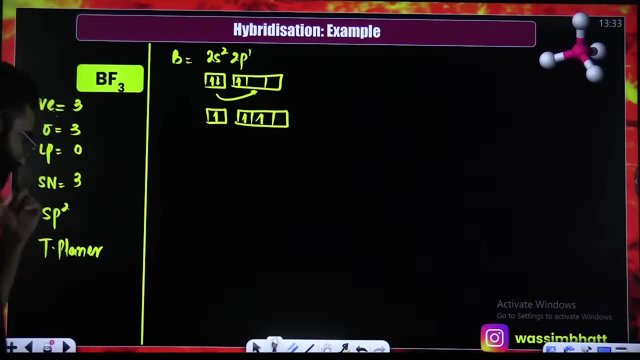 Now make the excited state. When you make the excited state, there is 1 electron here, Right, And people, there is 1 here, 1 here. This is the excited state. Now which hybridization is taking place over here, sp2.. 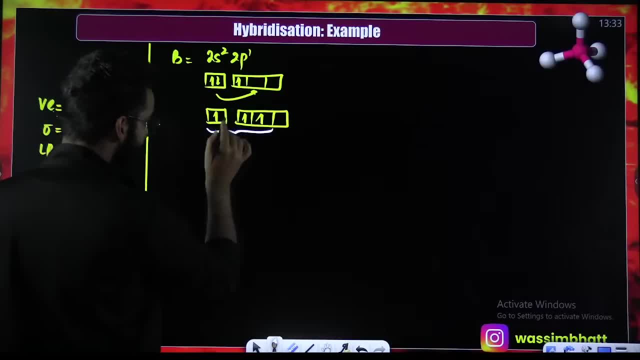 So this s and these 2p orbitals will start intermixing. And since 3 atomic orbitals are intermixing, So 3 hybrid orbitals will get formed. 3 hybrid orbitals will get formed Right. 3 hybrid orbitals will get formed. 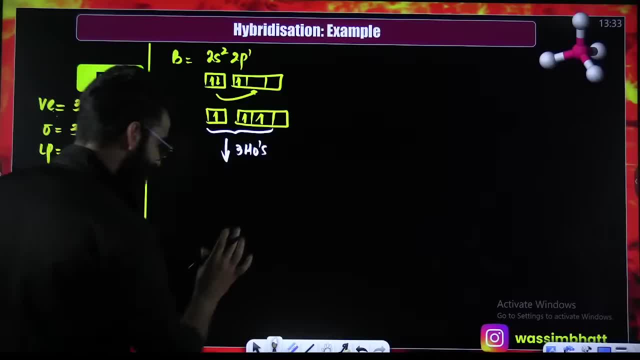 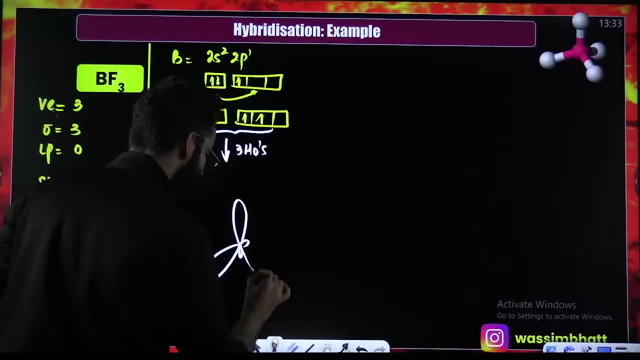 Perfect, Now those 3 hybrid orbitals. they will arrange themselves in such a way that there are minimum repulsions between them. So this is one of the hybrid orbital, This is one more hybrid orbital. And this is one more hybrid orbital. 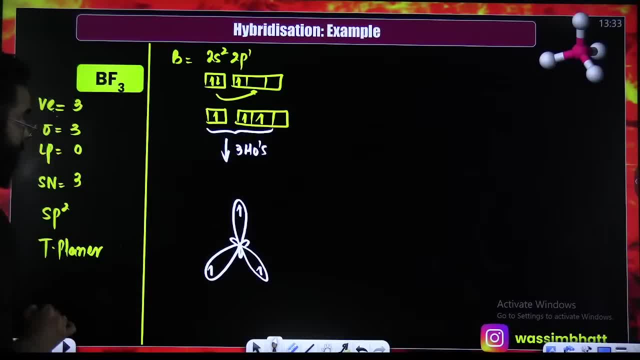 And all the hybrid orbitals are containing 1,1 electron each. Okay, Now boron has to form bond with fluorine. Fluorine's configuration is 2p5.. Right, This is 3p5. Sorry, Okay. 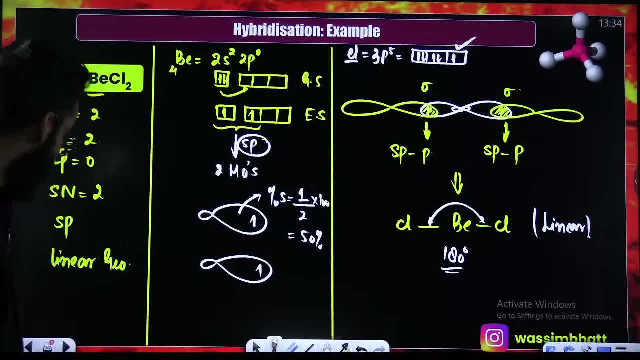 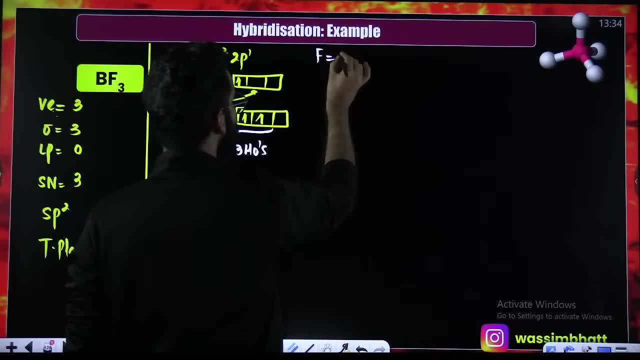 This is 3p5 in case of chlorine, Mistakenly I wrote 2p5.. Right, Okay, Perfect. Now boron has to form bonds with fluorine. If you talk about fluorine, fluorine configuration is 2p5. 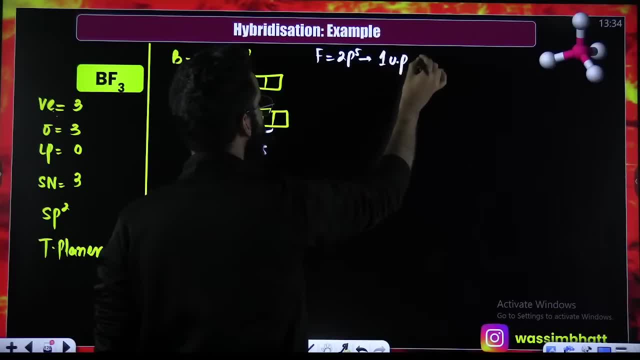 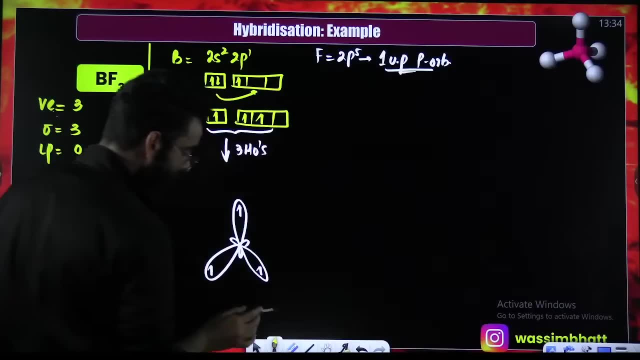 2p5.. In 2p5 there is one unpaired p orbital, One unpaired p orbital. So I would say, I would say I would say one of the p orbital of fluorine will come from this side and will show the overlap. 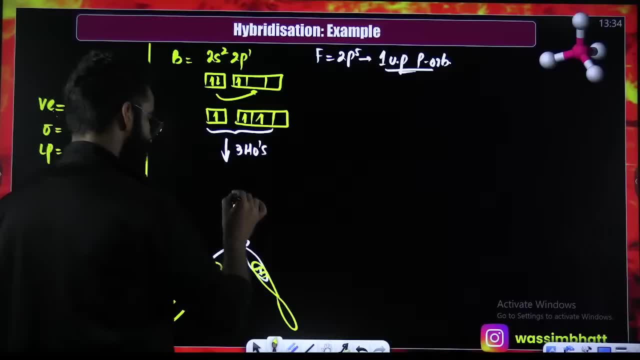 Right. One more will come from this side, will show the overlap. One more will come from this side, will show the overlap. Which overlap this is All. these overlaps are basically head on overlaps. Right, This is basically your overlap between. 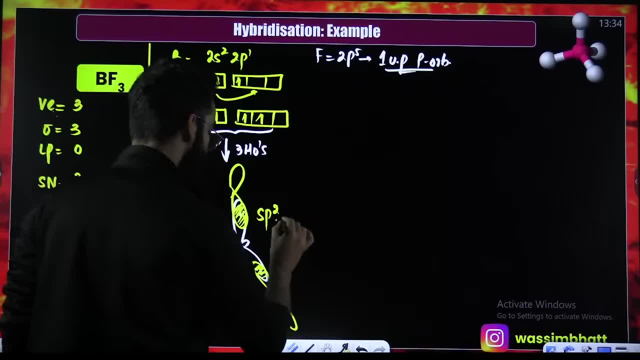 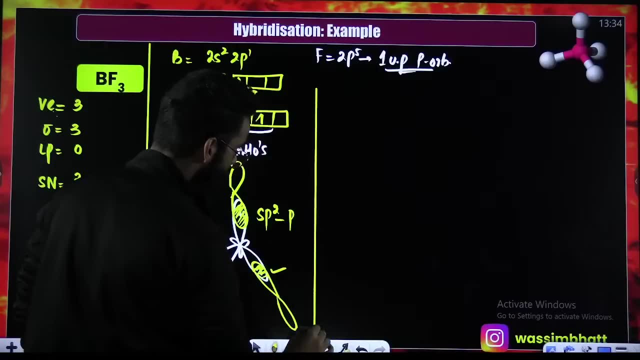 Sp2 hybrid orbital of boron with pure p orbital of fluorine. This is again the same. This is again the same. How do I represent it at the end? How do I represent it at the end? So, boron, this is fluorine, this is fluorine and this is fluorine. 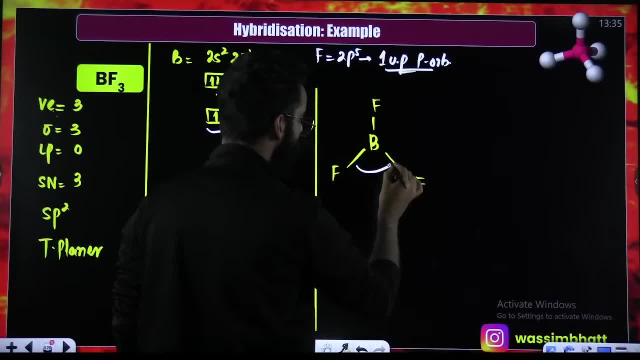 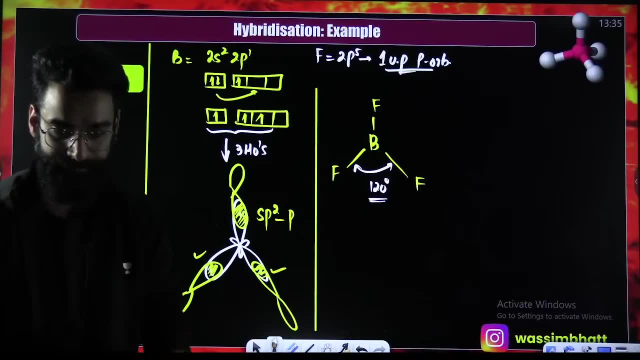 This particular geometry is what you call as trigonal planar geometry, And over here, over here, the angle is 120 degree. If I am clear, let me know once in the chats Done, Done industry people, Is it clear? 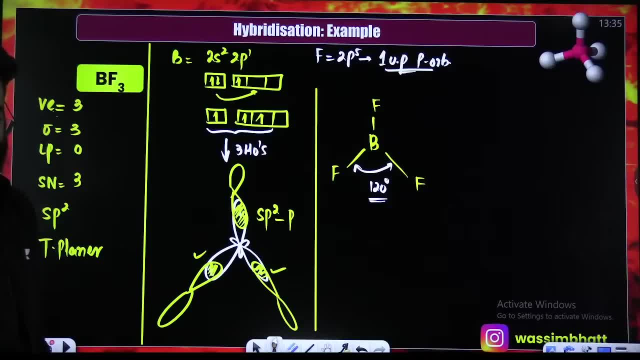 Is it clear? Quickly, Quickly, guys. Now I do not need to show all these stuff here again and again. Okay, I hope this particular part is clear. Right, This particular part is clear. Now I am directly showing you the example that I am using. 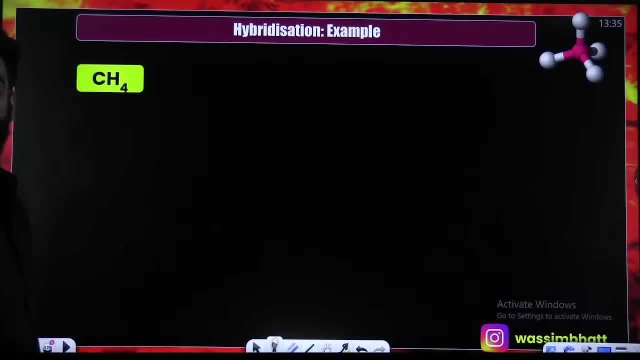 Okay, I am directly showing you the examples. Right, I am directly showing you the examples. You just need to tell me the hybridization, etc. etc. Okay, Carbon, How many valence electrons? 4. How many surrounding atoms? 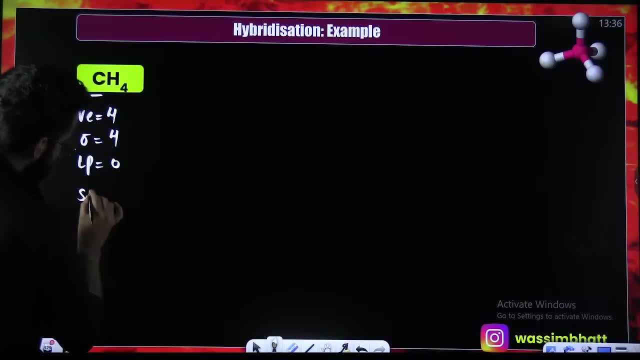 4. How many lone pairs: 0. Steric number 4 plus 0?. 4. Hybridization, Sp3.. Geometry which is predicted through hybridization. That is tetrahedral. If it is tetrahedral, tetrahedral looks like this: 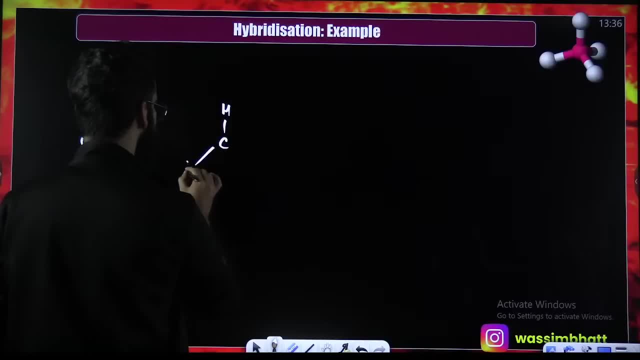 This is C, This is H, This is H, This is one more H, This is one more H. The bond angle over here is 190 degree. Okay, Okay, Okay, Okay, Okay, Okay. Hybridization is 109 degree, 28 minutes. 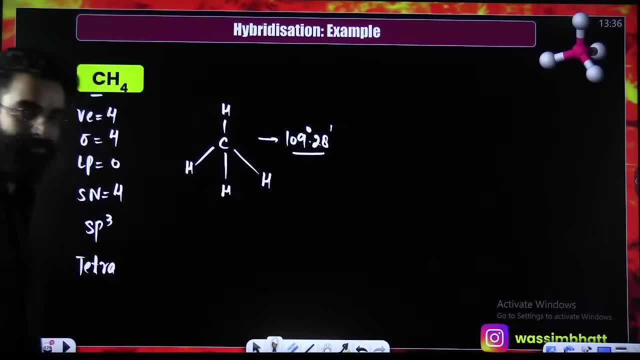 Perfect. Now, now I am asking you a question. I am asking you a question. Take any of the bond, Any of the bond. Take this bond. Can you tell me This bond has got formed by what kind of overlap? What is the overlap happened there? 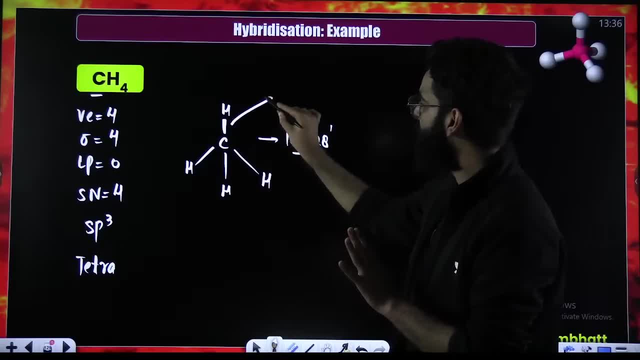 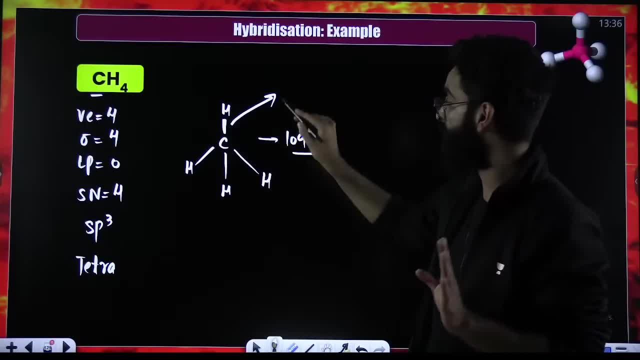 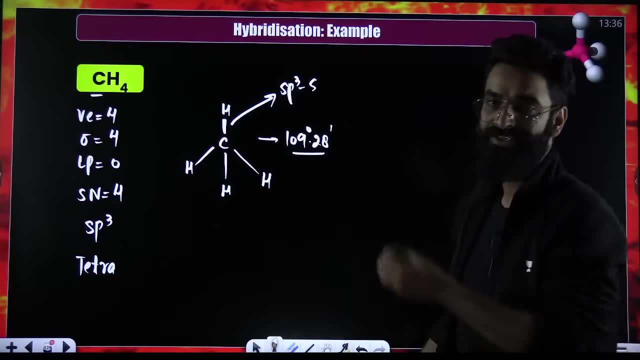 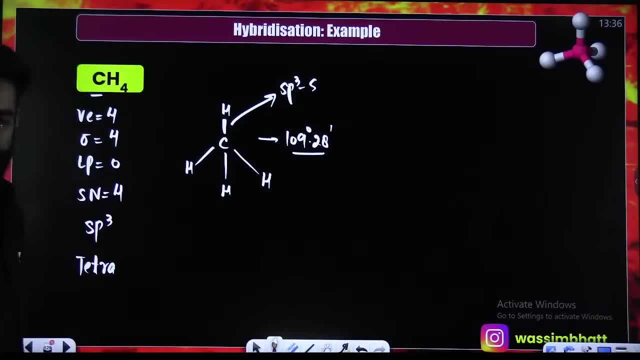 Sp3s. All the bonds are not the same. All the bond lines in case of CH4 are supposed to be same, Which are same actually? Right, Perfect, Perfect, guys, Perfect, Okay, Pcl 5.. Pcl 5.. 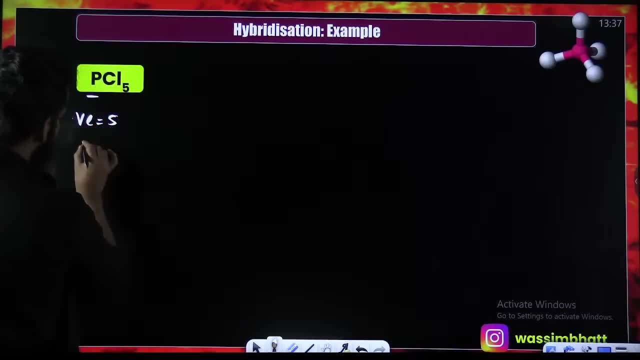 Pcl 5.. Phosphor is the central atom. How many valence electrons, Five Surrounding atoms, Five Lone pairs on phosphors, Zero Steric number Five: Hybridization: Sp3d Geometry- predicted hybridization. 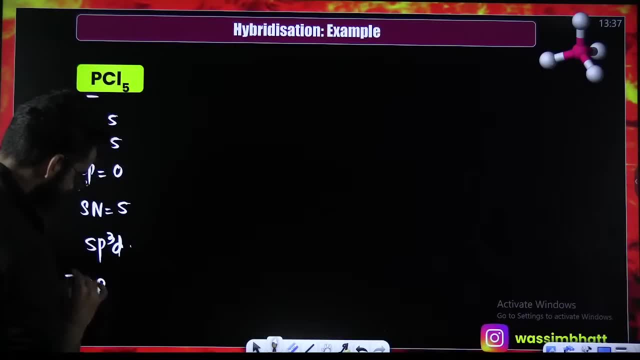 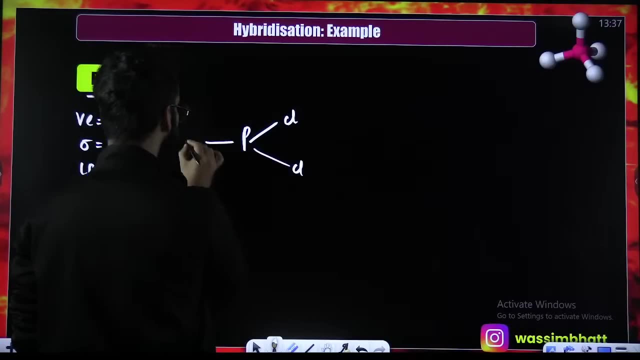 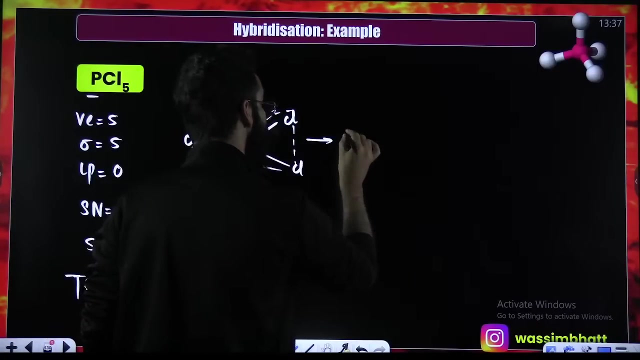 Triangular biperymetal. Now how it looks like this is P, one chlorine, one more chlorine and one more chlorine, and these three chlorine atoms, including phosphorous, these three chlorine atoms, including phosphorous, they are present on one plane. they are present on one plane, which is what you call as equatorial. 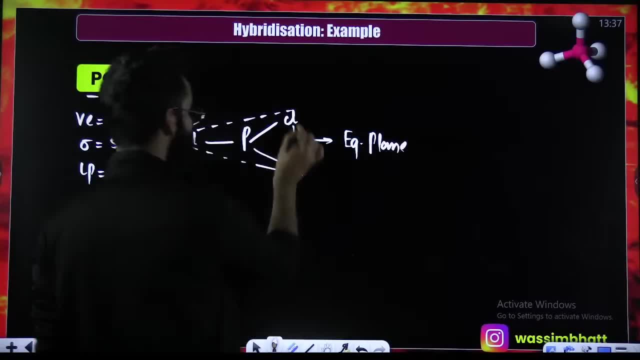 plane, This plane containing phosphorous and these three atoms, this plane is called as equatorial plane. Now, perpendicular to the plane upwards, perpendicular to the plane upwards, there is one more chlorine. perpendicular to the plane downwards, there is one more chlorine. and these two bonds, which 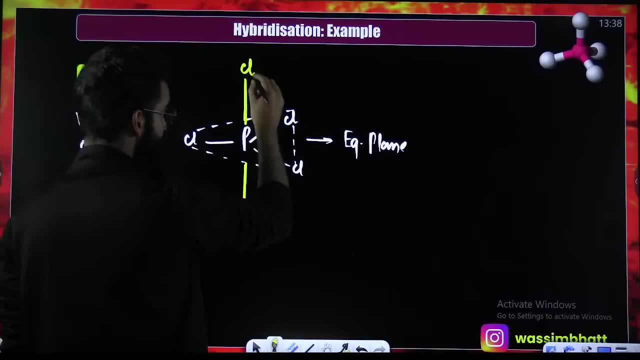 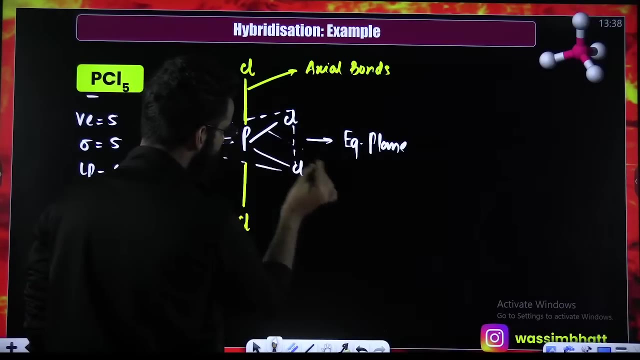 I have shown with yellow colour. these are what you call as axial bonds. All the bonds which are present on the equatorial plane, those are what you call as equatorial bonds, For example, this one. this one is what I call as equatorial bond. 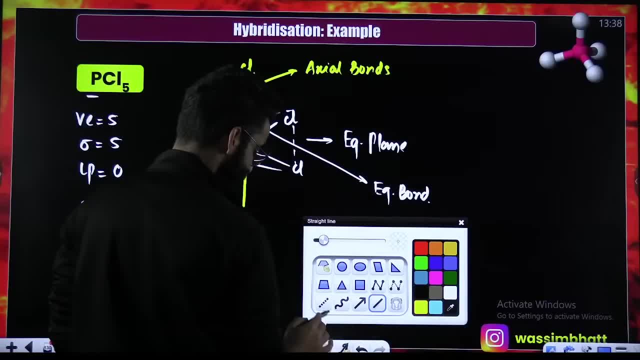 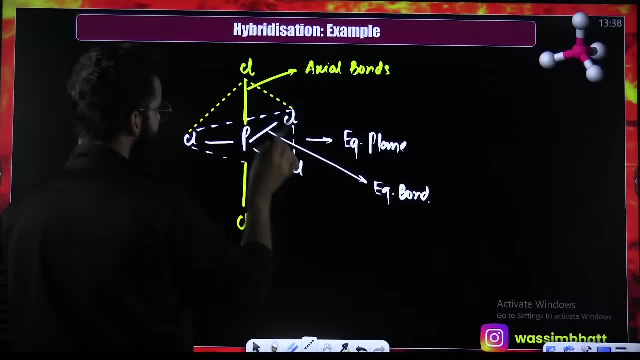 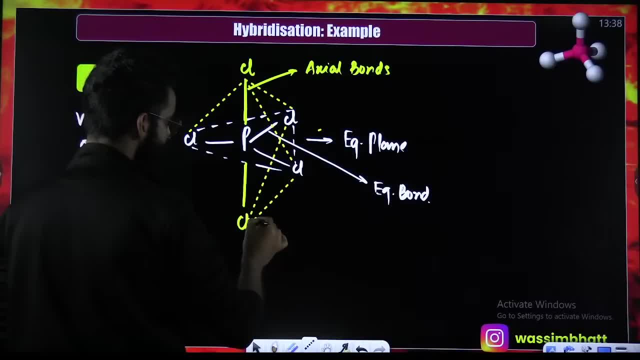 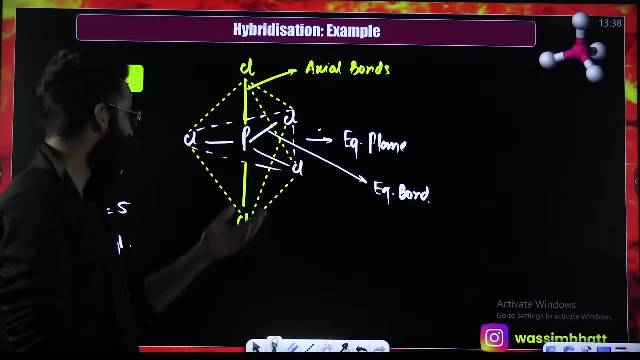 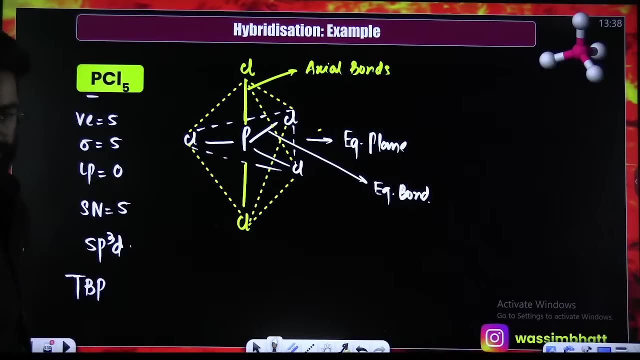 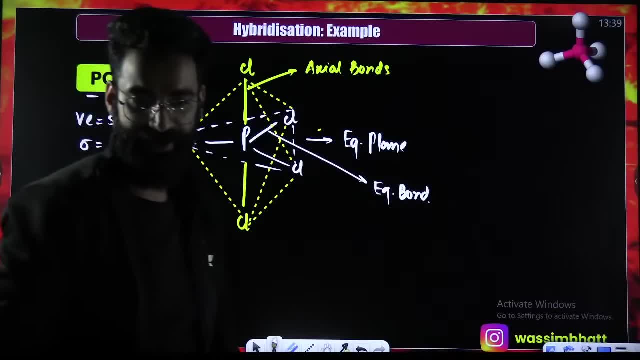 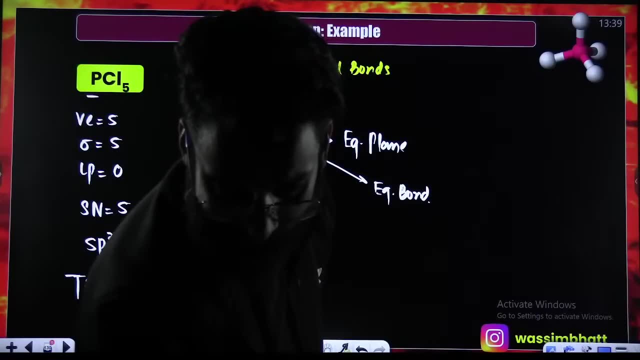 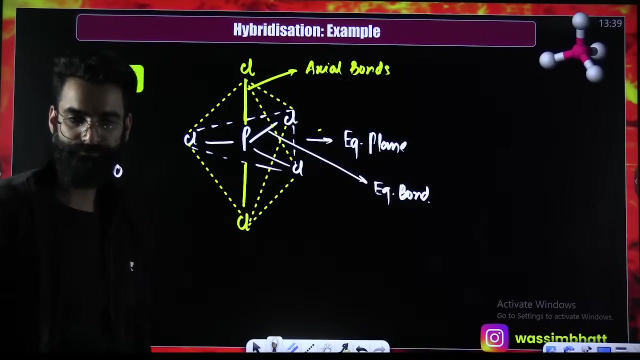 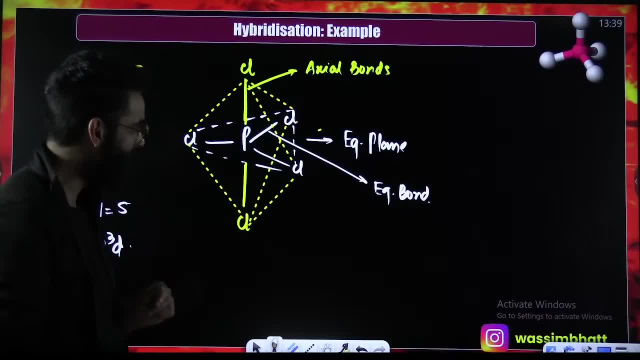 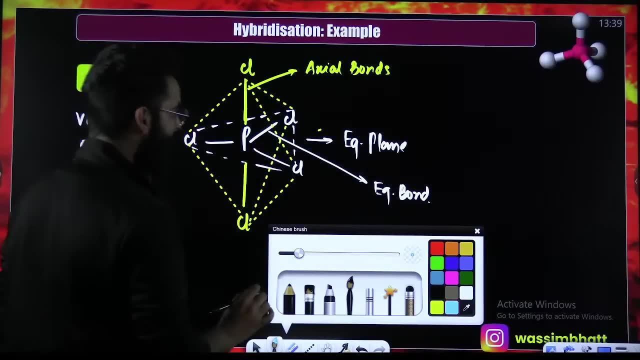 Okay, If I ask you one question here, think over it and let me know. think over it. Can you tell me what is going to be the bond angle in the equatorial plane? So basically I am asking you: what is the angle between? 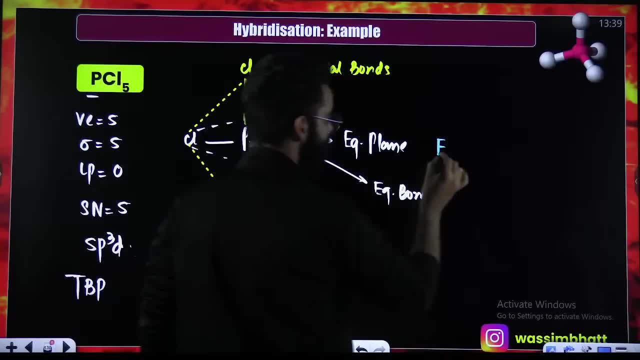 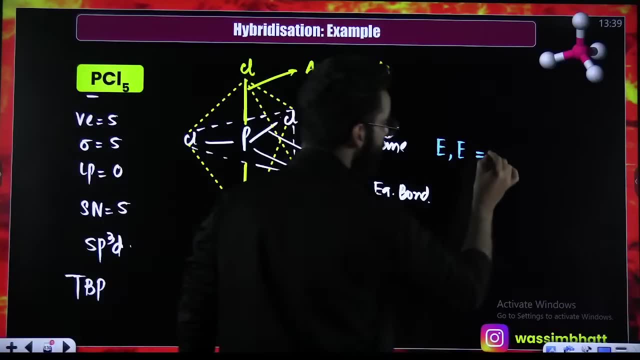 What is the angle between this equatorial and this equatorial Angle, between this equatorial and this equatorial bond, It is going to be 120 degree. If I ask you what is the angle between this axial and this equatorial Axial equatorial bond angle, that will be 90 degree. 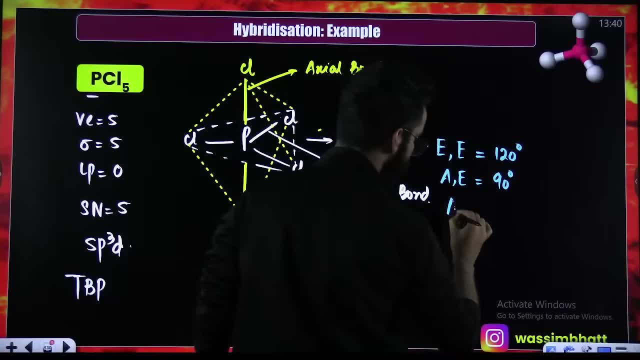 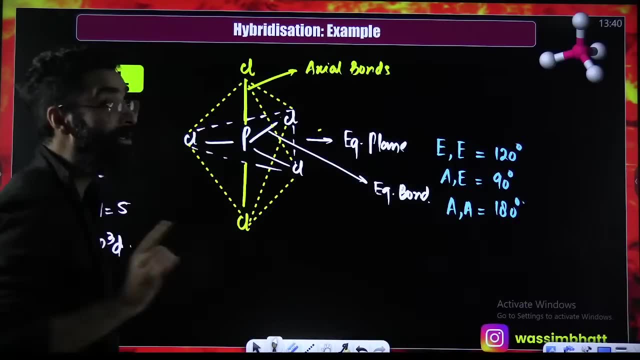 If I ask you what is the bond angle between axial and axial 180 degree? If I ask you: how many 120 degrees are there? How many 120 degrees? This is 120,, this is 120, this is 120.. 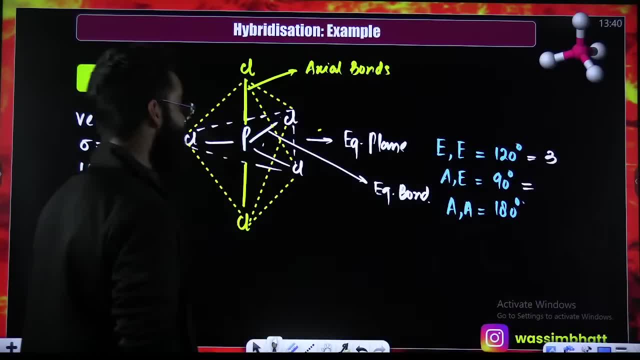 So there are three 120 degree angles. If I ask you, how many 90 degrees are there? This is forming 90 degree, with this 90 degree, with this 90 degree, with this. So three from upside, three from downside. 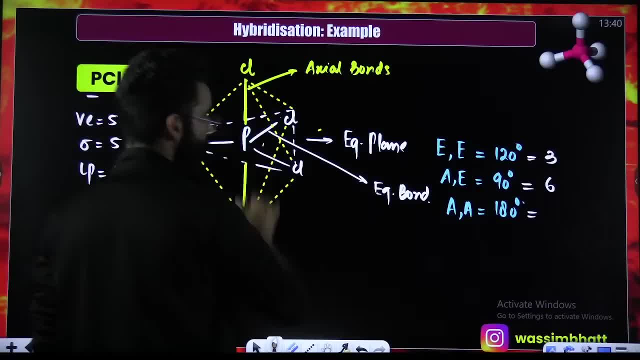 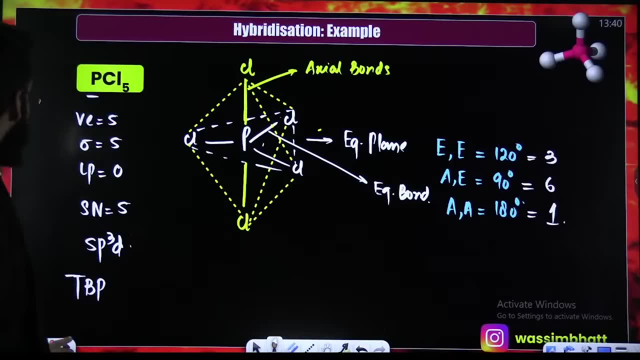 So six 90 degrees, Right, How many 180 degrees are there? One 180 degree, Okay, Perfect, perfect, perfect. Yes, Moving ahead. This was PCL5.. Now talking about SF6.. Talking about SF6.. 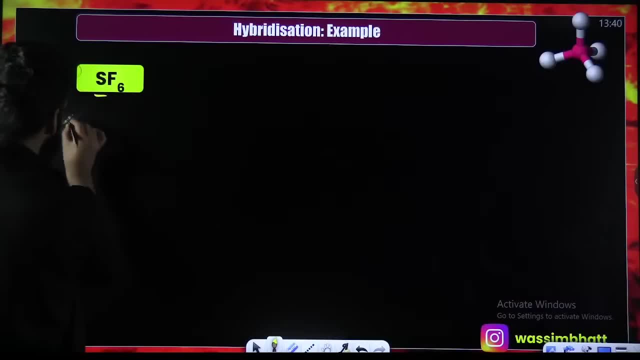 How many valence electrons? sulfur has Six Surrounding atoms, Six Lone pairs, Six minus six, Zero Steric number: Six plus zero, Six. Hybridization- SP3D2.. Geometry predicted through hybridization: That is octahedral. 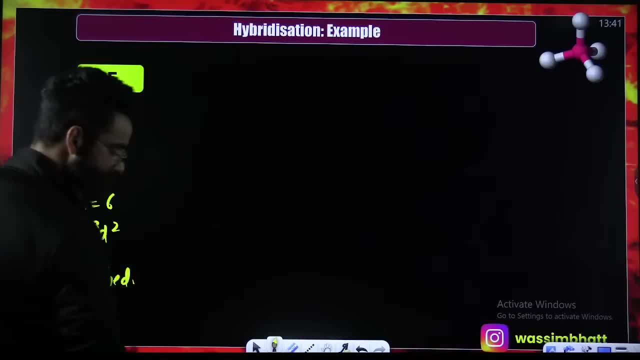 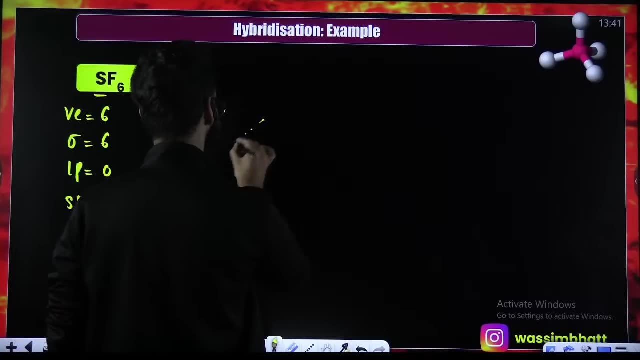 That is octahedral, Right, That is octahedral. Now, how it looks like. Have a look, Have a look. Understand, Okay, Okay, Understand, Understand Octahedral geometry. How it looks like. This is your sulfur present here. 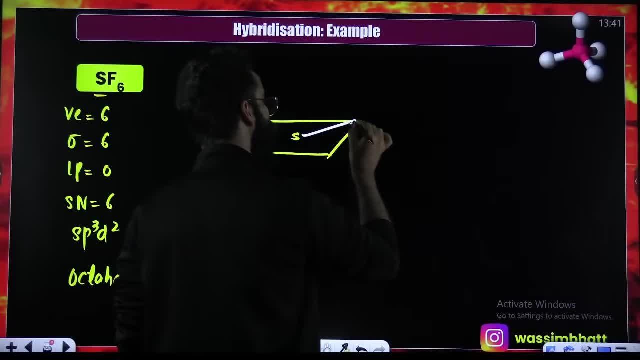 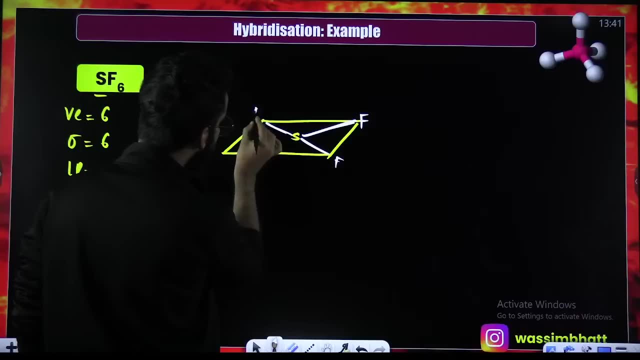 This is your sulfur. It is forming one of the bond with fluorine here. It is forming one more bond with fluorine here. It is forming one more bond with fluorine here It is forming one more bond with fluorine here. So on this equatorial plane, 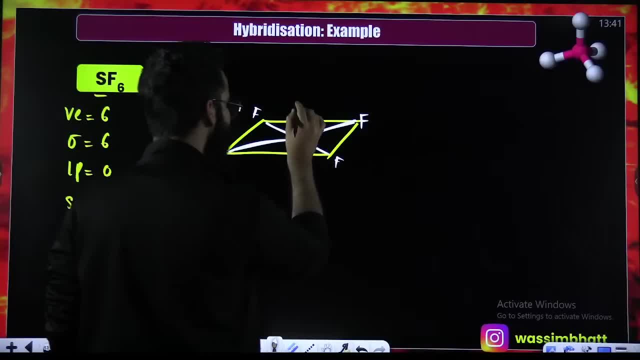 How many bonds are there? Four bonds Right. This is your equatorial plane Right Now. But now, if we look at the pentagon flourine's perpendicular transverse, it is forming just like this. Now we are going to see about the pass through current, flowing through the atmosphere from. 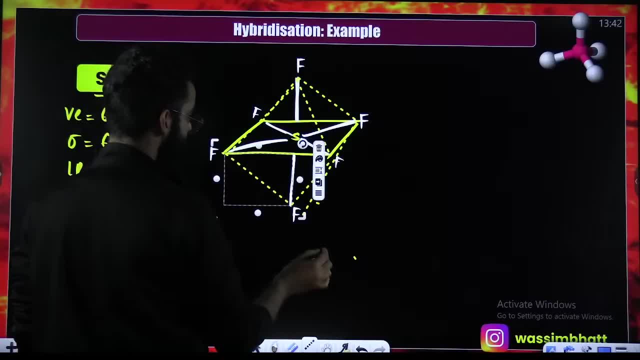 what it looks like right now and that you can see clearly from really simple results. This particular geometry is what you call as octahedral geometry. This is what you call as octahedral geometry. Octahedral geometry- Now, now. now, if I ask you, which d orbitals are involved here? 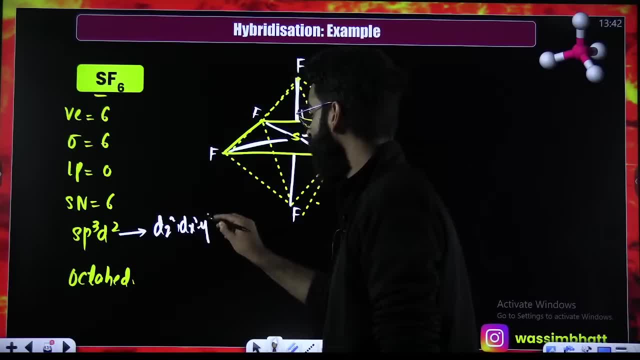 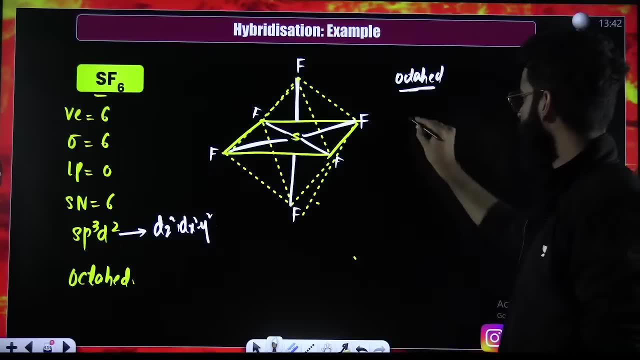 it is dz square and dx square minus y square. Okay, This geometry is what you call as octahedral. Look at all the bond angles. Look at all the bond angles, people. If I ask you, what is the bond angle between equatorial and equatorial? 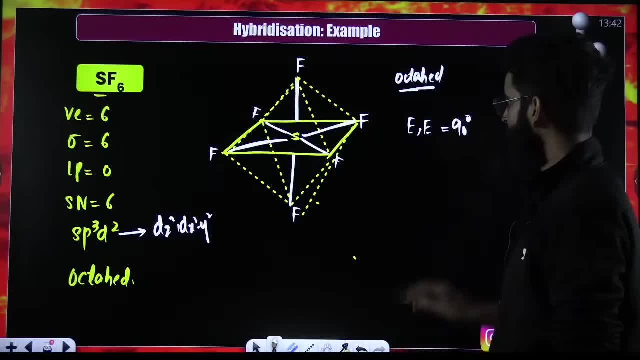 Equatorial, equatorial. This is bond angle. This will be 90, right Bond angle between axial and equatorial. Bond angle between axial and equatorial: It will be 90.. Bond angle between axial and axial. It will be what? 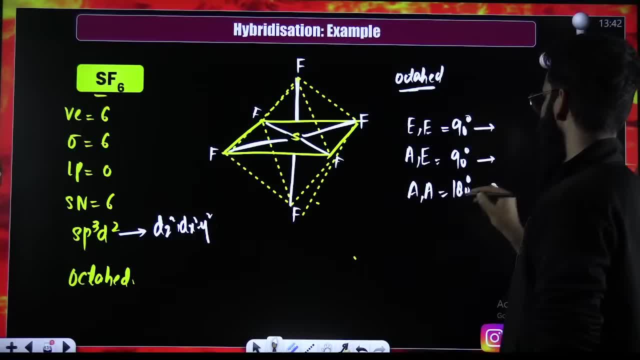 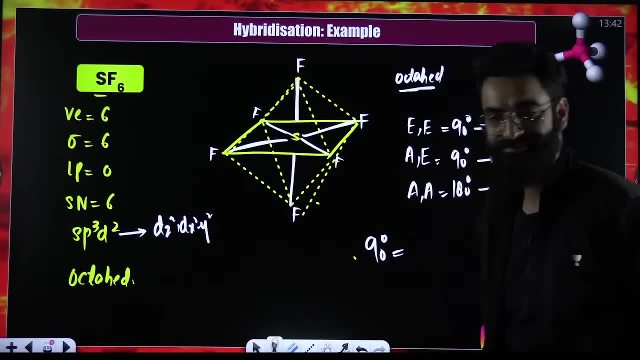 It will be 180.. Now I am asking you a question. Now I am asking you a question: How many 90 degrees are there? How many 90 degrees are there? Quickly, How many 90 degrees are there? First of all, this is 90.. 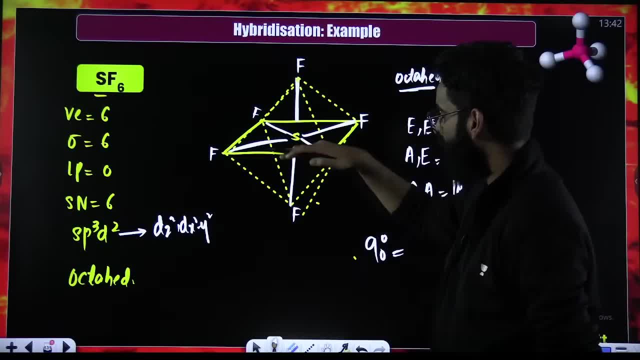 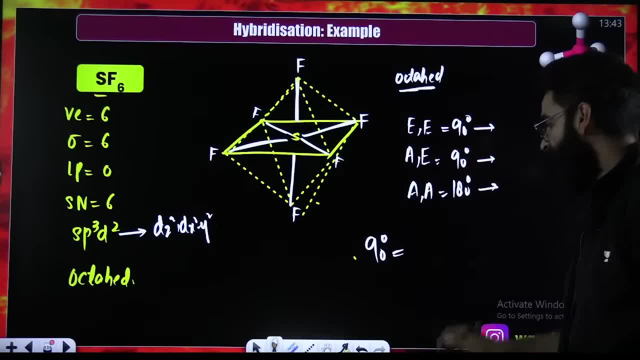 So 4 from top, 4 from bottom, 4 from bottom right. So 4, 4,, 8,, 4,, 12.. So 12,, 90 degrees. Okay, If I ask you, how many 180 degrees are there? How many 180 degrees are there? How many 180 degrees are there Between axial and axial? 180.. Now, between this equatorial and this equatorial: 180.. Between this equatorial and this equatorial: 180.. So there are 3 180 degrees. 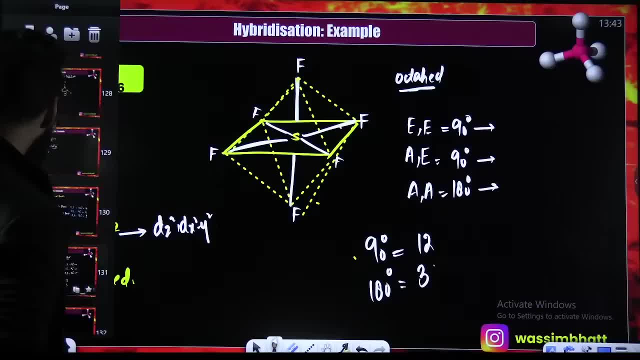 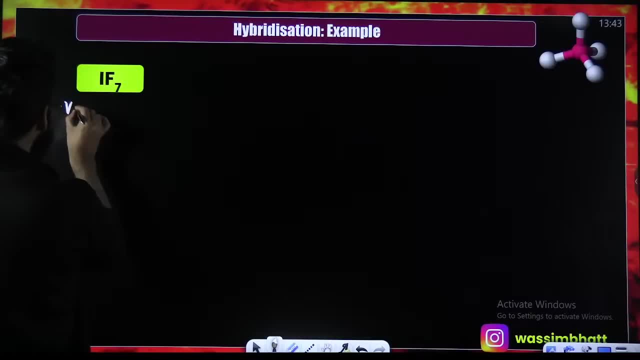 Yes, there are 3 180 degrees. I hope this is clear. I hope this is clear. I hope this is clear. Right, I have 7.. I would even say being the central atom, how many valence electrons? 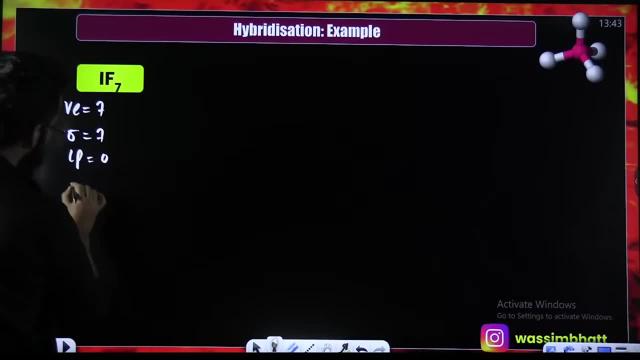 7. Sigma bonds: 7. Lone pairs: 0.. Steric number 7. Hybridization sp3d3.. Which d orbitals, dz square, dx square minus y square and dxy Right Geometry predicted through hybridization. 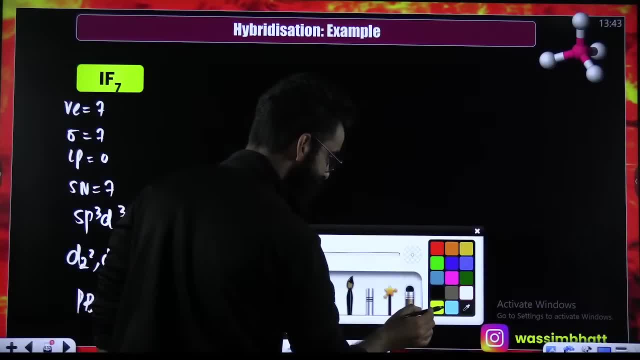 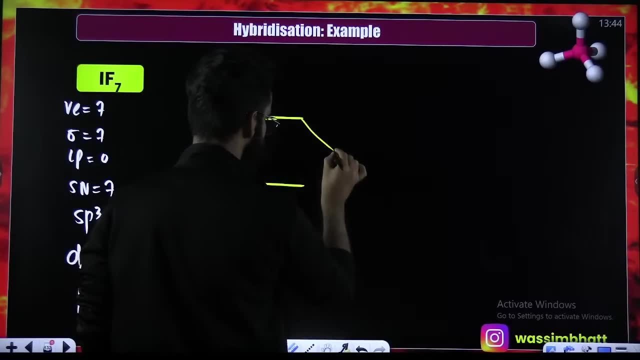 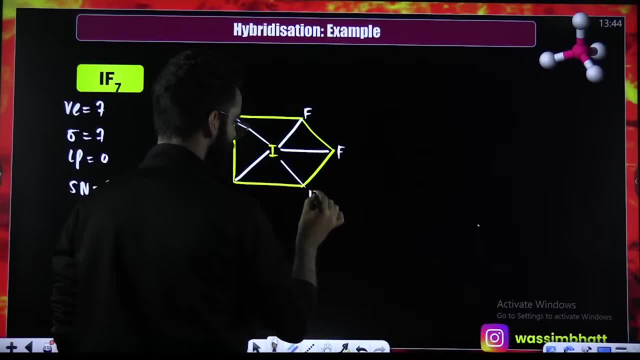 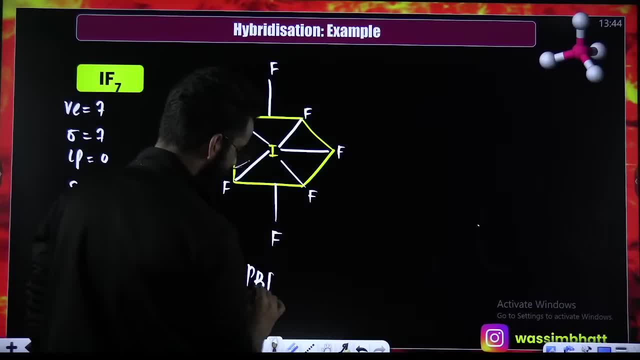 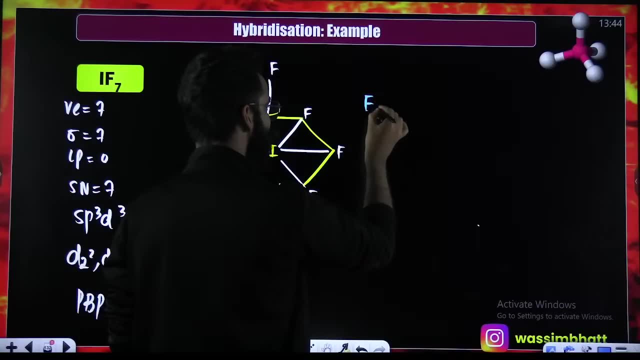 Right, This geometry is pentagonal bipyramidal geometry, Pentagonal bipyramidal geometry. Now, people, if I ask you something, The angle between equatorial equatorial, The angle between equatorial equatorial, Where it is going to be, 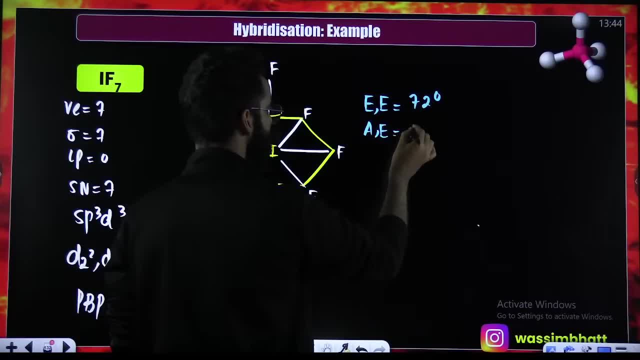 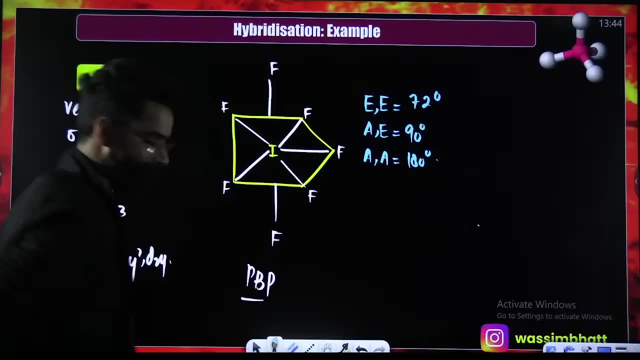 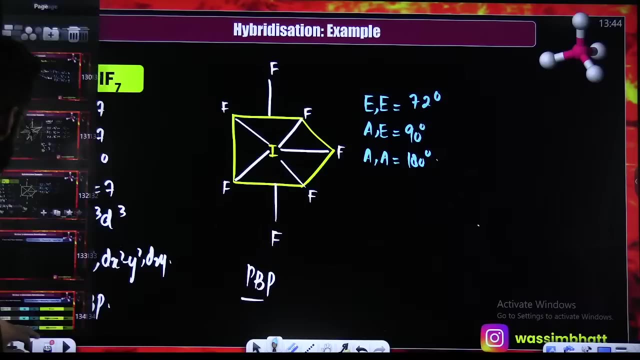 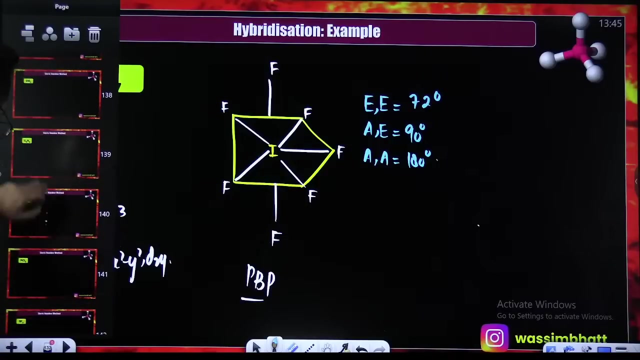 72 degree. The angle between axial and equatorial, that is 90 degree Right. The angle between axial and axial, that is 180 degree. Am I clear? Am I clear people? Am I clear, people? Am I clear? Am I clear? 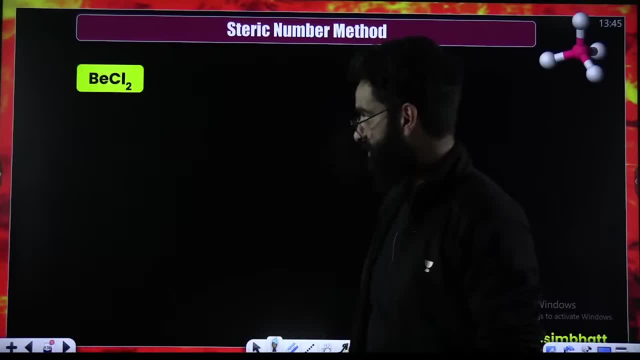 Now tell me- these are few questions which I have for all of you. tell me for this BECL2, this you can make on your own: C2H6, C2H6, make it like this: see C2, this is H6, C2,. 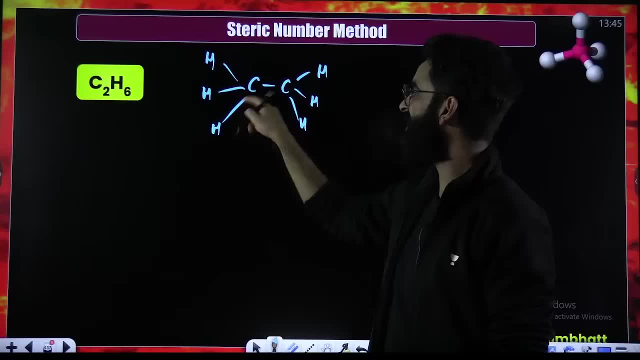 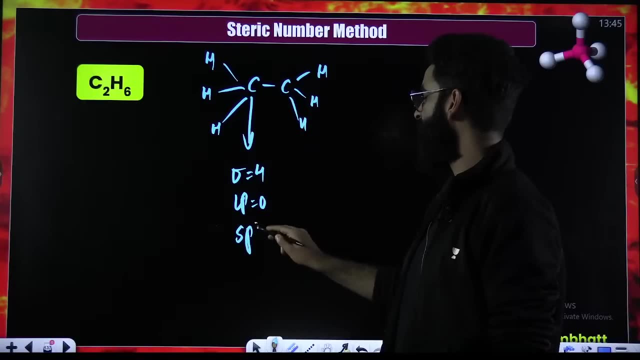 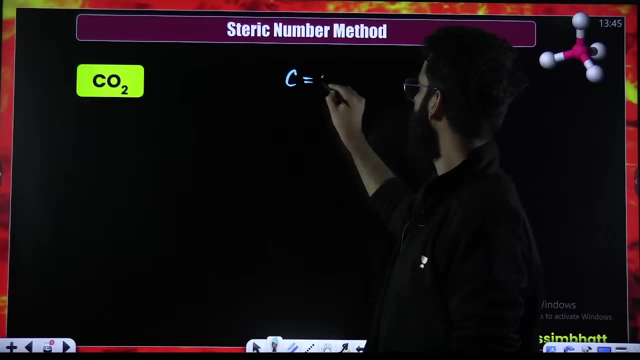 this is H6, carbon. how many sigma it is forming? it is forming 4 sigma. 4 sigma. that means it will have no lone pair. steric number is 4, hybridization is sp3, similarly, this will have sp3 hybridization- simple carbon dioxide. you know it? carbon dioxide, perfect this. 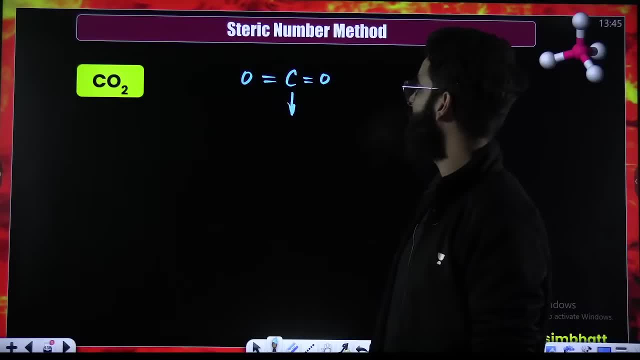 carbon. it is hybridization. it is hybridization. it is forming how many sigma, 2 sigma. it is forming 2 sigma. how many valence electrons it had? how many valence electrons it had? 4, but it is forming 4 bonds as well. so all the 4 valence electrons have been used right. 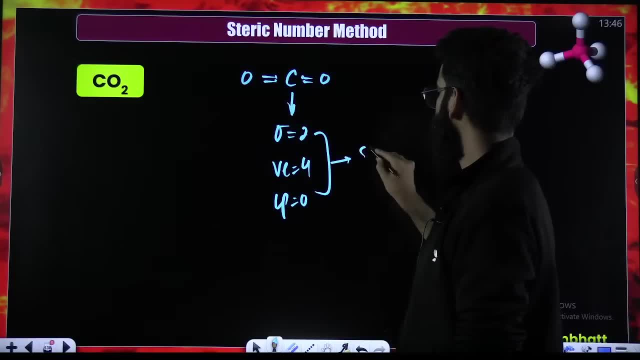 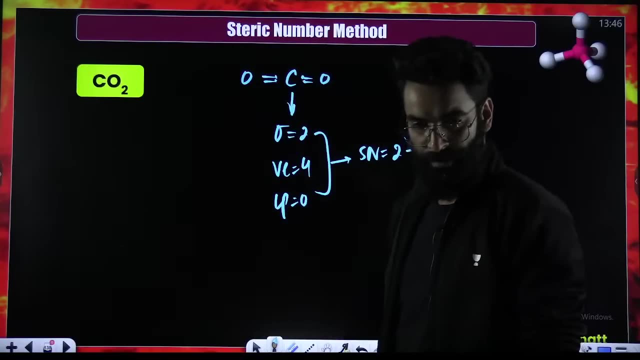 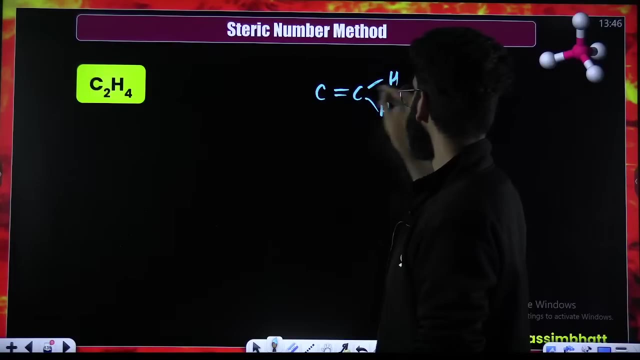 so lone pair is 0, steric number is: steric number is 2 plus 0, 2,. hybridization involved. is sp done and understood, right? sp okay, C2H4,. this is your C2H4,. tell me how many. 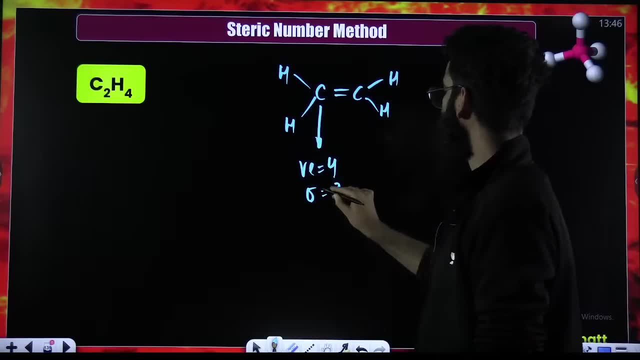 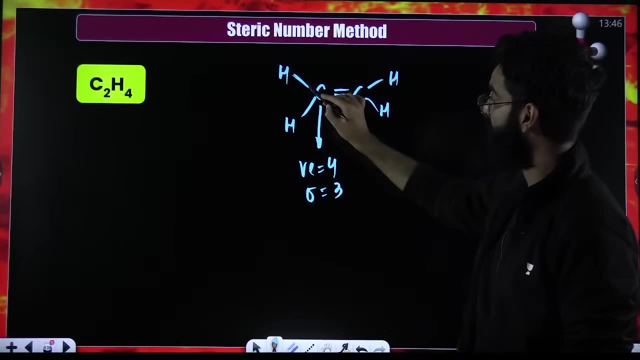 valence electrons. carbon has 4,. how many sigma it is forming? It is forming 3 sigma, 1, 2 and 3, 3 sigma. how many lone pairs it has it had? 4 valence electrons and it is using all the 4 valence electrons, see 1, 2,, 3, 4, 4,. all the 4 are: 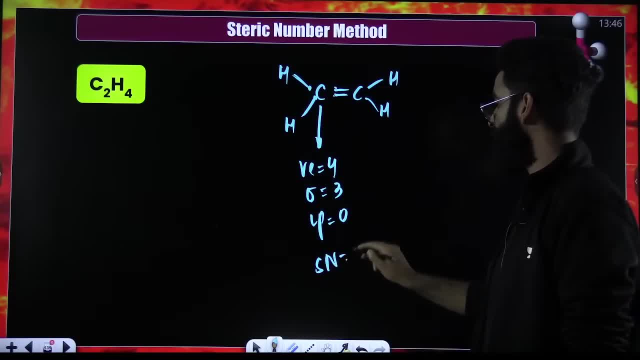 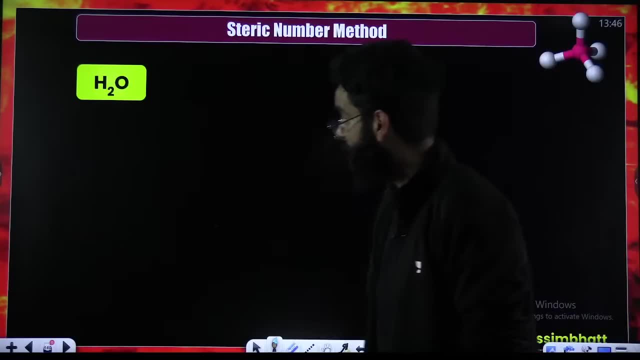 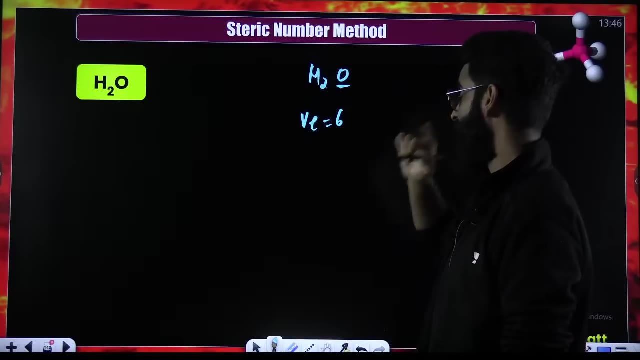 used. so lone pair 0, steric number: sigma plus lone pair. sigma plus lone pair 3, hybridization: sp2, yes, similarly H2O. H2O oxygen: how many valence electrons? 6, right, how many? 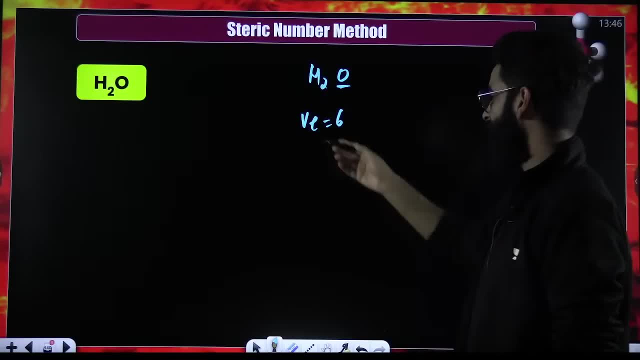 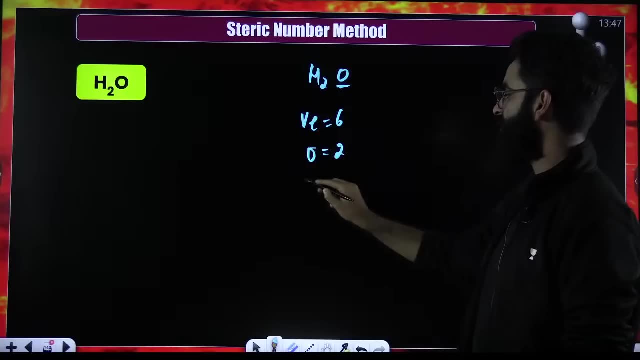 valence electrons 6. 6. How many surrounding atoms 2, right, so out of 6 valence electrons, 2 have been used to form 2 sigma bonds. so there are 4 electrons left. as such, there are 4 electrons left as: 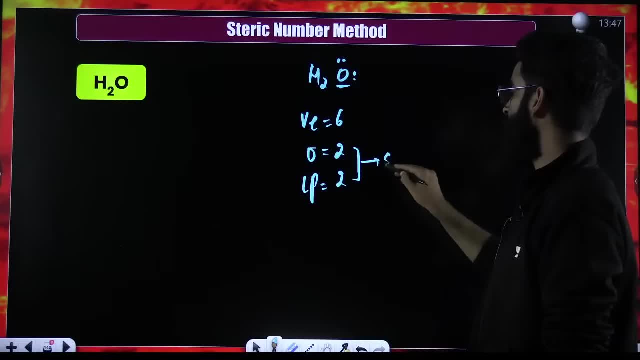 such on oxygen on, in the form of 2 lone pairs, so sigma plus lone pair, steric number is 4, if steric number is 4, hybridization involves sp3, geometry which is predicted through hybridization. geometry which is predicted through hybridization I am not talking about. 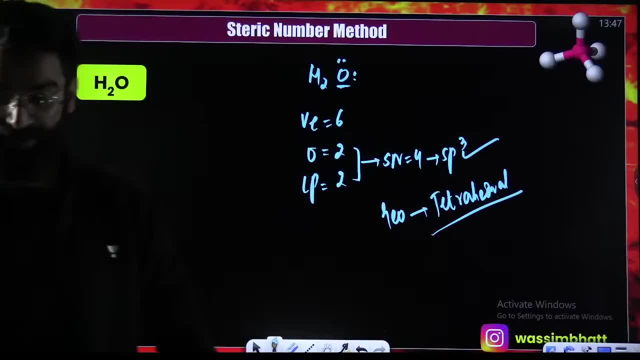 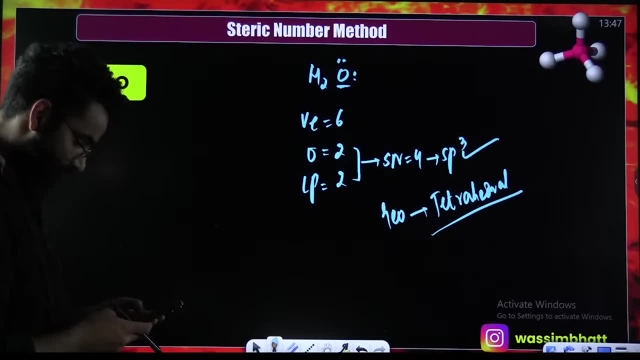 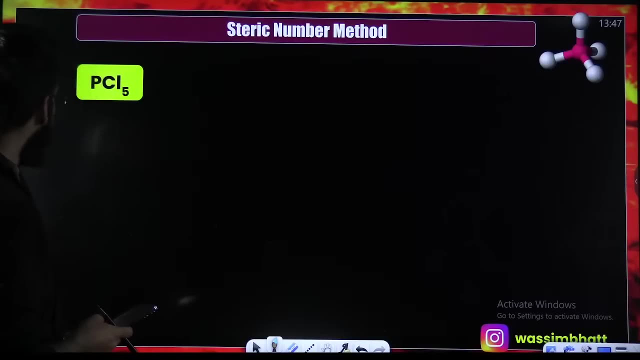 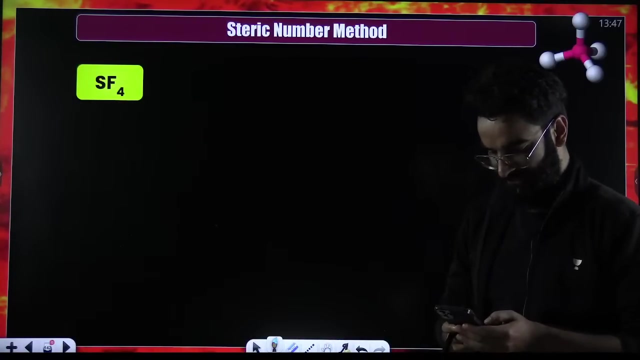 the actual shape. I am talking about the geometry which is predicted through hybridization, that is, That is sp3, right, tell me PCL5, we are done. SF4, quick SF4, SF4,, SF4,, SF4, right. 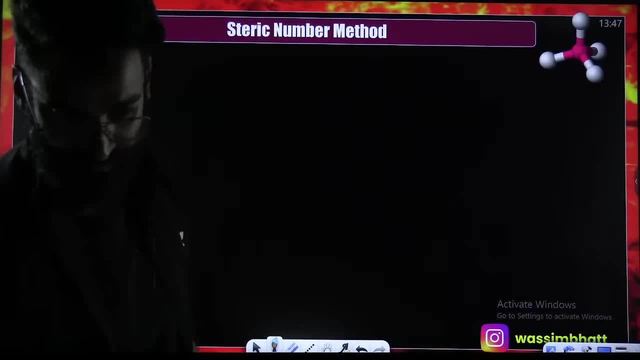 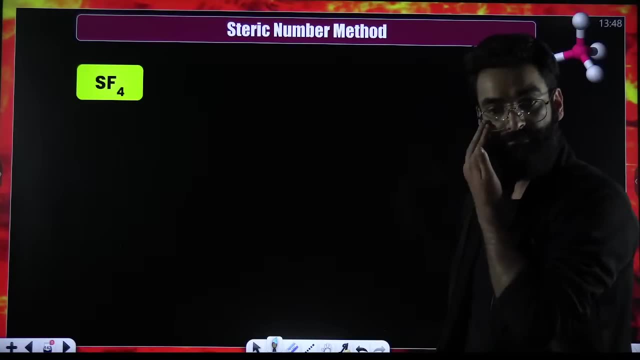 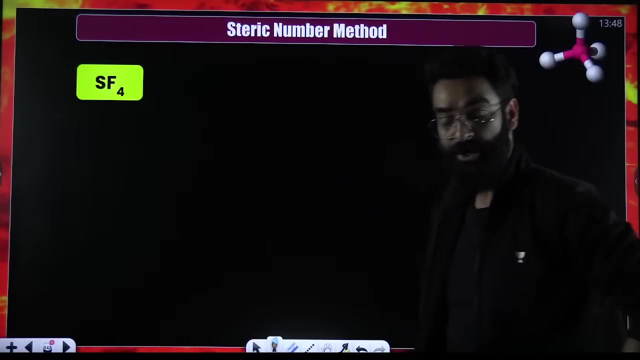 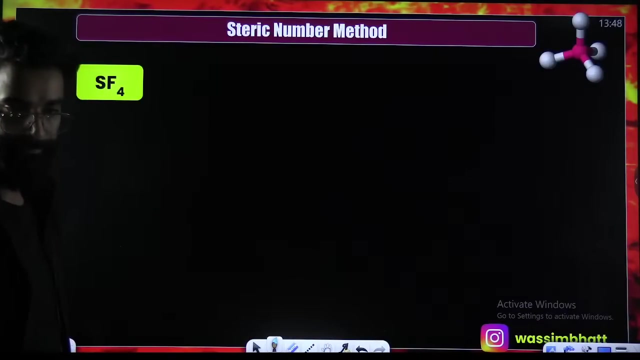 SF4, quick, quick people. SF4, quickly, quickly, quickly. guys, you have to be super fast, you need to be super fast. perfect, we will be done. 4 sigma bonds, 1 lone pair. steric number is 5.. 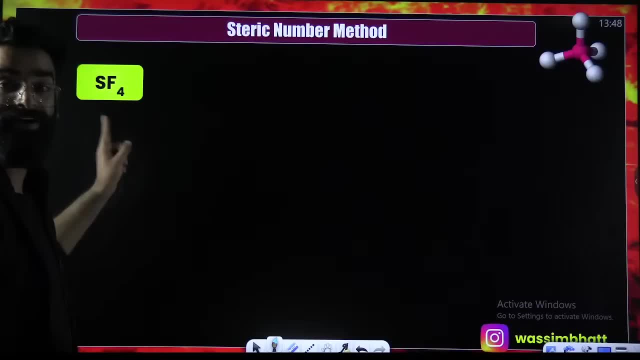 Steric number 5 means sp3d. geometry predicted through hybridization is a trigonal bipyramidal dusted. okay, XCO2F2, see, see, see. what do you do in this particular case? this is: 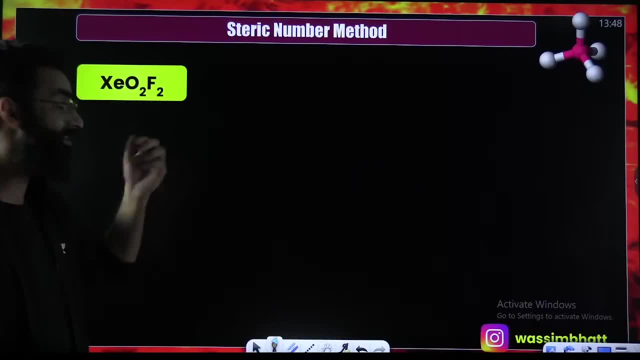 a special case. why is that? whenever you see oxygen as the surrounding atom, whenever you see oxygen as a surrounding atom, at that point of time there is something which you need to do. see valence: electrons in xenon are 8, surrounding atoms are 4, surrounding. 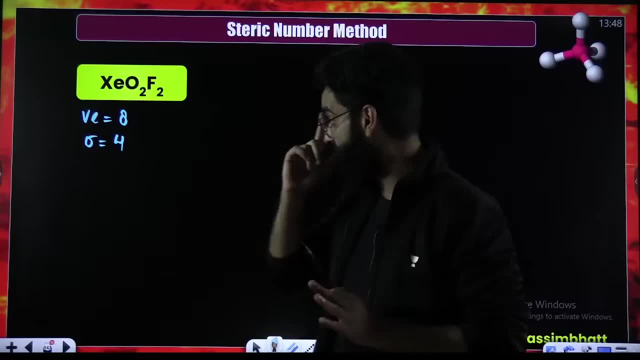 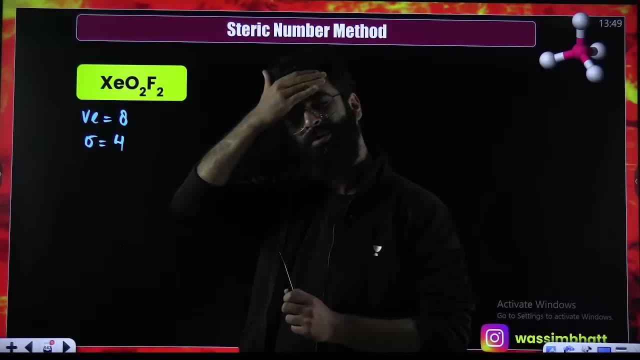 atoms are 4, right of 4.. Assume now, assume certain things. Oxygen is a surrounding atom, It's a divalent, It's divalent. So, normally, what do we see? Divalent atoms, they form 2 bonds, right? So these? 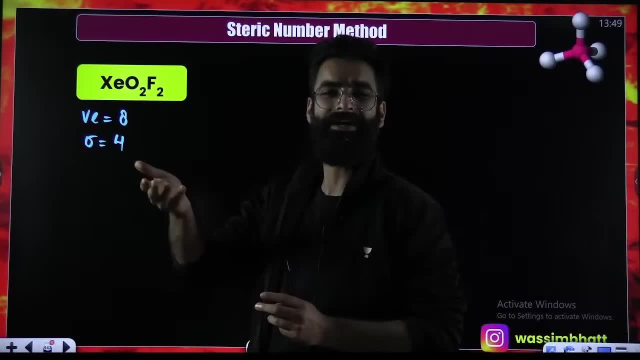 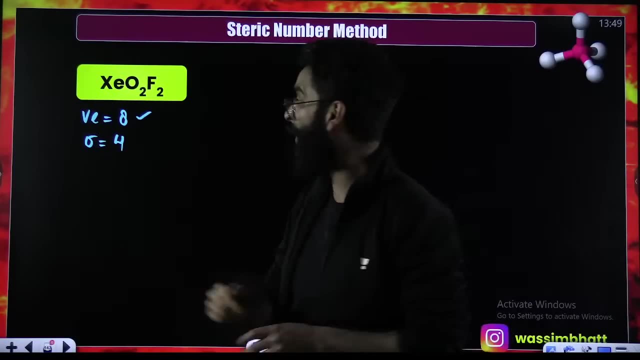 two oxygens. understand it like this, Remember it like this. These two oxygens will form 4.. 4 plus 2 is 6.. So out of 8 valence electrons, 6 have been used. So there will be 2 valence. 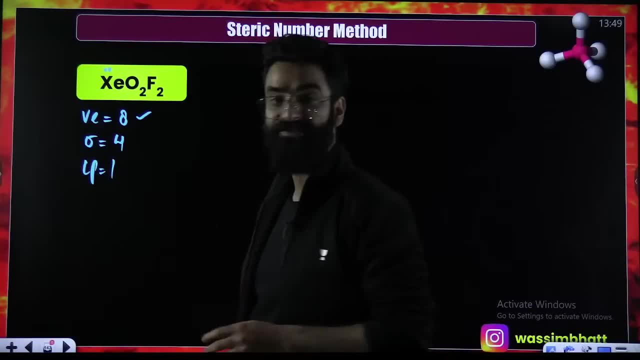 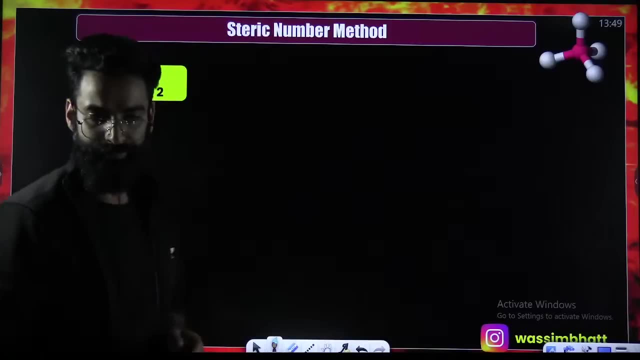 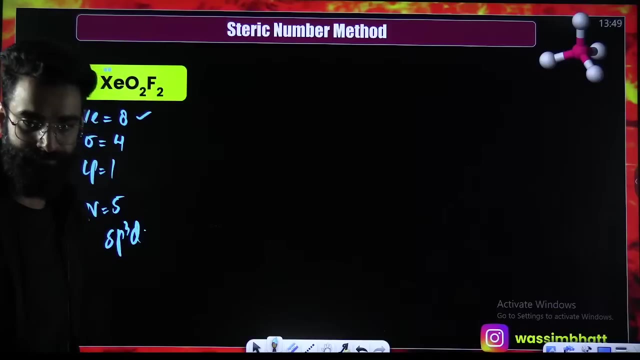 electrons on xenon in the form of a lone pair, right In the form of a lone pair. Now steric number 4 plus 1, 5.. This is sp3d. Am I clear? Am I clear people? Am I clear people? Yes, 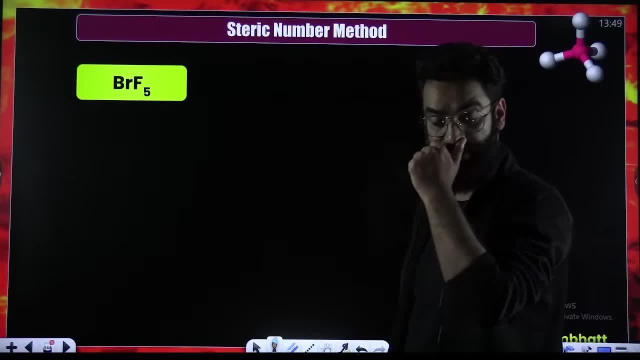 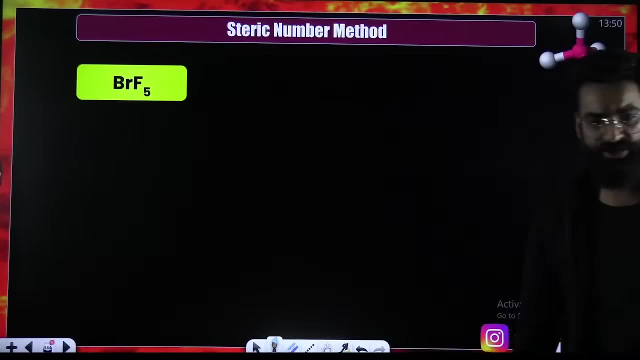 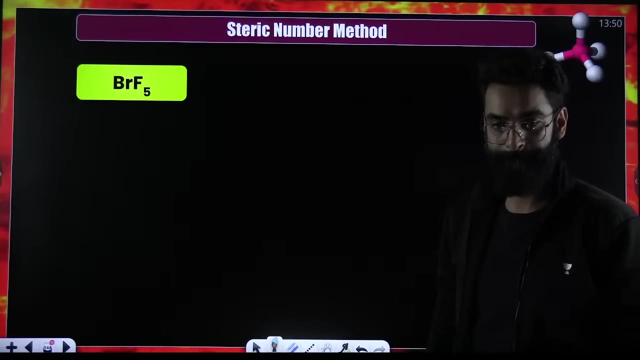 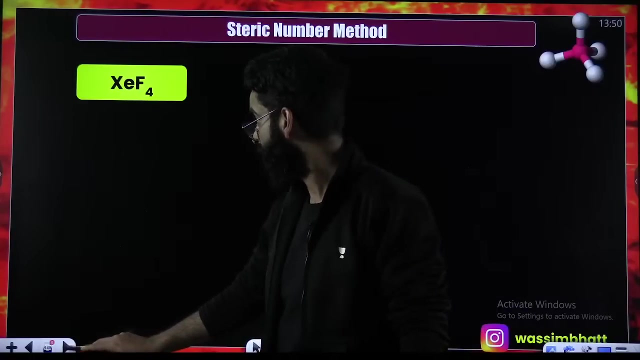 Tell me the answer of this one quickly. Brf5.. Hybridization of Br. Hybridization of Br. Hybridization of bromine. Hybridization of bromine. Hybridization of bromine. 5 sigma bonds: 1 lone pair, right- sp3d2.. Xcf4.. Xcf4.. Quick, quick, You have to be very quick. Xcf4.. 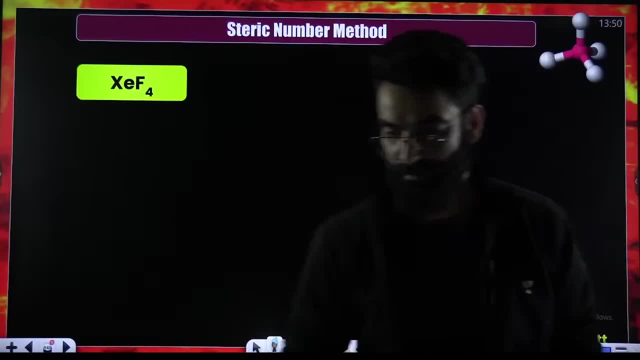 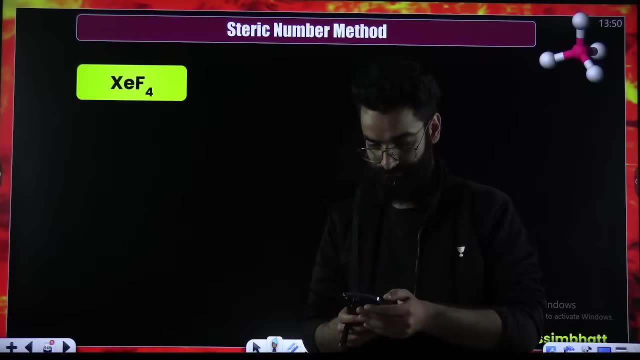 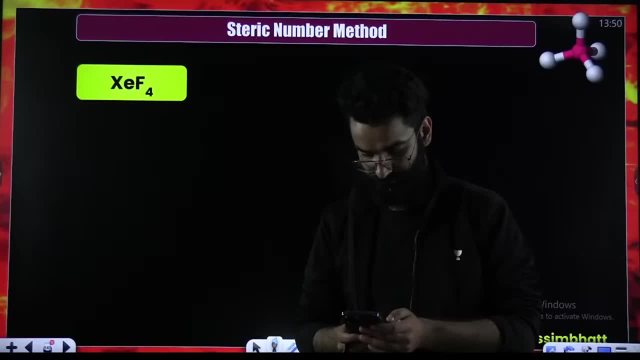 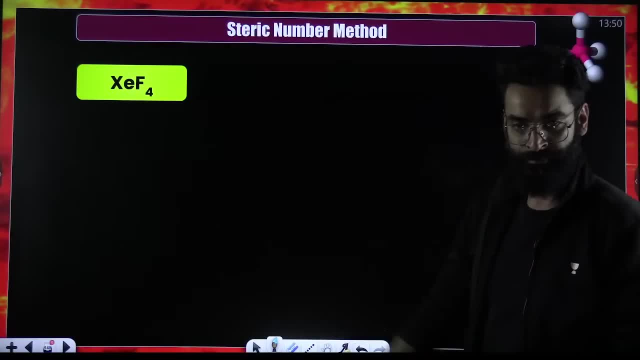 6x, SC4, S3, 6648.. Tempo 4ה: No more Warehouse miracle. fast trip worked with state 1.. CPU W: clearer than cash. Career itself is better than thirdopot silly. 4 sigma, 2 lone pairs. 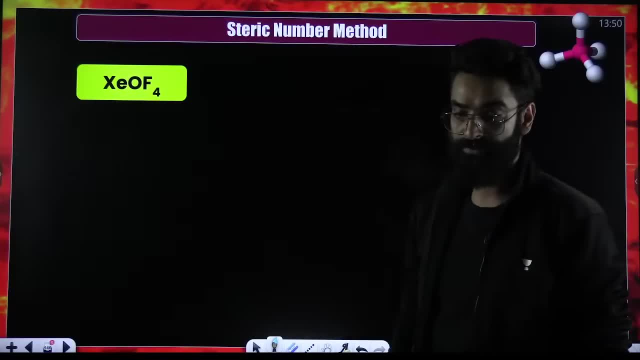 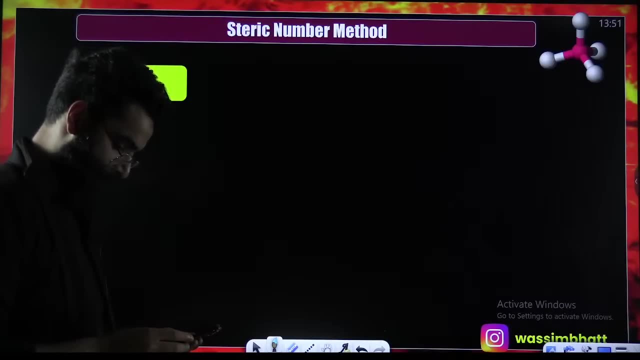 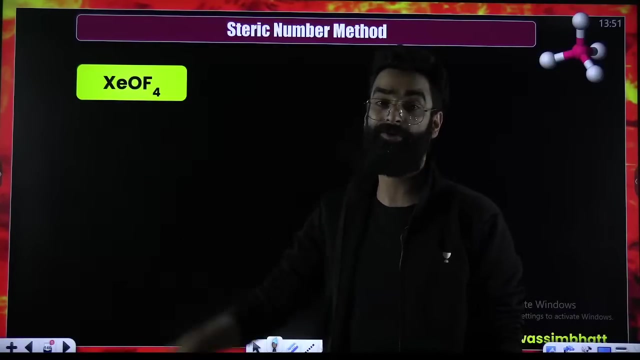 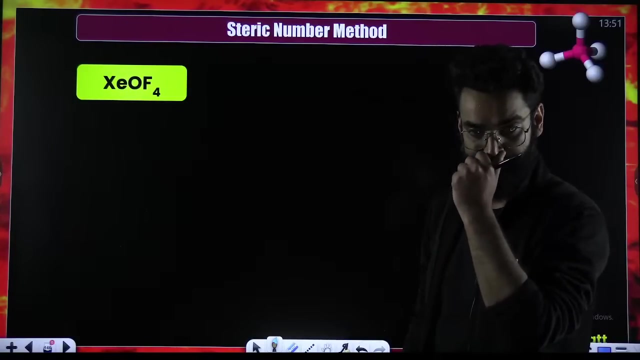 sp3, d2, perfect xe of4, xe of4, everyone xe of4, xe of4. look here, oxygen here is not the central atom, oxygen is the surrounding right. so one oxygen. you have to consider two bonds done. Sudhir, I am sorry, I need to block you bro. 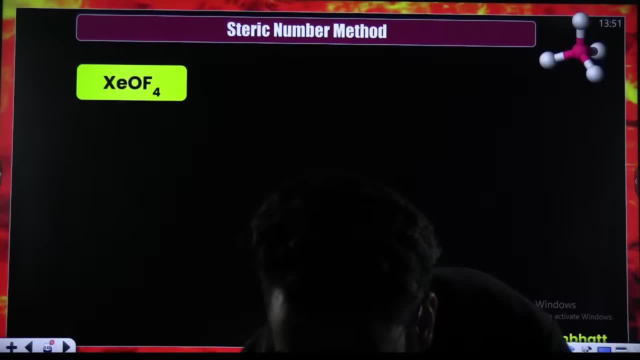 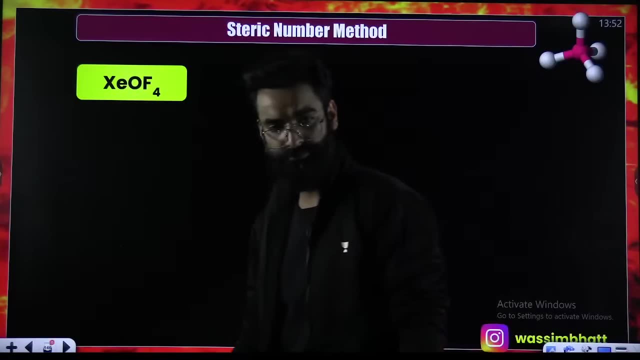 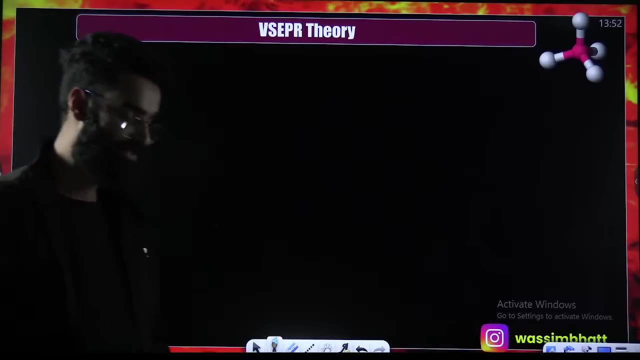 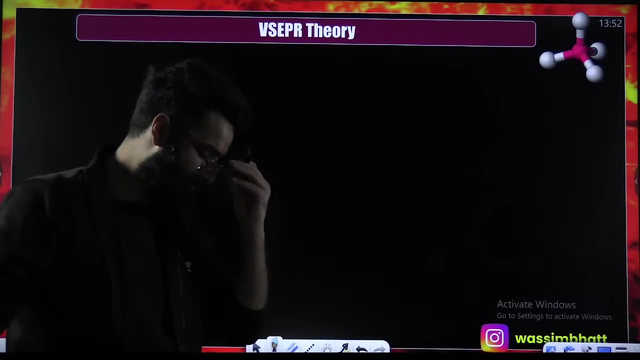 you are creating a lot of there in the chats. yeah, god bless, you come on. xe of4 done perfect. so I believe, whenever a question comes from hybridization, geometry, character number, bond angle between axial, axial, number of number of bond angles, etc. etc. I hope this should be a 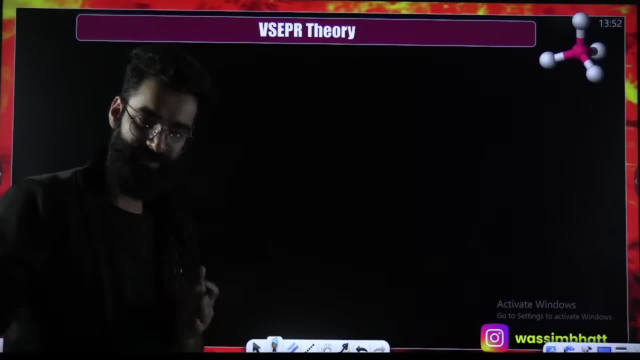 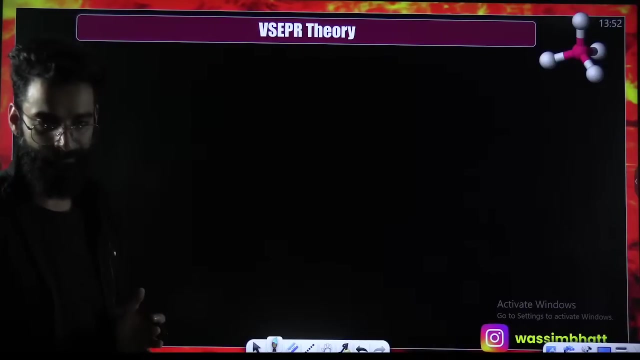 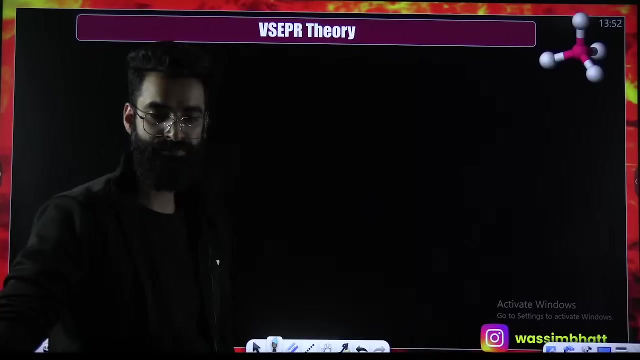 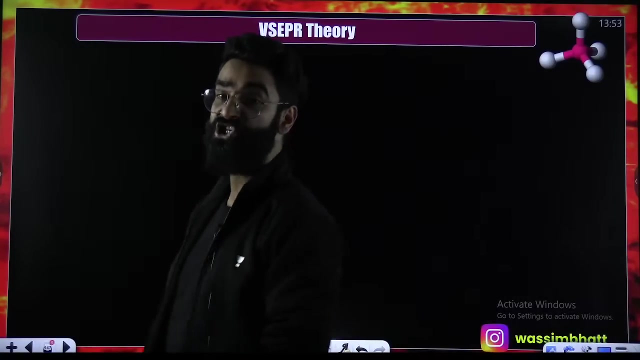 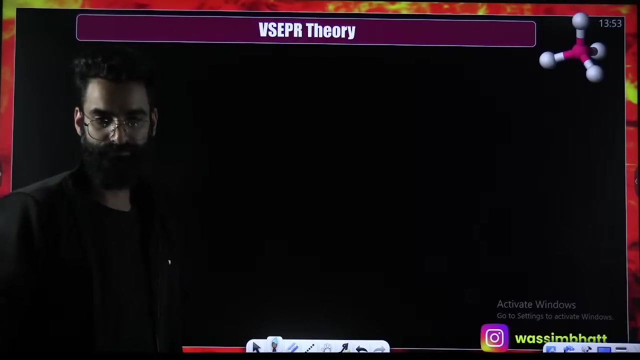 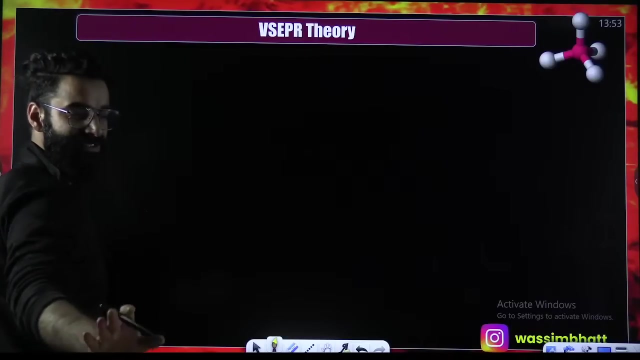 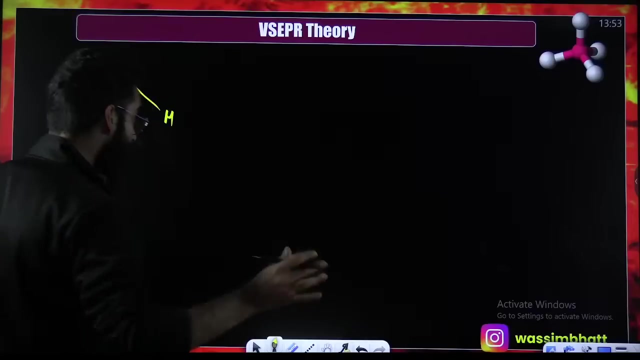 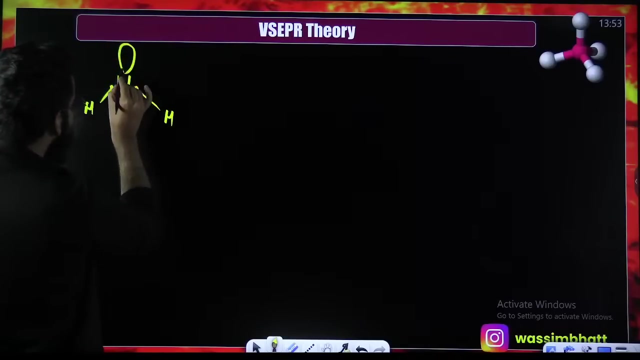 cakewalk for all of you. yeah, am I done? say it in the chats everyone and trust me. sure, short question will be there from hybridization. sure, short question. click the link in description to form a bonds. so two electrons will be there on nitrogen in the form of a lone. 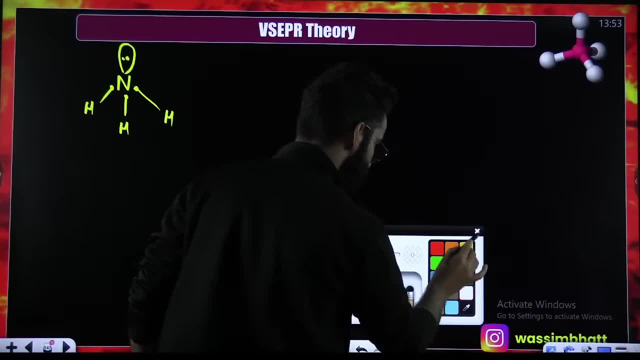 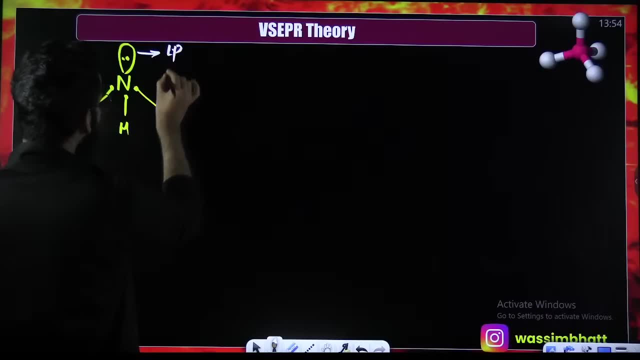 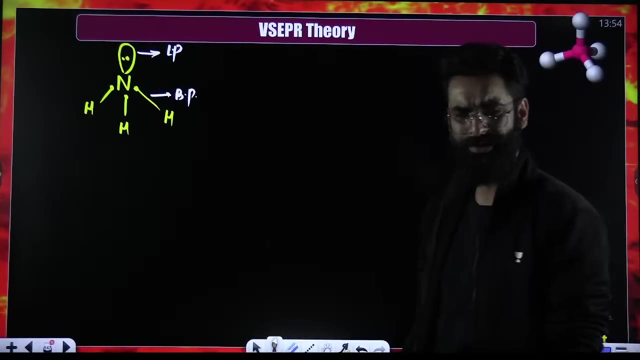 pair right in the form of a lone pair. perfect now, my dear students, this is something which you call as non bonded pair or lone pair. right, this is something which you call as bond pair. basically, in the molecule, you have got lone pairs and bond pairs. in the molecule, you have got lone pairs and bond pairs. 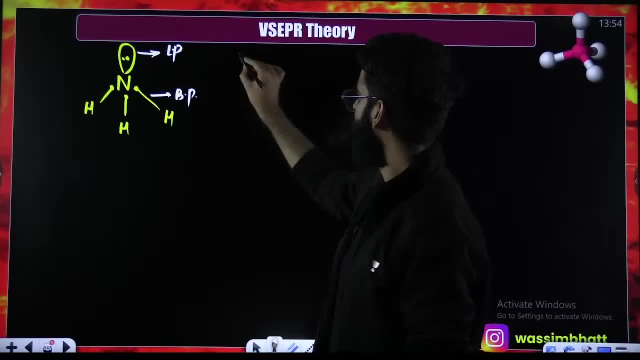 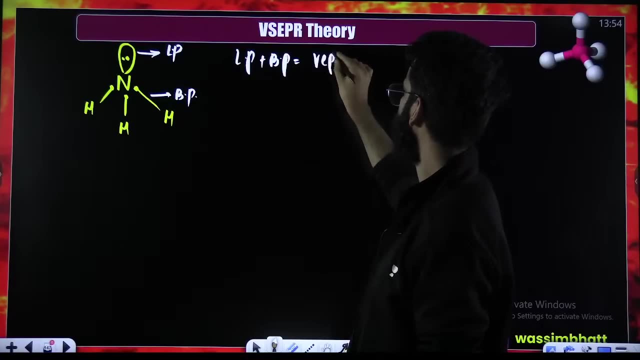 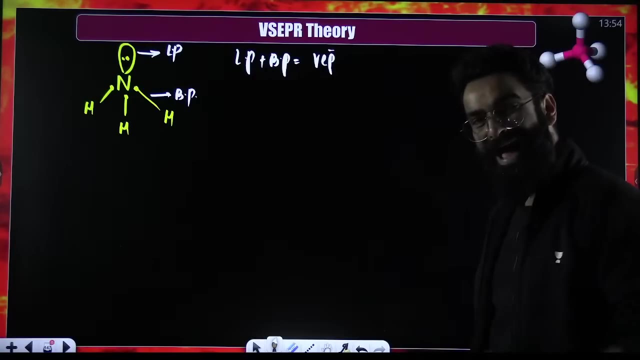 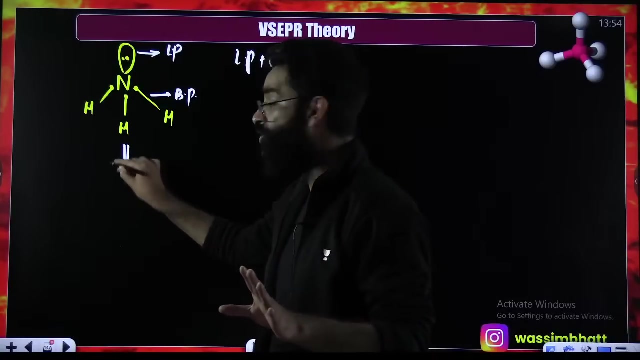 as per VSEPR, lone pairs plus bond pairs. they are called as, basically, total valence electron pairs. total valence electron pairs, right, they are called as total valence electron pairs. now, as per VSEPR. as per VSEPR, the molecule tries to acquire. the molecule tries to acquire that shape. 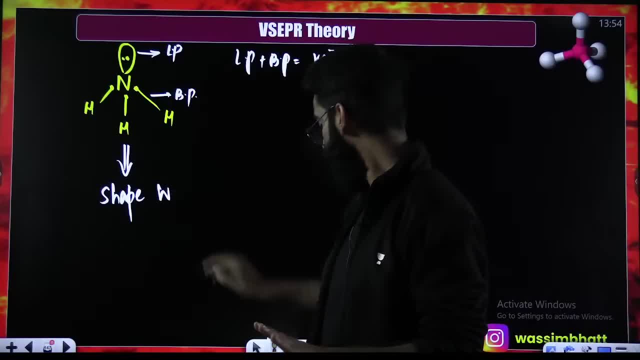 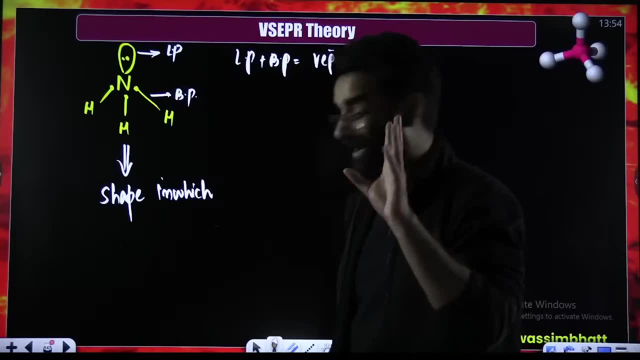 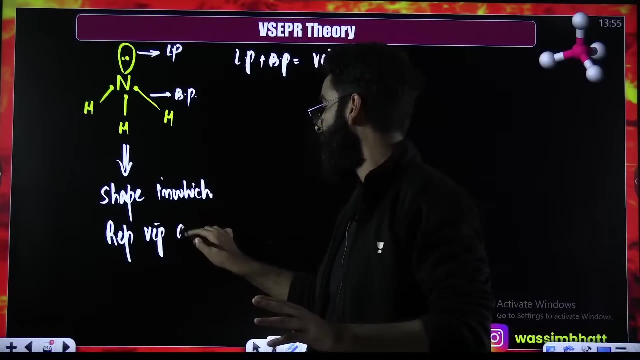 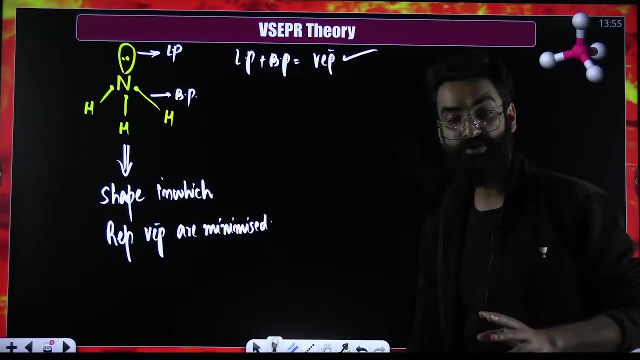 that shape in which the molecule tries to acquire, that shape in which in which repulsions, in which repulsions between the valence electron pairs are minimized, are minimized. molecule tries to acquire that shape in which the repulsions between the valence shell electron pairs are minimized and 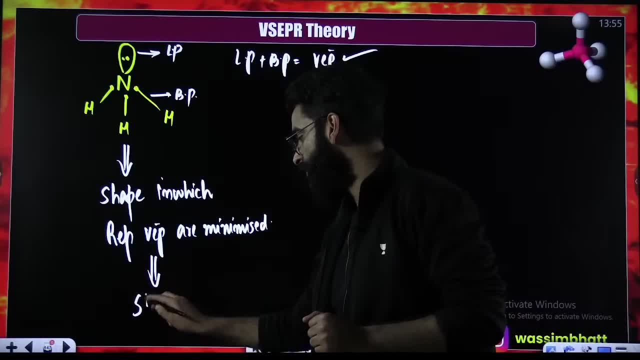 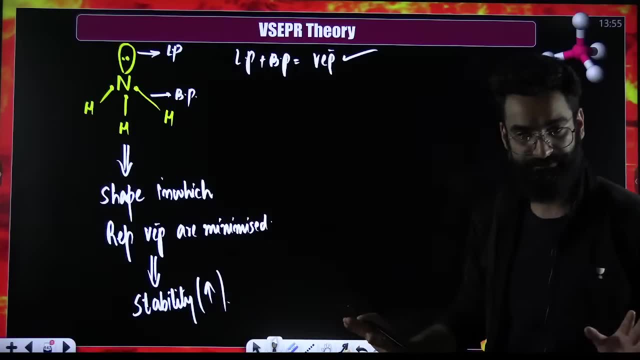 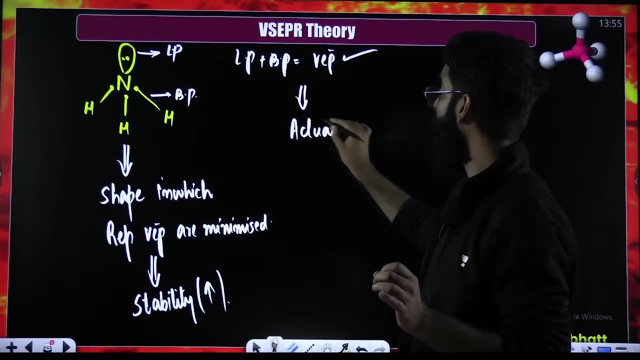 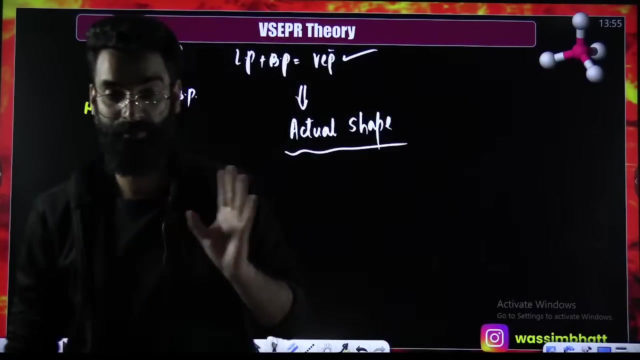 once the repulsions are minimized, we say stability is maximized, stability is maximized. so basically, your valence electron pair repulsion theory. it gives you the idea about the actual shape of the molecule. it gives you the idea about the actual shape of the molecule. okay, now try to understand how exactly it is. 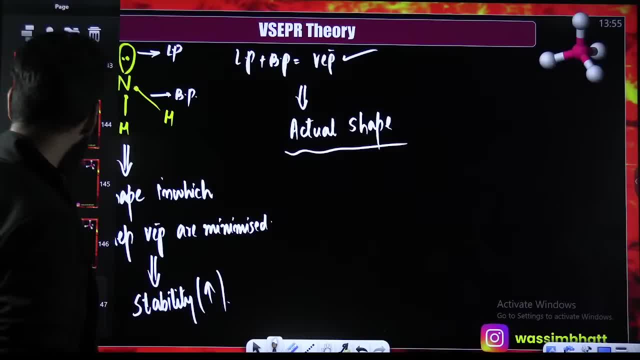 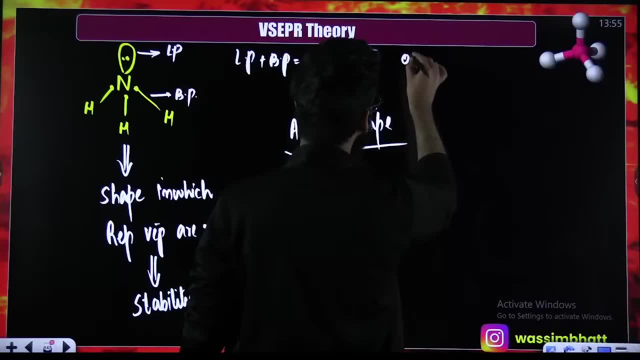 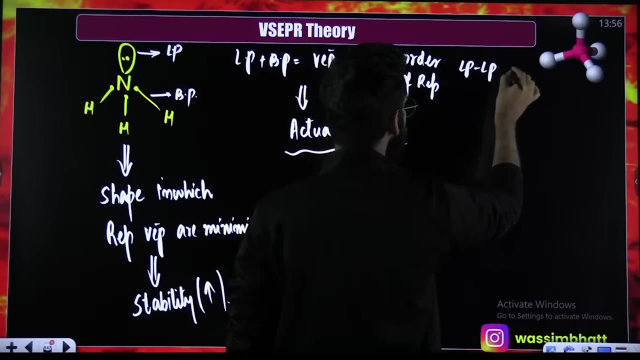 how exactly it is. try to understand how exactly. but before that one thing: there was a question asked long back: order of repulsions. you know what loan pair-loan pair repulsions are maximum all a load. you know it's following the bond pair. 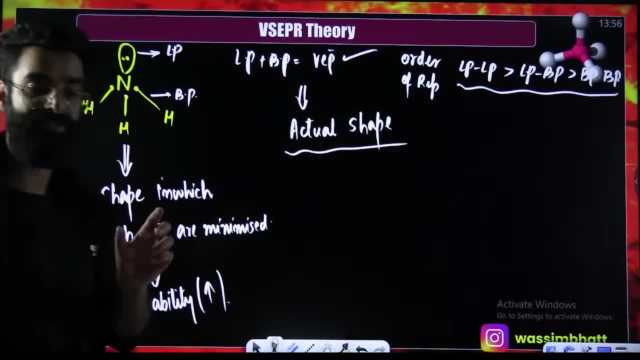 That is the order of repulsion. right lecture repulsion, that is a maximum gardelrepulsion, distinctive maximize the full definition of single line bangpair, bonding, followed by bond pair, bondpair, all of gorgeous, If you calculate the nonbalancing first phase, letterrosoft's boundary. 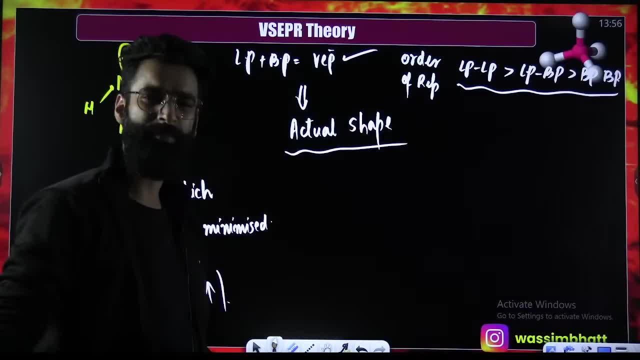 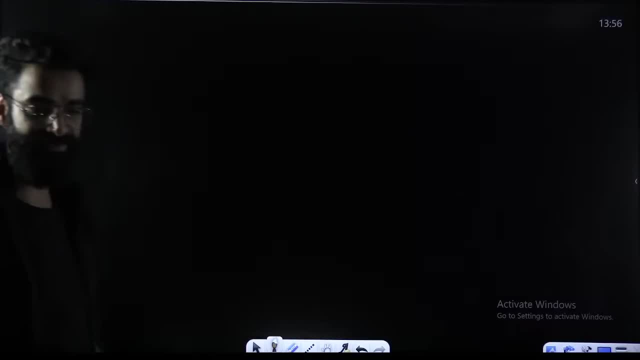 you can see bosanna r��植 members or Libre eighteen there if you calculate Molina. problems speaking half modic follower by bond pair bond. okay, now see exactly how i'm going to utilize this via cpr and it will solve a lot of our issues. 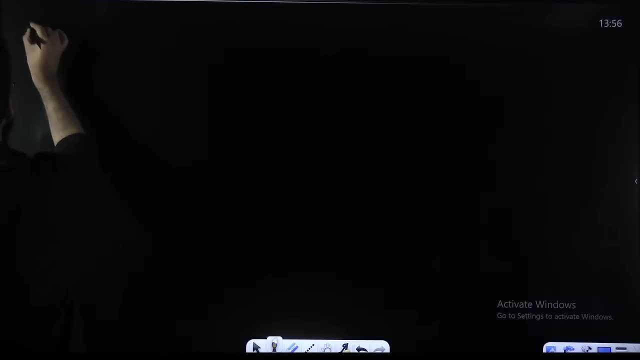 try to understand the first case i'm writing over here. what is that i'm writing? if steric number, if steric number is equal to three, if steric number is equal to three, you know. if steric number is three, you know. if steric number is three, the geometry predicted through hybridization is trigonal planar. you know it. for steric number three, geometry predicted through hybridization is hybridization is trigonal planar. now, guys, what is steric number? sigma plus lone pair? so there are two possibilities here. there are two possibilities here if there are three sigma and zero lone. 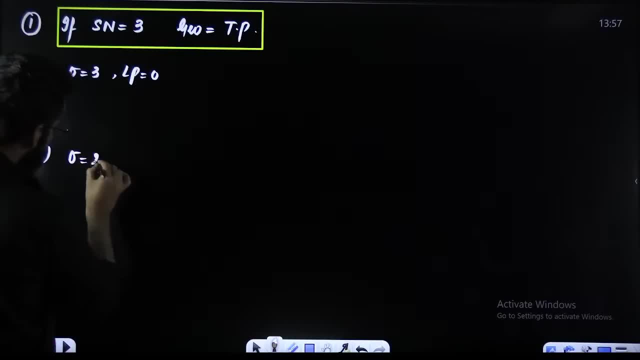 pairs. second, if there are two sigma and zero lone pairs, sorry- and one lone pair, sigma plus lone pair is three, sigma plus lone pair is three. so steric number in both the, in both the ones, is three. right, steric number three, steric number three. now, first of all, that molecule wherein the central atom is forming three sigma. 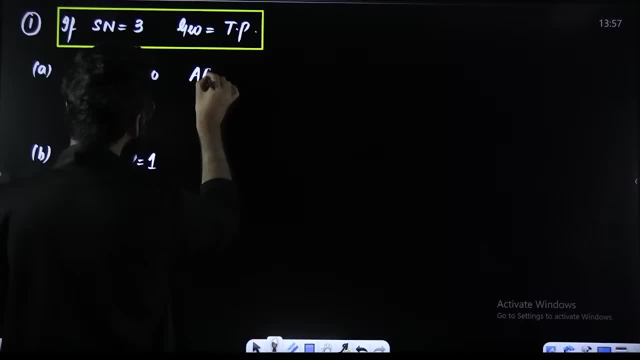 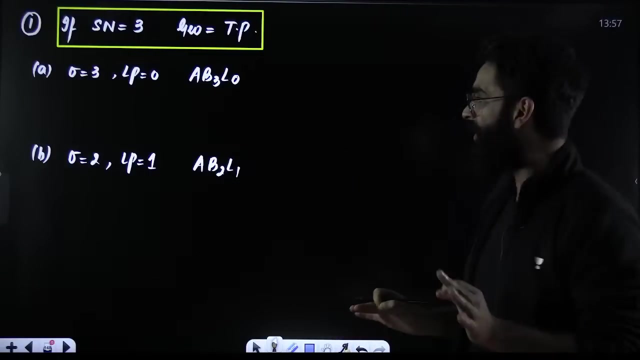 bonds and has got zero lone pair. we say the type of the molecule is ab3l0. a is the central atom, three sigma bonds, zero lone pair. the type of this molecule is going to be ab2l1, ab2l1. do remember, do remember, do remember. when the central atom, when the central atom. 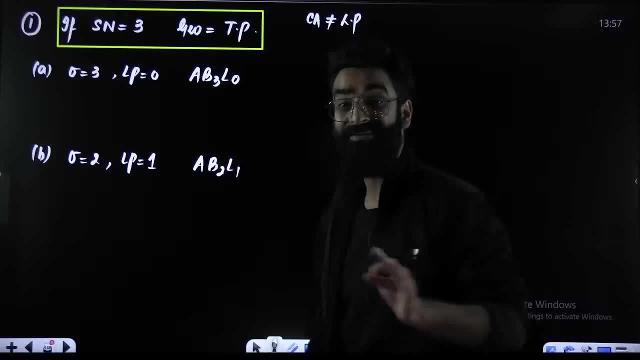 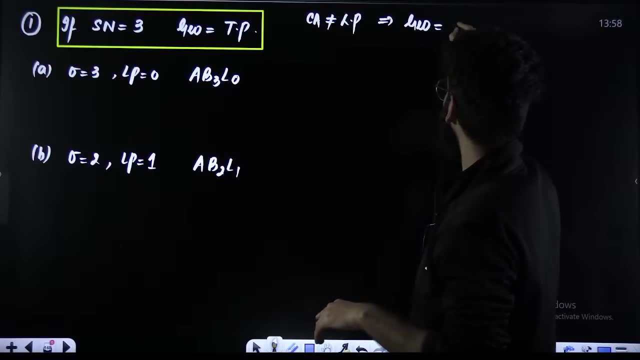 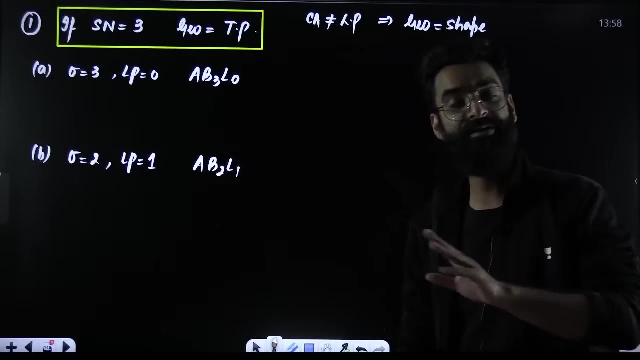 does not have any lone pair, does not have any lone pair at that point of time, whatever was the geometry predicted, the hybridization that is the actual shape of the molecule. so when geometry and shape are same, when central atom does not have any lone pair, right over here, 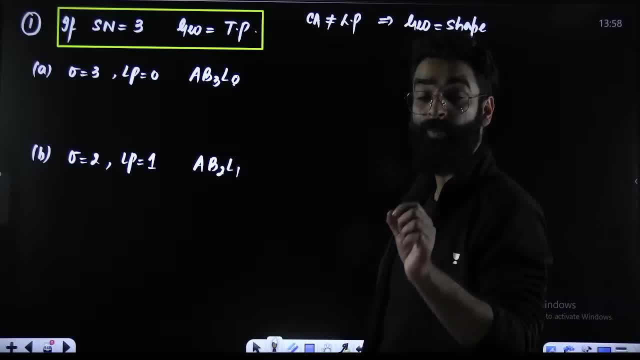 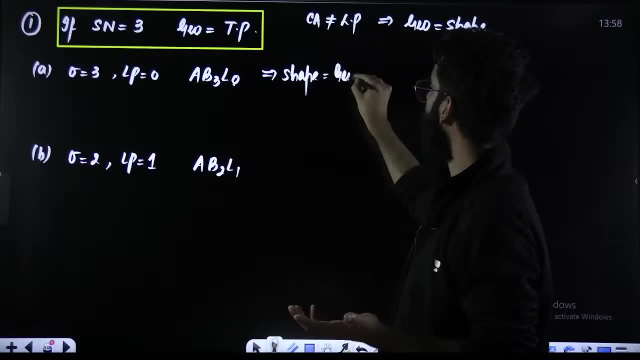 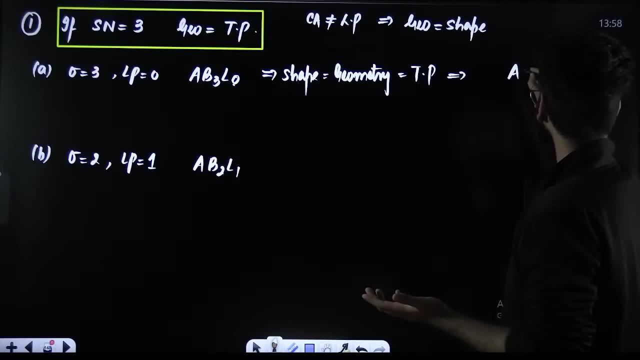 central atom is not having any lone pair l0. so geometry predicted through hybridization is the actual shape, right? i'll say, in this particular case, your shape geometry is same and both are what trigonal planar and how do you represent it? this is a, this is b, this is b and this is b. 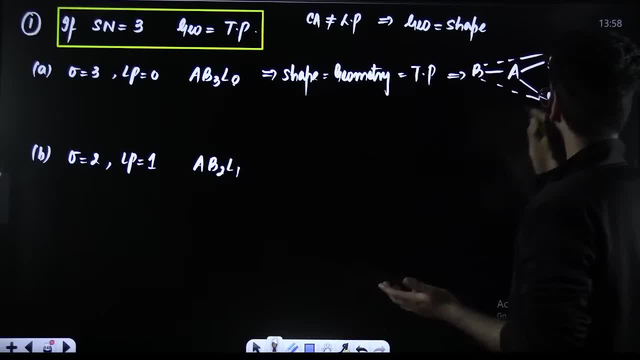 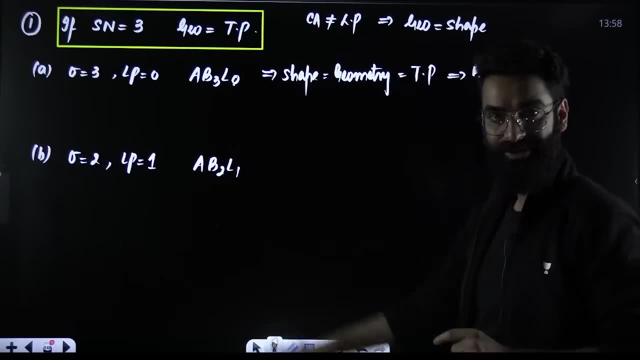 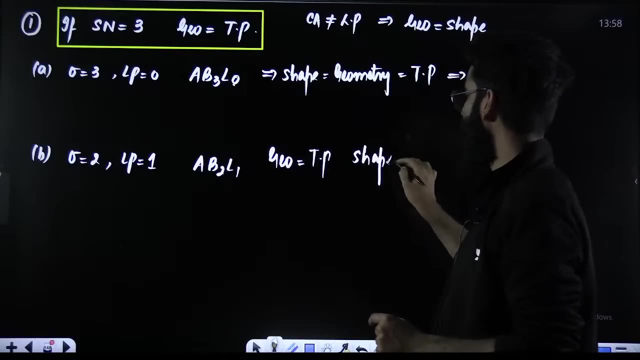 this is your trigonal planar geometry, am i clear? i should be clear: sigma, loan pair one. sigma two, loan pair. one loan pair one. what is the geometry which is predicted through hybridization? that is trigonal planar, but what about the shape? what about the shape? what about the shape? make the geometry first. geometry is 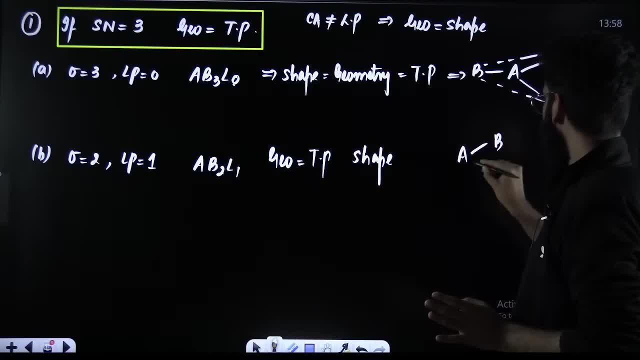 trigonal, Quindi planar, right. so this A, this B, this is B, this is B. I made the geometry right. this AB3C0 type. now do one thing: remove one of the bond pair and place a lone pair. remove one of the one pair of Omaha. 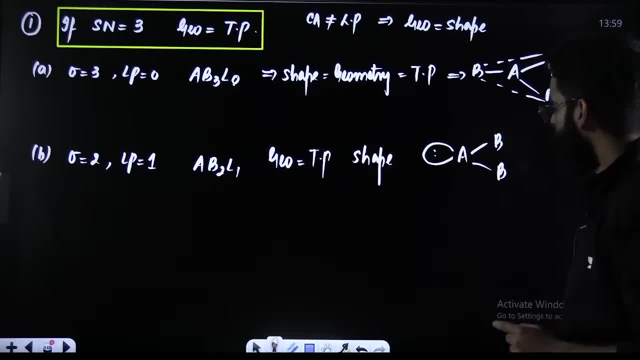 and place a lone pair. one pair plays a lone pair. So 2 sigma one lone pair, 2 sigma one lone pair. Now if I ask you, just hide this lone pair. When you hide this lone pair, how this molecule? 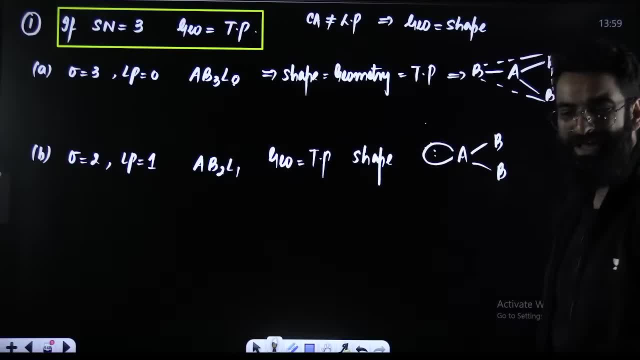 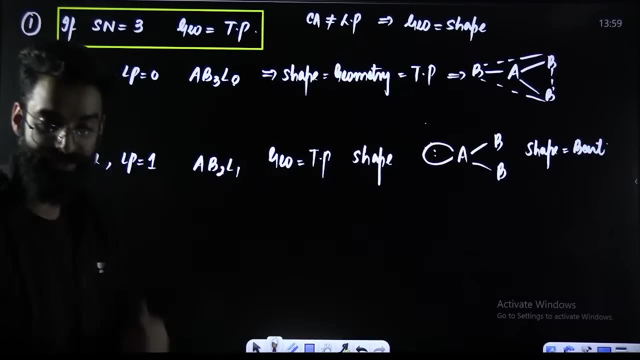 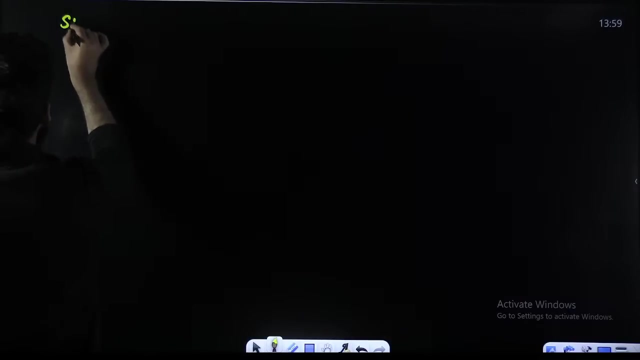 looks like When you hide this lone pair how this molecule looks like Bent. It looks bent, So its actual shape is bent. Am I clear with this? This was your first case wherein steric number is 3.. Wherein steric number is 3.. Right Second, Second, If steric number: is 4, hybridization will be sp3.. Geometry predicted through hybridization is tetrahedral. Geometry predicted through hybridization is tetrahedral. Now, now, now, Now, Understand, Understand people. When can be steric number 4?? There are few case which arise. First case, If there are. 4 sigma bonds and 0 lone pair. Second one: If there are 3 sigma bonds and 1 lone pair. Third one: If there are 2 sigma bonds and 2 lone pairs. In all these cases, steric number will be 4.. Right, In all these cases, steric number will be 4.. In the first one, what is? 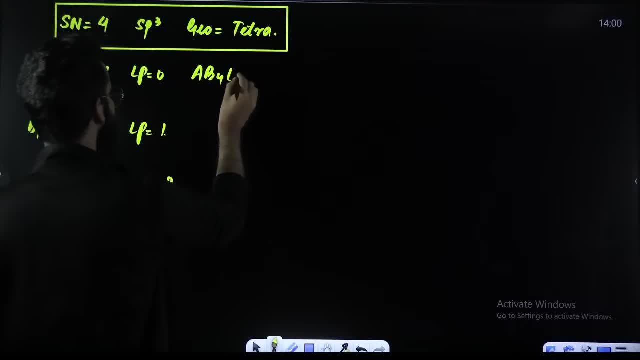 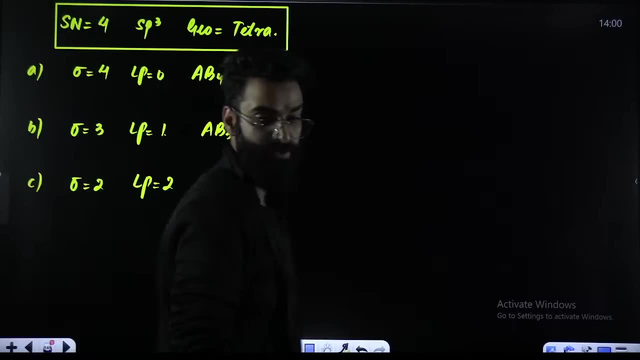 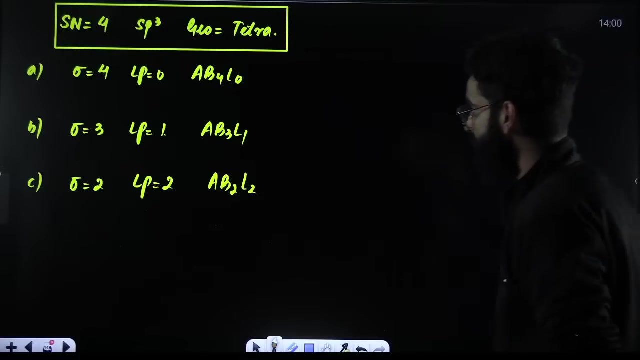 the type of the molecule. Type of the molecule: here will be AB4L0.. Here it is going to be AB3L1.. And here it is going to be AB2L2.. AB2L2.. Right, AB2L2.. AB2L2.. Now, people, let me ask you certain things Over here, lone. 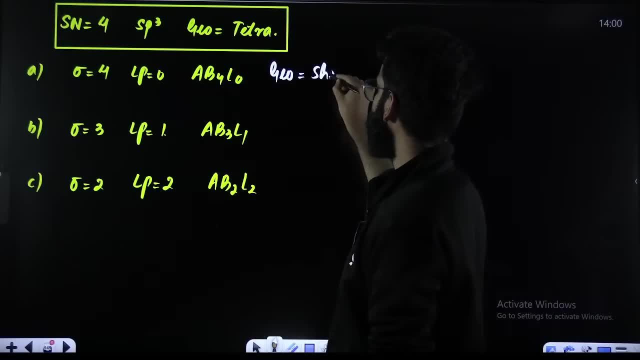 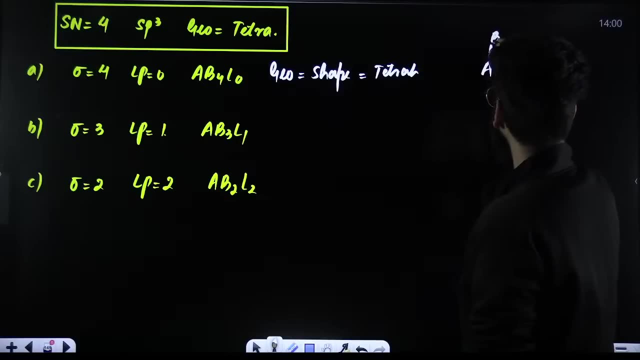 pairs are 0.. So geometry predicted through hybridization is basically the actual shape of the molecule and both are tetrahedral. And how do you show this tetrahedral molecule? This is A, This is B, This is B, This is B And this is B. So this is AB4. Tetrahedral. 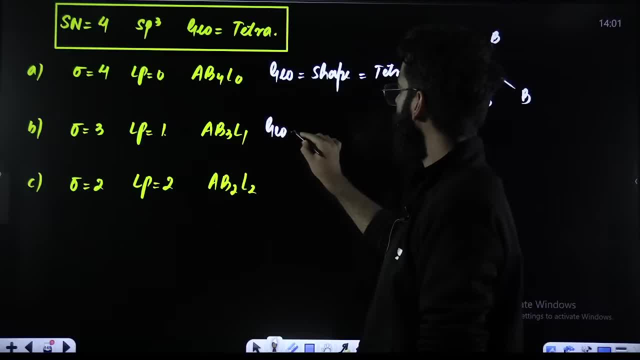 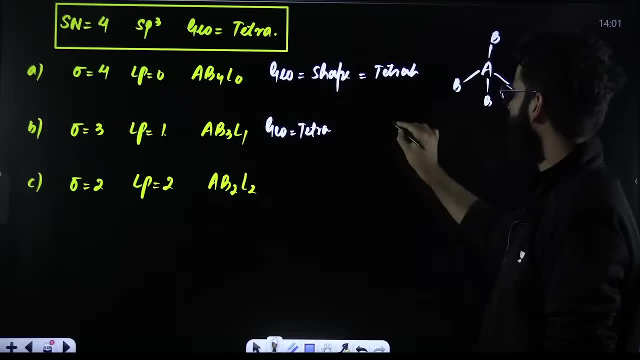 Okay, So AB3L1.. Geometry: already we know that is tetrahedral. But shape won't be tetrahedral because there is a lone pair associated with the central atom, Right? So how do you make the shape? Just do one thing: Make the geometry first. Make the geometry first, Now remove. 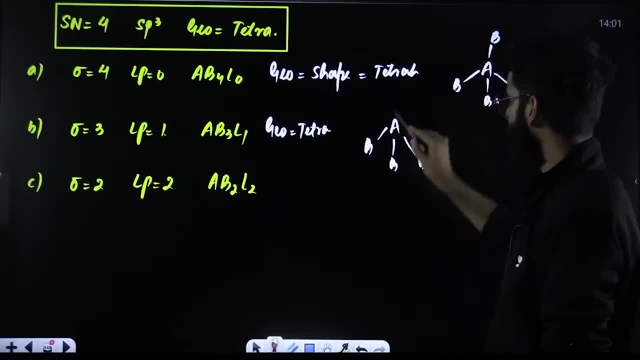 one lone pair. Remove one lone, Remove one bond pair And instead of that put a lone pair. Now do you see 3 sigma 1 lone pair. Just hide this lone pair. How it looks like. It looks like a pyramid Right. Actual shape of this particular molecule of the type AB3L1.. 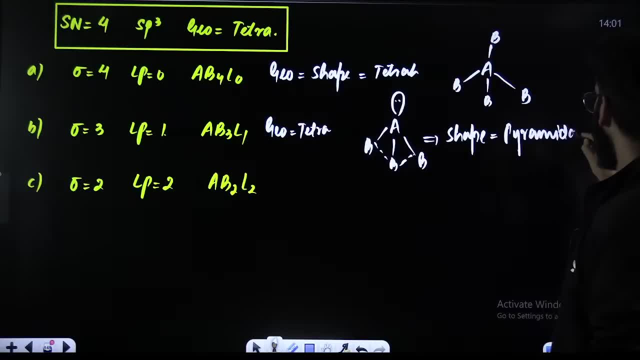 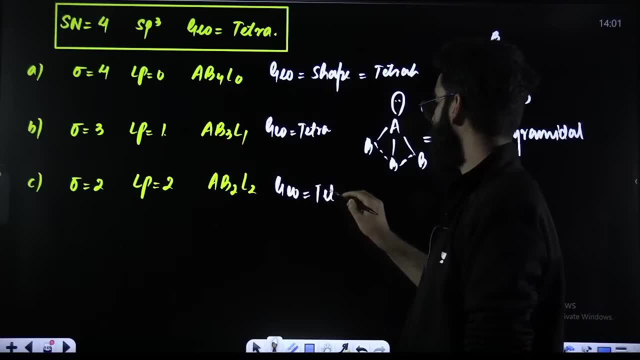 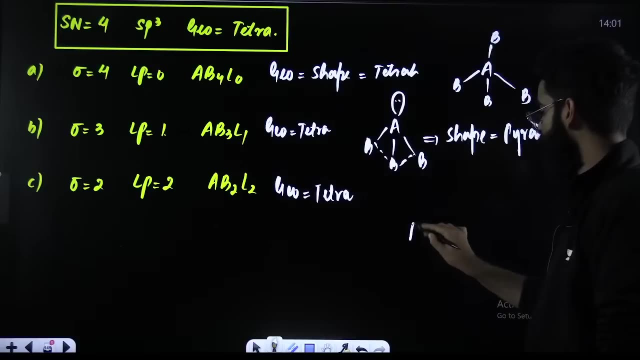 It is pyramidal, It is pyramidal Right, It is pyramidal, It is pyramidal: AB2L2.. Geometry is. Geometry is tetrahedral. Geometry is tetrahedral. What about the shape? Make the geometry first. 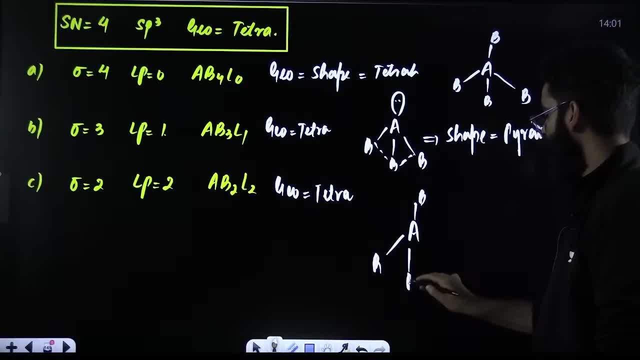 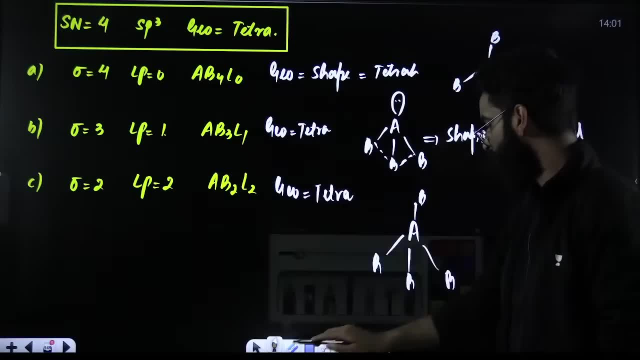 Make the geometry first. Right, Make the geometry first. There are 4 sigma, 0 lone pairs. Now I have to introduce two lone pairs. So I will be removing, I will be removing two, Two bond pairs and place two lone pairs. So this is A, For example, this is B, For example, this: 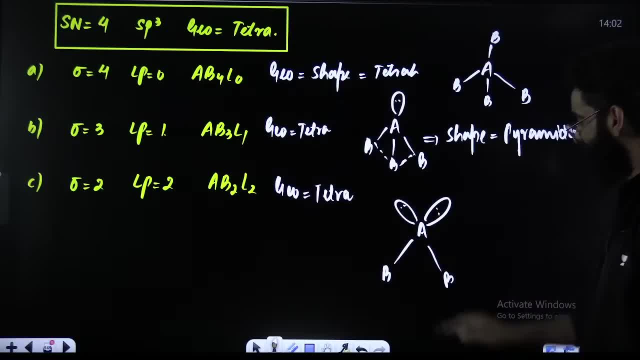 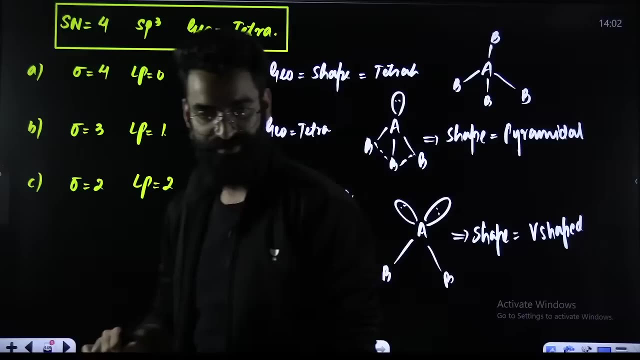 is B. One lone pair is here. One lone pair is here, Right. So this is AB2L2 type. What will be the actual shape? Actual shape of the molecule will be. What is it going to be? Quickly, It is V shaped. It is V shaped, Right. It is V shaped. 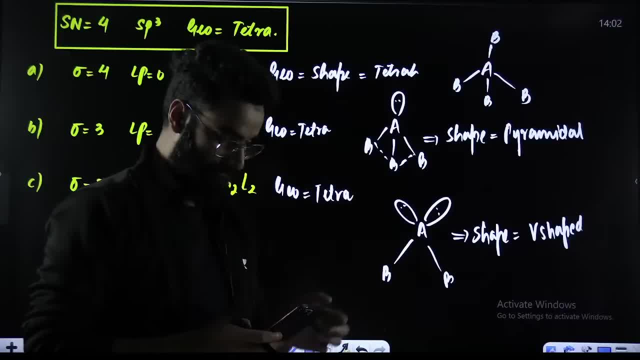 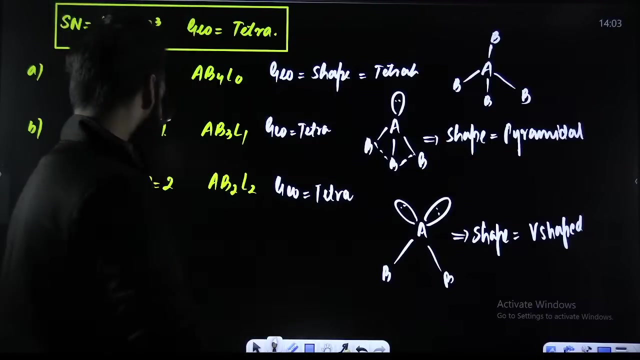 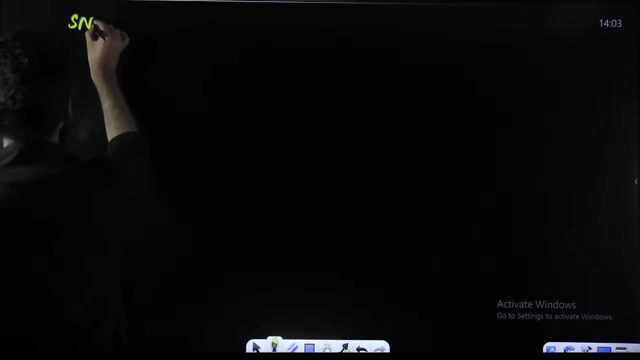 Yes, Yes, Yeah, Yes, V. Yes, That is it Alright, moving ahead. So this was your steric number 4, guys. okay, Now steric number 5.. Steric number 5.. Steric number 5 means: 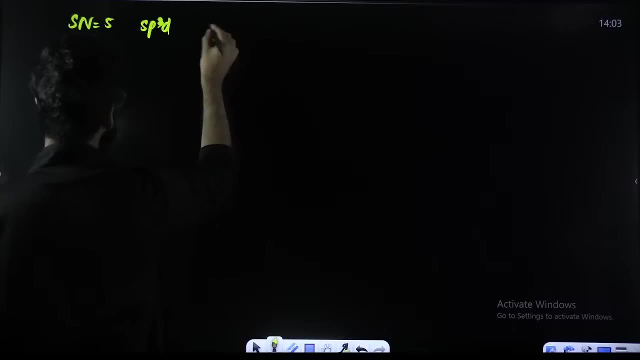 hybridization is sp3d right. Hybridization is sp3d Geometry, which is predicted through hybridization. That is trigonal bipyramid, That is trigonal bipyramidal. Now tell me the cases. people Tell me the cases. 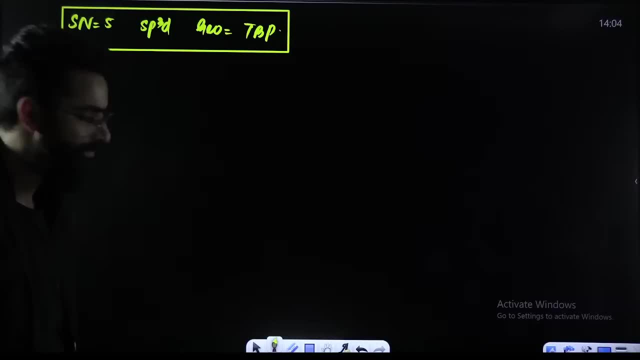 Tell me the cases quick. Tell me the cases. The first case which is involved here, That will be 5 sigma 0 lone pair. The second case which is involved: 4 sigma 1 lone pair. The third case which is involved: 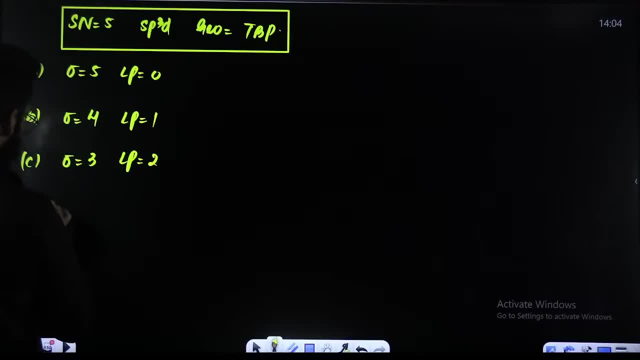 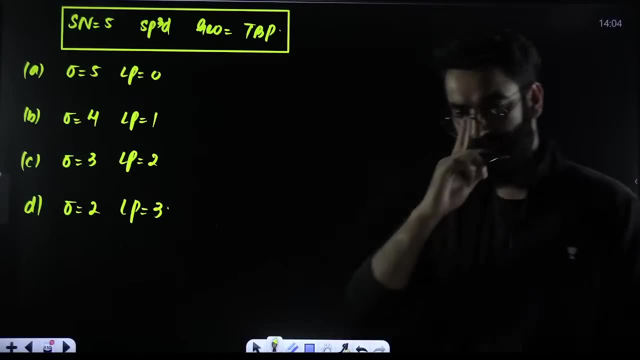 3 sigma, 2 lone pairs. The fourth case which is involved: 2 sigma and 3 lone pairs. These are the possible cases which arise over here. These are the possible cases which arise over here. Now, people, what is the type of this molecule? 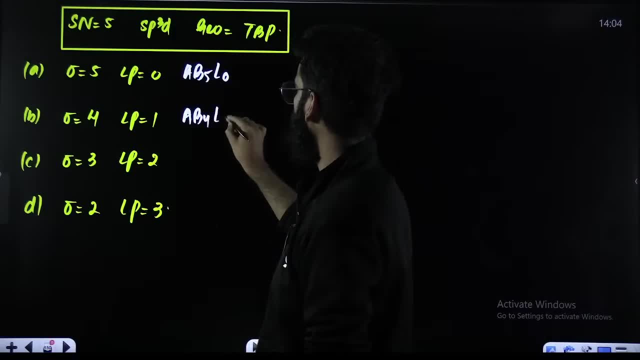 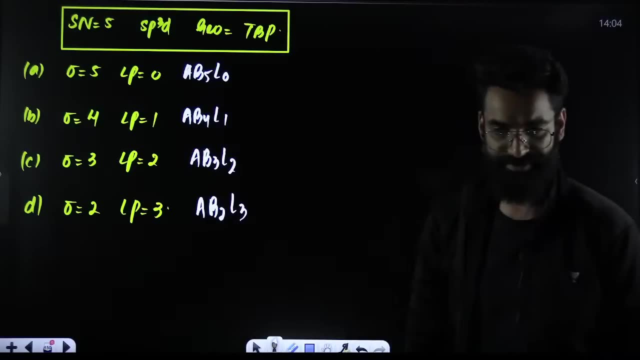 Tell me quickly: AB 5 L 0.. This is AB 4 L 1.. This is AB 3 L 2.. And this is AB 2 L 3.. Yes, Type is done. What is the geometry everywhere? 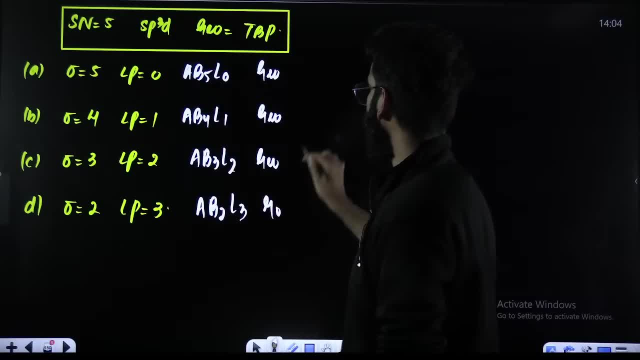 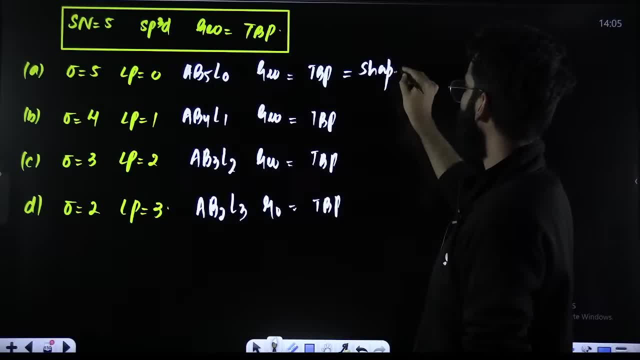 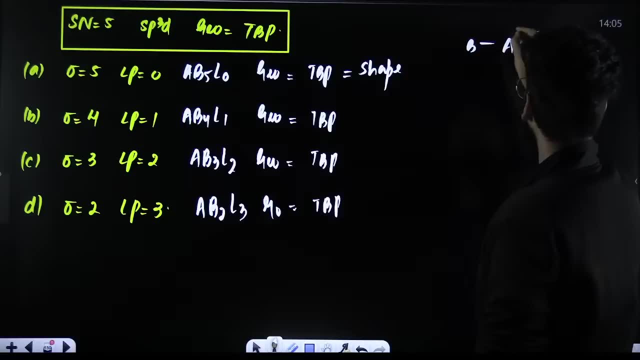 First one does not contain any lone pair, So it will be its actual shape as well And how you represent it. This is A. This is B. This is B. This is B, Present in the equatorial plane. One more B and one more B. 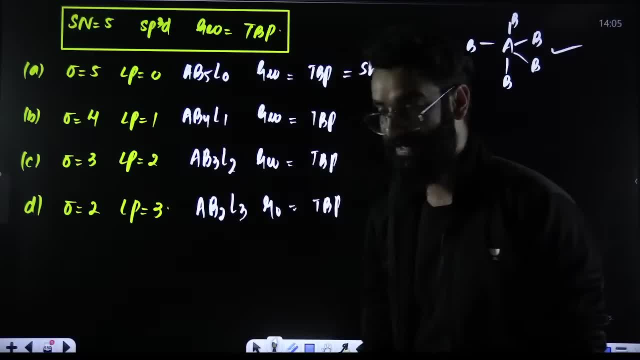 Right, This is your pentagonal trigonal bipyramidal geometry, Trigonal bipyramidal. Now what about the shape of this one? AB 4 L 1.. AB 4. AB 4 L 1.. 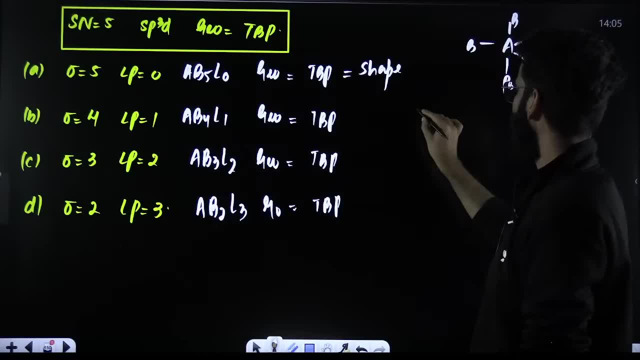 What do I do? I will remove one of the bond pair. here. Place a lone pair. I will remove one of the bond pair. here, Place a lone pair. See how I will remove one of the bond pair And instead of that I will place a lone pair. 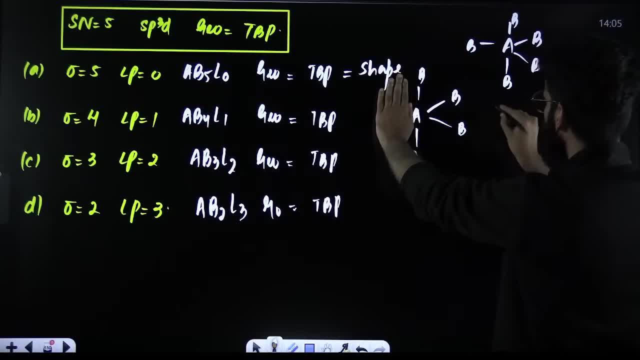 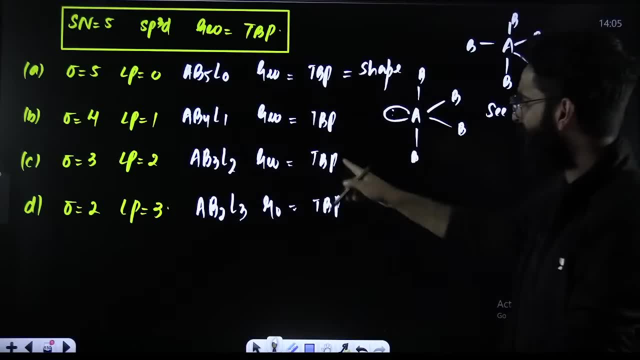 If you hide this lone pair, how it looks like. It looks like a seesaw shape, So it is a seesaw shaped one. It is a seesaw shaped Right. Look at this one: AB 3, L 2.. 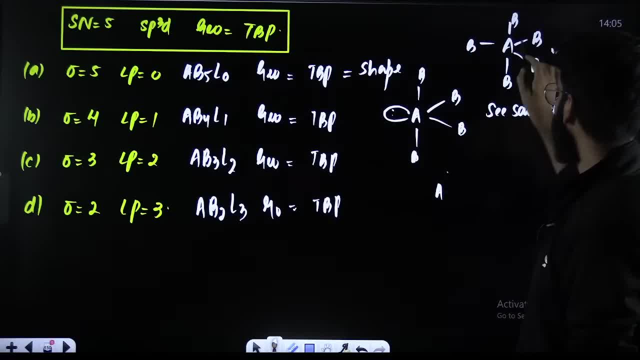 AB 3 L 2.. This is A Right: B 3 L 2.. AB 3 L 2.. So I will be doing what: AB 3 L 2.. I will be doing what I will be: removing two bond pairs and place two lone pairs there. 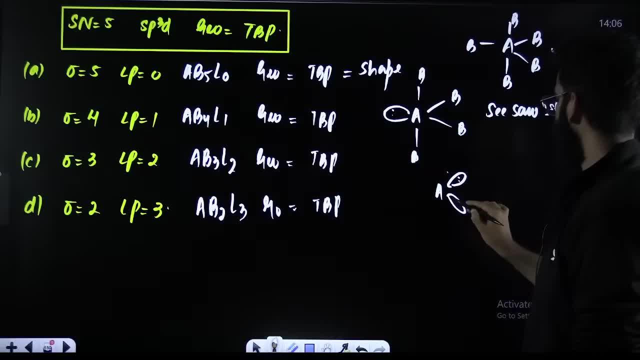 So let me remove these two bond pairs and place two lone pairs. This is AB 3, L 2.. Now hide these lone pairs. How it looks like? It looks like a T shaped molecule, So its actual shape is T shaped. 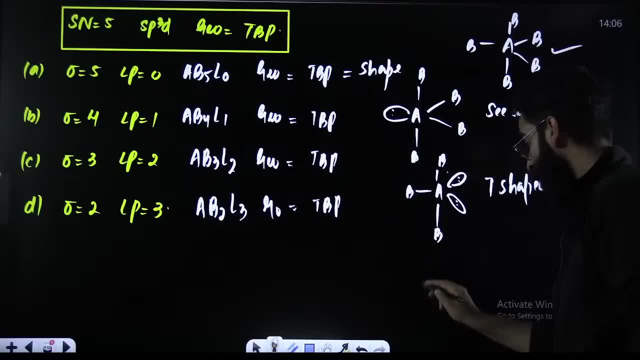 What about the next one? AB 3.. Sorry, AB 2, L 3.. AB 2, L 3.. This is A Right. AB 2, L 3.. So three lone pairs at the equatorial position. This is B and this is B. 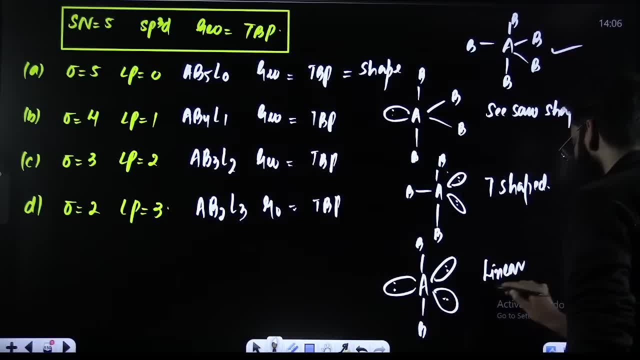 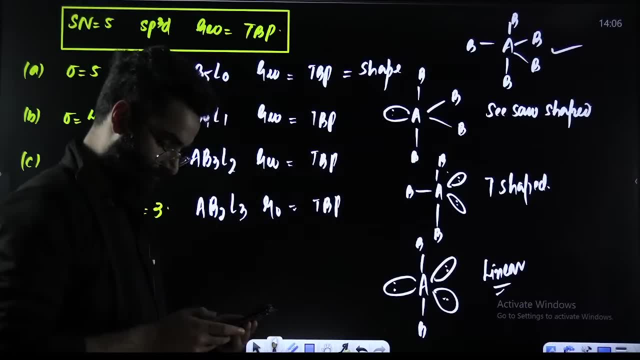 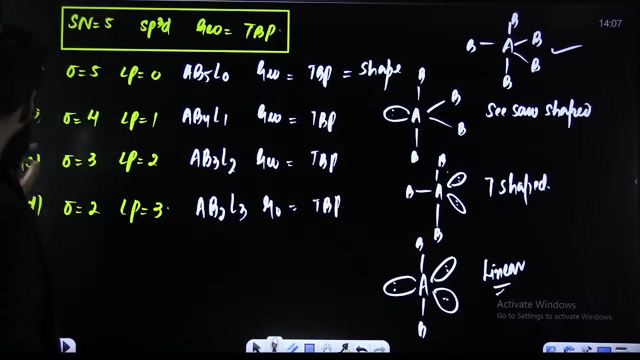 Hide these. It looks like linear. It is a linear one. Perfect, Its shape is linear. I hope I am clear. I hope I am clear to everyone. Done people Okay. So moving on to one more, This was steric number 5.. 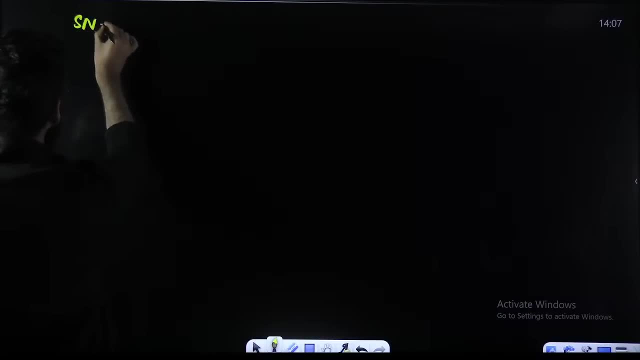 Now I am going to move on to steric number 6.. You tell me Steric number 6.. Tell me everything. Steric number 6. Hybridization. Quick In the charts. Steric number 6. Hybridization. 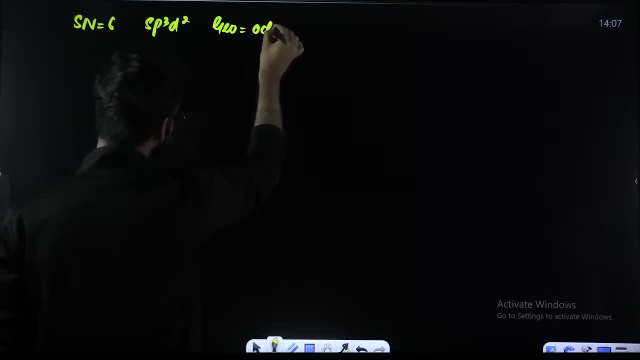 SP 3 D: 2. Geometry predicted through hybridization. That is, That is octet. right, That is octet. Now tell me what all possible cases arise here. What all possible cases arise here, people. The first one: 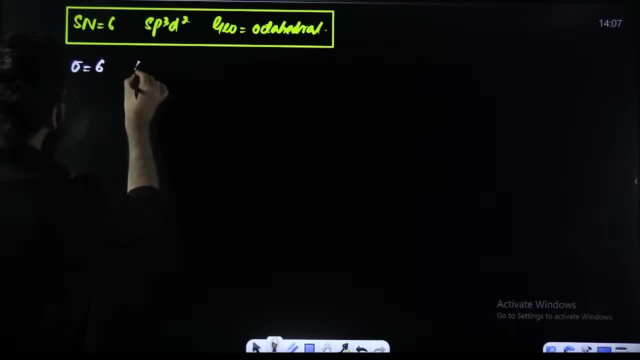 The first one, Sigma 6. Sigma 6. Lone pair 0.. Second one: Sigma 5. Lone pair 1.. Third one: Sigma 4. Lone pair 2.. These are the three possibilities which arise over here. 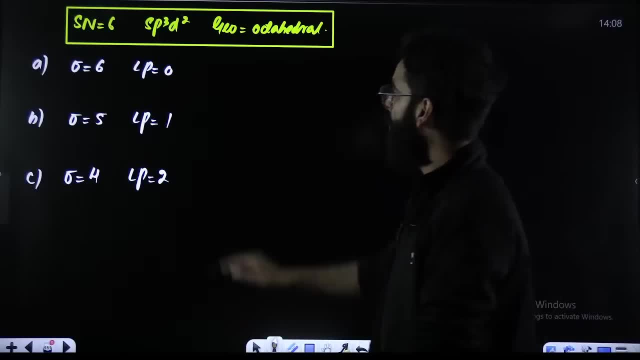 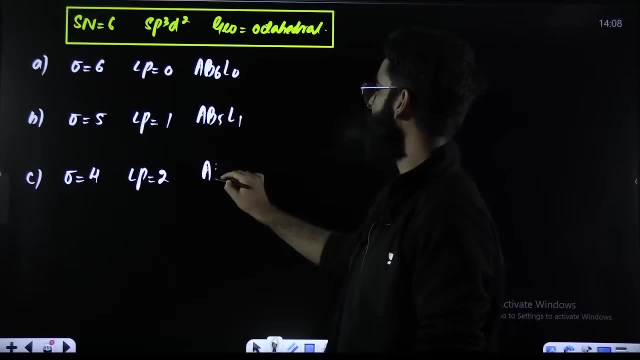 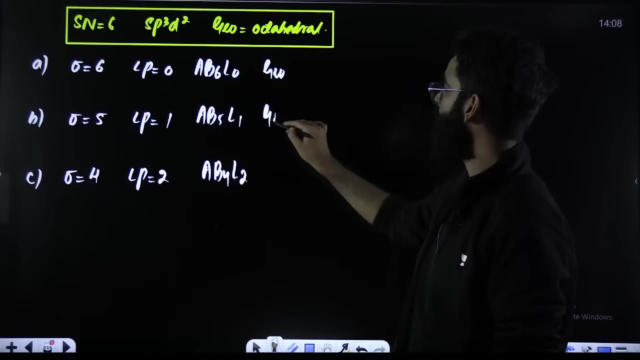 These are the three possibilities which arise over here Now. first thing, the type of this molecule is AB6L0.. This is AB5L1.. This is AB4L2.. Yes, Geometry, Geometry. What is the geometry which is predicted through hybridization? 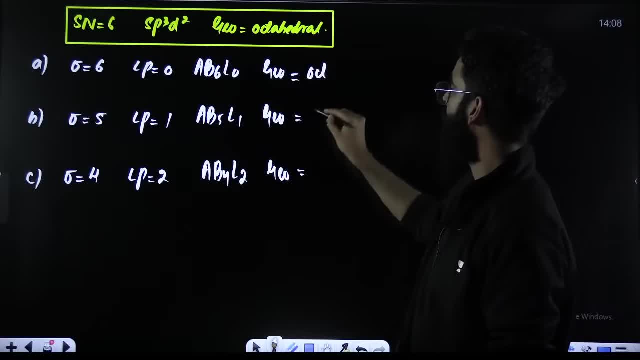 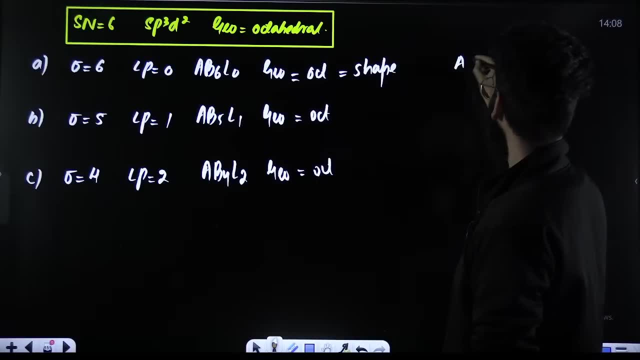 Everywhere, Geometry predicted through hybridization is octahedral, Octahedral, Octahedral Right. This is going to be its actual shape as well, because there is no lone pair. So this is A, This is B, This is B. 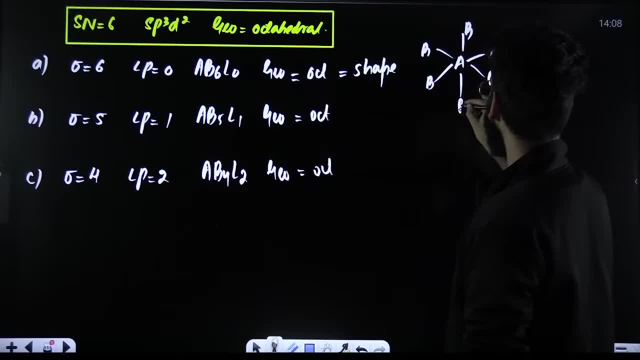 And this is B, This is B, This is B on this side, This is B on this side. This is octahedral geometry: right, Perfect. You know the equatorial axial, etc. etc. We have discussed that. 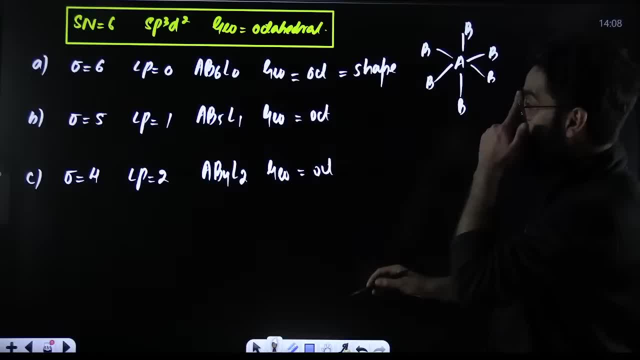 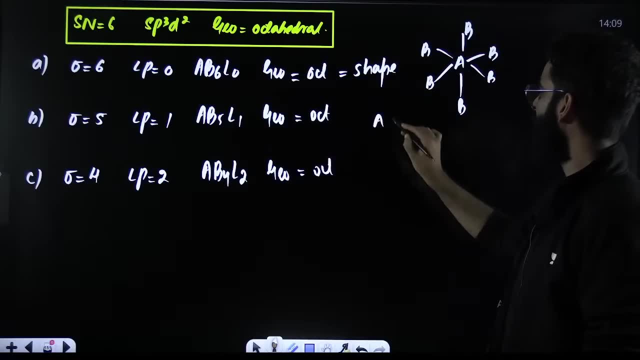 Now, guys, one thing Over here: AB5L1.. AB5L1.. What I'll be doing In the geometry: I'll be removing one of the bond pairs. Right, I'm removing one of the bond pairs. 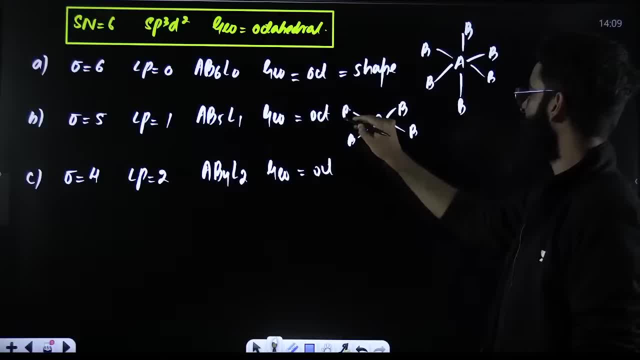 And in place of that, I'm keeping a lone pair. In place of that, I'm keeping a lone pair. In place of that, I'm keeping a lone pair. This is AB5L1.. How do you do this lone pair? 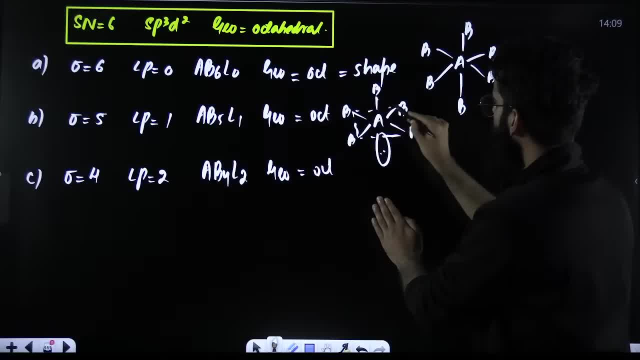 How it looks like. This is a square here in the equatorial plane. It is a square pyramid. Right It looks like a square pyramid, A square pyramidal shape, A square pyramidal shape, Now AB4L2.. 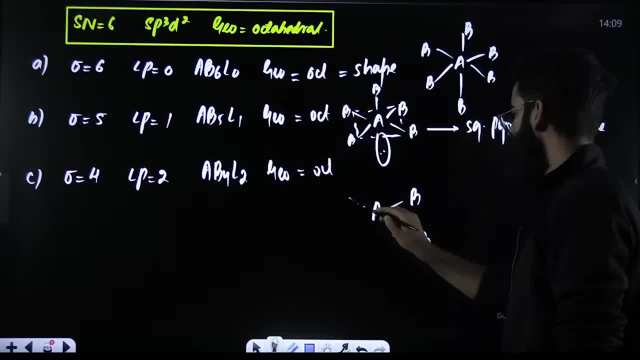 AB4L2.. This A, This is B, This is B, This is B And this is B. One lone pair here. One lone pair here. Hide these lone pairs How it looks like. It looks like a square planar shape. 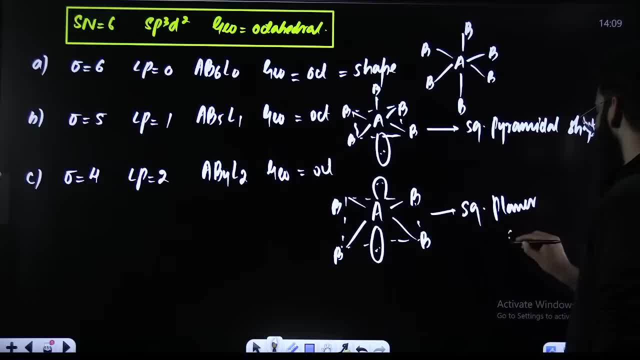 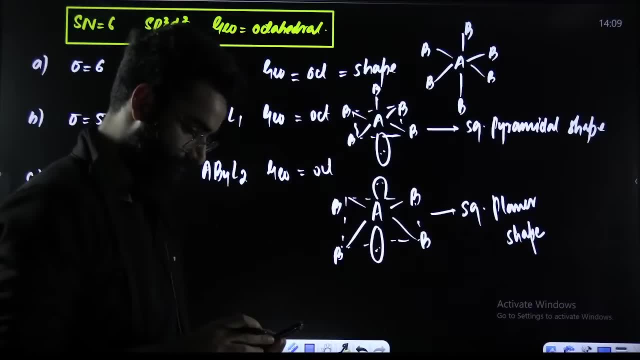 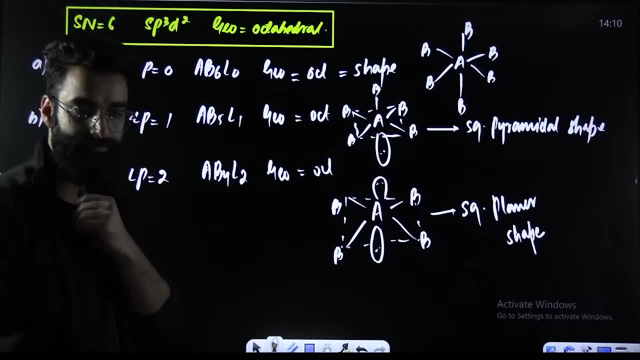 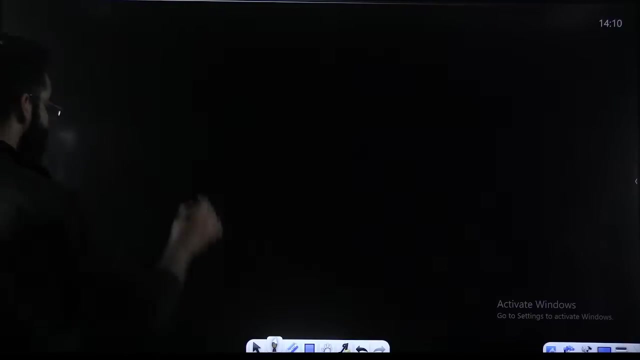 Right, It's a square planar shape. Square planar shape. Yes, Yes, It's a square planar shape, Perfect. Now comes the last, That is steric number 7.. Steric number 7.. Hybridization- SP3D3.. 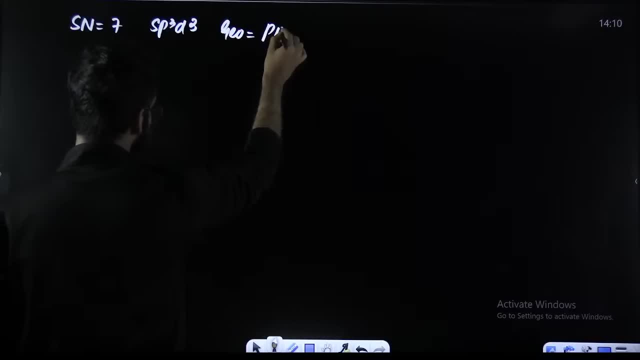 SP3D3.. Geometry is going to be positive. It's going to be pentagonal bipyramidal. Geometry is going to be pentagonal bipyramidal. Now, the first case here. The first case here, First case: 7 sigma. 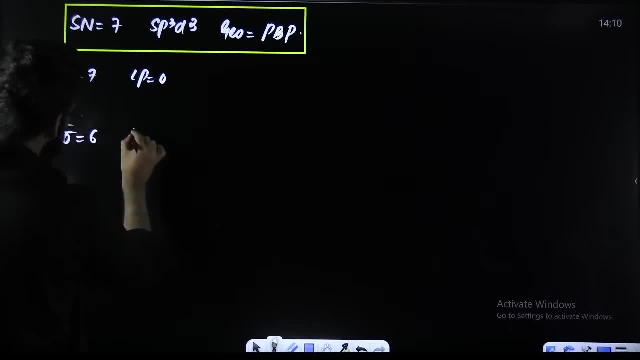 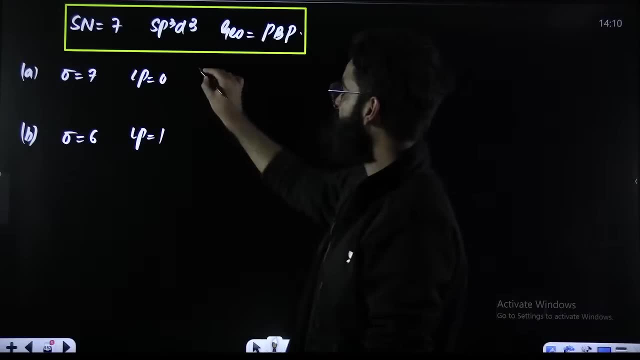 Zero lone pair. Second one is 6 sigma One lone pair. These are the two cases which arise here. These are the two cases which arise here. Tell me the type. first of all, This is AB7L0.. This is AB6L1. 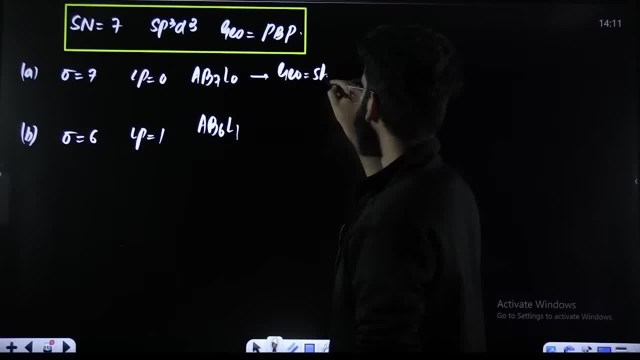 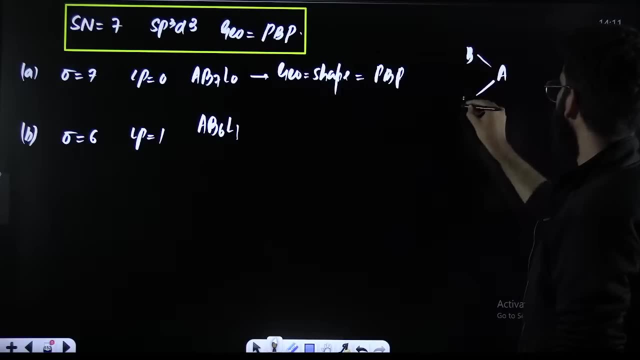 Over here. geometry and shape, both are pentagonal, bipyramidal. This is A, This is, for example, B, This is B, This is B, This is B And this is B, So it looks like a plane now. 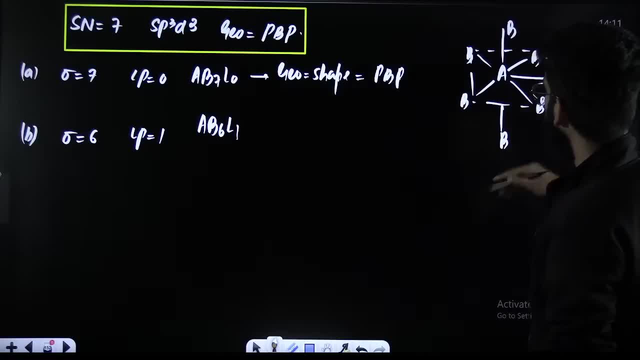 This is one B here, One B here. So pentagonal bipyramidal: One pyramid from the top, One from the bottom. Okay, Perfect, Now AB6L1.. So remove one of the bond pair. Remove one of the bond pair and place a lone pair. 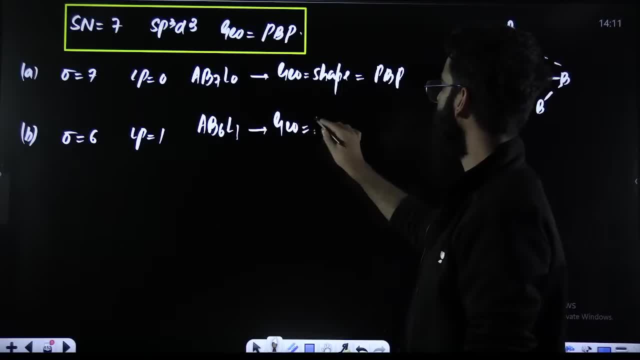 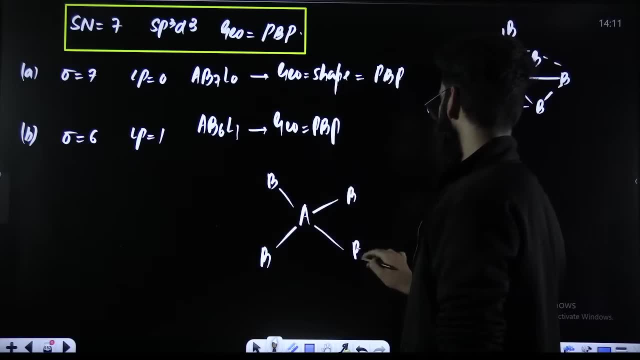 Right, Remove. see first of all geometry over here is pentagonal bipyramidal. What about the actual shape? This is A, This is B here. This is B, This is B, This is B. Right Place, a lone pair now. 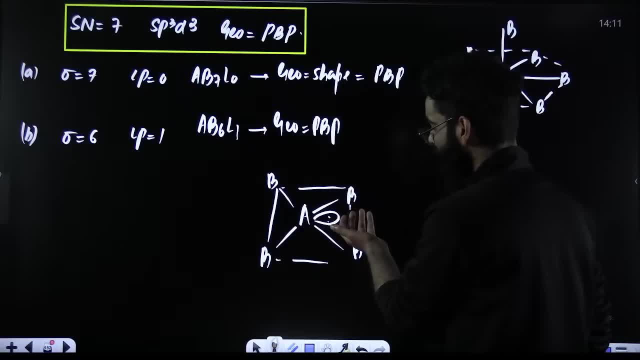 Lone pair will be here. But lone pair won't be present on this plane Right. It will be above or below the plane. Lone pair will be above or below the plane Right. Lone pair will be above or below the plane. It won't be present on the same plane. 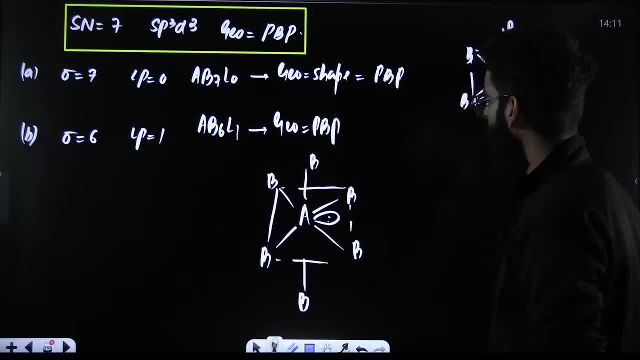 So this is AB6L1.. B over here. this is B over here. how it looks like. how it looks like hide, this lone pair. it looks like octahedron and we call this as distorted octahedron. distorted octahedron. 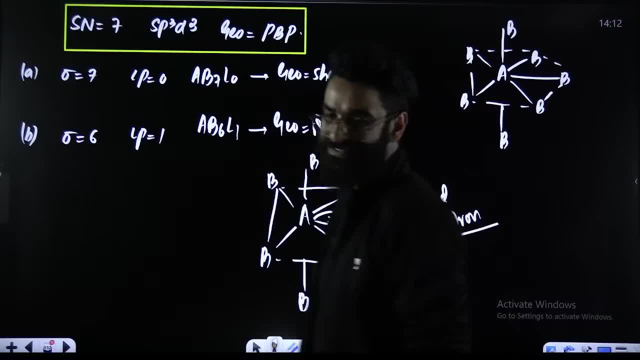 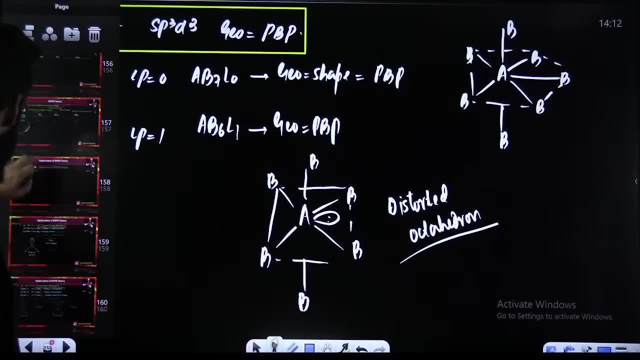 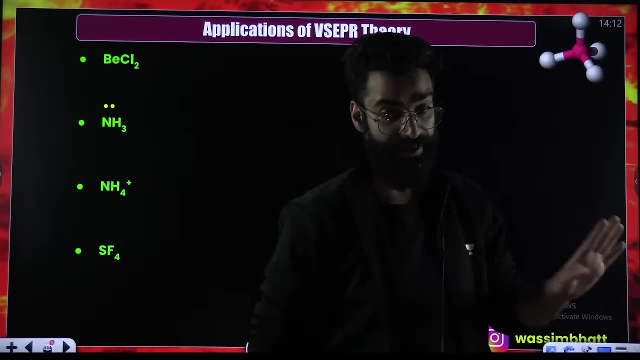 right guys. tell me now: if any question is asked from this, will you be able to solve it? will you be able to solve it? will you be able to solve it quickly? if yes, tell me the answer of all these: everything, everything, everything, everything, Bcl2 quick. 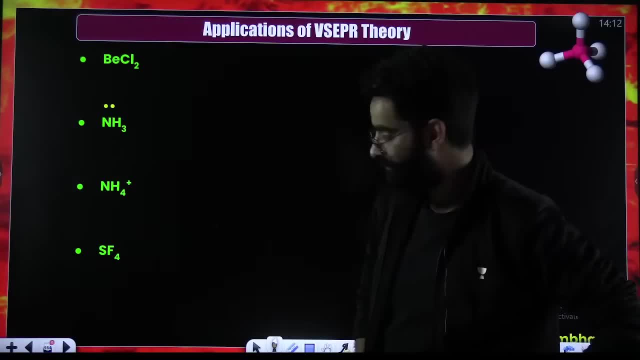 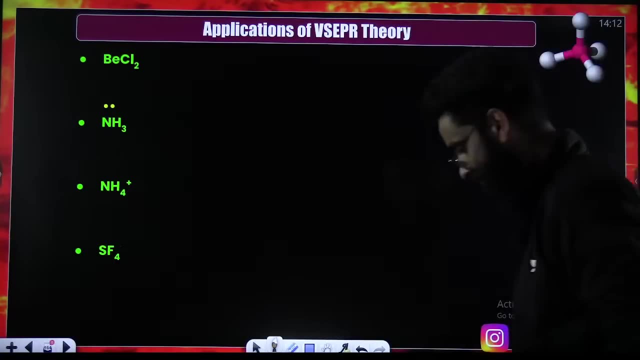 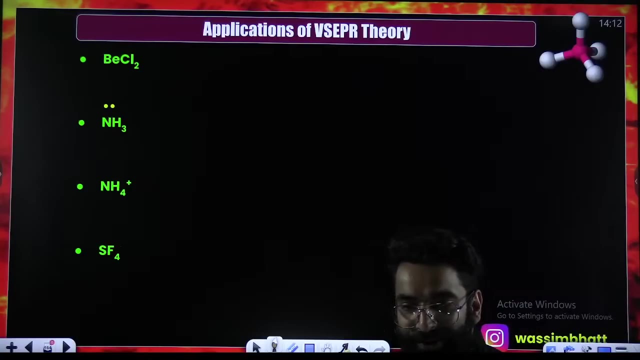 let me sit for two minutes and solve right. so someone is asking why this is happening. why that is happening. you do not have time for why. right now, whatever, imagine you are telling you remember it. okay. bcl2- if you have got bcl2 guys, bcl2 first of all, how many sigma? 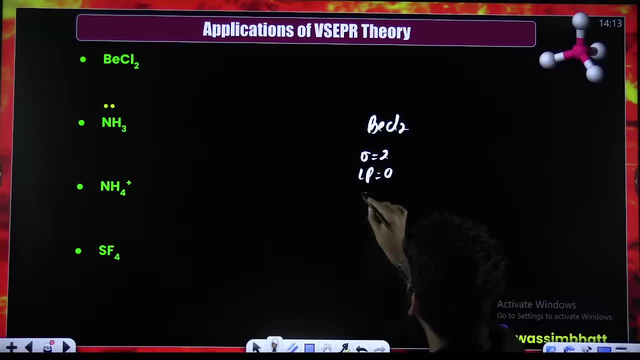 1s, 2 sigma 1s. how many lone pairs? how many lone pairs: 0 lone pair steric number. steric number is 2. type of the molecule is ab2l0. ab2l0 geometry predated through hybridization, that is, that is. 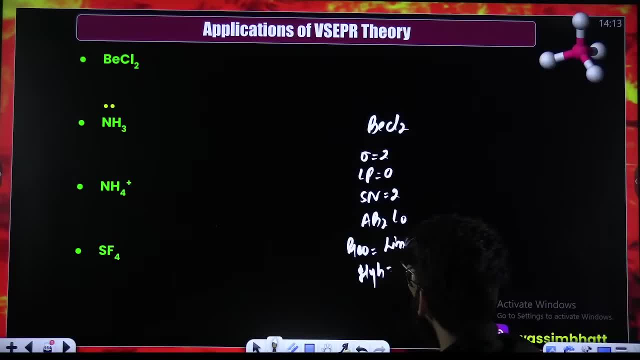 linear. hybridization is sp. central atom does not have any lone pair, right? so shape also is. shape also is linear. so all these things can be done now. all these things can be done now easily, easily, guys, right right. for example, you have got sf4. for example, you have got 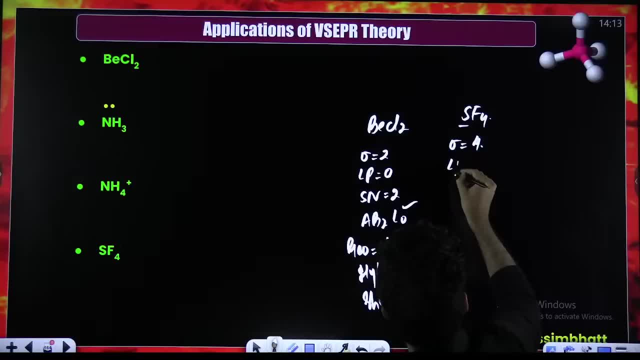 sf4. how many sigma it's forming? 4 sigma. how many lone pairs on sulfur? 1 lone pair. steric number 4 plus 1, 5. hybridization: sp 3d geometry: a trigonal bipyramidal type of the molecule: ab4l1- ab4l1 shape: shape: ab4l1 is seesaw shaped, correct. yes. 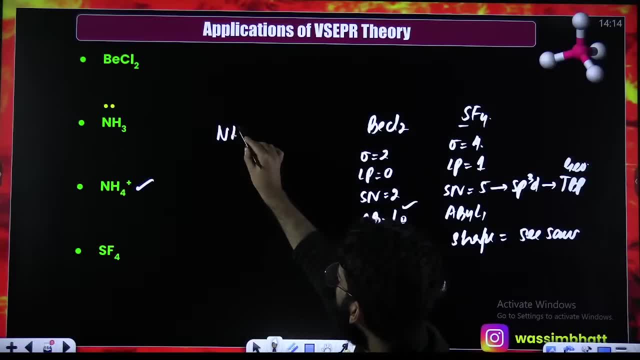 what else do we have? let's say we have got nh4 positive. nh4 positive. if i ask you how many valence electrons with nitrogen, it has 5, but there's a positive charge. so 5, 5 is 4.. sigma bonds are 4.. 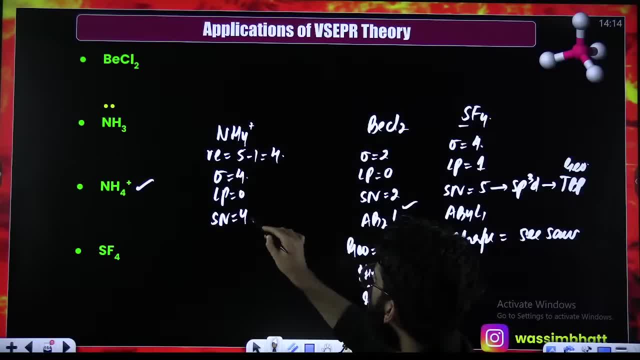 right. sigma bonds: 0. steric number: 4 plus 0, 4. hybridization, sp 3. type of the molecule: ab4l0- ab4l0. geometry: predated through hybridization: that is tetrahedral. shape, actual shape: that is also tetrahedral. 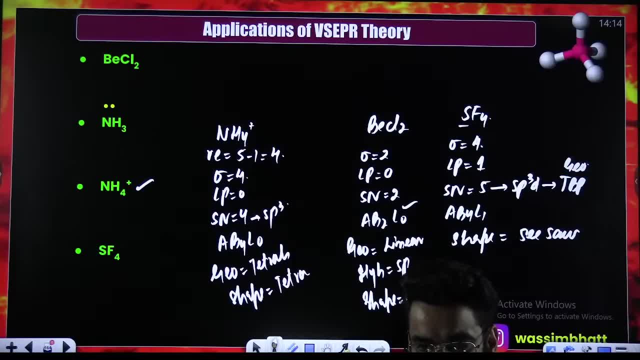 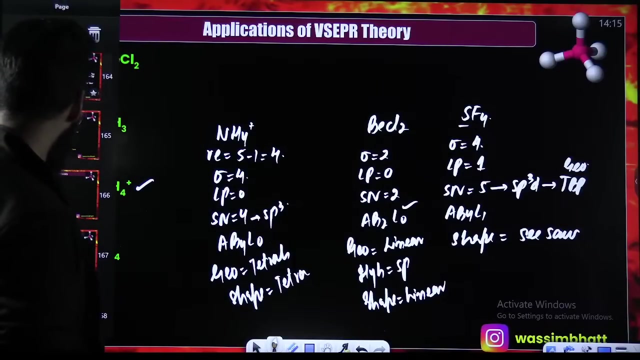 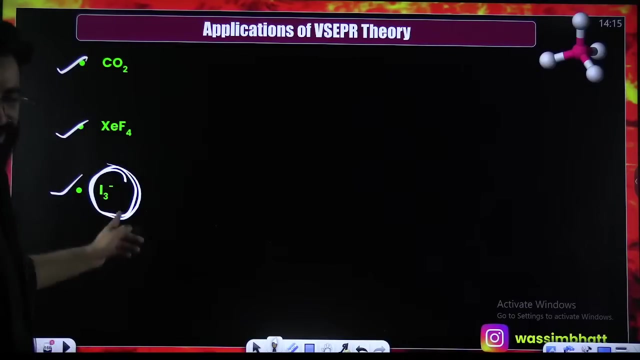 so i believe all these type of questions you can do now. is it looking easy? now, trust me, if you got to know how to do this, you are done. yeah, perfect, perfect, perfect. these three are all asked questions in your net. and je- this has been many times repeated in james- i3 negative. give me all the data about i3 negative. see these two. you can. 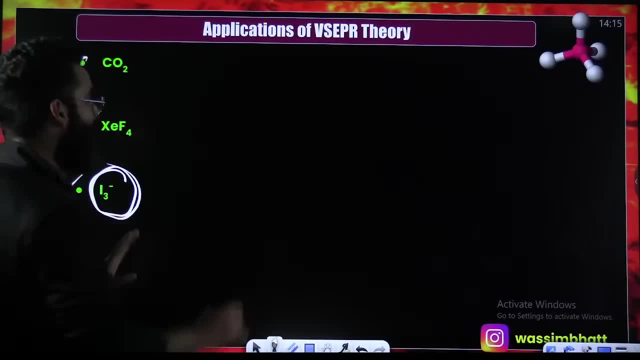 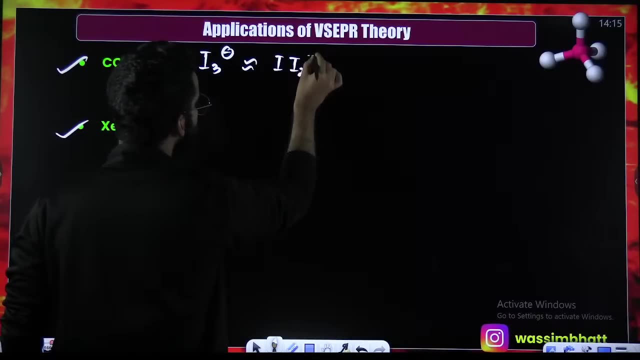 do easily. we have done them. i3 negative: give me all the data about i3 negative. first of all: i3 negative. you can write it like this: i i2 negative. you can write it like this: i i2 negative, correct? yes, now call this a central atom. how many valence electrons? seven. there is a negative charge, so seven. 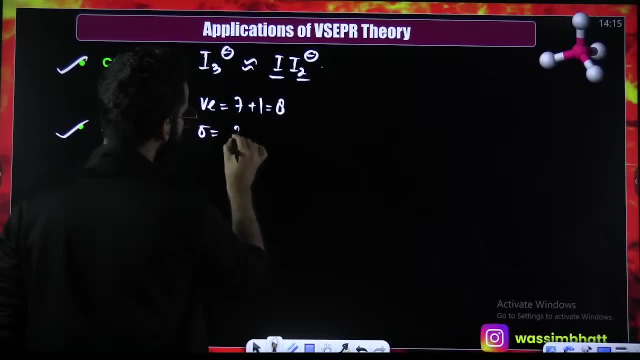 plus one is eight. okay, sigma bonds: two lone pairs out of eight. two are used, so six will be as such, in the form of three lone pairs. steric number: t plus two, five. hybridization: sp3d- right type of molecule. a, b to l3 geometry predicted through hybridization. uh geometry predicted through hybridization. 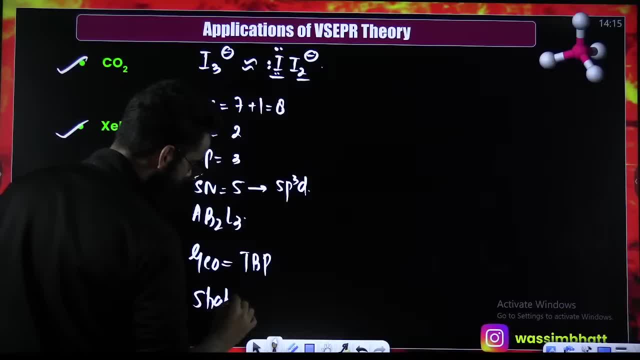 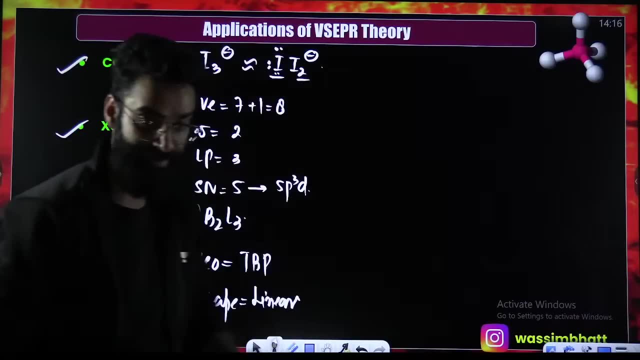 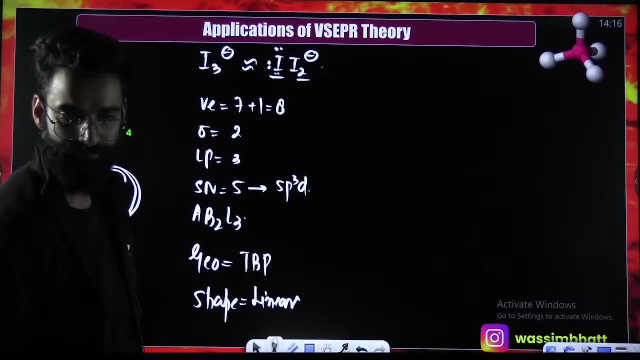 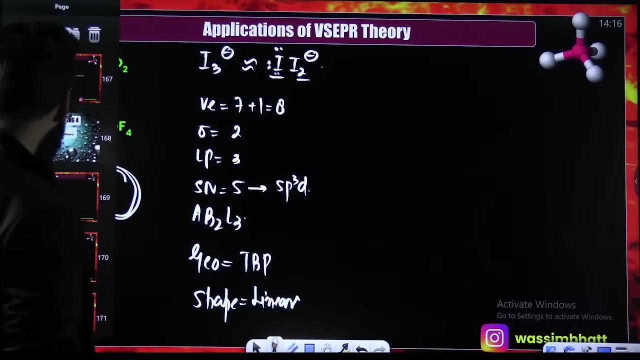 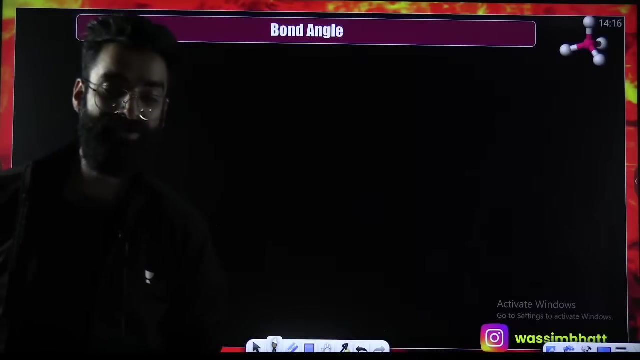 trigonal bipyramidal actual shape, actual shape, a, b to l3 means linear. yes, am i clear? am i clear? am i clear? quick, right people, now, now. now, a sure short question, a sure short question which is asked about the bond angle, which is asked about bond angle. here, i am going to give you one table, guys. 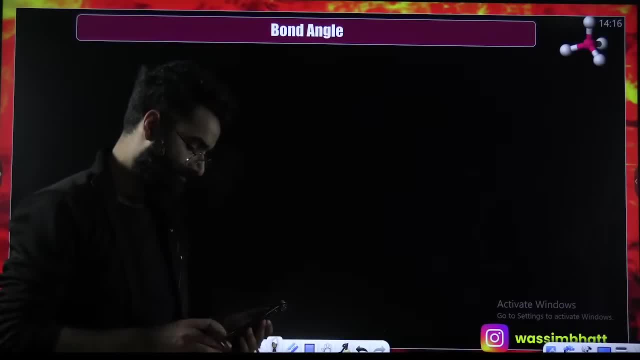 here, i'm going to give you one table. just remember that. just remember that table. i am going to give you one table and you need to remember that. and whenever a question is asked from from the one angle, you are done. yeah, your life is sorted if you remember that table. 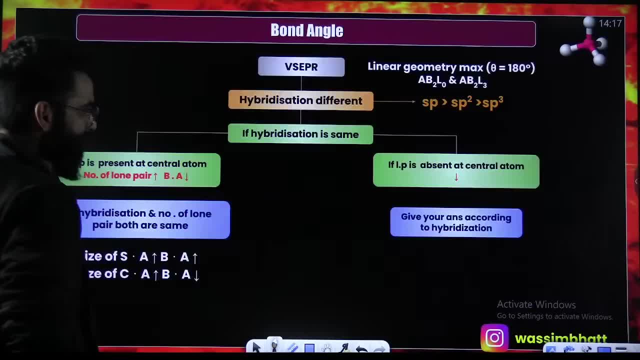 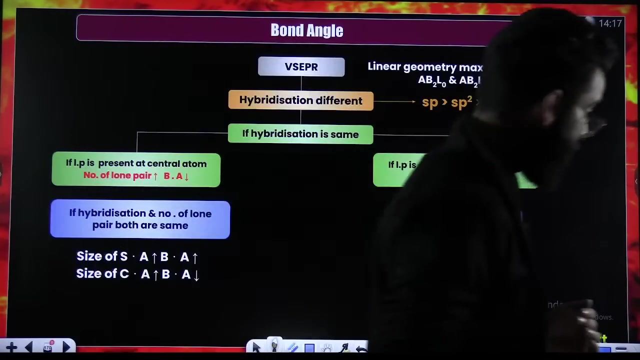 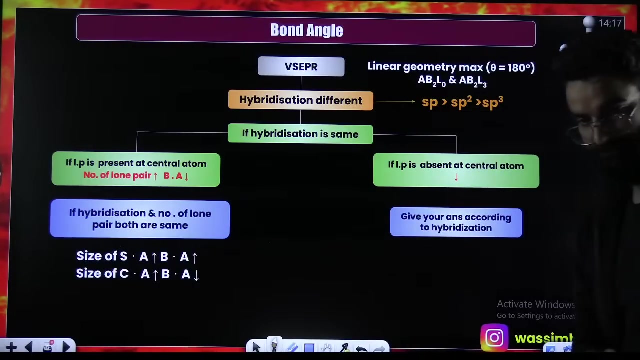 okay. so look at this table carefully, guys. look at this particular table carefully. look at this particular table carefully. this table is used when a question is asked about the bond angle. when a question is asked about the bond angle, just give me a second why there is no electricity. 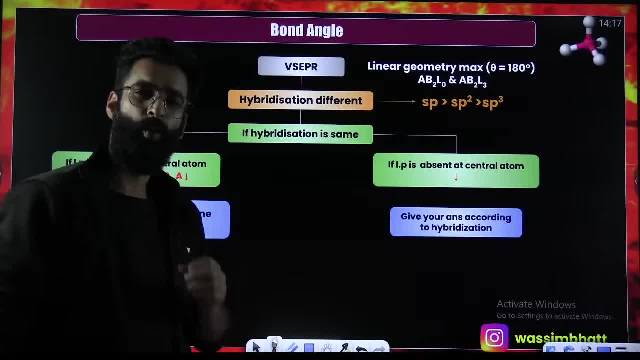 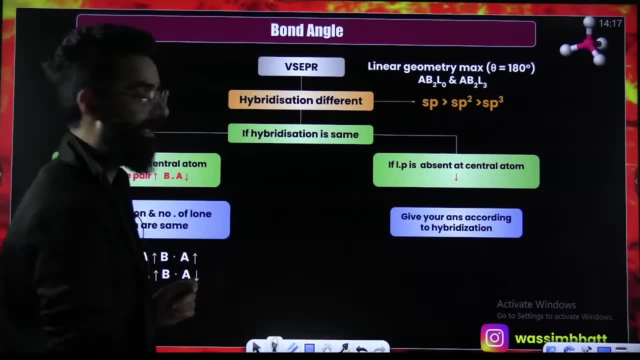 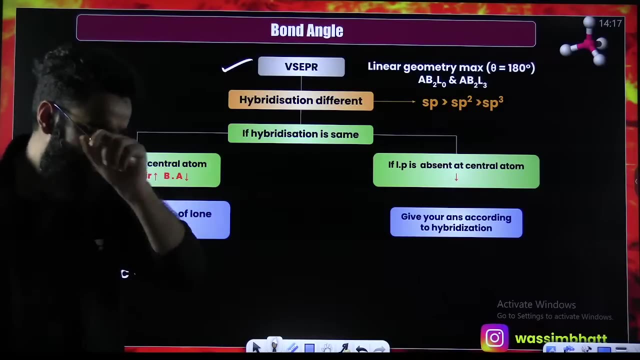 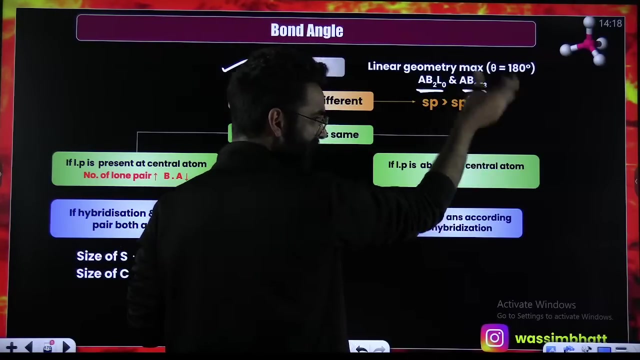 okay, my dear students, whenever you have to compare the bond angles, whenever you have to compare the bond angles, first thing that should strike your mind: vscpr, first thing, vscpr. so whatever molecules will be given with first check, is there any molecule of the type ab2l0 or ab2l3? if there was any molecule of the type ab2l0, ab2l3, they will have maximum. 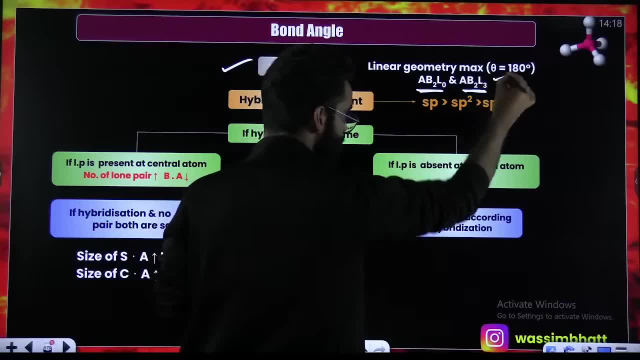 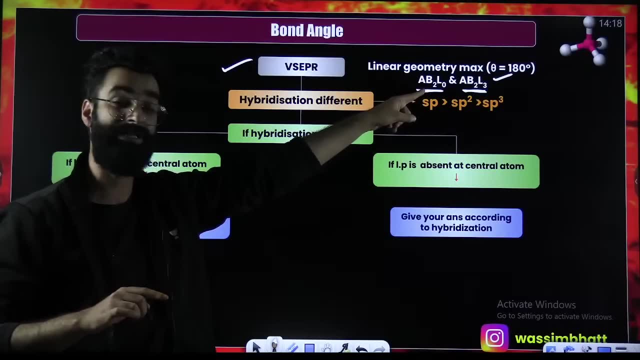 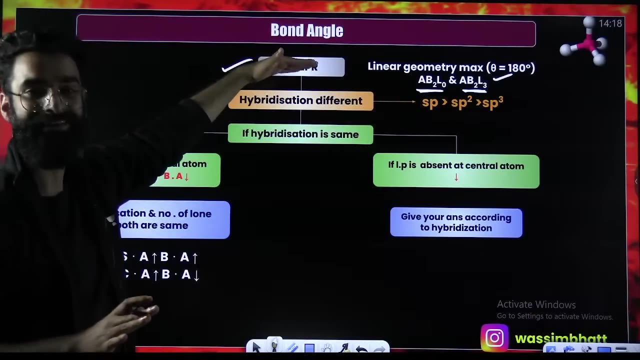 bond angle of 180, they'll have maximum bonding of 180.. first you need to check through vscpr. if you see any molecule of the type ab2l0 or ab2l3, maximum bond angle of 180, right right. then if you are unable to decide from vscpr. 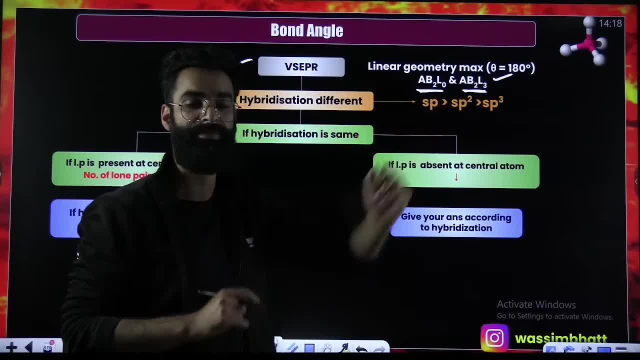 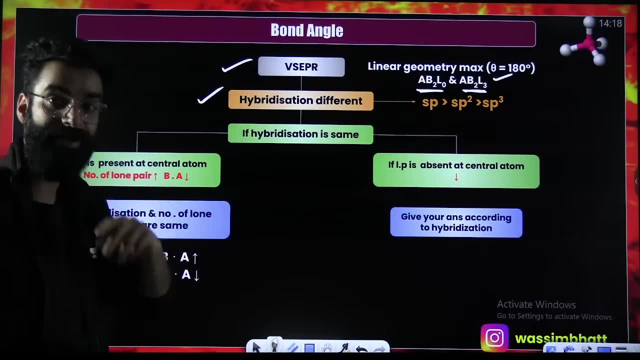 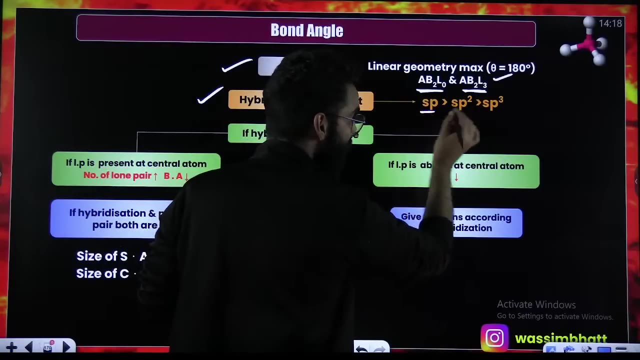 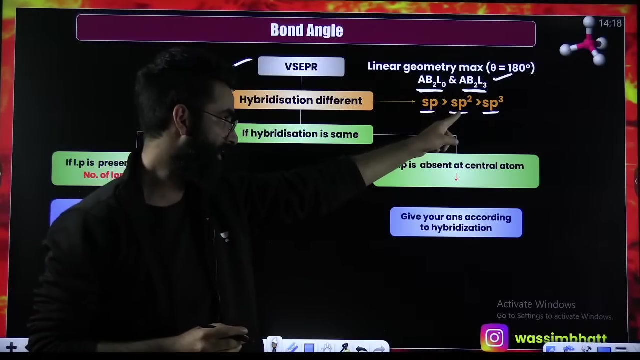 if there was no molecule which of which was of the type ab2l0, ab2l3, then you will move on to hybridization. then you will move on to hybridization, right? if hybridization of the molecules were different, you know, in sp 180, sp2, 120, sp3, 109, right? then sp will have maximum one angle, followed by sp2. 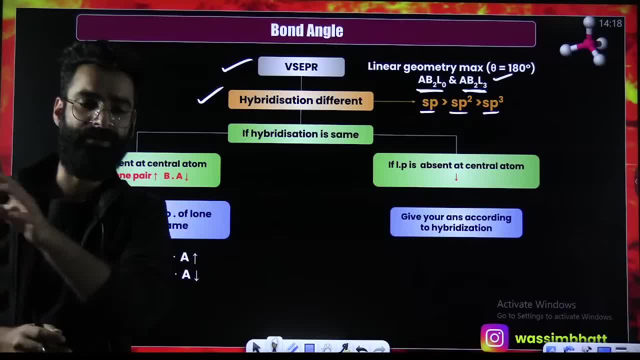 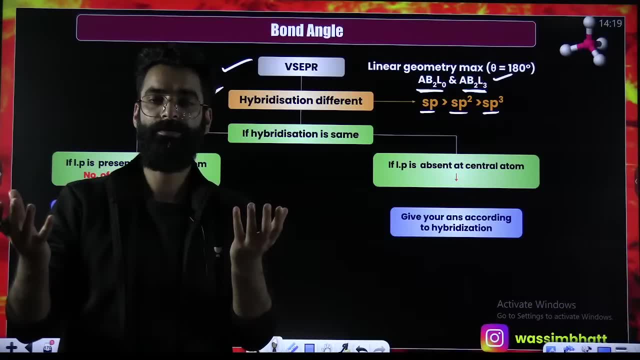 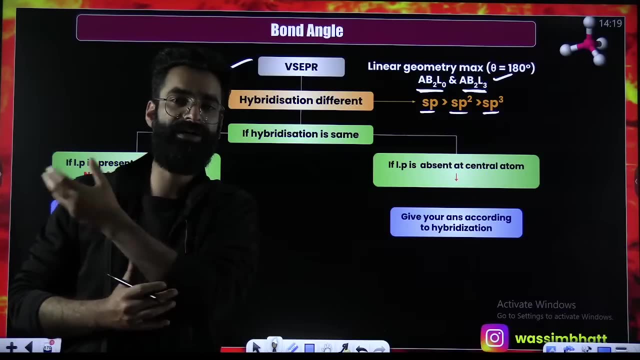 followed by sp3. if hybridization of the central atom is different, you're- let's say you're- given three molecules. i'm showing you examples in some time. if you are given three molecules and you calculated the hybridization of the central atom everywhere, right, if one central atom has got sp, another one has got sp2, another one is going to sp3. sp will have maximum bond angle. 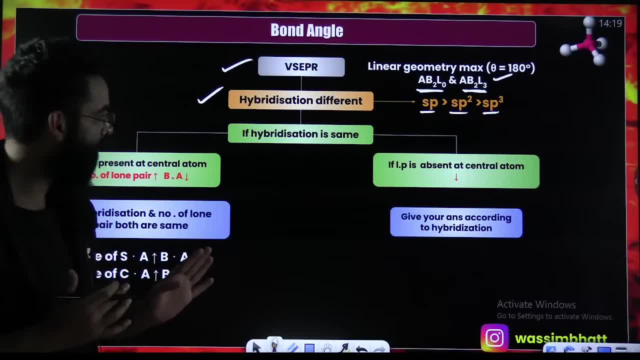 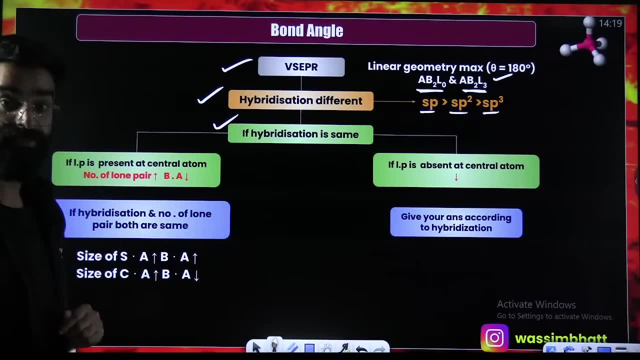 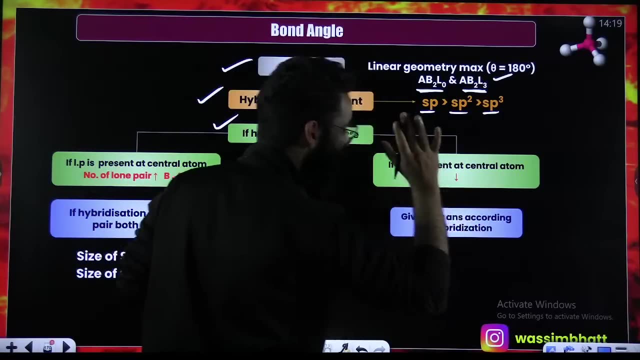 right sp will have maximum bond angle. yeah, now, if hybridization is different, if hybridization is different, if hybridization is different, then i break it into two parts. then i break it in two parts. number one: if lone pair is absent at the central atom, if lone pair is absent in the central 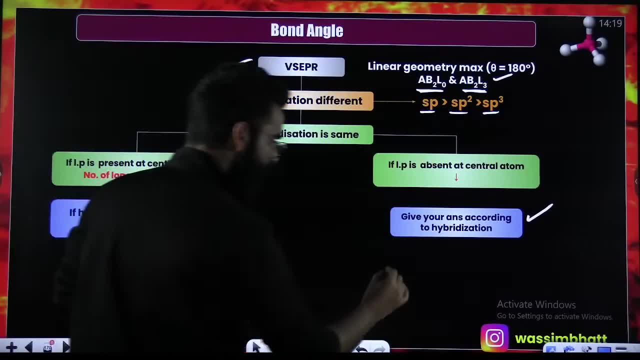 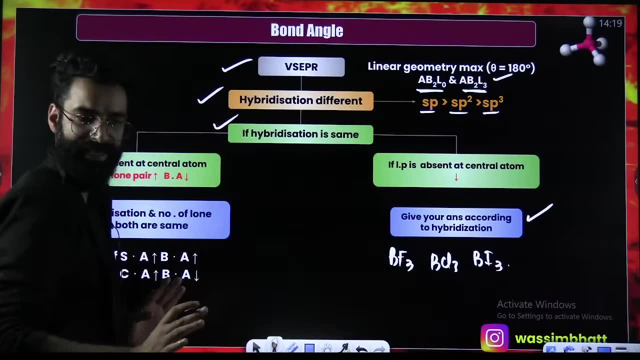 atom. you'll give the answer as per hybridization. for example, you have got bf3- understand bf3, bcl3 and bi3, right? bf3, bcl3, bi3- understand hybridization. here is sp2. hybridization. here is sp2. hybridization is an sp2. no lone pair. no lone pair. give your answer as per hybridization, since hybridization is same, so bond angle will be same. bond angle will be same if hybridization is same, if hybridization is same, if hybrid is the same- and there was a lone pair on the central atom- if hybridization. 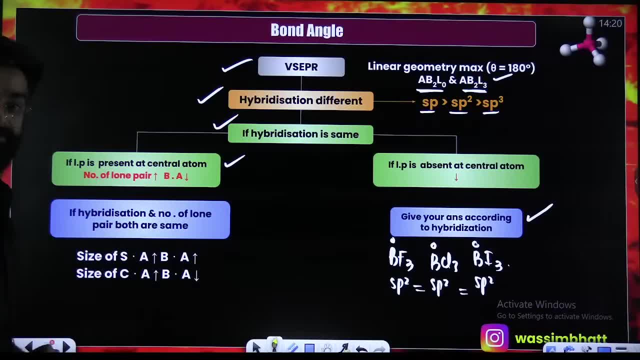 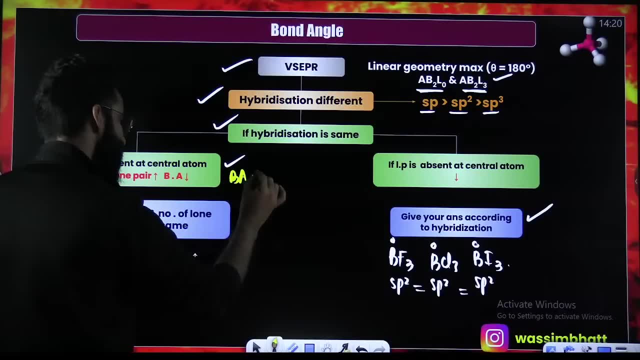 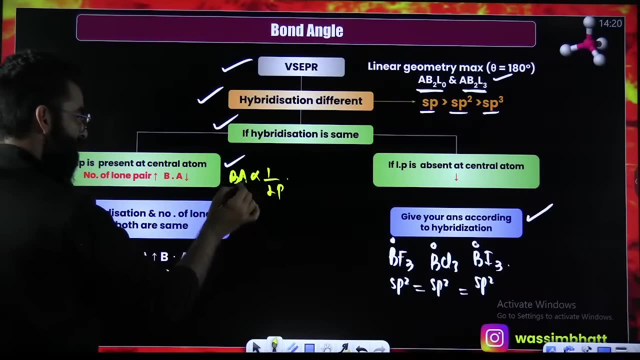 is same and there was lone pair on the central atom. if hybridization is same and there was lone pair on the central atom is present everywhere. if hybridizing is same on the central atom, then bond angle is inversely proportional to lone pair. more lone pairs, lesser slogan. if hybridization is same and there was a lone pair, present everywhere. 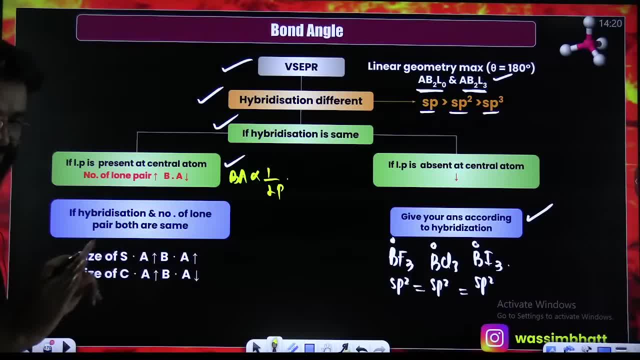 there was a lone pair represent everywhere on the central atom. remember born angle will be inversely proportional. number of loan pairs. you'll see its application in some time. now if lone pairs are same, let's say you are given three molecules, hybridization, same for the. 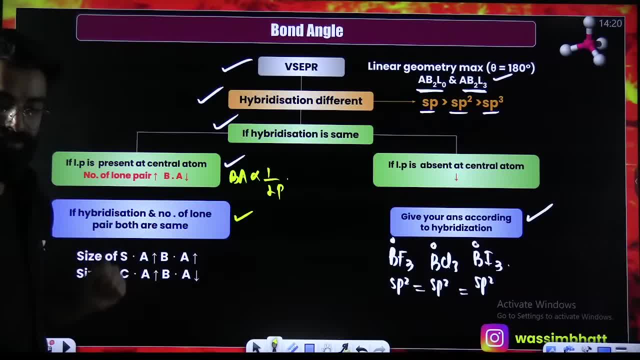 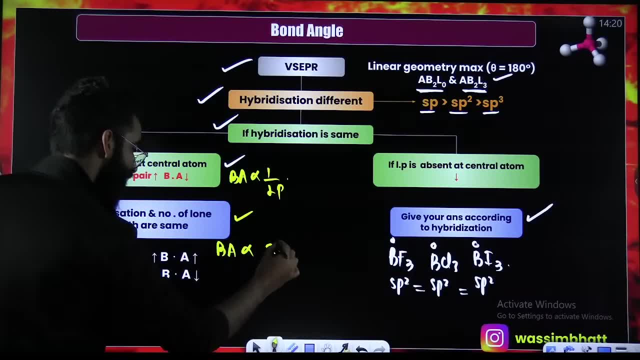 central atom. number of lone pairs on the central atom also same. then two things arise here. Remember, bond angle is directly proportional to size of the surrounding atom. Bond angle is directly proportional to size of the surrounding atom. Remember, bond angle is inversely proportional. 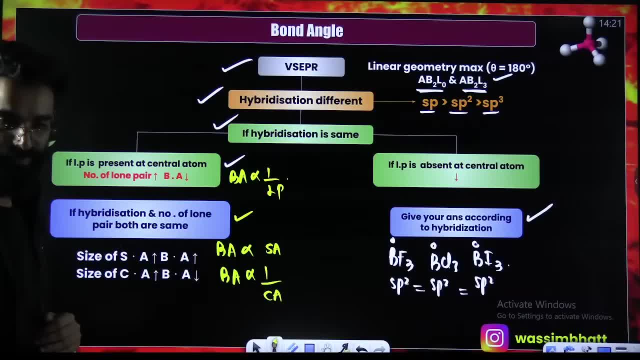 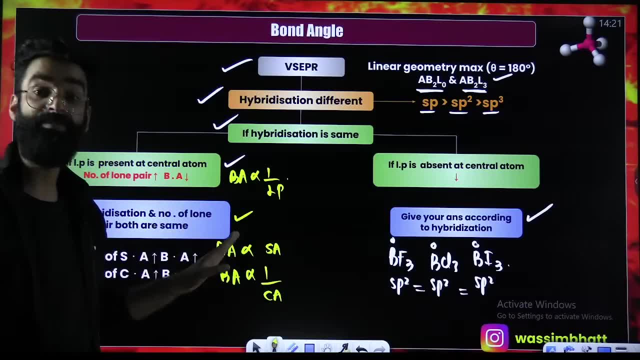 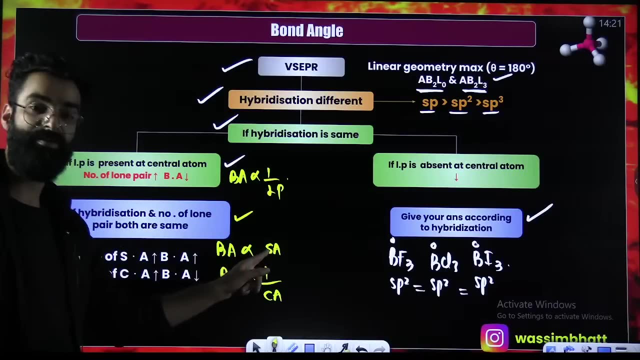 to here. size of the central atom. What mistake you do. normally you only remember these two things. You only remember these two things. But this is the actual table. Whatever equation comes from the bond angle, you are done. Have a look. Have a look. Bond angle here is directly. 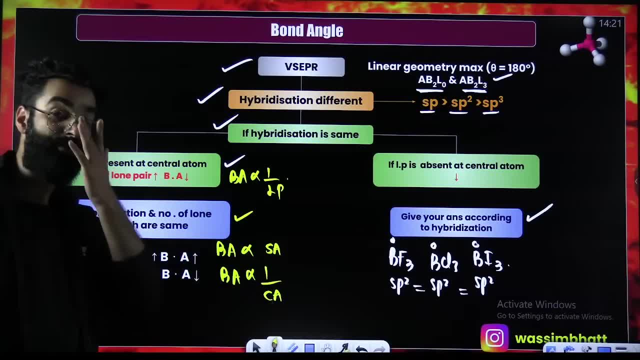 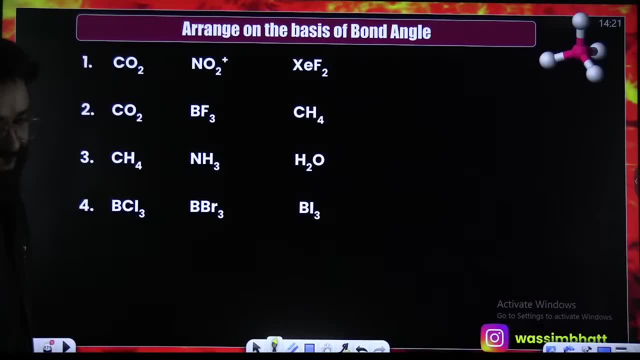 proportional to size of surrounding atom. Bond angle here is inversely proportional to size of central atom. Whatever question is asked, you are done, Sorted for life. Have a look, people. Carbon dioxide, NO2 bonds to XCF2.. First of all, we are CPR, If there is. 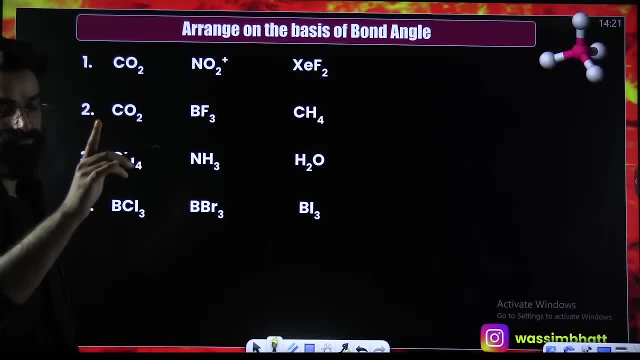 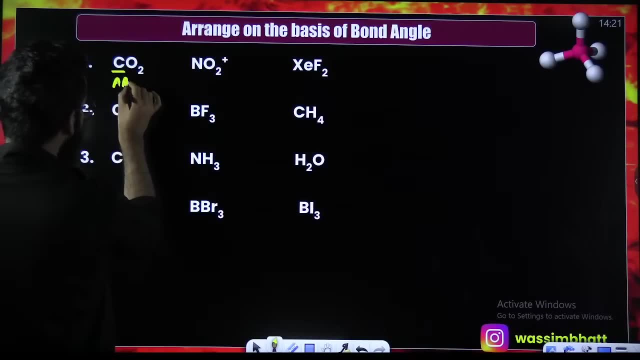 any molecule of the type of carbon dioxide. we are CPR. If there is any molecule of the type AB2L3 or AB4L2, right See, guys. See, this is of the type AB2L0.. This is of the 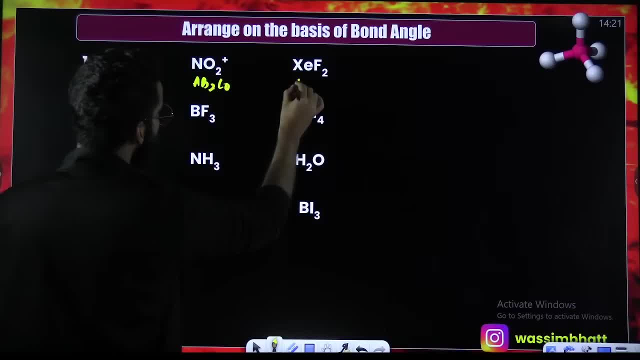 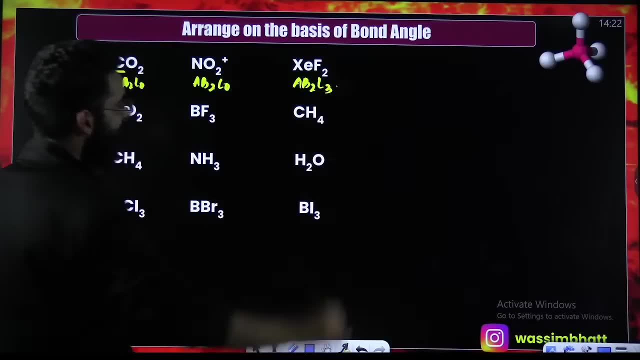 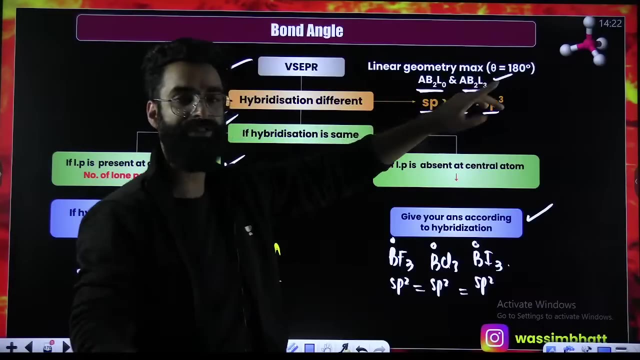 type AB2L0.. This is of the type AB2.. What AB2?? AB2L3.. AB2L3, right, Already, I have told you AB2L0, AB2L3.. They have got the maximum bond angle of 180.. So all the three, all the three, here they. 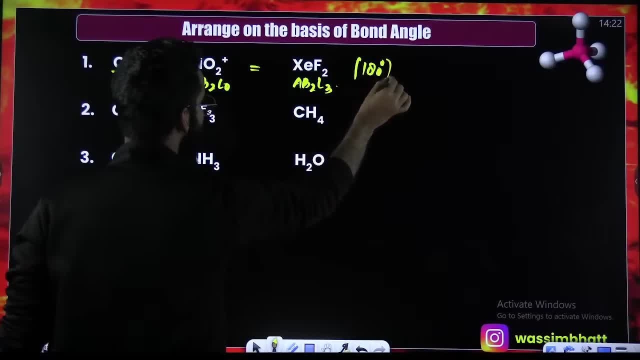 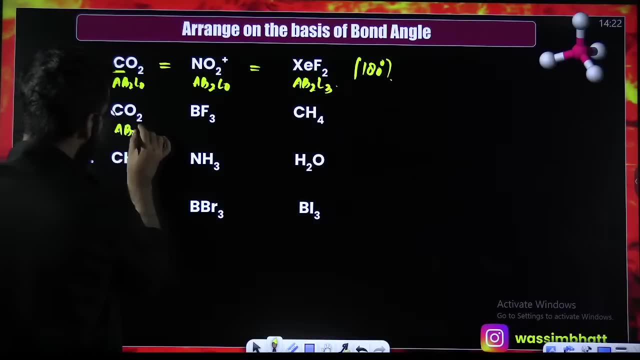 will have equal bond angles and all the bond angles here will be 180.. Done, Look at the next one. First, check the type of the molecule. This is AB2L0.. This is AB3L0.. This is AB4L0. 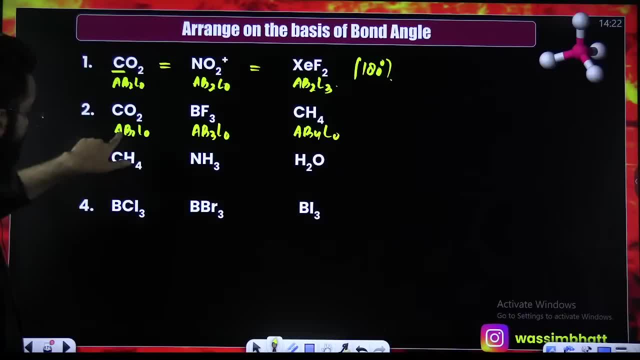 There is no one here, as yes, yes, wait, We have got AB2L0 here. This is AB2L0.. This is AB2L0. if from here it looks okay, It will look okay. This is exactly exactly as provided. 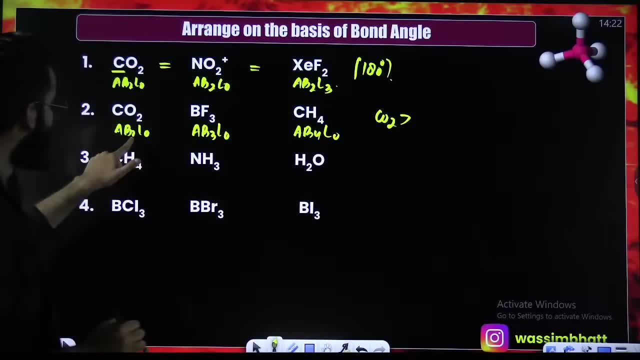 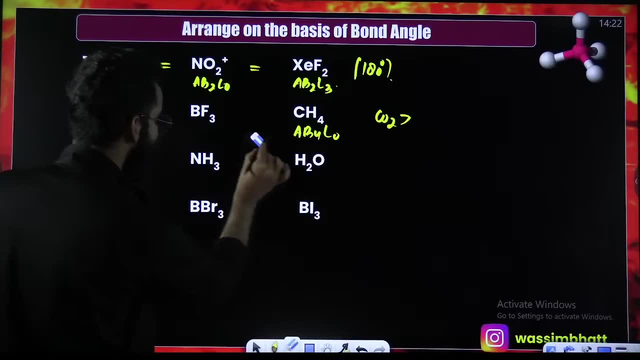 here. All right. And AB2L0, as per VS-CPR, will have maximum bond angle. So carbon dioxide will have maximum bond angle, AB2L0.. Perfect, AB2L0.. Now is there any AB2L3? No, So leave it. leave it aside, Now go to hybridization. This is SP. 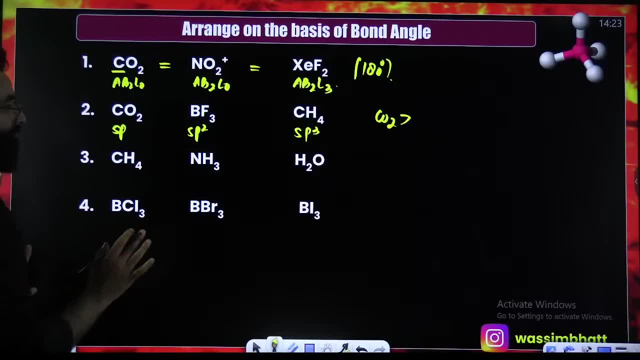 This is SP2.. This is SP3.. Hybridization is differentubradition is different. You go for hybridization. Hubradition is different. SP will have maximum. SP will have maximum. SP will have maximum vikt likes, Bk likes. So we have. have we had any friends? Yes, 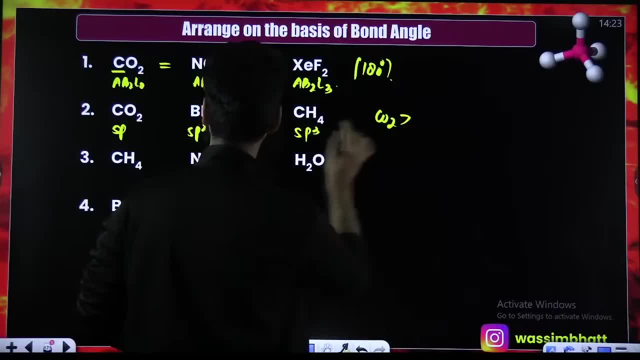 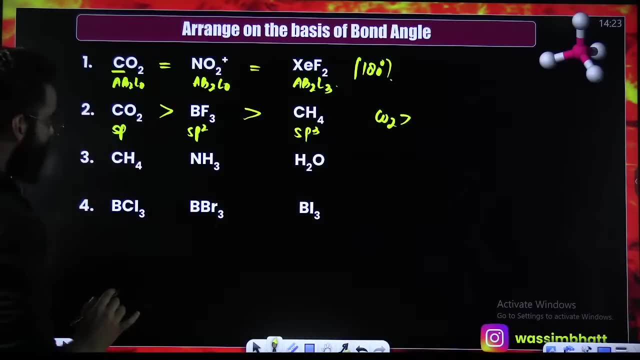 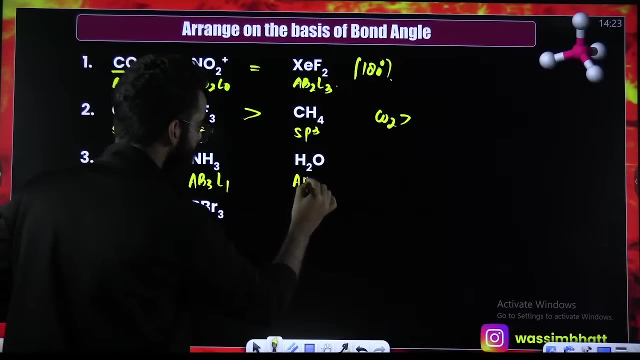 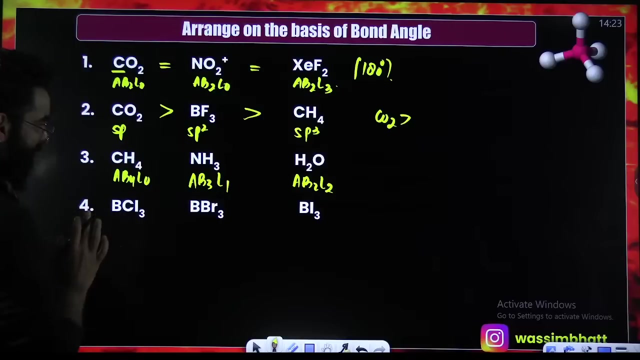 we have. So now we got, we got three, three big wild. And in uh how? What �� all three SP will be the maximum. SP will be the maximum followed by BF3 followed by CH4. Done? Go to the next one. First AB4L0, AB3L1, AB2L2. Is there any one which resembles with AB2L0 or AB2L3? 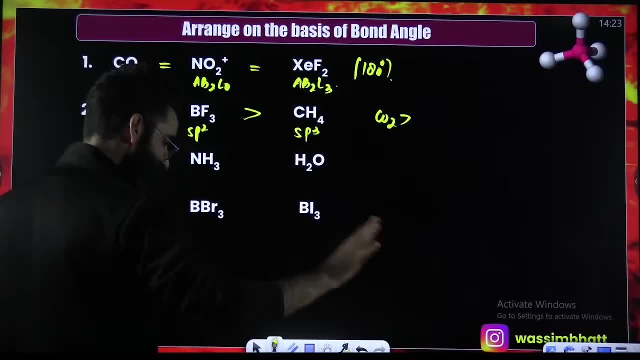 No, nothing like that. So we are unable to judge on the basis of ESC pair. leave ESC pair. Talk about hybridization, SP3.. This is also SP3. This is also SP3. Why? Because there are two lone pairs here on oxygen. There is one lone pair here. There is no lone pair here. Hybridization: 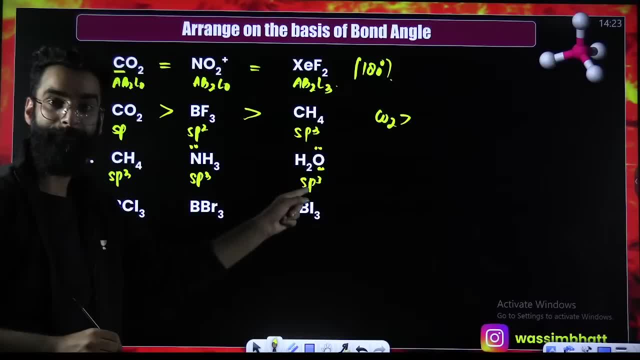 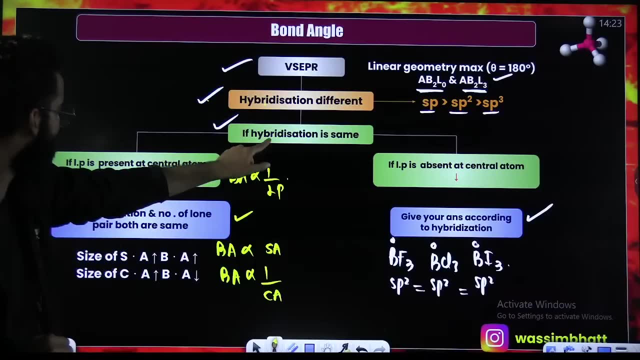 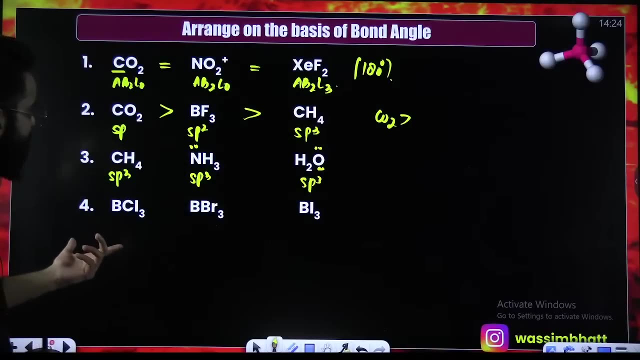 is same. Do you see? Hybridization is same. Hybridization is same and there are lone pairs on the central atom. Hybridization is same and there is lone pair on the central atom. Bond angle is inversely proportional to number of lone pairs, More the lone pairs. 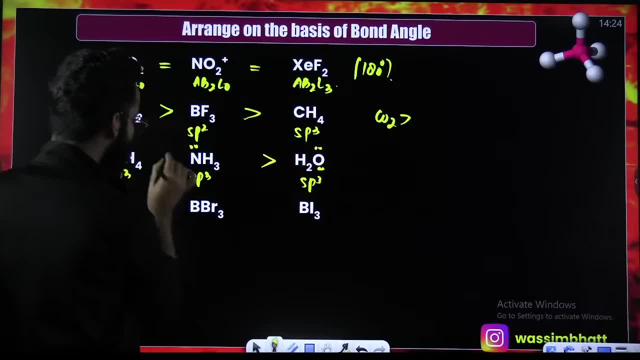 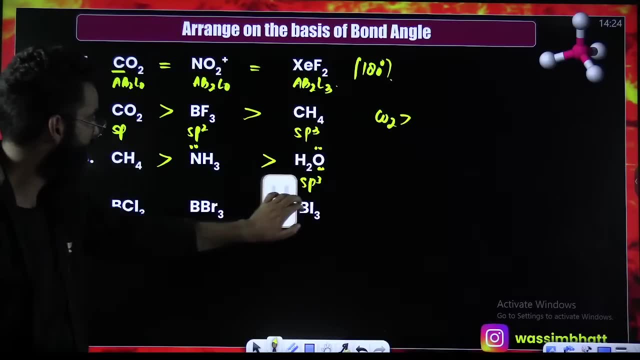 more the lone pairs, lesser the bond angle. More the lone pairs, lesser the bond angle. Done, Do you see the technique? Do you see the technique, people? BCL3, BBR3, BI3.. This is AB3L0,. 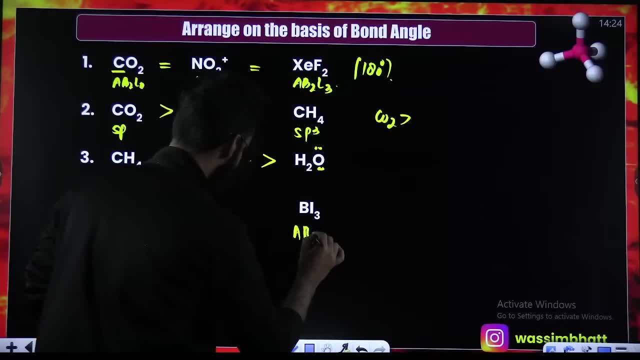 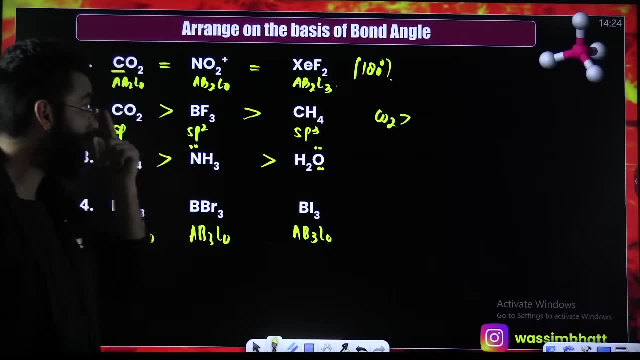 AB3L0 and AB3L0 as well. Right, So there is no one of the type, either AB2L0 or AB or AB2L3.. Leave ESC pair. Talk about hybridization. Talk about hybridization: SP2, SP2, SP2.. Hybridization. 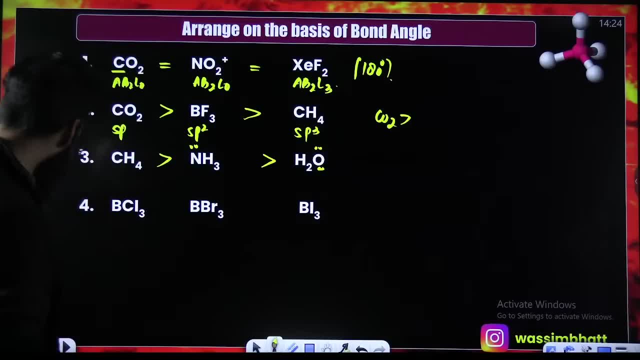 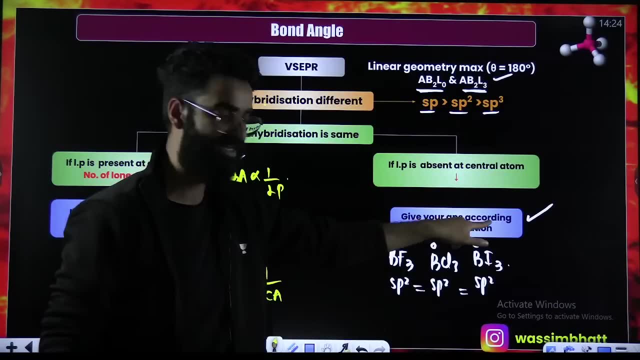 is also same, Hybridization is same. and when hybridization is same and there is no lone pair on the central atom, When hybridization is same, there is no lone pair on the central atom. Give your answer as per hybridization. Give your answer as per hybridization. This is SP2.. This is SP2.. 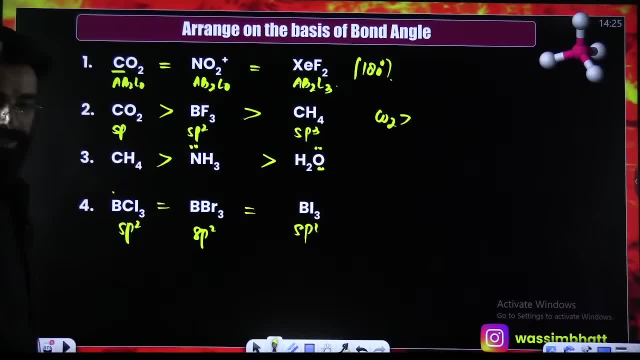 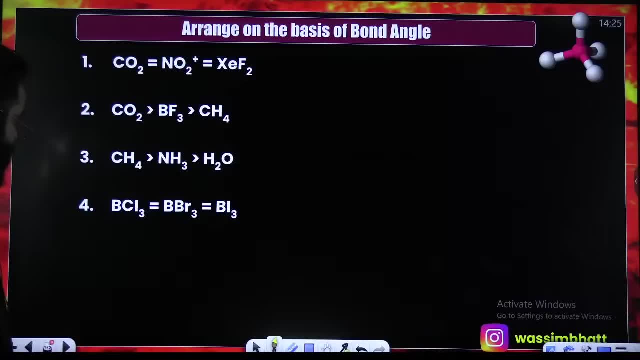 This is SP2.. Same bond angle, Right. Same bond angle. Yes, Got it. people Moving ahead, Moving ahead. Tell me the answer of the fifth one. I want to see whether you got it or not. Tell me the answer of the fifth one, people. 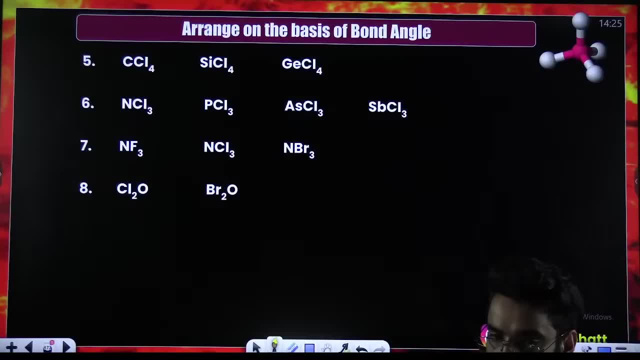 Tell me the answer of the fifth one quickly. You want the answer of the fifth one or not. Tell the answer of the fifth one or not. Tell me the answer of the fifth one: CCl4,, SICl4, GECl4.. 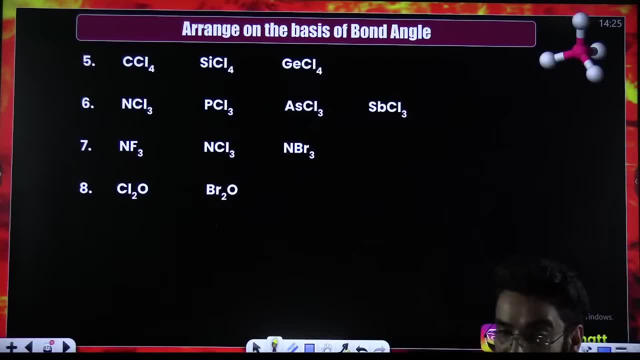 Let me give the answer of the fifth one. Thanks, Anil, Sir. You cannot always bring crypto rice up Quickly. quickly. I want everyone answer it. Type everywhere is same: AB4L0, AB4L0, AB4L0.. Hybridization is same. Spoilers are same: lingu�stäwn. 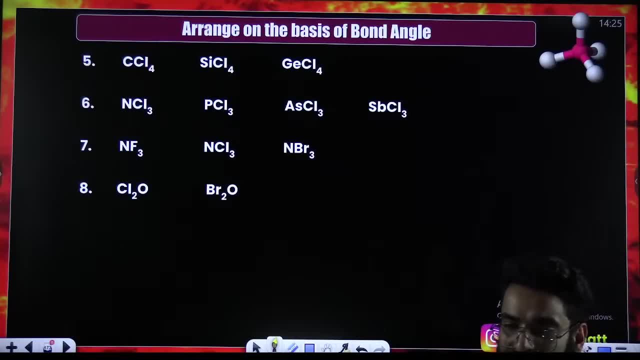 and связzi beurtric beleum. what is menstrua gem? same sp3, sp3, sp3. there is no lone pair on the central atom, so all will have same bond angles. same, all love same bond angles. ncl3, pcl3, ascl3, sbcl3. hybridization: everywhere is same sp3. 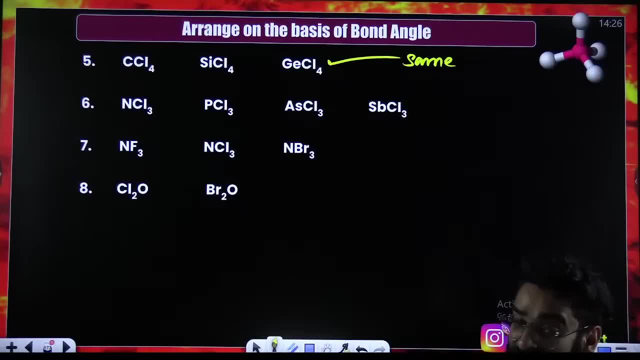 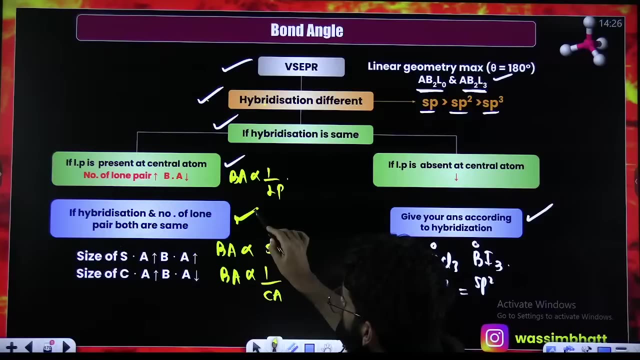 and hybridization, as well as the lone pair on the central atom is same. hybridization as well as lone pair on the central atom is same. and you know when hybridization and lone pair, both are same. you know when hybridization and lone pair, when hybridization and lone pair, both are same. 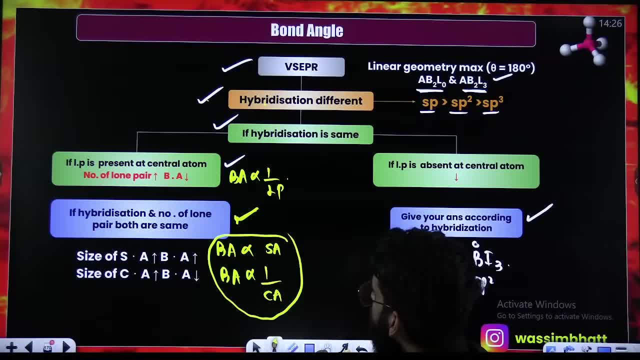 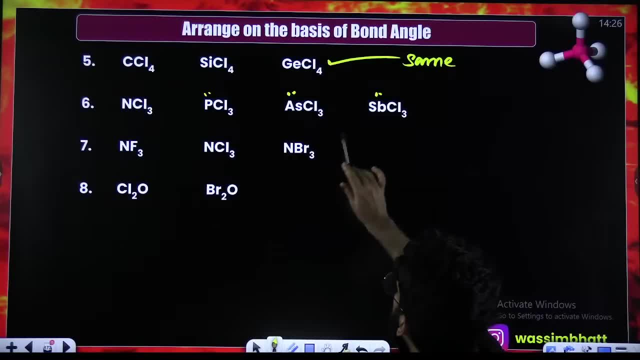 then talk about these two factors. talk about these two factors. bond angle is inversely proportional to size of central atom. bond angle is inversely proportional to size of central atom. bond angle is inversely proportional to size of central atom. right size of central atom is maximum here. 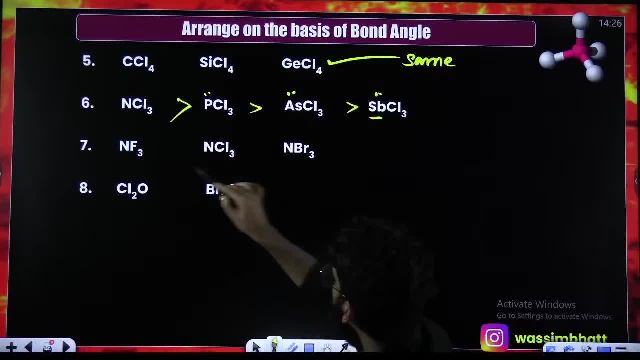 so bond angle minimum? give me the answer of this one. seventh one, seventh one, people, seventh one, quickly. seventh one here in the seventh one. bond angle is directly proportional to size of surrounding atom. bond angle is directly proportional to size of surrounding atom. right, perfect, because hybridization as well as lone pairs are lone pairs are same, and you know. 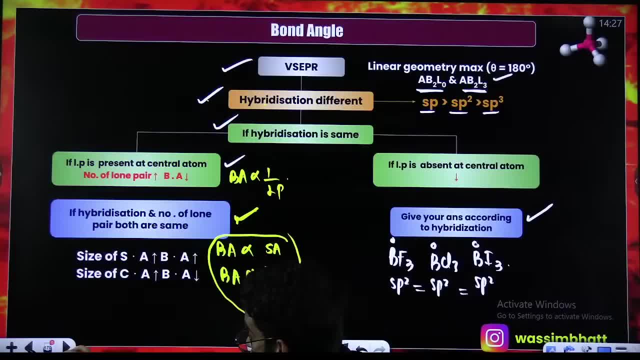 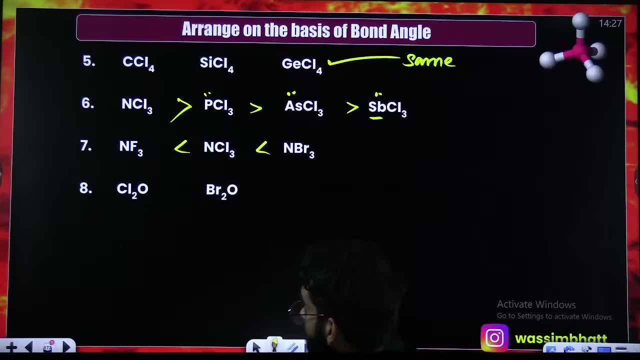 bond angle is directly proportional to size of bond angle is directly proportional to size of bond angle is directly proportional to size of surrounding atom. okay, bond angle is directly proportional size of surrounding atom. swirling atom is directly proportional to size of surrounding atom. this fast three to one. tell me the last one. 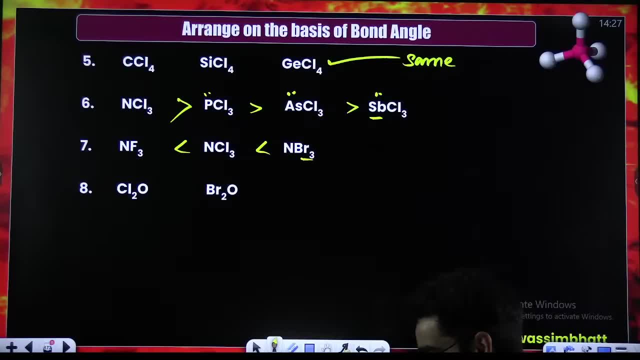 cel 2o br2, cl 2o br2, cl 2o br2. quick, see guys. oxygen hair has got two lone pairs. situation here: has got two lone pairs and also has two lone pairs. hyporgression involved is sp3. upa region of oxygen: here is sp3. 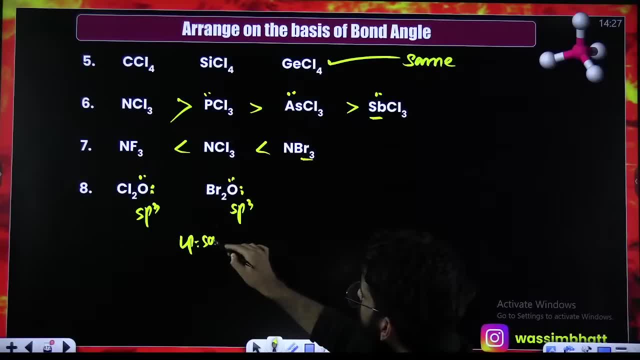 hyporgression. involved is sp3: same lone pair, same Hybrid addition. same lone pair, same. Right Now, surrounding atom is different. Surrounding atom is different. More the size of surrounding atom, more the size of surrounding atom, more will be the bond. 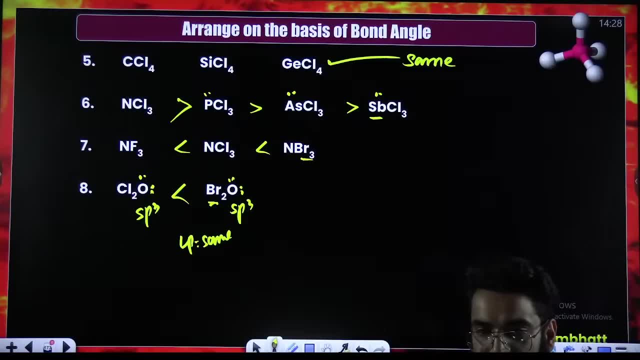 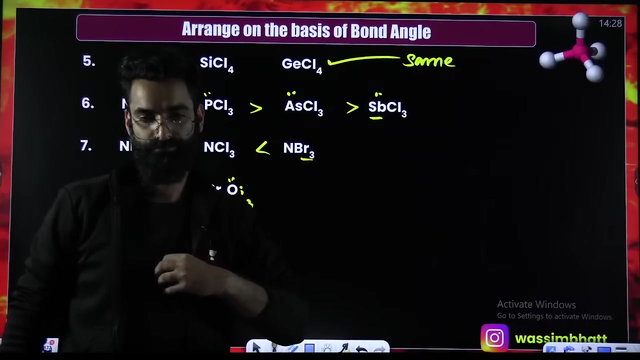 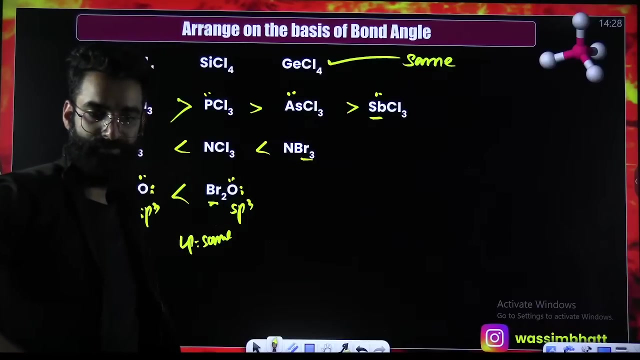 angle. Am I clear to everyone: From now onwards, if a question is asked from bond angle people, you should kill it. You must kill it. Yes, Are we done? Our physical chemistry class 11th marathon will be on Friday. 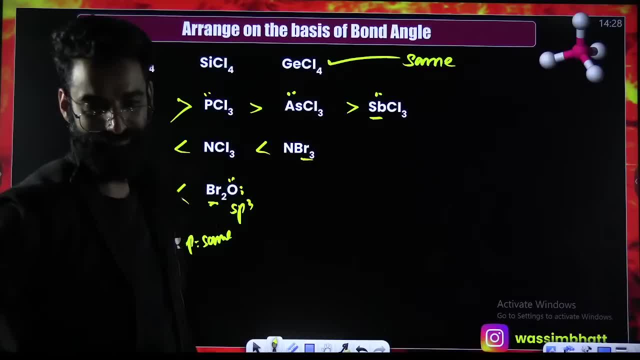 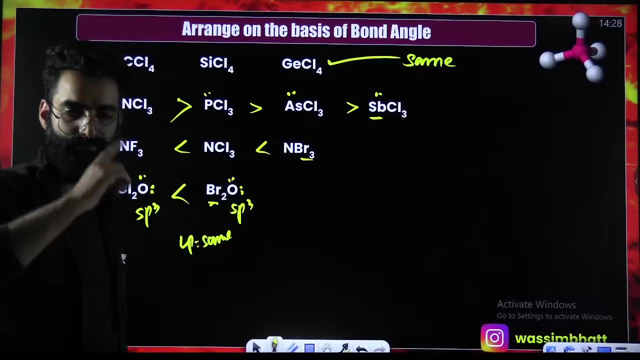 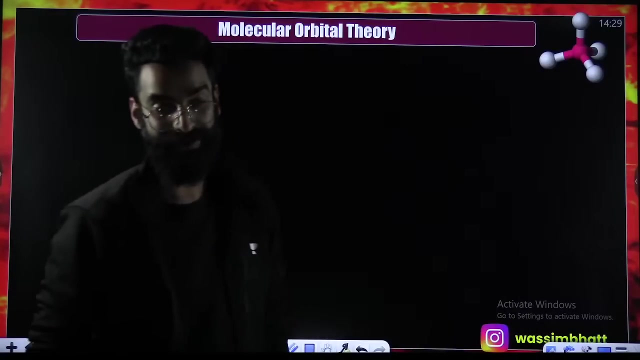 10th, 11th, something like that. Perfect, Okay, Now comes the last topic of the chemical bonding, that is, your molecular orbital theory. Okay, Molecular orbital theory. See, as I told you, I don't want to teach. 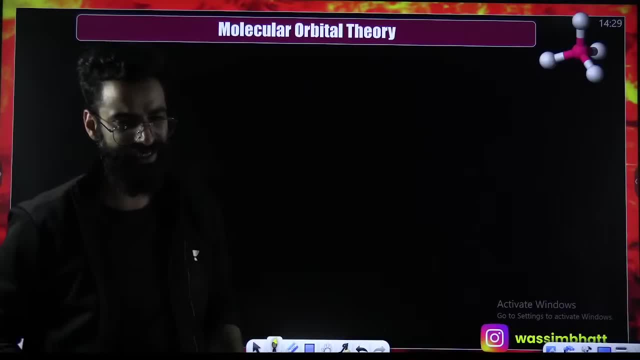 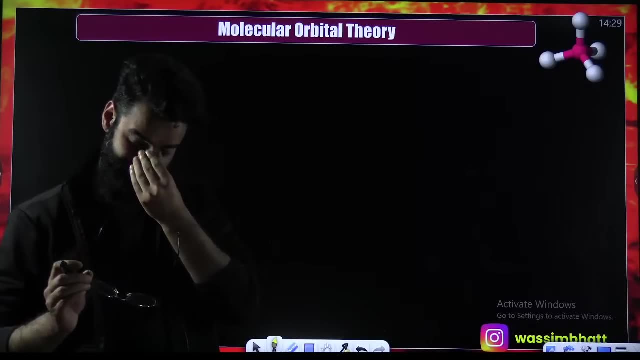 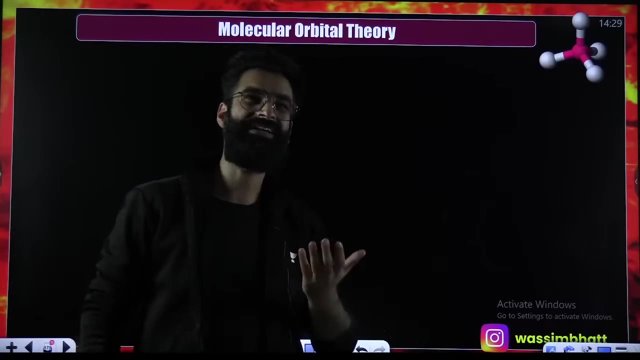 I don't want to teach you in very depth. I just want to give you that amount of theory which is required to solve the questions Right. Perfect, If you would have watched my one shot of chemical bonding, I have done this chapter in 9-10 hours, I believe. 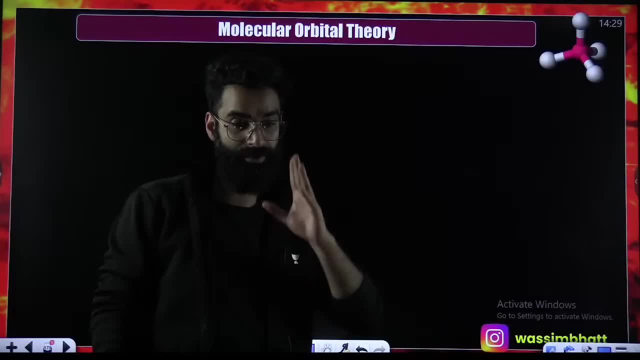 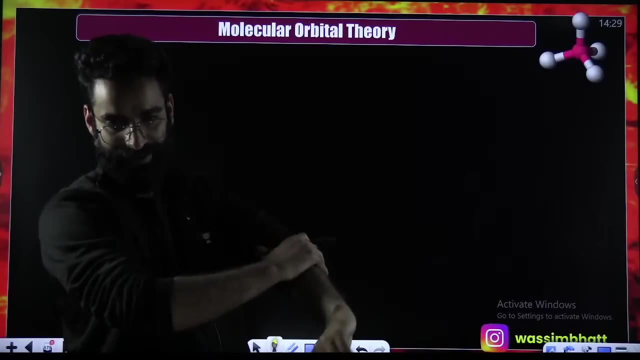 Right, But right now, as I told you already, only that much I am teaching you, which is required for the questions to be solved. That's all. That's all. So let's complete this MOT over here. Let's complete this MOT over here. 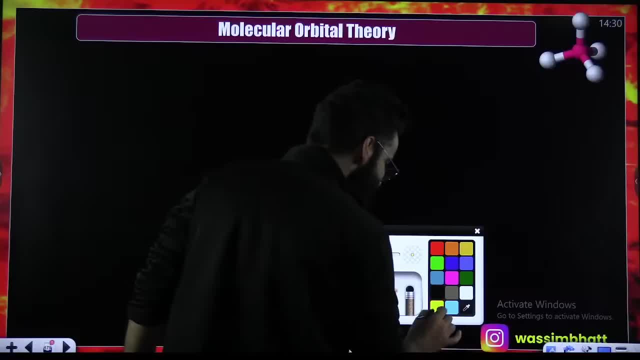 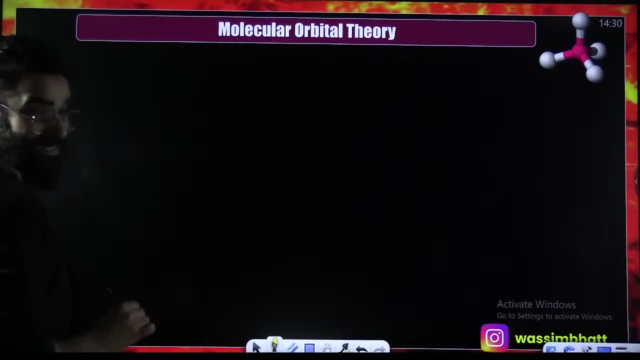 Okay, See, guys, as per molecular orbital theory is concerned, what happens, basically, What happens? Molecular orbital theory says that atomic orbitals, atomic orbitals. first of all, this molecular orbital theory, let me tell you it is the extension of VBT. 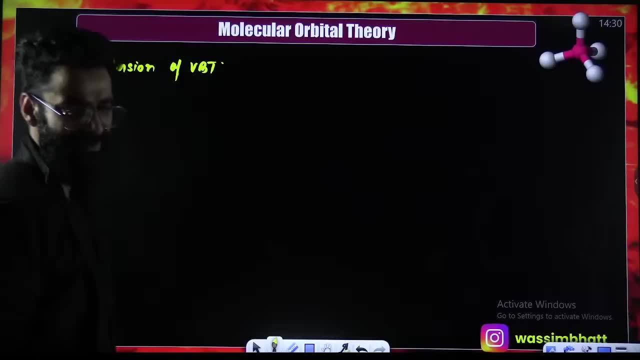 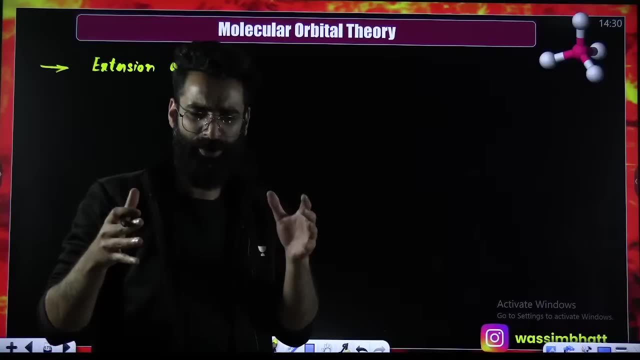 It is the extension of VBT, What VBT used to say. VBT used to say that atomic orbitals overlap Atomic orbitals of the bonding atoms. they overlap Right Atomic orbitals of the bonding atoms- they overlap That VBT used to say. 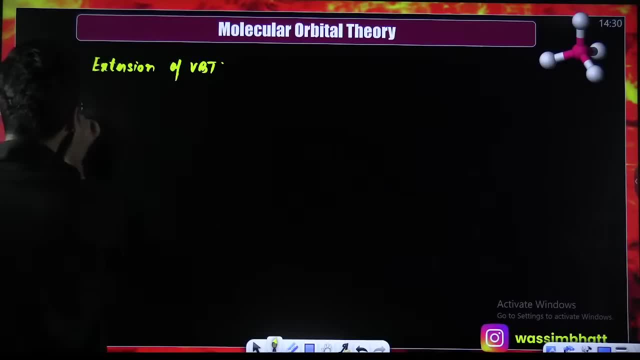 This theory says the similar stuff. This theory says that atomic orbitals of the bonding atoms, atomic orbitals of the bonding atoms, they combine, they combine and they lead to the formation of what They lead to the formation of molecular orbitals. 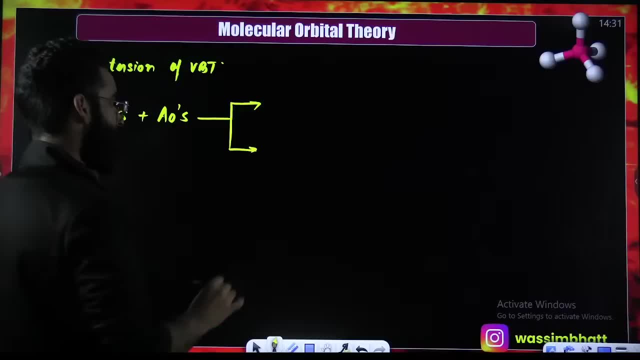 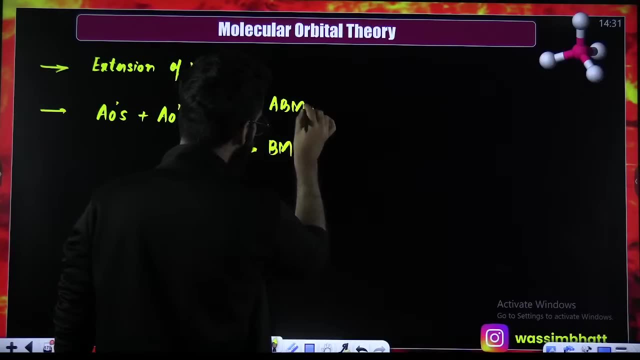 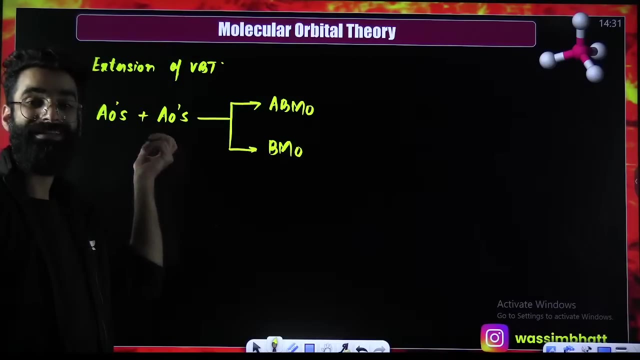 Atomic orbitals combine, lead to the formation of molecular orbitals. One will be called as bonding molecular orbital, Another one will be called as antibonding molecular orbital. Atomic orbitals of the combining atoms. they combine, they lead to the formation of molecular orbitals. 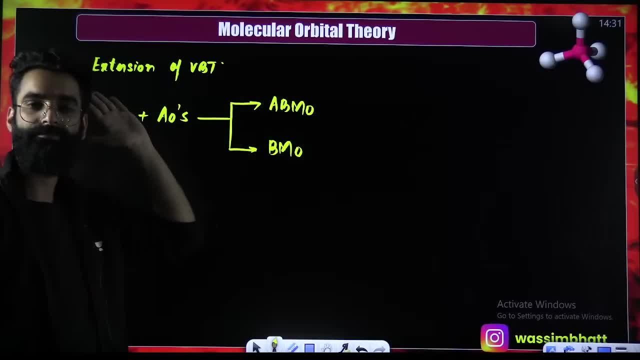 One will be called as bonding, one will be called as antibonding. Number of atomic orbitals combined is equal to number of molecular orbitals formed. Here two atomic orbitals are combined, So two molecular orbitals are being formed. One is bonding, one is antibonding. 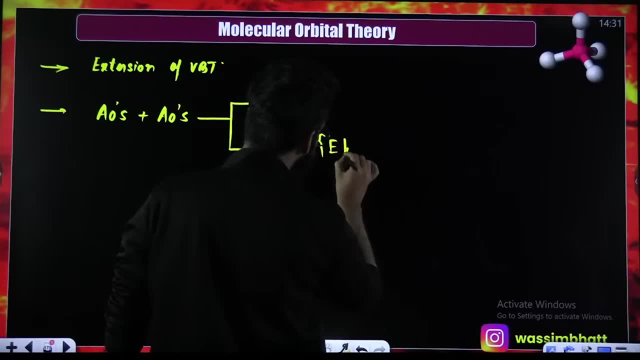 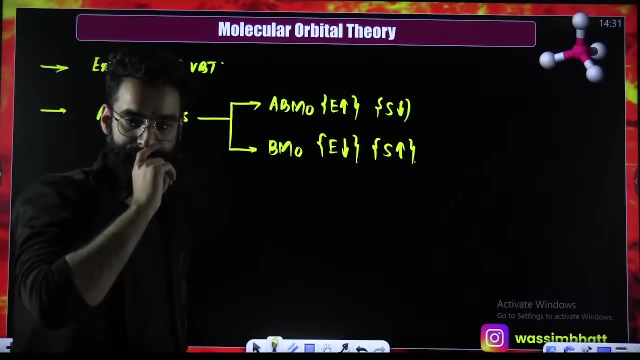 Let me tell you: energy of bonding is less, energy of antibonding is more. That means stability of antibonding is less. stability of bonding is more. Stability of bonding is more. Okay, This bonding, for example, for example, understand like this: 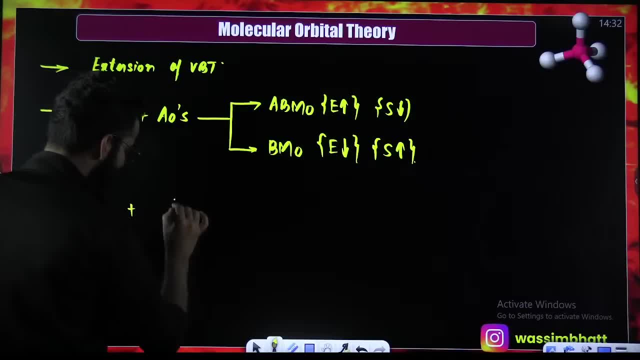 Let's say I have got 1s orbital of one atom And similarly 1s orbital of another atom. 1s, 1s. perfect Now these 1s 1s, they are combining. They are combining. 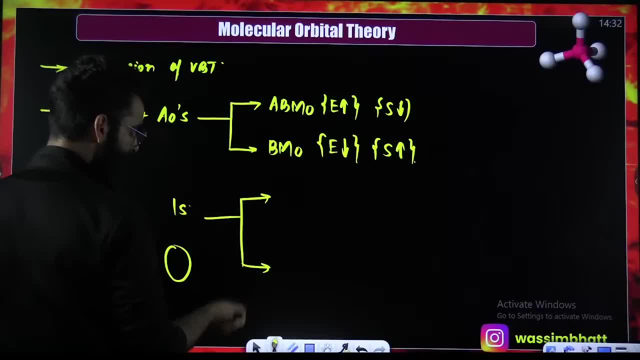 And they will lead to the formation of two molecular orbitals. One will be bonding, one will be bonding. One will be bonding molecular orbital. Another one will be antibonding molecular orbital. Bonding molecular orbital. I will be representing here by sigma 1s. 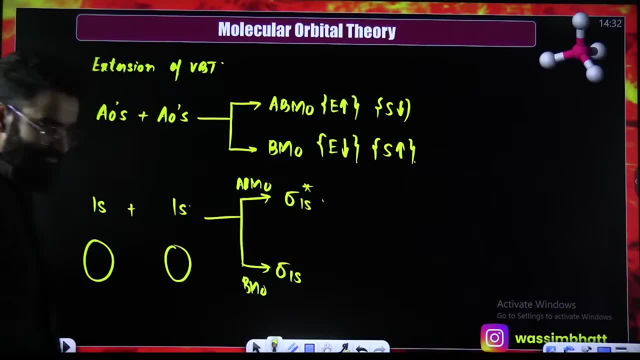 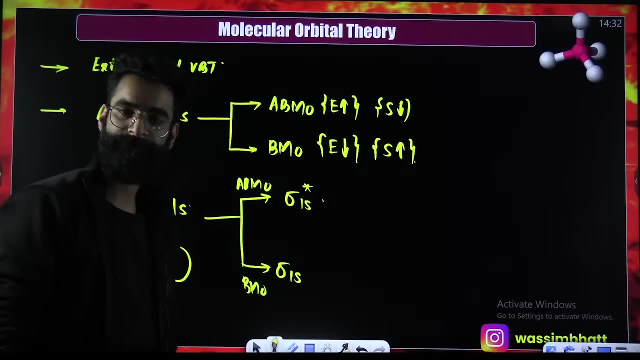 Antibonding I will be representing was by sigma 1s star. Sigma 1s star, Sigma 1s star, Okay, sigma 1s star, Remember directly: bonding molecular orbital is formed through constructive interference, Through in-phase interference. 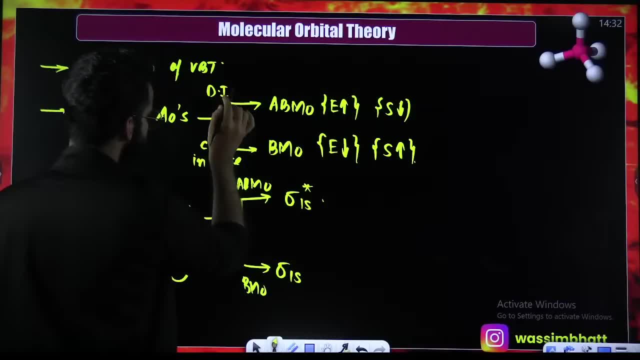 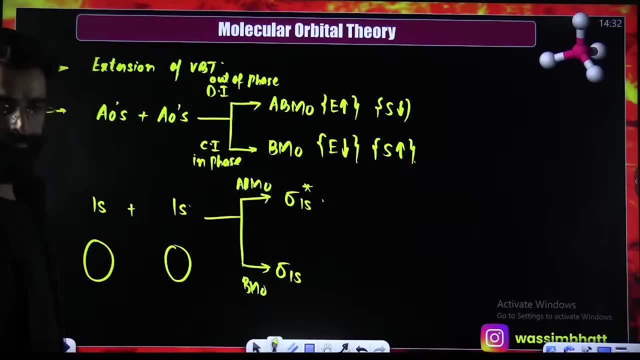 This is formed through destructive interference, Right Through out-of-phase interference. Right, Constructive interference leads to the formation of bonding. Destructive interference leads to formation of antibonding. Okay, Now, my dear students understand And remember. 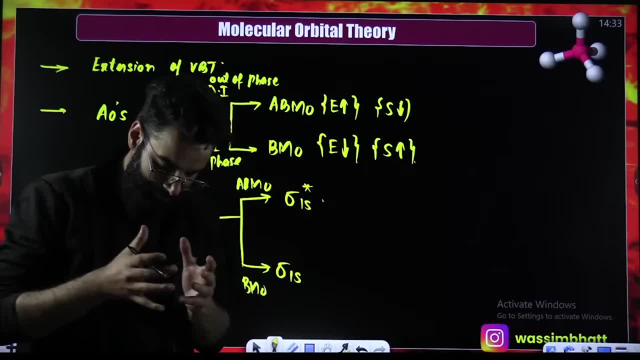 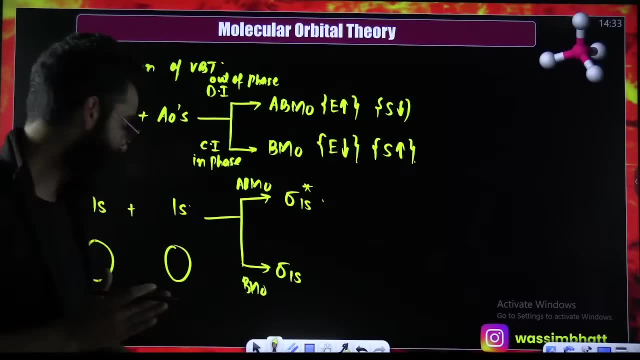 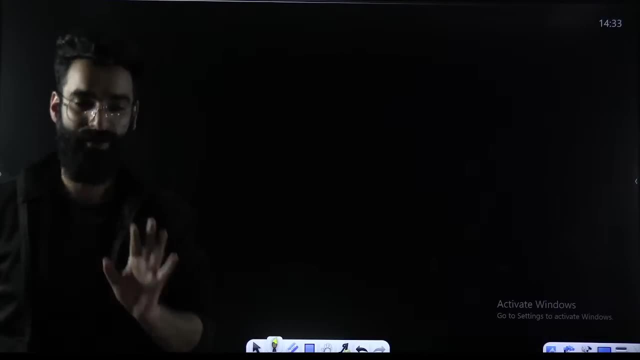 When two combining atoms, when their atomic orbitals combine, they lead to the formation of molecular orbitals. Once these molecular orbitals are formed, Once these molecular orbitals are formed, Then in these molecular orbitals we have to fill the electrons. 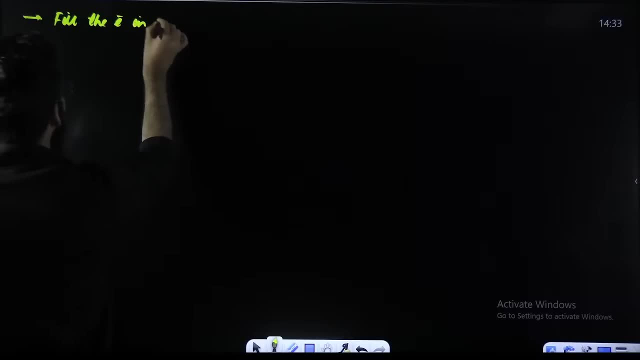 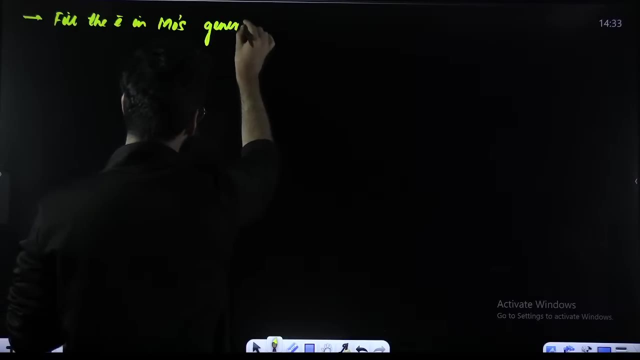 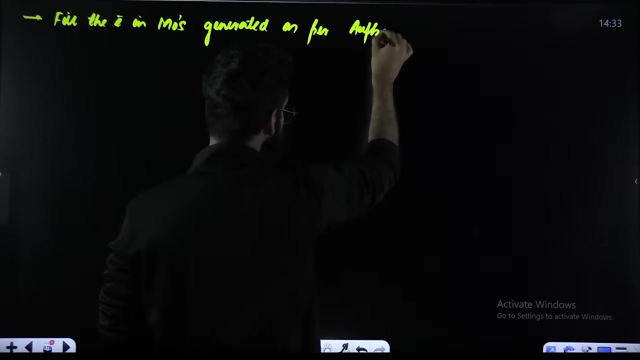 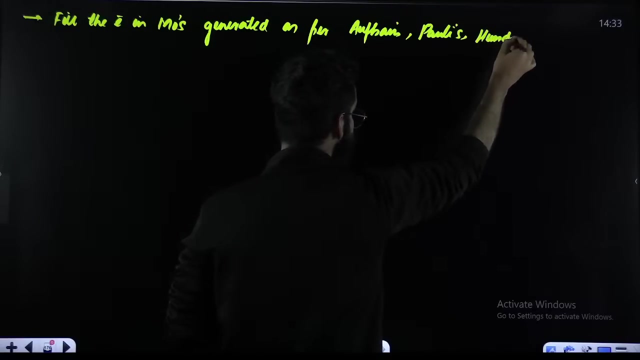 We will fill the electrons in the molecular orbitals. we'll fill the electrons In the molecular orbitals which got generated, Which got generated As per, as per Abba's principle, a Pauli's exclusion principle and as per Hund's rule. 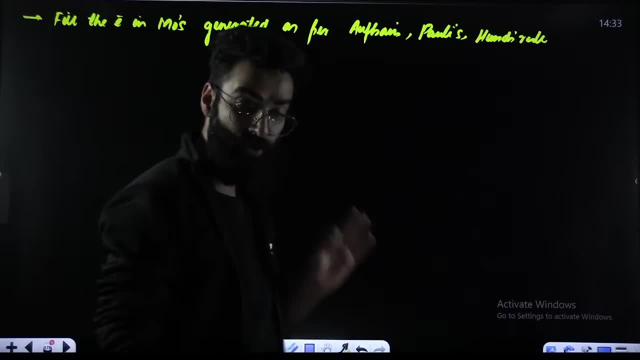 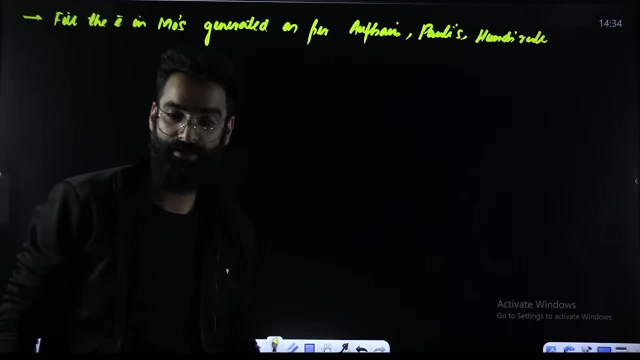 Once these molecular orbitals are generated, then we are going to start filling the electrons in those molecular orbitals. as per what? As per your, as per Abba's principle, Pauli's exclusion principle, as well as the Hund's rule, as well as the Hund's rule as well as the Hund's rule. 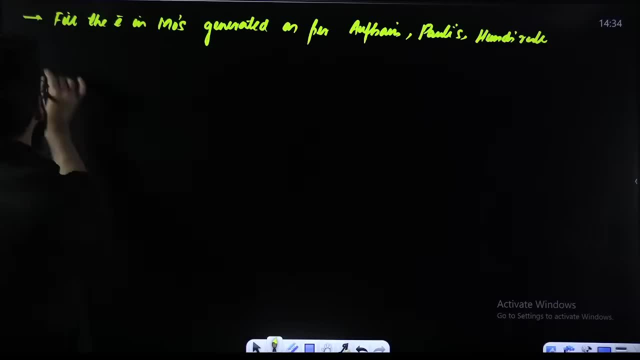 And once we are done filling electrons in these molecular orbitals, then, my dear students, the most important thing which is calculated here, that is bond order, which is calculated: half of number of electrons in bonding molecular orbital minus the number of electrons in anti-bonding. 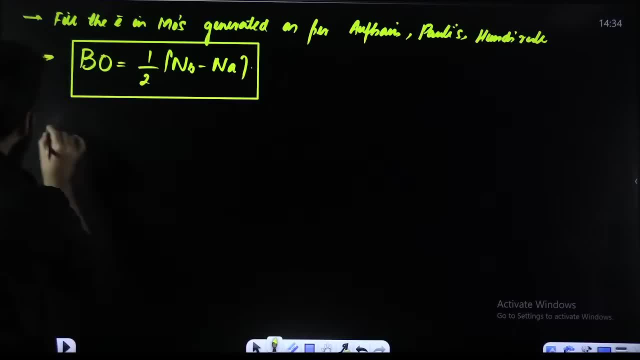 molecular orbital. This is the most important stuff here. And remember: if the bond order comes out to be 1, that means there is a single bond between the atoms. If the bond order comes out to be 2, that means there is a double bond. 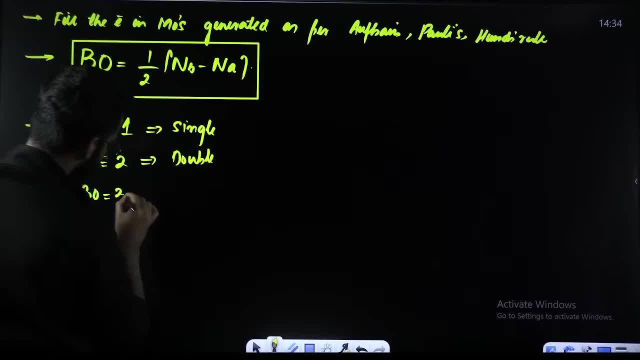 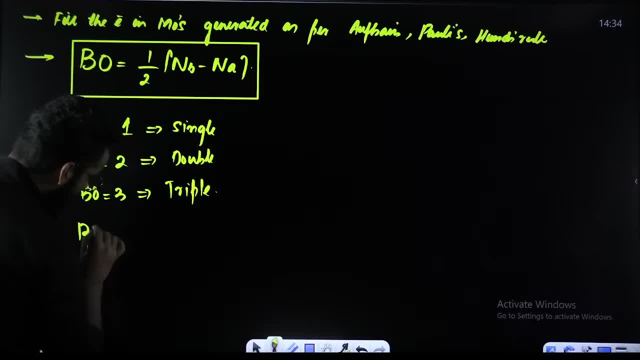 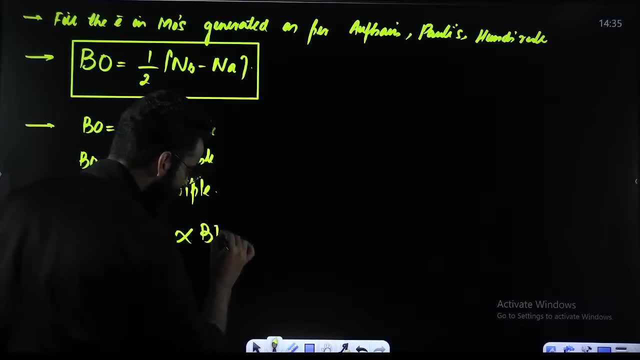 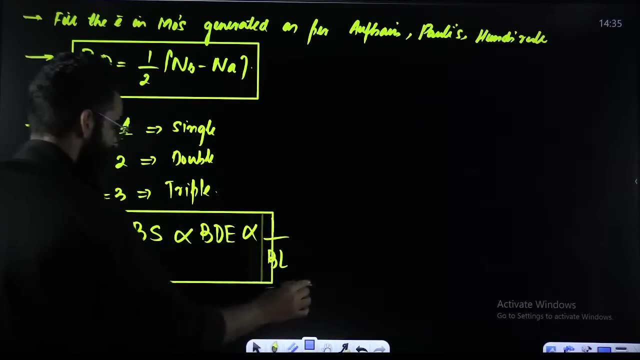 Let me tell you one more thing. Bond order is directly proportional to bond. strength is directly proportional to bond. dissociation energy is inversely proportional to bond length, inversely proportional to bond length. question can either be asked on bond order or it can be. 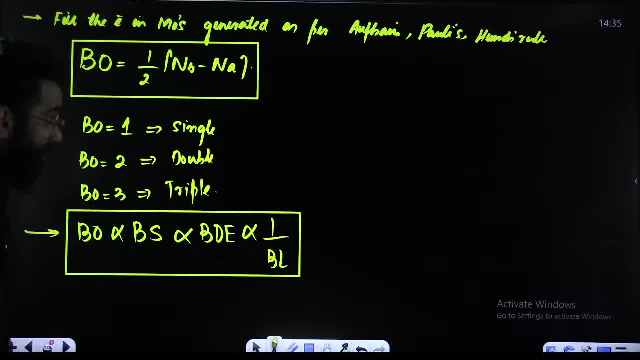 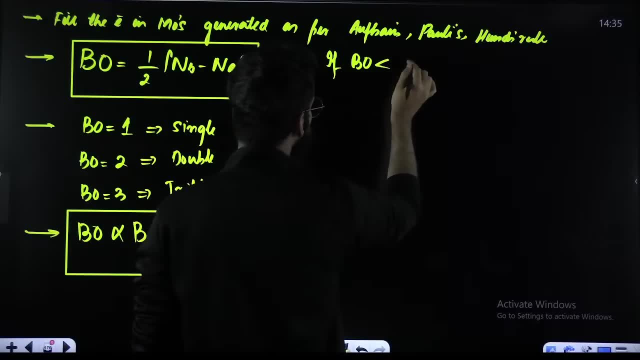 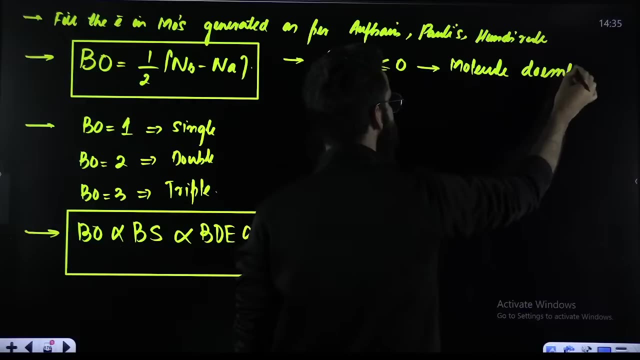 asked on bond strength or bond associate energy or bond length. one more thing which i would want to tell you: if the bond odd, if the bond order as per this formula comes out to be less or equal to zero, that means the molecule does not exist. molecule does not exist, or you say molecule is. 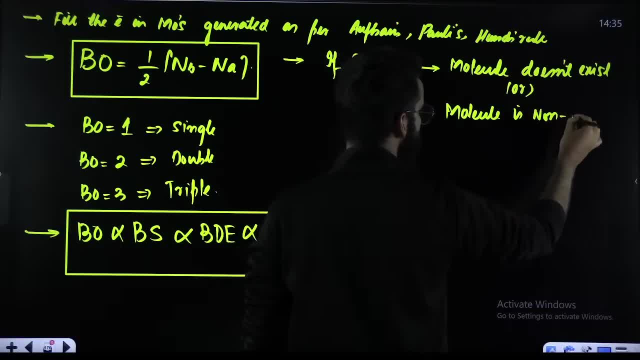 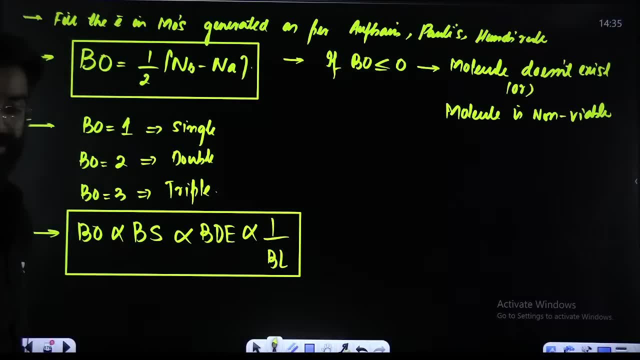 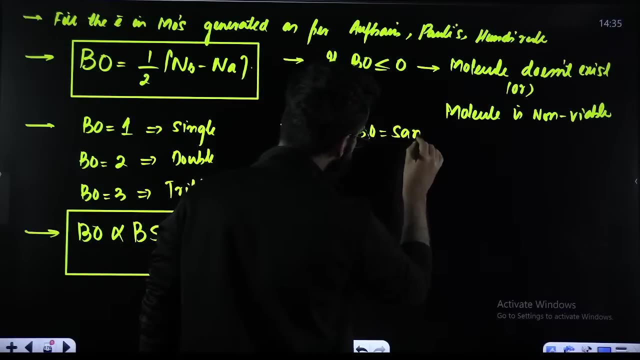 a non-viable molecule is non-viable when, when the bond order comes out with less than zero right. remember if the bond order of two species comes out to be same. if the bond order of two species comes out to be same, remember at that point of time. 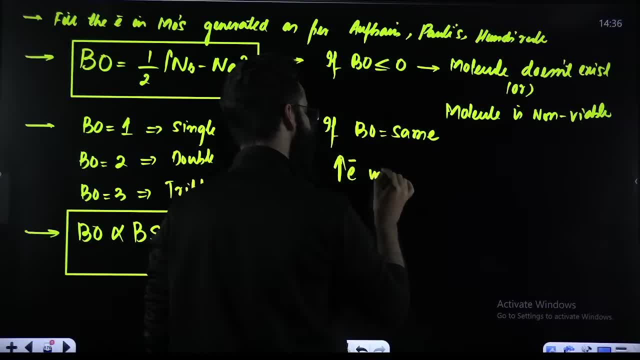 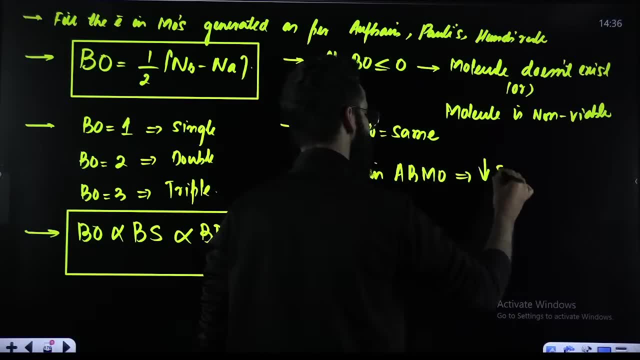 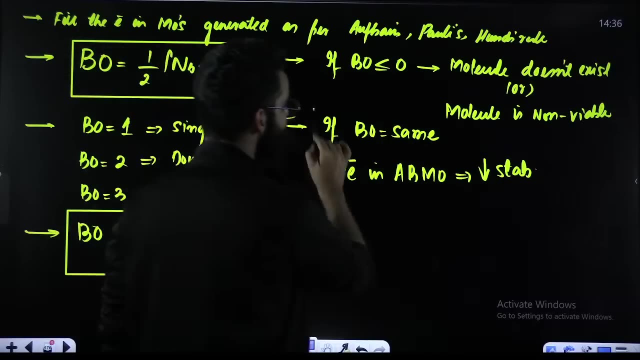 at that point of time, more the electrons in anti-bonding molecular orbital, more the electrons in anti-bonding molecular orbital lesser is going to be the stability, more the electrons in anti-bonding molecular orbital lesser is going to be stability. lesser is going to be stability when? when is this case if the bond order is same? 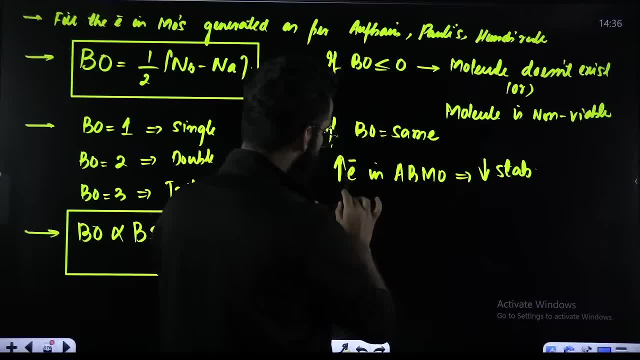 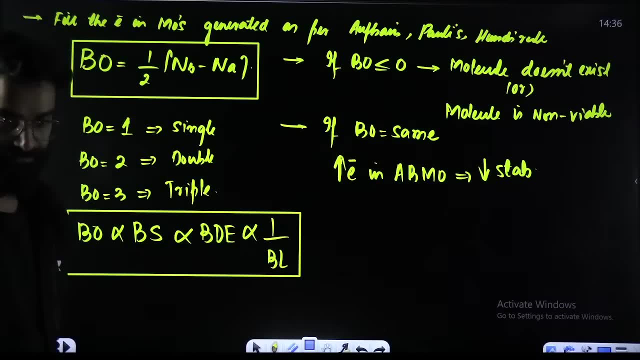 if the bond of two species is the same, and, and, and, and and more electrons are present in anti-bonding that species. wherein more electrons are present in anti-bonding bond, a stability will be less. stability will be less. okay, what else can be asked from that? 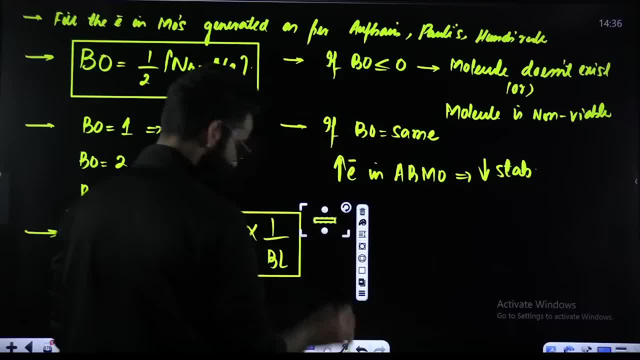 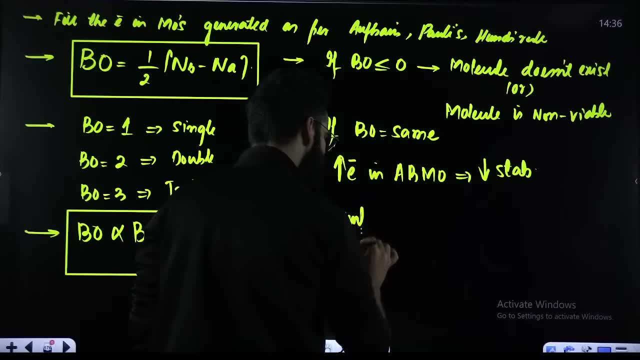 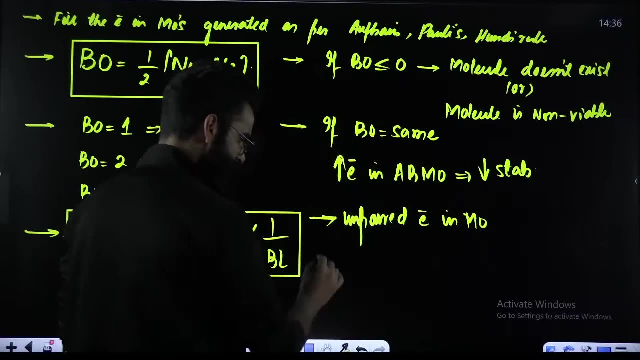 this. yeah, next point which can be asked. next point which can be asked: if there were unpaired electrons, if there were unpaired electrons in the molecular orbitals in the mole, there can be two cases: either there will be paired electrons in all molecular orbitals, right, or there can be unpaired electron in some of the molecular orbitals. if you see unpaired electron, 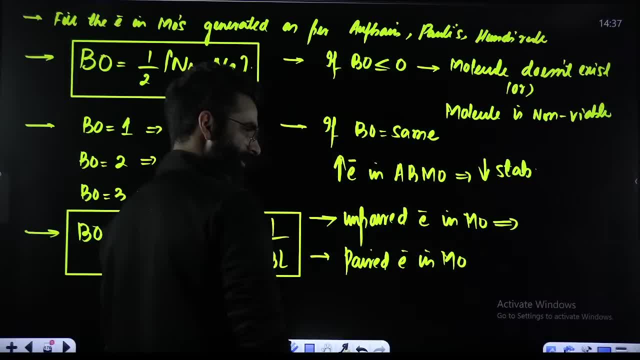 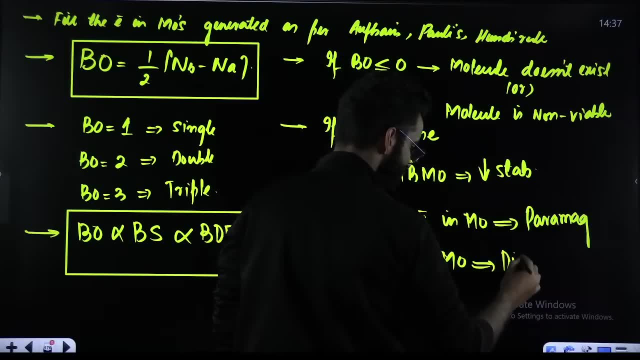 in. if you see unpaired electron in the molecular orbital, any molecular orbital- do remember that species is going to be paramagnetic. this particular species is going to be diamagnetic. this species is going to be diamagnetic and at the same time. how do you calculate this? 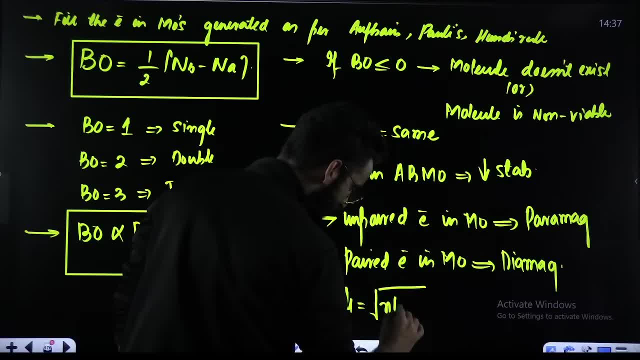 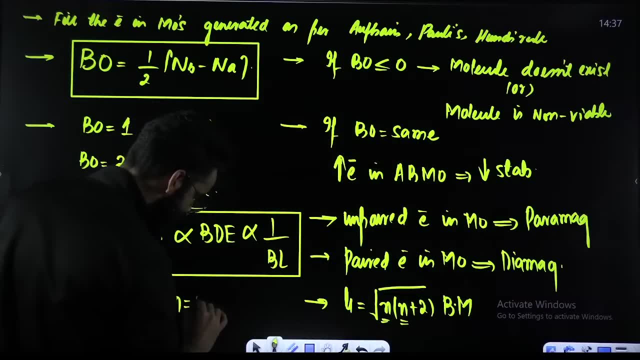 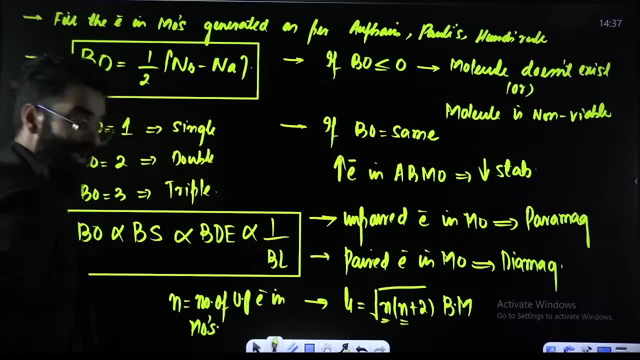 magnetic moment. magnetic moment is calculated by the formula under root of n into n plus 2 bohor magnetrons, where n represents where n represents number of unpaired electrons in the molecular orbitals. number of unpaired electrons in the molecular orbital. okay, okay. now guys directly jump into the questions and kill all the questions. 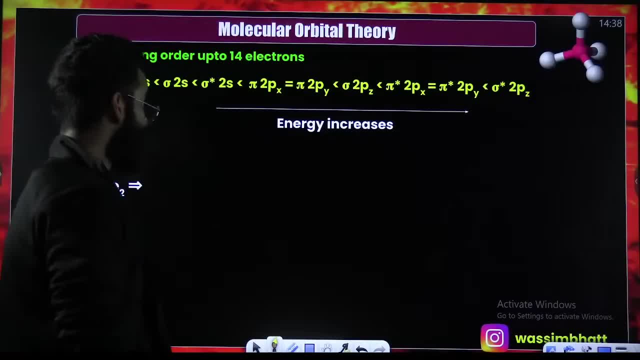 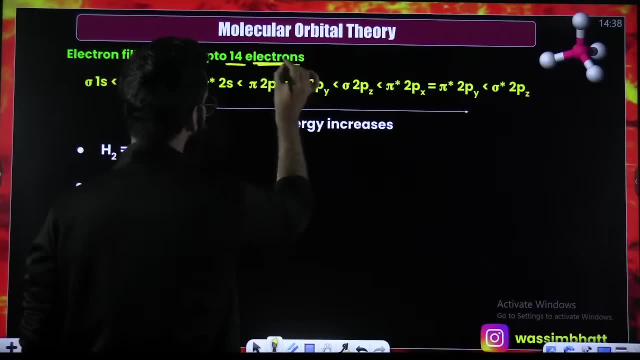 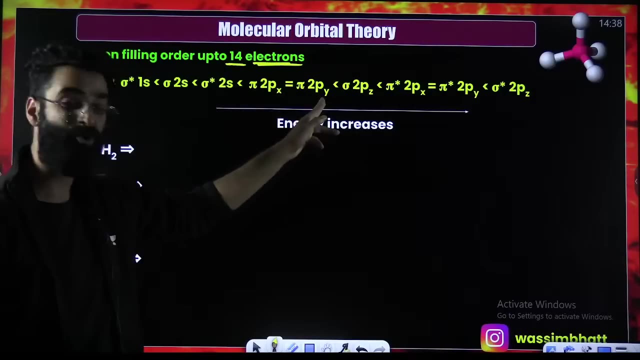 right now. so first of all, we'll see. we'll see the electron filling order in those species which have got electrons up to 14, which have got electrons up to 14.. see, these are all the molecular orbitals, sigma 1 and sigma star. 1 is sigma 2s, sigma star 2s, pi 2p x, pi 2p 1, and i have 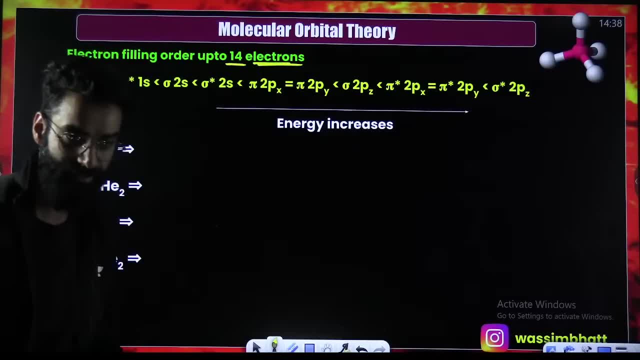 written all these molecular orbitals as per the increasing order of their energies. why did i do that? because abbas principle says that electrons are to be filled in the increasing order of the. So this order you have to remember first of all, and this order is valid only up to. 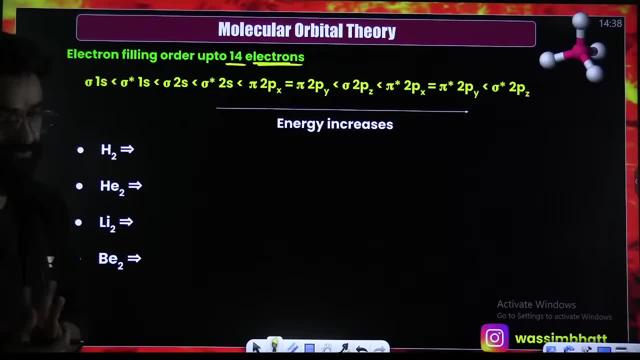 14 electrons. this order is valid only up to 14 electrons. now try to understand how exactly I am going to use this order. understand In case of H2, in 1 hydrogen there is 1 electron. in 2 hydrogen there are 2 electrons- 2 electrons. 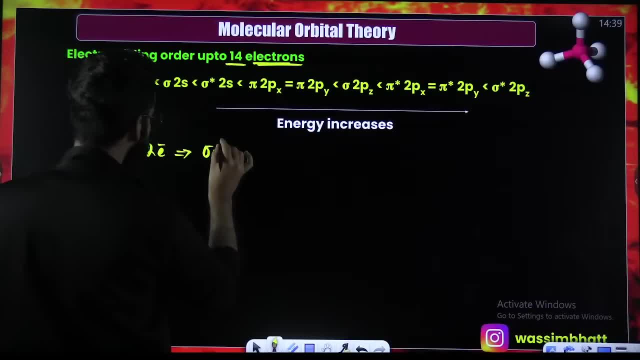 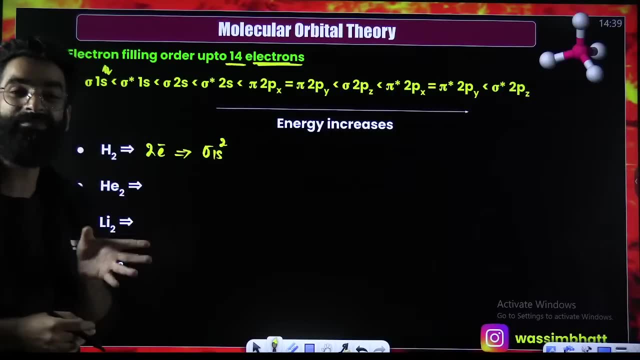 those 2 electrons will go here. so it is going to be sigma 1 is 2, sigma 1 is 2 configuration, All the starred 1s, the ones which have got star on them, they are anti-bonding molecular. 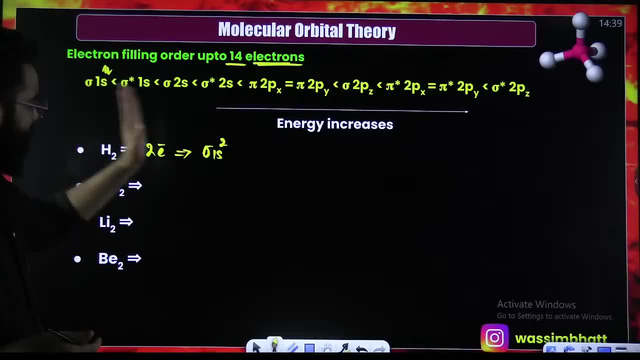 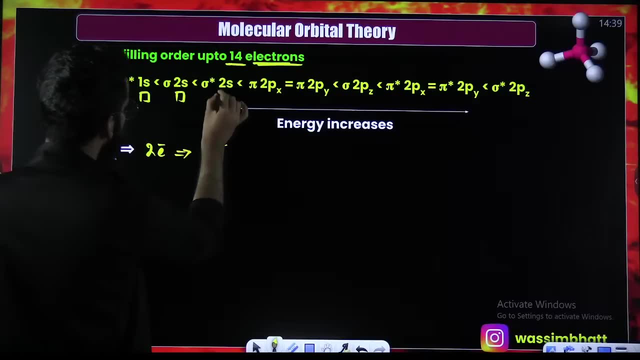 orbital, the ones without star. they are bonding molecular orbital. so the configuration here is the molecular orbital configuration is sigma, 1 is 2, this is all. these are your molecular orbitals. this is P. do not do this. all these are molecular orbitals and every. 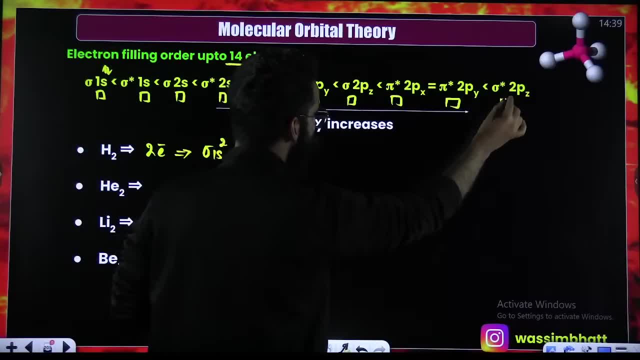 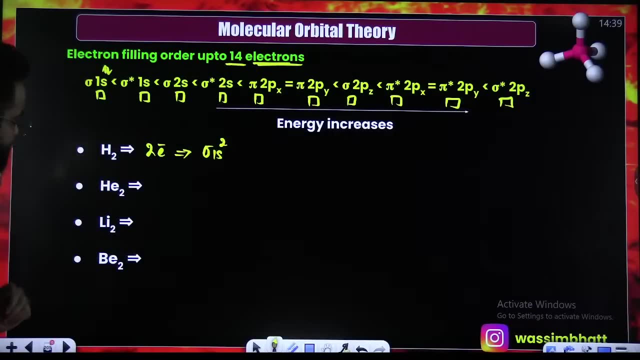 molecular orbital here can accommodate maximum of 2 electrons. all these molecular orbitals maximum can accommodate. Now guys understand, sigma 1 is 2, sigma 1 is 2, over here total 4 electrons. so adjust those 4 electrons, 2 here, 2 here. so this is sigma 1 is 2, sigma star 1 is 2, 6 electrons. 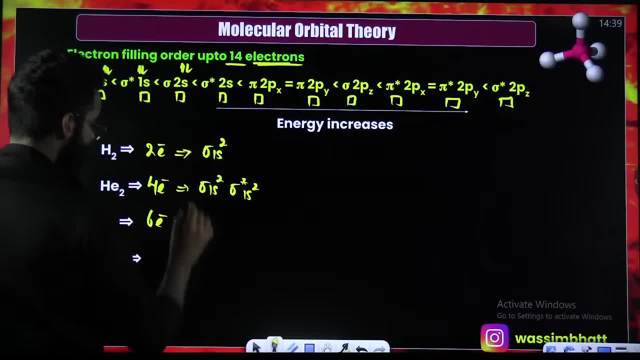 in total 6 electrons: 2 here, 2 here, 2 here. so this is: sigma 1 is 2, sigma star 1 is 2, sigma 2 is 2.. 8 electrons in total: 8 electrons: 2, 4, 6, 2, 4, 6, 8.. 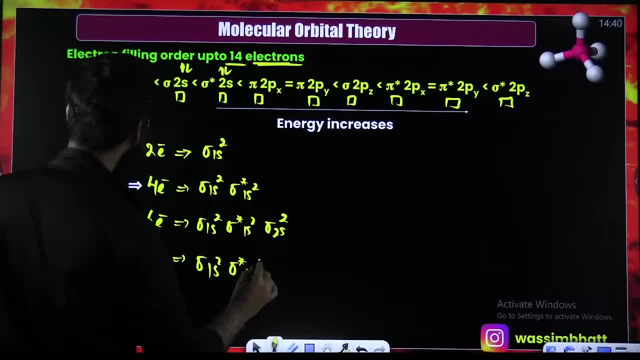 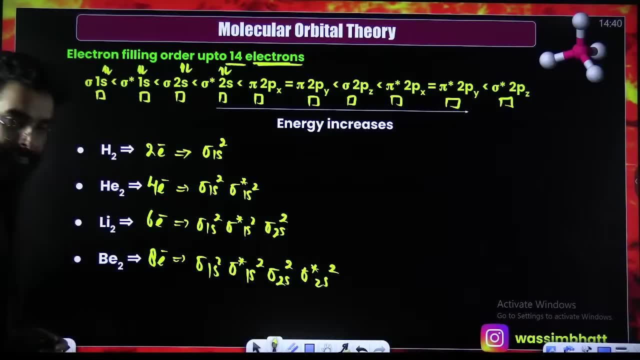 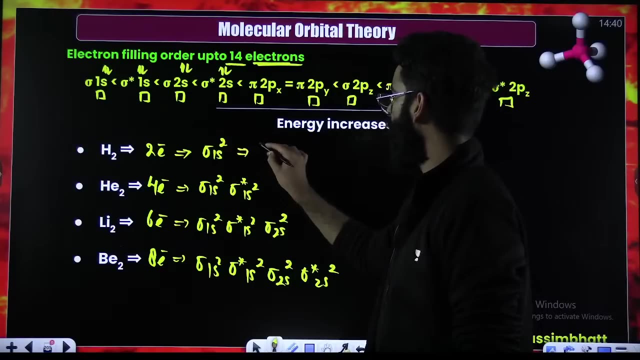 This is: sigma 1 is 2, sigma star 1 is 2, sigma 2 is 2, sigma star 2 is 2,. okay, I wrote the molecular orbital configurations of these species. After writing the molecular orbital configurations of these species, now what do I need to calculate? 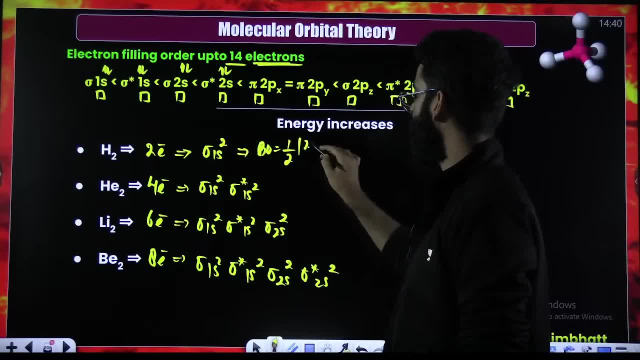 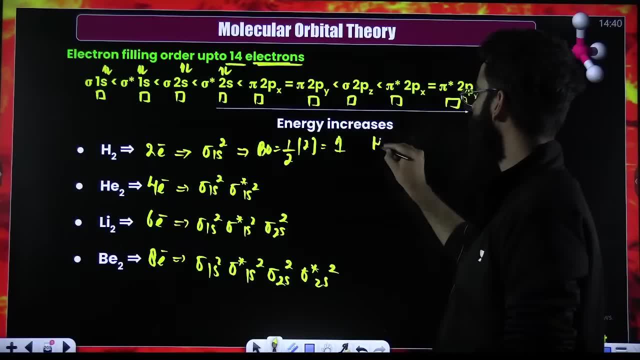 bond order. It is half of number of electrons in bonding, 2.. Minus anti-bonding is 2.. Okay, Bonding is 0, so the value comes out to be 1.. Bond order is 1.. If bond order is 1,, that means between 2 hydrogen atoms there is a single bond. 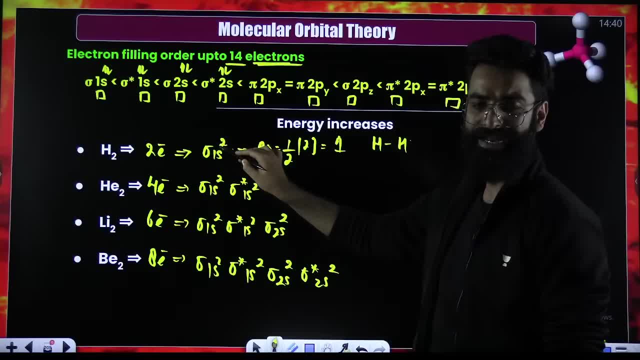 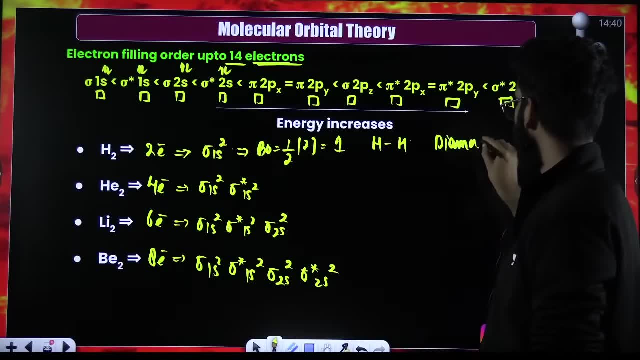 Do you see any unpaired electron here? Every molecular orbital can adjust maximum of 2 electrons and those 2 are equal right. So this species is basically diamagnetic. If you ask me its magnetic moment, it's going to be 0.. 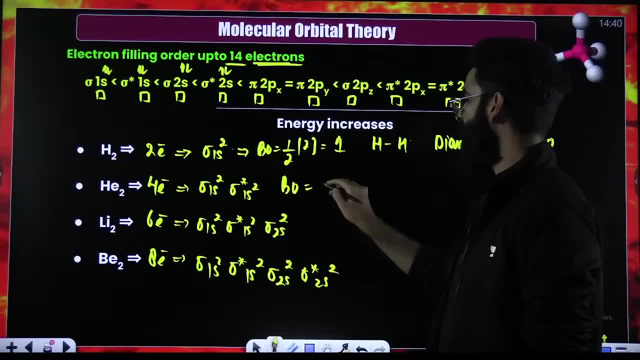 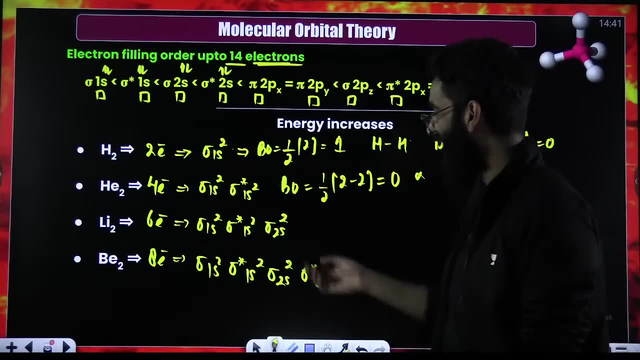 Over here: 2 electrons in bonding, 2 in anti-bonding. Calculate the bond order: It is half of number of electrons in bonding minus number of electrons in anti-bonding. bond order is 0.. So this molecule does not exist, right. 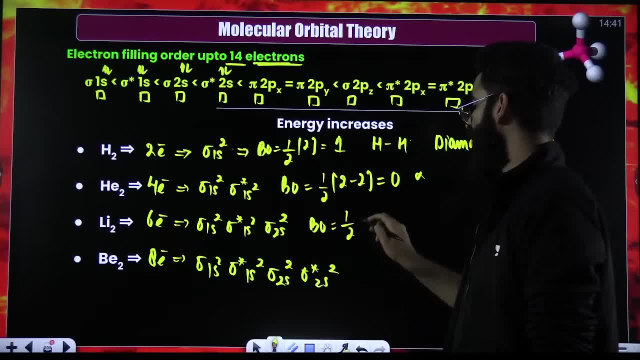 Li2.. Li2.. Calculate the bond order: Half of number of electrons in bonding 2, 4.. Minus anti-bonding: 2.. 4 minus 2 is 2.. 2 by 2 is 1.. 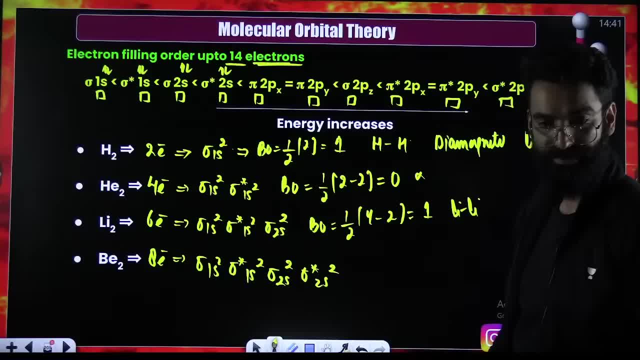 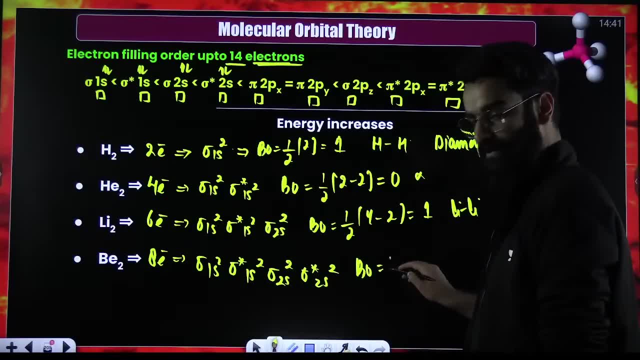 So bond order is 1.. That means there is a single bond between 2 lithium atoms. Single bond between 2 lithium atoms right. Look at the next one: Be2.. 8 electrons. Calculate the bond order. Calculate the bond order. 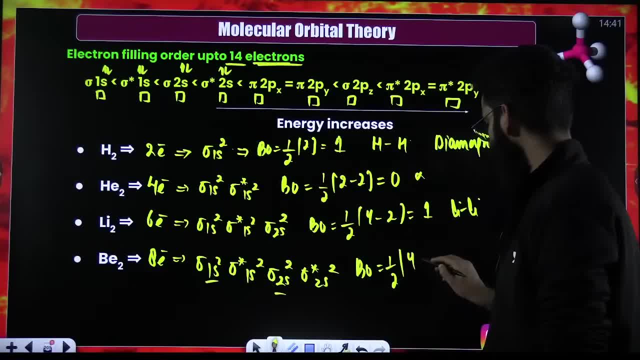 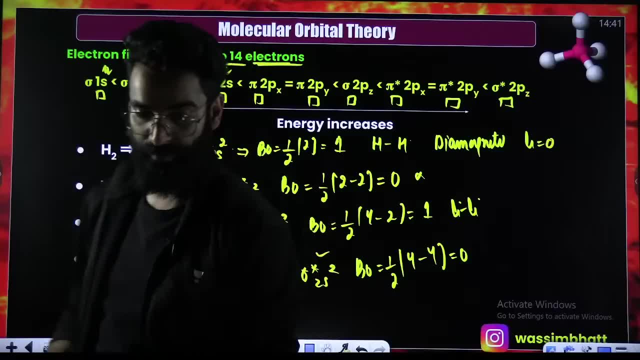 Half of number of electrons in bonding 2, 4.. Minus anti-bonding 2, 4.. Right, The value comes out to be 0.. Molecule does not exist. Non-viable, Non-viable molecule. 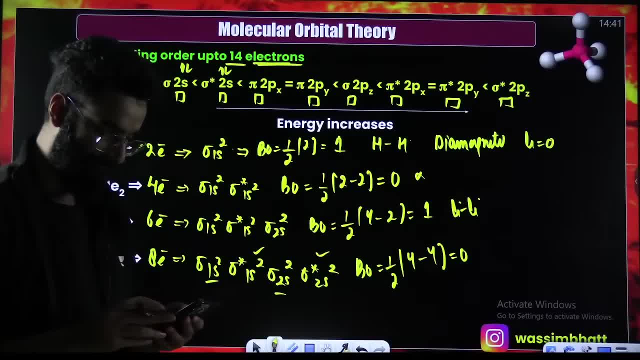 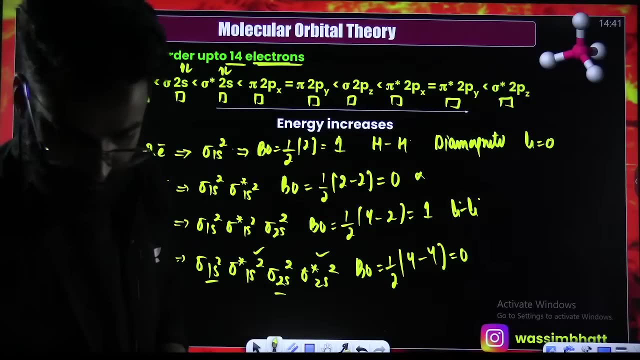 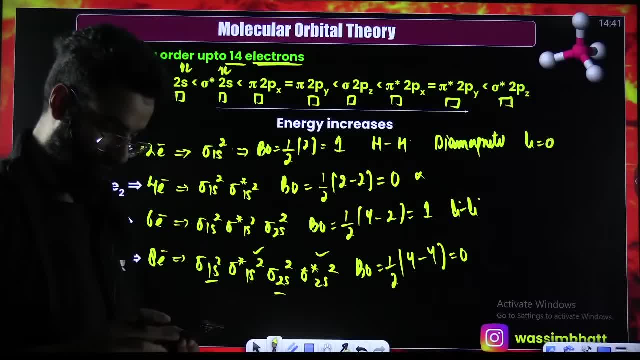 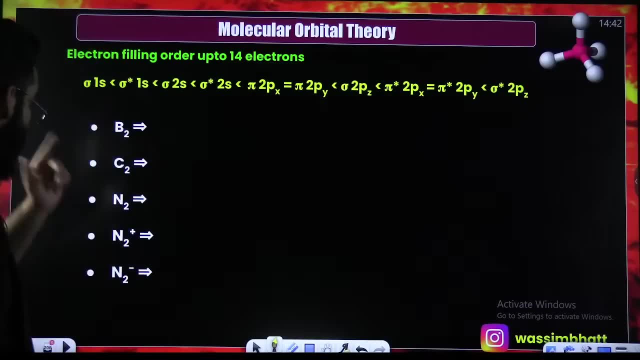 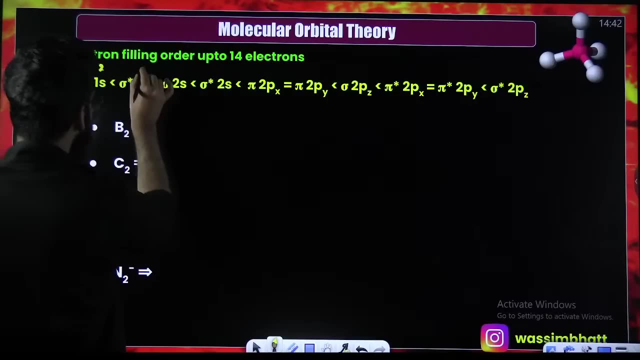 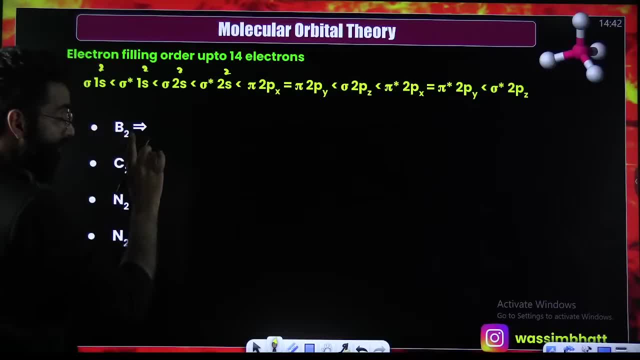 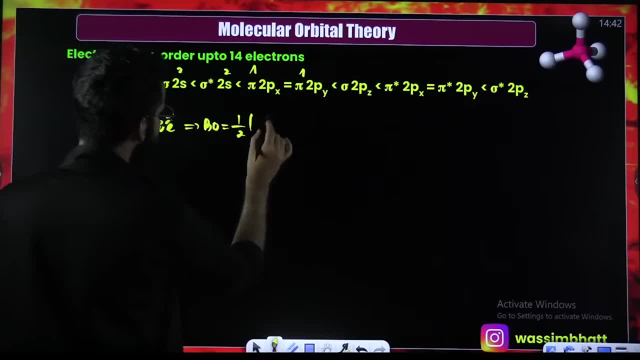 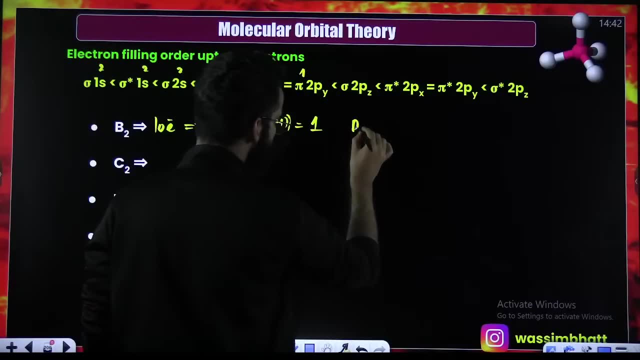 of Number of electrons in bonding: 2,, 4,, 5,, 6.. Minus anti-bonding: 2,, 4.. Right, The value comes out to be 1.. So in case of B2, there is a single bond. There is a single bond. 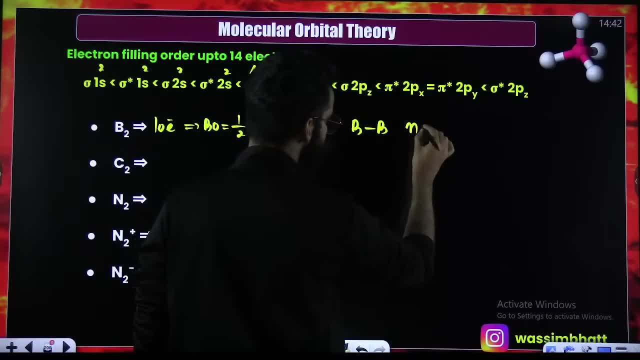 Is there unpaired electron? Yes, This is unpaired. This is unpaired. There are 2 unpaired electrons, 2 unpaired electrons. Calculate the magnetic moment Under root of 2 into 2 plus 2.. 2 plus. 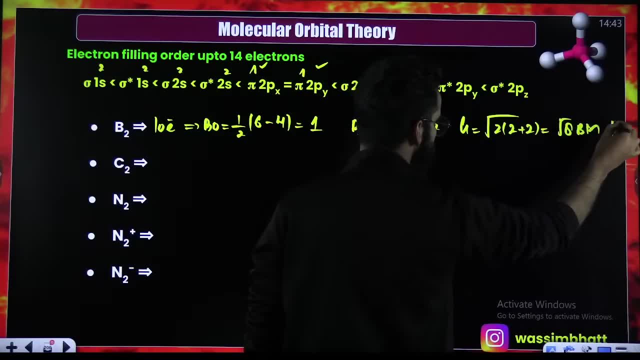 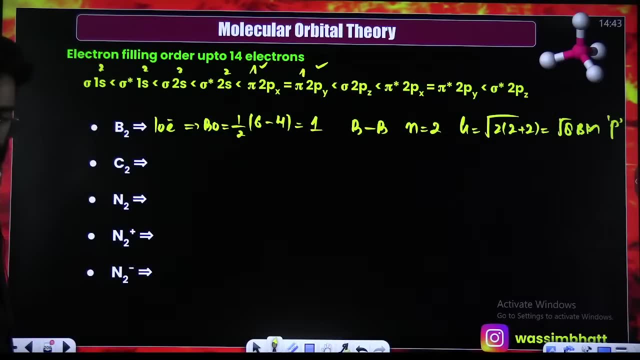 2 is 4.. 4 plus 2 is 8.. Root: 8 Bohr magnetrons. So this particular species is paramagnetic. This particular species is paramagnetic in nature. Paramagnetic in nature, Okay, Talk about C2.. Total: 2 electrons: 10. we have already filled Now 11.. Right, So calculate the bond. 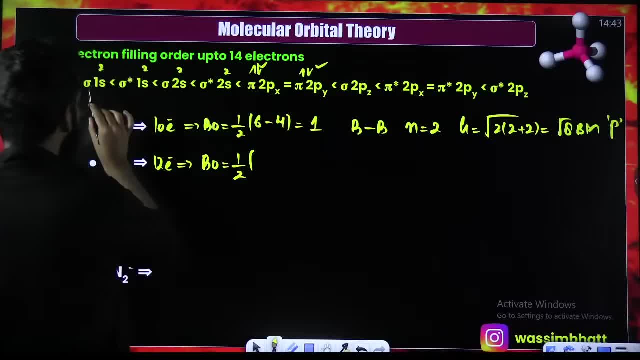 order: Half of Number of electrons in bonding 2,, 4,, 6,, 8.. Minus anti-bonding 2, 4.. 8 minus 4 is 4.. Right, So calculate the bond order. Half of Number of electrons in bonding 2,. 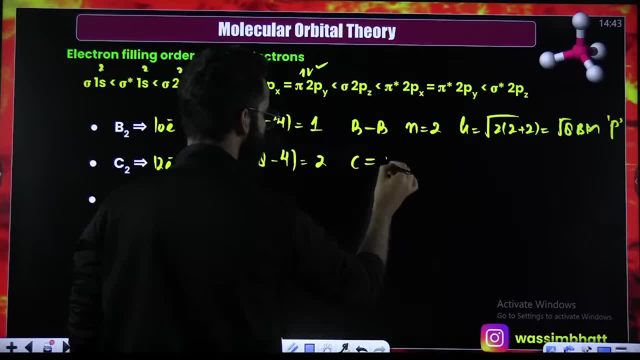 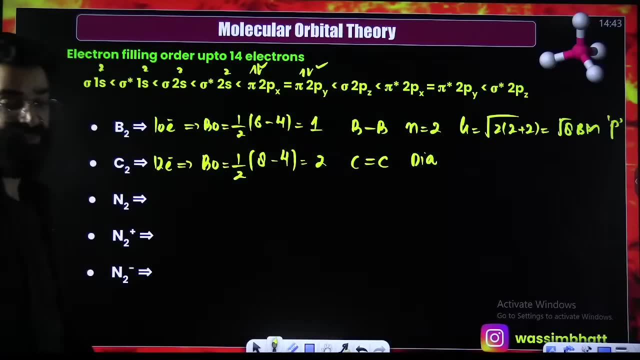 4.. 4 divided by 2 is 2.. So bond order is 2.. So in case of C2, the bond order is 2.. Is there any unpaired electron? No Species is diamagnetic Now C2.. There is a special 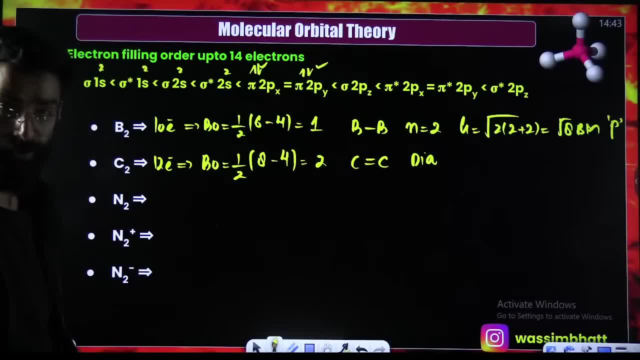 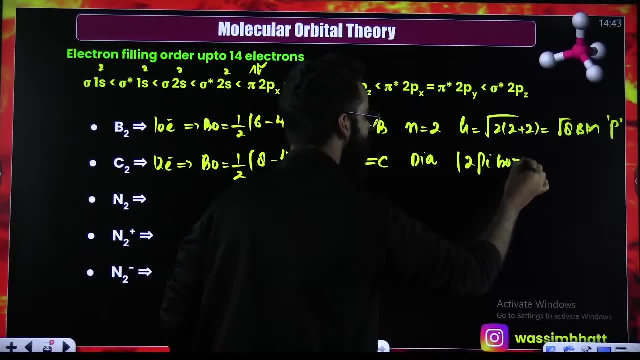 case, C2 is the only molecule. Let me tell you C2, it is the only molecule wherein both the bonds here are pi bonds. Otherwise it should have been what It should have been, what One should have been sigma, One should have been pi. But C2 is the only molecule. 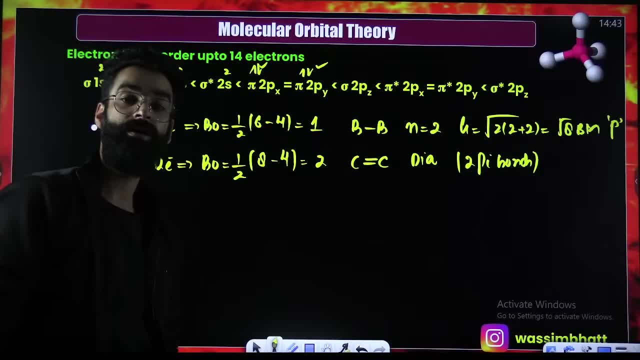 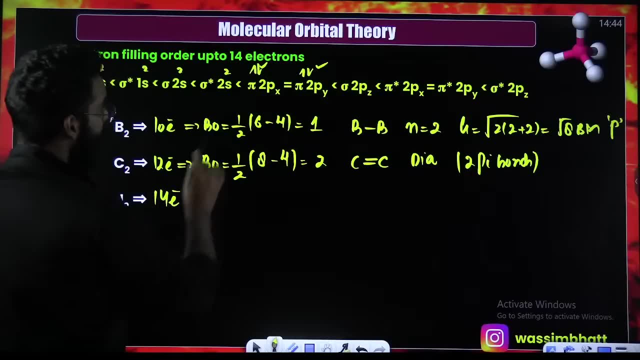 which MOT says that it has got both the bonds. So it is the only molecule which MOT says it has got both the bonds. So oh, is this the other one? So we have caught both 2 electrons. We have caught both C2 and C3 here. Of course, this is not the only molecule. Ok, Let us. 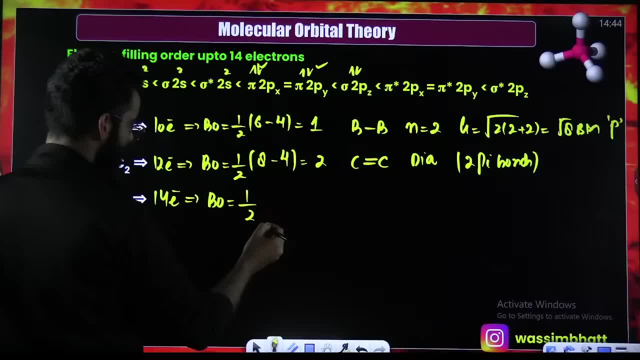 switch it to the other side. We have caught both 2 electrons. Now it says C2.. And here is the third molecule. so the second molecule. This marker tells us its number 2 is 4.. We will check this number. I have made abeca succeeding 5 in this value line issue. If�ju. 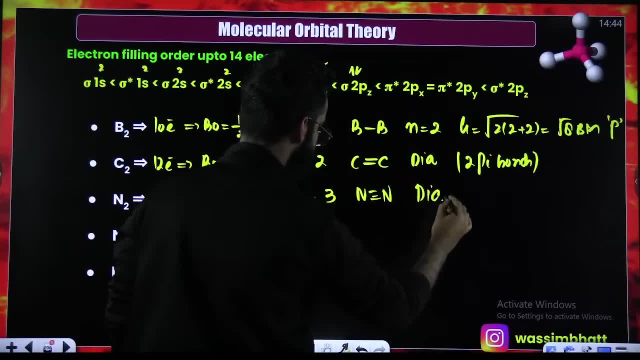 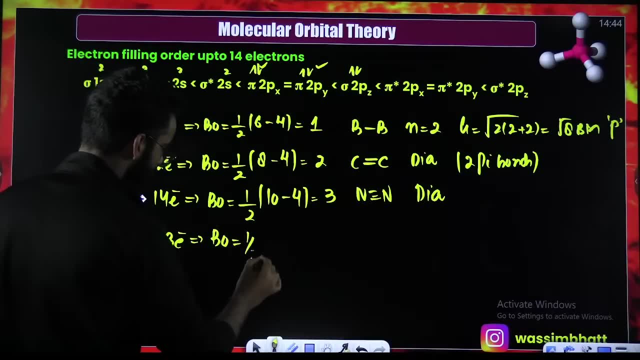 lyIi Combined as π bonds: N2.. 14-lectron species: Right, 12, we have filled 12, n2 makes it 14.. Right, So bond order: you right: N2. positive 14 minus 1, 13 electrons: 13 electrons Bond order is equal Half of electrons. 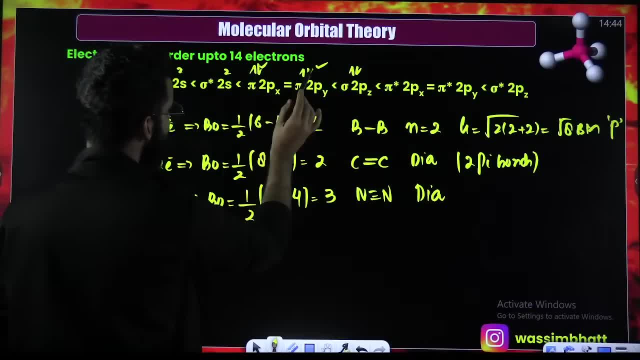 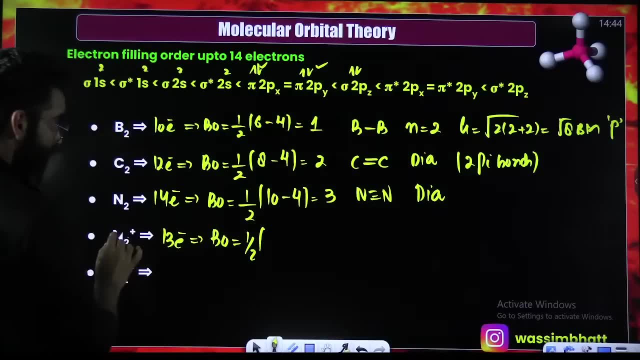 bonding 2, 4, 6, 8 and 1, 9.. 1, 9 because I am not going to consider 2 because 1 electron has been taken out. It is N2 positive, right, It is 13 electron. It is 13 electron 1. you have to. 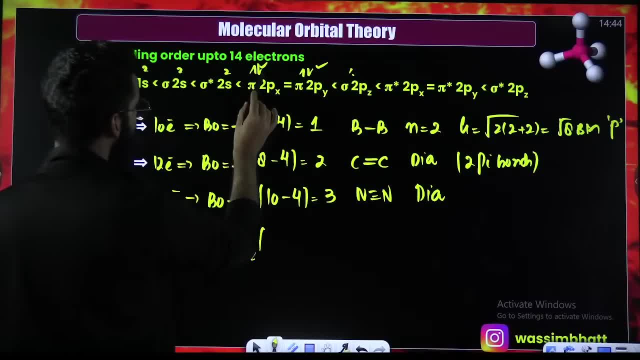 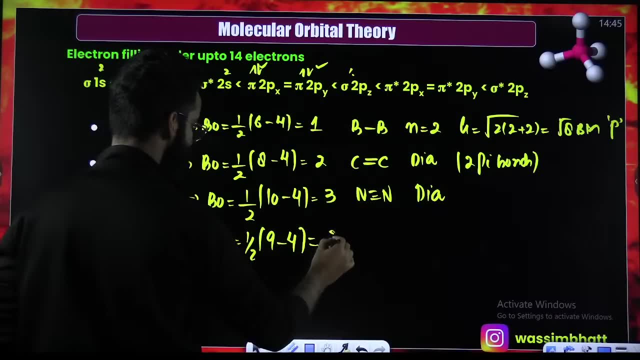 remove How much. it was 2, 4,, 6, 8, 9.. Minus Entity bonding: 2, 4.. Correct: 9 minus 4 is 5. 2.5. Perfect. Similarly, when you calculate this, it will also come out to be 2.5 only. 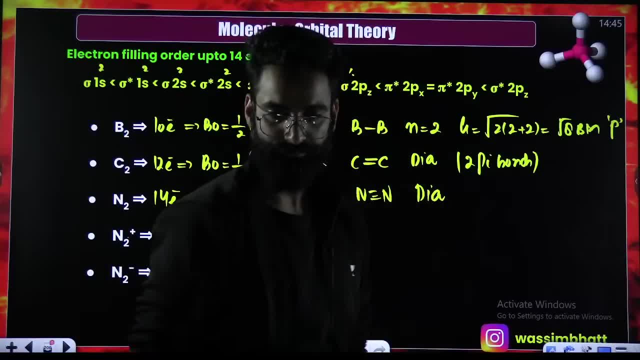 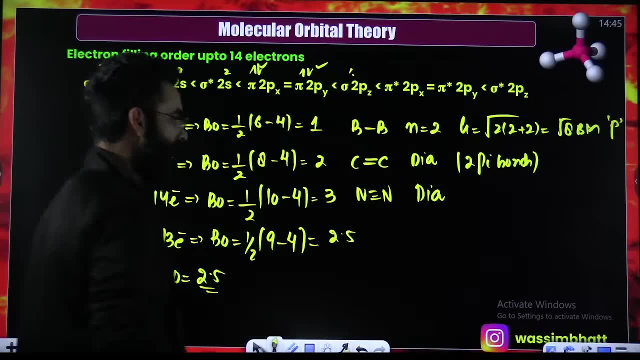 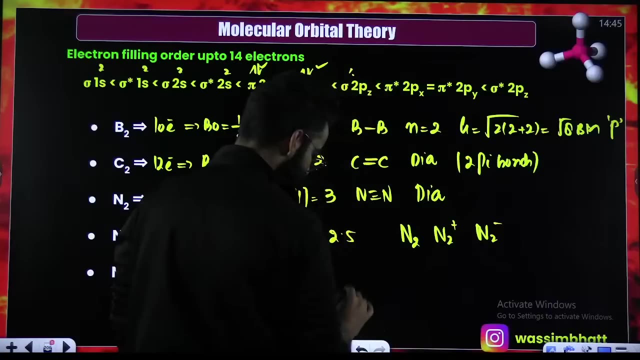 Am I clear? Am I clear? people, Am I clear? Am I clear? Am I clear? Quickly, Am I clear? One question: I have One question I have. I have got N2.. I have got N2 positive, I have got N2 negative. Can you give me the order of their stability? 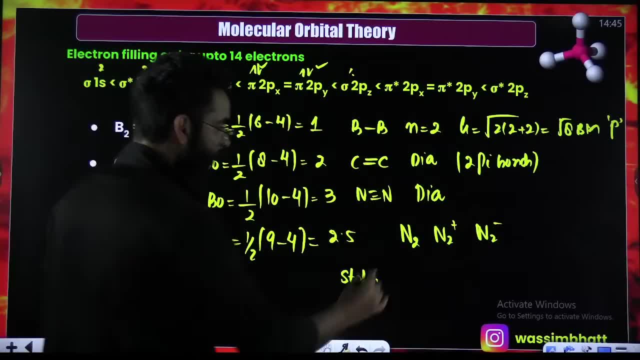 Can you give me the order of their stability? More the bond order, more the stability. Bond order: here is 3.. Here it is 2.5.. Here it is 2.5.. So more the bond order, more the stability. 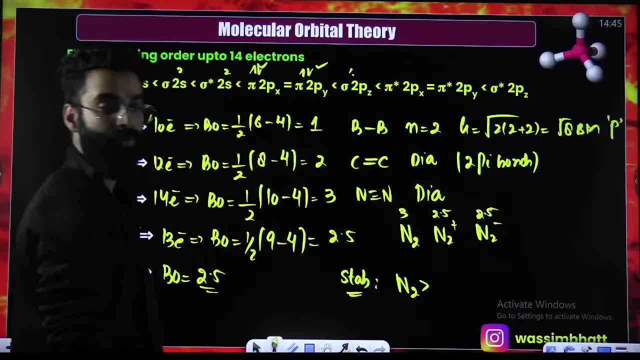 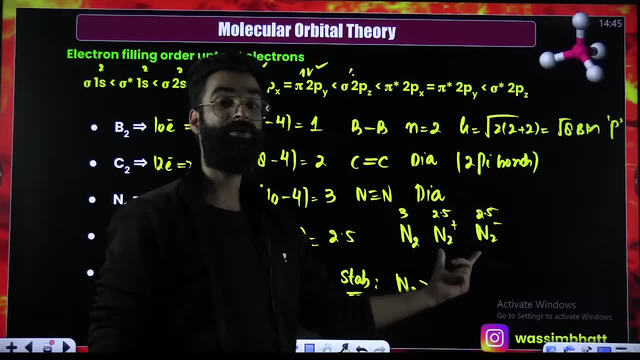 So N2 will be maximum stable right Now among N2 positive and N2 negative, Since bond order is same. now you will write their molecular orbital configurations and then you will see the number of entity bonding electrons. More entity bonding electrons- less electrons. 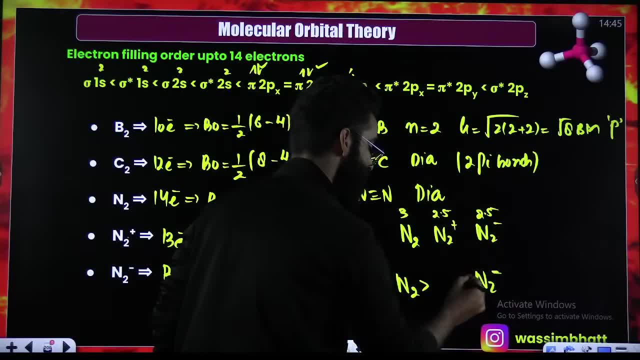 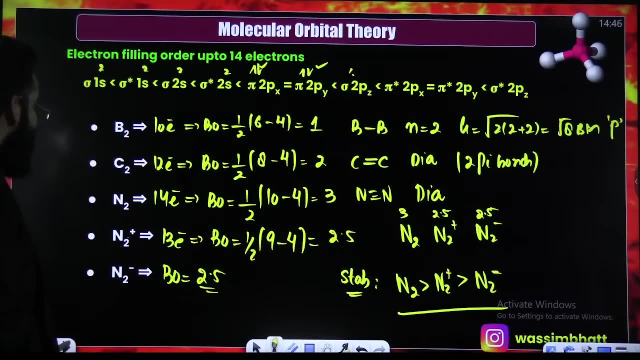 That is stability. Entity bonding electrons are more in N2 negative right, So least stable, and N2 positive comes in the middle. This is the stability order. Got it? This is the stability order. Similarly, guys, this is the electron filling order of the species which. 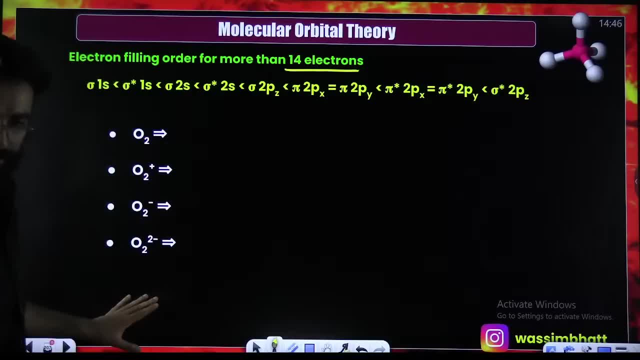 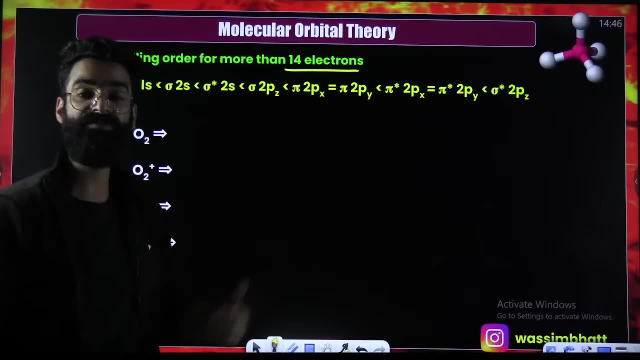 contain more than 14 electrons. Accordingly, same thing you need to do here. Accordingly, same thing you need to do here. This is the electron filling order of those species which contains electrons greater than 14.. Okay, Greater than 14.. 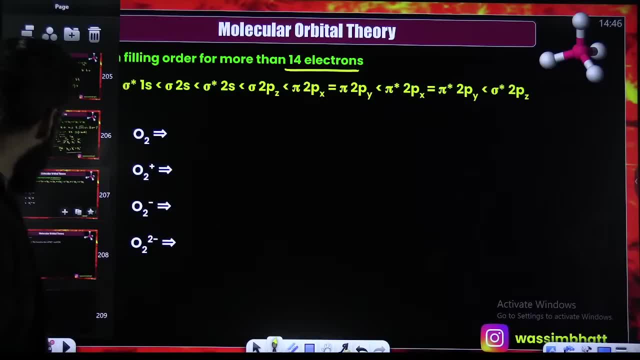 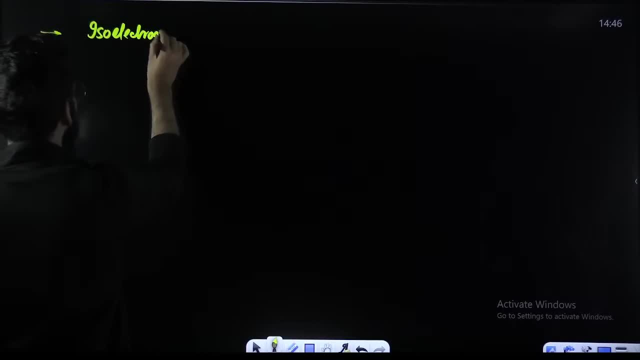 Greater than 14.. There is one thing which I would want to tell you right now. I hope you know what are isoelectronic species. I hope you exactly know what are isoelectronic species. Tell me what are isoelectronic species. 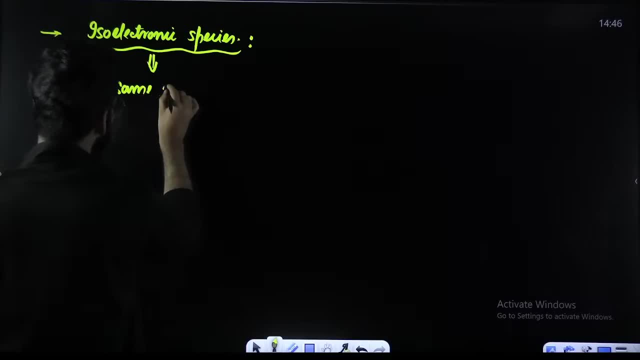 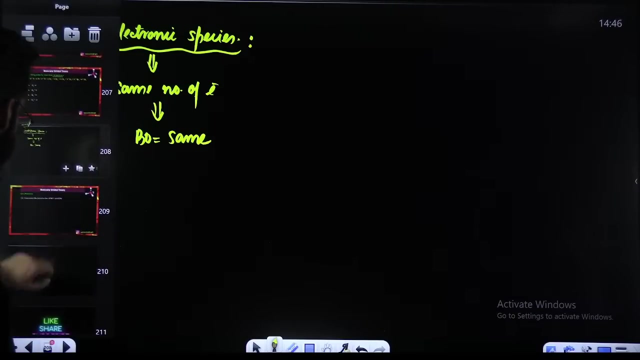 Isoelectronic species are the ones which have got same number of electrons. And whenever you see isoelectronic species, do remember their bond order is same. Do remember their bond order is same. Do remember their bond order is same. Okay, There is a question asked from that as well. 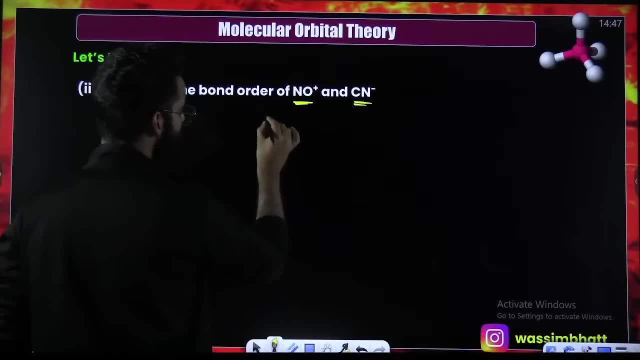 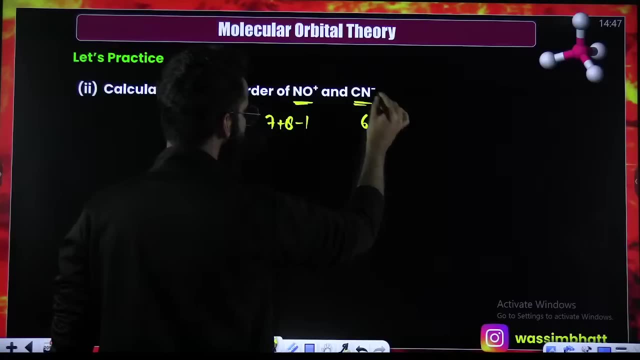 Calculate the bond order of NO positive and CN negative. NO positive: Nitrogen 7, oxygen- 8.. Subtract this positive charge: Carbon 6, right. Carbon 6, nitrogen 7, negative charge, So add this one, So 8, 7, 15 minus 1, 14.. This is a 14 electron species: 7, 6,, 13,, 1,. 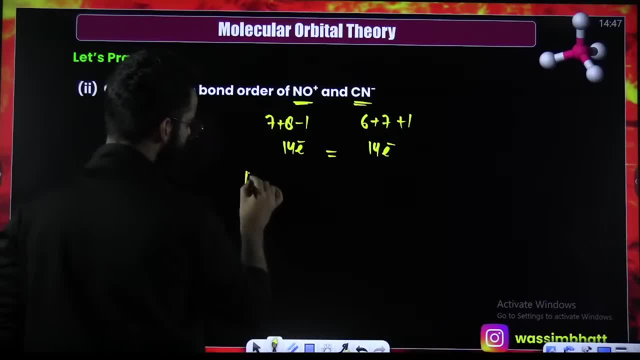 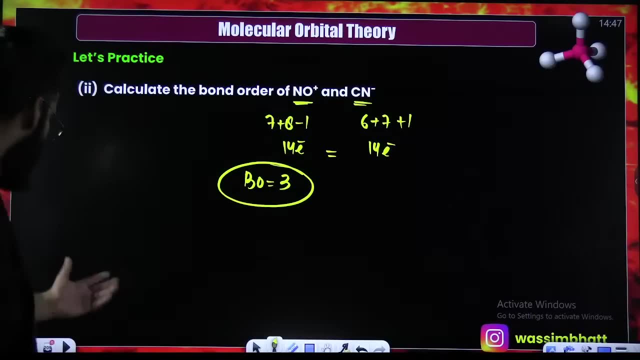 14. It is a 14 electron species If electrons are same. but all the 14 electron species, they have got bond order 3, right, They have got bond order 3.. And I hope you know the trick also to calculate the bond order. Perfect. Let me write the trick. If the total electrons are 14,, 15,, 16,, 17,, 18,, 13,, 12,, 11, 10.. All the 14 electron species, they have got bond order 3.. Now decrease by 0.5.. Decrease by 0.5. 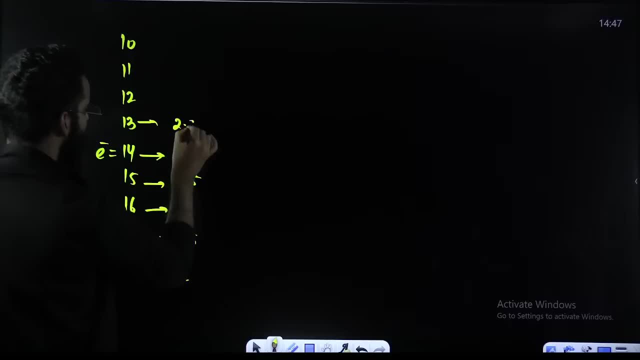 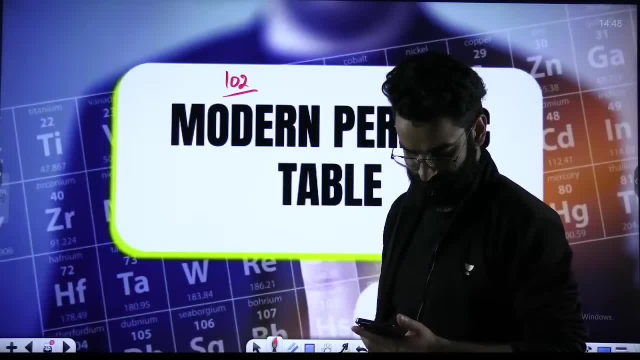 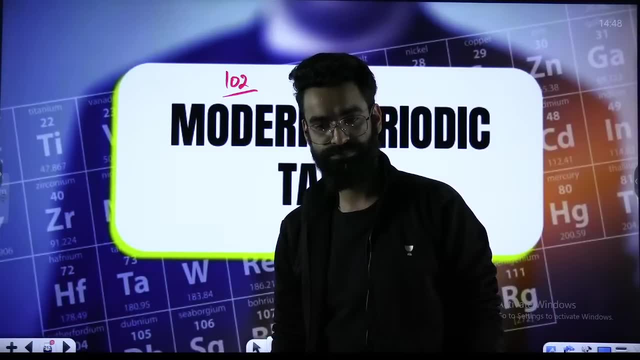 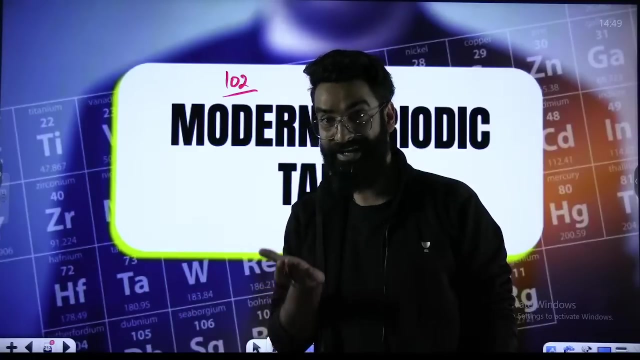 by 0.5.. Decrease by 0.5.. Decrease by 0.5.. Decrease, See, you get intensity of how unwell I am. Trust me, I'm standing right now. I feel like my legs will break in between. 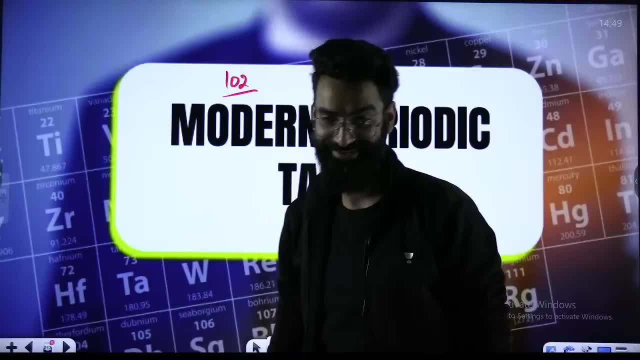 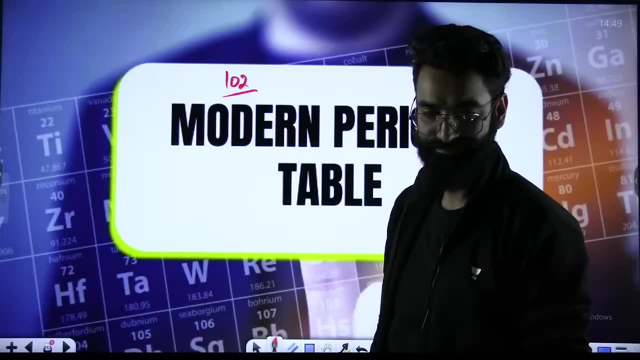 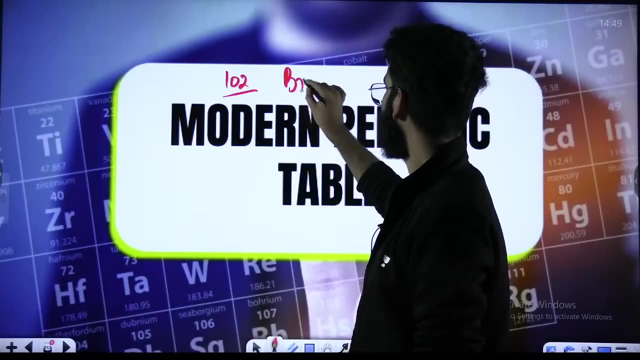 It will break at the knees, trust me on that. So I would need more breaks today. So it's 2.50 right now. let's get back at 3.10.. But I would want you guys to be back on time. 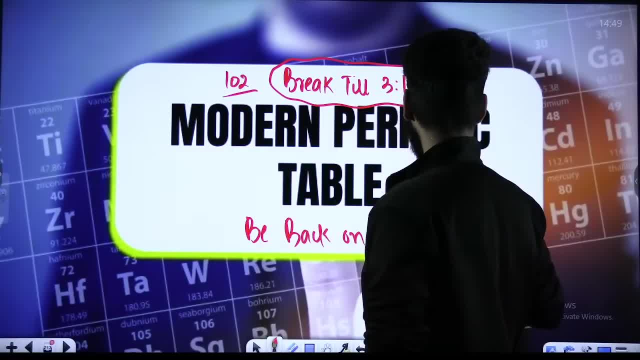 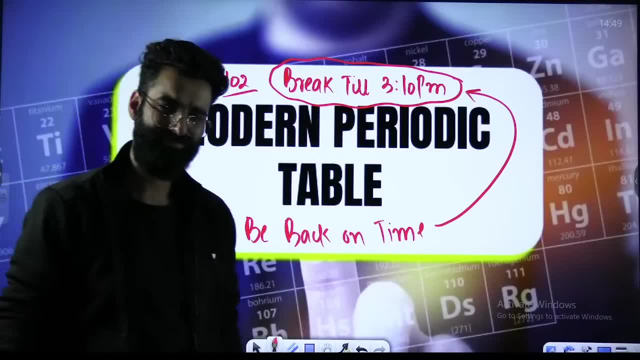 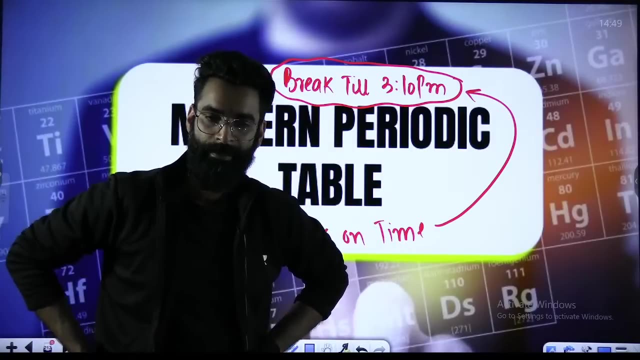 Because this is the only chapter which we have to do: Periodic Classification. and we are done, And we are done. Periodic Classification will not take more than two hours, Not more than two hours, And everything will be taught. Everything will be taught. 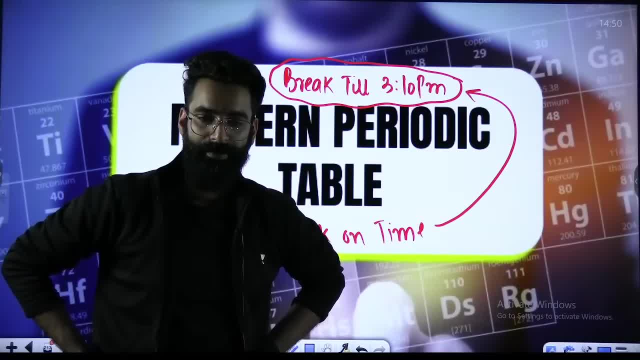 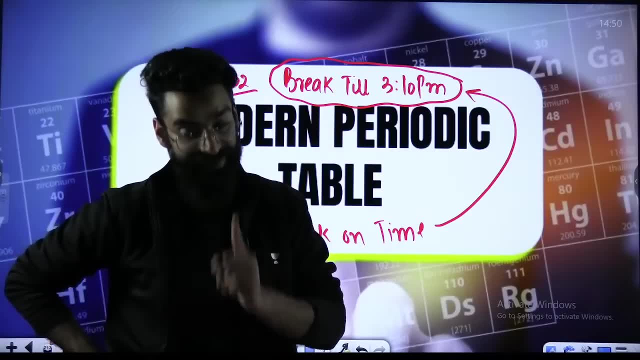 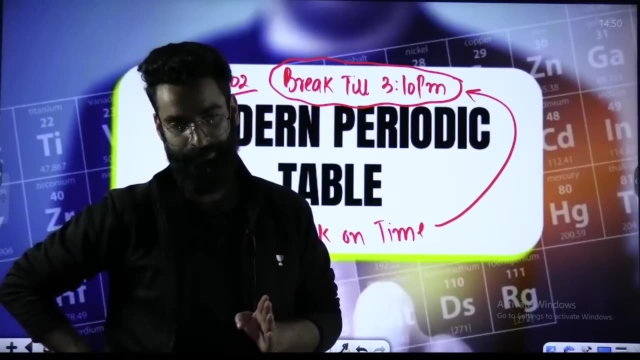 P Block. guys listen P Block we'll do in class 12th in Organic Marathon. Today it's the 12th, It's class 11th in Organic Marathon. let me tell you once again: It's class 11th in Organic Marathon today. 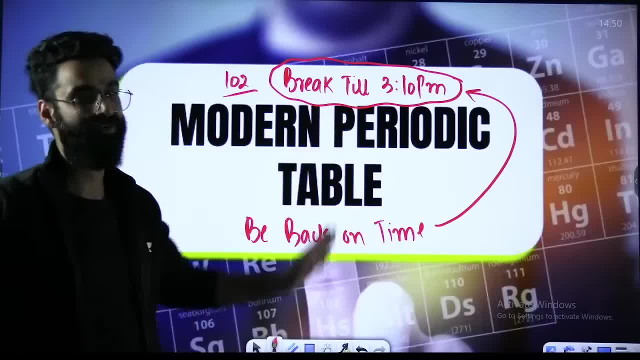 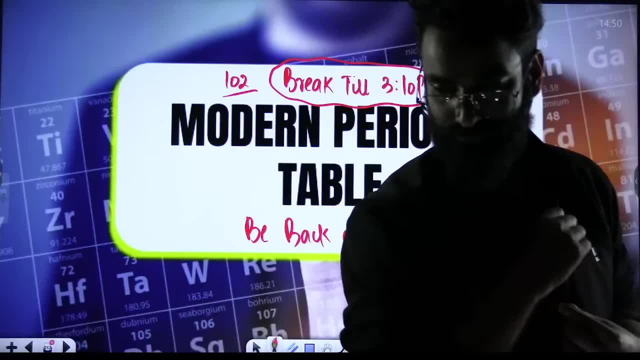 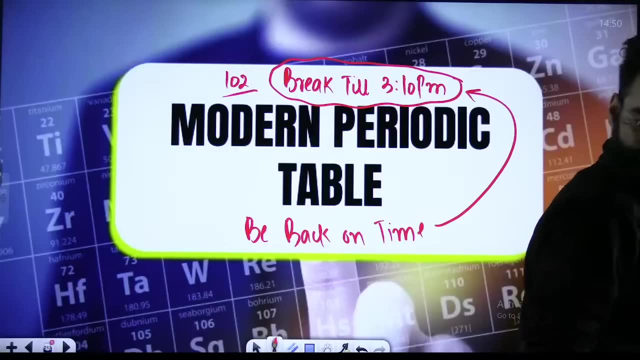 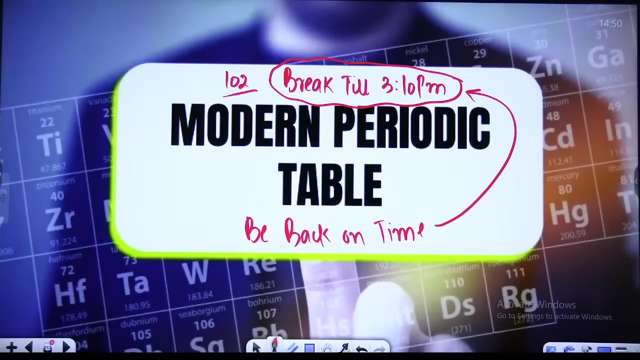 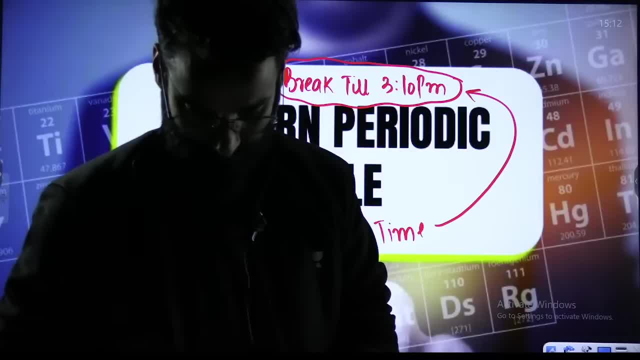 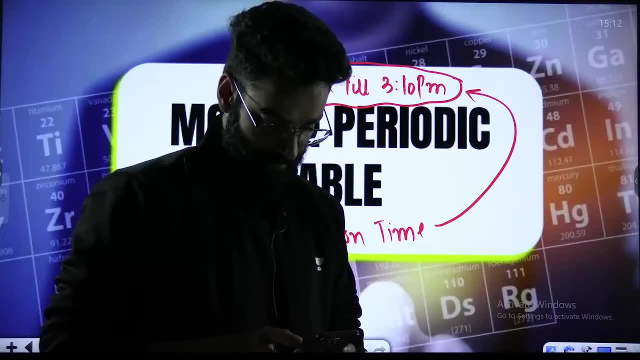 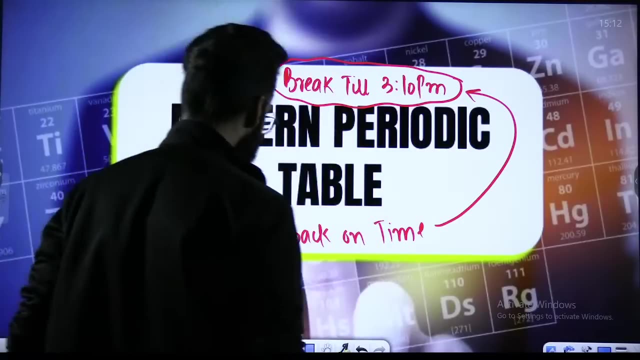 Bye, Bye, Bye, Bye. Is everyone back? Is everyone back? Yes, Let's complete this chapter. also Periodic classification, And we are done with class 11th in organic chemistry. guys, Okay, And tomorrow we will have the extra question practice session. 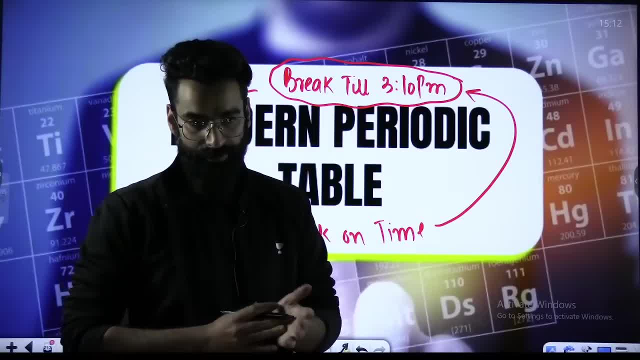 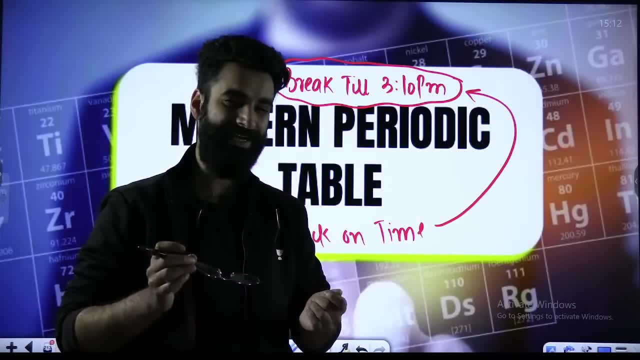 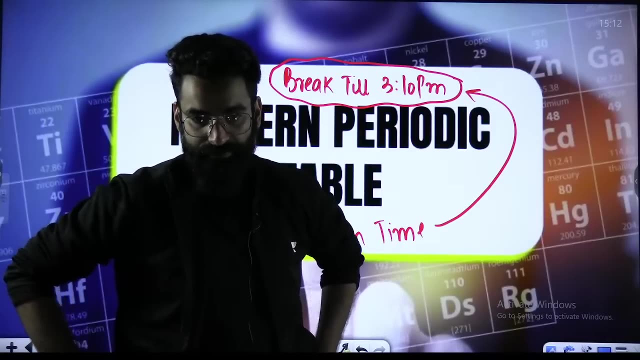 Perfect. After watching these two sessions- Today's session and tomorrow's session- You are not supposed to solve any other thing. Okay, That is more than sufficient. That is more than sufficient for you. That is more than sufficient for you. Welcome back. 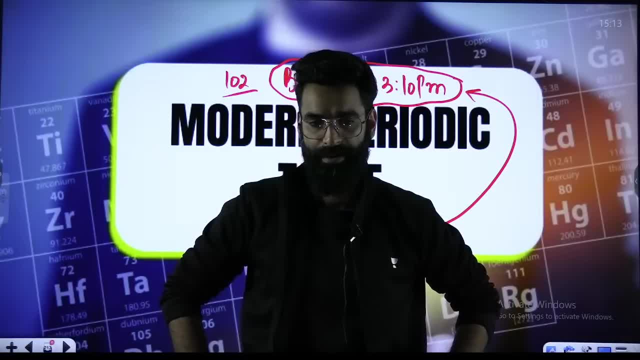 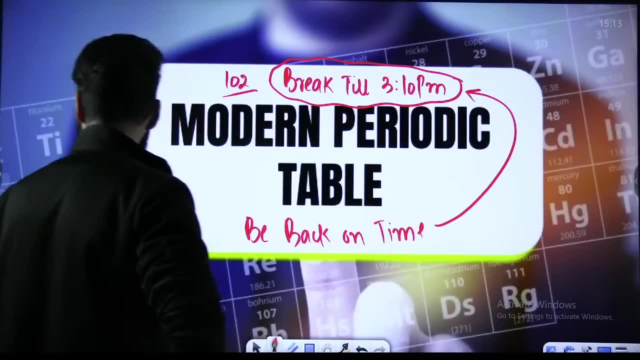 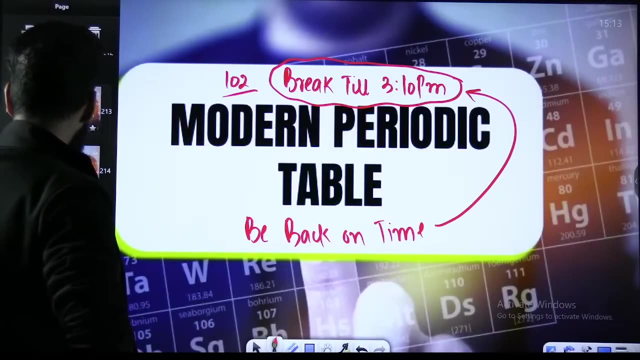 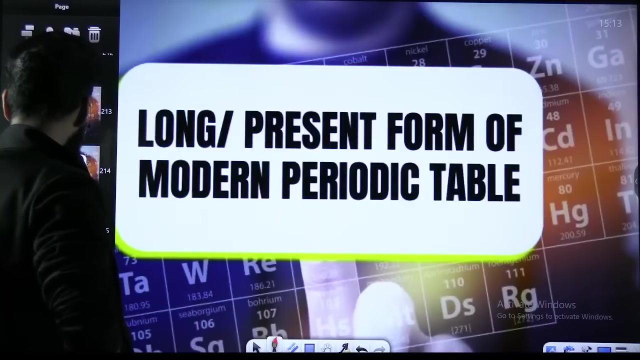 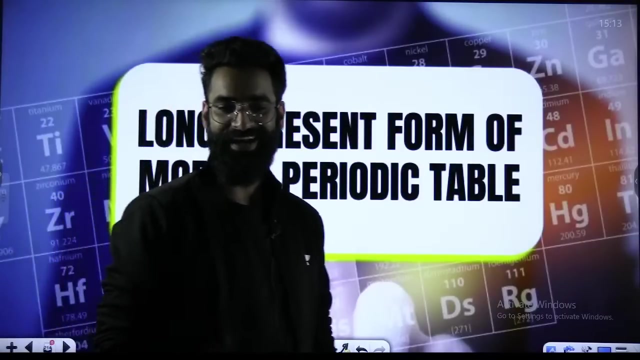 Welcome back. Okay, Have you studied this chapter before? Have you studied this particular chapter before? Tell me once in the chats. Tell me once in the chats. Have you studied this chapter before? Yeah, I know you have studied this for 9 hours. 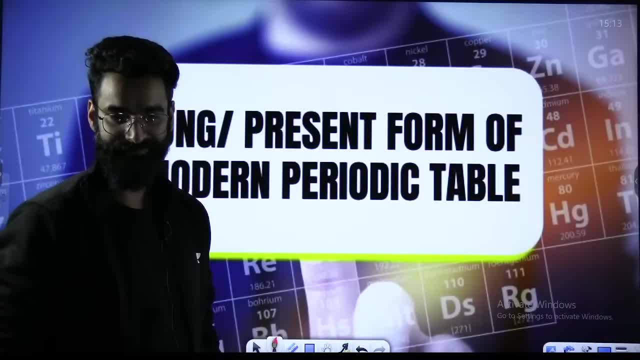 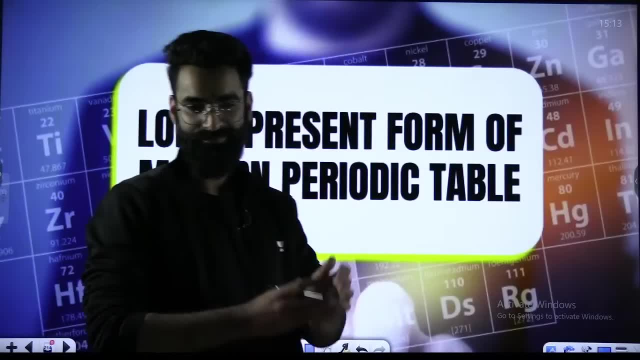 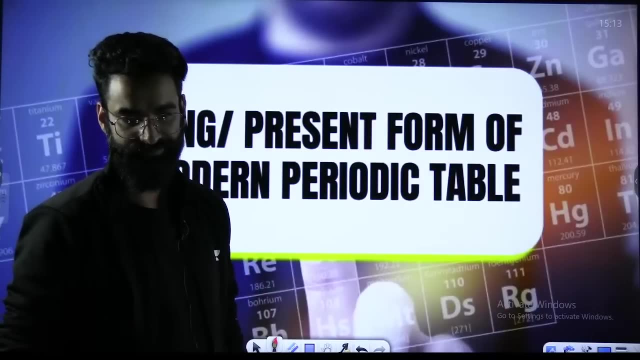 But I will complete it in just 2 hours. This is the easiest of all the chapters. You should know it. This is the easiest of all the chapters. You should know it. Okay, There is no need to remember all the elements in the Period table. 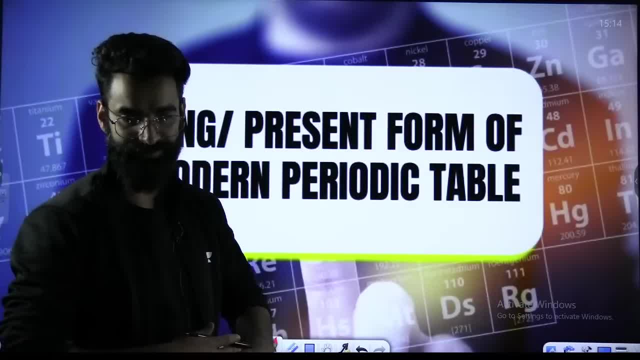 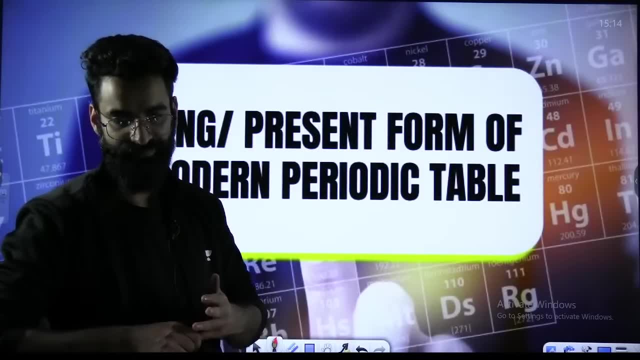 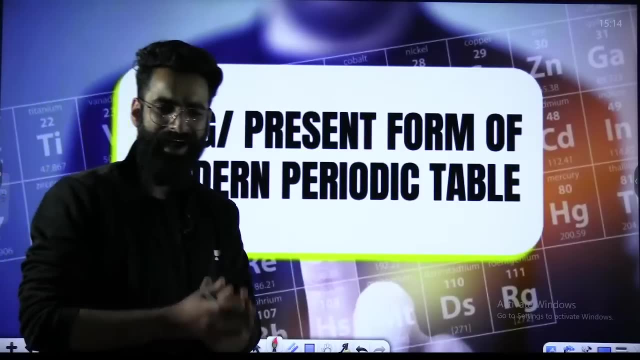 There is no need to remember all the elements in the Period table. Why would you do that? Why would you do that? Okay, Let's start with the Modern Period table. I believe at least you would have seen the Modern Period table once. 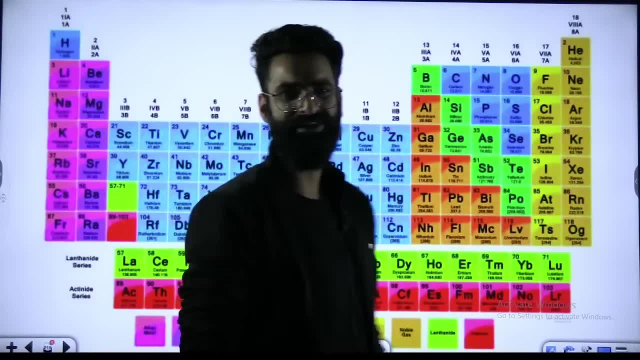 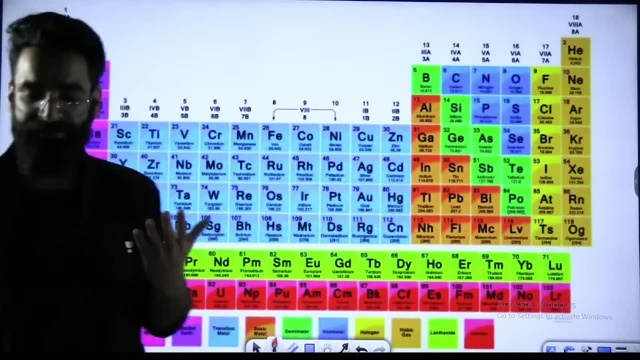 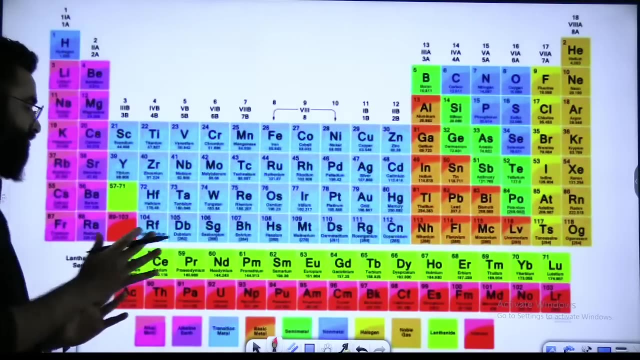 Right, This is your Modern Period table. this is your modern period table. you would have seen this, I believe. now, my dear students, there is some general information which you need to know about the modern period table. first. what is that general information? what is that general information? I'll be asking you the questions which I believe you all 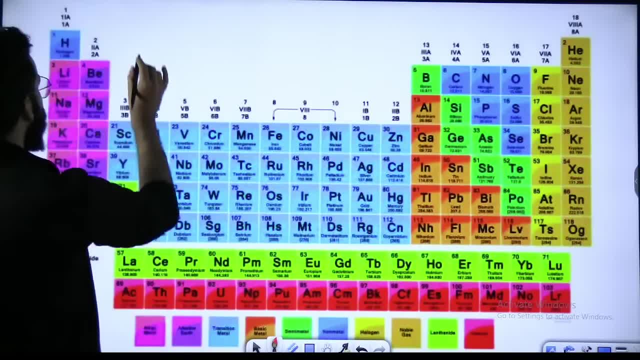 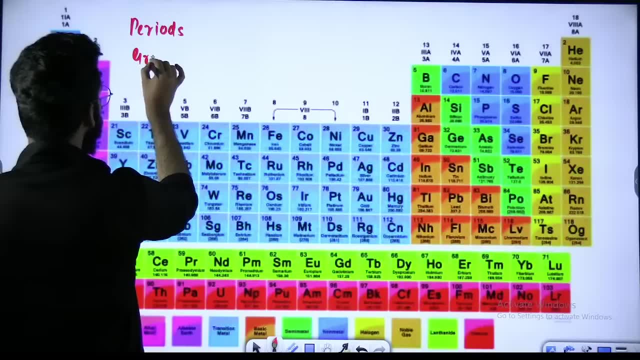 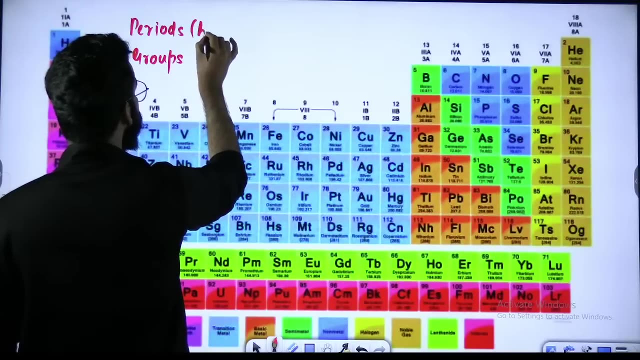 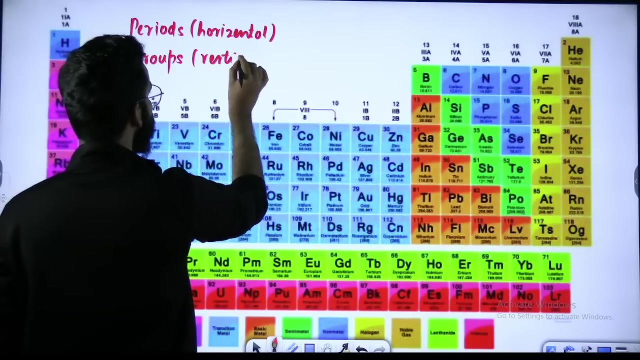 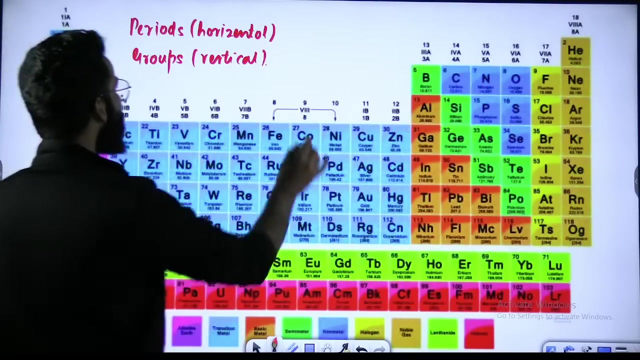 know right. can you let me know in the modern periodic table how many periods and how many groups are there? how many periods and how many groups are there quickly, everyone? this is something I believe everybody would be knowing right. there are seven periods here and there are 18. 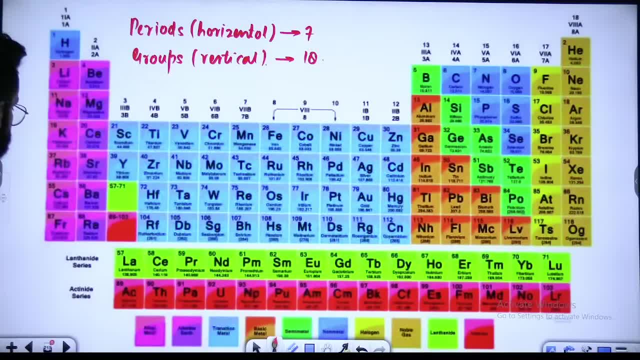 groups. there are 18 groups in total, right? if you see, this is your period 1, this is your period 2, 3, 4, 5, 6 and 7. so these horizontal rows over here are called periods. so you have got 7 periods in. 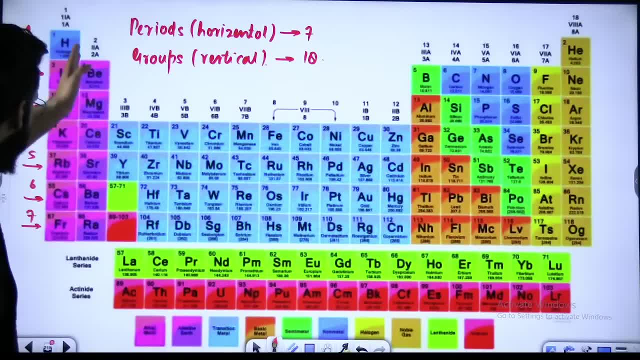 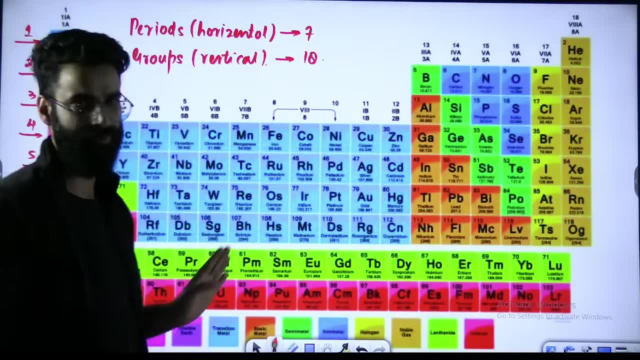 the periodic table. right and how many groups groups are these vertical verticals? one right: this is your group 1. this is group 2. this is group 3, group 4. so in total, we have got a 18 groups. Perfect, My dear students. this periodic table, the modern periodic table. 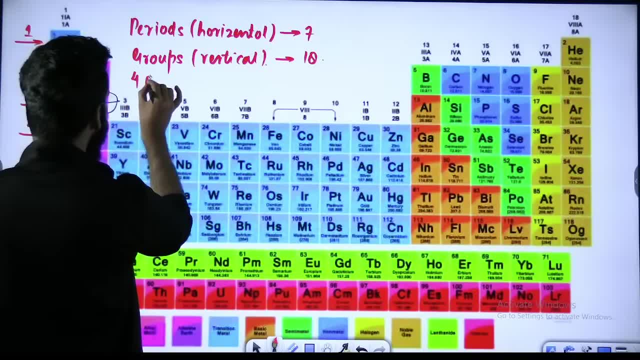 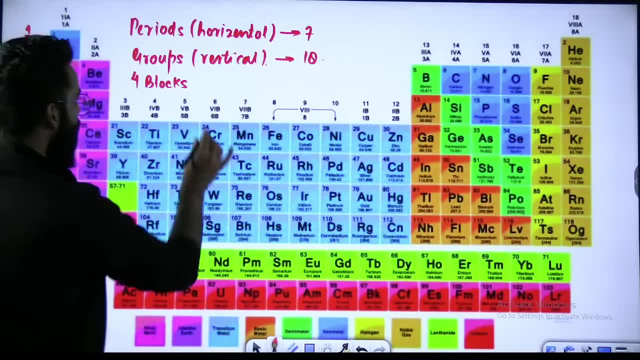 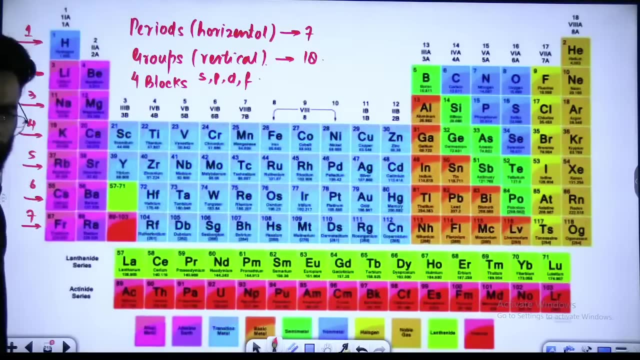 we have how many blocks are there? It is divided into four blocks. It is divided into four blocks. You should know it, Okay. S block, P block, D block and F block. Okay, If you see these two groups, the first two groups, the first two groups over here combinedly, 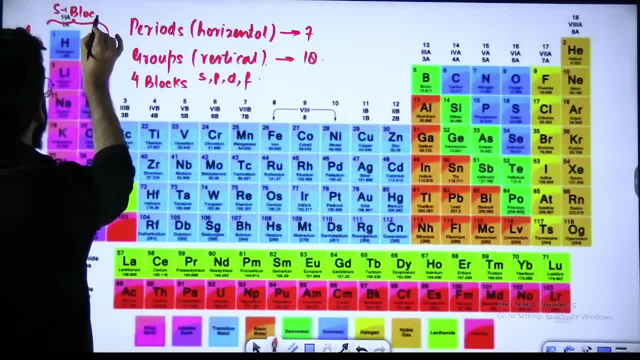 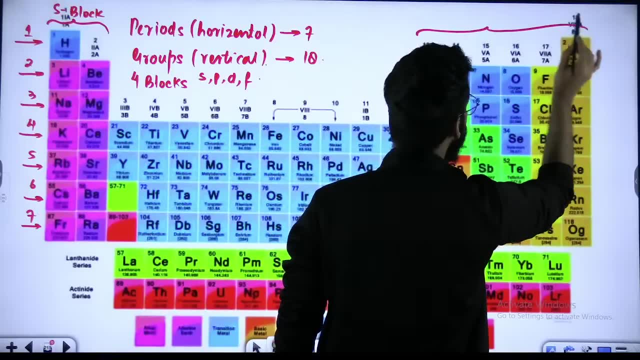 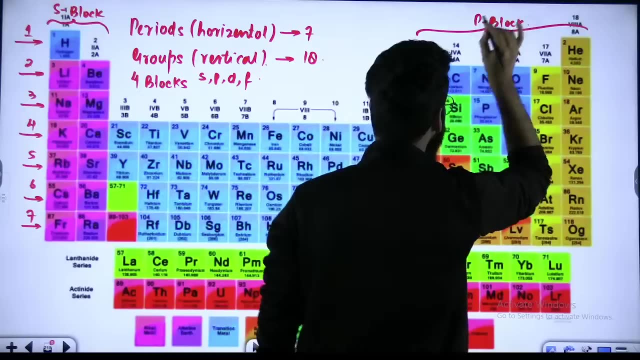 is called as S block, It contains your S block. Whatever P block: group 13 to the final group. group 13 till 18,: right, It is your P block. It is your P block, right. Perfect, And this. 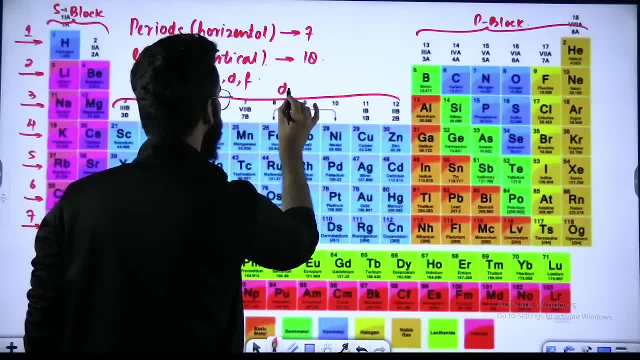 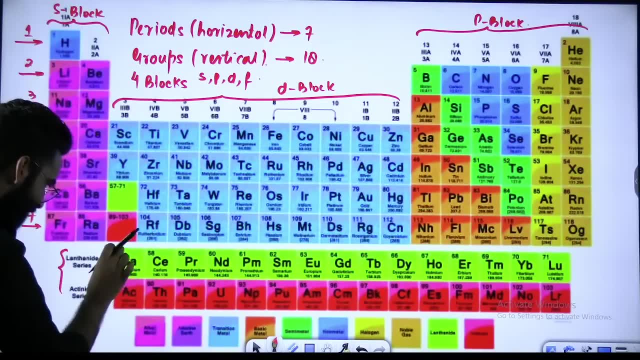 remaining P block. this remaining part, it is your D block And something which is excluded. I mean these two. they consist of your F block, elements Perfect. The first series over here is called as lanthanide series, starting from 57.. The second series over here is called as actinide. 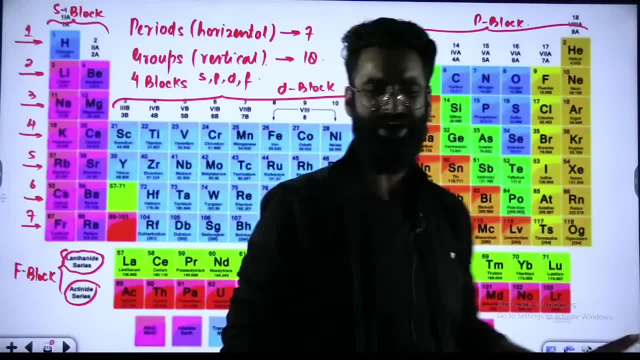 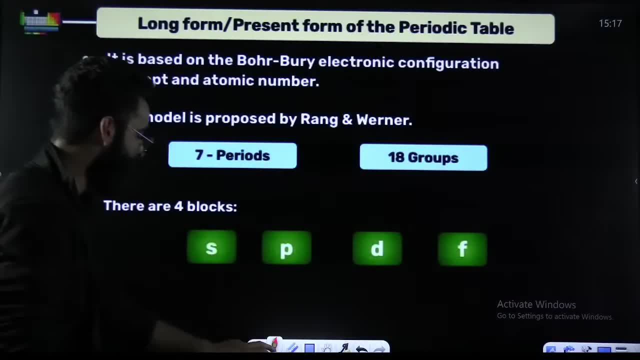 series. This is the general information about what. This is the general information about the periodic table. So, basically, what you have to remember over here in the period table: First of all, this period table, the modern period table which we have, it is based on Bohr-Burry's electronic configuration right. It is based 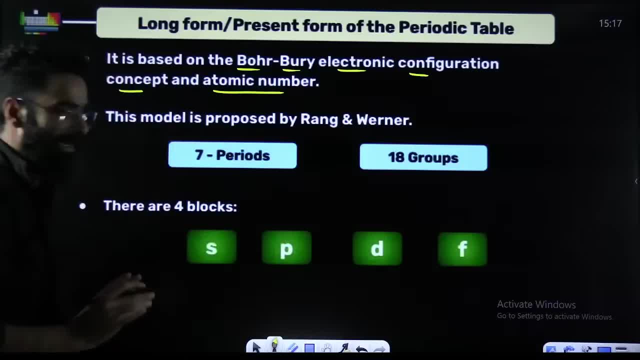 on the Bohr-Burry's electronic configuration concept and as per atomic number. Now the point is this model, this modern period table, this modern period table, it was proposed by Rang and Werner And, as per the modern period table is concerned, it consists of seven periods. 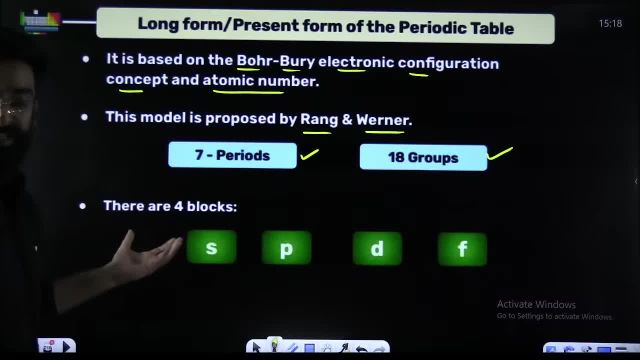 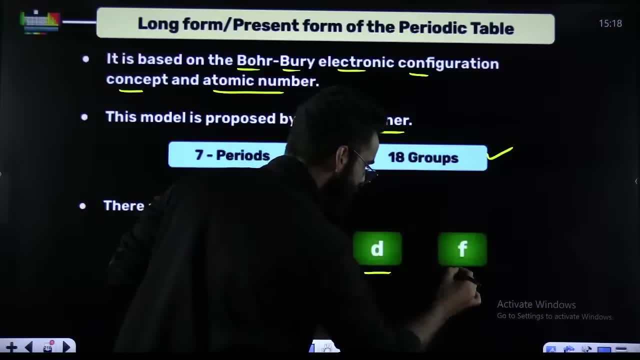 and it consists of 18 periods. So this is the modern period table. So this is the modern period table And we divide this particular, the modern period table, into four blocks, As I told you. one is called as S block, one is P, one is D and one is F. This is the general information. 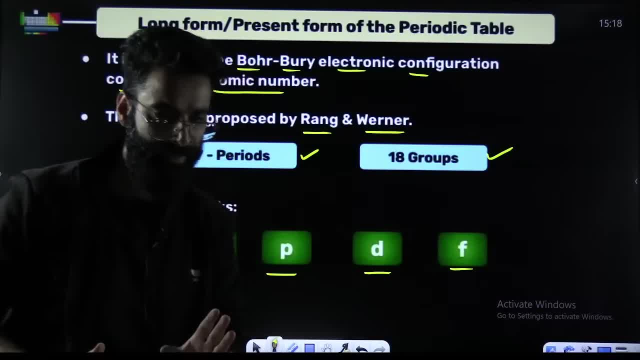 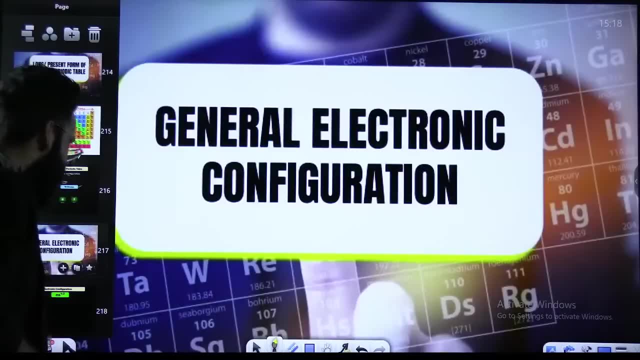 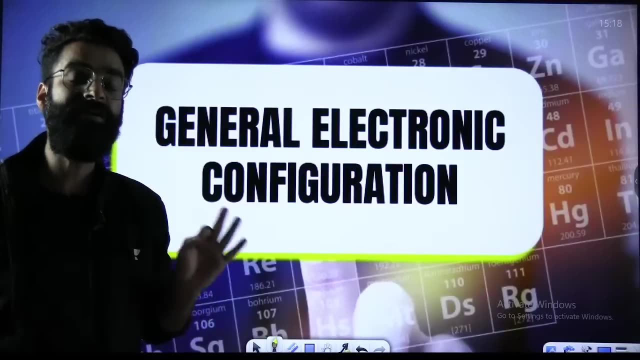 about the modern periodic table. Right, Perfect, This is all factual, which you have to remember. basically Now, what about the general configuration of S block elements, P block elements, B block elements and F block elements? That general electronic configuration you will have to. 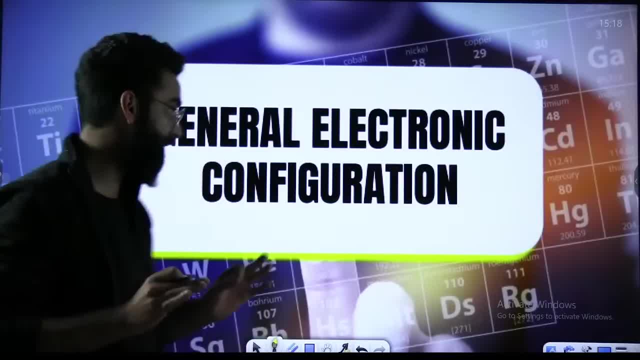 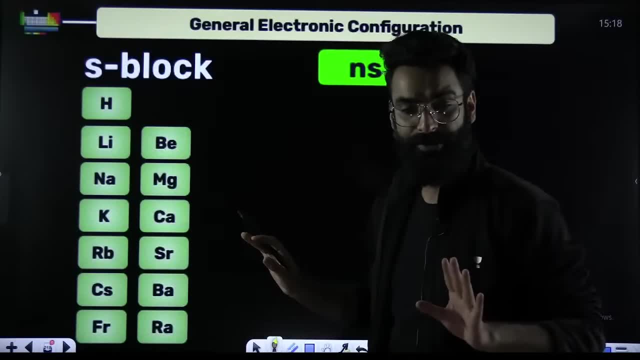 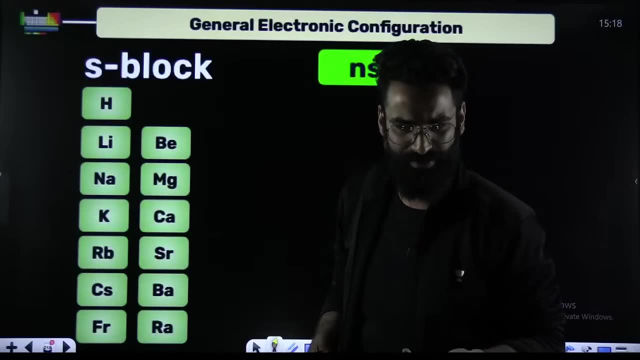 to remember for sure that general electronic configuration you will have to remember for sure. for example, if i talk about s block elements, your group 1 and group 2. they consist of what group 1, group 2 elements? they are what you call us combinedly, your s block elements, right, if you? 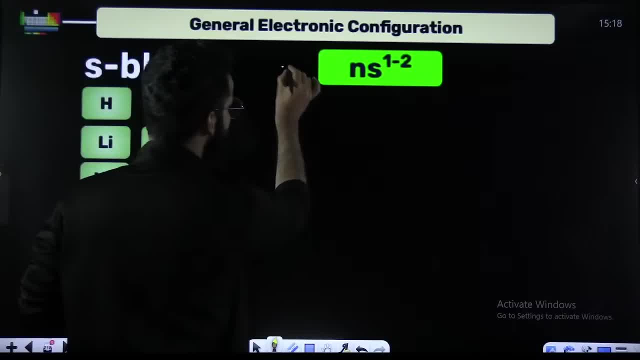 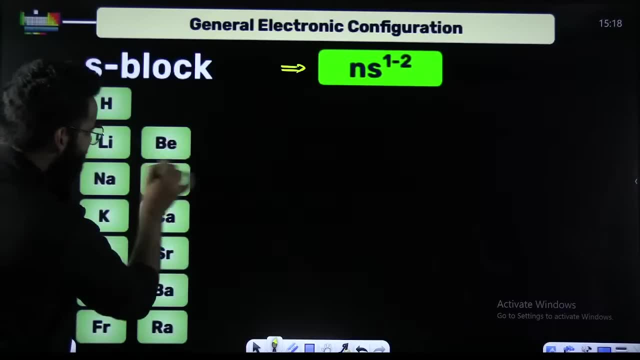 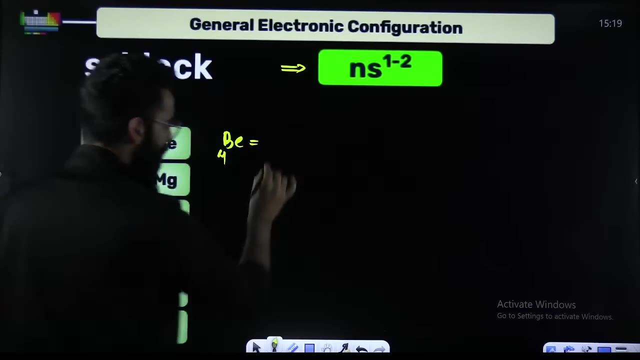 look at their general configuration. their general configuration is ns 1 to 2. ns 1 to 2, for example. take the element, let's say beryllium. right, take the element beryllium. its atomic number is: its atomic number is 4 right now. its configuration is 1s2, 1s2, 2s2, perfect, what is the highest principal? 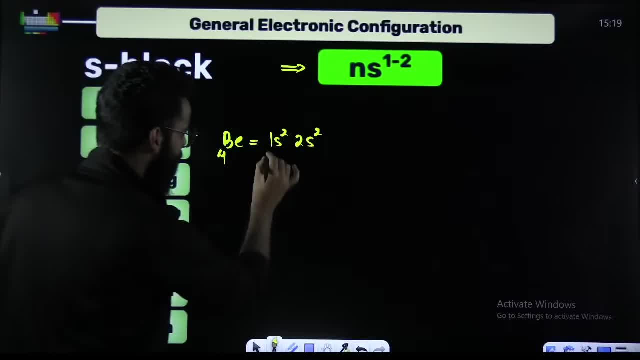 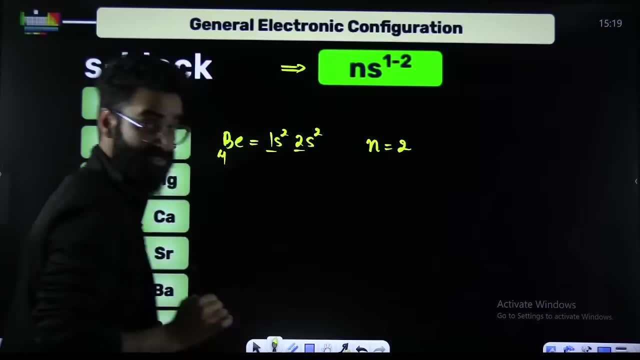 quantum number over here, highest principal quantum number is 2, so n value n stands for highest principal quantum number. it's 2, it is 2.. if you look at its outermost configuration, outermost configuration it is 2 and n is n minus 1.. so here it is. this is the n value. 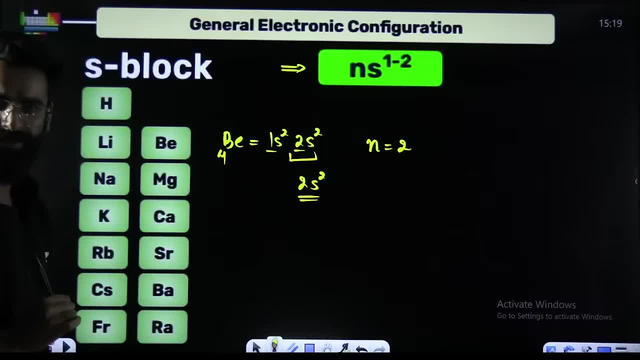 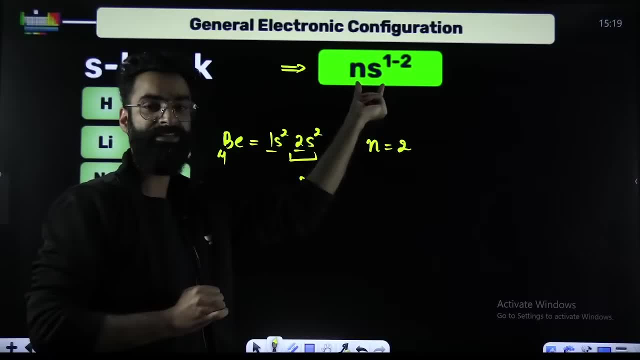 2s2.. It is 2s2.. Perfect Is 2s2. satisfying this n value is 2.. s can be 1 or 2.. 2s2 is satisfying this Perfect. So your beryllium, it is what It is: an s block element, If you. 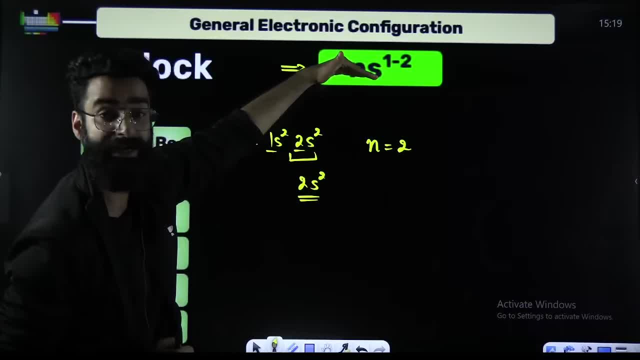 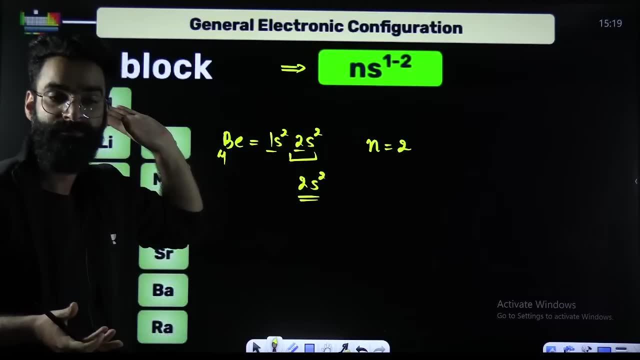 know the general electronic configuration. if you know the general electronic configuration of a particular block, you can identify whether the element is from that block or not, The way I did. For example, you have got, let's say, let's say you have got magnesium, Let's. 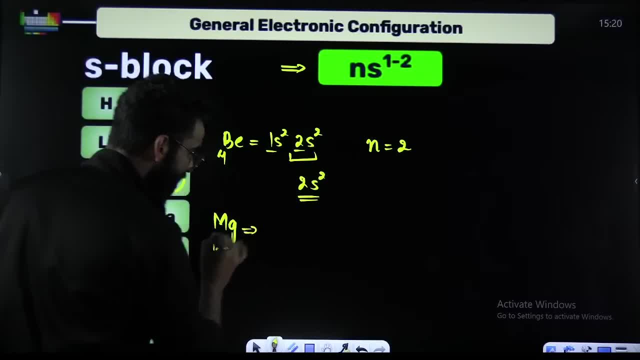 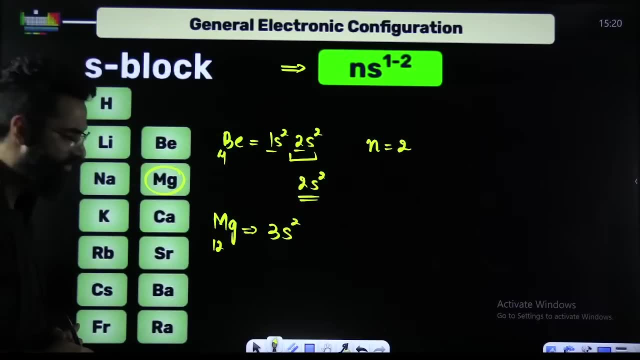 say you have got magnesium, Its atomic number is 12.. Its atomic number is 12.. If you write its outermost configuration, its outermost configuration is 3s2.. Its outermost configuration is 3s2.. The maximum principal quantum number here is 3.. Right, The maximum principal quantum. 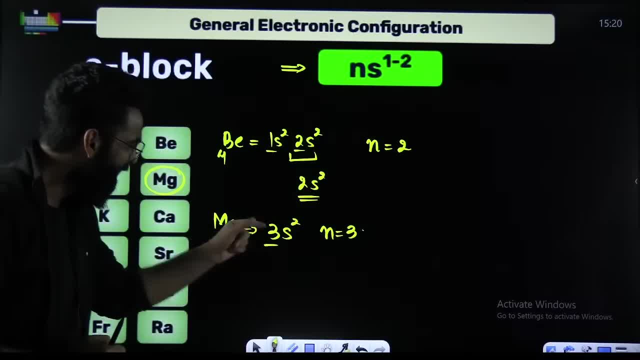 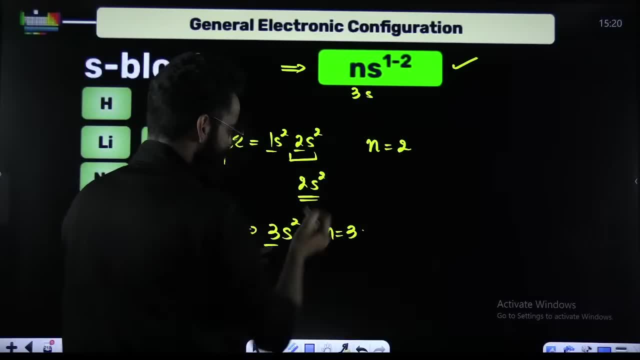 number here is 3. Right Check Is this: is this 3s2 satisfying our general configuration? ns1 to 2? n value, if you put as 3s2. s can be 1 to 2. And here s is 2. Right. So this is your s block element, Perfect Right. 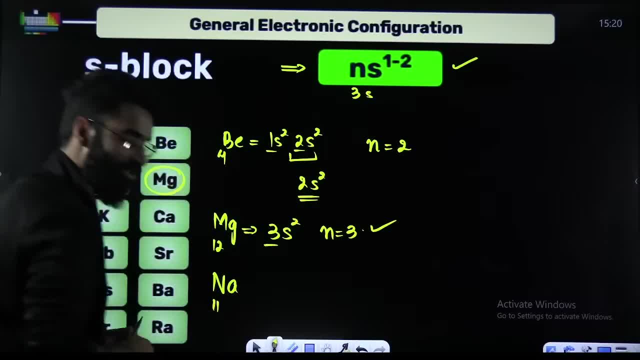 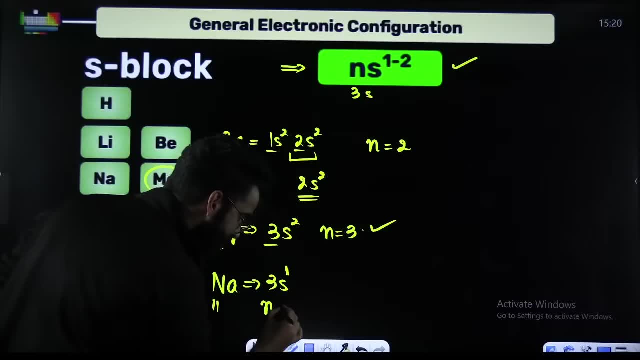 For example, talk about sodium. Talk about sodium. Its atomic number is how much? 11.. Its atomic number is 11.. If you write its outermost configuration it is 3s1.. Outer I mean the maximum principal quantum number here is 3.. Check whether this particular configuration. 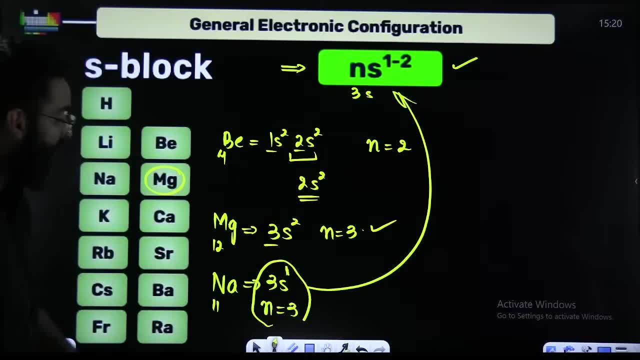 is satisfying our general configuration or not. It is satisfying. n value is 3.. s can be 1 or 2.. And here I am writing s1.. s can be 1 or 2.. And here I am writing s1.. s can. 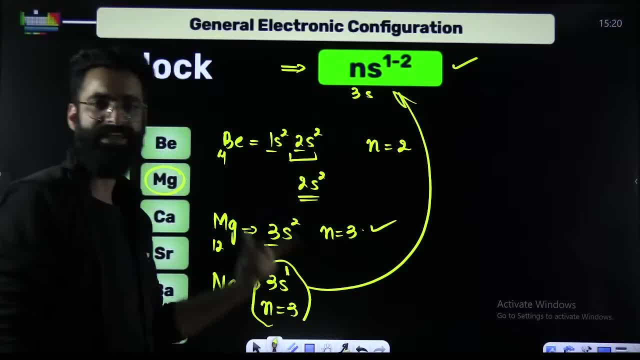 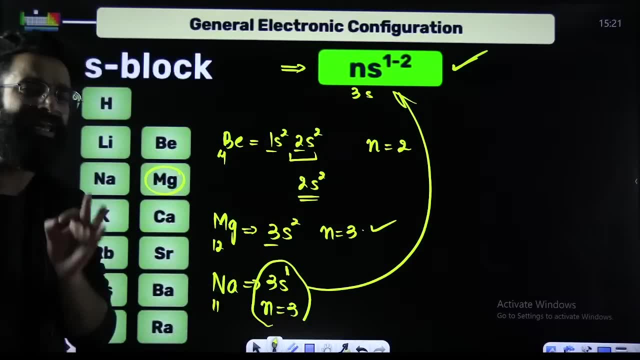 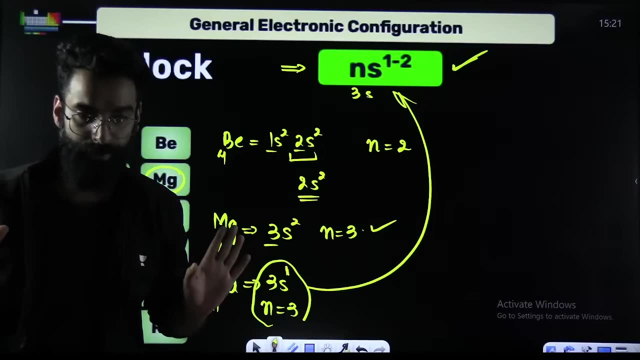 be 1 or 2.. Perfect Right, So this is your what, This is your s block element. So, my dear students, what is something which I want you guys to remember here? The general configuration of s block elements from now onwards is going to be ns1 to 2.. That's all Okay, ns1 to 2.. 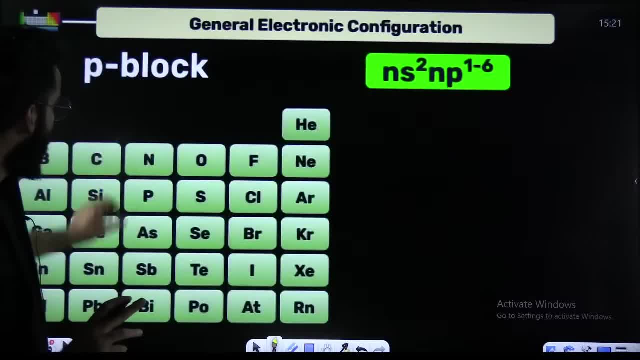 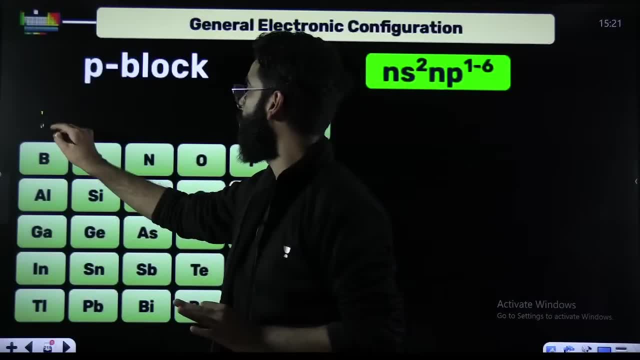 This is something which I want you guys to remember, Number 1. If I talk about p block elements, in case of the p block elements, in case of the p block elements, these are all your P block elements, from your group 13 to group 18.. These are your P block elements. 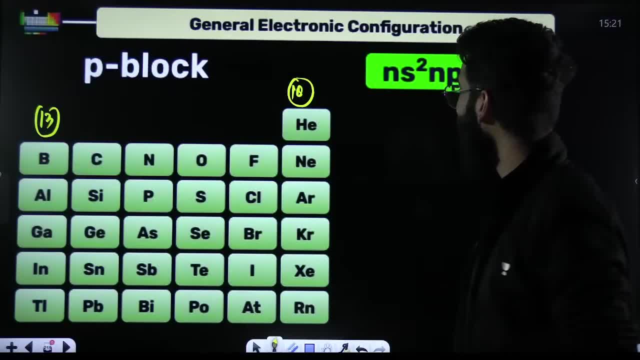 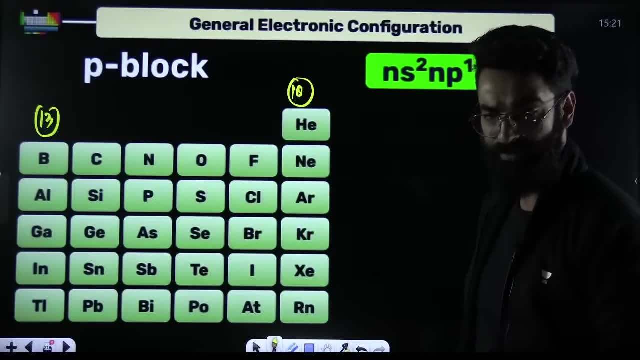 Ideas: students, in case of your P block elements, the general configuration is what? NS2, NP1 to 6.. You can check it: NS2, NP1 to 6.. NS2, NP1 to 6.. Take any element, For example. 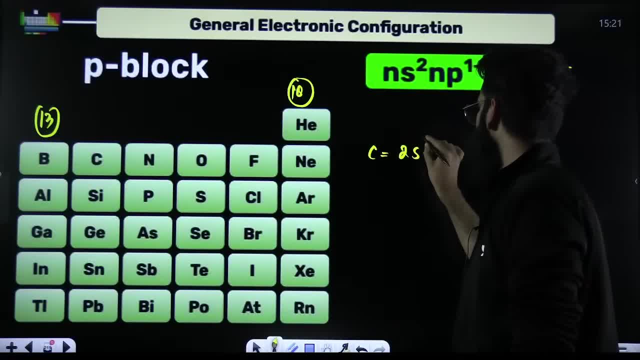 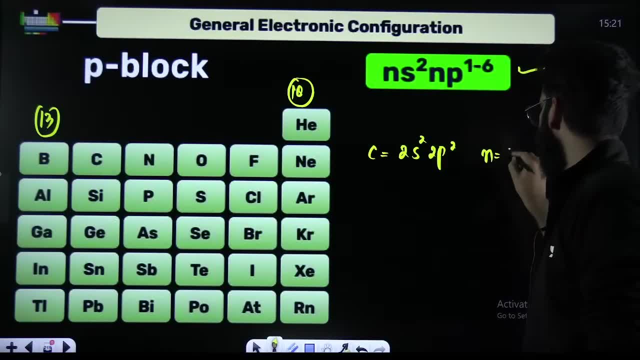 I am taking carbon. If I take carbon right its outermost configuration, 2S2,, 2P2.. What is the maximum principal quantum number here? Maximum principal quantum number N is equal to 2.. N is equal to 2.. Put this value of N over here. So 2S2,, 2P1 to 6.. It can be 1,, it can be 2,. 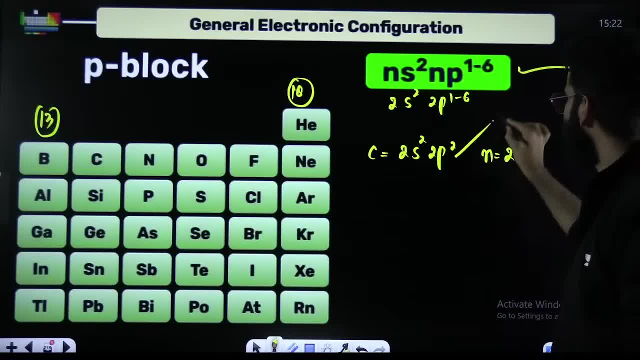 it can be 3,, it can be 4,, it can be 5 or it can be 6.. So this is satisfying it, Perfect, This is satisfying it. For example, if I take, let's say, chlorine. If I take chlorine, its outermost. 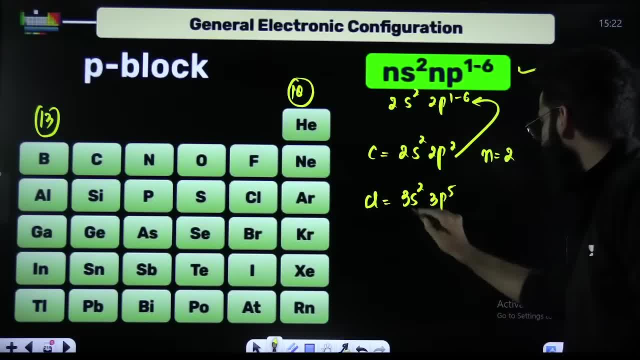 configuration is 3S2 and 3P5, right. What is the maximum principal quantum number here? It is 3.. Put the value of N3 in the general General configuration. it becomes what It becomes. 3S2 and 3P can be 1 to 6.. It is containing 5,. 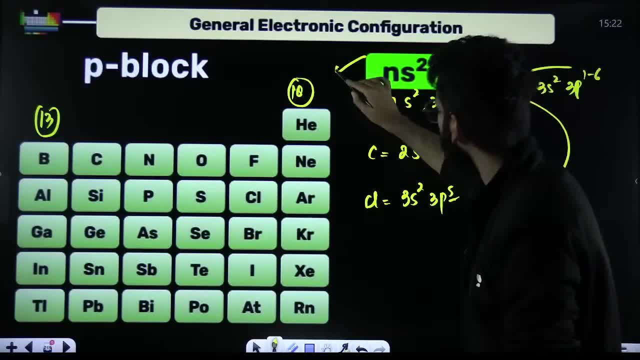 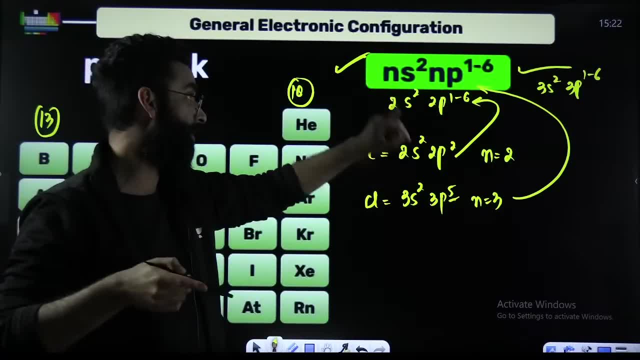 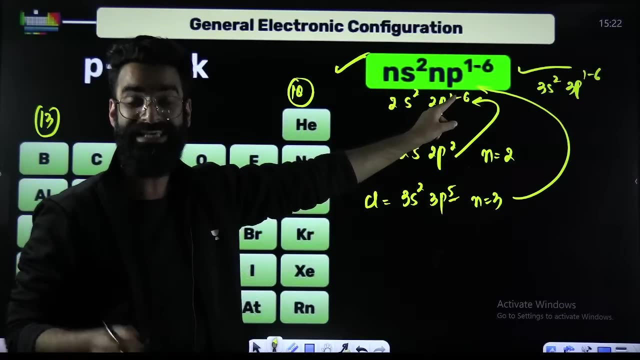 it can be 1 to 6.. So it is satisfying it. So, basically, this is your general outermost configuration of your P block elements, which you have to remember. It is what was S block: NS1 to 2.. P block is NS2, NP1 to 6.. NS2, NP1 to 6.. NS2, NP1 to 6.. These can be direct questions. 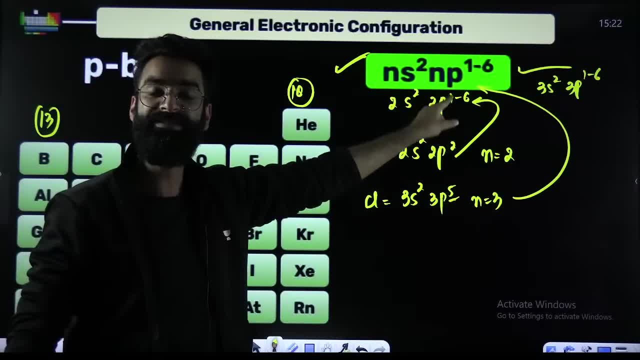 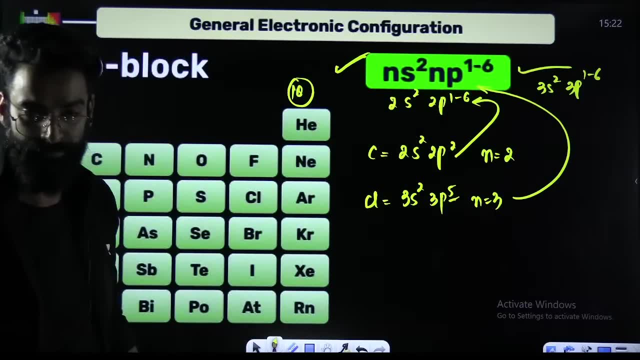 asked What is the general configuration of S block, P block, D block, F block, S block NS1 to 2.. P block NS2, NP1 to 6. P will contain 1 to 6 electrons right. Similarly, if I talk about D block. 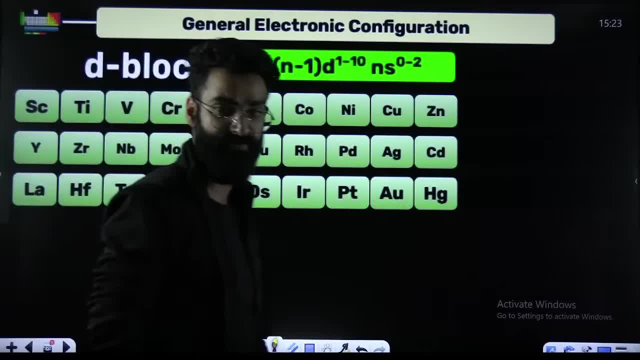 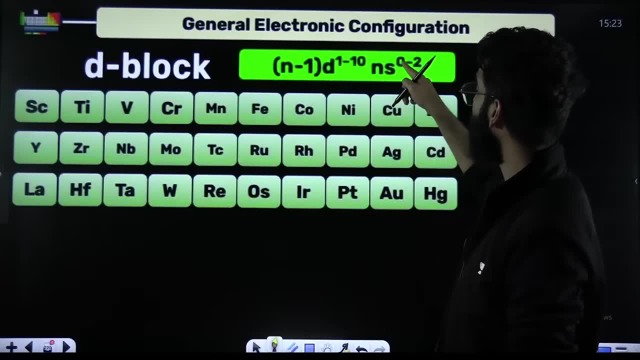 elements. if I talk about D block elements, the general outermost configuration of the D block elements is N minus 1, D1 to 10 and NS can be 0 to 2.. NS can be 0 to 2.. For example, take any. 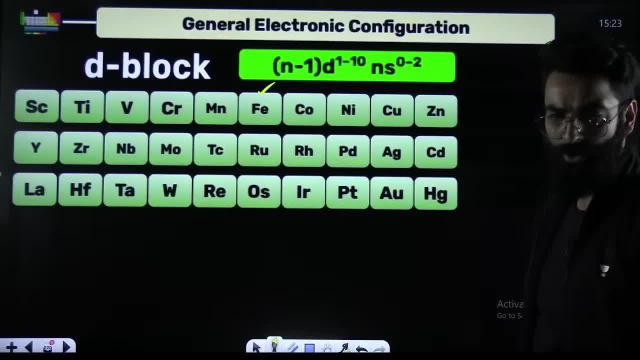 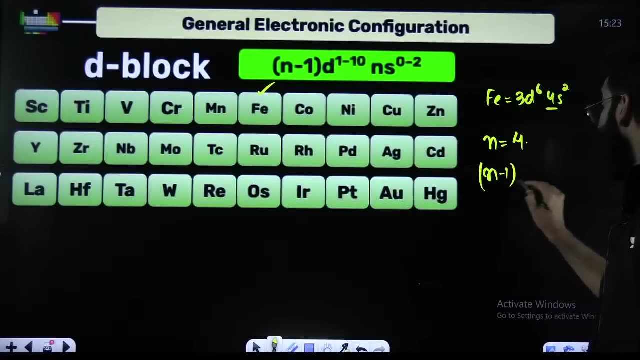 element. Take iron, Take iron. You know the outermost configuration of iron: 3D6, 4S2.. This is the outermost configuration of iron. What is the highest principal quantum number here? Highest principal quantum number is 4.. If N is equal to 4, that means N minus 1 has. 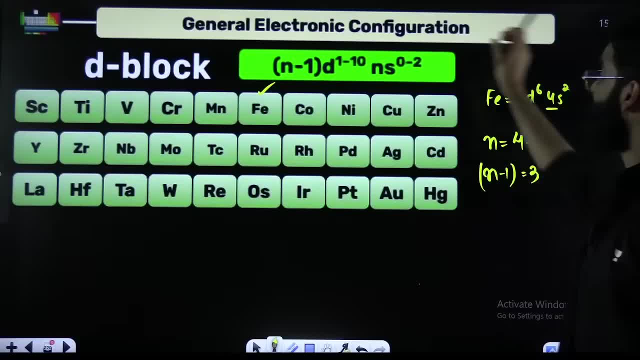 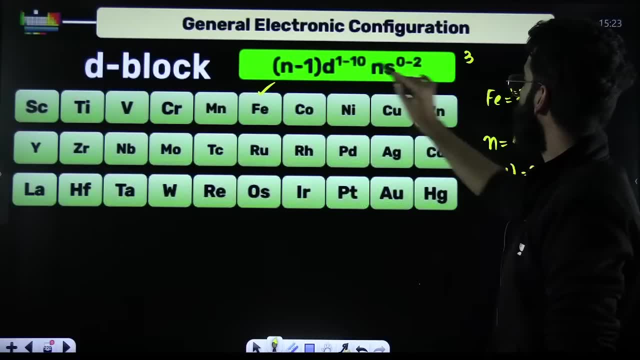 to be: N minus 1 will be 3.. Check whether it is satisfying this or not. Put N is equal to 4.. Put N is equal to 4 in this equation. So 4 minus 1 is 3, right, So 3D. it can contain electrons from. 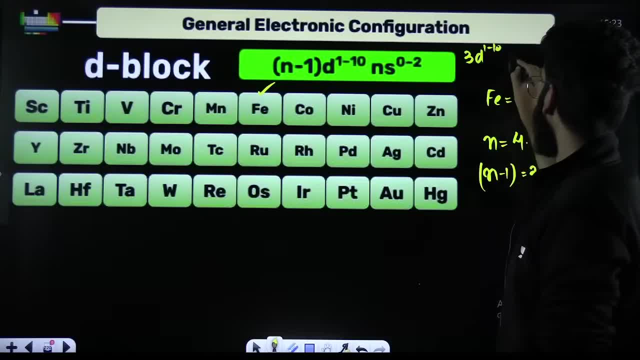 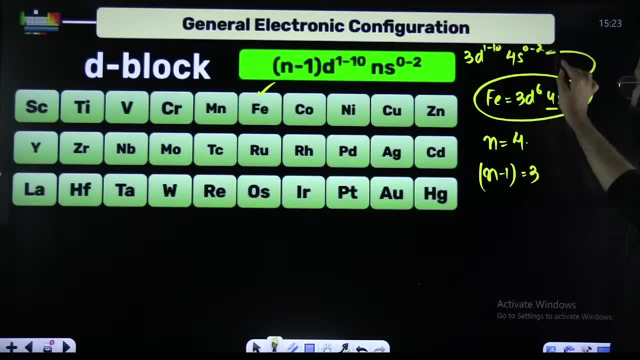 1 to 10.. Anything between 1 to 10. N value is 4.. N value is 4.. NS can have the electrons from 0 to 2, right? Is this configuration satisfying the general? Check it out This particular configuration. it is satisfying the general. 3D is containing: 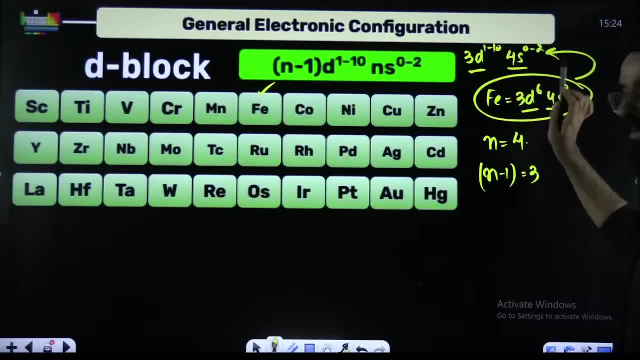 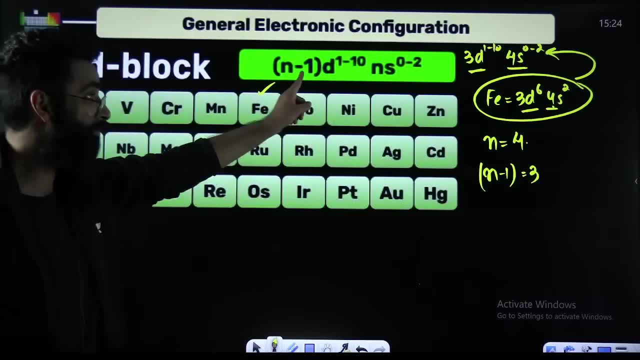 6. Valid 4S is containing 2. Valid right. So this is basically your D block element, basically right. So, in short, what I want to convey over here, remember the general configuration. that is very important: N minus 1, D1 to 10, NS 0 to 2, okay. 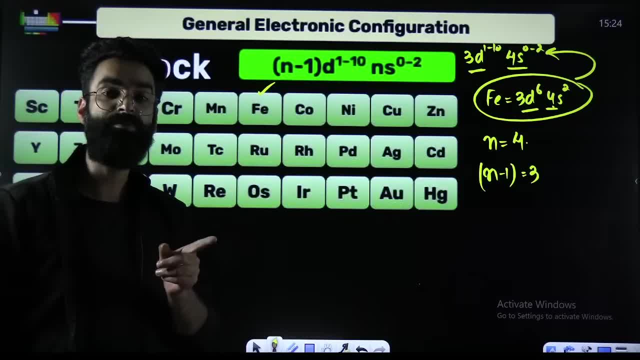 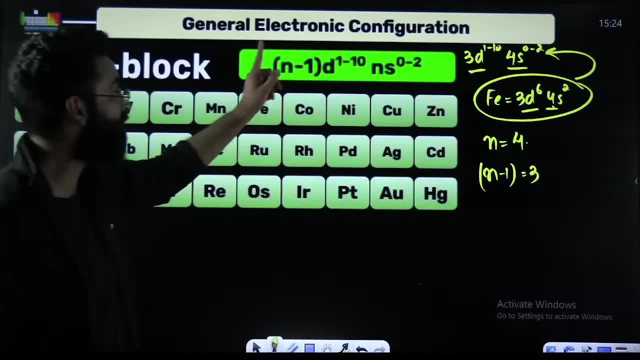 So say it with me. For S block it was NS2.. For P block, quickly in the charts NS2, NP 1 to 6.. For D block elements, the general configuration is N minus 1, D1 to 10, N minus 1, D1 to 10,. 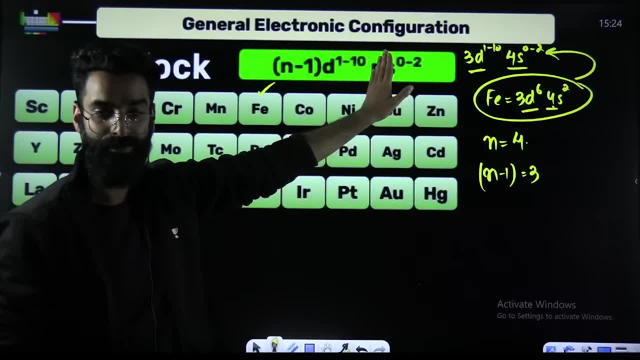 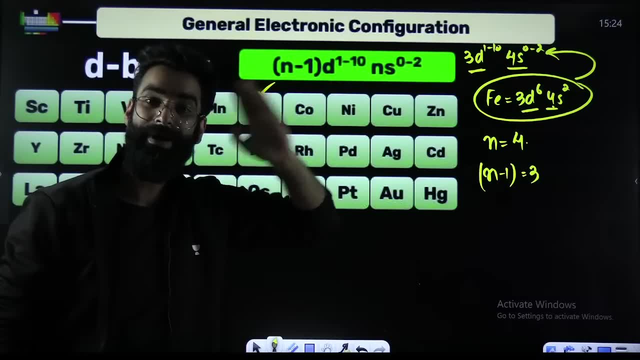 NS2.. I mean NS0 to 2, right Perfect N minus 1, D1 to 10, NS0 to 2.. Where N is the maximum principal quantum number. Highest principal quantum number. Highest principal quantum number. 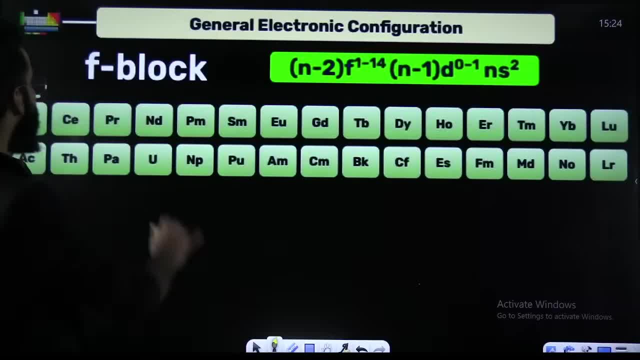 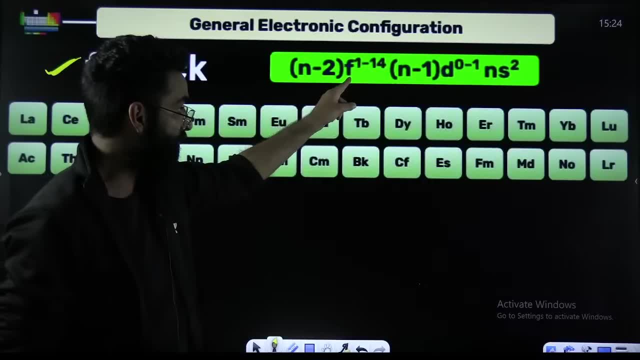 right. Same goes for what Same. Remember the general outermost configuration of F block elements as well. right: N minus 2, F from 1 to 14.. N minus 1, D: 0 to 1, NS2.. Perfect, This is. 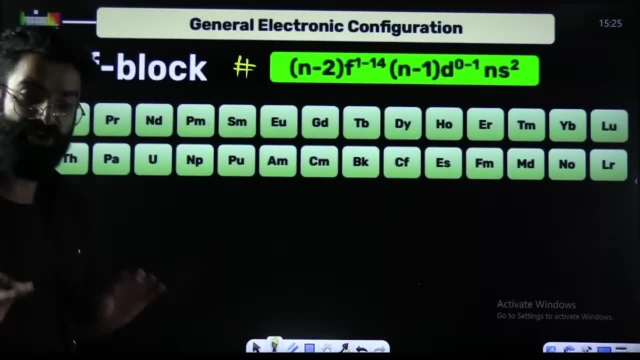 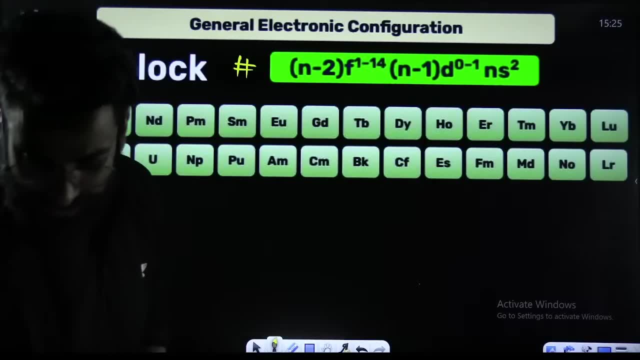 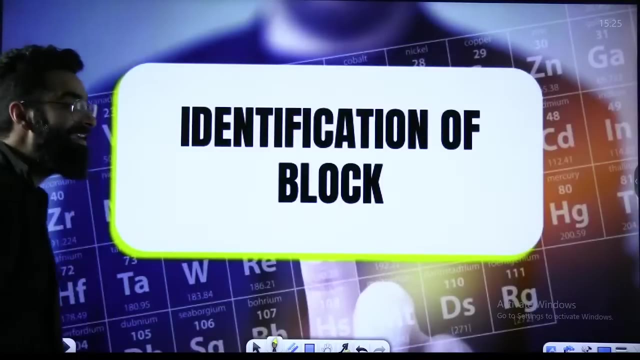 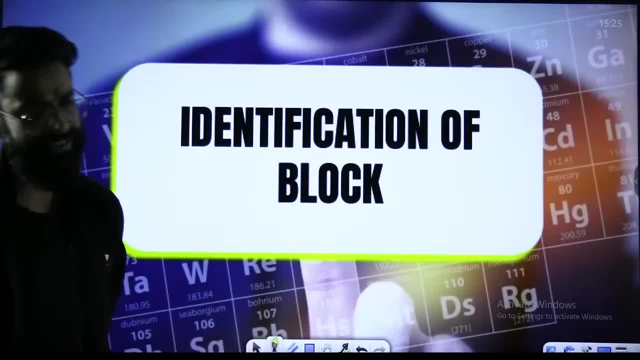 identify whether the element is from S block, whether the element is from P block, D block, F block, whatever right Identification of the block. How do we do that? First of all? first of all, if you look at this particular slide, 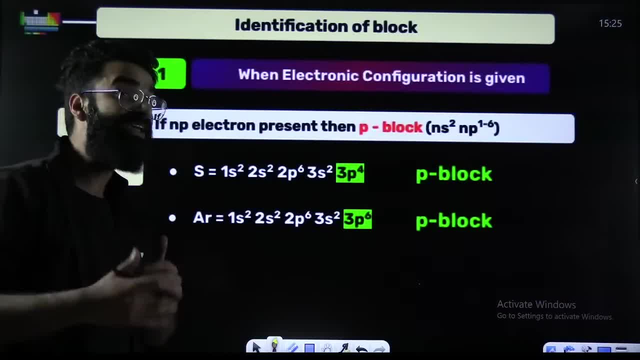 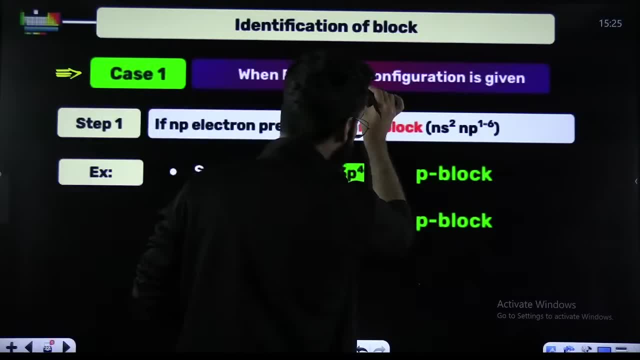 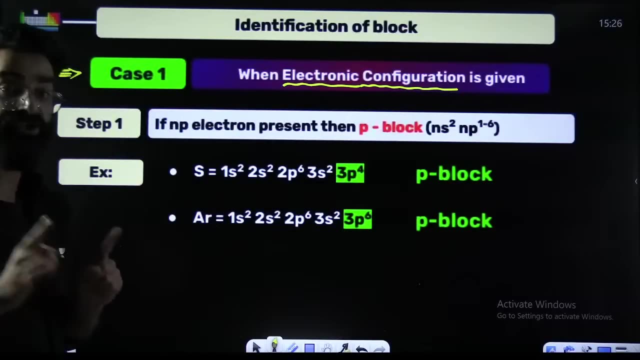 if you look at this particular slide: Identification of the block. My dear students, I will start with case 1.. If, in a question, you are given with the electronic configuration of an element, if you are given with the electronic configuration of an element, okay. If you are given with 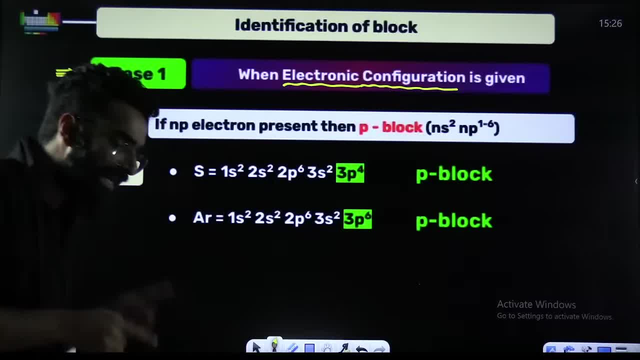 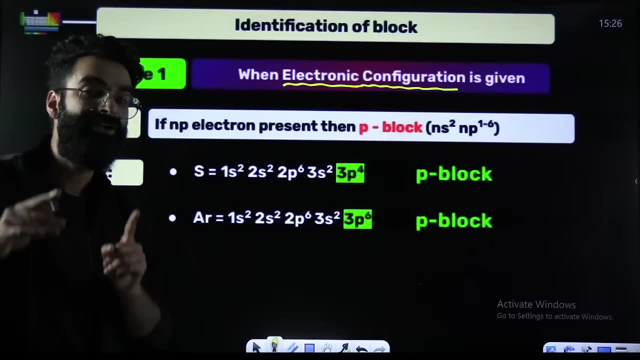 the electronic configuration of an element and from the electronic configuration you have to identify element belongs to element. belongs to Element belongs to which block? Okay, How do we do that? How do we do that? For that purpose, you need to remember the general outermost configuration of all the blocks. 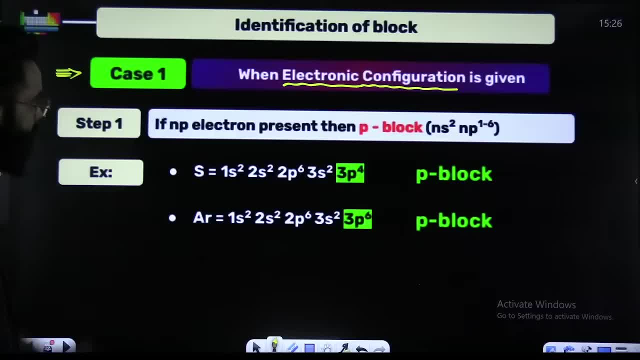 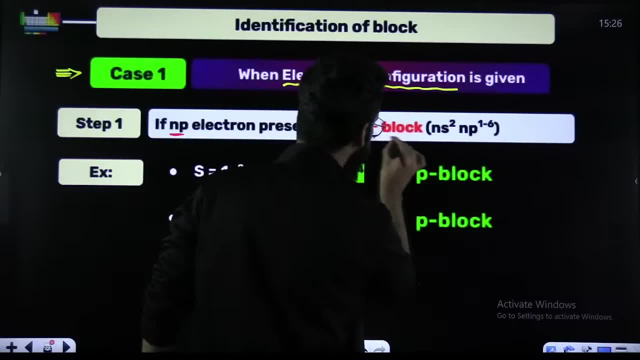 first. For example, for example, for example, have a look. I have mentioned over here: if NP electron is present, then P block. What is meant by this? What is meant by this? For example, my dear students, look at this particular element. This is sulfur. Understand carefully. 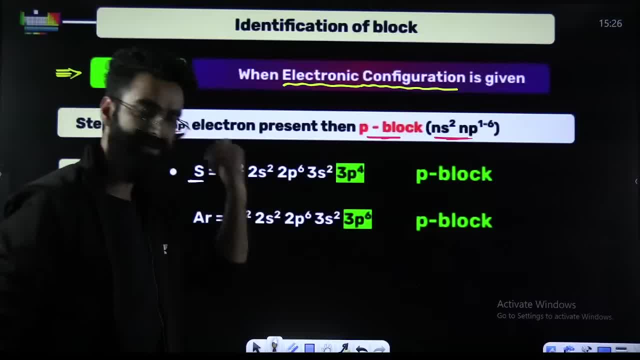 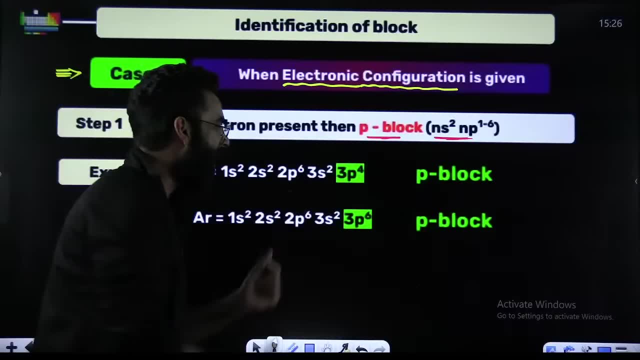 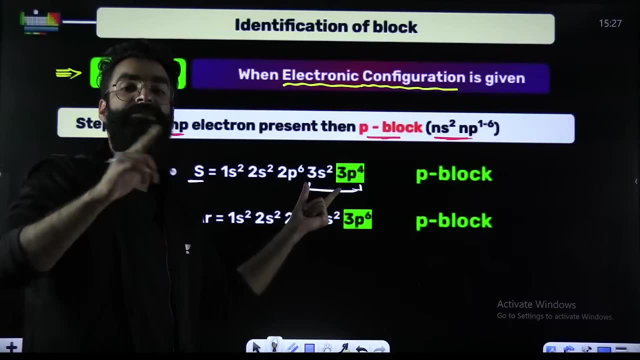 This is sulfur, right. You wrote its configuration. You wrote its configuration right. You wrote its configuration. Now check whether the outermost configuration is resembling, whether the outermost configuration is satisfying the general configuration of S, P, D or F. Check it out. Check it out. 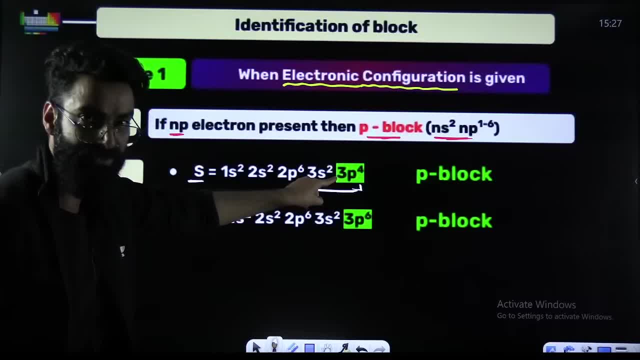 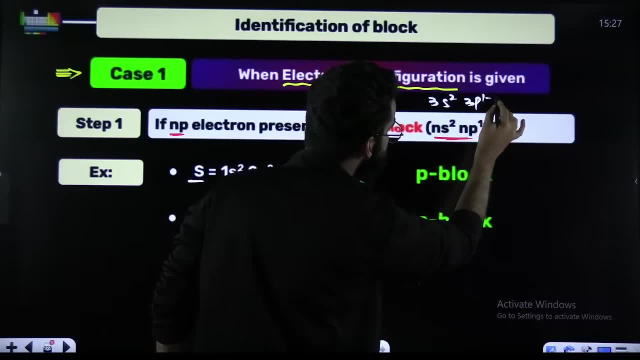 Highest principal quantum number is 3.. Highest principal quantum number is 3.. Perfect, So highest principal quantum number is 3.. So if I put 3 here, it is 3s2 and it can be 3p126.. 3p will be. 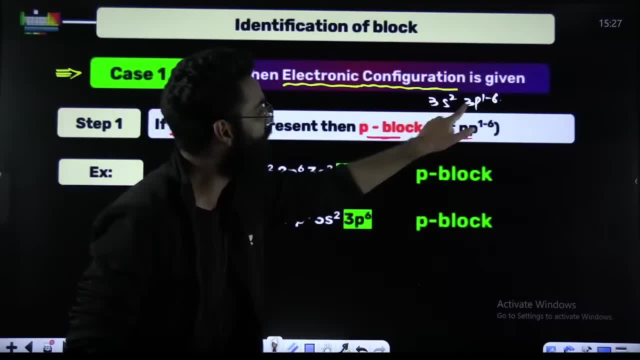 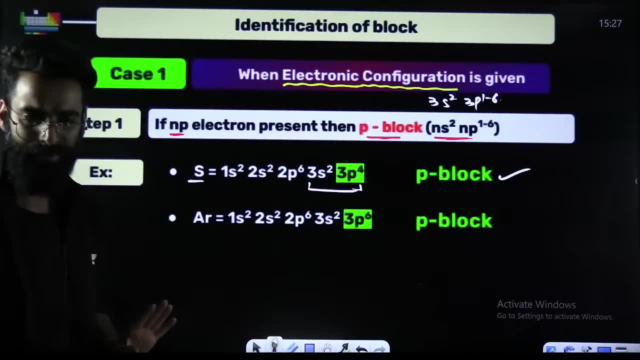 1 to 6.. So 3s2 and 3p4, which is present here, It can be 3p126.. So directly you will say it is a P block element. Directly you will say it is a P block element. What you? 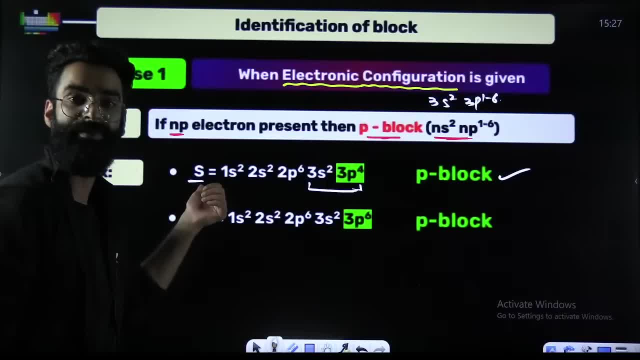 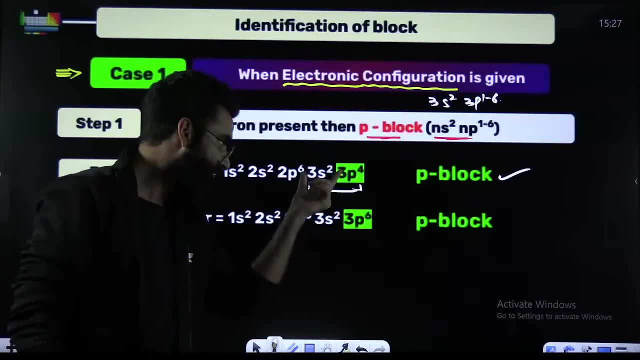 need to do. For example, if you have got a question wherein you are given an element, sulfur, you have written the. I mean the electronic configuration of sulfur is given Perfect. If the outermost configuration of sulfur is satisfying this particular condition, then 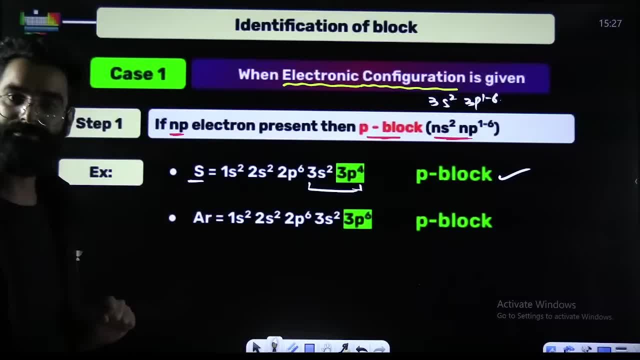 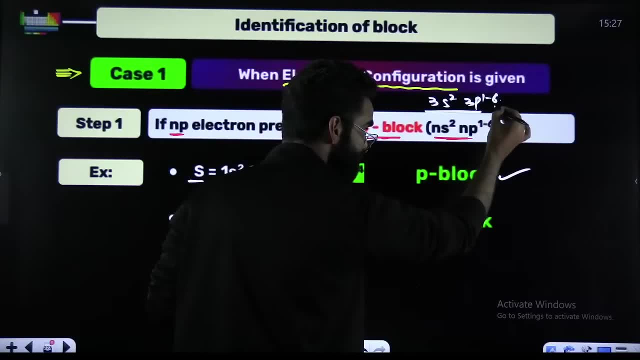 it is a P block element. As simple as that. look at the second one. look at the second one again: 3s2, 3p6. if you put ns3, 3s2, 3p6, 3s2, 3p6 is present here. that means directly: you can say it's a p block element. 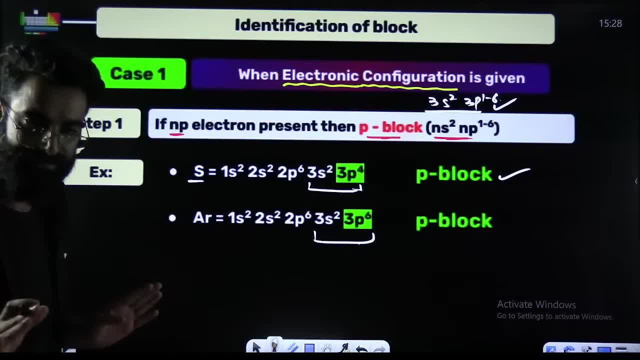 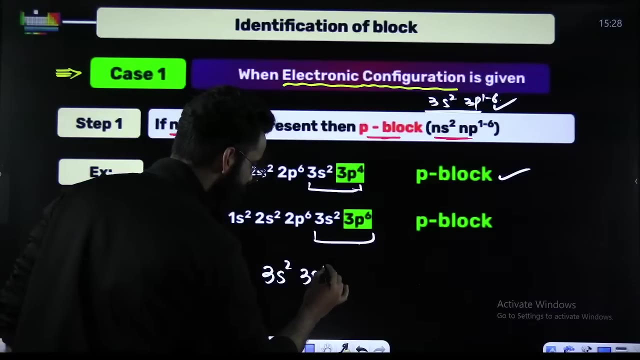 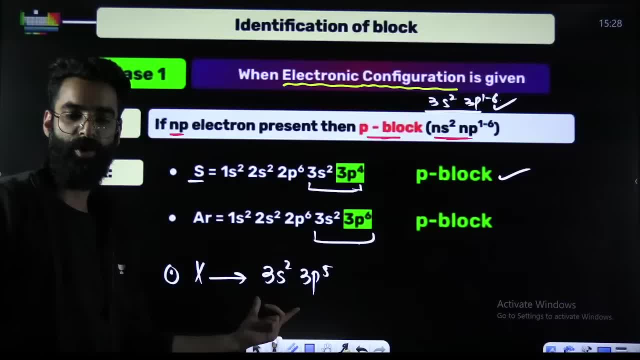 can you let me know what is going to be the block of this element quickly, guys? i want you guys to let me know in the chats quick. it's a p block element. it's a p block element because this particular outermost configuration it is satisfying our general configuration. 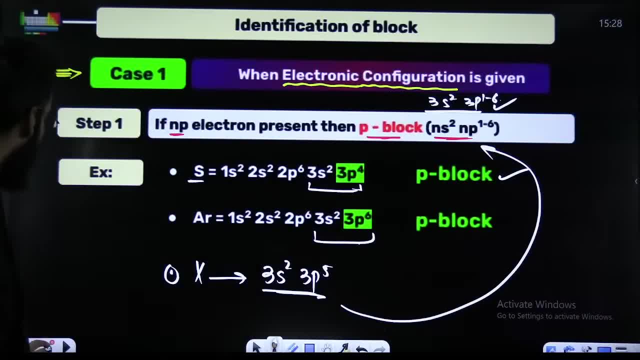 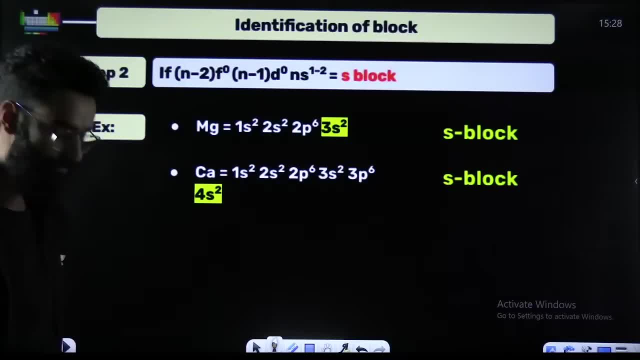 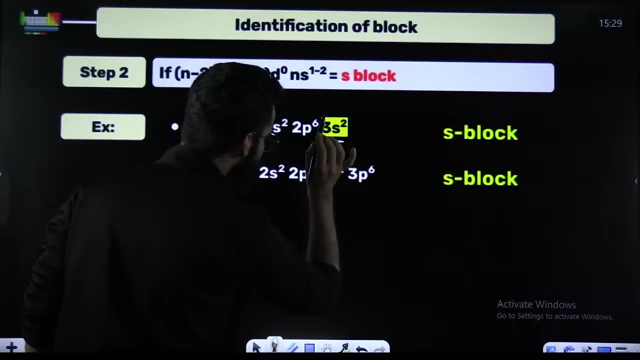 you, you right, it's satisfying our general configuration. i hope step number one is clear, right. step number two. step number two, my dear students, i have mentioned over here two elements. i mentioned over here, two elements, perfect, two elements i mentioned over here. outermost configuration is 3s2. here, electronic configuration is given. 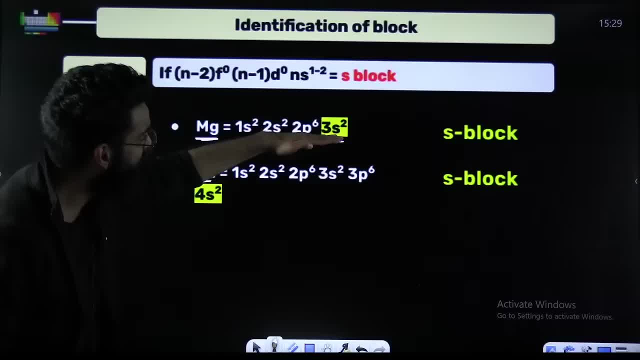 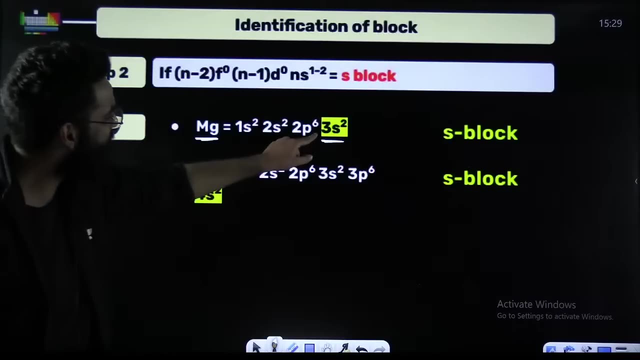 electronic configuration is given. now check whether this. now check whether this electronic configuration, whether this outermost configuration, is satisfying our general configuration or not. check it out, check it out, check down highest principal contour on this tree. so 3s, 1 to 2 vs 1to 2, ps 1 to 2, you can but right. 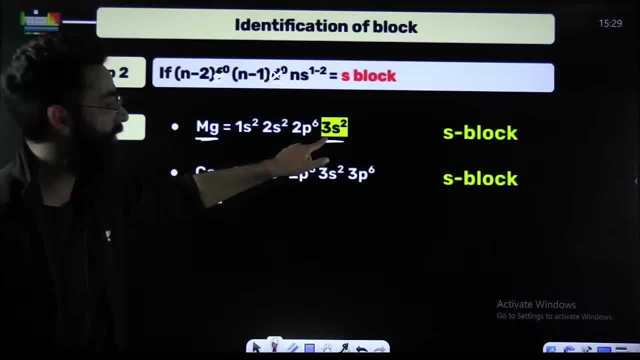 this is the, this is the zero, this is f0- right, leave it aside, perfect. and values 3 and values 3. so it is set, spraying this non-terminal configuration. this is standard configuration and by restaurant us, ie for me this It is satisfying, this Perfect, It is satisfying, this Correct, It is satisfying. 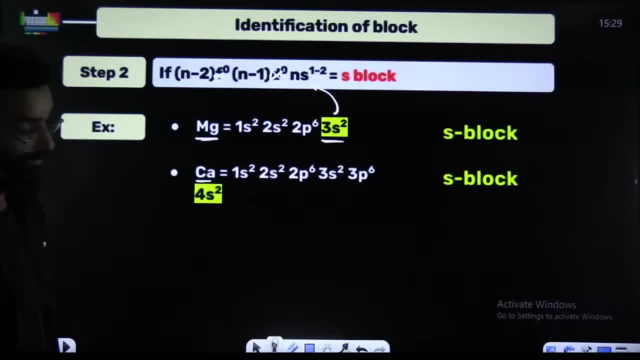 this. So it belongs to which. It belongs to which block. It belongs to S block. It belongs to S block. Look at the next configuration. Next configuration is here: 3s2, 3p6, 4s2.. 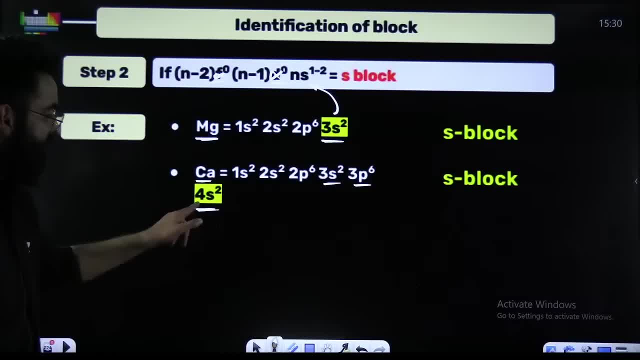 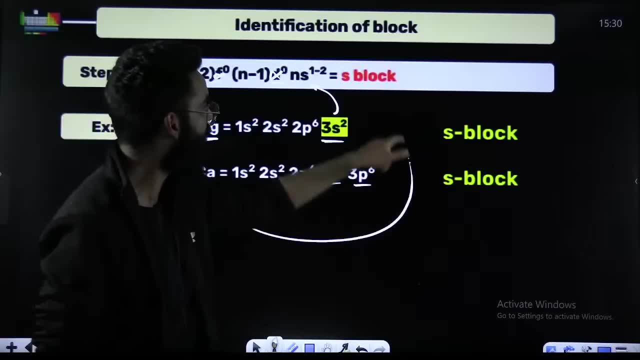 3s2,, 3p6, 4s2.. Look at this configuration: 4s2.. Put n value as 4.. Put n value as 4.. 4s1 and 4s2.. This is also satisfying it. If it is satisfying, if the configuration which 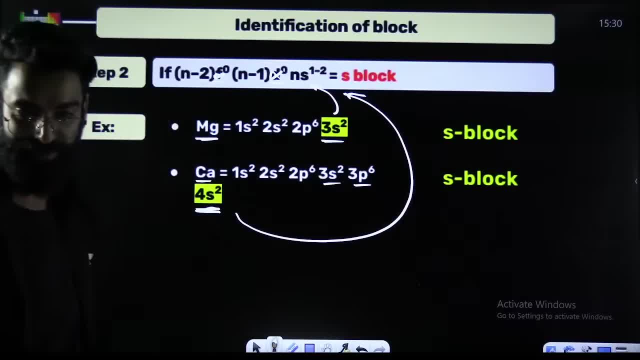 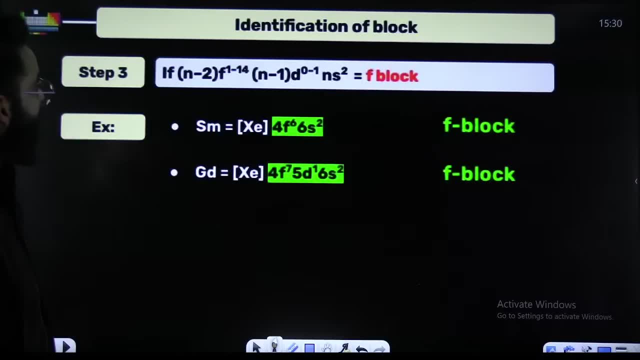 is given to us, if it is satisfying this particular configuration, then it is the S block element. As simple as that. As simple as that. As simple as that. Similarly, similarly, this is the general configuration of S block. Now you are given with the element whose electronic 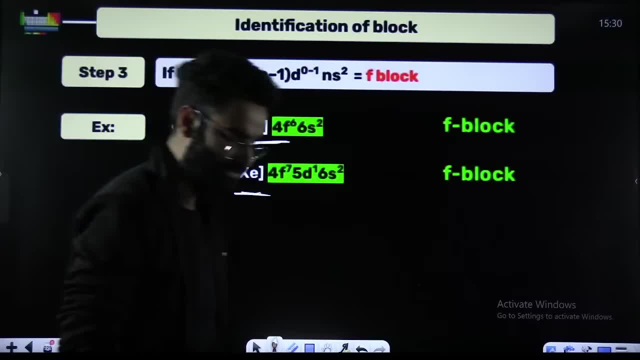 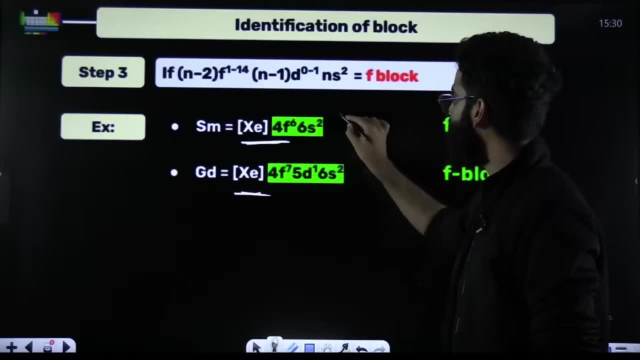 configuration is given Right. These are the two elements which are given to us Right. These are the two electronic configurations which are given to us, Perfect. What is the highest principle? quantum over here. 6.. n value is 6.. n value is 6.. If n is 6, n is: 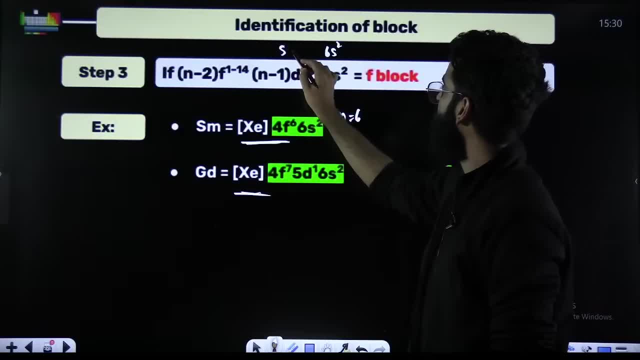 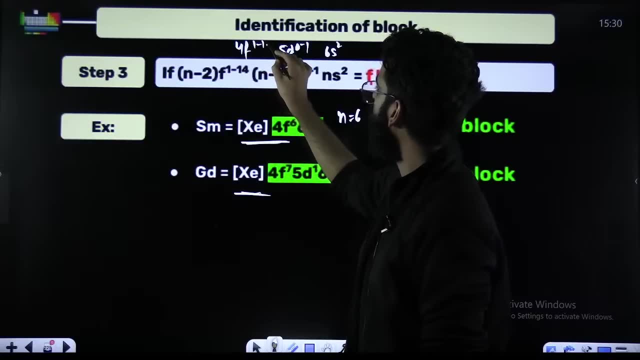 6, it will be 6s2.. 6 minus 1 is 5.. So 5d will contain 0 to 1 electron. Right n is 6.. 6 minus 2 is 4.. So it is going to be 4.. f can contain 1 to 14 electrons. Look at this particular. 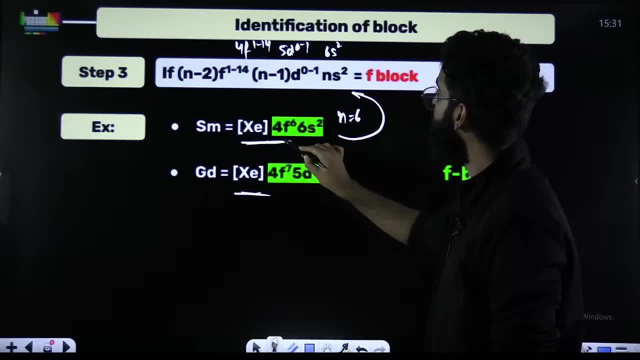 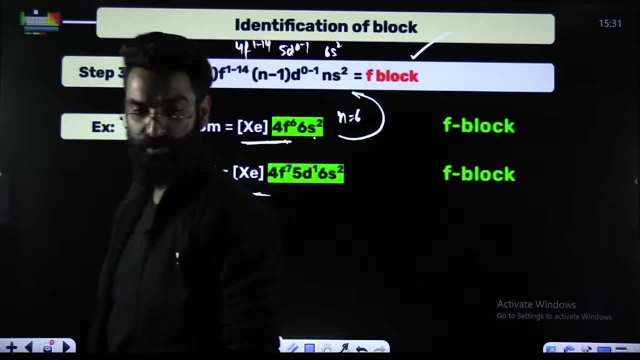 configuration. It is satisfying this particular configuration: 4f6.. 4f6.. 6s2.. 6s2.. It is satisfying it. So this particular element which is given to us, whose electronic configuration is given to us, it is basically your f block element. 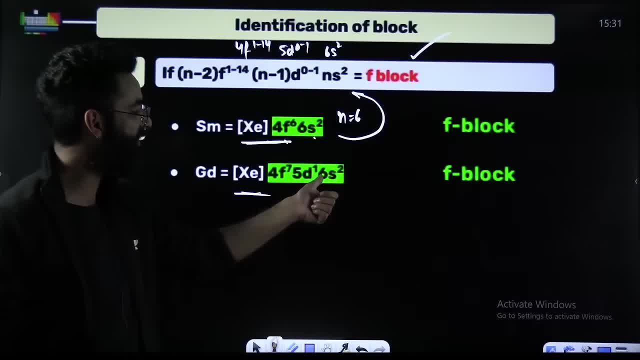 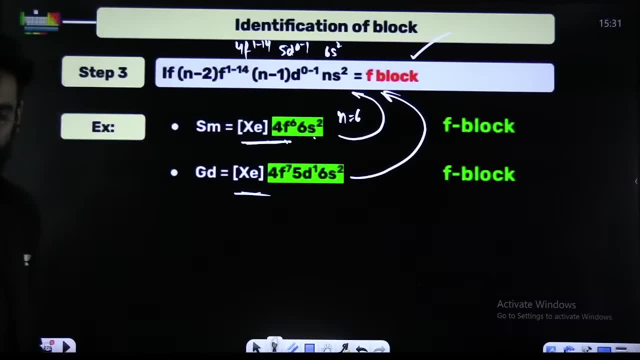 Look at the next one. Look at the next one. What is the highest principle? quantum over 6? here Again, if you see, when you put 6 here, right, it will say it is 5.. It will say it is 5.. So, basically the point is, that is why I told you you have to remember the. 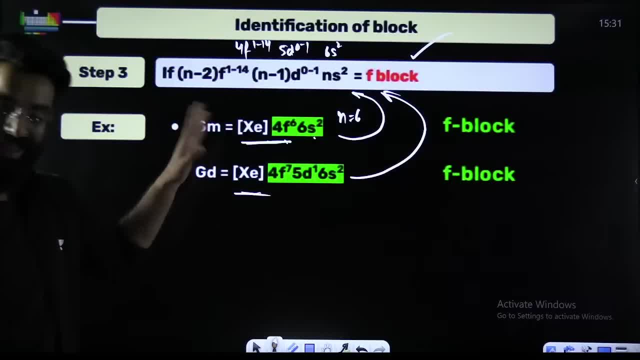 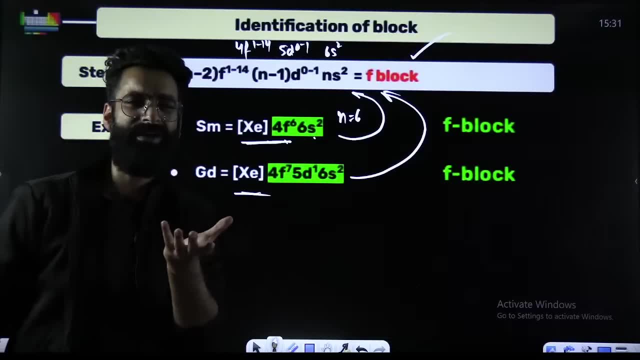 general outermost configurations, Right, And if you remember the general outermost configuration? if the question is asked like this, You are given with some electronic configuration And you have to check whether the element is s block, p block, d block or f block. You have to check whether the given configuration. 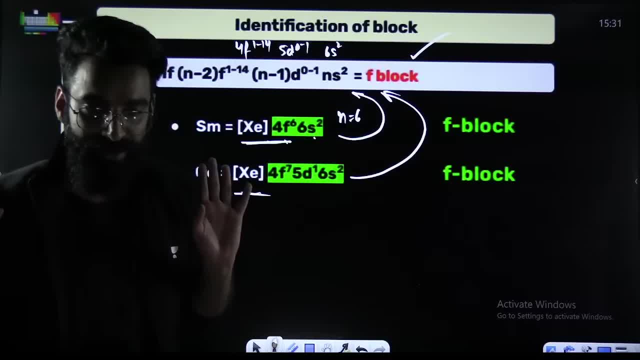 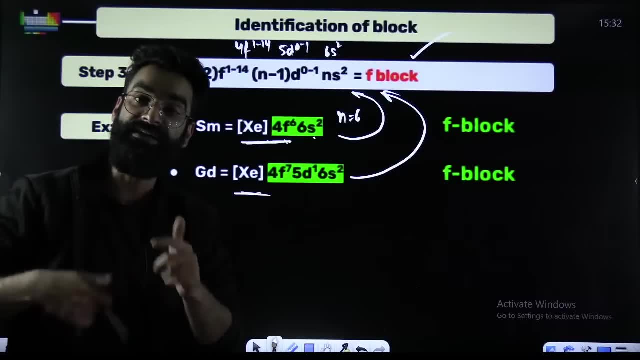 is satisfying our general configuration or not. If it is satisfying the s block configuration, it is s block element. If it is satisfying the p block configuration, then it is p block. If it is satisfying the d block configuration, then d And eventually f. This was case number. 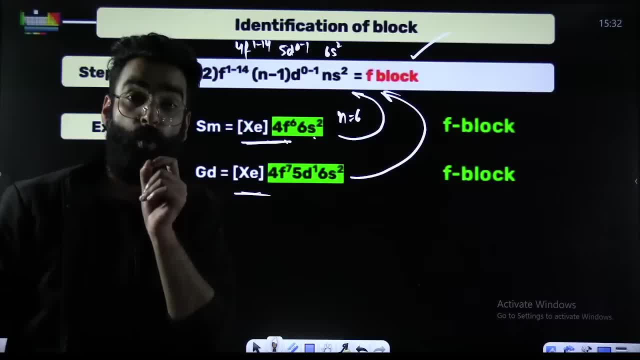 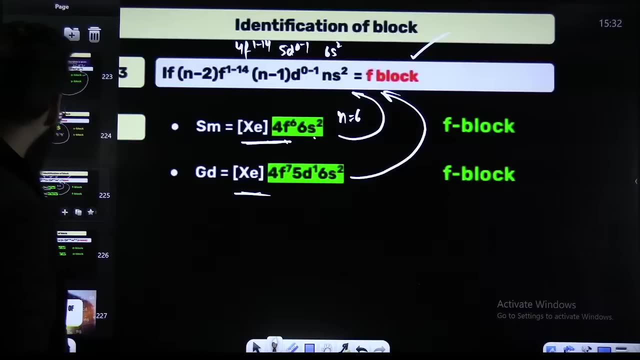 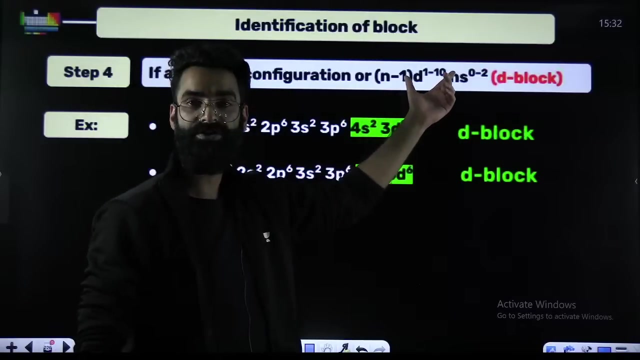 1. That is, identification of the block When, When electronic configuration of an element is given. Identification of the block when the electronic configuration is given. Correct Identification of the block. Identification of the block when the general electronic configuration is given. Similarly, this is your d block configuration. 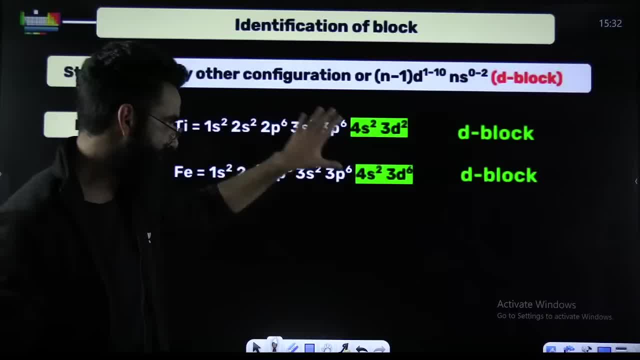 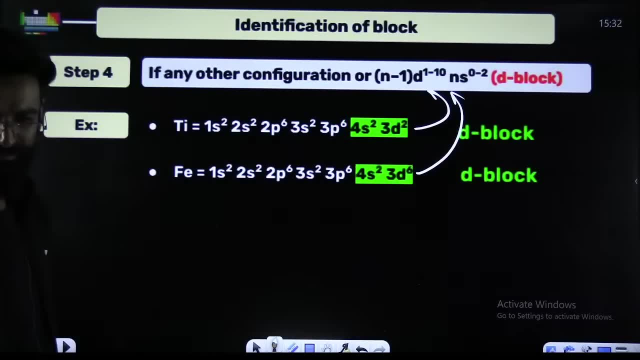 If you are given with a question, electronic configuration is given. If this electronic configuration is satisfying the general one, then the given element is your d block element, which is pretty much simple now. I believe. I believe this is pretty much simple now. 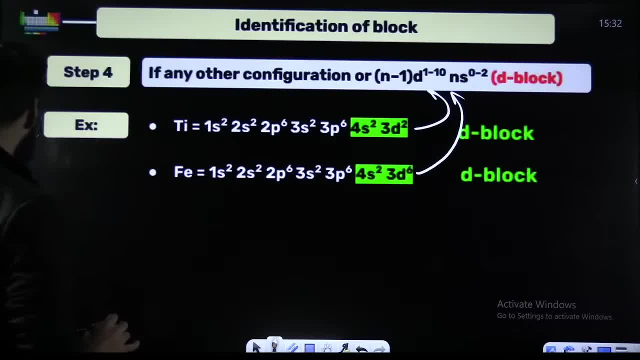 So question number 1.. Question number 1.. What was this question? What was this question? Question was identification. You can write it in your notes in the form of questions: Identification of the block, If electronic configuration of an element is given to us. 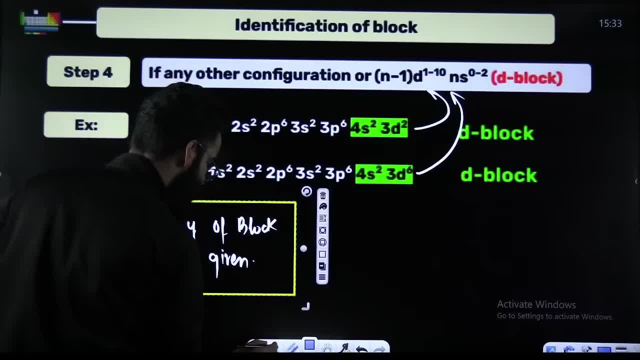 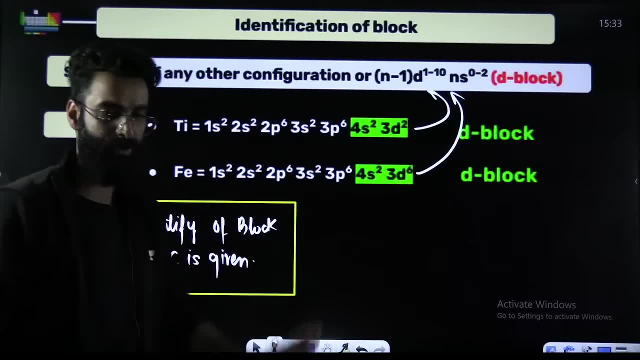 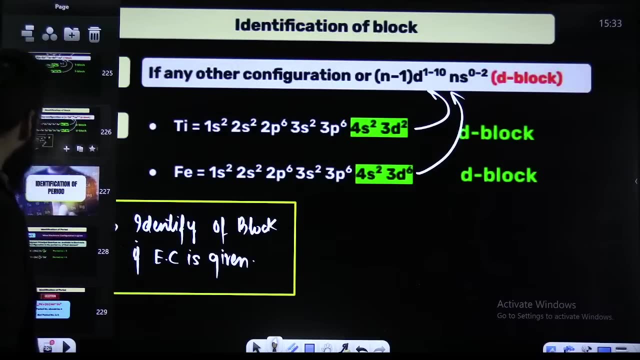 How do we do that? For that purpose, first of all, we have to remember the general outermost configuration. If the given configuration is satisfying whatever block configuration, accordingly you can solve it. Yes, Perfect, Number 1.. Number 2. That is identification of the period, Identification. 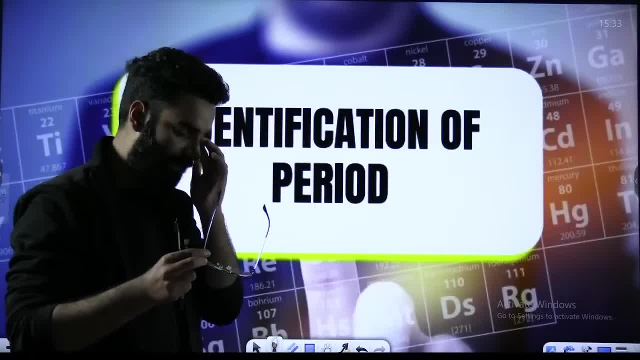 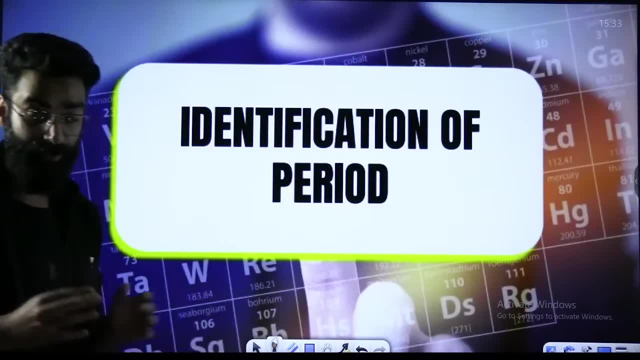 of the period. How do we exactly identify Whether the element is from period number 1, period 2, period 3,, period 7 or whatever? Right, There are 7 periods in total. How do we check? How do we check The period number 1,, period 2, period 3,, period 7 or whatever? 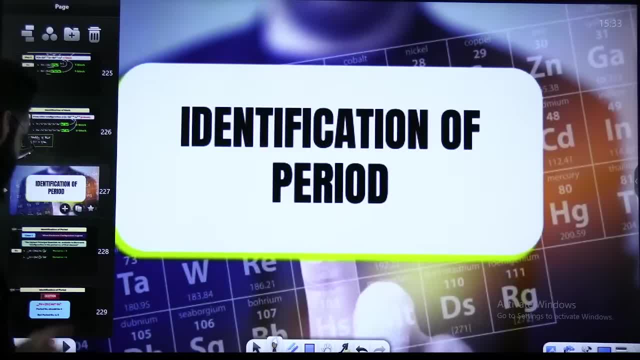 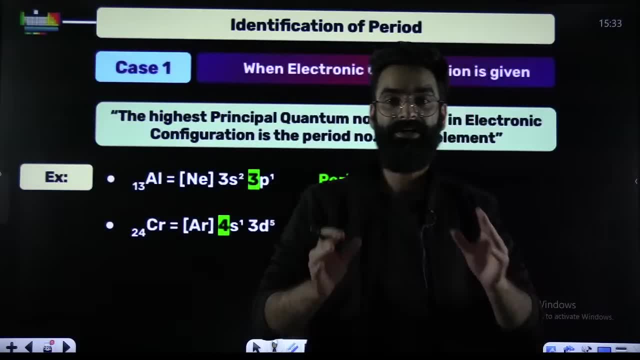 Right, There are 7 periods in total. How do we check? How do we check The period number of an element? Again, case number 1.. Again, case number 1.. If, If, If You are given with an element and its electronic configuration, Imagine you are given with element X, Its. 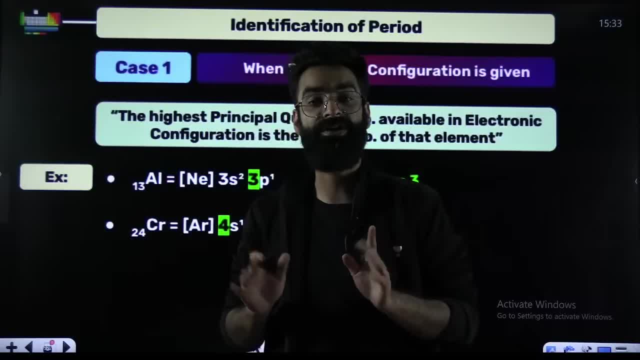 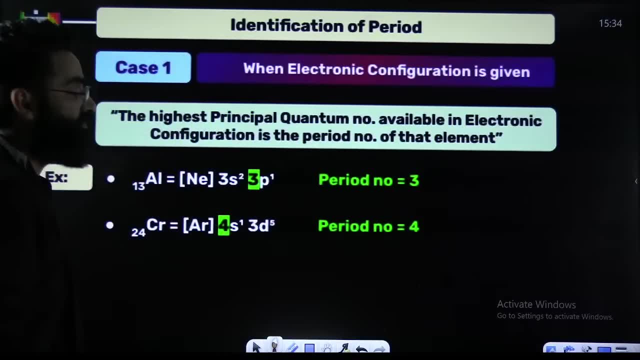 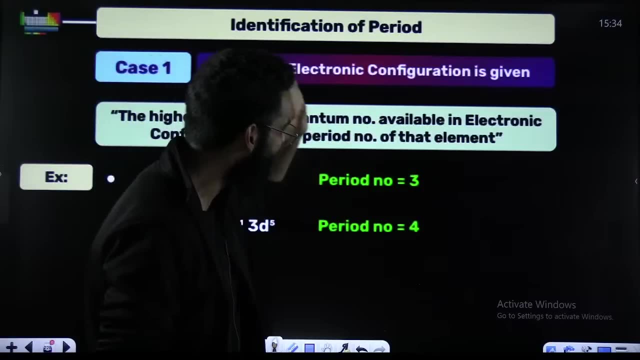 electronic configuration is given. From the electronic configuration, How do you check? how do you check which period element belongs to? How do you check which period element belongs to? Look at this particular statement here. Obviously, this particular statement, statement here, guys, The highest principal quantum number available in the electronic configuration. 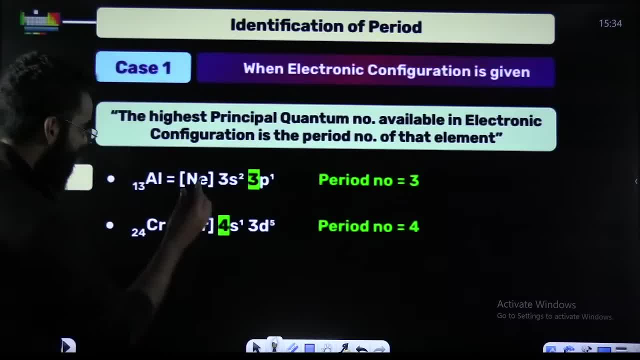 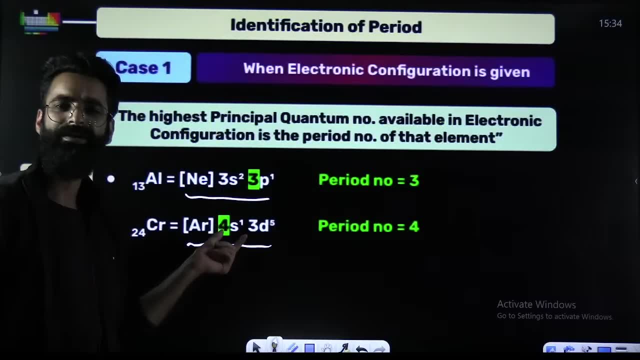 is always the period number of that element. For example, I am given two configurations like this. I am given two configurations like this: Perfect. Two electronic configurations have been given to me. I am asked to check the period of these two elements. How do I do it? I will check the highest. 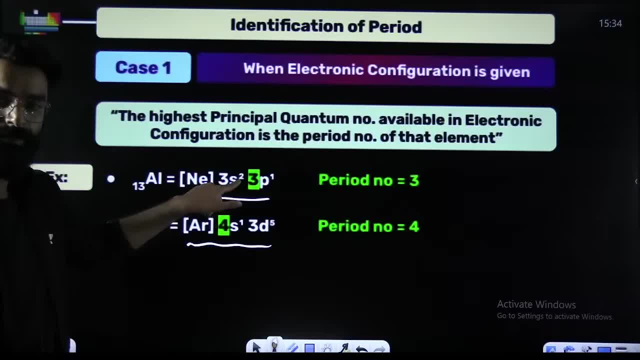 principal quantum number. What is the highest principal quantum number here? 3, right, So directly, I will say its period number is 3.. What is the highest principal quantum number? 3 or 4? 4. I will say its period number is 4.. So, in short, if electronic configuration is given. 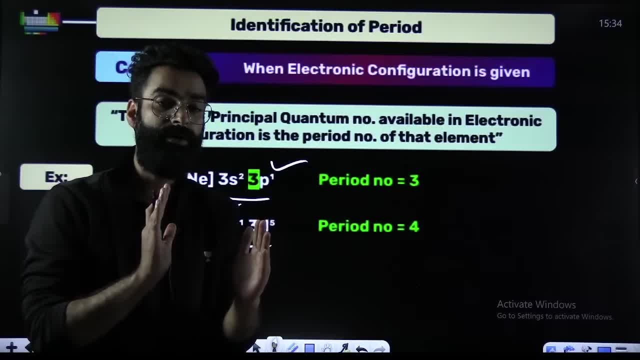 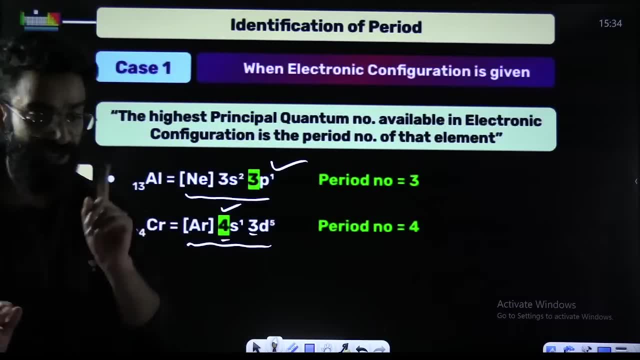 if electronic configuration is given, check the highest principal quantum number. Whatever is the highest principal quantum number, that is going to be your period number. That is going to be your period number. Okay, That is going to be your period number. Point number 1.. Point: 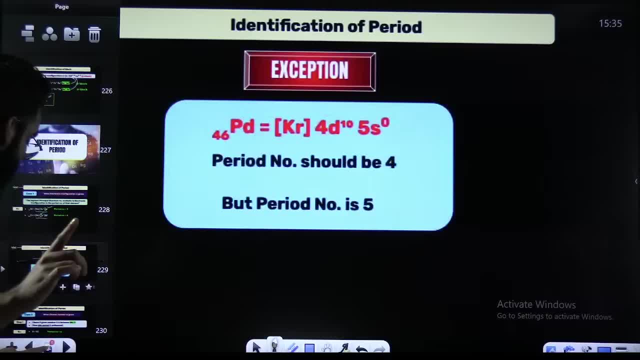 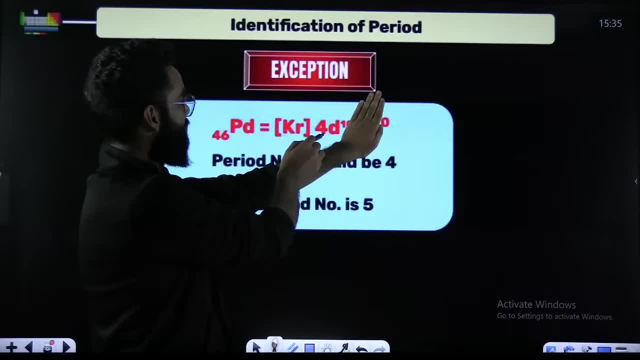 number 2.. Okay, Here we have got one exception for palladium. Do remember this one. Okay, Just leave this 5 as 0.. If I ask you, look at this configuration, Look at this configuration. If I ask you, from this configuration, what has to be its period, 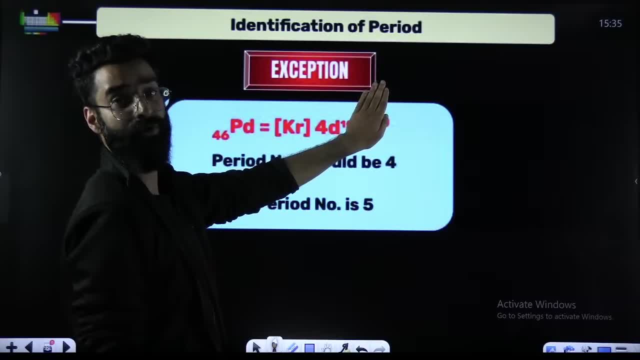 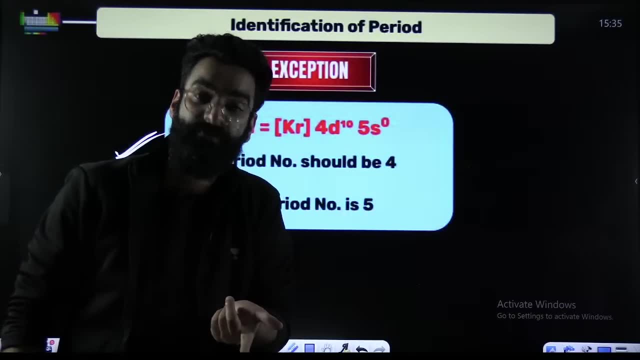 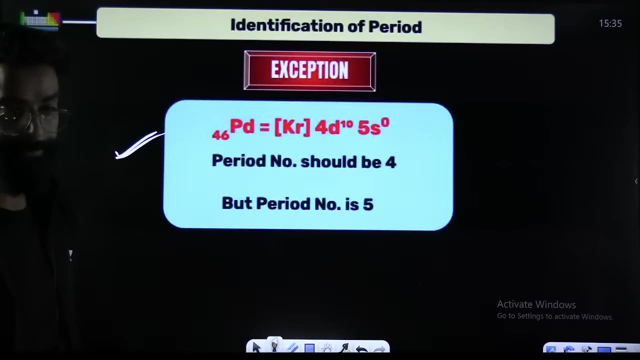 number. Its expected period number is supposed to be 4. But actually it is 5. Okay, Remember this in the form of exception: Palladium: its expected period number is 4. But its actual period number is 5. Okay, But its actual period number is 5. Okay. So right now I am making you understand. 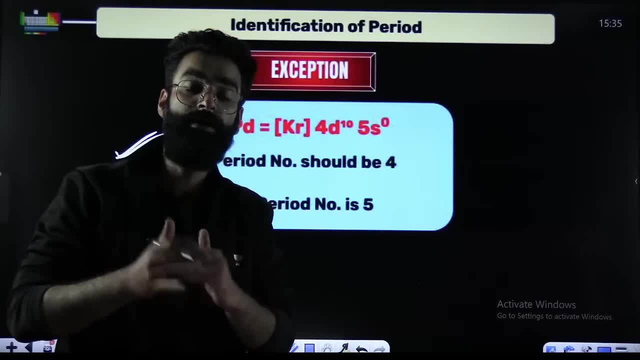 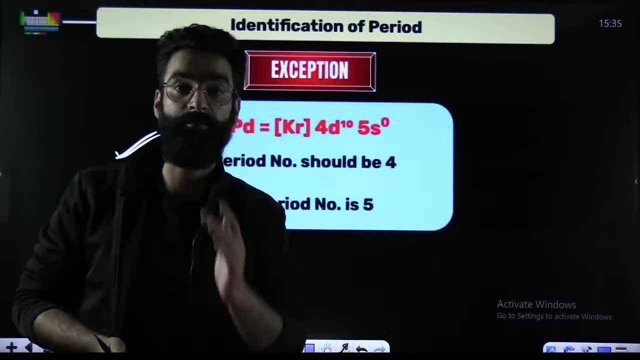 If you are given with some electronic configuration and you have to identify the period number, what do you have to do? You have to check the highest principal quantum number. Highest principal quantum number is always your what. It is always your period number. Okay, Exception 1 is there. That is palladium. 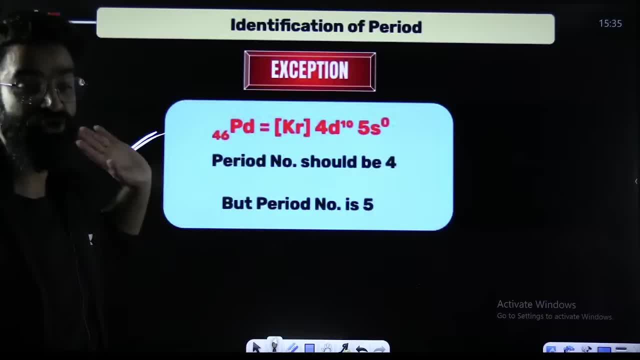 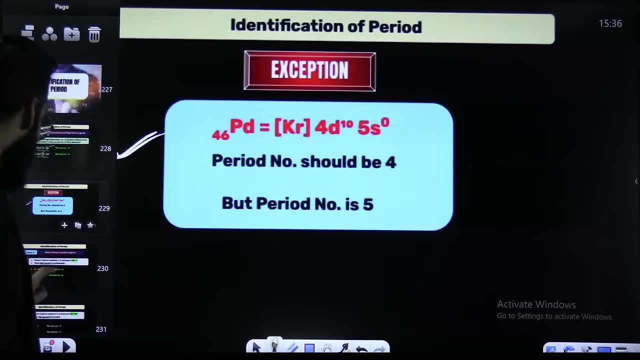 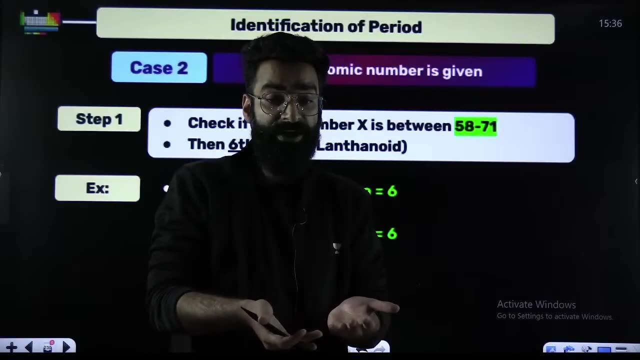 Perfect. Its period number should be 4.. But it is actually 5.. Remember it in the form of exception itself. Okay, This was question number 1 on period, Question number 2.. What if electronic configuration is not given? What if you are given with atomic number? What if you are given with 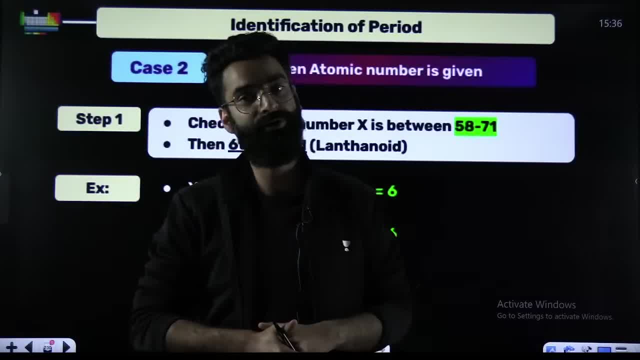 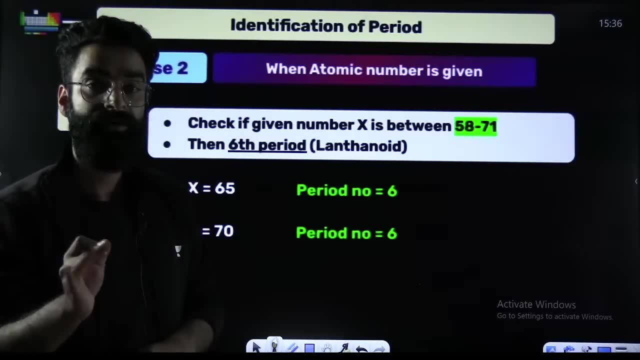 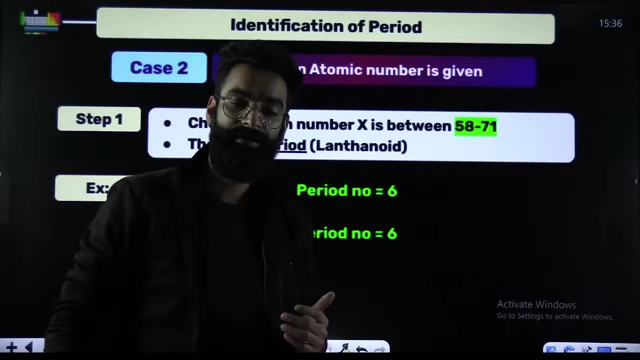 atomic number to identify the period. How do you do that? How do you do that? What if? what if you are not given with electronic configuration? What if you were unable to write electronic configuration Right? What if only atomic number is given and you are supposed to check the period? 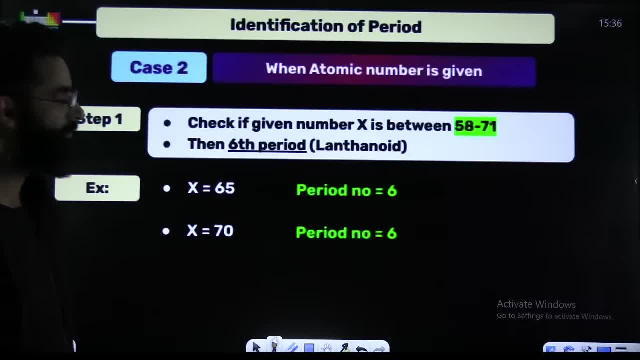 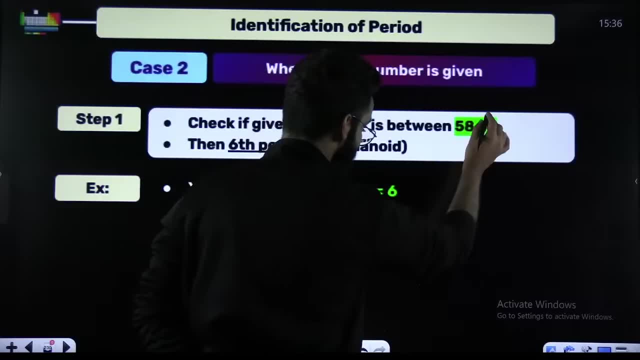 How do we do that? There are few things which you need to remember. There are few things which you need to remember, My dear students. remember this number 58 to 71. If you are given with the element, if you are given with the element x, for example, 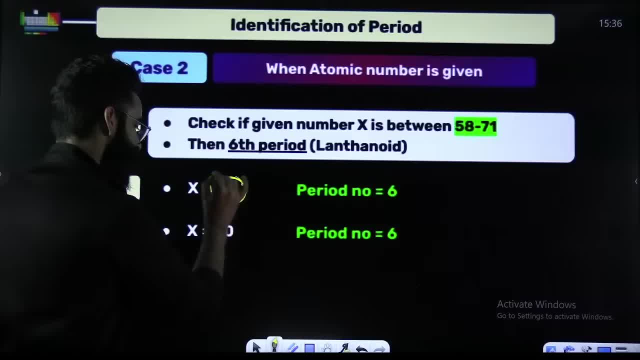 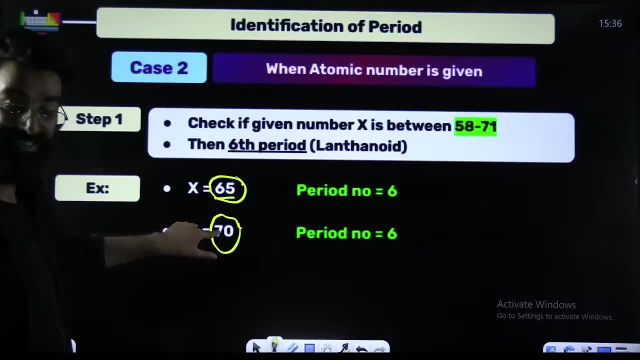 I mean if you are given with the element whose atomic number is 65 or atomic number is 70. Let's say, you are given with a general element whose atomic number is 65 or atomic number is 6, atomic number is 70. You have to identify their period numbers. You have to identify their period. 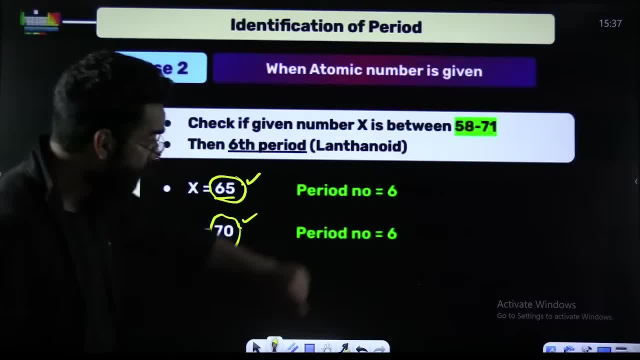 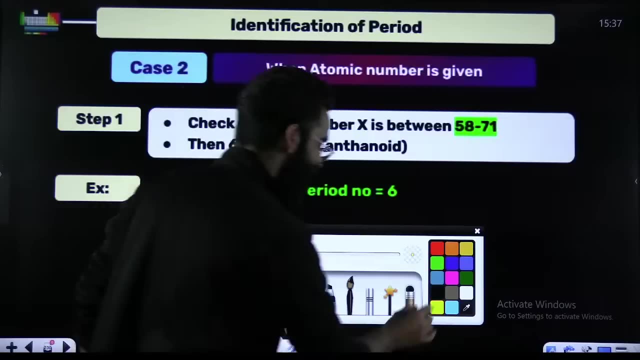 numbers. How, How you are going to do that? I am telling you to remember this number: 58 to 71.. If the atomic number given to you lies between 58 to 71,. if the atomic number given to you lies between 58 to 71,, then then directly remember its period. 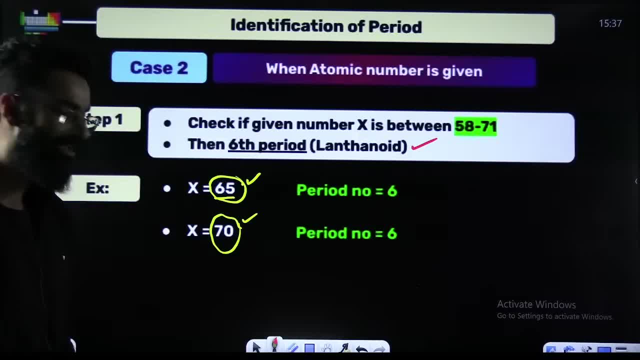 number is going to be 6.. Its period number is going to be 6.. Let's say atomic number 65. Atomic number 65 lies between 58 to 71. So directly remember, its period number is 6.. Directly remember. 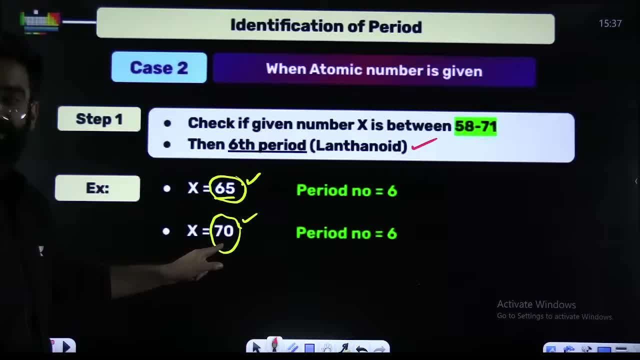 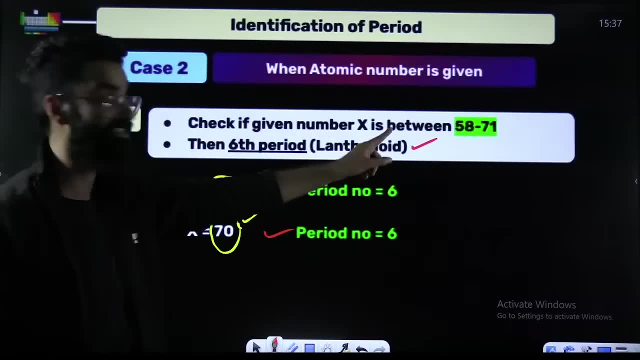 its period number is 6.. Atomic number 70. Atomic number 70. It lies between 58 to 71. It lies between 58 to 71. Its period number, again, is 6.. So remember this number first of all: 58 to 71. Perfect. 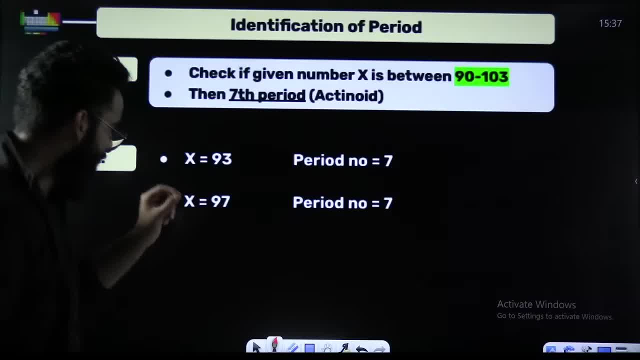 Now, that's not only it. That's not only it If the atomic number given to you, if the atomic number given to you lies between 90 and 103.. If the atomic number given to you lies between 90 to 103,. 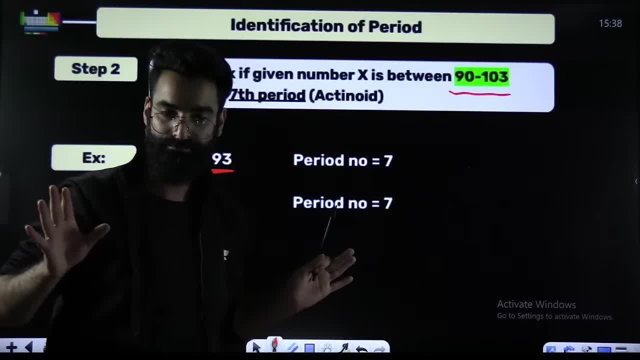 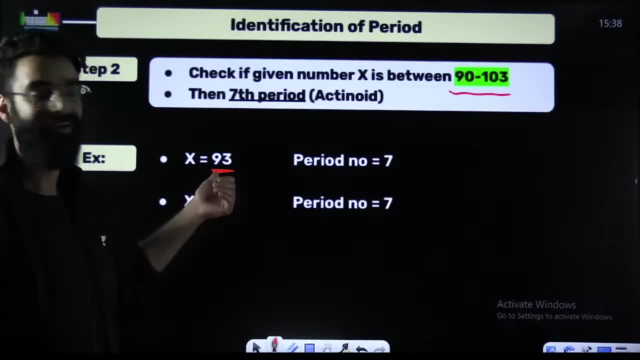 directly, you are going to remember its period number is 7.. Directly, you are going to remember, its period number is 7.. For example, 93 atomic number. It lies between 90 to 103.. Yes, This lies between 90 to 103.. Yes, So period number for both of them. 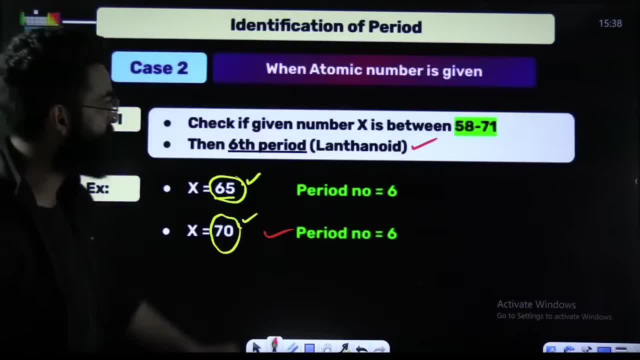 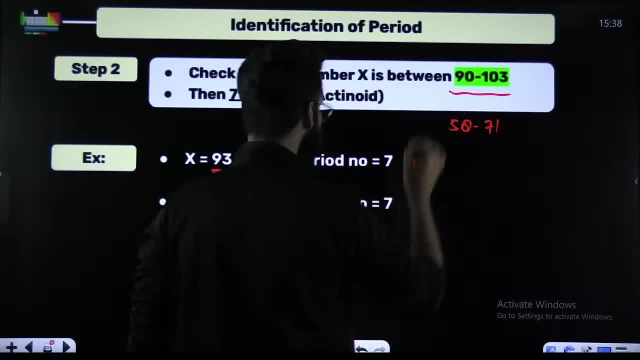 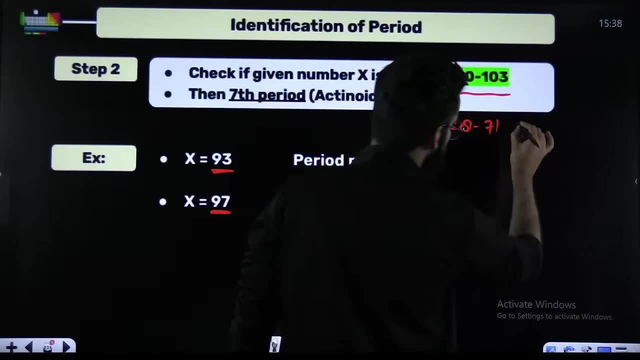 is 7.. So two things, Two numbers. First number is 58 to 71.. First number is 58 to 71.. 58 to 71. Second number is Second number is. Second number is 90 to 103.. Perfect, If atomic number lies. 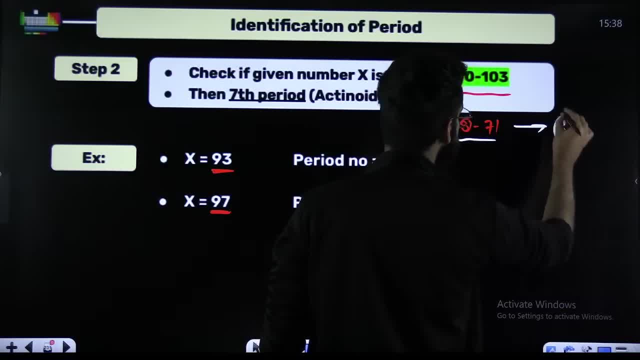 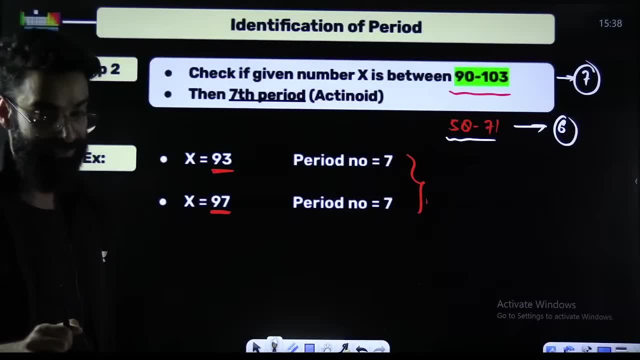 between these two. its period number is 6 and over here, period number is 7.. This is how This is not done yet, by the way, This is not done yet. by the way This is not done yet, I am showing you how to calculate the period from the atomic number. 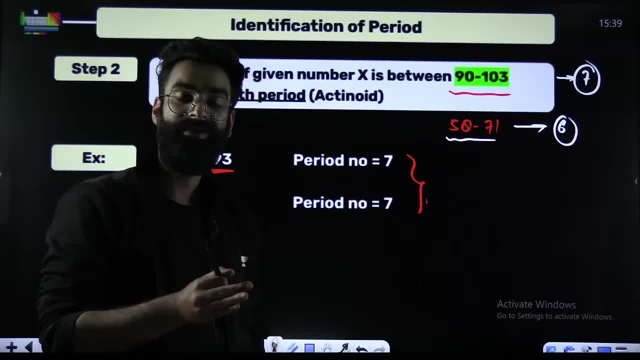 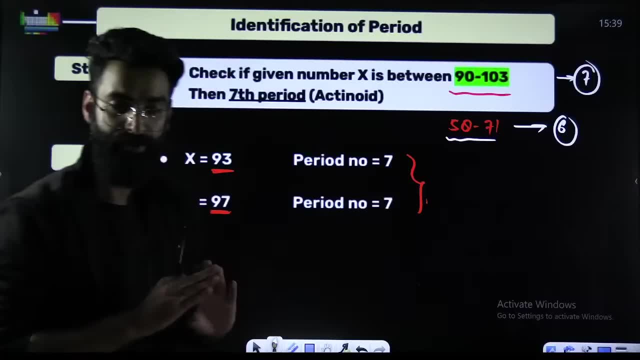 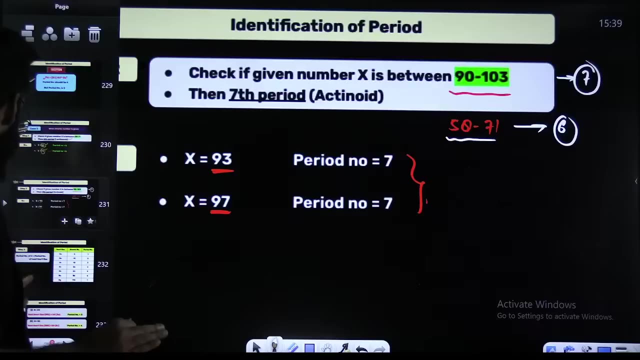 How to calculate period from the atomic number. If your atomic number lies between 58 to 71, period number 6.. If it lies between 90 to 103, directly, period number 7.. No need to check anything. No need to check anything. No need to check anything. Now understand, Now understand. 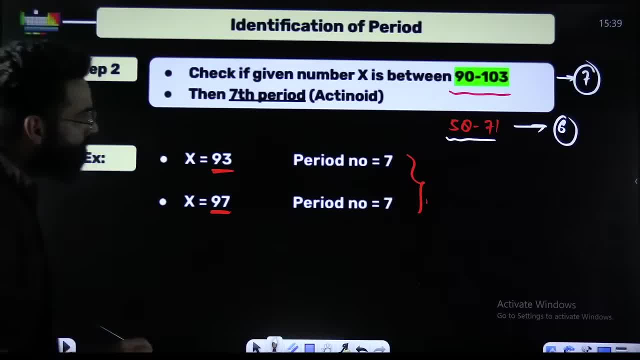 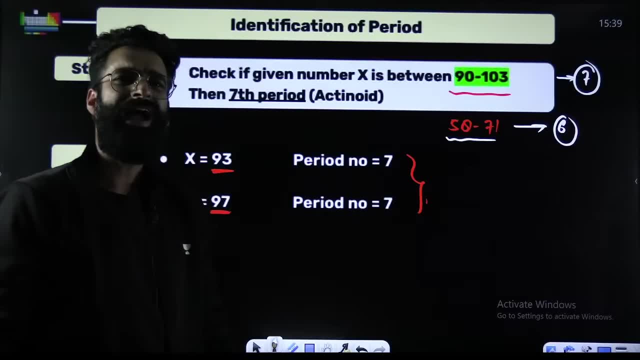 Now understand. So two numbers. I gave you 158 to 71 atomic number 190 to 103.. What if you are given with some atomic number which does not lie in this, Which does not lie in this as well? What if? What if, For example, I am given with the: 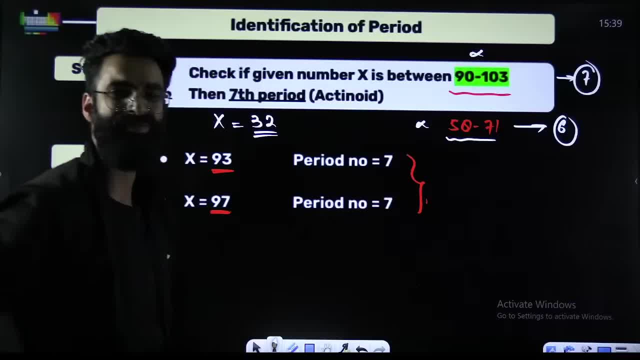 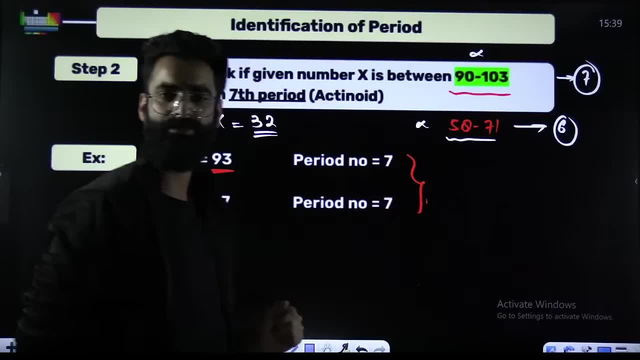 element x, whose atomic number is 32.. I have to check its period. I have to check its period. Now, this atomic number, neither it lies between these 2 nor it lies between these 2.. Perfect, How do we check at that point of time? All right, Dear students, first of all. First of all, You have to 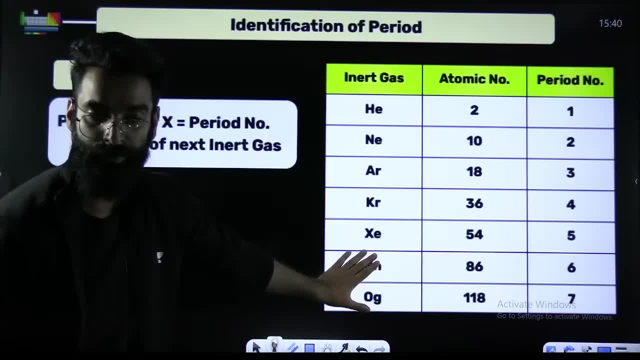 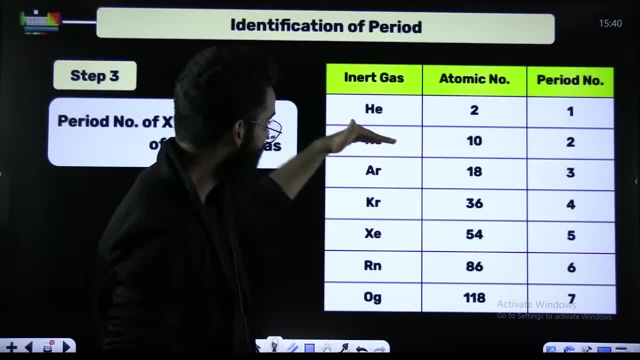 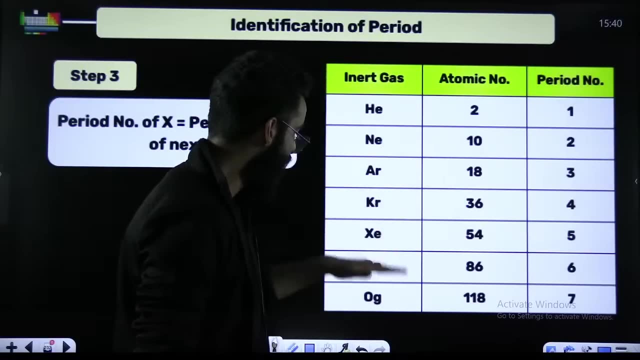 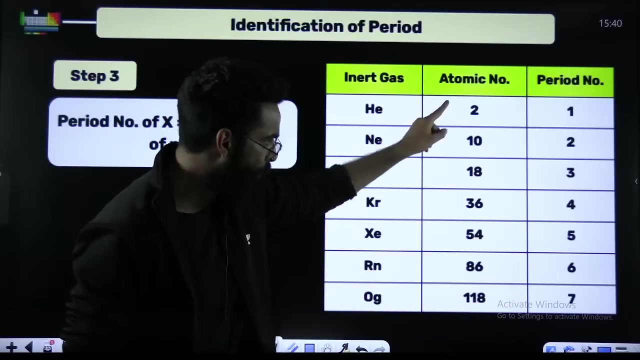 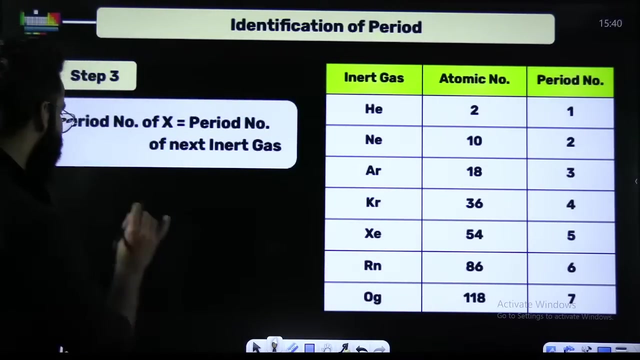 remember the atomic numbers of your noble gases. You have to remember the atomic numbers of your noble gases. Helium, Atomic number 2.. It belongs to period number 1.. Right Neon, Atomic number 10.. 18, Krypton, 36,. Xenon, 54,, Redon, 86,. you have to remember their atomic numbers 2, 10,, 18,, 36,, 54,, 86,, 118,. 2, 10,, 18,, 36,, 54,, 86,, 118,. now, now, now understand, understand. for example, I am given with the element whose atomic number is 32, its atomic number is 32,. 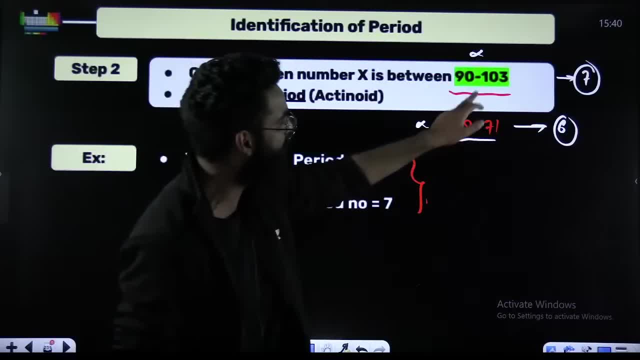 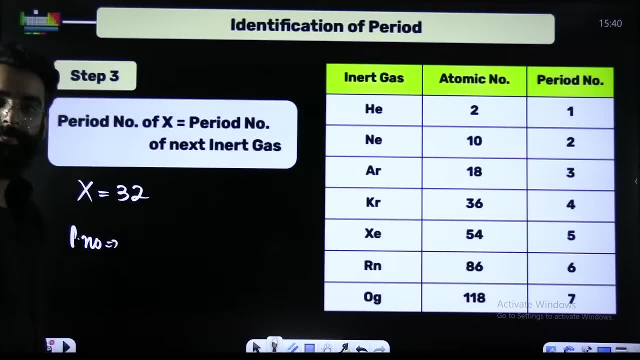 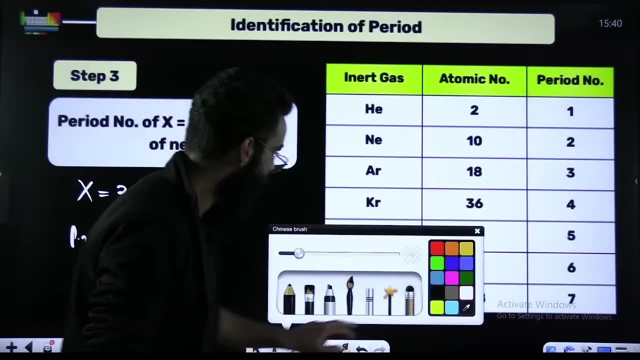 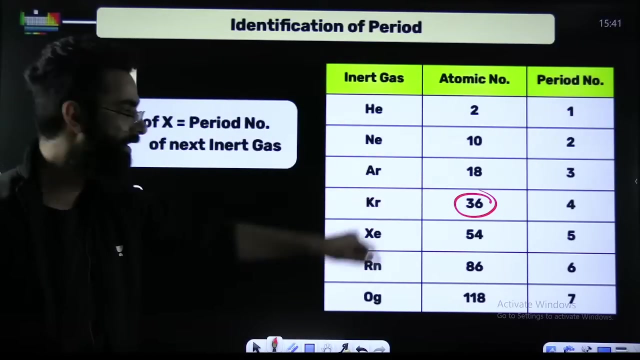 32 atomic number. neither lies between this number nor with this number. now, how do I check its period number? how do I check its period number? now, my dear students, tell me one thing: after 32, which noble gas do you have? after 32,, you will have this noble gas. after 32,, you will have this noble gas. right after 32, atomic number, you will have this noble gas, perfect. what is its period number? 4, so its period number will be also 4, am I clear? 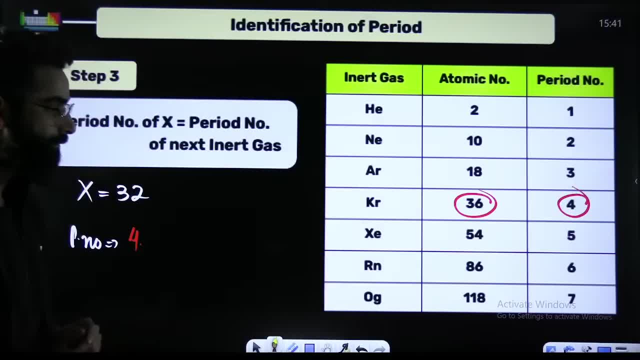 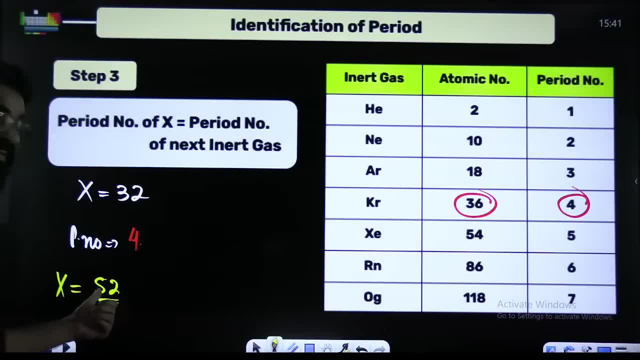 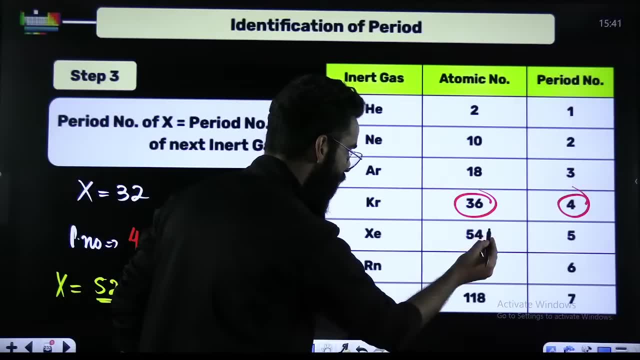 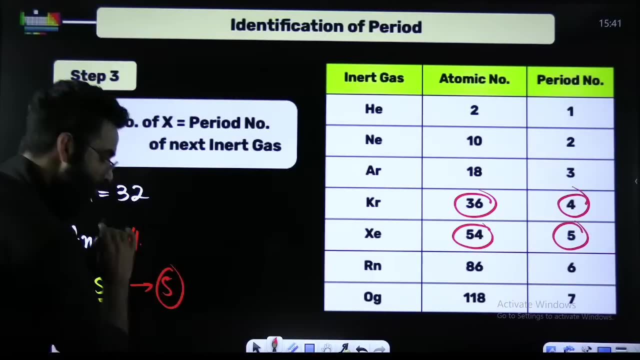 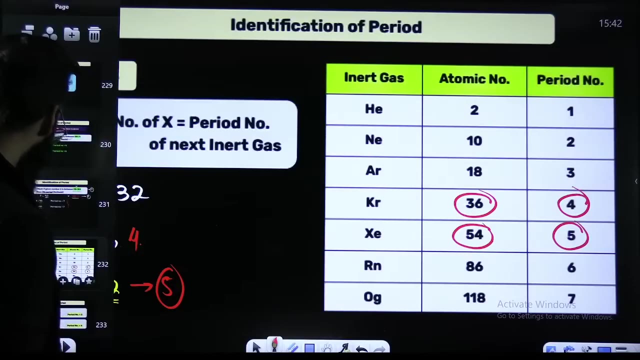 it's not now. now, what is the next noble gas atomic number after 52,? after 52, the noble gas atomic number is what? after 52, noble gas atomic number is 54,. it belongs to period 5, so I will say: this particular element will be belonging to period 5, am I clear? am I clear? am I clear people? am I clear? am I clear? 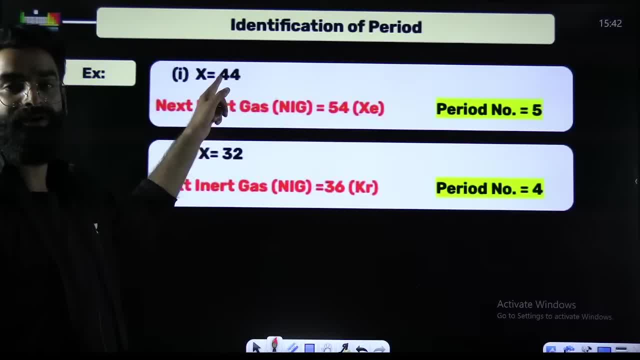 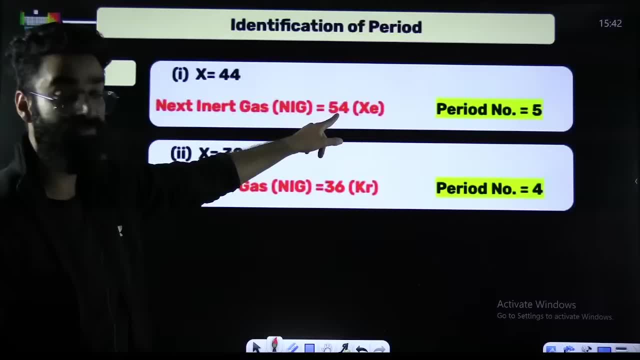 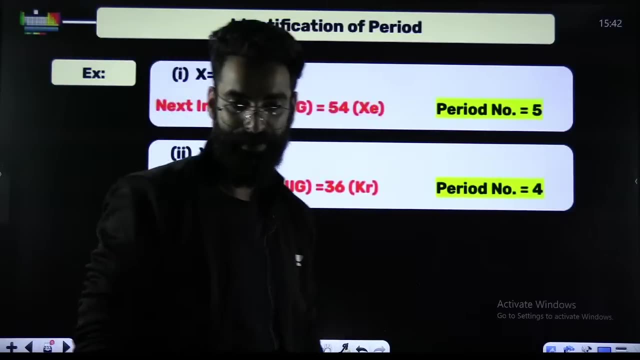 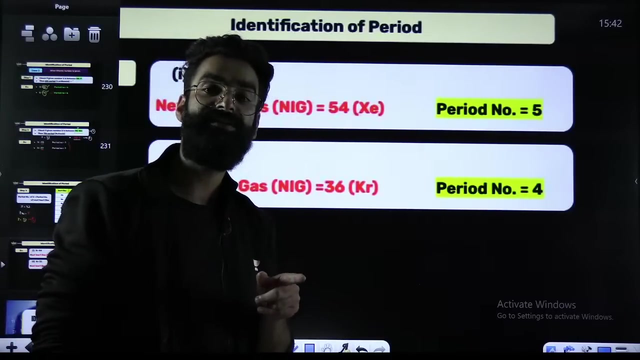 we are given element x, whose atomic number is 44,. after 44,, the next, the next noble gas configuration, the next noble gas atomic number is 54, 54,. its period number is how much? 5, so its period number is 5, and same goes for the other ones. I believe it's clear. I believe it's clear. this was identification of the period if atomic number is given, and that atomic number does not lie among those two values which I gave you. 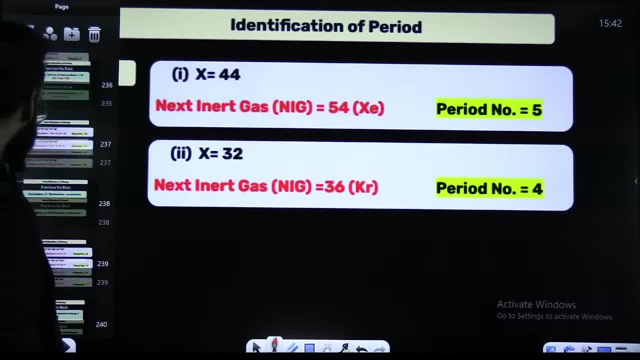 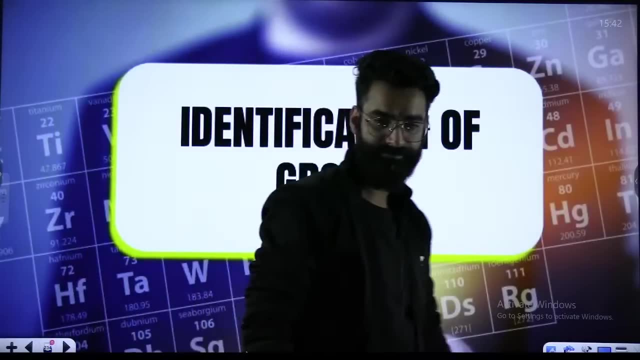 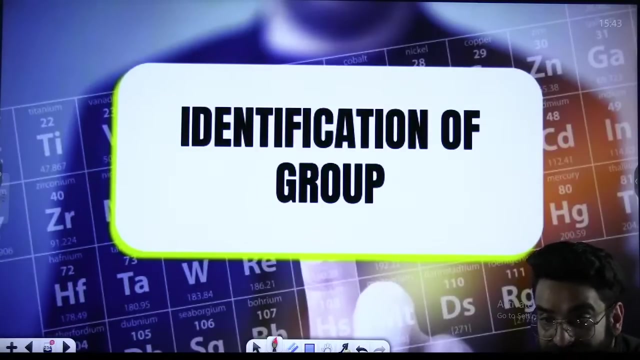 let me know once in the chats if I am clear. let me know once in the chats if I am clear. yes, is it clear, but but. but this is all volatile. if you do not remember all these things afterwards, you are gone, you are over. 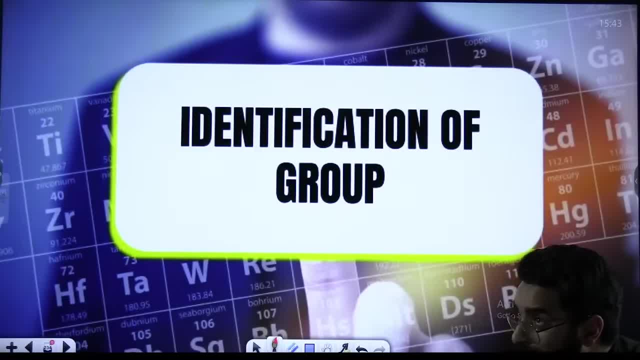 you are over, guys. let me tell you, when I earlier used to teach this periodic classification, it used to take me 7 to 10 hours. why? because in this chapter itself I used to deal with all the compounds of S block. 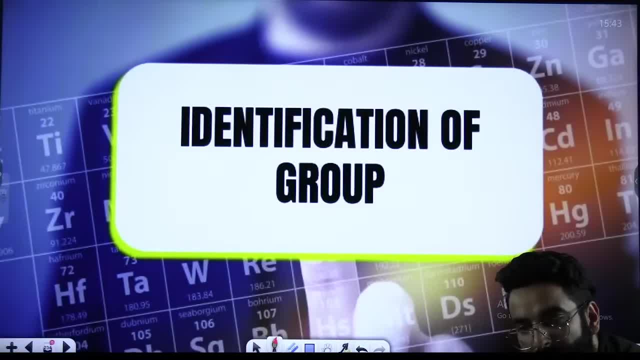 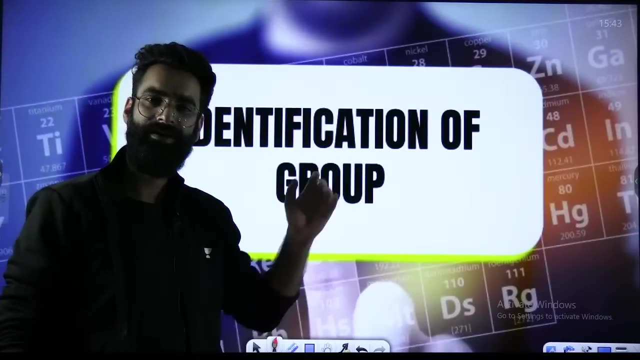 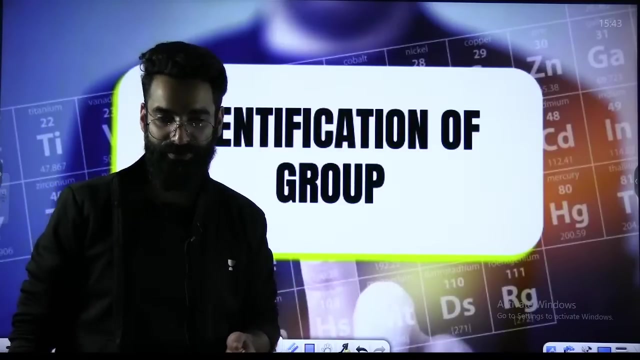 all those trends of S block. but now your S block is over, that is deleted, right, so we do not need to relate this particular chapter with S block, right, all the trends. you would have seen a lot of lectures where in teachers, in periodic classification, they complete all the trends of inorganic from S block at least, right, that's why it used to take time. but now S block is not there, so you are not supposed to do that. yeah, now, now comes identification of the group. 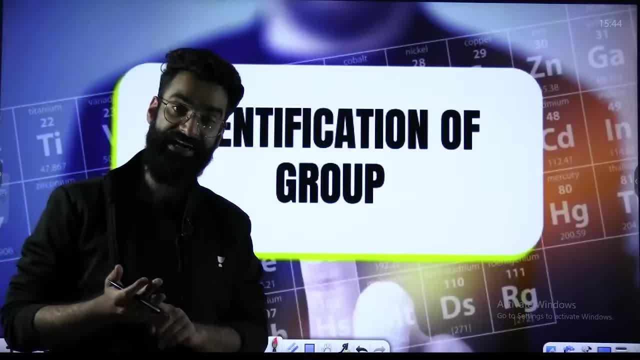 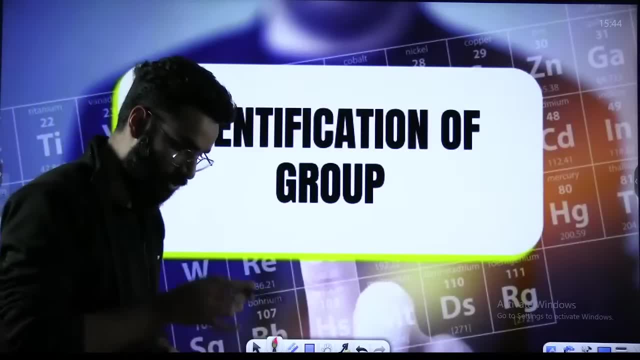 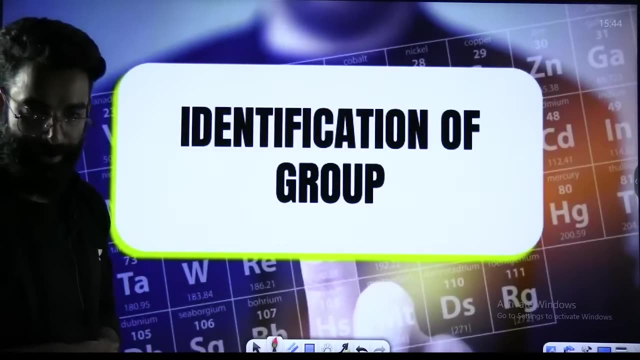 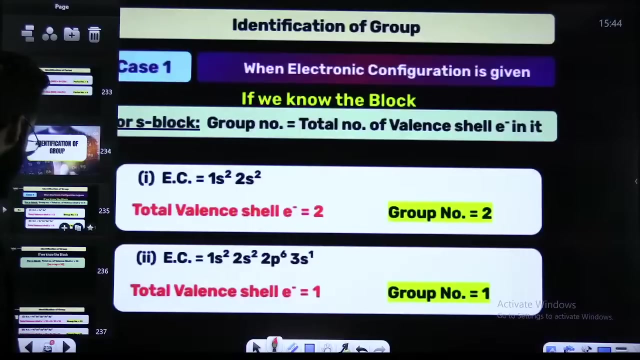 first one was identification of block. second one is identification of period. third one is identification of what, identification of group, whether element belongs to first group, second group, third group, fourth group, fifth, sixth till 18th. right, okay, right now, have a look. now have a look. few things, that's what. few things to remember, few things to remember. 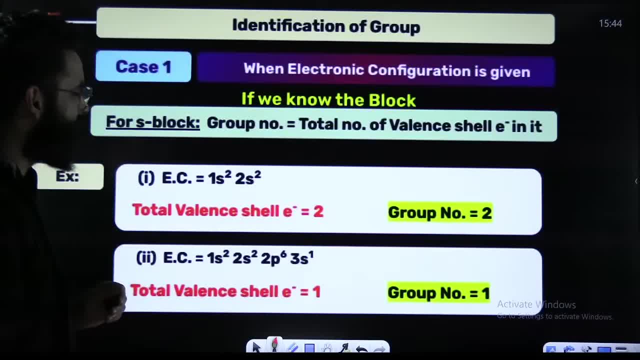 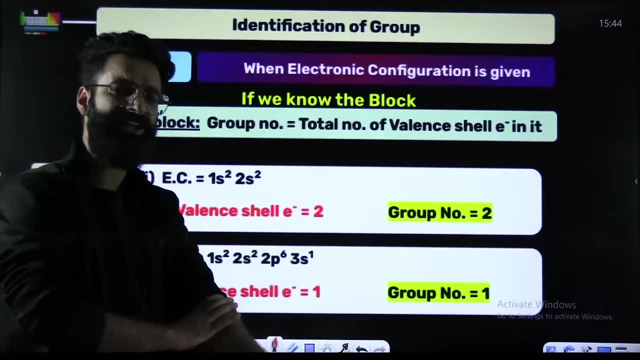 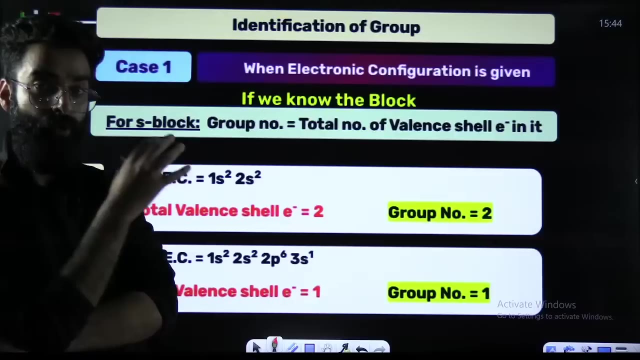 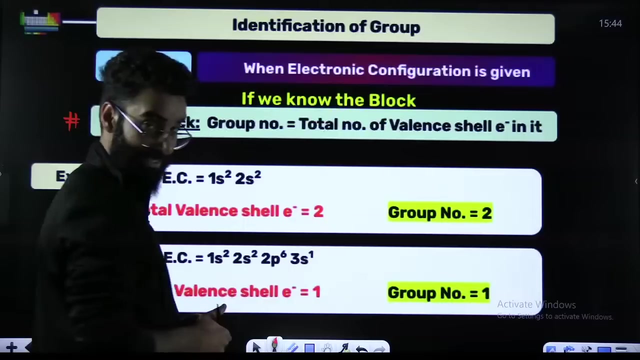 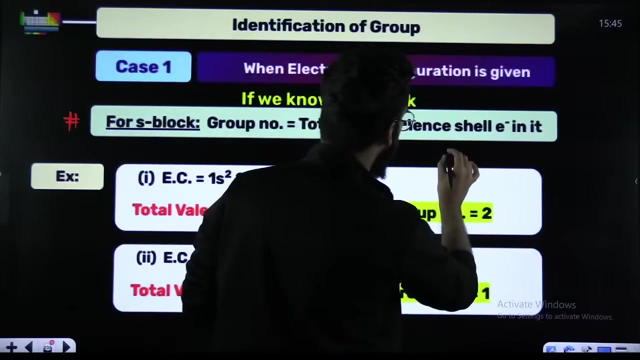 first of all, let's say you are given the question in which you are given with the electronic configuration of an element. let's say you are given with the electronic configuration of an element. okay, let's say you are given with electronic configuration of an element. from the electronic configuration, can you identify the block? you can identify the block. you can identify the block. once you identify the block, if the element belongs to S block, if the element belongs to S block. if the element belongs to S block, then then then. total number of electrons in valence shell. 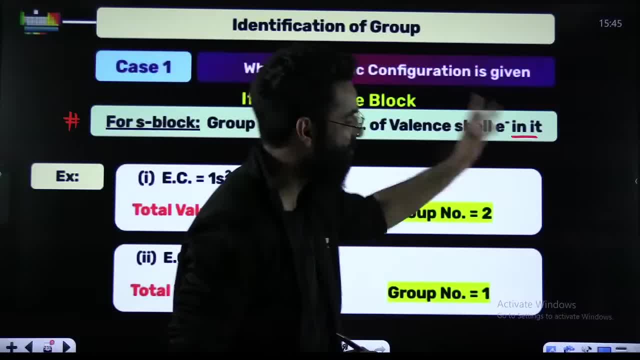 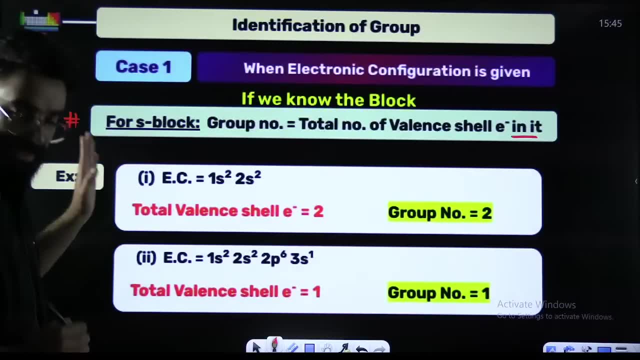 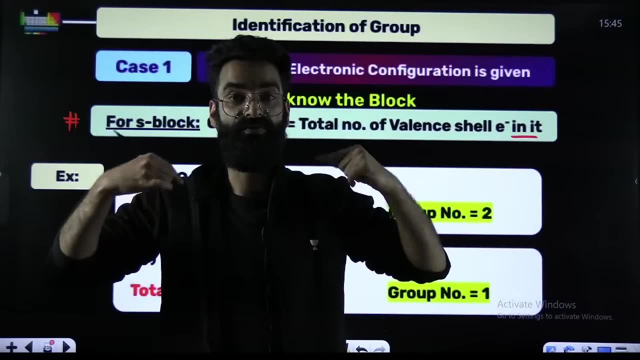 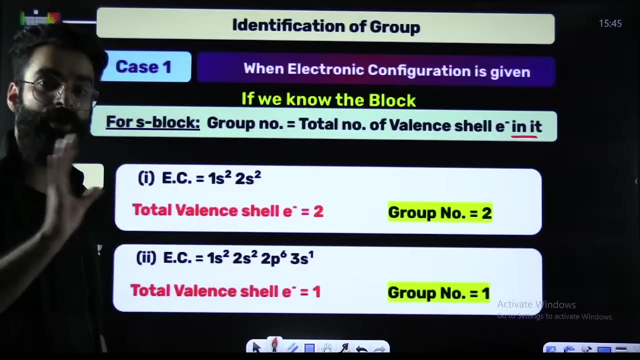 total number of valence shell electrons. total number of valence shell electrons is equal to its group number if the element belongs to S block. so, first of all, first of all, if electronic configuration is given from the electronic configuration, what am I supposed to do? I am supposed to check the block of the element. if the element belongs to S block, then just check the total valence electrons. 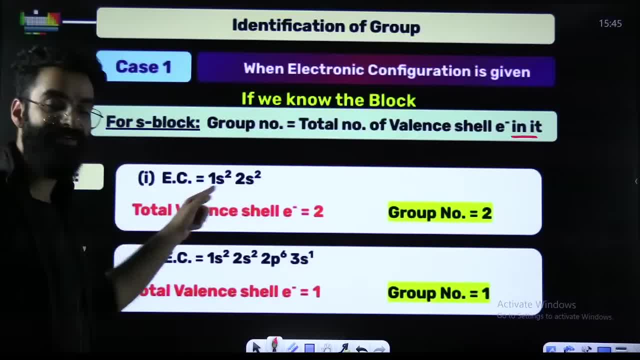 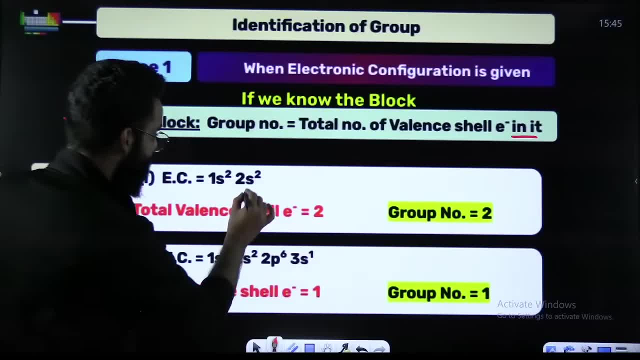 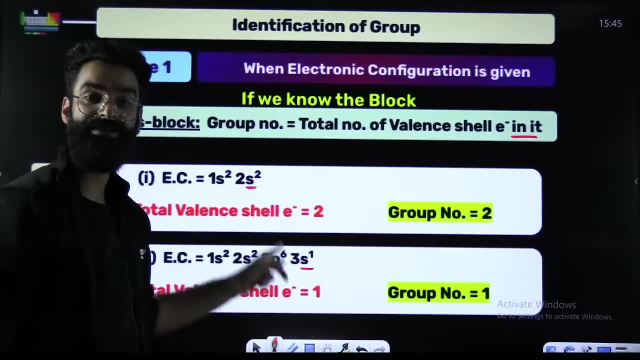 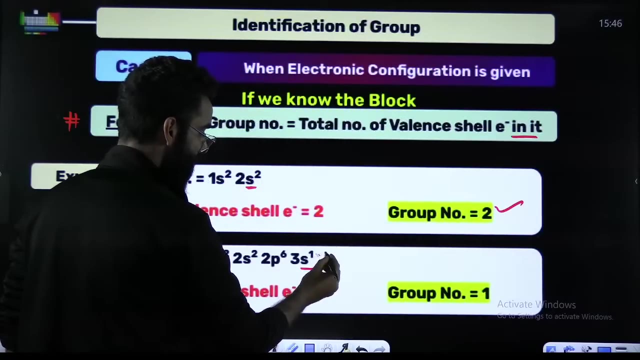 if the element belongs to S block, then just check the total valence electrons. this is the electronic configuration given to me, right? I identified it as an S block element. I identified this is an S block element. now check the valence electrons. valence electrons here are 2, valence electron here is 1, here is 1, and in this particular case, in S block elements, number of valence electrons is equal to group number. so group number here will be 2, group number here will be 1, right? group number here will be 1, am I clear? am I clear? 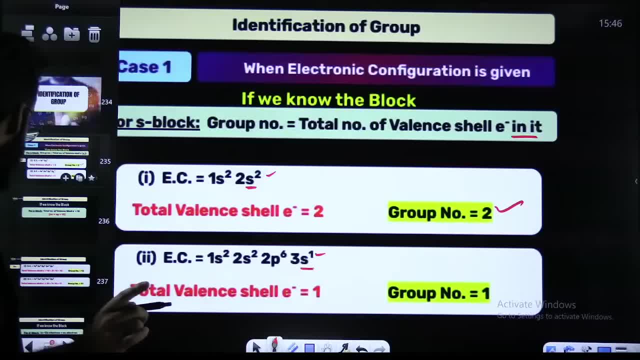 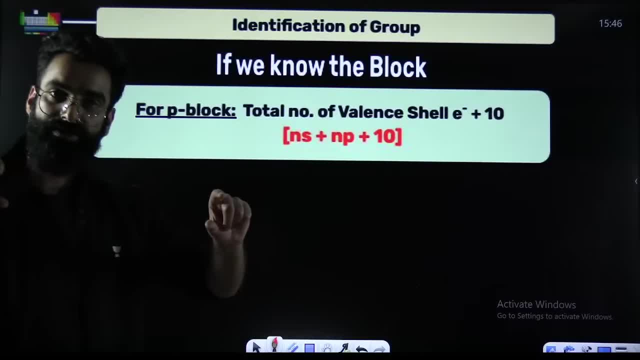 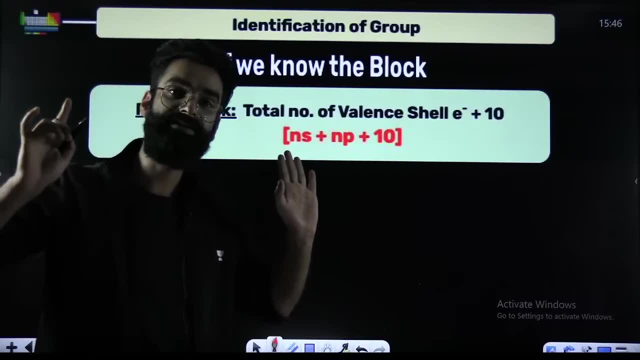 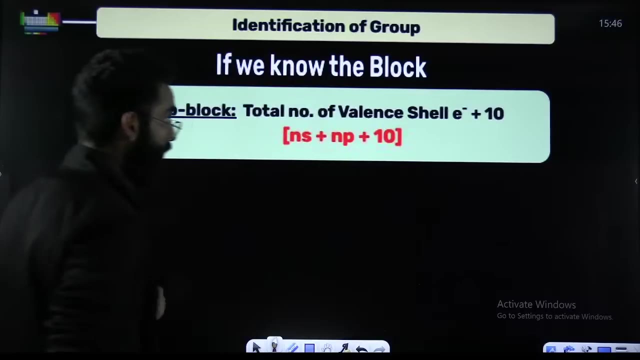 am I clear? this is for what? this is, for S block elements. this is for S block elements. now, now, if you are geared with electronic configuration, right, if you are geared with electronic configuration and you identified which block element it is, if the element is from P block, if the element is from P block, if the element is from P block, how to identify its group? then? simple, simple. 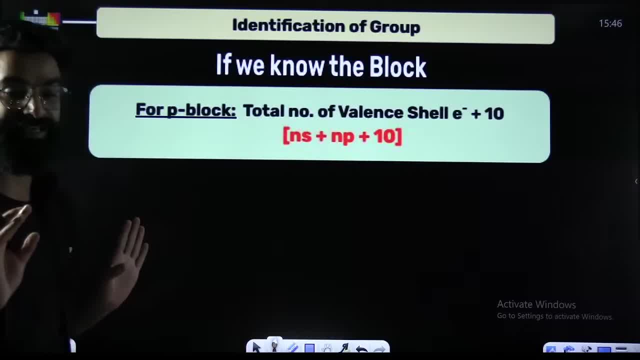 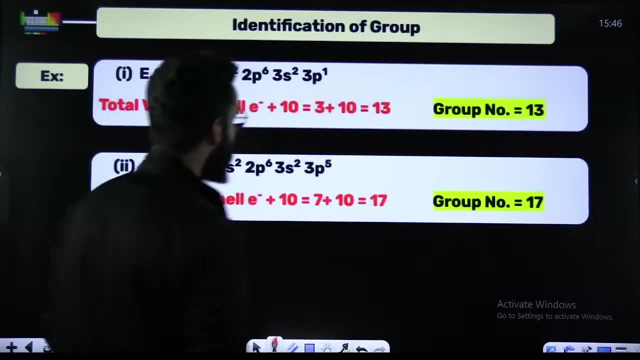 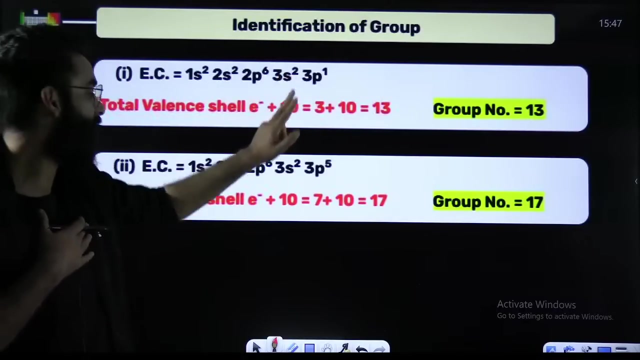 Ns plus Np plus 10,. total number of valence electrons plus 10, or you can remember it like this: Ns electrons plus Np electrons plus 10,. what it means: Ns electrons plus Np electrons plus 10,. have a look on the examples: Ns plus Np plus 10,. Ns plus Np plus 10, right. first of all, this is the general electronic configuration that is given. I identified that this configuration is it belongs to P block element. this also belongs to P block element, right. Ns plus Np plus 10,. Ns plus Np plus 10, right. 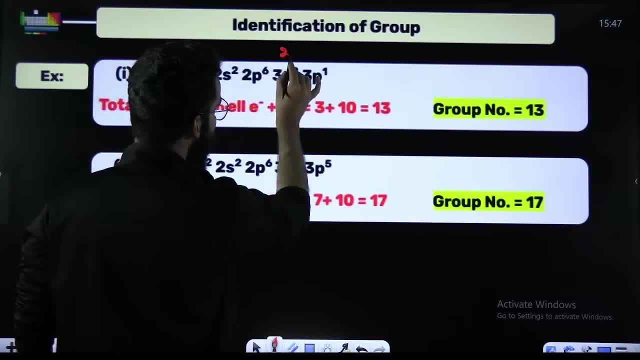 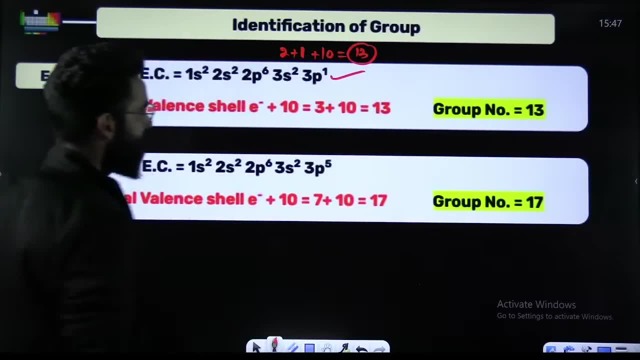 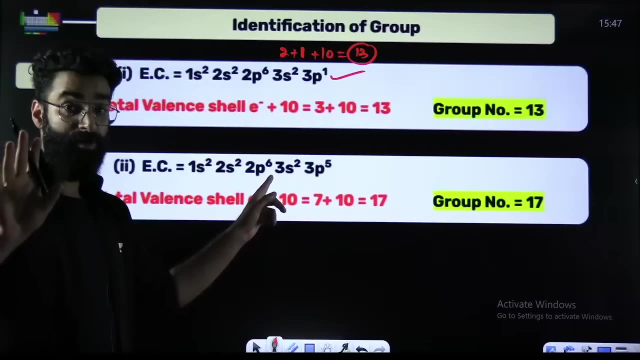 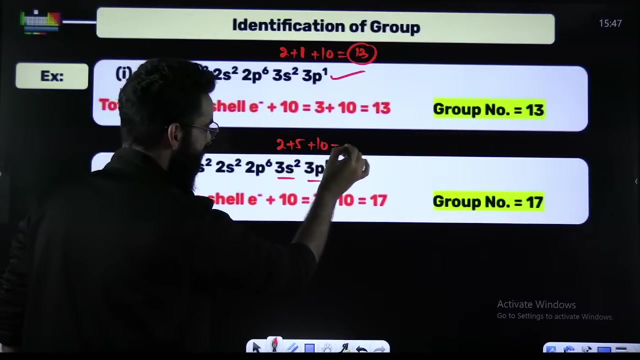 Ns is here 2, Ns is here 2 electrons. Np contains 1 electron. plus what? plus 10, it comes out to be 13,. so 13 is the group number of this particular element whose configuration is given right, perfect N. N is the principal quantum number, by the way, right Ns is containing Ns is containing 2 electrons. Np is containing 6 electrons and it is a P block element. so plus 10,. so group number here is nothing but 17,. 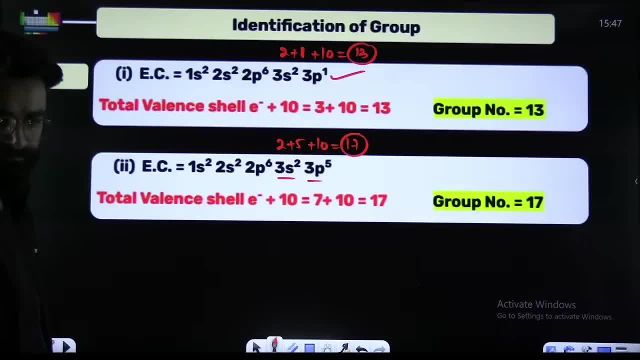 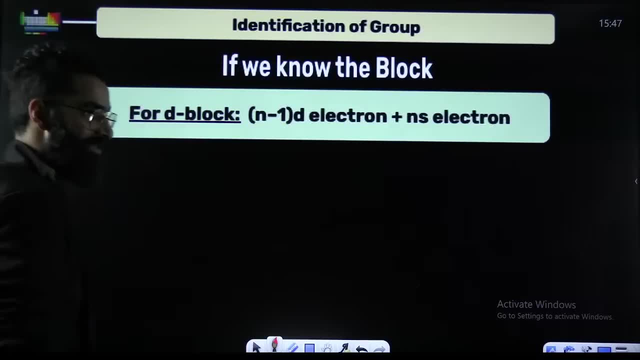 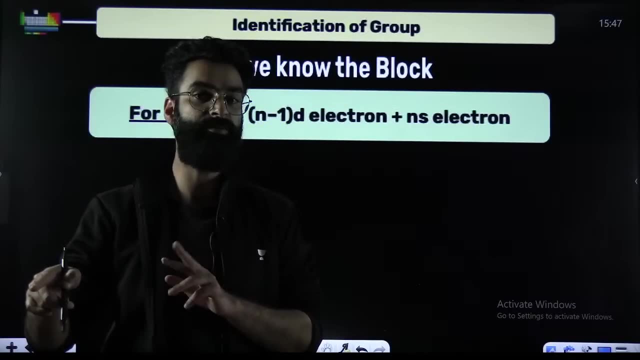 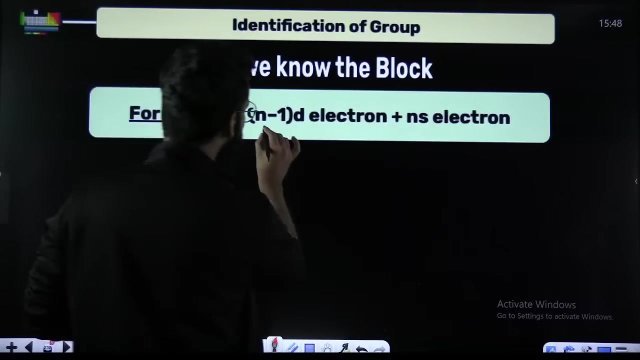 group number: here is nothing but 17,. group number: here is nothing but 17,. right now, for the D block elements, for the D, for S block elements: total number of electrons in Ns: right, that gives you the block number. here it was Ns electrons plus Np electrons plus 10, in case of D block it is N minus 1 D electrons plus Ns electrons. 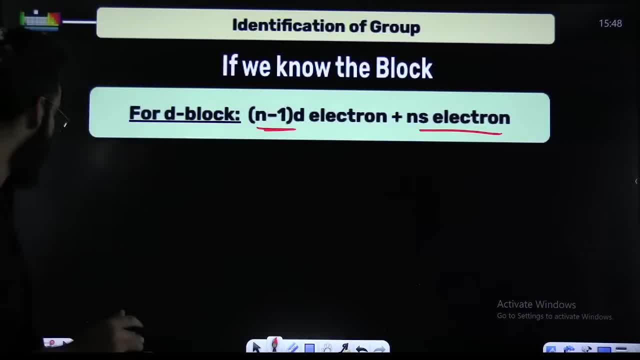 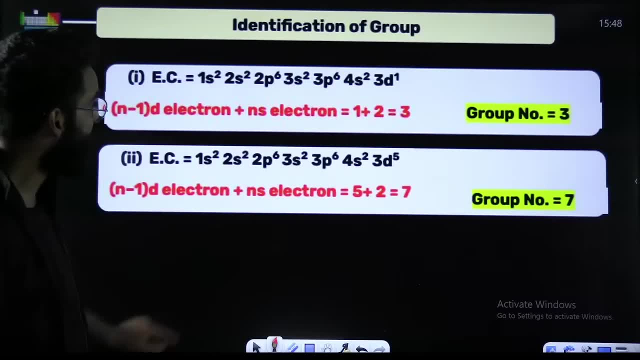 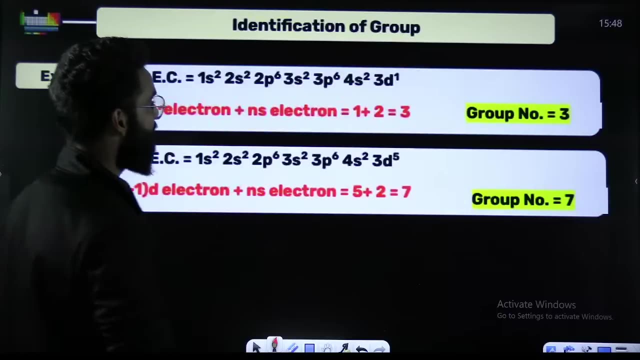 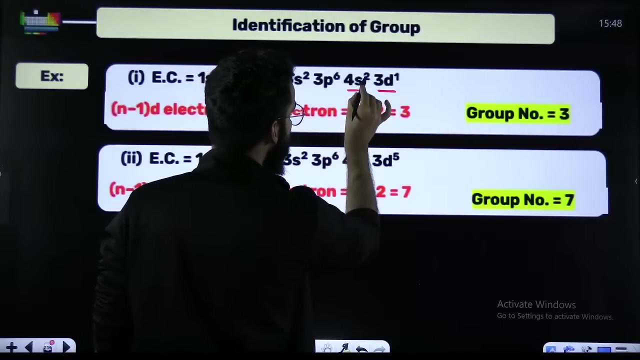 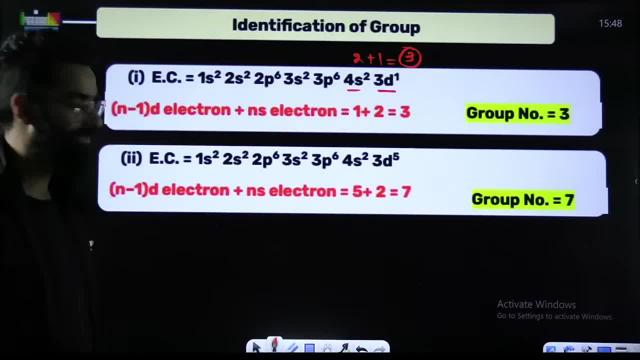 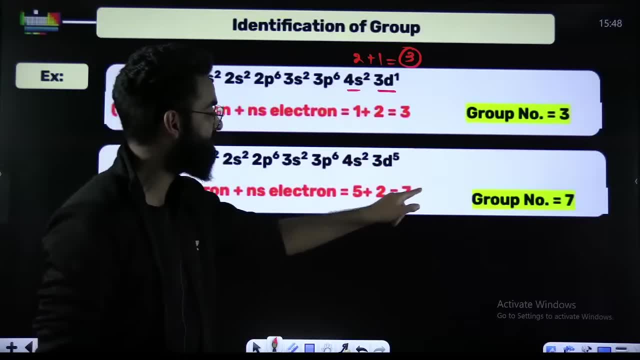 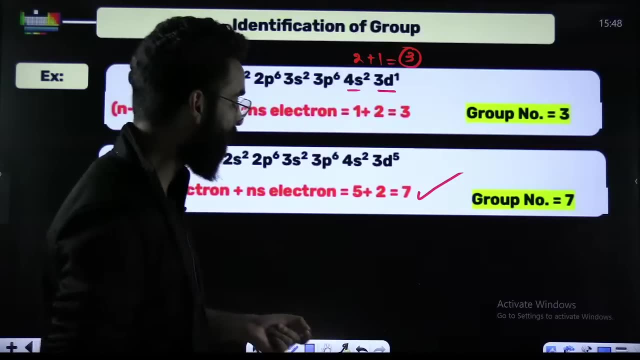 perfect. now look at this one. look at the next one: Ns is containing two electrons, N minus 1. D is containing 5 electrons, so 5 plus 2 is 7, so if electronic configuration is given and from the given electronic configuration you identified that element is from D block, then you can identify its group number as well, right, 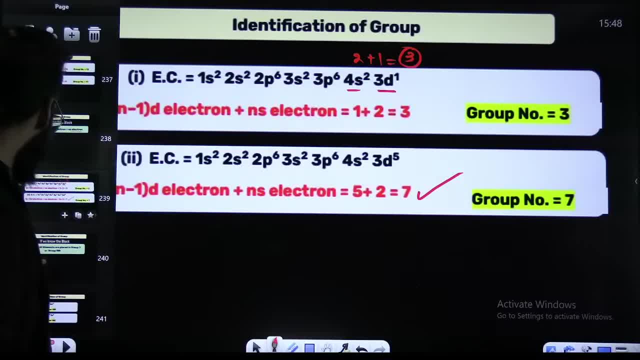 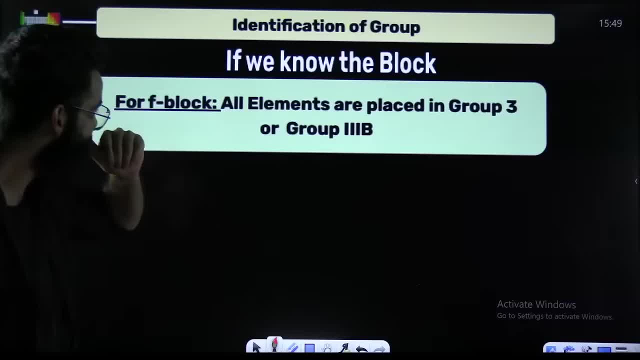 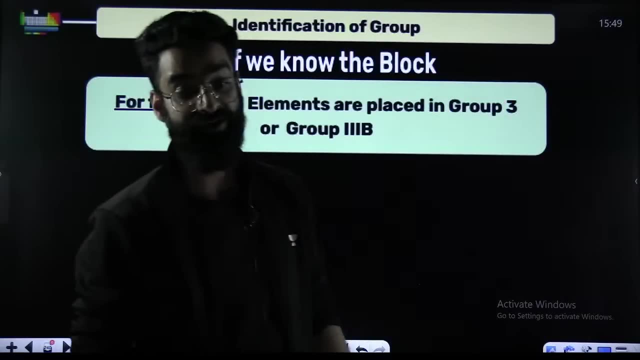 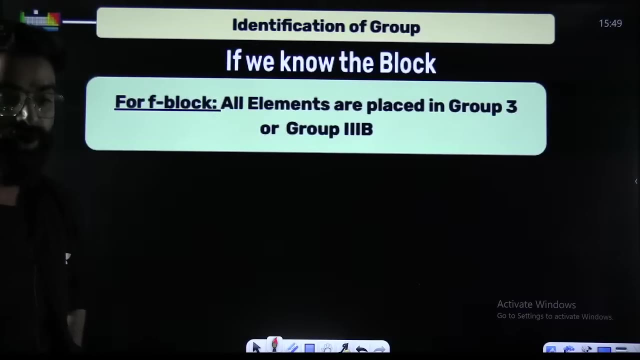 now, what about? what about the F block elements? what about the F block elements? all the elements, all the elements based in group 3? here you do not have to remember any formula. here you do not have to remember any formula. guys, right here, you are not supposed to remember any formula. perfect, perfect, perfect. 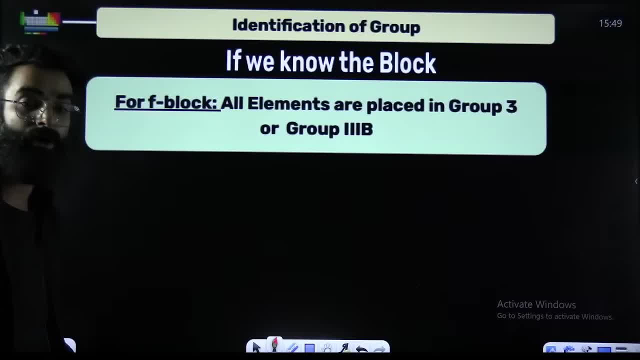 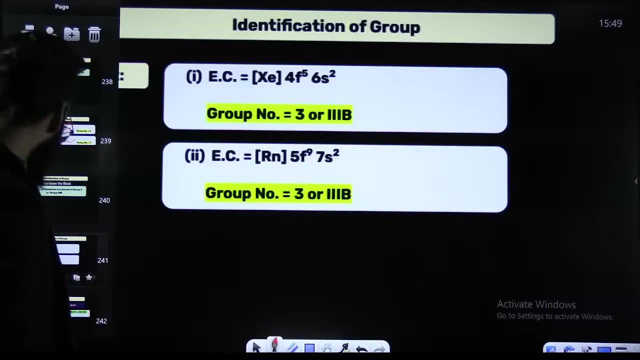 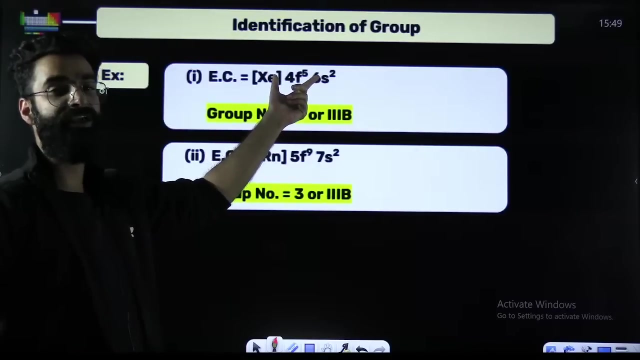 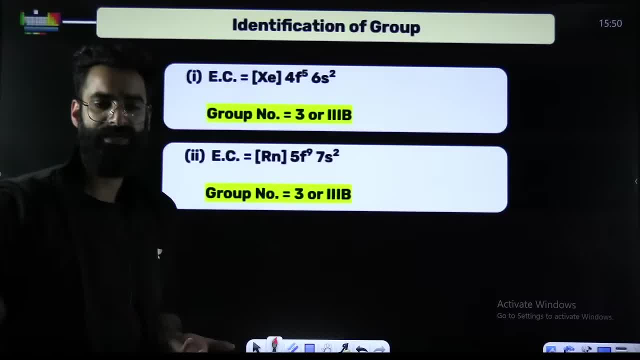 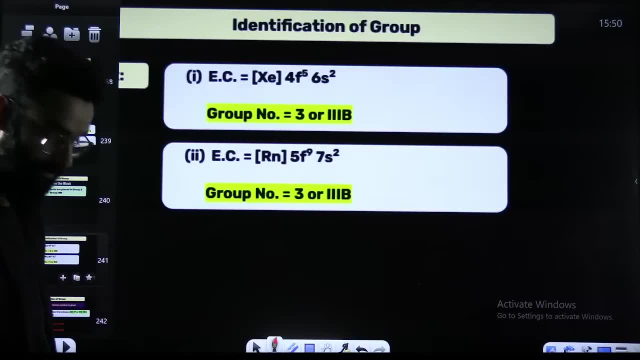 elements, its group number is three. if this is a block element, its group number is three. that's what? yeah, that's what, now, now. i was telling you how to identify the group. if electronic configuration is given, if electronic configuration is given now, now, how do you identify? 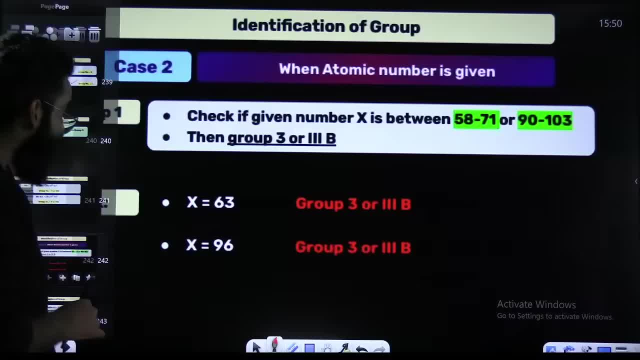 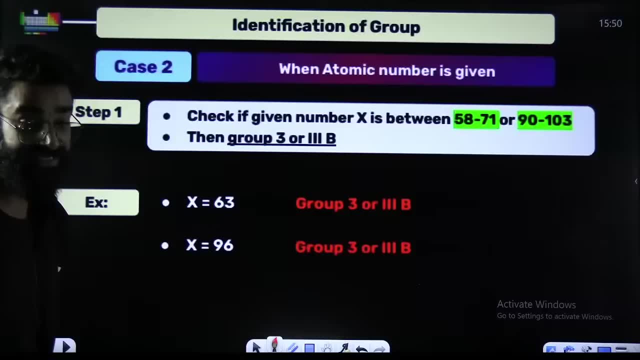 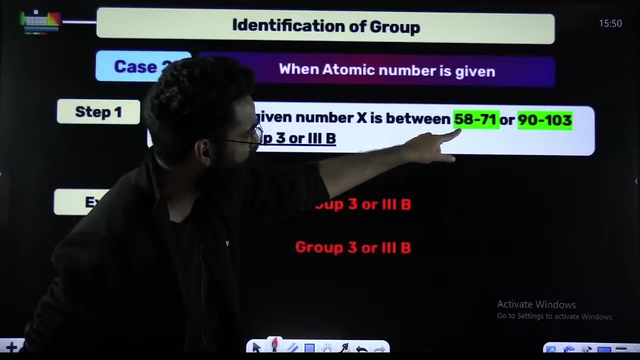 the group if atomic number is given? how do you identify the group if its atomic number is given? how do we identify the group if its atomic number is given? look at this particular slide once. how do you identify the group if its atomic number is given? look at this particular slide. check if the given number is between 58 to 71 or 90 to 103. 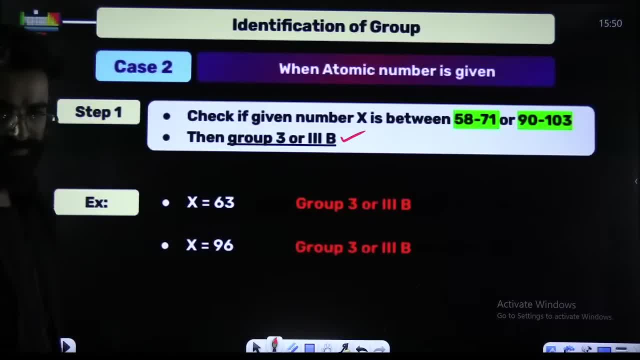 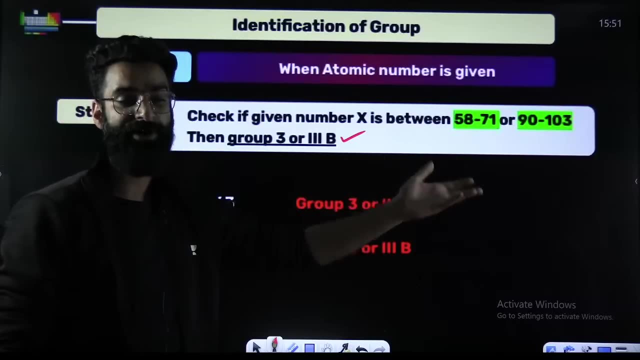 then the elements element belongs to third group. right, then the element belongs to third group. third group, a block- this is. this is something which you know. now, right, perfect, element belongs to third group and you can identify whether it's lanthanoid or actinide. you can identify whether it's lanthanoid or actinide- perfect, if atomic number is given. 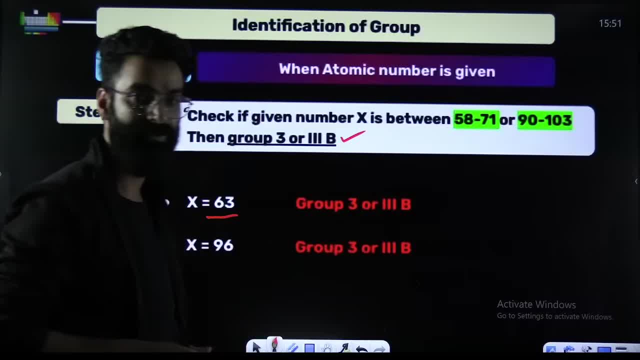 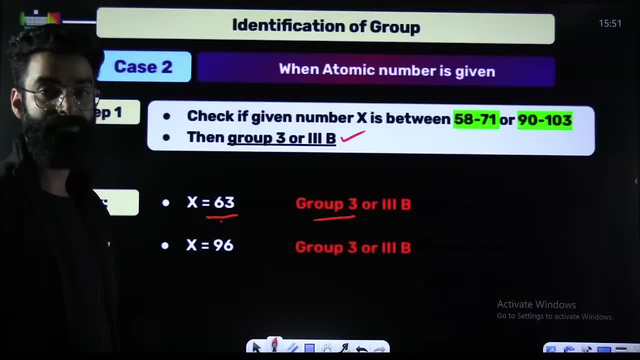 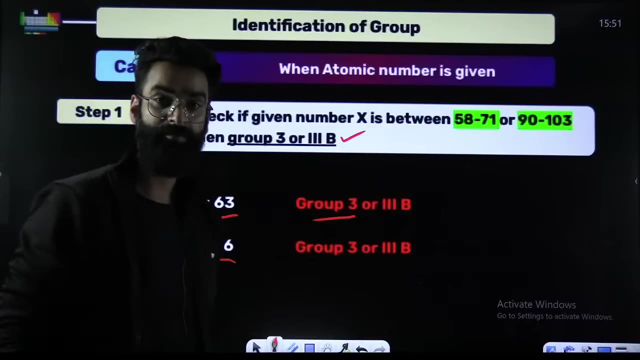 as 63, for example, 63 is lying between this particular number, so group number is three. 63 means a block right. and which, which one, which one lanthanoid perfect? similarly 96. it belongs to that particular number, between that particular number: 90 to 103. so at that point of time, 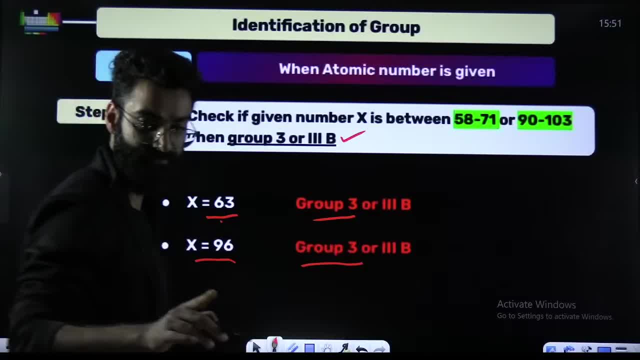 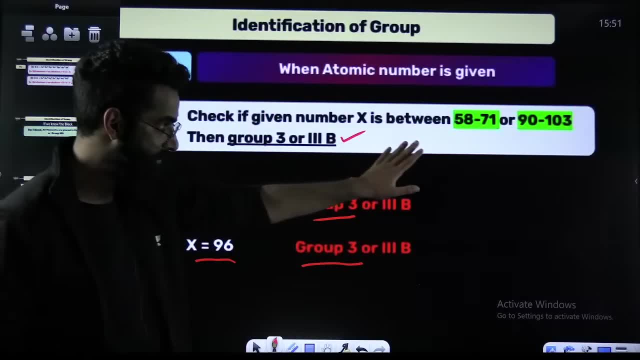 group number is three. this is the first case if, if my dear students, atomic number is given and you're supposed to check the group number first, remember these two numbers: 58 to 71, 90 to 103, if atomic number is coming in between them. so 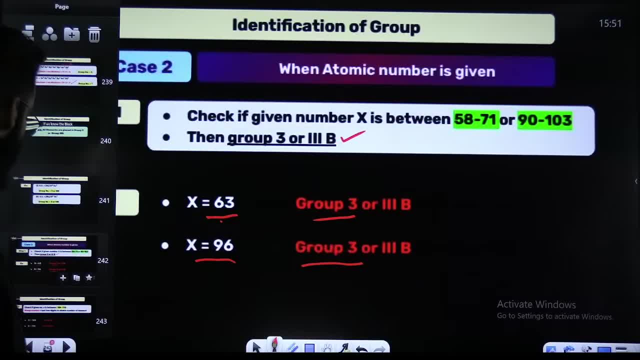 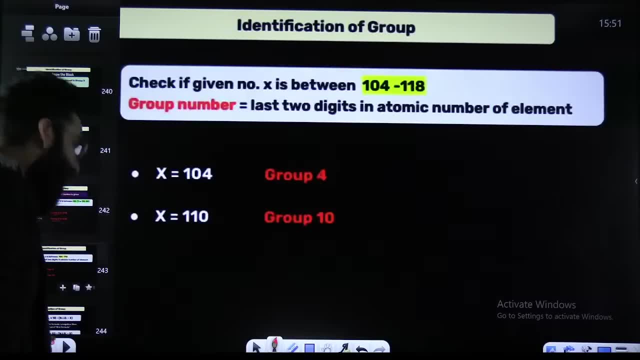 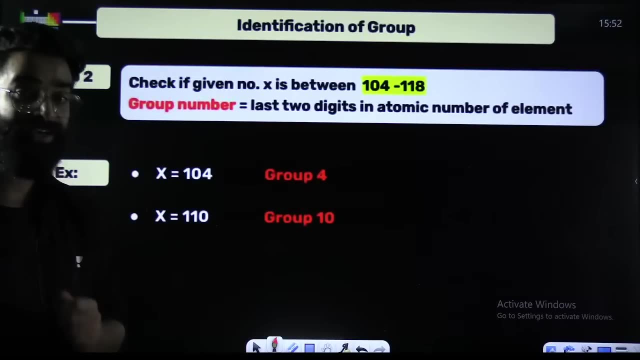 do remember: the element is your, a block right and all your block elements. they lie in group 3.. they lie in group 3.. now, if the atomic number given to us, if the atomic number given to us- i'm giving you all the tricks- if atomic number given to us is between is between 104 to 118. if the atomic number given to us is: 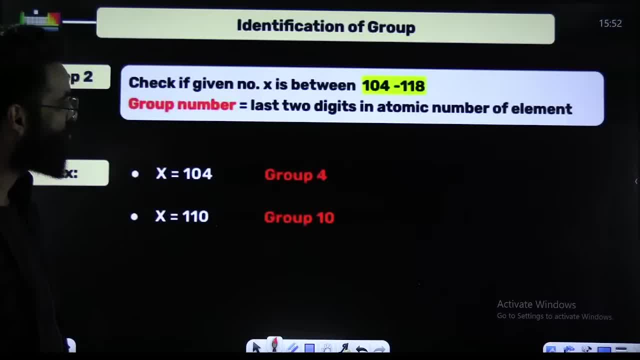 between 104 to 118. then check the last two digits in the atomic number, for example 110. check the last two digits, digits 10. so its group number is 10, 104. coming in between those two values, 104 to 118. last two digits, right group number four. isn't it easy, guys, isn't it easy. 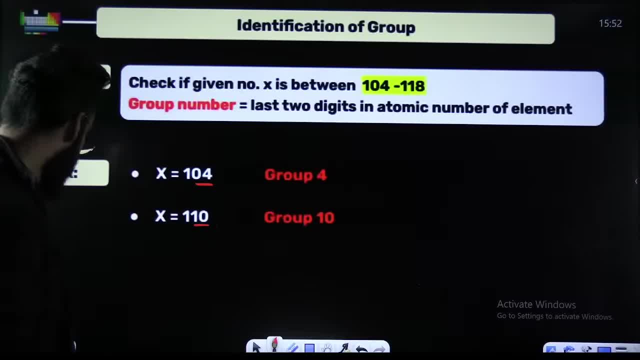 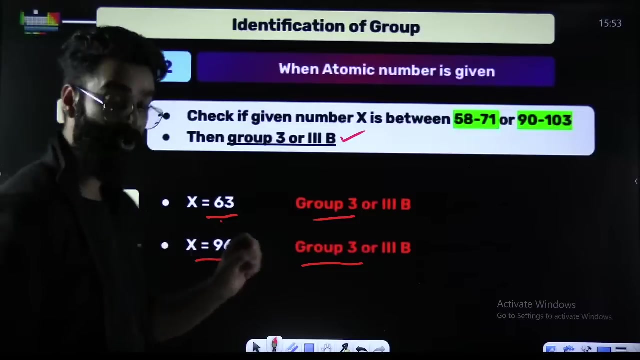 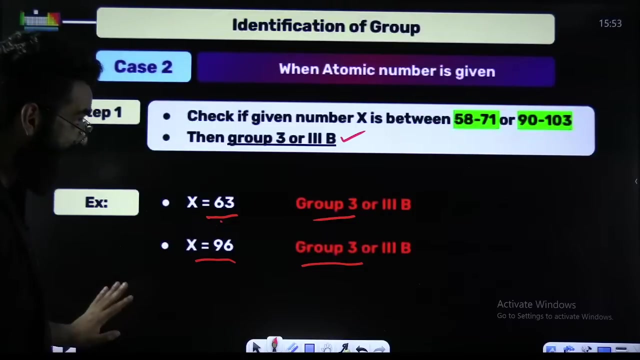 isn't it easy? okay, right now, guys, the first thing which i told you here, that was that was if the atomic number is between these two or between these two, group number directly is three, right, and if the atomic number given to, is given to us, is between: 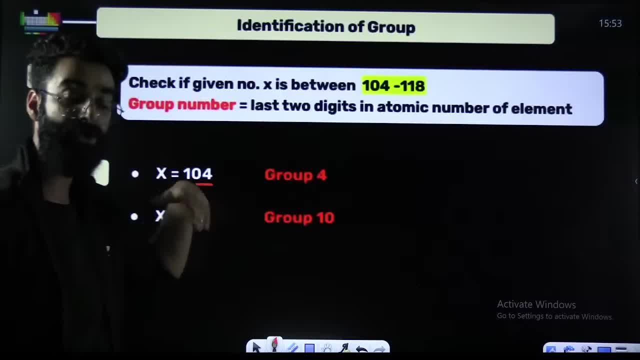 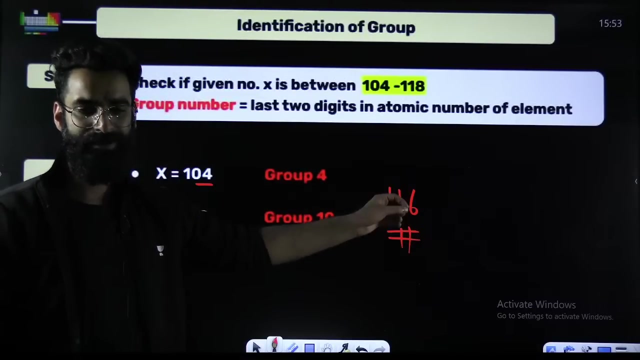 these two values. then last two: digit is the group number. what about all the other atomic numbers except these? what about all the other atomic numbers except these? okay, tell me one thing. tell me one thing: 116, atomic number, 116. tell me the group number quickly. it is not lying in between any two numbers which i gave you already right. so last two done. 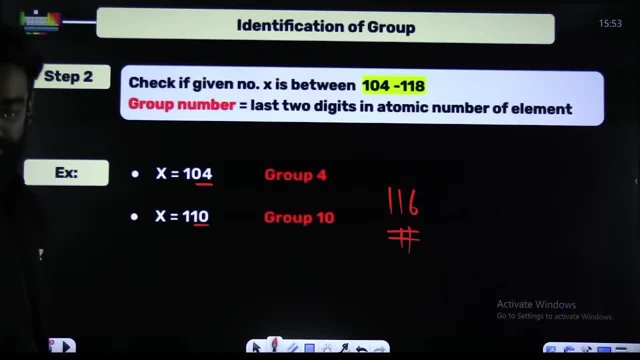 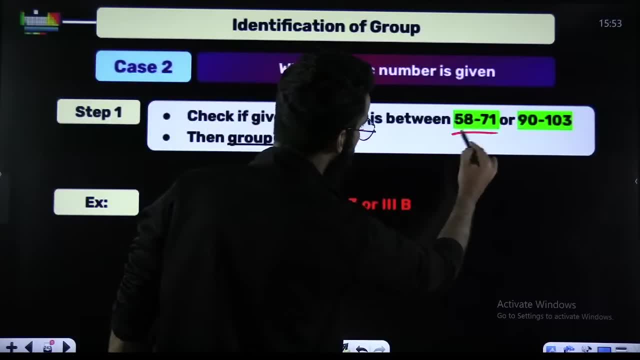 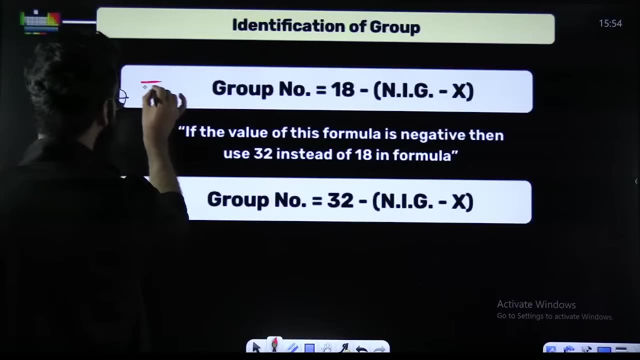 is that group number sixteen now, what about the other atomic numbers? now, what about the other atomic numbers? do not belong to this category, as well as which do not belong to what which do not belong to this particular category. what about them? what about them? what about them? their group number is calculated with the help of this. 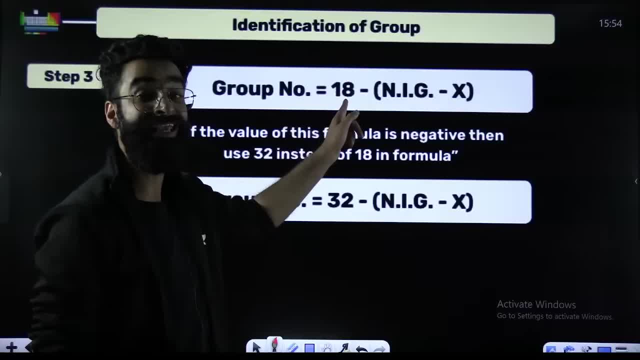 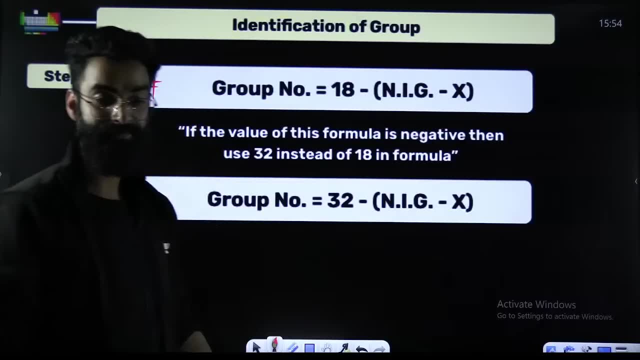 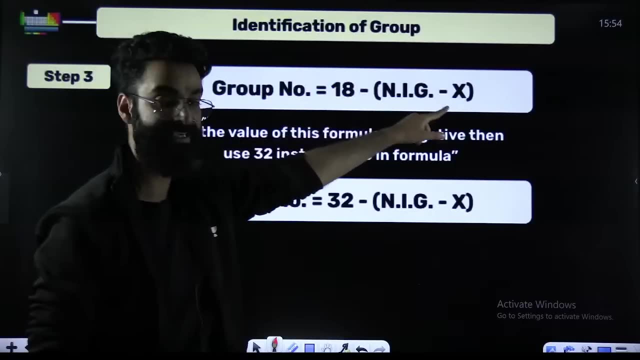 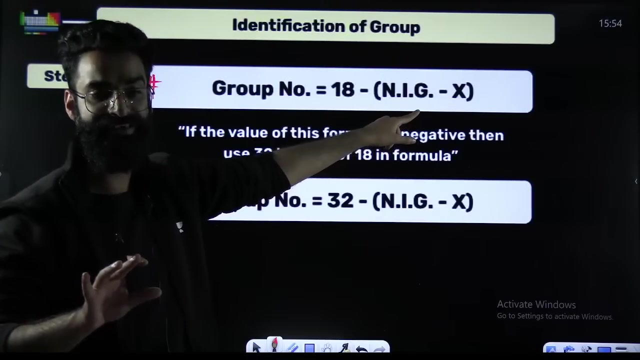 particular formula, group number is equal to 18 minus next inert gas number minus atomic number. what it means? what it means, let's have a look. let's have a look what it means. first remember this formula: 18 minus energy minus X, what is X? X is the given atomic number, X is a given atomic number, X is a given atomic. 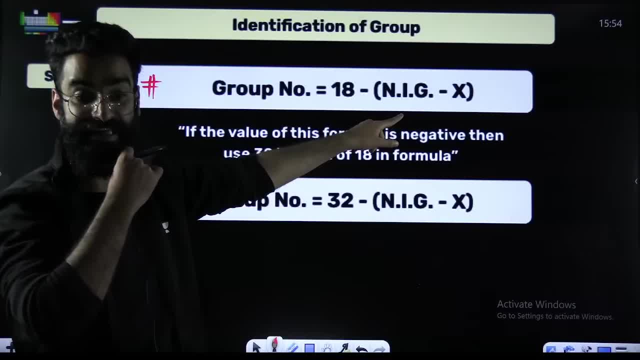 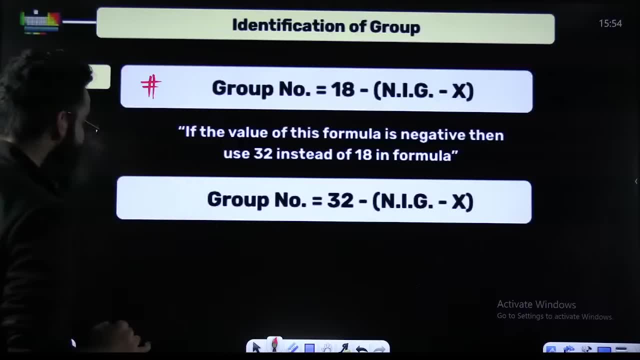 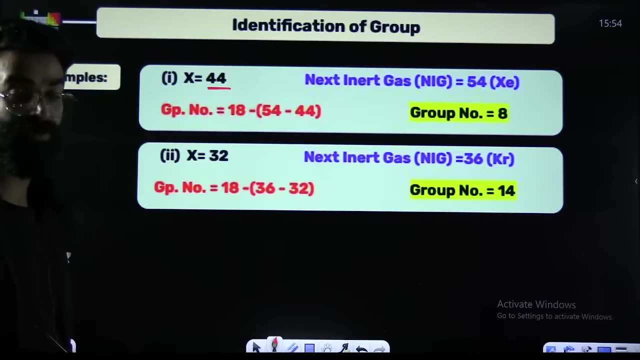 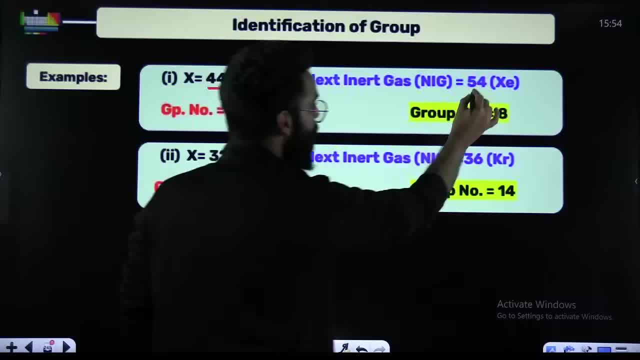 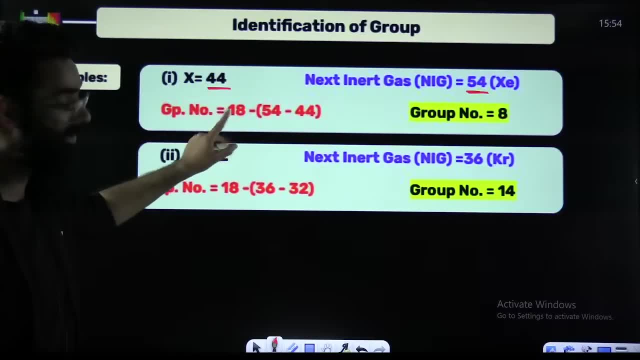 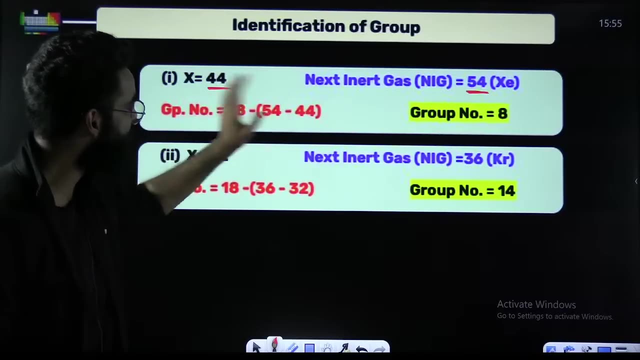 you, you? what is the next inert gas atomic number? that is 54. NIG values: 54. X is 44, NIG is 54, right? so put it in this formula: 18 minus 18 minus 54, 18 minus energy minus X, the value comes out. we have what value comes out: be 8. so it's. 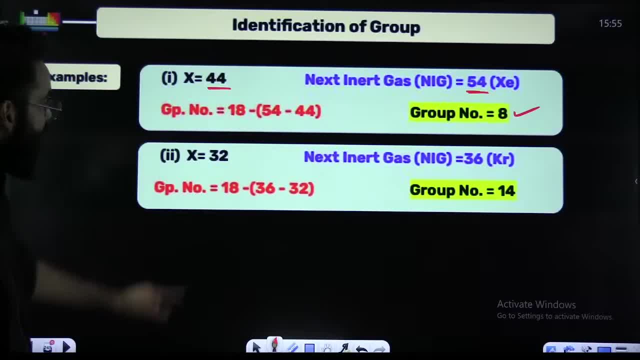 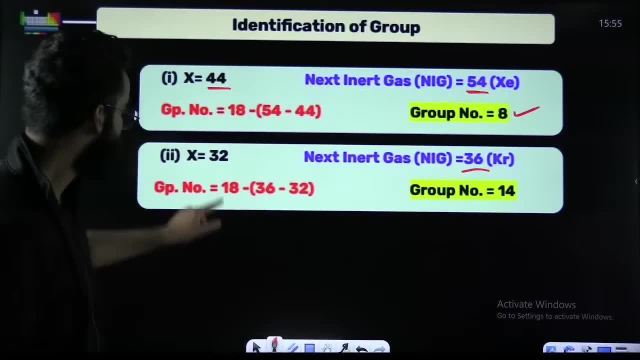 group number is 8, so group number is 8. if X is 32, for example, if X is 32, what is the next inert gas number? next inert gas number: NIG is 36, right, so it is 18. minus energy, minus X, right value comes out: be value. 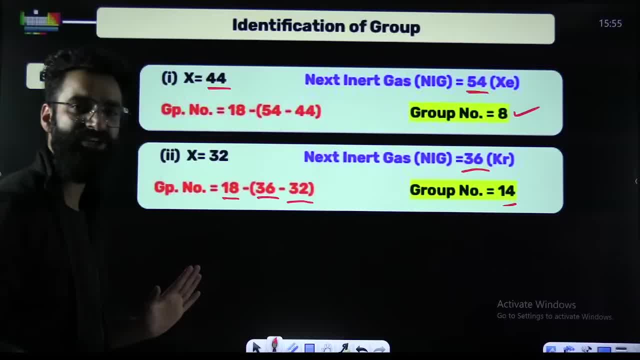 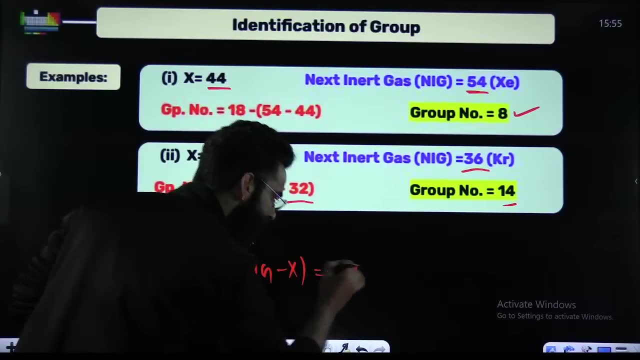 comes out be 14 and, by chance, by chance, by chance, if you are given with some number- X- right, you identified energy also- then you use this formula. then you use this formula: 18 minus NIG minus X. if this value comes out, be negative. if this: 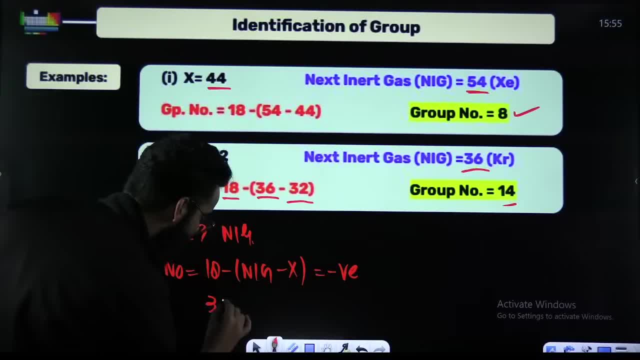 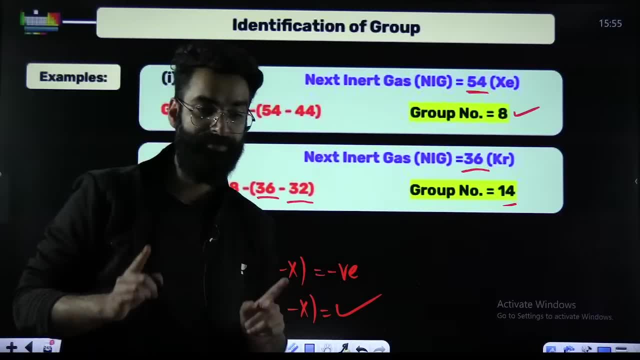 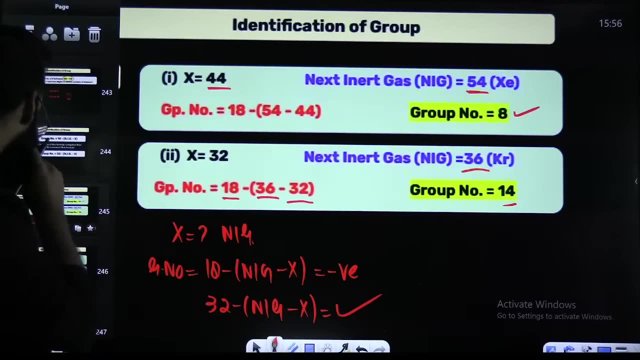 value comes out negative, then change the formula in stop 18 right 32 instead of 18 right 32. this will give the correct result. I hope you are getting what I'm trying to say. I hope you are getting what I'm trying to say. I hope you are getting what I'm trying to say. yes, 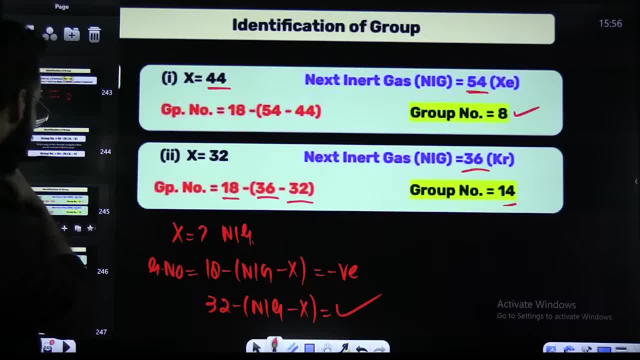 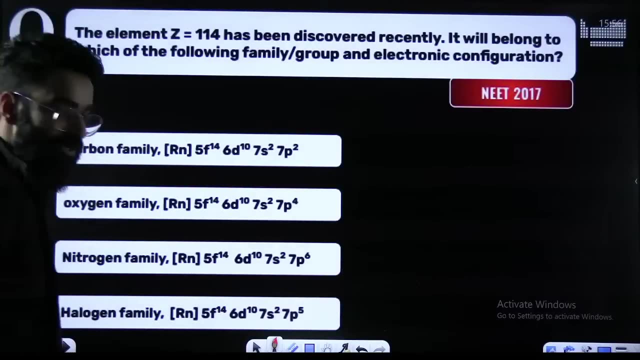 am I clear? people am I clear? you Am I clear? Am I clear? Tell me the answer of this question. Element with atomic number 114 has been discovered recently. It will belong to which of the following? family group and electronic configuration. Family group- electronic configuration. 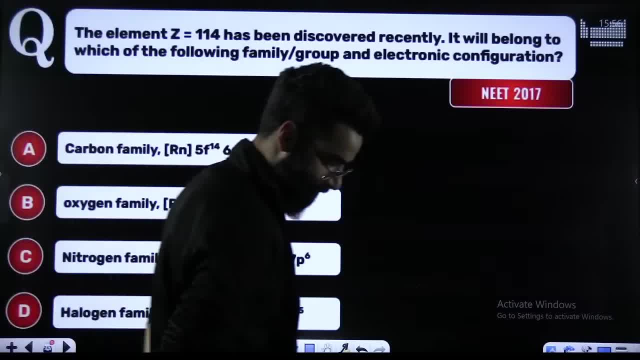 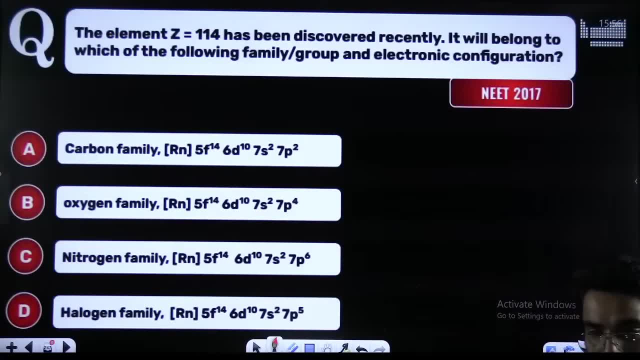 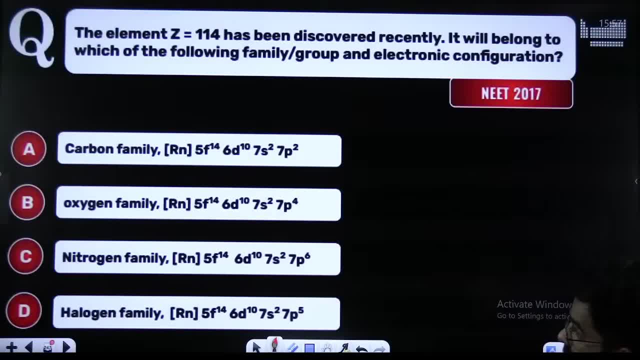 I need the logic. Did you use any formula? Did you use any formula? 114.. Last two digits: 114.. Which group? Which group? Group 14. Group 14. Which family? is that Carbon family? There is only one option, which is saying carbon family. 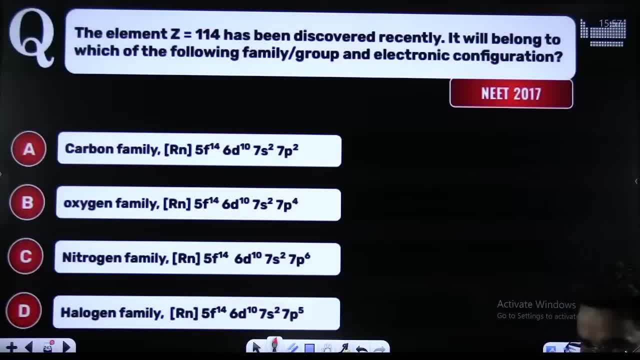 That's option A. Did you know this trick before? Did you know all these tricks before? Honestly, you can say yes or no. Accordingly, you can get the period group block, whatever. Even I struggled to do these questions when I was preparing for my JEE back in 2013, because 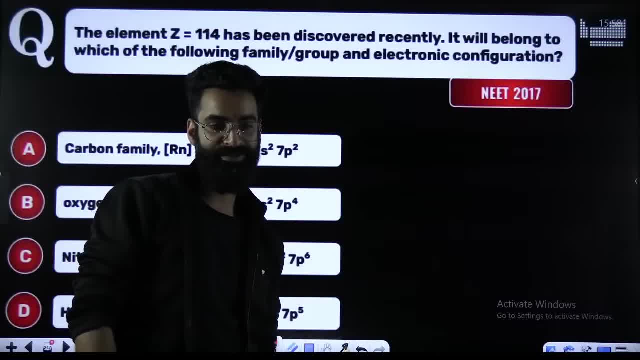 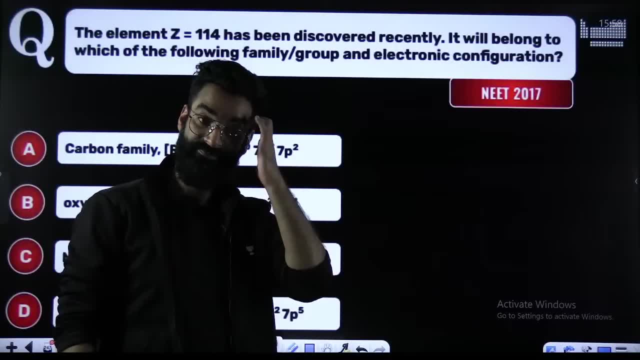 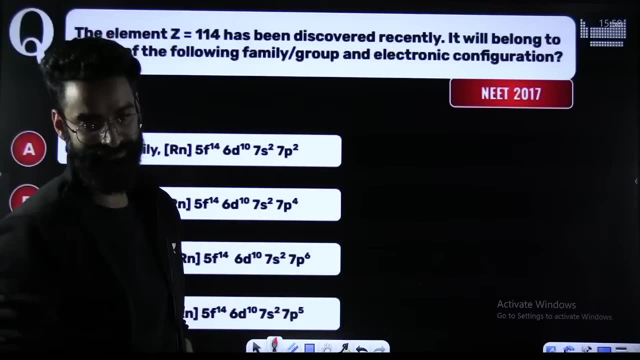 I did not knew. I did not know these things. Honestly, I'm saying, and I had to, for that I had to. I mean I had to remember the entire period table. That was a mess. But if you know all these things, you are not supposed to remember the period table. 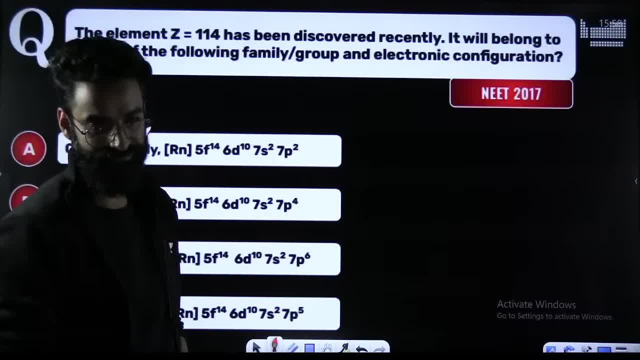 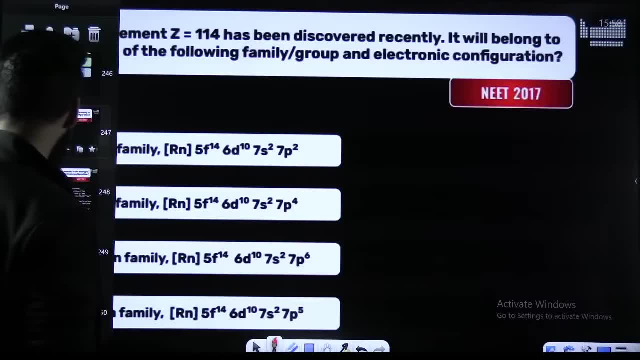 at all. Yeah, Done and dusted. Okay, one more question, Tell me. Tell me the answer Quickly. Okay, I have two questions. One is a question about the period table. What is the period table? Period table. 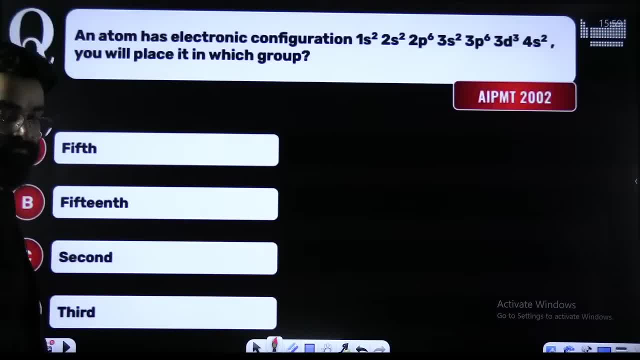 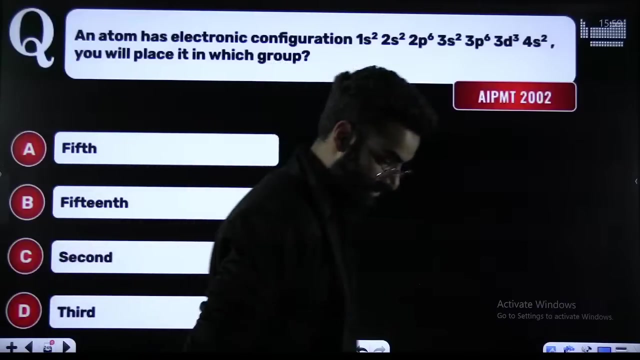 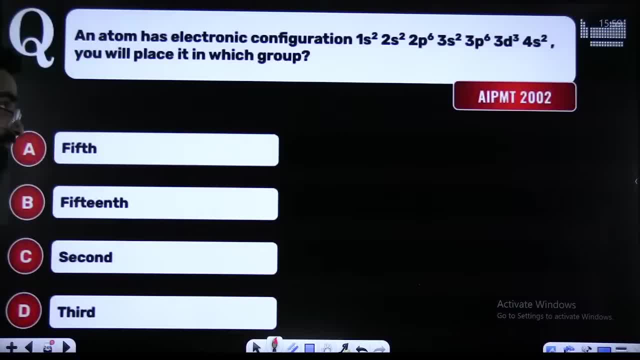 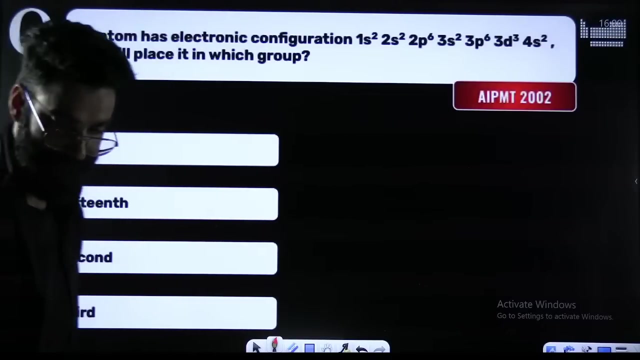 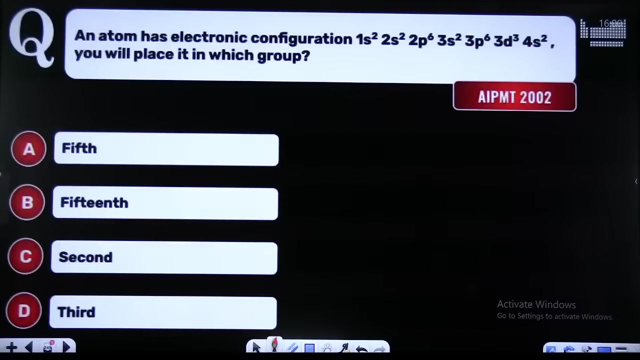 configuration. first of all, you need to identify which block it belongs to, which block it belongs to, and once you identify which block, which block it belongs to, then easily you can do it. what is the correct answer? just a second, guys: you need to close down one light. 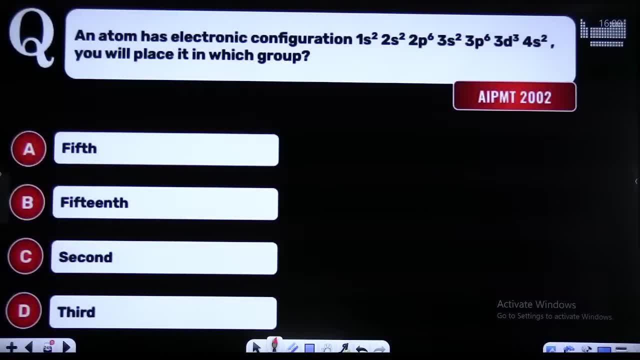 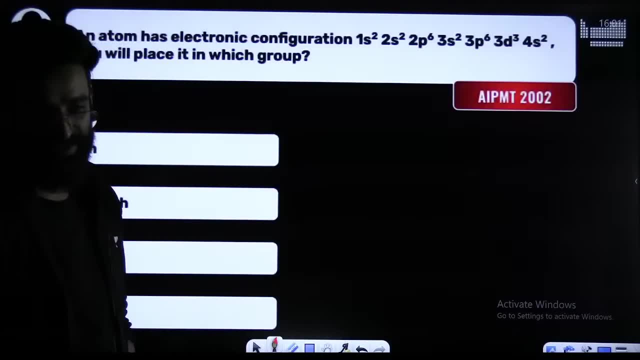 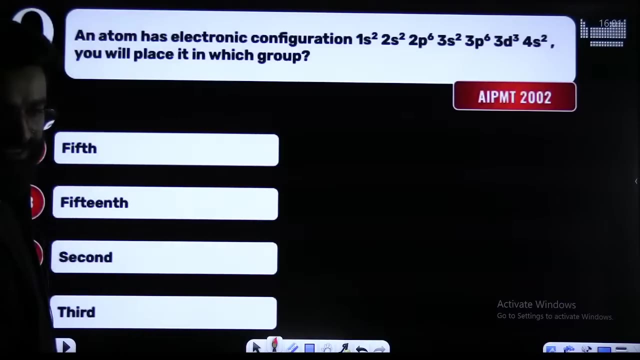 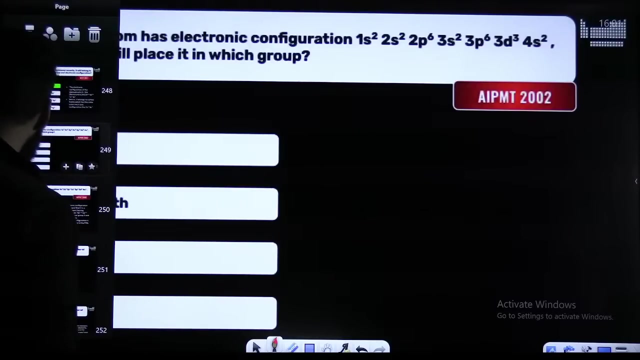 i don't know what happened to electricity since morning. since morning i'm teaching with the help of ups. absolutely, it's the fifth group, right, it's the. it's the fifth group, and next group is the fourth group and next group is the fifth group. ns plus n minus 1d. ns plus n minus 1d, right, okay. 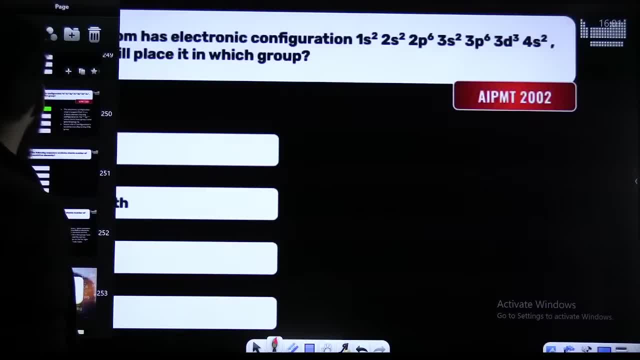 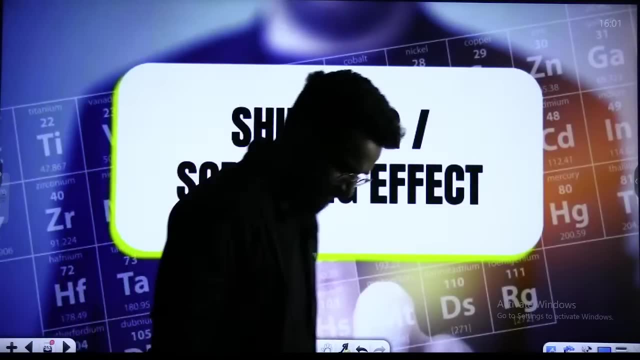 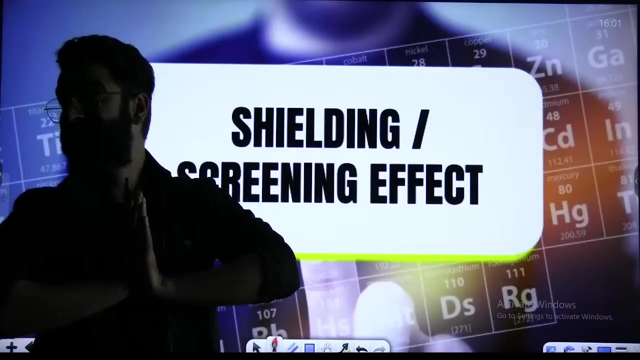 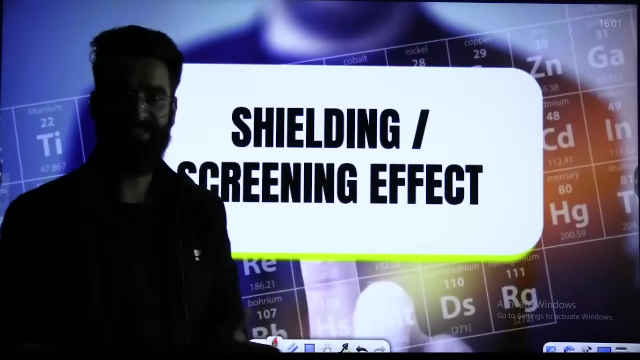 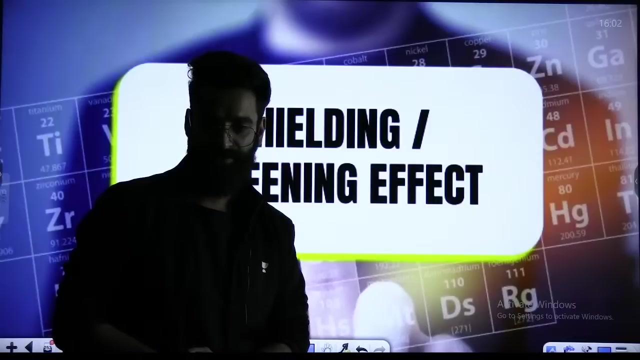 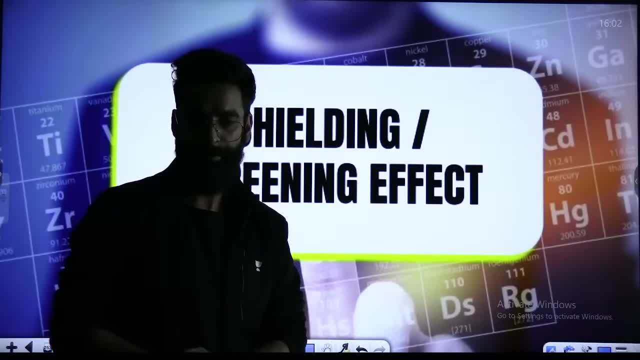 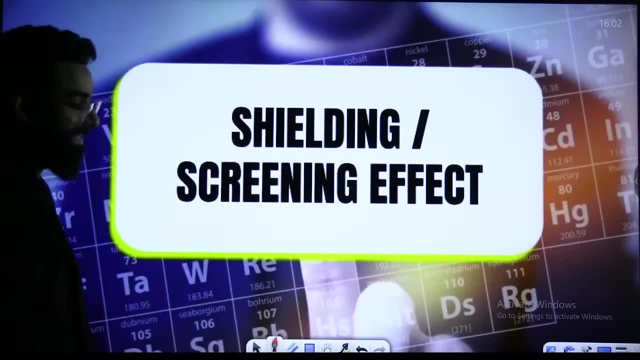 which will help us out in order, which will help us out in order to solve the equations, to solve the equations, to solve the equations. okay, okay, okay. what is the shielding effect? what is the shielding effect? what is the shielding effect, my dear students, as per the definition? 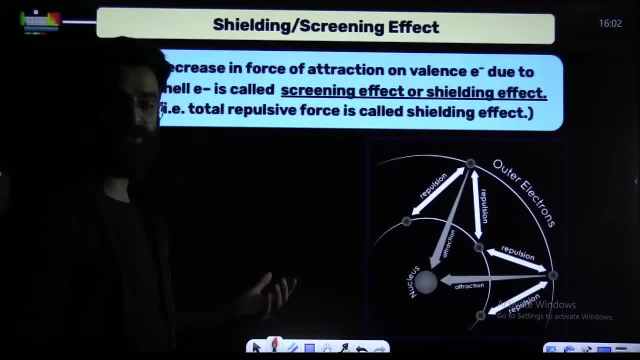 my dear students, as per the definition. my dear students, as per the definition. one of its definition. the decrease in the one of its definition. the decrease in the one of its definition. the decrease in the force of attraction. the decrease in force of attraction, the decrease in the. 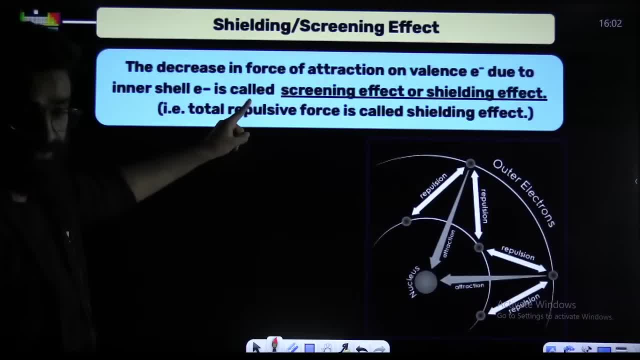 force of attraction. the decrease in the force of attraction on the valence. force of attraction on the valence. force of attraction on the valence electron- electron, electron. the decrease in the force of attraction, the. the decrease in the force of attraction on the valence electron. 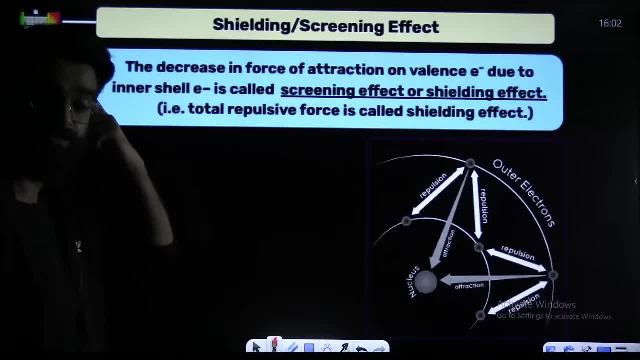 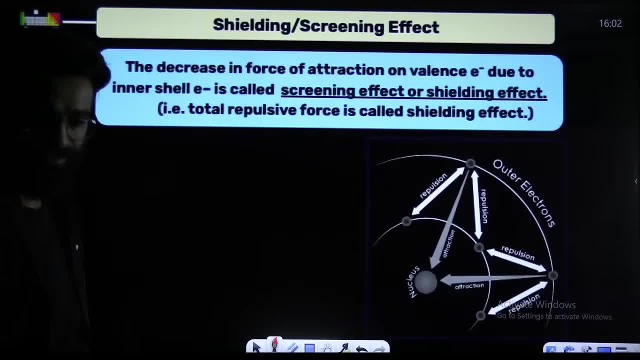 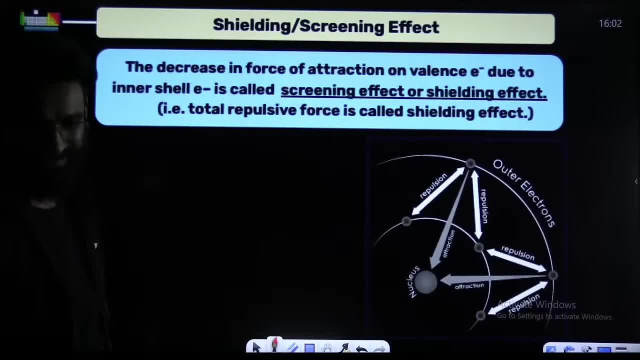 do you want to go for the slater's? do you want to go for the slater's rules, etc, etc. you do not have to study rules, etc, etc. you do not have to study rules, etc, etc. you do not have to study that, that, that. why do you want to go for that? 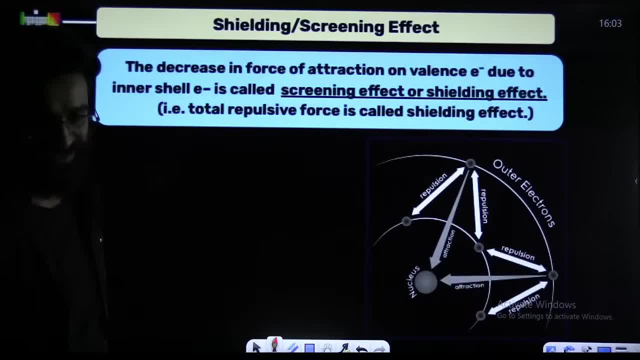 why do you want to go for that? why do you want to go for that? guys, guys, guys. whatever i'm teaching you, just whatever i'm teaching you, just whatever i'm teaching you, just keep this in your brain, keep this in your brain, keep this in your brain, right? 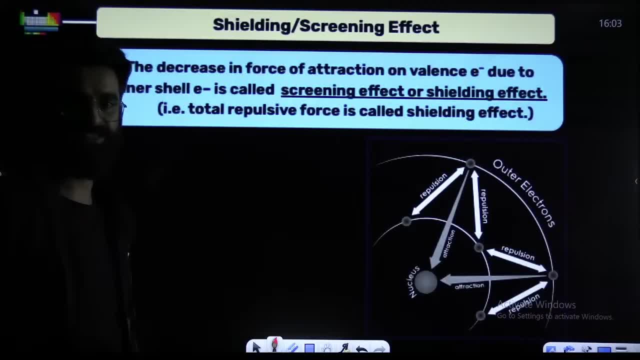 right, right. we do not need to remember the. we do not need to remember the. we do not need to remember the irrelevant things which are not asked. no irrelevant stuff. no irrelevant stuff, all right, all right, all right. have a look on what the shielding effect. have a look on what the shielding effect. 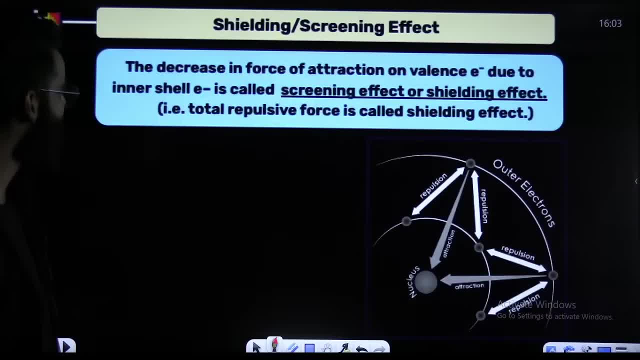 have a look on what the shielding effect is all about. the decrease in the force of is all about. the decrease in the force of is all about the decrease in the force of attraction on the valence electron. due attraction on the valence electron, due attraction on the valence electron due to the inertial electrons is called a. 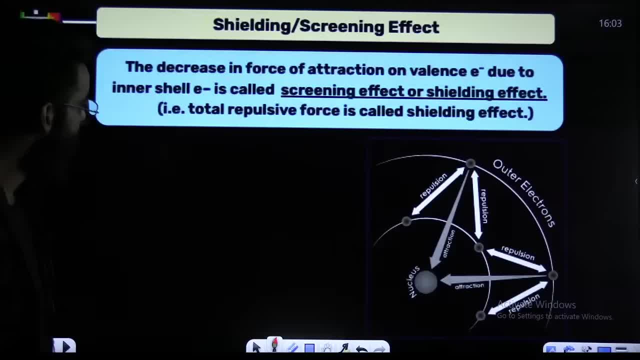 to the inertial electrons is called a to the inertial electrons is called a screening effect or shielding effect. screening effect or shielding effect. screening effect- right right, right. see see what it means, for example. see see what it means, for example. see see what it means, for example, for example: this is the nucleus. 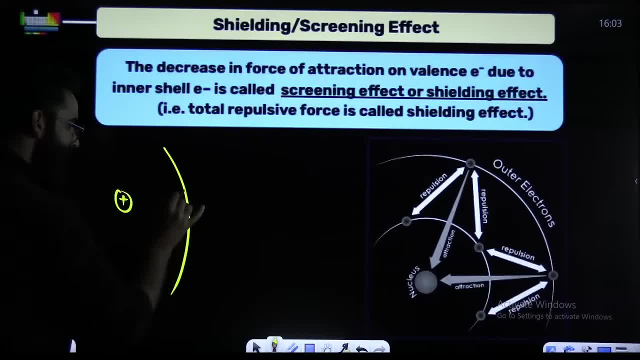 for example, this is the nucleus. for example, this is the nucleus. let's say: this is the nucleus perfect. let's say: this is the nucleus perfect. let's say: this is the nucleus perfect. electron which i'm taking into, electron which i'm taking into, electron which i'm taking into consideration. 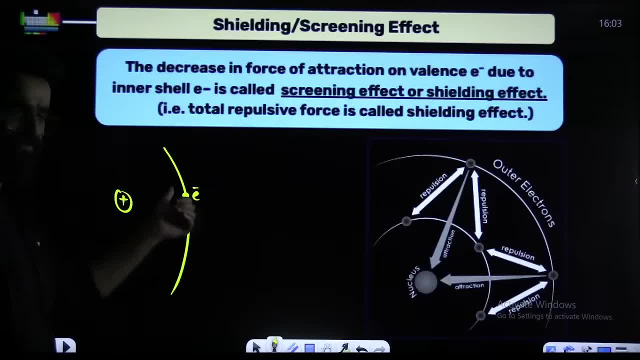 consideration, consideration. okay, this is the electron which i'm taking into. this is the electron which i'm taking into. this is the electron which i'm taking into consideration. consideration, consideration. now, my dear students, now my dear students, now, my dear students, this nucleus contains positive charge. this nucleus contains positive charge. 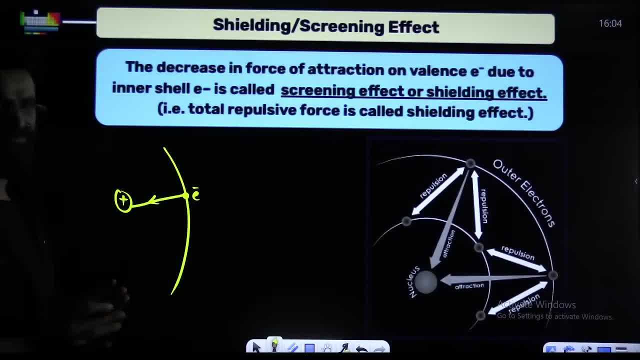 this nucleus contains positive charge. i'll say this nucleus will be holding. i'll say this nucleus will be holding. i'll say this nucleus will be holding this electron firmly, this electron firmly, this electron firmly. this nucleus will be holding this. this nucleus will be holding this. this nucleus will be holding this electron nucleus is positive electrons. 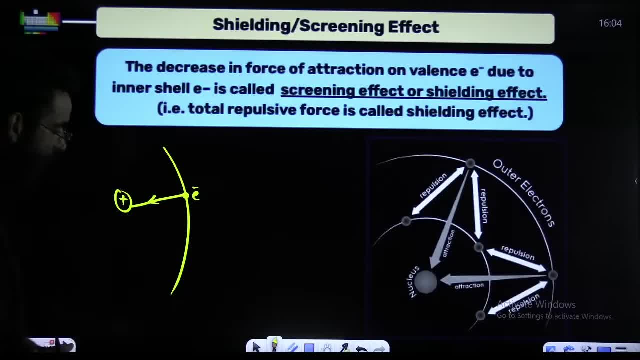 electron nucleus is positive electrons. electron nucleus is positive electrons, negative, negative, negative, right right, right now, now, now. this is my electron which is taken into. this is my electron which is taken into, this is my electron which is taken into consideration. consideration. consideration, perfect. imagine there are z protons here. 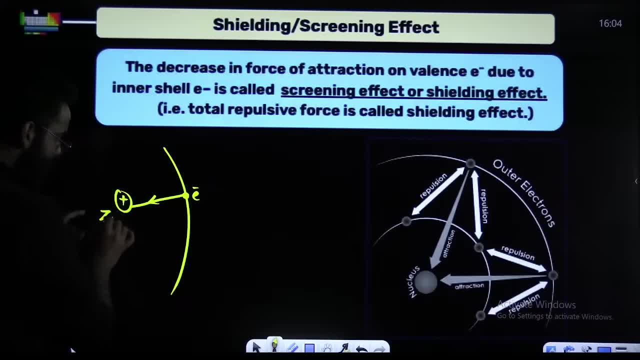 perfect imagine there are z protons here. perfect imagine there are z protons here inside the nucleus. so all these z inside the nucleus, so all these z inside the nucleus, so all these z protons, all these z protons, protons, all these z protons, they are all these z protons. 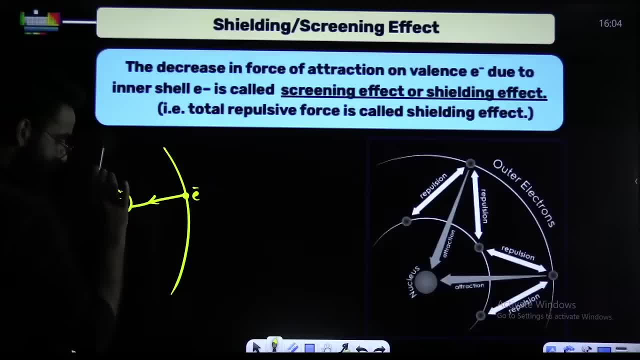 protons. they are all these z protons, protons. they are all these z protons, right? they are attracting this right. they are attracting this right. they are attracting this particular electron towards itself, particular electron towards itself, particular electron towards itself. correct, with the force of attraction z. 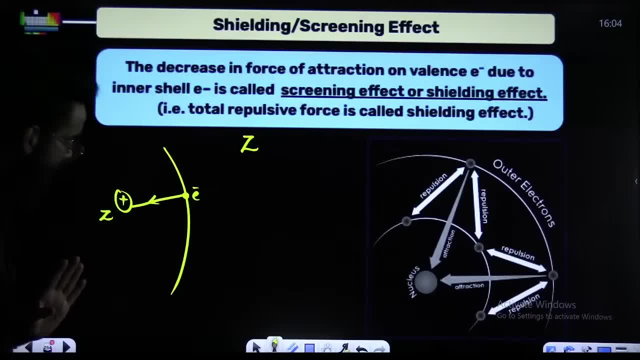 correct with the force of attraction: z. correct with the force of attraction: z with the force of attraction, for example, with the force of attraction. for example, with the force of attraction, for example, z. just to make you understand. correct with the force of attraction, for example, z. just to make you understand. 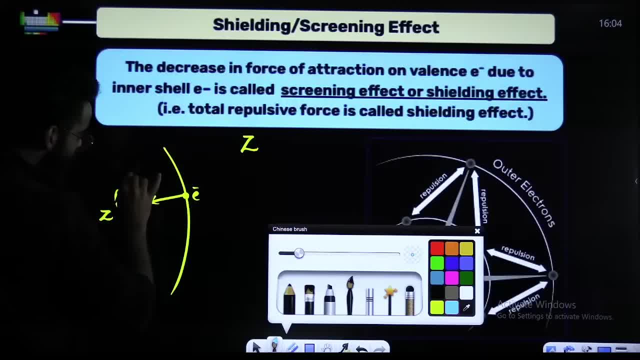 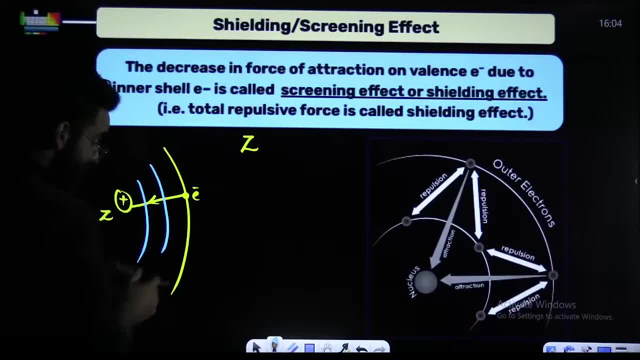 inertials as well. if there are inertials as well if there are inertials if there are inertials. inertials if there are inertials if there are inertials. inertials if there are inertials if there are inertials if, when there were no inertials. 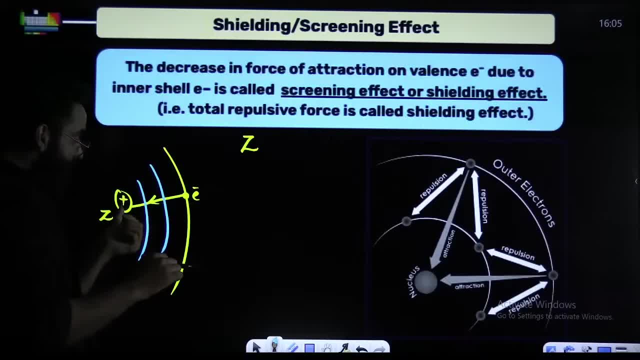 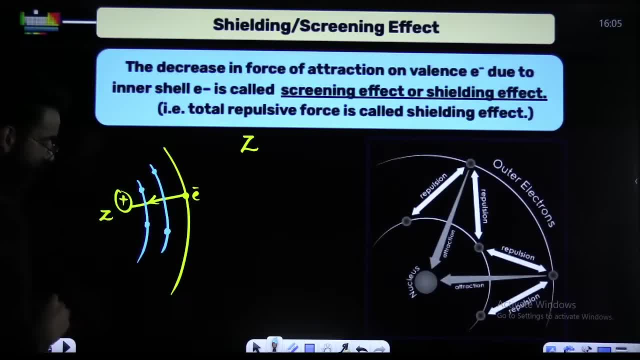 now, if there are, let's say, inertial? now, if there are, let's say, inertial- electrons, electrons, electrons, what will happen? what will happen now? what will happen? what will happen now? what will happen what will happen now? this nucleus has got a lot of other work. this nucleus has got a lot of other work. this nucleus has got a lot of other work to do. it has to attract this one also. it to do. it has to attract this one also. it to do. it has to attract this one also. it has to attract this one also. it has to. 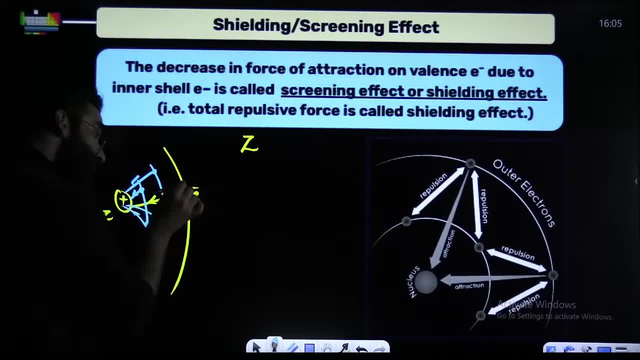 has to attract this one also. it has to has to attract this one also. it has to attract this one also. attract this one also. attract this one also. now the same electron. is it going to now the same electron? is it going to now the same electron? is it going to experience the same attraction which it? 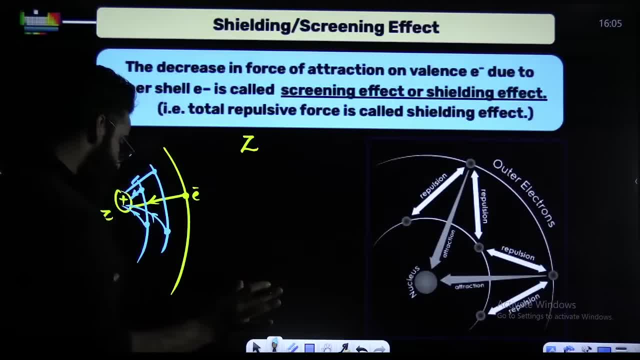 experience the same attraction, which it experience, the same attraction which it was experiencing before, was experiencing before, was experiencing before. no, no, no, no, no, no. now, nucleus, it has got other work to do now. nucleus, it has got other work to do now. nucleus, it has got other work to do as well. number one, number two, number two. 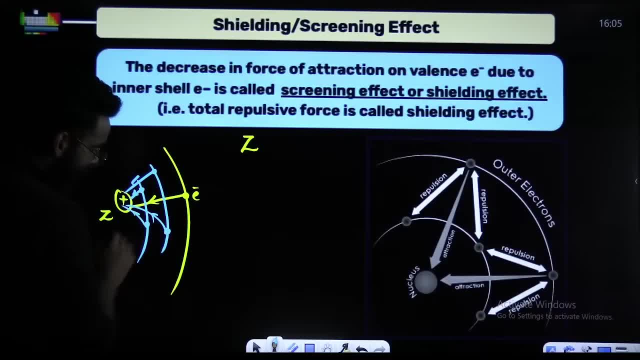 as well. number one, number two, number two as well, number one, number two, number two. just to make you understand number two, just to make you understand number two, just to make you understand number two, when you are putting the, when you are putting the, when you are putting the inertial electrons, can i say these: 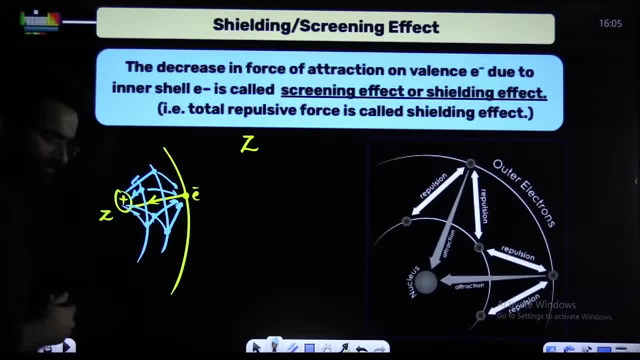 inertial electrons. can i say these inertial electrons, can i say these inertial electrons will be repelling inertial electrons will be repelling inertial electrons will be repelling this particular electron as well, this particular electron as well, this particular electron as well. so what is happening? due to the inertial 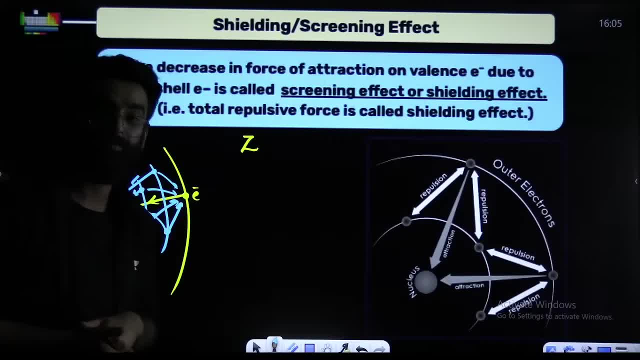 so what is happening due to the inertial? so what is happening due to the inertial electron? the force experience the force electron, the force experience the force electron, the force experience, the force experienced by the outermost electron, experienced by the outermost electron, experienced by the outermost electron. does it increase or decrease? 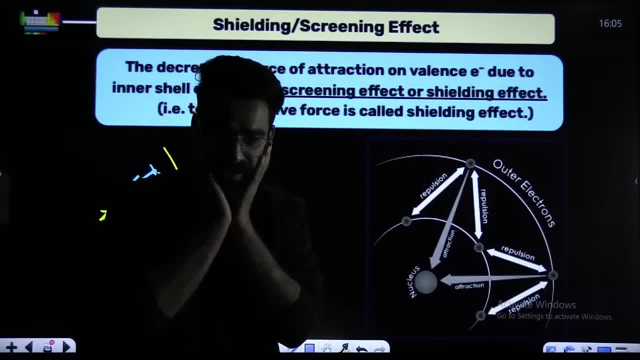 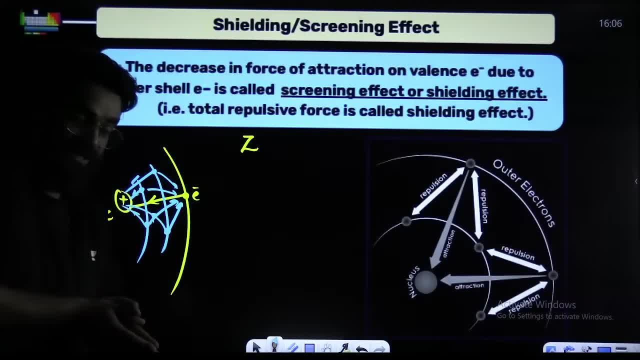 by the outermost electron. does it increase? by the outermost electron. does it increase or decrease? it decreases or decrease. it decreases or decrease. it decreases due to the inertial electrons. due to the inertial electrons. due to the inertial electrons, due to the repulsions caused by the. 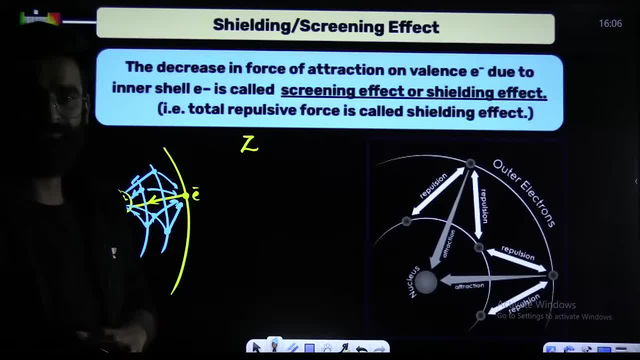 due to the inertial electrons caused by the. due to the inertial electrons caused by the inertial electrons, inertial electrons, inertial electrons, and this decrease in the force of, and this decrease in the force of, and this decrease in the force of attraction, attraction, attraction. this decrease in the force of attraction. 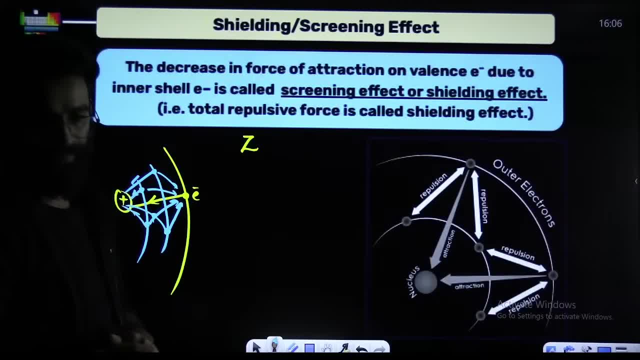 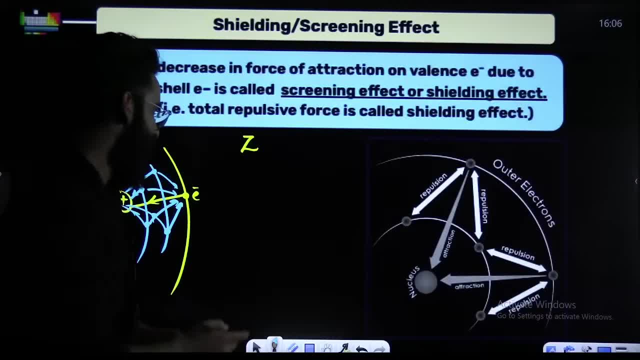 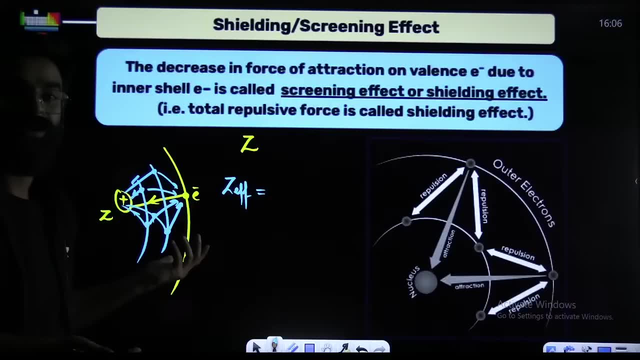 shielding effect. shielding effect: right, perfect, right, perfect, right, perfect. so if i ask you about the effective, so if i ask you about the effective, so if i ask you about the effective nuclear charge, nuclear charge, nuclear charge, effective nuclear charge, effective nuclear charge, effective nuclear charge, effectively now, 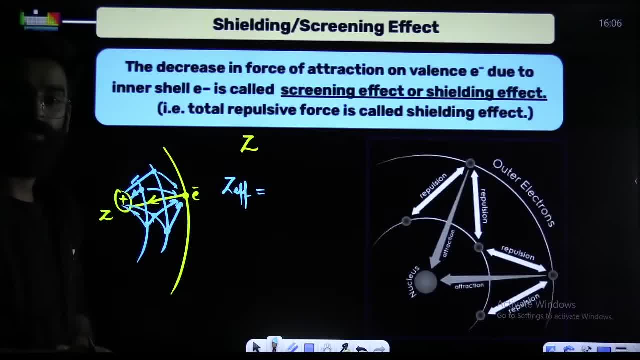 effectively now. effectively now, what will be the nuclear charge? is it what will be the nuclear charge? is it what will be the nuclear charge? is it going to be same z, going to be same z, going to be same z, or you'll be subtracting something you'll. 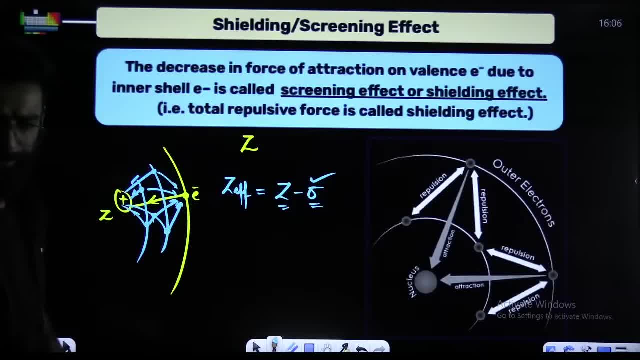 or you'll be subtracting something. you'll or you'll be subtracting something. you'll be subtracting something. signal- be subtracting something. signal- be subtracting something. signal- right, no, redox reaction will be taken, right? no, redox reaction will be taken, right no, redox reaction will be taken in the physical chemistry, class 11. 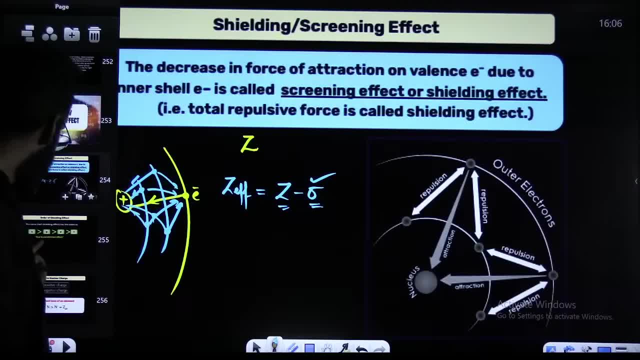 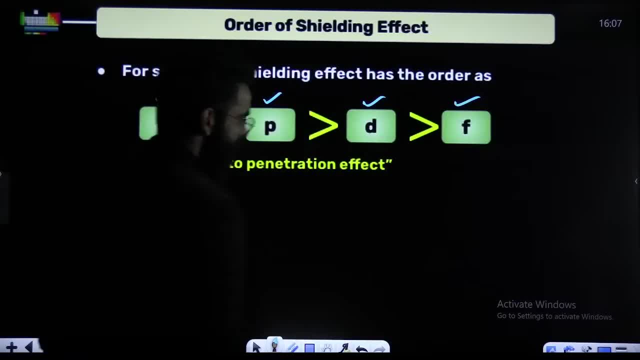 in the physical chemistry, class 11. in the physical chemistry, class 11: marathon okay, marathon okay, marathon okay, perfect. now people do remember: s shows maximum shielding, then p, then d? s shows maximum shielding, then p, then d? s shows maximum shielding, then p, then d, then f. this is something which i believe. 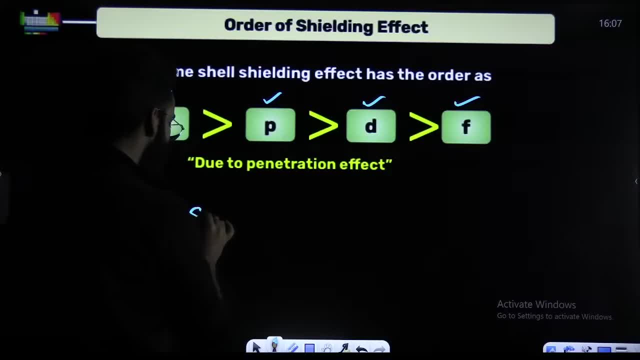 then f this is something which i believe, then f? this is something which i believe every one of you would be knowing, even s every one of you would be knowing, even s every one of you would be knowing even s has more penetrating power. has more penetrating power. 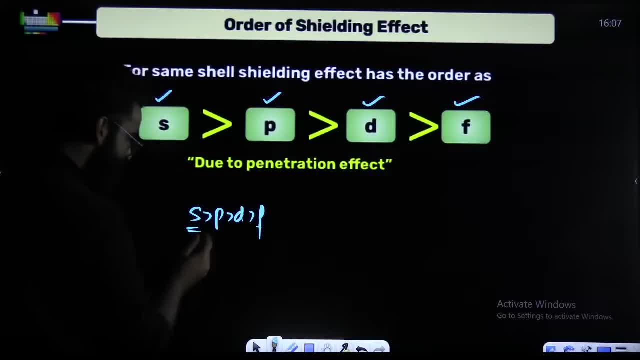 has more penetrating power. then p, then d, then f. why is that? because then p, then d, then f. why is that because, then p, then d, then f. why is that? because s is closest to the nucleus, followed by s is closest to the nucleus, followed by s is closest to the nucleus, followed by p, followed by d, followed by f. 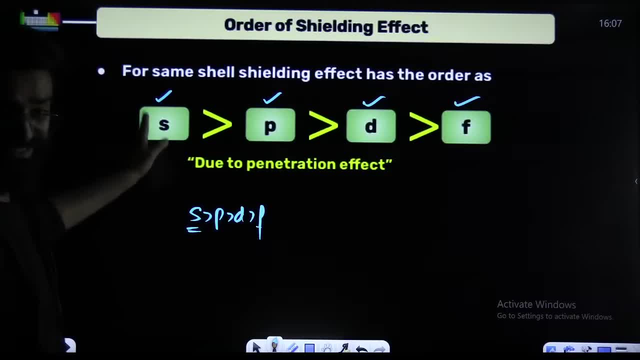 p, followed by d, followed by f p, followed by d, followed by f. right, this is something which i believe right. this is something which i believe right. this is something which i believe you all would be knowing already. you all would be knowing already, you all would be knowing already s maximum shielding, followed by p. 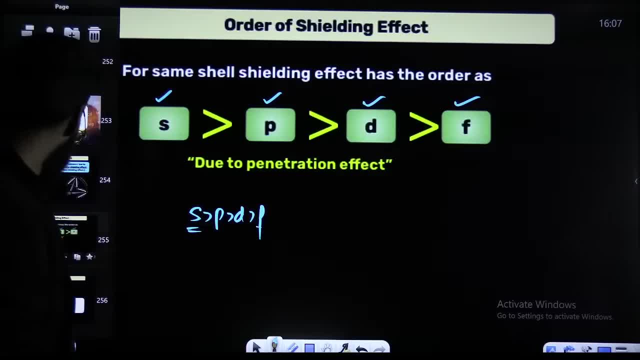 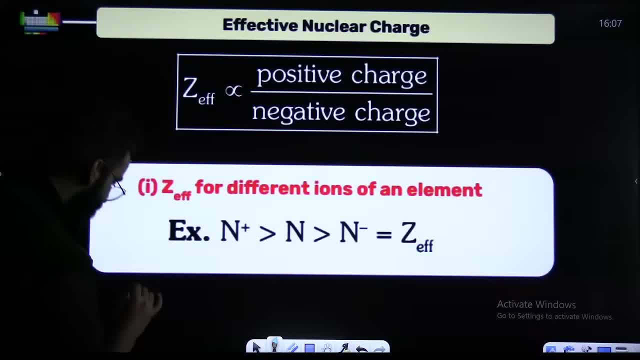 now tell me one thing: i have taken n positive, n and n. i have taken n positive, n and n. i have taken n positive n and n negative, negative, negative. i have taken n positive. i have taken n positive n. i have taken n positive n. i have taken n positive n and n negative. 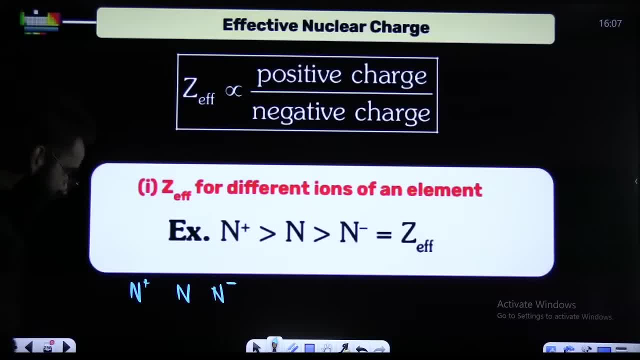 and n negative and n negative. these are the species which i have. these are the species which i have. these are the species which i have. understand carefully what i'll say. understand carefully what i'll say. understand carefully what i'll say. in case of nitrogen, there are seven. 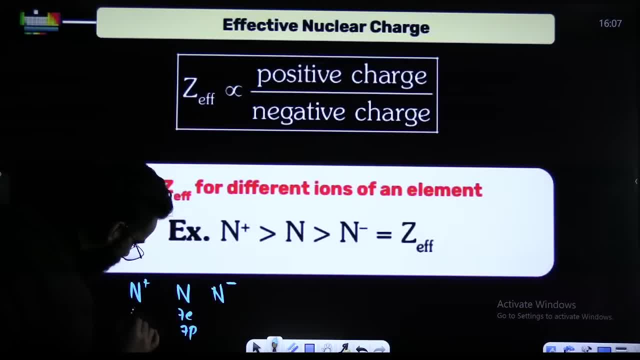 in case of nitrogen, there are seven. in case of nitrogen, there are seven electrons, seven protons electrons. here you have got seven protons, but here you have got seven protons. but here you have got seven protons, but only six electrons. here you have got only six electrons. here you have got. 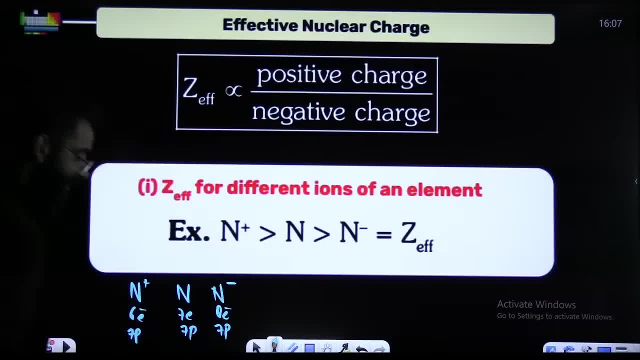 only six electrons here. you have got uh seven protons but eight electrons. uh seven protons but eight electrons. uh seven protons but eight electrons but eight electrons, if you look carefully. but eight electrons, if you look carefully, but eight electrons if you look carefully. if you look carefully in this particular 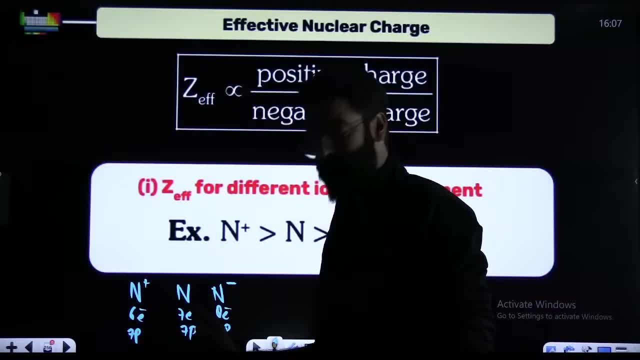 if you look carefully in this particular, if you look carefully in this particular case, case, case: seven protons. they are holding seven, seven protons. they are holding seven, seven protons. they are holding seven electrons, electrons, electrons here. these seven protons now are not here. these seven protons now are not. 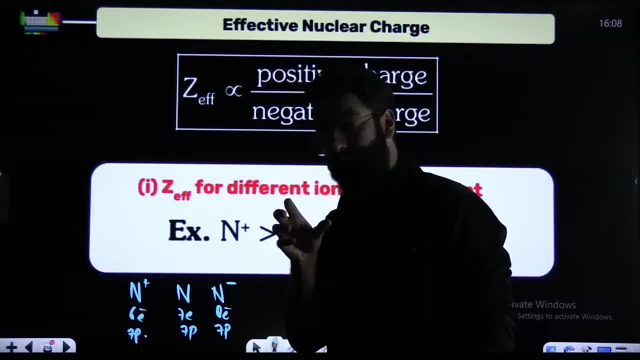 here, these seven protons now are not holding seven electrons. now they are holding seven electrons. now they are holding seven electrons. now they are holding only six electrons, holding only six electrons, holding only six electrons. so the force experienced by the outermost, so the force experienced by the outermost. 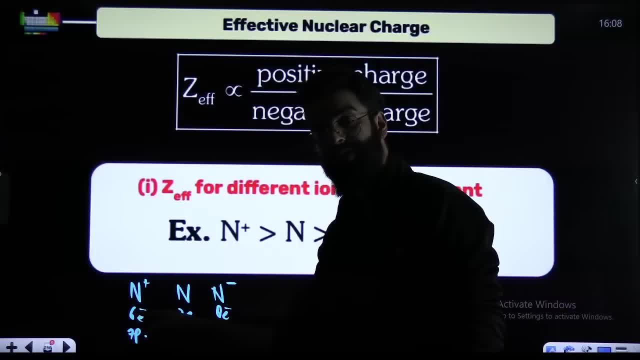 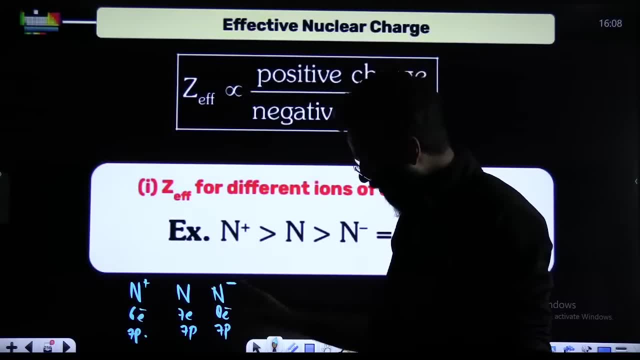 so the force experienced by the outermost electron: here will be comparatively more, electron here will be comparatively more electron, here will be comparatively more right, right, right, perfect, perfect, perfect. the force experienced by the outermost, the force experienced by the outermost, the force experienced by the outermost electron: here, that will be least, because 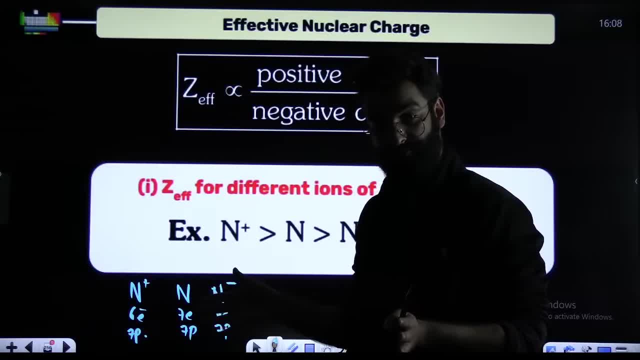 electron here, that will be least, because electron here, that will be least because seven protons are now holding eight. seven protons are now holding eight. seven protons are now holding eight electrons, electrons, electrons, which is completely difficult. you can which is completely difficult. you can, which is completely difficult. you can understand it like this: 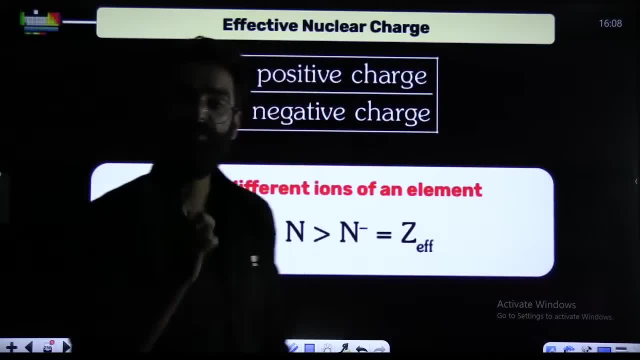 understand it like this, understand it like this. so what will be the effect in nuclear? so what will be the effect in nuclear. so what will be the effect in nuclear charge? where is the force of attraction charge? where is the force of attraction charge? where is the force of attraction experienced by the outer electron, the 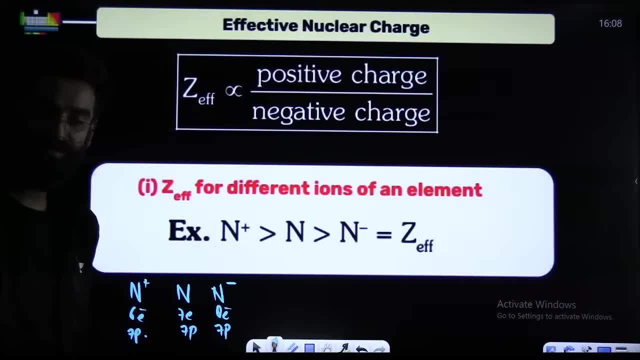 experienced by the outer electron. the experienced by the outer electron. the maximum maximum. maximum where, where, where, where there are lesser electrons, lesser where there are lesser electrons, lesser where there are lesser electrons, lesser number of electrons so that repulsions number of electrons, so that repulsions. 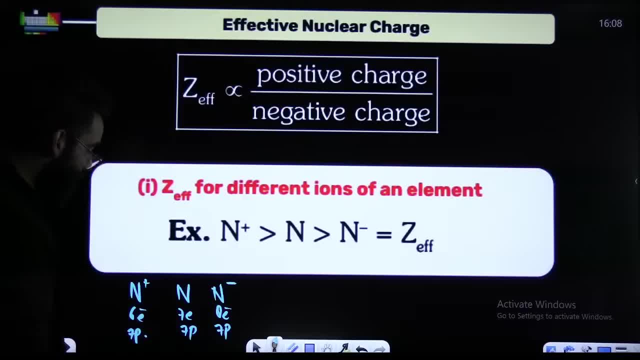 number of electrons so that repulsions are minimum, etc, etc. are minimum, etc, etc are minimum, etc, etc. perfect. so what is the effective nuclear? perfect. so what is the effective nuclear, perfect. so what is the effective nuclear? charge order, charge order, charge order. let me see if this is the effective. 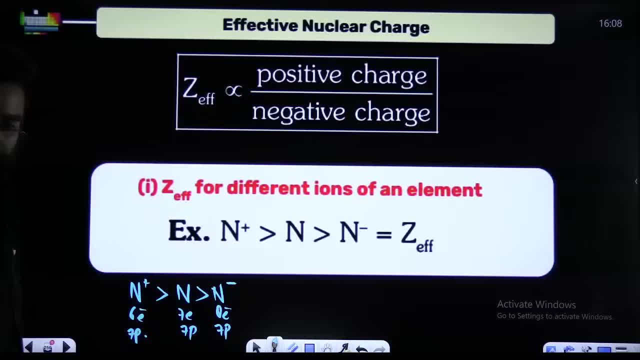 let me see if this is the effective. let me see if this is the effective nuclear charge order. i hope you got what i said. see, i hope you got what i said. see, i hope you got what i said. see, seven protons are holding seven electrons. seven protons are holding seven electrons. 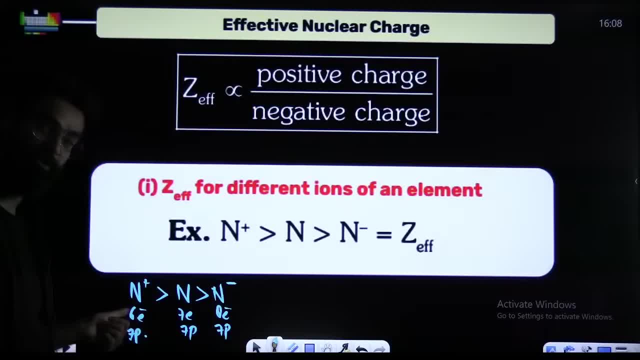 seven protons are holding seven electrons. seven protons here are holding only six. seven protons here are holding only six. seven protons here are holding only six electrons. that means force experienced by electrons. that means force experienced by electrons, that means force experienced by the outermost electron will be more. 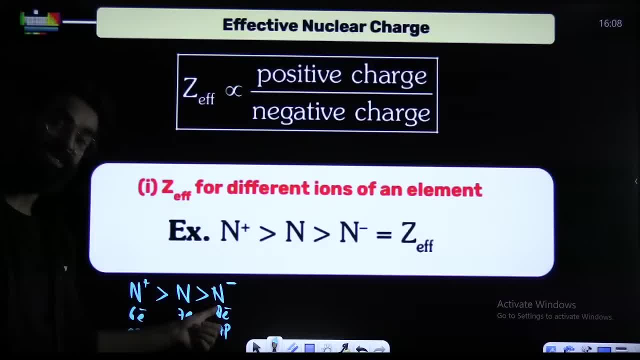 the outermost electron will be more. the outermost electron will be more. seven protons are holding eight. seven protons are holding eight. seven protons are holding eight electrons. force experienced by the electrons. force experienced by the electrons. force experienced by the outermost electron will be less. 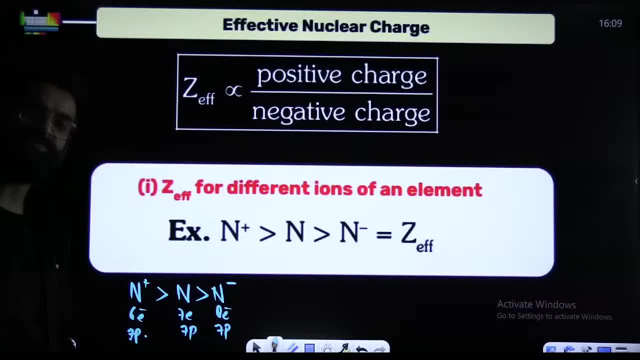 outermost electron will be less. outermost electron will be less comparatively, comparatively, comparatively right. more the force experienced by the right. more the force experienced by the right. more the force experienced by the outermost electron. more the z effective outermost electron, more the z effective outermost electron, more the z effective. so where is the z defective more. 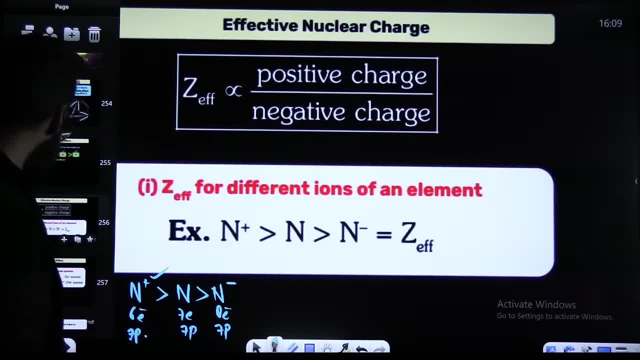 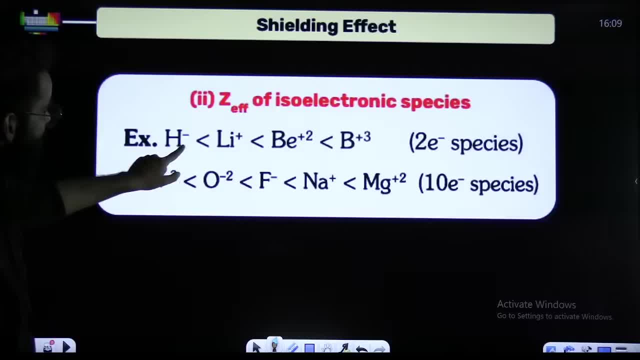 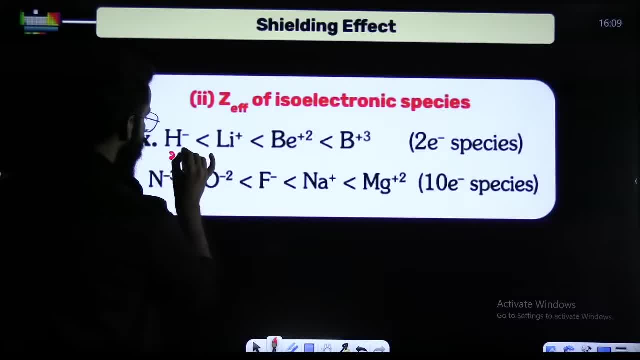 try positive are, try positive, are all all of them. they have got same number, all all of them. they have got same number, all all of them. they have got same number of electrons. two electrons here of electrons. two electrons here of electrons. two electrons here, two electrons here, right, 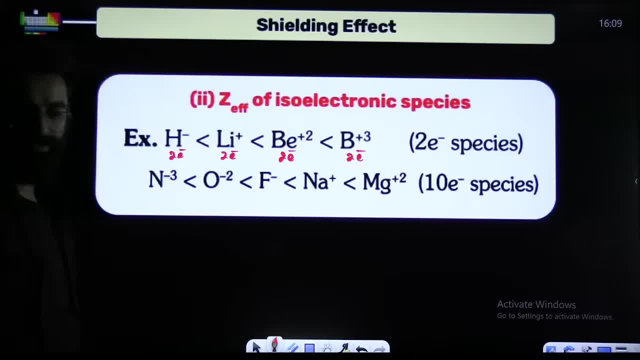 two electrons here, right, two electrons here, right, two electrons here, two electrons here, two electrons here and two electrons here isoelectronic and two electrons here isoelectronic and two electrons here isoelectronic. isoelectron, they've got same electrons. isoelectron, they've got same electrons. 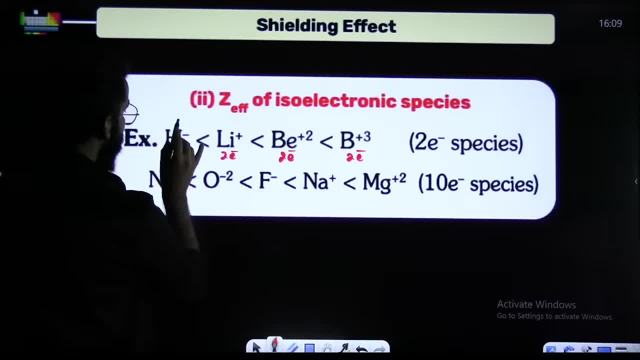 isoelectron. they've got same electrons: perfect. but what about protons? perfect. but what about protons? perfect, but what about protons? hydrogen? its atomic number is one right hydrogen: its atomic number is one right hydrogen: its atomic number is one right one proton, one proton. 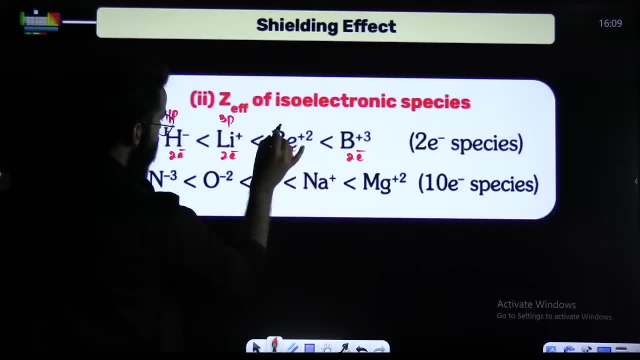 one proton. lithium- hydrogen lithium. its atomic lithium- hydrogen lithium. its atomic lithium- hydrogen lithium. its atomic number is three. three protons number is three. three protons. number is three, three protons, four protons, five protons, four protons, five protons, four protons, five protons over. in the last case, five protons are. 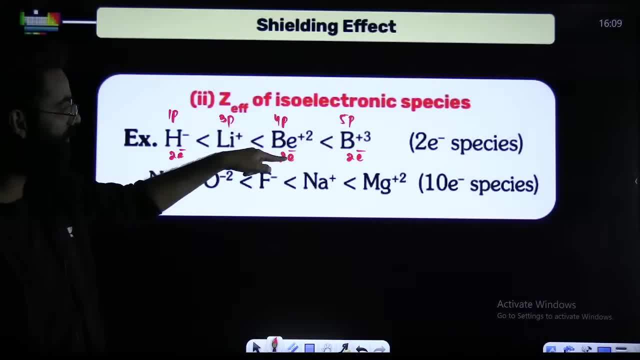 over in the last case. five protons are over in the last case. five protons are holding two electrons holding two electrons holding two electrons. right five protons are holding four. right five protons are holding four. right five protons are holding four protons are holding two electrons three. protons are holding two electrons. three protons are holding two electrons. three protons are holding two electrons. one protons are holding two electrons. one protons are holding two electrons. one proton is holding two electron. can i say: proton is holding two electron? can i say? 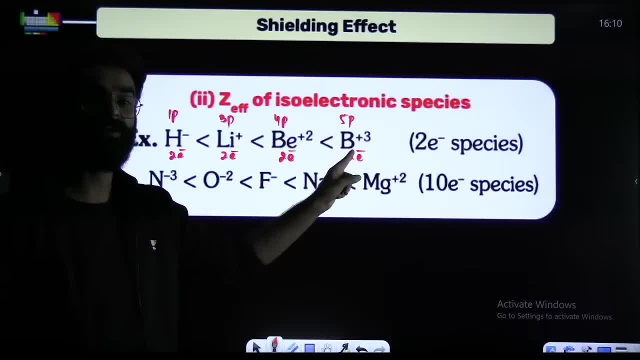 proton is holding two electron. can i say, over here, outermost electron will be over here, outermost electron will be over here. outermost electron will be experiencing maximum attraction, experiencing maximum attraction, experiencing maximum attraction, more the attraction experienced by, the more the attraction experienced by, the more the attraction experienced by the outermost electron, more is going to be. 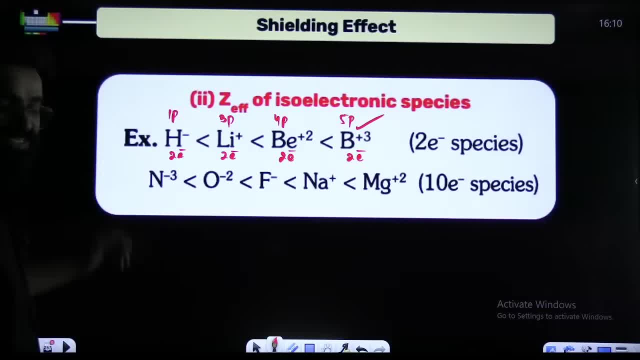 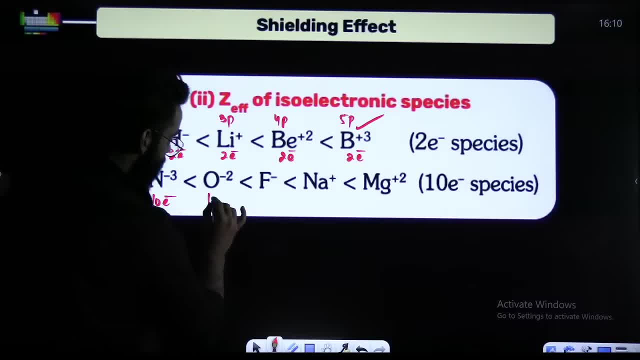 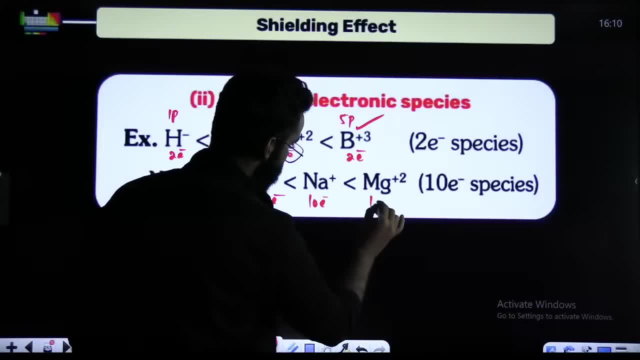 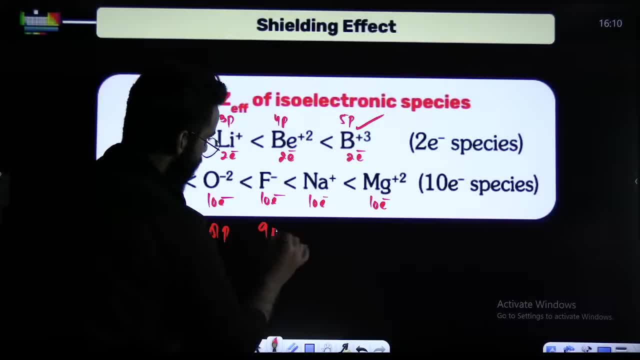 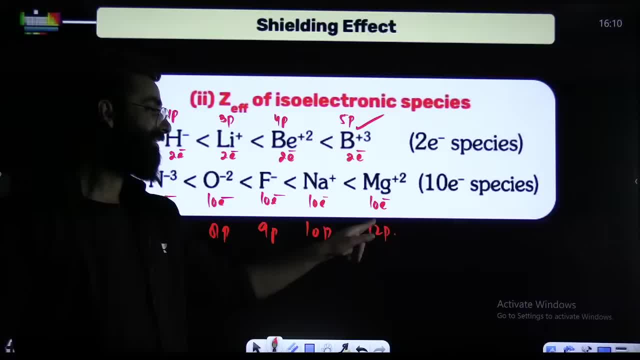 eight protons, nine protons, ten protons, twelve protons, twelve protons, twelve protons, more protons, less electrons, so more protons, less electrons, so more protons, less electrons, so outermost electron. here will be outermost electron, here will be outermost electron, here will be experiencing maximum attraction. so 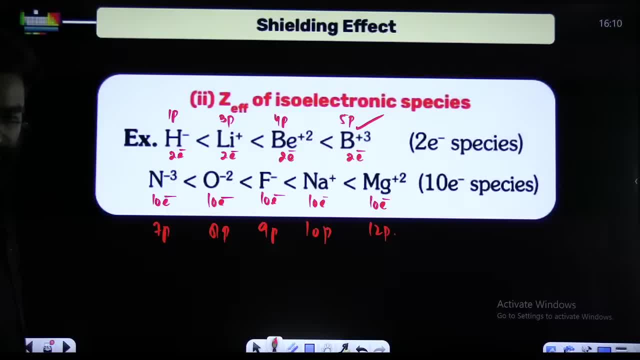 experiencing maximum attraction. so experiencing maximum attraction, so maximum effective nuclear charge in the maximum effective nuclear charge, in the maximum effective nuclear charge. in the last case, last case, last case. right, perfect, right, perfect, right, perfect. okay, can you tell me the answer of this? okay, can you tell me the answer of this? 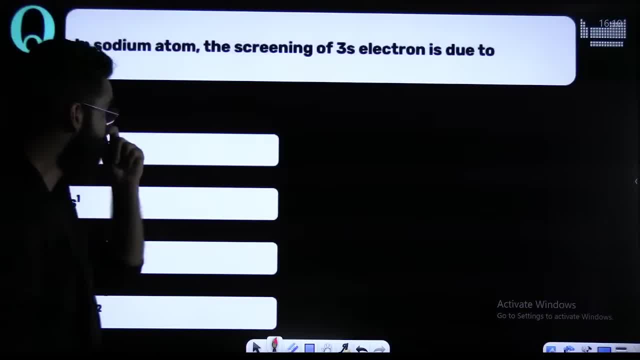 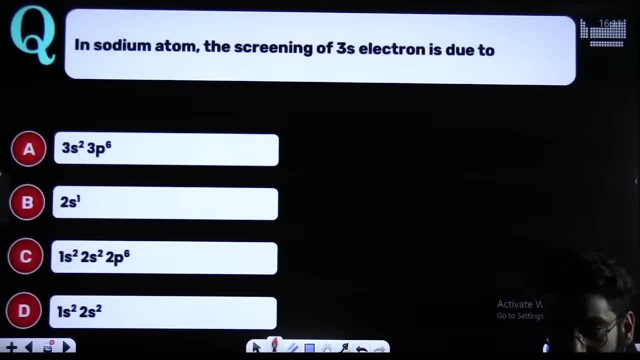 okay, can you tell me the answer of this question? quick question. quick question quick. in sodium atom- the screening of 3s in sodium atom. the screening of 3s in sodium atom. the screening of 3s. electron is due to electron is due to. electron is due to. screening of 3s electron is due to. 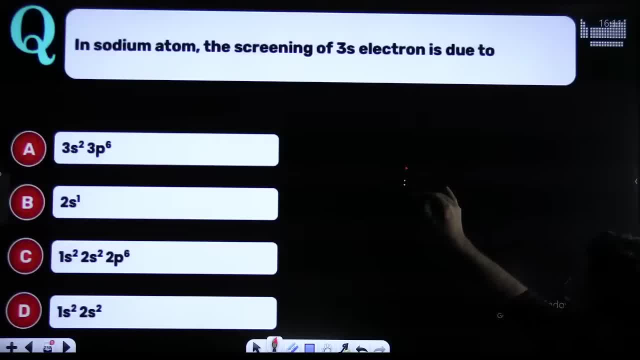 screening of 3s electron is due to. screening of 3s electron is due to, is due to what is due to what is due to what in sodium, in sodium, in sodium. one is two, one is two, one is two, two s2, two s2. 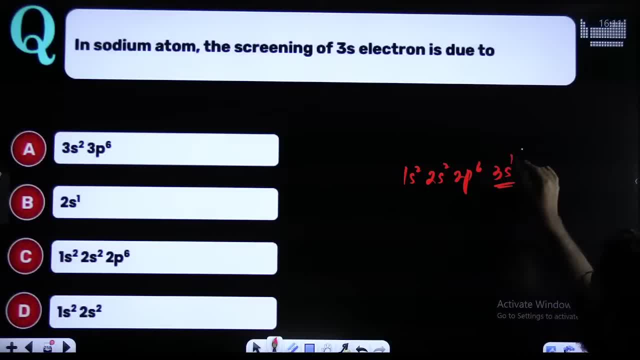 two: s2, 2p6, 2p6, 2p6, ps1: the screening of this particular one. ps1: the screening of this particular one. ps1: the screening of this particular one. the shielding of this particular one is. the shielding of this particular one is. 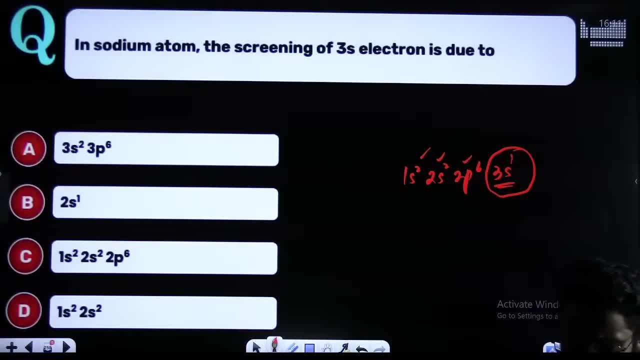 the shielding of this particular one is done by all these electrons, done by all these electrons, done by all these electrons. right, all these electrons, the inner right, all these electrons, the inner right, all these electrons, the inner electrons. i say perfect the inner electrons, i say perfect the inner electrons. i say: 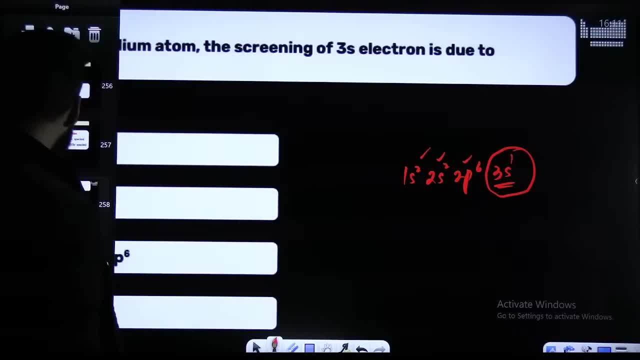 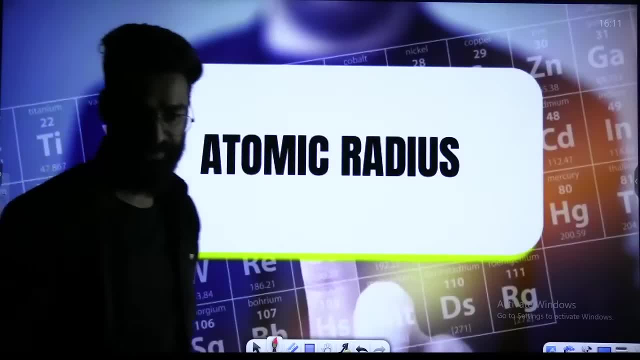 perfect the inner electrons. i say, i hope this also clear. now, my dear students, comes your topic. now, my dear students, comes your topic. now, my dear students, comes your topic. that is atomic radius. i believe atomic, that is atomic radius, i believe atomic. that is atomic radius. i believe atomic radius, everyone would have. 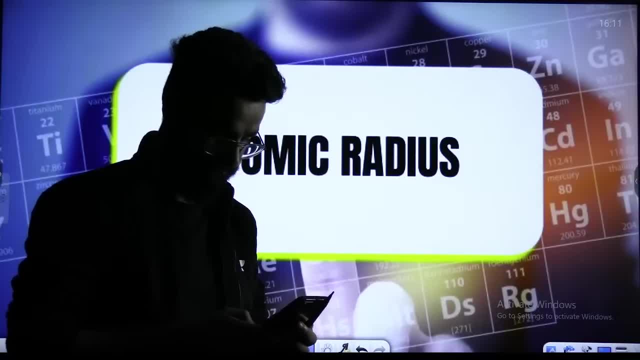 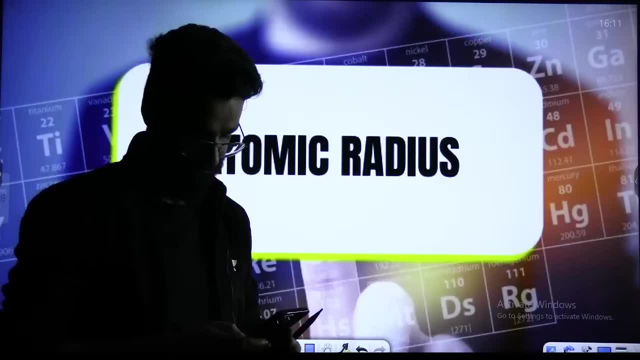 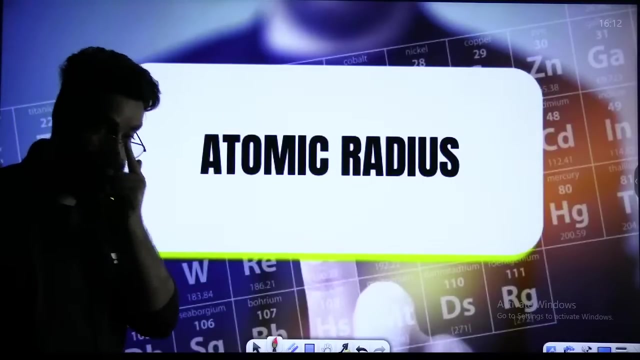 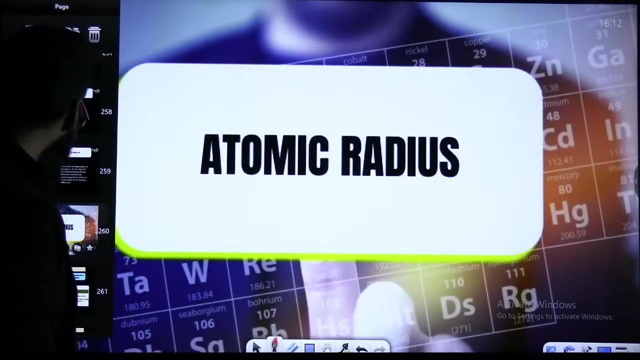 radius, everyone would have radius. everyone would have studied right, studied right, studied right. have you have you? have you? see guys, if you talk about the atomic, see guys, if you talk about the atomic, see guys, if you talk about the atomic radius, radius, radius. let's read its definition. 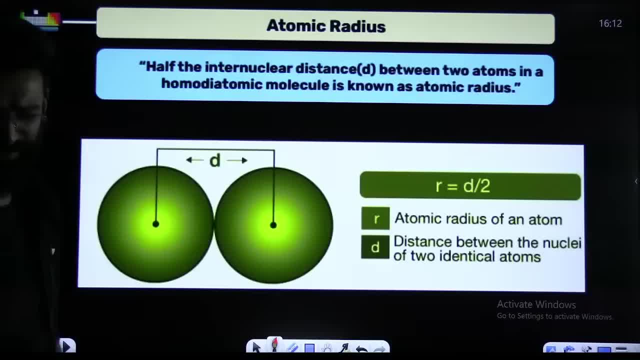 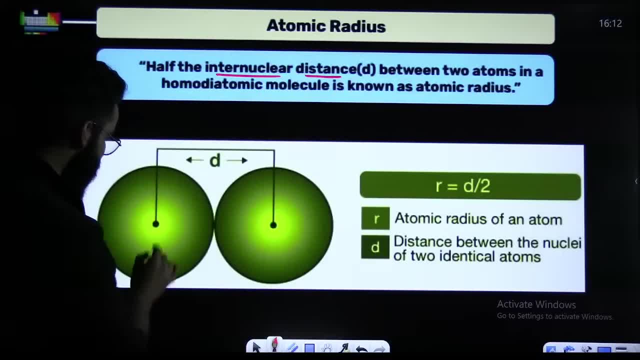 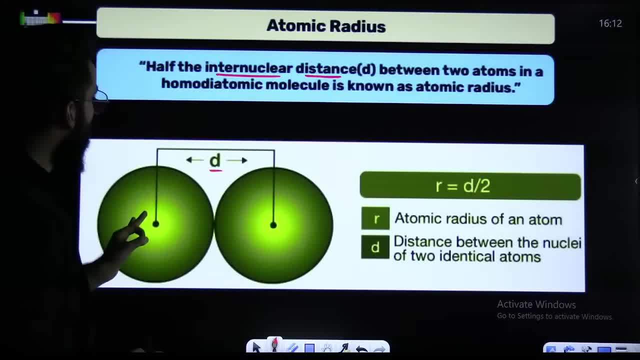 two nuclei. the distance between two nuclei is the inter nuclear distance, is the inter nuclear distance, is the inter nuclear distance half the inter nuclear distance between half the inter nuclear distance, between half the inter nuclear distance between the two atoms in the homo diatomic, the two atoms in the homo diatomic. 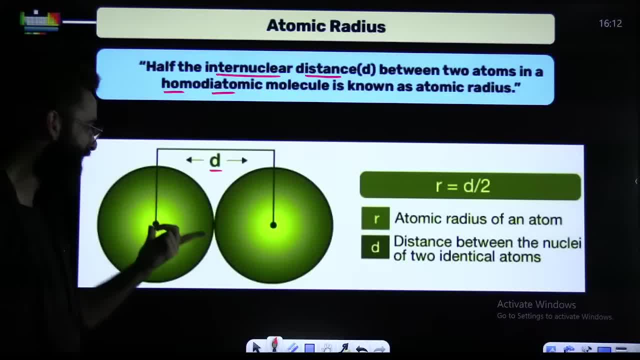 the two atoms in the homo diatomic molecule. homo means same data means two. molecule homo means same data means two. molecule homo means same data means two atoms. so i believe atoms, so i believe atoms, so i believe this is atom a. this is atom a same. this is atom a this is atom a same. 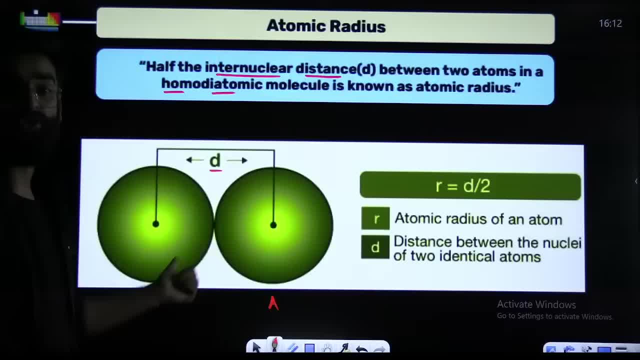 this is atom, a. this is atom, a same atoms, right same atoms as well as atoms, right same atoms as well as atoms, right same atoms as well as two atoms. we have two atoms, we have two atoms. we have so this particular molecule which we have. so this particular molecule which we have. 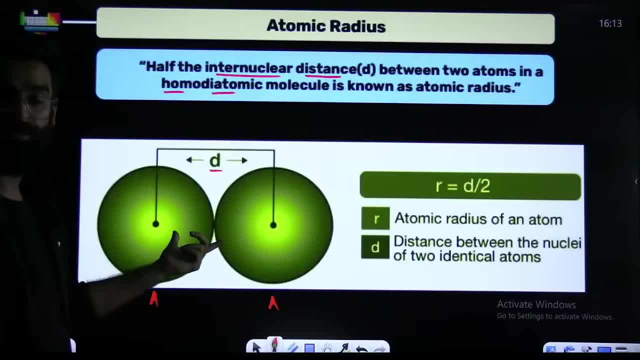 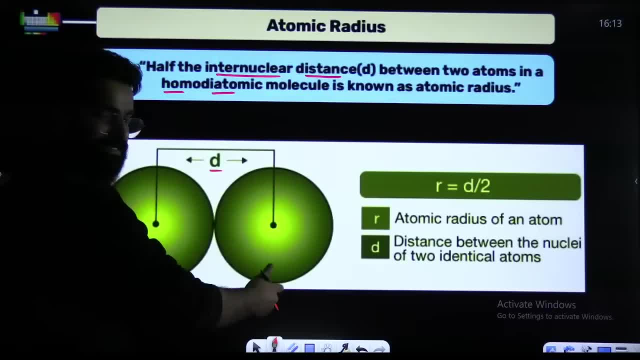 so what you need to do over here is, in order to define the atomic radius, what order to define the atomic radius, what order to define the atomic radius? what you need to do: get the inter nuclear, you need to do, get the inter nuclear, you need to do. get the inter nuclear distance, get the integral distance. 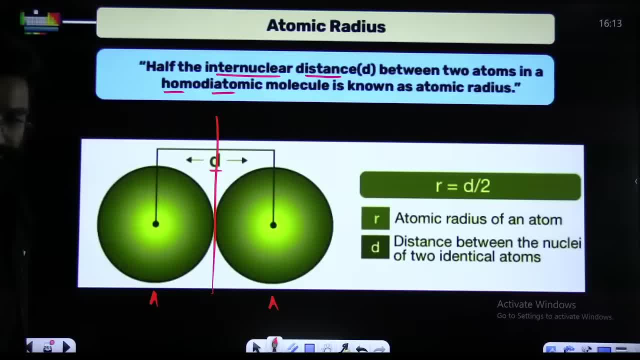 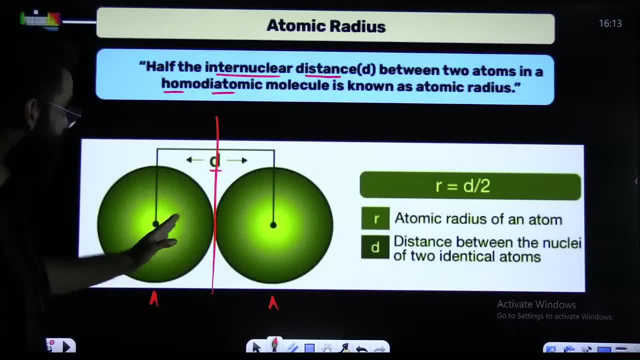 you'll be getting the atomic radius. so you'll be getting the atomic radius. so atomic radius is nothing. it is just atomic radius is nothing. it is just atomic radius is nothing. it is just defined as half the inter nuclear, defined as half the inter nuclear, defined as half the inter nuclear distance between the two atoms. but in 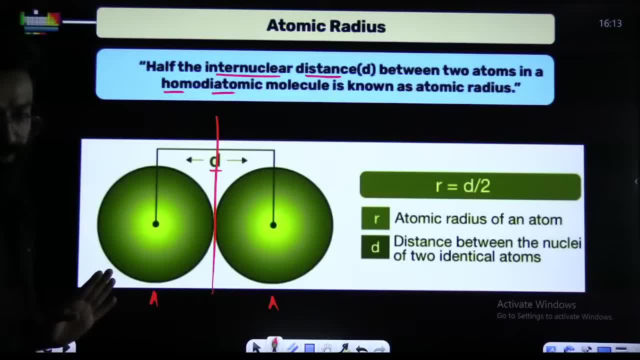 distance between the two atoms, but in distance between the two atoms. but in what? in homo diatomic? what in homo diatomic? what in homo diatomic? atomic radius of the atom, atomic radius of the atom, atomic radius of the atom. till now you used to say atomic radius. 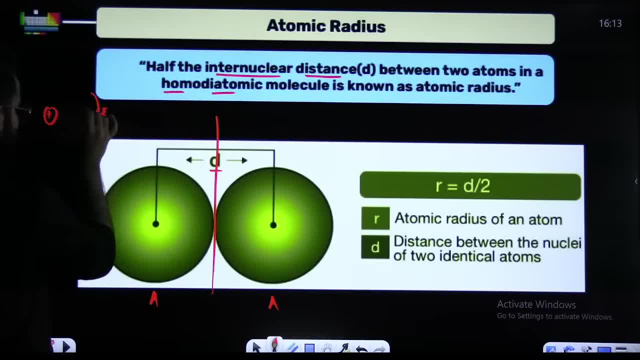 till now you used to say atomic radius. till now you used to say atomic radius is basically the distance from the is basically the distance from the is basically the distance from the nucleus to the outermost electron, right nucleus to the outermost electron, right nucleus to the outermost electron. right till now we used to say that. correct. but 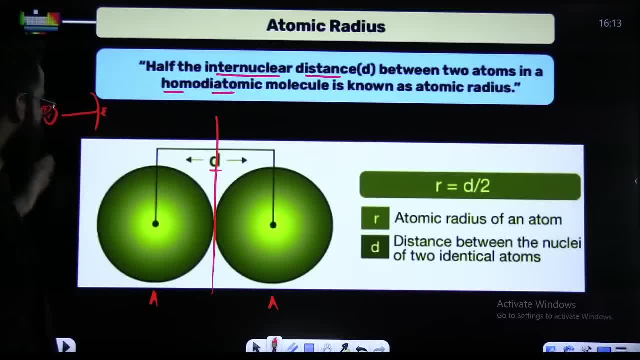 till now we used to say that correct. but till now we used to say that correct. but, my dear students, you know the position, my dear students, you know the position, my dear students, you know the position of the outermost electron, the boundary of the outermost electron, the boundary. 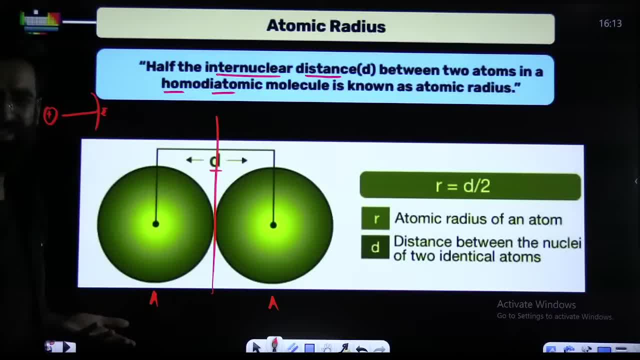 of the outermost electron, the boundary. i mean this, i mean this, i mean this: this glass surface is not defined, this glass surface is not defined, this glass surface is not defined. basically, we talk in terms of basically, we talk in terms of basically, we talk in terms of probabilities as per quantum mechanical. 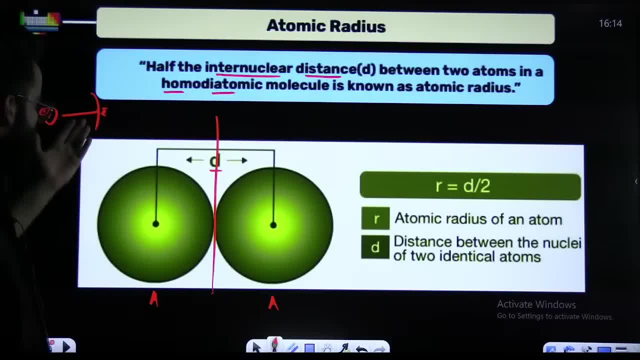 probabilities as per quantum mechanical probabilities, as per quantum mechanical model model. model as per quantum mechanical model. we talk in as per quantum mechanical model, we talk in as per quantum mechanical model, we talk in terms of probabilities. so you cannot terms of probabilities, so you cannot terms of probabilities, so you cannot define the surface over. 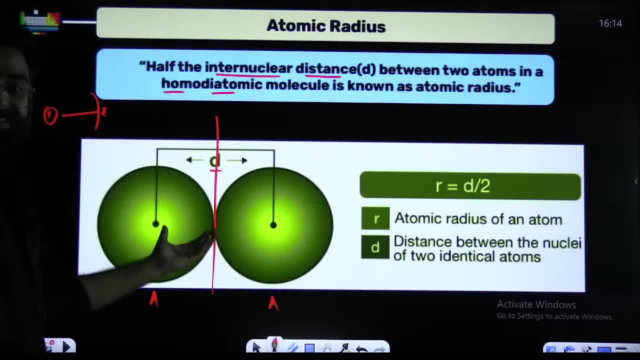 define the surface over, define the surface over perfect. that's why we calculate atomic perfect. that's why we calculate atomic perfect. that's why we calculate atomic radius like this radius, like this radius, like this. get the internuclear distance divide it. get the internuclear distance divide it. 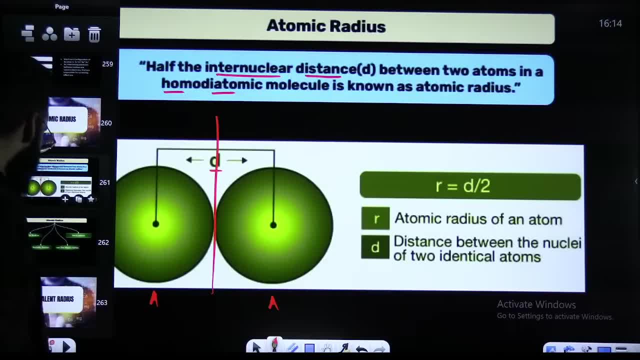 get the internuclear distance, divide it with two. get the atomic radius- now this with two. get the atomic radius, now this with two. get the atomic radius, now this atomic radius. we classify into four types atomic radius. we classify into four types atomic radius. we classify into four types. one is: 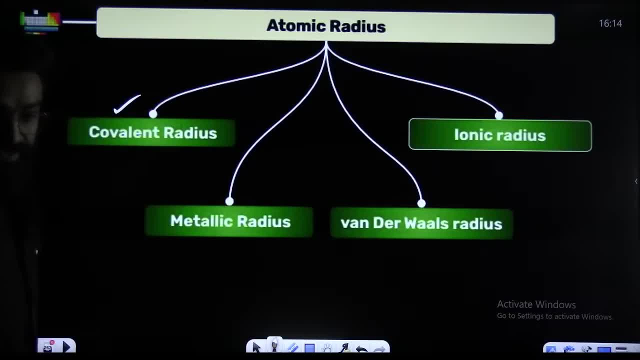 one is one is oval and radius, oval and radius. oval and radius right one is covalent radius. right one is covalent radius. right one is covalent radius, which is defined for covalent molecules. which is defined for covalent molecules. which is defined for covalent molecules. metallic radius, which is defined. 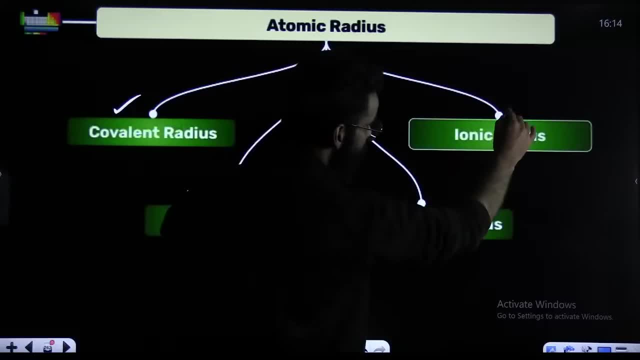 metallic radius which is defined. metallic radius which is defined in case of metallic bonds etc. in case of metallic bonds, etc. in case of metallic bonds etc. uh. ionic radius, which is defined for uh. ionic radius which is defined for uh. ionic radius which is defined for ionic compounds, and van der waals radius. 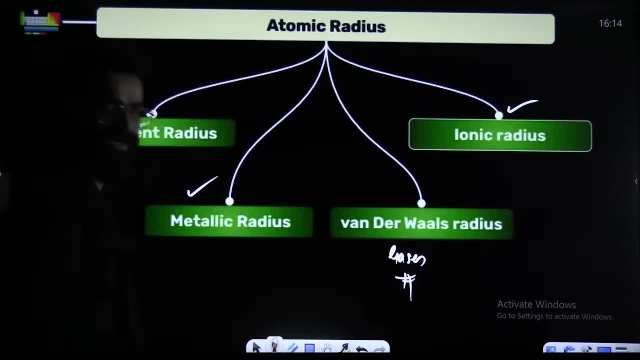 ionic compounds and van der waals radius, ionic compounds and van der waals radius, which is particularly defined for gases, which is particularly defined for gases, which is particularly defined for gases, right, which is particularly defined for right, which is particularly defined for gases, and it's not only defined for 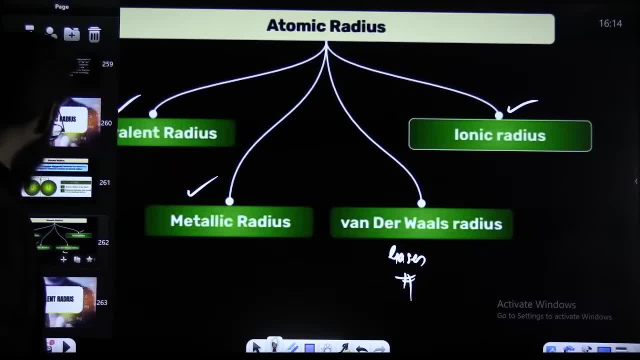 and it's not only defined for, and it's not only defined for noble gas, by the way. so we'll start with the covalent radius. so we'll start with the covalent radius. so we'll start with the covalent radius. first of all, what this covalent rate is. 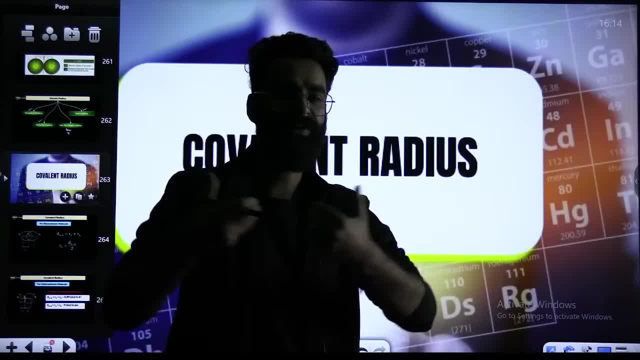 first of all, what this covalent rate is. first of all, what this covalent rate is all about. do you remember how covalent all about? do you remember how covalent all about? do you remember how covalent bond is formed? penetration of atomic. 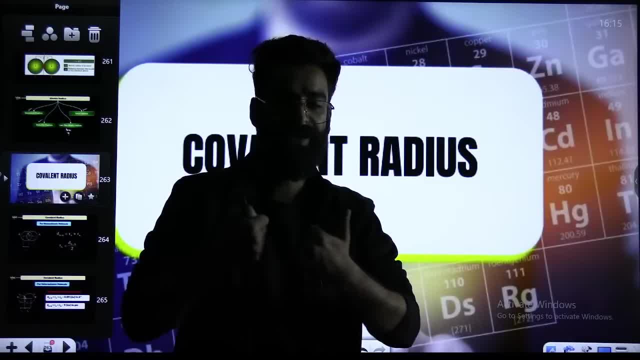 bond is formed. penetration of atomic bond is formed. penetration of atomic orbitals into each other, orbitals into each other, orbitals into each other. penetration of atomic orbitals into each. penetration of atomic orbitals into each. penetration of atomic orbitals into each other other other. do you remember that? 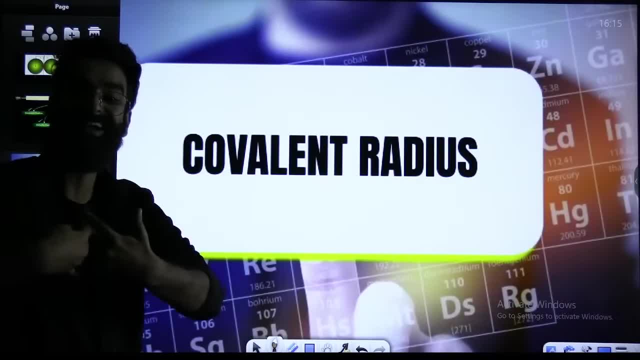 do you remember that? do you remember that when you talk about the covalent compound, when you talk about the covalent compound, when you talk about the covalent compound, atomic orbitals, they penetrate into each atomic orbitals. they penetrate into each atomic orbitals. they penetrate into each other. overlapping happens. 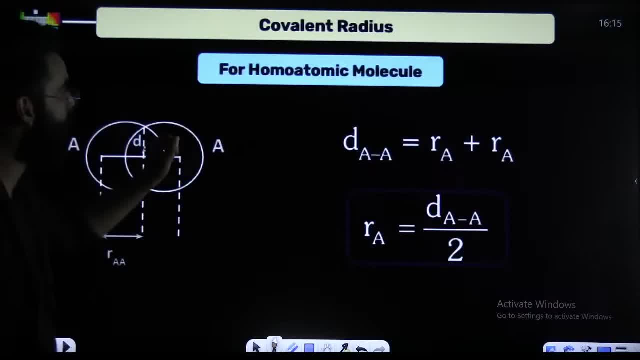 other overlapping happens, other overlapping happens. so imagine, so imagine, so imagine. imagine i've got a homo atomic, homo atomic. imagine i've got a homo atomic, homo atomic. imagine i've got a homo atomic, homo atomic, molecule, molecule, molecule, same atoms, a atom, a atom right? imagine i've. 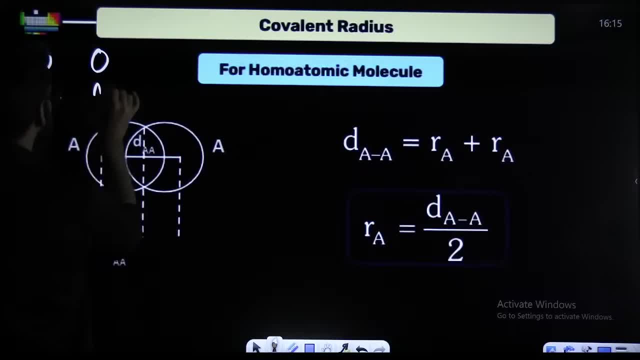 same atoms, a atom, a atom. right. imagine i've same atoms, a atom, a atom, right. imagine, i've got, got got a atom here. i've got a atom here, now for a atom here. i've got a atom here, now for a atom here. i've got a atom here now for the covalent bond formation. the covalent bond formation. the covalent bond formation, their electron clouds have to merge into their electron clouds have to merge into their electron clouds have to merge into each other. let's say: this is the nucleus. each other, let's say this is the nucleus. each other. let's say: this is the nucleus of this. this is the nucleus of this i'll of this. this is the nucleus of this i'll of this. this is the nucleus of this. i'll be calling this particular distance as be calling this particular distance as 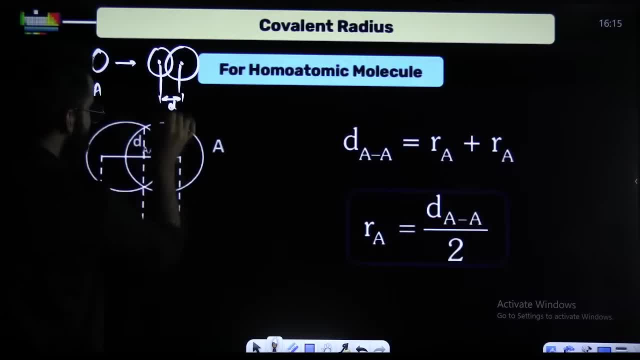 be calling this particular distance as the inter-nuclear distance b right, so the inter-nuclear distance b right, so the inter-nuclear distance b right. so divide this inter-nuclear distance by two, divide this inter-nuclear distance by two, divide this inter-nuclear distance by two, you'll be getting what you'll be getting. 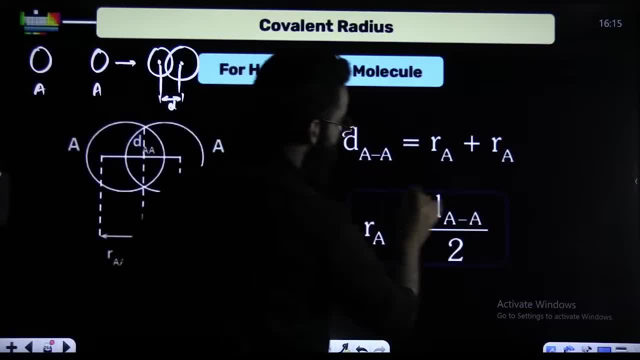 you'll be getting. you'll be getting the covalent radius, okay, the covalent radius, okay, the covalent radius, okay, divide the divide, the inter-nuclear divide, the divide, the inter-nuclear divide, the divide, the inter-nuclear distance by two. you'll be getting the. 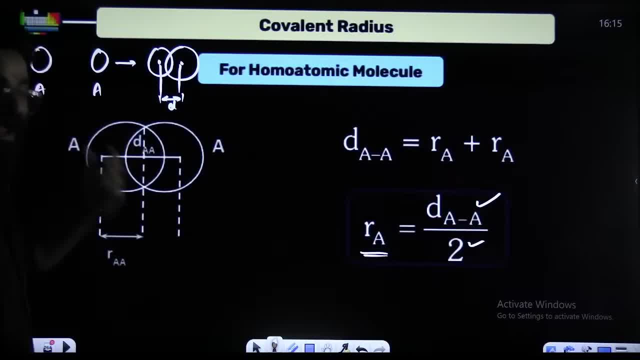 distance by two, you'll be getting the distance by two, you'll be getting the covalent radius of the covalent radius of the covalent radius of the atom over here. correct, atom over here, correct. atom over here, correct, correct. this is for homo atomic. 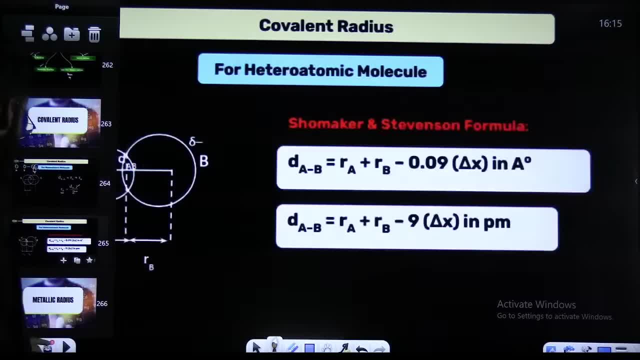 correct. this is for homo atomic, correct. this is for homo atomic molecule. now, if you'll be having a molecule now, if you'll be having a molecule, now if you'll be having a heterotomic molecule, heterotomic molecule, heterotomic molecule, if you're having the hetero atomic. 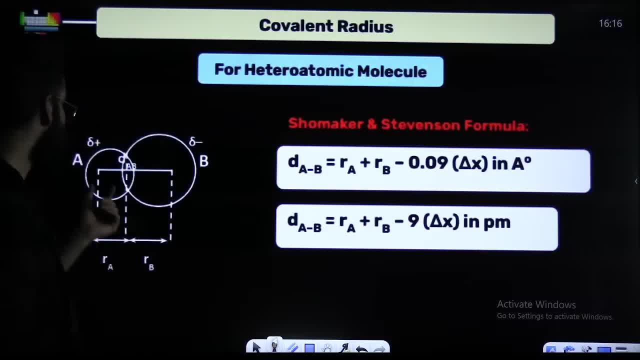 if you're having the hetero atomic, if you're having the hetero atomic molecule, if you're having the hetero molecule, if you're having the hetero molecule, if you're having the hetero atomic molecule, for example, this is atom. atomic molecule, for example, this is atom. 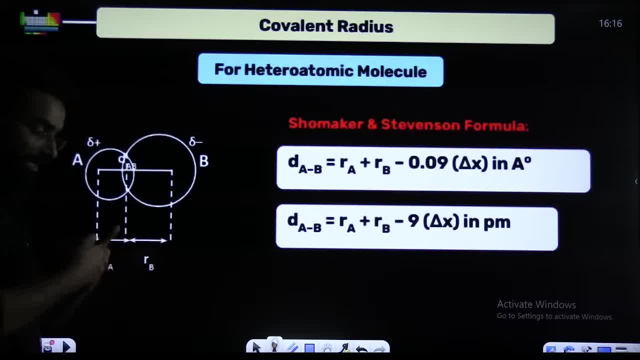 atomic molecule, for example. this is atom a. this is atom b. their electron clouds a. this is atom b. their electron clouds a. this is atom b. their electron clouds have merged. their electron clouds have have merged. their electron clouds have have merged. their electron clouds have merged, but atoms are different. there is 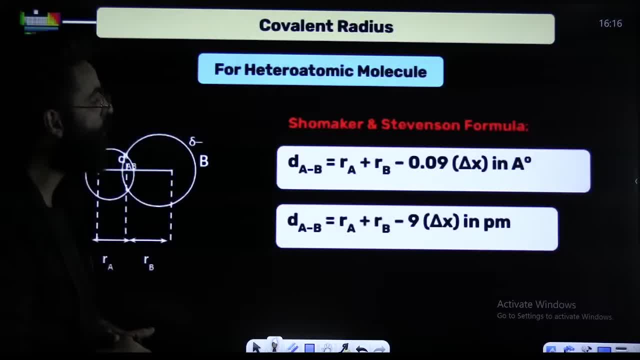 merged, but atoms are different. there is merged, but atoms are different. there is some electro negative difference as well, some electro negative difference as well, some electro negative difference as well. then how do you calculate then? what kind then? how do you calculate then? what kind then? how do you calculate then? what kind of result do you use? 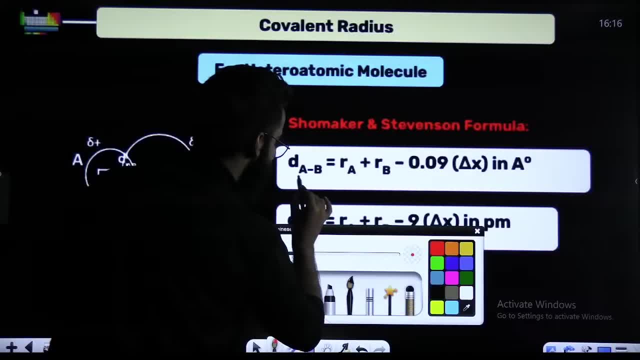 of result do you use? of result do you use? what kind of result do you use? this is: what kind of result do you use? this is: what kind of result do you use? this is this: d a b. it represents the. this is this: d a b. it represents the. 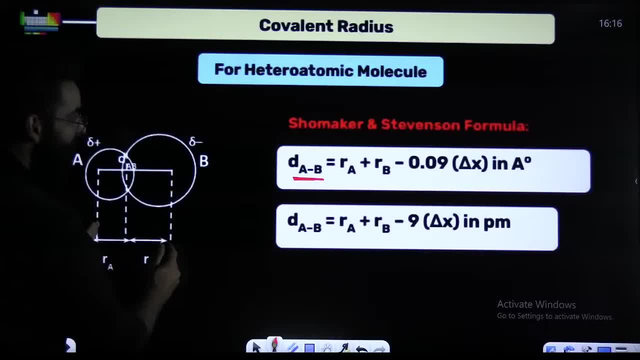 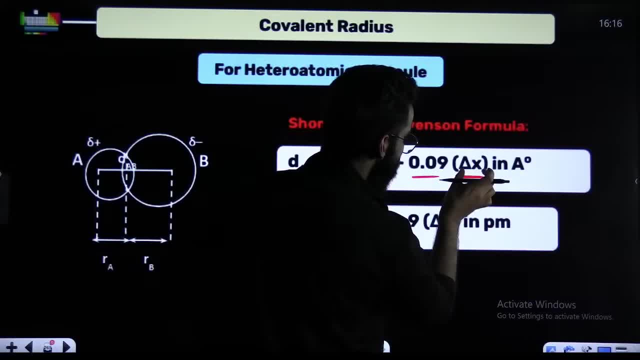 equaled radius of atom a plus radius of equaled radius of atom a plus radius of atom b minus 0.09. atom b minus 0.09. atom b minus 0.09 multiplied by electro negativity. multiplied by electro negativity. multiplied by electro negativity difference. 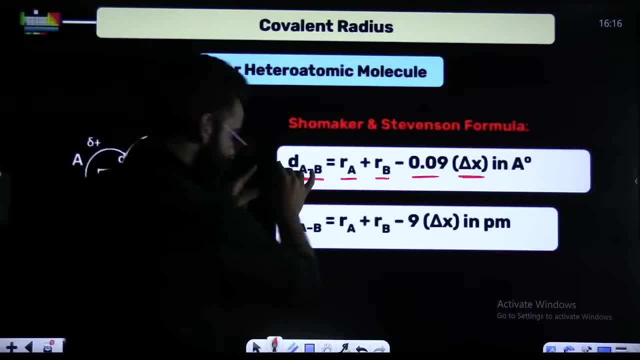 difference, difference, electro negativity, difference between the electro negativity, difference between the electro negativity difference between the two atoms. and if you are, you are using two atoms and if you are, you are using two atoms. and if you are, you are using this particular result, you will be this particular result, you will be. 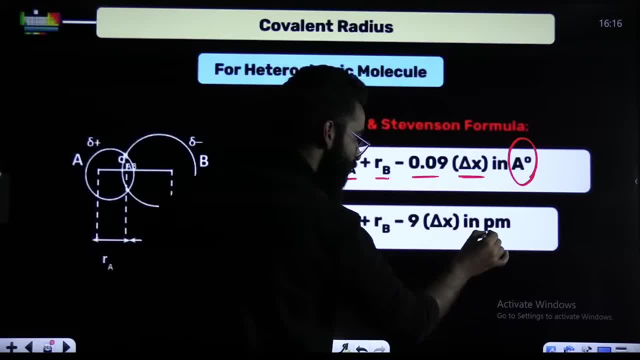 this particular result. you will be getting the answer in angstroms. if you getting the answer in angstroms, if you getting the answer in angstroms, if you are using this particular result, you are, are using this particular result. you are, are using this particular result. you are using, you are getting the answer in. 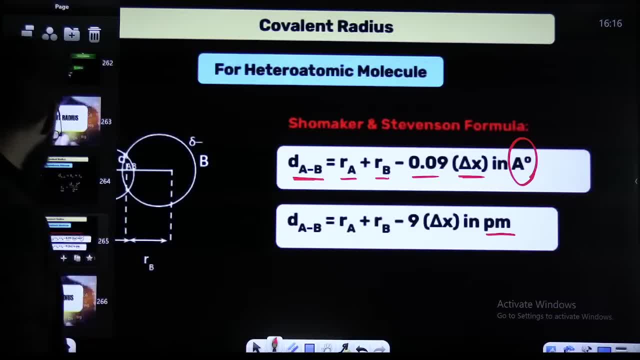 using. you are getting the answer in using. you are getting the answer in picometers, for example, picometers, for example, picometers, for example. you are, you are, you are- i hope this is clear- all the values, all i hope this is clear. all the values, all i hope this is clear, all the values, all the values here will be given. 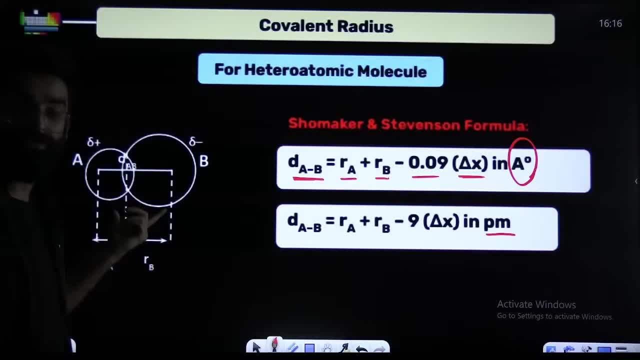 the values here will be given. the values here will be given. if you get a question from this, if you, if you get a question from this, if you, if you get a question from this, if you get a hetero atomic molecule, get a hetero atomic molecule. 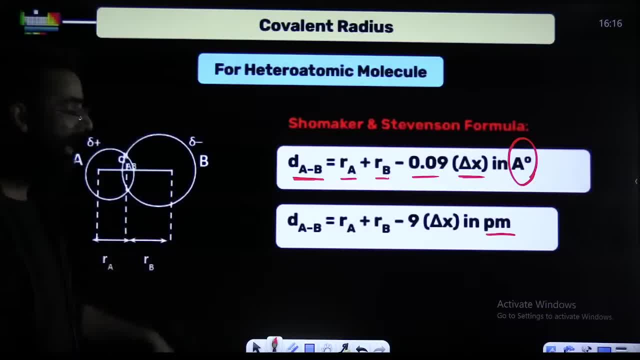 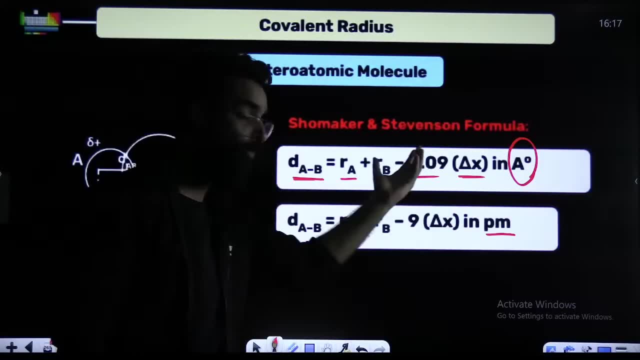 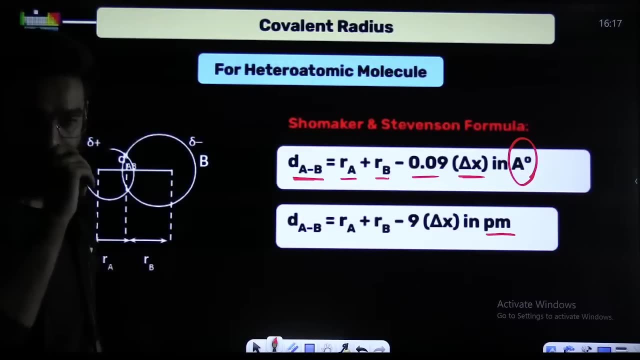 if you get the heteroatomic molecule, my dear students, right and out of all these things over here, right, see how many unknowns we are: one, two, three, four, four unknowns out of four unknowns. if three are given, fourth one you can calculate. yeah, fourth one you can calculate, it is just. 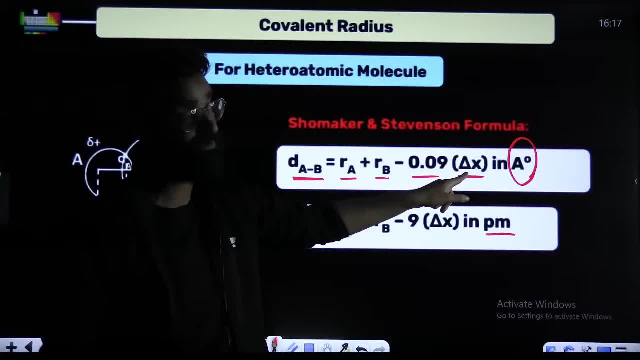 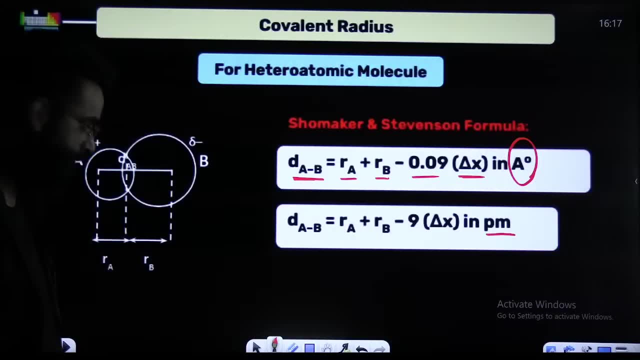 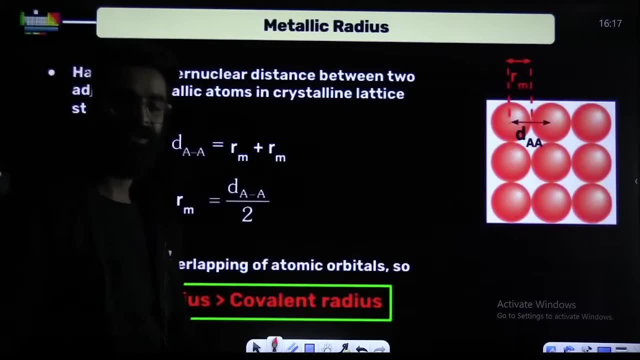 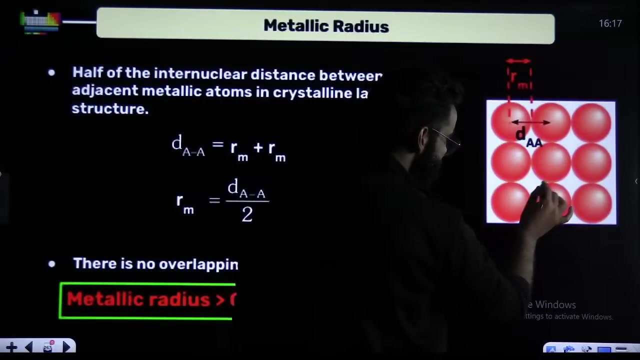 remember this particular delta x represents electron negativity difference between the two atoms which will be given in the equation. okay, perfect. now if i talk about metallic radius, what is metallic radius? metallic radius, my dear students, let's say this is metal, let's say this metal, and these are the positively charged kernels. these are the positively charged kernels, right? 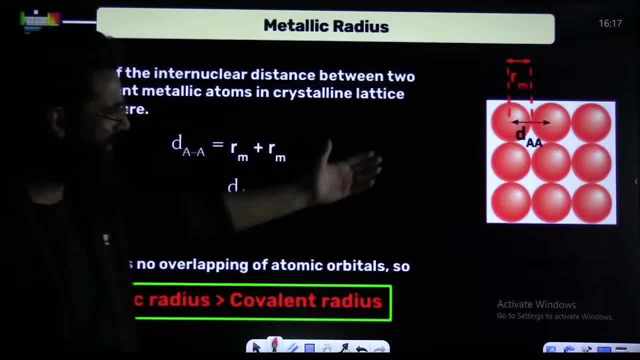 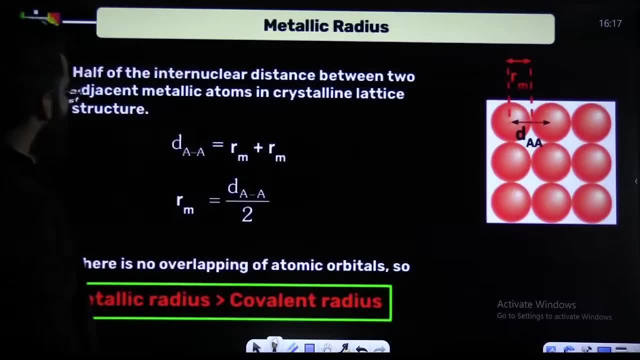 positively charged kernels we have okay. so basically, metallic bond exists in this particular metal right now. how, what do we do here? how do we calculate the metallic radius? it is the. it is again half the internuclear distance between the two adjacent metallic atoms in the crystal line. 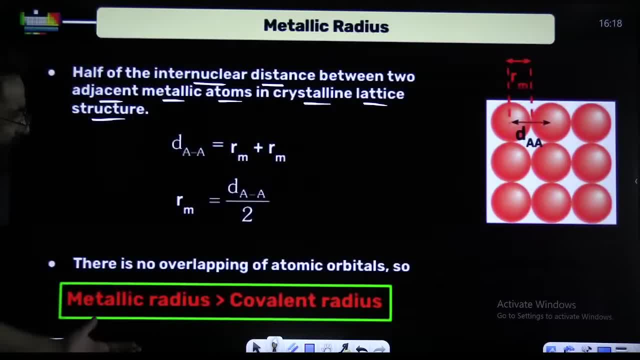 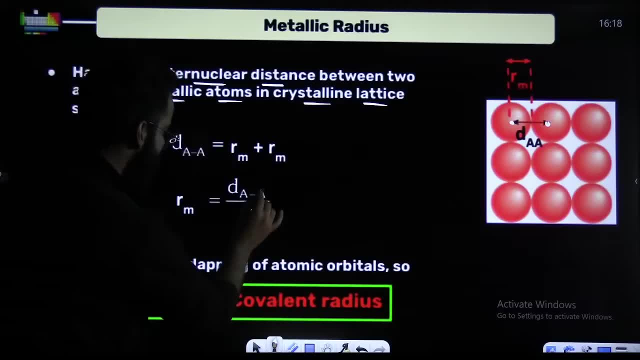 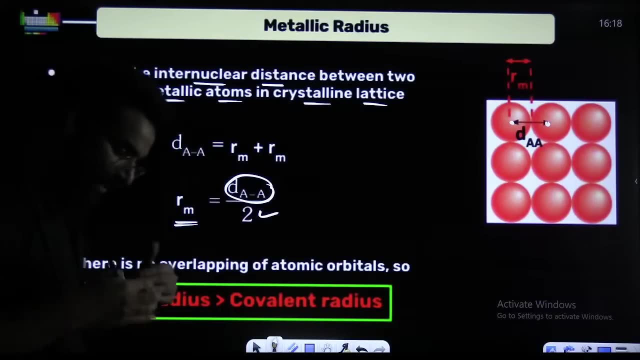 in the crystalline lattice structure. it is again what you need to do. what you need to do: get the internuclear distance and divide it with half right. get the internuclear distance, divide it with two, you'll be getting the radius of the metal. you'll be getting the radius of the metal. overlapping was 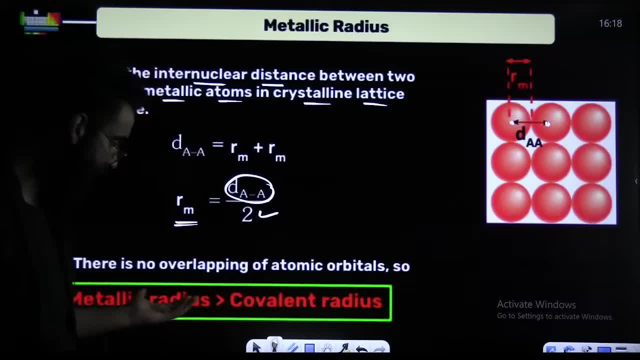 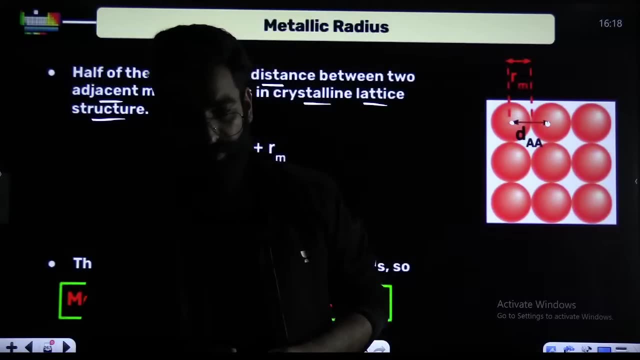 there in when i defined the covalent radius. but here you are not. you are not going to define overlapping here. perfect, you are not going to define overlapping right now. guys understand, understand. if i need to compare covalent radius with metallic radius, which will be more covalent? 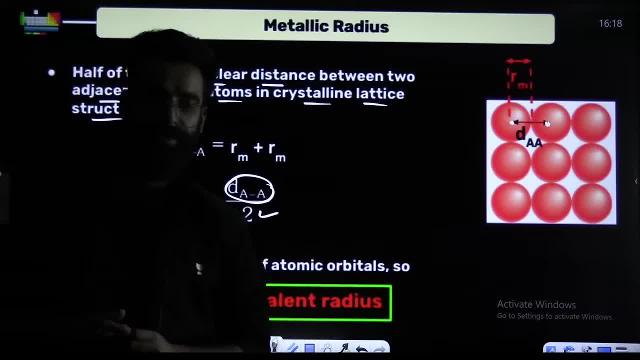 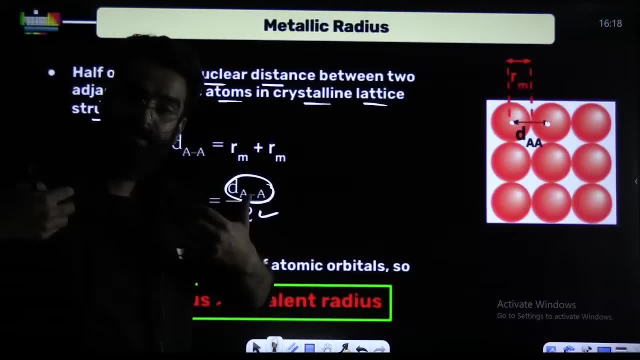 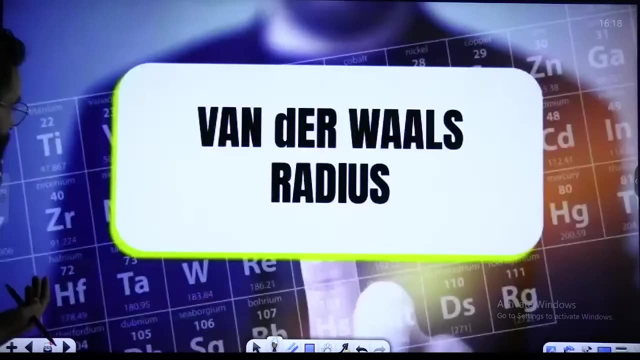 radius or metallic radius, which will be more? which one is going to be more? covalent radius or metallic radius? which one? which one metallic radius will be more? because in covalent atomic orbitals they merge into each other, right? perfect, if i talk about vanderwald's radius? if i talk about vanderwald's radius, let's. 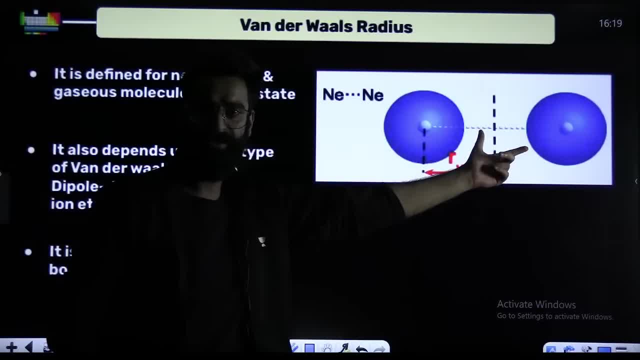 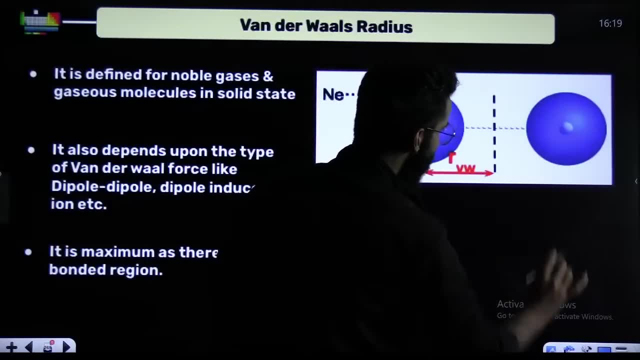 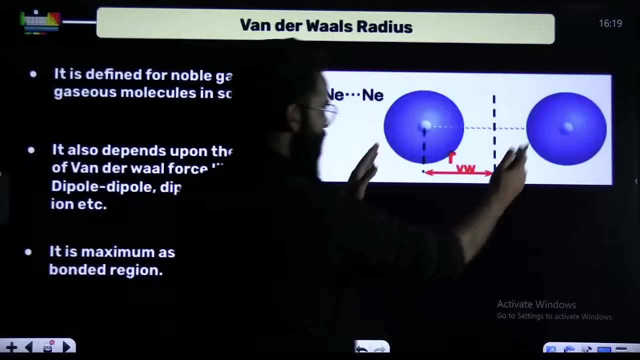 say you are taking two noble gases: neon, neon. perfect. there will be vanderwald's force of attraction between them. there will be vanderwall's forces of attraction between them. perfect, the distance between their nuclei is what you call as internuclear distance. perfect, right, it is called as internuclear distance. again, get, get the inter nuclear distance. divide it with two. 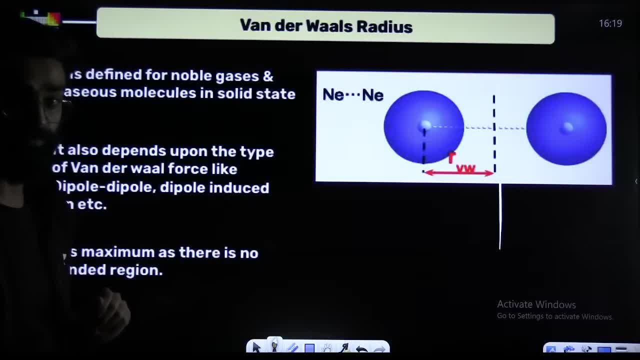 2, you will be getting what. You will be getting: the Van der Waals radius. You will be getting the Van der Waals radius. Perfect. Now, it is not only for what? It is not only for noble gases, For example. 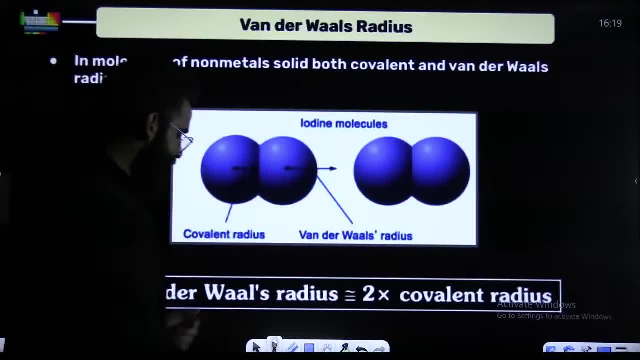 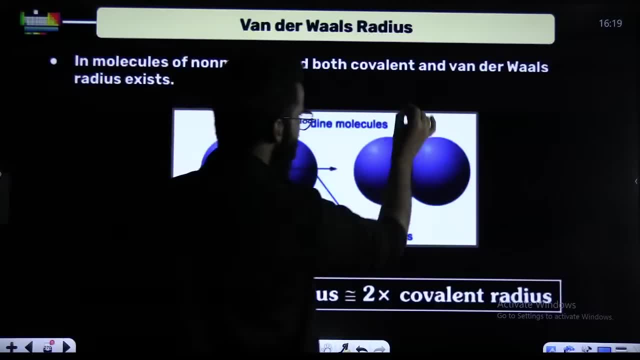 for example, for example. let's say you are taking: this is I2 molecule. Let's say you are taking I2 molecule. This is iodine, iodine. This is I2.. This is I2.. This is again one more I2.. This is iodine. 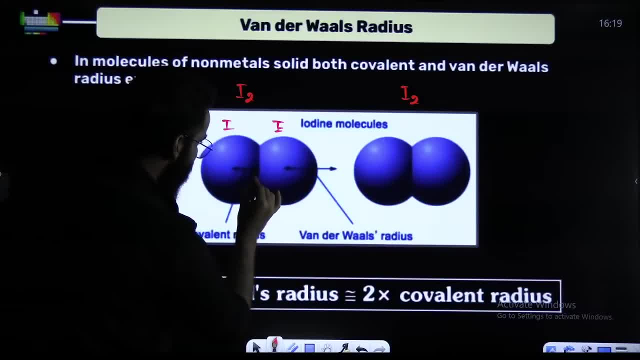 this is iodine, this is I2.. Right, Between this iodine and this iodine, you are going to define covalent radius. Between this iodine and this iodine, you are going to define covalent radius, But, but, but. 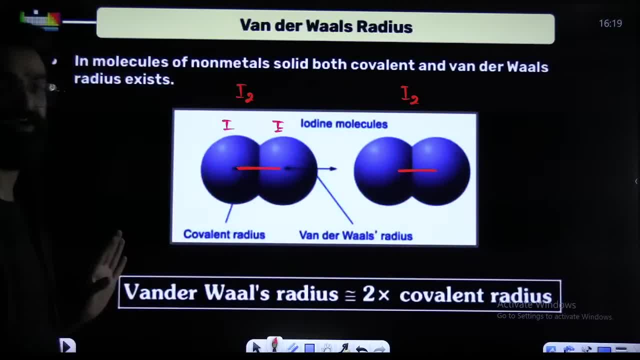 between these two iodine molecules you are going to define what You are going to define Van der Waals radius. And how do I get the Van der Waals radius? Get the inter-nuclear distance, divide it with 2, you will be getting what You will be getting the Van der Waals radius over here. 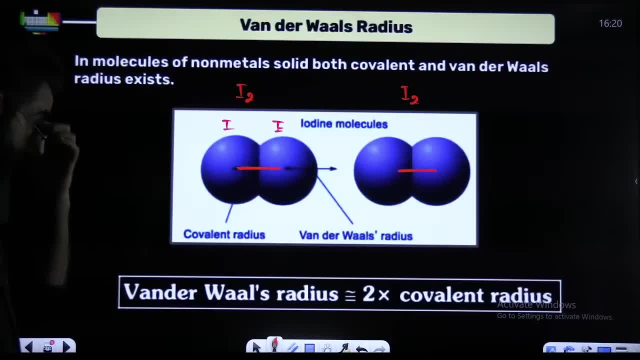 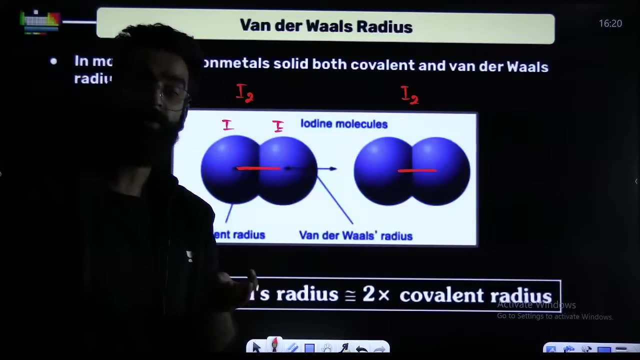 Okay, Perfect, Okay, guys, Remember this thing And I believe you already understood this. Now tell me one thing: Metallic covalent or Van der Waals radius, Which one will be maximum? Which one will be maximum? 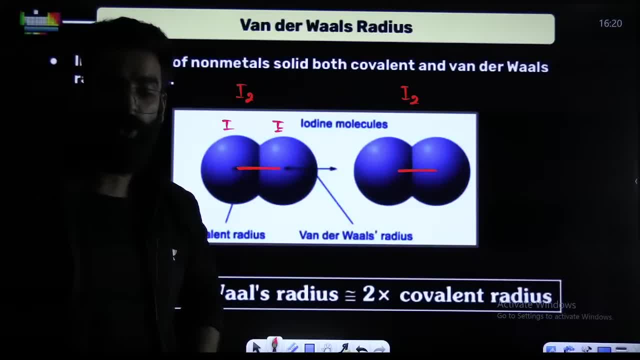 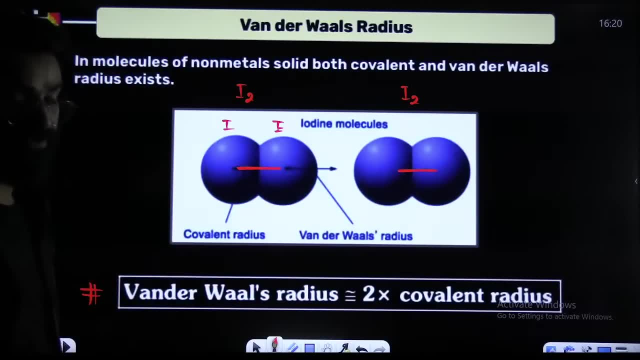 Which one will be maximum Metallic covalent or Van der Waals? Van der Waals will be maximum, followed by, followed by metallic. followed by, followed by your covalent radius. Okay, Okay, Followed by your covalent radius. 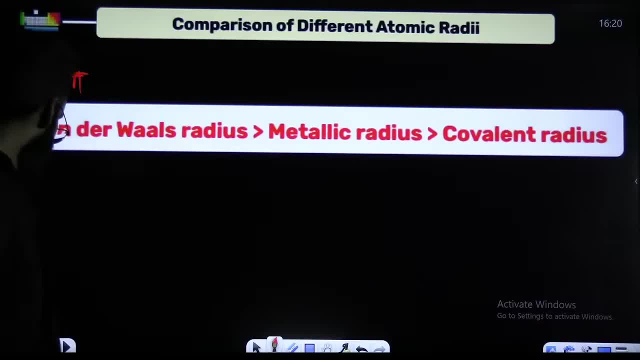 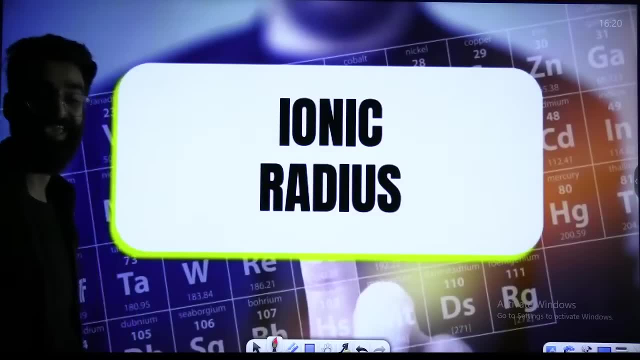 This is the order which you have to remember. This can be asked as well. This can be asked as well. Now one more, that is, ionic radius. Ionic radius we define for ionic compounds like NaCl. Like NaCl, Okay. 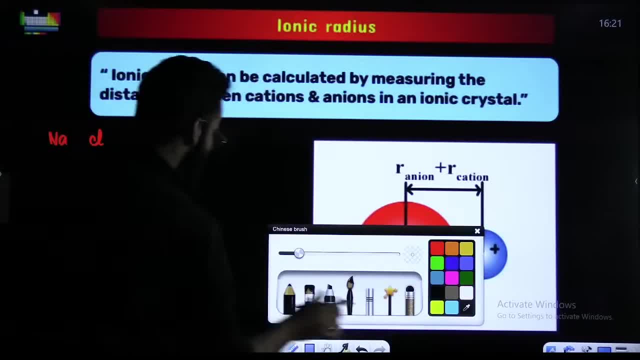 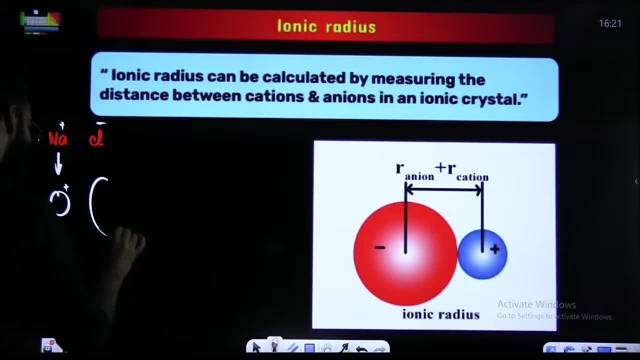 Generally, my dear students, if I talk about NaCl, if I talk about NaCl, this is your cation and this is your anion. Generally generally, what do you observe? You observe: cation is smaller sized and anion is larger sized. 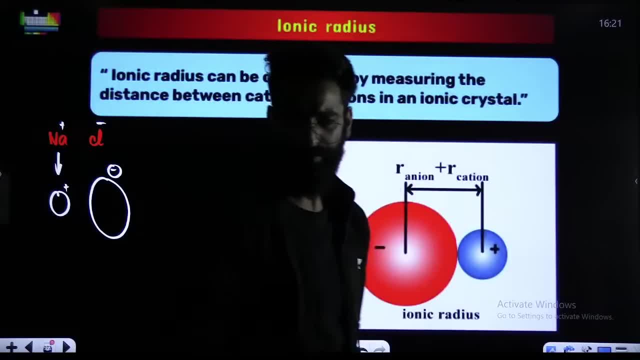 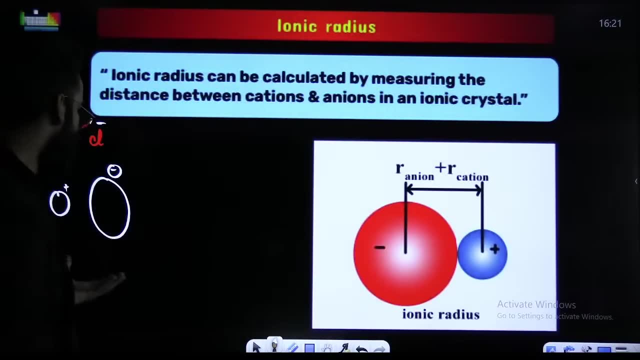 And generally it happens- Not every time, Okay, Generally it happens- Cation is smaller sized and anion is larger sized. Right Now, in case of the ionic compound, in case of the ionic compound, imagine this is your cation and this is your anion. 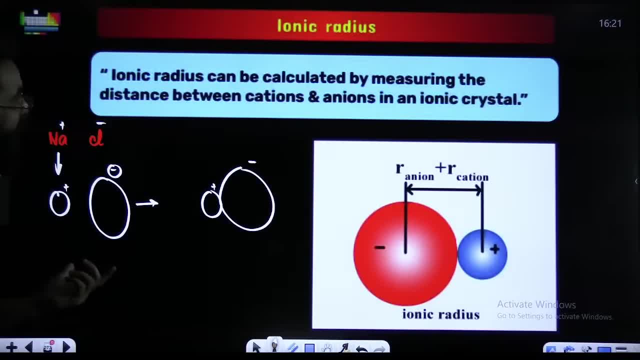 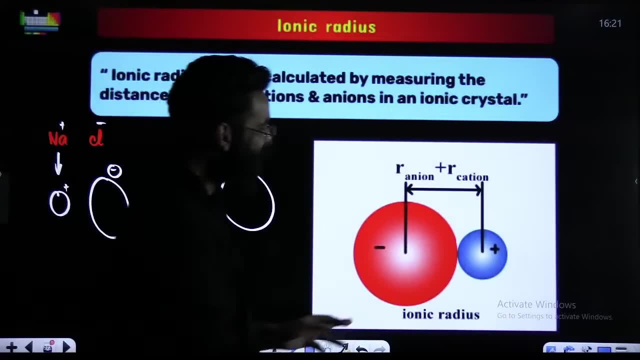 This is your anion, Right? How do I define the ionic radius over here? How do I define the ionic radius over here, First of all? first of all, your inter-nuclear distance, that means distance between the nuclei, is going to be equal to. 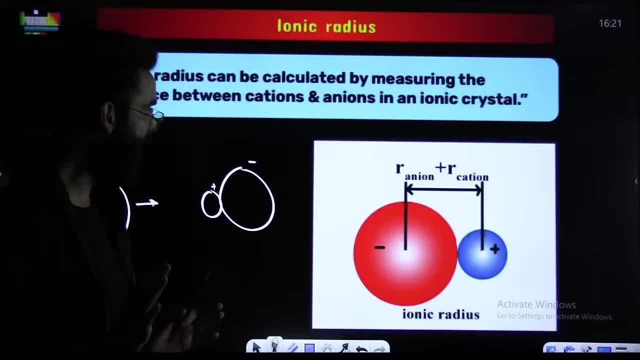 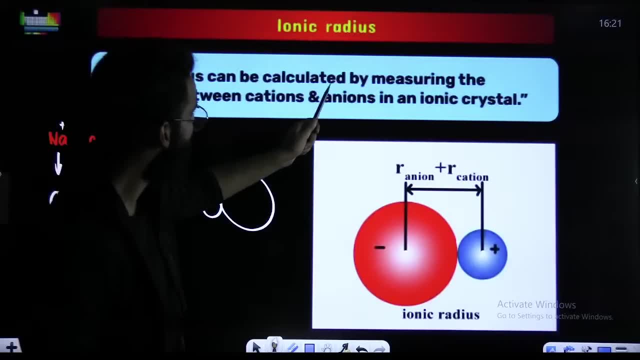 radius of anion plus radius of cation. You know it Right: Radius of cation plus radius of anion. Again, what you have to do: ionic radius can be calculated by measuring the distance between the cations and ions in anionic crystal. 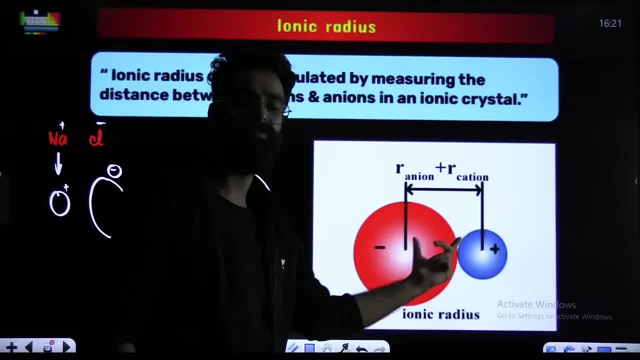 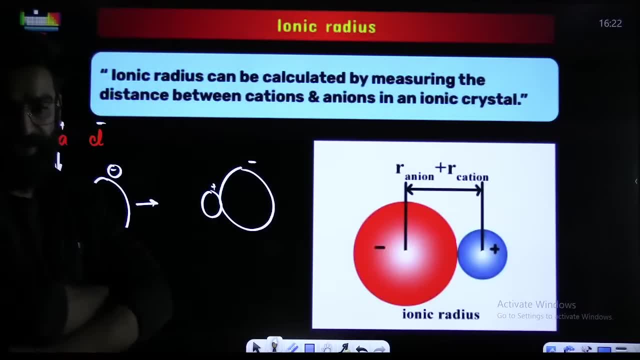 In case of ionic compounds, you need to get the radius of cation, radius of anion. Accordingly, you can get what? Accordingly, you can get ionic radius over here. Accordingly, you can get ionic radius over here by dividing it with 2.. 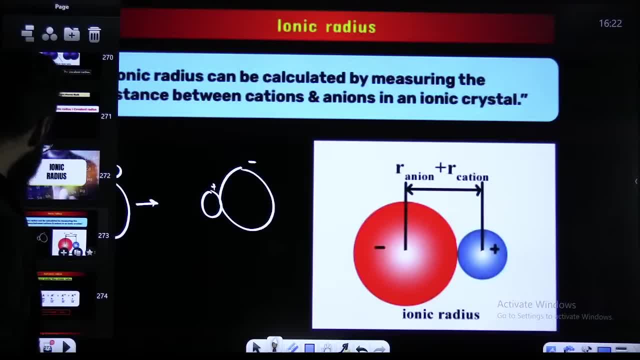 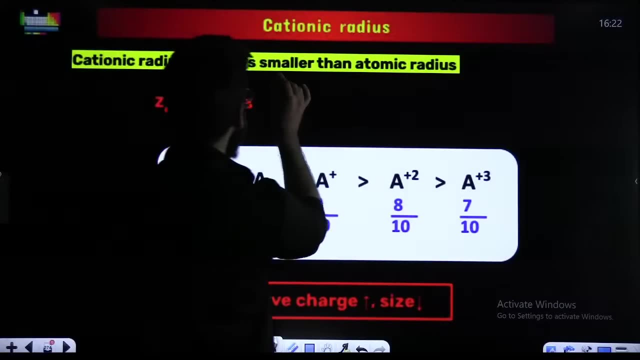 By dividing it with 2.. By dividing it with 2.. Okay, Alright, tell me one thing. Look at this particular statement. Ket-ionic radius is always smaller than the atomic radius. What does that mean? That means radius of cation. 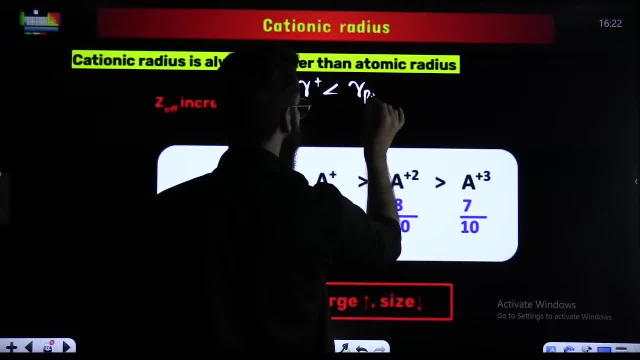 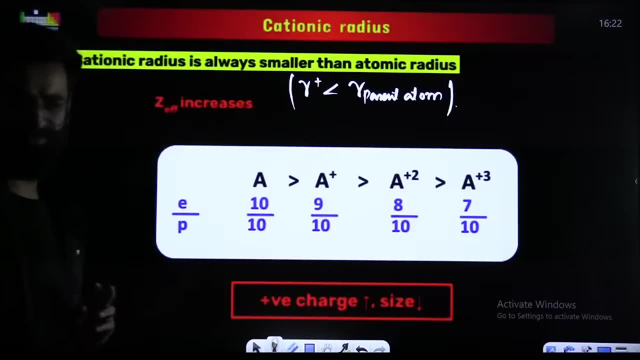 Radius of cation is always less than the radius of its parent atom, And it can be explained with the help of z-effective. Okay, it can be explained with the help of z effective. it can be explained with the help of what z effective. right, perfect. for example, let's say you have got sodium, you have got any positive correct. 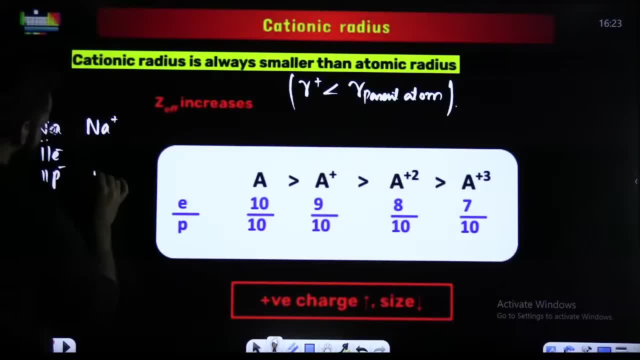 11 electrons, 11 protons, perfect 11 protons: 10 electrons, 11 protons, 10 electrons. right now, my dear students, 11 protons are holding 11 electrons. 11 protons are holding 10 electrons. the force experienced by the outermost electron will be more. z effect is more if z effect is more if the 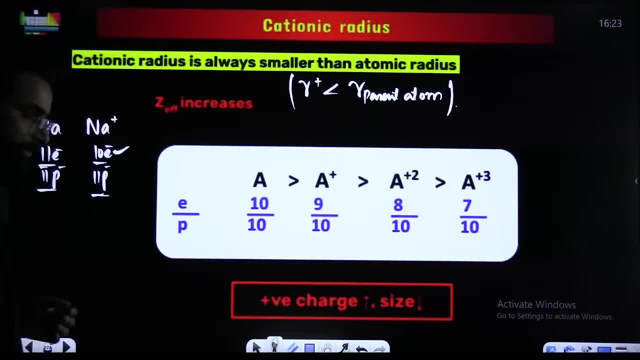 outermost electron is is getting more attraction from the nucleus, right it will come closer. size decreases, right. so this is the size order, basically perfect. so basically, your cationic size, your cationic size, your cationic radius is always less than the radius of the parent atom. okay, for. 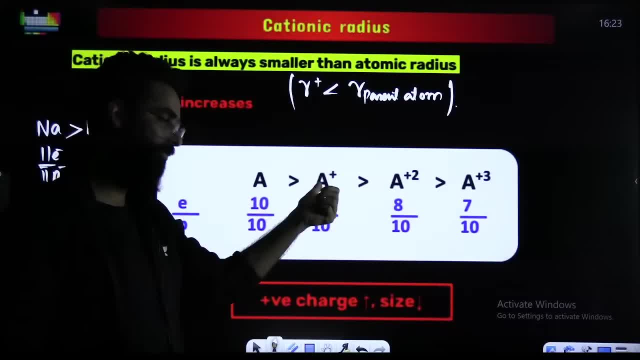 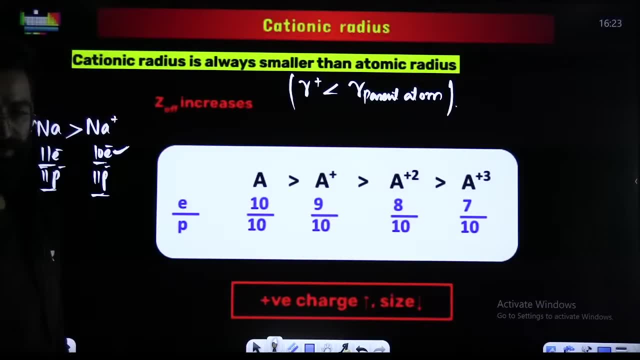 example, you have got atom a, then you are taking one electron out a positive. take one electron out eight, eight i positive. take one electron out eight a tri positive, a tri positive, perfect. right now you can easily define their radiuses, you can easily compare their radiuses. 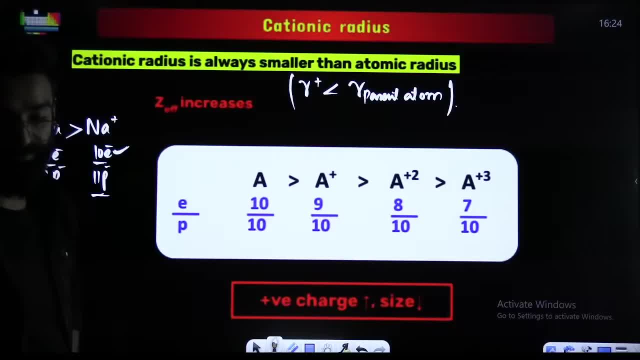 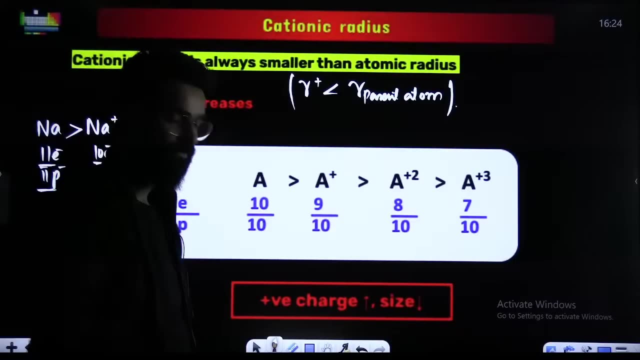 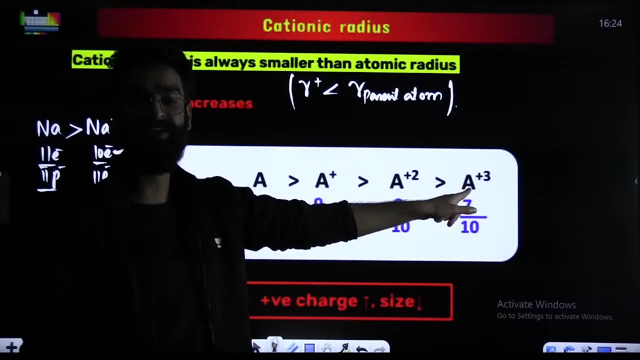 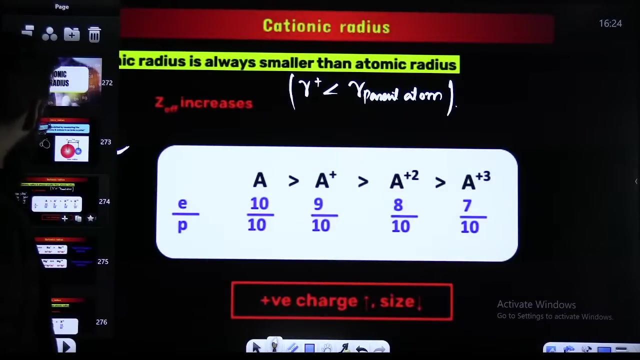 a p block will be done in class 12 in organic marathon. this is class 11, right? can you compare, guys? can you compare? can you compare? this one will be having the least radius because effective nuclear charge is maximum here. more effective nuclear charge, lesser the size. in short, in short, in short, 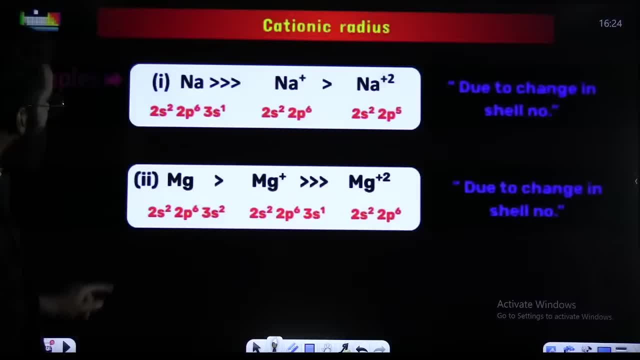 now, guys, here i have to tell you one more thing: na na positive, na2 positive, na na positive, na2 positive. we know, we know, when you take 1, 1 electron effect to nuclear charge increases size, decreases, right size decreases. get down to greatest decreases, get any greatest. 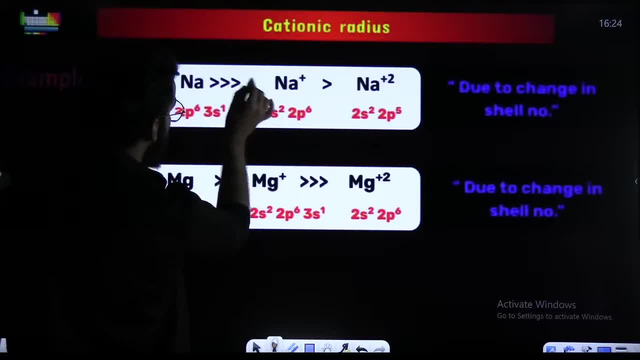 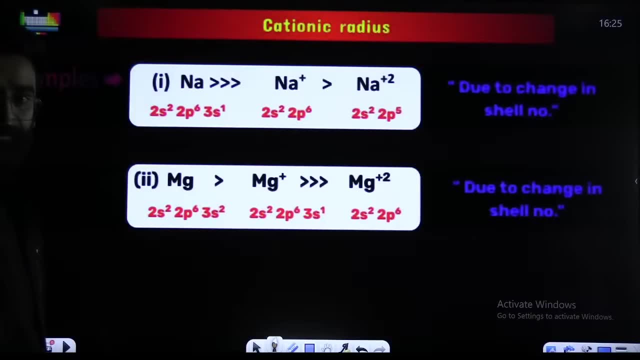 decreases. but do you see this, any size is far, far, far greater than than that of any positive, and over here it is not. why is that? why is that? because, if you see, here you had three shells, now here you have, you have, you have only two shells, right, so shell number is changing. 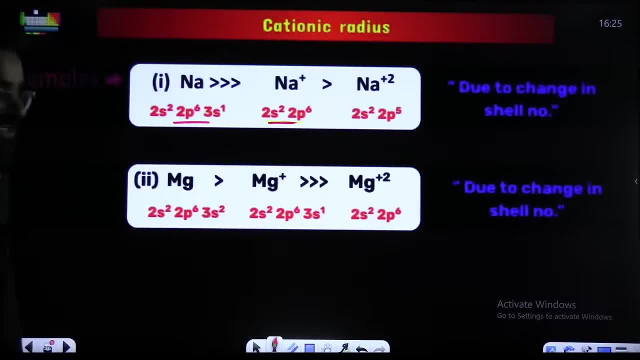 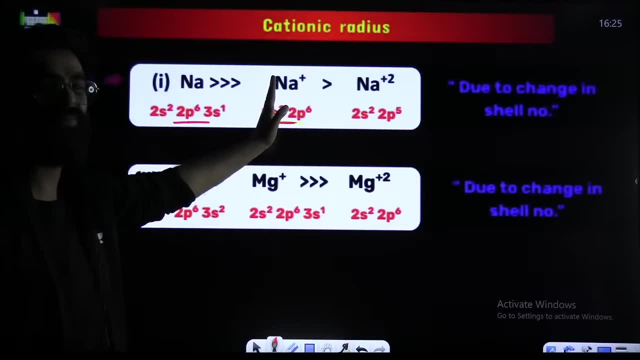 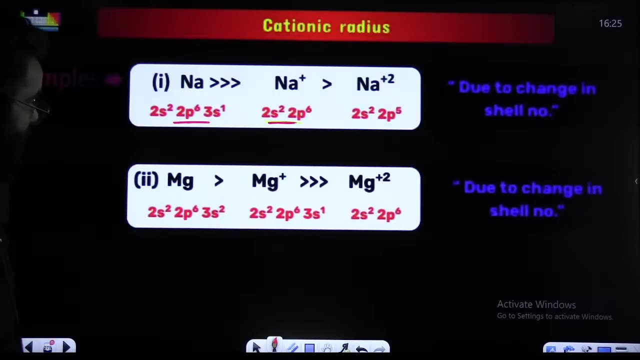 right. so shell number is changing. number is changing here, right. Shell number is changing Over here. you have got 3 shells, only 2 here, So the decrease in the size here is completely drastic. then decrease from here to here. Okay, Similarly, similarly, similarly when you take one electron out. 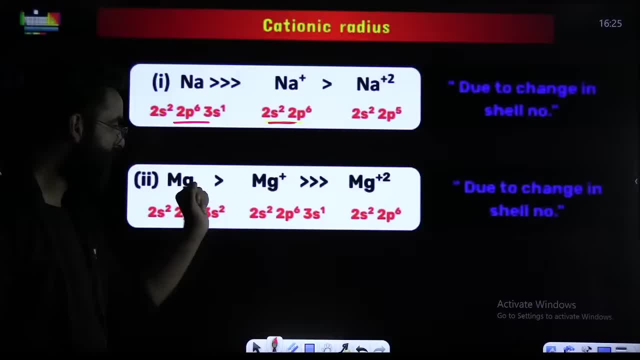 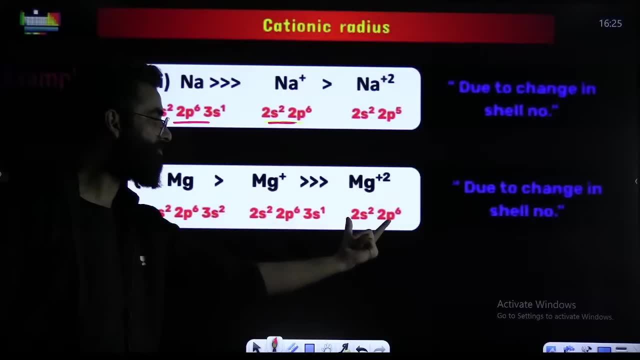 from Mg, it has to be from 3s. it gets converted into Mg positive. Now, when you are taking this electron out, right, Perfect, When you are taking this electron out, it becomes Mg di positive. Now, Mg di positive, there are only 2 shells. So, again, difference in the 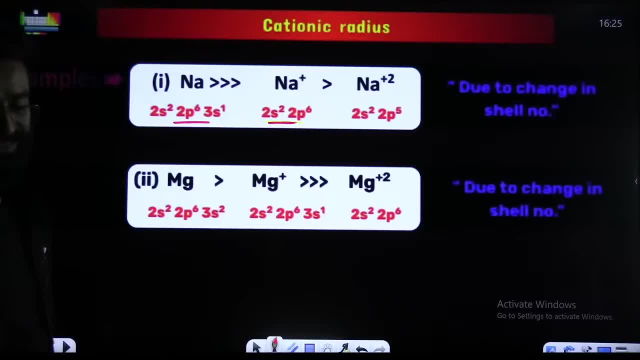 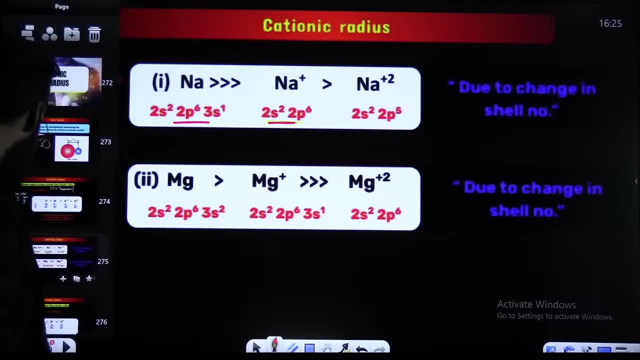 shells here. So that is the reason why drastic decrease, increase is happening because of the change in the shell number. I hope it is clear. I hope it is clear. I hope it is clear. Perfect. So till now it was about what It was about: the cationic species. Now, 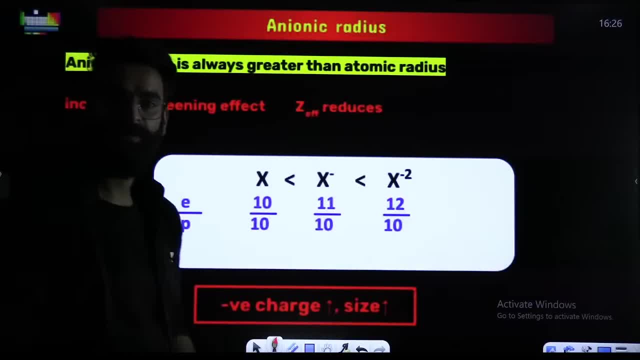 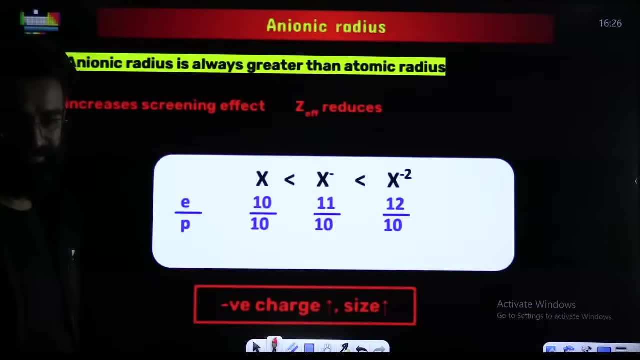 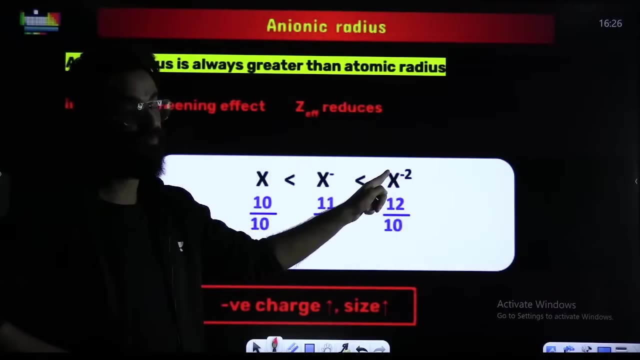 what about the anionic species? What about the anionic species? What about the anionic species? Talk about their size. Talk about their size X, X, negative, X, di negative. There are more electrons here. more electrons, same number. 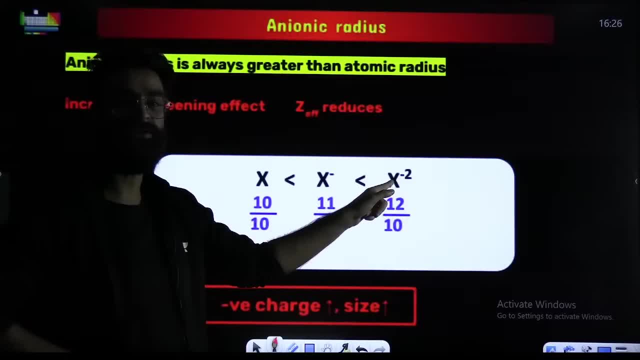 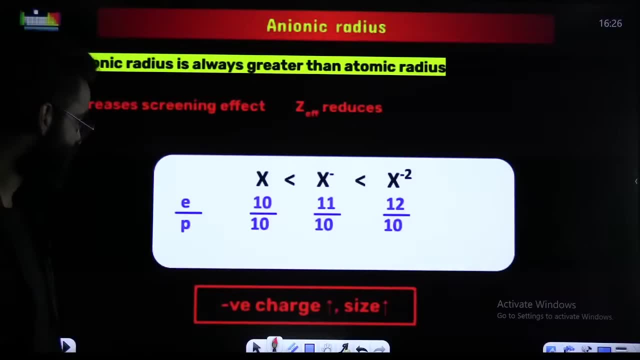 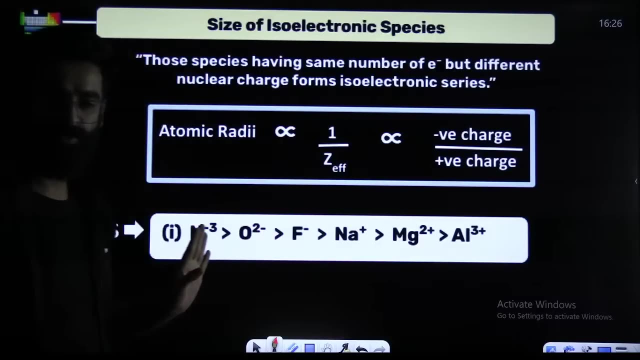 of protons everywhere. So nuclear charge, effective nuclear charge- is least here. Effective nuclear charge is least. Size will be maximum. Size will be maximum. Size will be maximum. Now, all these are isoelectronic species. isoelectronic species, How do you compare their size? They 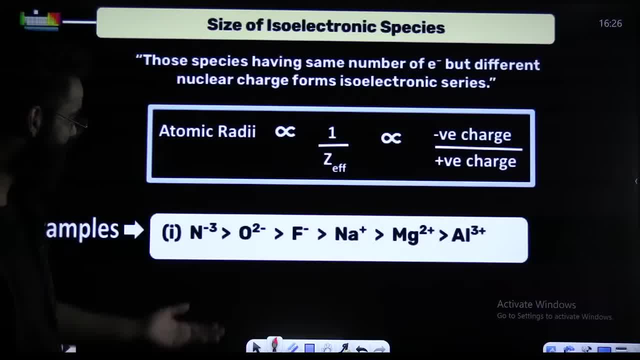 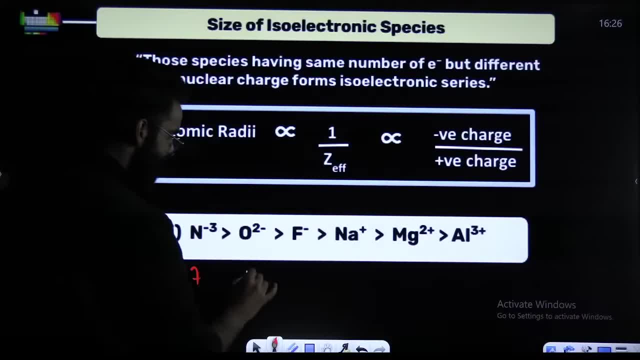 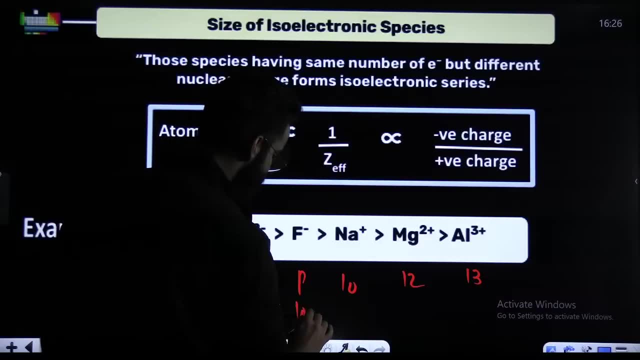 are almost equal as such, right? This is the very basic question: How do you compare their size On the basis of effective nuclear charge? on the basis of effective nuclear charge. this is the asked question. 10 electrons, 10 electrons everywhere. Now talk about protons. 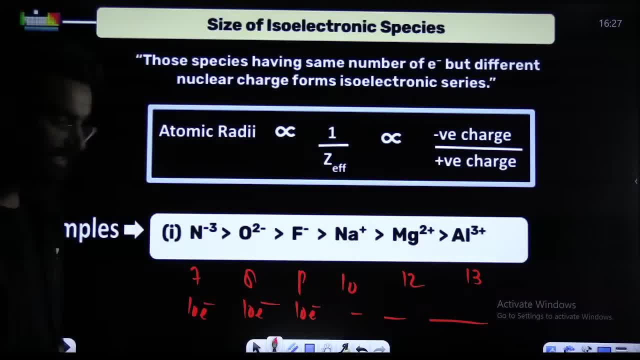 7 protons, 8 protons, 9 protons, 10 protons, 12 protons, 13 protons. Electrons are same everywhere: 10 electrons, 10 electrons, 10 electrons. everywhere electrons are same. Where is the effective nuclear charge? more Effective nuclear charge is more. in the last case, More the effective nuclear charge, lesser is going to be the size Right, Lesser is going to be the size. So you can talk in terms of this as well. 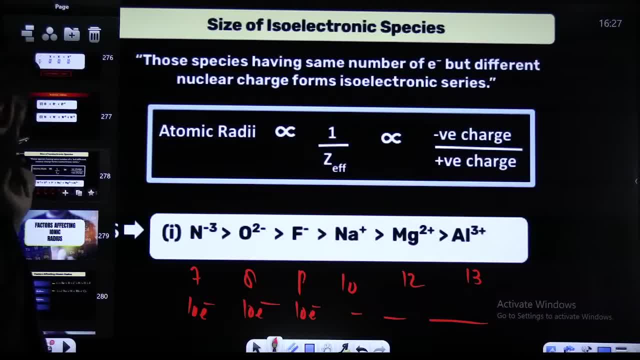 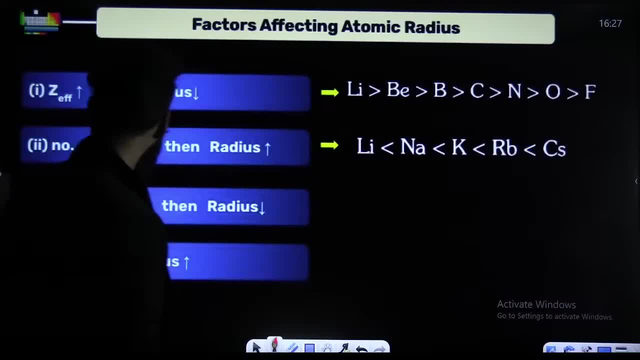 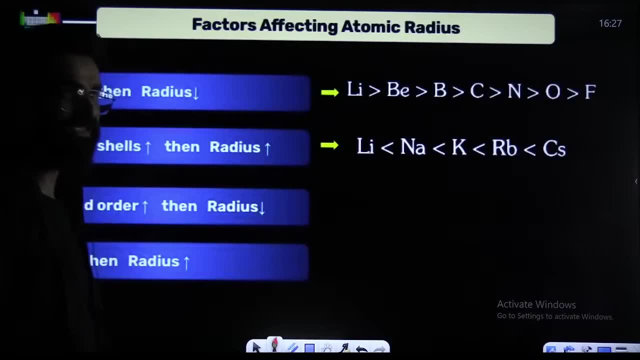 one, Correct guys. What are the factors? what are the factors which exactly affect the radius? atomic radius, Ideas, students, there are few factors which exactly affect the radius. One is effective nuclear charge. You should be knowing it right: Radius and effective nuclear. 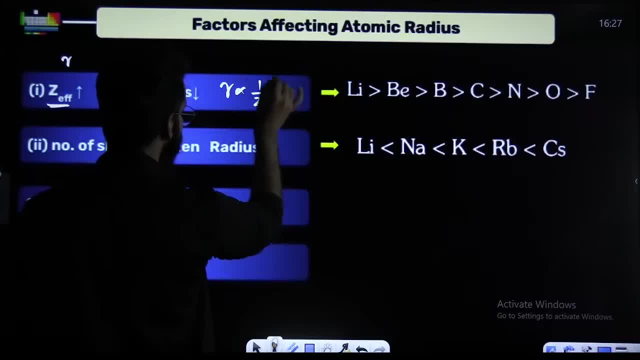 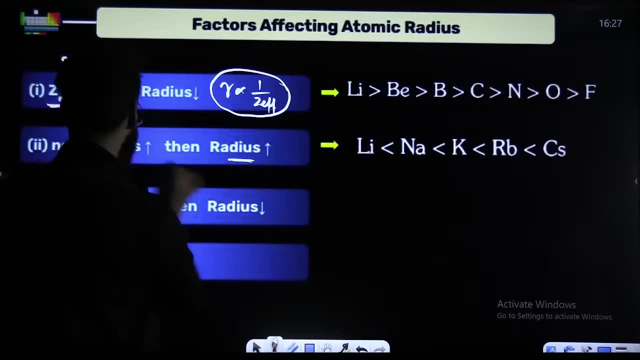 charge. Radius and effective nuclear charge. They are inversely proportional. right More the effective nuclear charge, lesser the radius. This is one of the factors. Number of shells increases. radius increases. You know this right. Radius depends on number of shells. 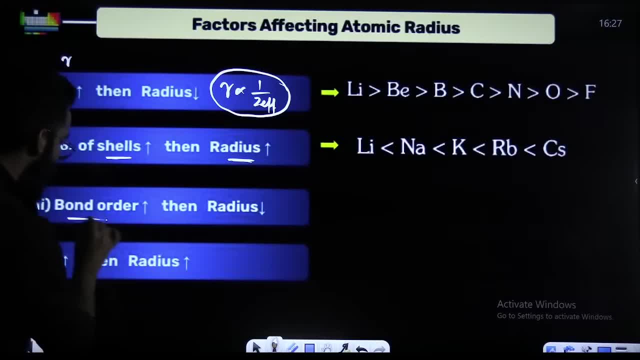 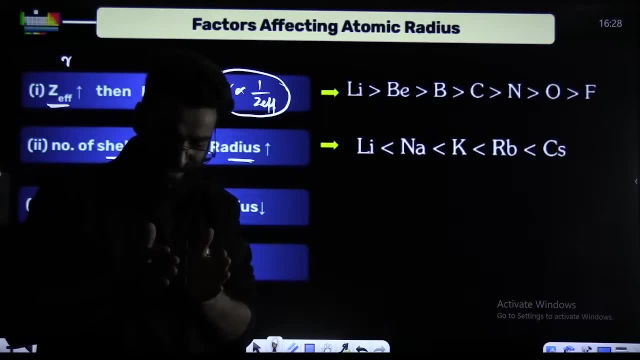 as well. More the shells, more the radius. Third is bond order. Bond order means number of bonds in between. More the bonds, more force of attraction. More the bonds, more force of attraction. Lesser the inter-nuclear distance, lesser the radius right, So more. 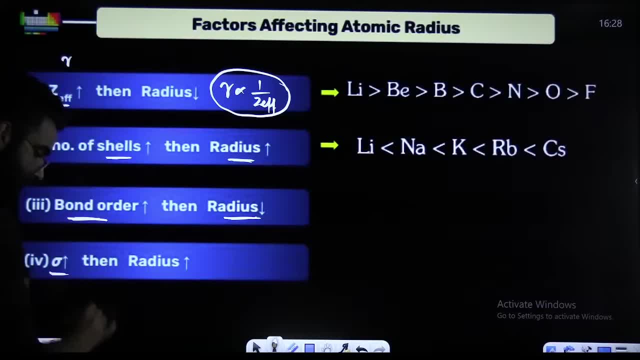 the bond order, lesser the radius, Perfect Cleaning, constant Sigma. It represents what Repulsions, Which, which, which inner shell electrons, which inner shell electrons are going to do with the outermost electron. More the repulsions, more the repulsions, more is going to be the radius, More the repulsions. 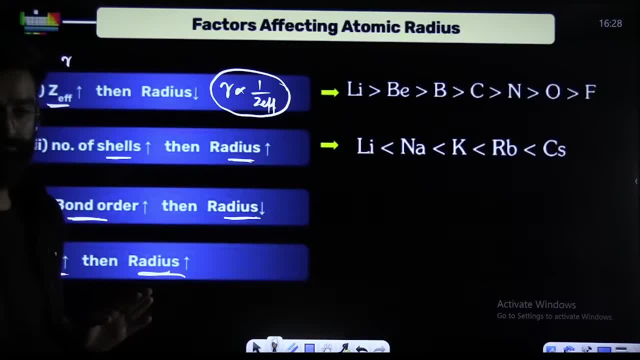 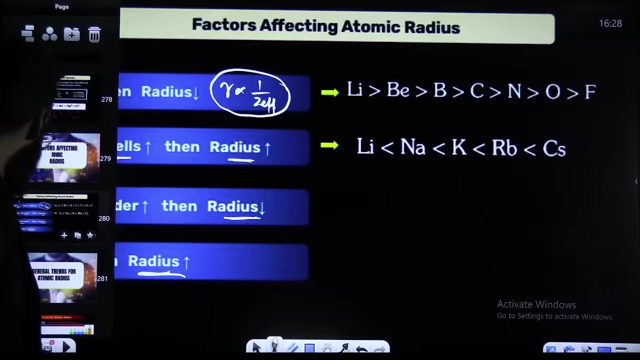 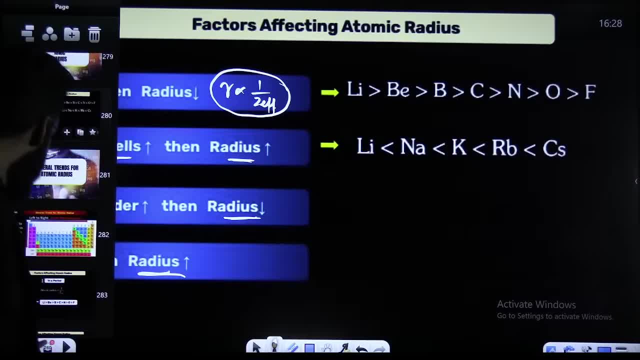 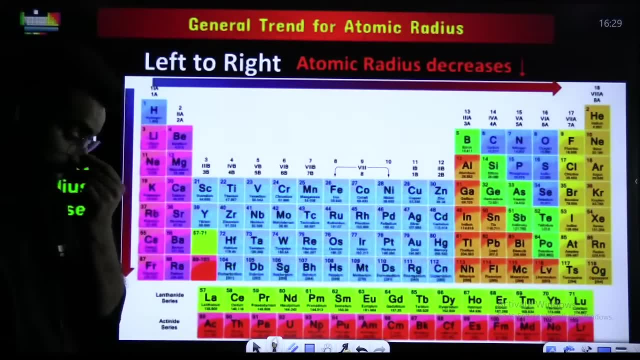 here now What happens- General trends you should know- on moving from left to right. On moving from left to right, what happens to the effective nuclear charge? Effective nuclear charge increases, Therefore atomic radius decreases. Okay, So what happens to? 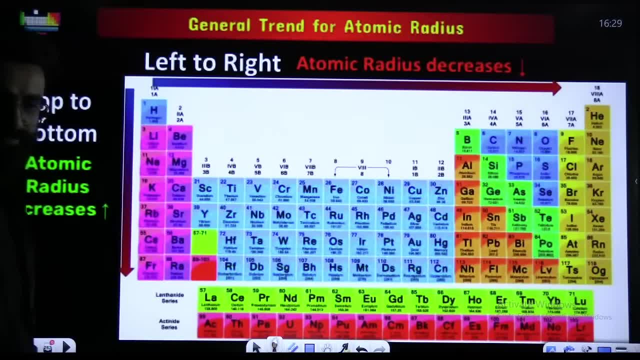 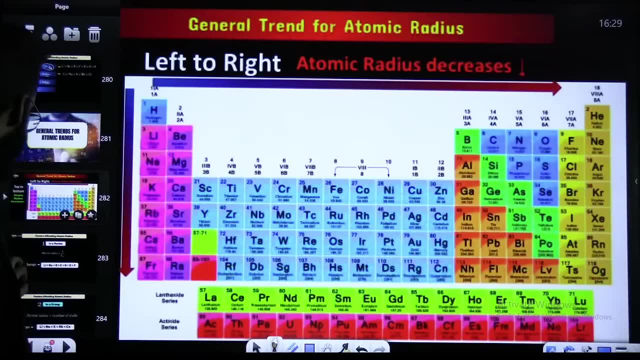 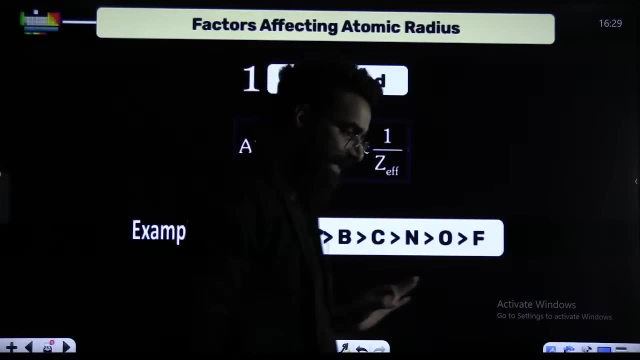 the effective nuclear charge. Effective nuclear charge increases. Therefore, atomic radius increases Down the group. atomic radius increases Left to right. atomic radius decreases Due to increase in the effective nuclear charge. down the group the atomic radius decreases. Okay, Now, people, whenever you need to compare atomic radius in the period, whenever you need, 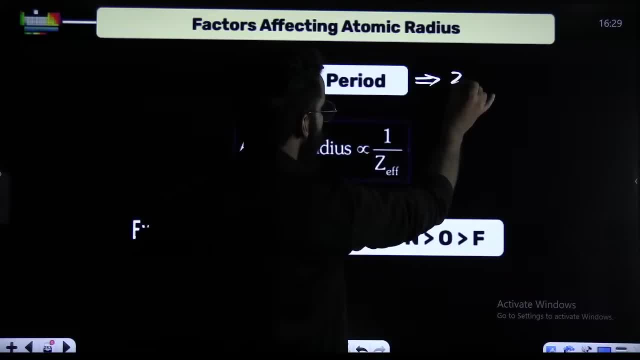 to compare atomic radius in the period. you will be comparing it with the help of effective nuclear charge And you know atomic radius that is inversely proportional to Z effective, For example, lithium, beryllium, boron, carbon, nitrogen, oxygen, fluorine- they belong to. 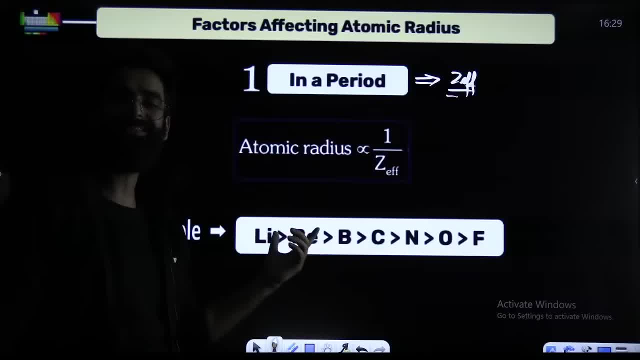 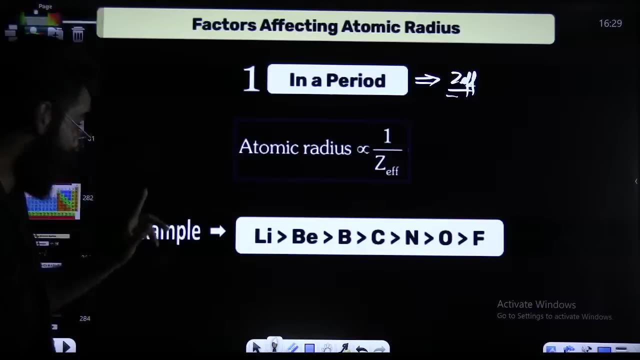 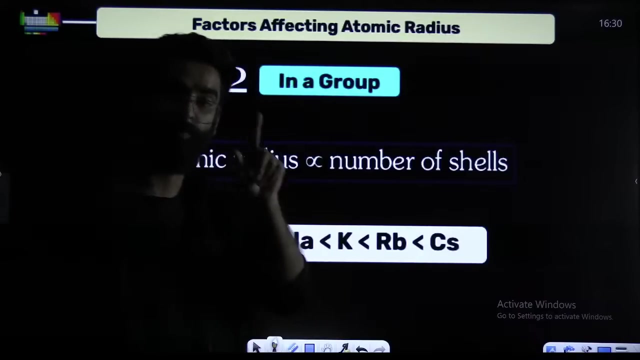 same period. So you will be comparing their atomic radius. with the help of what? With the help of effective nuclear charge. On moving from left to right, effective nuclear charge increases. Size automatically decreases. I mean the atomic radius decreases, Perfect. But in a period, In a period In the group, if you need to compare in the group, if you 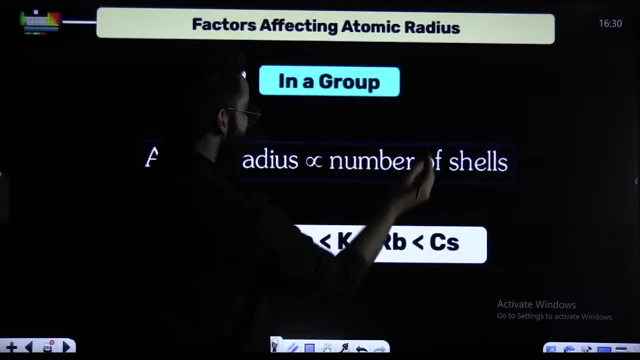 need to compare the atomic radius. you will be comparing it with the help of number of shells. So when you move from, for example, group 2 to group 3, shell number increases. 3 to 4, shell number increases. 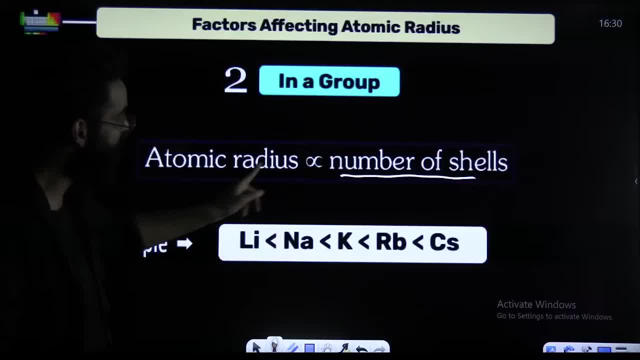 Perfect Right, Okay, So atomic radius is directly proportional to number of shells. So, on moving from top to the bottom, number of shells increases. That is the reason why atomic radius also increases. That is the reason why atomic radius also increases. 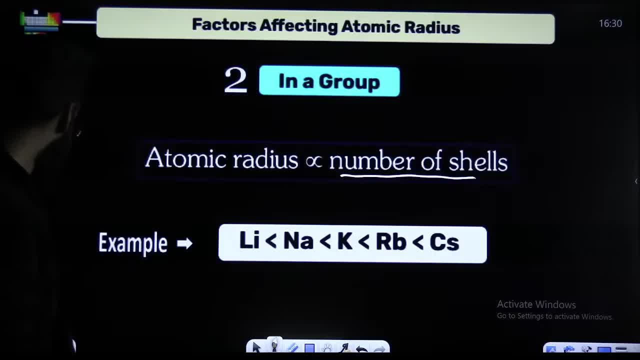 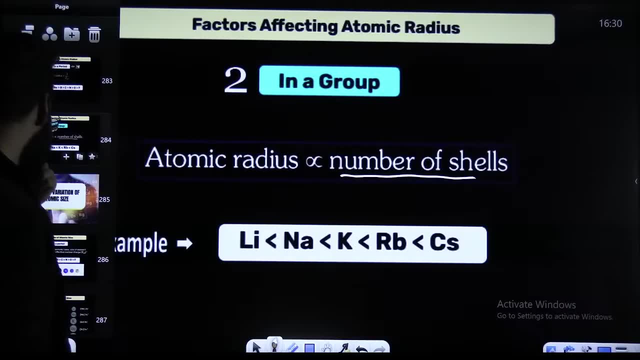 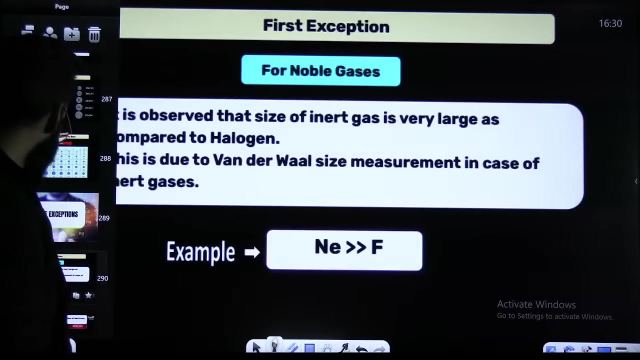 Lithium, sodium, potassium, rubidium, cesium Down. the group atomic radius increases Correct, Correct people, Okay, Okay, Just a second. Remember this particular exception over here. Well, you should be knowing it by now. 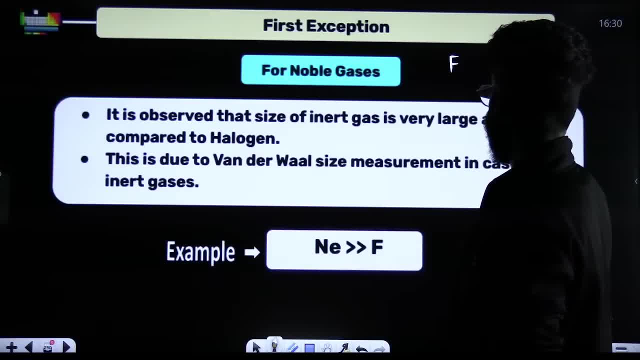 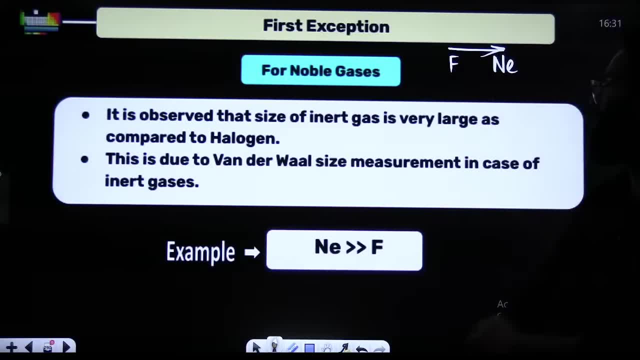 Let us say you are comparing fluorine with neon, Fluorine with neon- Same period. On moving from left to right. On moving from left to right, What happens? Size Size generally in the period decreases because effect of nuclear charge increases. 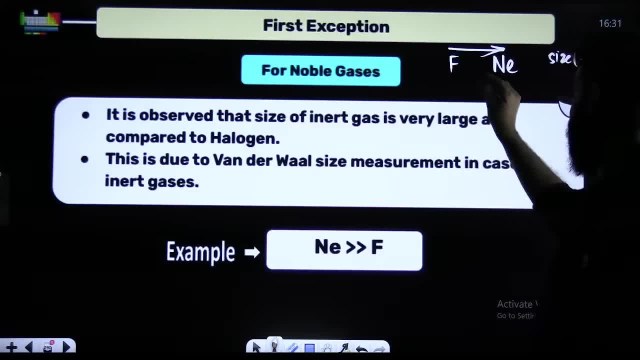 So it is. we are expecting fluorine should have more size than neon, But what happens? Neon has got more size than fluorine. It is the actual thing. Why is that? Because neon is a noble gas. For noble gas, what do we define? 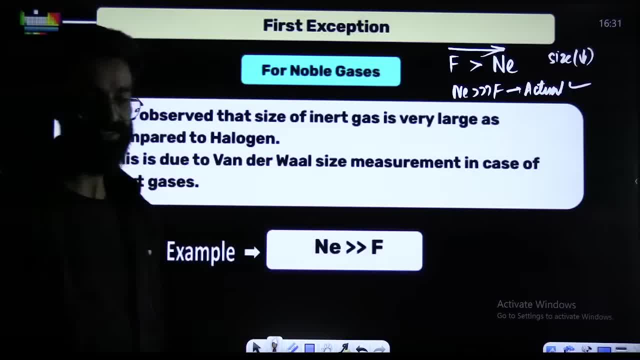 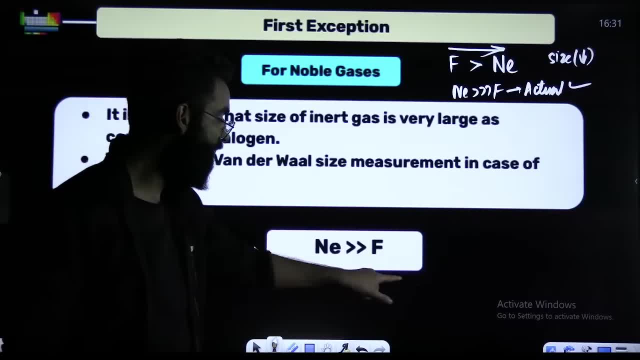 We define Van der Waals radius, And you know Van der Waals radius is far greater than covalent metallic, Ionic, etc. So do remember this particular thing: The size of neon will be basically the size of noble gases. 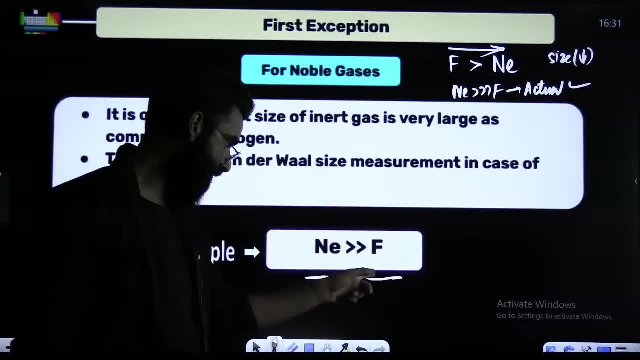 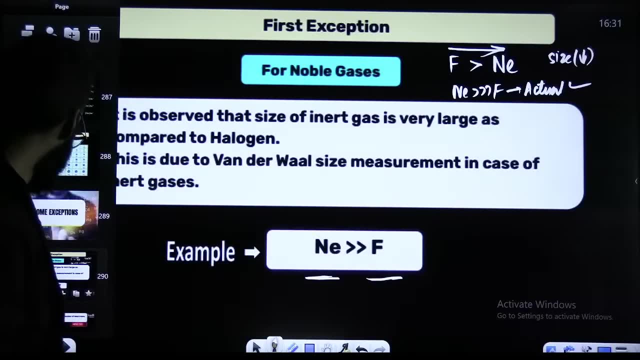 Perfect. In this particular case, size of your noble gas neon will be greater than that of fluorine. Remember this particular thing as well. It can be asked. It can be asked, Alright. These are some species which are given to us. 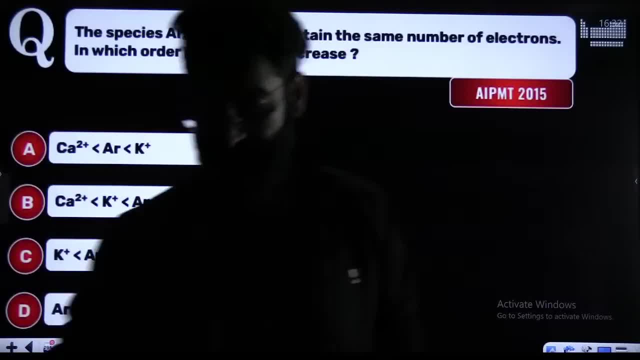 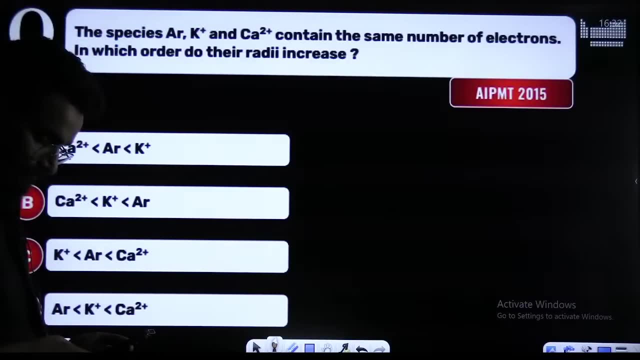 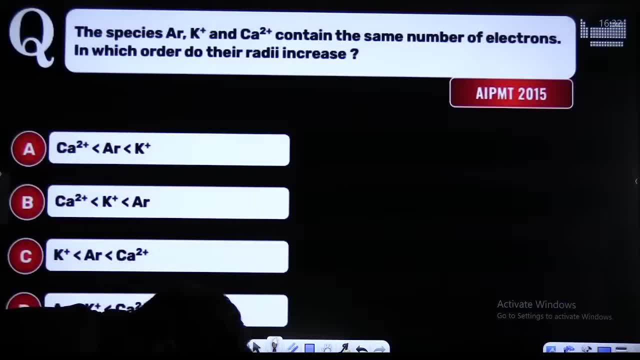 What is the correct answer of this question? What is the correct answer of this question? Anyone wants me to solve this? These are isoelectronic species, right? More the effect of nuclear charge, lesser the size. More the effect of nuclear charge, lesser the size. 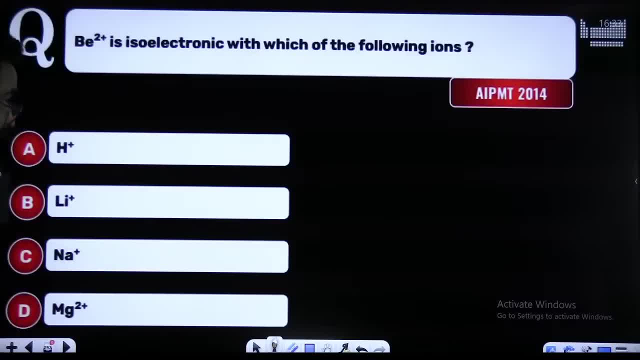 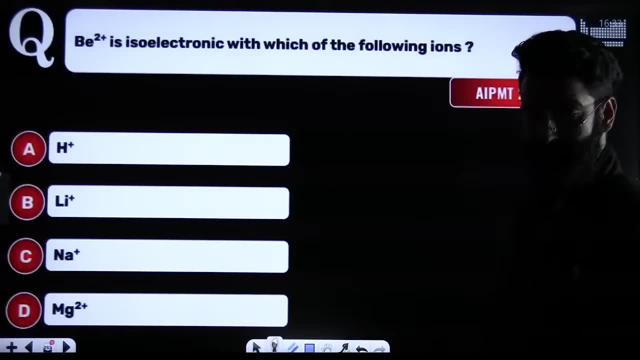 These are isoelectronic species. Tell me the answer of this one. Tell me the answer of this one. P di positive is isoelectronic with B di positive Contains how many electrons? P di positive contains 2 electrons. 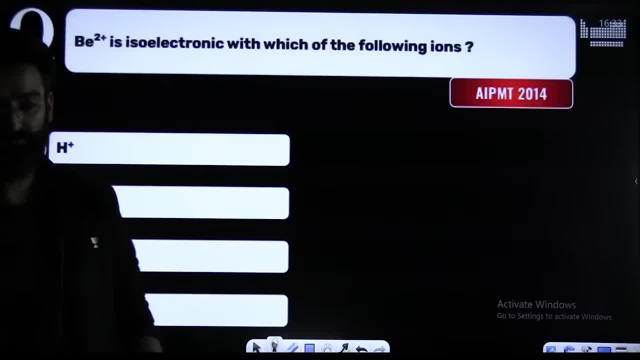 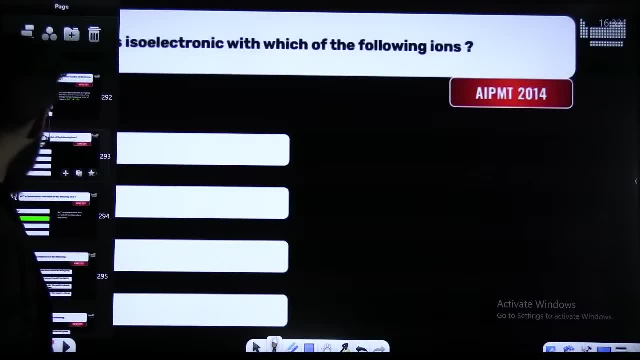 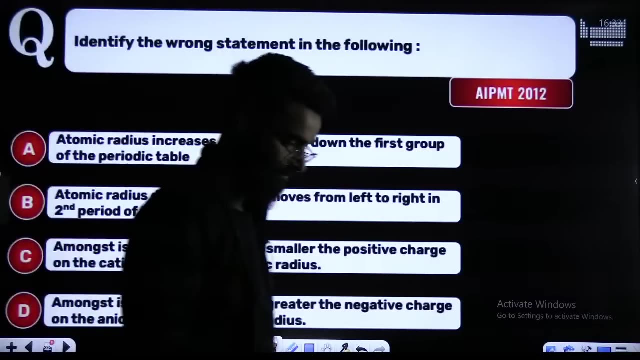 Now, which of the following here contains 2 electrons Li positive? Right Li positive also contains 2 electrons Li positive. What is the answer of this one? Identify the wrong statement in the following Wrong statement. Identify the wrong statement. 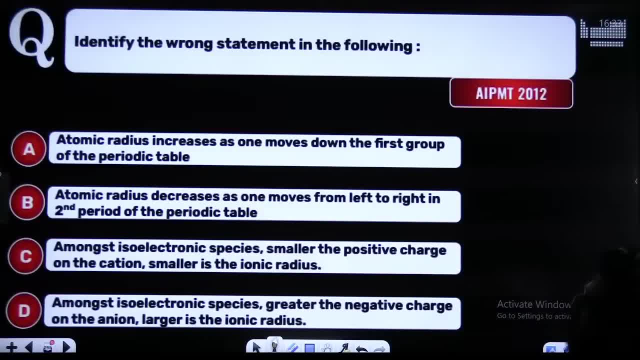 Quickly. Atomic radius increases as one moves down the first group. This is correct. Atomic radius decreases as one moves from left to right in the second period. Correct: Among isoelectronic species, smaller the positive charge on cation, smaller the ionic radius. 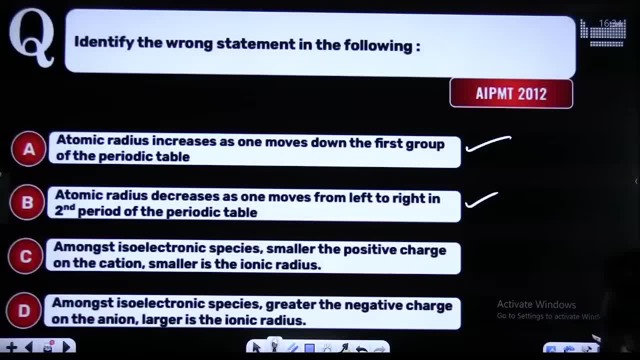 Atomic radius increases as one moves from left to right. in the second period, Smaller the positive charge on cation, smaller the ionic radius, Smaller the positive charge on cation. If there is more positive charge, lesser will be the size. 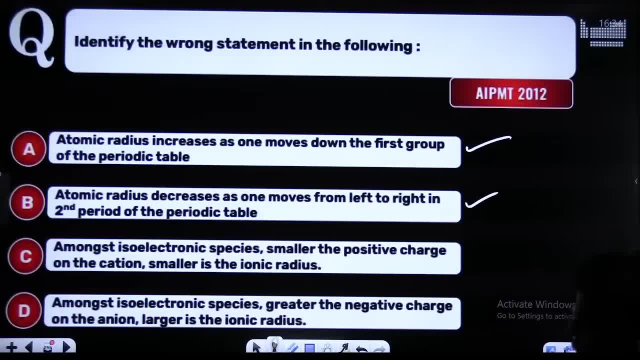 Right. More positive charge, lesser size. So it is reverse, Not correct. Greater the negative charge, larger the anionic radius. Option C is the one which is incorrect. Right, All these type of questions you should be able to solve, by the way. 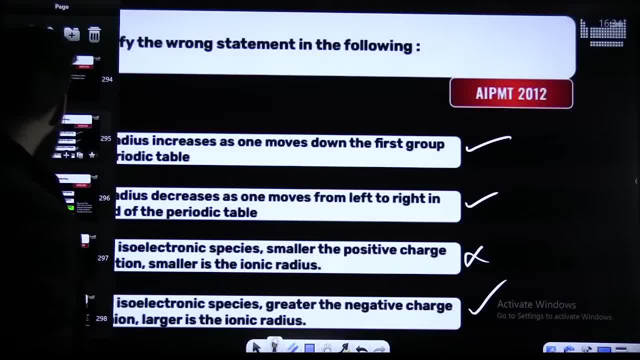 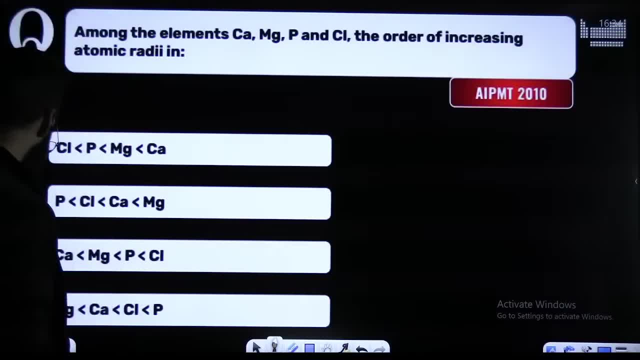 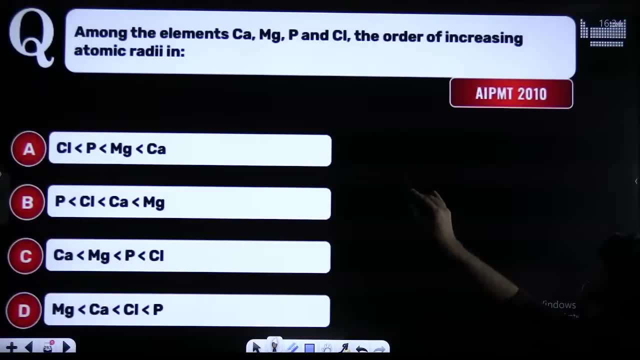 Okay, What do you think about this one? What do you think about this one? Quickly, Quickly, guys. Magnesium you have, Calcium you have. These are group second. Okay, These are group second. These are group second. Phosphorus you have here. 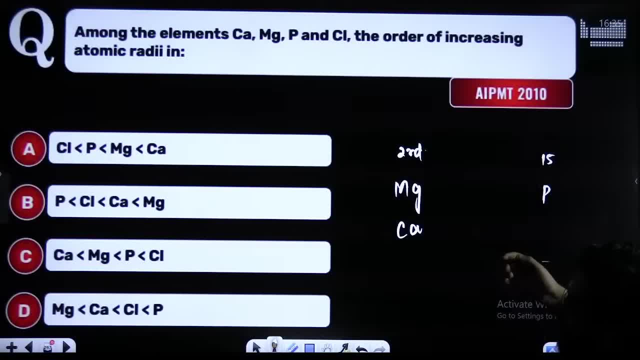 Okay, That is group 15.. Then you have got one more. Which one? Chlorine. This is group 17.. What is the correct answer? Okay, What is the correct answer? people Think over it Quickly. everyone, Among the following: the order of increasing atomic radii: 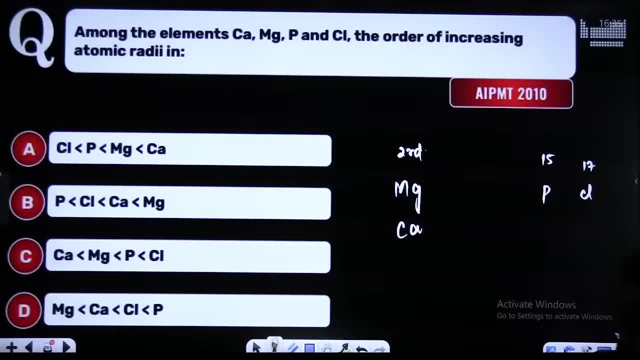 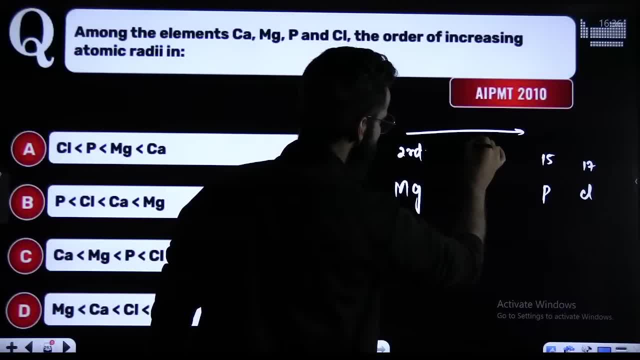 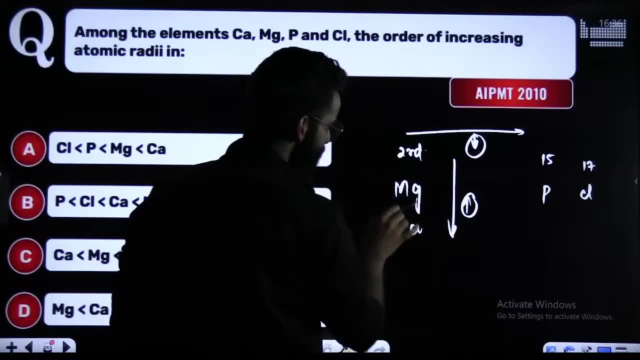 No, Absolutely guys. See, on moving from left to right, radius decreases. Top to bottom It increases. Correct Perfect: These 3, they belong to same period. Now here cell number is getting increased, So calcium have maximum radius Right. 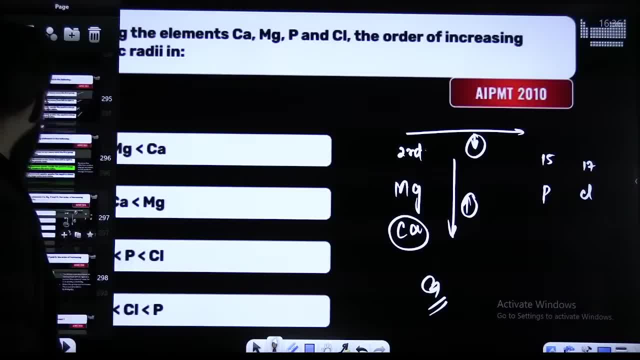 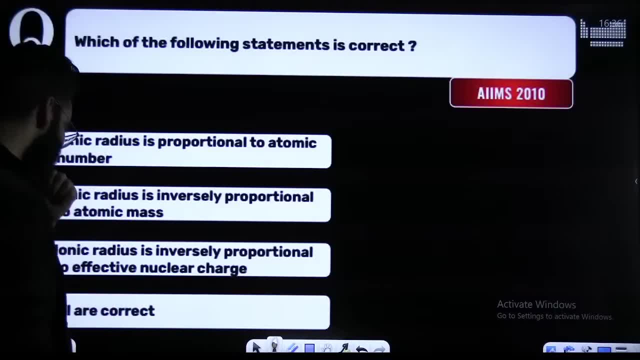 There is only one option which says calcium having maximum. That's option A. That is option A. What about this one? This has to be here. What about this one In your class 11th? in organic there are only two chapters: bonding and periodic classification. 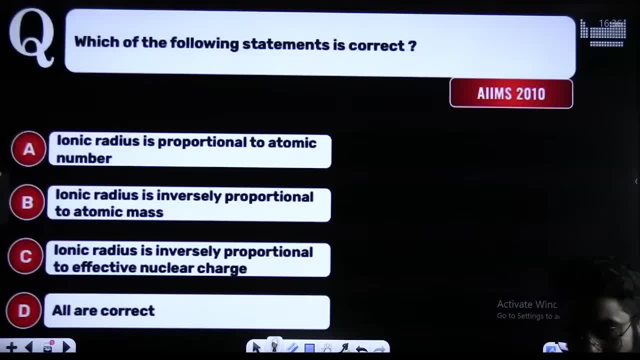 Your p block is from 12th part. now that will happen in class 12th in organic marathon. Quickly, which of the following statement is correct? Ionic radius is proportional to atomic number. Is that correct, Guys? look carefully, Look carefully. 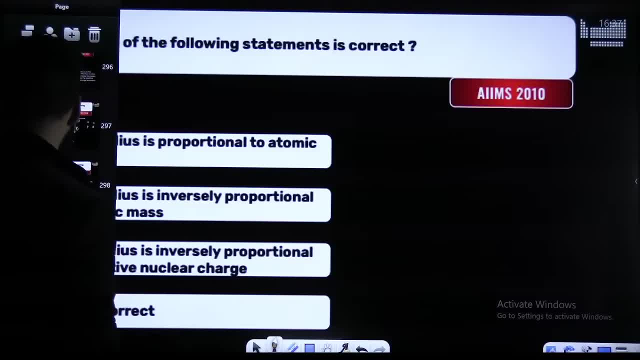 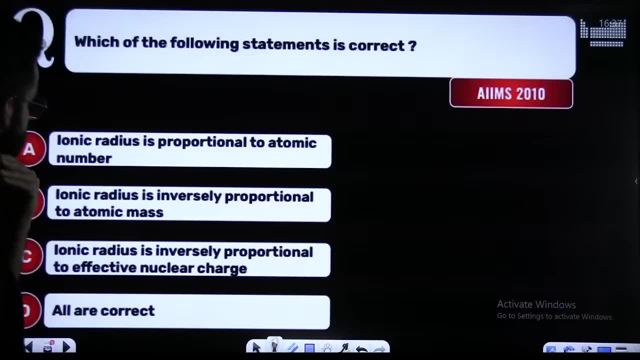 Be careful, Read all the statements carefully. Read all the statements carefully. I don't want you guys to make a mistake here. I don't want you to make a mistake here. read carefully. Atomic radius is proportional to atomic number, Is that? 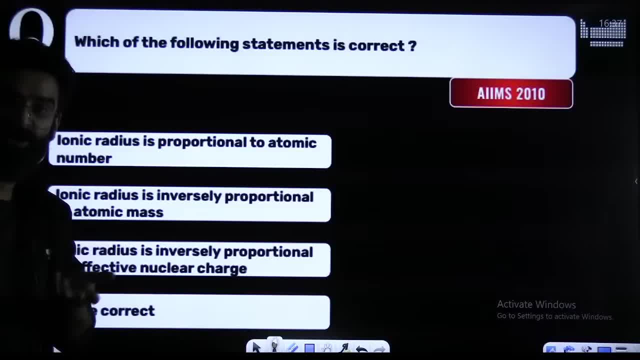 On moving from left to right, atomic number is increasing. Is atomic radius increasing? No, it decreases. on moving from left to right, No doubt Atomic number increases. At the same time atomic number increases. Does that mean atomic radius increases? 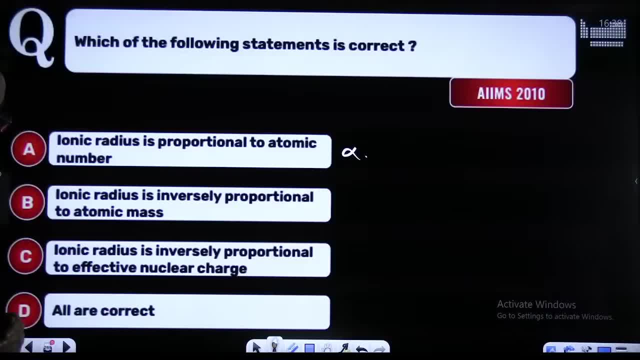 No, This is wrong. Did I ever talk in terms of atomic mass On moving from left to right? atomic mass increases. If atomic mass increases on moving from left to right, atomic mass no doubt is increasing, But is the atomic radius increasing? 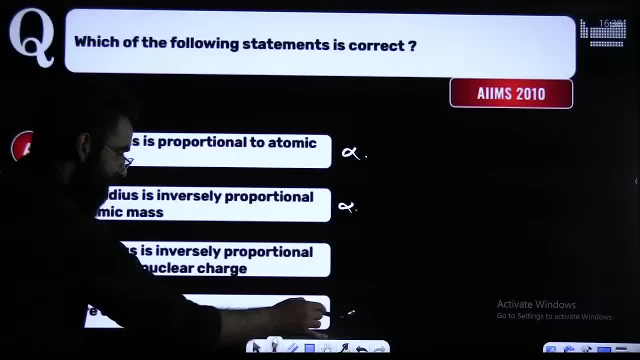 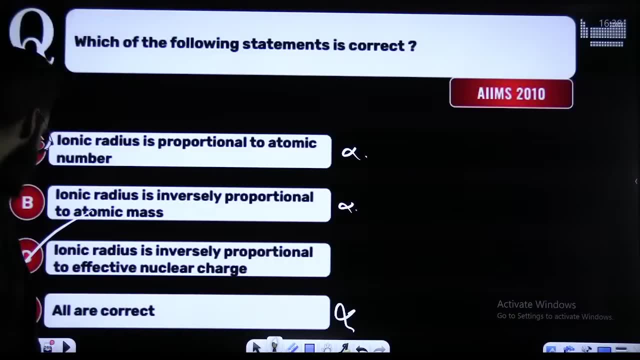 That is decreasing. It is wrong. So option D cannot be the answer. There is only one left, That is C. So be careful with these sort of questions. They can play with the words. They can play with the words, guys. They can play with the words. 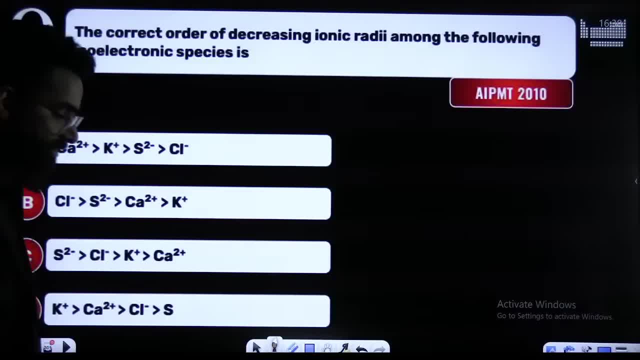 Tell me the answer of this question quick. The correct order of decreasing ionic radius. These are all isoelectronic Check the number of protons: More protons- lesser size. More protons- lesser size. Right: More protons- lesser size. 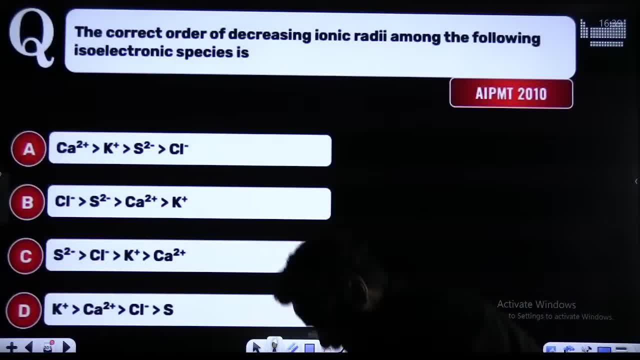 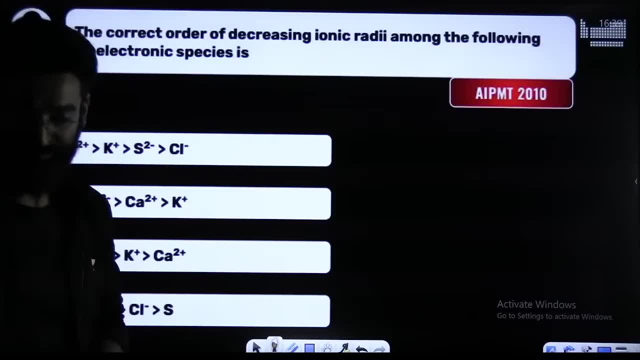 Redox does not belong to inorganic. Redox belongs to physical. It will be done in physical chemistry marathon of class 11th. No need to worry about that. Okay, Thank you, Bye, Bye, Bye, Bye, Bye. 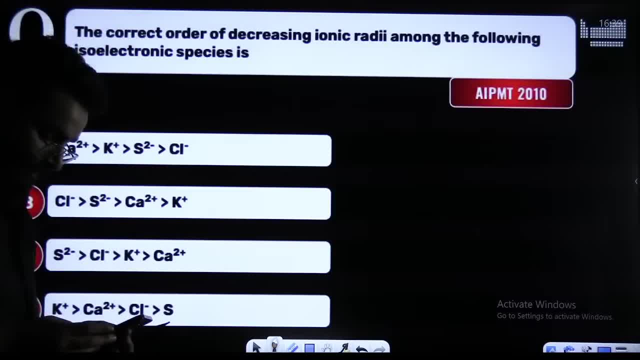 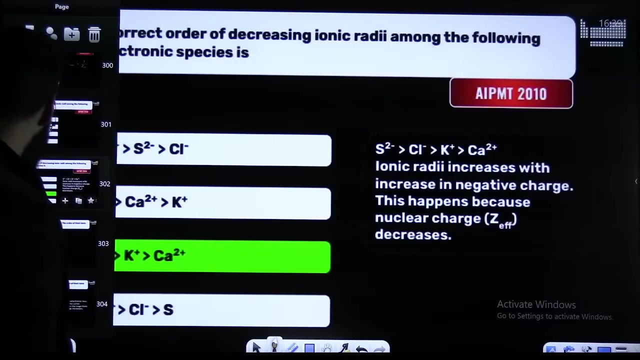 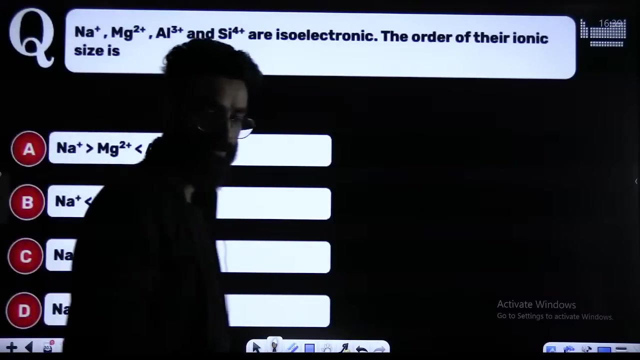 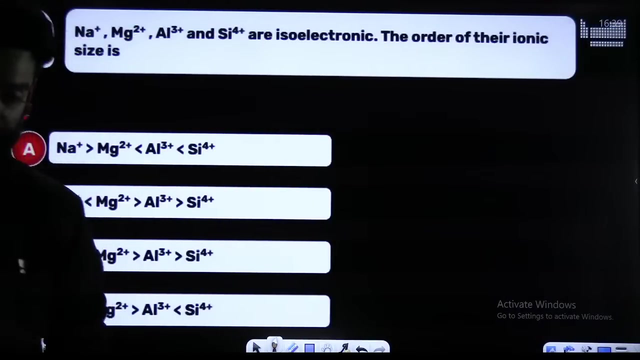 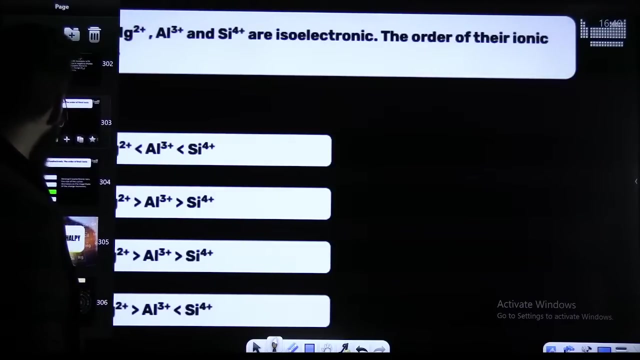 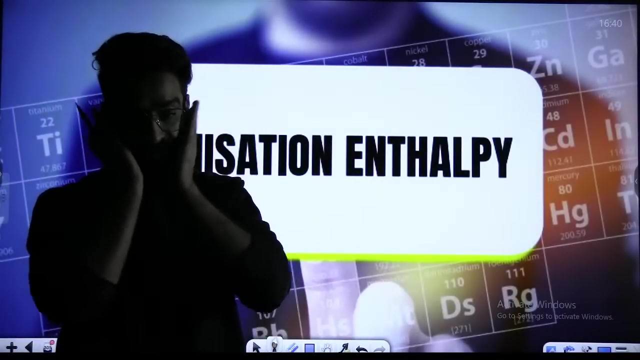 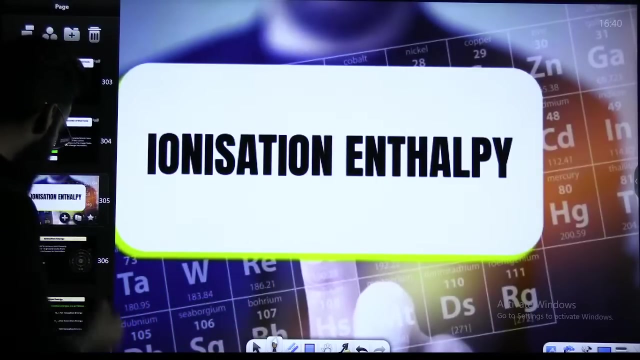 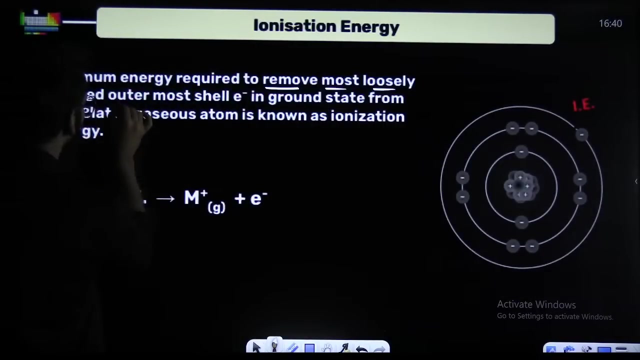 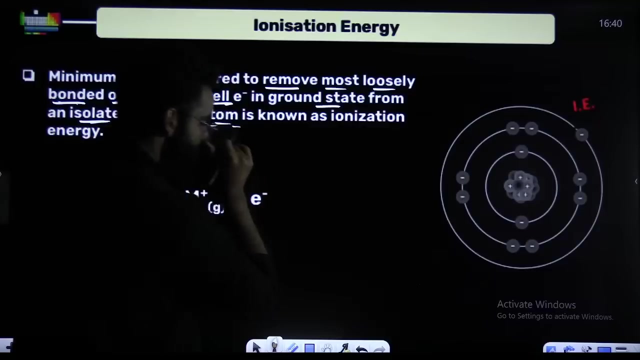 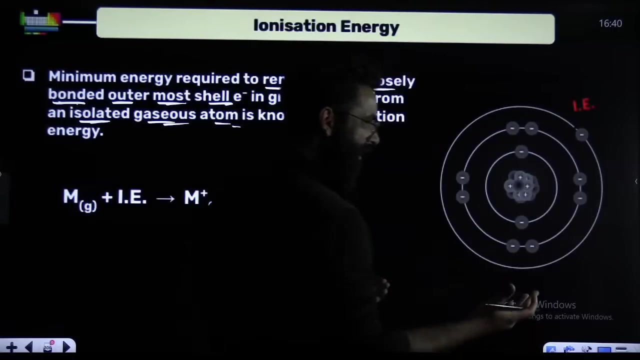 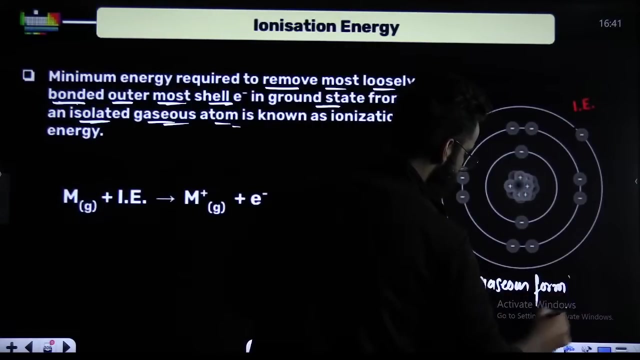 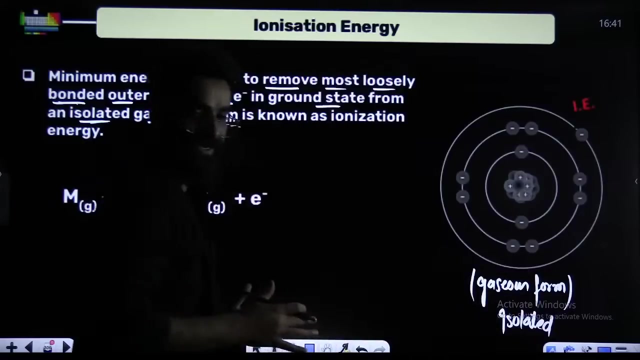 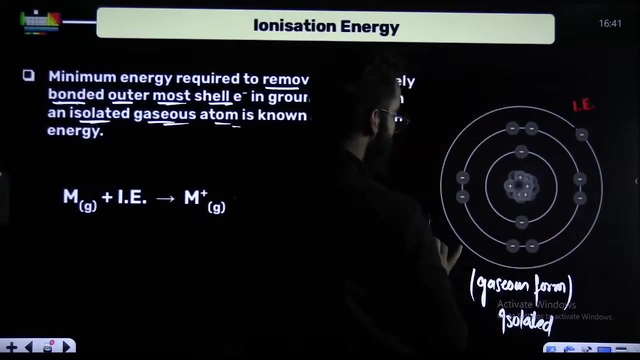 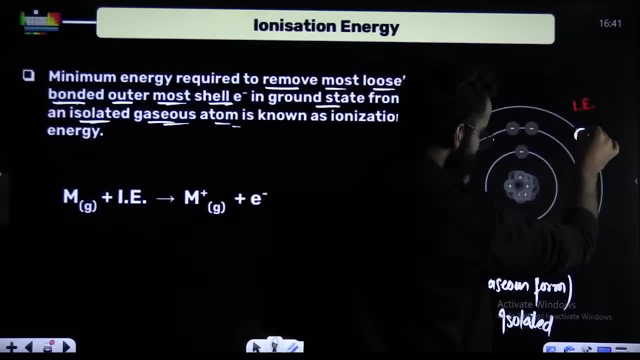 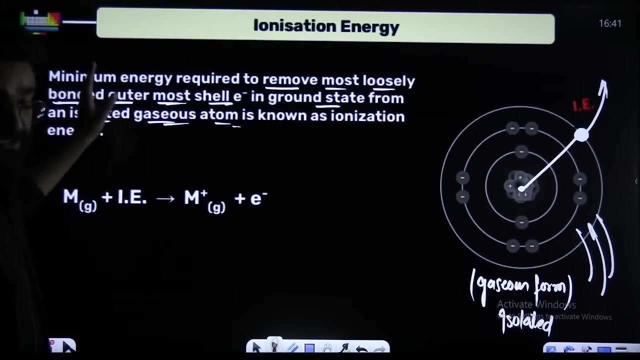 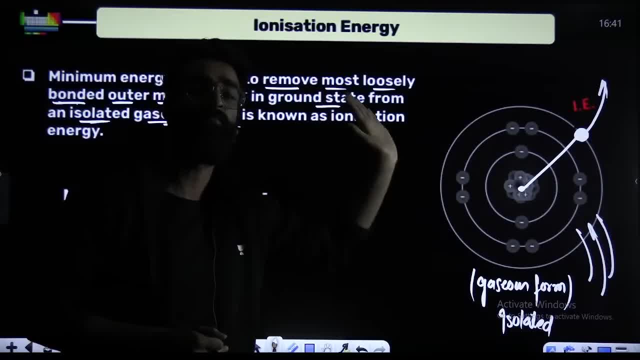 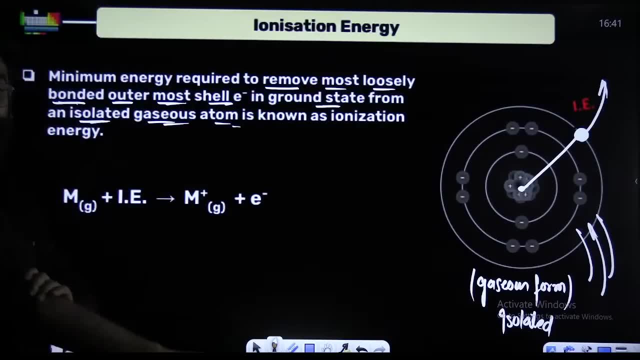 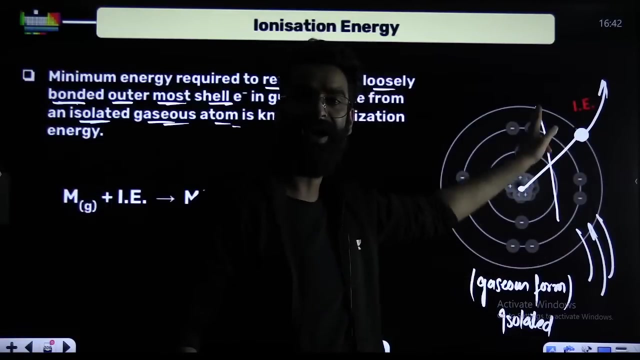 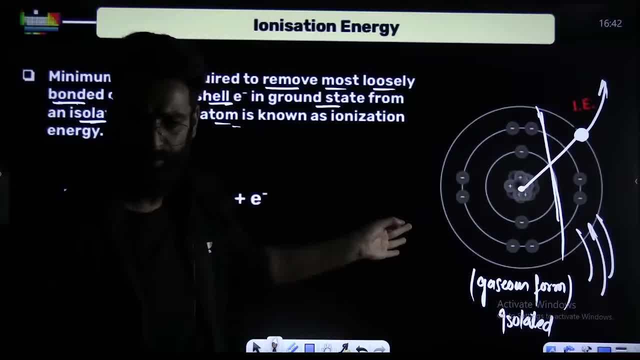 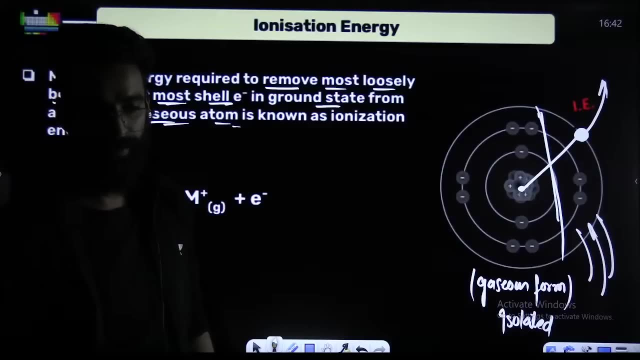 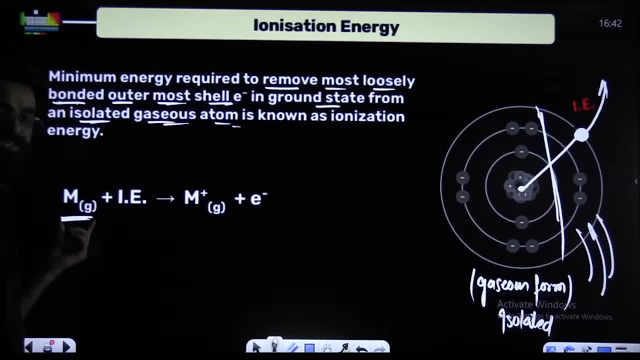 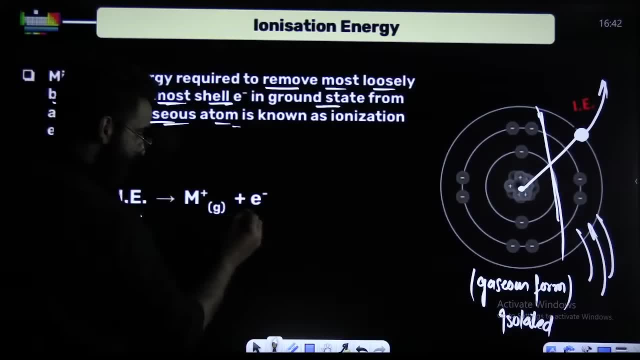 So, for example, you have got the metal, you have got the element which is in Isolated gaseous form. if you are giving it the Ionation energy, that means you are taking the electron out, the last electron you are taking out, and this atom gets converted into its cation. 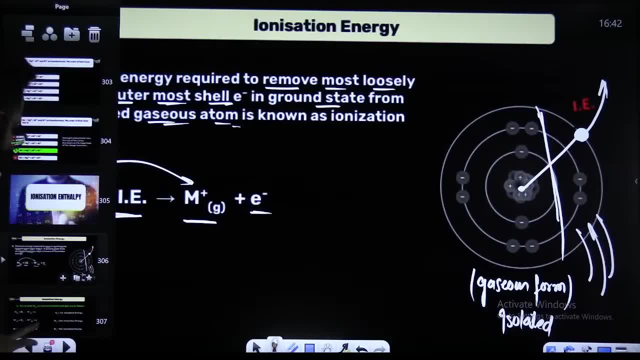 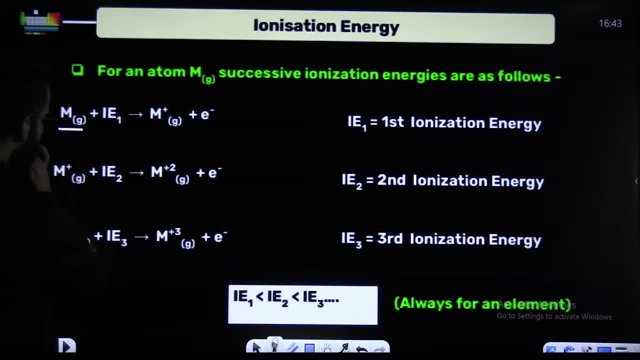 Very simple Now, if you talk about the consecutive Ionation energies, the consecutive Ionation energies, the successive Ionation energies, see guys, for example, you have got the element 1, you are giving it the Ionation energy. so you are taking one electron out, it is getting. 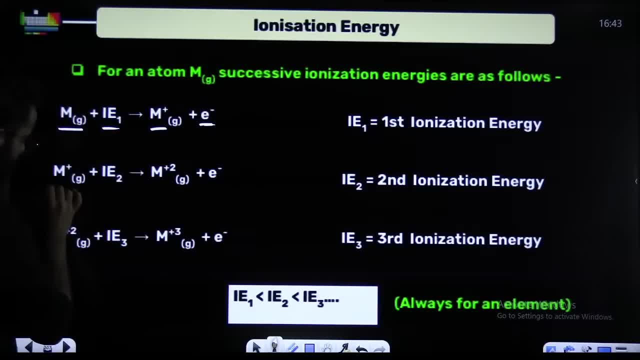 converted into M positive. perfect. Now, from this M positive you are giving, you are taking one more electron out. by supplying this much amount of energy, it gets converted into M dipositive. Now, from M dipositive again, you are giving Ionation energy right and taking one more. 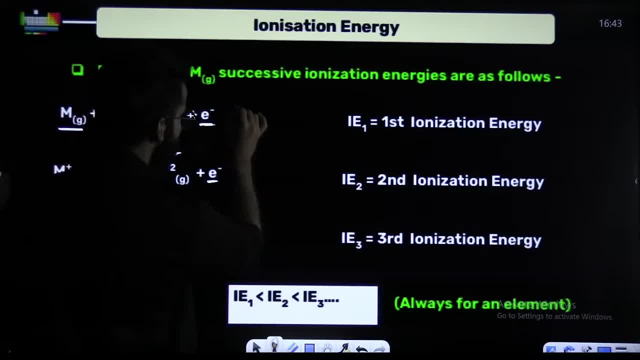 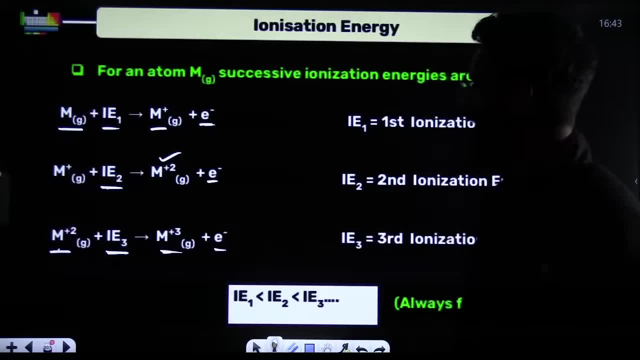 electron out, Perfect. What about these successive Ionation energies? right, What about these successive Ionation energies, guys? This is pretty much simple understand. For example, this had this was neutral. there were 7 protons, 7 electrons, for example. 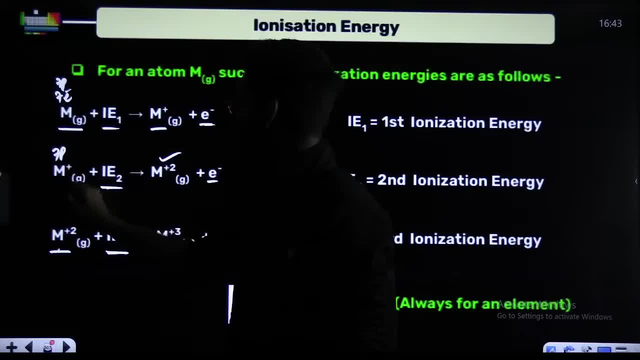 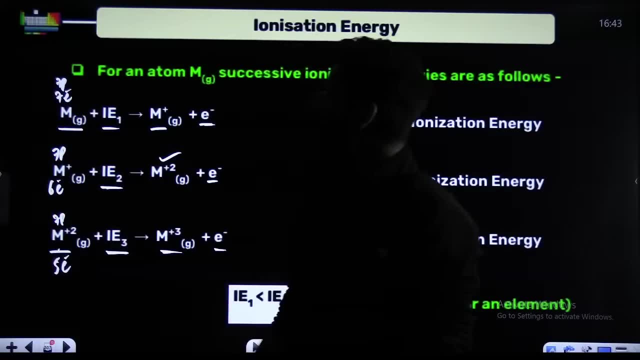 But here it got converted into M positive, so there will be 7 protons, but there will be only 6 electrons. right And over here there will be 7 protons, but only 5 electrons. perfect. So M M positive, M dipositive. 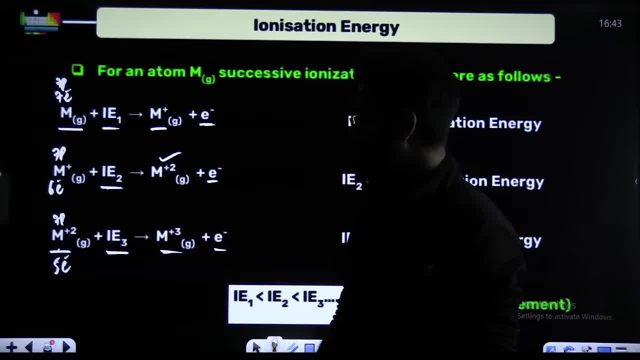 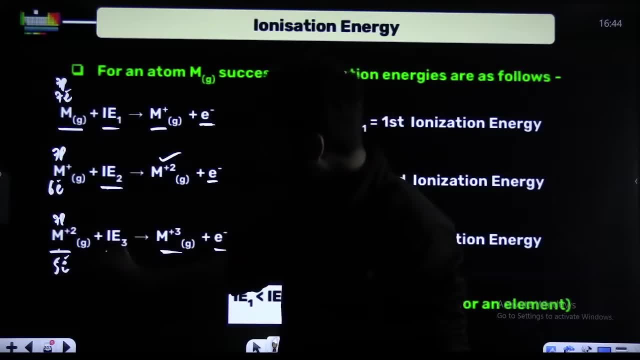 Perfect: M M positive, M dipositive, M M positive, M dipositive. 7 protons were holding 7 electrons. but 7 protons are holding only 6 here, only 5 here. The force of attraction which is experienced by the outermost electron here will be maximum. 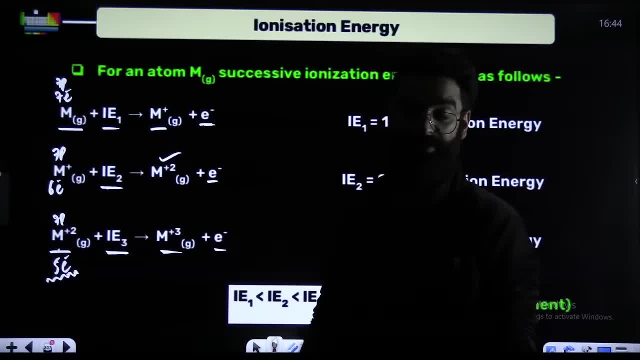 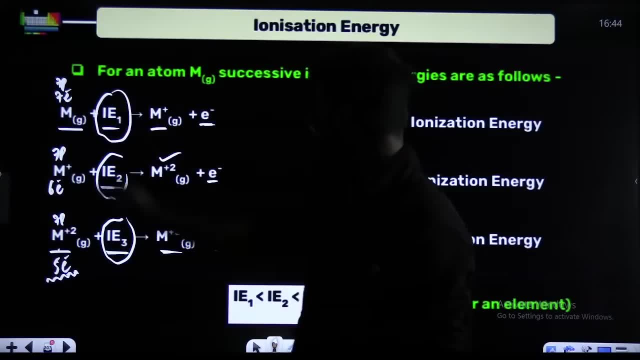 So to take that electron out, you have to supply more energy, lot of energy. So can I say, can I say, IE3 will be maximum, followed by IE2, followed by IE1, right, IE3 will be maximum, followed by IE2, followed by IE1.. 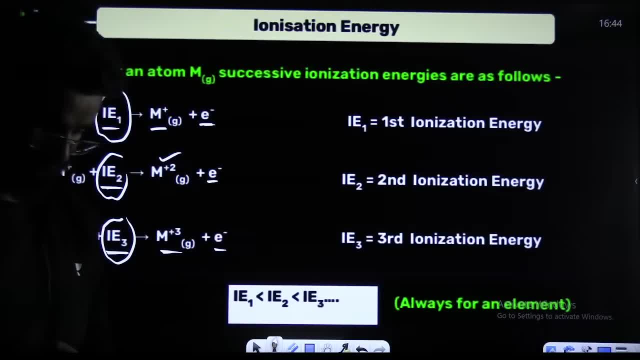 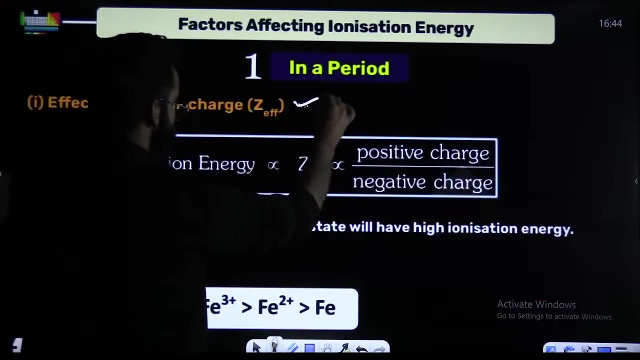 Because if I give you a factor of IE2, 1,, 1,, 1,, 0, you are good, OK, Is it clear? Is it clear, people? Now the factors on which ionization energy depends. Ionization energy first of all depends on effect: nuclear charge. 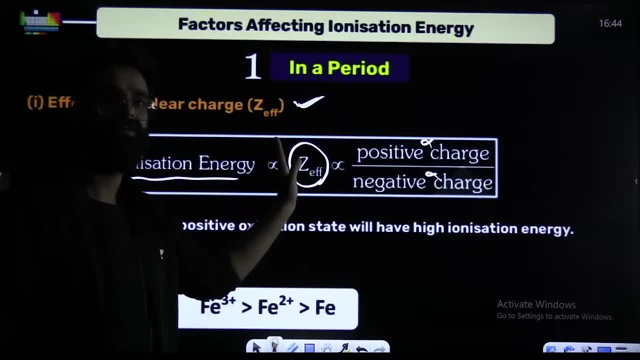 Simple Ionization energy. it depends on effect: nuclear charge. Leave this part. Leave this part right. more the effective nuclear charge. difficult it's going to be, difficult is difficult it will be. to take the outermost electron out. is more energy out of supply? that means indirectly. 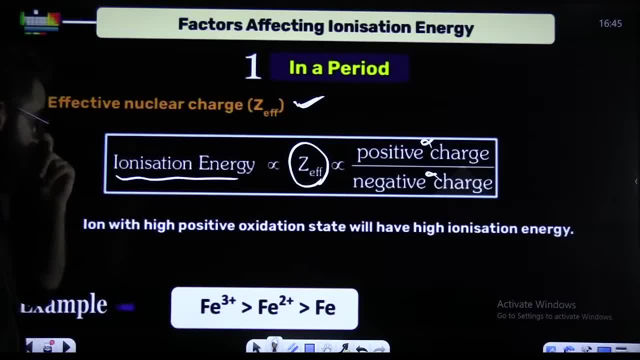 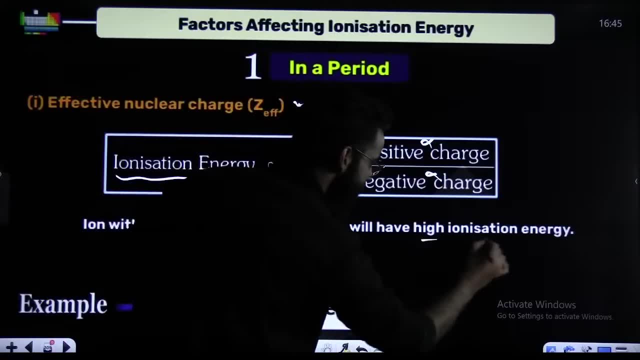 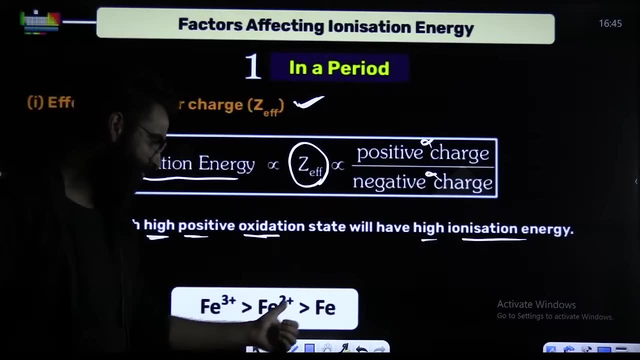 more will be the ionization energy, perfect right. similarly the iron, which will be in highest positive oxidation state, it will have highest ionization energy. for example, Fe tri positive, Fe dipositive Fe. here iron is in tri positive oxidation state, dipositive, zero. right over here you can say Fe tri positive, Fe tri positive because of more effective. 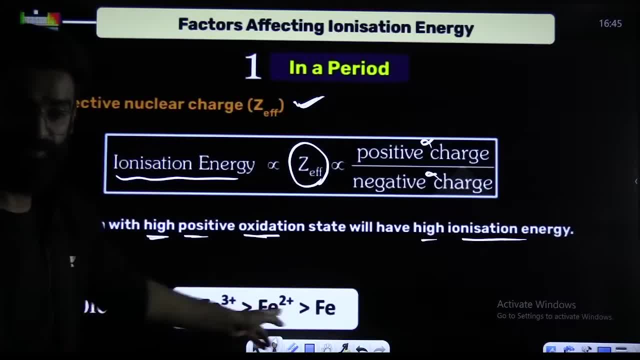 nuclear charge, it will show maximum ionization energy. among all these, to take electron out from Fe tri positive, it's completely difficult, as that of Fe, dipositive, as that of Fe, as that of Fe okay, as that of Fe. now one more thing: ionization energy. it depends on the